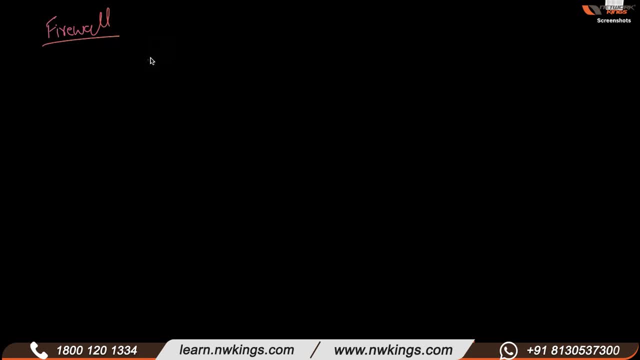 You are required to have a firewall in your network. Just an overview of firewall. okay, Because you need to protect the perimeter. okay, Also, you need to protect your application, So there can be different stages or different locations in your network where you would want a firewall to be implemented. 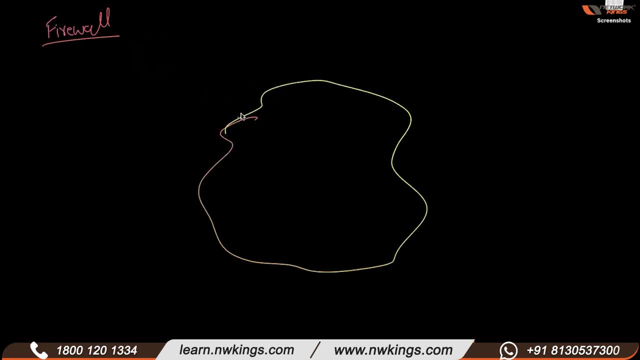 Right, The very first is: let's take The bigger picture. this is the perimeter of your network. This is where the network starts, or your enterprise network starts, or the data center starts, or whatever, right? So you call them the perimeter firewalls, right? 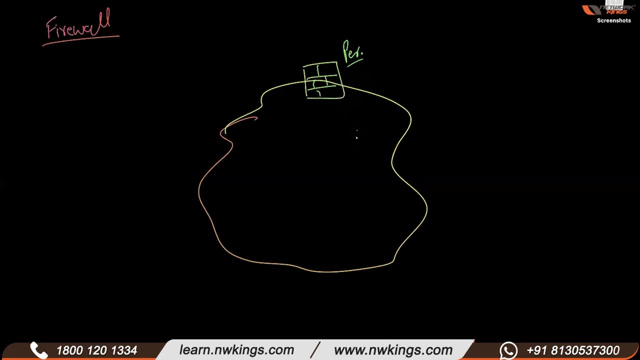 Here you would control who can access your network. These will have services like remote VPN and all. Okay, Uh, the work from home- uh doing people, they'll be, you know. connecting their uh remote. Okay, Uh, the work from home, uh doing people, they'll be, you know. connecting their uh remote access VPN or SSL VPNs to these firewalls. 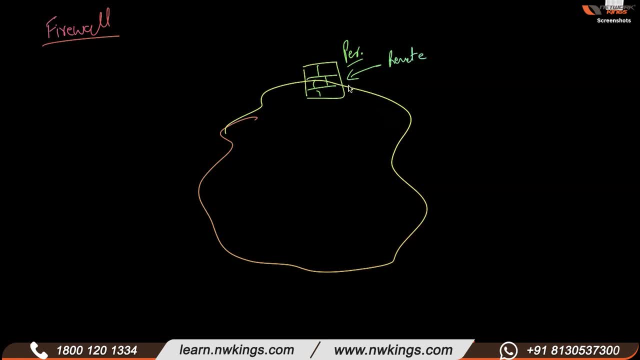 They'll be responsible for all the site to site VPN connectivity and all that. Right, We'll be looking at these terms in detail. but yeah, uh, this is one location where your firewall can be. The other location can be, uh, you know, right in front of the applications. 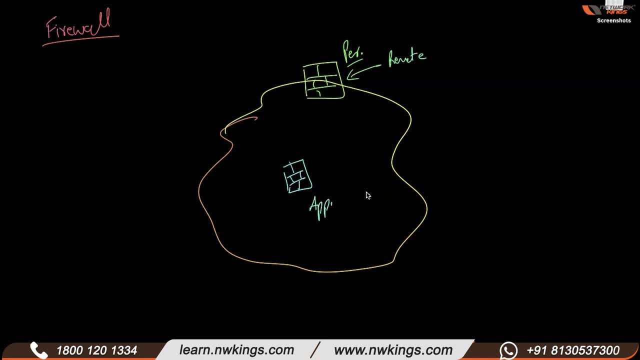 You call them internal firewalls or application firewalls. right, The basic network would look something like This: right, You'll have the inside Any firewall, would you know? basically divide your network into three different uh zones: Inside, outside and DMZ. 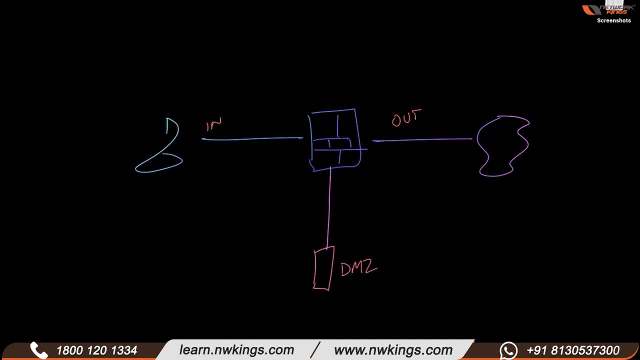 Right. So depending upon which vendor it is the, you will have naming convention of these uh sections of the network. DMZ is kind of a standard, okay, like Palo Alto likes to call it the trust zone, right? Cisco would call it inside. checkpoint would call it inside, right. 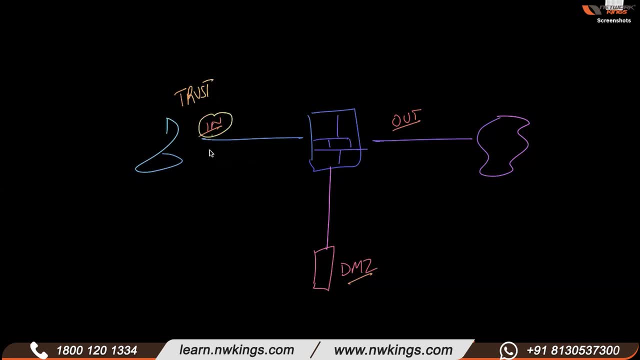 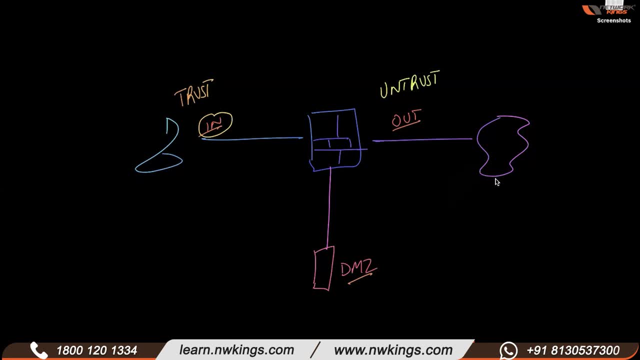 Same meaning Yeah, And there are standards, uh, which means you can say, uh, a predefined um, an unsaid rule. You can say, yeah, you may want uh inside users to be able to go out to internet, right. 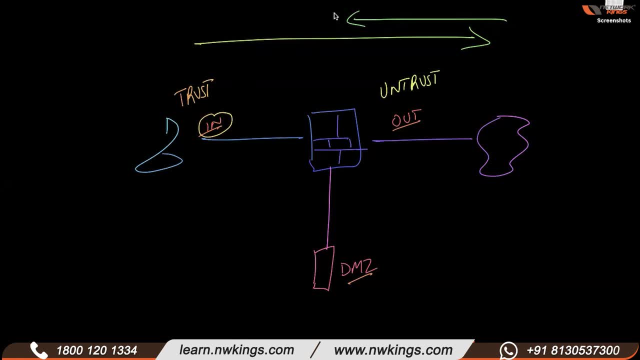 But you should not be having anybody coming from outside to inside, Right. Also, let's say, in the DMZ. DMZ is basically, if the term is new for uh, you all. DMZ is holding all your servers, right? 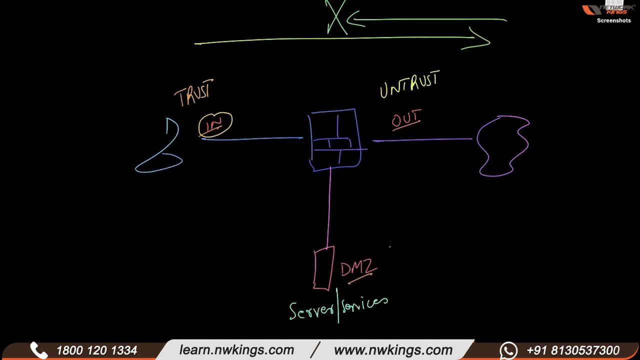 And services. let's say I am hosting some web service. I will have users on internet, So that service has to be accessible right, Which means the firewall needs to allow the users coming in for accessing these applications. right, The inside is your network, basically where your- uh, you know- employees would say it- or your internal users are sitting. 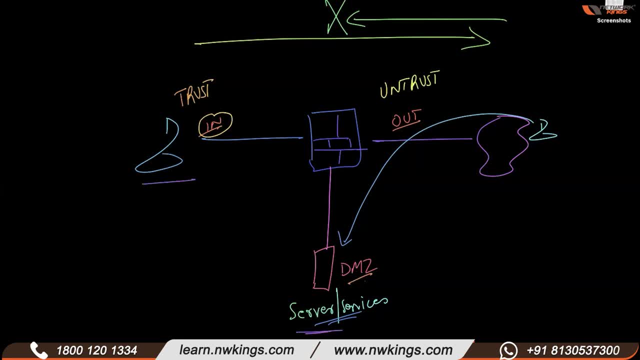 This is always segregated from the internal uh servers. Why is that? Because servers are something which are supposed to be accessed from outside, right? Not the PCs, not the employees. They don't their PCs, their machines, they don't have to be accessible from outside. 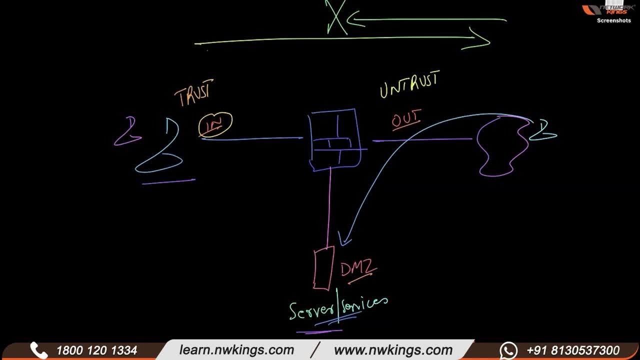 Okay, Okay. So the tools go like this: that you are allowed to go from inside to outside, or trust to untrust, and from untrust to trust. you don't really allow, uh, or you don't really make any policies right. 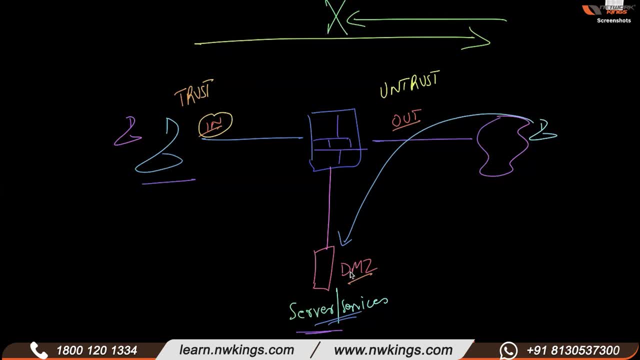 That's not a good practice. Yes, You will obviously have to make access from outside to DMZ, but again, you will never have DMZ talking to inside right. It will never be there. Not a good practice Why? Because if there are attackers on the outside right, they may act up as users get access to the DMZ. 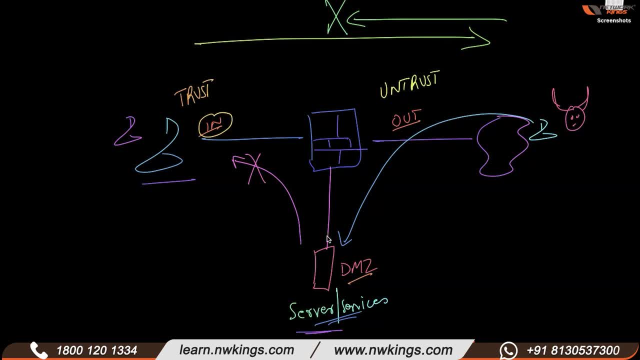 And from here they may try to exploit your internal network, right? So you would want um that to be blocked? Yeah, So no DMZ accessing trust, but, yes, your internal users should be able to access those websites, Right? 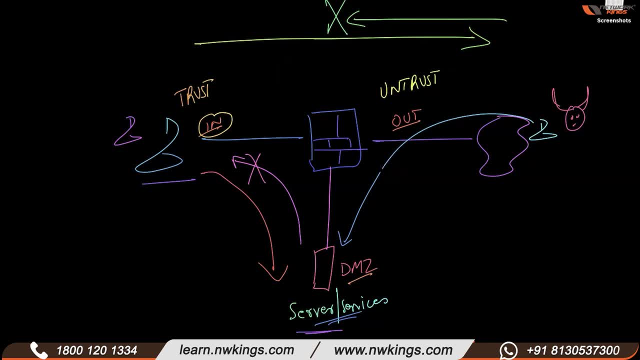 So all Both ways, single ways, communication- all can be controlled by the firewalls. Okay, No matter what uh place they are kept, be it at perimeter or be that application. it typically divides your network into these three portions. 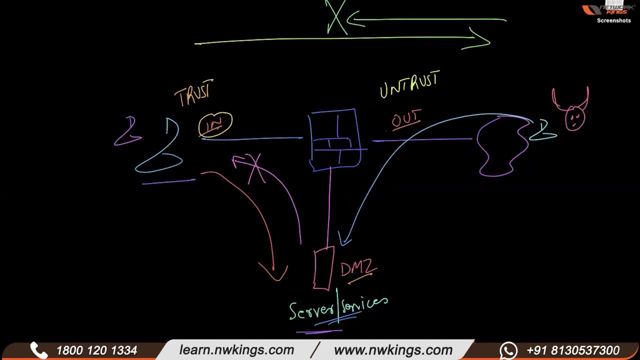 Right And, however, is the requirement: we can create the policies. whatever I just explained is more of a generic concept that this is how the firewalls will uh allow the traffic right, What traffic will be allowed, What policies will be uh created to allow this? 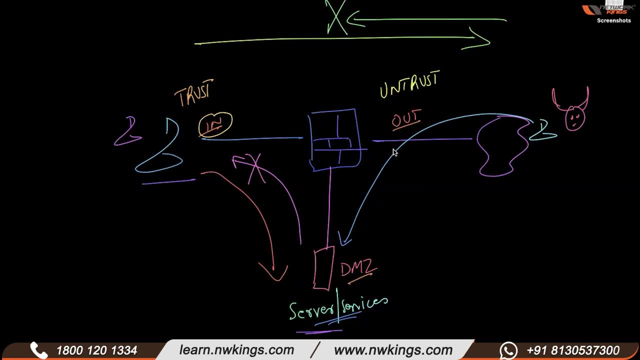 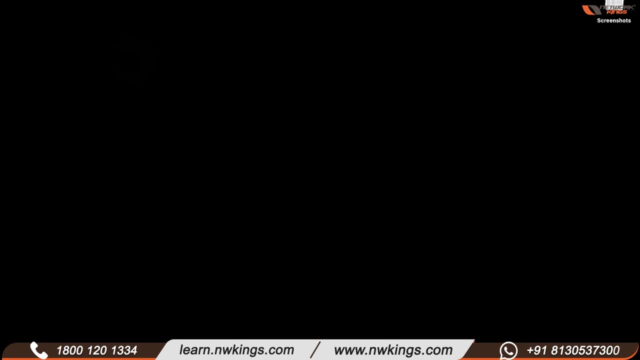 What will be the netting profiles? uh matting rule created and we will all uh look at that. Now there is a very important concept that you need to understand, uh, in case of firewalls, like you have uh worked on routers so far. routers: how do they take decisions? 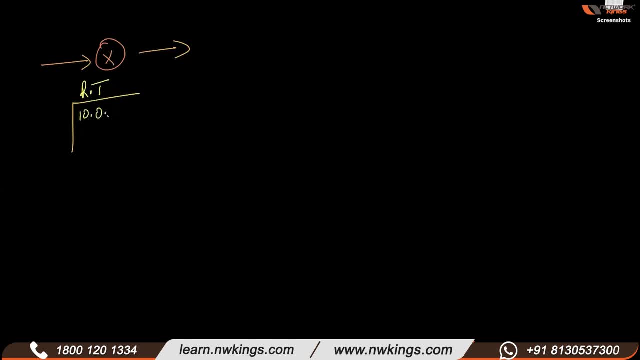 Routers take decisions on the basis of routing. table right You have similar entries. If a destination is matched in the route, it selects the outgoing interface and the router would simply forget about the packet. That's more like a packet forwarding or packet based uh processing. 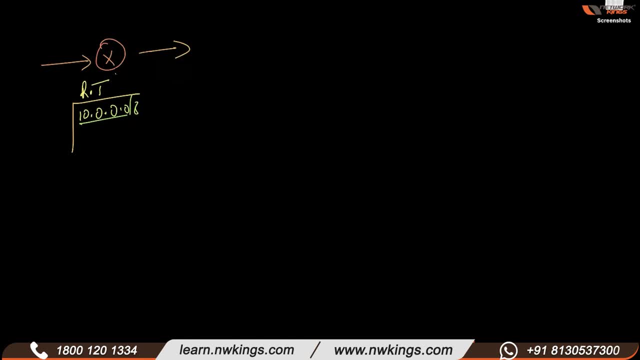 Same goes with uh switches, right? They also do the same thing. They would do the layer to look up, look at the MAC address, look at the destination MAC. uh, the packet is uh trying to go and forward it onto the exit interface. but this is not the case in firewalls, right? 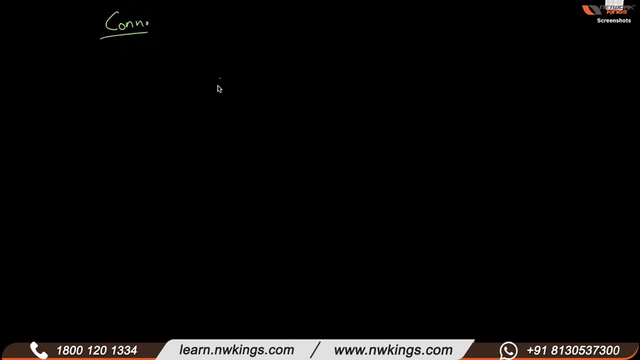 Firewalls. they do remember and they make connection tables. For example, this is my internal user trying to go out through the firewall. Right, Let's say these are the. my policy says that this is the trust Right. This is the trust user trying to go to the untrust environment and the direction is direction of communication is from trust to untrust. 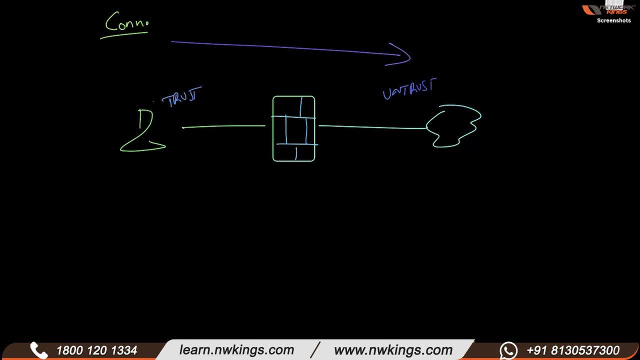 Now the communication is getting initiated from where? from the trusted side. So this is allowed, right. Let's say this is 10.001 trying to go to 100.001 on the internet. Now the communication. since the communication is initiated by the internal user, there will be response coming back. 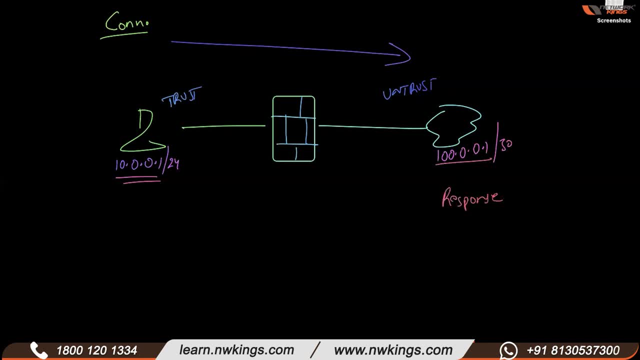 Yeah, simple things. response, coming back from the untrusted side trying to go to the trust. So this particular packet, the response packet, is allowed. How is this allowed? By looking at the connection entries, Because The firewall it remembers, it remembers the packets going through it, passing through it, right? 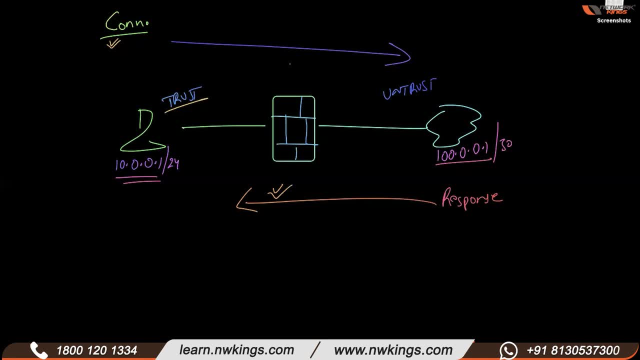 It remembers that there is a request made from the trust zone going towards the untrust right. Hence the response to that request is allowed. But if there is a fresh request trying to come from untrust Right, Trying to come from untrust and. 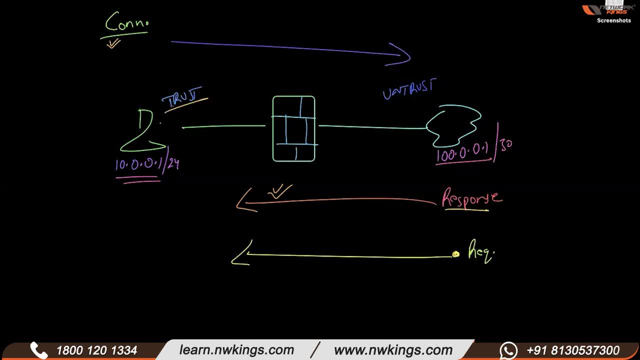 The destination is trust zone or anybody inside this trust zone, this will definitely be blocked by the same rule. okay, You don't have to have extra rule for blocking this communication, right, Blocking this request coming from outside. you have a single policy which says that. okay, let me put it here, which says 10 network- right. 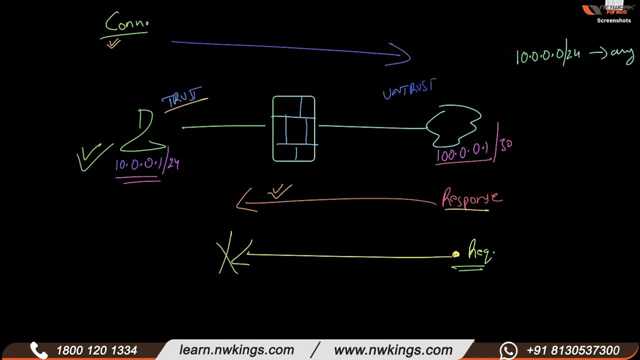 Is allowed to go to any destination, And this is my rule number one, for example. so the same rule will: will block it. okay, will block the request because these rules work in stateful manner, right? All of this concept is called stateful packet inspection. 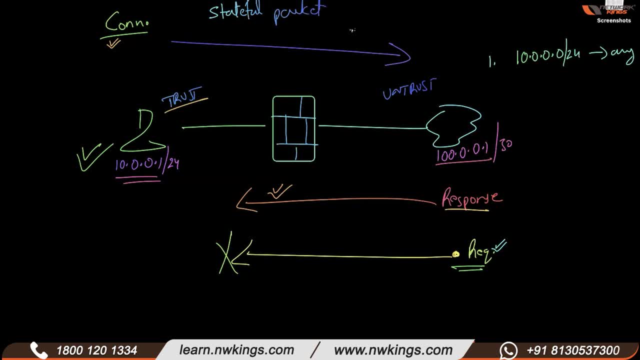 And we went a little reverse. I explained the logic and then the heading, but that's how it is best understood. Stateful packet inspection. This stateful behavior is kind of normal now in all of the firewalls. right, All of the firewalls will do this. 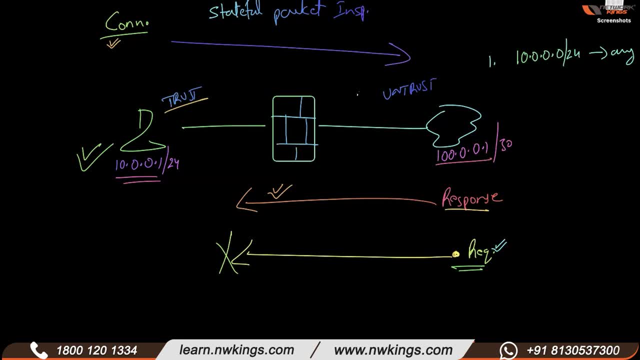 Okay, Any any questions in this? Let me explain one more time before you guys start asking questions. Stateful packet inspection. The behavior allows the firewall to allow the communication coming from trust to untrust. that is using this rule Right. The response will be allowed. 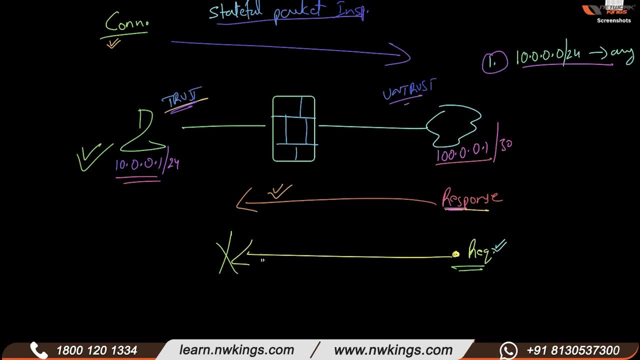 Right, but not the request coming from contrast to trust right. To have the request allowed, we will have to have a policy which will say something like this: Anybody should be allowed to talk to 10.0.0 slash twenty four. We would have to have this kind of rule right. and there is no good reason to have these rules because you don't want anybody on Internet to simply talk to your internal network for the first time. 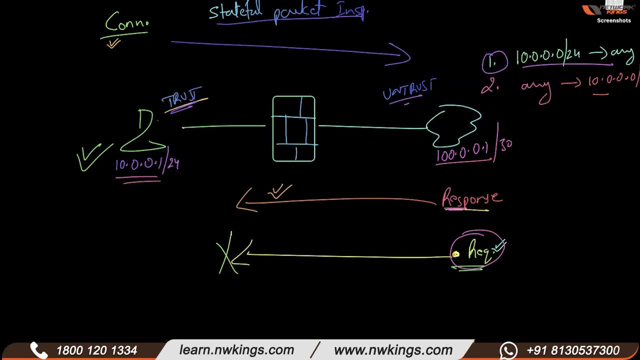 Okay, That's by default. No, Matt, The response will be allowed. right, internal network. right, there's no point of firewall then, so you would never create this rule. all right, so this is stateful packet inspection and this is common, uh, behavior of all of the 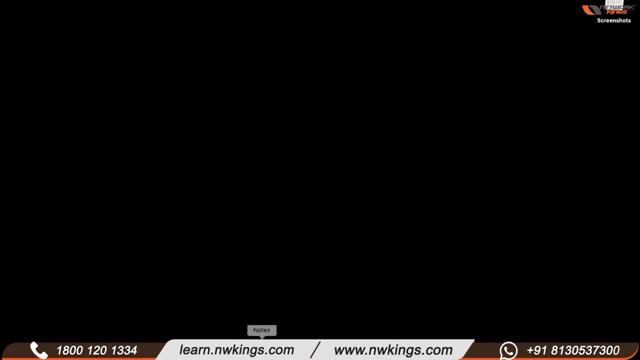 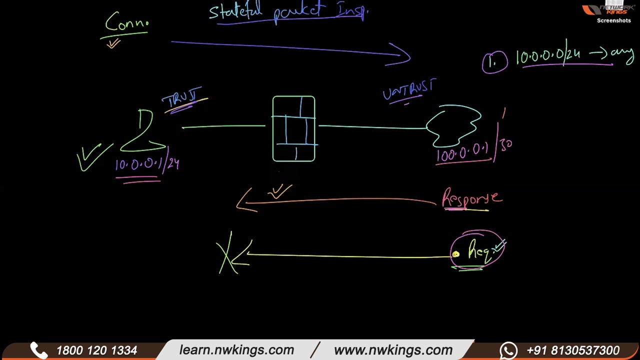 firewalls. okay, let me know if you have any questions, sir. the first question is: uh, uh. in the first slide you said uh, trust to dmz. it's uh, it's allowed by default means we can. we can make the connection right. the first, the first select and the second, i mean the on the 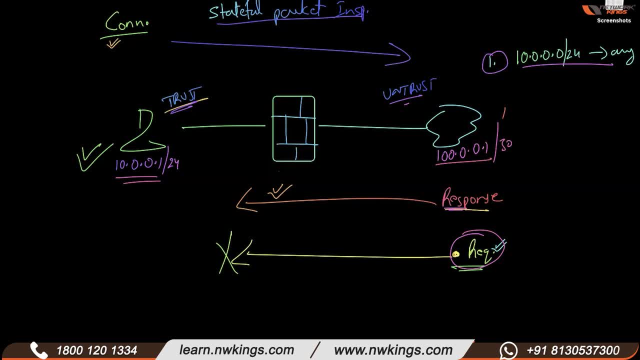 it is not uh like it is allowed or disallowed. it is a general practice that this is how we design our policies, that you would want to allow trust to dmz and then outside to dmz and inside to outside. but inside, uh, means anyone can access the dmz zone right, but not from outside: untrust. 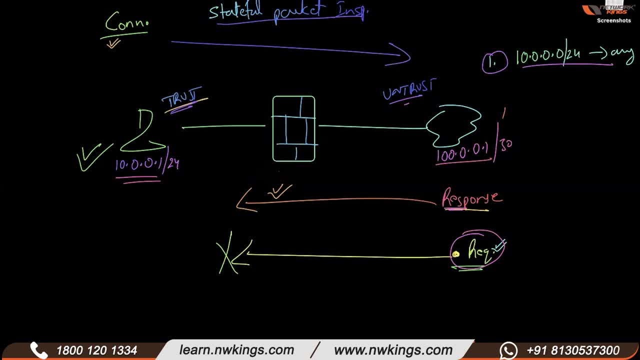 no, uh, dmz. dmz is meant to be accessed from outside. dmz is holding all the services that you are offering, okay, so, so we need to make the policy then. uh, then it can happen, right, yes, okay. and the second we will get into: uh, like, what are the default behavior of the firewall and 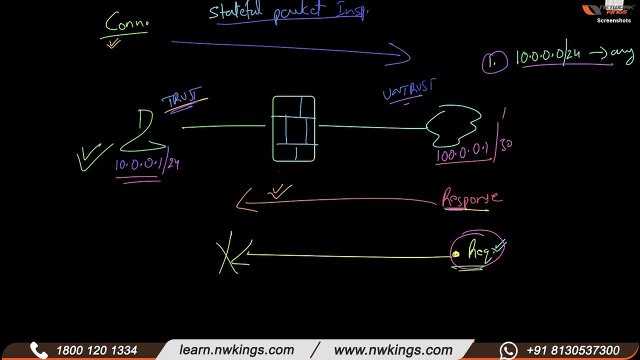 all that okay. okay, i'm not telling you the defaults right now. i'm telling you a generic way that this is how you will build your security policies. okay, so, and so that's from the trust to untrust zone. okay, uh, if 10.0.0.1 is trying to access. 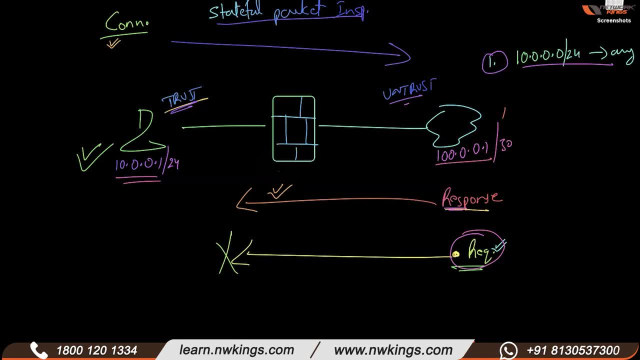 100.0.1 connection will um. first of all, the firewall will check the connection means which port that means. i mean to say the stateful packet inspection will check and it will make the connection entry in the in the in the table, right. right, okay, but once the response is coming it. 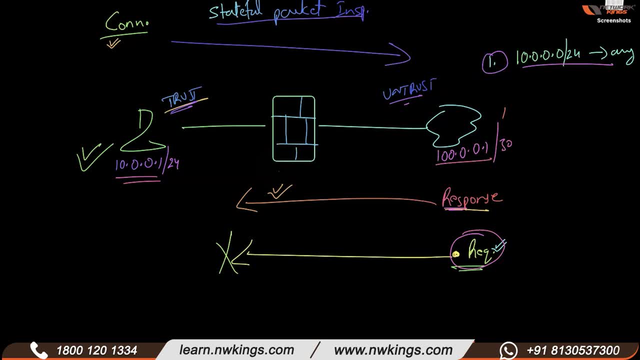 won't check because the connection would be there, so no need to check. so it will, it will bypass, simply right. yes, yes, but from the untrust zone in: if 100.0.0.1, how can net that you said the 10.0.0. 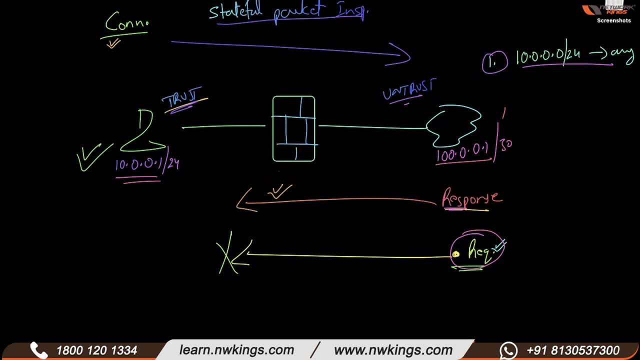 uh. it will be applied for the same uh rule. so it will. it will deny if anyone is for a firewall, uh, for a firewall to allow a particular packet, there has to be uh either of the condition that should match right first is either there should be an entry in the connection table- okay, if there is an entry in the connection. 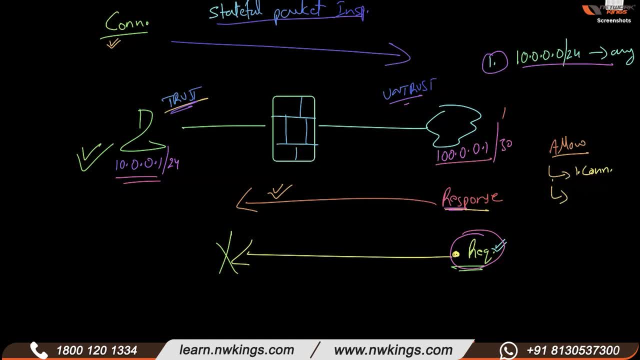 table for that particular packet. yes, it is good to uh go to the destination. second is there has to be a policy. if there is no existing connection, there has to be a matching policy. okay, if connection is not, that the policy should be there, then we can bypass the traffic right, right, okay. 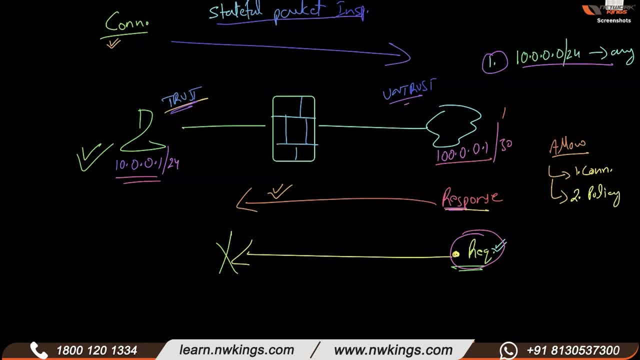 and in palo alto, sir, we we call it uh in second, we call it rules and palo alto, we call it policy. right, hello, uh, give me a minute, sam, just give me a minute. some student calling was not able to join. okay, yeah you, you could call it a policy or rule, doesn't matter. on what? uh? firewall, um vendor. 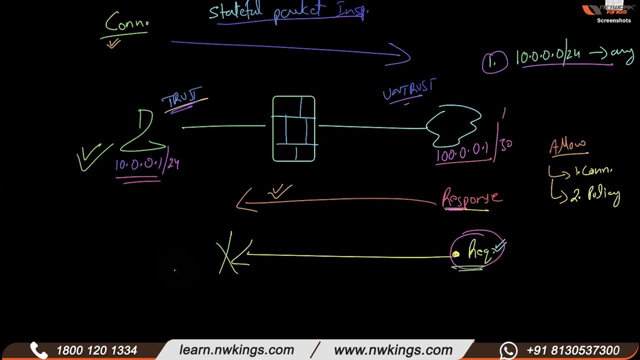 you're using- okay, doesn't matter- policy, a rule you could, you could, you could call it. i mean, if you go back to the example that what he was saying, let's say you're having a party, right, and you have 15 people inside that party- those people, you have a list of people that can come into that party, right, okay. and if 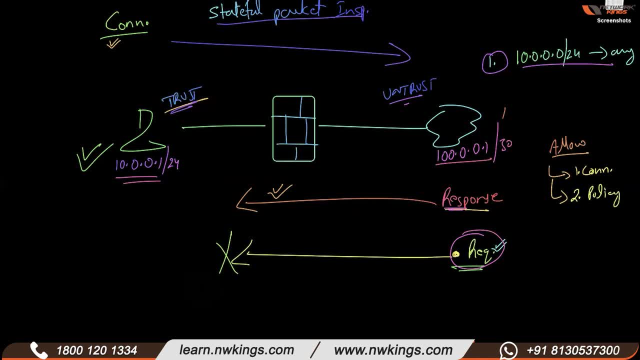 somebody has came out, went out, right. then then it said: oh, i'm gonna go out check something real quick, then when that person comes back you're gonna let him in, right? yeah, because he was there before. so the picture is. it's just a small video file, very luxury, but okay. but you know, you can, you can. 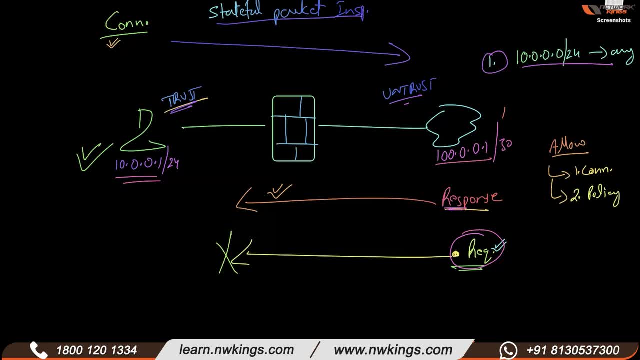 do. that's right. yeah, so the fact that you have this kind of a uh, photographic um was gonna say: hey, wait a minute, this is a new connections, i'm gonna drop that traffic. that's that. that that's well. that's what dcp three-way handshake also happens in that case, i think. 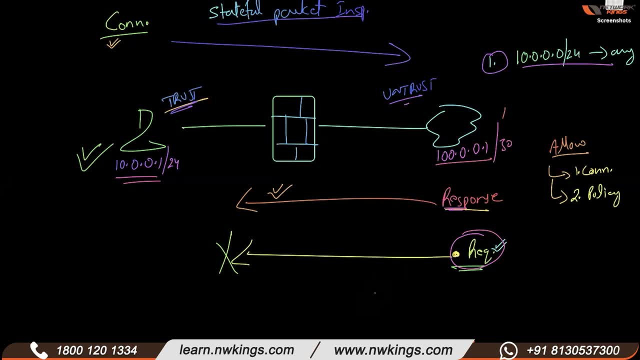 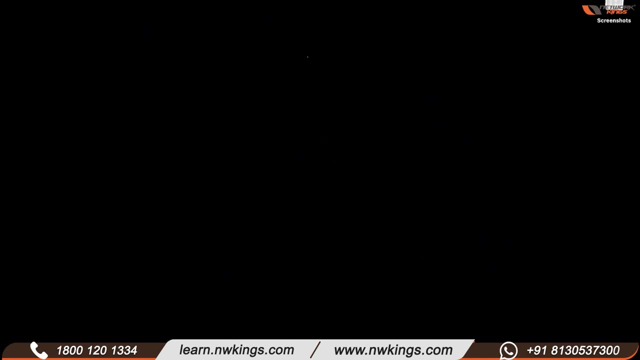 break? yes, it keeps. it has this database that keeps all the connections the same, the same act, the act, the, the all that. okay, okay, hey, sam, uh, hey, thanks, uh, who is that of the name? got it, sir, you got it okay, yes, sir, uh, sir. one more question actually: how many connections they can store in in his database? 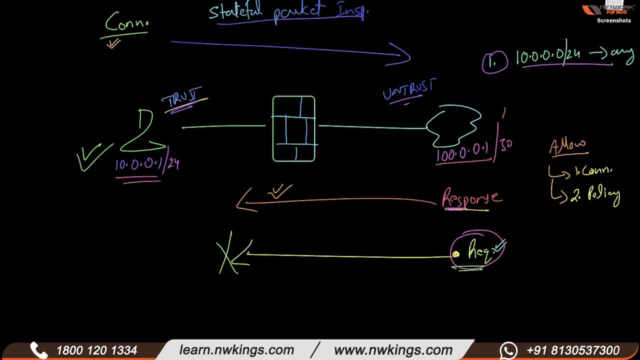 uh, that depends on the hardware model, right? uh, that depends on um which there any maintain any session like? uh, that can store up to this, like this, and that's what i'm saying. uh, palo alto starts with the basic model, that is, the vm 50. right, it's a virtual machine and it goes up to. 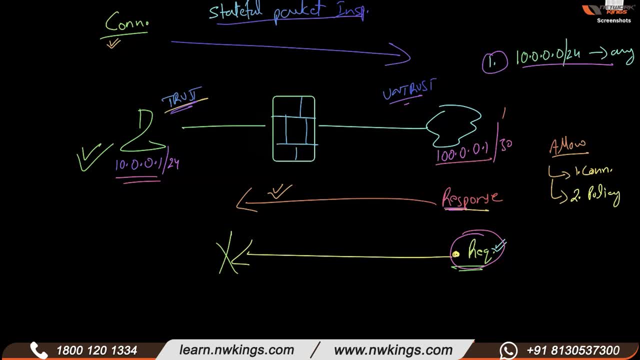 500 model. so it all depends on the hardware specifications, right, how? it's like, uh, if i ask you how much processing your laptop can do? right, so it depends on how much ram and how much cpu that your machine has, right, okay, so that will be. uh, you know something that you can check in the data sheet. 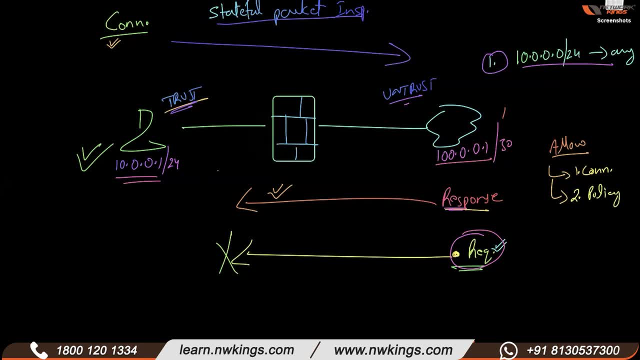 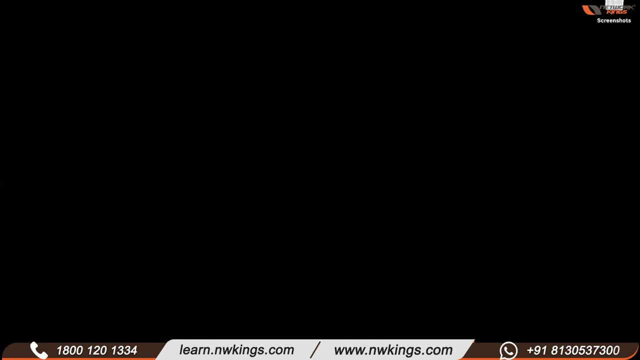 of, uh, individual model. okay, thanks, mostly right now. companies. it's the basic concept, guys, right? it's like when, when there is lockdown, right, and all of your family members that are inside the house, right, and somebody knocks at the door, you, you will be asking 10 questions to them, right, why do you want to come in? and those are your security. 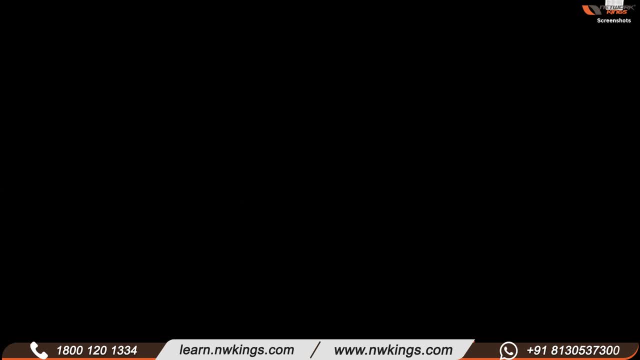 policies. so when there is no existing connection, right, you would want to have security policies on the firewall that will allow the connection. but if the connection is already out, right, you may simply check the connection table. that do we have a request for this packet, right? so if 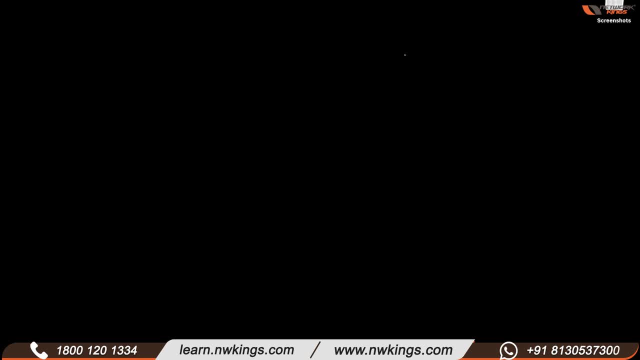 there is an existing connection that exists for this communication. uh, that bypasses the policy check, right. okay, so that's the uh generic concept of faithfulness. that's the stateful behavior, right. all of the security policies. they will be stateful in nature. all of the dynamic. 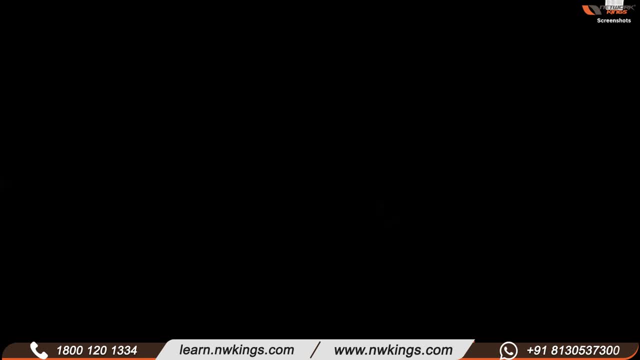 uh, netting and all those. we will talk more about it when we do nothing, all of them. they are bi-directional and stateful in nature, right, not bi-directional, let's just stick to one term for now. that is stateful, right? and somebody has turned the video on. you don't want to see faces, guys? right, you can turn off the video. 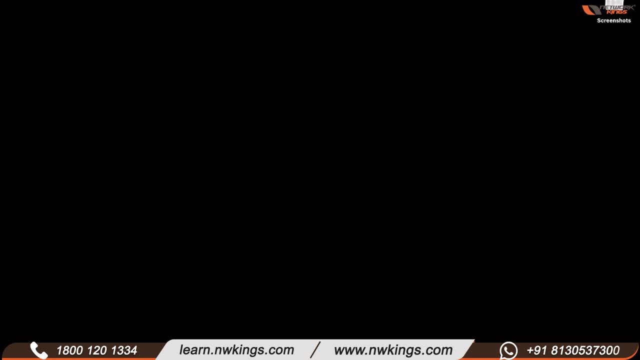 you can turn it off as well, but you don't want to see faces, guys, you can turn off the video. so that's the thing that you have to do, and let me just turn off the video, all right? so let's come back to palo alto. let's talk about some palo alto basic stuff, right, uh, as i 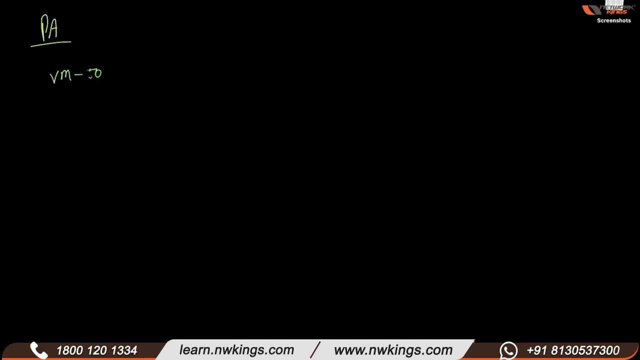 mentioned. uh starts with vm 50.. right, go ahead and check the data sheets on the palo alto website websites and the data center version. i think it is the 8500 series which is used in the data center, which is like a multi-chassis device. right, the operating system here which is running on palo. 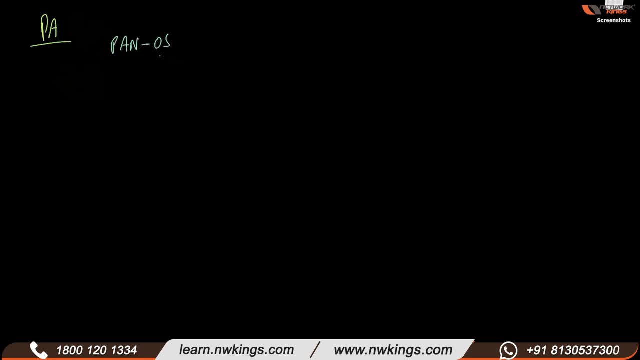 alto is known as panos and palo alto network operating system. the version, uh, we can look at. the latest i think they are running is 11. i'm not very sure on this, but the point is we will be doing things on 9 or 10. i'll check whichever version is there in the lab with us for most of 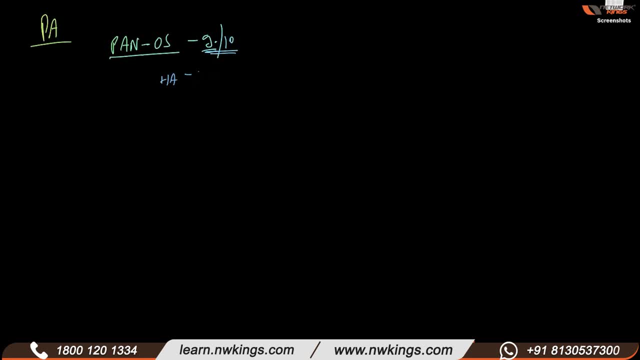 the practicals, but for the ha right, we will have to go back to version 8. i'll tell you the reasons when we do it. okay, so that's what we will do, and not much of a difference. beyond 10, like 10, and beyond 10, there are some cloud features that have been added. so 9, you can say. 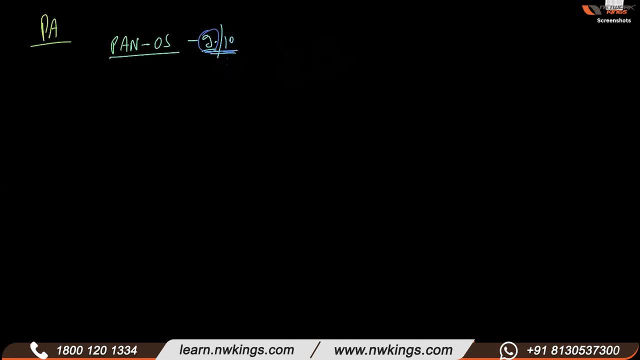 the latest if you exclude all the cloud features. okay, so 10 and beyond. they're all about uh features added like sd van support and all that. yeah, okay, some basics about uh. palo alto firewall. now let's place the same in the same network. this time it's a palo alto firewall. okay, now palo alto firewall is a zone based firewall. 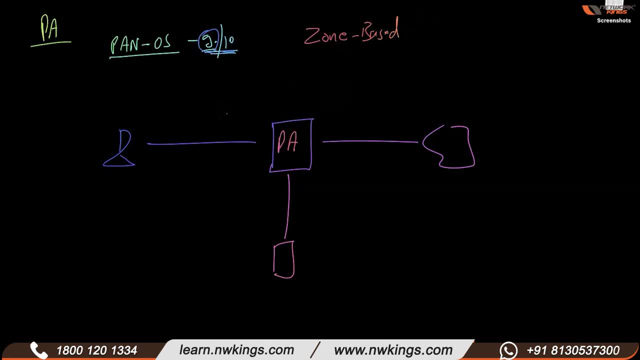 okay, it is zone based. by default, you have two zones. that is trust, untrust, and then you can create a dmc. there are some meanings of these zones, meaning as in interzone. interzone means between two different zones. right, the communication between two different zones is not allowed, which means by default, if you place the 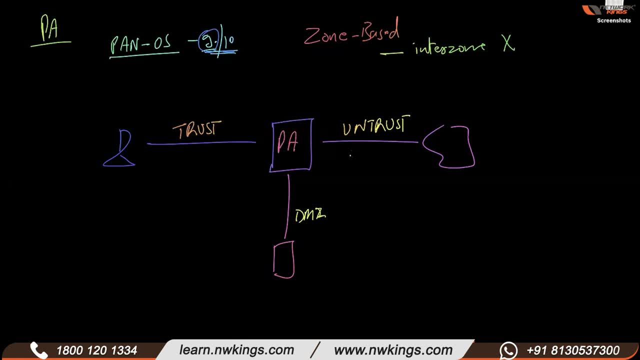 firewall in between and you expect it to work. the default way will be: all of the communication will be stopped, right, even if you are trying to go from trust to untrust or or however right, all the communication going from one zone to the other will be blocked by default. the intrazone communication. 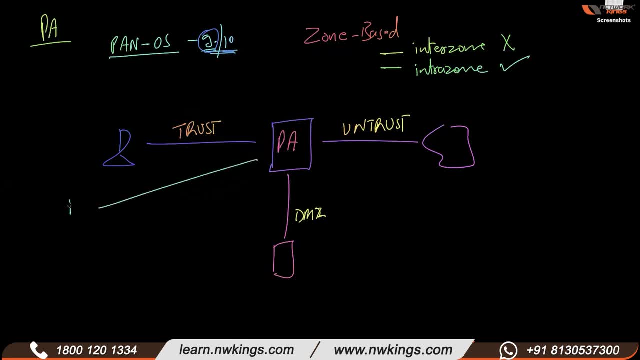 will be allowed. for example, if you have another vlan here, they both are in, right, they both are in trust zone. say, this is 10 network, 20 network, they both can communicate with each other without any restrictions. right, so this is the default behavior of the firewall. 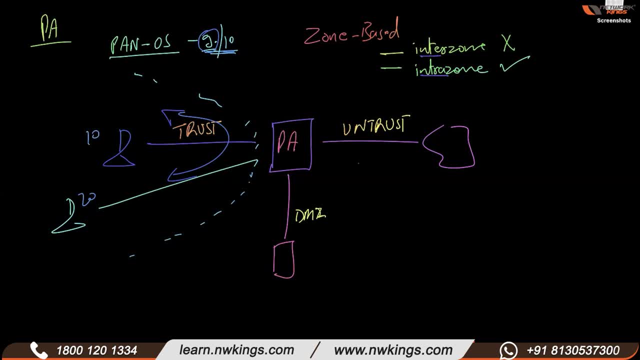 intrazone communication is allowed. interzone communication is blocked, right and beyond this, on top of this, all of our security policies, all of our manual security policies will be created. okay, any questions in here? are we good? all good sir? okay, awesome. and when you so same, so same, for dmz as well means: 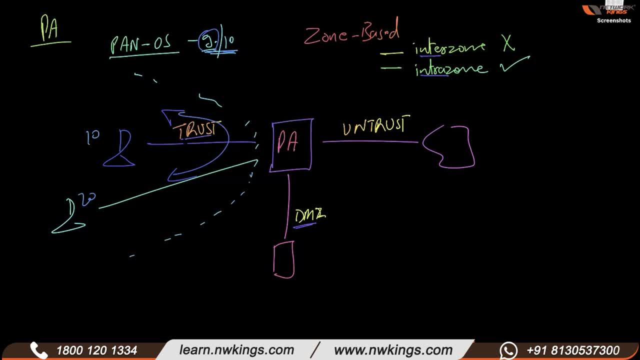 okay, and you know, the names are, uh, more like they're picked up from the documentation of palo alto, right? uh, all of the documentation that palo alto has created. they follow this naming convention, but when you create zones in production, you can give pretty much any name. 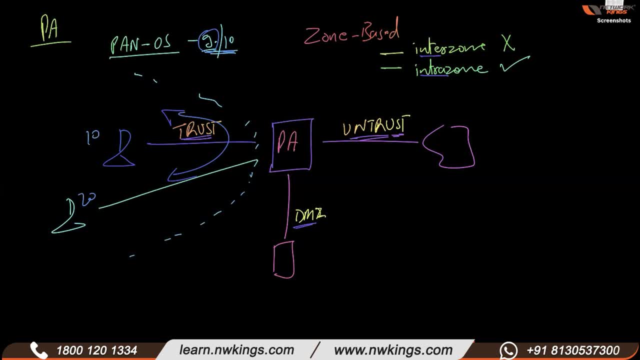 to these zones any name which is, uh, meaningful, which is, which goes with the naming convention in your network, right, you can put pretty much any name to these zones, right, and and the the rules will still exist. interzone and intrazone communication: intrazone is allowed, interzone is. 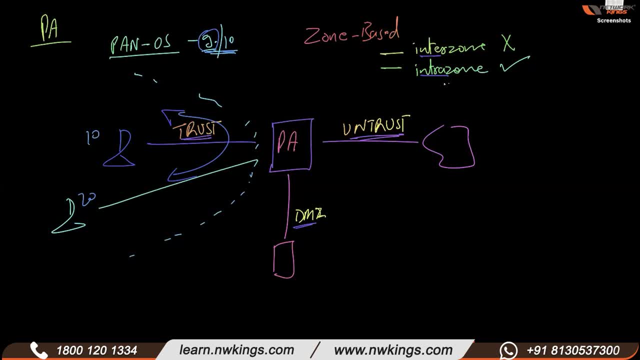 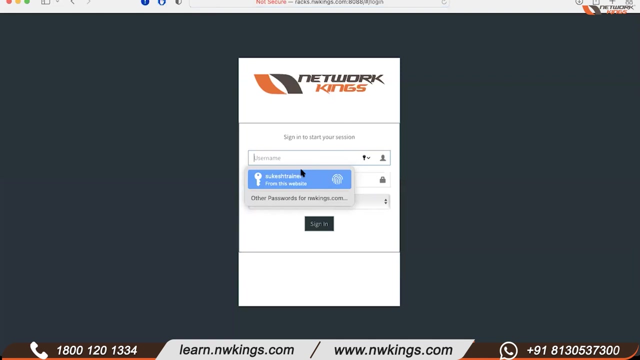 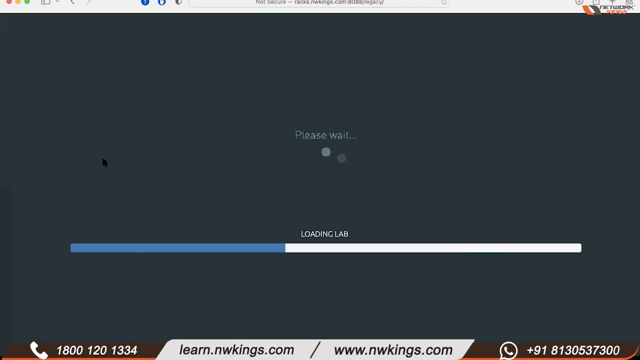 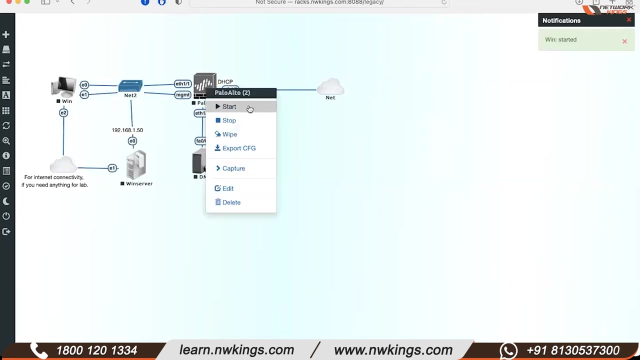 blocked by default. cool, yes, sir. now let's look at the gui of the firewall. let's do some uh basic configuration i'll talk about how do you assign ip addresses, how to get the firewall running, and all this is a Anytime thanks, okay, in the meantime, while, uh, the devices are starting up, uh, let me just explain. 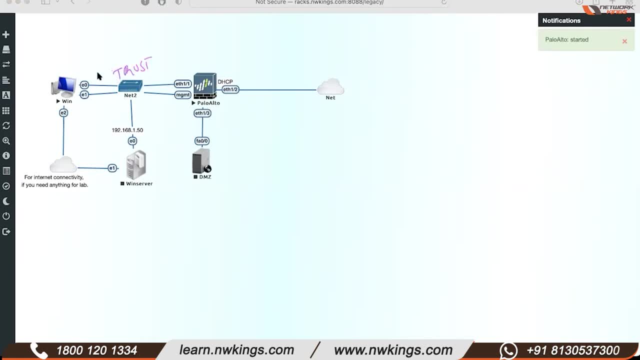 the topology here. we will be using this as the trust machine or or the trust zone. right, this is, of course, the dmz and this is your chị outside, or untrust. okay, this is taking ip address from dhcp. at times you may face errors with this, but i'll tell you how to sort out those. 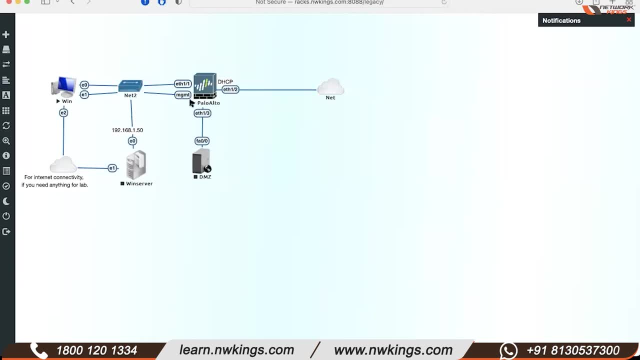 and there is a dedicated management interface on all of the palo alto firewall models, right right from uh vm 50 to all the way to the top end firewall. so a dedicated management interface is there, okay, and that reminds me of a few more things that i should be telling you. 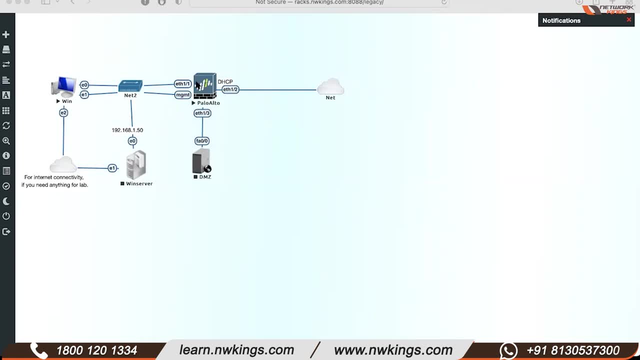 while the device is starting up any communication. okay, listen to me very carefully. there can be two type of uh communication: the communication which is going through the firewall, which means you have some source ip communicating to some destination ip and this destination ip is not residing on the 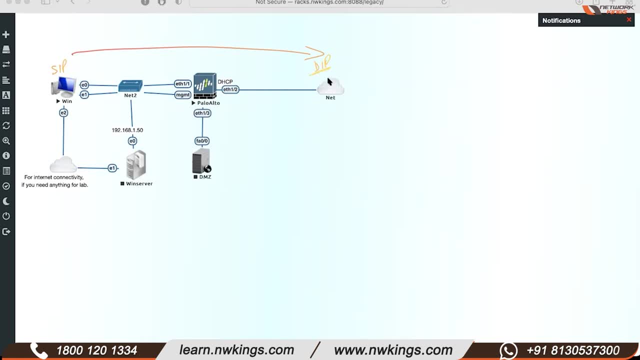 right, it is some destination on the internet, so that is the communication which is going through the firewall. okay, there can be a communication which is going to the firewall right, where the destination ip address is sitting on the firewall. it could be the interface ip address or a loopback ip address right, or the management ip. let's say you are trying to do. 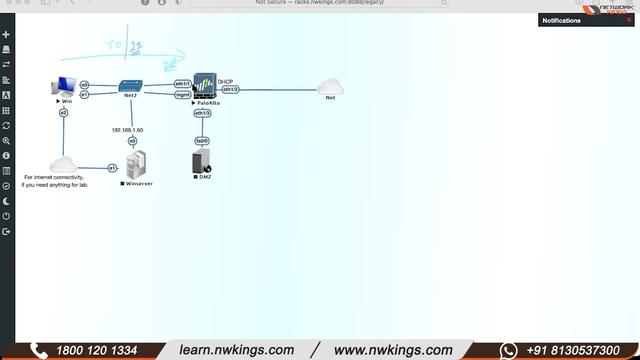 uh ssh on port 22, right on ethernet one slash one. or you are trying to ping the interface of the firewall. not allowed, right? you cannot. and all of this is by default, by the way, right, by default. if you're trying to ping the firewall, let's say this is 10.001- you try to ping 10.1. it will not be uh pinging. 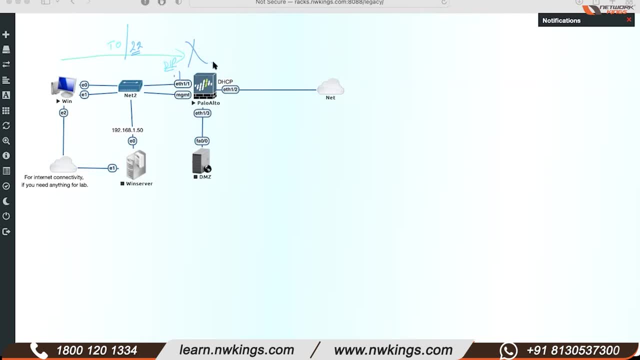 okay, so you mean to say that, uh, through the, through the firewall, the traffic will pass through the firewall to? yeah, through the firewall again. uh, by default the two rules- inter zone and intra zone- that will be applicable. plus, on top of this, you will have your manual rules. yeah, okay, so if the security policies allow the communication, yes, that will be allowed. 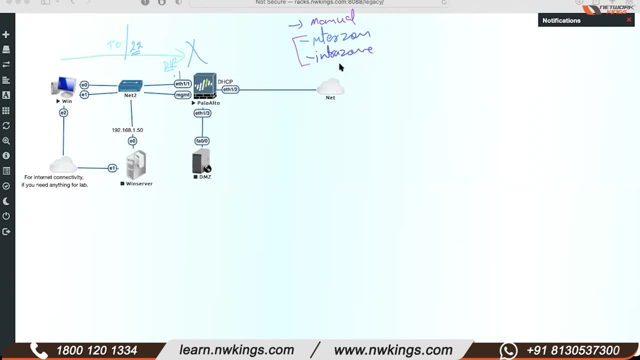 otherwise the intra zone and inter zone defaults will be applicable. apart from this, if the communication is intended to the firewall, you're trying to ping the interface. you're trying to do ssh telnet http. you're trying to ping the interface. you're trying to do ssh, telnet http. 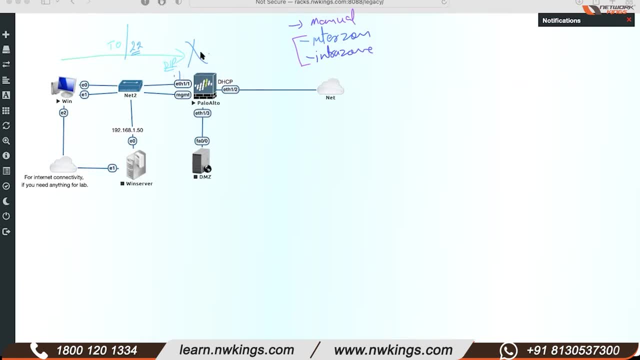 yes, or whatever, right, you will have to make amendments. yes, you'll have to make amendments to the configuration. by default, that will not be allowed. yes, you can let me speak. you can ping the management interface. you can do ssh, you can do https on the management, but not on the data. 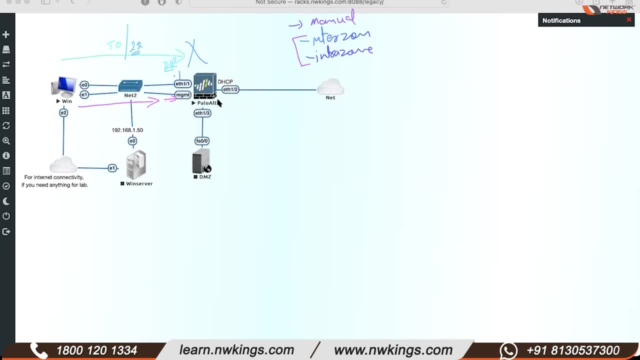 interfaces. sir, can we ping that dmg server through that machine? to which machine? uh, that windows machine we will talk about later on. let's just focus on things which i am talking about. all right, so if you're trying to communicate with the firewall on the management, there are some default protocols through which you can communicate. icmp is allowed. 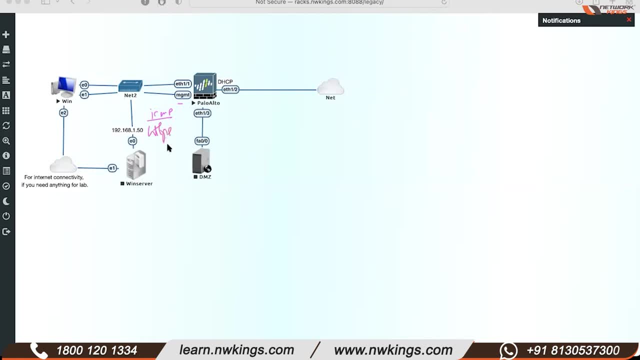 right, that uses ping. you have uh https. that is allowed and ssh is allowed, so, which means we can tweak this and we can also tweak that- who can access the firewall on the management interface? right, for example, we can dedicate a server, let's say its ip address is dot 10, so we can put a configuration on the firewall that only and only. 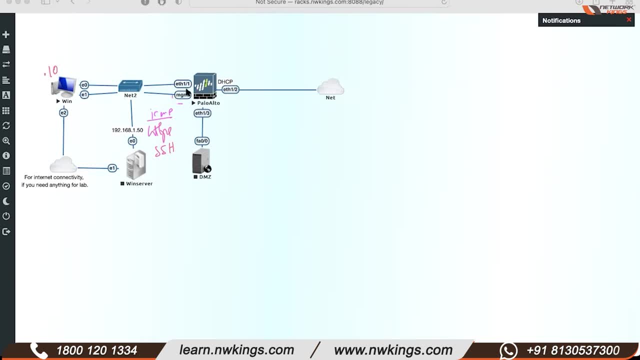 10.0010, can access the firewall on the management interface with these protocols, right? so, having said that, let's. this is for particular users that they can access, not for all. yeah, uh, like all of your corporate networks, you will have dedicated management network, right? you'll have a subnet dedicated for management access, right? sir? 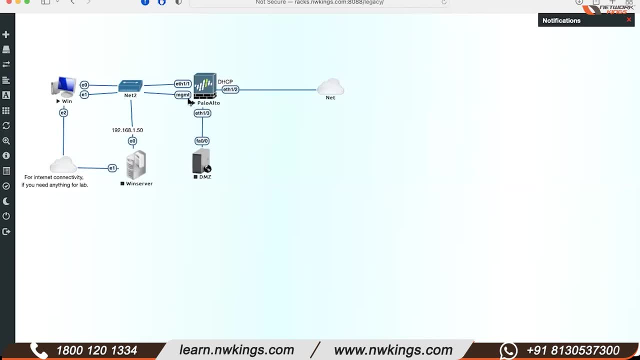 so in in those cases you may want to put, maybe not host specific, but you may want to put a network at least. let's say your management is 10.000 0, 24, that's your management network. so on the firewall you will uh put that network that only this network can access the firewall. on the, on the 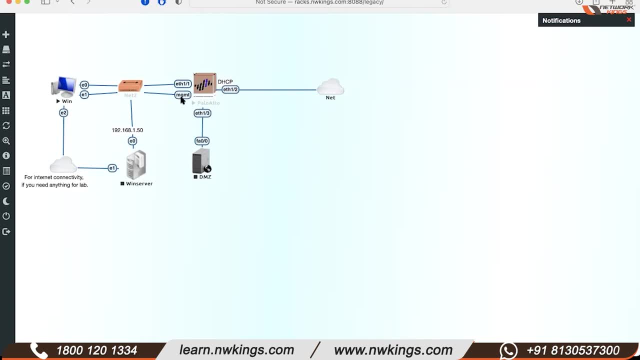 management interface. okay, okay, okay, sir. by default, sir, three things allowed: ssh and ping. and yeah, to manage. yes, on the management: okay. and when you uh access the device- uh, i'm not sure which version it is, let's check that when you will uh power it on. just give it some time on this prompt, okay now i think. 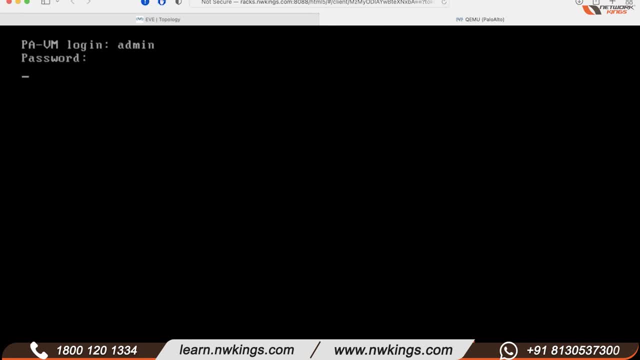 we should be able to log in. the default is admin. admin. yes, we are able to log in, but you know the firewall is quick to boot and in no time you will see this prompt. but uh, if you immediately try to log in through these credentials, you will not be able to log in. it will say wrong password and all. 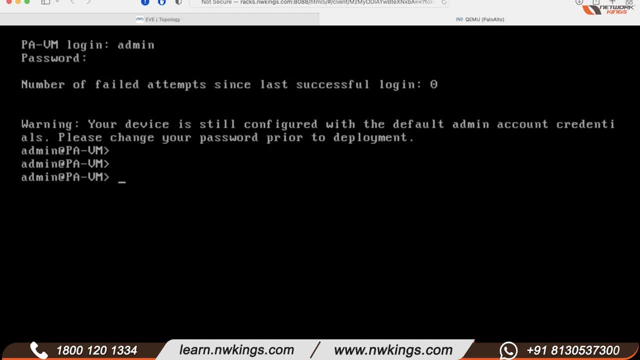 that right. that is because the firewall in the backend is still processing and getting the database ready for you to log in, right? so just be patient and, uh, give it five minutes to to settle down and then try to log in. you'll be able to log in. 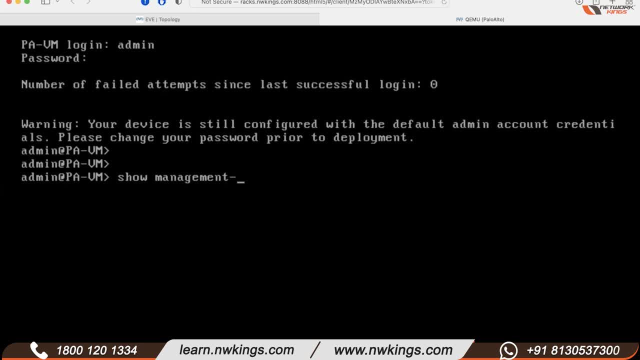 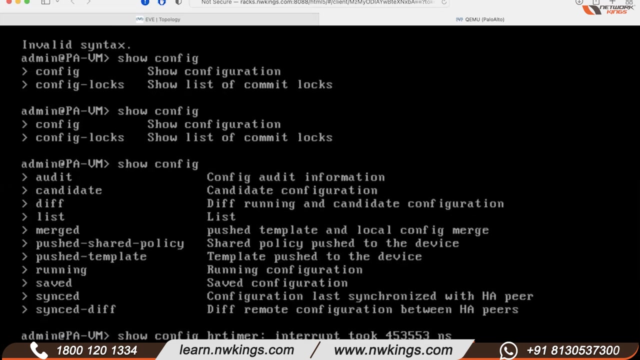 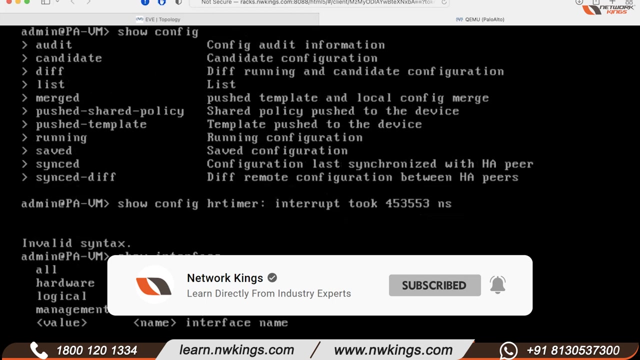 i'm checking the management interface also. this is because we don't have input and no end of IP and when we log in, once we do the command, we get the status unknown because we don't have anything available. the end part, the end part of the handicap is on the results. that's why this is very important. 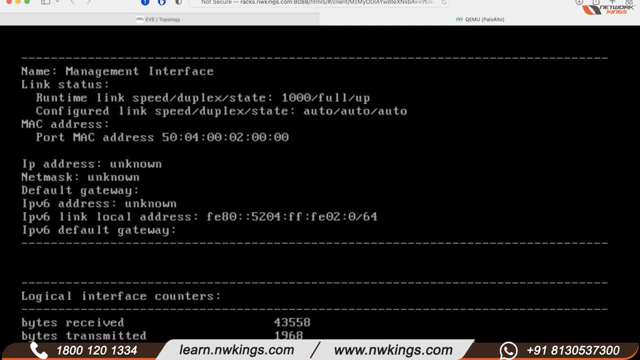 okay, right now you see, it is set to unknown. that is because by default also, when the firewall is out of the box, it is said to have uh ip address via dhcp. okay, on the management. and here you can see there is no DHCP server for the management. 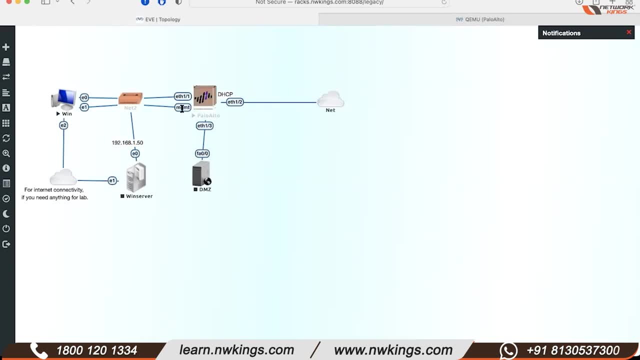 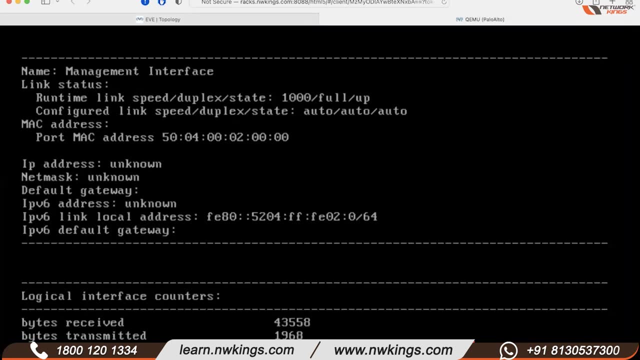 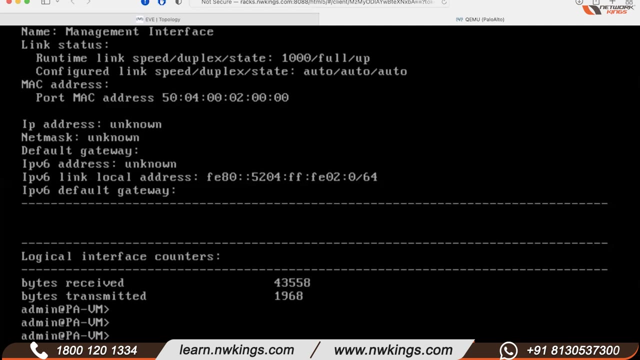 interface. so I will change the configuration to a static IP address. right, and let me show you how do we do that. have you guys worked on Juniper devices? if yes, you will feel at home on Palo Alto firewalls, because the CLI is more like Juniper devices. 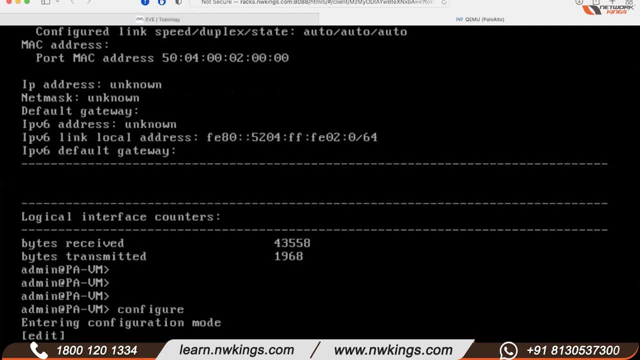 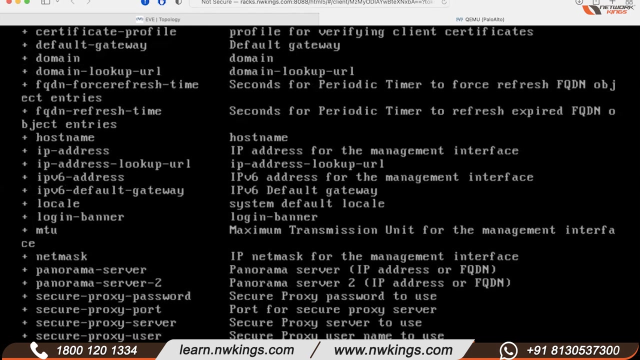 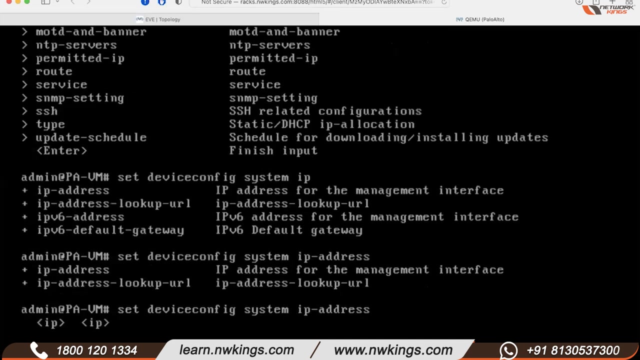 and get into the config mode anything related to the device, be it the device name, management, IP address, DNS, NTP, information right or any other system setting. you always go under device config, so set device config system. before you give IP address, you need to change the type from DHCP to static. okay. 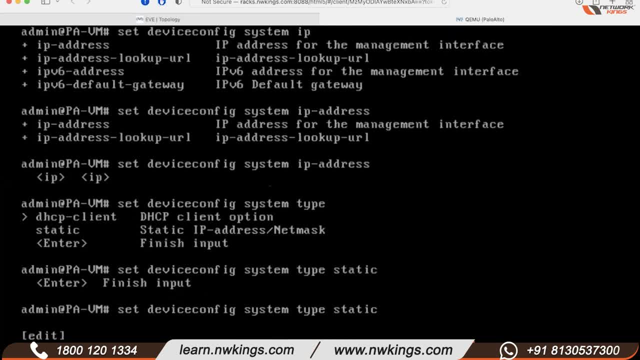 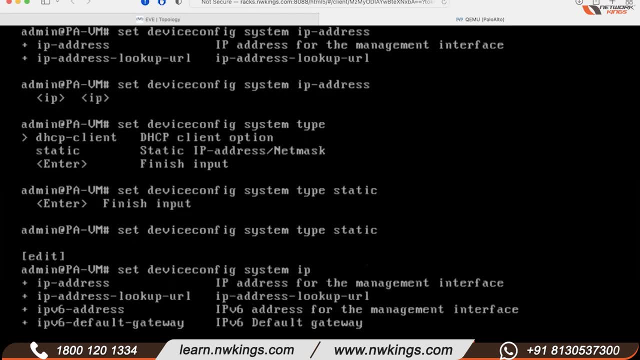 so first I change the system configuration type from DHCP to static and then I show the same command, the DHCP address N.0.0.254. for example, for the management I'll use 192.168.1.1. netmask slash 24. right, and are we good yet the? is the configuration set up perfect for that? 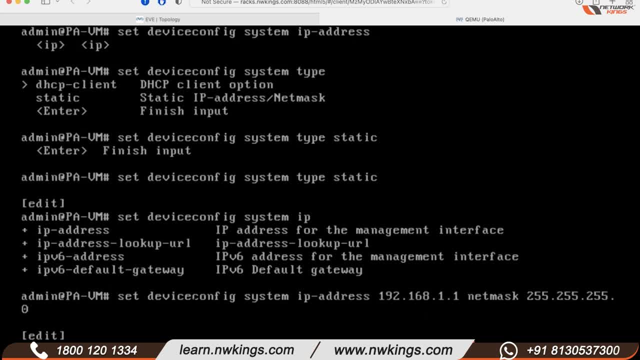 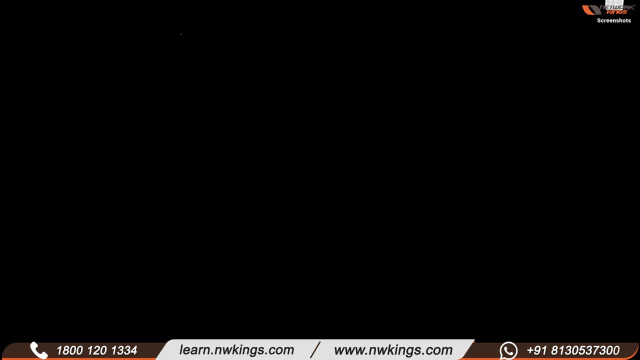 one. right now. I'm setting the IP address to a static IP address and my system is running, yet the is the configuration saved? no, on the Palo Alto firewall you have running config and you have candidate config and you have stored config or saved config, right, so whatever. 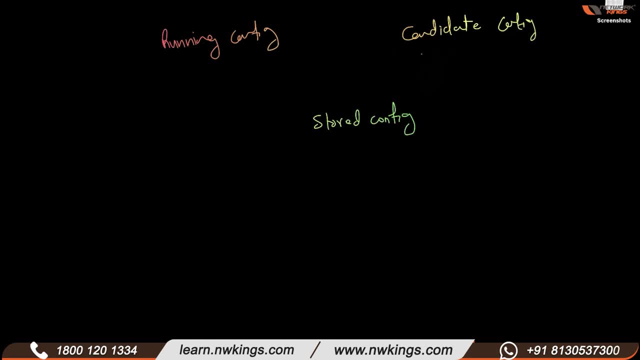 changes we are making live right through the CLI or through the GUI. they are happening here in the candidate config, which means you see them happening but they are not really applied to the running configuration right. so we will have always have to do you commit and you will have to commit your changes. 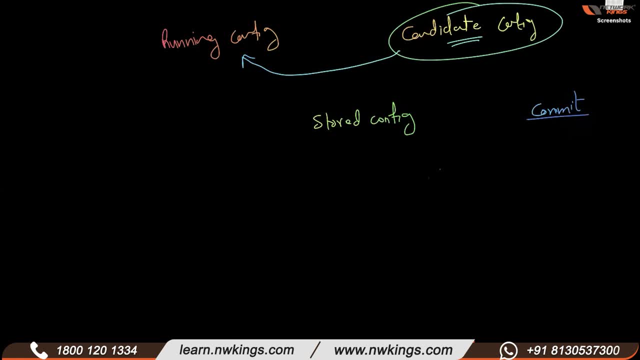 always right. this is specific to Palo Alto. like in Cisco, you don't have a concept of candidate config. all the changes you do, they are directly impacting on the running config, right? so having the candidate config gives you an added advantage. what is the advantage? the leverage to make mistakes, yeah, you. 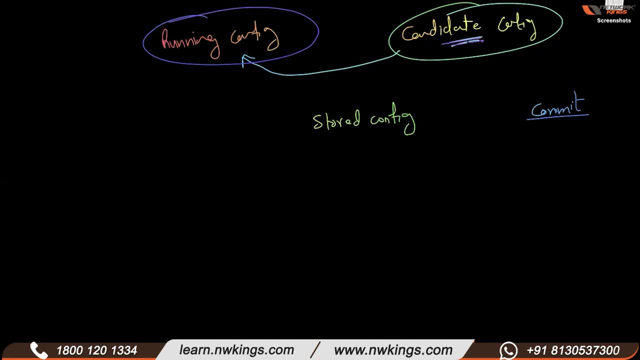 can make mistakes. you still have time to realize that. okay, I've done a mistake. let me revert back. let me correct the configuration before I push. the changes to the running configuration means before you commit. so when you commit, two things happen. your candidate config gets copied to the system. memory means it goes to the 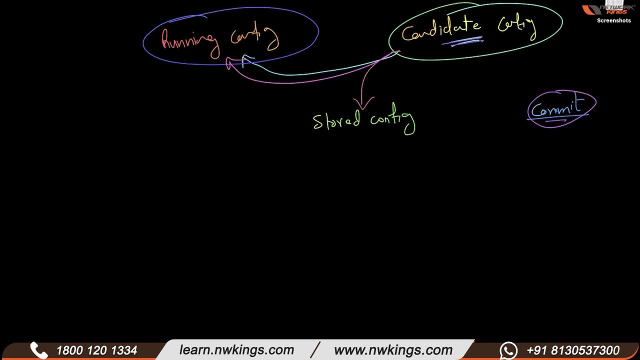 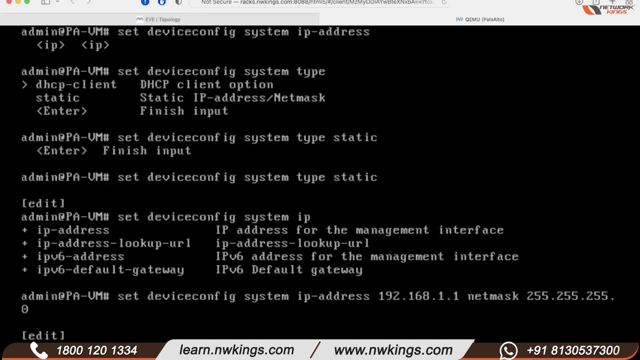 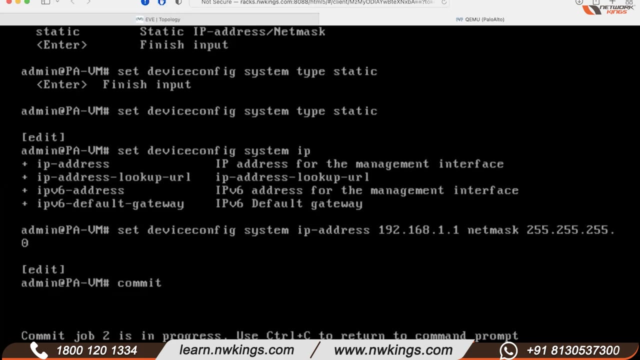 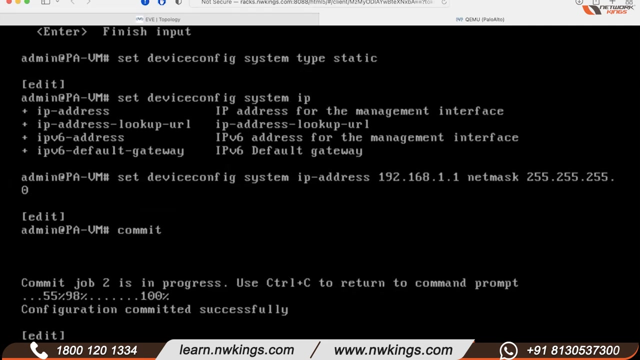 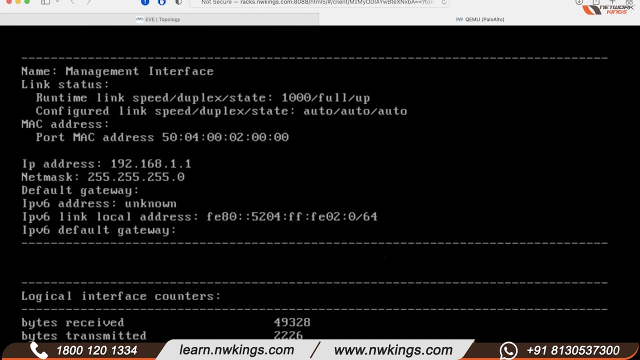 running configuration and also it gets saved okay. so always, whenever you are making changes, make sure that you commit the changes. sorry, same like Juniper system. yeah, as I mentioned earlier, if you worked on Juniper, the CLI will be, you know, very familiar, right? we check again, show interface management and we now have 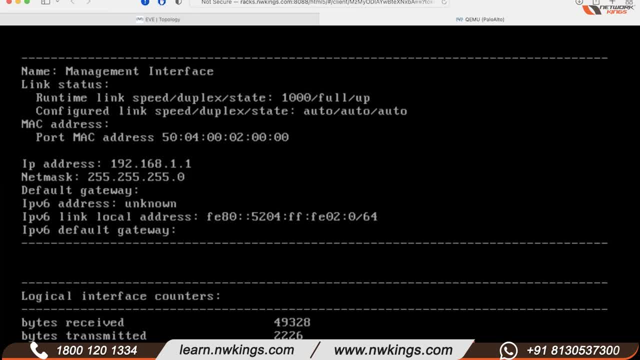 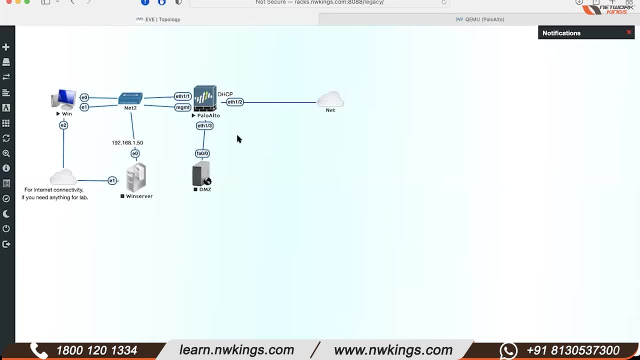 the IP address right. let me revert back to the running configuration, and this time let's, and by default. there's one more default that you should be aware of, for example, that i am on the firewall right and i am trying to- uh, trying to reach some destination. let's say i'm on the. 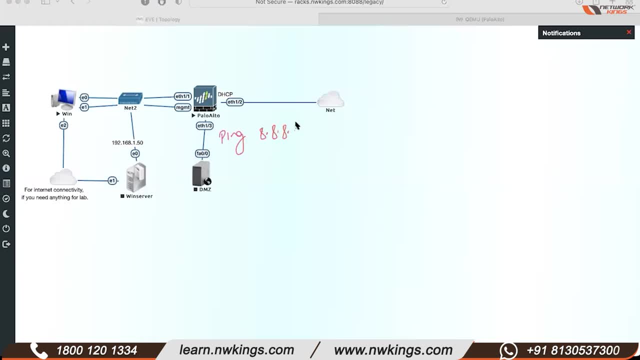 firewall and i do ping 8.8.8.8 in this situation, right, will i be able to ping? the answer is no and i will not be able to communicate with being uh, with this public ip address, right, even though i have public connection, even though i have default route connected and everything in place. 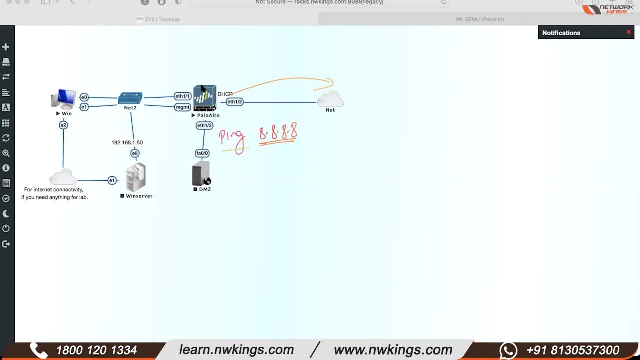 right because by default, when the firewall initiates communication- and not just for ping, be it any communication- the communication initiated by the firewall always gets initiated from the management interface. so if you simply ping 8.8.8, the source ip in the packet will be. off the map management. that is, 190 to 168, 1.1 and the destination IP will be 8.8.8 right and this will try to go out via management. so whenever you are doing, either do one thing. you change in the production, you can. you can change the default and you can make it behave like normal. 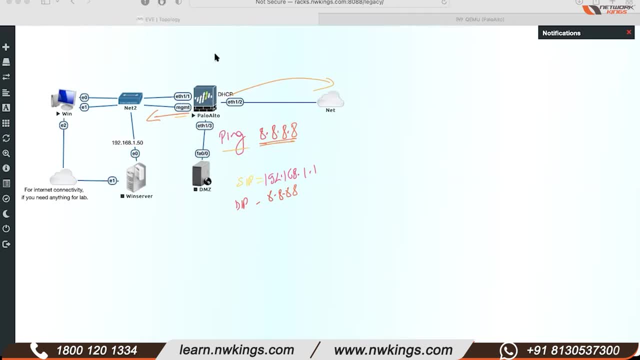 devices right, but that is not recommended because in the in the corporate, you will always have your management interface having a separate network and that separate network will have its own security levels and that will communicate with the Palo Alto servers for license and getting the update. so that will not be a good idea to change that right. 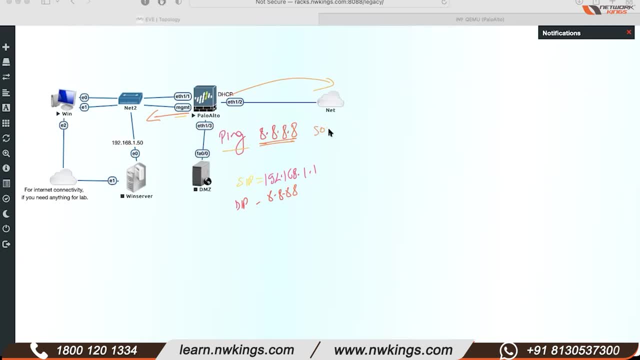 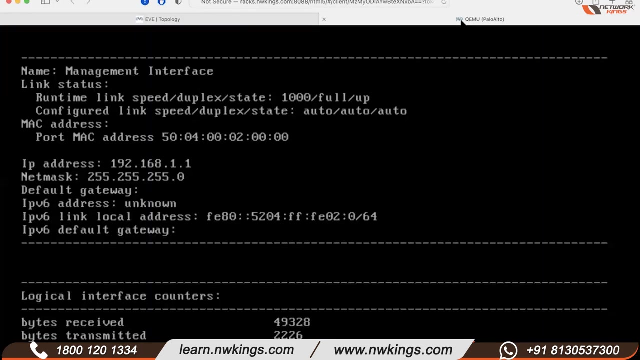 So always when you do ping, add a source to that right source. whatever IP address is there on Ethernet 1 slash 2, right, that's when it will be forced to go out via 1 slash 2. okay, I'll show you, I'll, I'll demonstrate all this. 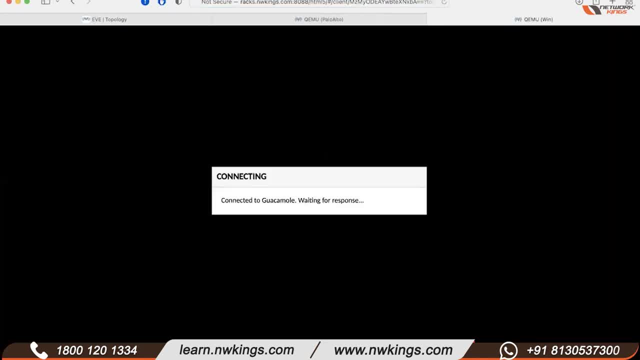 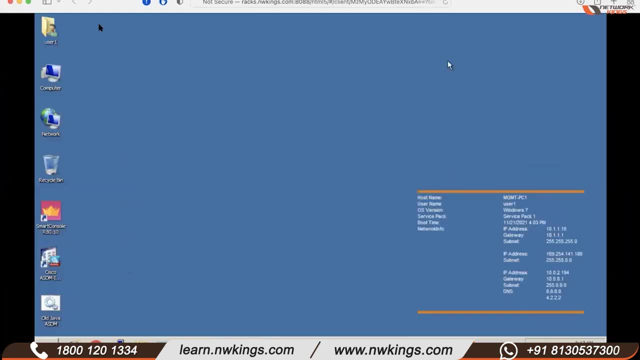 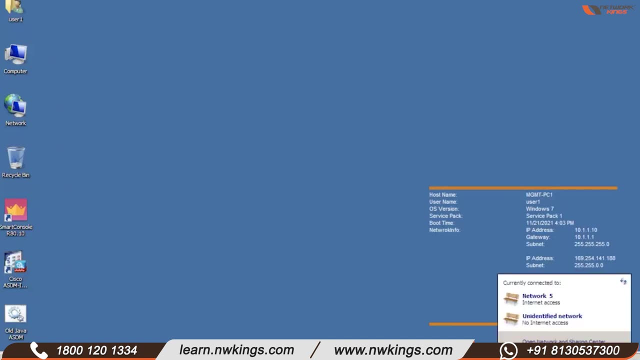 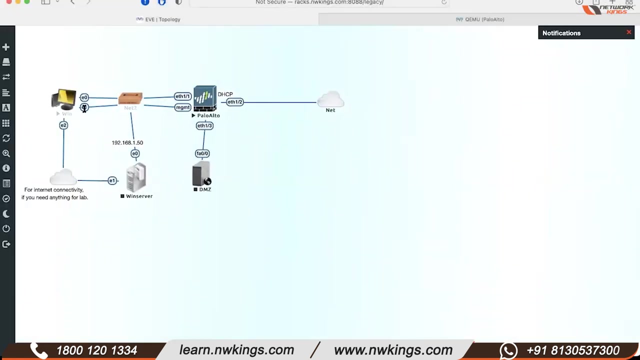 okay, let's get into the PC. Okay, let's get into the PC. So I think we need to change the IP address. yeah, that's the first thing you'll have to do. yes, I have connected this hub for a reason, so that you don't get confused which one to connect with what right? so Ethernet 0 and Ethernet 1.. 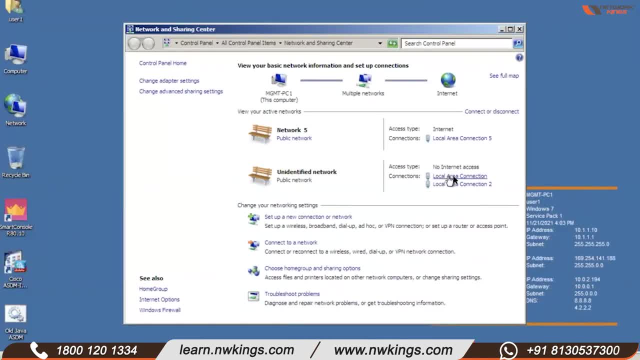 So simply replay. So in this case I will replace Ethernet with local area connection. so Ethernet 0 is local area connection and Ethernet 1 is local area connection too, and Ethernet two is locally that connection 5.. Okay, so in the increasing order simply read Ethernet as local area and go on the increasing order. 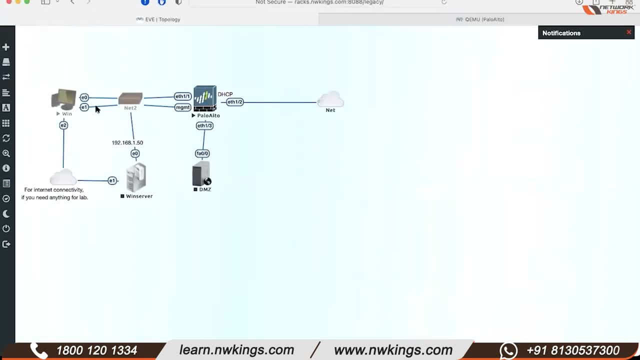 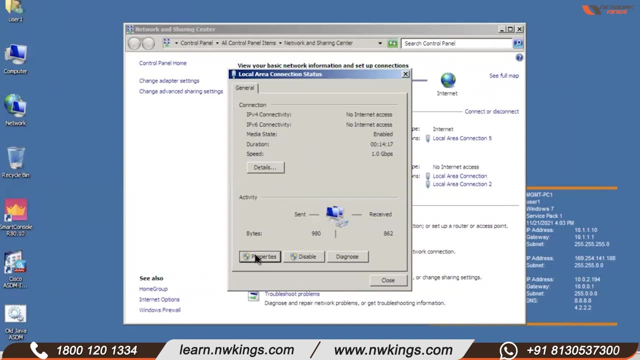 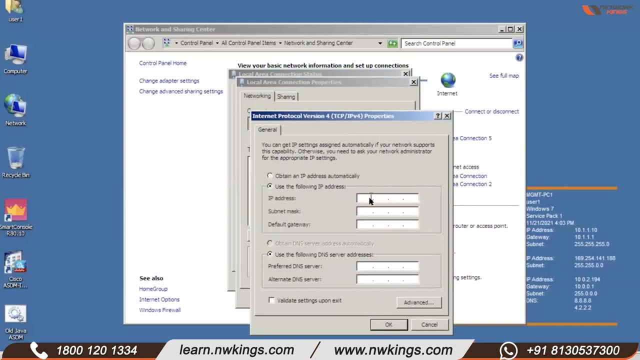 So if I were to give IP address to Ethernet Zero, I will go to. Okay, so Music local area connection. i will dedicate this for the management. 192 168, 1.10. no dns. no gateway needed as we are directly connected. 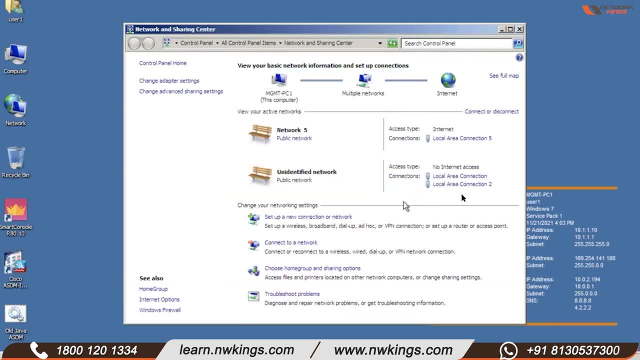 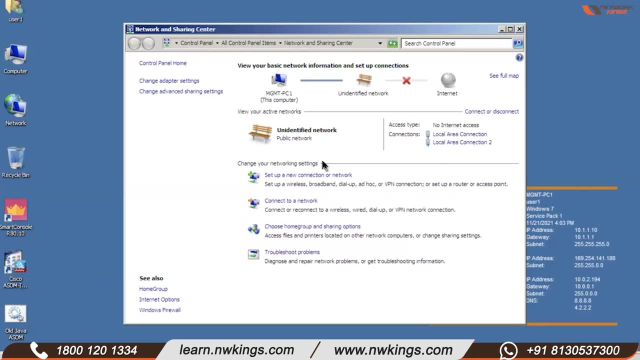 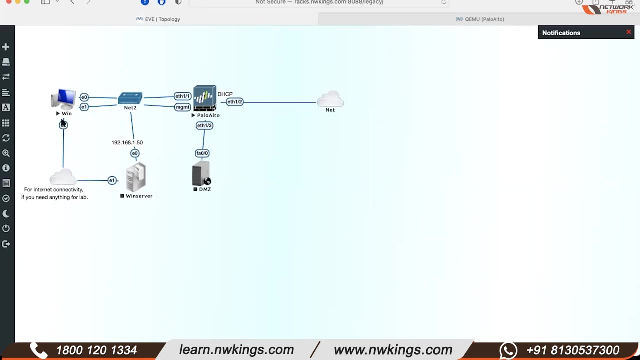 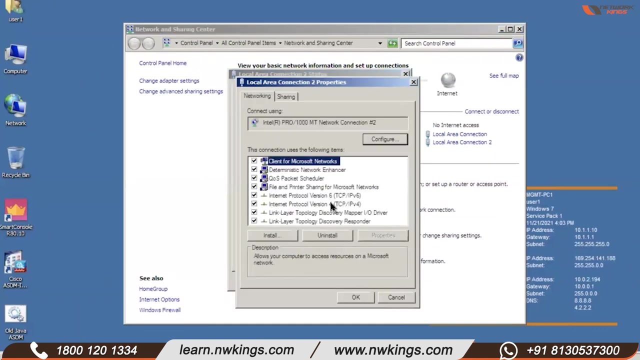 right and for now i will disable the internet connection on the pc. we will try to in the coming classes. we will try to reach the internet via the firewall, not directly. okay, so i have disabled this on the local area connection 2, that is, ethernet 1. 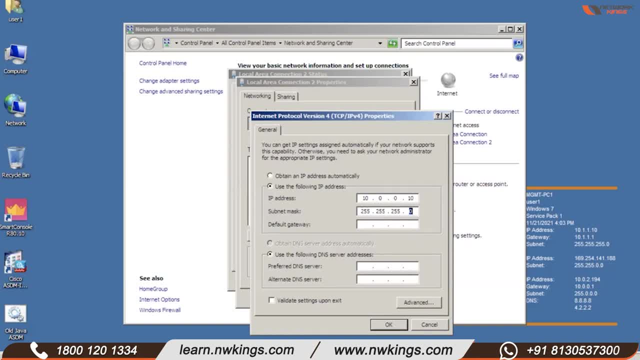 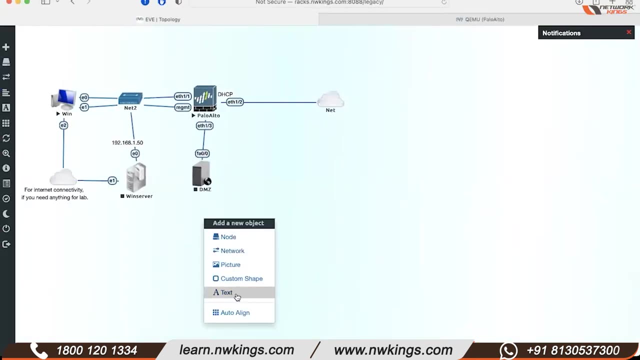 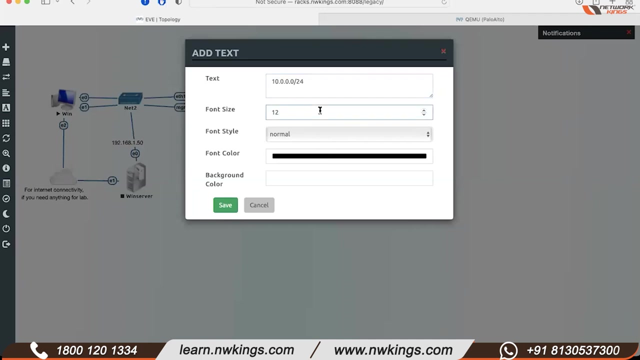 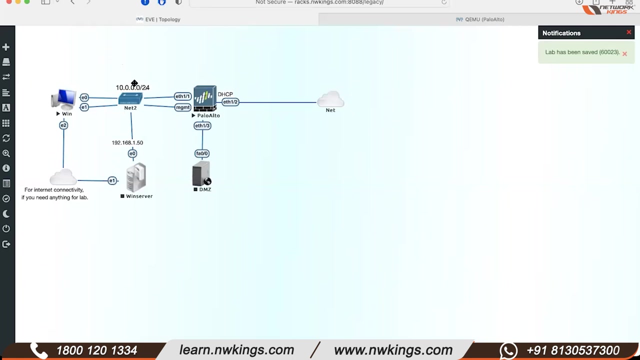 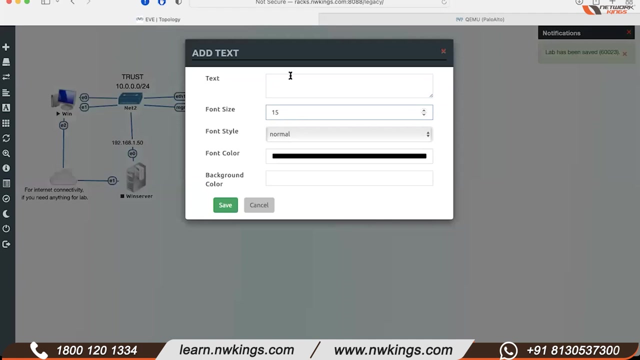 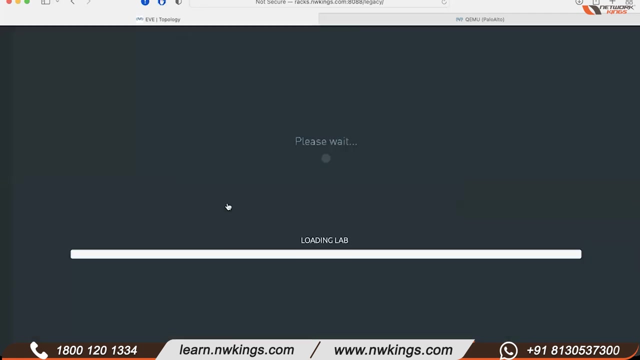 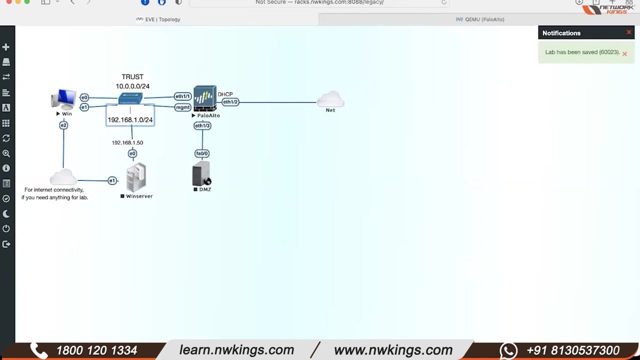 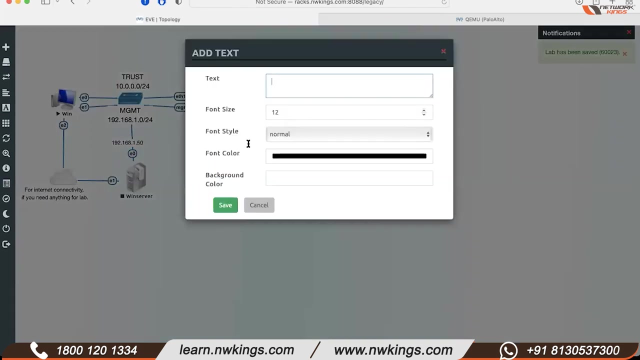 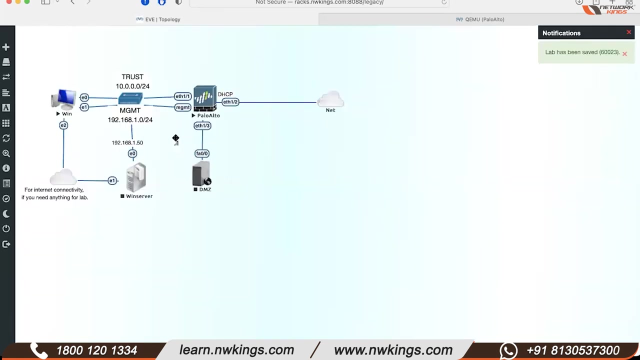 so all right. so let me just add a little text: 10.2.0.0.0. this is your trusted network. okay, and this is for management. the firewall is dot one on both right and the pc is dot 10 for both, like 10.10 for ethernet, 10.1 for development. 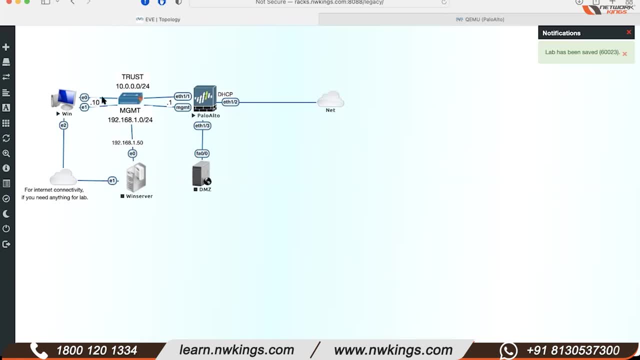 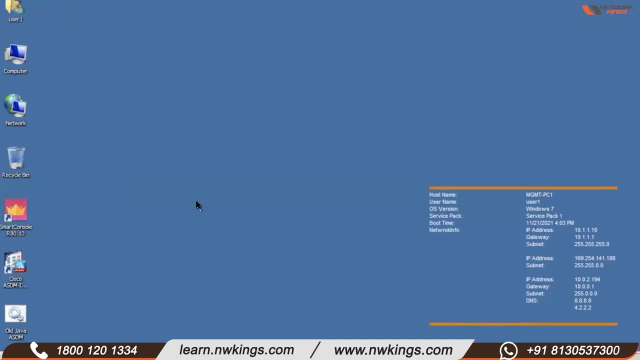 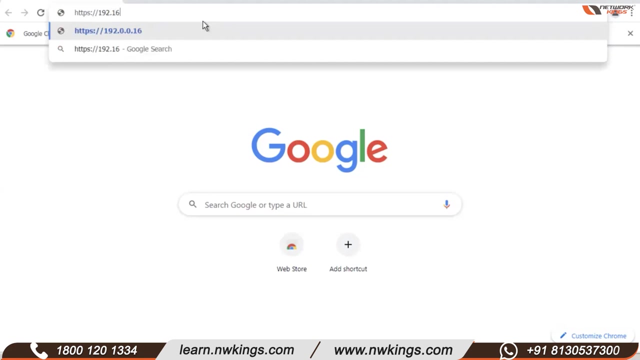 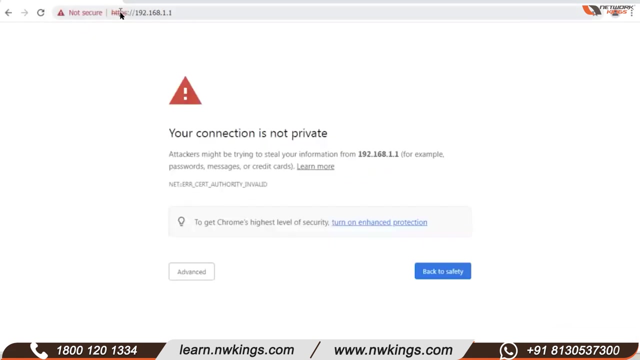 one which is connecting, and 190 to 168, 1.10, which connects to the management. all right, so once that is done, you can access the firewall through the browser. so, okay, i think we are on version 9 or something, definitely not 10.. 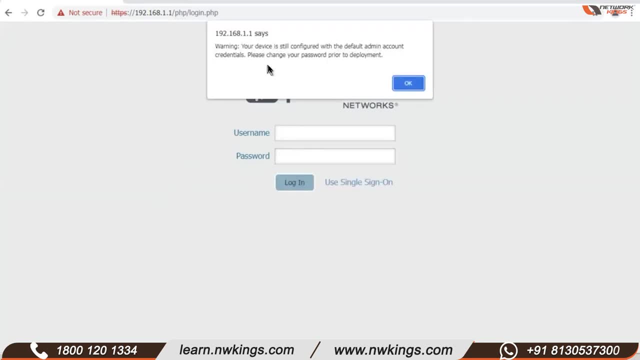 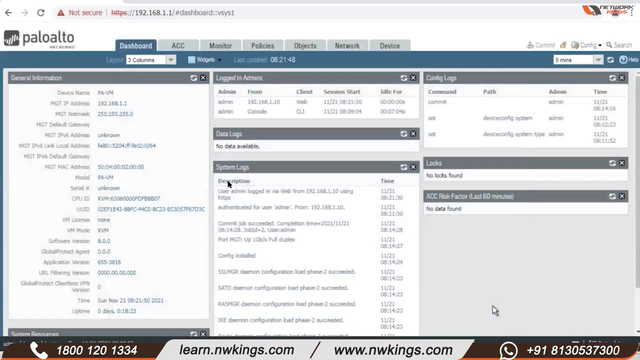 okay, the message is: you're using the default admin account. right, consider changing the password before you deploy this in production, right? obvious things. you would not want to have default password on your firewall. okay, even better, we are running version 8. this is good for ha and other things as well. 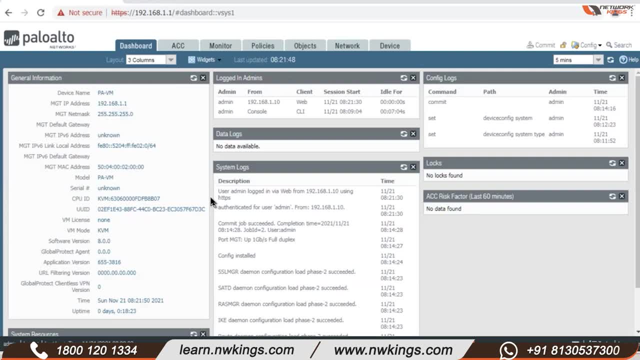 right, but coming, uh, in the coming classes i'll try to show you version 10 right, which is the latest. 10 and 11 is like more or less the same, so we'll go through the newer gui, trust me. just the changes in color, no changes in the placement of objects right and some additional cloud features. 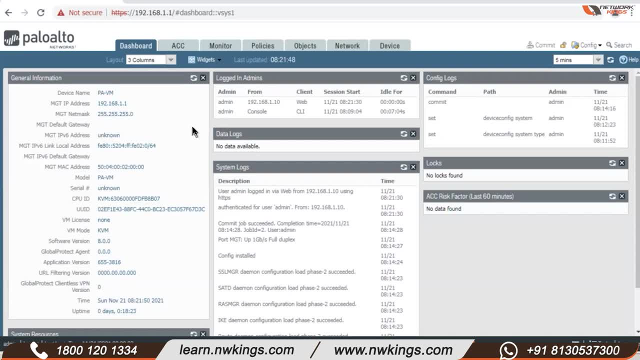 that's it. so for now, let's uh do things on this as well. as you can see, this is a virtual machine model, right, it's a palo alto vm and the vm mode that it runs on is kvm, that is, uh specific to even g, that is the hypervisor, which is uh, you know, facilitating the hardware to this virtual machine. 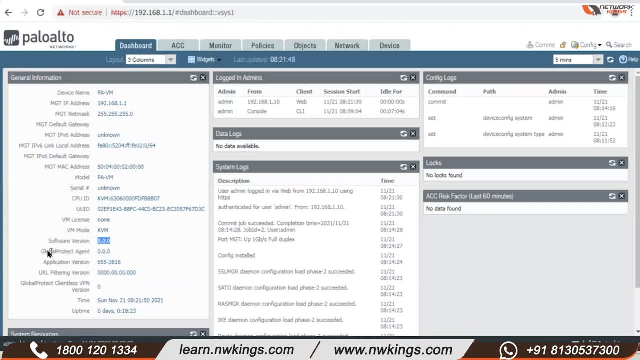 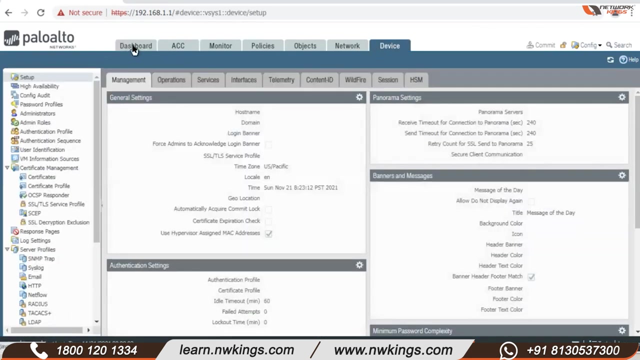 the version. software version is eight. right, these are the other next generation features, like application version, url filtering version. all of this needs- uh, uh needs licensing, right. so i'll be telling you we'll. we'll talk about this, uh, but not practically. and these are the widgets. by the way, these are on the dashboard. these are default. 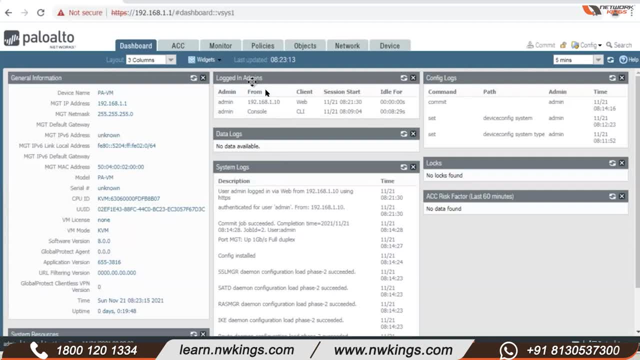 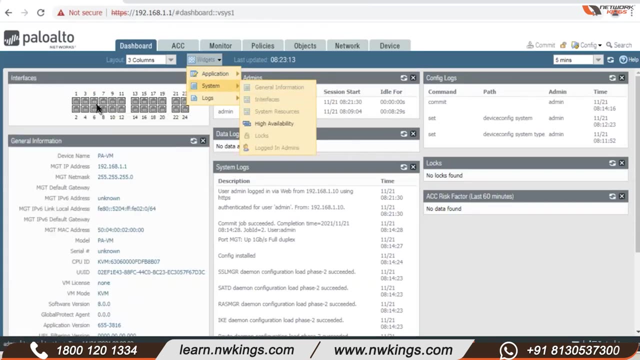 widgets talks about system, system logs, logged in, administration, administrator, and we can, you know, have more of the widgets. for example, you can have it for interfaces. these are the ones that we'll be. These are the interfaces. If anything goes, the change in status will be reflected here. 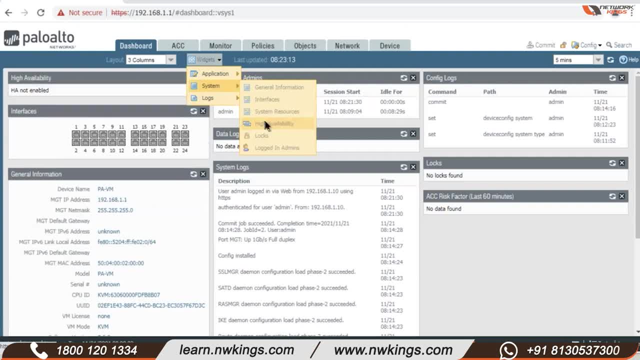 and very useful. the HA widget. These are like the widgets that you see on your smartphones. They don't actually hold the data. You cannot really configure things here, but it is pulling information and displaying it here. Any device changes, as I mentioned in the CLI. 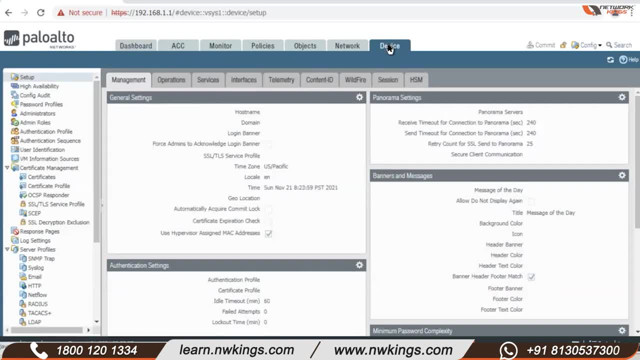 And the CLI guys. it is designed in such a way that if I were to tell you a command, I can look at the GUI and tell you the command. For example, I have to change the IP address. It will be under the device config. 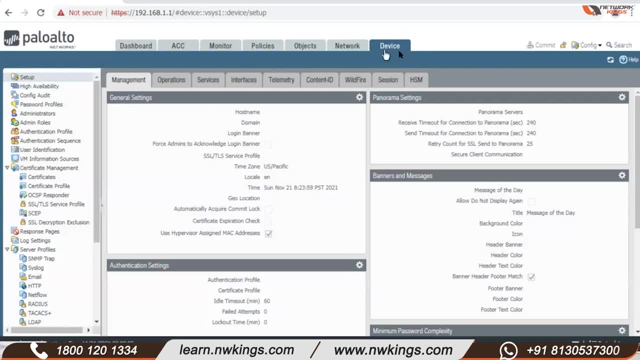 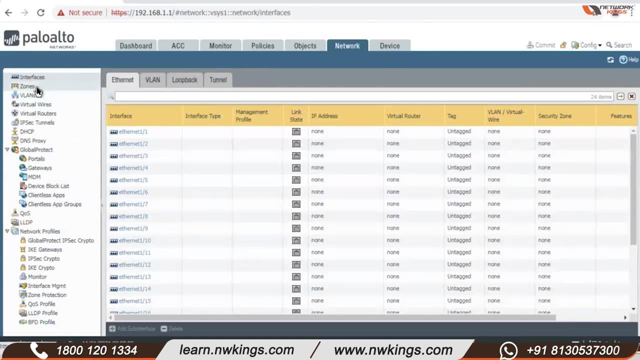 Set device config management or set device config system Similar to it. When I have to change the IP address, the command will be set network and the interface or set network and zone. So the CLI is more like aligned with the GUI, And that's the best part. 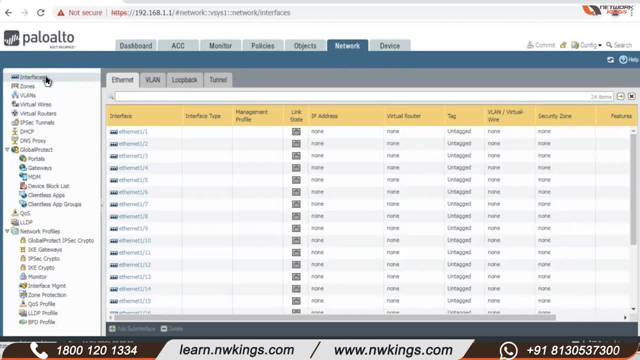 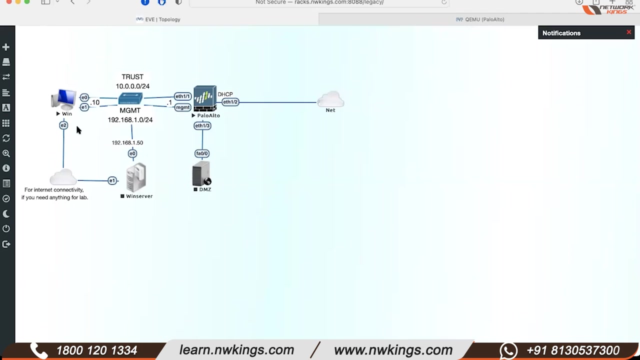 Before going forward, I have one question which you have already just explained. Can you just show me this picture again, Sorry? Which picture? Network diagram. Okay, This one Yeah, Why we disable this E2 port And if we not disable it, what will happen. 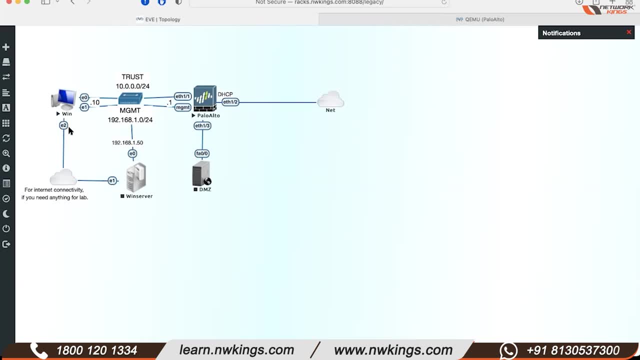 Or else why we are using this here. Because we are using this external traffic. For that we have connected this. We are using this here just in case that you need internet connectivity from the device, This server. This for you, Not just for the server. 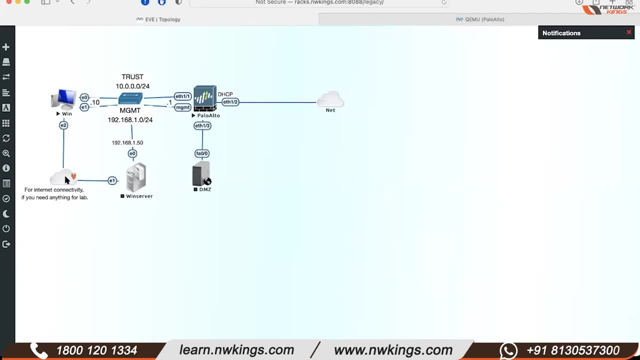 for example, this server or this PC. If you require any software from internet, you can download that. You can simply enable this and download software from the internet. right, It is just to give you internet accessibility from the inside of, directly from Windows Server, to outside. 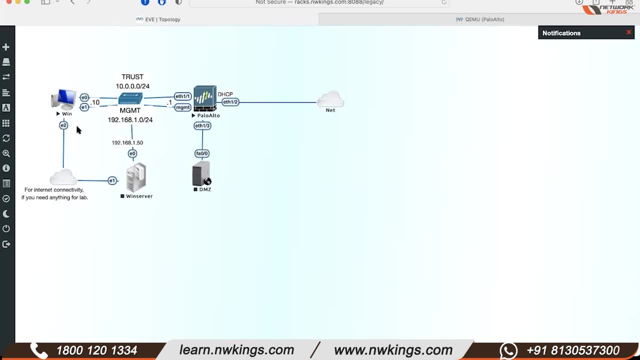 That's why you just stop it. I mean, I disabled it because we are now about to learn that. How would you create policies on the firewall that will allow the communication from the PC to internet? If you not disable this one, it will create problem. 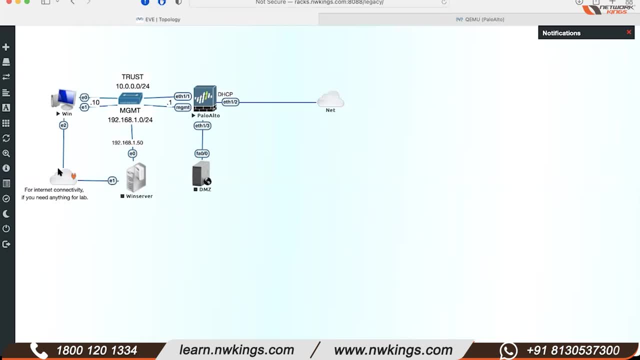 Yes, you will directly go through this path, right? If you have to reach a particular destination, there is a direct flight and then there is a layover. which one you will you choose, Okay. So actually I thought that when you will, you know. that's more of a layman way to explain. 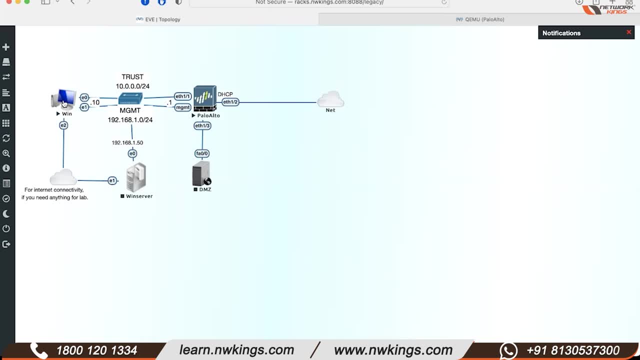 But technically, if you see, you will have to assign gateway on the PC, right? So the default gateway can be either this or this. That's what we have configured. management gateway- no, Management is only for management Management, But we have configured this Ethernet one gateway, also already configured in the Palo Alto 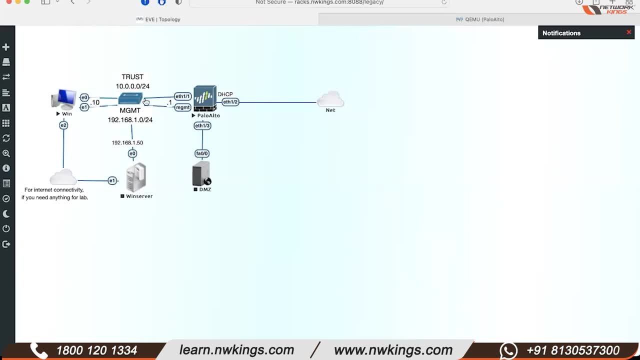 This Right. The net one is connecting to Ethernet one slash one here on the firewall. So the firewall becomes the gateway. So you have to give the gateway information right. So that will be also configured on the firewall, sir, right. 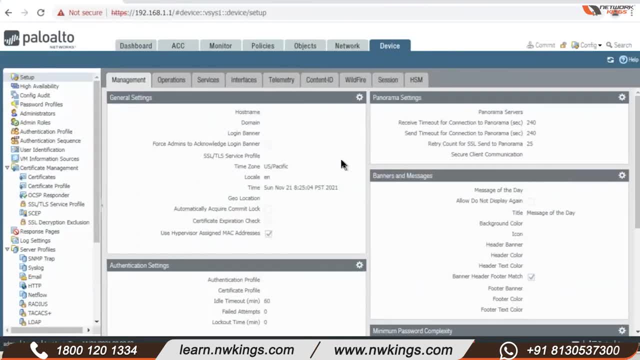 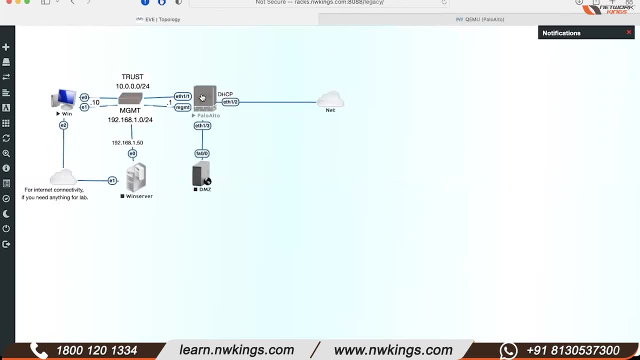 If that one means in the confusion, and this is that this is directly connected. And if you want the firewall to forward your package, you have to make sure that you have the, the, the. The packet from the PC reaches the firewall right, Okay? 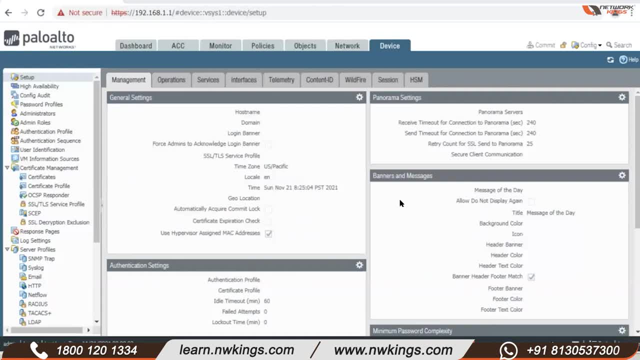 What is the purpose of? So it is configured. You see that already. No, no, no, Tell me what is the purpose of this. Oh, It is the default gateway, right? Yes, Yes, To reach any destination, you go to the firewall. 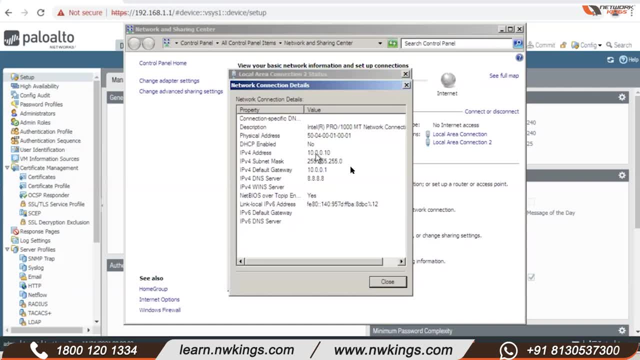 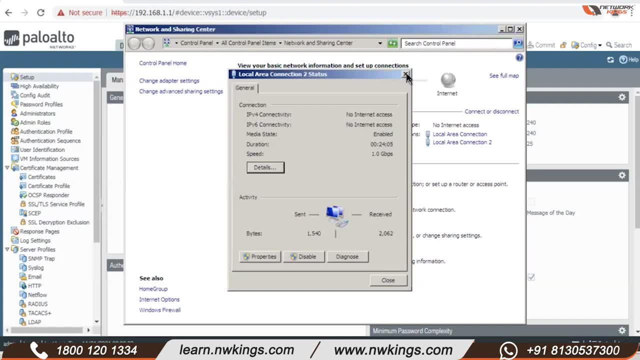 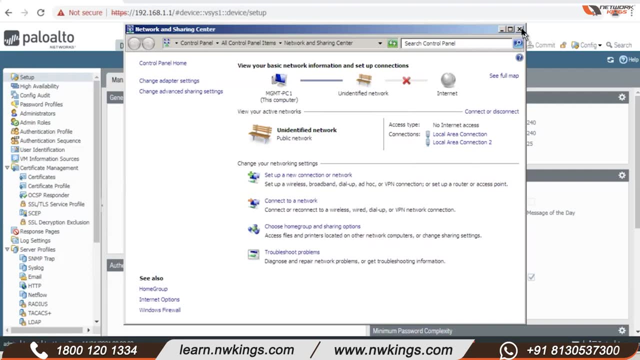 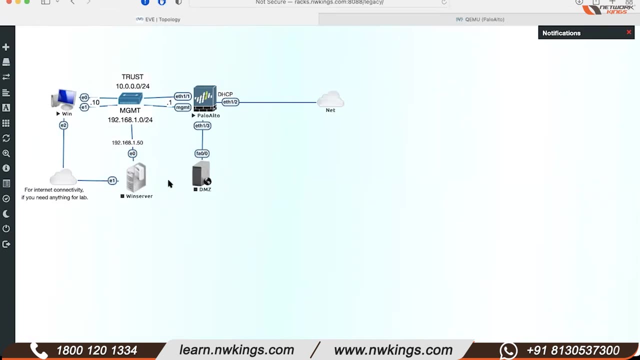 interpreter on the file, But with my question. So is there any purpose do to keep that? that's over. The server is missing. the coming feature, Yeah, this one, the win-win. So I have not even turned it on, Okay. 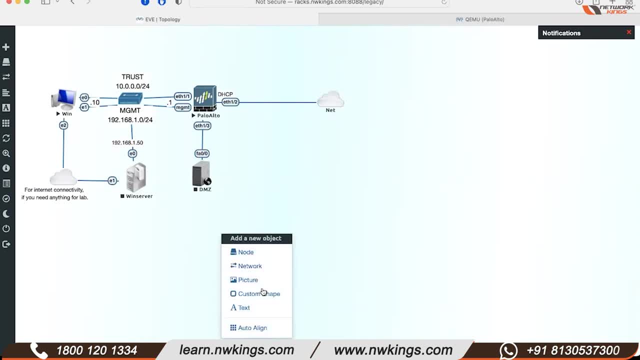 This factor. Okay, Okay, It is Okay. i have a question like: uh, the ethernet zero and ethernet, so both is assigned dot 10, or like, sorry come again. or the ethernet zero and ethernet one of this uh windows server, so is it like dot 10 is assigned for both the interface, or like 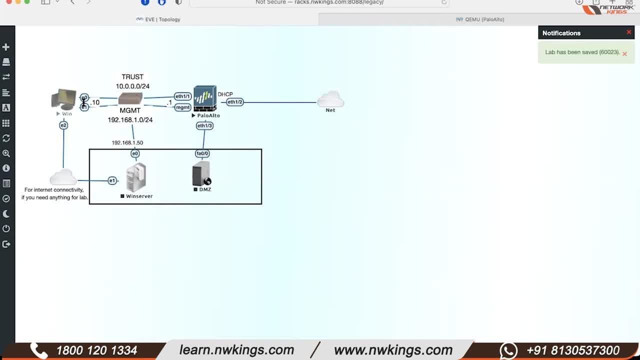 dot 10 is assigned for both. yes, only data interface, not management interface. can you guys stop overthinking? right basic logic. right, two interfaces will have different networks. right, two interfaces of any layer 3 device will be part of different networks. so ethernet 0 is part of 190 to 168. 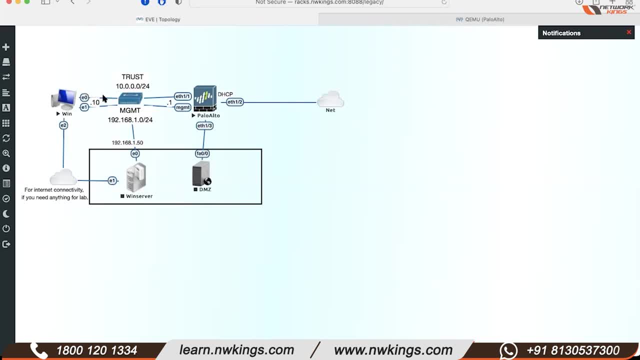 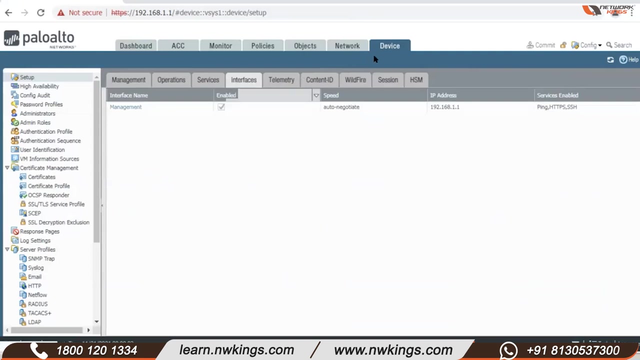 1.0 network, that's dot 10 on ethernet 0 and ethernet 1 has 10.0010, right, yeah, so this is this is basic stuff. okay, forget it, no battery. now let's try to configure the interfaces of the firewall. so under devices, it's just management. 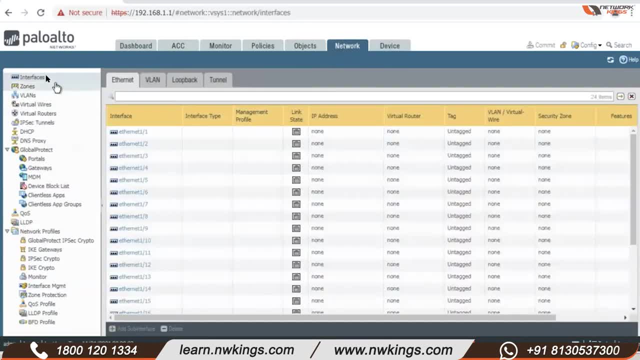 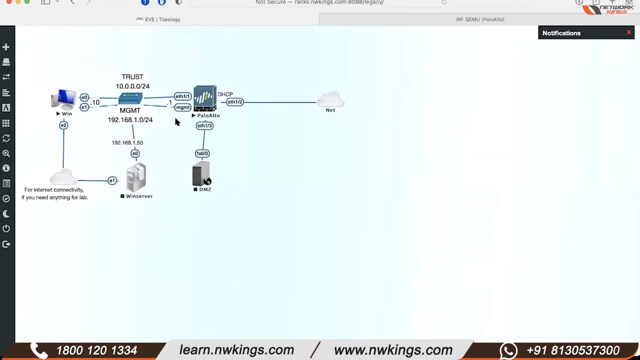 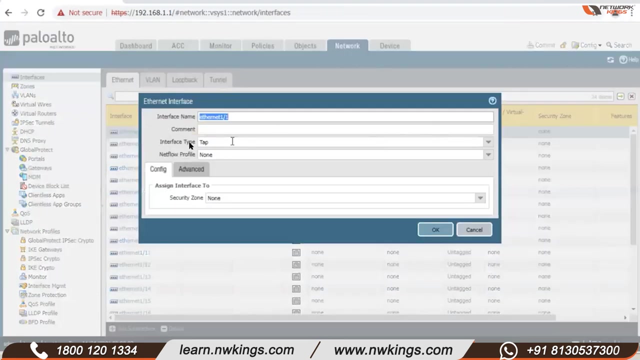 interface, the data interfaces are under network and even before configuring the interfaces, the interfaces have to be part of some zone. okay, it is mandatory for uh, the interface to be part of a particular zone. all right, so slash one. there are different type of interfaces. I'll talk about them one by 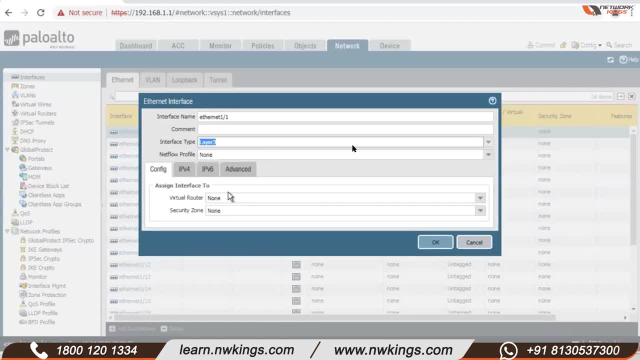 one. let me just configure it first. so the type right now is layer 3, because I'm going to assign an IP address to it and, IP address being a layer 3, I layer 3 entity, right, hence the type: layer 3, virtual router. okay, and the security. 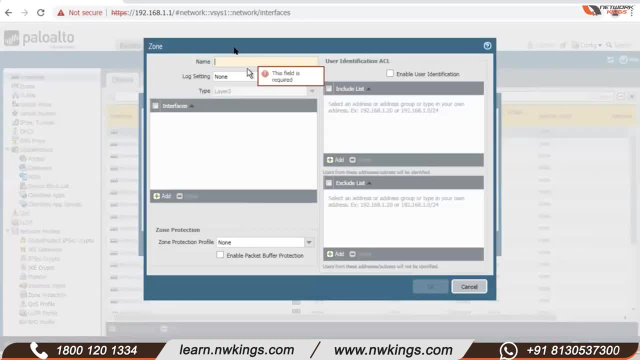 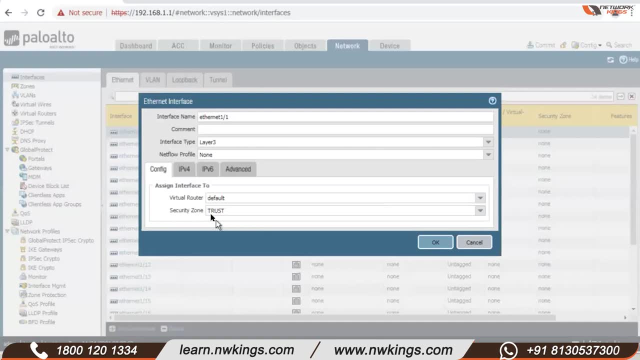 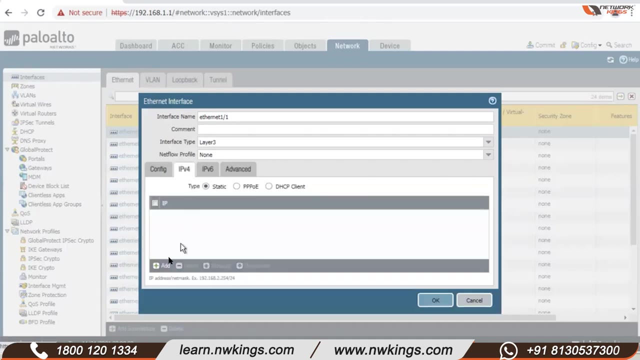 zone. let me just create a zone, then I explain about the virtual router as well. so I name it trust and simply okay, right, which means now Ethernet 1, slash 1 is part of the zone. trust, right, and the IP address on this is ten dot zero dot zero. 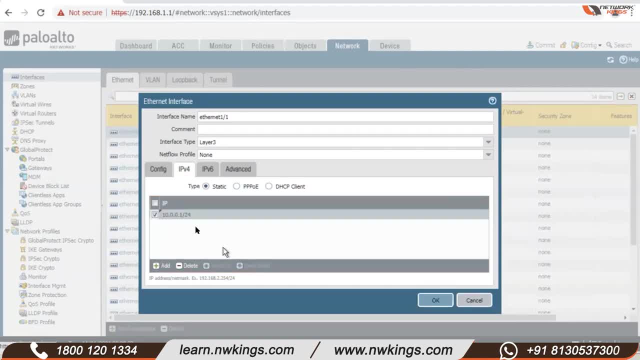 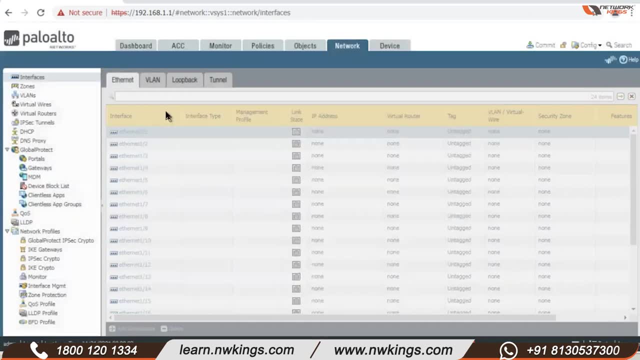 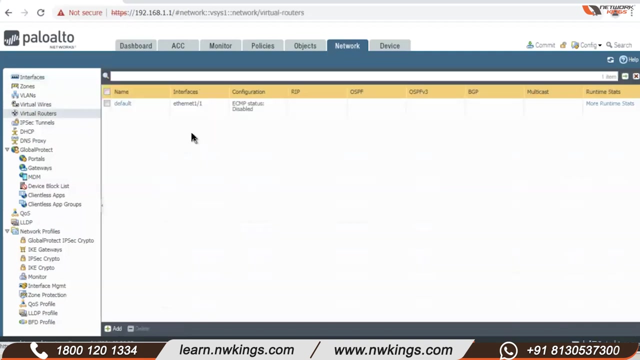 dot one 1, slash 24. yes, you can write like this in the GUI. all right, and about the virtual router: each interface have to be part of some virtual router in order to be able to do routing. okay, the firewall basically has an option to create multiple routing domains, for example in routers. we have VRF right where you can. 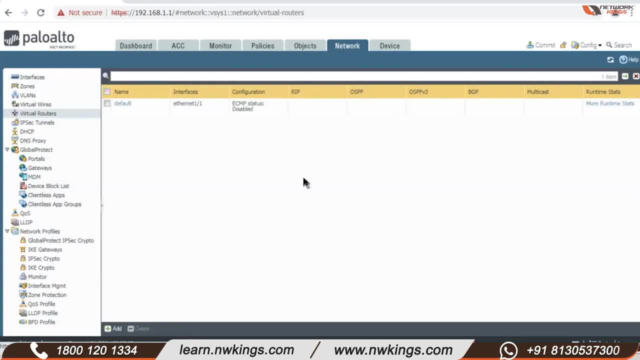 create VRF instances and different interfaces can be part of different VRFs, right. so with the same logic, by default there is this default virtual router, right named as default, but you can create more if needed. when would you need it? right? you may think that why would I need? 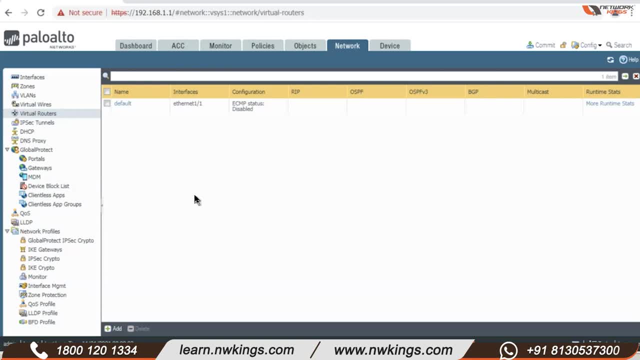 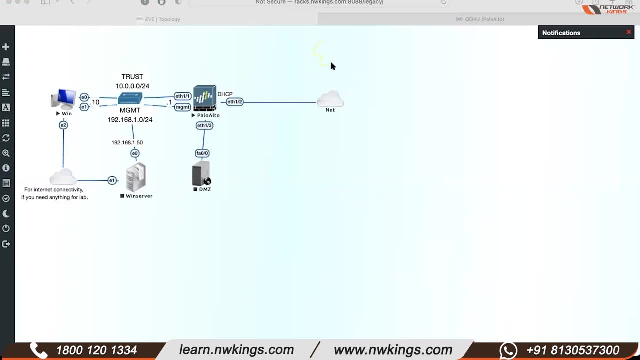 multiple virtual routers. if I need multiple virtual routers, if I need multiple routing domains in firewall- right, that is, if at all, you have to create a BGP peering with different AS numbers, right. for example, this is Google Cloud, this is Amazon and the the private clouds need the. 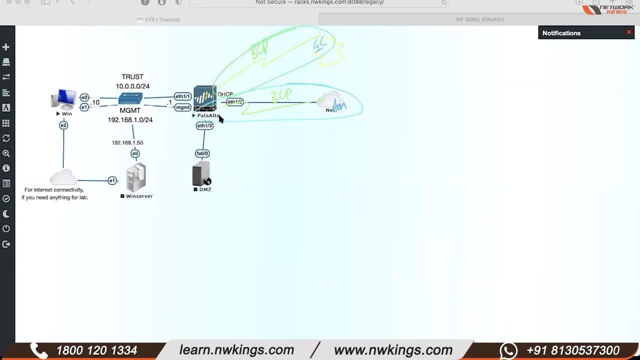 the AS number to be a particular number on your firewall. so the requirement for Google Cloud is, let's say, 65,000, right, and for Amazon it is say 64,000, right. so you cannot have, you cannot have two different AS numbers on the same router. 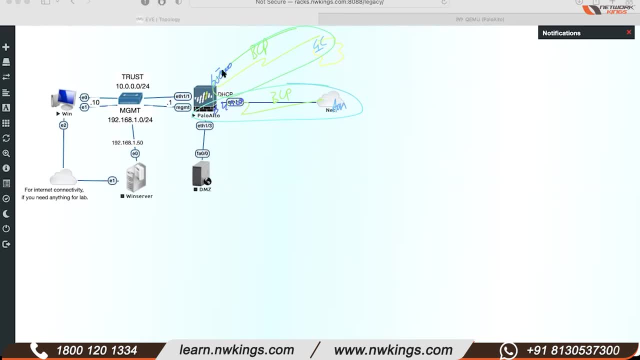 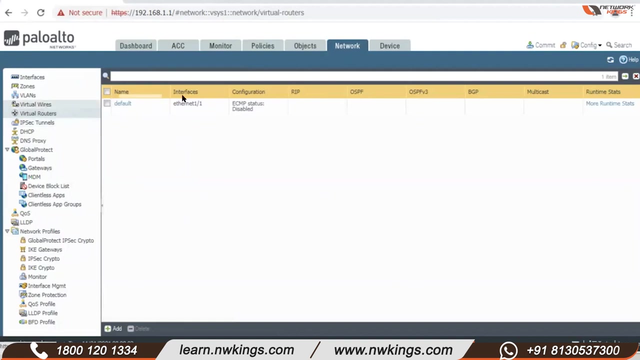 and for BGP configuration right. so that way you can have virtual router 1 and virtual router 2. so this way you can have two BGP pairings on the same firewall right, very specific use cases. but yes, it is what it is. so for now, just understand that to do routing, the interface has to be part. 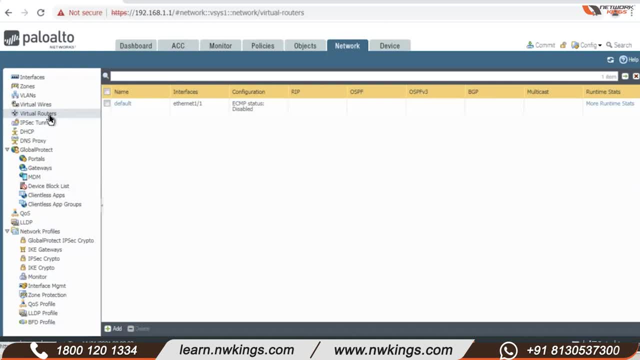 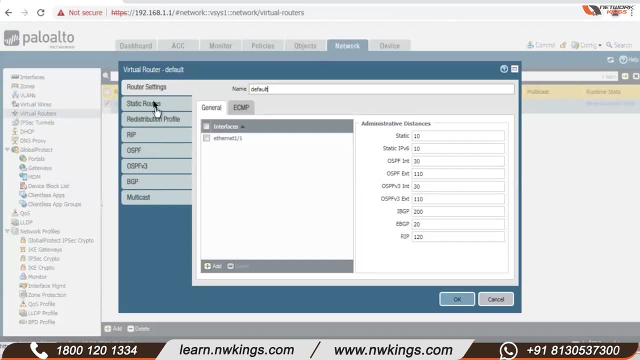 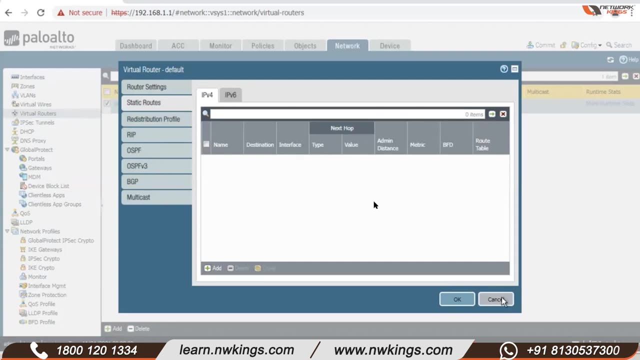 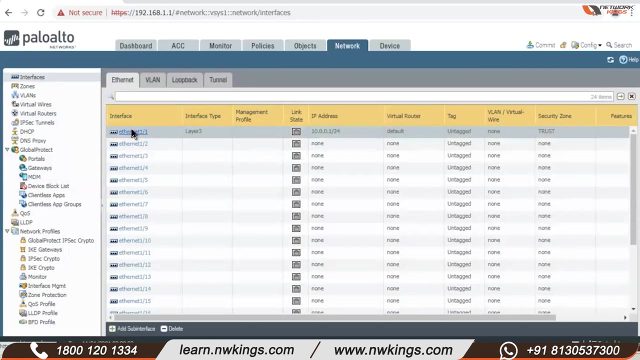 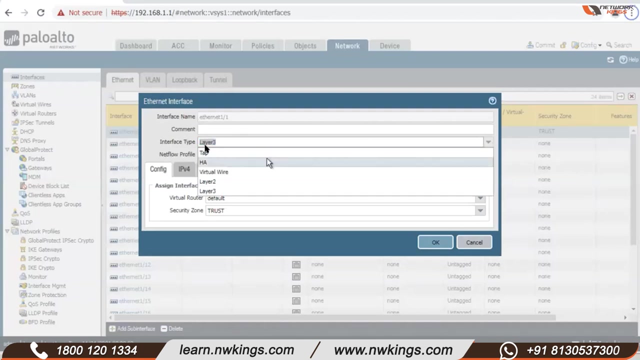 of the virtual routers. obviously you can configure OSPF, BGP and all that right. all the protocols are here. you can do static routing, you can do ospf version 2, version 3, bgp, everything is there about the interface types: tap, tap. interface is literally like a tap. okay, you have the pc talking to the firewall. 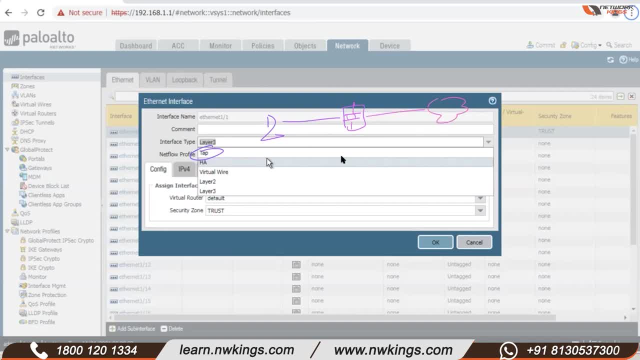 or communicating through the firewall. right, and you as, as as part of uh troubleshooting, you want to collect the data traveling from this interface to that interface. right, you want sampling, so you would simply connect a pc to this interface, make this as a tap interface, and this is literally. 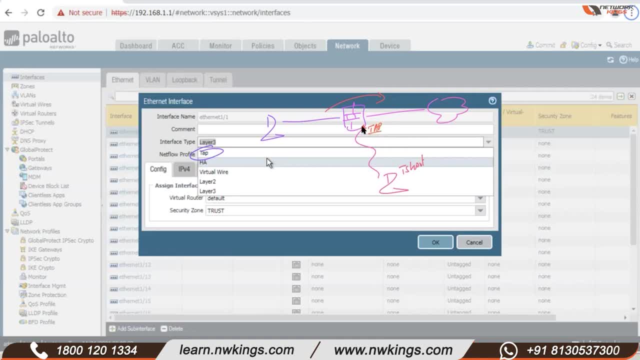 like you, open up the water tap every morning, right, the water flows through it, so simply, a tap interface will give you all of the data and you can collect it on the wireshark and you can do analysis and all that. okay, so very specific use case in production do we use this answer is no right because 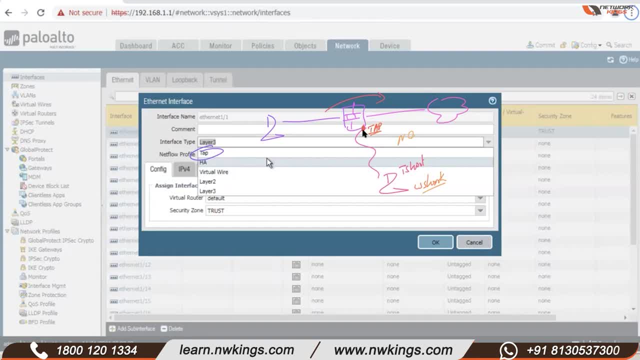 firewall is a device with limited number of interfaces and you wouldn't? the chances are very high that you will not have a interface which is empty and you can simply connect a laptop to it. right, you will always have to work it through the switches and through uh span ports, if you guys. 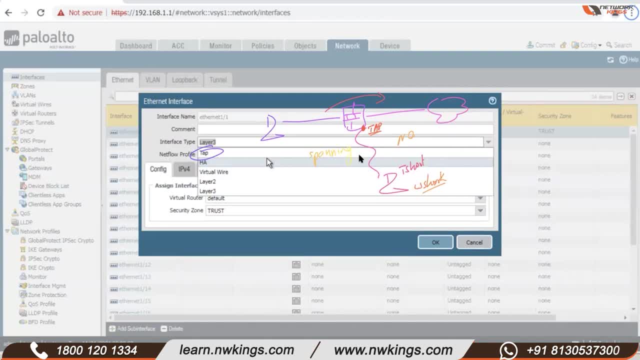 know, spanning remote span or local span, you can refer it right. it's like, uh, it's like mirroring the port. anything that is inbound to this has to be shared on the on the other port right, and the pc connects to the switch port and that collects and collects in the wireshark. 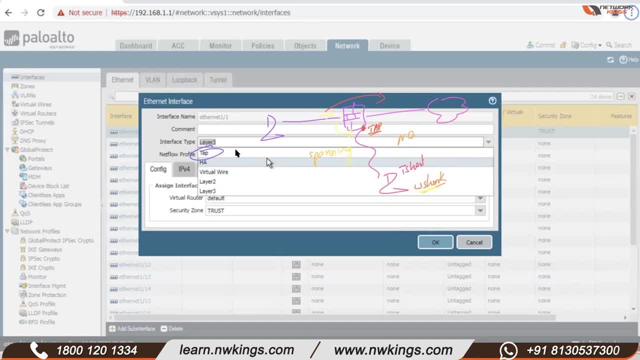 and you can analyze. so it is basically for troubleshooting. ha port is for ha. i'll talk about it later on. yeah, virtual wire, virtual wire is literally like like a soft wire, again a firewall connecting two interfaces and if they are a virtual wire, virtual wire will be. 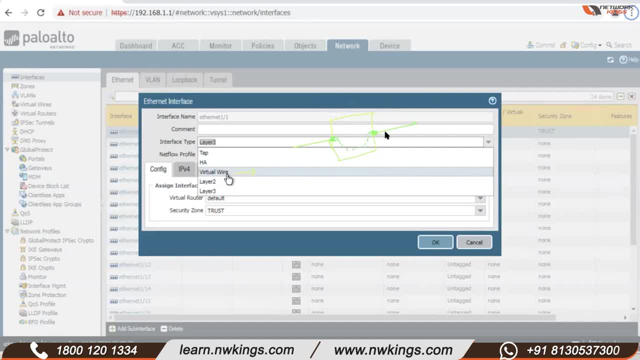 something which connects them, bypassing everything, and the firewall will be bypassed and it will be like a simple wire in between right, no policies, nothing. when would you want to do this? when you want to configure the firewall, you're putting it new in the network. you would simply ruck it up and then. 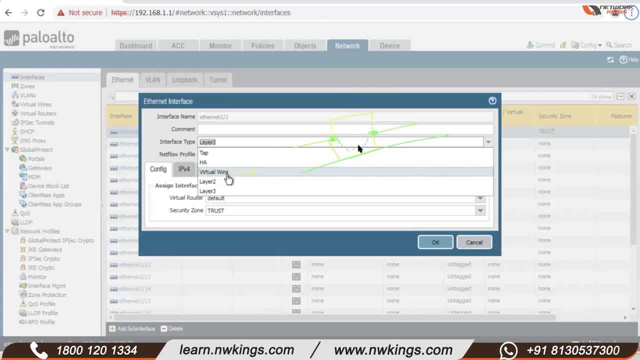 connect the management, connect all the cables and you know you, you put them in the virtual wire by default out of the box. the firewall is in this virtual wire mode, right? you don't. you can do things like either you don't connect the wireless or you can connect the wire back where it was active. 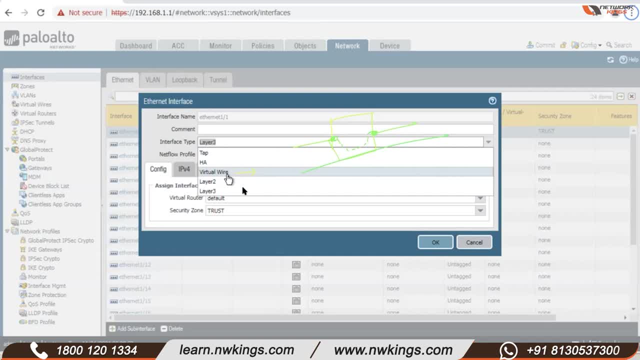 don't connect any data interface, or you connect them, configure the virtual wire and when all of the remaining configuration is done, you remove the virtual wire and put the actual configuration, which will be the layer 3 config. okay, so it is again a very specific use case. 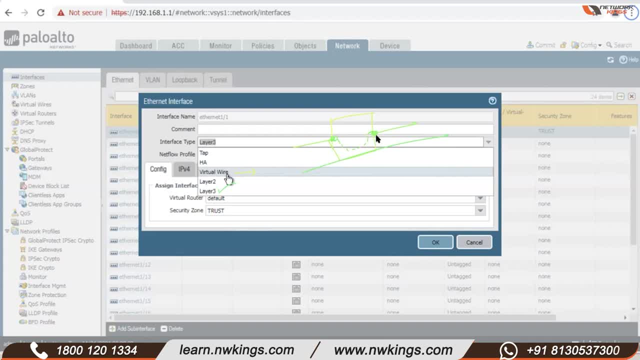 in production. do you really use this? again? the answer is yes or no, both depending upon how do you want to implement your firewall. you want to configure everything first and then rack it, or you want to rack it first and then remotely access it. it all depends on the different scenarios. 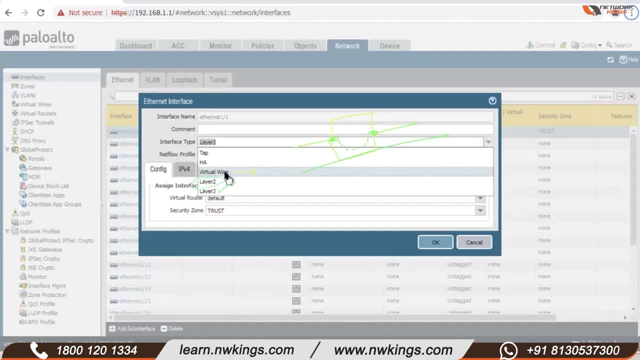 again. the other mode is layer 2 interface. layer 2 interface means it's still layer 2, it's still as good as a cable, but you can still have policies in place now. it's not a wire that is connecting internally. you will have, you can still have. 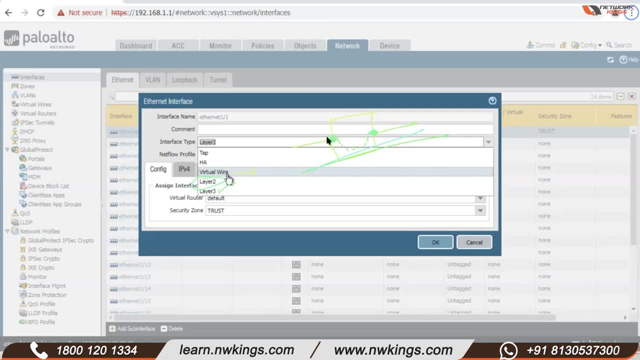 layer 2 interfaces, but you can still have policies in place. now it's not a wire that is connected internally. you will have. you can still have policies in place. now it's not a wire that is layer 2 communication through it and some limited firewall features can be used here. 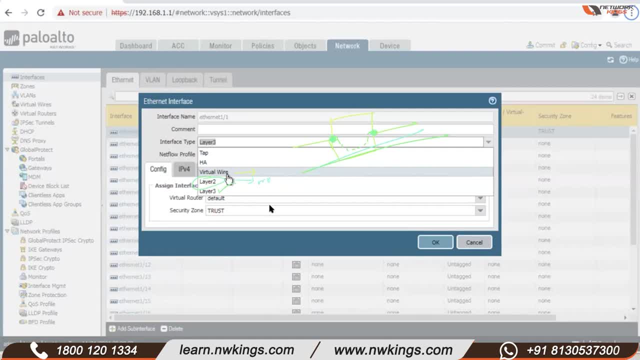 do we use this in production? no, right, because, uh, you can use only limited features of the firewall when it is running in layer 2 mode. right, layer 2 is like uh, buying a super bike and not going on weekend rides. yeah, you are uh under utilizing the firewall if you are running this in layer 2 mode. 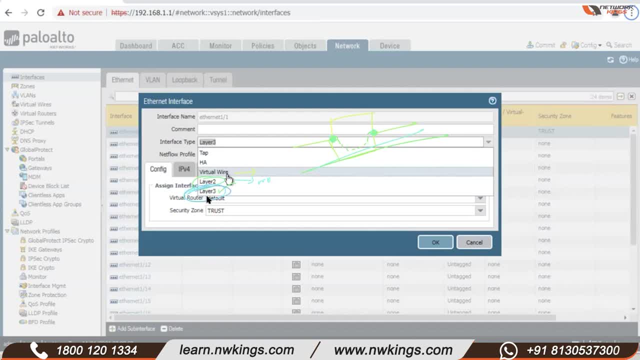 yeah, so most of the time- right like all of the time, not even most all of the times- the interfaces used will be either layer 3 or they will be he right. having said that, let's configure the other interface. or even before doing that, let me show. 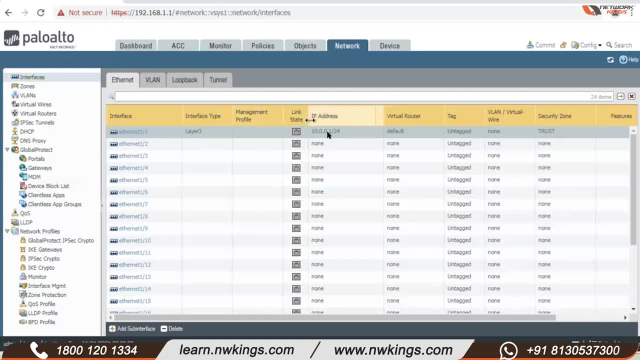 you something: we have to make the changes. do you see the links taken in there? we can just pull up her state. it's still grayed out, which means the link is not up. you see, it is not configured and down and that is because we have not committed the changes. 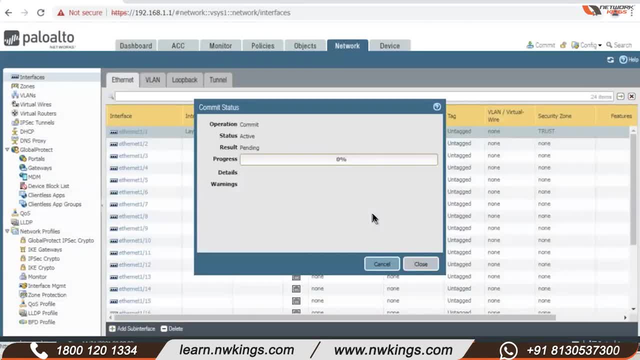 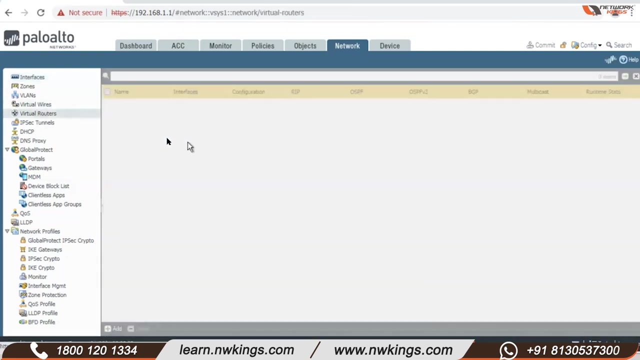 sir, can we create sub interfaces for these? yes, we can. so while configuring the interface, uh, you, uh, you selected default there, so we could also configure virtual order from there as well. right, yes, uh, but the virtual router is. it's already there named as default. you may want to rename this. you can do. yeah, normally in production people. 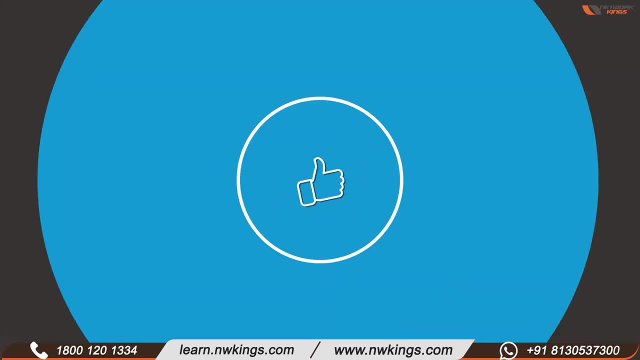 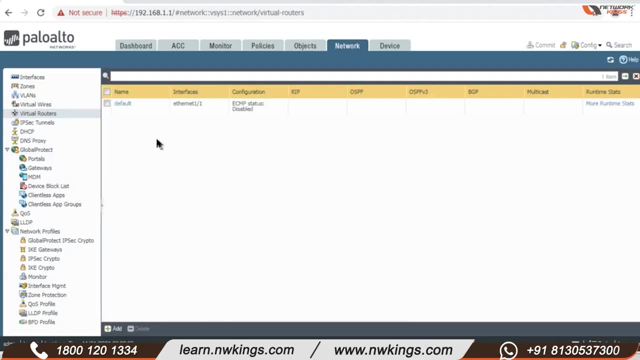 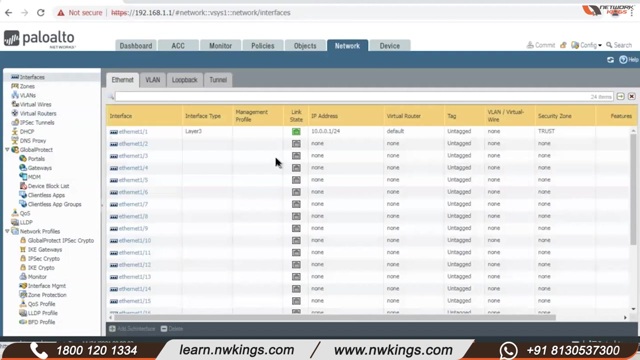 don't do it unless you need multiple routing domains. right, hi, you are watching the recording from one of our live session. hit like share and subscribe for more future updates. okay, uh, sir, there is zone and, uh, security zone. what is the difference? zone and security zone? like you just see zone where is security zone? no, you choose in ethernet one. 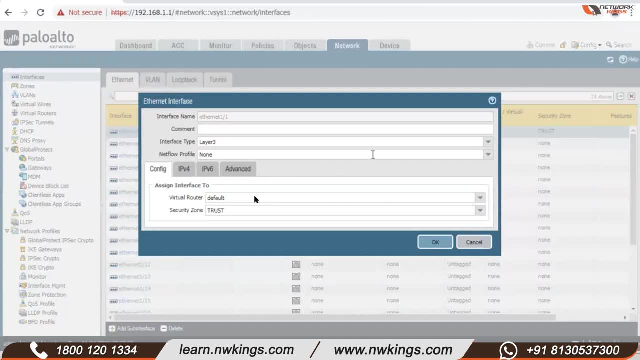 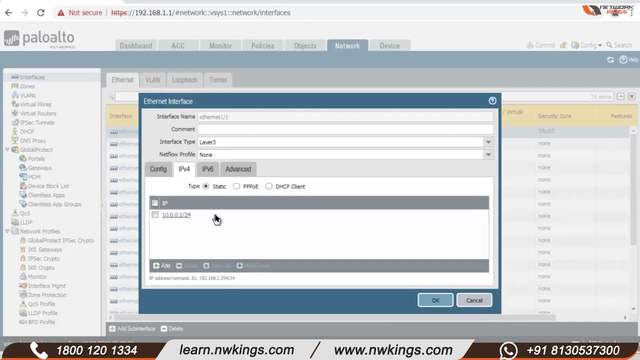 and uh, yeah, inside, yeah, it's one and the same thing. it's one and the same thing. zone or security zone, it's the same right. so for now we have uh created one zone that is trust, and we have made ethernet one slash, one part of it, security zone, and there was a left side showing it's only zones in that. 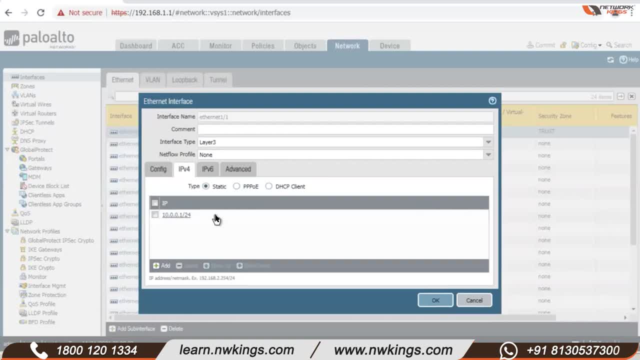 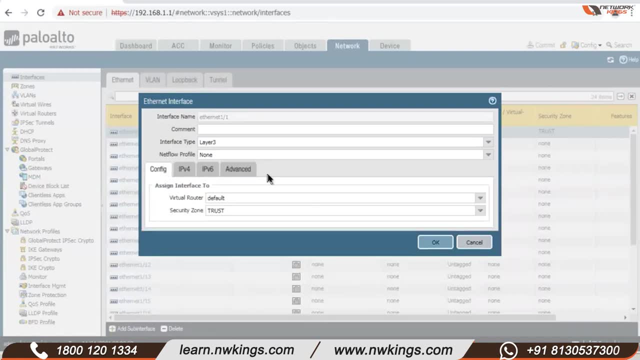 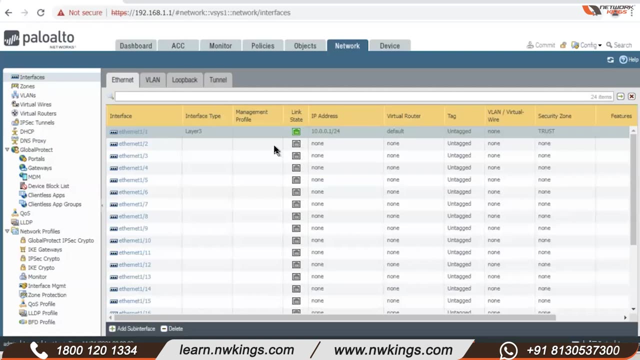 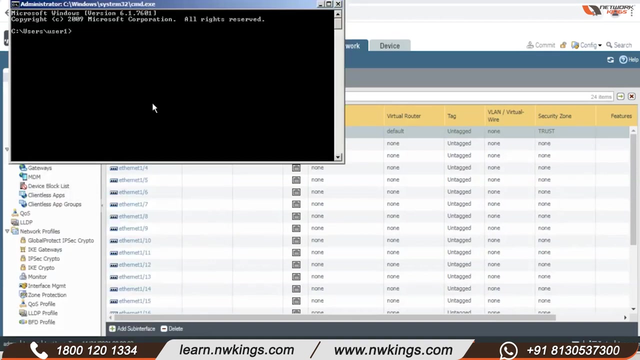 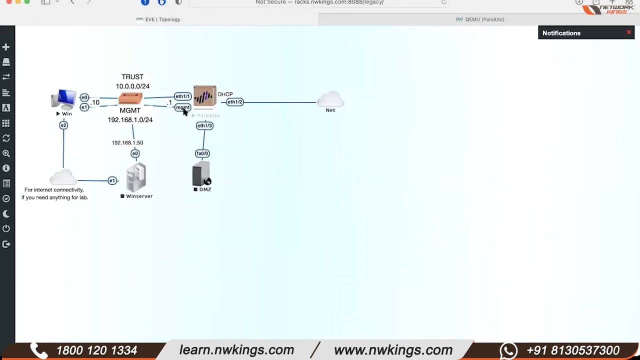 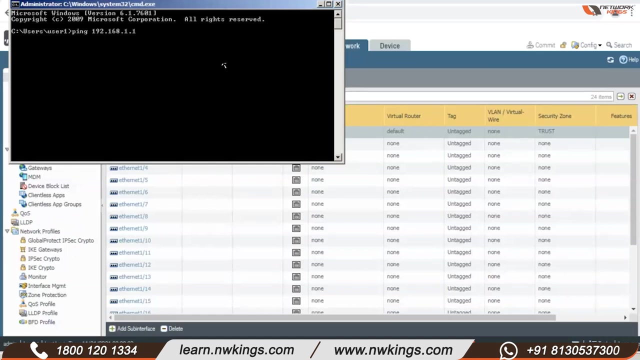 okay, okay, sir, uh, okay, now let's verify things which we have been talking about, and i try to ping 192 168 1.1, which is the management interface of the firewall. will i be able to ping this? no, this is the management. i think yes, sir. 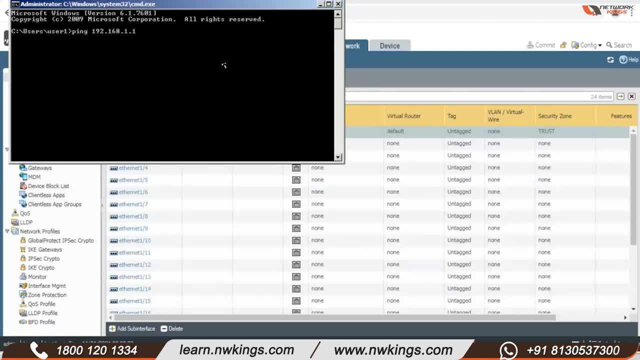 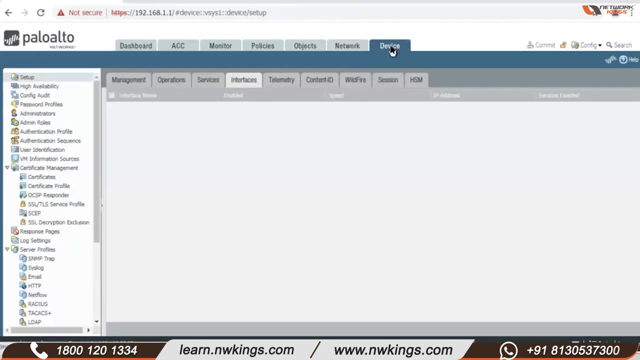 oh, yes, yes, right, we should be able to, because this is the management interface and by default, uh, communication going to the management interface is allowed, right. where do you have that configuration over here under devices? so three things are allowed, right, sir, guys, open up for questions only when i allow you. 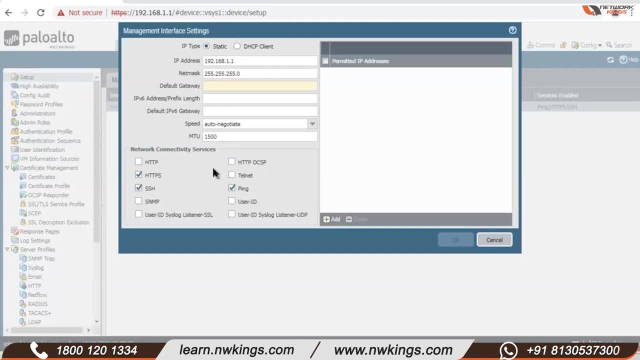 so three things are allowed, right, sir, guys, open up for questions only when i allow you. okay, otherwise we will break the flow and it will more of uh. okay, otherwise we will break the flow and it will more of uh, it will be like my interview. okay, you will be asking random questions, i'll. 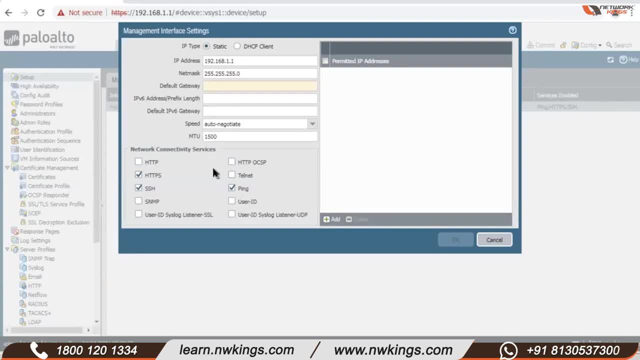 it will be like my interview. okay, you will be asking random questions, i'll keep on answering and keep on answering, and keep on answering, and i may miss out certain topics. yeah, i may miss out certain topics. yeah, i may miss out certain topics. yeah, so, so, so, just just keep a pen paper with you, if you. 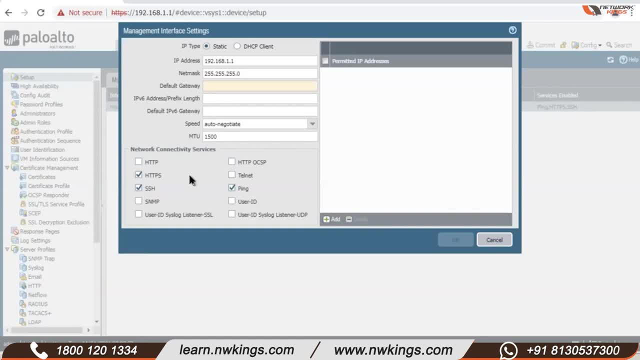 just just keep a pen paper with you. if you just just keep a pen paper with you, if you have doubt- you know have doubt, you know have doubt, you know just write it. and when we open up, for just write it. and when we open up, for just write it, and when we open up for questions, and that time you can ask. 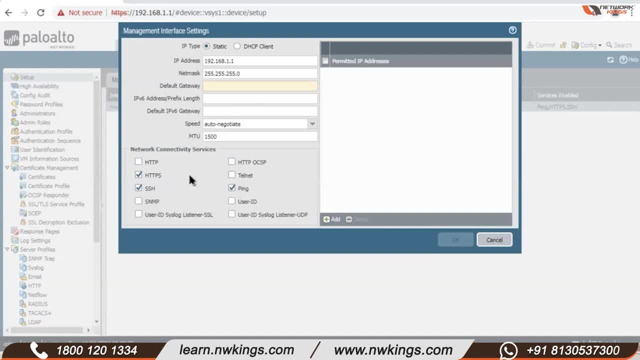 questions, and that time you can ask questions and that time you can ask: yeah, yeah, let's go uh in a planned way. let's go uh in a planned way. let's go uh in a planned way, all right, all right, all right. no hard feelings to anybody not running. 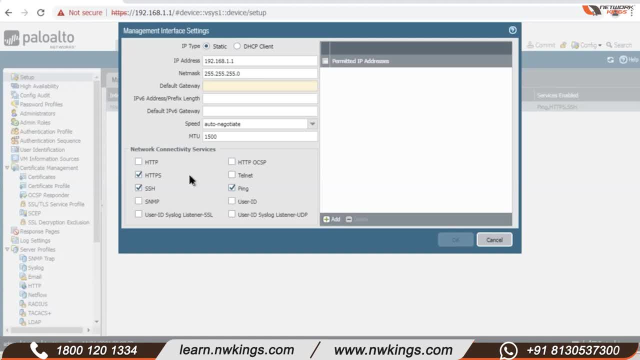 no hard feelings to anybody not running, no hard feelings to anybody not running away from questions, but let's do it away from questions. but let's do it away from questions, but let's do it systematically. all right, so here is the configuration. all right, so here is the configuration. 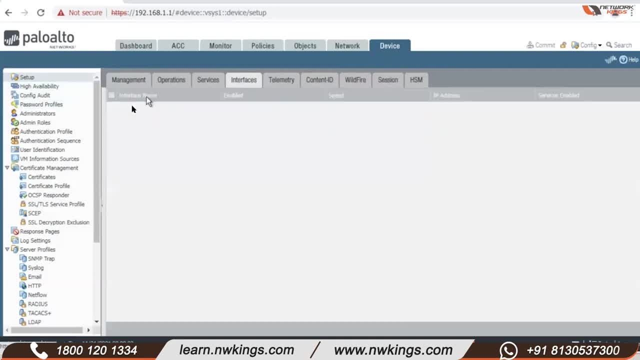 all right. so here is the configuration: under under under devices, you go to setup and under setup devices, you go to setup and under setup devices, you go to setup and under setup, you have management, you have management, you have management, and this is where the configuration is, and this is where the configuration is. 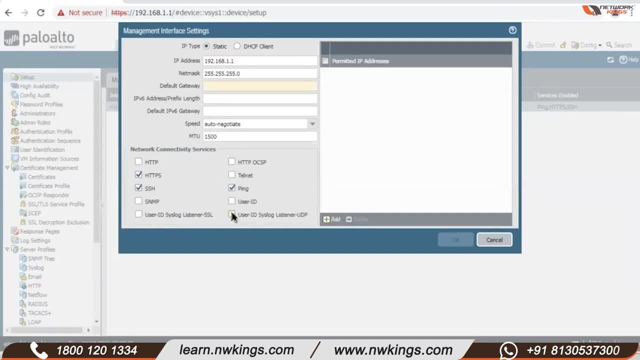 and this is where the configuration is. these are the allowed protocols. these are the allowed protocols. these are the allowed protocols. right, right, right. if i select telnet, telnet will also be. if i select telnet, telnet will also be. if i select telnet, telnet will also be allowed on the management. 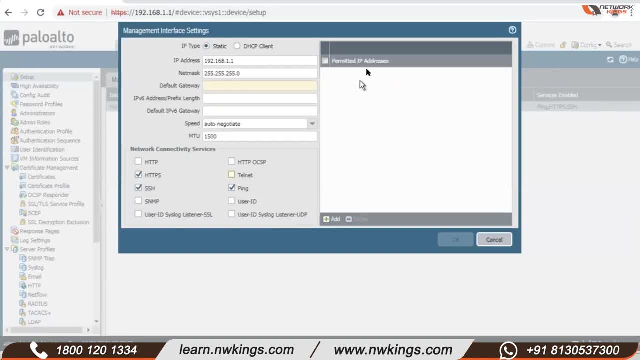 allowed on the management, allowed on the management, and this is where we can add permitted and this is where we can add permitted and this is where we can add permitted. ip addresses: right now, there is nothing ip addresses right now. there is nothing ip addresses right now. there is nothing right, so that means everybody. 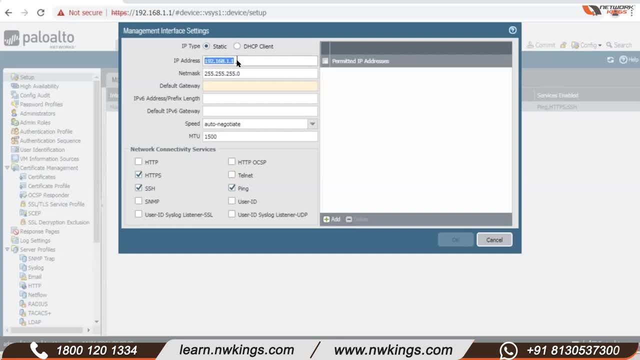 right, so that means everybody. right, so that means everybody who has access to 190 to 168 1.1, or who has access to 190 to 168 1.1, or who has access to 190 to 168 1.1, or anybody who can reach to 1.1 will be. 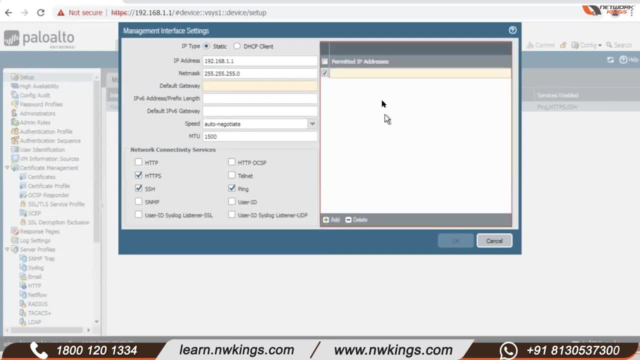 anybody who can reach to 1.1 will be. anybody who can reach to 1.1 will be allowed to communicate with the firewall, allowed to communicate with the firewall. allowed to communicate with the firewall. if i were to limit that, let's say i type: 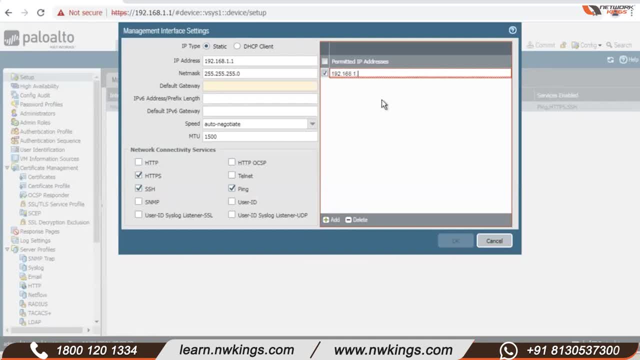 if i were to limit that? let's say i type. if i were to limit that, let's say i type in 190 to 168: 1.10. in 190 to 168: 1.10. in 190 to 168: 1.10. that is what our ip address is. 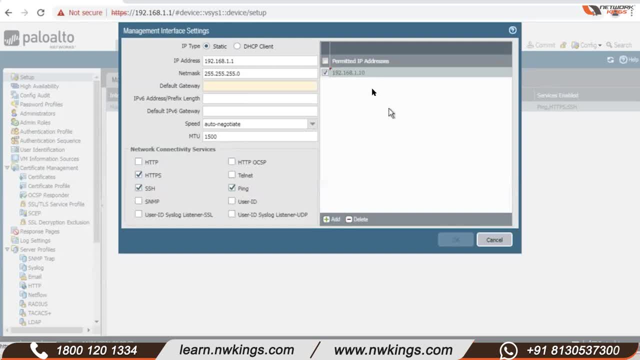 that is what our ip address is. that is what our ip address is, and anywhere in the gui, and anywhere in the gui, and anywhere in the gui. one more thing, let me tell you anywhere. one more thing. let me tell you anywhere. one more thing. let me tell you anywhere in the gui. when you mention the ip, 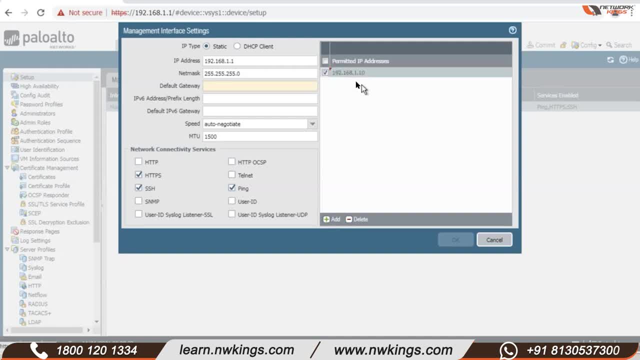 in the gui, when you mention the ip in the gui, when you mention the ip address without defining the mask like address, without defining the mask like address, without defining the mask, like. here i did 1.10, i did not mention the. here i did 1.10, i did not mention the. 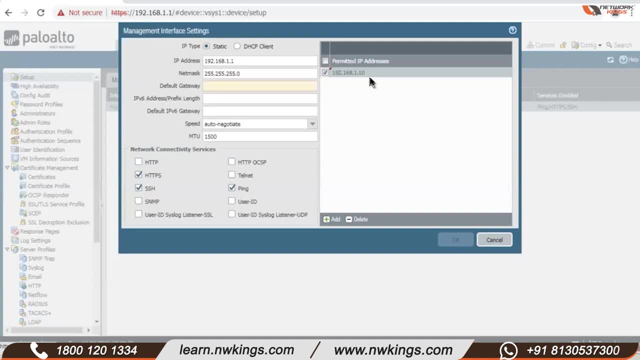 here i did 1.10. i did not mention the mask mask mask. so by default, the firewall treats it as so. by default, the firewall treats it as so. by default, the firewall treats it as slash 32. okay, okay, okay. so keep that in mind and 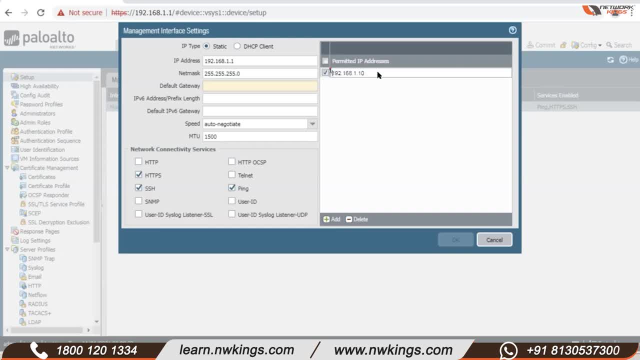 and and are we making any mistake? look like here. it won't mask. no, still, you see the ok button is not. no, still, you see the ok button is not. no, still, you see the ok button is not highlighted, highlighted, highlighted it. does that okay, just ignore it. does that okay, just ignore. 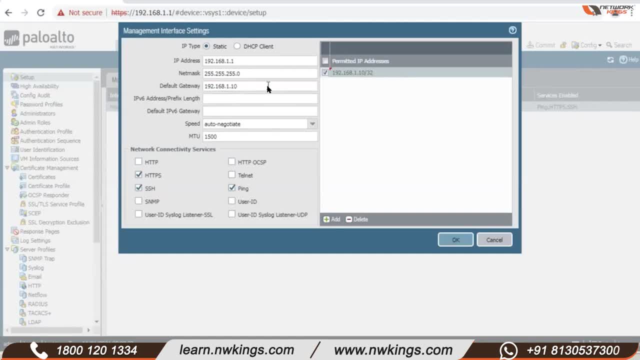 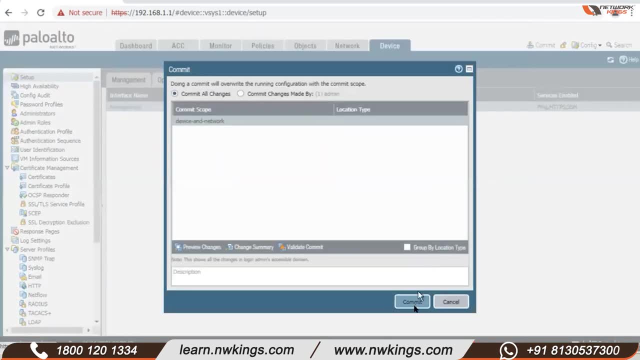 it does that. okay, just ignore. and 1.10 is just our gateway, the directly. and 1.10 is just our gateway, the directly- and 1.10 is just our gateway, the directly connected pc. only now i will have to change this. now i will have to change this. 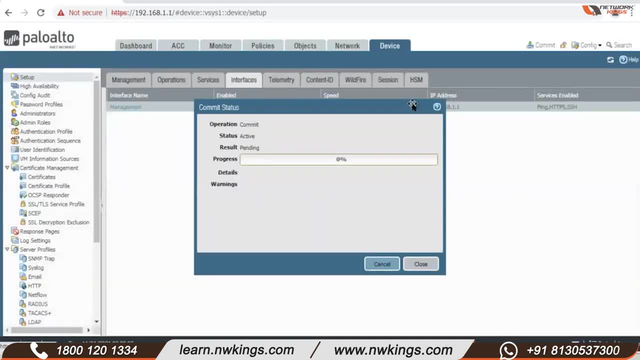 now. i will have to change this. make sure i commit to apply the changes. make sure i commit to apply the changes. make sure i commit to apply the changes now. what did we do now? what did we do now? what did we do? we are allowing. we are allowing. 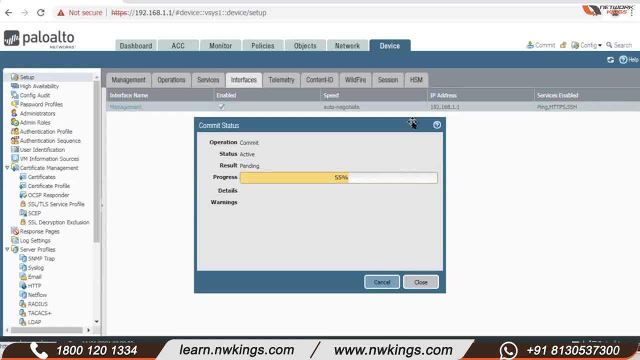 we are allowing only and only 1.10 to communicate with only and only 1.10 to communicate with only and only 1.10 to communicate with the firewall management ip. why does it show one dot okay? why does it show one dot okay? 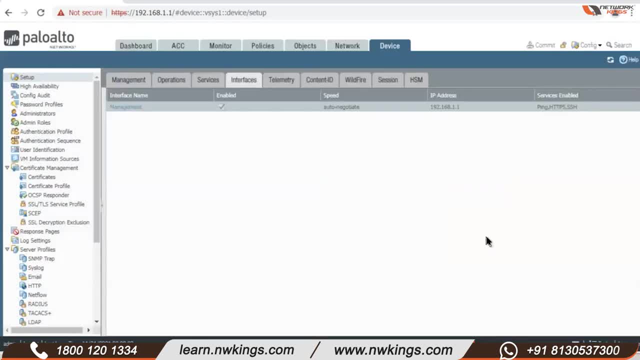 why does it show one dot: okay, service enabled. okay, permitted ip service enabled. okay, permitted ip service enabled. okay, permitted ip address is good. 1.10 address is good. 1.10 address is good 1.10. now let's say, if i change the, 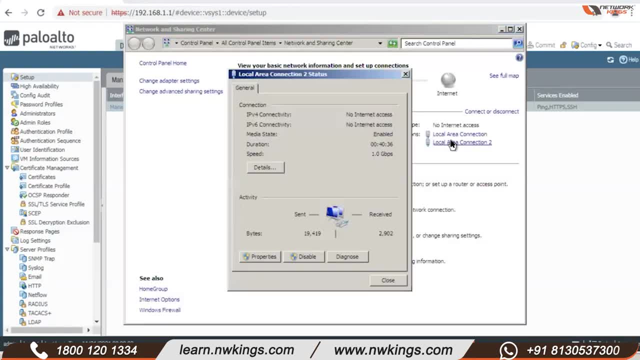 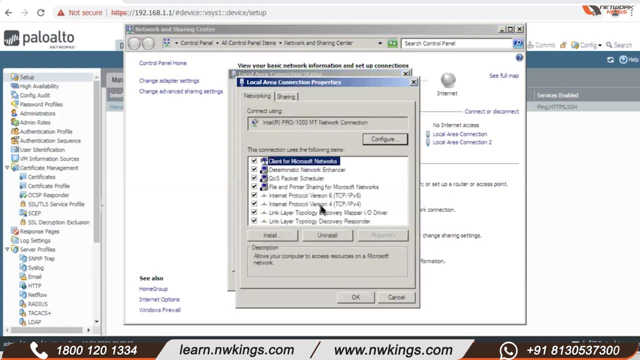 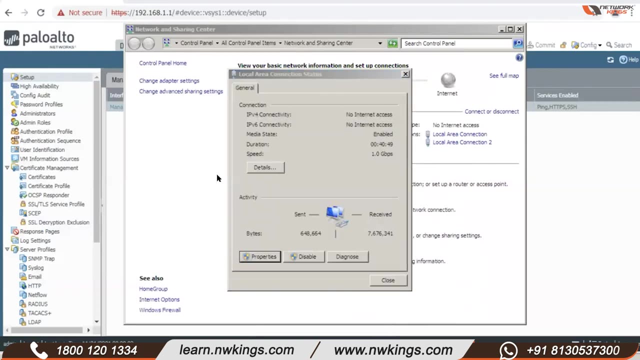 ip address. now. let's say: if i change the ip address now, let's say: if i change the ip address, right, let's say i make it 11. right, let's say i make it 11. right, let's say i make it 11 and i try to bring the firewall. will i? 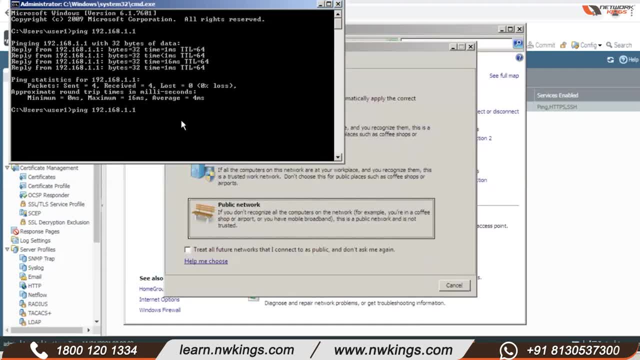 and i try to bring the firewall. will i- and i try to bring the firewall, will i be able to bring, be able to bring, be able to bring? no, no, no, no, no, no. anybody who wants to say yes, anybody who wants to say yes, anybody who wants to say yes, where i fixed that? 32? 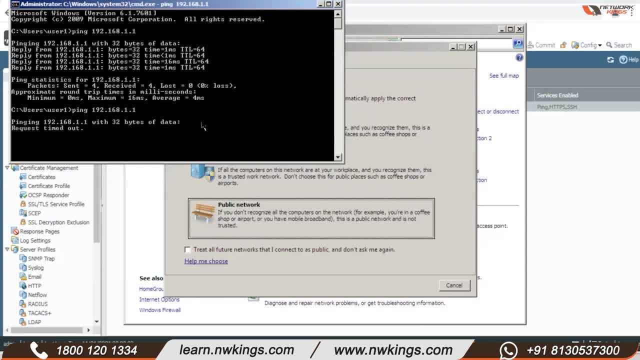 where i fixed that 32, where i fixed that 32 right, because we have right, because we have right, because we have restricted the communication, the restricted the communication, the restricted the communication. the firewall is expecting communication. firewall is expecting communication. firewall is expecting communication only from 1.10. 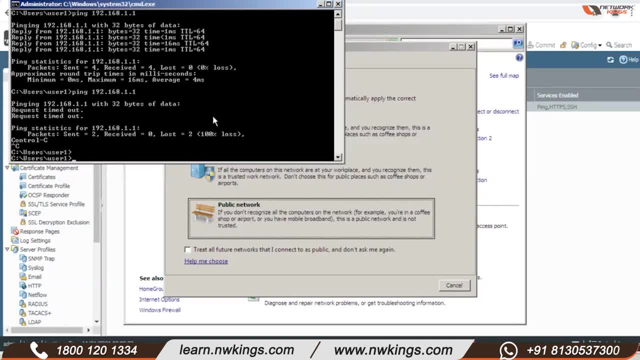 only from 1.10. only from 1.10 right now. this is for only the management right now. this is for only the management right now. this is for only the management ip address. this is for the communication ip address. this is for the communication ip address. this is for the communication which is going on: the management. 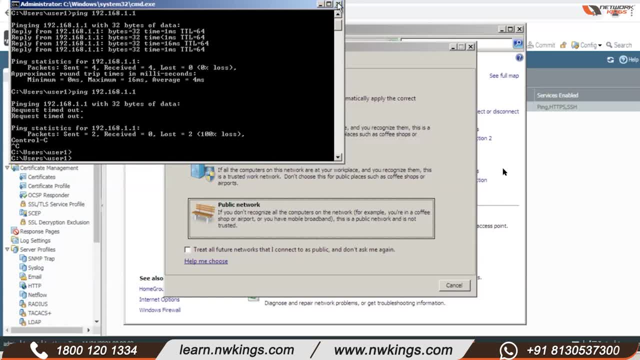 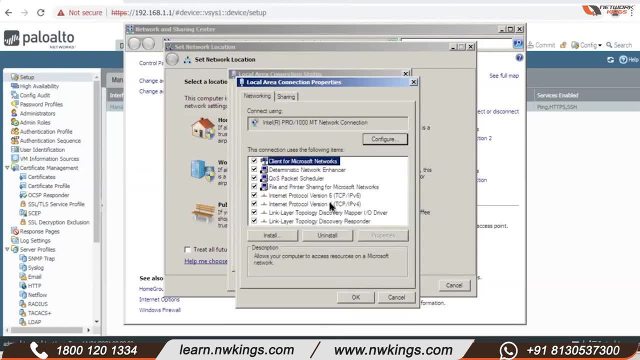 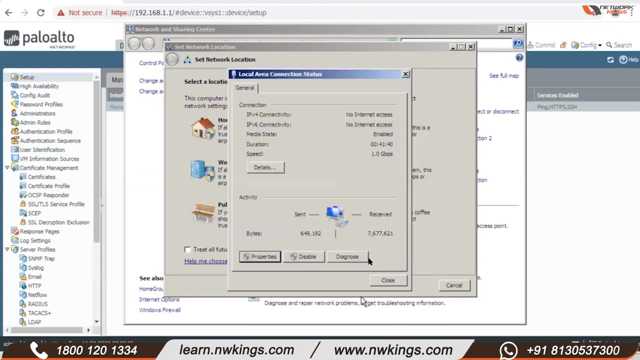 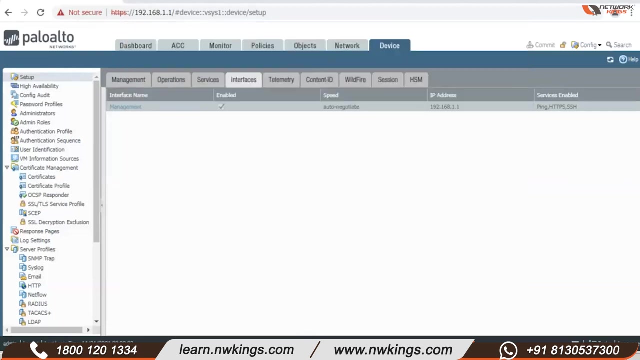 which is going on the management, which is going on the management interface. let's change this back to. let's change this back to. let's change this back to 10 so that we can 10, so that we can 10, so that we can do further things. 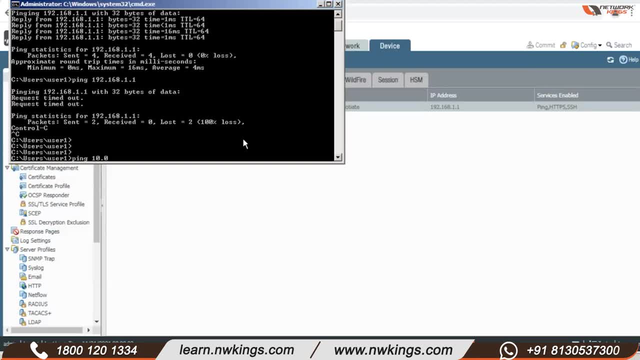 now the firewall has one more ip. now the firewall has one more ip. now the firewall has one more ip address. that is 10.0.0.1 address. that is 10.0.0.1 address. that is 10.0.0.1. if i try to ping that, will i be able to? 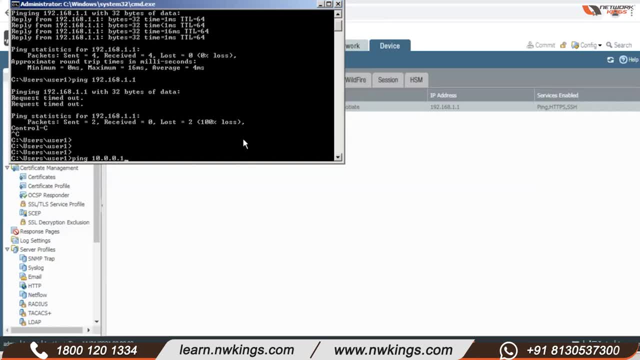 if i try to ping that, will i be able to. if i try to ping that, will i be able to do, do, do, no, no. why is that no, no? why is that no, no? why is that? because by the fall it's blocked that, because by the fall it's blocked that. 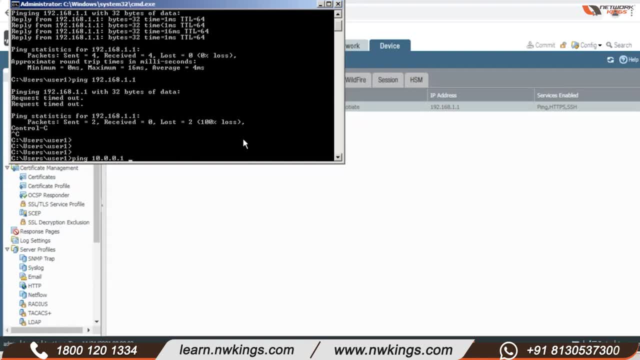 because by the fall it's blocked. that traffic, traffic, traffic- yeah, it blocks that traffic because we- yeah, it blocks that traffic because we- yeah, it blocks that traffic because we are trying to communicate to the, are trying to communicate to the are trying to communicate to the firewall. 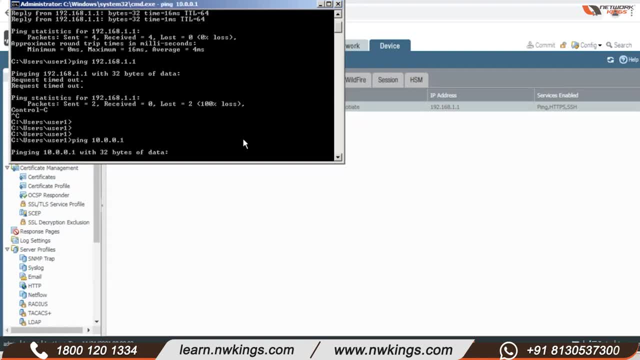 firewall, firewall on the data interface- right, but isn't this uh, right, but isn't this uh, right, but isn't this, uh? isn't this not cool when you have to do? isn't this not cool when you have to do? isn't this not cool when you have to do some troubleshooting and when you are? 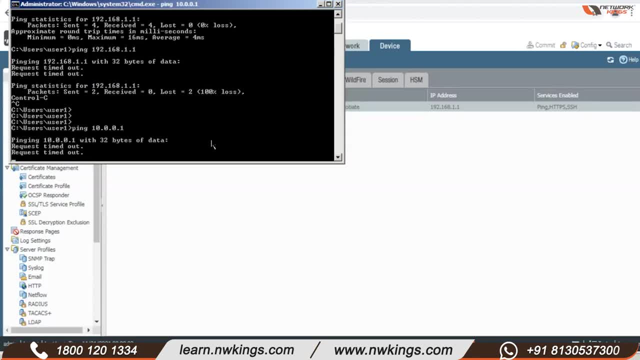 some troubleshooting and when you are some troubleshooting and when you are implementing the firewall and you want implementing the firewall and you want implementing the firewall and you want to ensure if the firewall as a gateway, to ensure if the firewall as a gateway, to ensure if the firewall as a gateway is reachable or not reachable- right. 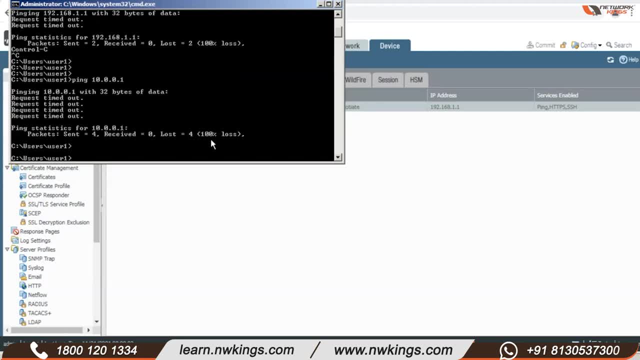 is reachable or not reachable. right is reachable or not reachable right. so at least uh ping should be allowed. so at least uh ping should be allowed. so at least uh ping should be allowed, right, don't you guys think so? don't you guys think so? no, well, i don't, for security reason. uh, we don't you. we don't allow paying on the firewall, i think. 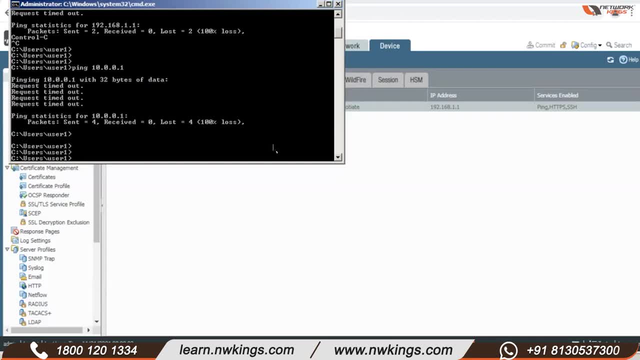 uh in my environment so we can't paint the uh uh. okay, but you have a. you have a bunch of uh workloads, uh connected to the firewall and the firewall is called gateway and uh they complain about. you know, we are not able to communicate so you're not able to test whether the gateway 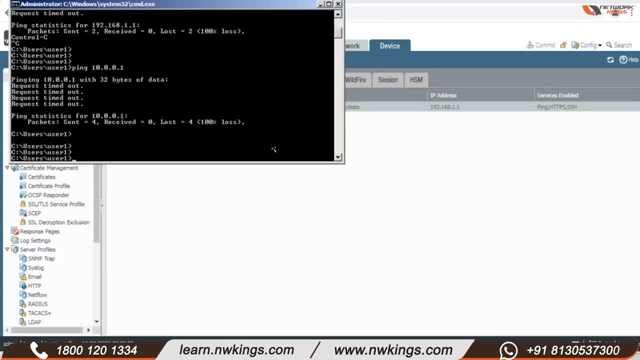 is reachable or no. so how do you check that, right? maybe, i don't know. yeah, so when you're blocking icmp, traced out would also not work, right? oh, okay, so in in such cases, uh, you know, you may be forced, uh, maybe not by choice, but by scenarios- you may have to allow icmp on data interfaces of the 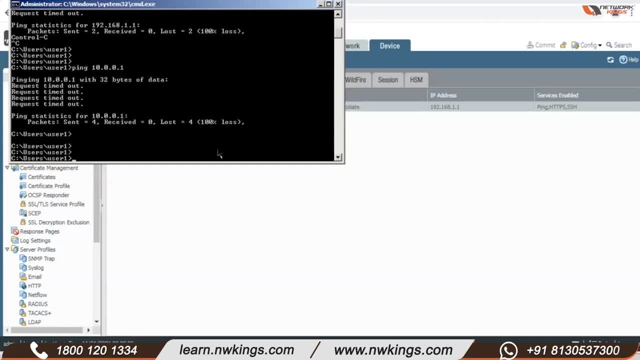 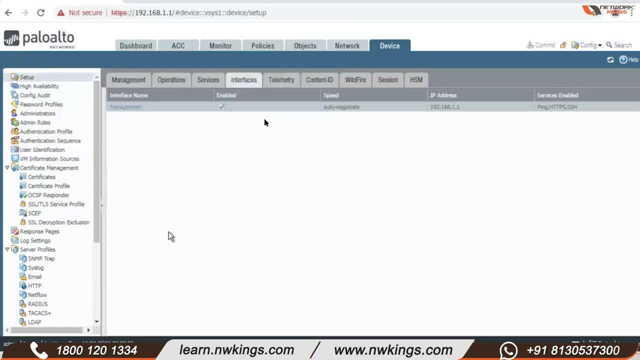 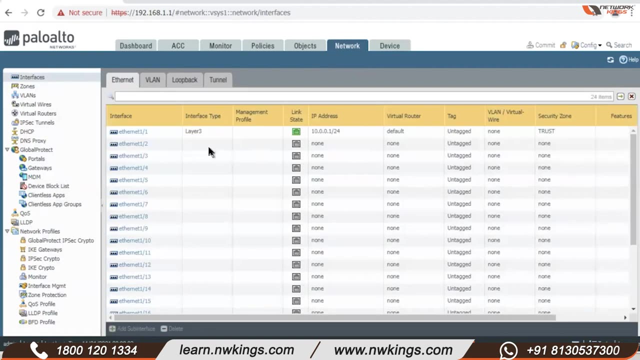 firewall. you may not allow ping through the firewall, but you may allow ping to the firewall, right? so two different things that can be done here under networks, we are still not making policies, guys, we are still talking to the firewall only, right. so under interfaces, there is an option here. 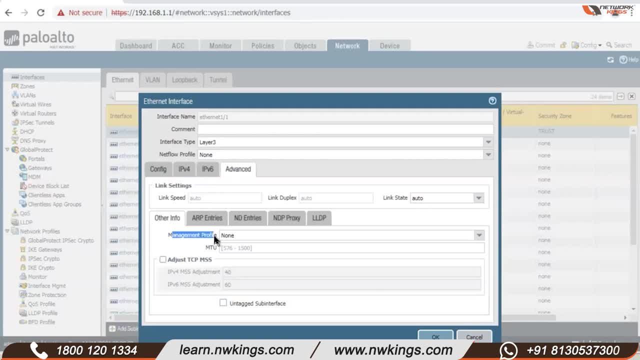 go to advanced and you have management profile, right. this management profile talks about, uh, what all protocols or what all communication can happen to the data interfaces. right, either you can go here in the drop down and create a new management profile, or it's all the way down here. 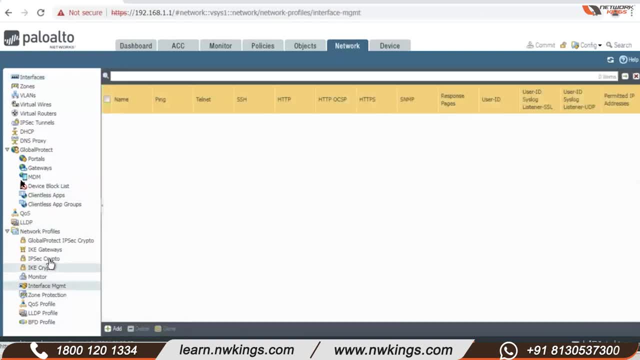 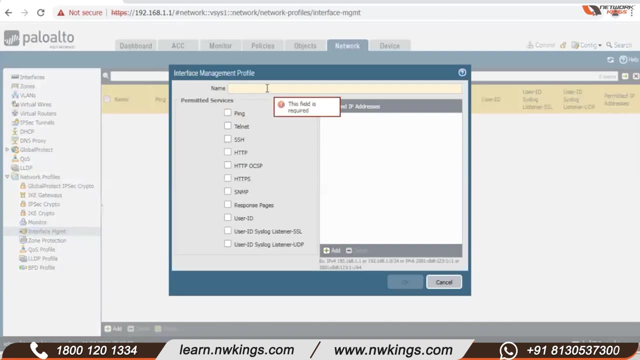 in interface management and by default, when you run it for the first time, it will appear something like this: right, so you go under network profile and it is interface management that we can add. so let's add an interface management profile. let's just allow ping on this. i select ping. 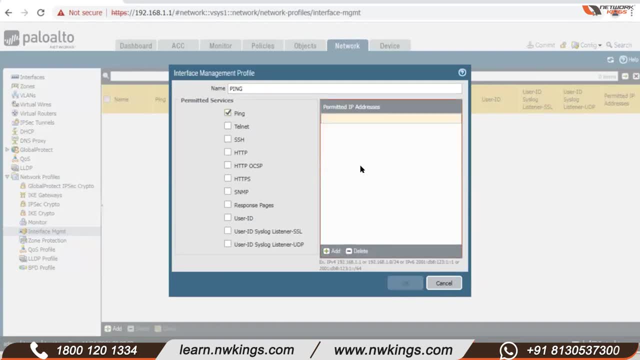 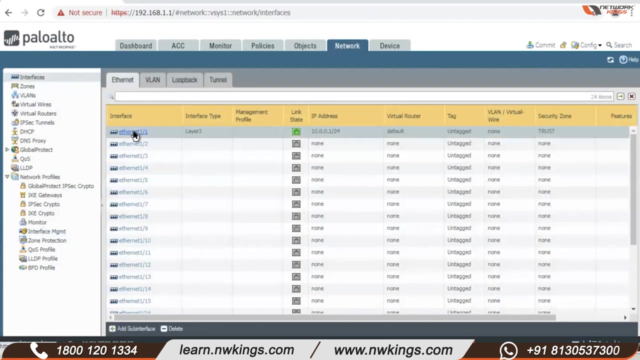 and i can select a permitted ip address, for example 190 to 168, one dot. not sorry, we're using the data interface right, the 10.00, right 10, 10, 32. so this is the only pc i want to allow right, not commit. yet you go to interface and make sure the profile is added on the interface. 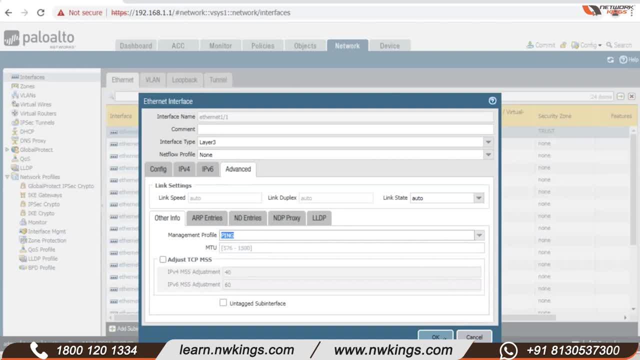 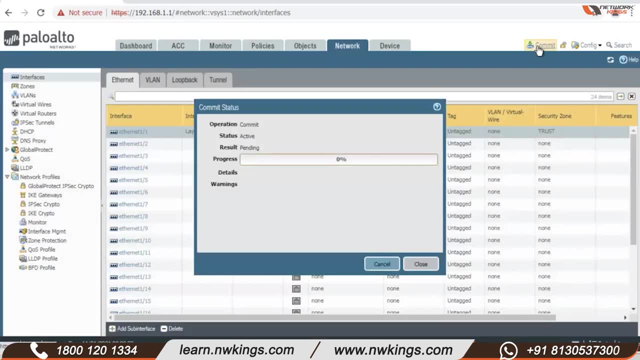 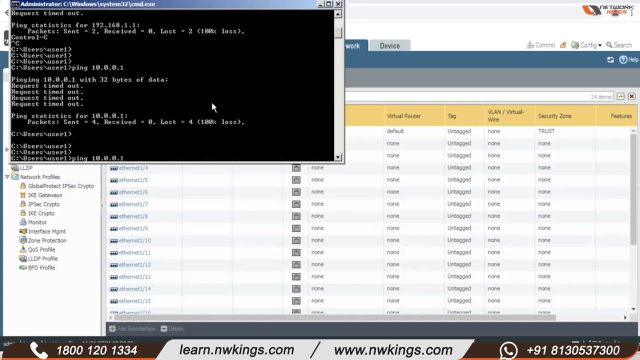 go to the drop down and select your profile we just created, do ok and do commit, okay, so. So i'm just going to create a new one, all right, so we're good to go to test again. i try to ping it again. will i be able to ping? 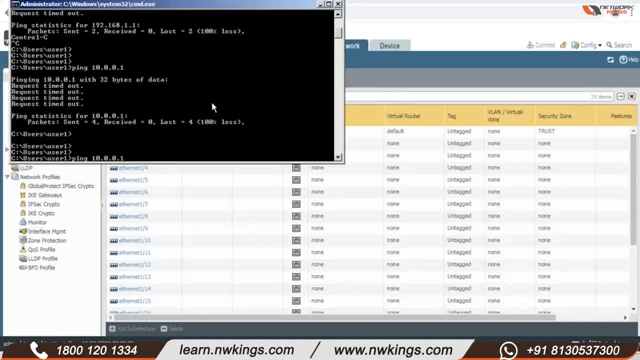 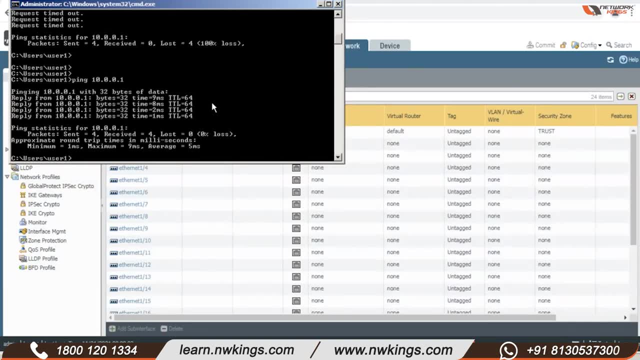 yes, you should, you should, you should be able to, right, and we are able to now. so we are still not allowing ping to go through the firewall and get the dashboard to work right now. so that's what we're, you know, bombarding the entire network we are just allowing to communicate with. 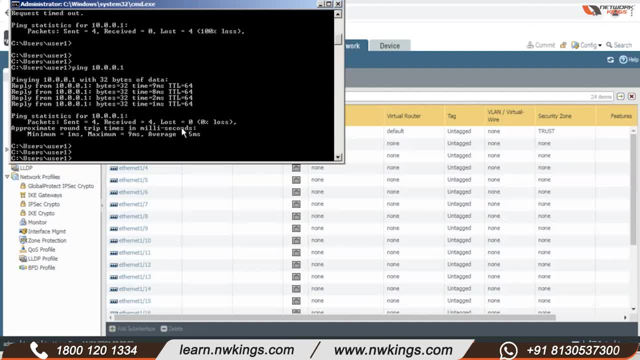 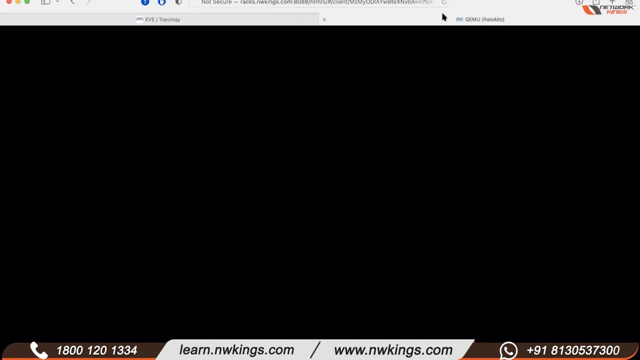 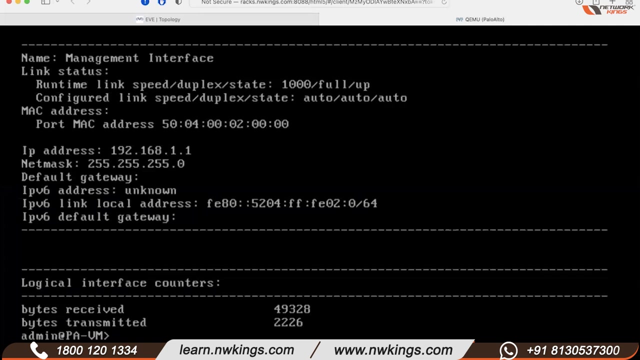 the firewall. so that's one cool way to allow ICMP and and what else I have to show you. yeah, one more thing: the firewall communicating with others. and let's go to the firewall console being 192, 168, 1.10. that is our management PC. 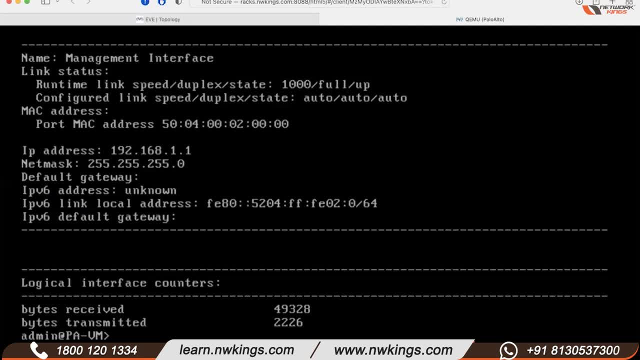 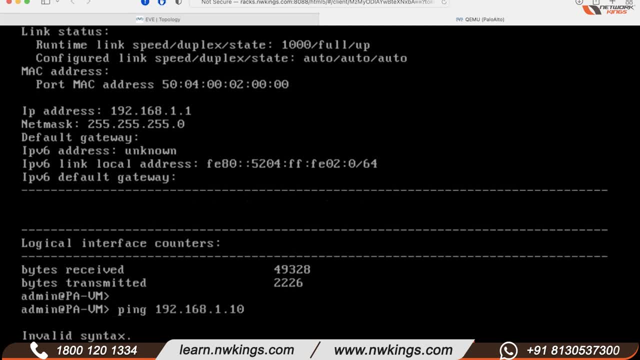 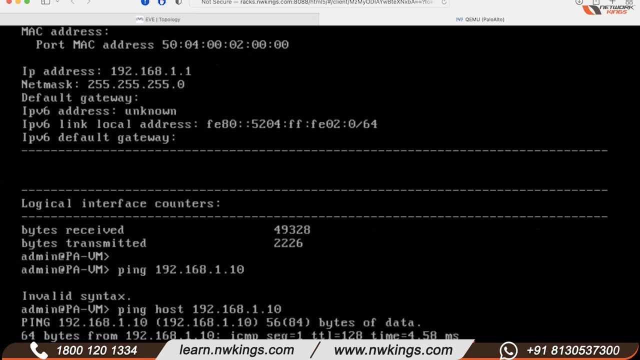 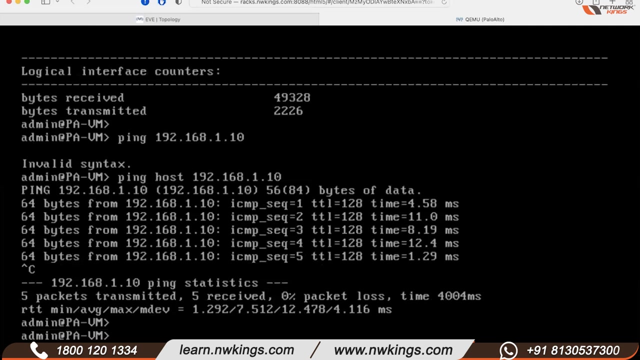 right. should I be able to ping yes, yes, yes, we are. we are in the management network. okay, the the syntax, so we are able to. that's cool, but if I try to ping 10 dot 0, dot 0, dot 10, sorry, we need to add host. 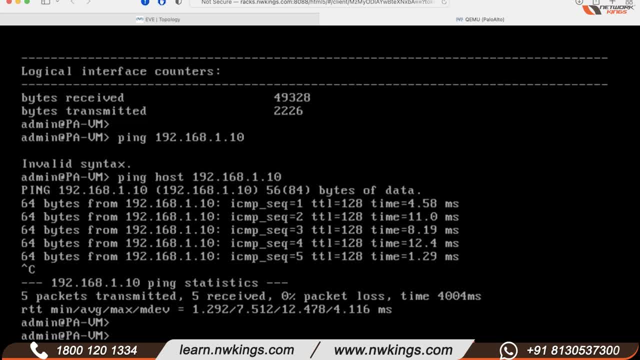 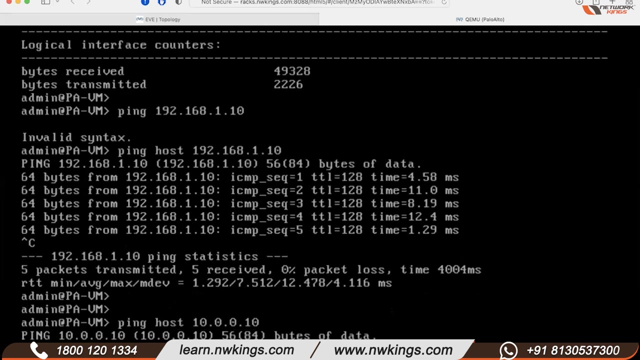 again. will I be able to ping? yes, because no? no, I don't think so, because you only permitted that 10 on that interface. yeah, but we are talking to the same IP which we permitted. yes, we permitted. this is: yeah, OK, we should be able to reach right. yeah, yeah, OK. Surprise, we are not able. 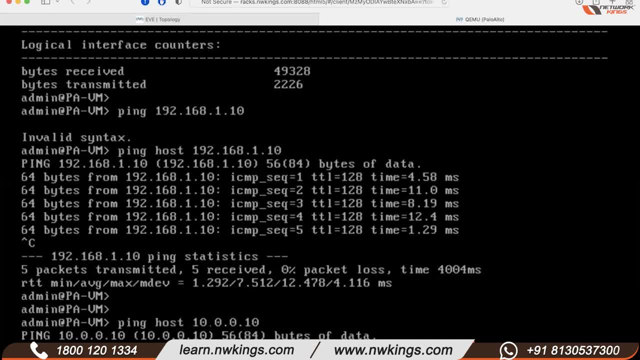 to communicate? right, because now the firewall is initiating the communication. oh right, because we are now it's sitting in Yosh protein on Parallel. this is a viral portal, right? so we are now trying to ping from the firewall what we are doing, isça, and dispatch writing the next kind ofviw. 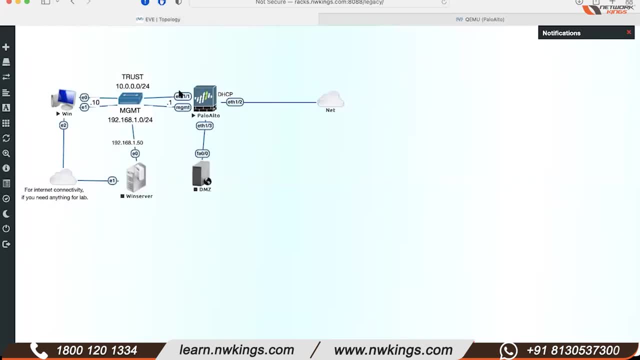 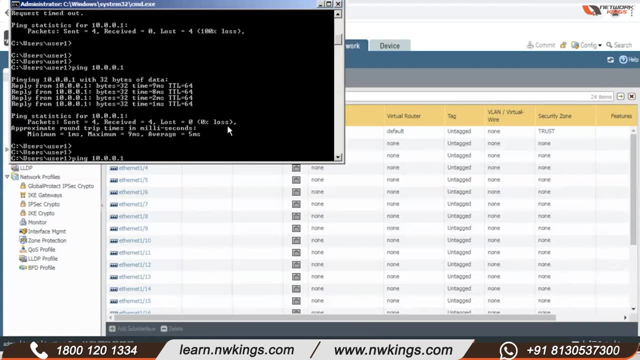 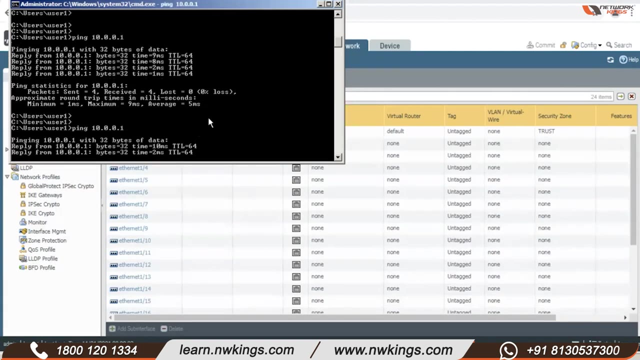 from the firewall to the PC, right, And we are not able to communicate. I see what you're saying, That's right. Earlier we have tried from PC to firewall. Hold on, guys, Hold on. But I am able to communicate this way. 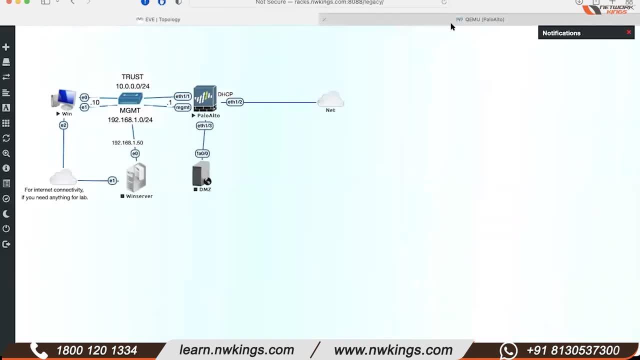 The PC can talk to the firewall, but the firewall is not able to talk to the PC. Why is that? Because, as I mentioned earlier, whenever the firewall is communicating, it tries to communicate with its best port, that is, the management port. 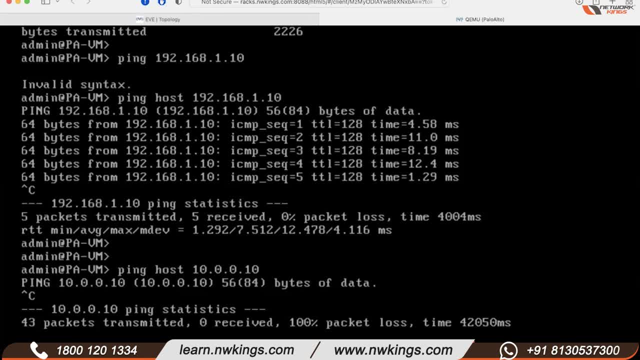 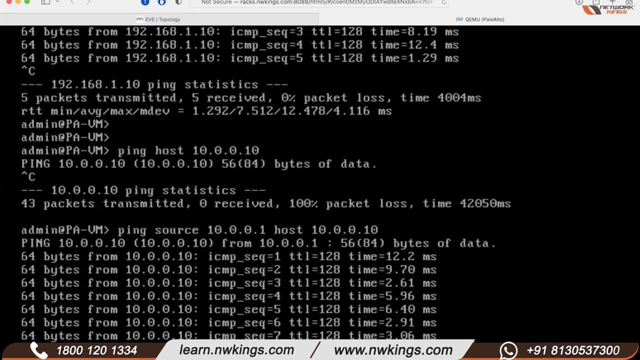 Right. So if you want to actually talk to Ethernet 1 slash 1, you will have to define the source. It will be something like this: Right, And now the firewall will try to communicate via Ethernet 1 slash 1.. So the firewall can communicate. 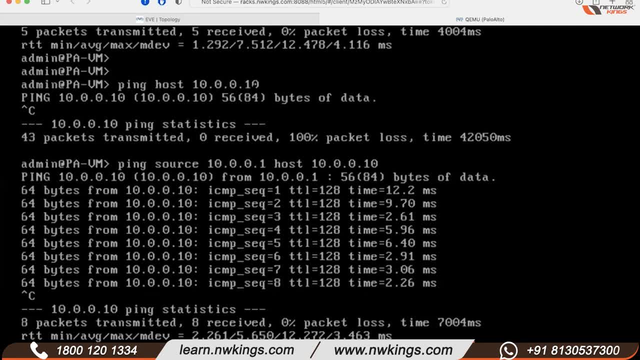 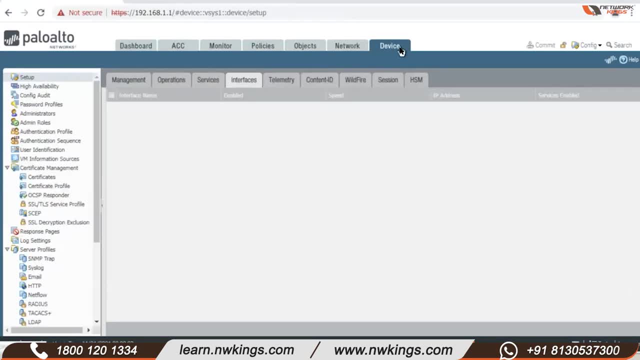 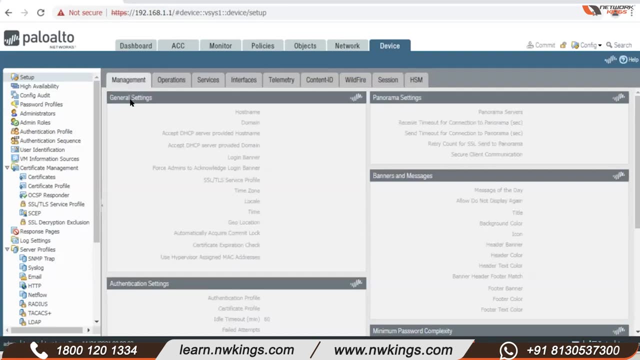 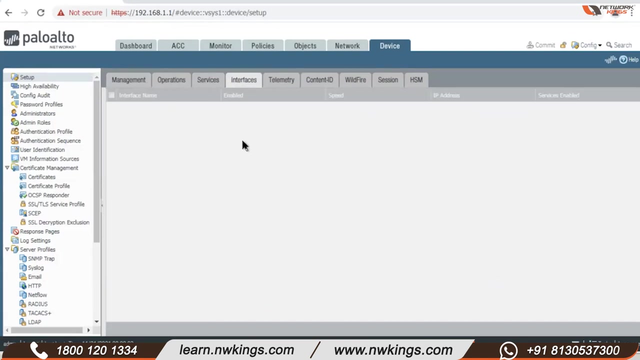 Obviously, we were testing with the wrong command. We can change this behavior. by the way, We can change this behavior here under devices Again, because this is a system-specific thing. We come under management. Hold on Services. Yeah, Under services. you have option. 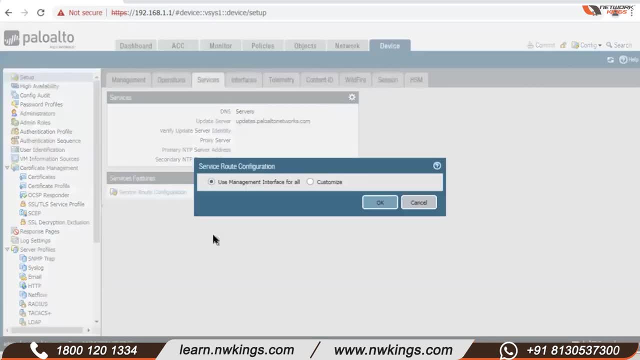 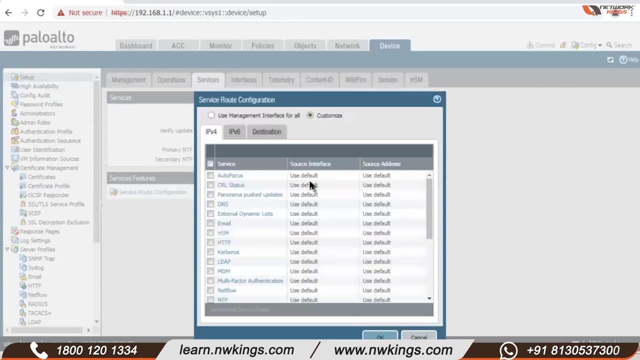 of service route configuration. By default, it is set to use management interface for all. Okay, Any service the firewall is trying to communicate on, it should be using management interface. We can customize this, of course. Right, And these are the different services that the 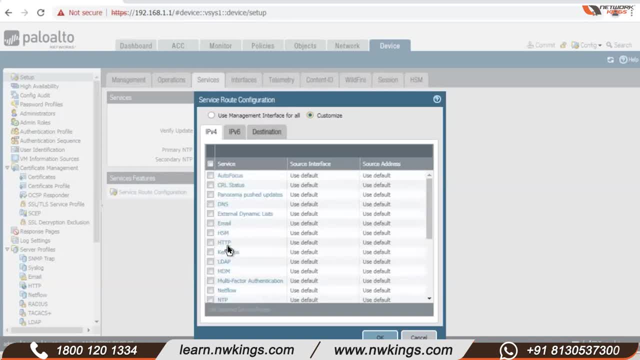 firewall can communicate on. So on this, you can select your desired service and you can change it from default. From default to whatever interface you want to choose, For example DNS Right. At times the management network does not have. 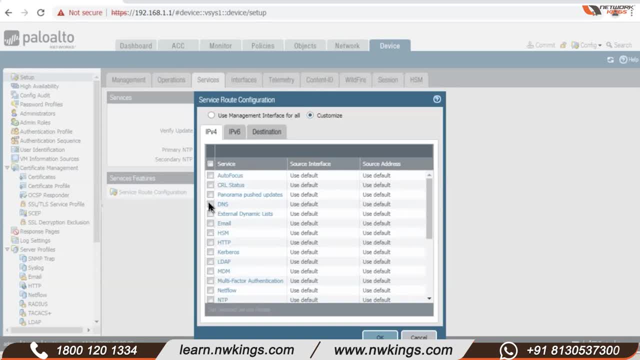 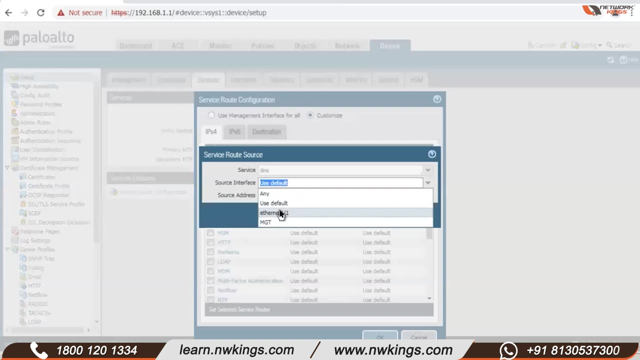 internet connectivity. So the firewall will keep sending DNS queries out through the management and they will keep on failing. So you would select this Simply and you change the interface. So when we configure one, slash two here it will be available. 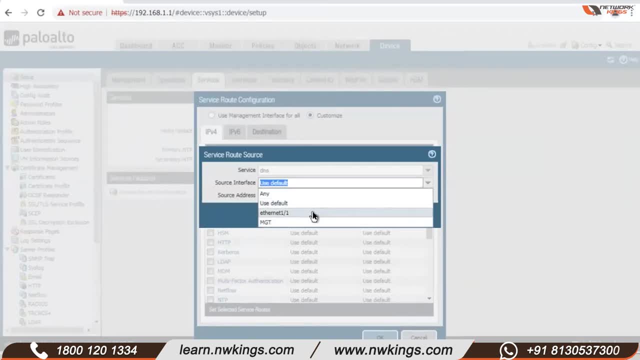 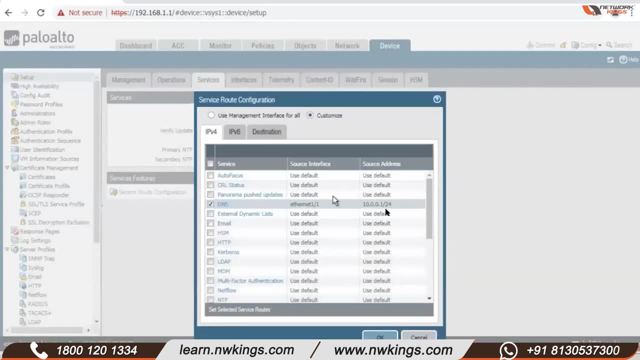 Okay, For now, let's just for the sake of it. you can select this interface and the source IP address will be displayed and it will look something like this. So this is again. you may or may not require this in your. 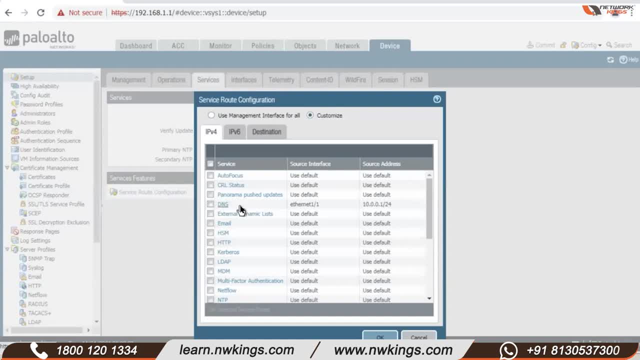 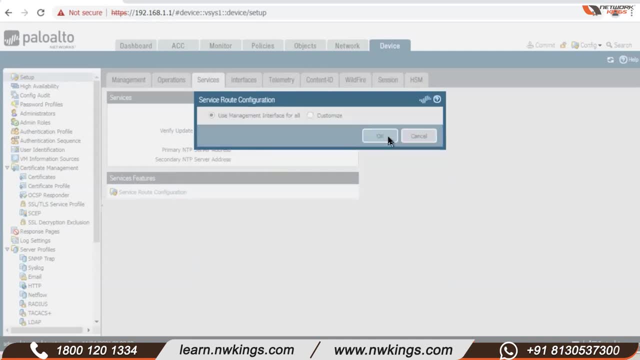 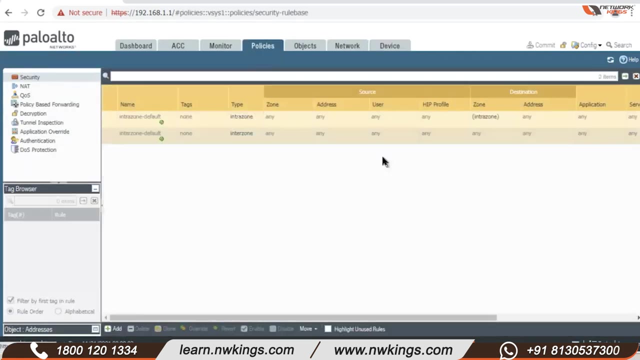 production network. It all depends how it is set up and you know on the requirement. So this is the option. This is where you will find it Cool. Any questions now? That's pretty neat. This option is good. 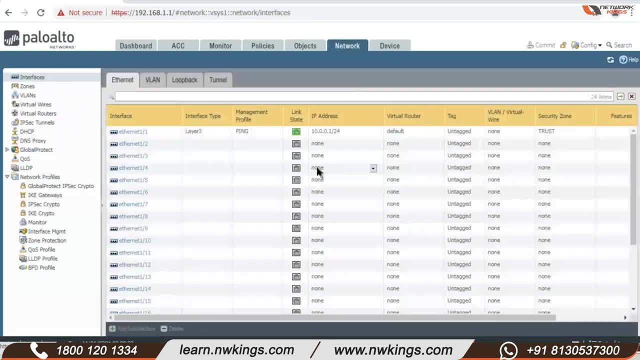 One. we can do it. Sorry, come again please. Yes, This option is nice. Yeah, it is a very useful option, but you know, use this very carefully, So production also will be used, right, Right. 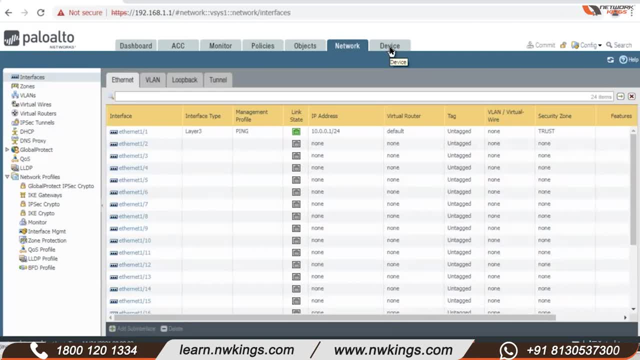 In production also it is used, So I have seen the TACACS also there. So suppose you want to communicate with TACACS server. Right, If the TACACS server is not sitting in the management network, then you will have to change that. 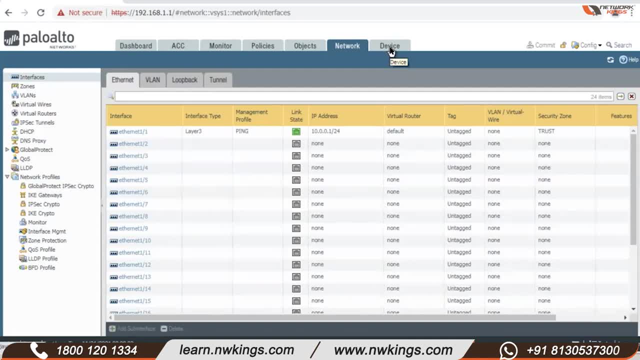 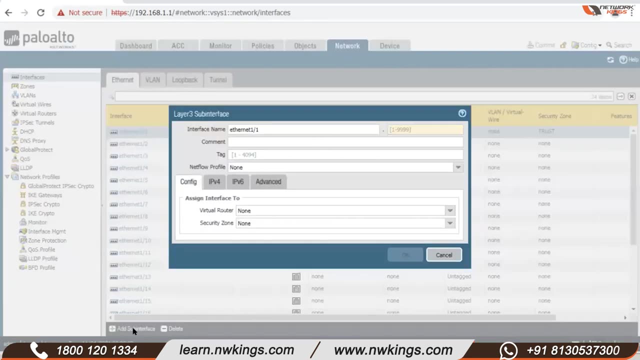 Yes, For example, it's sitting in some DMZ VLAN- then you'll have to. you know you're forced to change it. Any option, Nice option, Right. And again, if you have to add the sub-interface, simply select the interface and click here. 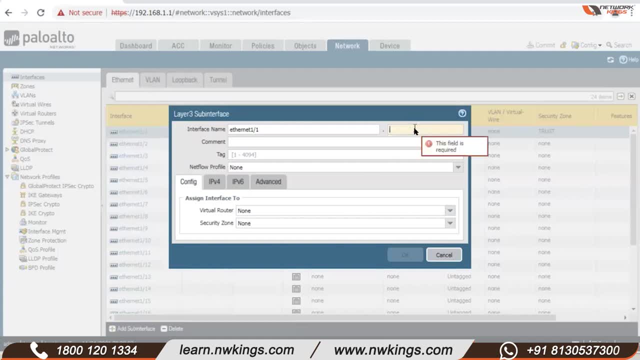 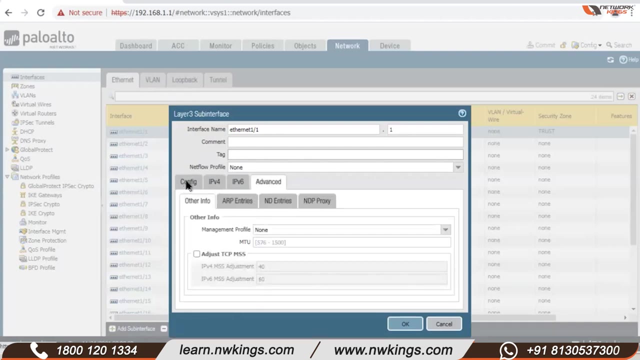 in the bottom left corner, add sub-interface, give it a number right And of course, you cannot be in a different type. Whatever is there on this will be selected. IPv4 and all that. it's a normal thing now, Yeah. 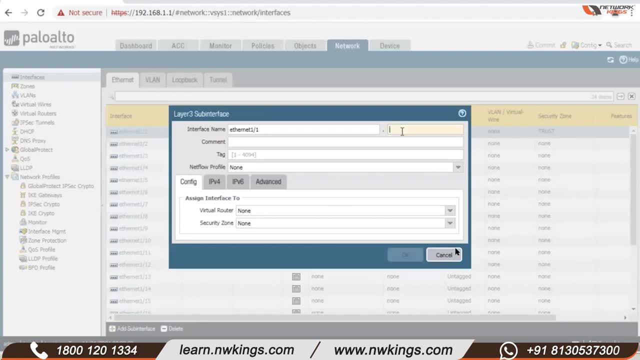 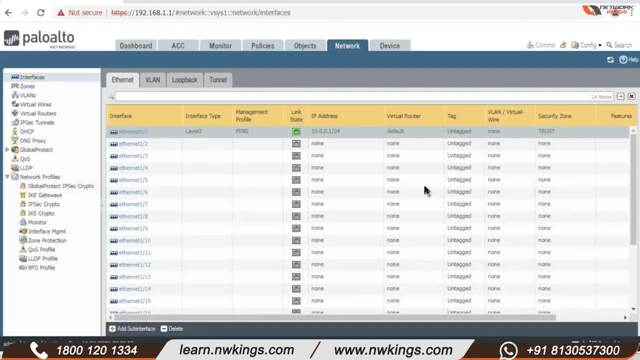 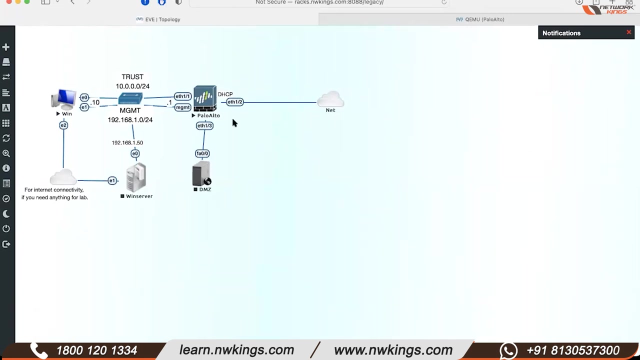 You can configure it the same way you configured Ethernet 1 slash 1.. So suppose, sir, if there is another system we will connect with that firewall. Will he be able to ping Another system where, On some other interface? Let's say, let's say this DMZ trying to talk to 1 slash 3.. 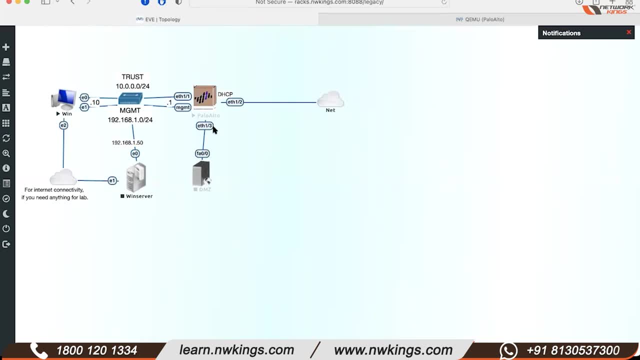 Is that what you're saying? No, no, no. I like some 1 slash 2 interface or 1 slash 5 interface. Let's consider: this is the other. Let's consider this is the other system. right, 1 slash 3.. 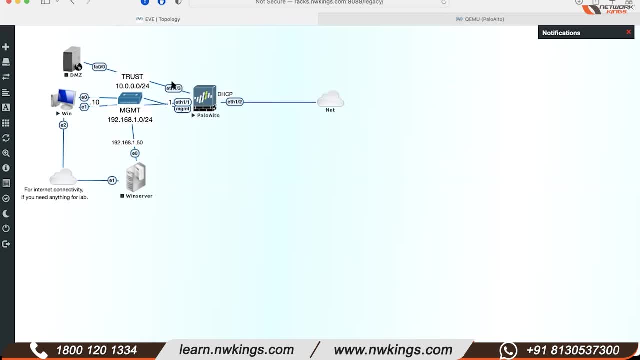 This is what you're saying, right? So if 1 slash 3 has the interface management profile connected with it and it has the network allowed to communicate with it, Yes, it will be able to communicate, Else it won't be able to. 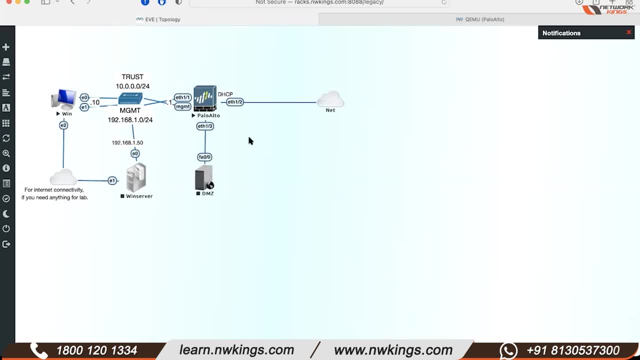 No from the firewall and to the system. Yeah, Again from the firewall. Also, if you choose the source, properly, it will go out through this source, Else it will keep using management, unless you have modified the service out. Okay, 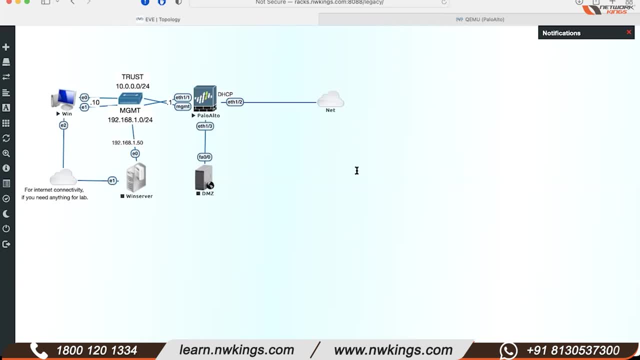 Okay, Somebody has put up a question. Sure, Is there CCNA knowledge required to do firewall codes. CCNA knowledge to nowadays is required to make Maggie also. Okay, It's, it's that basic. So even if you are not into networking, 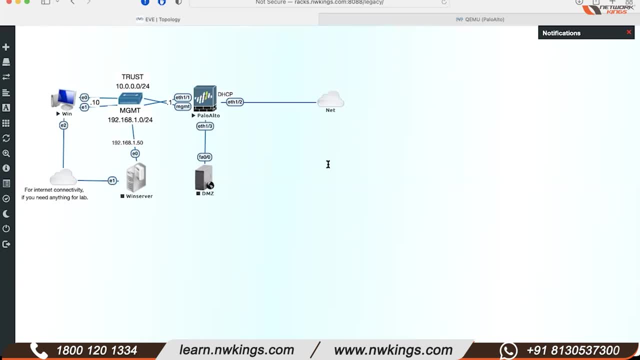 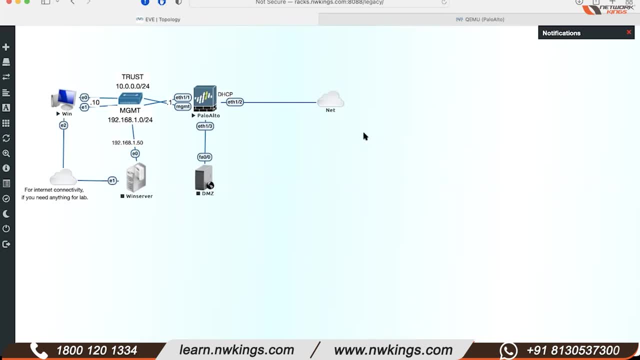 Yeah, Yeah, Yeah, You're aware of basic things of networking. It helps achieve your tasks. I mean, I see developers struggling where the IP address and netmask and gateways and all those things. So if they know those, the job will be easier for them. 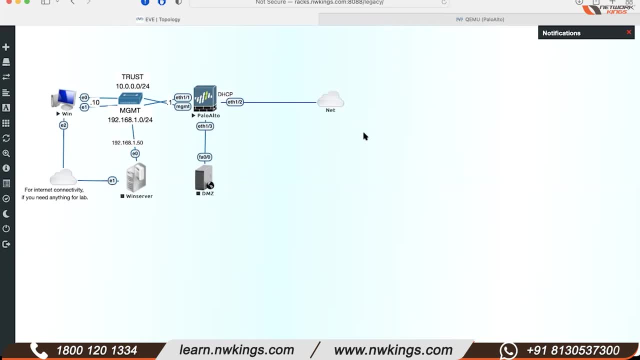 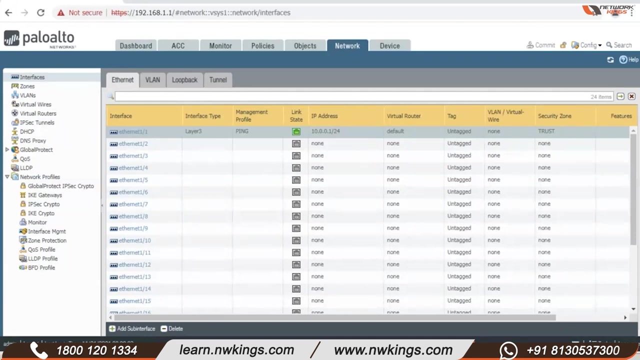 Right. So yeah, it is kind of important things to know. ranado Sabah Sab gloves DOU there, But I don't know everything. There's maybe, but I don't know, a Himalaya side of this. Exactly, if the active firewall cannot process the traffic, the secondary will take. 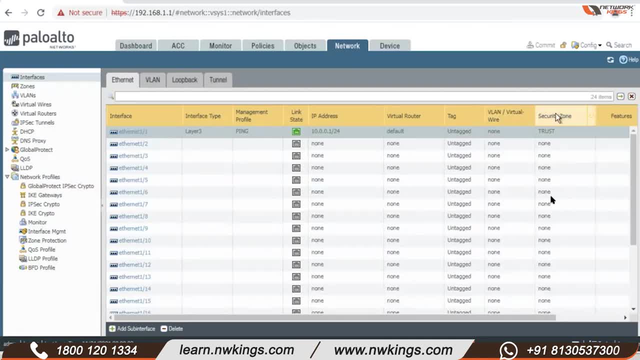 this. this is for only one million. yeah, all millions, yeah, uh, all the device traffic is for all the villains and every traffic is uh shifted on secondary firewall, right, sir? yes, yes, not single. yes, can you ship the traffic in single wheel and on a secondary? is this possible? yes, we. 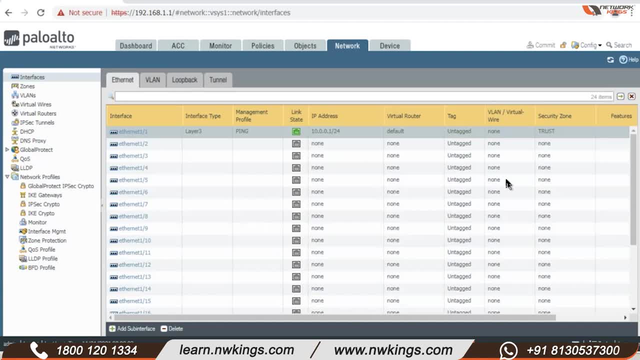 can do that. there are two ways you can do: h- a active, active and active standby. okay, okay, okay, and so half of the v-lens can be active on one firewall. the other half of the vlan can be active on the other firewall. both firewalls will. 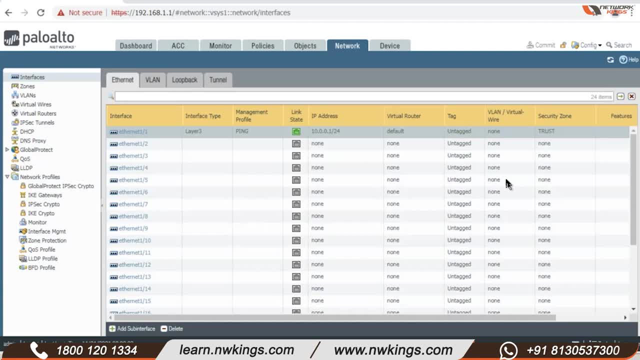 be active and backup of each other. okay. okay means this is required. uh, both are the firewall activity, those only. we can like that to back up for each other, like that, vice versa. yes, yes, but that is not a recommendation, recommended way to do h a right in productions. we don't really follow that. it's always active. 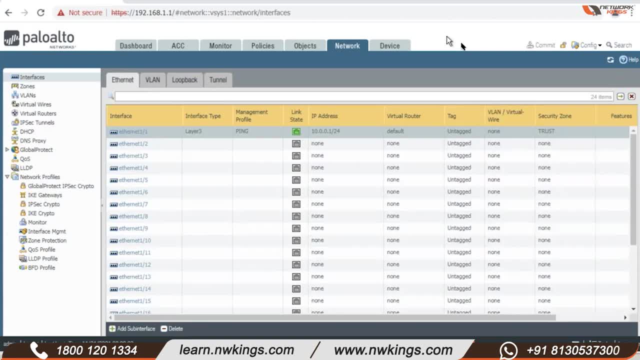 standby. why, sir? why behind the reason, any that is the vendor uh recommendation, and it is easier and more stable, it is easier to troubleshoot and it is easier to implement, easier to manage right easier to make changes on it. so that's why, because this question is asked by intel, that's why i think this is a tricky question only. 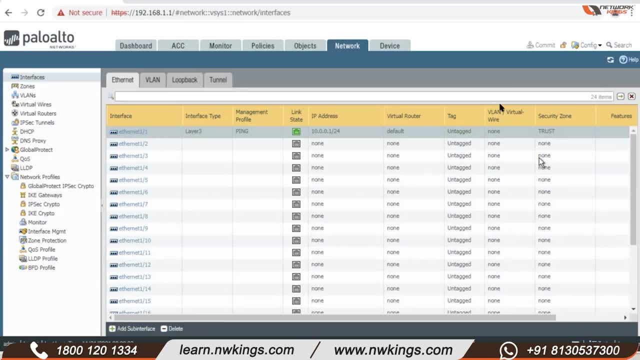 yeah, they just try to judge your uh understanding. how well do you understand a particular topic? yes, that's why i'm also asking the uh question. if you've got your answer right, did you understand or you will understand more when we fine. can you ask a revancho mute please? 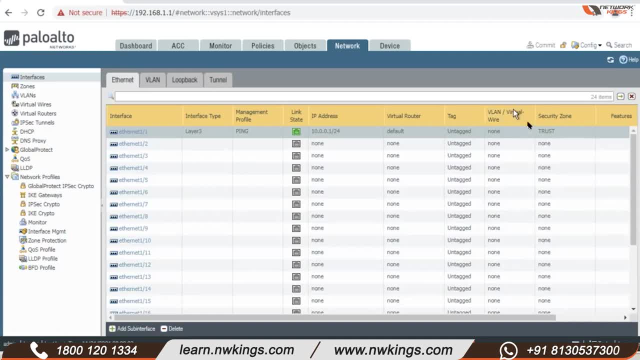 he is who is talking and he somebody is sitting right beside to him, it seems. yeah, okay, anyway, the question is done. so, yeah, guys, try to uh sit a little isolated right, it is good for everybody, i don't mind. but when you guys the recordings, you'll be like uh. 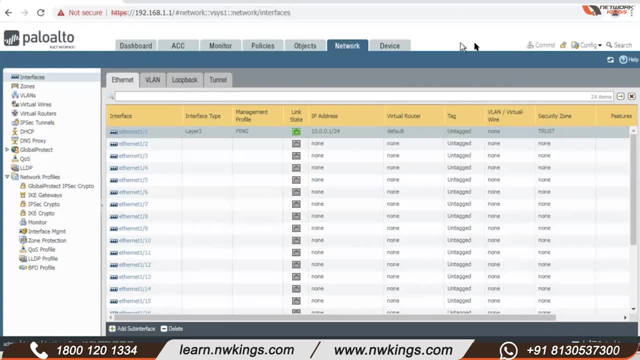 you will be the one watching the recordings. i'm okay with everything right and let's be mindful about others. yeah, okay, any more questions guys. sir, which lab you have just ran it? can we also do it? yeah, you can also do it. uh, i don't think you guys have the credentials yet to to the portal. 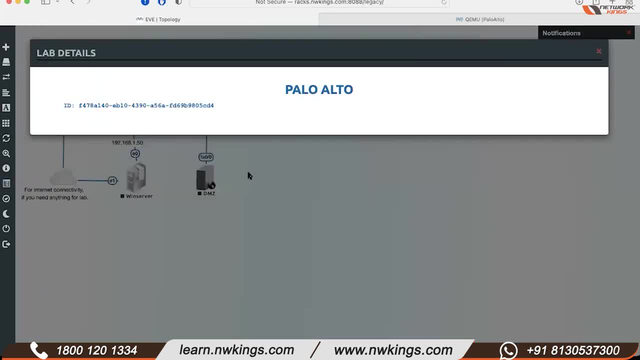 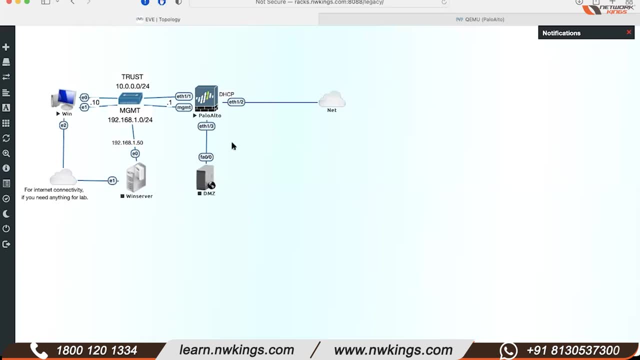 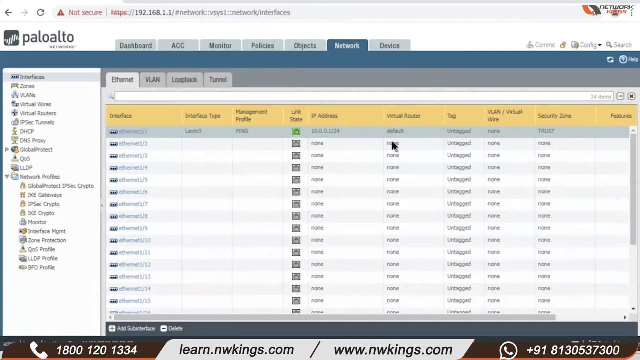 but the the name is. the name is just private. i think Palo Alto, it's lab 1 or lab 2 and the name just is Palo Alto. name of the lab is Palo Alto no 1, 2 or anything. hi, sir, I just have a one question. actually I'm pretty much fresh. 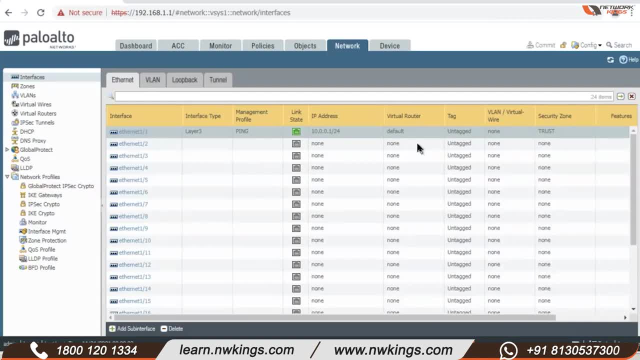 to this firewall. so usually this firewall, it's done on GUI only, sir. yes, because you know these. unless you have to do bulk configuration, GUI is the preferred way. okay, fine, right, let's say this is how it looks, right like not. yeah, this is how it looks. yes, even the panorama. 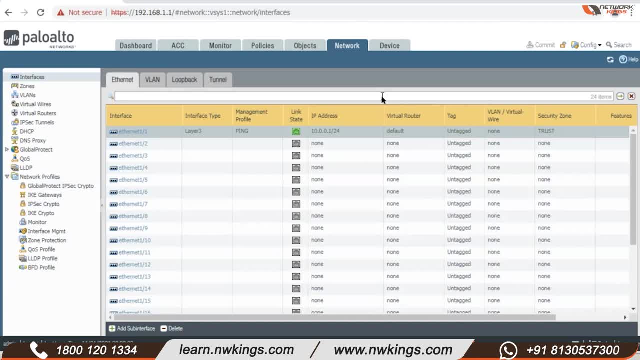 would look same. okay, sir, thank you that you have in the. in the next session we will talk about panorama and we will do further things and we'll we'll talk about security policies and all that. sure, sir, thanks. so there's one one question. yeah, only we can able to ping management IP. 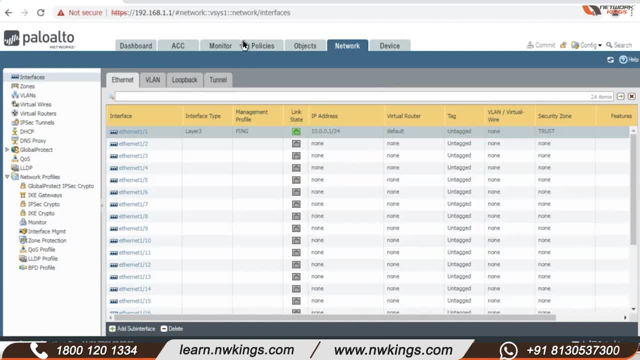 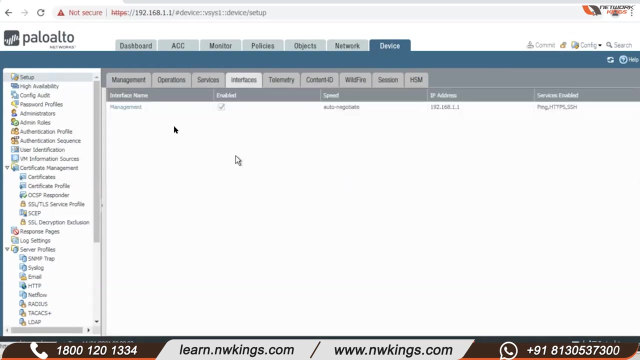 only right. yes, if it is the other other IPs- Ethernet one, zero slash one- it gives me a gateway, means we can't able to pay. if it is a gateway, no, no, no, I think you, you, you missed it. you go to this device gateway. we gave the gateway IP because it was giving some error. 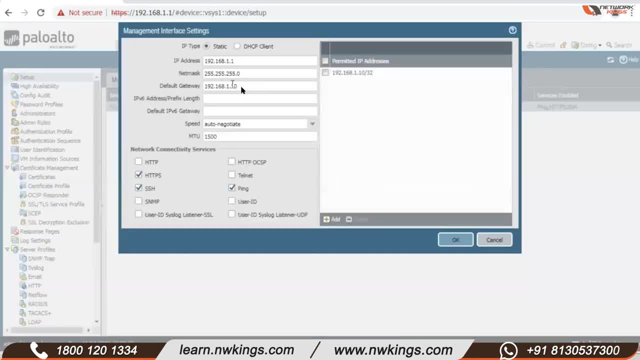 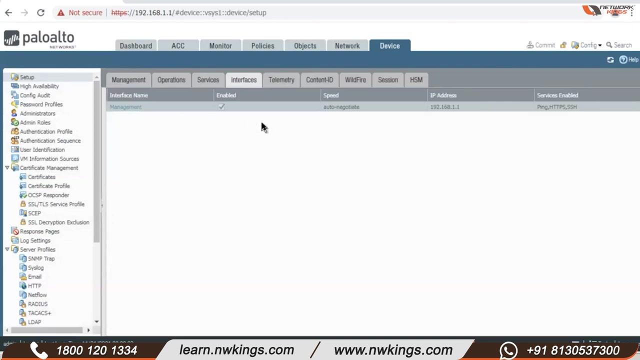 right, it was not letting us. it wanted us to fill the blank. okay, that's why we gave it, but the actual configuration is here. that's where we permitted 1.10. okay, okay, okay, yeah, okay, okay, yeah, Yeah, yeah, we have been doing some just simple things. we'll get Ether net 1, slash 2 running. 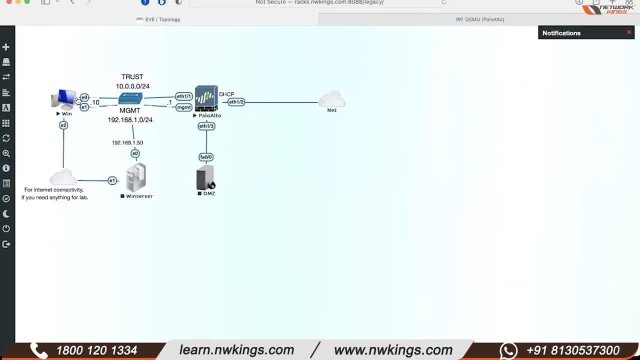 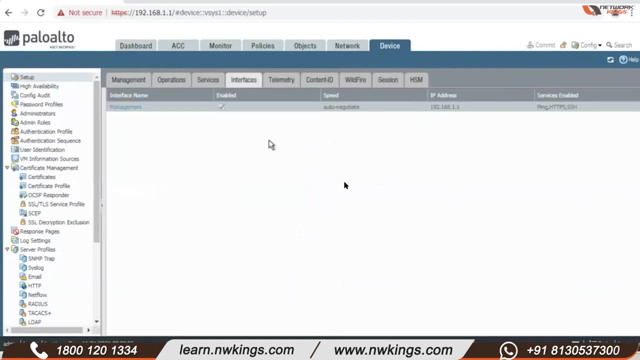 and we will see. how do we get this guy talk to internet via the firewall when I'm going to post this video? when am I going to what? okay, poster the video. they should be on the portal by tomorrow. Thank You, Hey, Kenny. how are you? Hello, my name is Kenny. how are you? 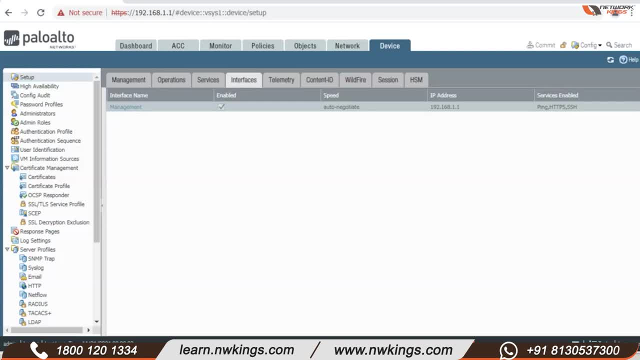 fine, how are you? yeah, i'm fine. kenny is back. kenny is back. yes, kenny is back from after checkpoint. now, kenny is back. yeah, i'm back. hasta la vista, sir. i have one, one small question. uh, parallel to it could be a checkpoint, it's. 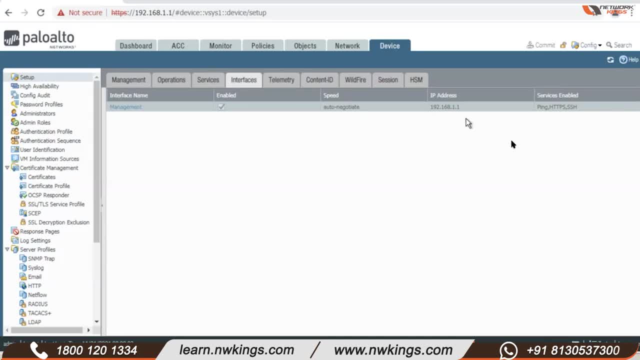 which is a more scope? um, that's a that's a creepy question. both of the fireworks- okay the proof- are good. uh, they both have their uh, their share of market captured right when you, when you're working for uh clients in middle east and all, and that's all checkpoint right when you talk about us, europe and that area, that's all, palo alto. 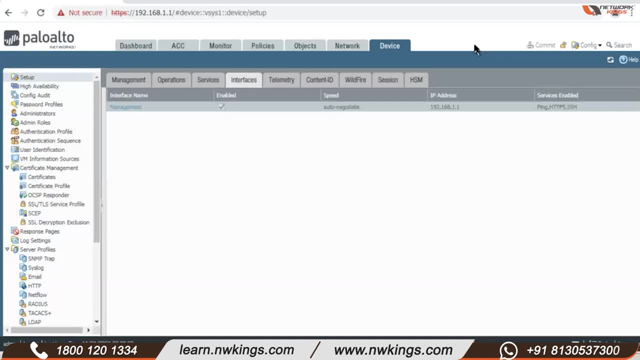 and in india? in india, it's cyber room. what do you need cyber room? yeah, those things. okay, because a 48 is a good firewall. it's a, you know, one of the best uh software clubbed with one of the worst hardware. okay, thank you. so suitcase, like uh, we'll be receiving the like uh. uh uh web details. like uh website. 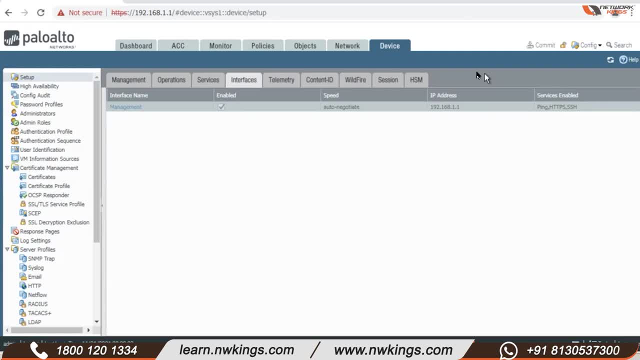 details, along with credential, to get that video, or how will this? yes, uh, within the week, uh, within this week, you'll be getting all of the information on your email. you'll get the access to the lab. you'll get access to the, to the video portal where you can watch the videos after the glass is done. 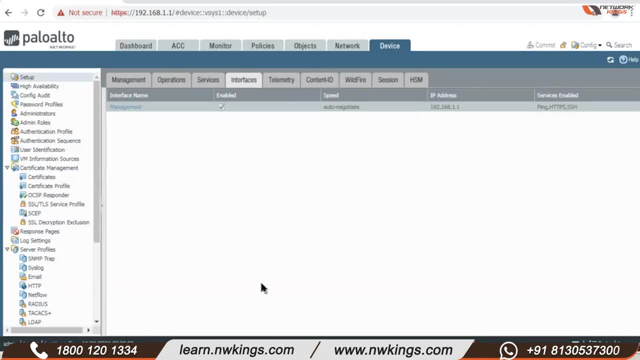 so okay, and this week you should be getting it, and provided, obviously, when you have done your payments and all. yes, yeah, i got it. i have received the lab access. yeah, so the sooner you pay, the earlier you get these things. i have joined the combo firewall for this right. so, like, sir, how to like prepare the? 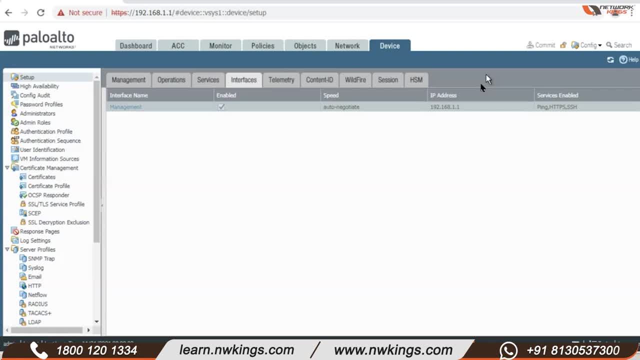 notes for what's the video. watch the video again and uh, note down the key points, like all the defaults that we talked about today. right, you can note down those defaults like interzone, intrazone, the default communication on management, uh, default communication on the data interfaces- how to change those defaults, right. 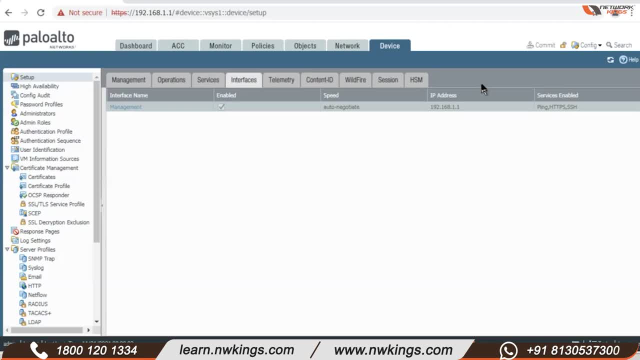 notes of all that directly. this question is a word. it is going to be: uh, how do i put this um power packed session right where we will not be, uh, wasting time on any any of the other things, and everything that i speak is important, kind of a. 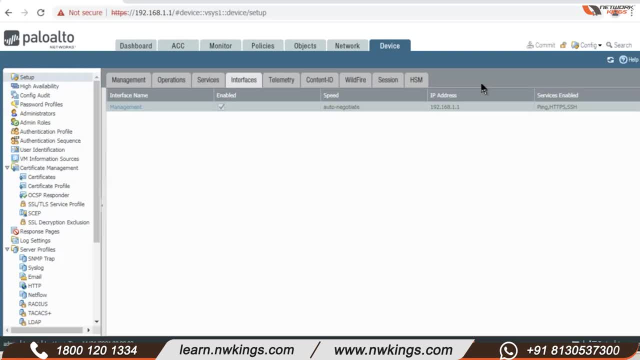 thing right, because the topics that we will cover, they all are very crucial. topic, uh, when it comes to working on daily basis. okay, to accomplish those, uh, business as usual tasks and also the interviews right after we you are done with uh, two, three labs, you'll be. 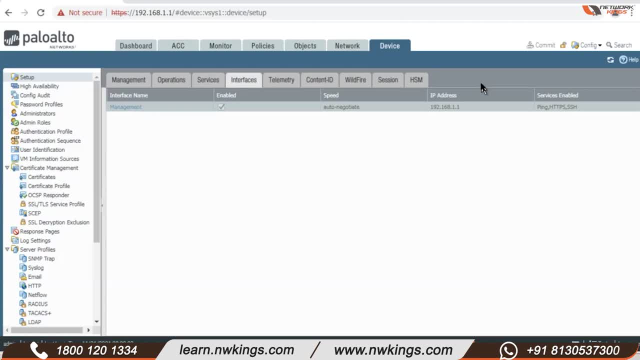 very confident. i have seen people adding, check, uh, adding the firewall to their resume even before they finish the course. right? so let's let three, four classes pass and once we are done with security policies, then matting and when we start with user ID and those stuff, that that's when you. 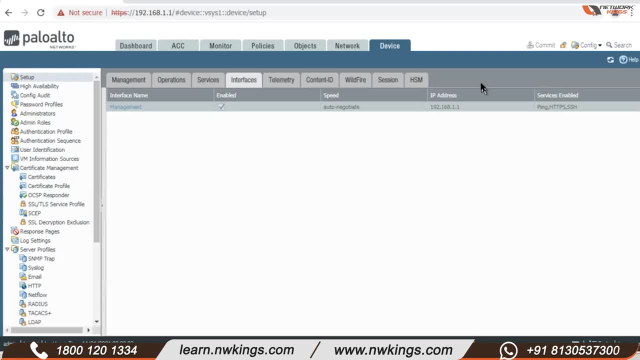 will you know, love it to the to the most and you will start adding it to your resume, provided you do practical. yeah, what was that? yeah, sir, in VPN is asking a lot of the times in interviews at VPN and netting, don't worry, don't worry you. 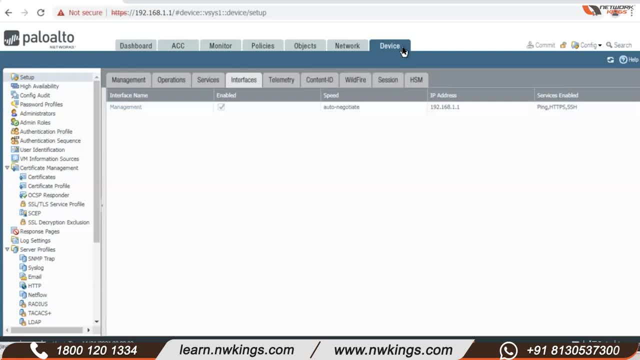 will love it so much that you would want to pay extra for VPN lectures, although you don't have to, but out of out of love, you would want to pay extra for those VPN lectures. we will cover them in such a simple and explanatory way. means for VPN: I. 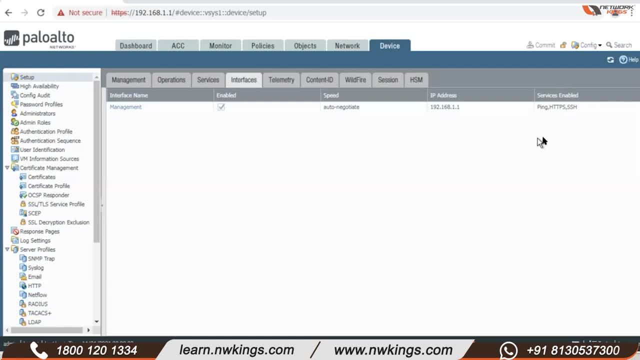 required more like that. no, no, no, I'm just kidding. actually don't worry about anything. right, there are people who have done checkpoint and f5 and now they are sitting for Palo Alto and so, don't worry, we will cover everything. let's keep it short. let's start the fresh topic. 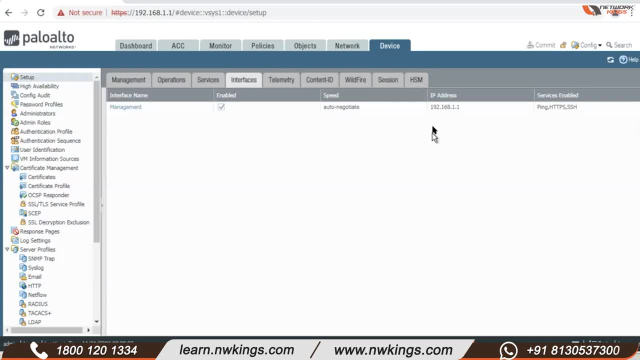 you said that correct. um, yeah you. next class is next saturday, I mean coming Saturday. okay, Pradeep say: is VPN again. when is the next class? next class is next saturdayhunkomingsaturday, I mean coming saturday, Same time, right. 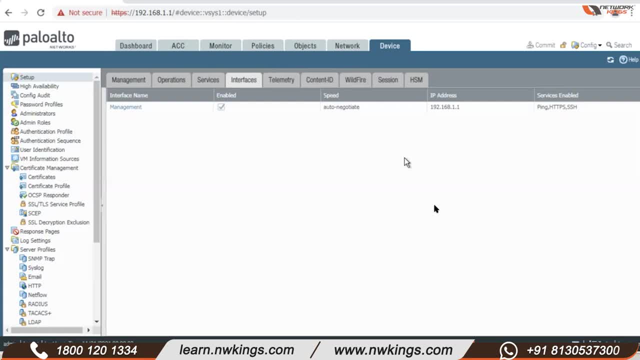 Yeah, same time. Are you still in Ireland? Yes, I am still in Ireland. I am in Ireland for the next year, One year. Enjoy, man. Which project are you on? I have come to do my Masters. I have left my job and come to chill a bit. 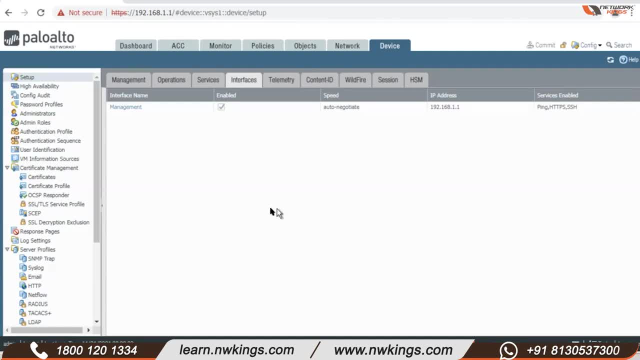 I have come to live my college life again, Say, yes, I am watching. Actually, I am trying to move away from networks, I am trying to get into cyber security. So I have come to do my Masters. for that I will get a degree and certification. 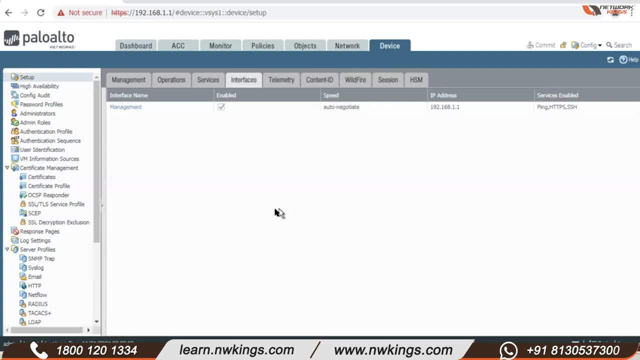 I may get a job. Don't stop studying, sir. Sir, there is one more out of the box question. My routing has been switched And this firewall has also happened. I will do this as well. So what is the next good technology? 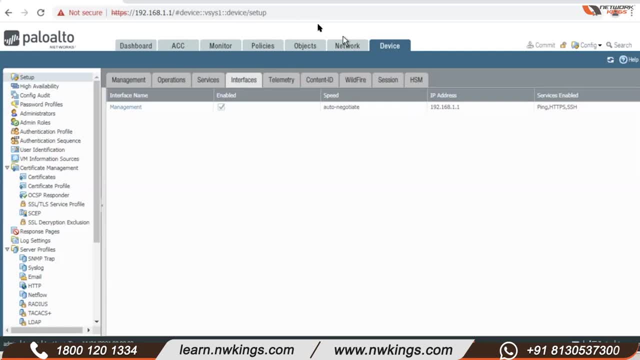 I have heard that automation is good. Yes, network automation is good. Cyber security is good. Cloud administration, cloud architect is good. Yes, I have also done cloud by doing AWS architect. Yes, So keep studying, Keep studying all the new technologies. 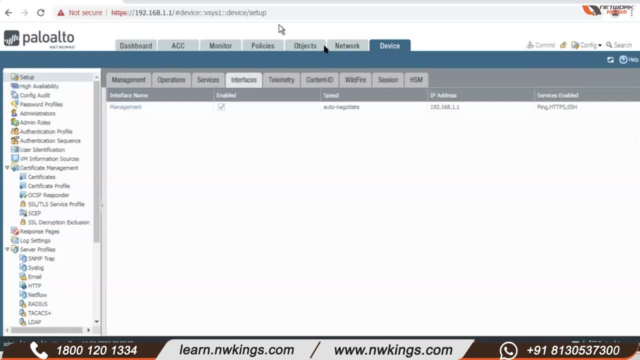 Keep studying. I have done a lot of fun in college. I will have to study as much as I have done in college. Okay, You will have to do a lot of fun, sir. I have also enjoyed a lot in college. You have also done. 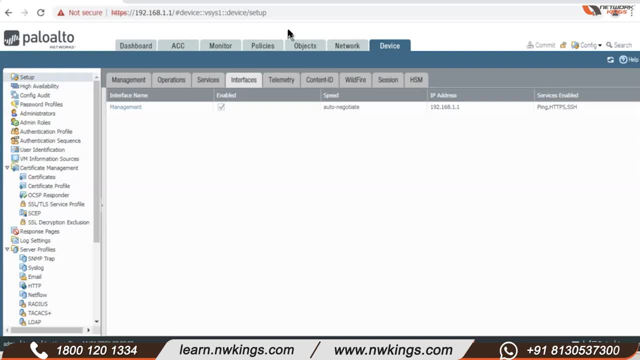 The studies in college are not useful outside. No, sir, There is a certification. Do certifications. If you don't want to do certifications, then at least do their studies, And when the company pays, then get a certification. Yes, sir, 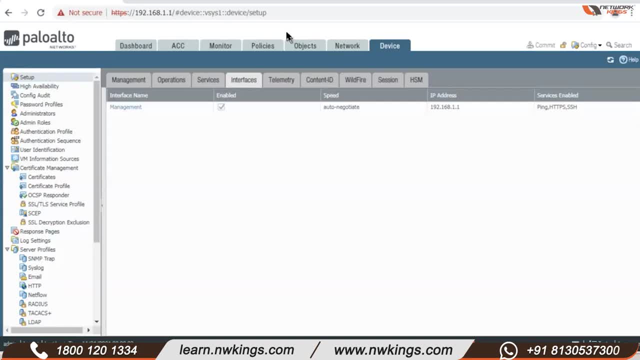 Yes, sir. So please give your googles. Yes, sir, Perfect. Yes, All right, That was In exchange. I want to give you my card. It worked. What is the NFT? you are kidding me? refused. 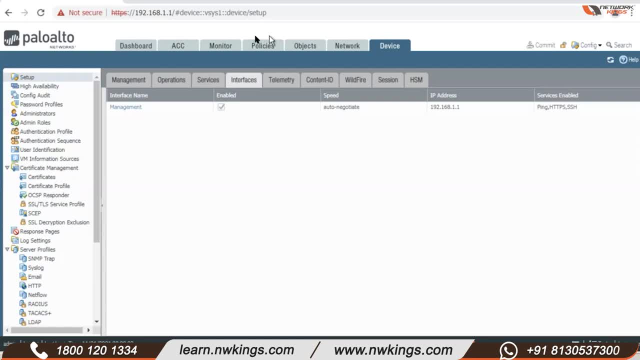 He did not need attentions to do. son of Are you there for some. This should be followed. the server should also be managed. the network should also be looked at. So these are some topics that you should know. well, If you know a little bit, then it will be fine. 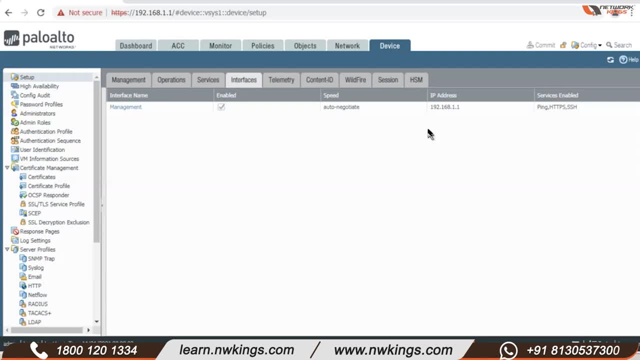 Now, for example, firewall has happened, load balancer has happened. If you do this well, then it is fine. Then the server and Linux know a little bit. They call it working knowledge. If there is working knowledge, then that is enough. 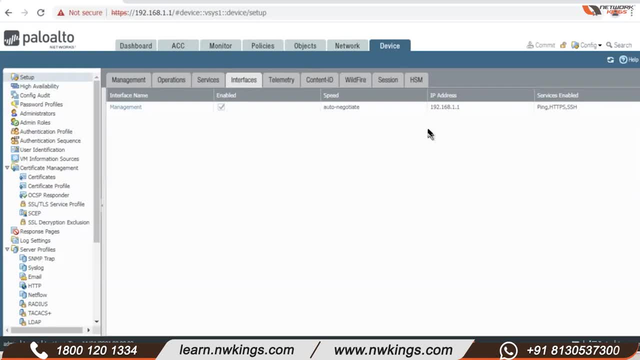 Then they do not take interviews on Linux, They just ask that. tell me one command, then it is fine. But, sir, these days scenario-based questions are coming in interviews. Yes, because that is the best way to filter out, But anyone can read the theory. 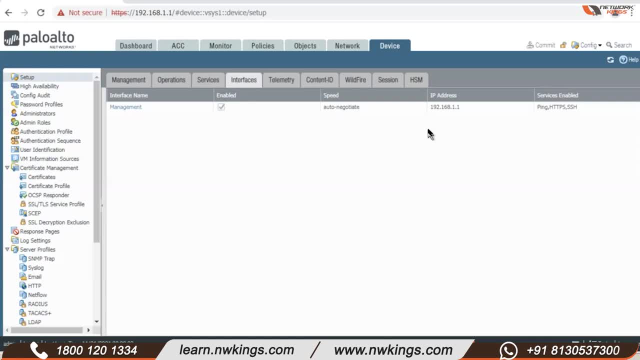 Now everything is happening online. A person like me opens a portal and sits and gives an interview. So if you give a scenario, then at least the logic will come out. That is why scenario-based questions are there. Sir, what is the demand for Palo Alto SD-WAN? Sorry, Palo Alto has SD-WAN right. Yes, What is the demand for that? I mean, Cisco is also running, So is there anything like this? SD-WAN is a different world in itself. SD-WAN is for people who are into service provider domain. 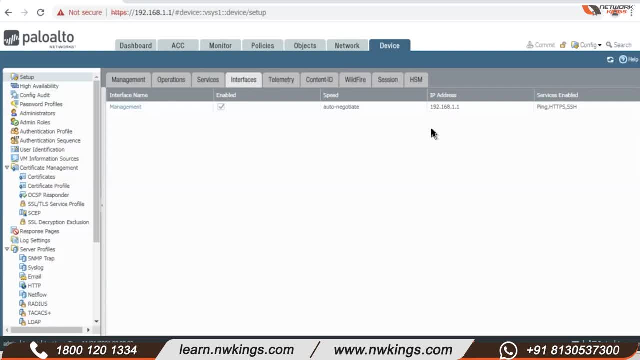 Those who have always been in the enterprise domain, in operations, in enterprise operations on the data center side. For them, SD-WAN is like changing the field. You will have to work on BGP, MPLS and all this Plus SD-WAN. 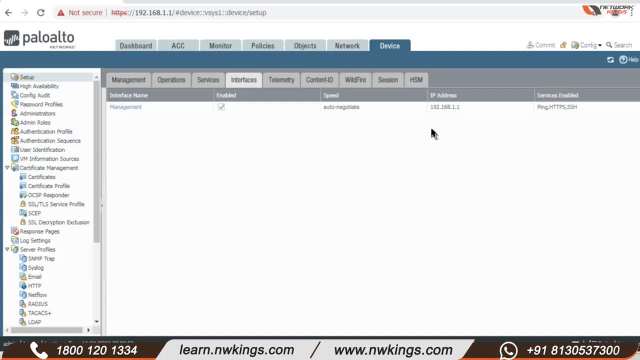 Those things. The person who works in the service provider SD-WAN is perfect for him. He should learn it. He should learn about cloud and cloud architecture. Okay, I just got the job. here I mean routing, switching and SD-WAN. 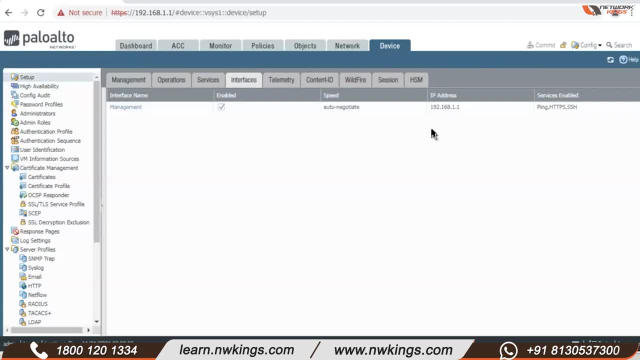 Okay, That's good, Then you will learn while working. I have never worked on SD-WAN. Okay, Sir, what is the difference between the SD-WAN in Palo Alto and the normal SD-WAN? SD-WAN is SD-WAN. 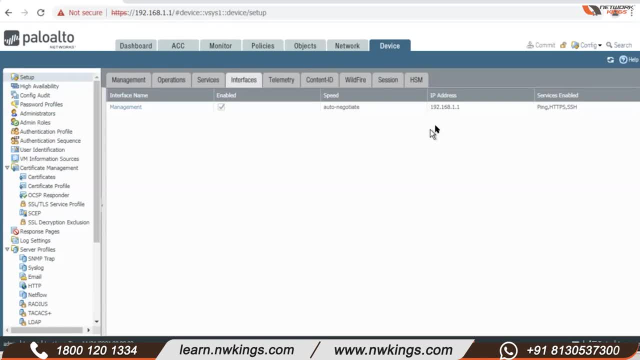 Palo Alto is just adding capability of you know being used with SD-WAN. SD-WAN is a feature in 14.8 as well. Yes, They are making everything compatible. SD-WAN is so generic and they want those capabilities in their devices. 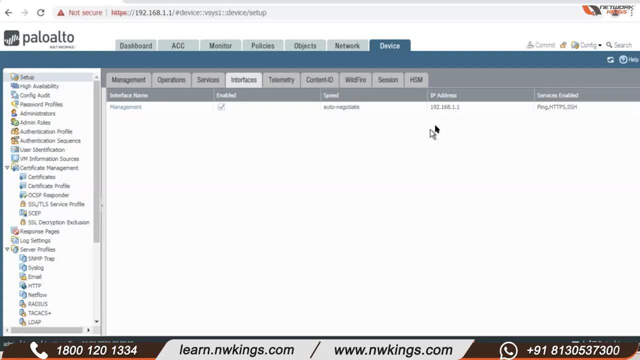 That's why they are adding everything In that feature. actually, they have given the feature of load balancing- Yes, Include balancing: Yes, Right, Right. There is more automation in SD-WAN, The IPsecs that are formed branch-to-branch. 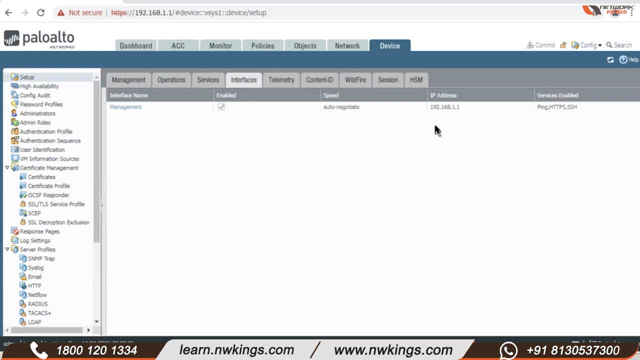 they are automatically formed. Yes, So in this? Yes, The automation has come everywhere now, Yes, That's the money of that thing, That's all. Yes, Yes. So in this Palo Alto, this SD-WAN. 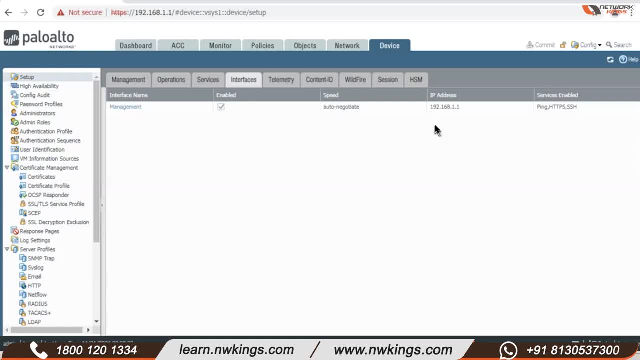 will it work like link load balancing? Yes, The main funda of SD-WAN is that you can have multiple links and all will work as backup for each other. Ok, They will be used together as well. All right, Ok, So getting to know the market leader. 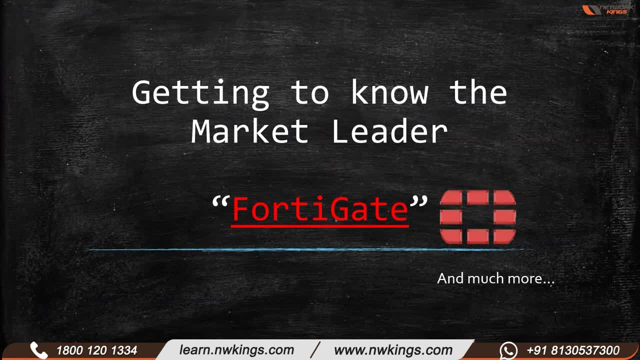 So we are going to talk about FortiGate firewall Now. FortiGate is the product and Fortinet is the company. all right. so just like you have Cisco as a company and ASA it is its product, right? so just like that, FortiGate is a product and Fortinet is the company. 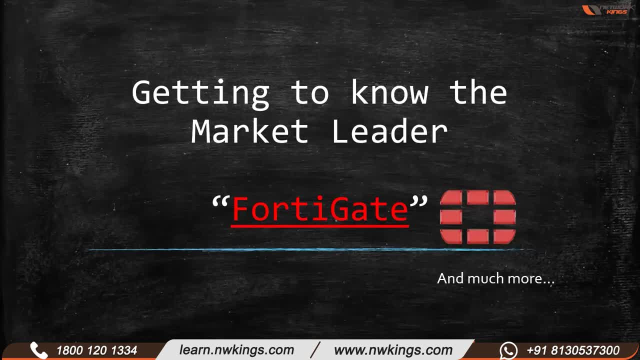 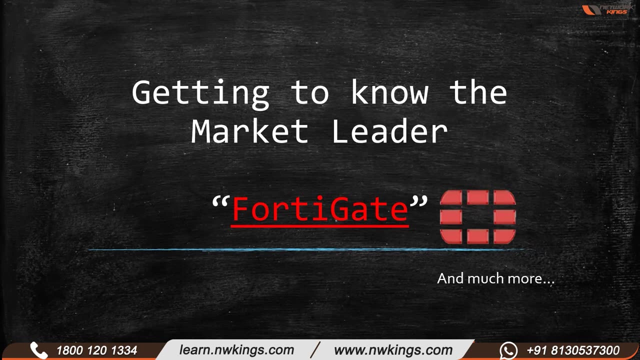 a lot of students, you know. at times they do ask me: you know that, is it Fortinet or is it FortiGate? so I told them: see, it's a product. Fortinet is basically the company. all right, okay. now, when it comes to the FortiGate, you can all see right in the screen that it says getting to know. 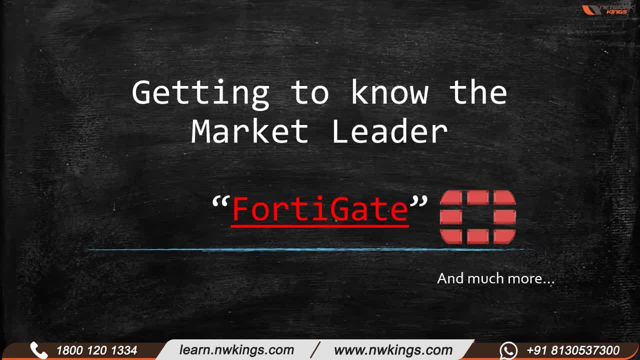 the market leader. so why is it a market leader? why are we saying this that it is a market leader? I mean just because I said it is a market leader, just because I am saying this is market leader. so is it a market leader? I don't know. let's see, let's try to figure out. why is it so okay, and 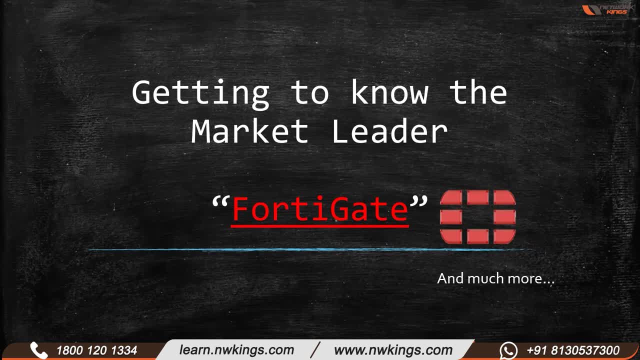 we'll all talk about the facts and figures. okay, nothing you know, just promises or something like that. very much plain old, simple facts, figures. and then we'll work on why we need know FortiGate and why we need to learn FortiGate right now, because if anybody who wants to, you know, take. 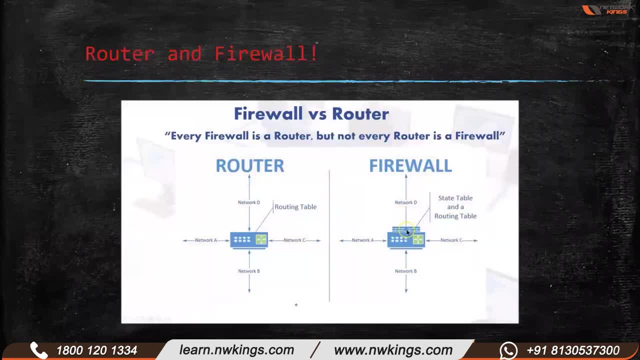 that jump in his career or in his or her career. now, before I go ahead and, you know, start talking about this FortiGate firewall, let's do one thing. let's, you know, make this an interactive session and let's try. you know, this is just for all- that- all those person who are 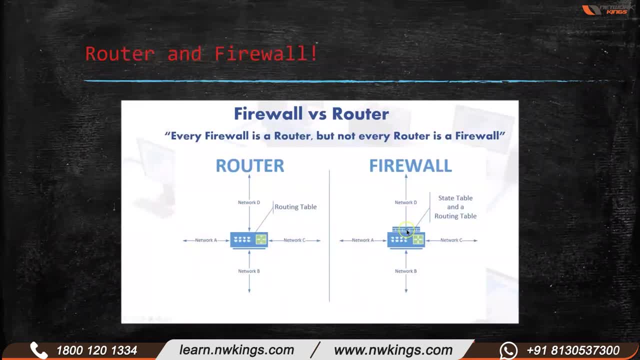 either you know who are interested in FortiGate, or who are interested in FortiGate, or who are either new to the networking field, or they are people who are basically new to the firewall or basically new to the security team. okay, all right, so let's keep this a little bit of interactive. 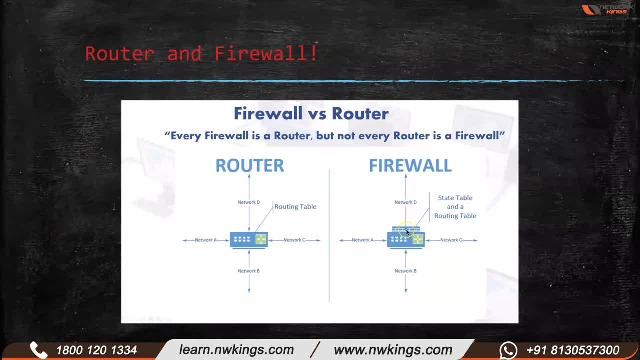 all of you guys. just let me know in the chat window, what do you think is the difference between a firewall and a router? according to you, what is the difference between a firewall and a router? chat window- youtube, sorry, zoom pedal. oh, all of you guys, what is the difference between a router and a firewall? okay, yes, okay. so a lot of. 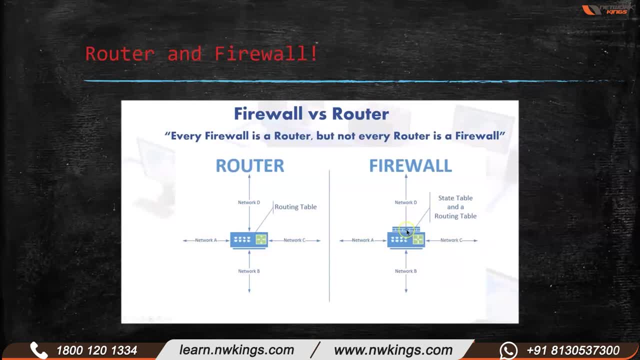 people are saying router's job is to route the data. okay, so in a way, yes, what else does the anything else that the router can do, apart from, you know, routing the traffic? anything else that the router can do? that says no difference. both act the same. okay, firewall is a security device. 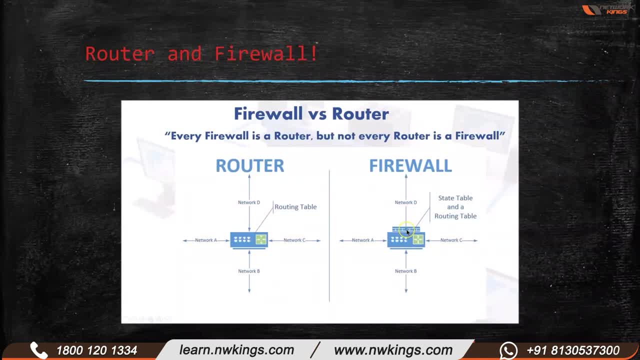 router is a connection, okay, okay. venkat says can block the traffic. abhinav firewall, maintain session table and routing table- okay, all right. venkat says: with the ACI as well, all right, okay. so yes, in a way you are correct. now see, what happens is when we are talking about a right router, right. and whenever we are talking 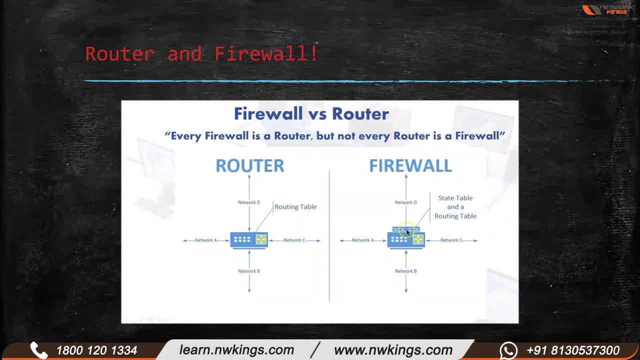 about something which is called as a firewall. okay, obviously, when it comes to a router, the main job is to ensure that you are able to, you know, route the traffic okay. so i mean, if there is any traffic like that, you can route the traffic okay. so, I mean, if there is any traffic like that. 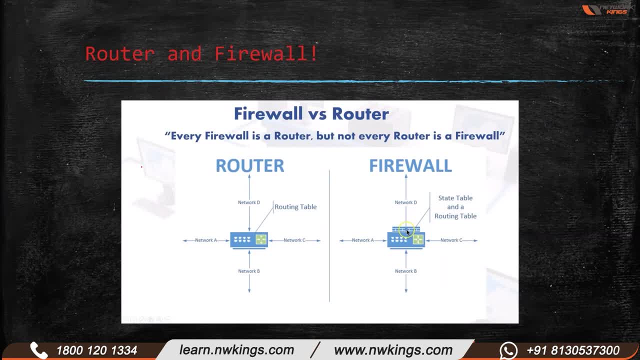 say, for example: okay, let's do one thing, let's just again, let's do this. what is the first thing that the router will do when it when it reach? so? so let's say, for example, this is a pc- okay, now this pc is trying to get to another pc which is over here. let's say: this is google- okay now. 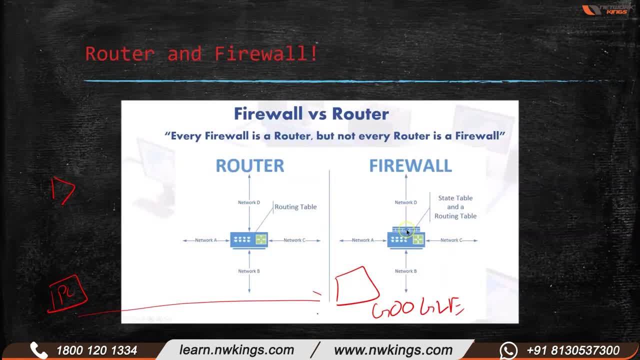 uh, pc1 is trying to connect to googlecom. as soon as this traffic, or as soon as this uh packet reaches the router, what is the first thing that the router will do, first thing that the router would do over here? okay, check the destination. okay, uh, it is going to check the routing table, okay. 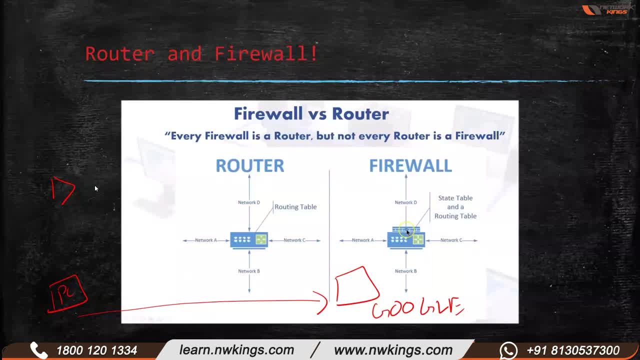 all right, so let's, let's, um, what do you think? what is the first thing that the router would do? will it check the destination? always going to check the? uh, you know the routing table. okay, okay, all right, destination prefix. okay, go dynamic routing. okay, dynamic routing again. uh, it's, it's, after you know, it checks the router. 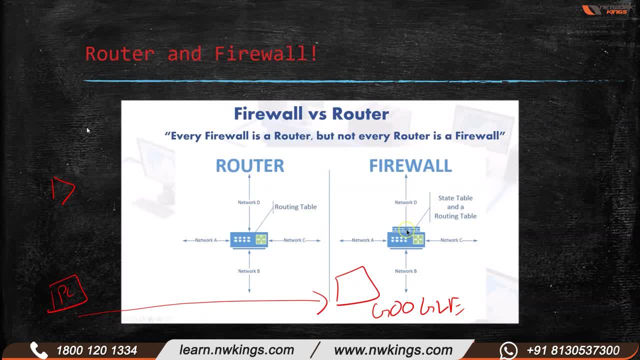 you know it checks the routing path. okay, first of all, obviously, it's going to look into the destination prefix. okay, and oopsie, it's going to look into the destination prefix. and once it knows that, okay, if the destination is part of the local segment or not. if it is a part. 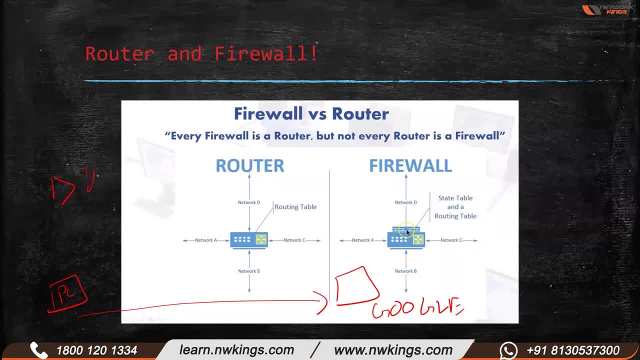 of a different segment. it is going to look for the routes. okay, so it is going to do, uh, something which is called as the route lookup. what is the next thing that the router would do? route lookup is done. okay, i know what route i need to take. what else, right, actually? okay, right, see. so, once the 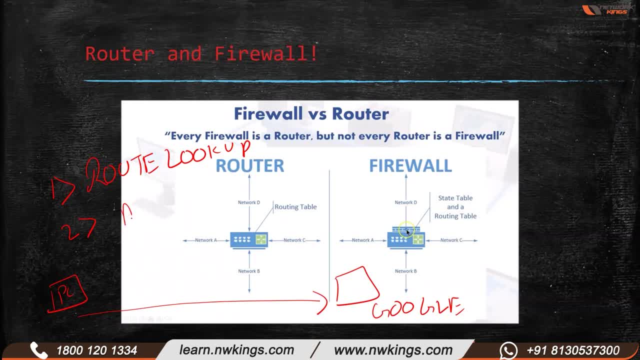 route lookup is done. there is also one thing which is called as the acl right. i need to figure out that. whether whatever the traffic is okay, is it allowed or not? because if it is not allowed, i'm basically going to drop that packet okay. so acl is also a major part when it comes to a router. i mean if it has been implemented. 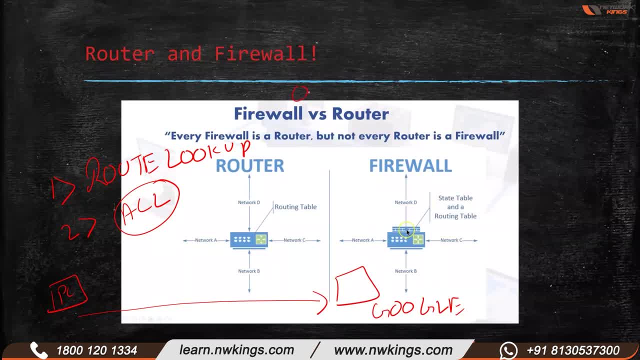 okay. so if let's say, for example, let's say i have something which is called a 0.0.0.0, 0.0.0.0, and i say 192.168.10.1, which is my gateway, this is the destination, okay, and i say ip out. 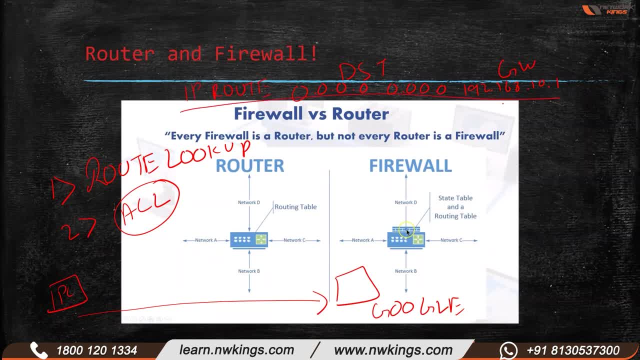 what does this command is telling you? this command is basically telling you that if there is any, whatever the destination is, any destination, just forward that traffic to the gateway, and my gateway is 192.168.10.1. okay, and this is also, uh, an acl in pace, which basically says whatever the traffic is, it is. 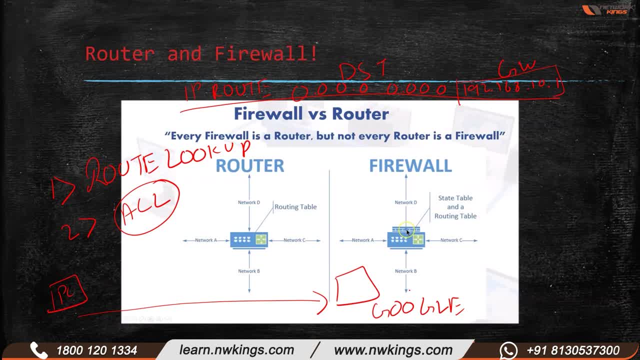 allowed. now tell me one thing. let's say i'm trying to access googlecom right now. if i'm accessing googlecom, what is the first packet that goes? it's a tcp sin packet, right, correct or not? yes or no? is it the pcp sin packet or is it something else? 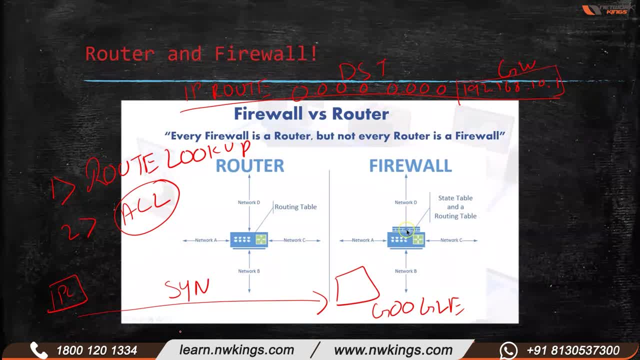 yes, right, so it's a tcp sin packet. so what should i expect from the googlecom or from the server? what should i expect? what should be the next packet? okay, so joy says sanak, abhinav says sin reply: uh, aisen would be. this would be basically snack sin plus. 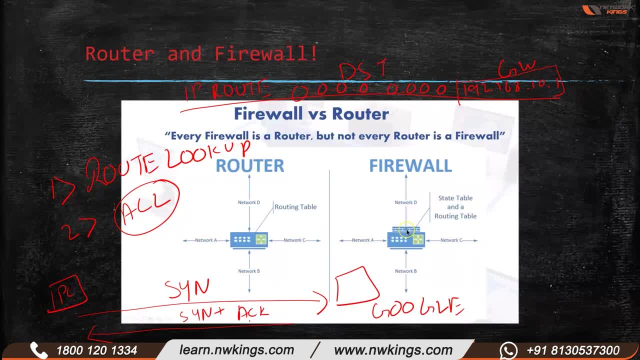 in a way, reply also, you can say, but then the more technical terminology that to be used would be a sinac, okay, is basically its own synchronization. uh, packet and act is basically the acknowledgement number that has been used to. um, you know, tell this, uh, tell the pc that i have also uh acknowledged your. 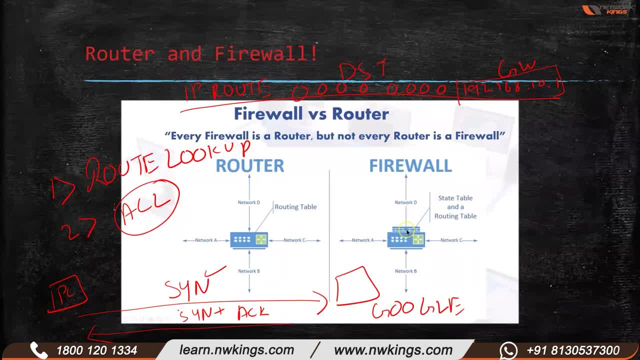 sync packet. okay, okay. now tell me one thing: if this sin plus act comes to the router, router is going to do what? it's going to drop the packet. why? because acl is just from inside to outside. okay, the acl that i have in place is only for inside to outside, to ensure 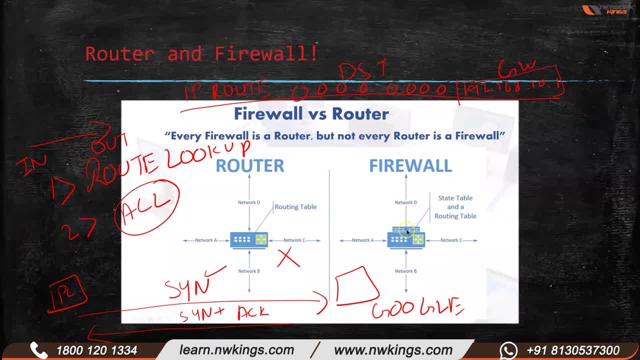 that i also receive the traffic. i need to again create an acl which is from outside to inside. right, so i should have two acls, right, am i not? yes, no, maybe correct, okay, all right. so what i know over here is that if in i'm working with the router, i need to have two acn. okay, why? because one would be to 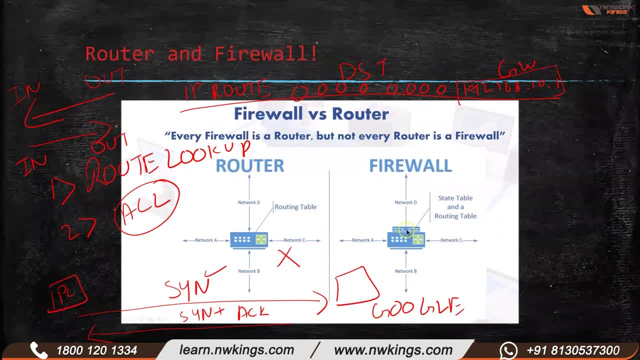 ensure that the traffic is basically going from inside to outside and one from outside to the inside. okay, all right, do you know what this concept is called? this is, this is basically. this is see. what is this in and out and out to? in, what am i trying to do over here? what i'm trying to do? 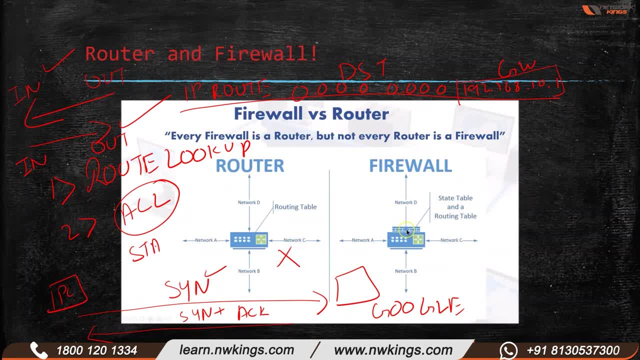 over here is basically this is a state state of who the packet right now router does not have any, you know intelligence that it could save this information, the state of the packet, so that it can understand what i need to do. but when it comes to a firewall, okay, apart from having a routing, 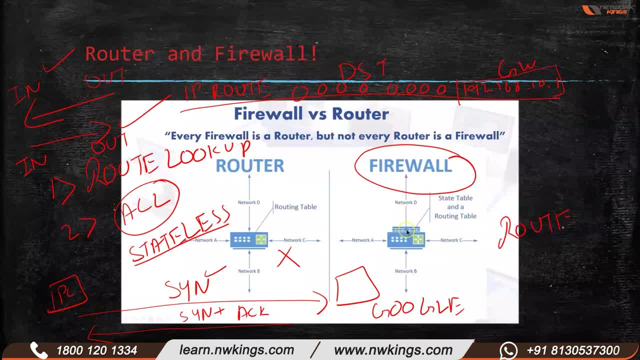 table, which it obviously have. okay, apart from your route table, they also have something which is called as the tell me what happens. what do you say? state, state table, stateful table, okay. stateful table, state table, okay. this is the only thing. shakespeare also said. what is in the name? 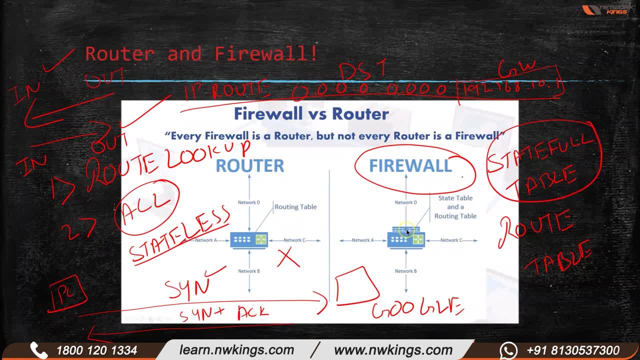 okay, but my point over here is: he firewall basically also have one thing which is called as the stateful firewall. it basically has something which is called as a stateful table or a session table. now what this means to us, what it means to us as a, as an engineer or a firewall administrator. 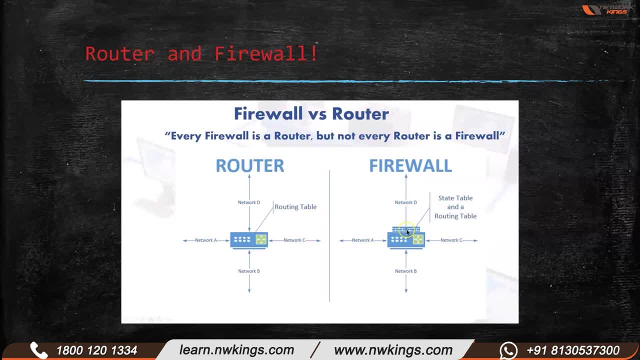 okay, see what does. what this basically means for us is quite simple: see, whenever there is, let's say, this is a pc, over here, again, same same setup. okay, this is google. now, as soon as i send this traffic, i have a syntax and going in. okay, now what the firewall will do is: 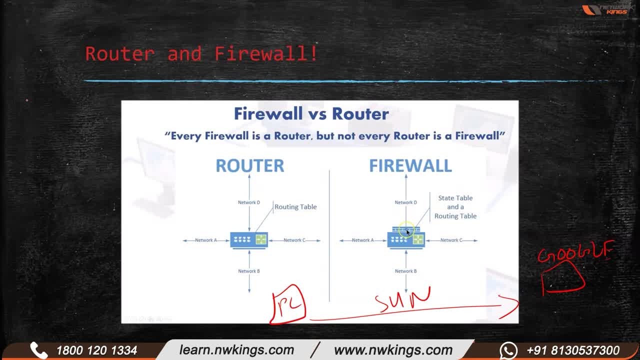 i'll see, rather than having an acl firewall, have something which is called as a policy right. policy is also a way. in a way it's an acl which basically tells that what kind of traffic is either allowed or what kind of traffic is denied. right now, over here also, i say: 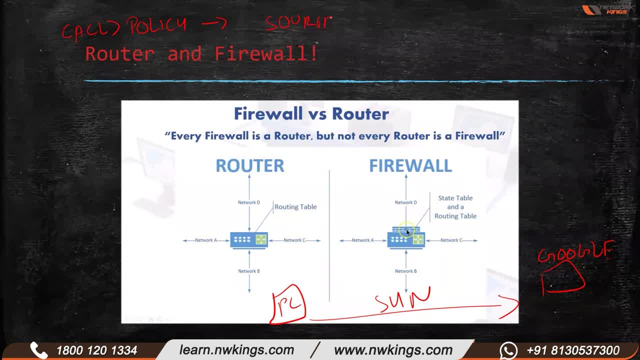 you know, source can be any, destination can be any. just an example: service can please never do this in your environment. service any okay, and i say allow. so this policy will do what. this policy will ensure that whatever the traffic which is coming from my inside to the outside is allowed. am i right or not? 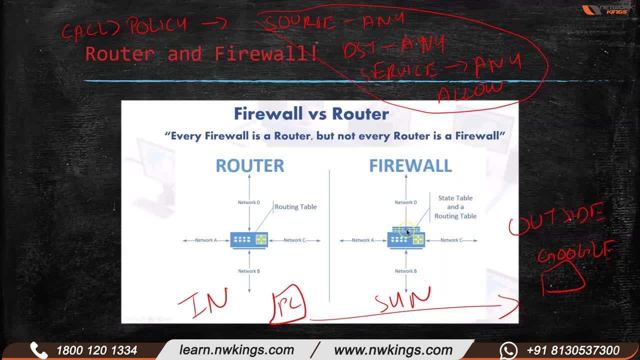 yes or no confusion. good, now i'm keeping it very simple, all right, so people who are basically starting off in the security department or in this field, who wants to basically learn this firewall, we'll keep this simple. okay, see, so we have this policy right now. this policy is allowing everything. 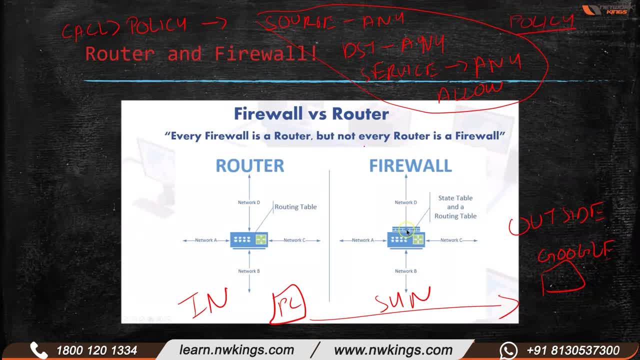 from inside to outside. okay, great, now tell me one thing once the traffic comes back, so i will also get us in act. google will also, you know, give me a reply back, so i'll get a snack now. what this firewall will do is it also has something which is called as the session table- right state table. straightforward. 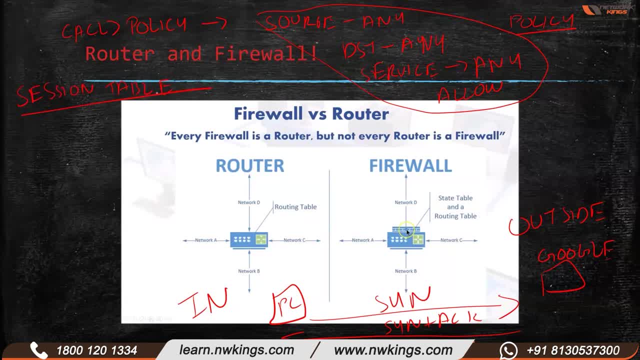 table, whatever you want to call this, but we have something which is called as a session table. now, what does this session table has see? session table basically has information about: first is the source- ip- okay. then you have something which is called the destination- ip. okay, Chalo batao, tell me kya, kya hogar. anybody who has experience or anybody who has worked on it, who might have seen it? 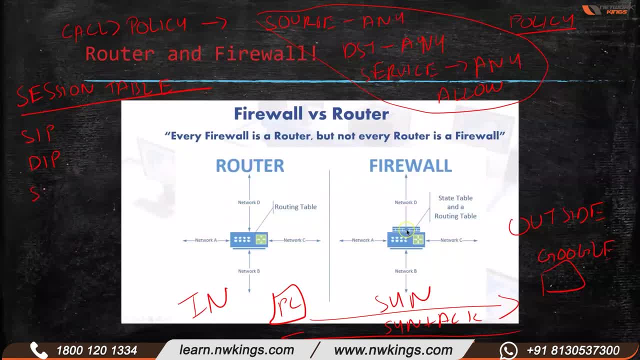 Okay. Venkat says source port. good, I have source port, what else? Rajneesh also source port. Abhinav says: DP, DP ka kya matla bata. Abhinav display picture: DP chalo destination port. 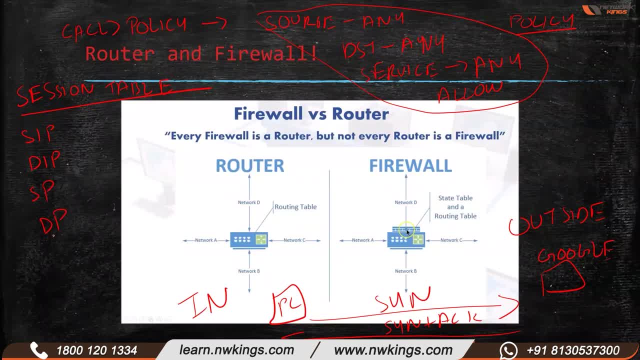 Okay. Rajneesh destination port. Abhinav destination port: okay, what else Aur kya hota hai? what else do we have? Kunal says session time, Let's say time. What else? Amit says source MAC, destination MAC: okay. 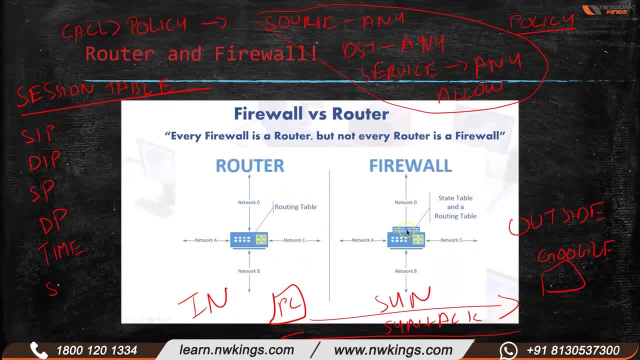 We have something which is called as the session- sorry, session ID. Okay, so what happens is I have source IP destination, IP, Source IP port, destination port: the time- uh, basically the time at which the traffic came to me, and the session id. so session id is basically an alphanumeric value. 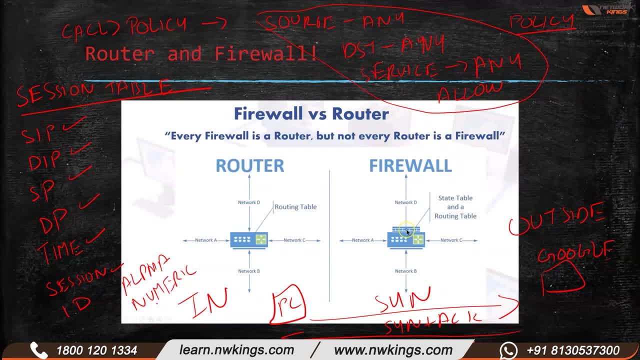 generated by the firewall, it by itself for its own identification. now what it does is, let's say, for example, ip address is 10.1.1.1. destination ip is um 164.100.1.1. okay, sports sport, sorry. so sport is, let's say, 51 265. destination port: googlecom and what should be the destination port. 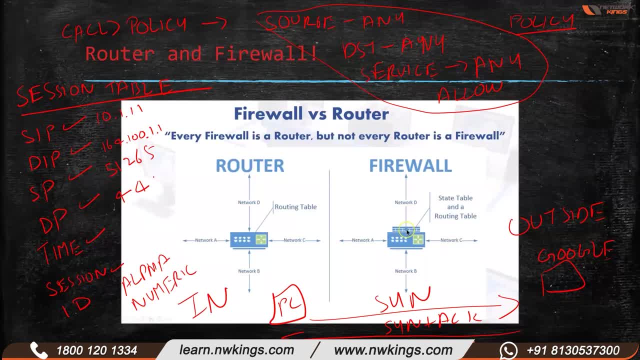 443. good, joy is very active. good, good, good, okay. so destination port: 443 time. so time basically depends on wherever your forticate firewall is, or basically whatever firewall that you have. time depends on where. where is your firewall location, geographical location and whatever time that it has received that packet. so abhi what time it is, it's 7- 20, okay. 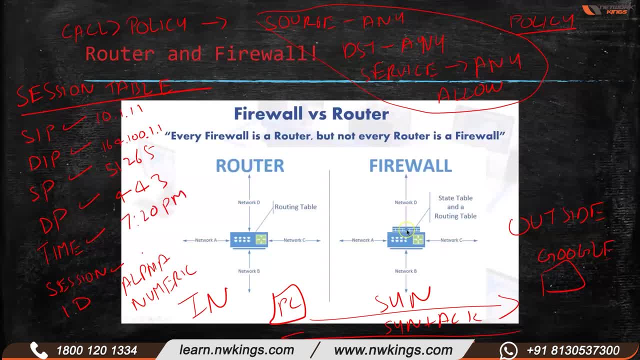 so 7- 20 pm. all right, then we have something, some session id. so let's say alpha hashtag: one, seven, b, h, five, let's just say eight number: okay, now see what happens is that, once i have all this information, information, okay, so let me just remove a couple of things. that becomes a little bit cleaner. 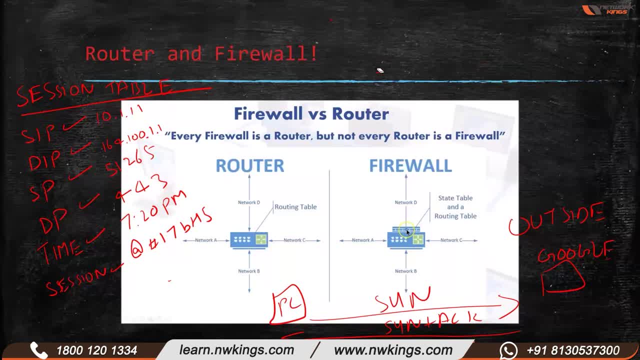 okay, see now. what happens over here is that, when i have all this information, what will happen is the traffic, whenever the traffic is going out, with this impact. right, i have saved all this information. okay, i've also saved something which is called as the pcp state. okay, this is also one. 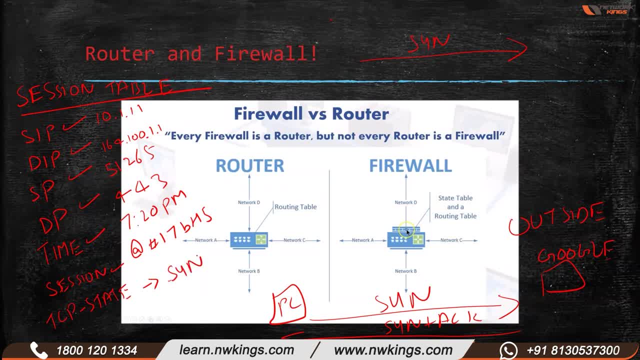 thing which is being saved. so it is send packet. okay, so i know that this sin packet is going out. i know the source, ip destination, ip source, port destination, power time session, id, all those things. i have this information. now what happens is when i get a sin back, when i get reply back as a sin, 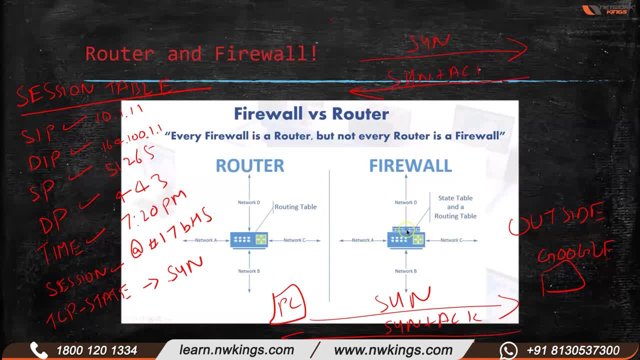 act right, sin plus act. what i have is first of all firewall, rather than looking into the routing table, rather than looking into the firewall policy. do you know what? what it does? the first time it is going to look into the session table. first thing it does it's going to look into the session table. it doesn't look for the route. 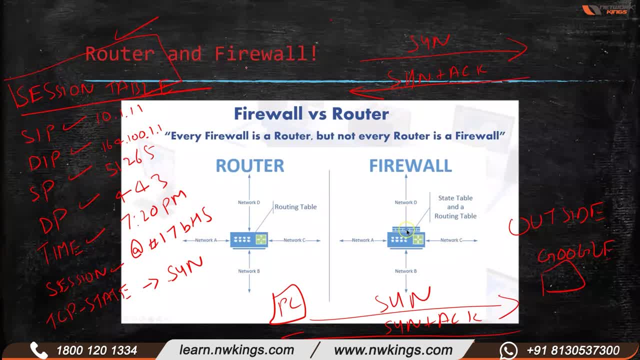 doesn't look for the firewall policy. it first checks the session table just to confirm whether the traffic which i have just received, this synthesis act, is it a part of a packet which was initiated internally or is it a new packet? okay, so it's going to look into the packet. sorry, it's going to look into the session table. 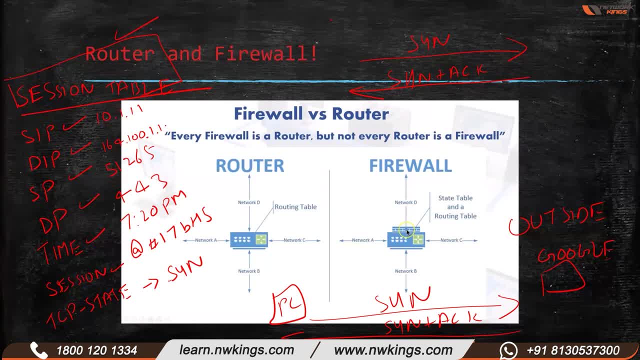 it finds out that, okay, i have source ip, this destination ip, this source port, this destination port, this and syn act would basically have destination port as 443 and uh sorry, this, uh sorry, the source port as 443 and destination port as 51265, because it's a reply right. 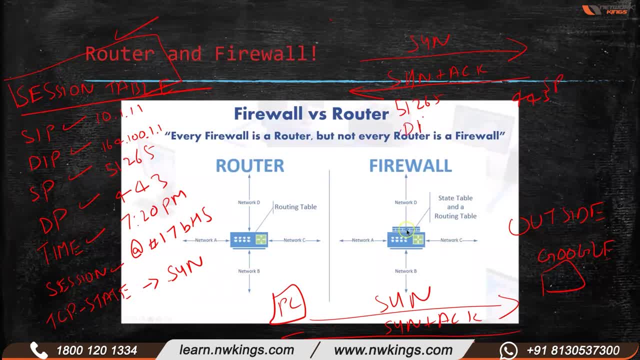 so this will be the source port, this will be the destination port, right. so now, by looking into this information- okay, not just this port information or the rest of the information as well- looking at that, the firewall knows that, okay, it's not a new packet, it's an old packet which was originated. 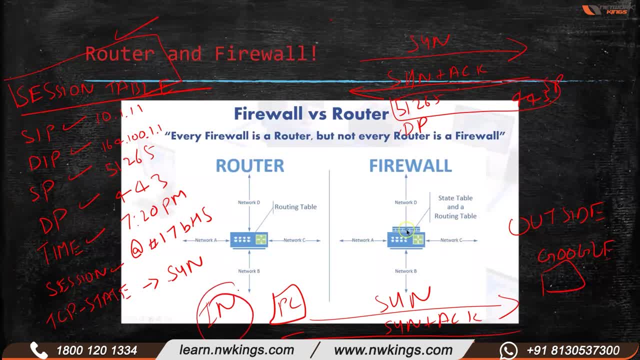 from the inside. okay now, since it's a packet which was originated from the inside, i do not need any other firewall policy or an acl be allowed applied on this. i will use the same firewall policy and allow the traffic. okay, so i'll be using just one policy and i'll be allowing the traffic. this is called as state. 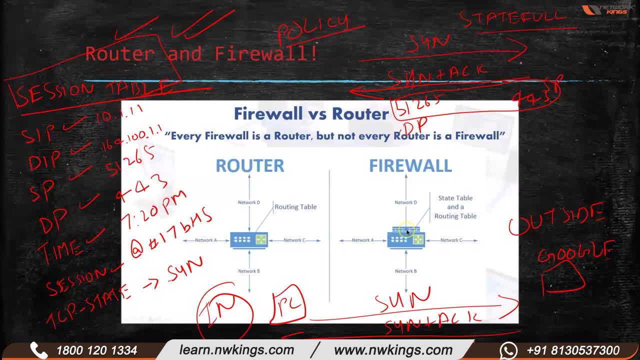 full sessions. okay, stateful technology, you can also say so. this is how, basically, a firewall ensures that just by using one firewall policy, you are allowing the traffic which is going from inside to outside and if the traffic from the outside is also coming for the same session, okay. 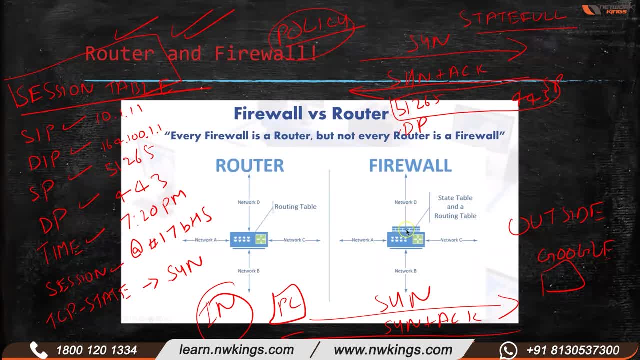 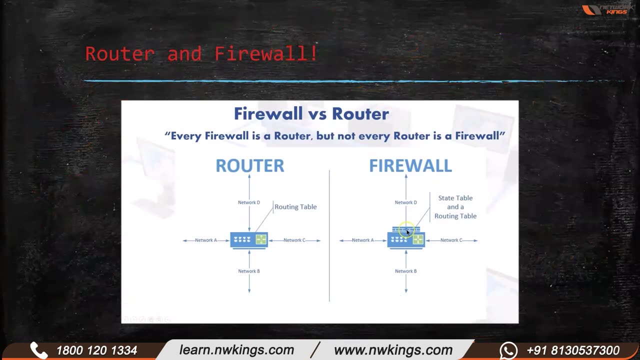 it is going to allow that traffic as well. you do not need to have two policies or two acls for the same traffic, which we had to do in in a router. okay, this is, uh, the major, major difference between your router and a firewall. now, why am i telling you all this? see, the reason is very simple, now that whenever you as a, so let's. 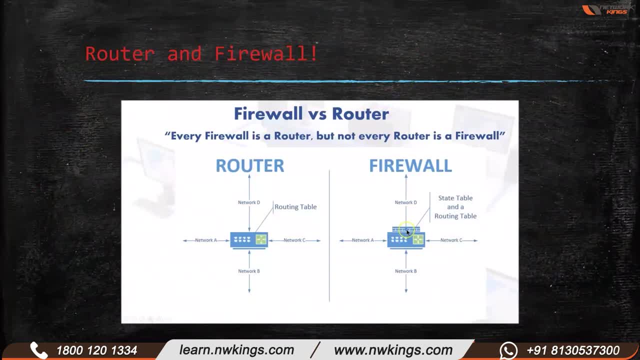 say, for example, a lot of my students, what they do is experience, experience, experience. they are looking to, you know, go into this field of security. they want to look, uh, you know, work on the firewalls and when they sit in an interview and interview, also know this guy is actually coming from a. 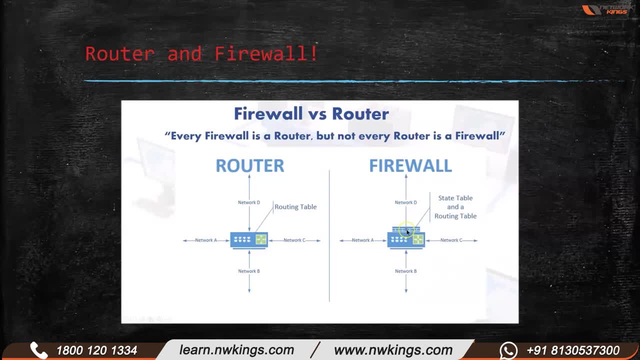 networking background. so he hasn't worked on the net um any firewalls. but then he does have favorite knowledge Cugs. Let's say: what is uh session table? what is uh um session list? uh connection, what is a stateful connection? what do we do? what exactly are these things okay? 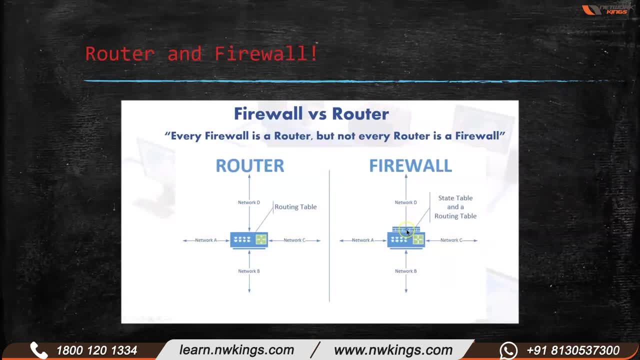 Only after you get the concept of the thing, でドン, you won't be allowed to sit in the interview later, right? And this is because you don't know the concept. in fact, if you don't know the concept, you don't know the concept, in fact. 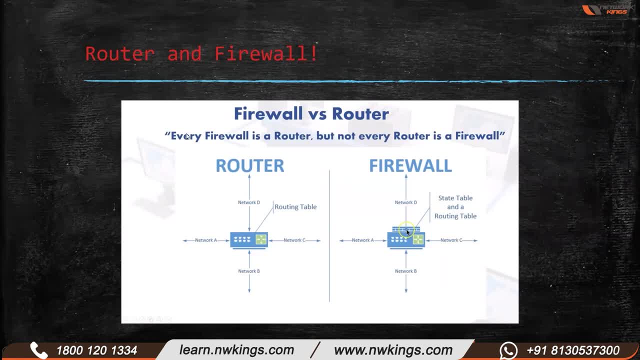 So you won't be allowed to participate in the interview later, that's okay, But just get simple: shi baate ek baar batao agar tumse koi puche ki bhai, how much experience you have in your networking field. you say, sir, i have, let's say, 3 years of experience. ok, he says: 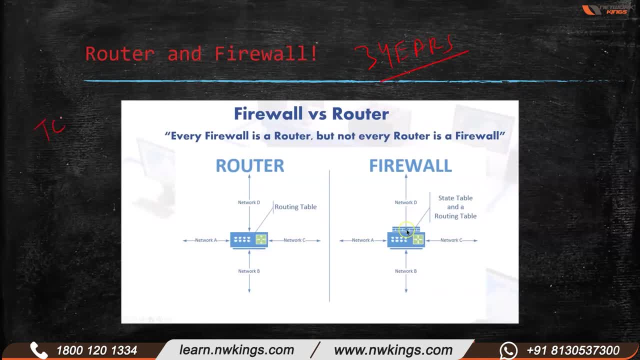 ok, alright, fine, go ahead and tell me, what is a tcp 3 way handshake. agar tumse tcp 3 way handshake nahi bataya gaya, toh tumse kya aage interview ka main kuch baat karega, nahi karega, right? this is exactly what happens when you are working on a firewall as well. 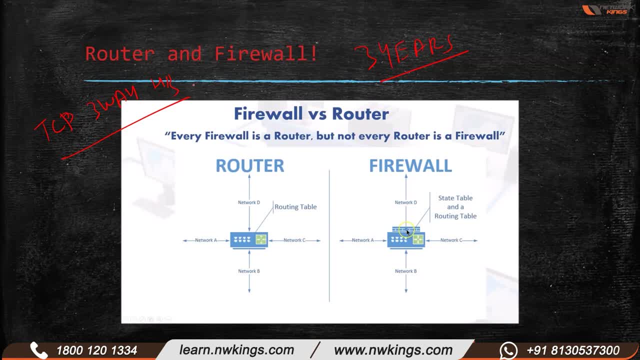 ok, if you do not know what is a stateful table or what is a stateless connection. what is a stateful connection? state table, kya hoti hai? session table, kya banti hai? firewall, kaise information check karta hai, kaise firewall policies apply hoti hai. agar yeh nahi pata, 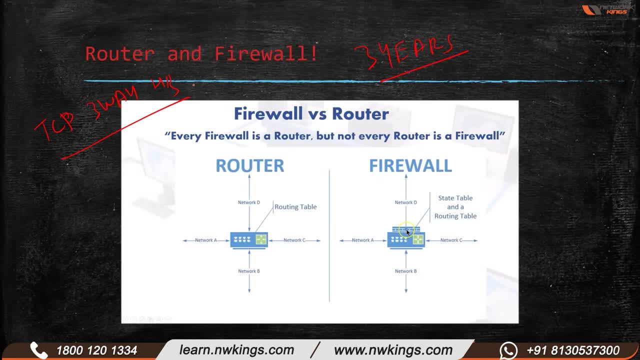 hoga. if you do not know this, alright, in the interview, basically, the interview, basically understand that he does not know much and this guy is not the right candidate for the job. ok, so, even if you go for 5 interviews, 10 interviews, end of the day, kya bologe? 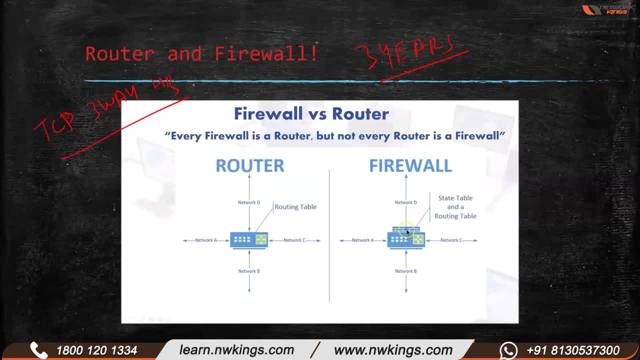 ok, kya naukari nahi malde, job nahi malde, interview bahut tough hai, but but actually problem kya? problem yeh hai that you do not have the right knowledge. ok, so what we are doing over here is giving you the right information, the right knowledge, practical knowledge which. 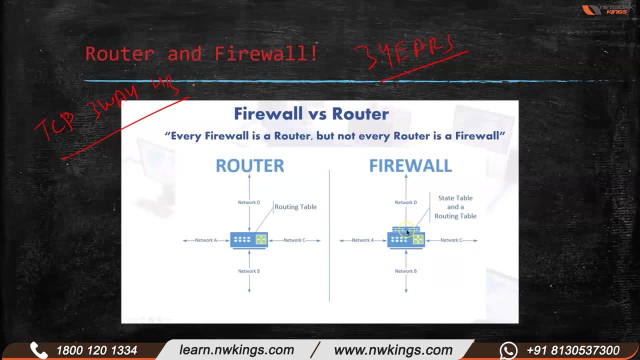 would help you basically gain confidence and apply that knowledge in your interview to get that job, to get that promotion that you want. ok, alright, so this is firewall versus router. just a quick discussion. what it was. ok, every firewall is a router, but not every router is a firewall. in a in one line, isko summarize: kar dete hai har ek firewall router. 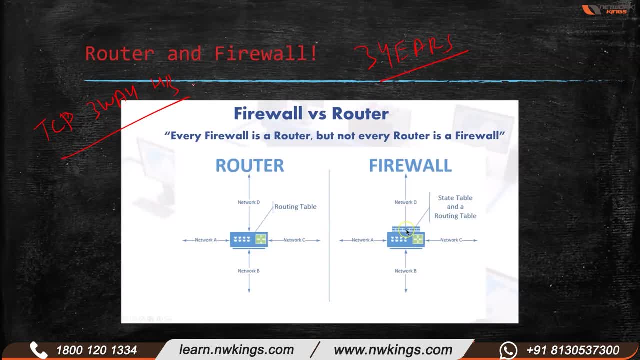 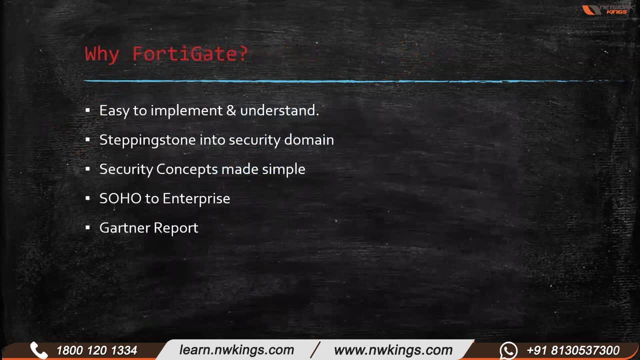 ki tarah to kaam karta hi hai, but har ek router jo hai, wo firewall ki tarah kaam nahi kar skta. alright, ok, so let's move ahead. ok now. why do we need 48 kyon cheyye bhai? why? why? 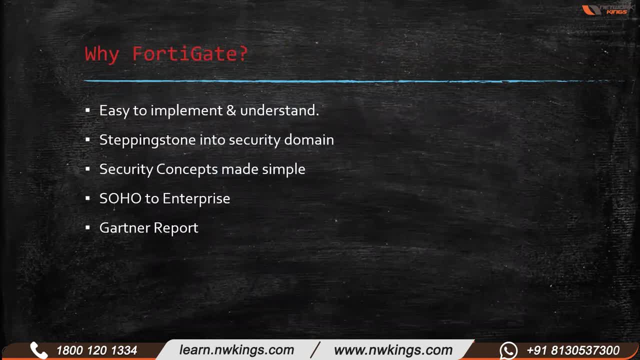 all the files, why all this thing see easy to implement and understand. one of the best features of your 48 firewall is that it is very easy to implement. ok, i will tell you why exactly this is because we have one more session tomorrow, okay, so it is very easy to implement as compared. 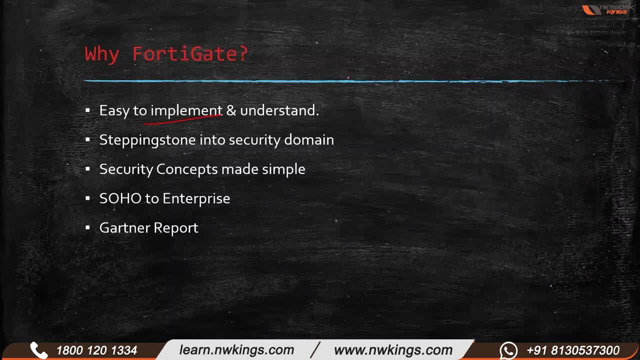 to. you know different vendors. they have a very complex setup, but then with photogate it is very easy to set up. okay, easy to understand. i'll let you know that tomorrow as well. uh, stepping stone into security domain. absolutely right, stepping stone for your security domain. 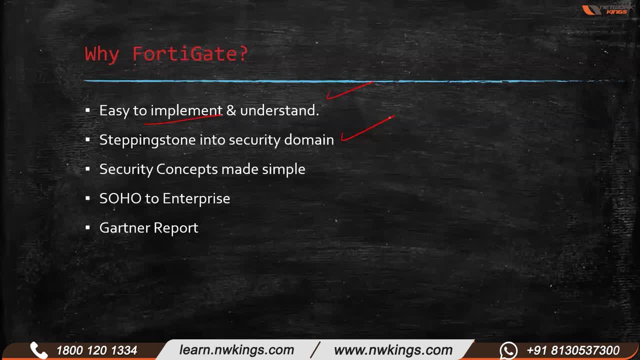 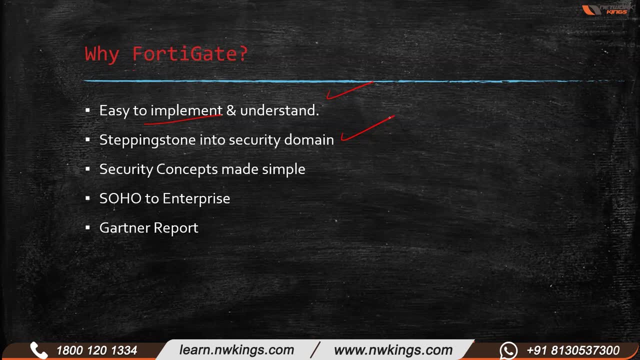 anybody who wants to get a career in this field. i would definitely go ahead and say that you know, rather than see. i do not say keep, i do not go for checkpoint or do not go for palo alto, absolutely go for them as well. but then, um, if you compare them, all right, uh, photogate. 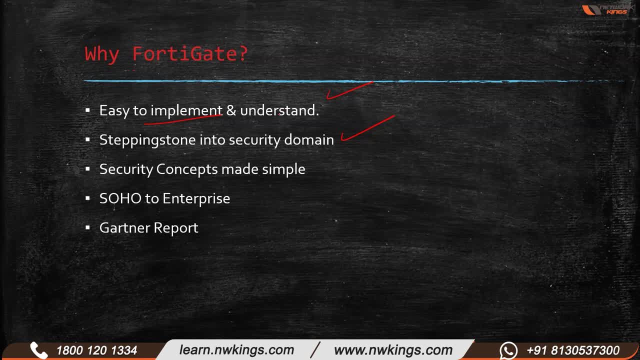 is much easier to understand- it must easier to, easier to grasp and work on as compared to the other vendors. once you understand this thing, your next step could be checkpoint or palo alto, whatever you want to, okay, but i would say, if you want to get into this field, this is the stepping. 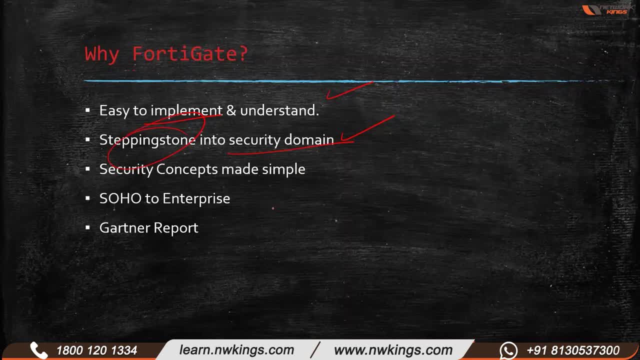 stone. okay, security concepts made simple. yes, that is why i'm here, this is my job: to make sure that the concept is very much simple for you guys. okay, even if you're a layman who does not have you know any knowledge, just you know basic networking. that is more than sufficient. but 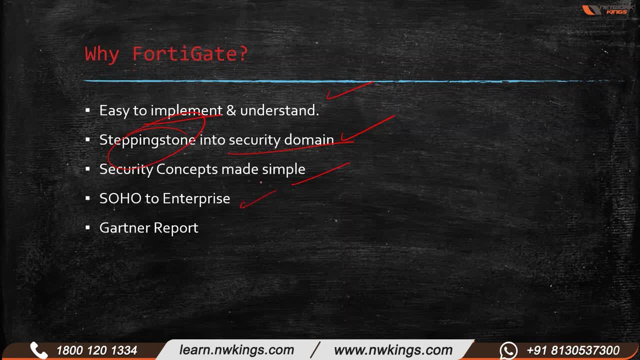 yes, at least basic networking. okay, so, who to enterprise? this is? this is basically a small office to home office, basically small set of four to five people or ten people to basically thousand of people, thousand of users or ten thousand users, or even more than that. we have something which is called as gardener report. okay, okay, uh, report card which i, we, we got. 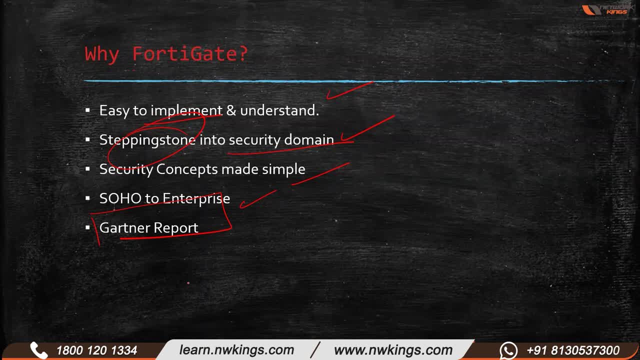 we used to get you know in school and we had to get this signed: um. more or less, it tells you about um, all the security vendors that you have. okay. whatever security vendors that you have, okay, it grades them, it ranks them according to the market standard, according to what is required in the 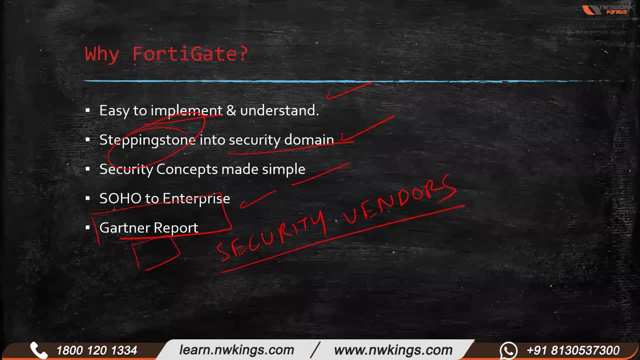 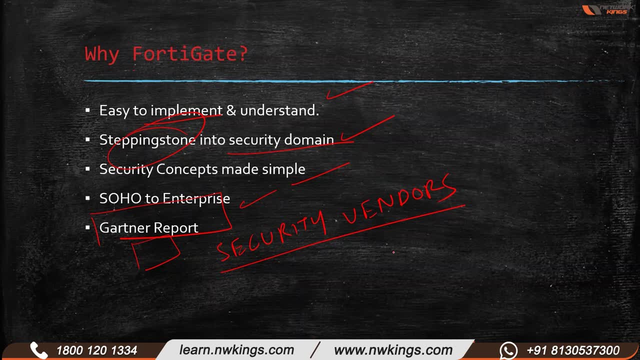 market and how are they performing in the market? okay, so this is what the garden report is. it is an organization, it is an entity, okay, which basically ranks these security vendors: palo, alto, checkpoint, fortnite, sonic, pulse, cyber rom, cisco, uh, you name it, f5 load balancer, whatever it is. so all these uh vendors are being dated, okay. 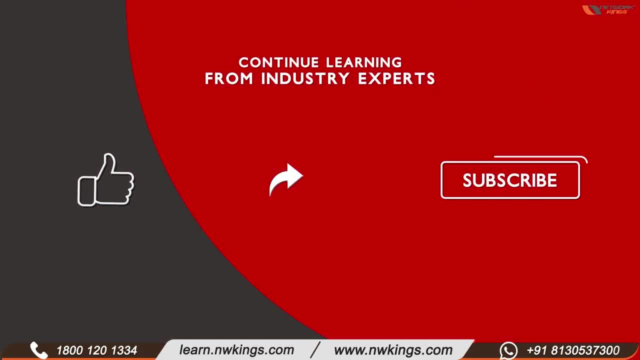 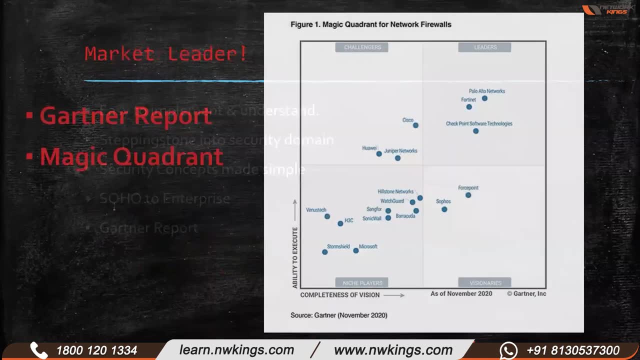 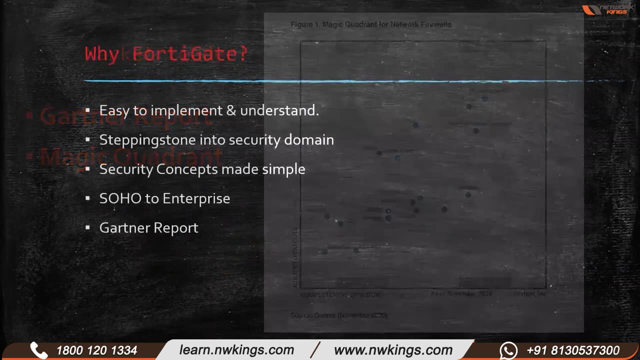 all, right now let's do hi. you are watching the recording from one of our live session. hit like share and subscribe for more future updates. one thing, let's- let's go ahead and show you. this is what is called as the gardener report. i'll go ahead and, you know, show this on the actual 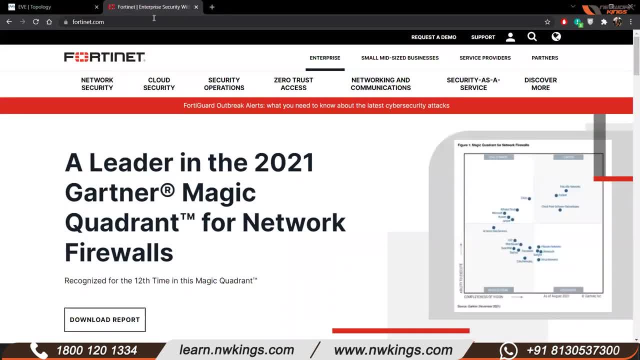 browser. okay, what you can do is do do this today. open up your browser, go ahead, search for fortnitecom. okay, this is the first page that you will get, and the first page is, say: the leader in the 2021 gardener's magic quadrant. so we, the gartner uh report is basically uh released every. 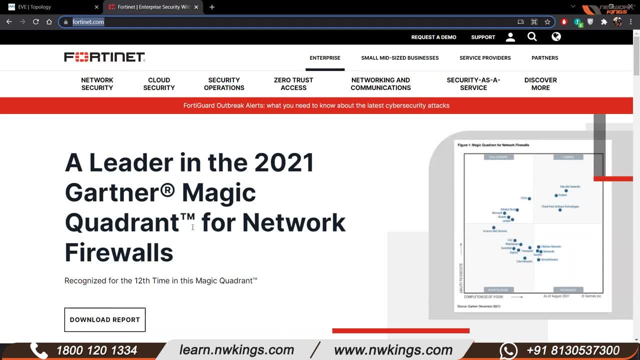 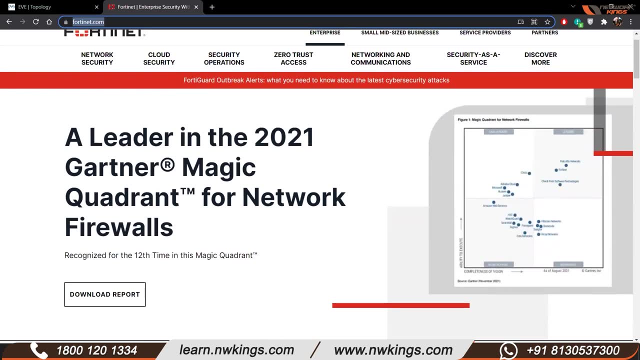 year. okay, by the time of october, november, and they rank all the kind of um, you know, firewall vendors and all the security vendors that they have. okay, so look over here, this is the gartner report. okay, now this is the 2021. let me show you if i can. 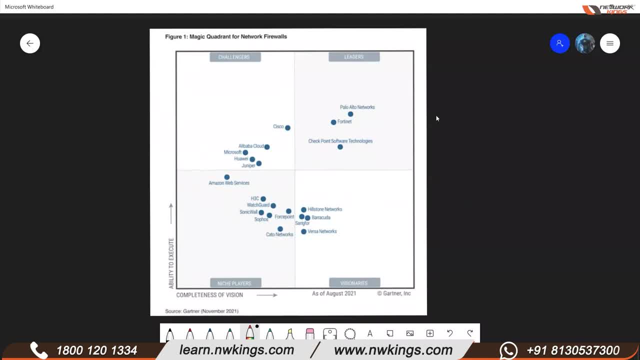 yes, are you able to see this? all of you? yes, no, maybe, okay, all right, good, see. now over here, what we are trying to talk is that. see, there is. this is called as the gardener report. okay, now gartner report has something which is called as the ability to. 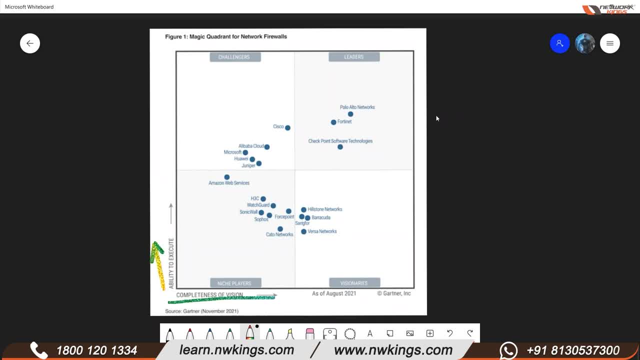 execute. and then you have something which is called as the competency of vision. right, all, if you are able to see the screen, no problem with the scene. yes, chat. your wav basically means is that, whatever company that you are, whatever company that we have over here on the market, how quickly they are able to take decisions? okay. 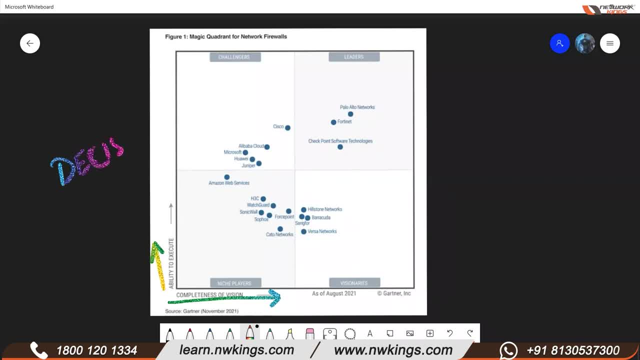 okay. completeness of vision: so vision is basically their target plan. okay, maybe for the next 10 years or 20 years? okay, 10 to 20 years, all right now. what happened is that? the decisions, how quickly they take the decisions and what is their plan? okay, so this. 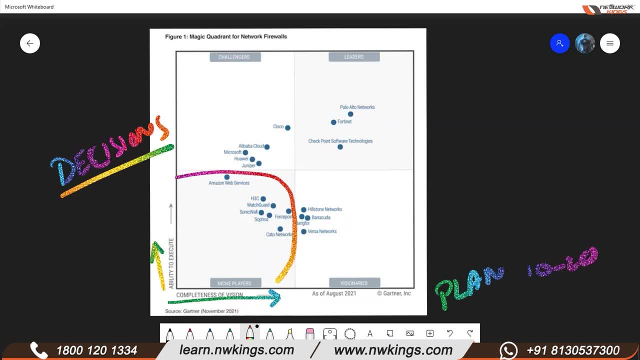 segment is basically people who are, you know, these are called niche players. niche players basically means that they do not have a great vision for the next 20 years, or maybe 30 years, okay, but they know what is required right now- okay, and they're able to do that as well. so whatever is required- right. 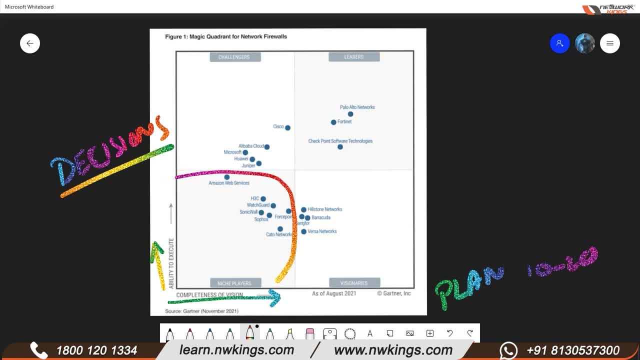 now in the market. they are able to provide that. okay. good, bad doesn't matter, but they're able to provide that. okay. this is one. second is called as the visionaries. now, visionaries basically means that they do have a great plan for the next coming 20 to 30 years. okay, but their ability. 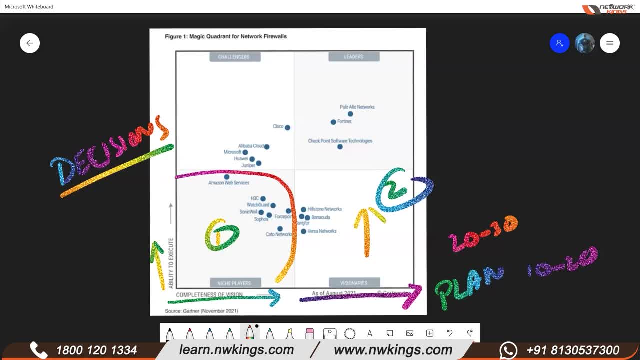 to execute is not that effective. okay, so they are good. what they need to do in the next 10, 20 years, 30 years, great, but they are not able to execute it fast enough to get to that particular plan that they have. so versa networks, barracuda, these kind of vendors- 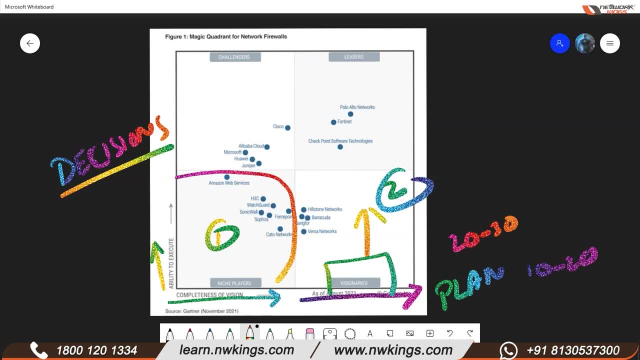 are come under the category of visionaries. all right, so there's a second. now we have some third, which is called as the challengers. challengers are people who have great executionary powers. great executionary powers, they, they, um, they might not have, you know, plans for 20 years, 30 years. 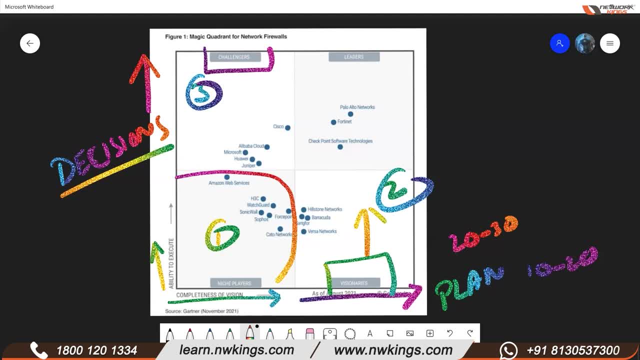 but whatever is required right now in the market, they are able to perform that, they are able to execute, they are able to provide that information or they are able to provide that services or features right now. so they are able to execute that information or they are able to provide that. 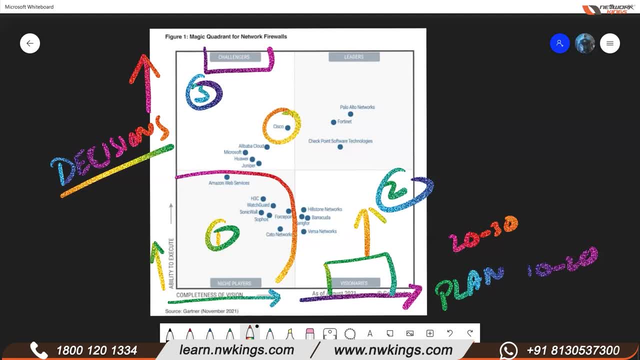 services right now, cisco, one of the people's, one of the challengers. okay, uh, juniper one of the challengers. it's basically sliding, i don't know. um, if you look into the last three years or four years- i've gotten a report- you will see that the juniper was basically one of one time it was a. 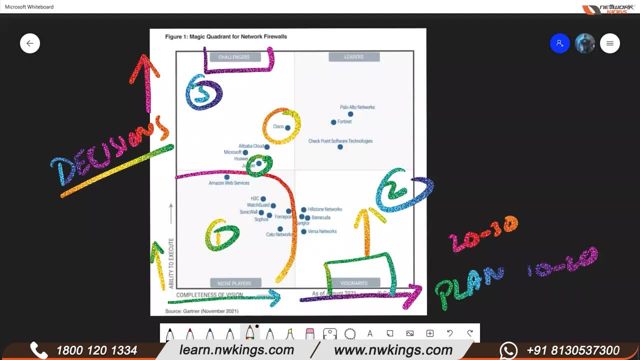 leader, but now it is slipping down to the challenger section. huawei, microsoft, alibaba- these are all challengers. great executionary powers- um, they are able to execute whatever is required right now. then you have something which is called as the fourth one, which is the leader section. now, leader section basically means great vision, great. 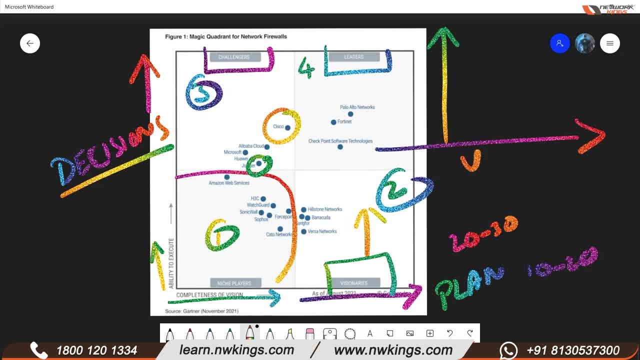 executionary powers okay, so they exactly know what they need to do in the next 20 years and 30 years, and their executionary powers is also impeccable so they are able to execute whatever is required right now plus what is required in the next come, you know, coming 10 years, coming 20 years. 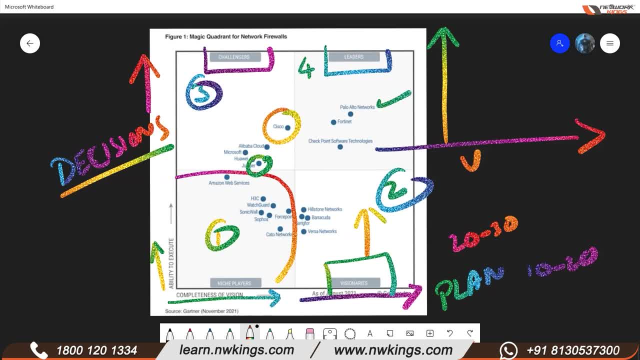 over here we have palo alto one number, then we have fortinet second number, and then we have, and then we have fortinet second number, and then we have fortinet second number, and then we have checkpoint and i don't know again. uh, they are sliding from the last couple of years, they are. 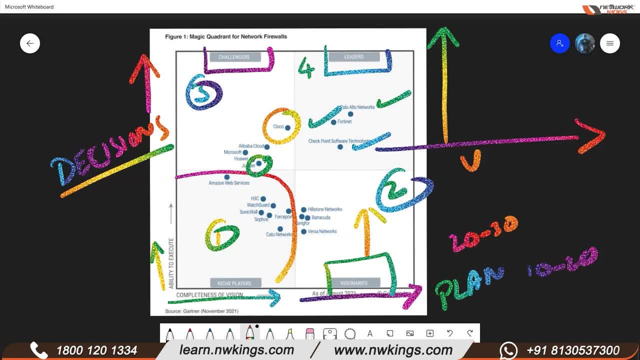 sliding down. um, not sure why, but anyways. parallel is at the top, a little beneath fortinet, and then we have checkpoint. okay, so see, when it comes to the leader quadrant, how many people you see over here. you have three people right. so the advice that i always say, or i always give, is that 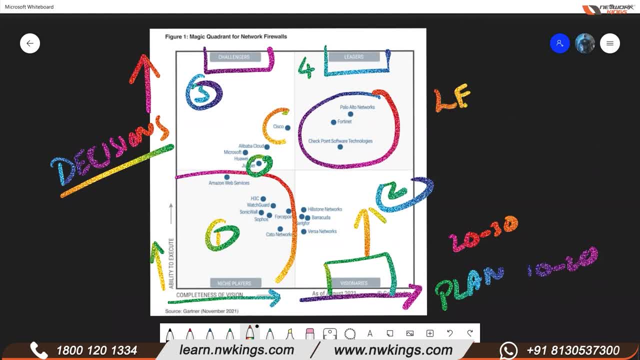 whoever is in the leader quadrant, learn them, because if you learn them you are going to be in the market. you are going to be in demand in the market because, obviously, palo alto is is required, fortinet is required, checkpoint is required. okay now, fortinet basically makes sure that your concepts is easy to understand. so if 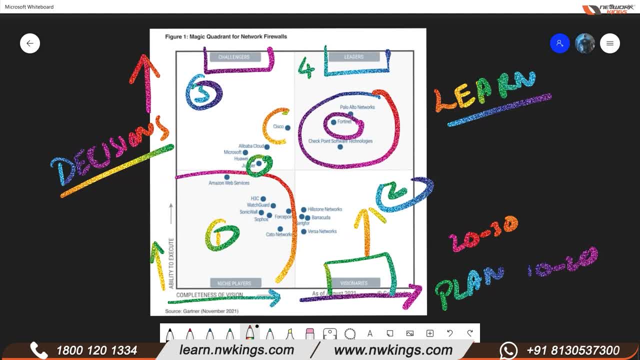 in case you want to move on to the next uh firewall, you can definitely go with the palo alto if you, if you understand fortinet clear enough, you would be able to understand palo alto much more easier if you directly go to that. i'm not saying you will not be able to understand, obviously, but 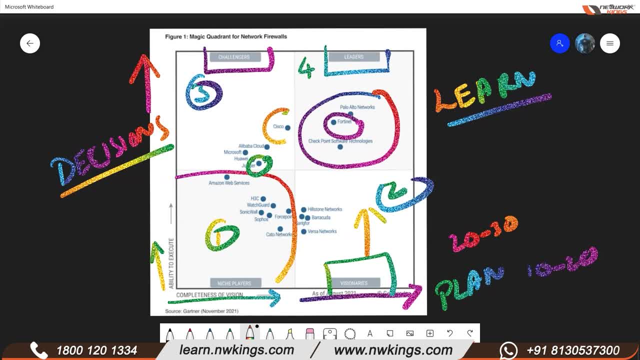 then it's like it's like taking the ccnp directly: okay, it's going to be a little bit tough, but then you will be able to eventually get that. but if you take the ccn and then ccnp, it will be easier for you because you already know the concepts. right, that is what it is, okay. so let me go ahead and 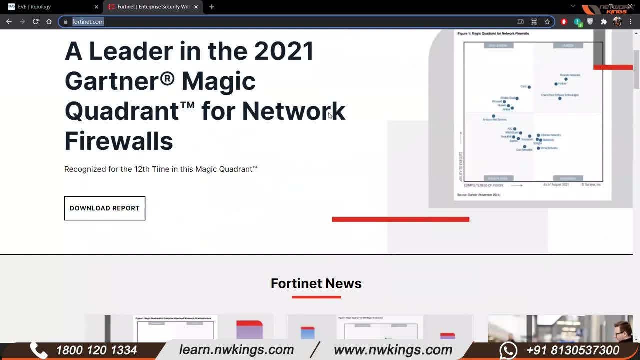 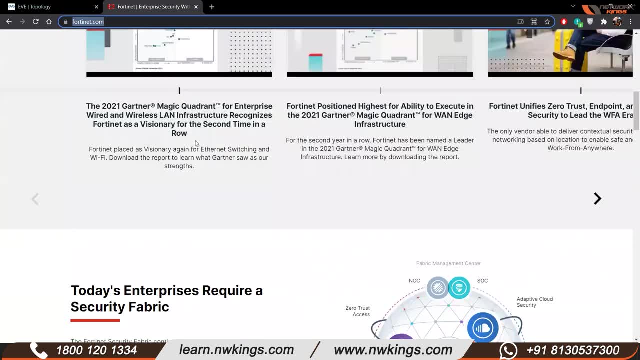 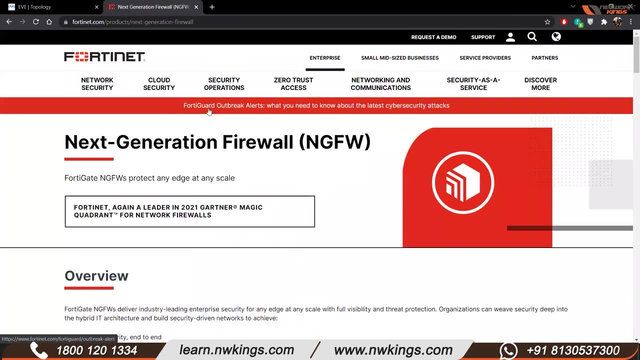 quickly show you a couple of uh fortinet products that we have. okay, so what you can do is we'll go into the network security next generation firewall. okay, just to give you an idea of what exactly fortinet is, what is fortigate, how may how the products look like? okay, see models and. 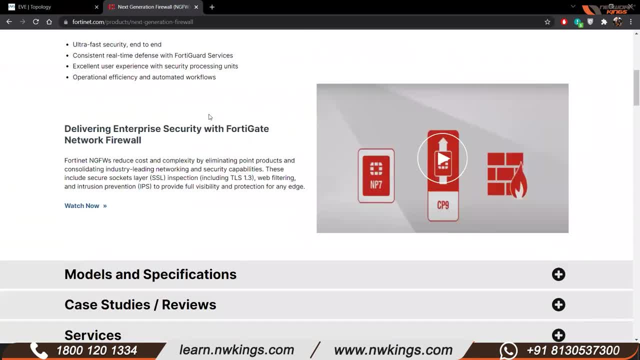 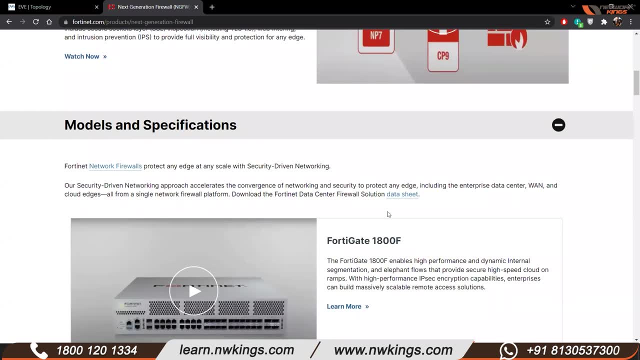 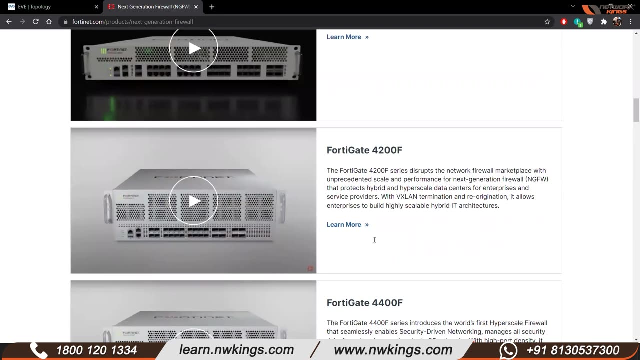 specifications. we click on this. okay, now 1800. so 1800 is like um is a high-end for to get firewall. twenty, six hundred, forty two hundred- these are all higher- and thousand cities or four thousand series of five thousand series are basically a high-end fortigate firewalls okay. 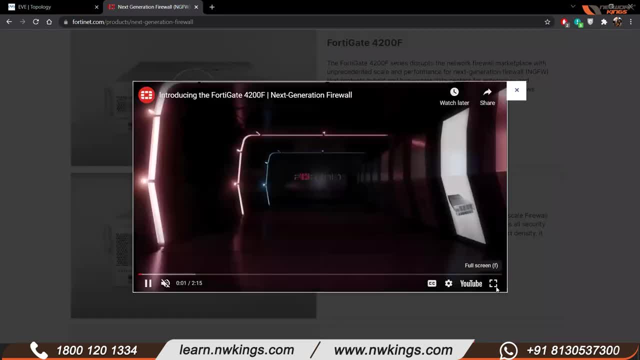 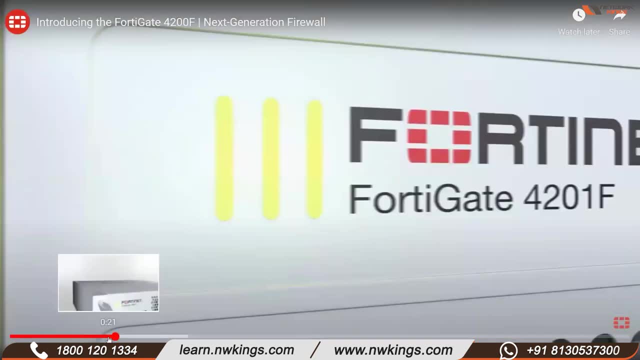 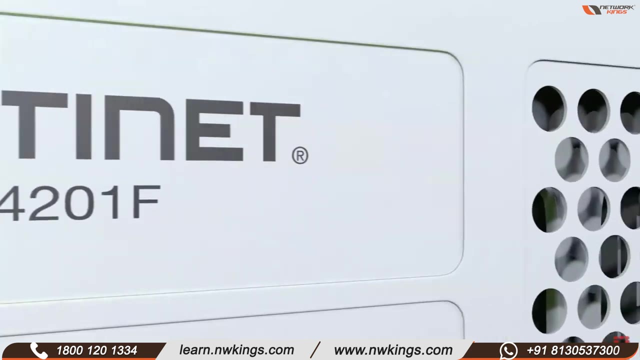 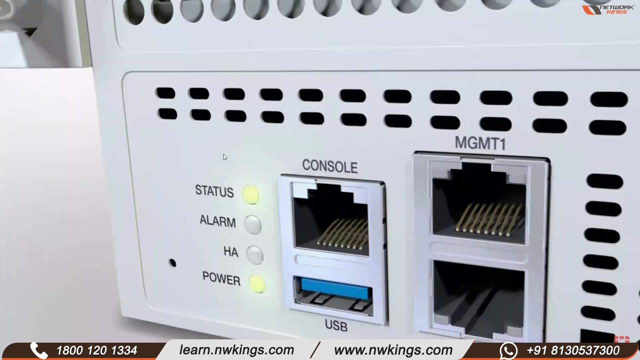 let's just take one of them, okay, okay, so this is fortinet 48 4201 f model. okay, this is a very higher and not very, but higher end for the gate firewall. okay, now see over here, you can very well see that the- uh, you have a console, you. 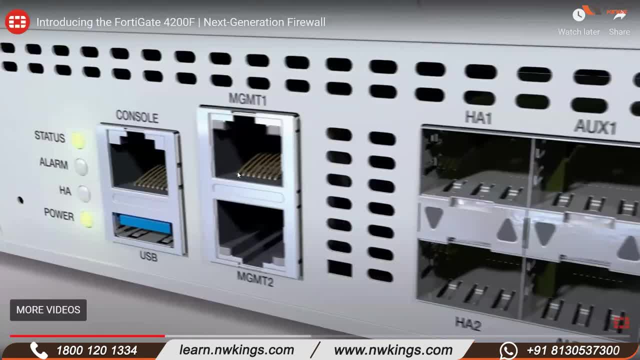 have a usb, you have two management interfaces. okay, now, these two management interfaces is basically: if you want to connect, or if you want to directly connect to the management of the 40 gate firewall, you can use the rj45 cable to do that. okay, then you have something which is called: 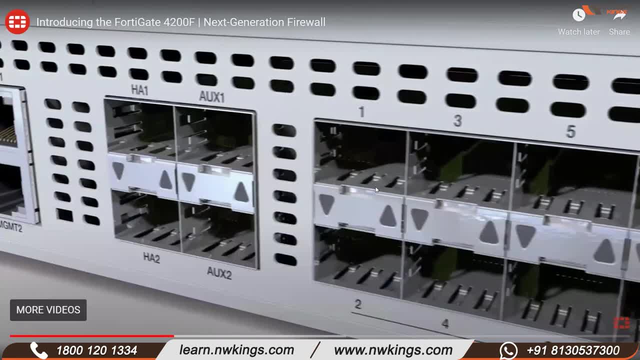 as the ha cable. you have ha1, ha2, then you have aux1 and aux2. aux1- aux1 is also called as auxiliary. auxiliary is just like an alternate of your console. if in case console goes bad, if the console is not available, you can use the auxiliary. it's more or less the same, okay. 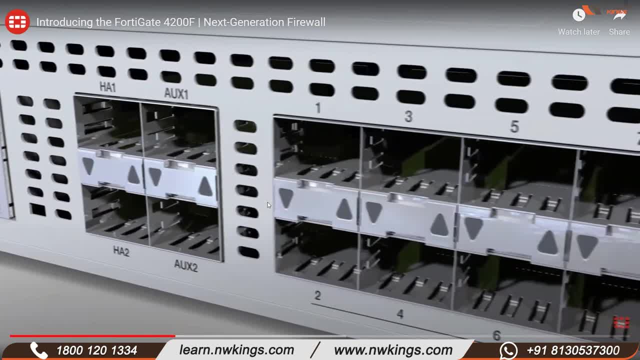 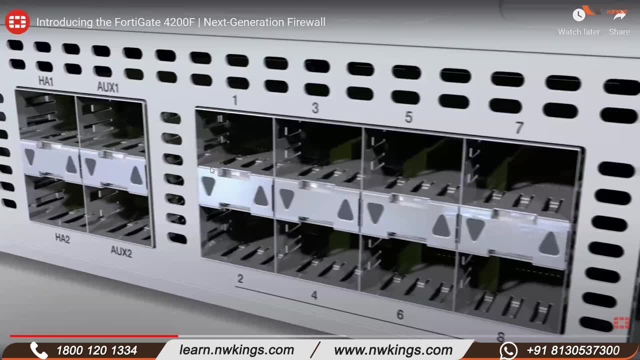 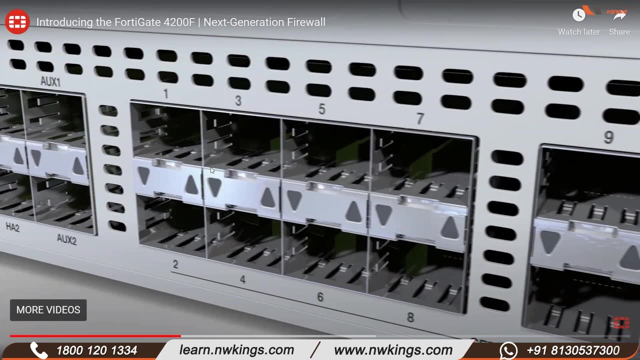 it is. have you guys noticed one thing, don't you? don't you feel this port's a little bit different? they do not look like a rj45 connector, right? what? what is this? anybody any guesses? what? what do you think? this is? a joy is always, you know, the first one to you know. type in good. 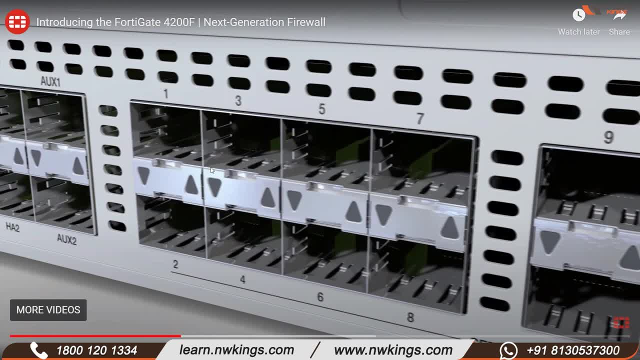 good is always the second one, and then we have rajneesh- okay, great. so these are all called as sfp ports. what is sfp? what is sfp? gordon says fiber, good, what is sfp? can anybody give me a full name, full form of sfp? come on, joy, can you? what is the full form of sfp? anybody in the youtube guys? 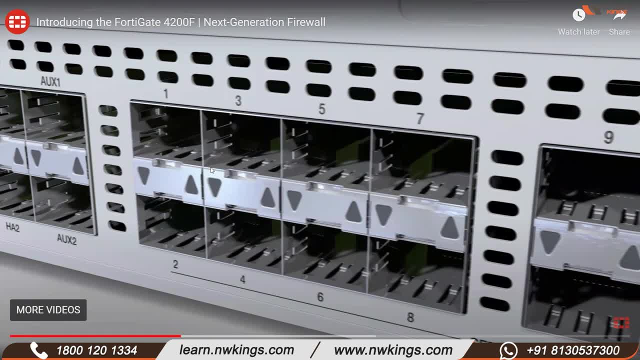 ashwat. what is sfp smithy? what is an sfp port? what? what is the full form of sfp port? any ideas? no problem, okay, all right. see, uh, sfp is called as small form factor portable. okay, small form factor portable, that is? um, no, it is not switch fabric port, smithy, it's small form factor. 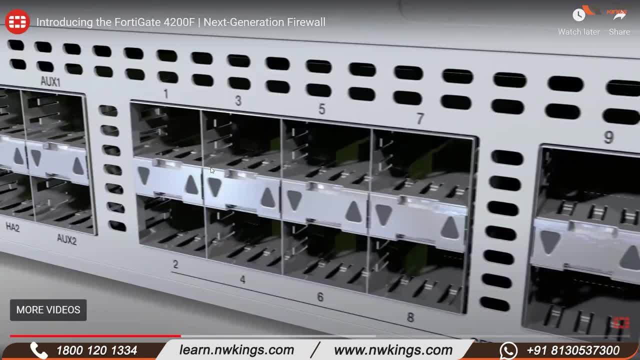 okay, uh, pluggable is also: uh, that is p is for pluggable, okay, um, okay. so these are basically. so what happens is rj45 or ethernet cabling goes still for one gig, okay. but sfp's or fiber starts from one gig, they go till 10 gig, they go over and above till 40 gig. okay, you can do that. 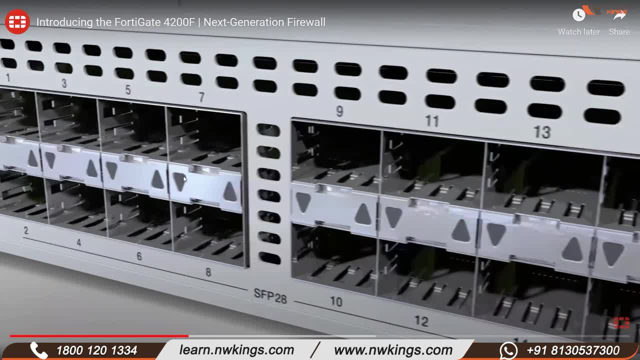 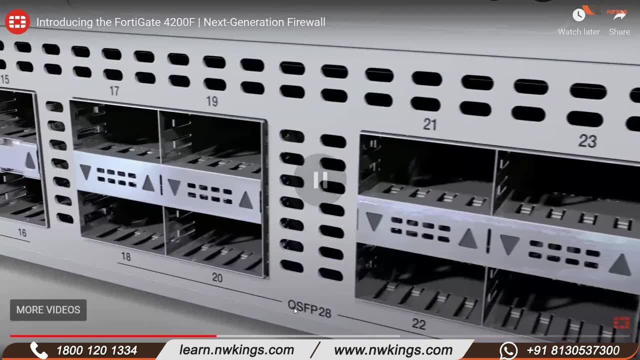 so that is what these ports are. we'll talk about this in great details so you can see till 16. you have these ports, then you have 17 and 18, which is: see again. do you see this qsfp? this is what i'm talking about. these are 10 gigs and 40 gigs. okay. 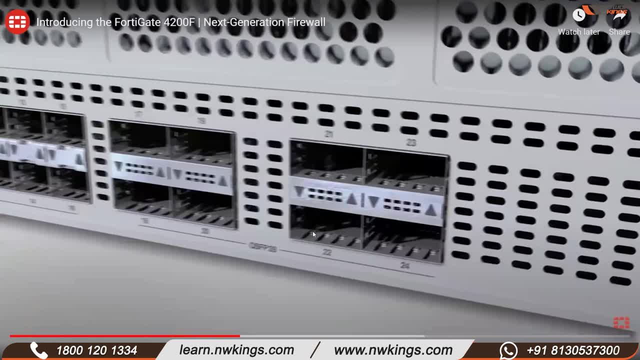 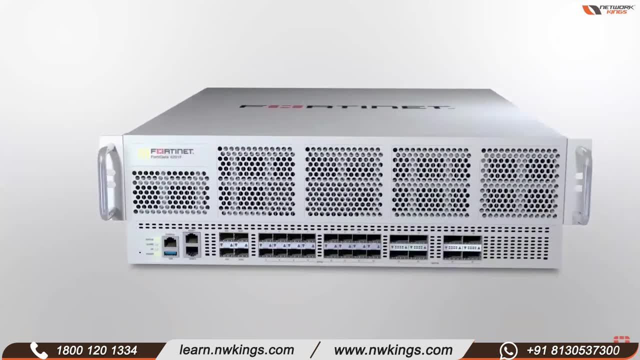 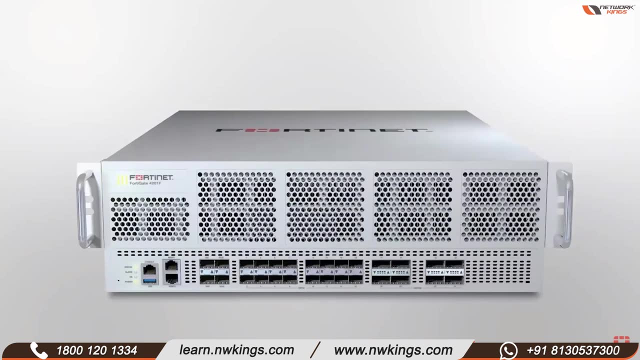 higher end, where you can basically have one cable which can be used for 40 gig of data coming in and out. that is what it is. okay, this is called as 4200 series for to get firewall. let's do one thing: let's get inside this 48 firewall and see what do we have inside this whole covering. okay, so let's. 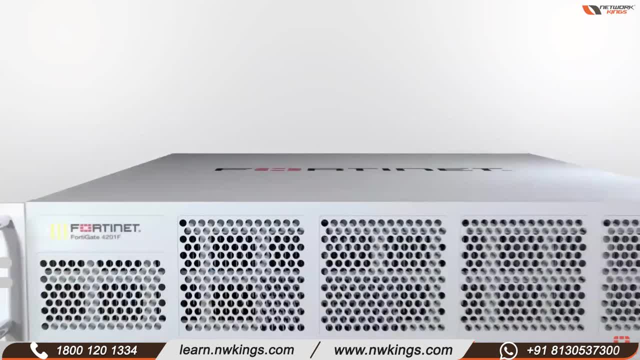 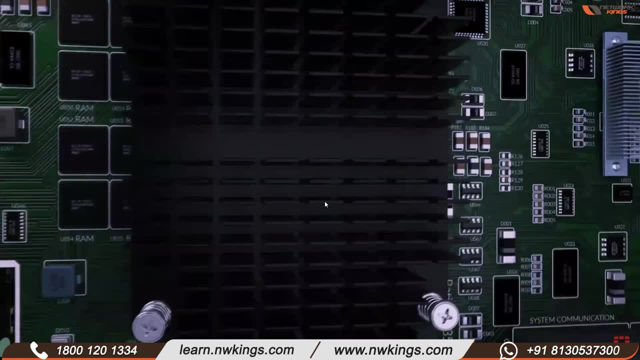 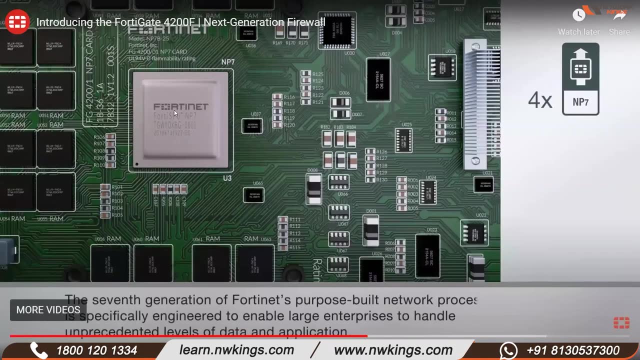 get in. okay, all right, so now over here we'll see information or we'll basically look into the- uh, the hardware chips that we have. okay, now let's let's have a look over here. do you see this fortinet? it says the chip that you have, the cpu chip. what is this? called as 40 spu. 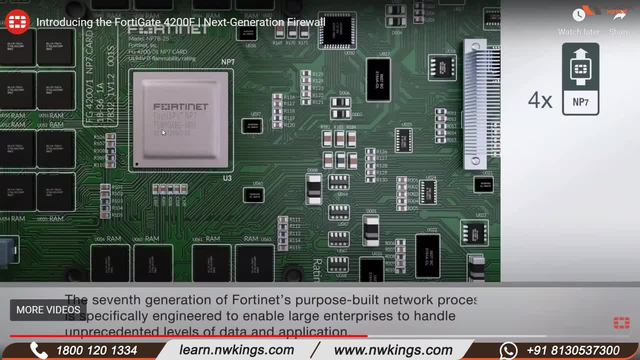 now 40 spu is basically these are called hardware chips. okay, these are called as 40 a6. okay, what is 40 asic? 40 asic are basically hardware chips which is installed, apart from um, you know, cpu and and your memory. why do we need that? see what happens is fortnite came uh with this idea. 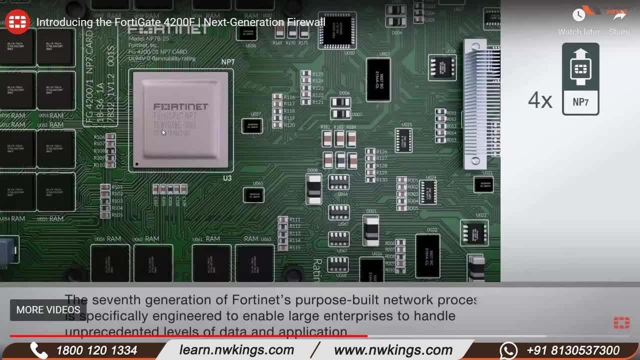 that if we have dedicated chips, okay, which would be able to handle the traffic, then my cpu and memory will be free to take up the new uh session which is coming in, okay. so what? the cpu and memory? what it does in the photogate firewall is that whatever kind of traffic comes in, first of all. 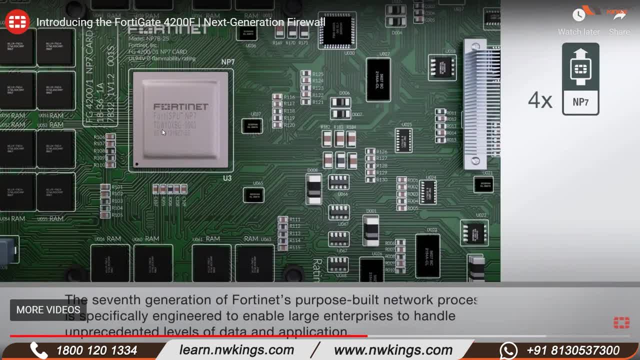 the first packet always goes to the cpu. that is, that is how it is designed. the first packet always goes to the cpu. cpu then decides whether do i have to send this traffic to whatever um hardware chip that i have, or do i have to process it again? okay, see, do you see this np7 right top. 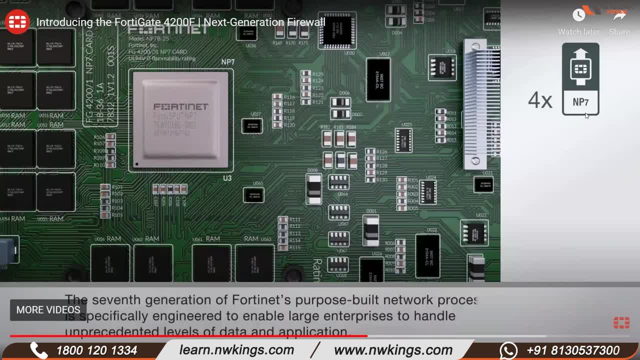 corner 4x into 4x np7. what do you do? you know what this is. see, np7 is like is the full form, is basically called as network processor. now, network processor, as the name goes, or as the name suggests all the traffic which is more or less dedicated to a network layer of the osi module. okay, now can anybody 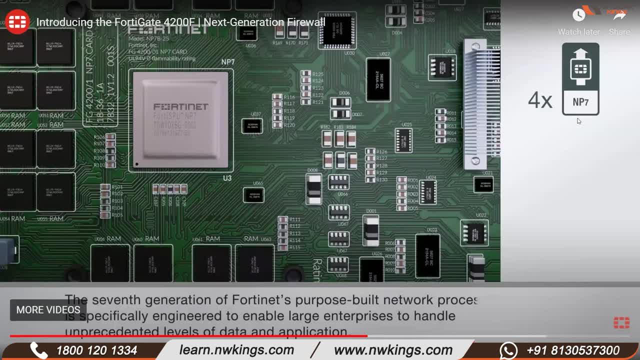 give me an example, any, any protocol or any traffic which is dedicated to network layer only. yeah, sorry, rejani says ip, sanchet says icmp konal, icmp sanche, ospr. good example, okay, i'm gonna say, sir, repeat the question. okay, uh, one of the question is that at network layer, 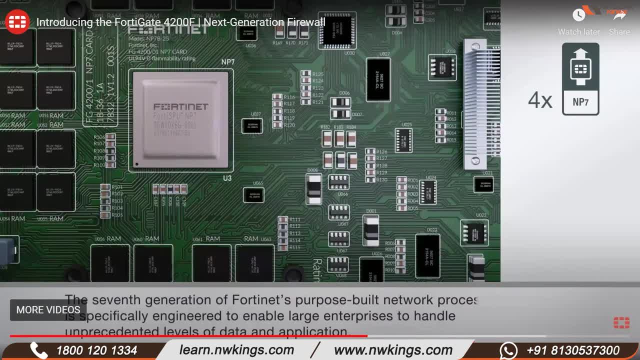 can you name any protocol which is used only on network layer? nowhere else. pratik says: ip, fruity, ip okay, But anything else apart from IP, okay. Guys, you are, you are, you are forgetting man. VPN also has something. VPN packets also exist. 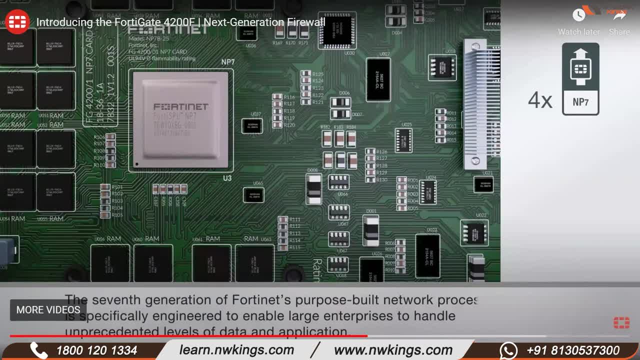 NAT also exists, right, But NAT is again it's not. it's not a protocol, right, IPsec okay. So again, my point over here is that all the traffic which is dedicated to the network layer, okay. 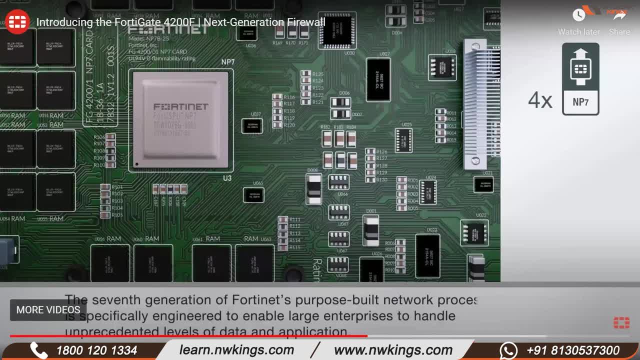 OSPF, BGP, IPsec, VPN, ICMP. okay, these things are basically handled by your network processors. Okay, Then we have something which is called as the CP. CP is called as content processor. okay, See, we'll talk about something which is called, as you know, content inspection, security inspection tomorrow. okay, 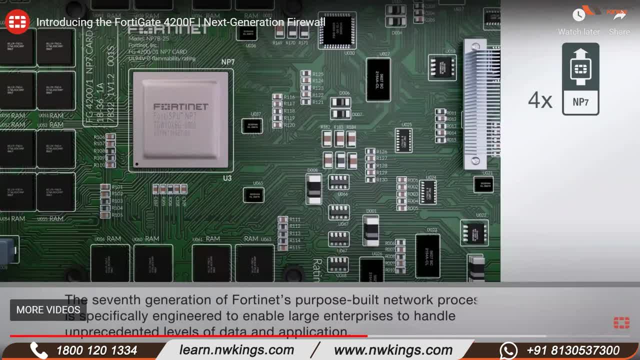 We'll talk about UTM, We'll talk about antivirus, We'll talk about IPS application control. okay, These are all. things are called a security inspection. Just to give you a layman example: all of you guys have a laptop, right? 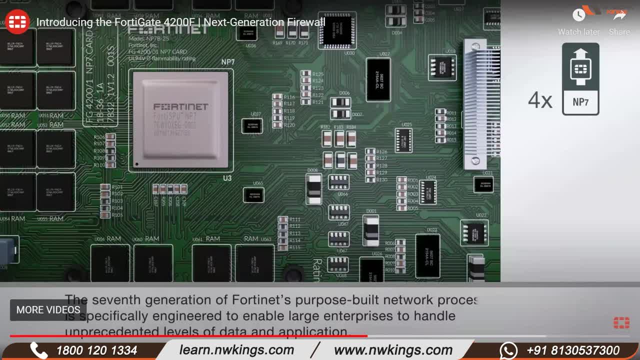 Yes, no, All of you guys have a laptop. All of you guys have a laptop. All of you guys have a laptop. All of you have an antivirus on your machine, right? All of you guys have an antivirus, right? Even if it's Windows Defender, all of you guys have an antivirus, right. 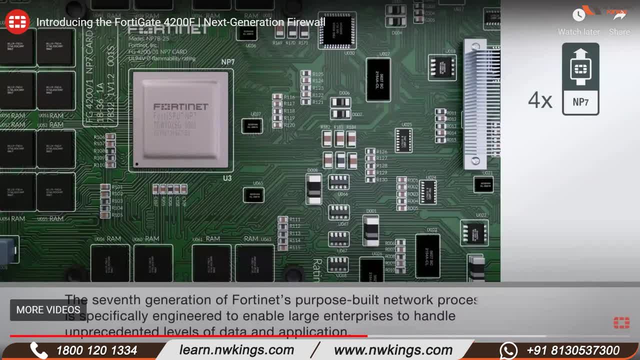 Windows Defender is also updated. Why does it update itself? To ensure that, whatever viruses are on the internet, your system is basically safe from them. That is why you update your antivirus right. So that has also happened on the firewall as well. 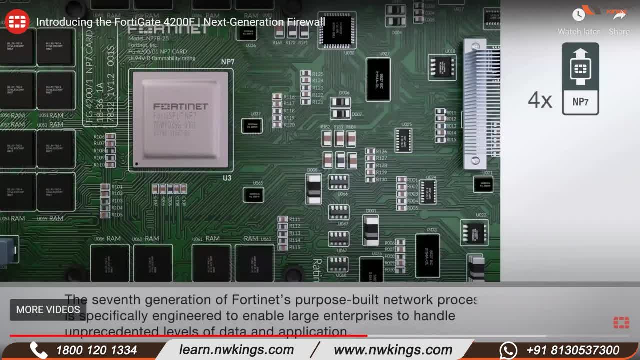 Any firewall at all. it also has antivirus. It also has IPS. It also has webcams. It also has web content filtering. okay, What all these things are. This is all security concerns, security features. okay, So anything which is dealing with the security inspection, security features of the traffic. 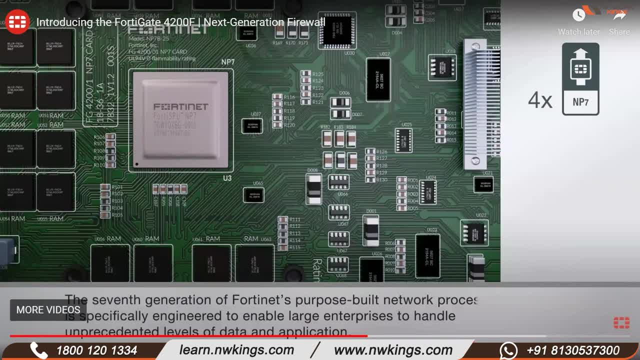 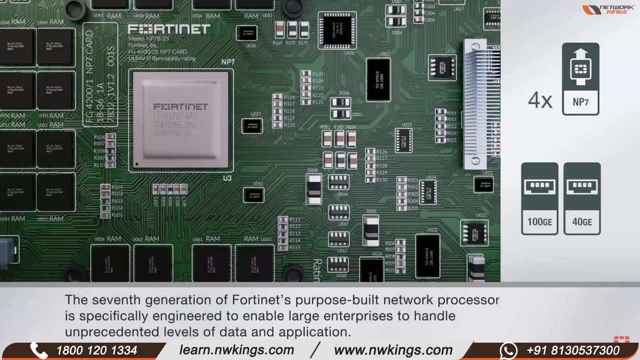 that is being handled by a hardware chip which is called as CP content processor. So let me unpause this. I hope this should tell that as well. Okay, Does it show about the CP? Yes, that is what I'm talking about. 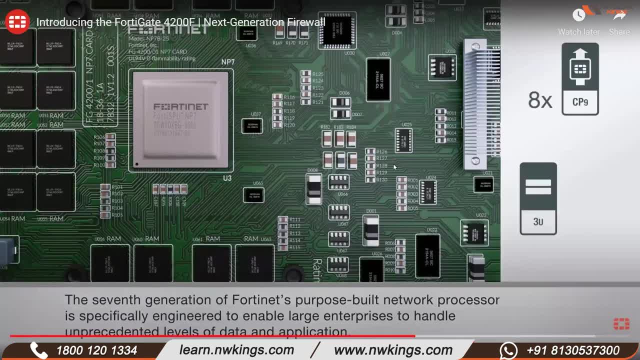 Okay, Does it show about the CP? Yes, that is what I'm talking about. Yes, that is what I'm talking about. CP. So A-Tech CP. So A-Tech CP is basically saying it has 8 hardware chips of CP. 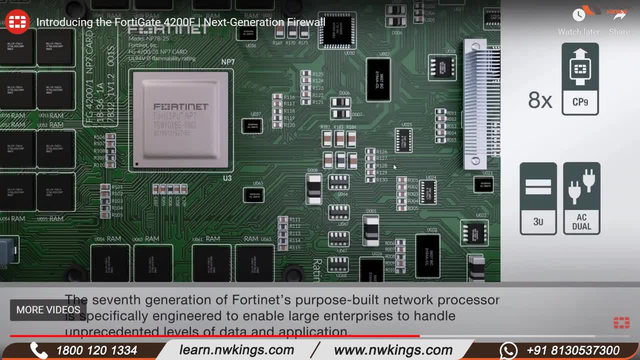 Now, what is CP9?? 9 is the level, So basically it starts off from CP1.. 2, 3, 4, 5, 6,, 7,, 8,, 9.. So if you have a smaller hardware, you'll have a smaller CP. 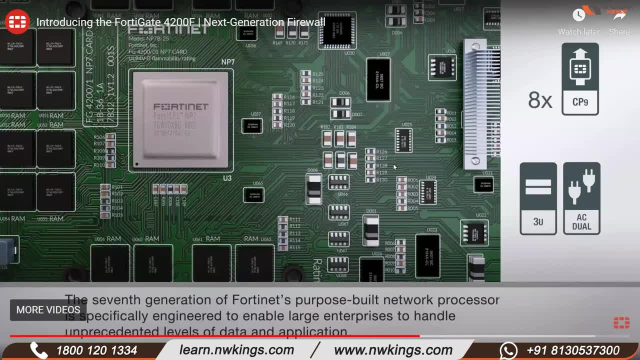 If you have a bigger hardware, you'll have a bigger hardware, CP. okay. So bigger hardware, have a CP9.. Smaller hardware may have 3,, CP3 or CP5.. But it also tells. It also tells you how many CP, how many content processor it has. 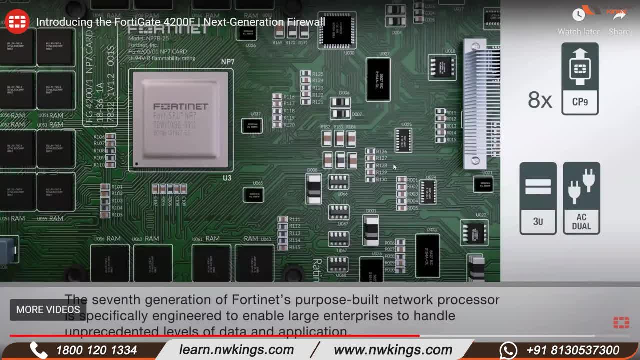 So you have 8 hardware chips which is being called as content processors. They are called as content processors 9, which is the latest one. okay, So all kind of inspection, all kind of security inspection which happens, content processor looks into that. 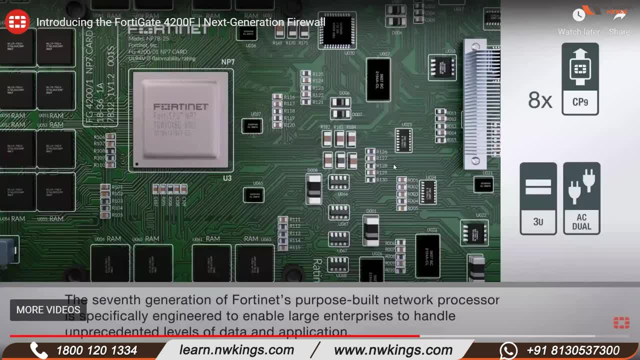 Okay, Now is it so clear: If someone will talk about network processor, you won't be able to tell him what is a network processor. If someone will ask you what is a content processor, you won't be able to tell him. 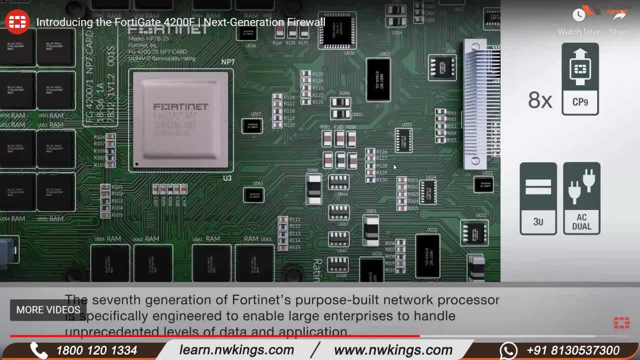 Yes or no? Yes or no, Would you be able to tell what is an NPO, What is an NPO CP? Would you be able to tell that much? At least nothing in one-liner. Yes, Good, Okay. 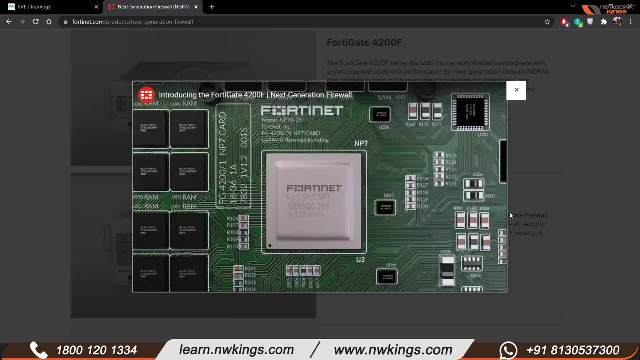 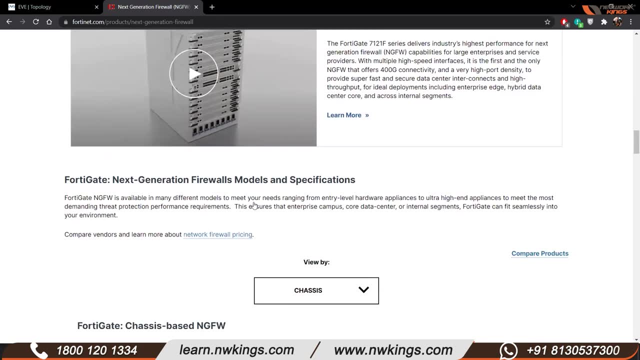 All right, So let me go ahead and exit this. Okay, See, so these are the files. okay, So 7000 series again. this is a huge, huge firewall. This is for ISP level, you know, ATLG or whatever it is, whatever company that you are working with. 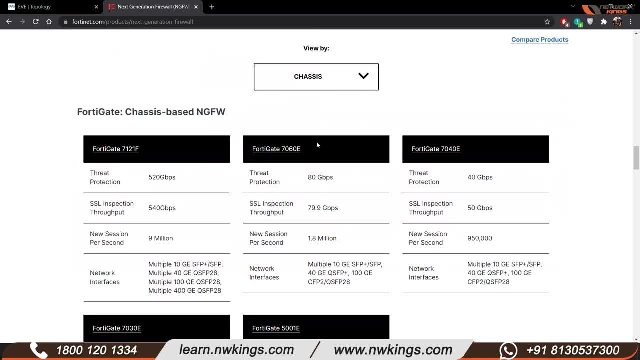 Okay, If you won't look into this, What you can do is you can go over here, you can select chassis, then you have the ultra high-end, then you have the high-end. So see, as of now, it is chassis. 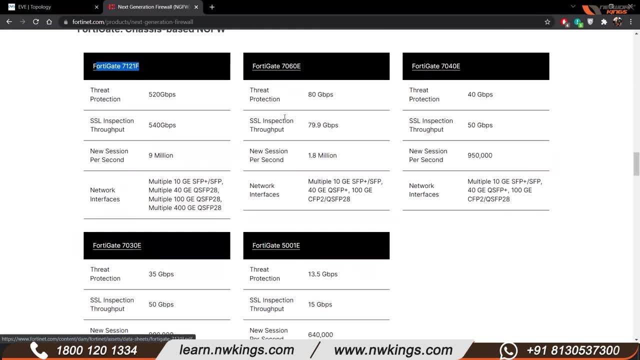 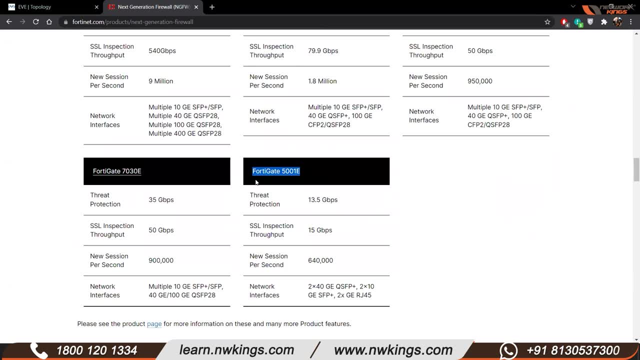 So what series you are getting? FortiGate 7000 series, FortiGate 5000 series. So I have this okay In my environment. I work on the 5000 series model. okay, Now I basically make sure that I, you know, handle traffic coming from Jammu Kashmir till Kanyakumari. 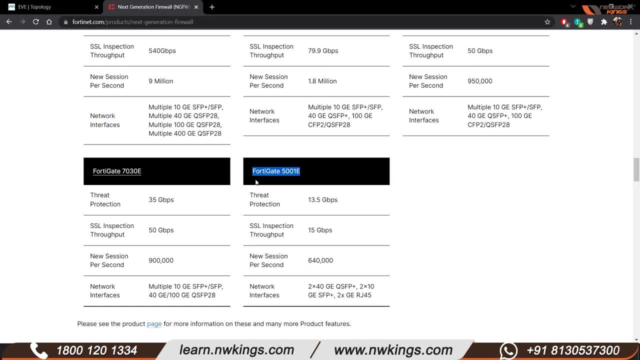 So all kinds of traffic. I have around 80 firewalls and all the other kind of devices as well. They are all in a centralized infrastructure and there are a couple of devices which is in a decentralized infrastructure. So I take care of all those guys. 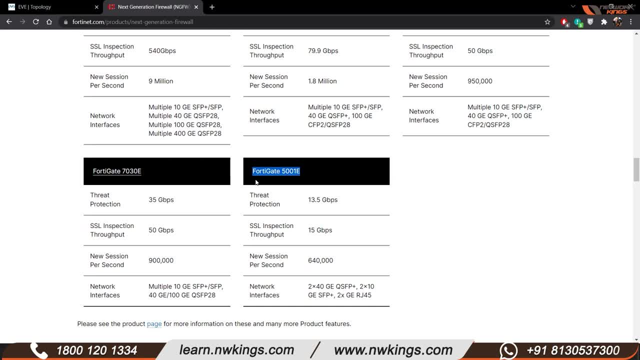 My point over here is that you should know the concepts in a way so that, even if the network is huge, you should not be able to, You should not panic and you should not be able to, you know- get into a place where you do not know what you need to do. 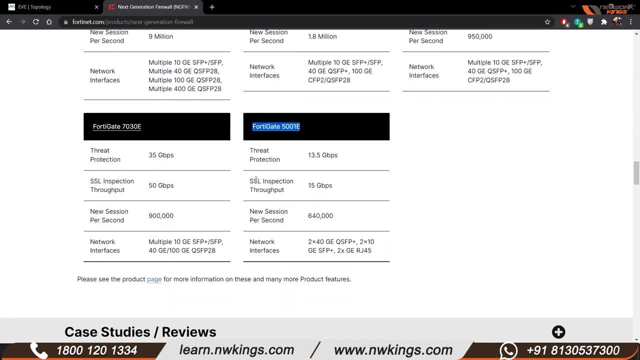 Okay, So FortiGate- FortiGate Basically gives you that space where you will be able to understand. See, the good thing is that once you understand the operating system of your FortiGate firewall, it does not matter what FortiGate model that you are using. 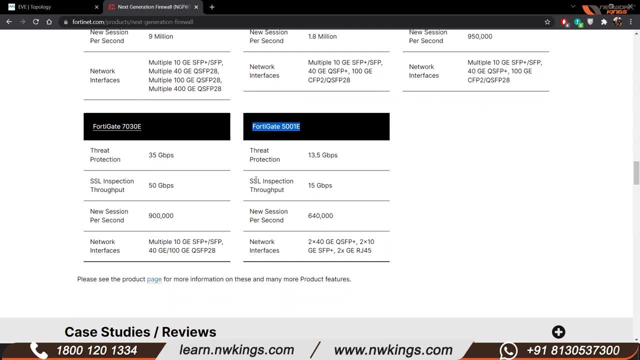 Smaller FortiGate firewall- no problem. Higher FortiGate model- no problem. Why? Because you know the operating system. See, I will tell you what. All of you guys have Windows 10 in your operating system. Okay, 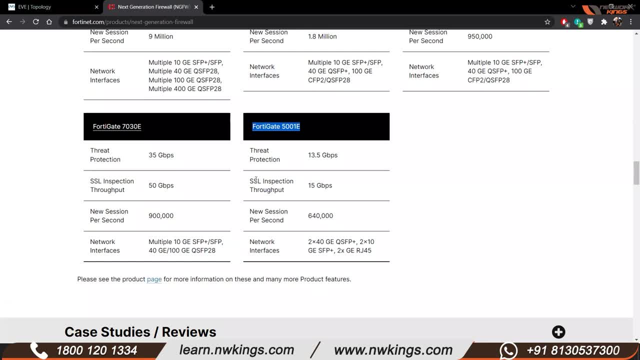 Does everyone have Windows 10 in their laptop, Yes or no? Okay, Now tell me one thing: Does it make a difference whether it is HP's laptop or Lenovo's laptop or Dell's or Sony's? Does it make a difference? 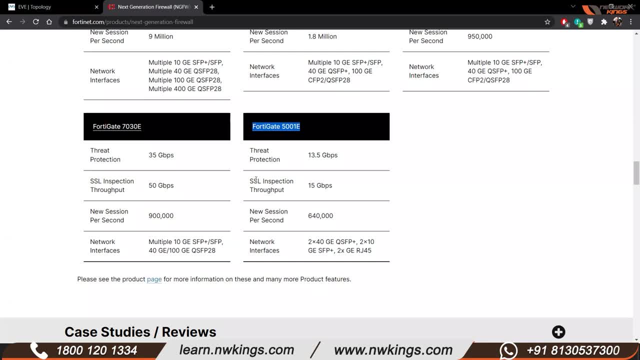 Do you know the operating system or not? When you know the operating system, you will not have to worry about the hardware. Okay, This is what I want to tell you over here: The way we are going to teach you this. this will basically help you to understand the operating system and its features. 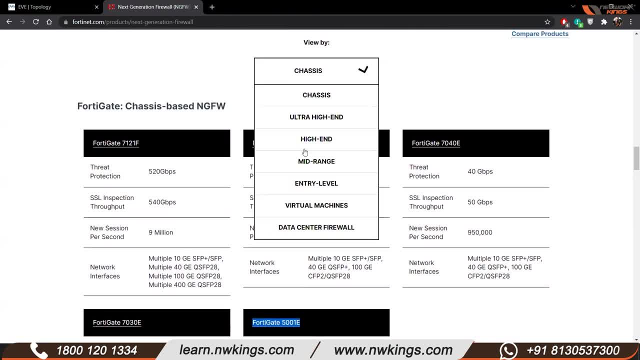 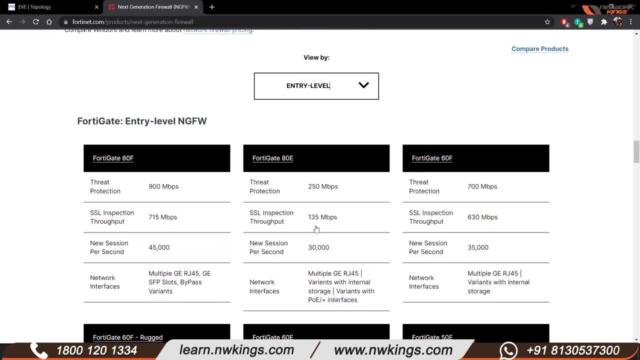 After that, it doesn't matter if you are working on the 5000 series or you are working on the entry-level 60E, It doesn't matter. Okay, So you would be able to cover up all this from the top chassis till entry-level, to the virtual machines. 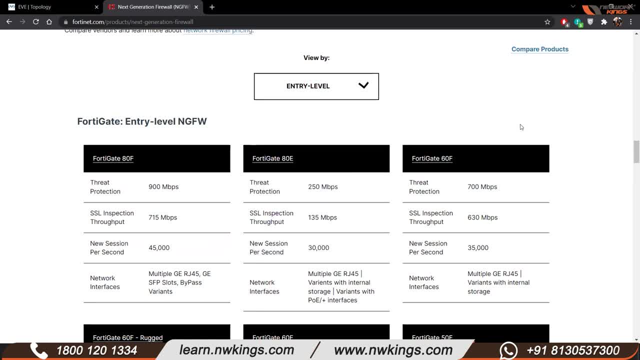 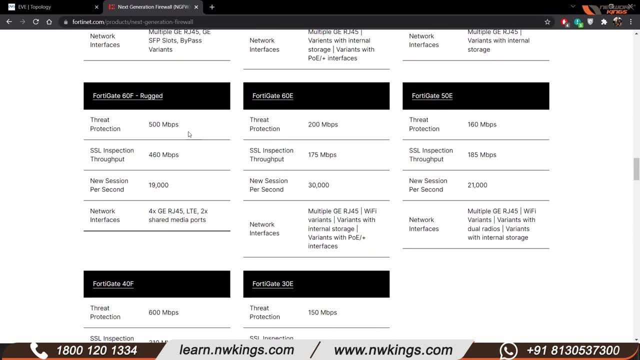 Okay, We are going to tell you the virtual machines as well. So, anyway, it will A to Z. it will be covered for you guys. Okay. So go over here, check out the different kinds of model that you have. how much of the threat protection, the NCCL inspection, all these things. 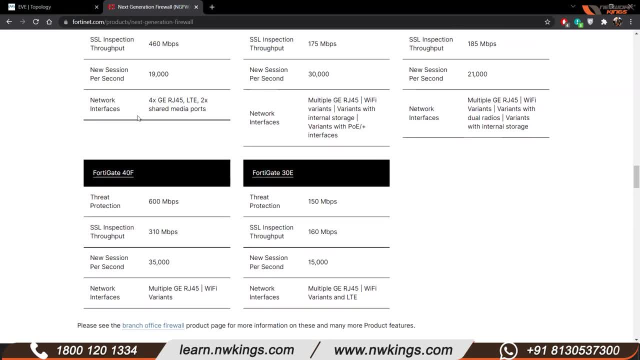 You know what are these things. Okay, do one thing: Go through them and tell me if you are able to understand these terminologies or not. If you are not able to understand these terminologies, We will talk about this again, maybe tomorrow. 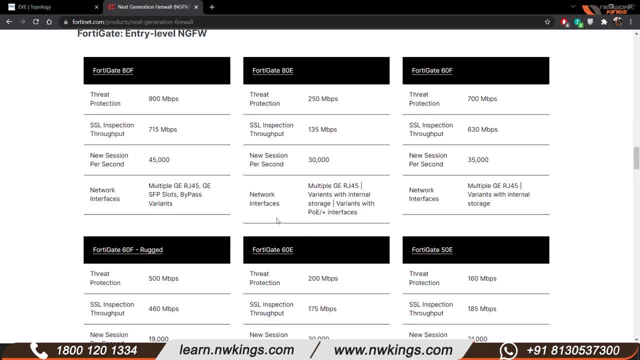 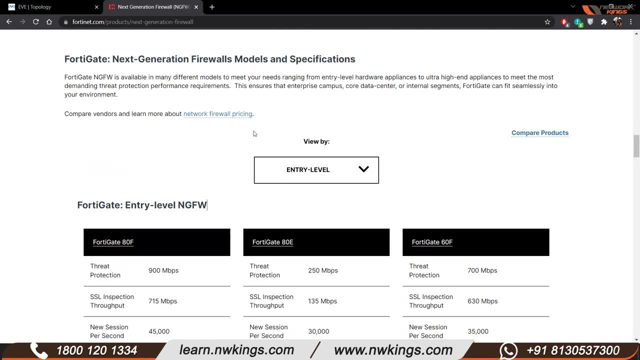 Okay, But I want you guys to question: Okay, Alright, Now next is okay, understood. fine, I went through the course, no problem at all. What about the job? So let's do one thing: Let's go into the nokricom portal. 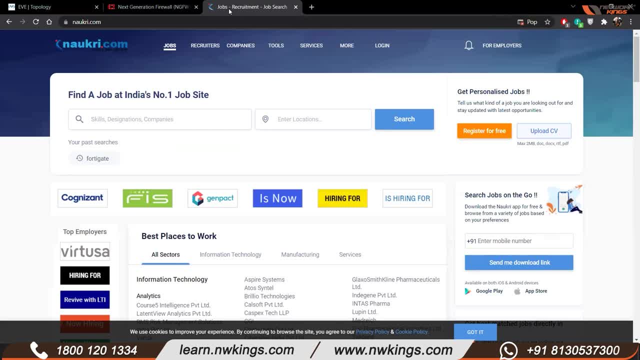 Now nokri is again. it's an Indian portal for all the kind of jobs that you have. Okay, Now, if anybody of you are basically outside the country, whatever job portal, So if anybody of you are outside the country, whatever job portal you have, you can go and search over there as well. 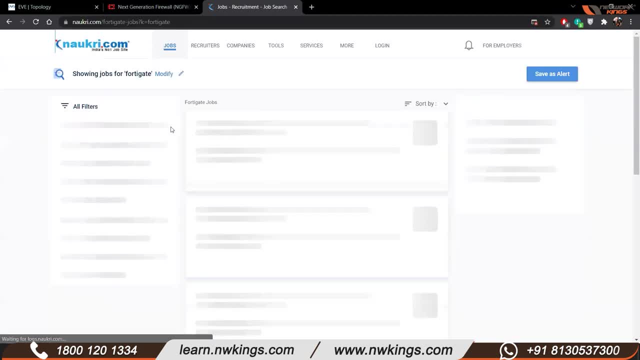 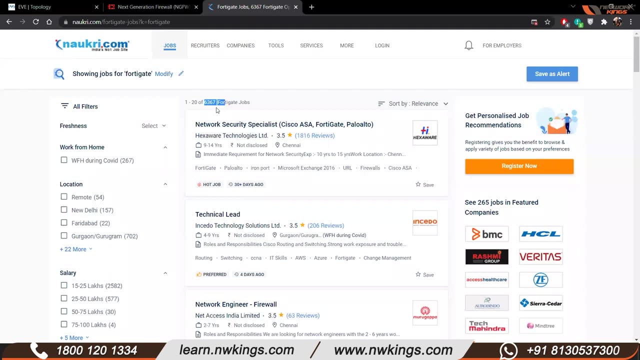 What do you need to search? Simple, Go ahead and type FortiGate Okay. So as of now it says that I have. I mean, over here we have around 6,367 jobs for FortiGate, Okay. 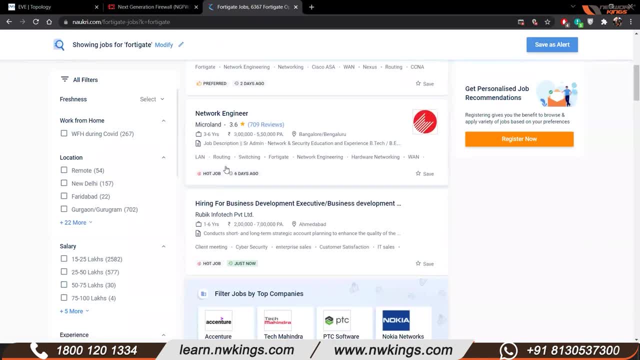 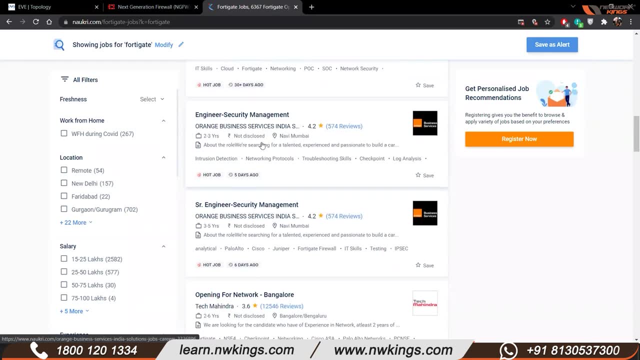 We have Hexaware, we have Indico, NetAxis, Microland, RubikInfoTech- That's a good company to work. FutureNet, NMS, Orange Business Services- That's also a good company to work with. Okay. 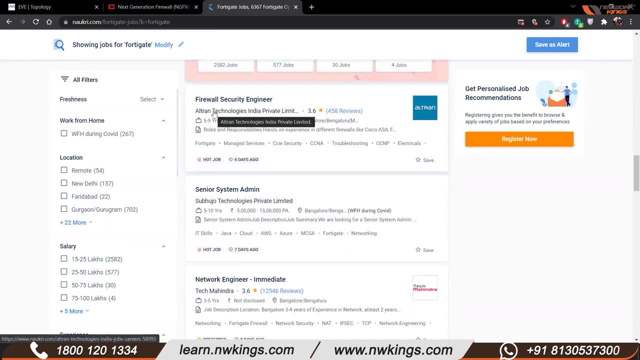 Tech Mahindra: Ultron, Ultron, Ultron, Ultron, Ultron, Ultron is very good if you are basically want to get into the tech field or if you want to go into hardcore. you know technology and networking and security. Ultron is also. 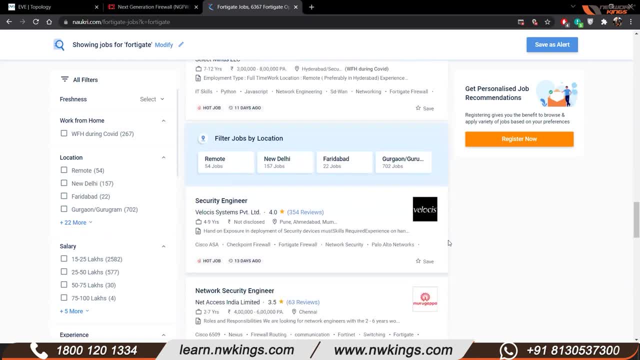 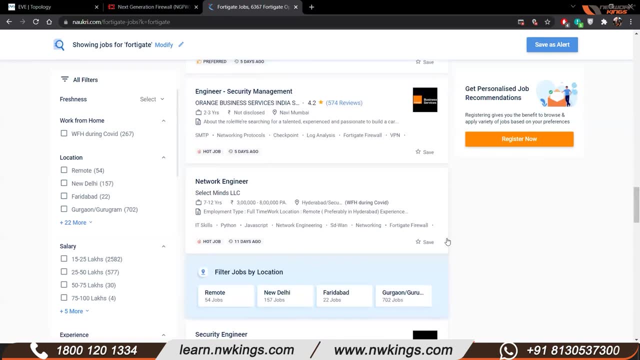 a good place to work with. Okay, My point over here is you have all the kind of job portals which are able to give you that experience which you are able to basically love to work with you, if, in case, you are. 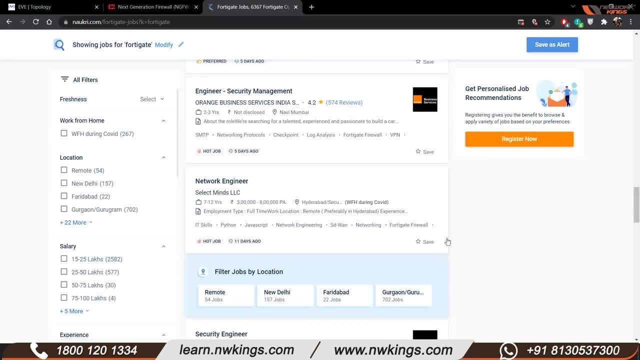 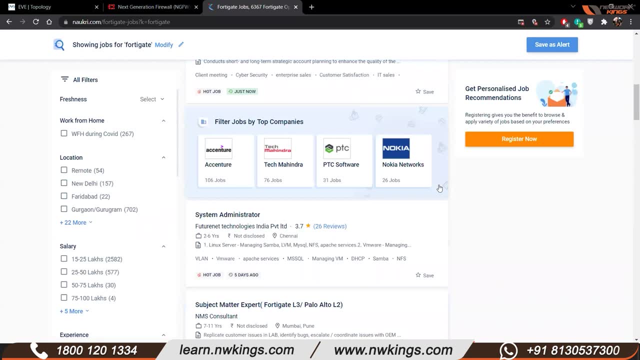 you know, in that company. Okay, So Ashwat says he is already working at Hortense. Great, Okay, All right. So my point over here, It is that there are jobs. You just need to ensure that if you have three years of experience or four years of experience, 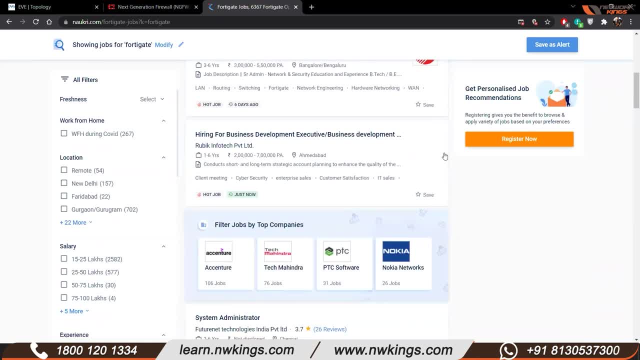 there are so many companies out there who would love to, you know, hire you. if you know the concept, you know fully. Okay, All right. Now what I wanted to tell you about this over here is that, fine, you know that. okay, we have all these things. 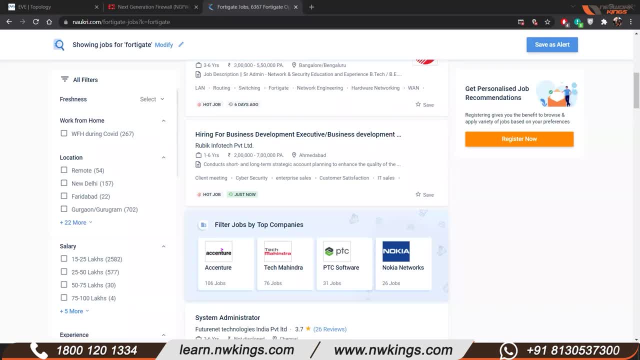 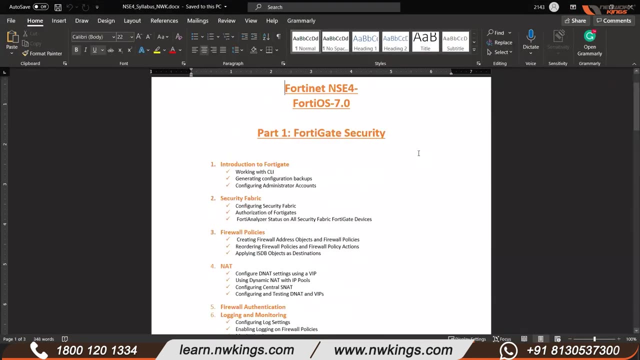 Fine, I got this Now. what next? What is the course all about? What information is covered, What all features is covered? So let me go ahead and show you. Okay, So this is the course Now. over here, the 40 OS 7.0 is basically the latest one. 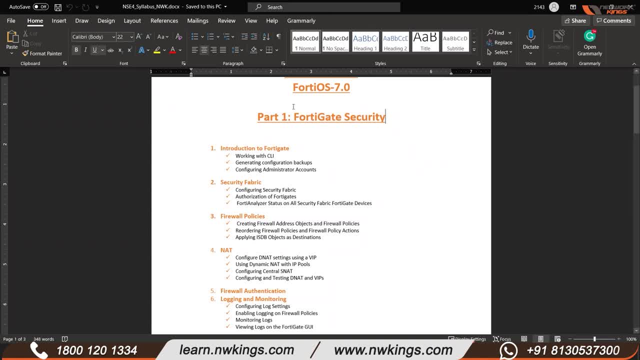 Okay Now. part one is called as the FortiGate security. This is very much, you know, in sync with the official curriculum of the FortiGate firewall. Now, why do I have this? See, the reason is very simple. 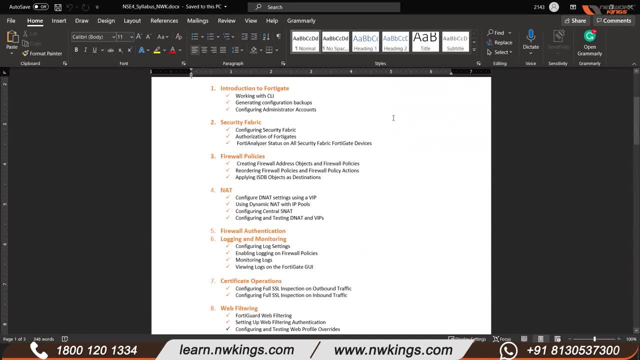 That over here, I want you guys to go through the official curriculum. The reason is that, if you know, and go through the official curriculum, even if you want, let's say, for example, maybe in December or maybe in January, Okay, 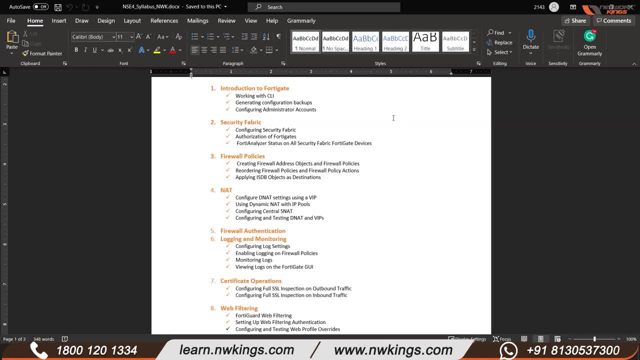 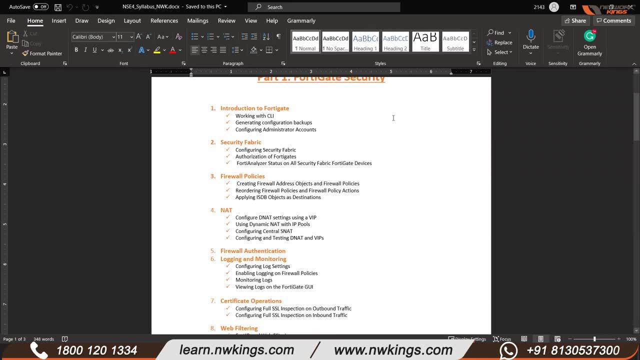 Not December, maybe in January or Feb. You want to go for a certification? You want to get into the FortiGate certification? Okay, You can go for that, Okay, And you would be able to get your certification for FortiGate. 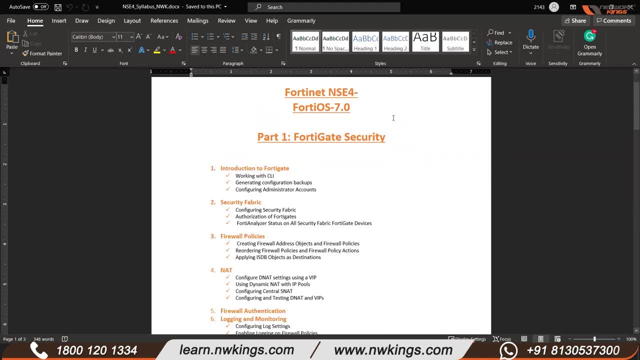 Okay, This is a hundred percent. But a hundred percent, of course, there is a course, but you also have to give a hundred percent from your side. Okay, I know how the you know the certification is. I have recently cracked the latest one as well. 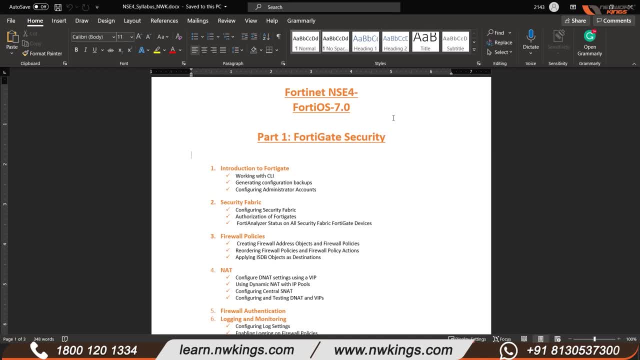 Let's ask a little bit. So the questions are simple, but they are just going round and round. So you have to read the questions a couple of times to understand what exactly the- you know- the question is saying. And then 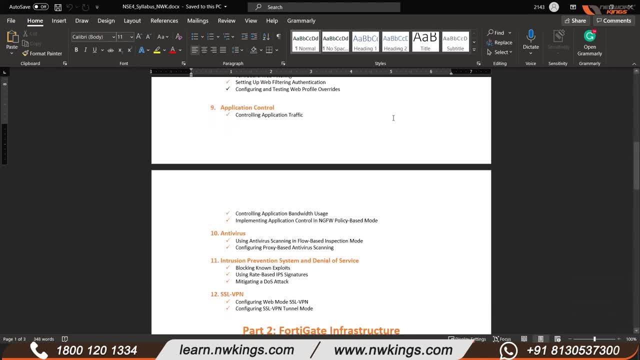 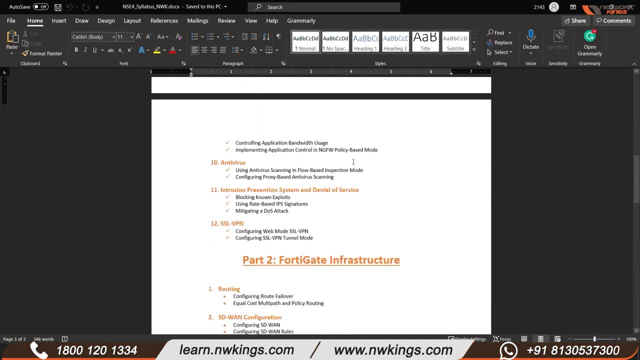 Give the answer. but you do not need to go. You do not need to learn anything else apart from what is mentioned over here. Okay, Uh, most and I will be able to give you this doc. no problem at all, Okay. 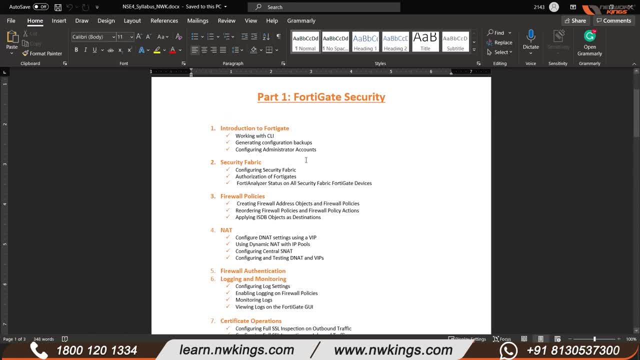 This is basically, um, this is your course. Okay, So you will be able to, uh, you know, go through this. So we'll be working. We'll start off with the introduction of the FortiGate firewall CLI. how do you work with a CLI? 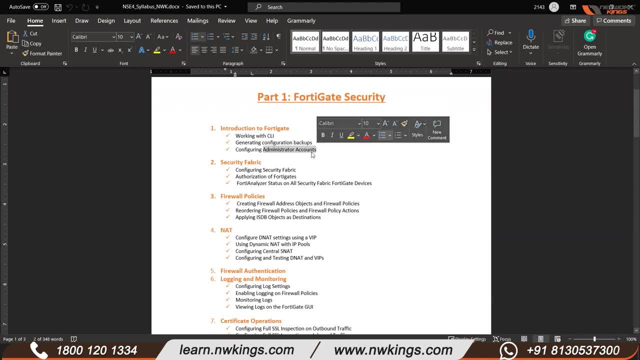 What is the configuration? backups, administrator accounts- We'll go starting, So we'll go basics, Yeah. Then we have something which is called as a security fabric. What is a security fabric? We'll talk about this one, Okay. And then we have the firewall policies. 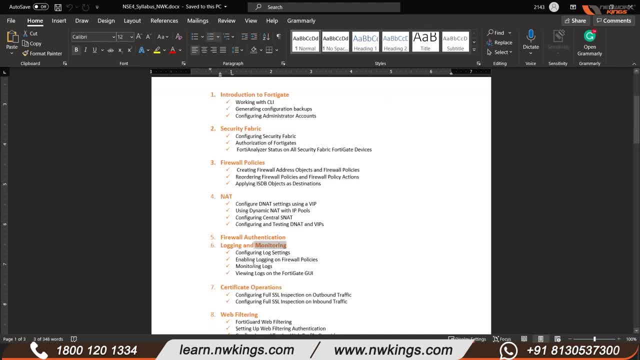 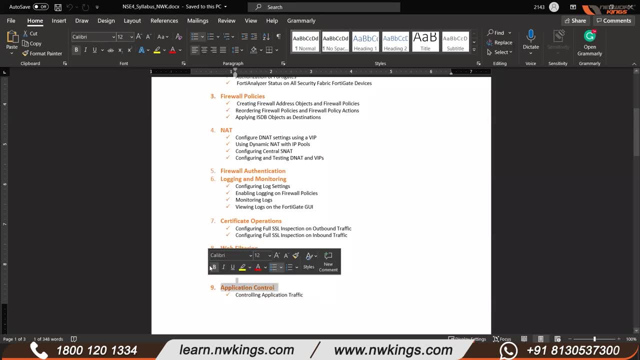 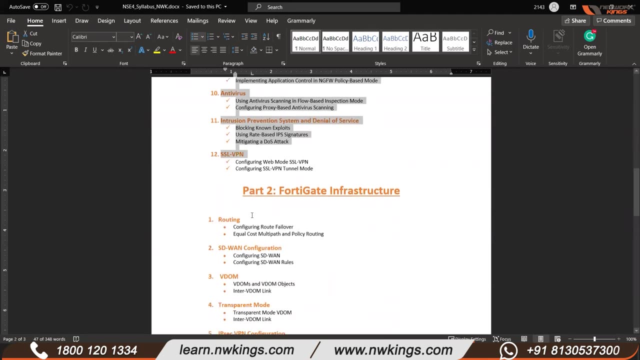 We have NAT, then we have the firewall, authentication, log certificate operations, web filtering Again. now this is all: security inspection, security features, application control. Okay, So we'll start off. we'll go one by one. These are the 12 topics when it comes to the security part. 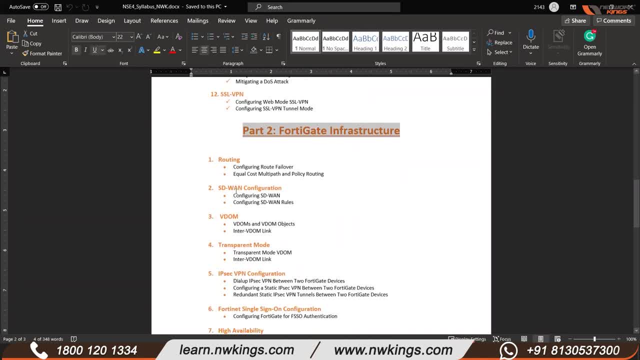 Then you have something which is called as the infrastructure, which is part two. infrastructure is um. this basically deals with a lot of um implementation. How do you implement? how do you? you know um install a firewall in the network. 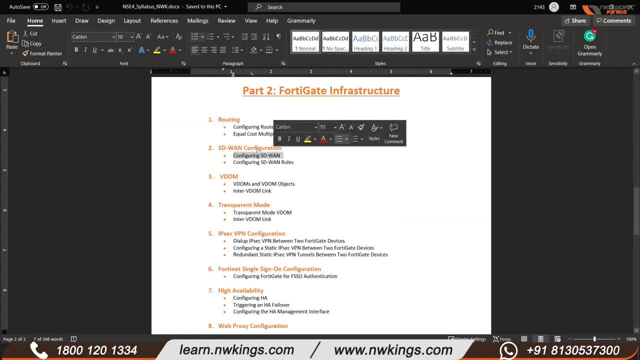 Okay. So what kind of routing will it? would it be? what kind of SD-WAN config? So okay, SD-WAN. I have implement, I have added the SD-WAN. Okay, The reason is that, uh, SD-WAN is very much required nowadays. 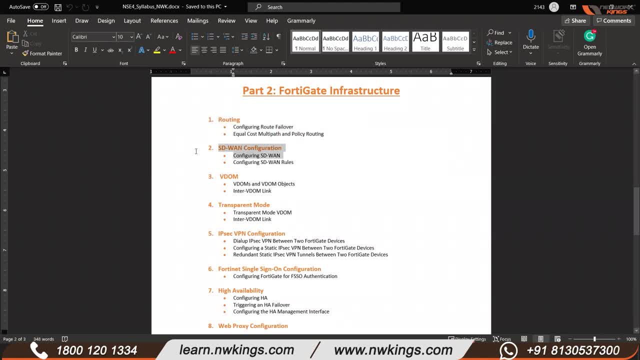 Everybody's looking for SD-WAN, So that is why I added this all as well. Okay, All right, Then we have VDOM, transparent mode, IPsec. Okay, Configuration SSO. This is all about how do you apply this in a network. 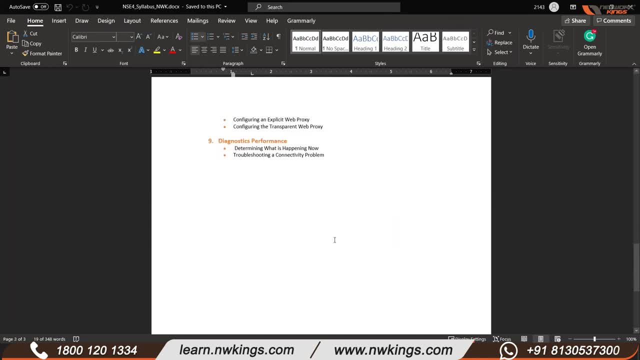 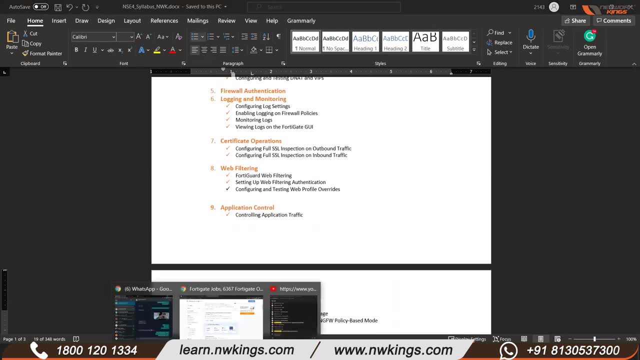 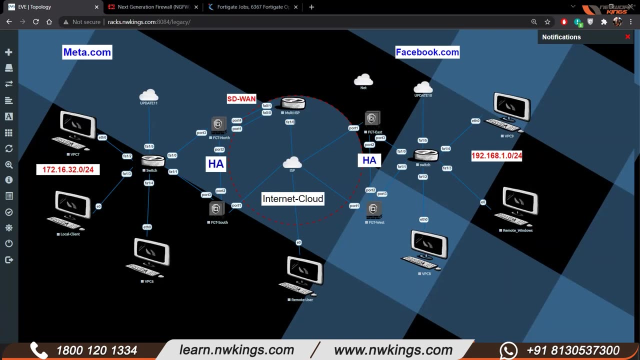 Okay, All right, This would be your course. We will go one by one, step by step. Okay, Let me go ahead and show you your lab. So I had a question, All right. So, guys, this will be your um topology that we are going to work with. 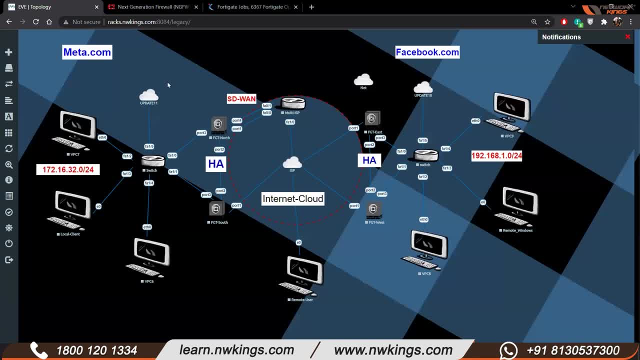 Okay, I'm not sure if you're able to Understand this, but then this is basically: one side is called as the metacom, The other side is called as the facebookcom. You will have your HA over here, The high availability. then you have an high availability over here as well. 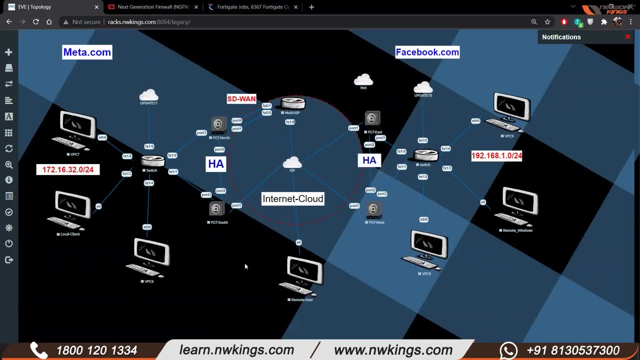 You are also implementing the SD-WAN. You have an MPLS network over here. Okay, You will be going in configuring different kinds of NAT environments. You will be, you know, switching over the HAs from one location to the other location and making sure that your connection does not break at all. 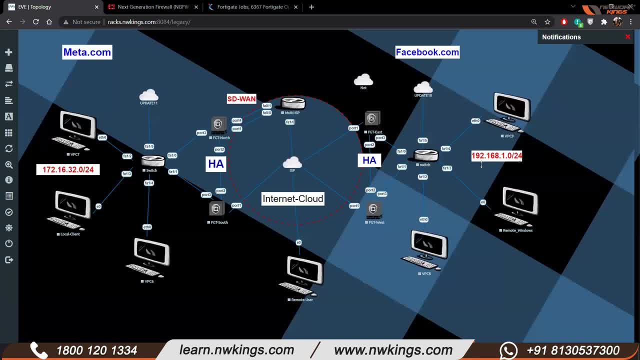 If you're able to work this through, Then you would be able to understand and you would be able to know what you need to do to get your FortiGate firewall to work the way you want. How do you troubleshoot this? What kind of troubleshooting logic you want to apply? 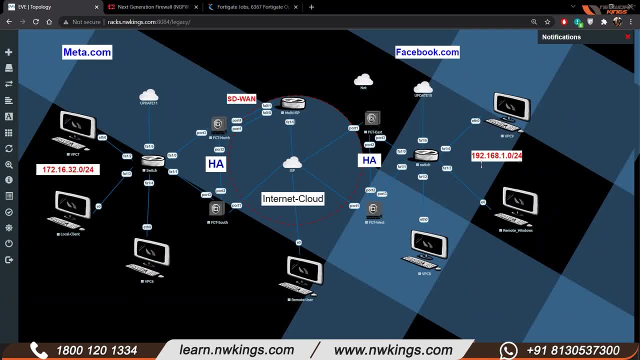 Okay, All these things would be able to you would be able to understand, figure out and give your best. when it comes to the FortiGate firewall, It's quite easy, uh, to work with this and quite easy to, um, you know, troubleshoot. 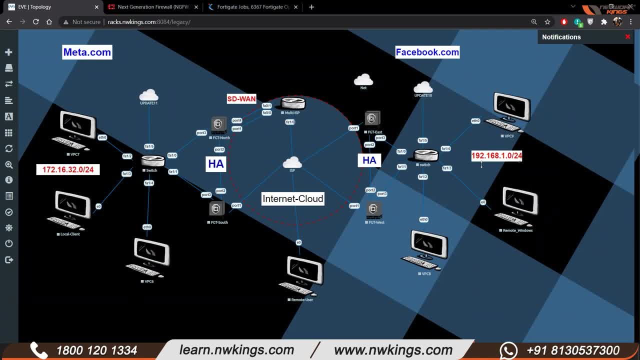 on this because it's it's command is easy and it's uh, the the interpretation, what it comes. whatever Debug debugging, you start, the debugging information that you get. It is very simple to understand. Okay, So if you are able to go through this topology by the end of the course, you 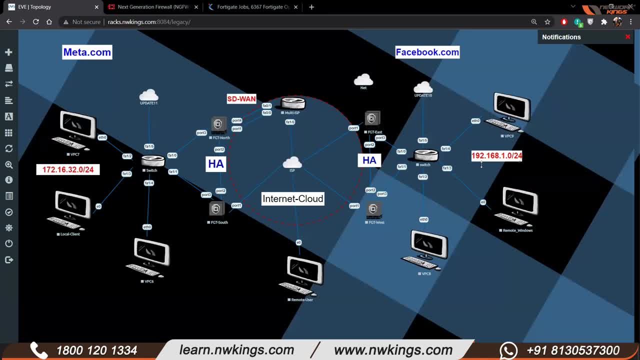 would be able to handle your FortiGate firewall. if it is implemented in your environment, you would be able to handle it very efficiently. Okay, All right, So this would be the lab that we are going to- uh, we are going to- work with now. 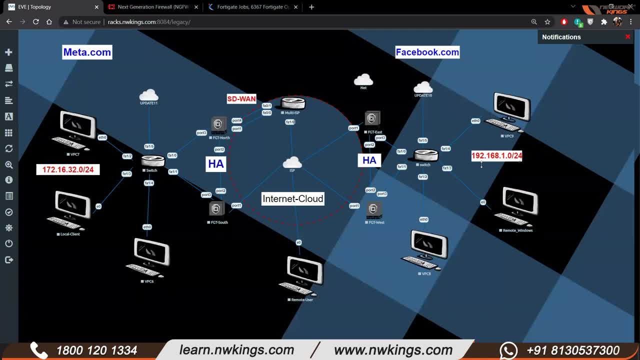 tomorrow. what we have in um store for you guys is that we are going to start off Um like maybe you can. you can say that this would be the first Class. we are going to talk about the UTM. What is a UTM? 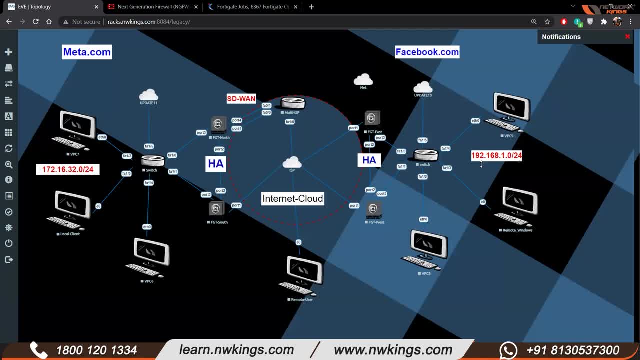 What exactly the firewall implementation is. How do you implement this? How do you start the firewall? What kind of configuration you want to go for? Okay, So we'll talk about all those things tomorrow. Okay, All right, Go ahead, Ask me questions. 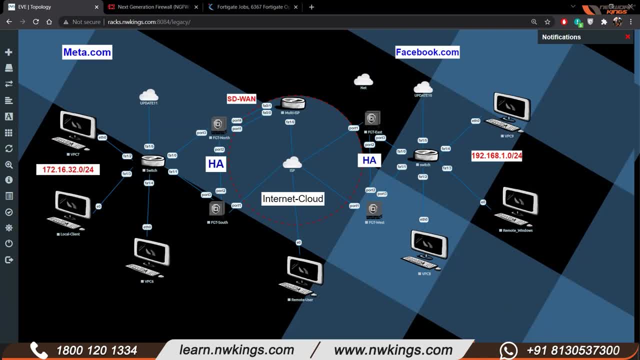 Mujhe mujhe pushna tha, jise mujhe uh firewall pe experience nahi hai. actually actually actually manager work kiya hai. Main abhi just philal work kar raha hoon, mikrotik router pe. 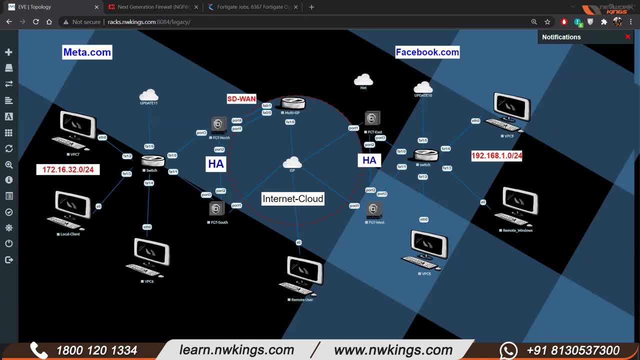 Okay, Okay, Toh fir mujhe iska kuch matlab hai. ho paega jaise fayda, ho paega Bilkul see yaha pe again, um jo maine pura, jo ye pura uh concept summe bataya hai ye. 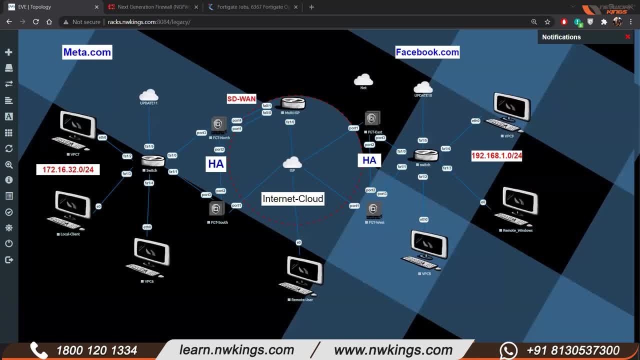 isley bataya hai, so that uh agar kisi ne sirf routers ke upar bhi kaam kiya hai, aur uske baad agar wo firewall ke upar kaam karna shuru karta hai, toh this is the. 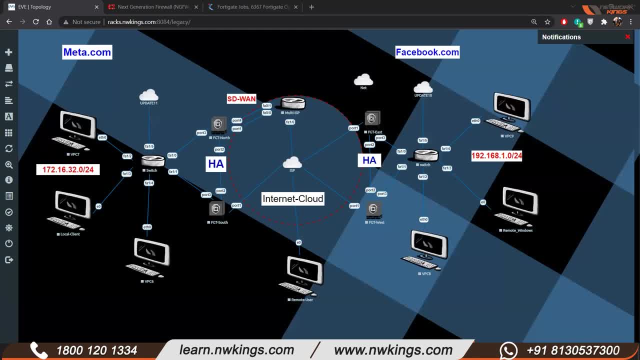 best place to start with that. The reason is that it is simple to understand: pehli cheez aur jitne bhi security concepts hai, Woh firewall ke saath ki cover up ho jata hai. Toh, agar kuch bhi nahi aata hai, toh bhi tum ussees ko jo hai acche se cover up kar. 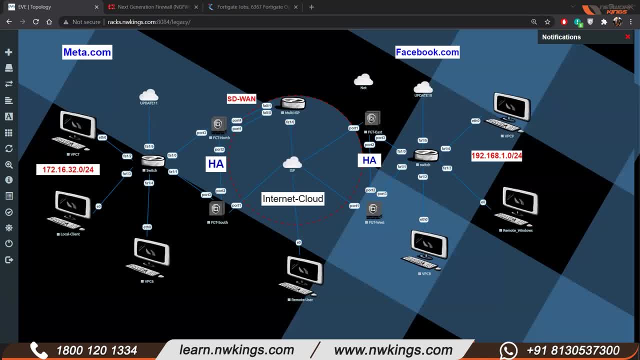 See, jab CCA ne padha tha, toh kya pata tha? kuch Nahi padha tha. But then slowly and gradually hum logo, concepts pata chalai, aur phir uske upar kaam karna shuru kya. 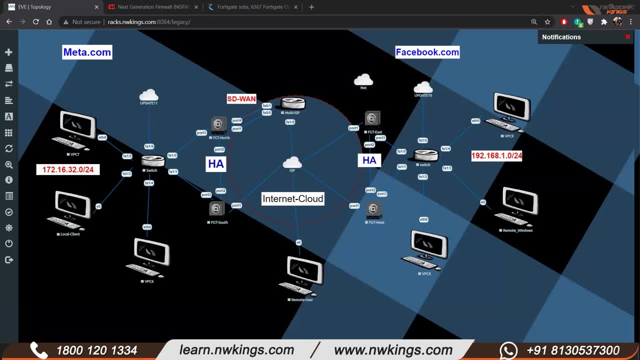 Same concept yaha pe bhi hai that if you want to get in the security field- agar, agar tumhe security mein concepts pata hona chahiye, firewalls ki baar hai hona pata hona chahiye- toh this is the best place to start with that. 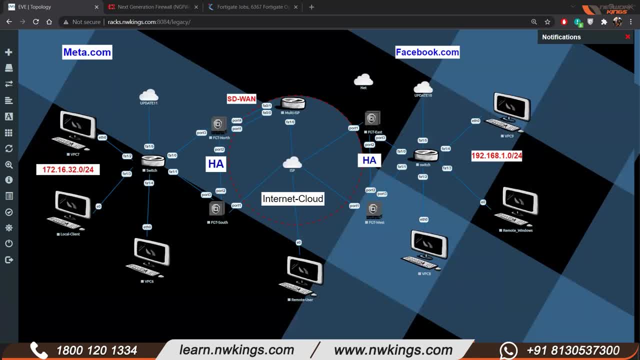 Uh-huh, Kuki, kuki minister, abhi, abhi just, uh, uh, just, just just just 10-15 din pehle se maine uh jo, Noah Solutions, Noah Solutions. 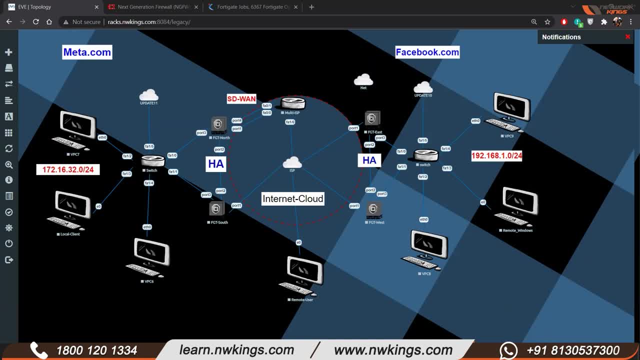 jo hai na uh Sikandar, Sikandar Sheikh Hyderabad ke waha, waha se mera bhi CCNP, maine chalo kiya hua hai. Okay, good hai, accha hai CCN, and CCN is actually very good, agar asa kar rahe ho kuki uh CCNP. 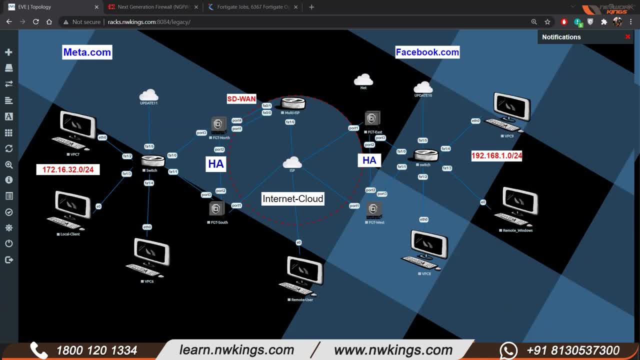 um, ek achchi knowledge, ek achcha base tayar kar leta hai right, Achchi networking, uh ki knowledge agar hoti hai, toh next step jo hota hai. na badhi simple se baat hai, agar tumhari building ka jo base hai. 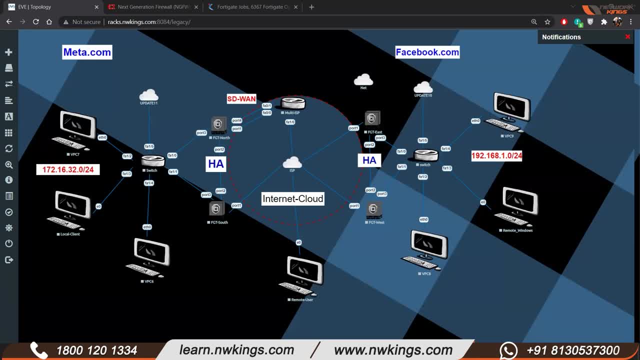 woh pahot strong hai, toh tumhari building bhi achchi rahe. Right Toh, agar CCNP tak kar rahe, ho bohot achchi baat hai. Okay, all right. Any more questions? Mohsin, yes, go ahead. 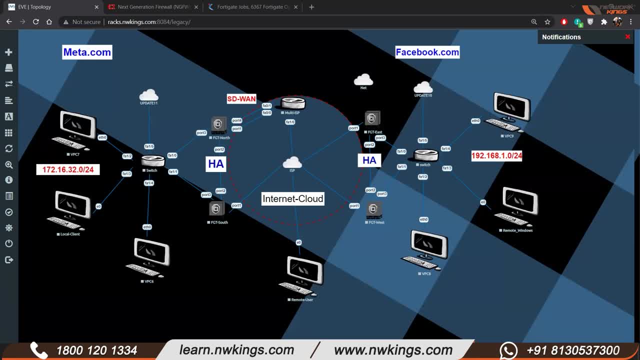 Yeah, uh, hello Rakshit. Yes, Richa Hi, good evening, Good evening, Yeah. so, uh, yeah, my question is similar to uh like: so even I do not have any experience in this, uh, you know networking or uh coordinate. 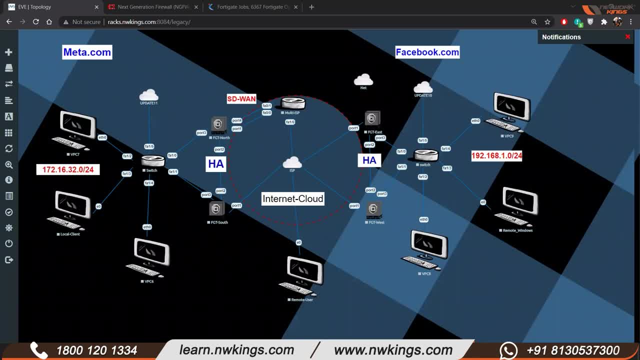 what we are going to right now. but but I'm like I am working in uh, in a support domain, like as a technicalist. Uh, I am an associate for CZI working as a systems engineer, so I just 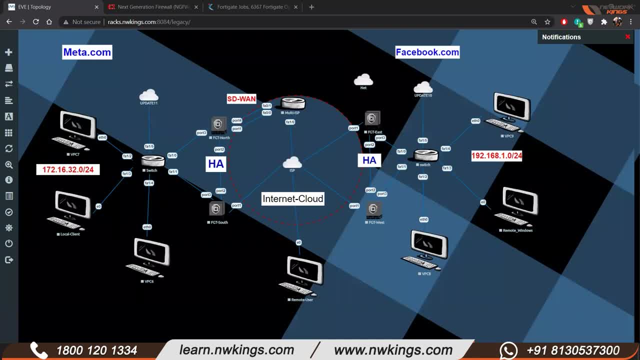 know the few basic things, what we deal in every day, our day to day life. That's the only thing I know. So, but uh, recently, I'm like, as I planned that I will do this coordinate course, a forticate course. uh, I initiated, uh, you know, the. 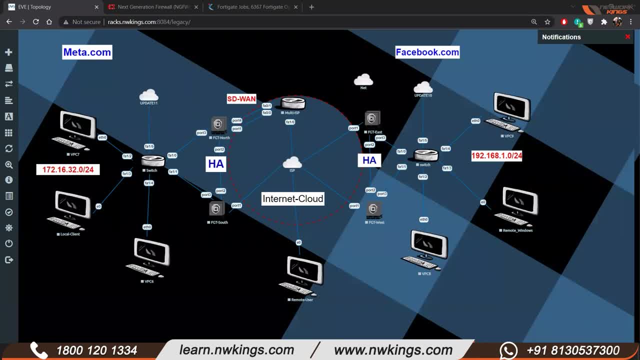 basics of networking, uh, through Udemy. So yeah, that's what my question is like. Uh, if you could suggest something what what I read before this and you know, just to cope up with what we are, 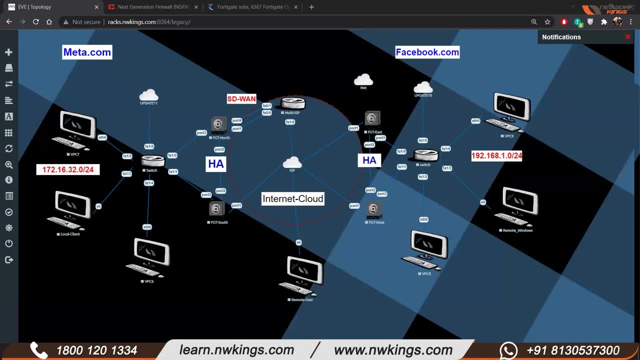 going to do the next thing, So that will be very helpful. And yeah, I'm like after today's session, I understood few things, but few things were like just uh, I was not able to catch up. So yeah, exactly. 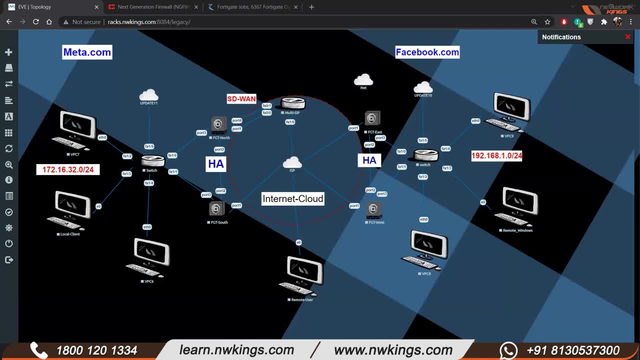 So the, if you could, you know, suggest something. uh, what I would suggest is basically that: um, again, basic networking, right? Because again, uh, let's say for example tomorrow, I say okay, by this is how you configure an IP address and you do not. 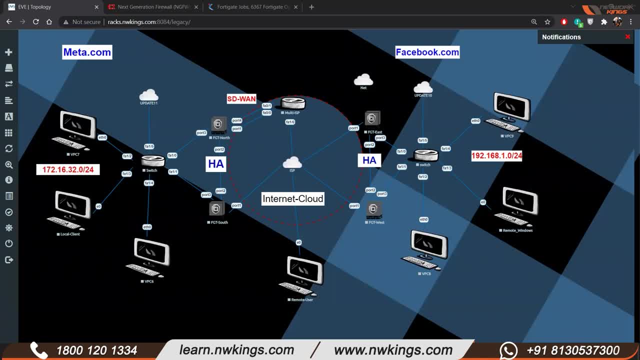 know what is an IP address, then challenge, right. So I would say: go ahead with CCNA first. Okay, Or at least side-by-side. start your CCNA so that you understand the concepts of networking, how the traffic or how the data from one device to the other. 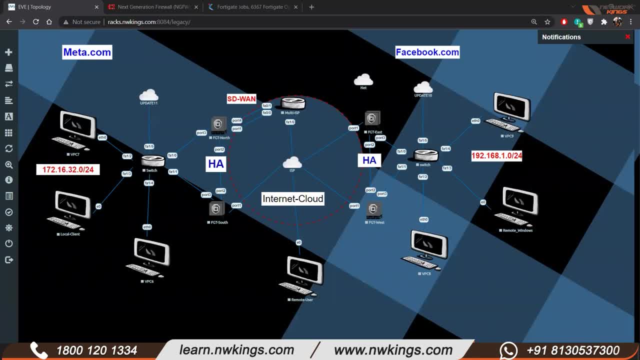 device travels. what is our? what is IP addresses? Okay. What is DHCP? Um, what is, uh? what is ISP, which is the entrance? What is the service provider? Okay. What is subnetting? Okay. What is routing? 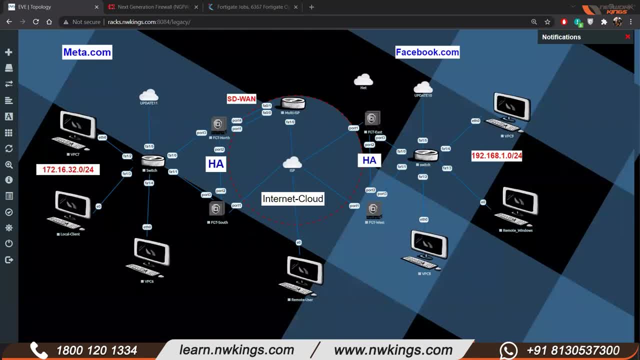 What is dynamic routing? Okay. What is high availability? Okay. This is basics. If you, if you know this firewall would be easier to understand, Okay. But uh, my recommendation is that, if you are, if you're already enrolled in this, I 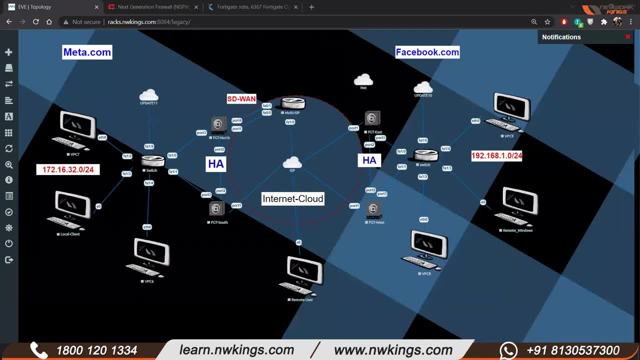 would suggest you to at least go through your CCNA side-by-side so that it becomes easy for you to understand. Otherwise it would be difficult for you. Okay, So Do you suggest to do some courses for CCNA, or just that I can go through the Udemy courses? 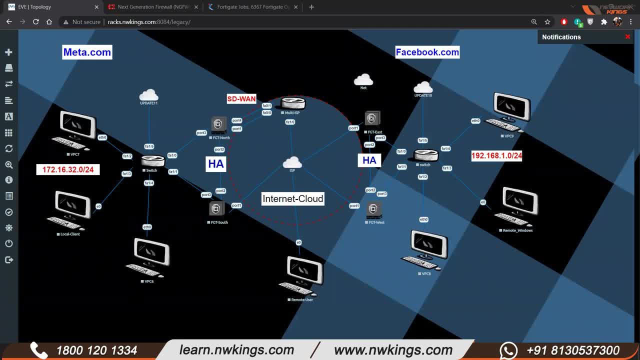 what we have Um Udemy is like a, it's like a refresher note. Okay, They, they, they do provide information, but then they do not provide information in depth, Right? So I would probably suggest you by- uh, you know, get in um, get in the course of CCNA. 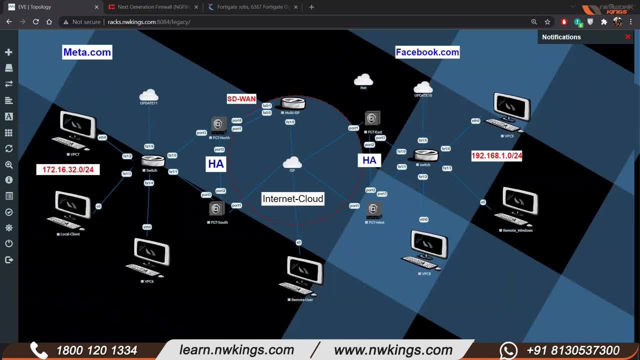 Okay, Because everything has to be in detail, because a lot of things in the firewall, once we, you know, dig deep, maybe you know, after maybe five years, After maybe five or 10 classes, it would be, it would start becoming difficult for you. 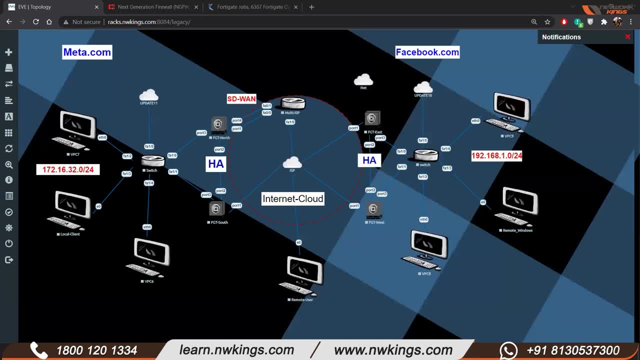 Okay, Because there are a lot of concepts which is already taught in the basic, networking and CCNA, and not all of the things you would be able to cover up with Udemy. Okay, Okay, Okay. So you, either you have to do one thing, that you have to basically buy a lot of Udemy courses. 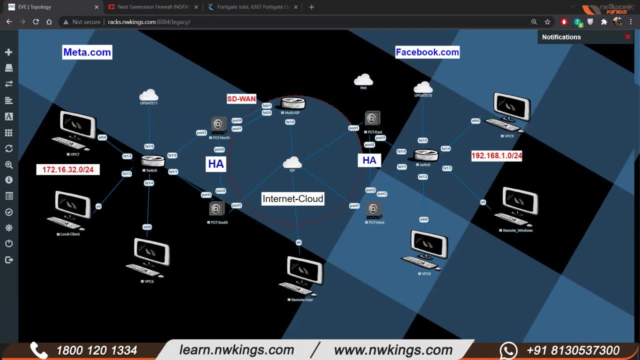 maybe five, seven, maybe 10.. Okay, And then you would be able to, you know, get all those information. but rather than doing that, I have, that, you know, corporate access for Udemy. Yeah, Okay, So I, so I know that I, well, I, my colleagues, are basically working with, uh, certain companies. 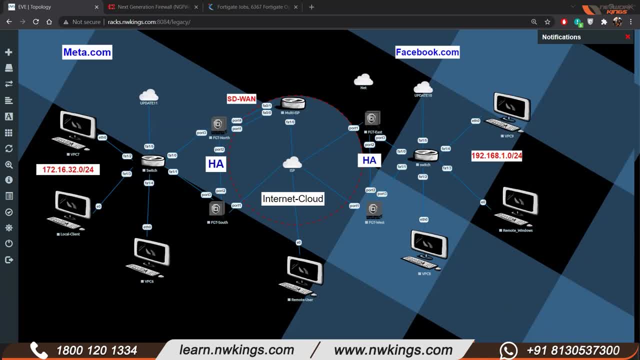 and they also have that. No problem, If you want to go that road you can do that. But again, I would suggest that uh take note of all those topics and options that I have said right And make sure that you have the- uh, you know- Udemy courses for that. go through them. 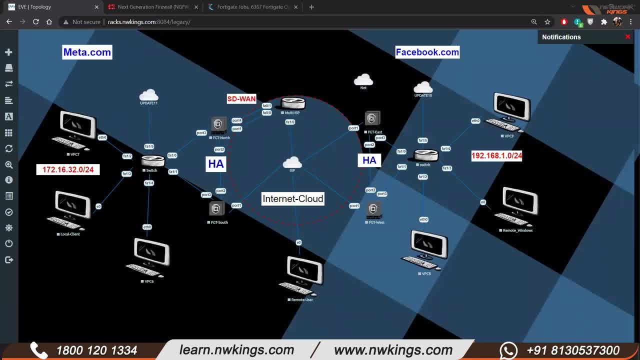 So it becomes easier for you. Okay And uh, once you are enrolled in the course, just make sure you ask me questions whenever it is required. Do not say Yeah, I will ask in late, I'll ask when the class is done. stop me there and there asked me the question, if it feels. 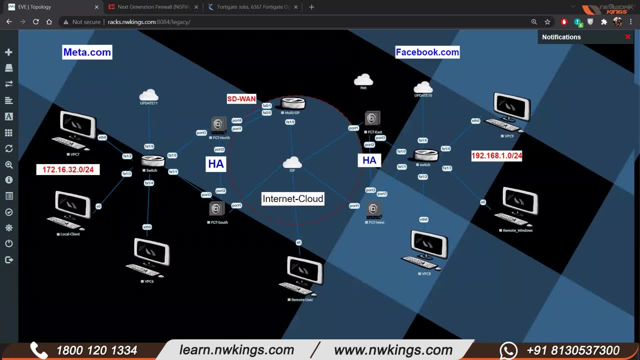 like to me that this is a basic question or is a networking question. I'll tell you by. you know, go ahead and you know, read this out. once you're done with that, we'll explain that. Okay. But again, higher recommendation: get your basic networking completed first. 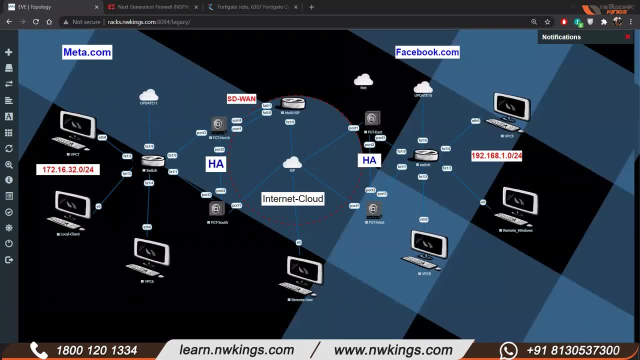 Okay, It becomes easier for you, Otherwise it will be difficult, a little bit difficult for you. Okay, All right, All right, No, Uh, yeah, sure, I will just look into that. I mean, like if I could do that. and one more thing, like tomorrow, what time we ha, we are. 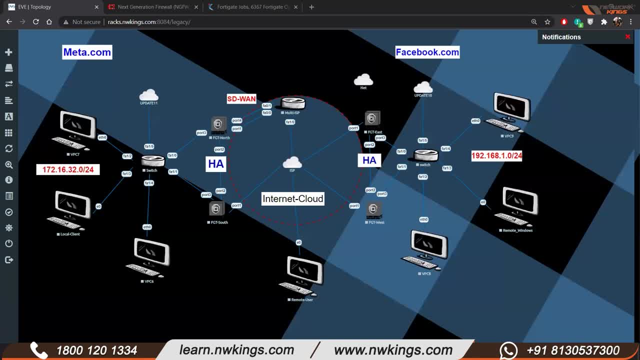 having this session. It's the same time, Seven o'clock, All right, All right, That was my question And thank you so much for answering it. No problem, Hi, sir. Uh yeah, Yeah, Most internally, Yes. 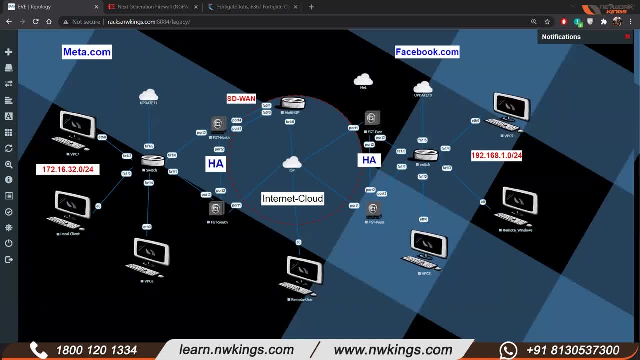 So I have done CCNA security in 2016.. Currently I'm working as an op lead and I'm also working on a 14 at uh 60, a hundred and 200. But uh, recently I have changed the job. 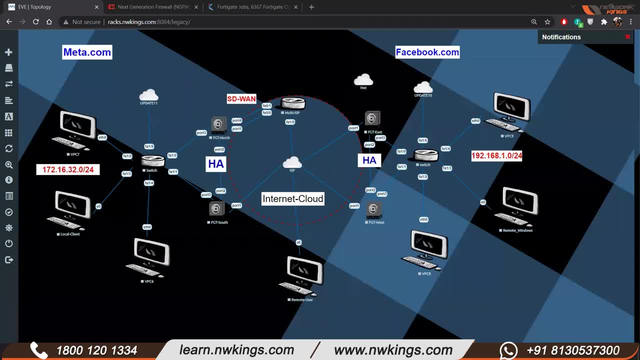 Mm-hmm Net environment. So, uh, my question is, uh, do I need to pursue the course? Because I'm interested in, uh in, you know, security field, but my job, current job, is, uh, uh, quite related to the wireless. 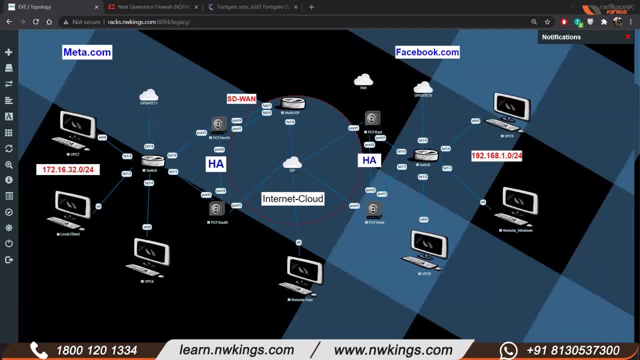 Okay, Again, most in. uh, my suggestion is not for what you're doing right now. My suggestion is: what do you want to do in the next couple of years? maybe, you know, five years or so, Okay, Okay. 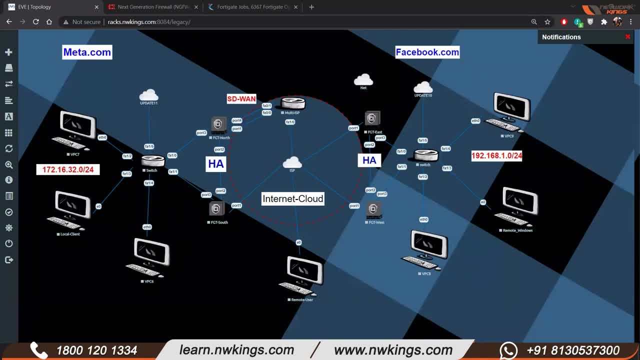 So, basically, uh determine your whole career. If you want to get into security of I would see security as of now, it's a good place to go. Uh, it has a lot of- uh you know- benefits. If you go into this field, that would be easier for you to understand as well and uh get. 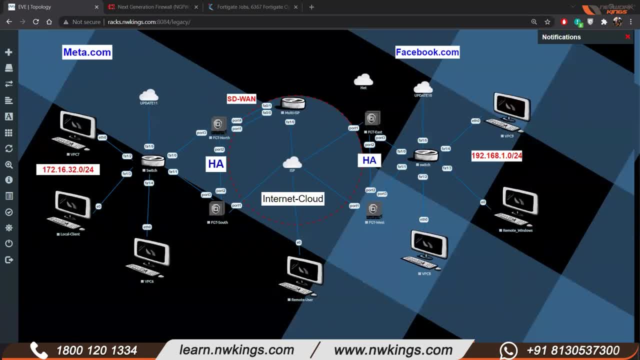 a good Pay job as well, Okay, But again, if it is right now not, uh, your field, if it is just wifi, um, you have to first of all decide: do you really want to go into the field of security or you want? 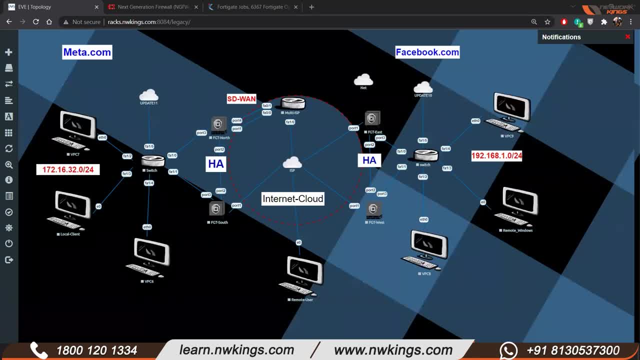 to get into the field of wireless. Okay, If you are interested in the security food, I would definitely say: go ahead and, you know, enroll yourself in the in this course. that would be helpful for you because, end of the day, you have to basically understand what you have to do in the next five years. 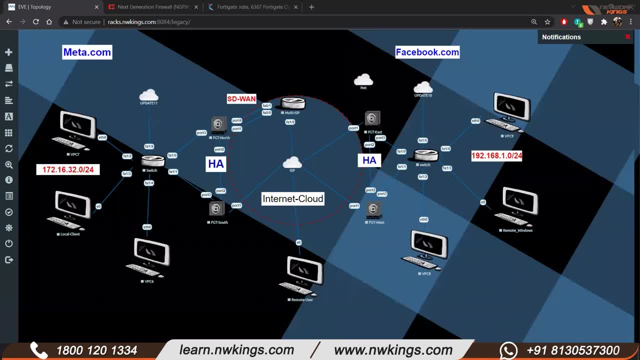 what you have to do in the next seven years. Okay, Whatever your salary is. Let's say, for example, I have five lacks, but, um, do I have to make this five legs, 10 legs, in the next three years? then what steps do I need to take? 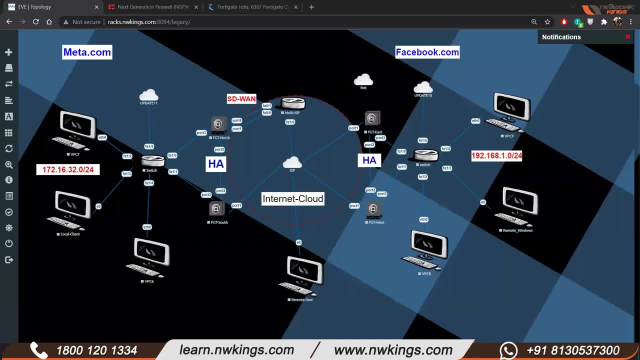 If I have to make that 10 legs, 20 legs in the next five years, what do I need to do? Okay, With security. I know this five legs can be converted into 15 next, within one year or two year, But again, it takes a lot of effort. 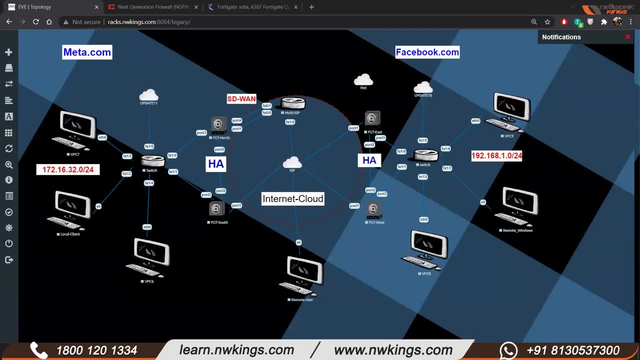 It takes a lot of um, you know, um courses and efforts and certifications, but that is very much possible. If you want to get into this package of 15 or 20 or even more, you have to and you have. 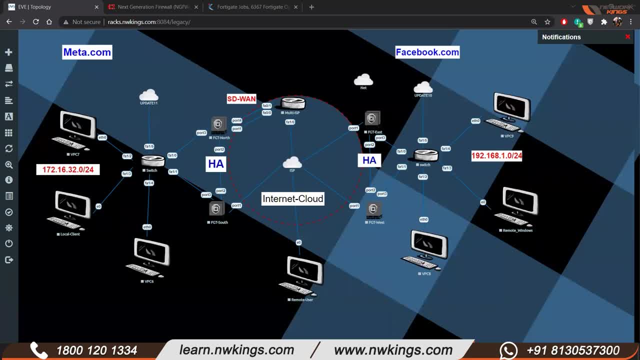 to. you know um, go through security courses, uh, multiple uh vendors, multiple firewalls and multiple technologies you have to work with. If you own all those things, it would be easier for you. Okay, Yes, Actually, basically I, I didn't want to. you know, uh, one uh technology or one uh? 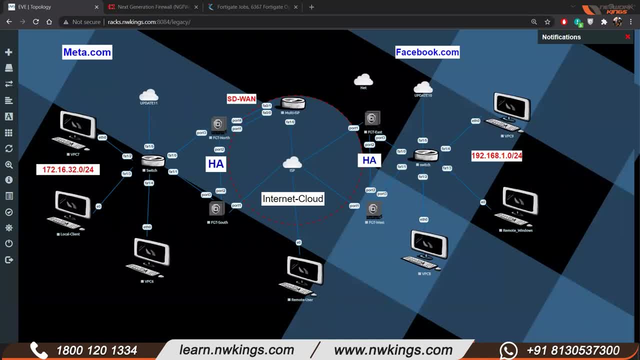 product. That's why I was, you know, pursuing for Arba, because currently I also have Arba wireless and switches, So I have both the things. So having wireless knowledge is good, but that is not your, that would not be your frontline. 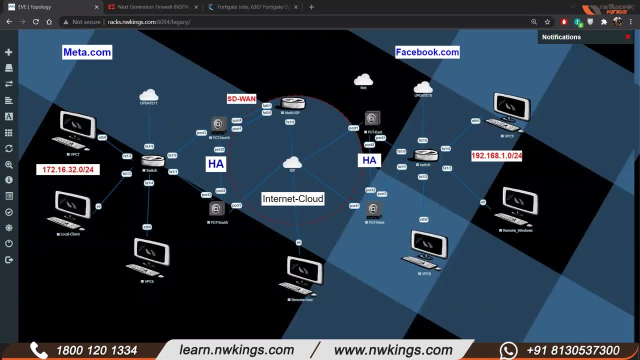 technology to work with Firewall would be a better option. to go for Wireless is just like an additional advantage or just like a cherry on the cake. Yeah, Okay, Okay. Okay, I'm getting short of time. Uh, so how pretty it says. what will the class time daily? 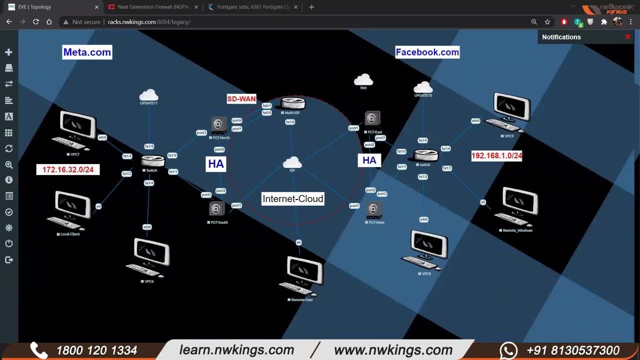 Uh, this will, uh, the time would be basically eight o'clock. Okay, Uh, the daily classes, but tomorrow we are going to do another session at seven o'clock, So I would like all of you guys- um, you know, take all your questions, be ready. 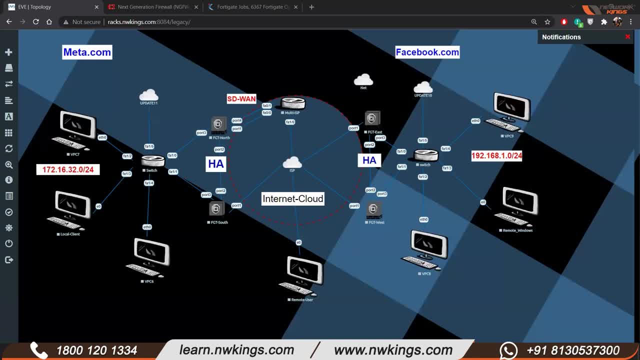 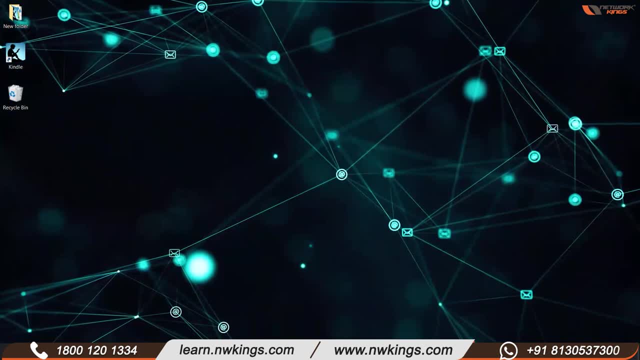 And by tomorrow I'll probably start the session by seven, 45 and then 15 minutes around the discussion, Okay, Okay, Now today what I'm going to do is, I was wondering to you know, go, let you go through. 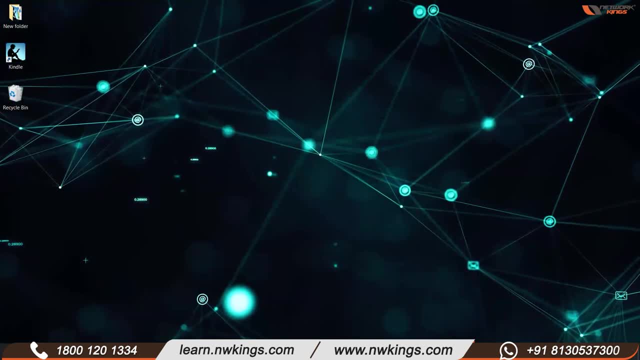 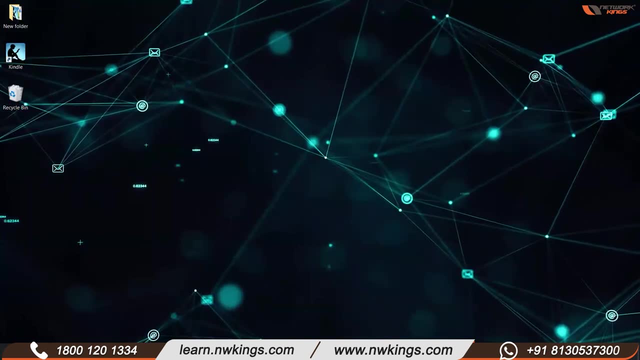 uh, you know some of the concepts and definitions but I thought let's do one thing, since most of you guys yesterday I I kinda liked, because a lot of you were quite interactive and I liked that. Uh, I thought let's do one thing. 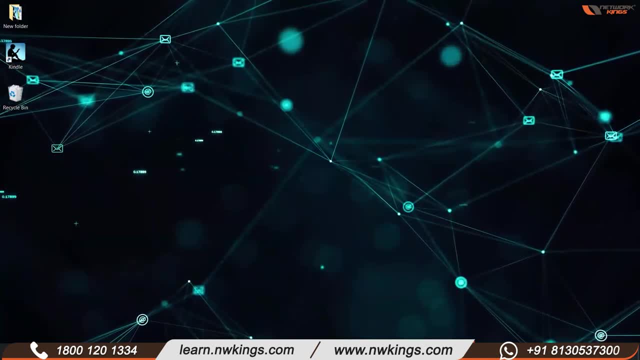 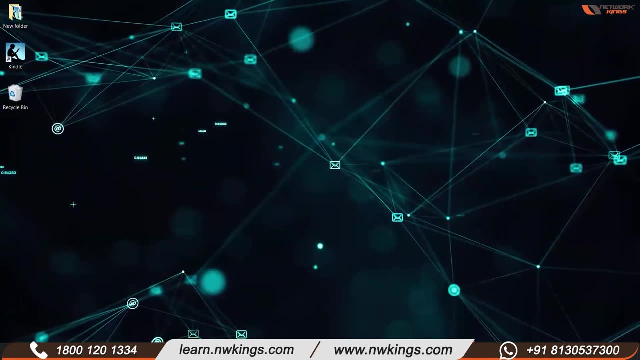 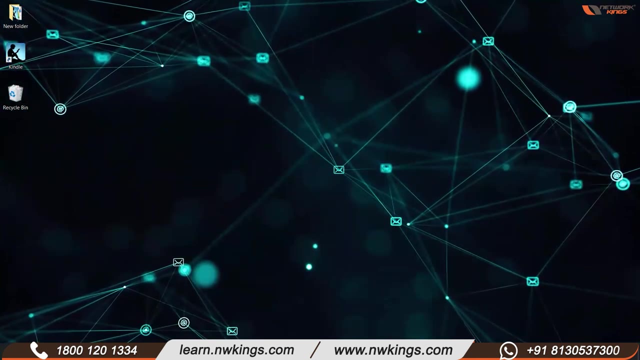 Um, practicals, and at least, if nothing, right, So let's do that. Uh, we'll have a session So that after this one hour of session, you would, You would be able to know at least something from the what do you get for one. 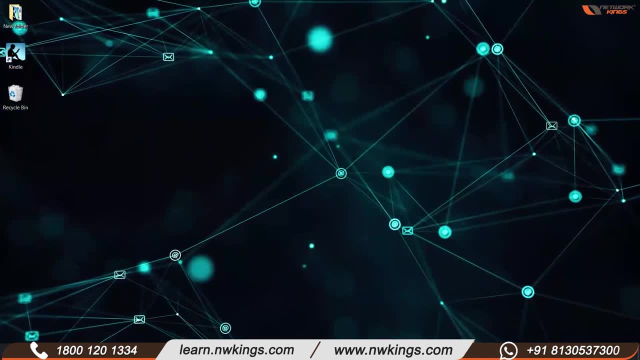 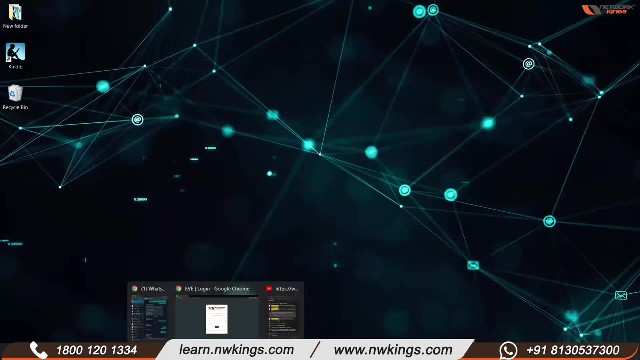 Right, Okay, So let's do one thing. Uh, I'll go ahead and show you the lab that your guys would be getting once you get enrolled. Okay, So what would be the lab? All right, So this would be the page and this would possibly be. you will be the URL that you will might. 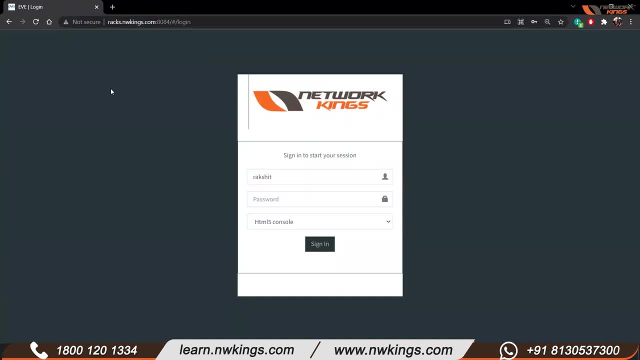 get Okay, Which is rank start networkingcom? Okay, You don't need to have your own uh VMware set up or you don't need to have your own uh laptop which has maybe 16 GB of Ram or maybe a laptop. 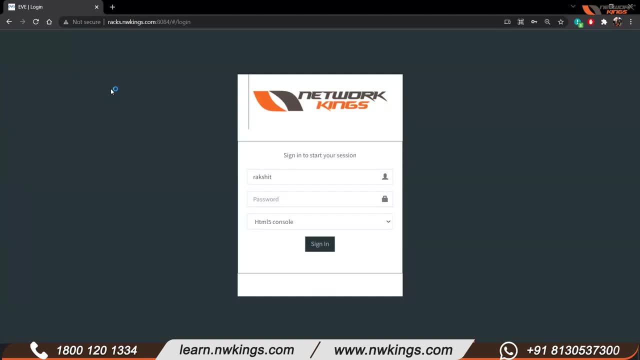 Okay, You do not need. it's just a plain simple um laptop would do. You just need to go to this particular uh URL and that's it. Go ahead, You'll get the credentials to log in, All right. 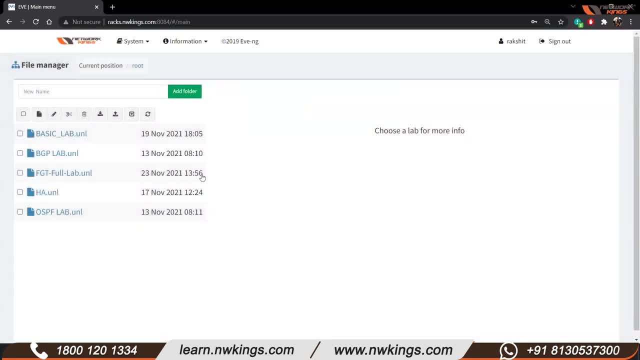 Once you do that, sign in and you will be able to see a couple of labs over here. Okay, Now, over here, if you look over on this third one, which is called as the FGT for lab, Okay, So, FGT for lab. 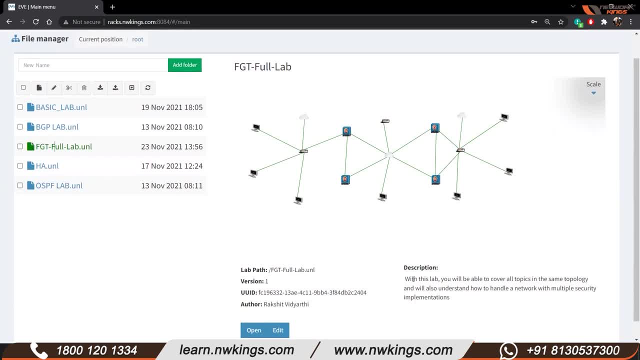 This is basically the lab which I have created for all of you guys. So with this lab, we would be able to cover all the topics in the same topology, And we'll also understand how to handle network with multiple security implementations. All right, 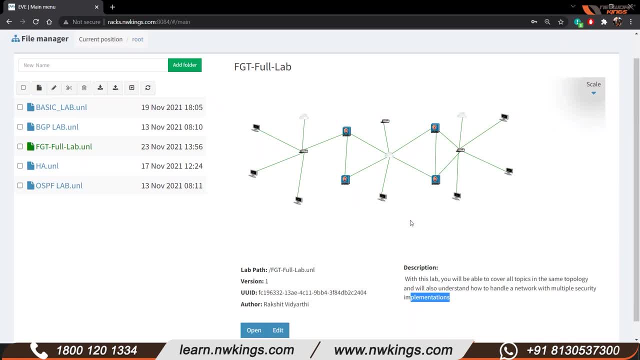 This will give you an idea of how, uh you know, practical scenarios, practical situations um you have to handle. how do you? uh, whatever changes you make, what kind of issues it could create in the network in the same um design that you have? 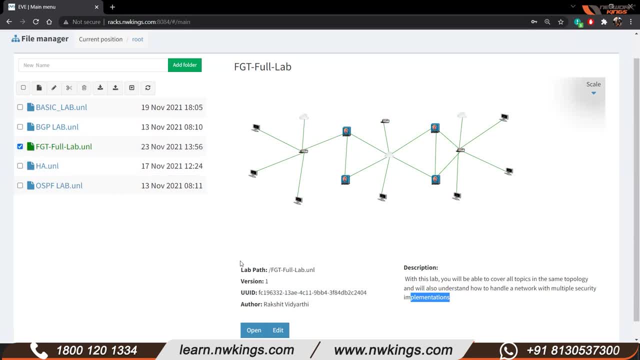 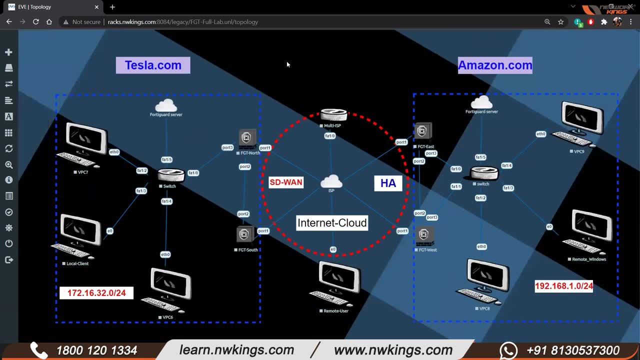 So let's do one thing: Let's open this up. If you want to do that, just check this up, click on open. Okay, All right. So I'll a little bit. I'll zoom out, Okay, All right. 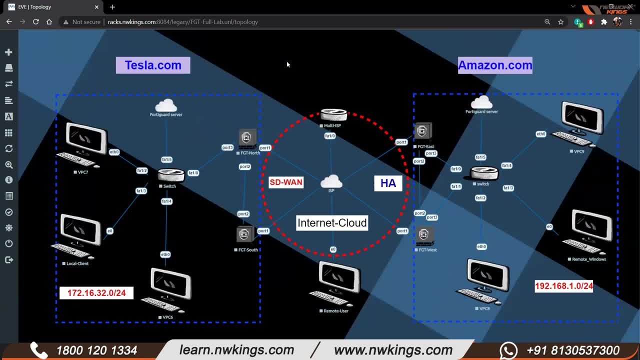 So, guys, this is the lab that you will be getting. Okay. So if you look on the left side, you have a company who is who's go by the name of teslacom- Okay. Then, on the right side, you have a company which goes by the name of amazoncom- right, 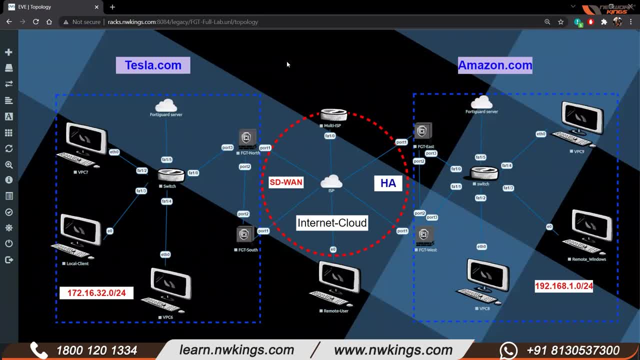 So the big companies are there in the world right now. So consider a situation or a scenario where there is a collaboration with the individual- Okay, And they would like to share their network, They would like to share the resources and they have a very complex environment, which 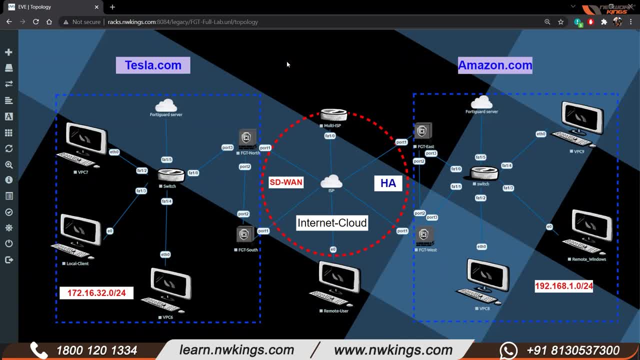 for which they have some SD-WAN implementations. They have a high availability also going. they have an MP-less network. They have an internet cloud as well. They have their internal land segments plus some DMZ servers as well. So it's it's a proper full fledged network individually for these two companies. 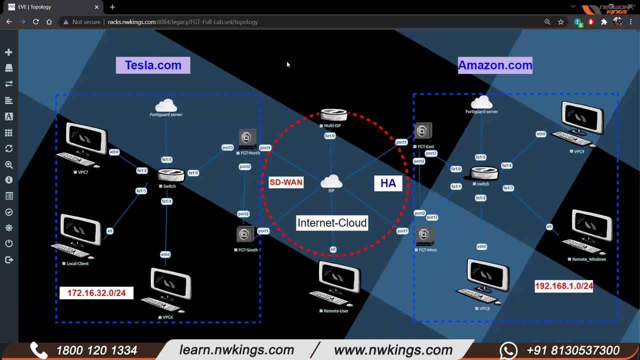 Now they would like to get this thing in. you know, in collaboration, they would like to share resources. So you see every service, service whose very, very ultimate right, And on the black square, you would like to, you would like you have this data set. 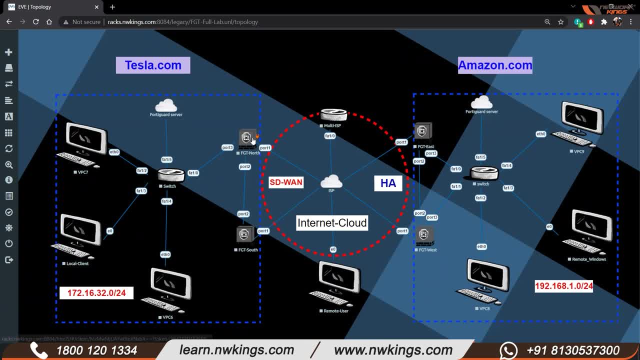 What you would like to do is you are going to go here in the data center. you would like to do this as a meeting. the events itself will be what you would like to do, Because all the events need the specific information. So you just highlight a range, even if it's not that big, it's no big deal. 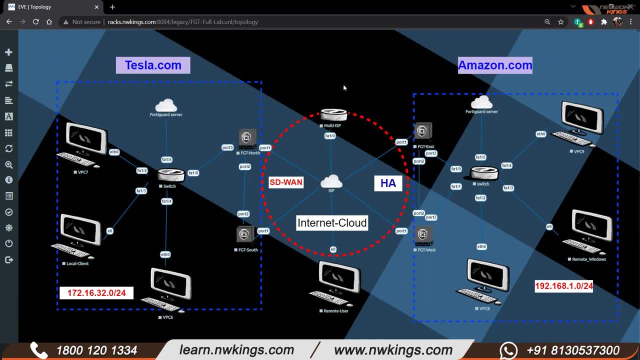 It's just referable. Then you copy that, The agreement forms. Okay, okay. um guys, can you hear me any problem with the voice? uh, no, that's all good. okay, all right. so i think you might have to check your side. maybe there's some problem on the on your side. okay, good, okay. so now what we are going. 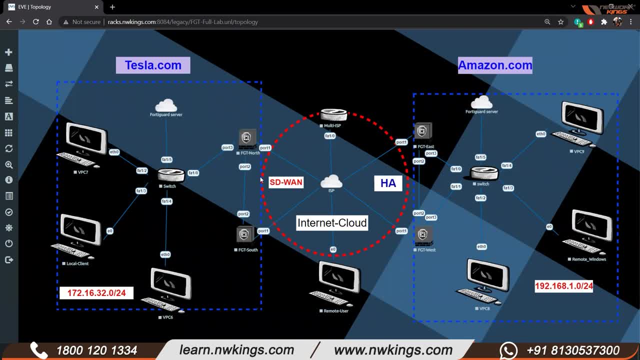 to do is- i'm going to tell you that- how you go about. first of all, uh, powering up all these devices. okay, all right, so you go ahead, right click and click on start. okay, so this way, one of the device will start booting up. okay, there is another way, which is: you do you see these a square, small? you. 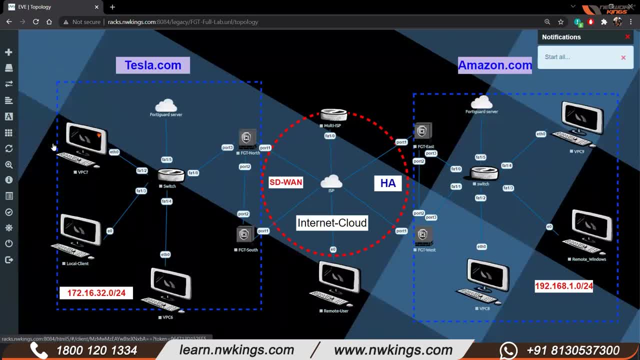 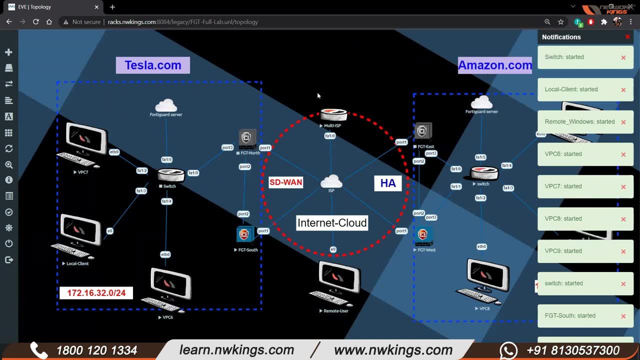 click on the more actions and then you have start all nodes. you can do that as well, so this would power on all the devices in your lab. okay, now what we are going to do is- so see, it's a heavy lab- like to request you all, if you guys, whenever you get this access right, give it about 15 to 20. 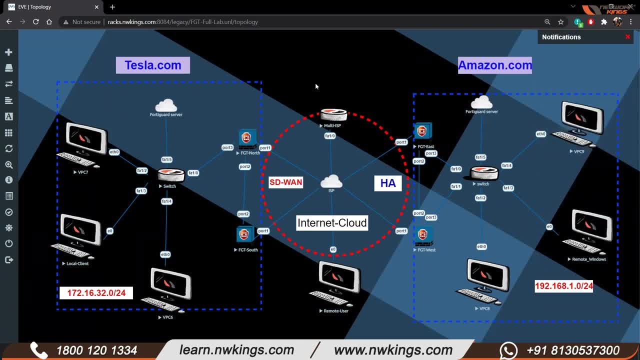 seconds. why? because every firewall, every network device, every switch, okay, every windows machine that you have, all of them would be booting up okay. so gives, give them 20, 20, 20 seconds. that is more than enough. once it is powered on, you can see this play icon, a little small play icon over. 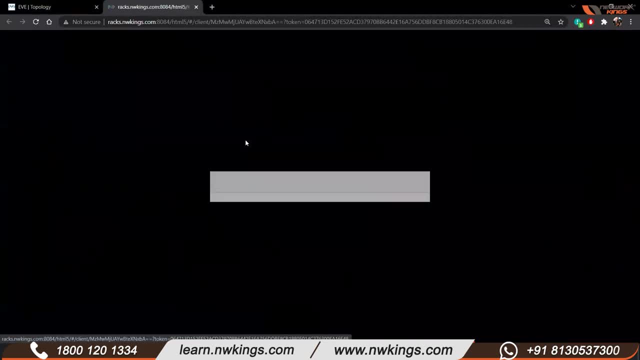 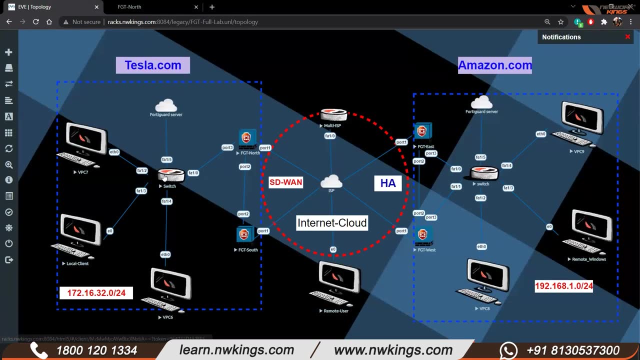 here. right. what you need to do is click on this, so it will open up a new tab and it will give you access of that particular firewall. or if, in case, you want to click on the switch, this will basically give you access to the switch. if you want to click on the local client, this will basically. 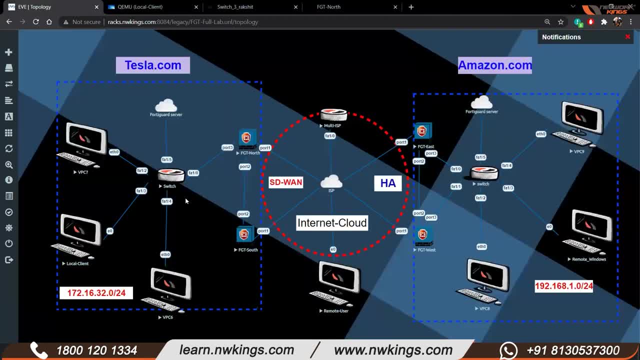 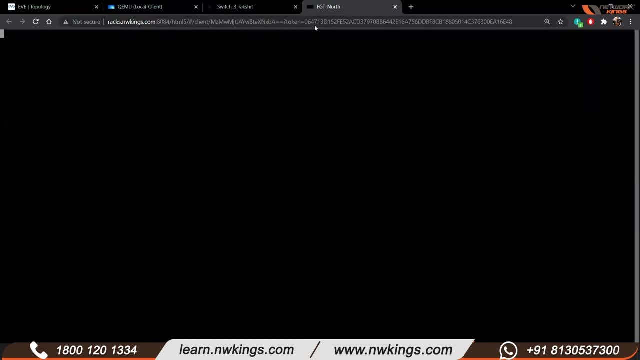 give you access to your windows machine, okay. so my point is: you just need to click on it and you'll get the access new tab and then you'll get the access. all right. so what we have done right now, we have go ahead, clicked on the 40 gate north. okay, and this is the windows. i'll just hit enter. 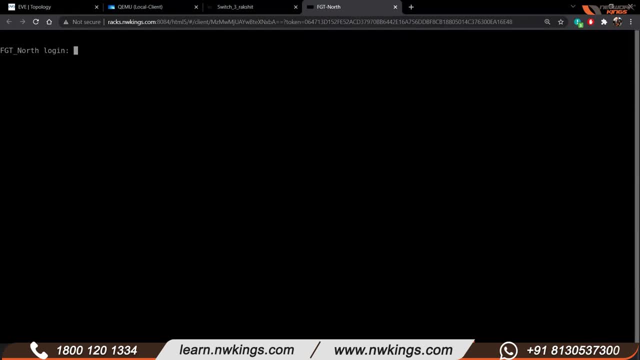 yes, see, so i have 40 gate north, log in. okay, now, once you get to this particular page, okay, you will be going and you know, making sure you can log in right now. first thing, if you have a brand new 40 gate firewall in your network, okay, and the client says: hey, you know what, just go ahead. 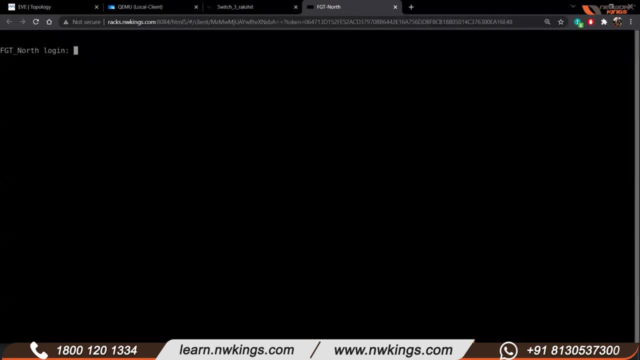 connect your console, configure your 48 firewall and, you know, install this on the network. so first thing is you have to basically log into the device. how do you do that? so the default administrative and password is called as admin, okay, and password is blank. you do not need to enter anything, okay. 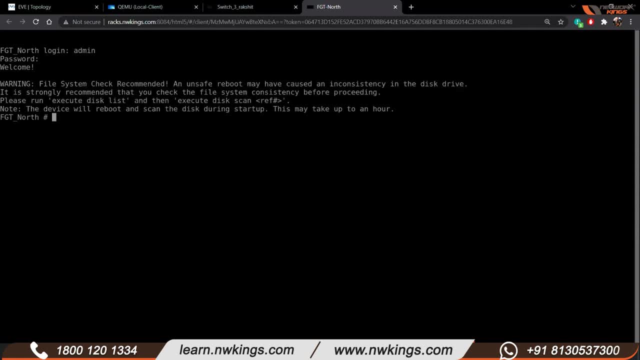 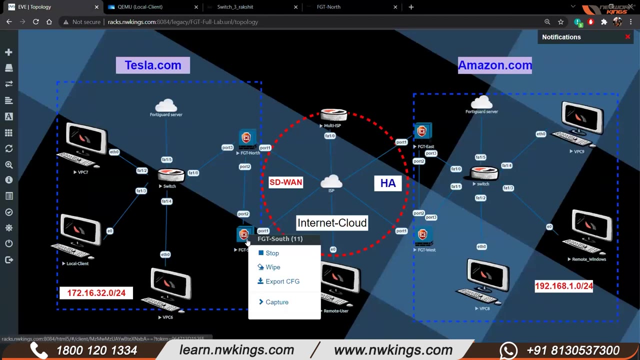 so that is the password, all right, so once you log in- okay, so i have already logged in many times, so it is not asking me to- uh, you know, uh, change the password. but once you would be able to log in, it will ask you to prompt: okay, let me show you. you know why not. let's do this, i'll so. wipe is an. 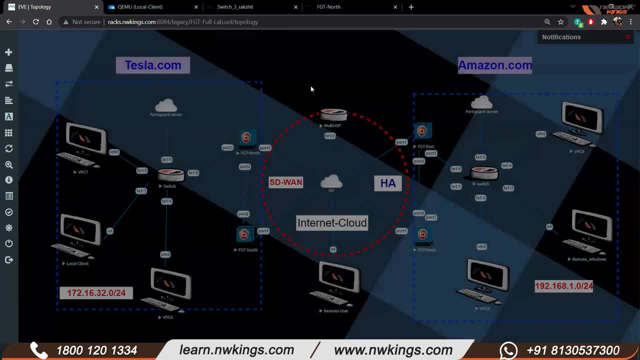 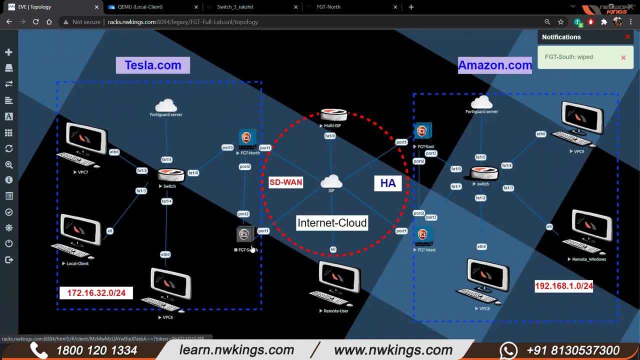 option. i'll tell you what it is um after some time, because i don't want to you know um burden you a lot of information, so i'll just click on one of the options, which is wipe, which is basically think of it like a factory format, just like you do this with the windows machine. you format the machine and then again install the. 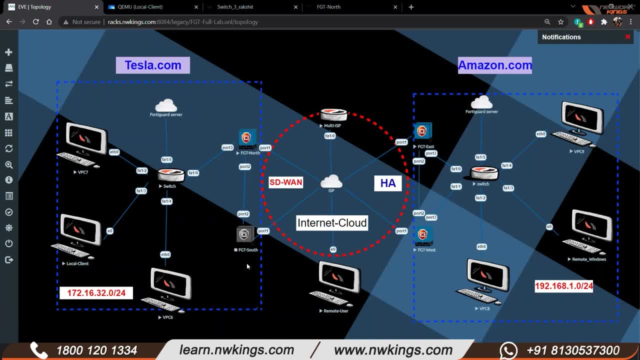 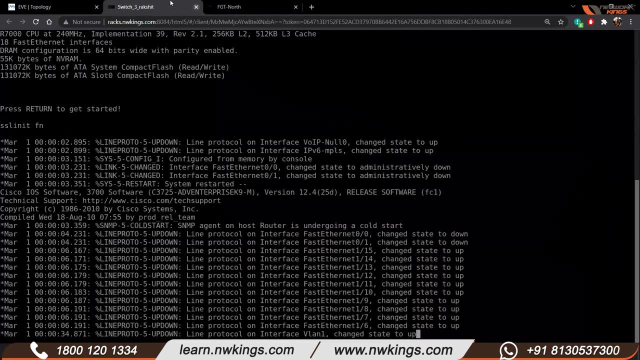 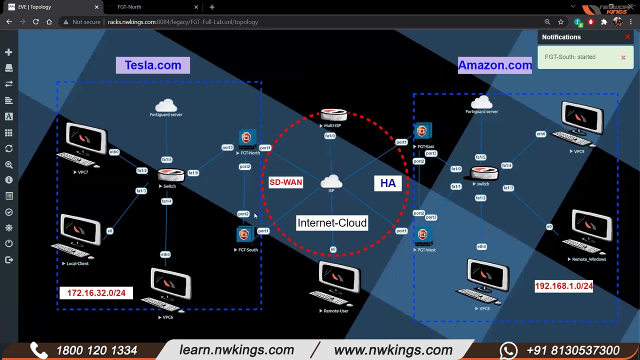 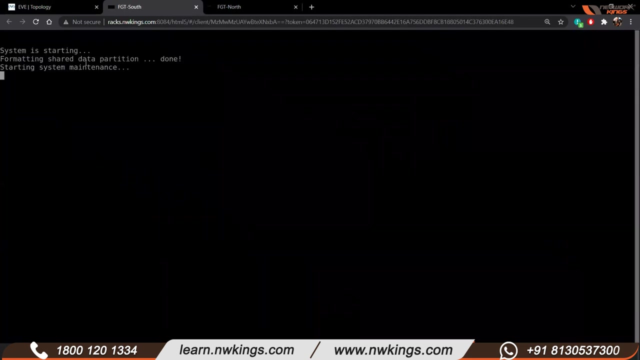 operating system so that it is a clean boot, just like that wipe is also doing the same stuff. okay, so i click on this. i'll power on this device once more. okay, in the meantime it comes up, let me close these out, okay. okay, click on it, open up a new tab automatically and then see. this is how it will start up once you. 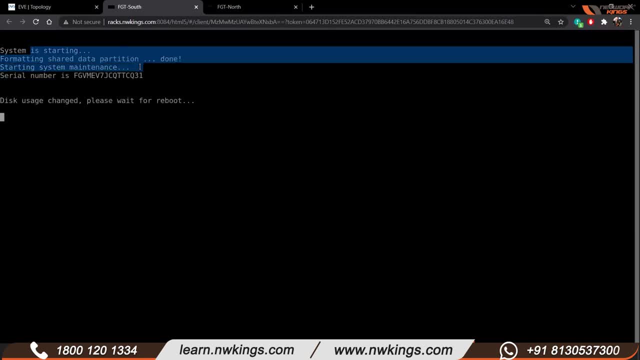 log in and if you- you know, if you power on the device, this is how it will come up. all right, it will basically tell you that system is starting formatting the partition. all right, and whatever the serial number which is being selected is going to be the serial number which is being selected. 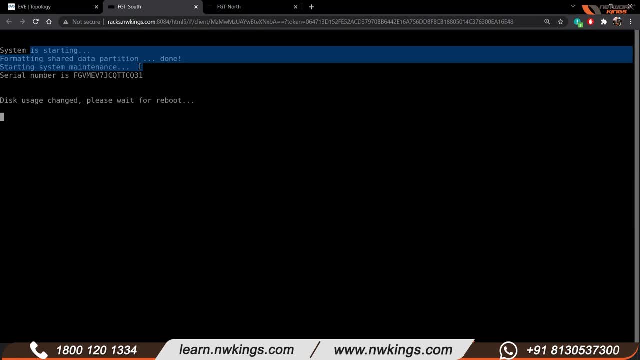 that's going to tell you that serial number. okay, now, that all depends, since i am basically working on a vm. right, look closely: it says fg, then it says vm. do you know why this is? fg basically are the initials for 40 gate, and vm is basically the initials for your virtual machine. okay, that. 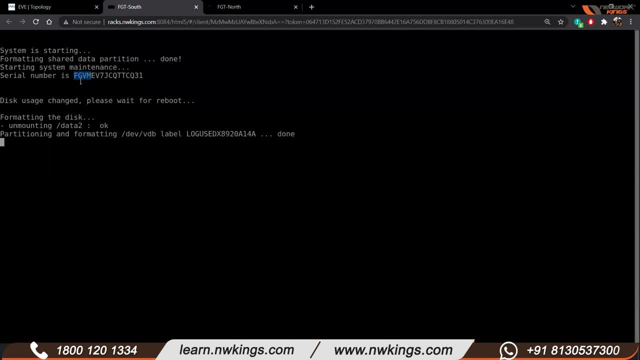 is why it says fg vm. whenever you see these two, these four letters, you can always, um, you know, get to know that, okay, whatever, uh, you know, whatever the uh operating system that i am working on, it is actually a virtual machine. okay, because if it is not a virtual machine, it will not. 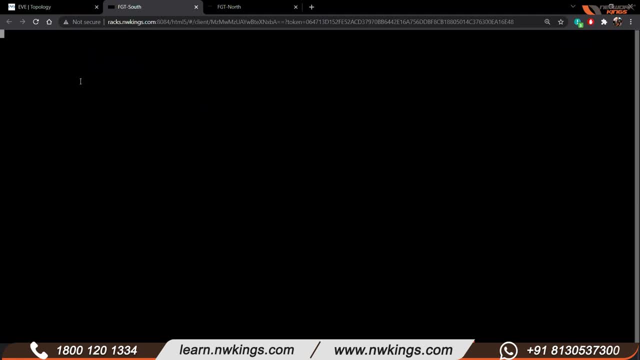 show you this vm. it will show you something else. okay, it might show you the hardware, whatever hardware that you have. so remember, yesterday we were talking about 4200f, um 1800f, so it will say fg and then 1800 or fg or 4200. so whatever is the hardware model, it is going to tell you that. 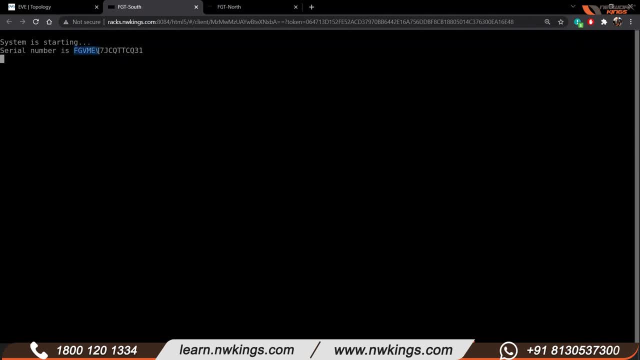 okay, all right, so now again it will. it is basically telling you what the- whatever is- the serial number system is starting. let's just give it about a sec, um 30 seconds, more or less, and then it should ideally come in. okay, great, so it is login. so. 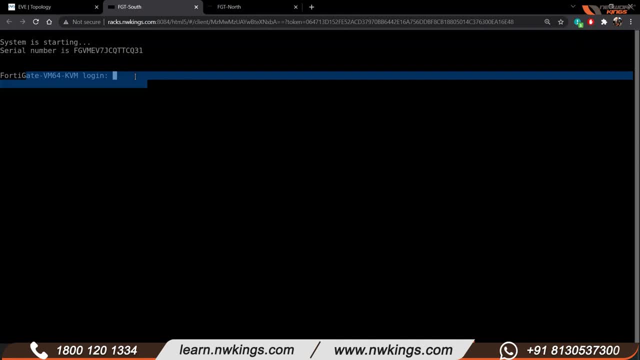 as i said, right, what is the by default username? can anybody tell me now, admin, admin, what is the default password? uh, blank, blank, right. so i do not have to put anything, i just need to enter, hit, enter, see what it says. you are forced to change your password, please in. 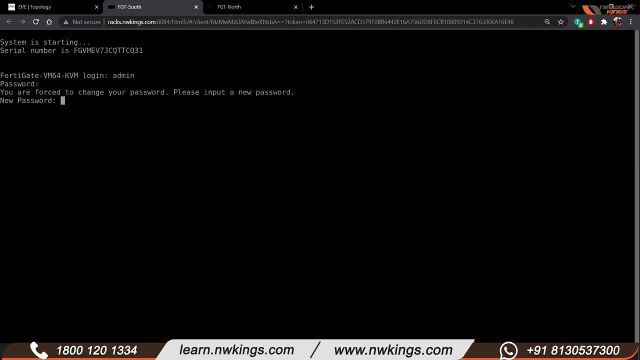 the description box and i will put a new password. okay, so what i'll do is i'll go ahead and enter a password. now, remember, i'm going to enter the password which is the highest, highly secured password in the world, which is called as password, just kidding. so, basically, i'm putting in password because, oh sorry, 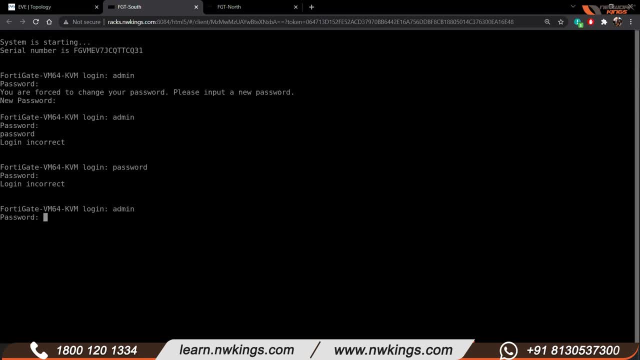 it is going to prompt me for a password and then i'll go ahead and you know, enter password, password, which is some confirmation. okay, so it says welcome, and now i have access to the porticate power. now, um relate this with cisco, so, um, all of you guys have any. all of you worked with ccna or have gone through the ccna course. 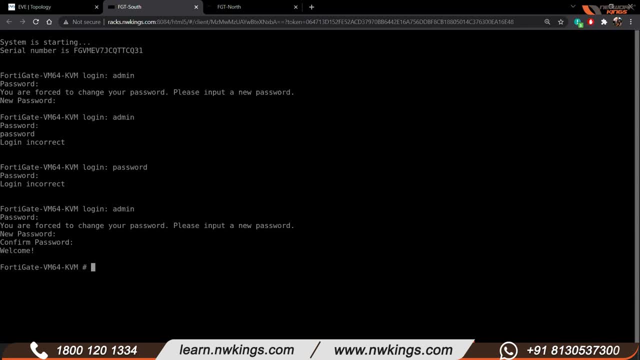 maybe, maybe, here or somewhere else, but have you, all of you guys, gone through the ccna? do you remember something? user privilege mode, global configuration mode- do you remember that? yes, whenever we get, whenever he used to get into the console, we also always get to say the. 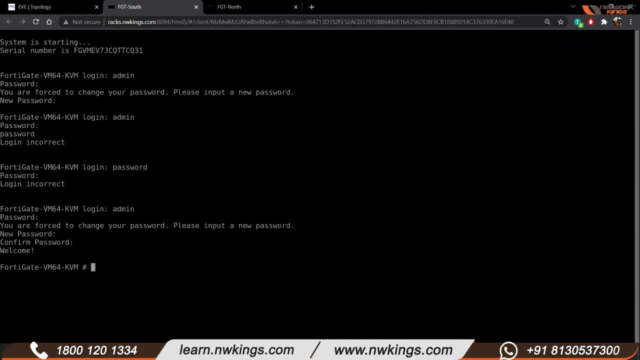 okay, this is. this is interface configuration mode. oh, this is global configuration mode. right, so we do not have something like that in the firewall, but i'm going to relate to that so that it becomes easy for you to understand. so see, this page is basically. basically, you can call this as a. 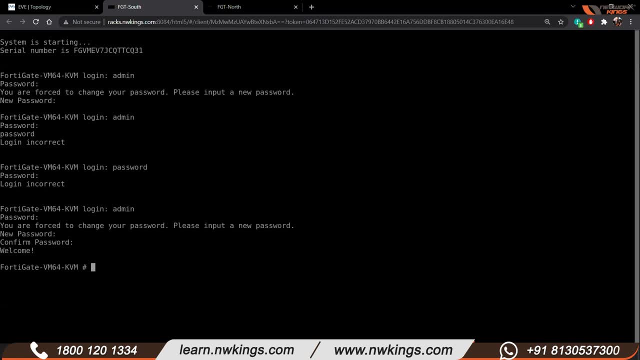 user privilege mode. okay, so you would be able to, you know, give uh basic commands, basic show commands that you can be, uh, you know, go for configure. you know, just to look into the configuration that you have, okay, uh, show commands are pretty uh, straightforward. but let's say, for example, you want to, you know, configure an interface. so how do you do that see? 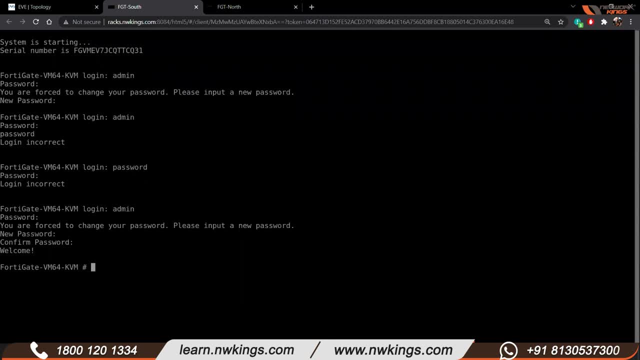 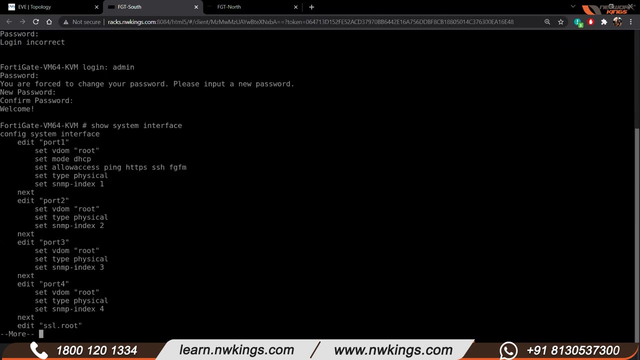 if i want to show, if i want to see the interfaces, the command says show system. because i'm actually looking at it- configuration, which is a system configuration. so show what system system, what interfaces. okay, and if i hit enter, it is basically going to show me whatever interfaces that i have. 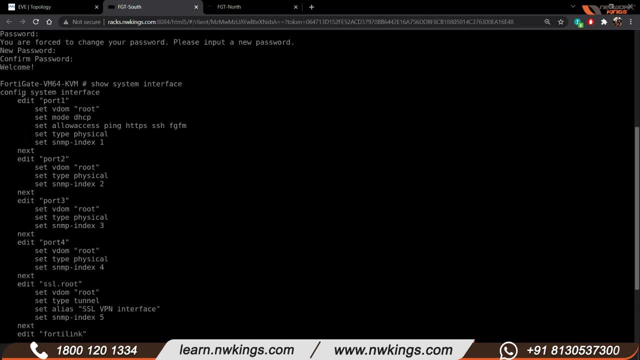 so see now, if i'll just little bit scroll up, it says config system interface. now see, this is the command. okay, do not bother, if it doesn't make sense to you right now, it's fine. but basically this command is able to tell you that these are the interfaces that i have. 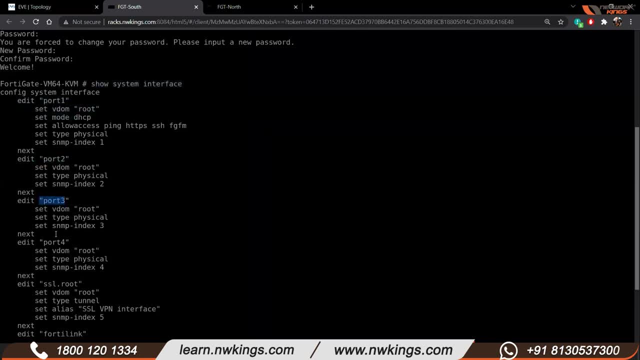 so i have put one. i have four, two, four, three, four, four. then we have something which is called ssl root- we'll talk about this- and then we have something which is called as a 40 link. okay, so consider this: you have four ports as of today. you think the list. how many points do i have? let's see, look, i can take two, maybe eight points. how many gates does that mean? i think two by a minute is JEM WAS THE KEY. JEM WAS THE KEY. JEM WAS THE KEY, like jm, where i think my command was built in. jась was the next level of, so you understand the Calledствие. hello is a domain, basically, and you have a. 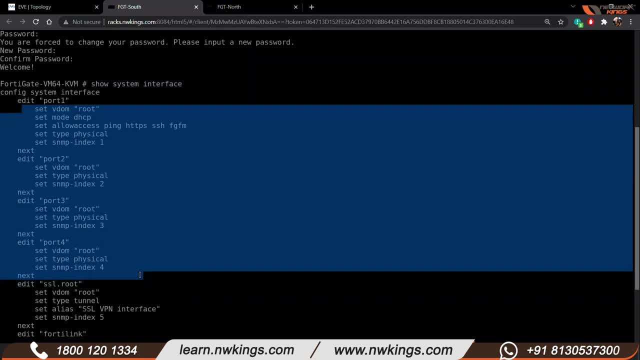 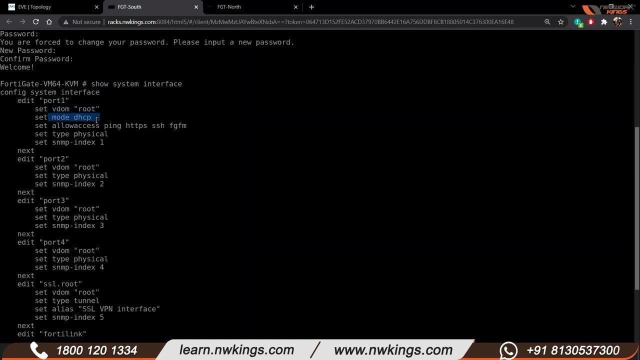 you have four ports as of now with this virtual machine. okay, all right. now see, one says vdom, we are going to talk about this, do not worry. then we it is. it says mode: dhcp. so it's quite simple that basically it is saying that port one is acting as a dhcp now, not dhcp server, it is acting. 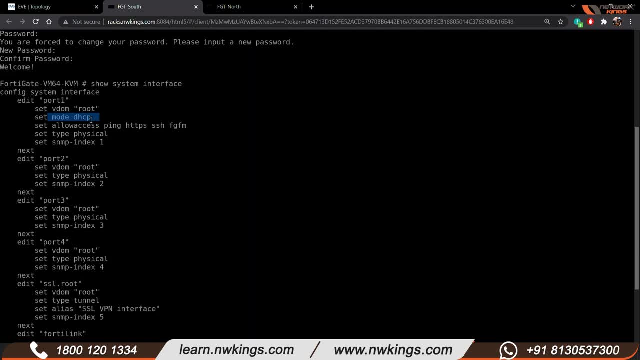 as a dhcp client. it is basically, uh, trying to find a dhcp server, trying to get an ip address, okay. so the mode dhcp basically means i'm trying to fetch an ip address. now look over here. in port two you do not see this mode option. okay, in port three, you do not see any mode option. 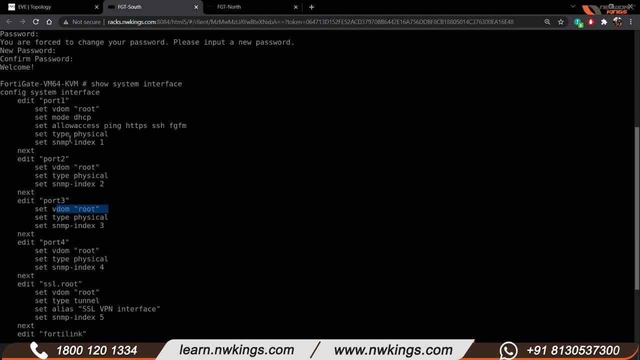 what it means from the fortinet perspective. this means it is a static entry. i have to manually get into the port two and then, you know, enter an ip address over here. okay, but if it has more dhcp, this basically means i do not have to enter an ip address. it should take the ip address. 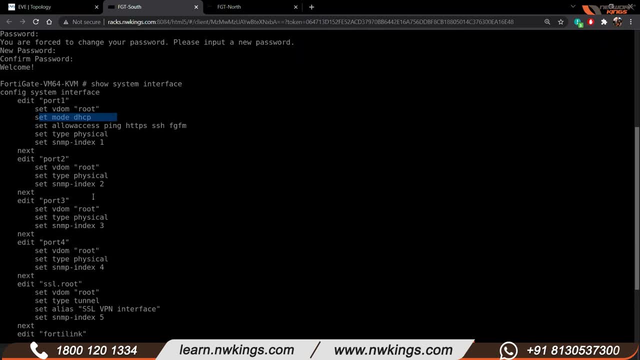 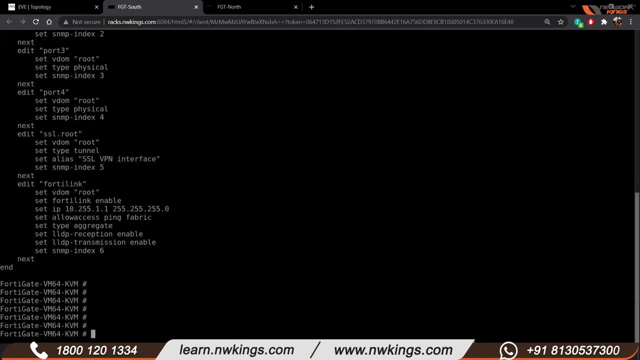 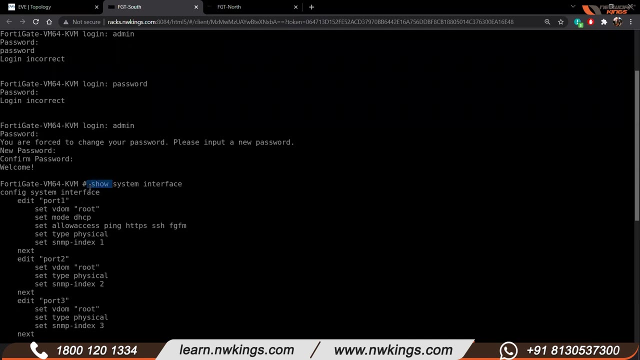 from a dhcp server. okay, so how do i see all the interfaces? show system interface. okay. now, if i want to configure an interface, the show command also tell me what should be the right syntax for me to configure an interface. so do you see this? it says config system interface. 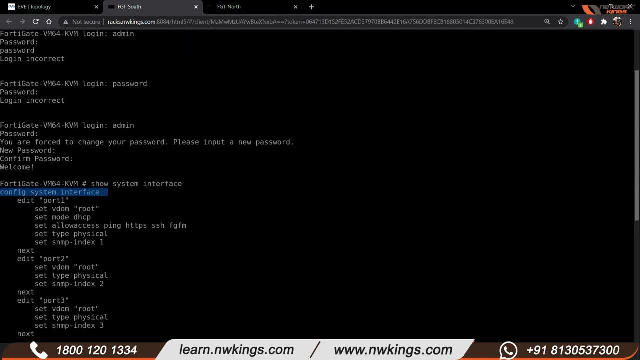 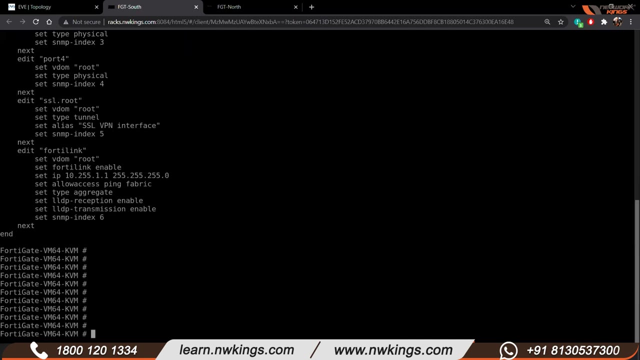 this is the syntax if i have to configure something. this is the. this is the syntax that i have to enter if i am, you know, configuring port one. this is the syntax i have to use if i am configuring port two. okay, so global configure. sorry, user privilege mode- show commands. okay, there are. 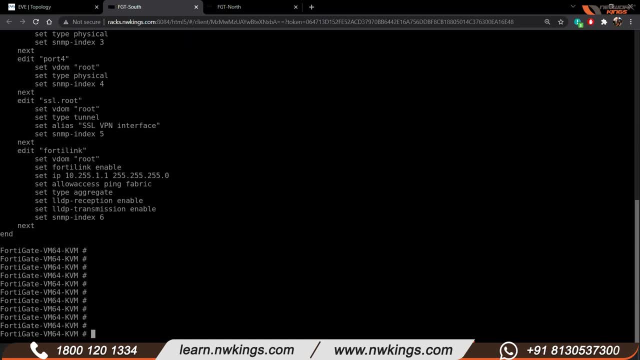 a lot of more commands. you know, uh, diagnostic commands and all that. we'll talk about that. but as of now, think of this as a user privilege mode where you are able to, you know, put in some user commands and put in some more commands. that is basically used to understand what kind of 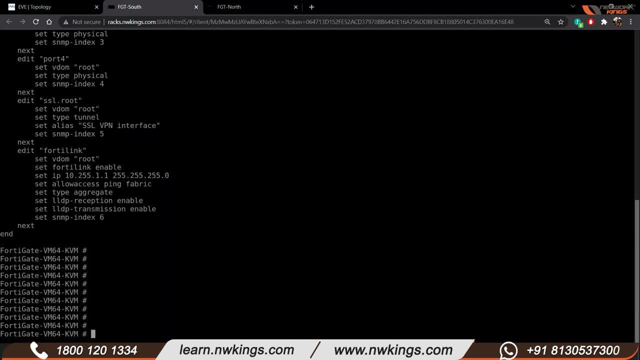 configuration that you are holding on this particular firewall. okay, then you have something which is called as um interface configuration mode, right from the cisco perspective. now, over here, what you do is: if i want to configure interface, what do i do? i say config. okay, because i want to configure something. right, so i'll say config now. 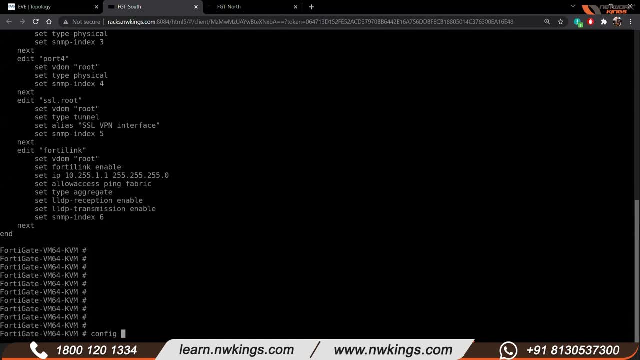 the 4d gate says: okay, if you want to configure something, what is it that you want to configure? so i say i need to change some system level settings. okay, what? what information do we want to change in the system? i say interfaces. so okay, this is the full command enter. now i am. in what mode from this script? terminology. 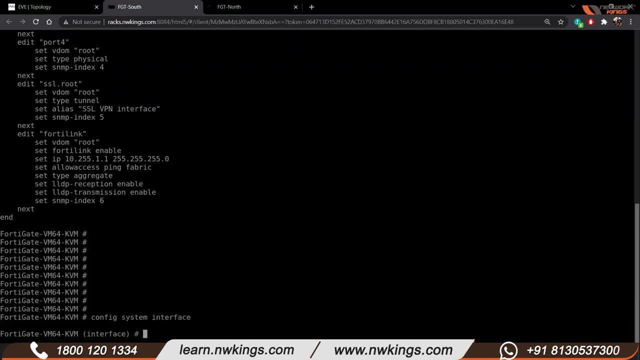 this is called as interface configuration mode. okay, now do not get confused that these are also something which works on 40 gate, user privilege mode and global configuration mode or interface. this is just to relate, okay, so that you understand that if you want to change anything where you want to go, okay, so now i am in config system: interface. 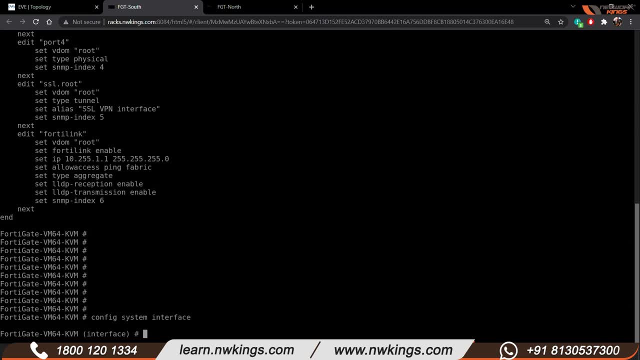 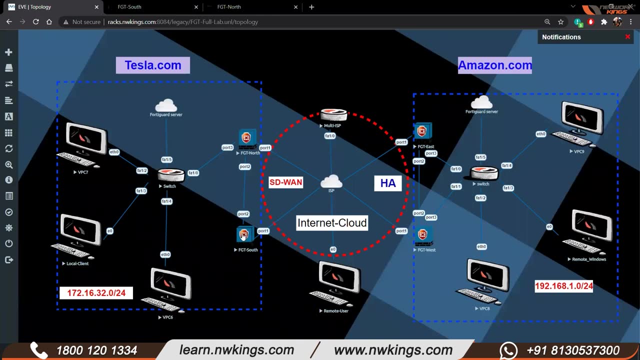 this command do? it will basically help me to configure interfaces of the 48 firewall. so let's say, for example: let's see, so i'm in 40 gate south right now. 40 gate south has a port connected to 40 gate north on port 2 right, and then i have a port 1 which is connected to the isp. okay, now do. 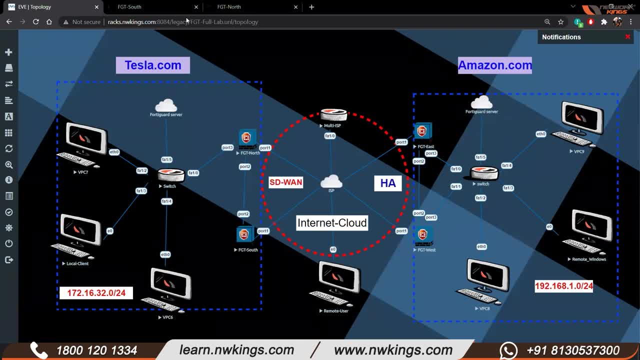 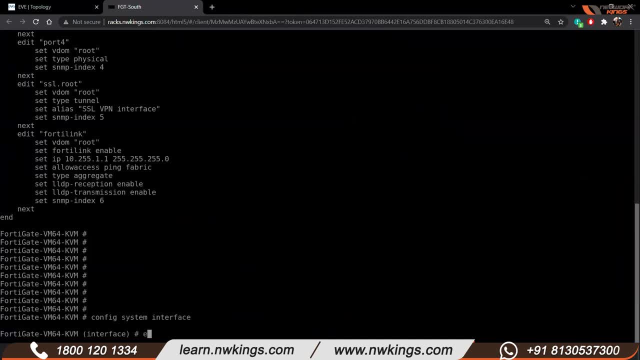 you remember this port 1 was dhcp, right? so i should be able to get some ip address, am i right? so what i'm going to do is let me come back. okay, i'll introduce you to one more command which says: now do you remember the last command, show system interface, right? what does it do? it basically show. 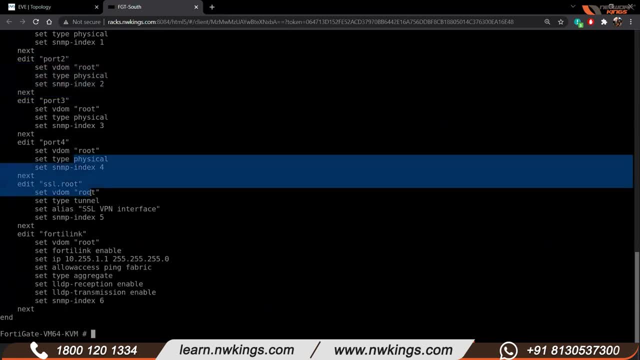 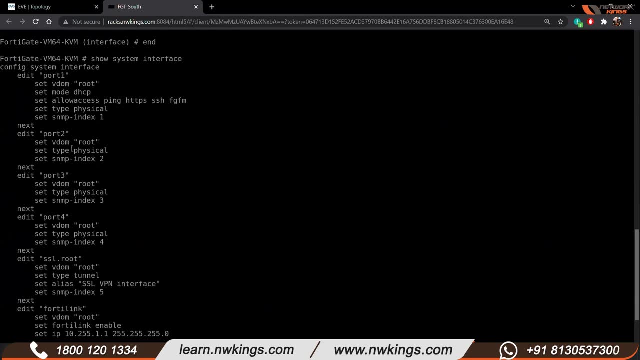 me the correct syntax value plus whatever ip address. if it is configured, it is going to tell me that, right, but as of now it is a brand new device, it does not have any configuration, so it is. that is why it is not showing me any ip address. now there is one more command which is called as: 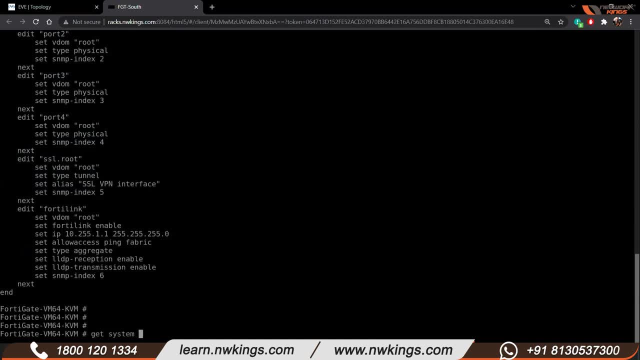 get system interface. let me show you get system interface. okay now, there is a slight difference between the show system interface and the get system interface. okay now, what is that? see, show system interface basically helps you to understand the syntax and information which has been uh stored in the configuration. okay, get system interface basically tells you that, whatever, 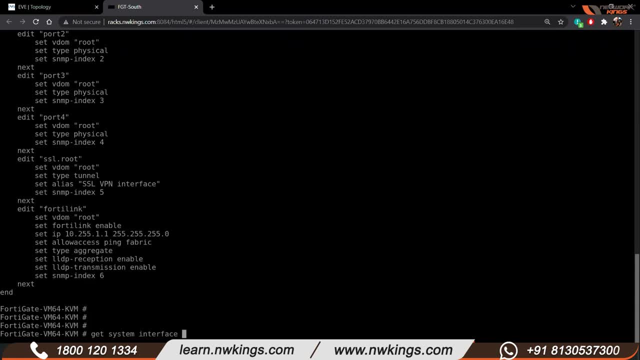 is there? what is the result of it? okay, so get command basically tells you about the result, the output, and show command tells you whatever the configuration that you have. is it clear all of you? yes, no, show command will tell you. whatever the configuration is, get command is going to tell you. 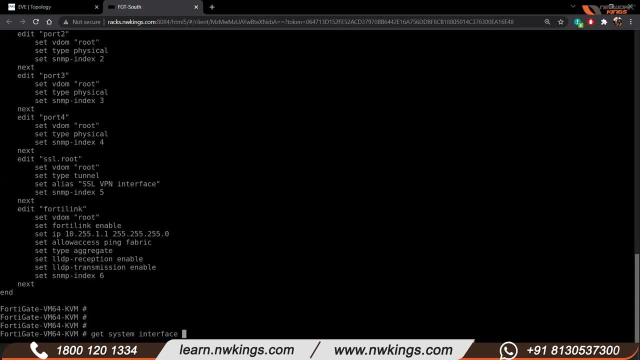 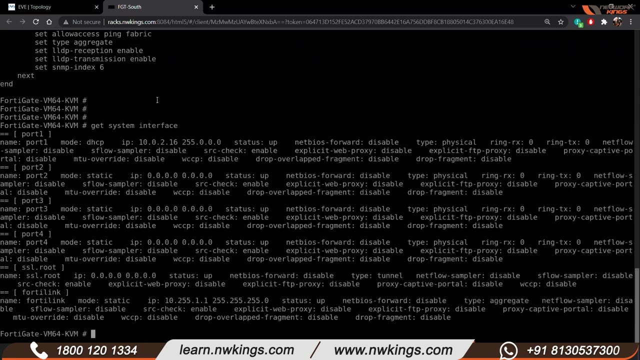 what is the output of the configuration? all of you, yes, no, yes, okay, good, so get system interface. i'll execute this command now. you see how the result is a little bit different from one what we are getting previously. see. now it says port 1, dhcp. but see, you are getting the ip address. okay, because in the show command it. 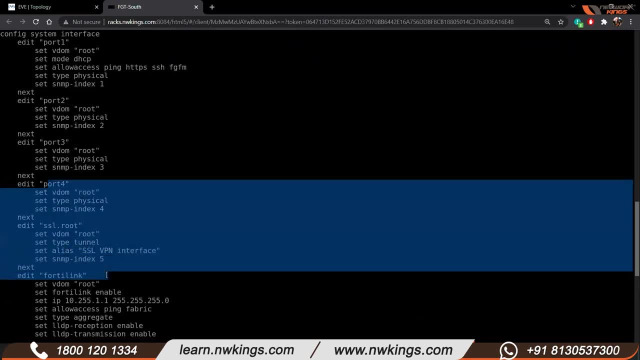 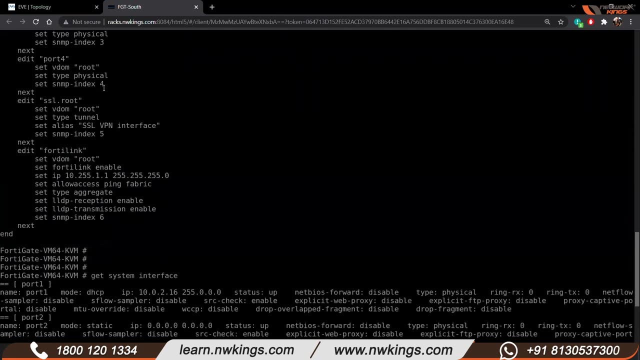 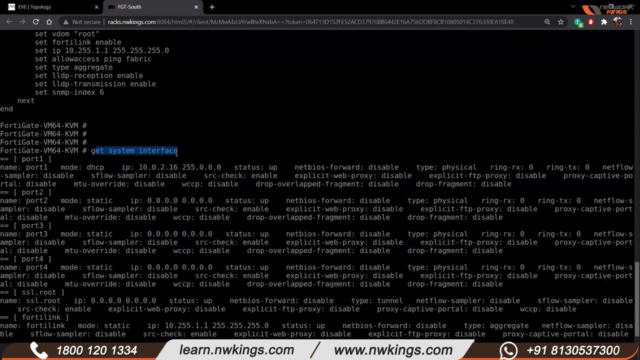 is only going to show you information or the configuration, which is manually, you know, configured over here. okay, but the dhcp is an automatic thing, so, as a result, i have to see the ip address. so if i have to see the ip address from the dhcp, get system interface is a good command to use, okay. 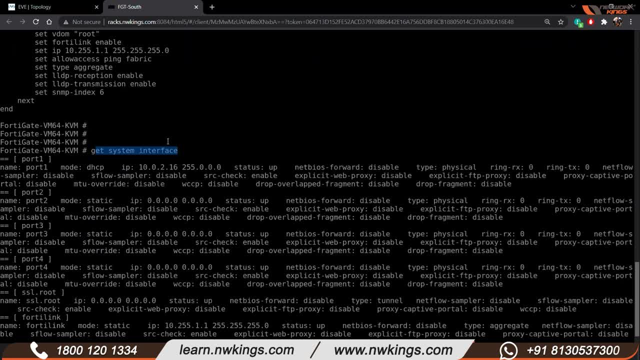 a lot of people, a lot of engineers who basically work um. see what happens is, i'll tell you a classic example. so one of my students is working in one company, and not name that, but in that particular company he only has access to the cli. he does not have access to the gui of the 48 firewall, all. 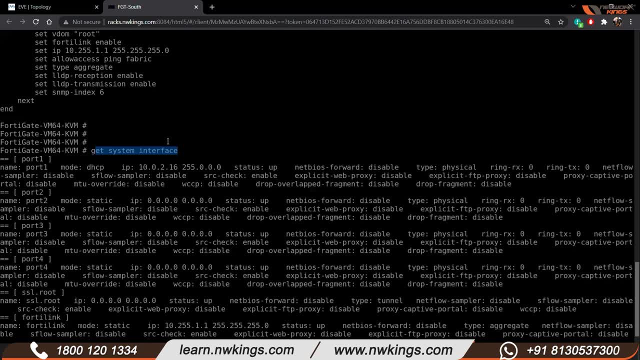 right now. he had certain interfaces which was configured for dhcp. now he was having a very, you know- hard time to understand that. okay, what do i need to do to get this uh information? all right, so i have. he called me up and you know it was still um very early for him, so i told him: okay, so 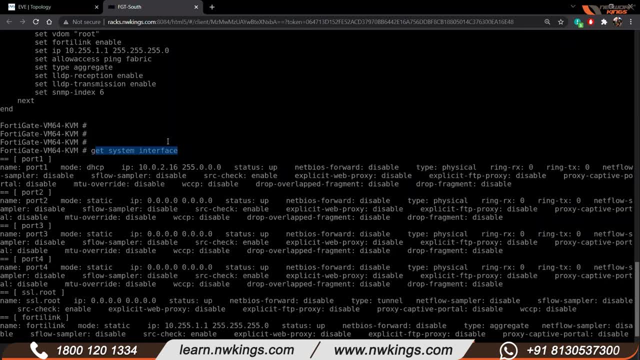 just go ahead and execute this command. you will be able to get the ip address. so he did that and he was able to get the information. so my point is that whatever we are going to teach you will basically help you on your practical implementation with whatever job profile that you are, you know, going to work on, okay, or maybe whatever job. 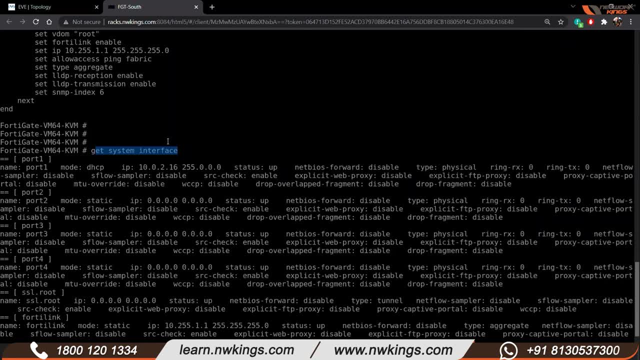 profile that you want to work on. okay, so get system interface. basically tells you about the information or the output of the configuration. so we know that. okay, 10.0.2.16 is the ip address on port one, but do you see any other information? see port two: zero four. three. zero, four, four, zero. right, why? because 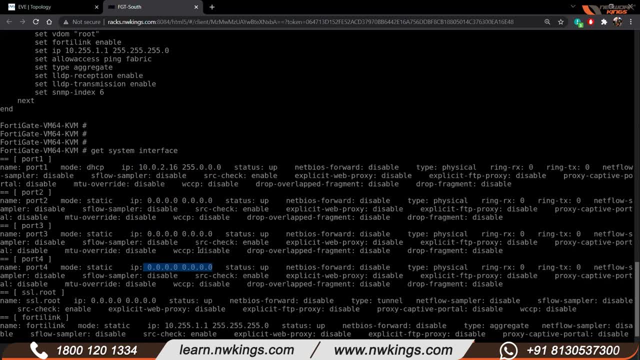 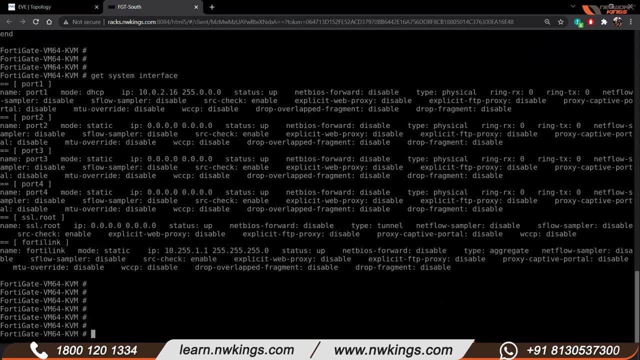 this is manual information. all right, it is not yet configured. so get is all about output, show is all about whatever the configurations. okay, all right. now i'll go ahead and tell you one more command which is used in the kind of user privilege mode or this mode that we are on. okay, very much important and very much required. 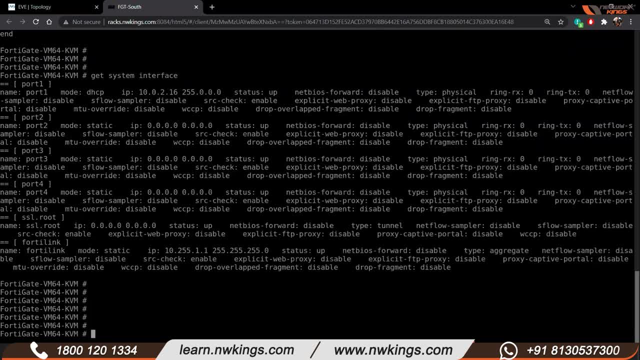 for you to understand if you are working on a forticate firewall. okay, so get. okay, get, you know right, whenever you see this, you know right, you know right whenever you see this, you know right. this: get information. you know that. okay, whatever the, whatever the display will be, it will be output. 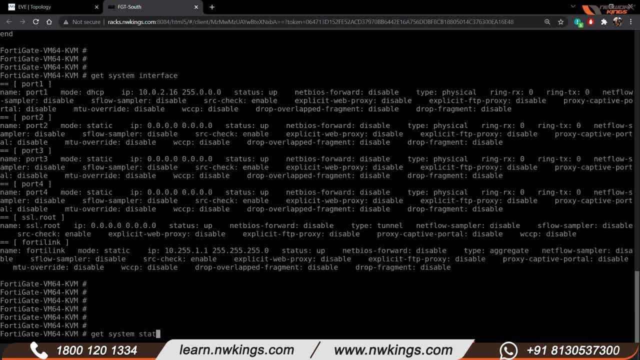 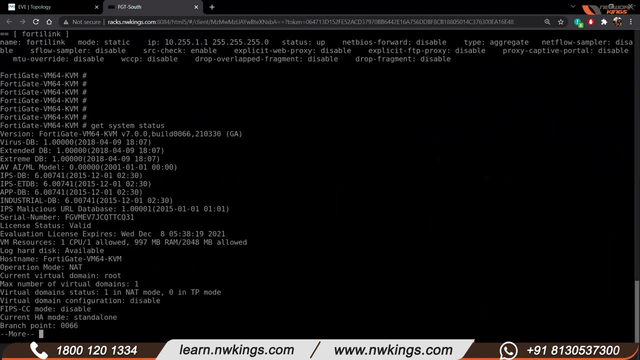 okay. so get system status. get system status basically tells you about the current um. you know the current setup, the current status of your 48 firewall, so i'll hit enter. okay now, see you, you're getting a lot of information over here now, um, i'll just quickly let you know whatever information which. 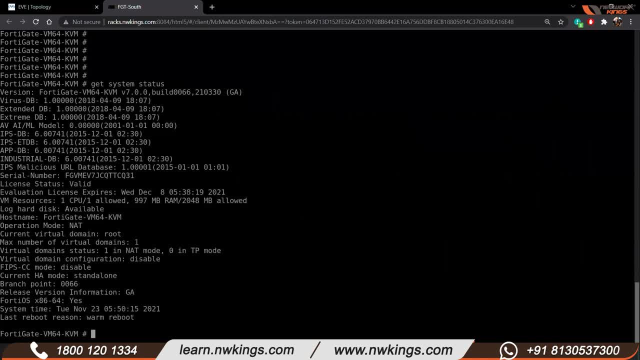 is um easier for you to understand and grasp. okay, see, this is the command. get system interface. so i get system status. see the next lines here. version- what do you mean by that? version basically tells you about whatever is the current operating system of your four digit firewall. see, remember, right uh. 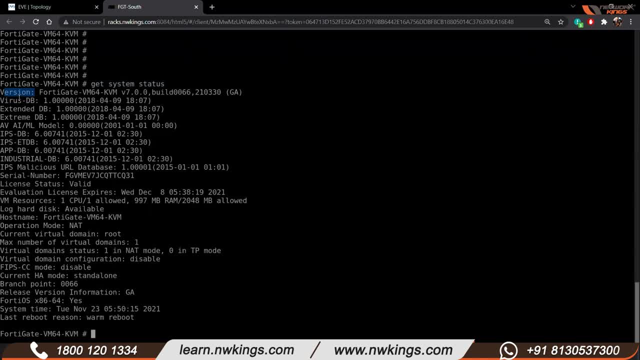 last time i told you maybe, yes, i uh, yesterday we were talking about that- um, it is like understanding or learning windows 10.. if you know windows 10- sorry, windows 10, that's right, it must be right um windows 10- then doesn't matter if you are working on lenovo or you're working on an hp or you're. 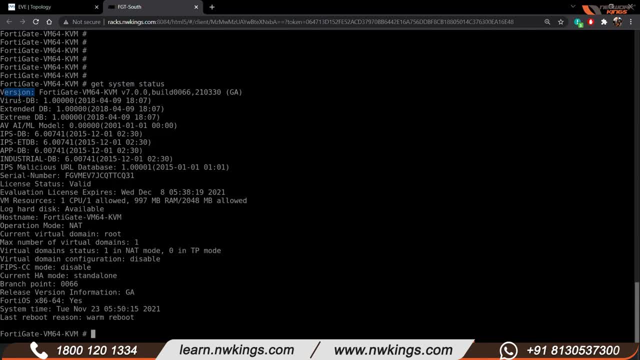 working on a dell doesn't matter, right? so over here fortigate is running a non-operating system. now operating system, because basically over here you can say version. so what version it is, it says the version is fortigate vm64, which is basically, uh, the vm. it is telling you that this is a vm. 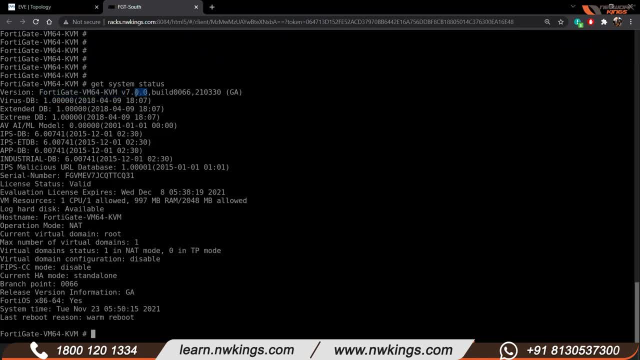 and then it says it is running on something which is called as v 7.0.0. now i'll tell you what the 0.0 is later, but as of now, just consider this that it is an operating system which is called as v7, and that is the operating system i'm working on. anybody can tell me what is this ga? 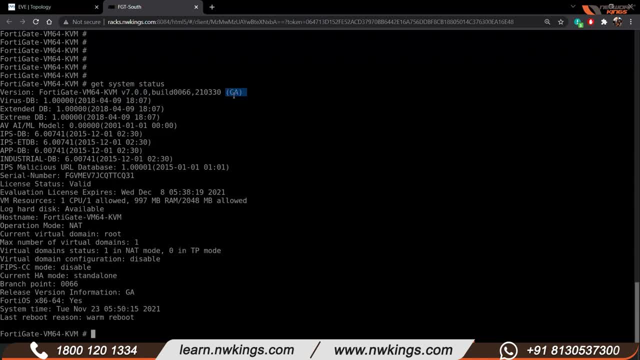 anybody any idea? wild guesses, even that will. that will also work. anybody who knows what is ga? no, okay, see, ga is called as general availability. okay now. general availability basically means: now, this is not just for 40 grid, it basically applies for all the you know vendors out there. 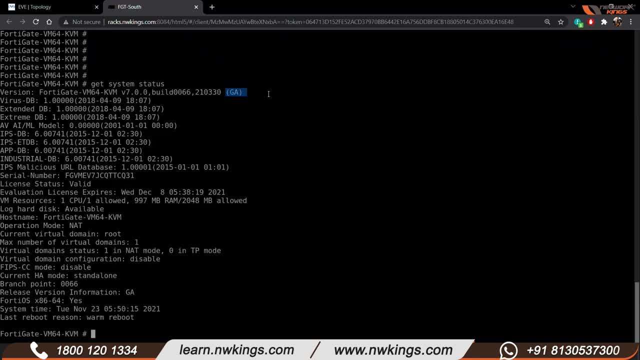 all the firewall vendors, cisco palo, checkpoints, cyber rom, sonic or whatever it is. ga basically is general availability. that means there is an operating system. this operating system is a general availability. operating system that means that it is, um, it is being uh, um, you know, given out. 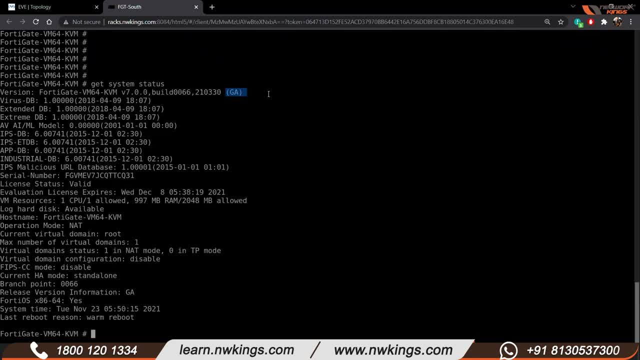 by the vendor to be used by all the models that uh can be used. so let's say, for example: um, the clients can be anywhere around the world, right, they log into the portal, they download the image and they'll go ahead and upgrade the 40 grid firewall. but they have to be very, very, very. 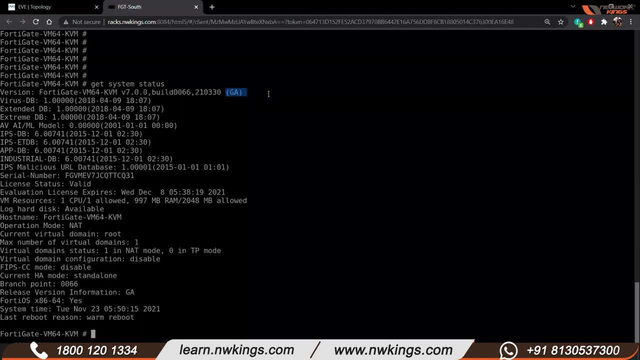 careful that whenever they are downloading the image, it has to be a ga general availability. okay, uh, it's considered. as you get windows, then you get windows beta, right, there are certain users, there are certain individuals who get beta operating system so that they can test out, okay, but that is not available for everybody. for everybody, there is a general availability. 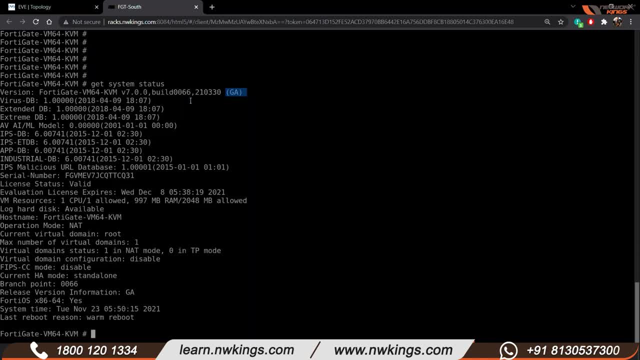 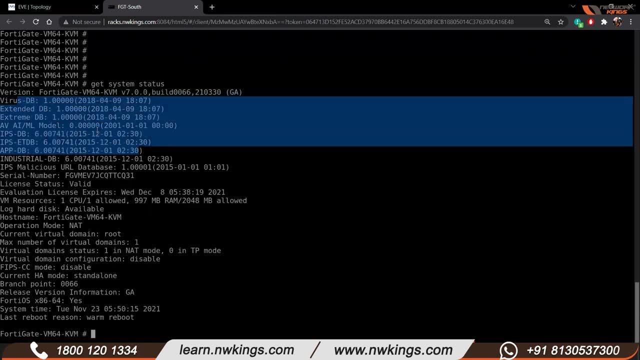 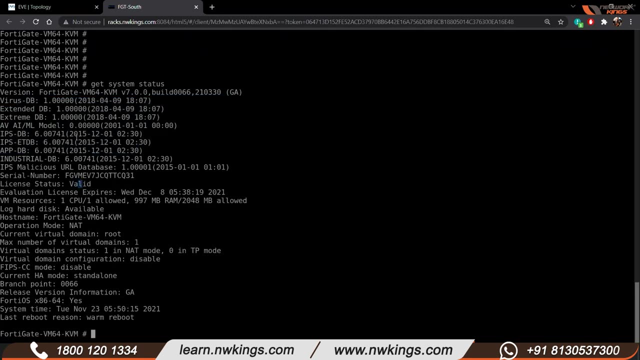 operating system. same goes over here as well. see, the next is called as the virus database. then you have extended database. now these database obviously are. if you look closely, these are: look at the value, look at the time frame: it's 2018. one is called as. one is on. 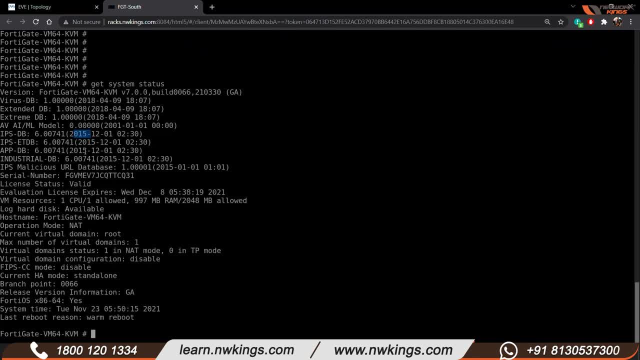 2015. do you know why this is? see as of now, we just booted up the 48 firewall. that is one second. this is an evaluation license, so it will not give you the updated or the existing signature database because the firewall is still not licensed. okay, once the device gets. 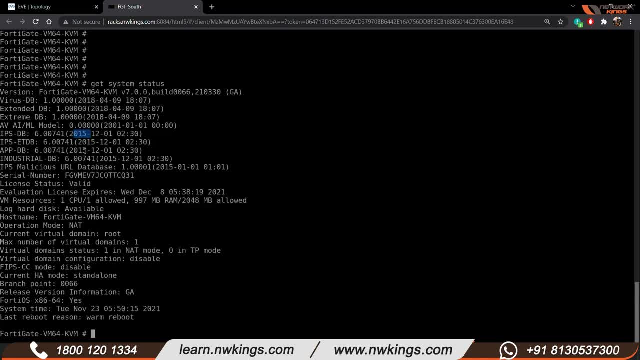 licensed, it will start taking up the latest updates. okay, you see, next look over here. i'll highlight this up: serial number: very much important whenever you are trying to work with the tack, whenever you are trying to uh. so let's say, for example, you have a environment where you have multiple firewalls. okay, you have to ensure that before. 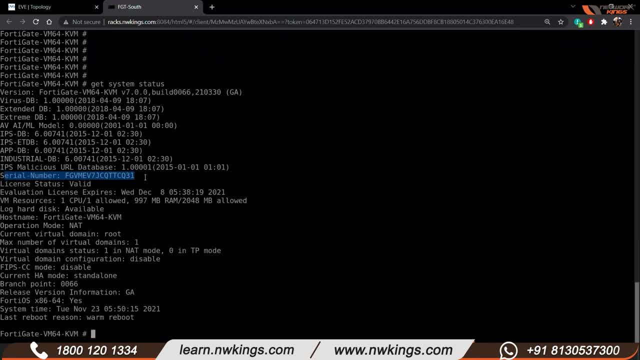 you make any changes to the firewall, you should be aware that which firewall are you on. okay, so the serial number. always make sure that you understand. okay, i'm on this particular firewall. okay, then this license status. it basically tells you that this particular operating system is it valid or not, because if it is expired, you will not be able to get access to the. 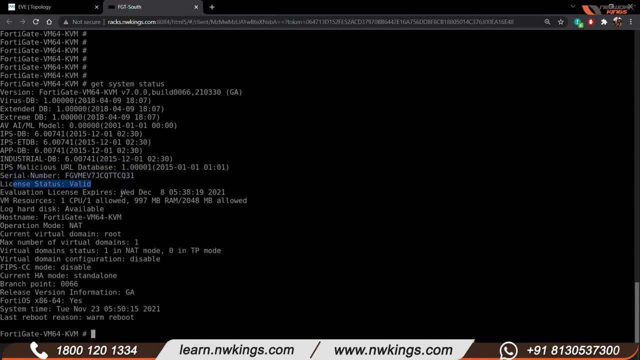 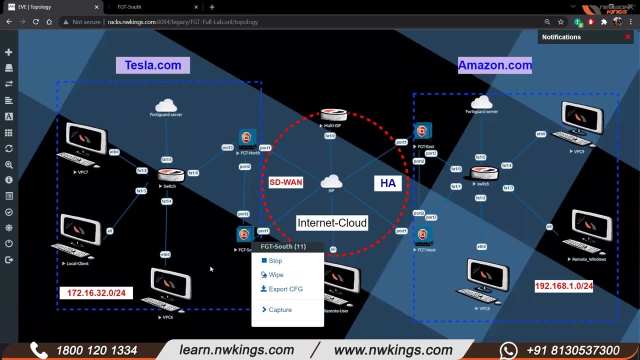 cli or the goi. okay, so you have access to this in mid-餐 8. what happens after that? any idea nothing. you remember what we did. you go ahead, right click, click on wipe and that is it again. you have factory formatted the system and then you will again have audio and also you will have yourself templated. 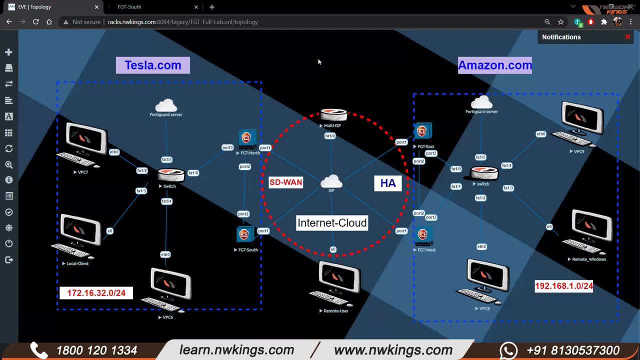 your license and if you have a first-time没有 login call you show phảiable cd, then this is 하고 isg. they a copyrighted license. they are part activity aboutTake from this aussi 15 days more. okay, now do not worry that what will happen to the configuration or whatever. 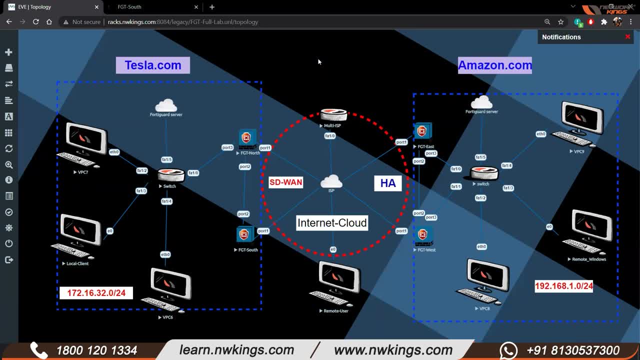 uh, you know changes we have made. what will happen to that? we are going to save those configuration changes- factory format- and then upload the same configuration changes, right, so you do not have to, you know, waste your time. you know, changing the information again and again you would be able to. 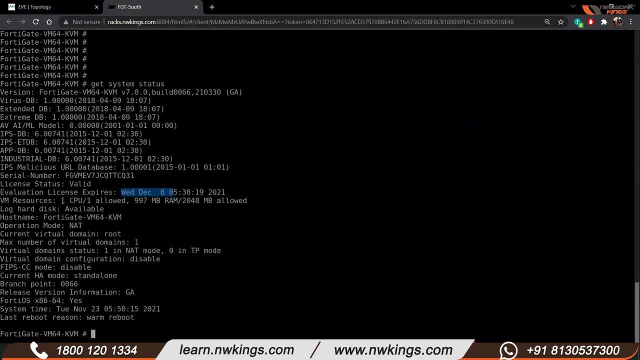 do it okay, all right, so let's go back. so now this over here says about the resources that is allowed to you. now see, we are working with evaluation license, right, so you are going to get one cpu and around 2 gb of ram. that is the limit. hi, you are watching the recording from one of our live. 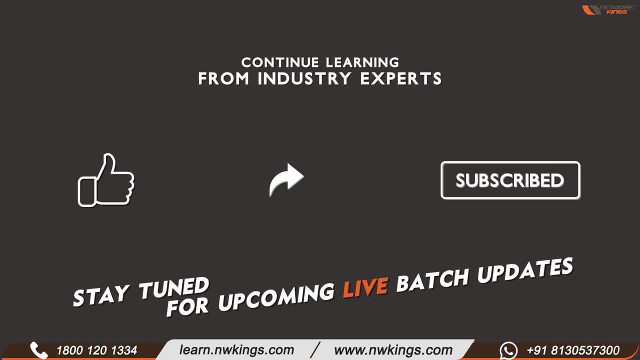 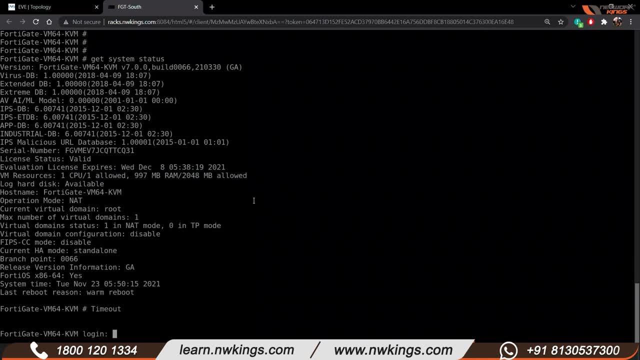 session. hit like share and subscribe for more future updates for you now. ideally, the vms that you have can go around 64 gb of ram, even more than that. there there is, there's a, there's a huge range, just like we saw yesterday for the hardware devices. same has. 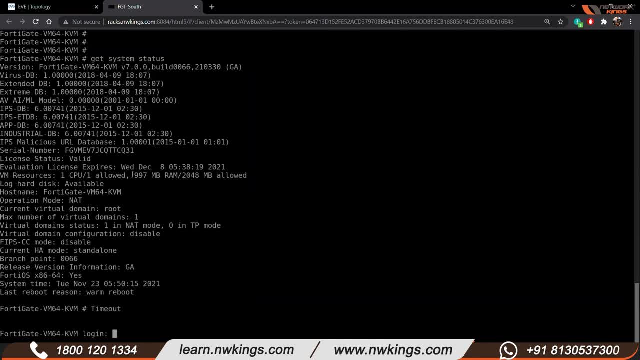 the same concept applies to the vm as well, but then, since we are in the evaluation license, this is the limit. okay, it doesn't matter to us, because anyway we are able to work on it. so doesn't matter. log hard disk, log heart, is basically that, it is a it just like your windows operating. 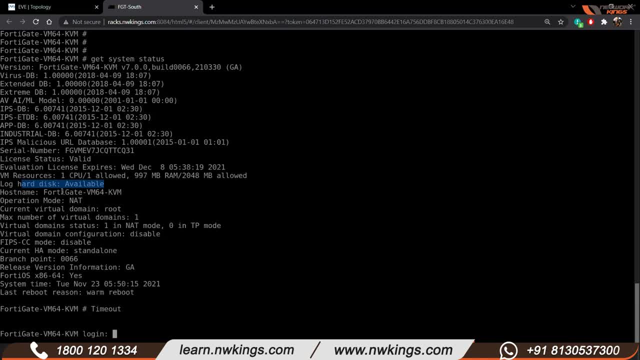 system has a hard disk of 500 gigs, maybe 1 db or 2 tv, just like that. you have a hard disk for 48 firewall as well. okay, this could be 1 tv, 5 tv, 10 tv, depending on whatever the hardware model you have. 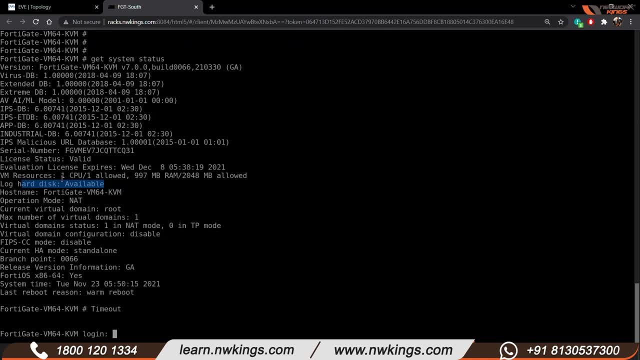 and if you have a virtual machine, then basically depends on you how much space that you want to give. it is up to you. okay, then you have the host name now see host name says 48 vm, 64 kvm. this is the default. you can always change this. we are going to tell you that. then you have something. 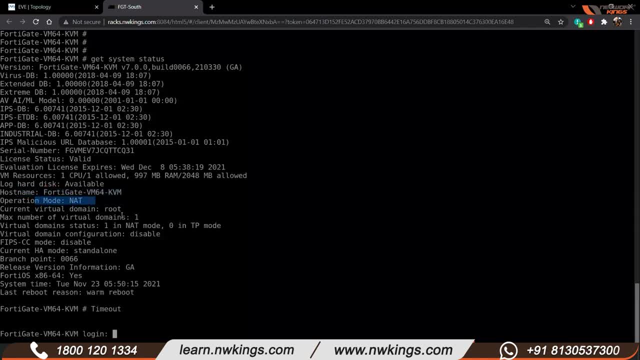 which is called as the operating nat, or sorry, operating mode which is called as nat. okay, now again, this will all be covered. that, what is a nat mode? what is a transparent mode? okay, how is it so? look over here. you have a current ha mode. then it says standalone. so standalone basically means 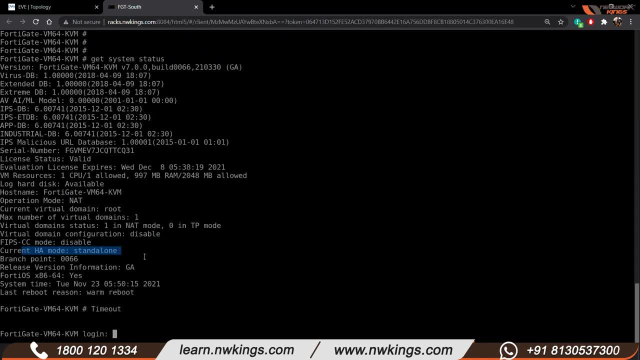 that, as of now, i haven't configured the high availability right, so it's a standalone device. now all this information is available on the get system data, so you know that. what is the time, what is the operating system, what is the operation mode? is it nat mode or transparent? 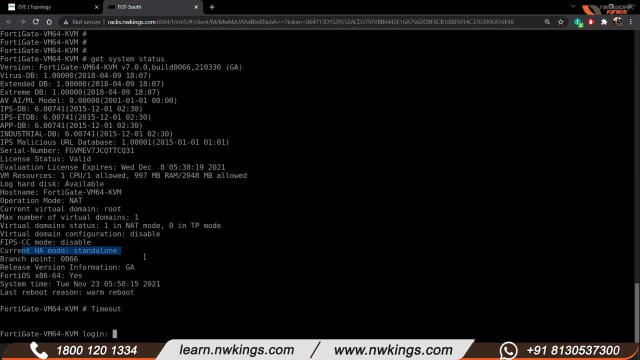 mode? what is the ha mode? is the standalone mode, or is it the active, active or active, passive it? all these information you would be able to get from this one command. okay, and just to give you a hint, this question comes in your exam as well, if anybody wants to. 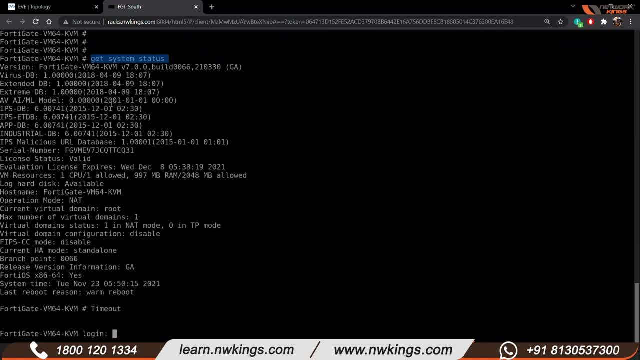 get the nst4 certification. this kind of information are asked in the in in the examination, not directly. that. what is the command that you will be using? basically you'll be giving you. they will be giving you a scenario that um tom is the firewall administrator and he is new to the. 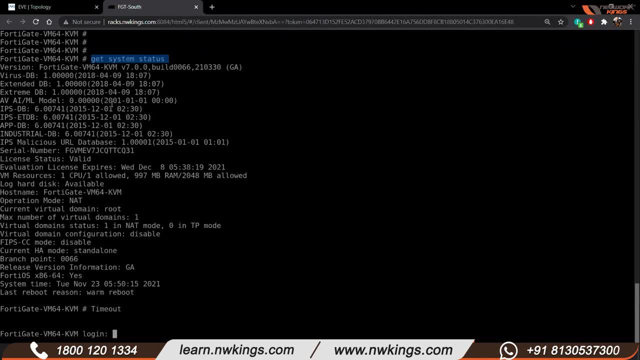 company. he would like to get information about the firewall and he only have access to these um four commands. which command he will be using to get this information? and then you will get you know multiple information and then you have to select the one which is the right. so you are going to select which one: get system status. okay, all right, is it clear? 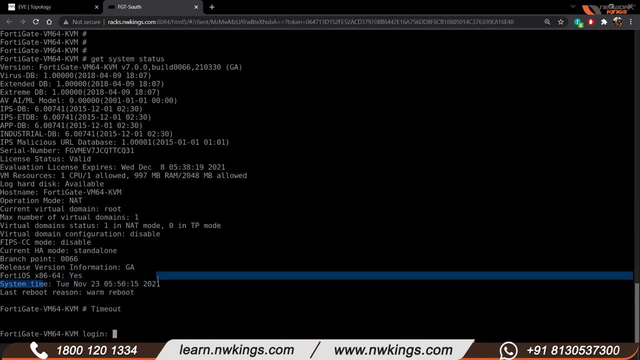 yes, okay, right now, system time again is basically to tell you that whatever- so see, this could be different. whatever your- you know- um location is, according to whatever the firewalls location is, you would be getting the different time. this is, you can change them as well, so every information can be changed, okay. 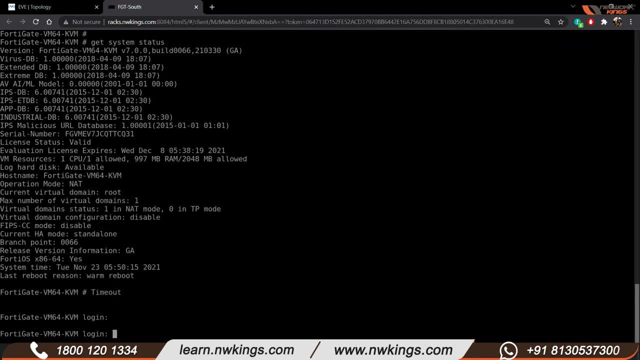 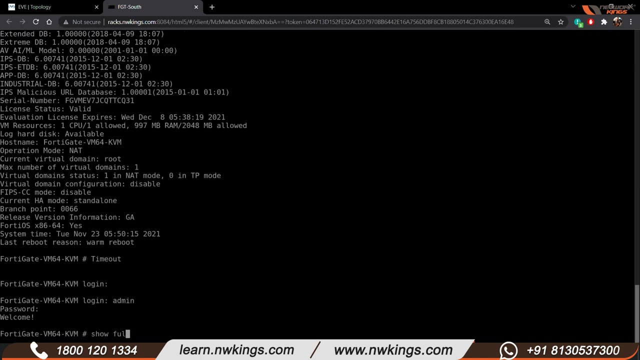 all right now. see, uh, what we discussed right now was mostly about interfaces, was mostly about you know how to get the information from basic commands- show commands. okay now, uh, do you remember that in cisco we have um, a command which is basically called as show? right, so you have show running configuration. so we also say the same thing. but then i'm 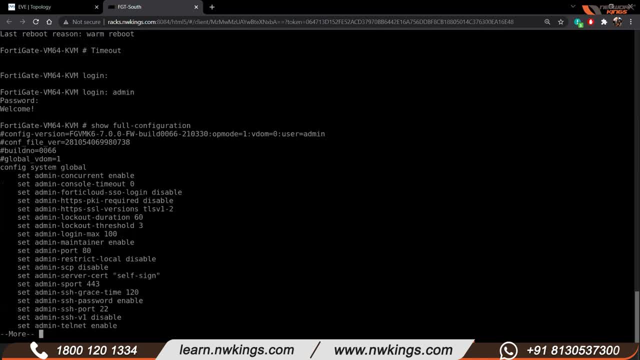 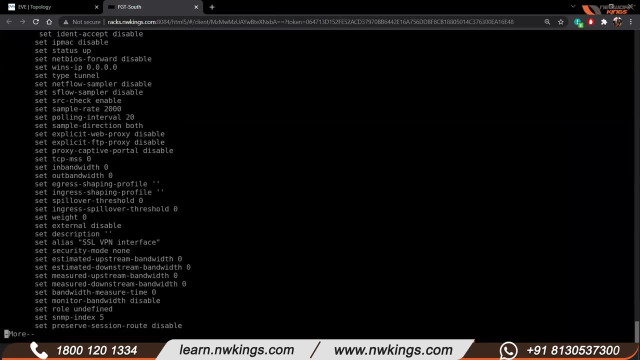 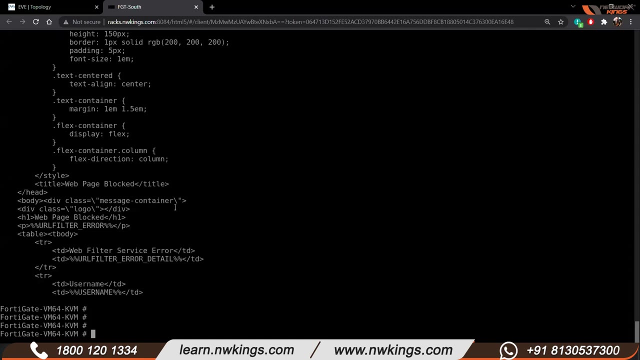 saying show running configuration, we say show full configuration. okay, this is also more or less the same thing, and you would be able to get all the information or all the configuration that is there on your photograph, all the default configuration plus whatever changes you have made. okay, all right, now let's go ahead and configure an interface, you know. let's. 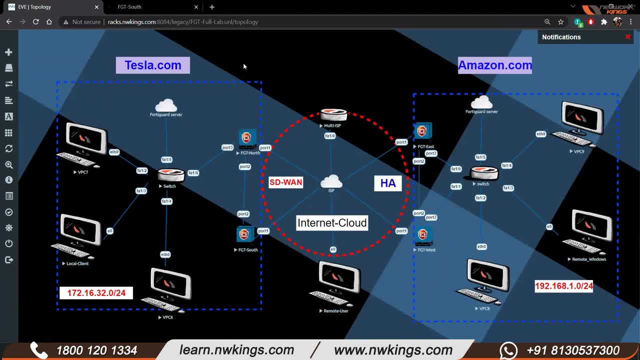 you know, you know discussions right. so let's do one thing: we'll take up the forticate north firewall. okay, we already have a local client connected to the switch. hello, yes, mayakush. maybe actually the as of noise is so um, um, um. we will configure interface as port 3. 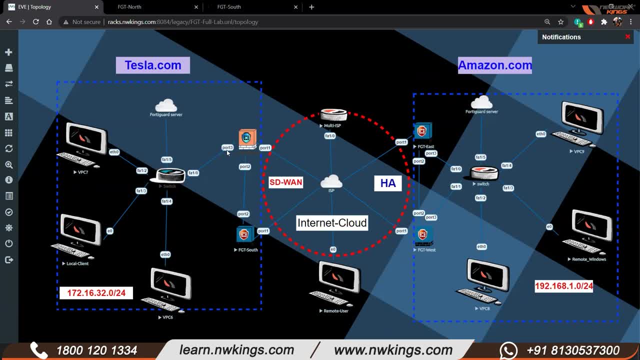 see port 3. we will configure this port 3 and after this, we will connect and check whether we get accessibility or not. ok, so, guys, what we are doing over here is we are going to configure port 3, ok, with an ip address, and that ip address should be able to reach. 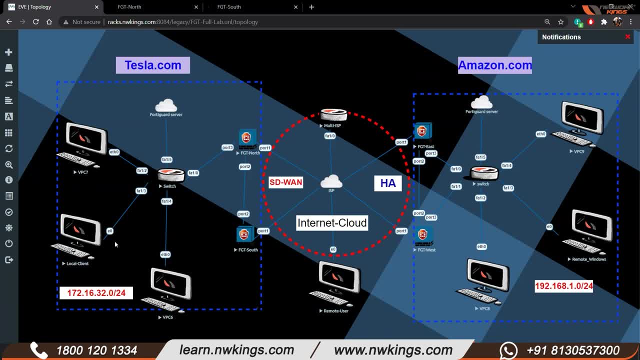 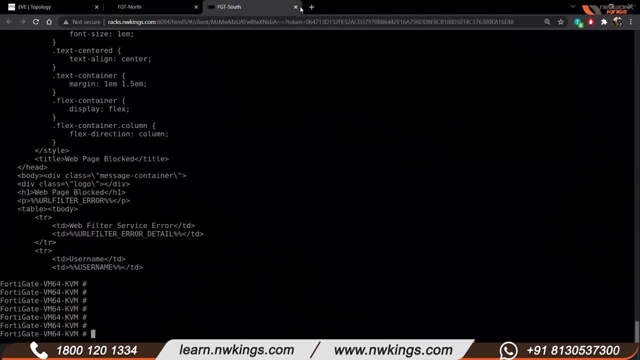 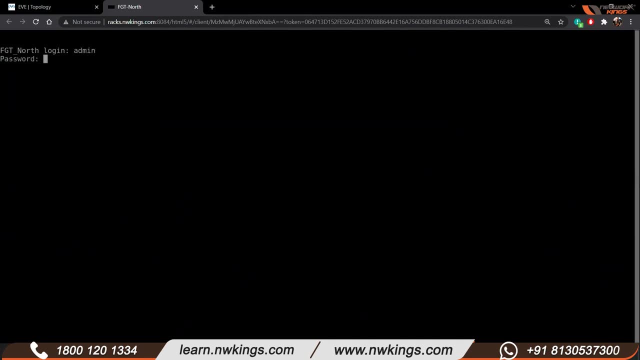 from the local client that we have, and we should be able to get the GUI page of the firewall. ok, so let's click on this, let's go over here. hmm, so let's login admin password. ok, alright, now remember whatever. ok, who is going to tell me what was the command I used? 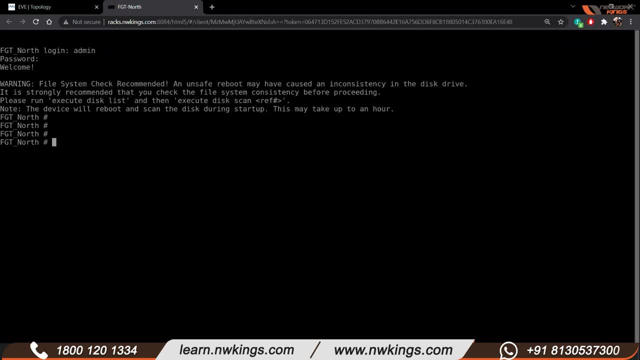 to get into the interfaces. what command I used? anyone remember? yes, config system interface. config system interface. very good, I like you guys. you guys are very good. config system interface. port number which port? port 3, port 3: good, ok, so now we are under interface configuration. 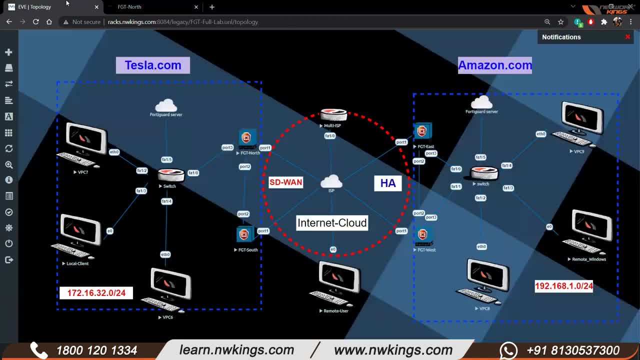 and we are configuring port 3. ok, now what I have to do is I have to make sure that whatever ip address I am giving to the local client, I should have the same ip address on port 3, right basic networking. two network devices can only communicate with each other if they are. 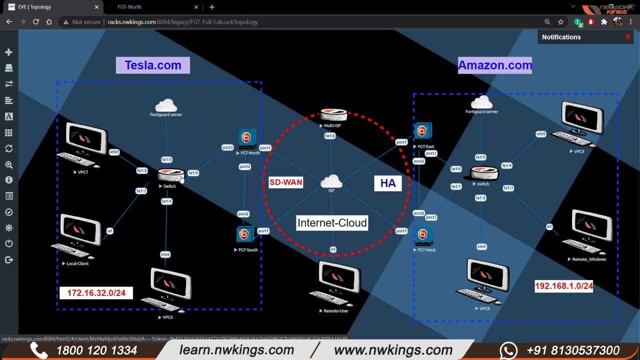 on the same segment. ok, two network devices can only communicate with each other when there is some kind of connectivity between them. if they are on the same segment, ok. so what we will do is we will give both of them one ip in the same ip address segment. 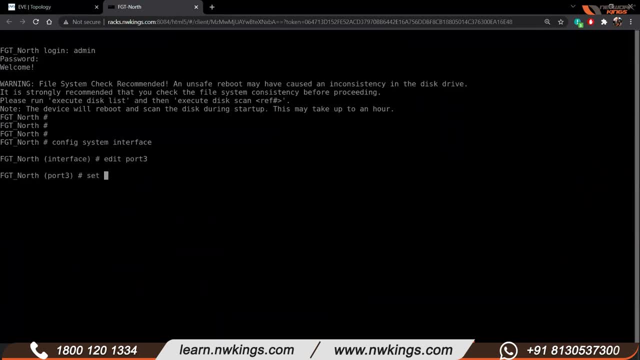 ok. so how do I give an ip address? you say: set, set mode static first. if we need static ip, hmm, very good, then enter, then ip. so I say: ip set ip. sir. ok, set ip. ok. so let's give an ip, let's say 16.1. 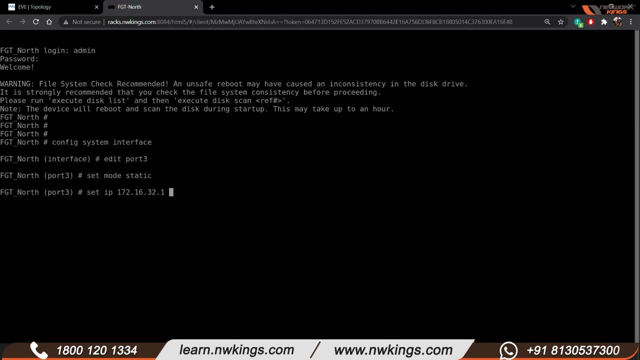 ok, so this is the ip address. now what happens is in cisco. normally what you do is you give the subnet mask. how do you give the subnet mask 255.255.255.0 right? what can the client do? you can also do what I have shown. 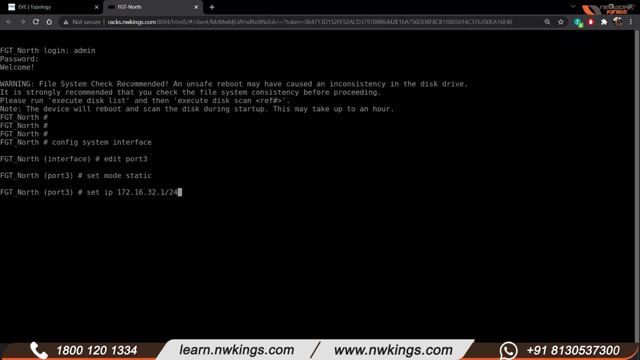 255.255.255.0, 24. yes, then enter right, so we have entered this. after entering this ip: see, if it does not take the ip, it will give you an error, ok. but if the syntax is fine, it will give you no errors, ok. 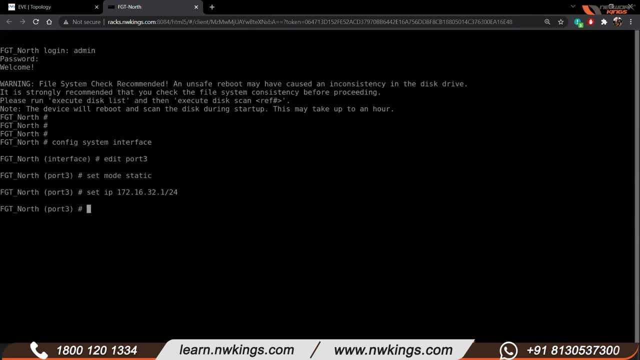 ok. so what we have done right now, we have given an ip address. ok, now there is another command. we have to run another command: allow access. why we have to run this, sir? for permission to do it or not. to allow https, everything is allowed. this allow access. 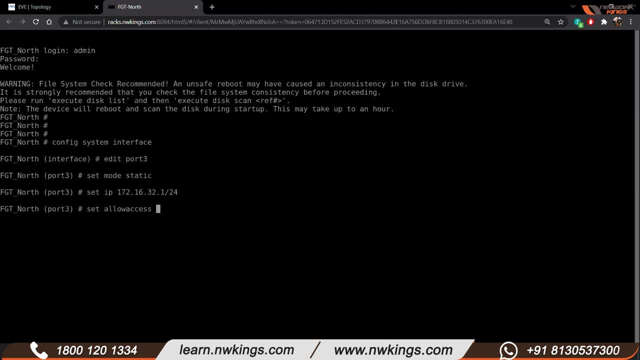 we basically do it because if we have to ping this interface, if we have to ssh that interface, if I have to take the https of that interface, then I should have that service enabled. if that service is not enabled, then how will I take it? I will not get access. 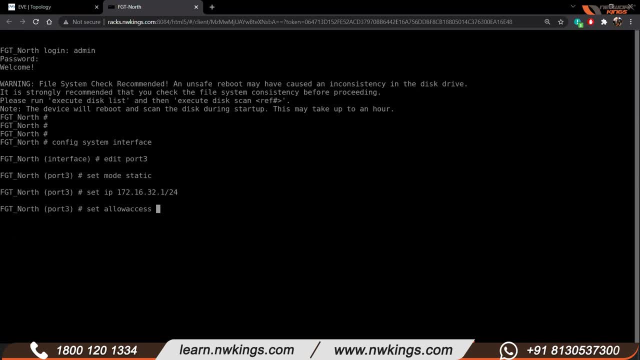 right. so what we are doing over here is, by using the command of set allow access. set allow access. what you are doing is we are allowing the FortiGate to basically entertain any request for ssh, maybe https, maybe telnet, maybe ping, whatever it is. so I will say that set allow. 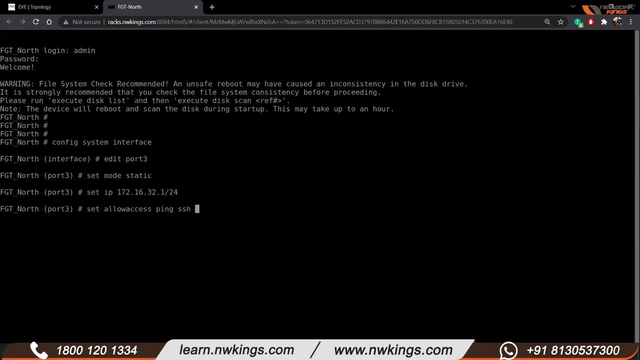 access and I say ping, I say ssh, I say http, https, this for now. this is more than sufficient, so I say enter. ok, now I can use a command which is called as show. what will happen with this? with show command, we will get to know what all configuration we have done in this interface. 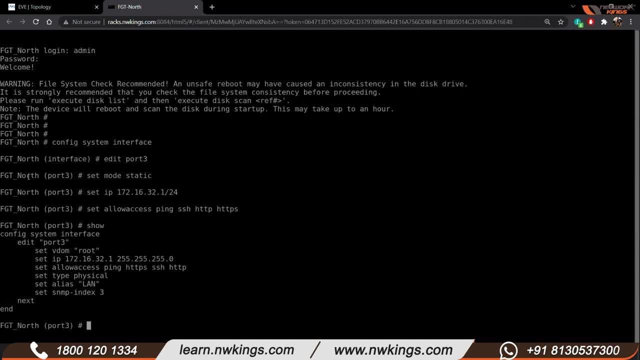 ok, if something will be miss out, then we will get to know. see what it is telling us. see this syntax is telling us: config system interface, edit port 3, then after that leave vdom. then see this IP. we have put IP. it has told 7th mass. 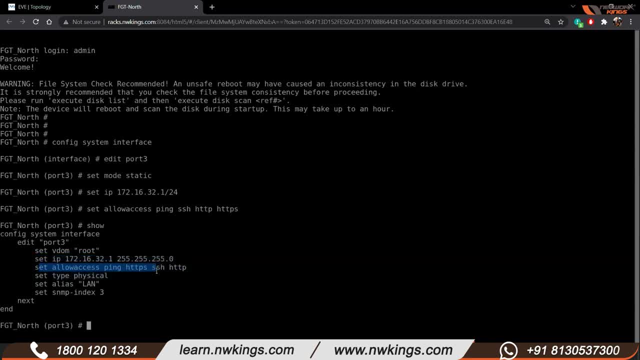 that this is IP and 7th mass. then it has told that you have ping http, ssh and http access, physical machine, physical type, alias, lan. alias lan means what name you have given to this interface for SNMP index. ignore it. ok, so this much information. I know that I have. 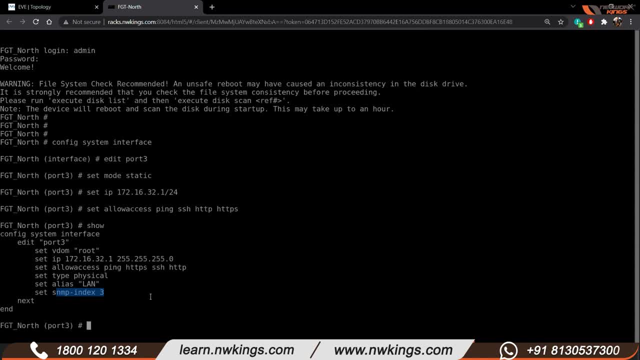 I am able to get from the interface show command. now one thing more. see, you have one command which says end. listen very carefully, carefully. end is going to save the configuration instantly. ok, it is not that you have to put in, copy, write configuration, nothing like that. as soon as you put the enter and you hit. 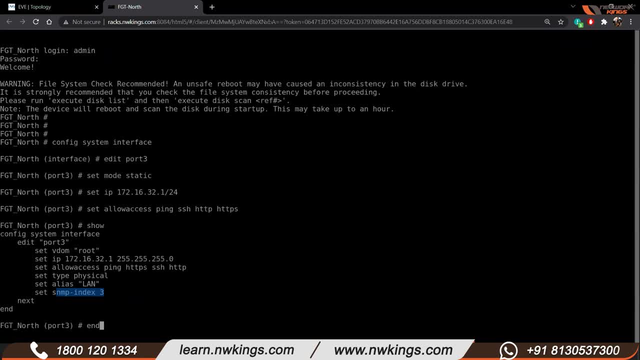 enter. ok, sorry, as soon as you put end command and hit enter, it is going to save that configuration instantly. ok, no, pushing the configuration, waiting for the configuration to be uploaded, something like blah, blah, blah, no, no, no, enter the command. hit enter- configuration is saved. so you have to be very, very careful. 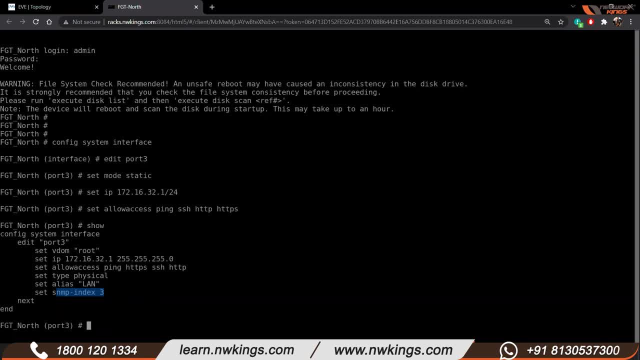 if let say, for example, I made some mistake, ok, and I want to get out of the interface, but I do not want to save the configuration, what will I do? I will say abort. so abort basically does not save the configuration and you will be able to come out. 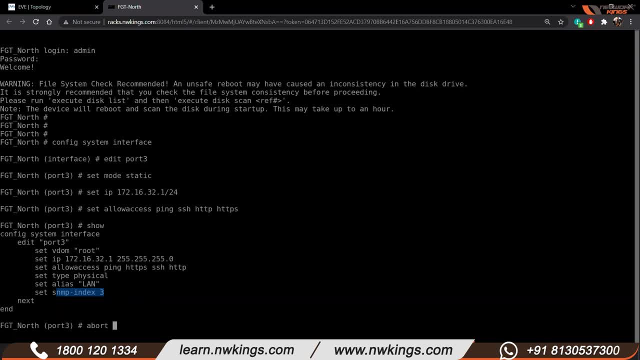 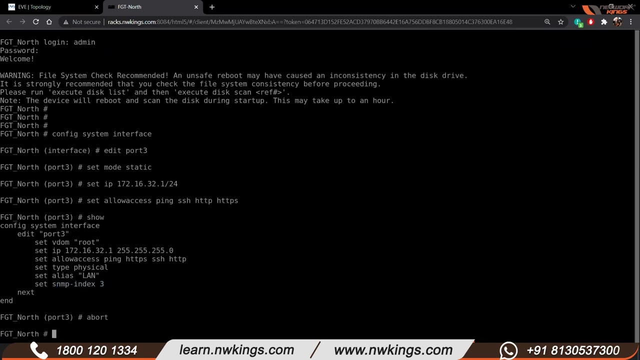 ok, everyone wants to see one second see. so show command. we have seen that. this information we have put now. now what I will do now I will write abort. ok, come out now. now I want to see that the configuration is saved or not. so I wrote show system interface. 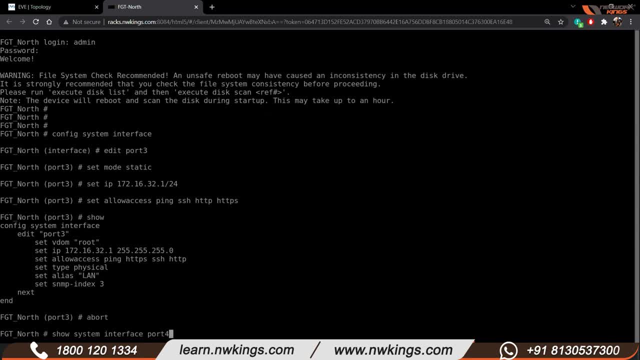 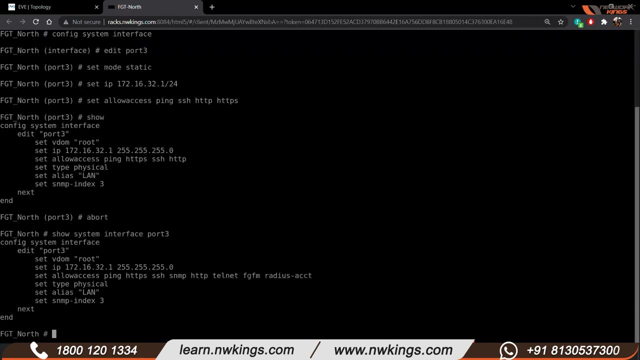 ok. one more thing. I am writing port 3, ok. so now what will happen? it will not show me all these ports, it will only show port 3. is everyone understanding? are you guys able to understand this? yes, sir, yes, sir, ok, so I save port 3, ok. 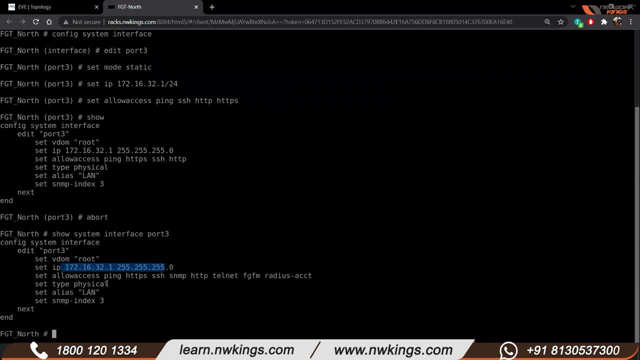 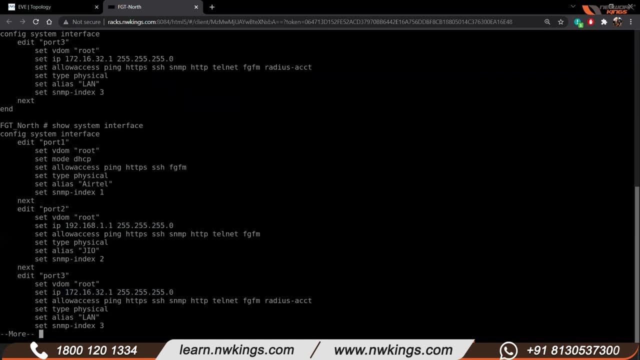 now see it is able to show me this information already. I have saved it, so I should show you some more information which I have not saved. one second show system interface. so see, there is nothing in port 4. ok, I will use port 4, config system interface. 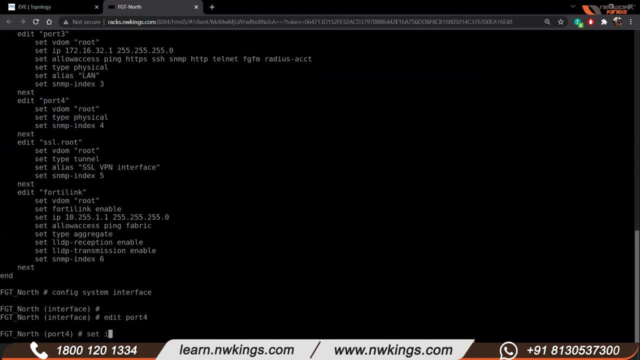 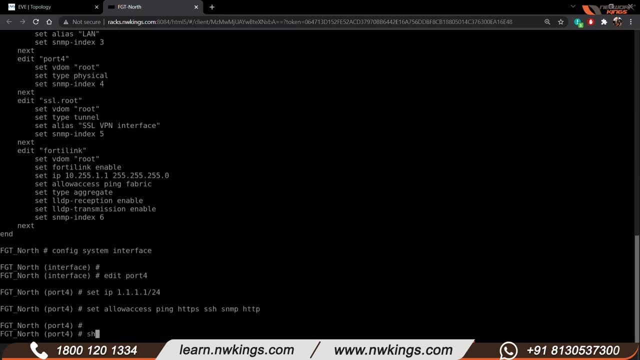 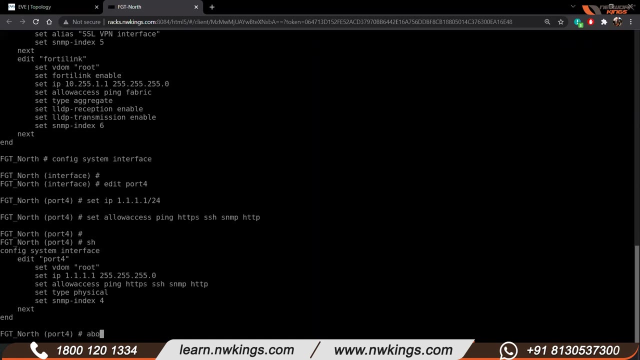 port 4, set ip, let's say 1.1.1, go ok. so now I have made two changes: ip address and allow access. ok, now what I am going to do is abort. I am coming, I came out. ok now if I say show system interface. 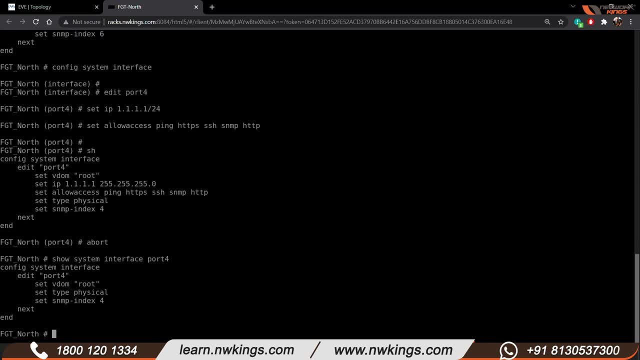 and port 4: see changes not saved right. so if- and this happens, guys, whenever you feel like you made some mistake and you are not, you do not want to save those, just use the command abort. ok, now I would basically change. ok, so I will say config: system interface. 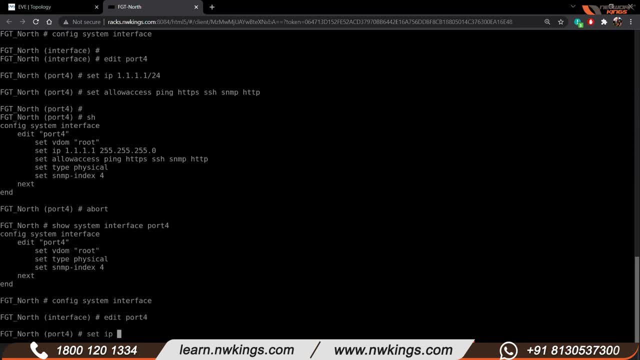 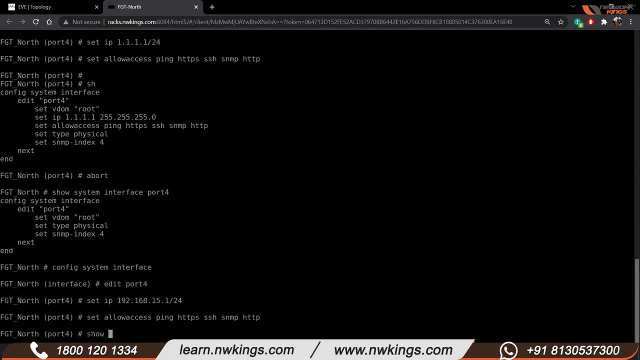 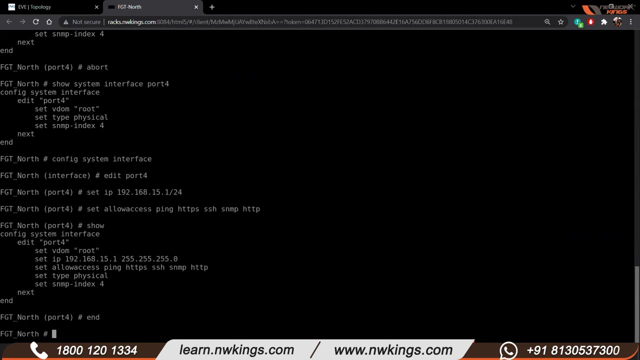 and write port 4, set ip, and I say 192.168.15.1 slash 24, set allow access and services. show command: enter. see, as soon as I hit enter with the end command, I came out. ok, but see what is the difference. the difference is: 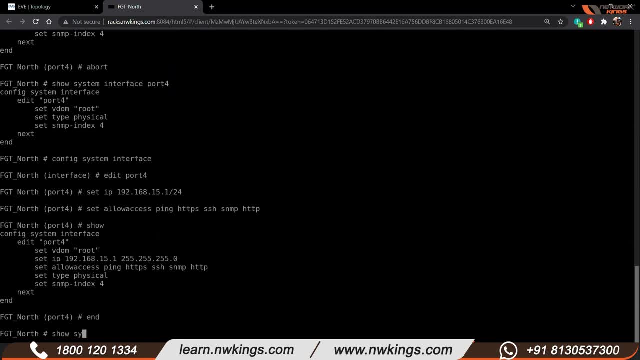 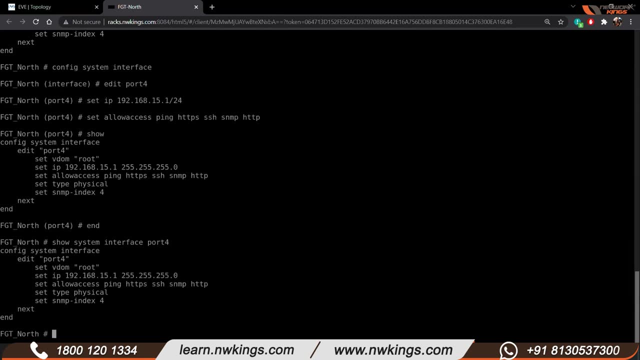 now, this information is saved in the interface. so show system interface. ok, so show system interface port 4. is it clear, all of you guys? end command will save the configuration. abort command is going to ignore the configuration. ok, clear enough. ok, now what we are going to do is so we 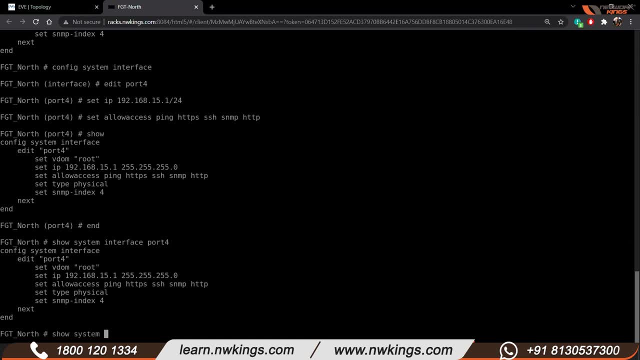 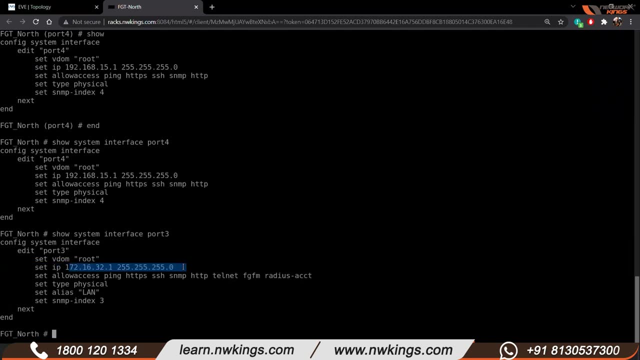 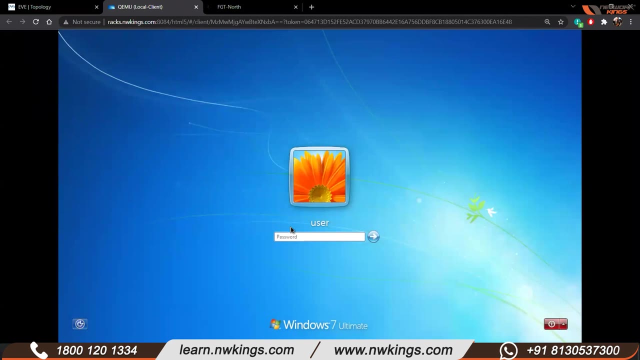 have configured the ip address of show system interface, port 3. let me show you guys. ok, so we have 172.16.32.1. all of you is it clear? ok, now let's click on the local client. ok, now, guys, the password here. 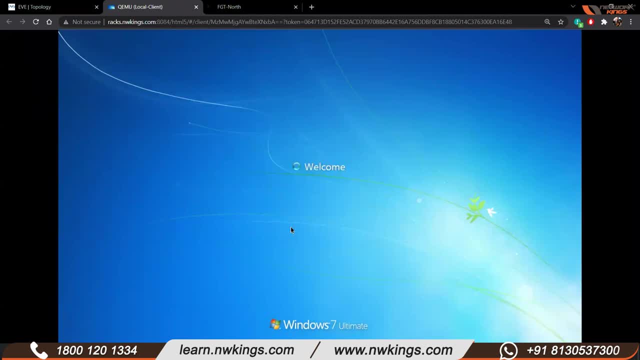 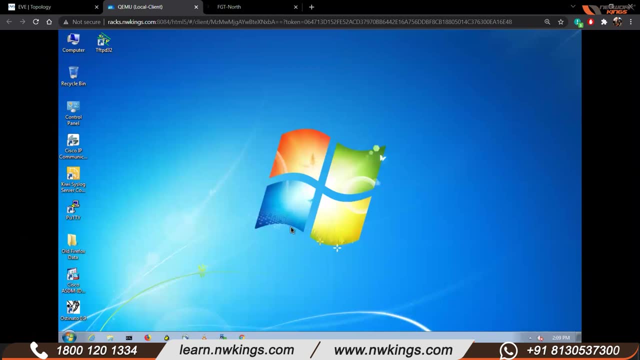 this is called as test 123. ok, so once you have the access to the lab, this is the password that you have to put in. ok, ok, so this is the configuration. sorry, this is sorry. the windows machine. ok, let's open up the command prompt. ok, I have already configured the ip address. 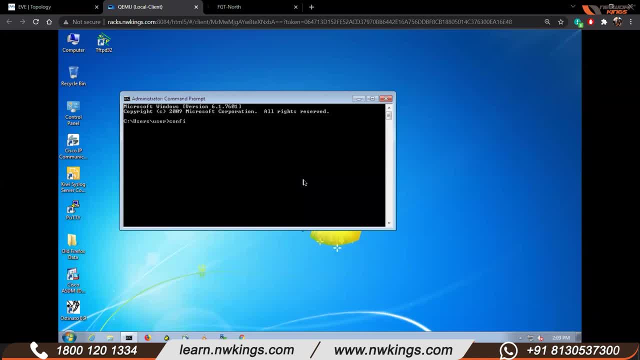 think over here. let me just see, sorry, alright. so see what is the ip address. we have 172.16.32.10, and then the gateway is 172.16.32.1. ok, so what we are basically doing over here is that we are going to ping this, ok. 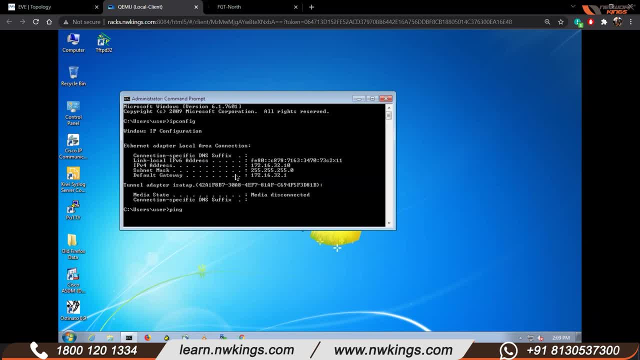 now, what do you? what do you think? will it ping or not? would I be able to ping this ip address or not done? do you know why I am able to ping? because I have enabled the ping services. ok, now let's do one thing. let's try and get. 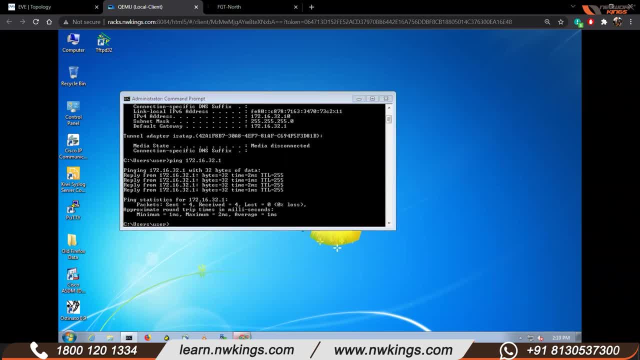 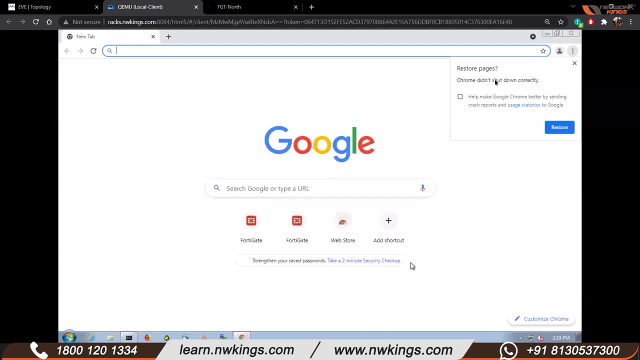 the GUI access of our firewall. no, Harpeet, we are able to get the access because we have enabled the- you know the ping services. ok, so what is the ip address of my firewall? 172.16.32.1. ok, so enter. so we got the page. 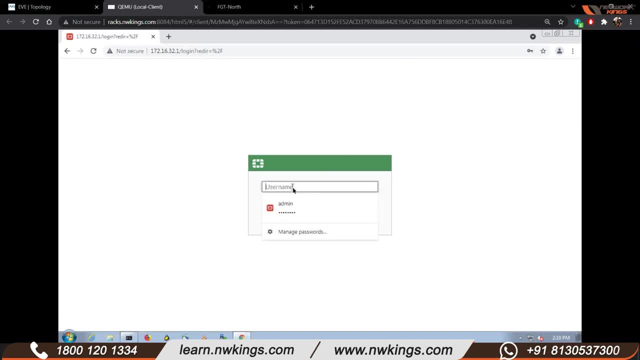 ok. so the same username and password that we used. ok to get the gui access. the same username and password we are going to use to get the GUI access. so we say admin and password. click on login. Hardik, you can unmute yourself if you want to. 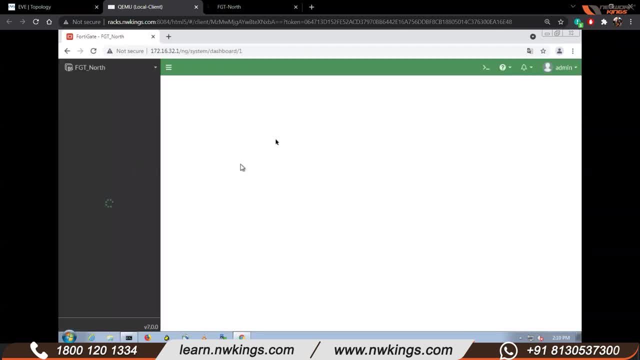 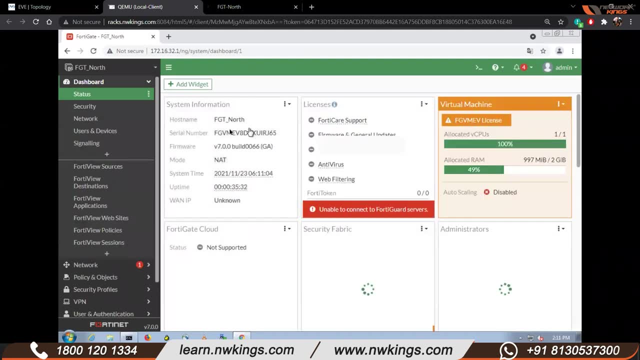 ok, so I will tell you what this is later. so you see, this is how the GUI would look for your FortiGate firewall. ok, so you will get a lot of information about the system. you know that: system information, the serial number, the firmware. ok, then license status. 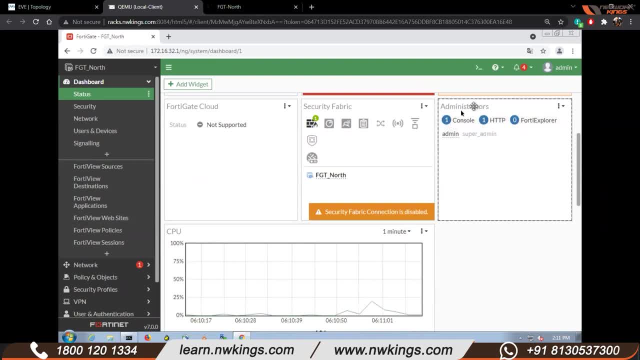 the VM resources that is being used. ok, now, if you look into the administrator section, you see that admin- this guy is already logged in, so this is me. then you have something which is called a security fabric. we are going to talk about this. then you have FortiGate clouds- lot of information. 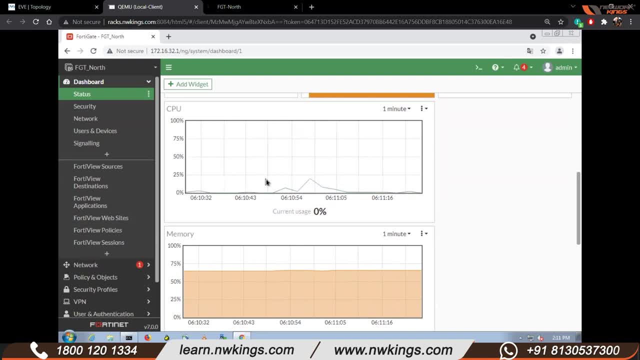 you see the CPU information. this is basically the dashboard, so you are able to, you know, just check the existing status. it is just like you have a task manager right where you see the CPU utilization, the memory utilization, just like that. you see the CPU utilization. now this: 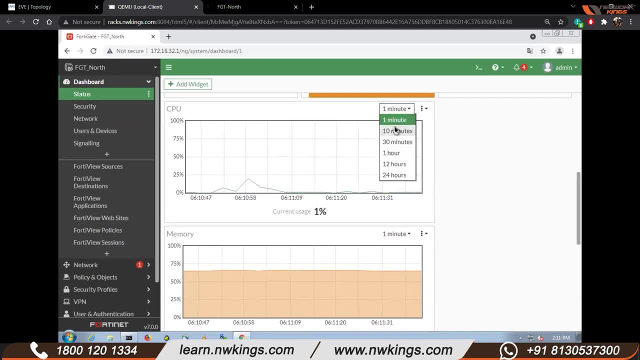 you can basically look for the drop down. you have 1 minute, 10 minutes, 30 minutes, 1 hour, 12 hours, 24 hours. ok, this is exactly how it is in a actual physical FortiGate firewall as well. ok, this is the information that you get and, according to, 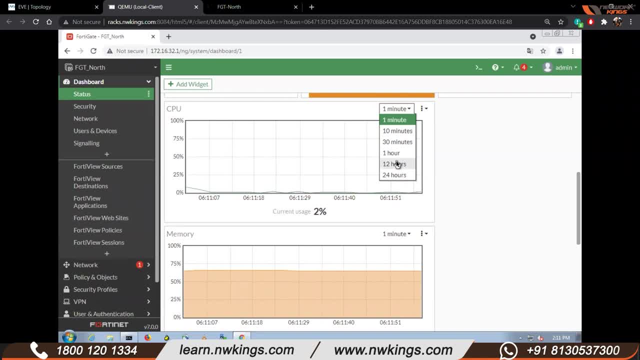 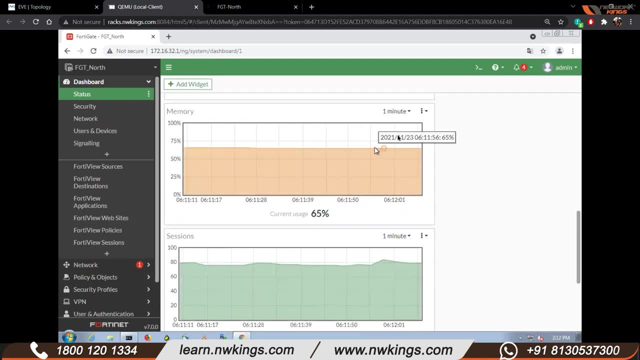 the client's requirement. you can make this change. you want to monitor this for each minute. you want to monitor this for 1 hour or 12 hours, or whatever the case may be. same goes with the memory as well. see, if I do this for 1 hour. 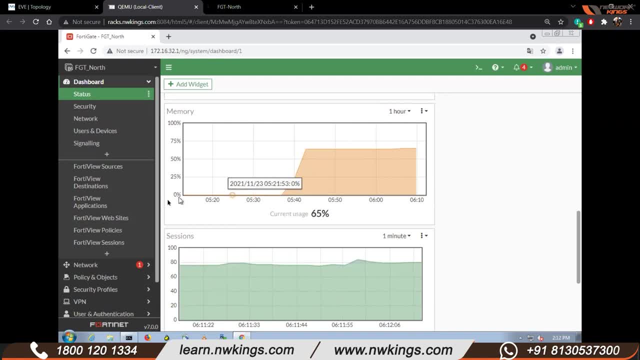 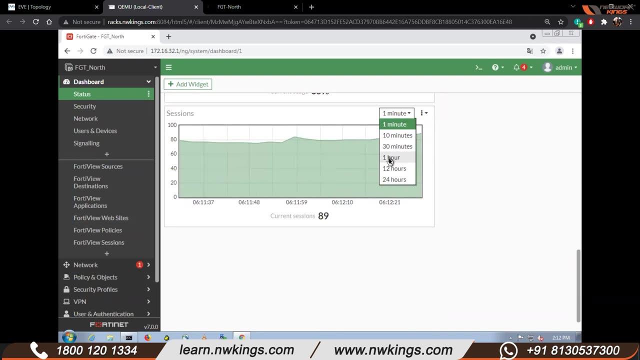 ok, you see this. nothing before 5.40, very obviously, right. I powered it on by that time, so the memory utilization then went up. ok, then there are certain sessions as well, so if I again go for 1 hour, see in the same time frame, so this is also, you would be able. 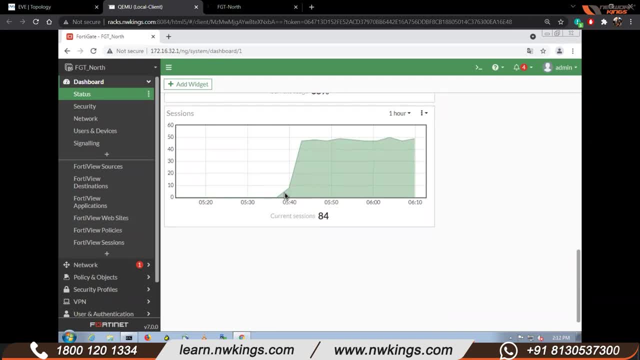 to understand that how much traffic, or when was the peak, when was the spike, or when the traffic is shooting up. you would be able to get this information from the dashboard. ok, ok, now. ah, ok, now see. do you remember that? the interfaces that we did? so you click on the network tab. 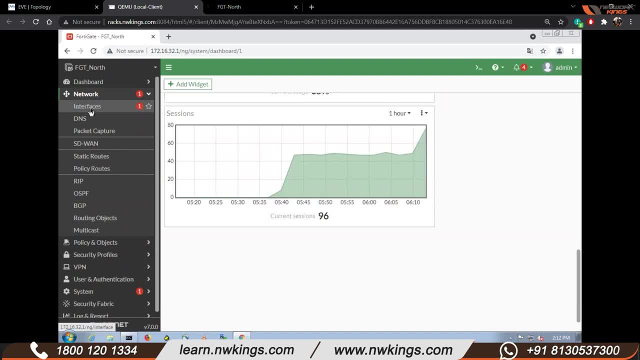 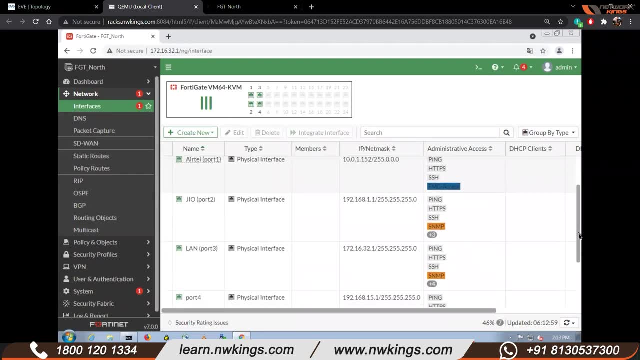 ok, now under the network you have something which is called as the interfaces. click on over here. you would be able to see the information which we saw in the CLI as well. ok, now see, you have port 1 configured. now airtel, geo and lan- this is I mean there is. 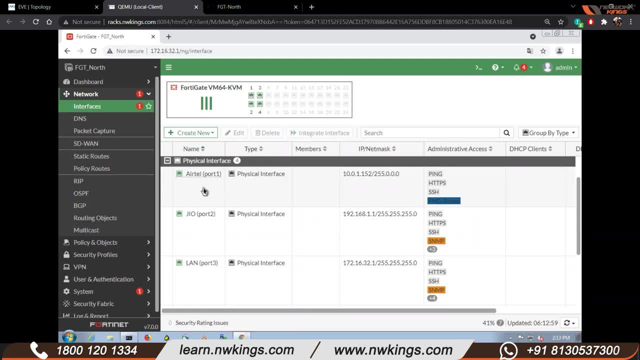 there is a batch going, so for them I have created the alias. now, alias is basically the name that you give to the interface, but you would be able to get the information over here. you see the IP address, the netmask. then you have port 2, which is the geo port. ok, basically I have made geo port 2 as an ISP. so there you have 192.168, then you have the lan port, which you have 172.16. so basically over here I would be able to see all the ports that I have. now I have. I was basically. 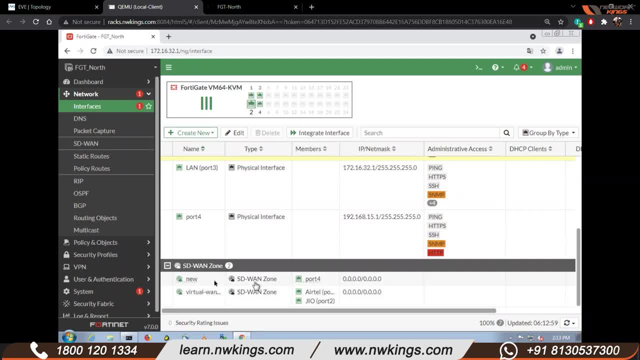 you know, training the people on the SD-WAN, so you are seeing the SD-WAN as well over here. ok, alright, so basically the interface section is the place. that where you would be able to look into all the interfaces. if, in case, you want to make any changes, you can. 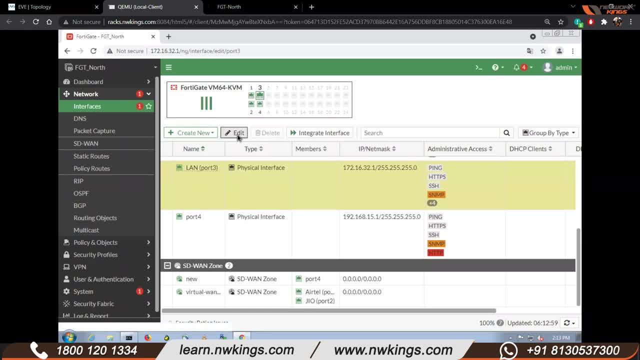 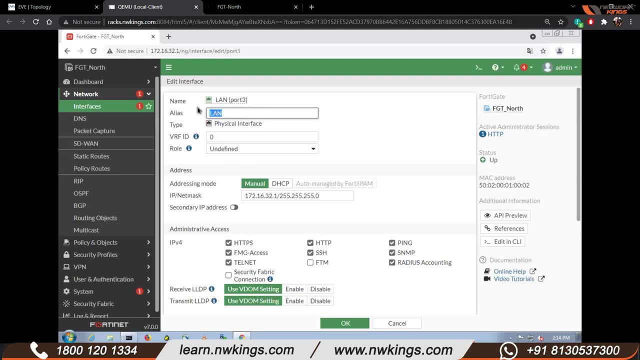 absolutely do it. select the interface, click on edit. ok, now over here you can make this change. if you want to make a different information, let's say, for example, this is tesla right, so tesla lan. ok, then, whatever the IP address that you want, manual or 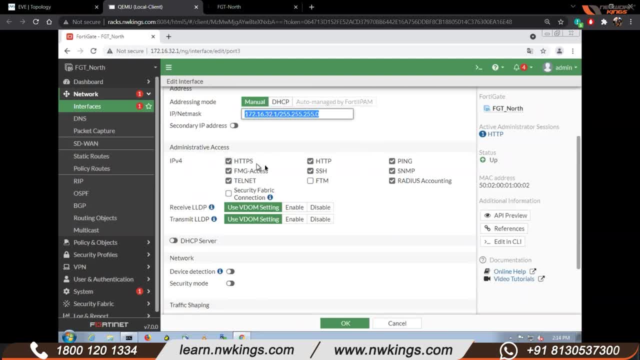 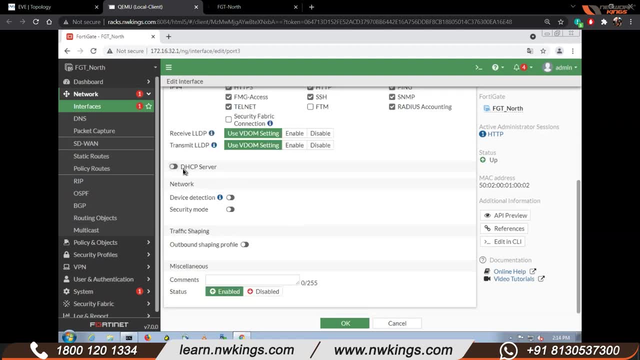 DHCP, then all the kind of administrative access, the HTTP ping, SNMP, SSH, all that stuff. then I'll tell you what is VDOM settings and all that. if, in case, you want to enable a DHCP server, you can. there are multiple options of device detection. now, what is device detection? 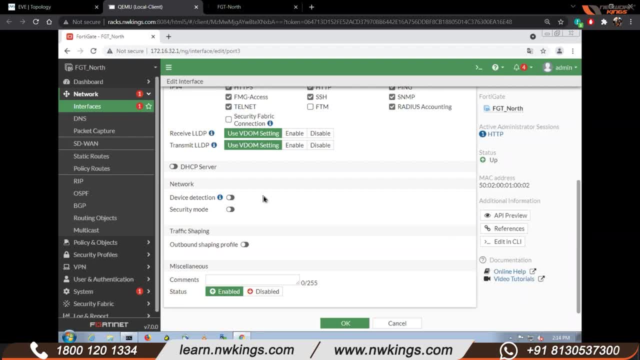 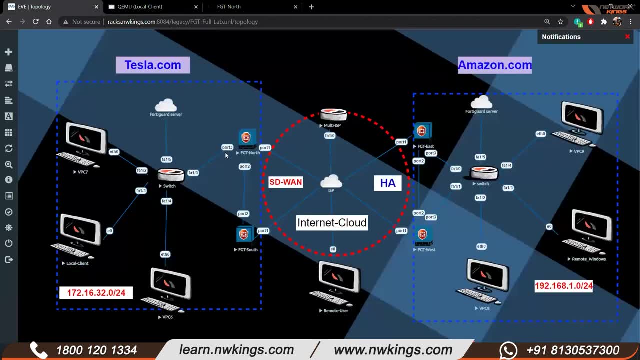 in a way it is going to fetch information about whatever the traffic is coming in, what device it is coming from. ok, so let's say, for example, over here, this port 3 is connected to these many operating systems. let's say, one is a Linux machine, one is a Windows machine. 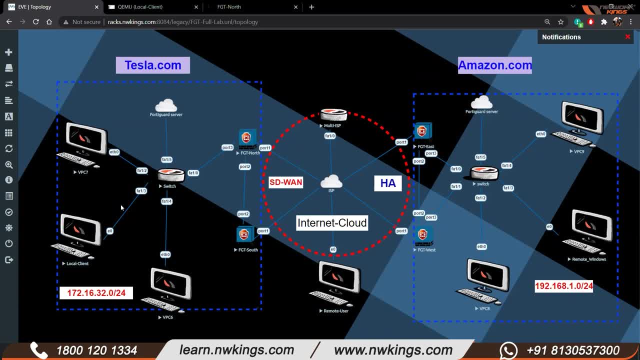 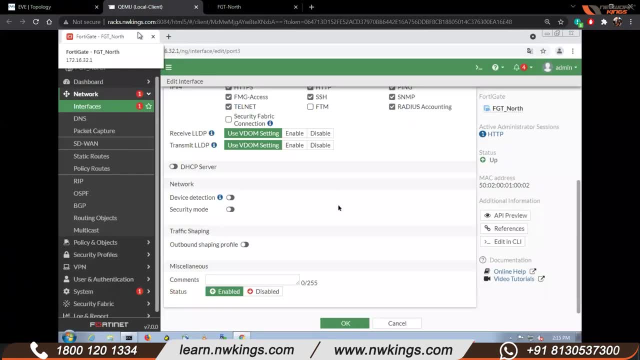 and one is a Mac machine. ok, this is going to basically identify that the traffic which is coming, is it coming from a Mac machine, Linux machine or Windows machine? ok, and it would be able to identify and then in the log section you would be able to see those information. 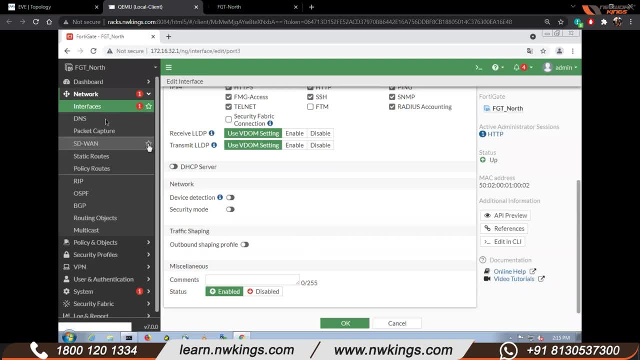 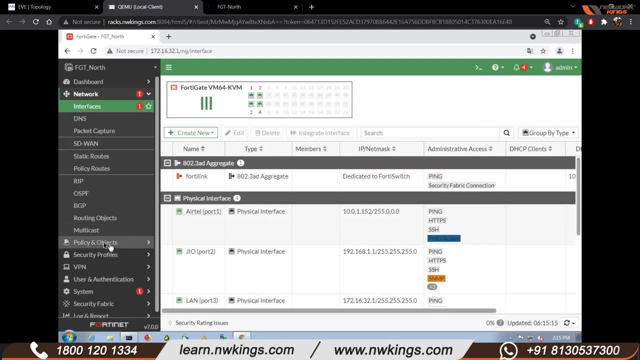 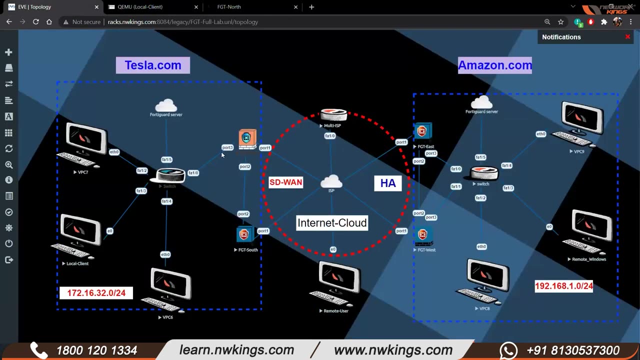 ok, so this information you can change whenever you want from the interface section. ok, alright, now what I am going to do next is basically the policies. so if you want to allow any traffic from your LAN, which is port 3, to maybe on the internet, which is SD-WAN, 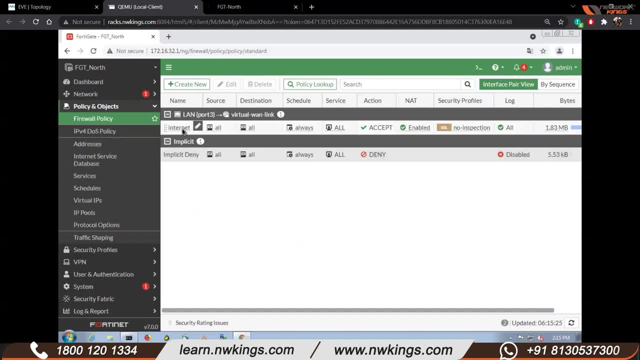 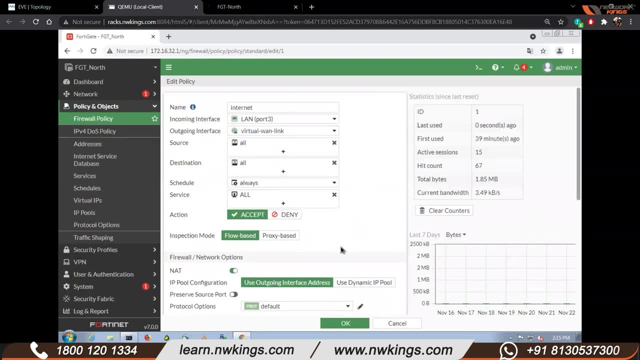 so you have to create a policy for that. so see, I already have a policy. ok, and look over here. there are couple of information that you can basically look: allow, deny the source, the destination. ok, now look in the outgoing interface. I am using the SD-WAN. 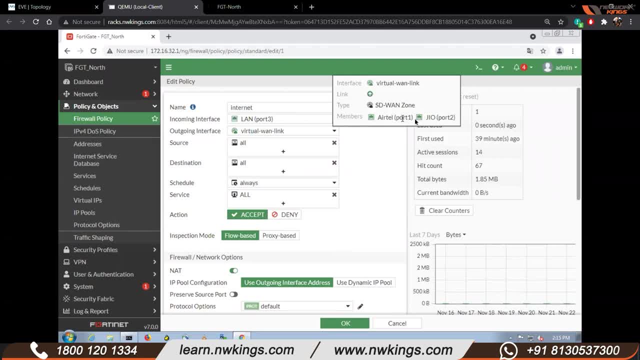 ok, so I am basically using two ports, which is Airtel and Jio. alright, so again, this is for a different session altogether. when we are going through the firewall policy session or maybe the SD-WAN session, then I will be able to explain you in deep that. why is it so? 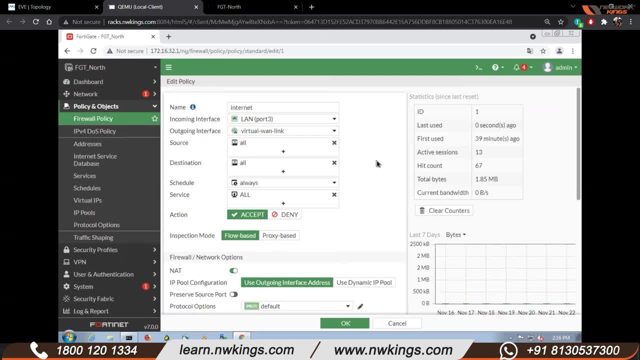 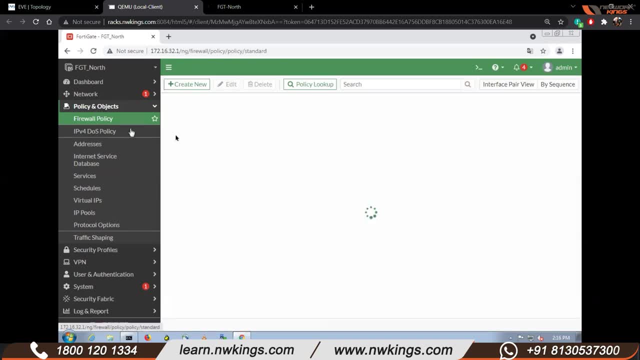 and how do you configure this, how do you troubleshoot this? but overall you get an idea that, ok, if you want to configure the firewall policy, you go into the policy objects, click on the firewall policy and then you can go ahead and even create a new firewall policy. 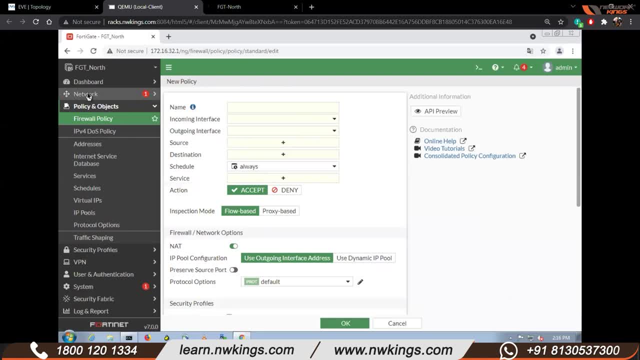 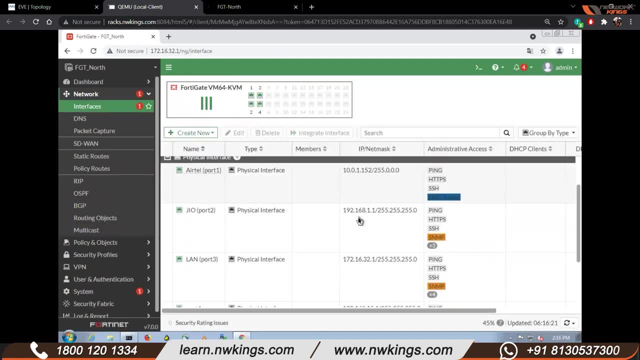 ok, so you can change all the information over here and if you want to look into the interfaces, you go into the network, click on the interfaces and then you can see that all the interfaces that you have, whatever, is configured. ok, alright. so, guys, as promised yesterday, I am going to stop right now. 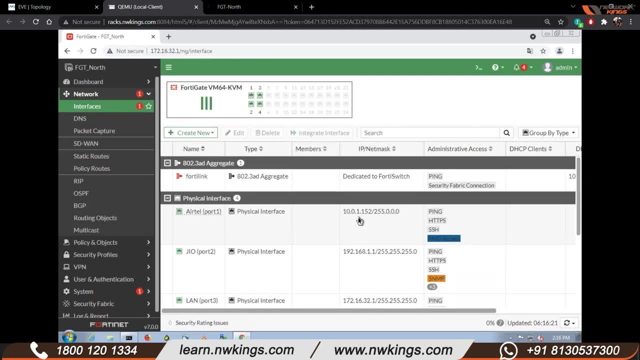 ok, now let's take a open discussion. whatever your questions are, we will discuss on that and we are going to start off the session from tomorrow 8 o'clock. alright, so by 8 pm tomorrow we are going to start the session with FortiGate Firewall. 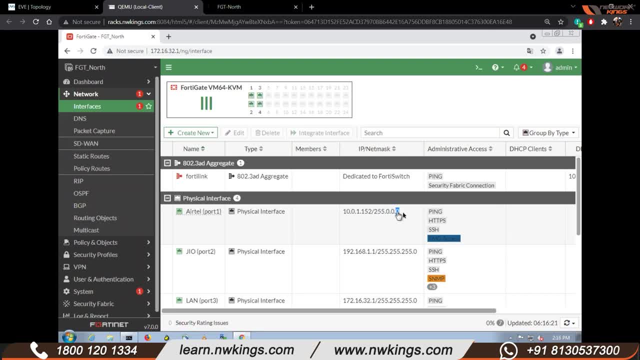 go ahead. you can go ahead and ask the questions, which is from 8 to when. it will be more or less about 9, 30, 9, 9, 30. ok, and one more thing: the commands that you, that you showed, do we need to note? 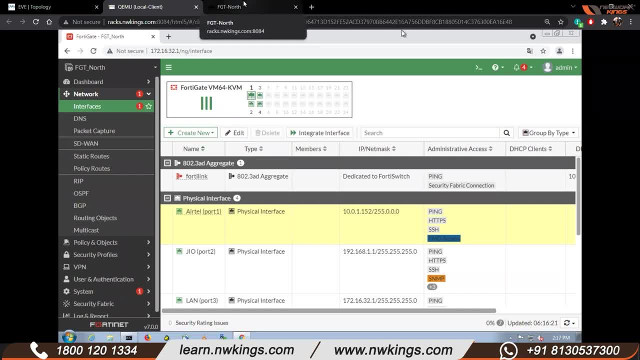 it down or we will be getting the documents which will have all the I am. so what I do normally is that. my personal experience is that whenever I have given documentation, people normally becomes a little bit lazy that, ok, I already have the commands, I already have the. 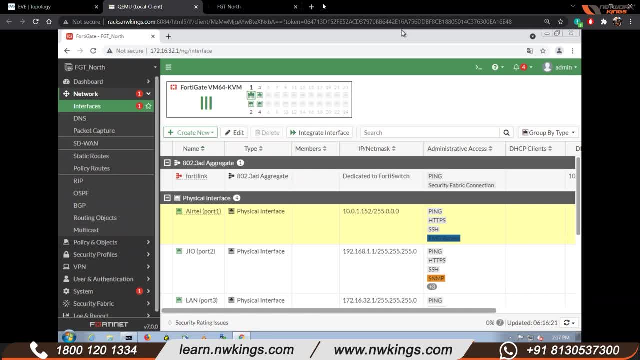 information in the document. so what I have started doing is I give the information, but then I give that documentation in the last till you are with me on the class, you have to make notes, just like you do it, you know, in the schools and the colleges make notes because 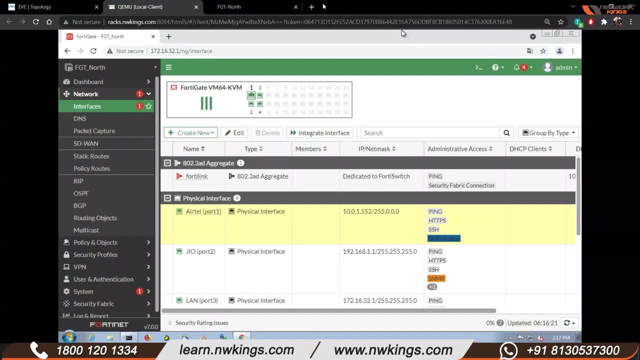 once you are making notes, you will remember those information. ok, so this is the. you know this is the process that I follow. don't worry, you will get the documentation. it is not that you will not get the documentation. you are going to get that, but maybe when we have completed. 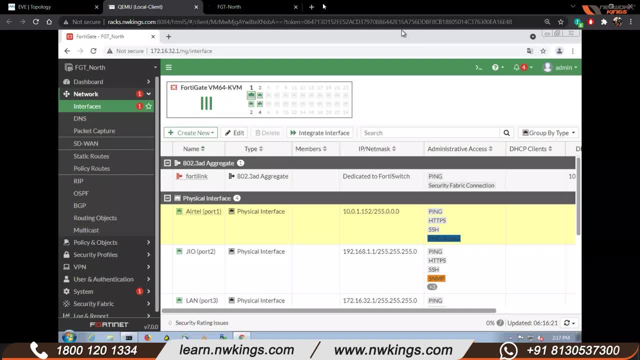 around 70% of the course and I personally know that, ok, you are well aware for the options, the configuration, the commands and all that stuff, then I will give you that, so it will be like a revision document for you, ok, yes, Munna, I have one question. 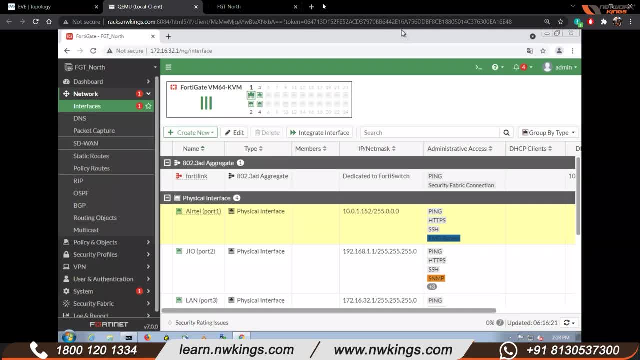 sir, like in Palo Alto, there is running configuration. so what happens in that in running configuration, if we change something, then running configuration remains after that. no, there is nothing like this. basically, there is only one configuration. I have said that it is simplest, so there is only one configuration in this. 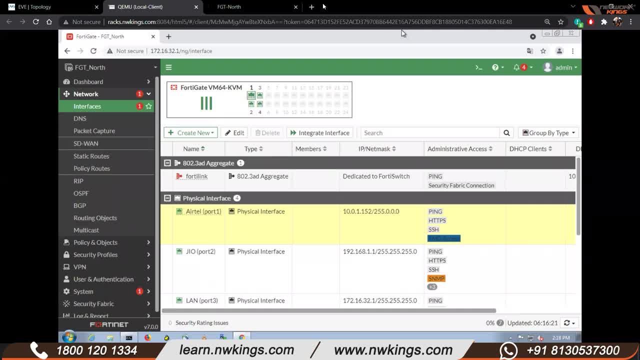 and whatever changes will be there. so consider running configuration: ok, and in running configuration, whatever changes you will do, changes will be saved in it. ok, if device is rebooted or you reboot it again, then also that same configuration will be taken. there is only one configuration and in that only all the changes are there. 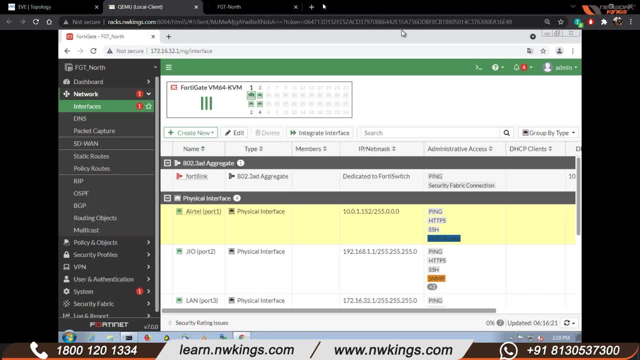 ok, thank you, sir, that if you have one ISP- suppose it is Jio's ISP and suppose there is some issue in Jio's network- then your network will be bad of the company. so what did you do that? you took one more ISP now, from now till now. 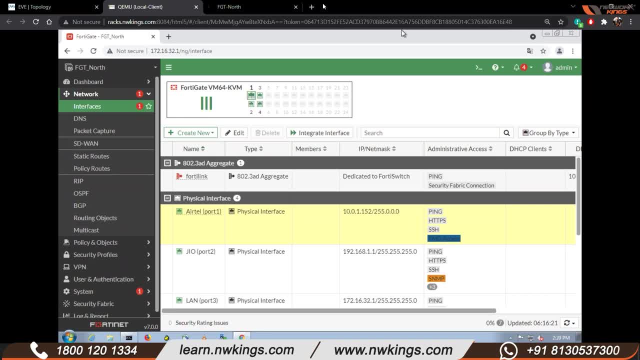 what used to happen was that manual changes had to be done, but with SD-WAN many changes are coming. now everything has become automatic, so you need to do something. if suppose there is some problem in network of Jio, then that automatically firewall whatever you have set up. 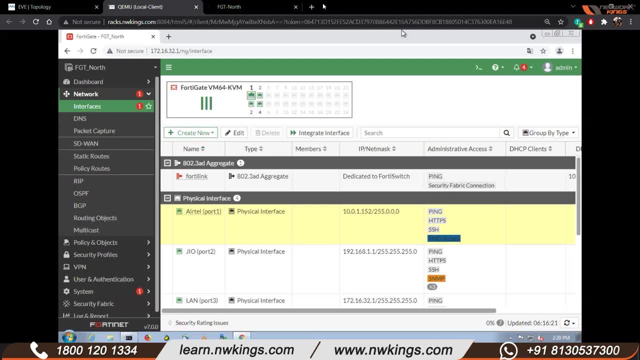 that if this happens or this connectivity gets loose, then change it, switch over it. do you know the concept of high availability of HA HA? yes, what happens in that if device gets down, if one device gets down, then traffic will go from other device. concept is same here also. 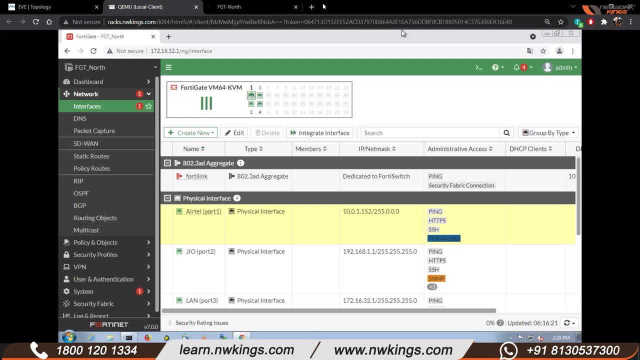 only thing is that instead of device ISP. sir, I want to ask one thing. that is not that multiple firewall is there in the company and I, manually, through one firewall, I push the configuration. no, no, no, that is manager, that is different thing. ok, sir, let me take one question. 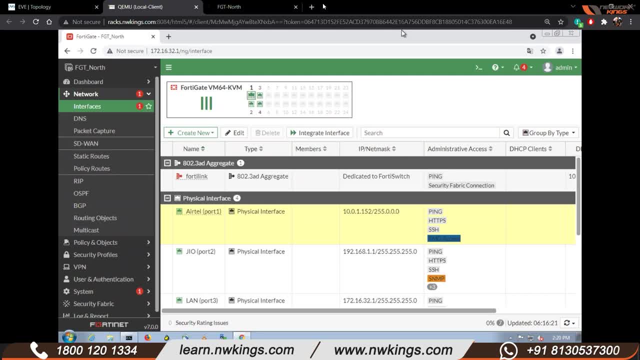 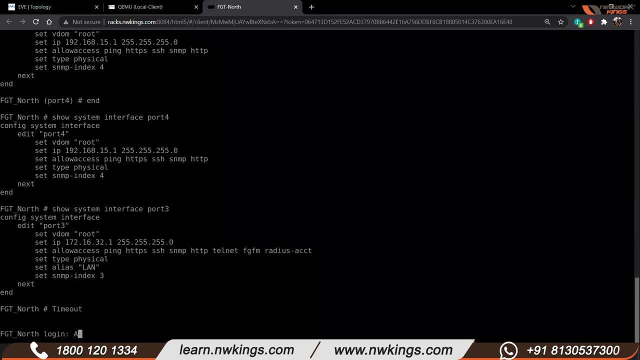 from guys who are basically on youtube. so Narlan has a question. give me one minute. so Narlan has a question. can you please tell me how to check the policy via CLI? Narlan, it's quite simple. basically, you get into the CLI mode first. ok, let's login. 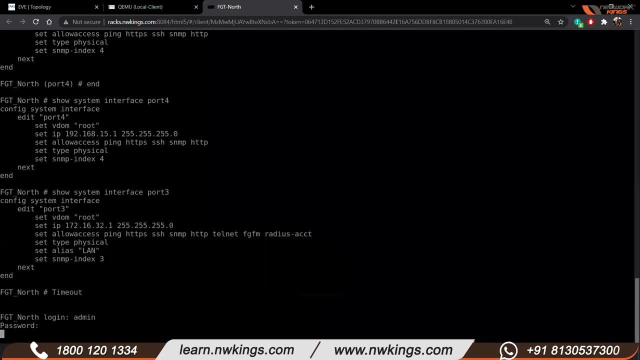 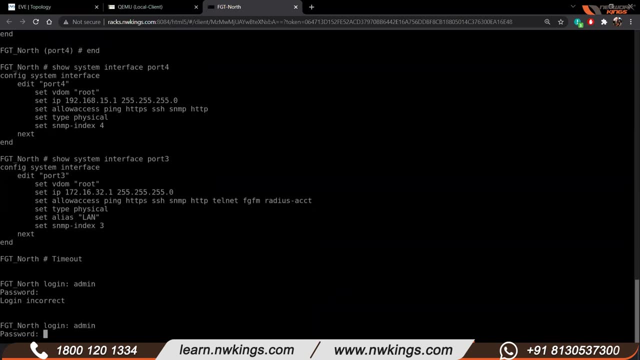 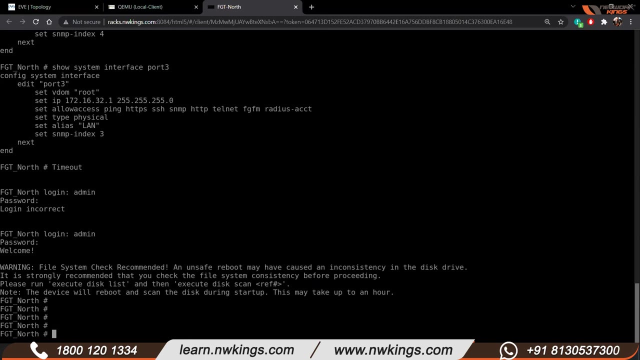 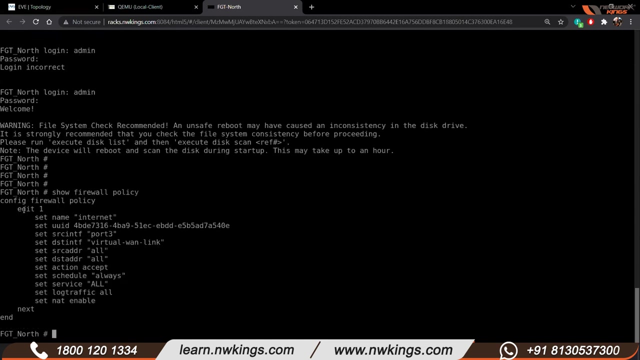 admin password. oops, I think I made a mistake. hold on admin password. ok, so if you, in case you want to, you know, find out the firewall policy, you say show firewall policy. ok, so see one firewall policy as of now, and it is basically showing me all the information. 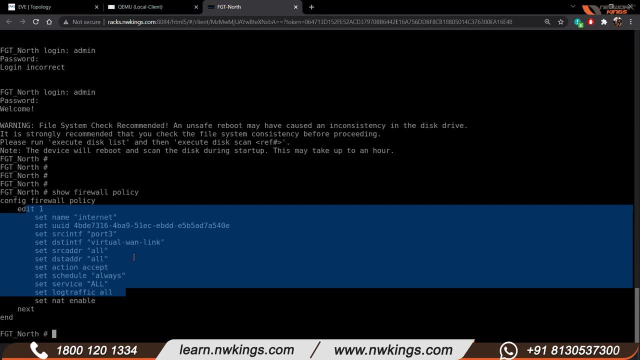 that? what is the source, the destination and everything? ok, yes, Madhi, tell me. I want to say what are the days class: Monday to Friday. thank you, hello. yes, Rajneesh, sir, I want to know why we use WAF and why, basically, this is deployed on DMZ. 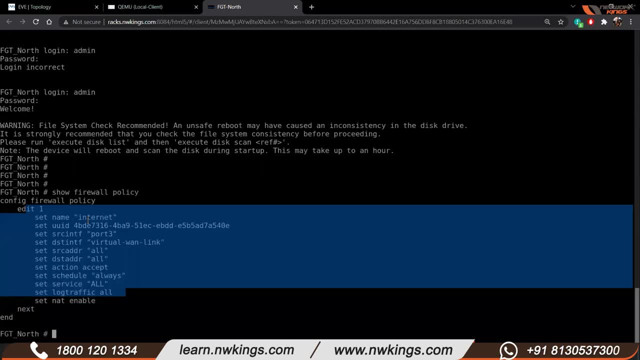 ok, see, WAF is basically a web application firewall. so web application firewall is dedicatedly web, basically OSI layer 7 application layer. but we have same feature in the web filtering in the firewall also. again, the FortiGate firewall is a UTM means 4-5 functions. 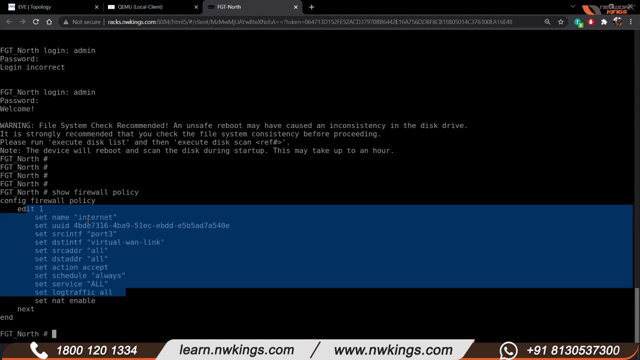 of devices, it does it alone. but see one thing in this, this web filtering option that you have. right, it is restricted to just web filtering URLs, ok, but if you look into the web application, it goes way beyond, way deep into the application level stuff. the web host. 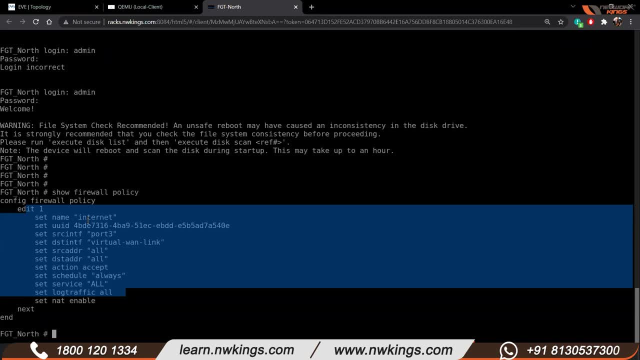 I understand. I understand like I am handling a Cisco iron port proxy, so over there also I am controlling application base. so is it the same thing happening in the WAF? it's the same application level control you. you do that same stuff, but then see, it is just like having an IPS on your. 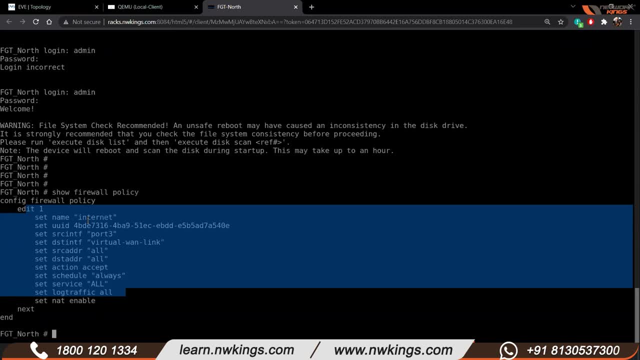 FortiGate firewall, and then you have a dedicated IPS. so who? which device would have much more functions? it's the dedicated IPS, right? so same concept applies over here as well, that you have a UTM and then you have a WAF, so WAF basically has much. 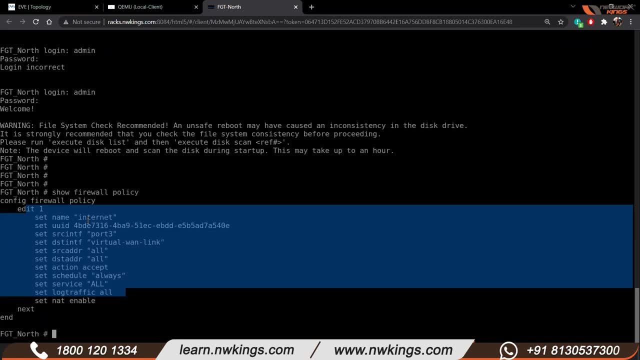 more features and functionalities for stopping the attacks on the application level, but you will not be able to get the same same features on a UTM. you might get basics, but not all. ok, ok, got it. thanks, alright, Sir. I don't have a firewall physically. it is not available physically. 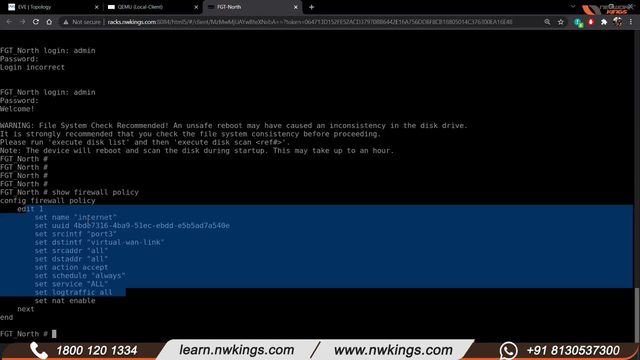 I am on location, so will I have to do it through FortiGate? I have to practice command, so how will I do it? you will get access in the lab in the same way, Sir. I have a firewall in front of me, but I don't have a 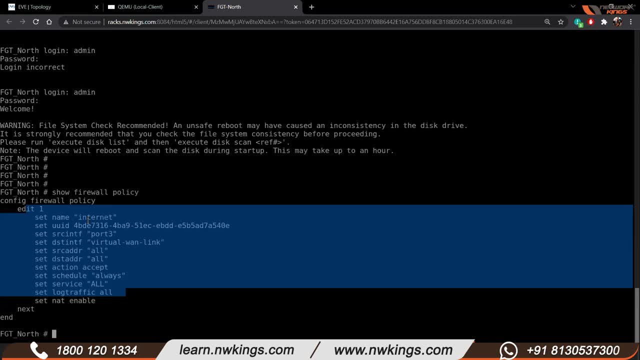 configure and I don't have a console cable. so in that case, how will I do it? in the management interface? in the management interface, you will go to the management interface, you will take the RJ45 cable, you will put one of its cable in your laptop and on the other side, you will put it in the management interface. 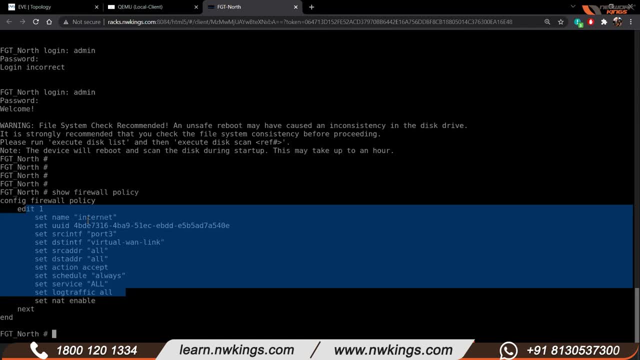 ok, in the management interface, the FortiGate firewall, as I told you. in this case, default username is admin. similarly, in the management interface, default IP is already there, which is 192.168. yes, ok, ok, Prashant, we are. this is the last session on the YouTube. 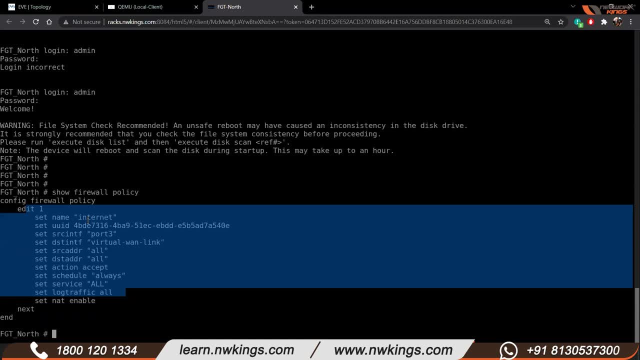 now, from tomorrow, we are basically starting off the classes, which will only be on the zoom sessions. ok, ok, Navin says FortiGate duration. so, guys, this is on a daily basis, one hour, maybe one and a half hours, so maybe you can think of what is. 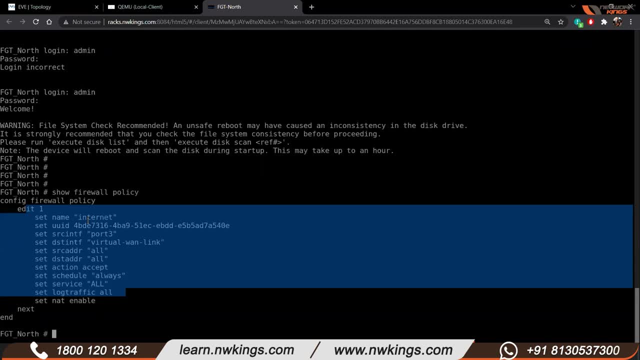 today's 23. so take December, whole of the December, you would be able to get this course completed. and again, it all depends on the number of students that I have and how much interactive they are. if there are a lot of interaction in the class, which I 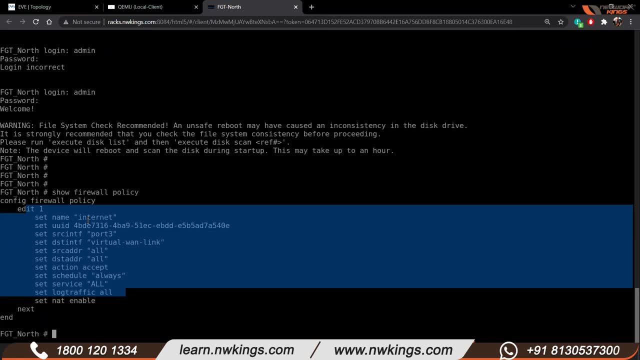 normally love. the class would basically extend because I would love to answer your doubts, your questions, and the more questions you ask, the more I will answer. the less questions you ask, the faster the course will end. now it is up to you, but yes, in general one month. 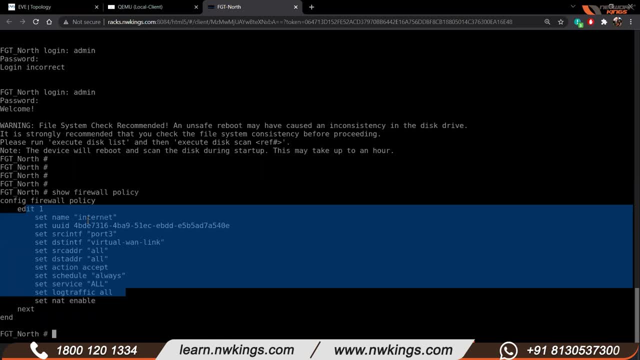 one month, one week, two weeks, it takes. sir, will you tell us something about SD-WAN? basically, of course, I will tell you. I have put SD-WAN in the course because nowadays everyone asks for it, and if not full-fledged, then at least. 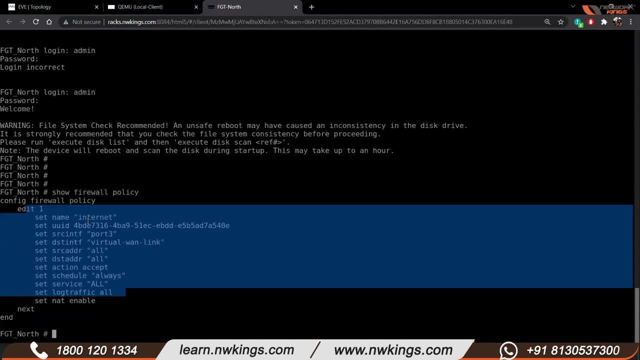 if someone asks you anything about SD-WAN, then you should be able to talk about it, so I have included that in this. actually, we don't have SD-WAN IDR and don't worry, I will tell you everything. in the interview of SE4 can we put a question about SD-WAN? 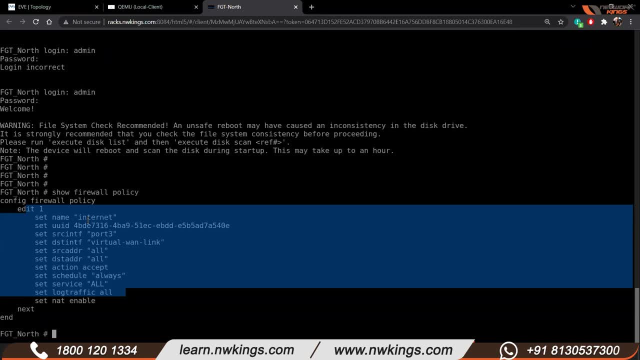 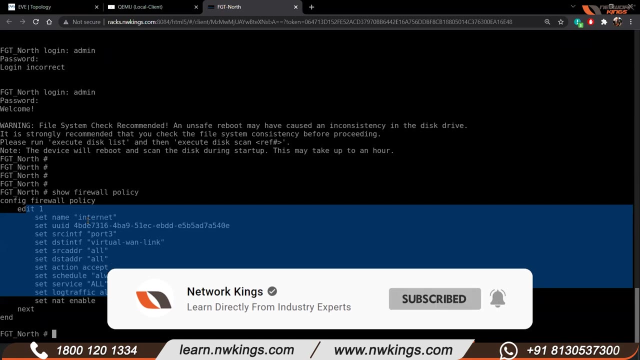 interviewer. if interviewer can ask absolutely, absolutely ask. in fact, if you have put in your resume that I know firewall, then they will ask absolutely: do you know anything about SD-WAN? if you say no, then there is no problem. but again. so let's say, for example: 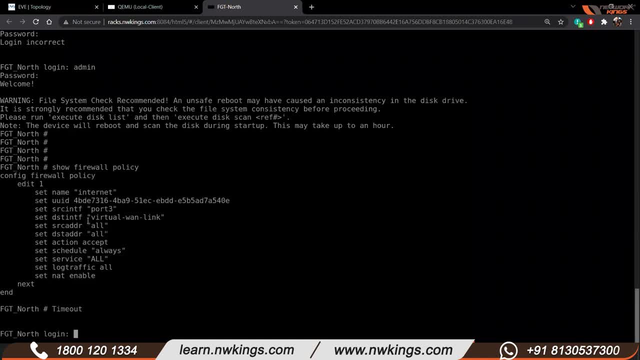 there are 10 people who are going for the interview and you are saying no, and then there is another person who is saying yes, I know SD-WAN, so obviously you know. you know who will get preference, so this is why I have included SD-WAN in this. 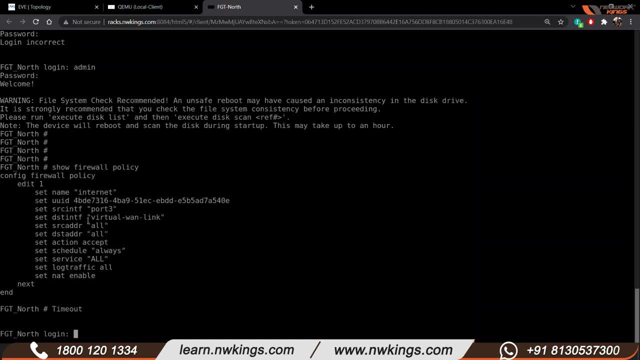 so that if, in case, there is any questions, which normally 70-80% there are, so you would be able to, you know, give an answer. that, okay, yes, I have worked on SD-WAN. I know how it works. I know how to troubleshoot all these things. 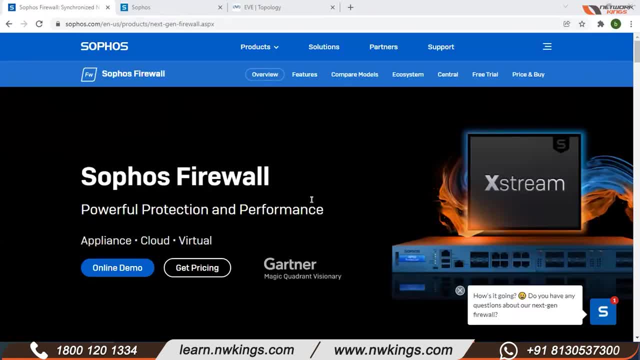 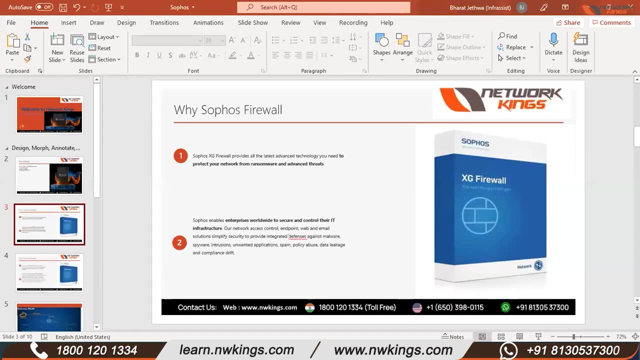 okay, sir, thank you. so first firewall, why we use so first firewall? generally we use so first firewall, like there are vendors in the market similarly. so first firewall is one of the choice, one of the best choice. I could say so if we, if we look at its features. 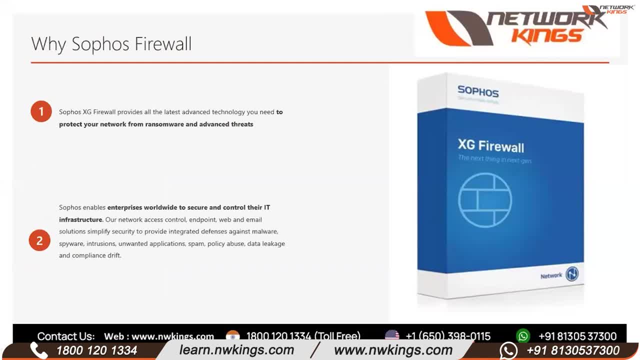 generally we use it for network protection, right where it uses the latest advanced technology for ransomware or advanced data detection, so any enterprise worldwide. if we want to secure it or control it in IT infrastructure, then so force is the best option we can get. so if in that 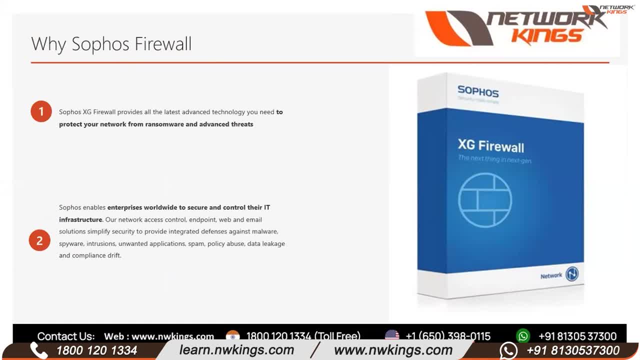 if we have access to network, it has control from end point web traffic email traffic. if it needs web traffic email solutions, then definitely so. force is best against the all type of attacks and malware, spywares, intrusion, unwanted applications like spam and policy based. so we can meet our requirement as per the business. 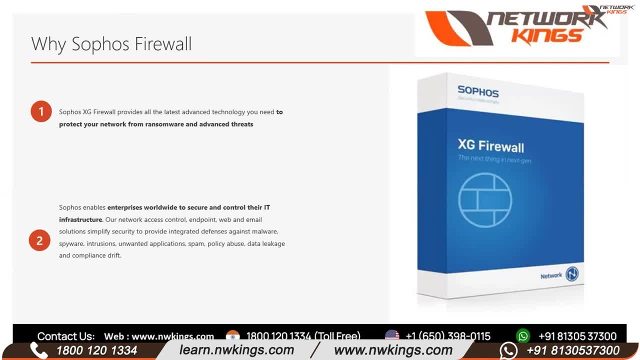 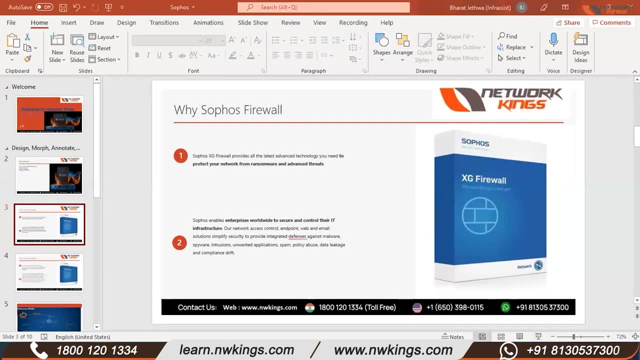 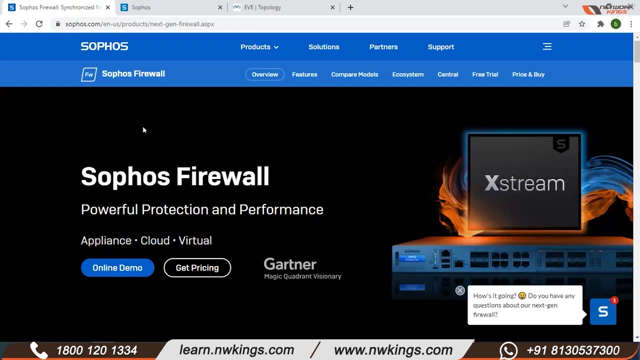 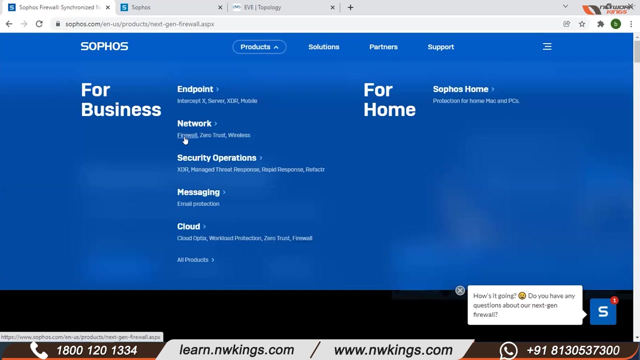 needs. so force firewall is fully compatible. so before we go ahead with this, so force, let me just try, try with you. so force website, so force website. we will get all the details, the products they are providing generally. so force firewall, we will focus on it completely next when we 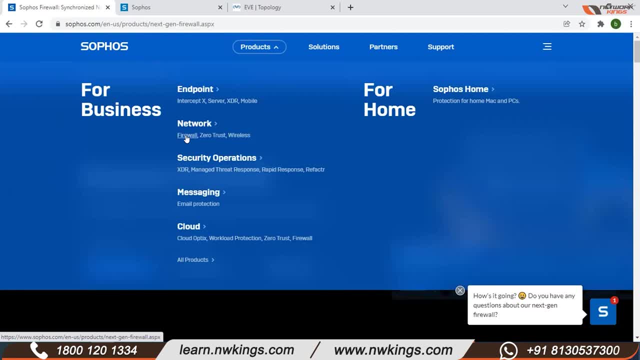 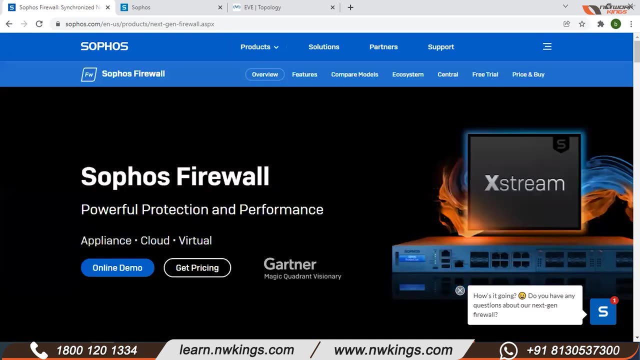 will explore all the scenarios, topologies of so force which are also features of so force. after exploring so force firewall, we will go to different products later on, but for now, completely we will concentrate on so force firewall, concentrate so here. this is how it looks like. it gives overview. 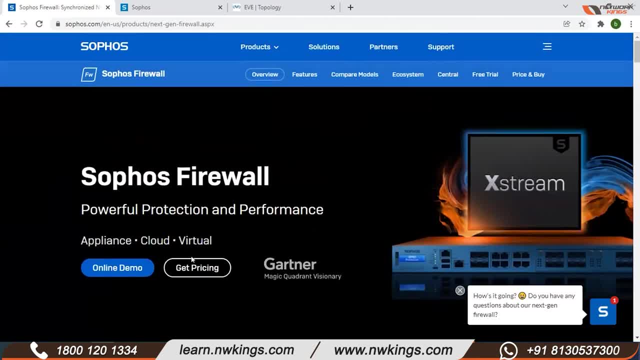 here you will get the full overview of so force xg on the website, along with the online online demo plus. if you want to use it for free, then we will definitely install the free one today, if possible at the end of the session. so, free firewall we will install. 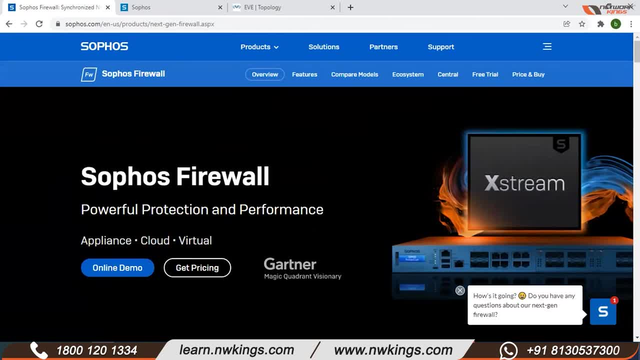 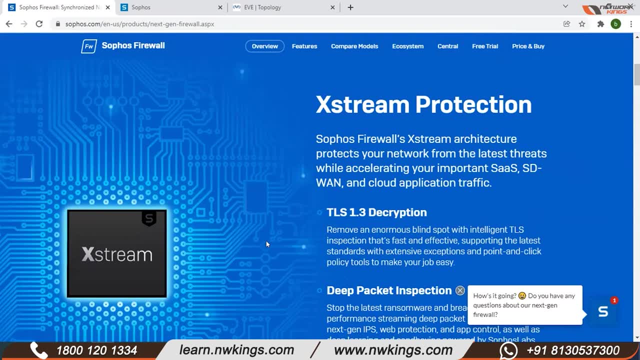 and see how it will work in the future. ok, if you want pricing, then we can get it. so force firewall for them. use extreme protection so their architecture is updated to the latest, so we can use it to protect advanced thread against the sas and sd ven. 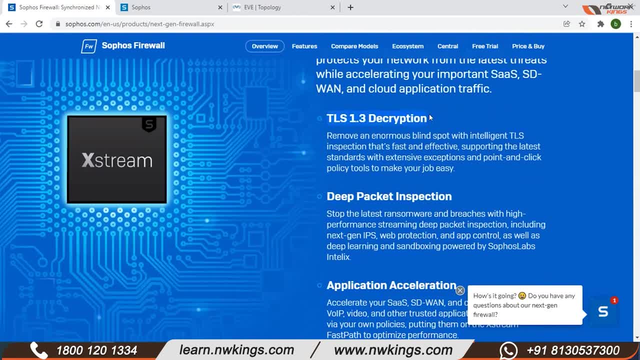 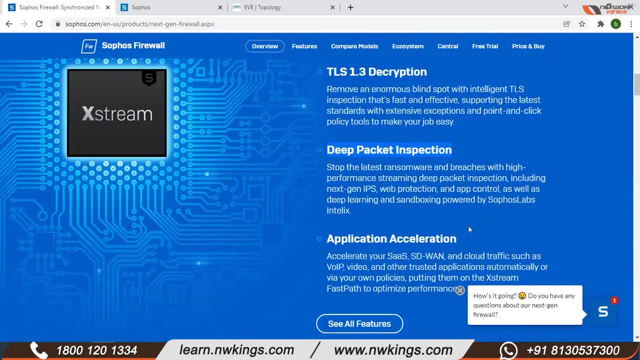 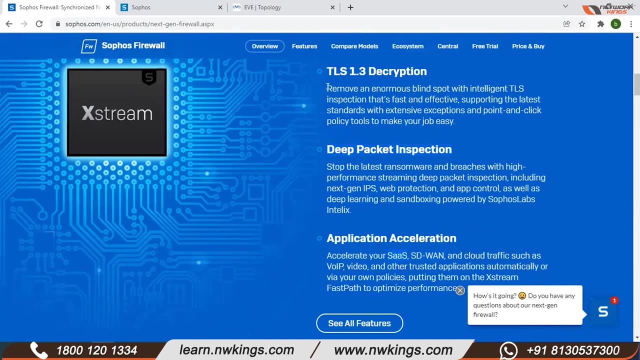 and cloud application traffic. so it uses all the features like the latest one, TLS 1.3 description. so yes, of course it uses packet inscription, application acceleration, that is through sd ven and a service. So definitely, we will go into detail about this one by one. whatever features are, 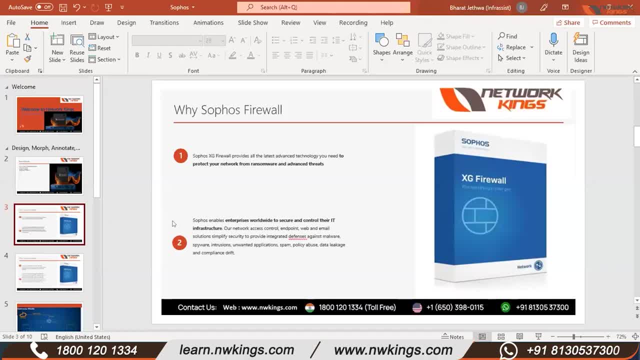 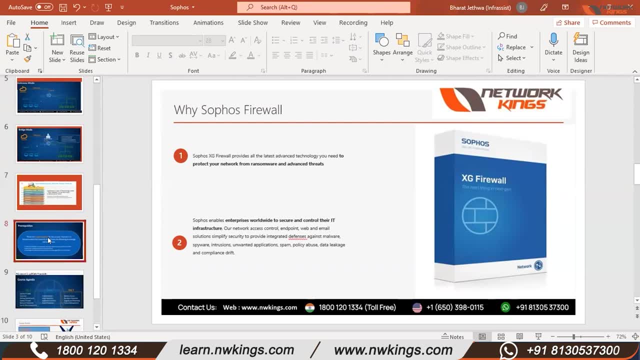 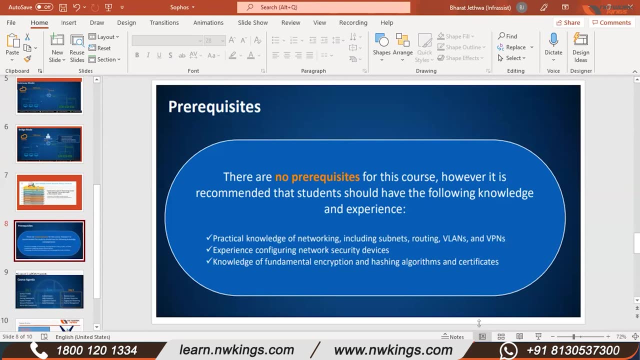 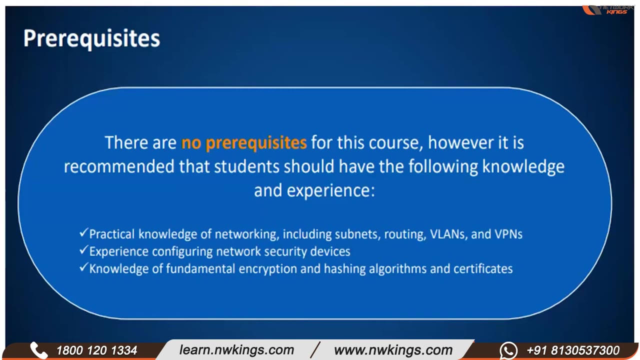 available here on firewall. If I go to the slides, if you go there, we can do different scenarios. but before we start this course- there is no prerequisite for now, Just generally we should have basic knowledge of basic networking or subnet routing- VLAN, DSCP, DLS- basic knowledge. 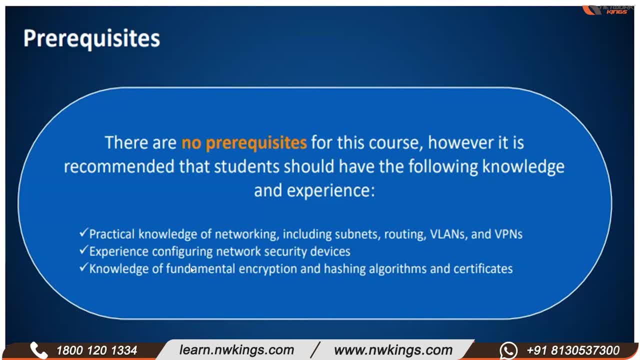 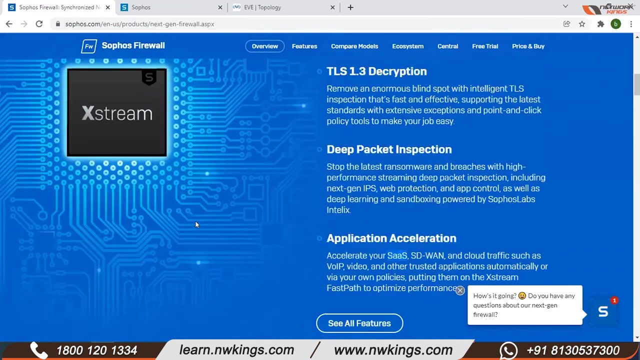 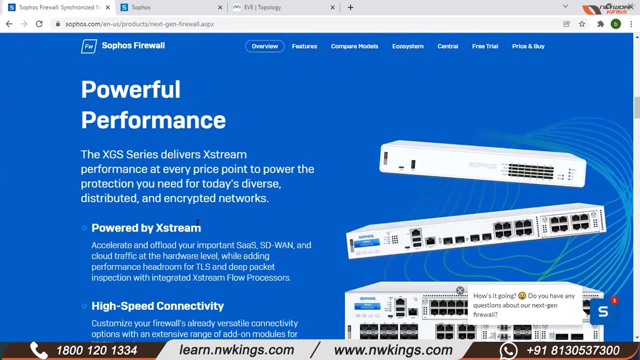 or we should have some experience in configuring a network device or any fundamental knowledge for encryption and hedging algorithms and certificates. We can say this is the prerequisite. If this is enough, then we will understand surface firewall easily. So let's go back to the website. So surface firewall provides a lot of modules, along with 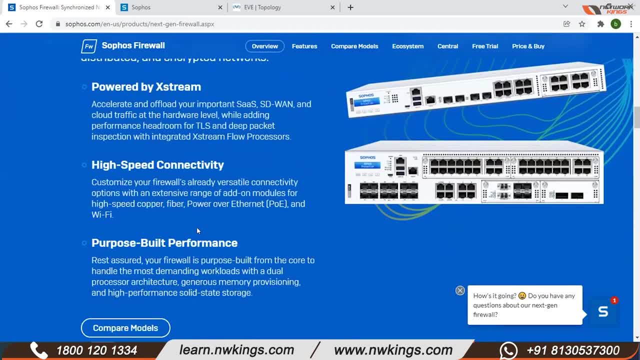 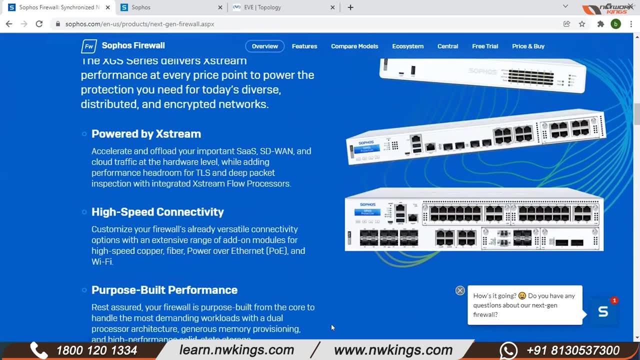 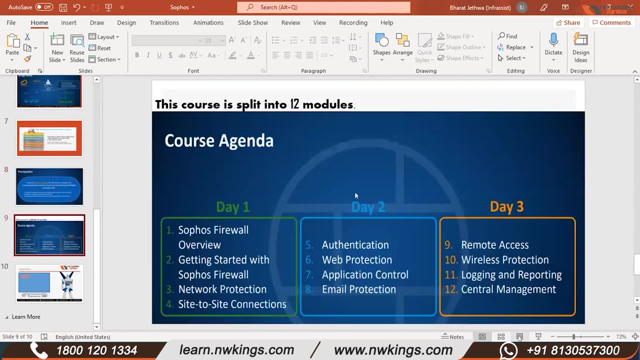 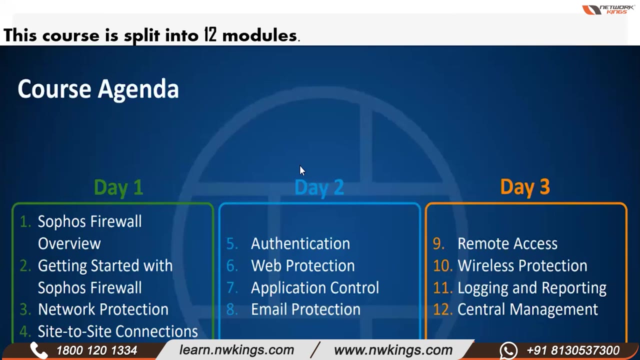 the features which are provided here. We will go through one by one each. So here we will start the course, our course agenda. I will tell you that once. So our course agenda would be like a complete overview of surface, just like we just told you. 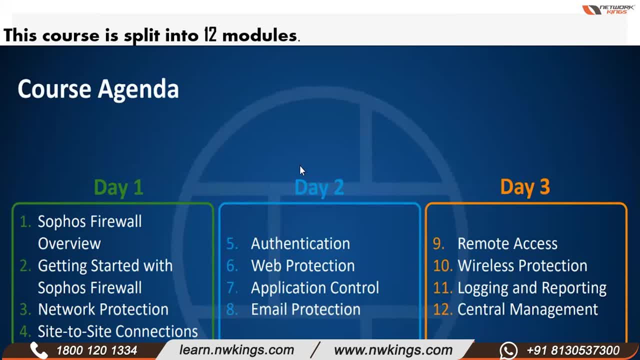 on the website, like how they have features and how we can meet them in our existing network or deploy a new network, Just like these features would be. So here we go to the website. So the overview. After that we are getting started with Sophos Firewall ie we can install. 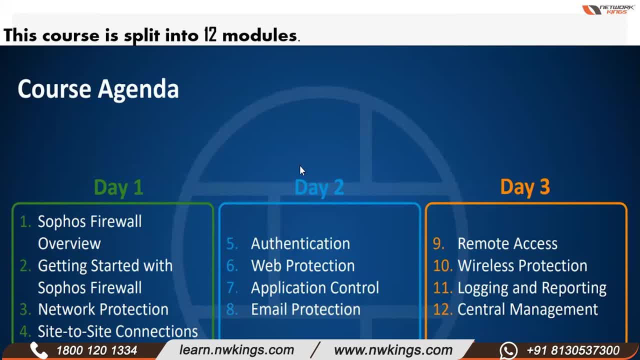 Sophos Firewall on which platforms to meet the business needs. It also has different scenarios and covers everything in the module. So how will we start Sophos? We will cover all the modules in the module. We will go to VMware at the end of the session and install. 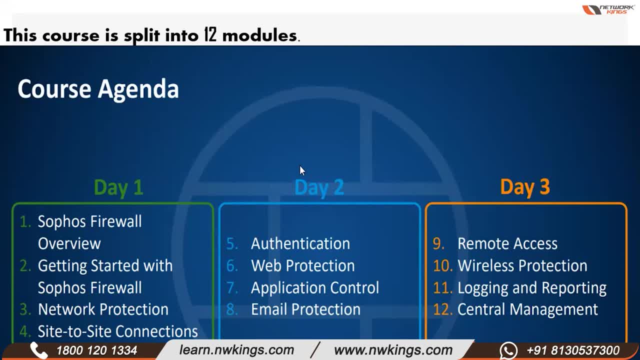 it at the end of the day. So the third module is here. We will cover all the network protection related configuration. Then we will cover the fourth module, ie site-to-site connections as well. It's not about day one, but if we have queries in between, we will definitely. 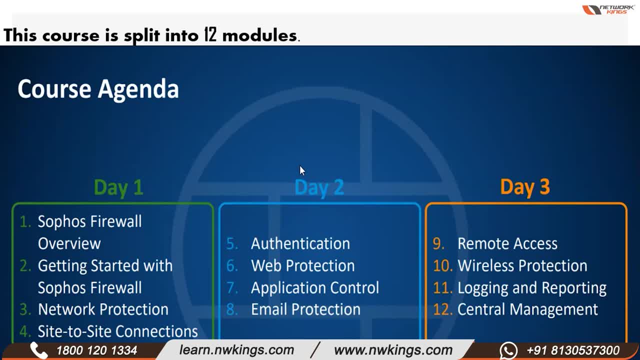 sort them out. If it takes time to go ahead, no worries, we will shift the module to day two, for example, and so on, like this way. So after site-to-site connection module, we will go through the authentication. How can we enable and use authentication in Sophos? 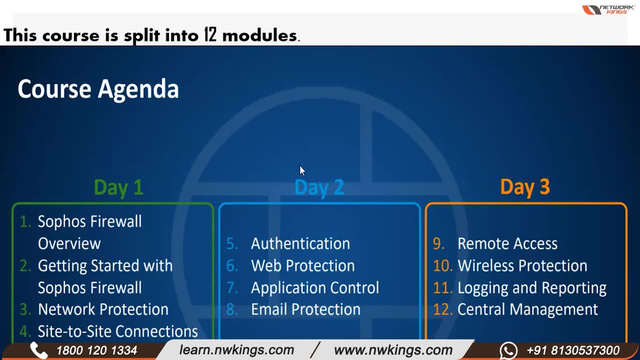 Firewall. In the same way, web protection and application control can also be used. So we will go through the authentication. How can we enable and use authentication in Sophos Firewall? In the same way, web protection and application control can also be used. So, after site-to-site connections, we can enable and use addition. 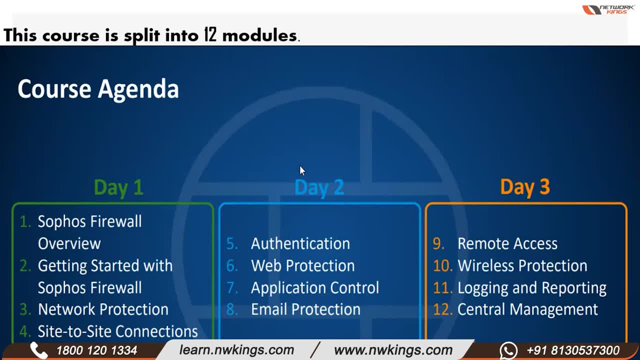 to the наконец business queue after the authentication. same with the email protection. We will also cover remote access like SSL IPsec in module nine And after that we will cover up module ten in wireless protection. When looking at wireless protection we notice 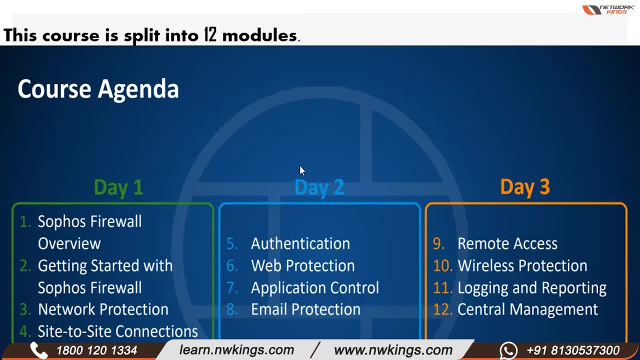 that products of Sophos only get AP. so generally, how can we secure or configure it? So we So everything is covered up in module number 10, then in module number 11, when we will do all the configuration after each module. 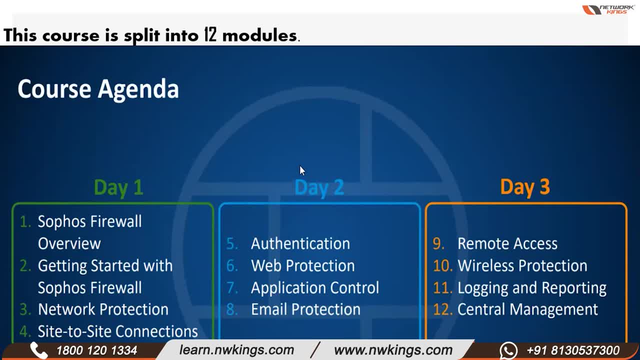 then how its log and reporting works with Sophos firewall. definitely we will cover up from 11 modules. Then, last, we will also look into the central manager, that is, Sophos central, how we can use it to tie up our error management security. 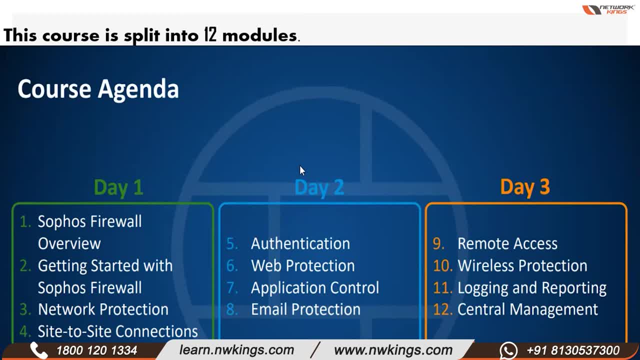 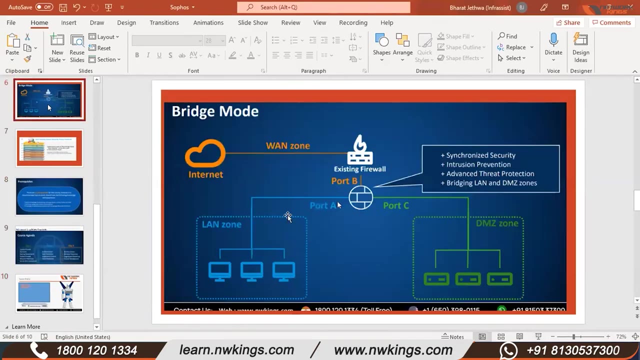 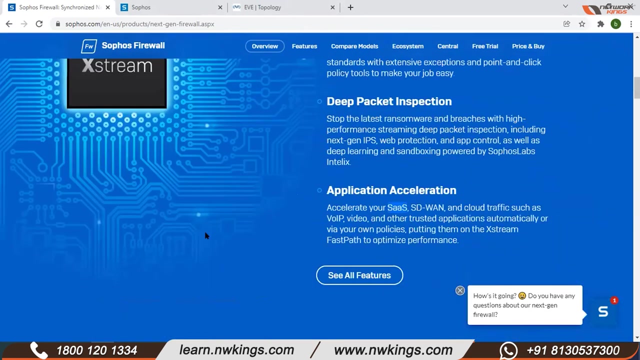 So here, generally, the motto of Sophos is Synchronized Security. So after, from 1 to 12, once we cover up all the modules, we will cover up all the modules of Synchronized Security. Okay, So if we go to the website? okay, we have already taken an overview of performance. 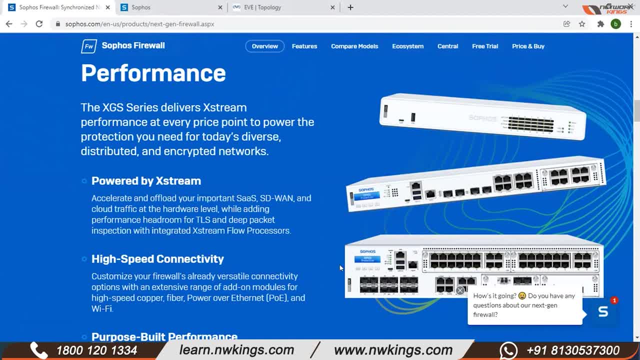 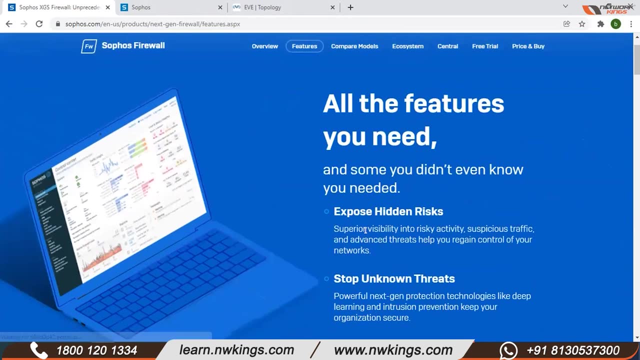 This is already told about our little modules of Sophos. But if we go in detail then we can compare models here according to our business need. So if we go to the features, then Sophos makes all those features available which are currently available in the market. 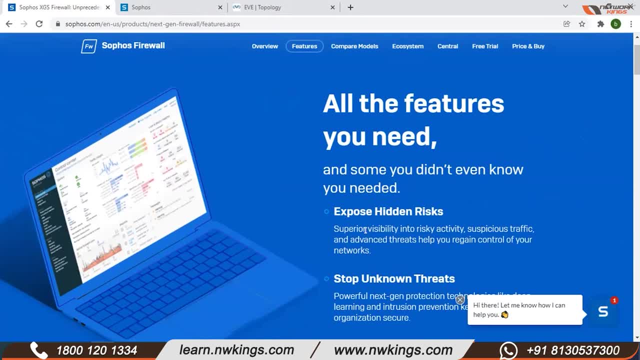 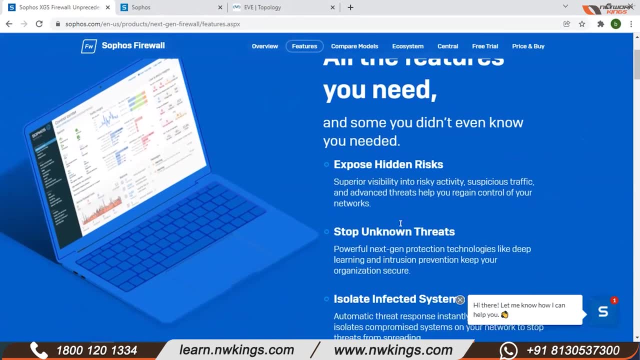 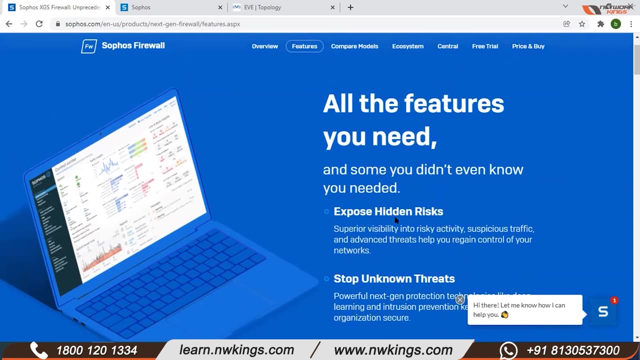 All other firewalls, like FortiGate, Palo Alto. there are many other firewalls too- The features that are available. Sophos also provides them. It will provide you here. So all the features of Sophos are already mentioned here, Like how we can protect from if we are exposed to high identities. 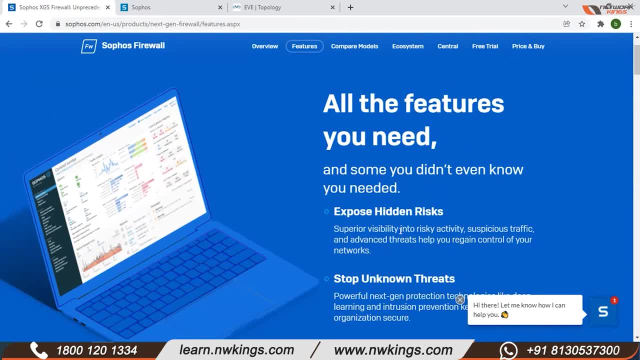 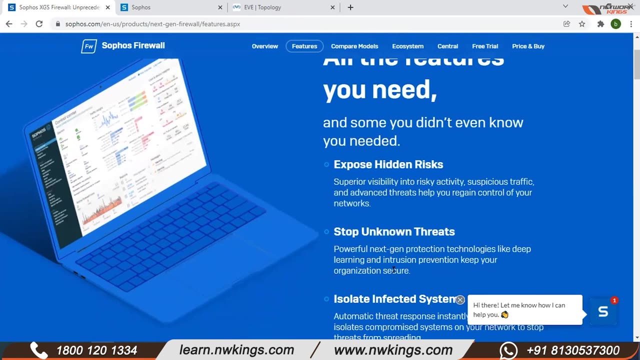 If we already have a network in which a lot of suspicious activities are going on and we have to protect it. So we have already provided Sophos firewall. By scanning it, we can sort out everything Same way. Sophos is also one of the features of the unknown threats. 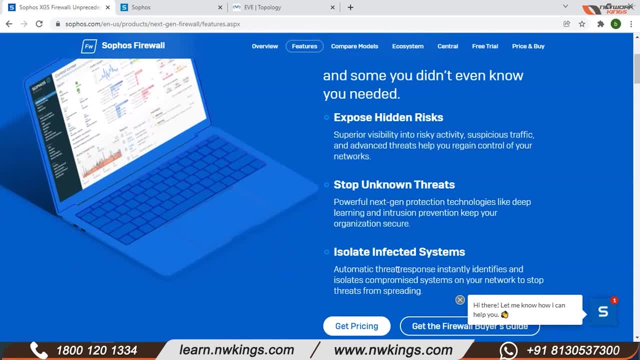 So it uses deep learning technology. So, generally, what we will do in Sophos firewall, we will enable all the scanning, like HTTPS Intrusion Prevention Systems. By enabling all these, we will verify how it works actually, Whatever the threat is Or any hidden exposure in any system. 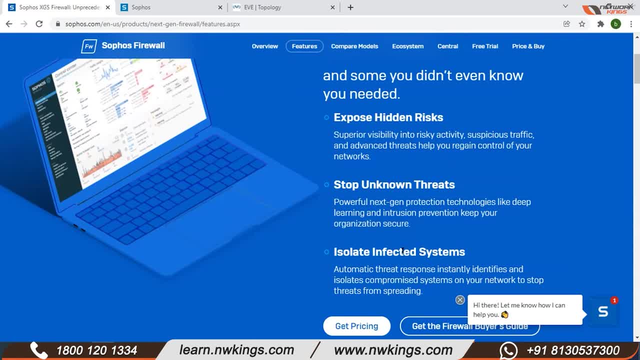 So how it works. We will also see this feature. Isolate infected system is also one of the features in Sophos. So generally, if there is any other compromised system, how it isolates it, We will also see that in the modules. 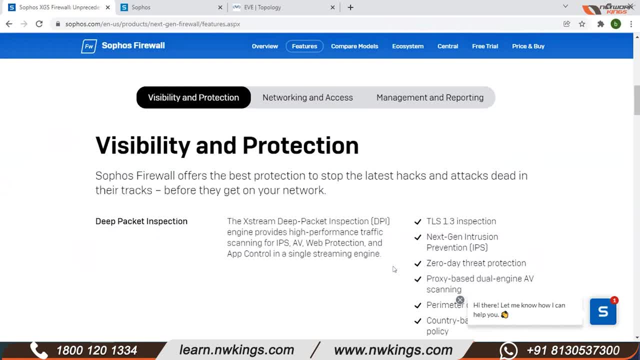 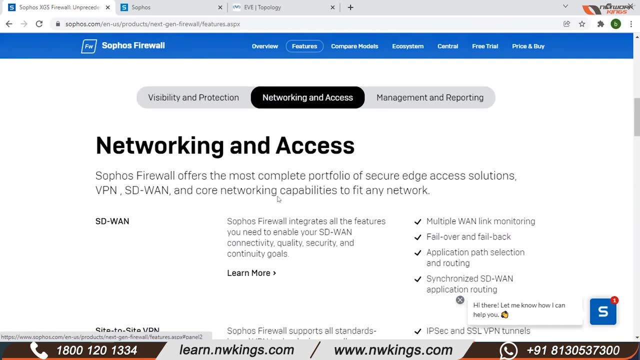 Same way if we go. So why Sophos firewall? Sophos has already provided a very good document here. So the visibility and protection, How we can configure the network, give it connectivity and give it protection, Same way, all the features are available. 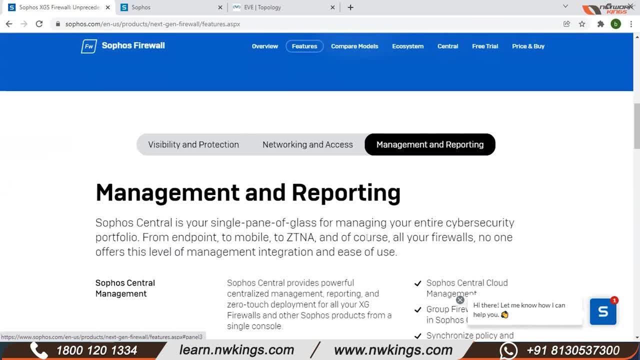 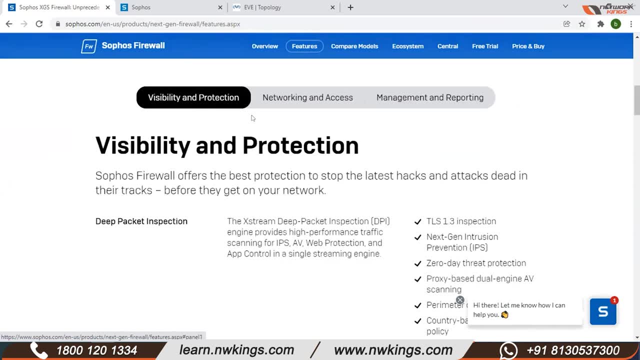 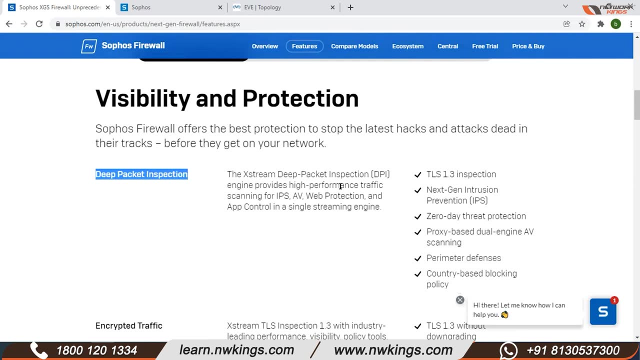 As well as management of reporting. So how we can manage it and how we can report it, All those features- Visibility protection, Deep packet inspection- will be done in it. Generally Its feature is extreme deep packet inspection. We will see how it works. 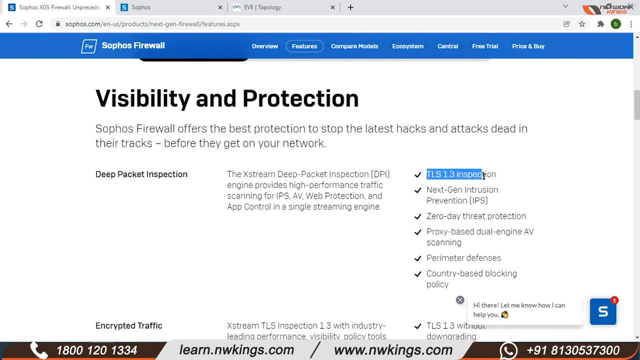 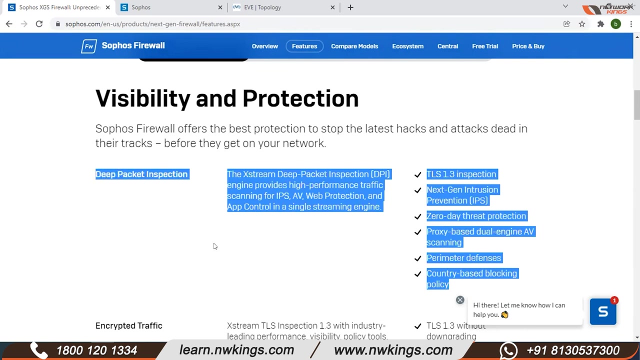 It uses all these features, like IPS, TLS inspection. It will do all the inspection. Then it will use the IPS technology As well as the zero threat protection, Proxy based dual engine scanning And perimeter for defense or country based booking. We will use all these features in the configuration. 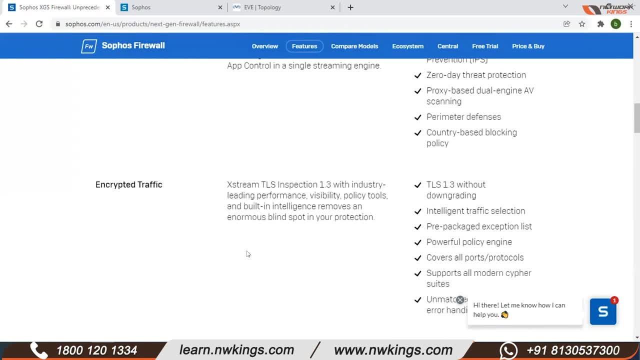 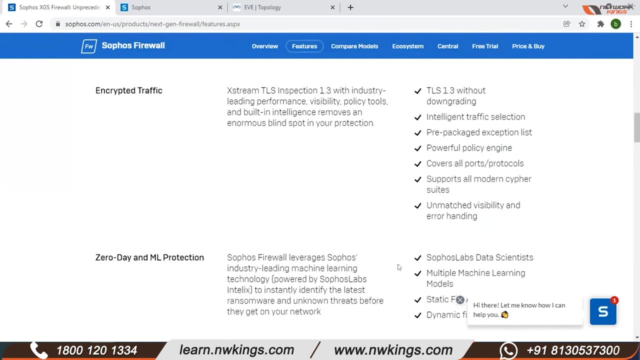 How it works Again, how it encrypts the traffic with the extreme protection, How the latest TLS3 version is being used, How it supports all these protocols. We will check that in our network operation. Same way with zero day and PL protection. 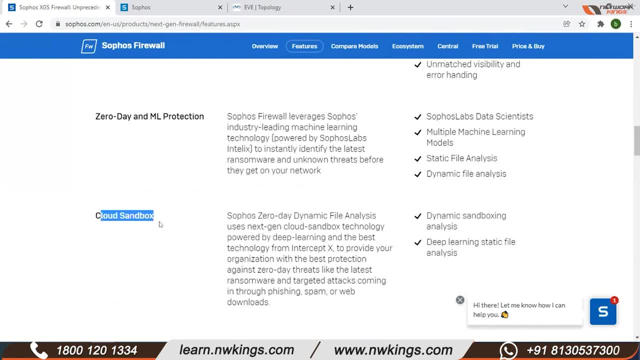 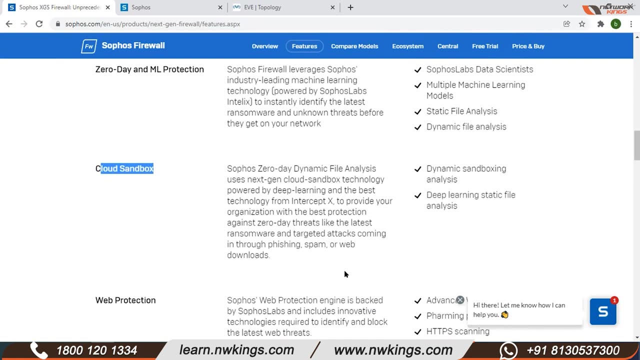 In this there are some features like sandstorm. So in sandstorm technology we will cover up in the module We will see in the lab, if I can provide you that, Because we will need a license in sandstorm If we are checking in the lab environment. 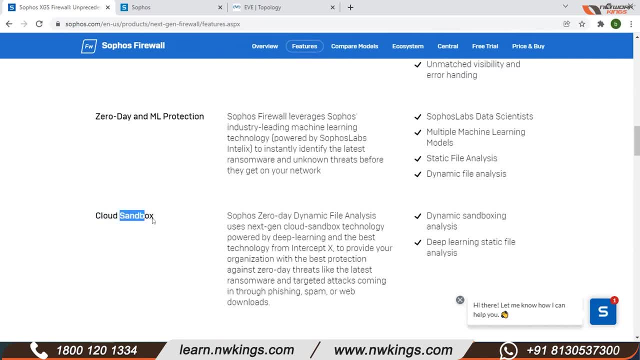 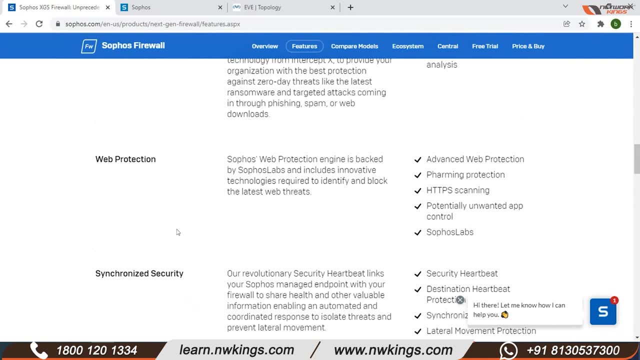 Okay, So it also uses sandstorm technology, Zero day protection, Encryption, packet inspection. Next, there is also web protection. Like it scans all HTTPS traffic On potential apps. How it will scan the software firewall From the firewall In all the systems. 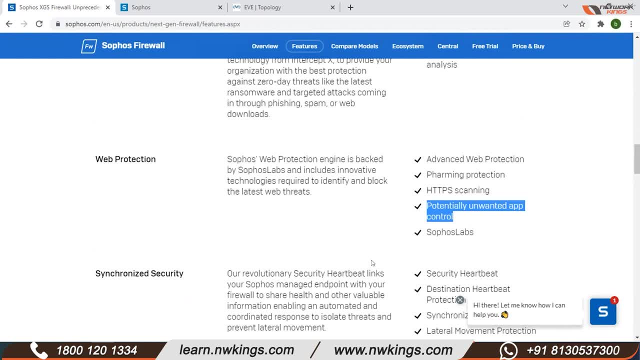 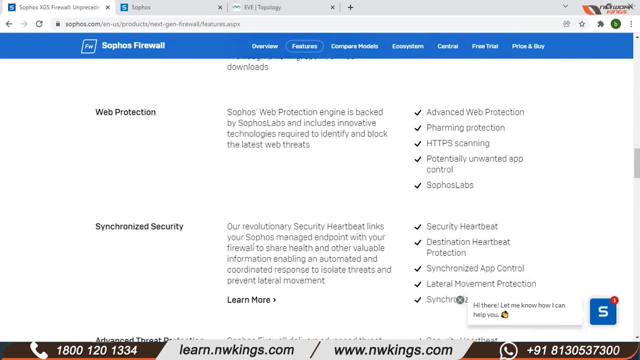 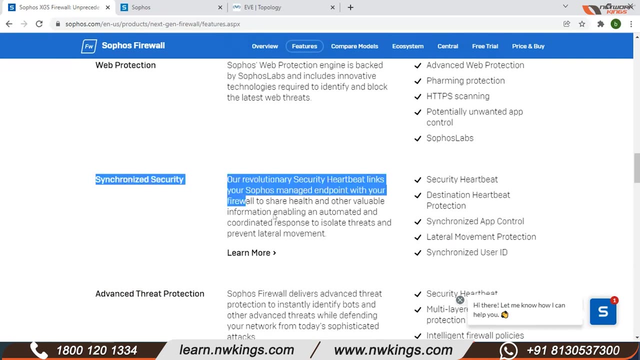 If there are any systems there In any organization, How it will scan it In web protection. We will see that. Then we will check the synchronized security, How we can enable synchronized security Generally in this, if we cover up all this in modules. 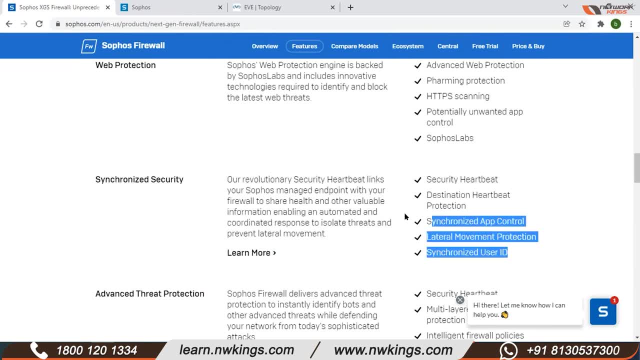 Generally, what happens is that there should be only softwares products in it To meet all these requirements. We will also see that in our lab environment. So how does synchronized security work, Especially with advanced threat protection? Whatever features are available, Like security heart beat? 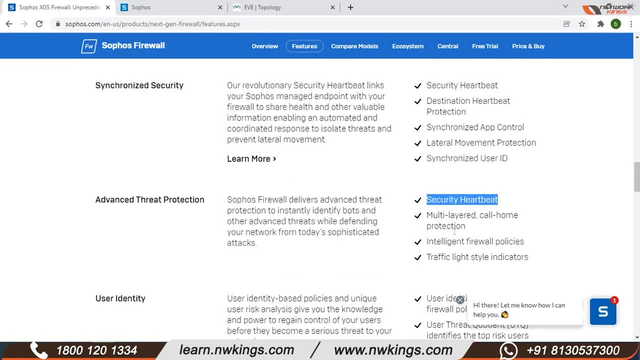 So how does security heart beat work? We will also go into detail about this. Generally, the health status of this device will give you in the firewall. I will tell you that soon, Right now. I will also tell you that. How is the insight of this? 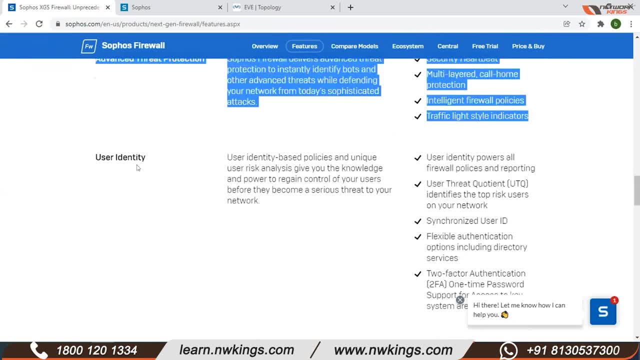 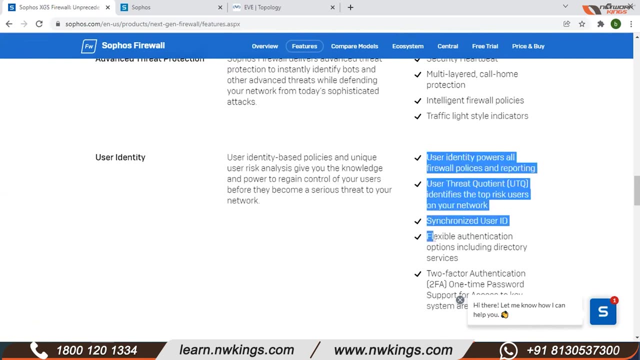 So advanced threat protection? Yes, of course. user identity, How authentication helps to analyze which user is doing such risky web browsing, For example. So that gives the full insight. So which features can we enable in it to overcome the serious threat? 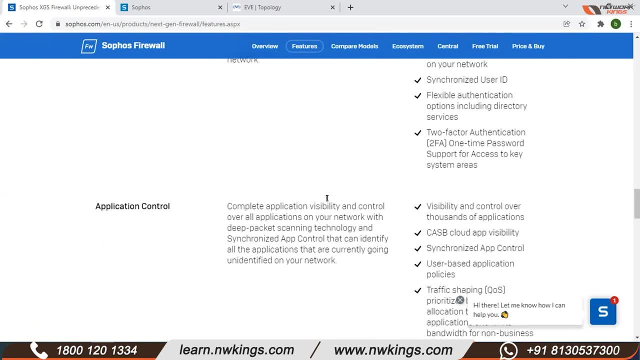 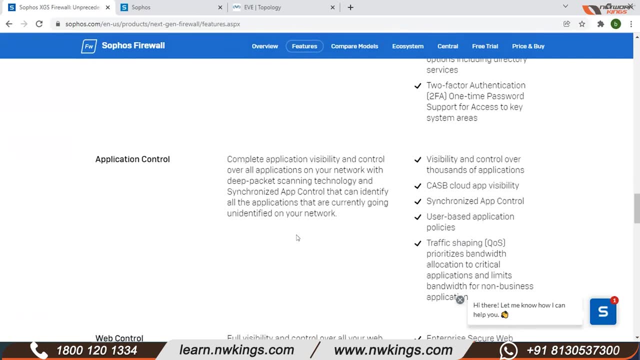 Okay, Same way with the application control. Just like we have web control in the web control, Like application control, So in that too we will use the feature of synchronized security Generally whenever we have this topology ready. So let's say, for example, if there is a user who has installed an unwanted application. 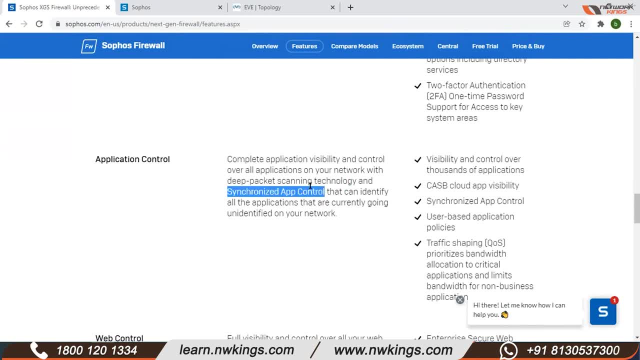 So synchronized security. You Send the application's detailed firewall from the central And you can categorize it accordingly. We are definitely going to go deep about this. How does it actually work And all the features we can enable it. We can enable it and check it. 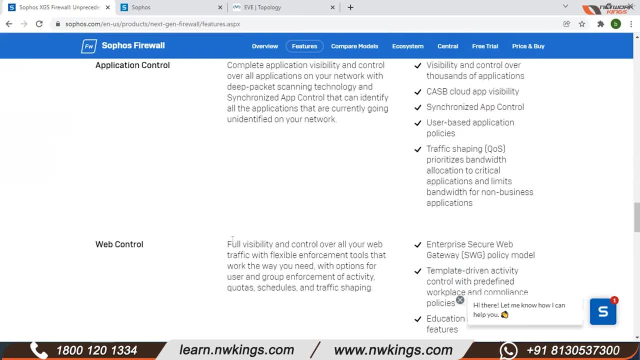 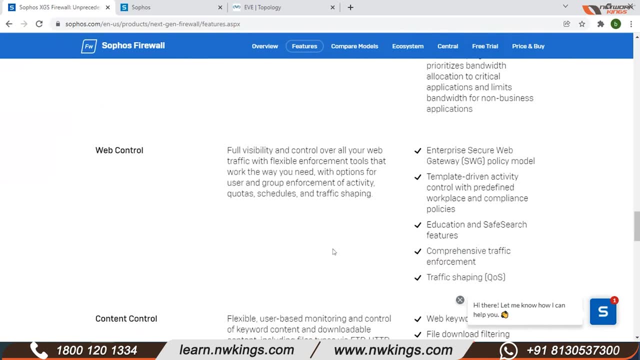 Okay, We will also see in the control How can we control the traffic With the help of the software firewall In it. Generally, we will use it. We will see in the lab environment. How can we apply policies As a user or as a user. 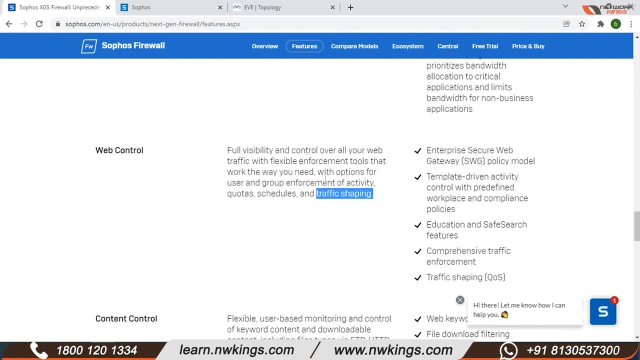 Like, for example, QoS Or bandwidth. So we will see all these features in the module As well as in our network topology On our course. Okay, So these are the features Which are provided by the web controls. Generally, the education's web feature is more important. 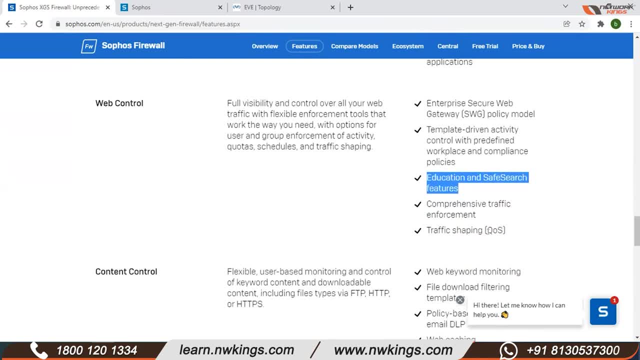 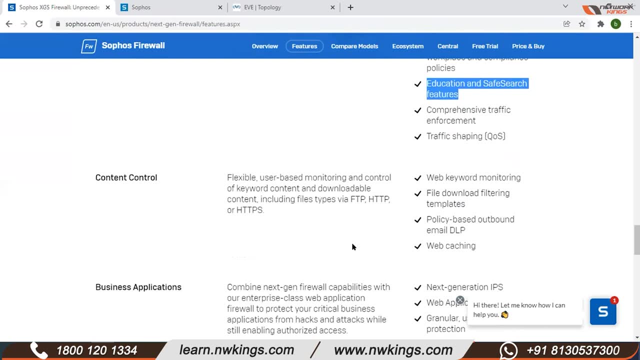 We will also look into that, How we can meet the requirement for the education's And rest of the organizations. Content controls, Like if there is a keyword related Download event content, How can we monitor it, How can we block it? 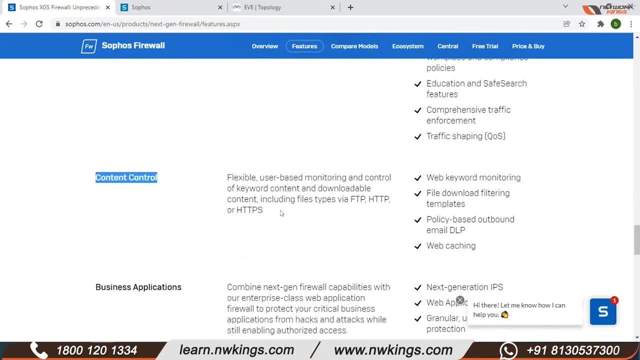 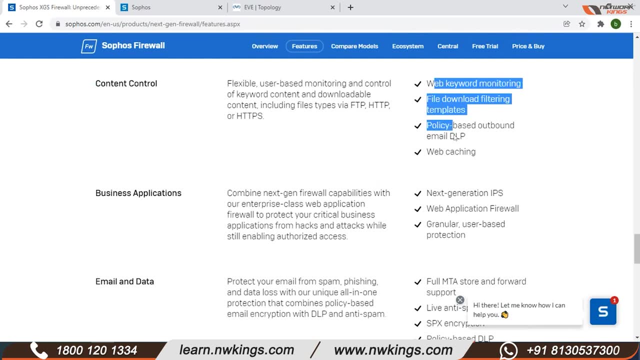 We can use content control. We can use that feature in the firewall Along with the web control. So all these features, How can we meet the requirements of our features From the firewall? We will see that. Application control: We will also look at the application control. 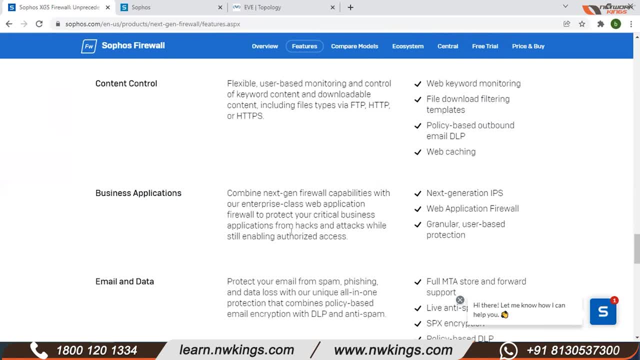 Like if you have an application In case you have to do port forwarding, But the software of the firewall. For example, on our premises There is a web server- If they have to host it from outside- Port 4434,, for example. 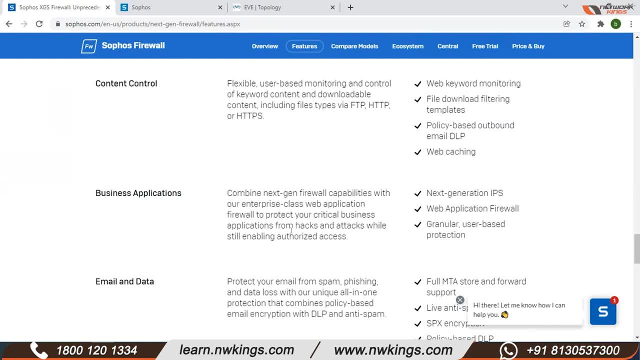 How can we protect it from hacking and attacks? We will see that here With the gun, With the web Generally. this is a web, So generally, how does it work? We will also see this Web. Lastly, email. 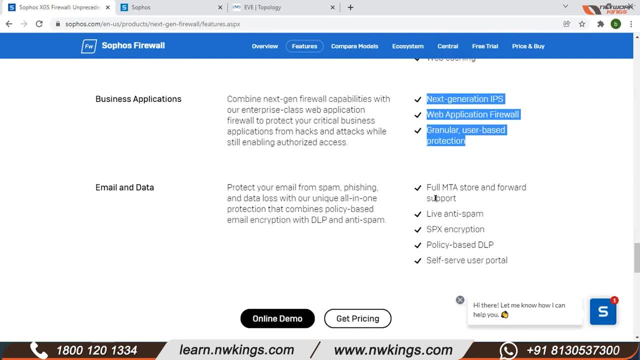 If any, If we From the software, The email traffic is going, For example. So, with the help of the MTA mode, Which we will discuss in the module too, How can we stop spam? We can stop it. We can stop phishing. 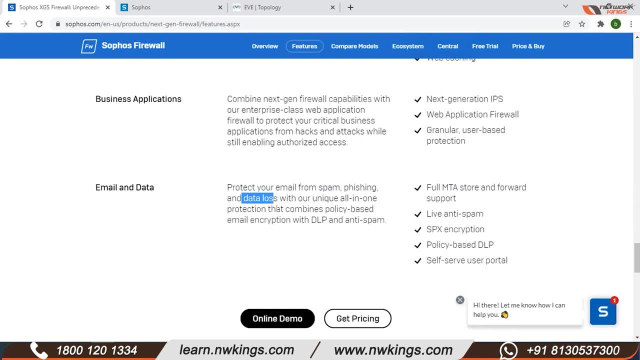 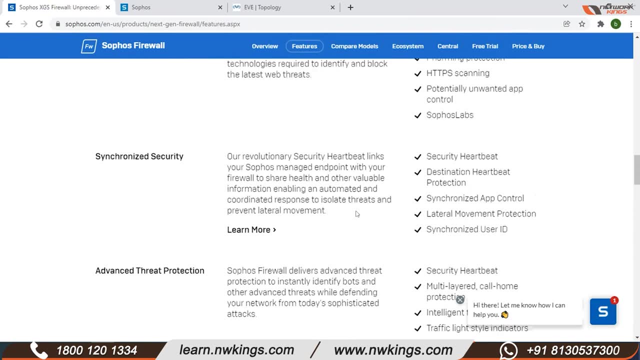 Or if there is any data, So how can we do that? We can meet it with email data. We will see that in detail. So here you will get visibility How. Which features are in the firewall, Which compared to other vendors. 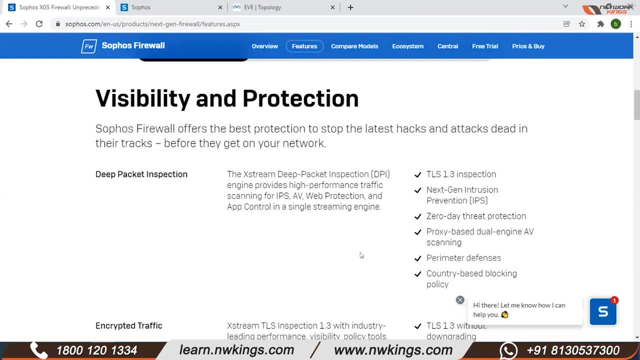 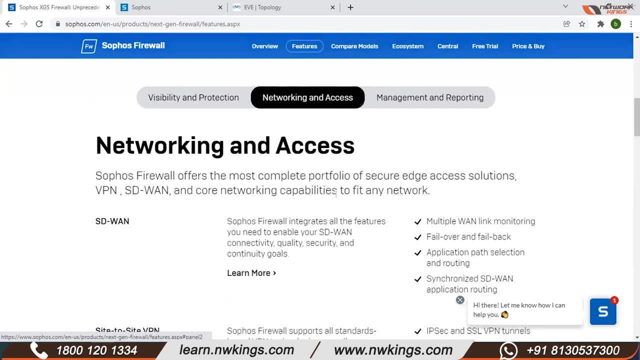 We can meet. There are more advanced features here Which will give us insight If there is any type of attack Or malware attack. So definitely The network will give the best security. Same way With the networking access. We 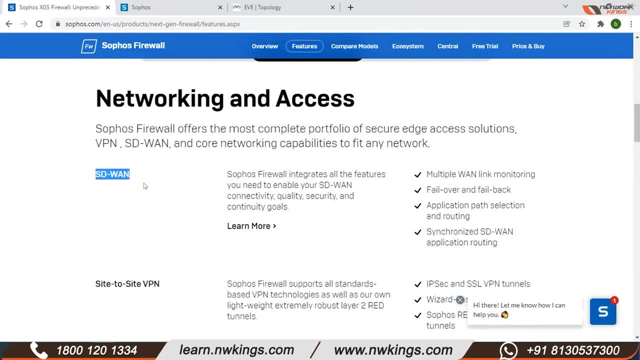 The features in it, Like Now Most popular SD-WAN. So how do we From SD-WAN software, How do we Our business Requirement Or, if Already, If the software is firewall? So How can we use SD-WAN? 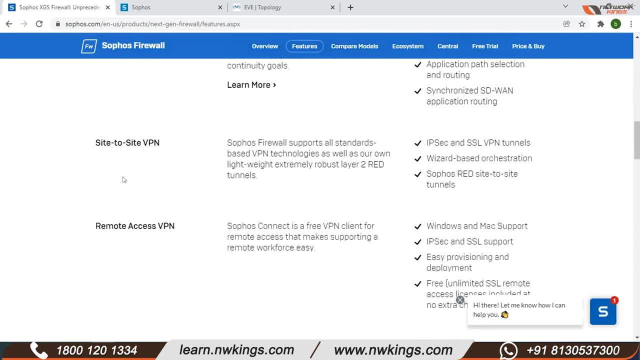 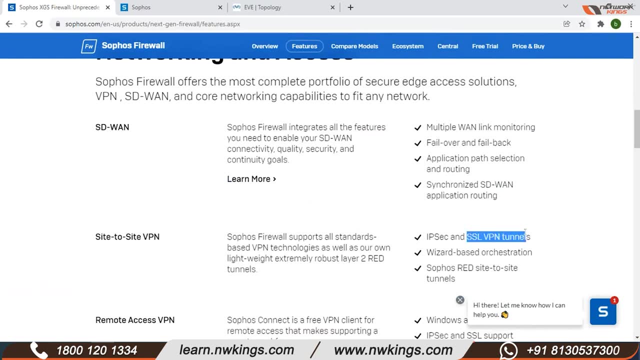 We will discuss that Similarly Site to site. Generally, In site to site, We IP sect, IP sect Or SSL Tunnel. So We will see that Even One of the software Red device. So 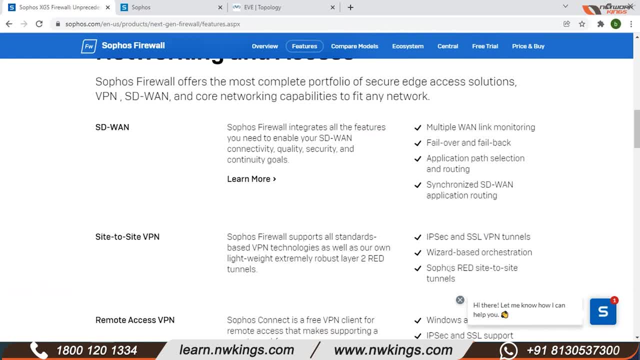 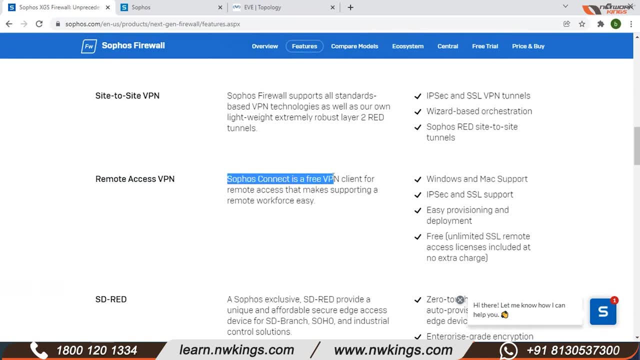 Remote Ethernet device Which Site to site Connect. How to use In the software. We will see that too. Then We have Remote access. How Software Connect Which is free? VPN, How? How? 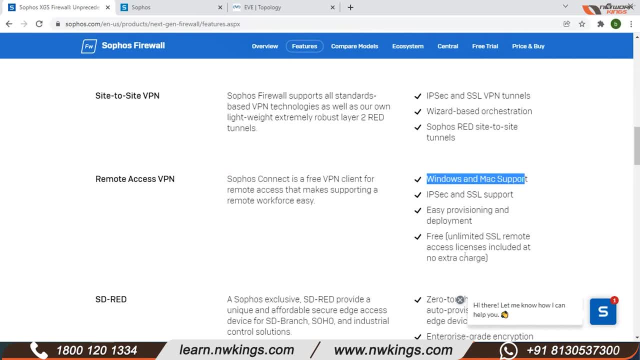 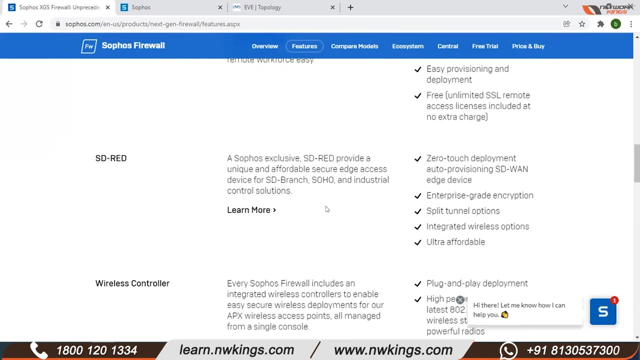 Mac Windows How Installed. If User Someone Out of Resource Access From Outside, We have A server From Outside Work From Home. Then We Can Use Remote. 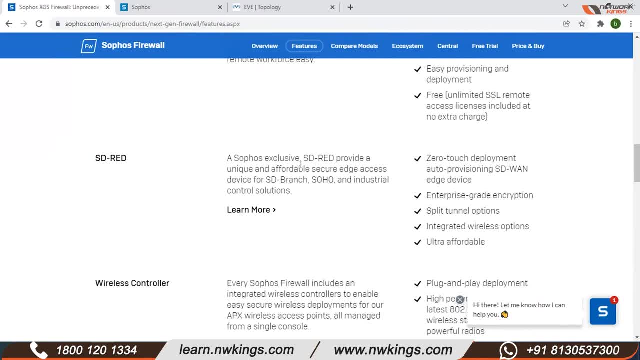 Software Connect Similarly So, Of Course, From SD Red Configure Generally Site To Site Any Head Of His Branch Of His, And It Provides Zero Touch. 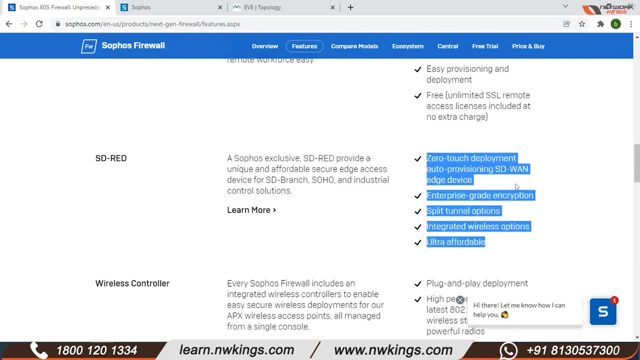 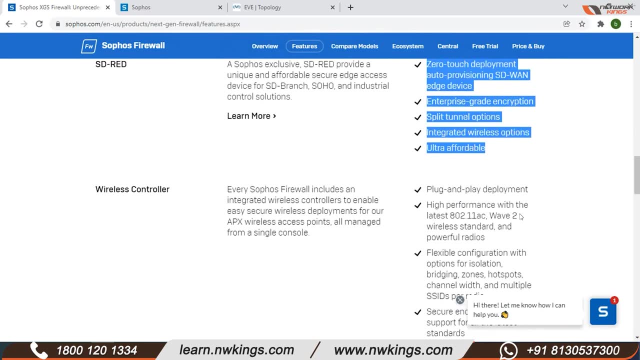 Development Plug And Play. So If I Will See You Later On, Then If You Go Ahead With The Wireless Controller, So Suppose It Is Generally. 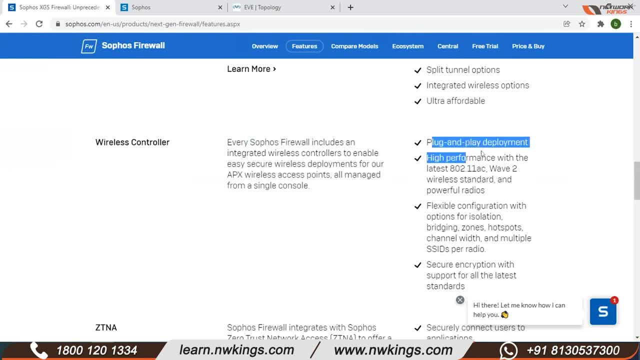 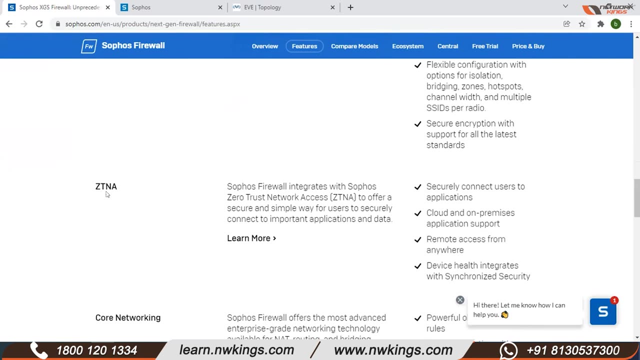 Work As A Manage. The First, I Will Say You Will Have A Look Into The APX As Well From The Website Only City And 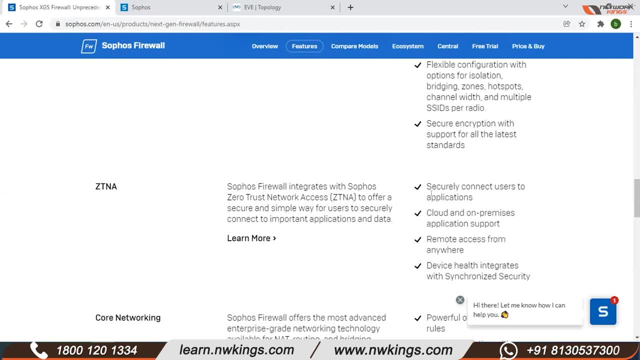 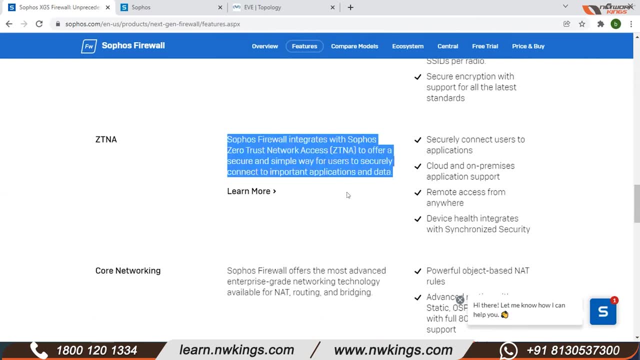 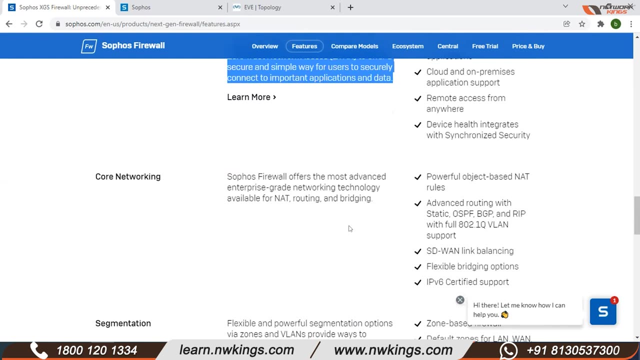 It Is Zero Trust Network Access. Who Be One Of The Another Features The Future. I Can Use Connect Working. I'm Connect Working, Be So. 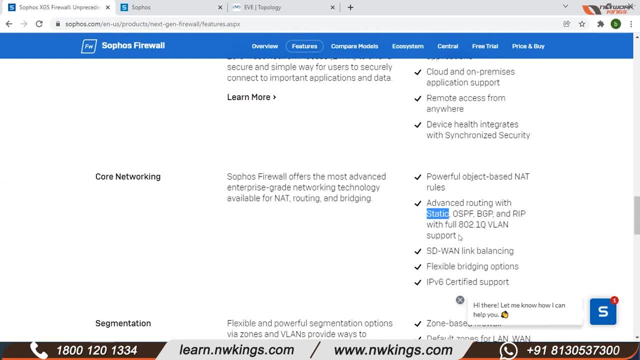 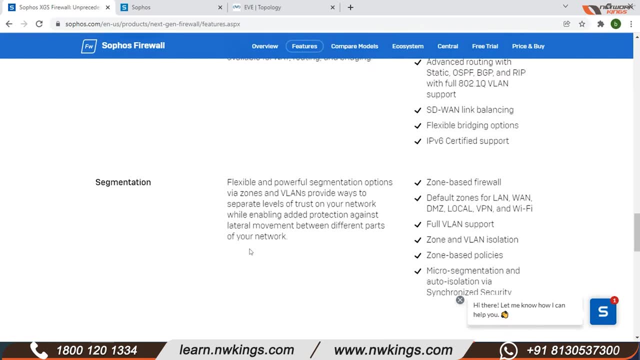 First File Maker, Like We Been Net Net Object. Yeah, Fear OSPF. Yes, You Have A Business Connectivity Thing. So Zone Base Riga, So It's. 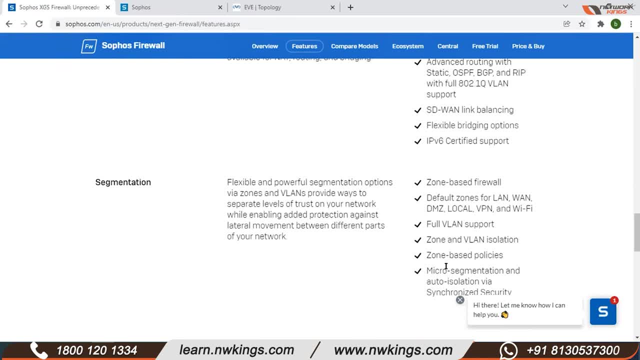 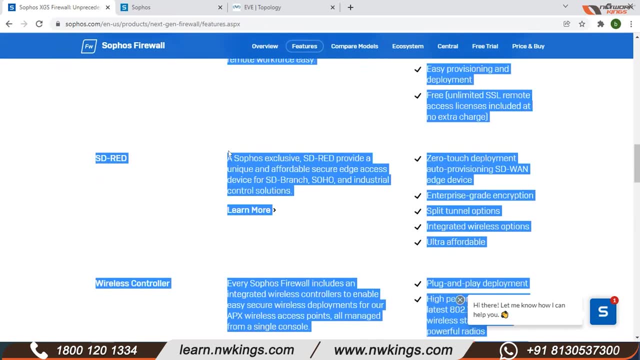 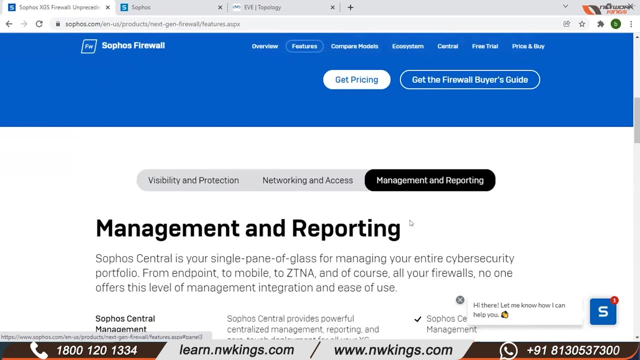 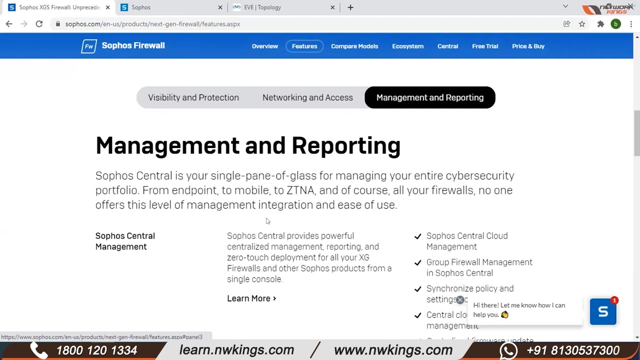 Support Full Will And Also The Zone Like DMC Or Wi-Fi VPN, So We Can Segment Our Network Is Simplified Segmentation, So Output Get. 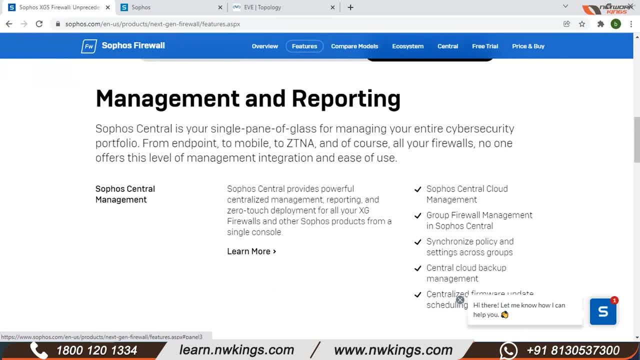 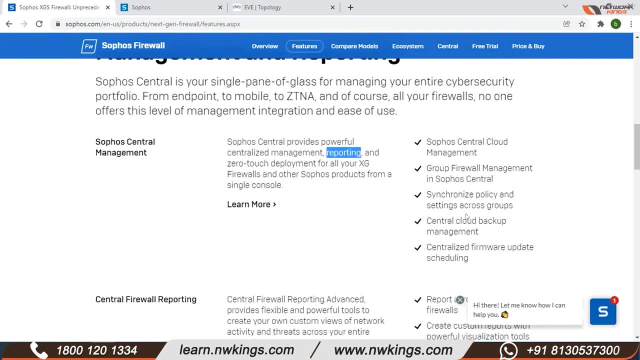 All The Other One. We Have A Site In In A On The Engine. It Can Gain In The Site. We Can Make A Site And 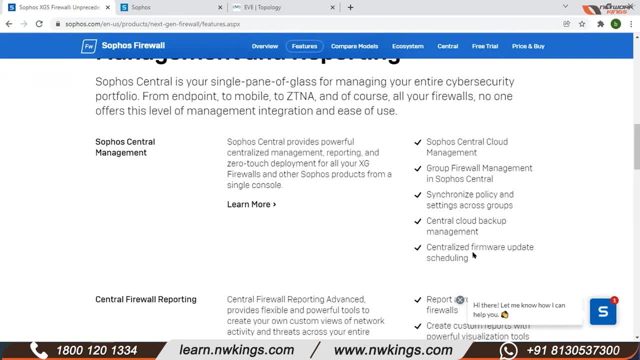 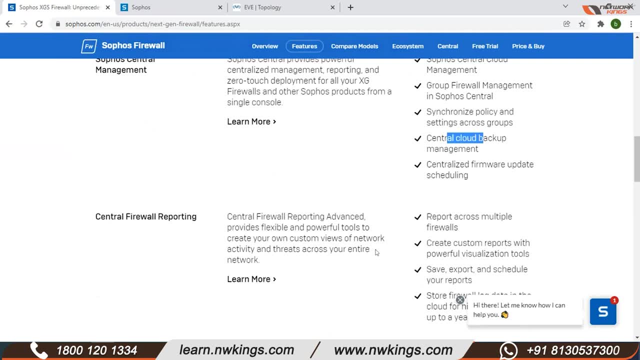 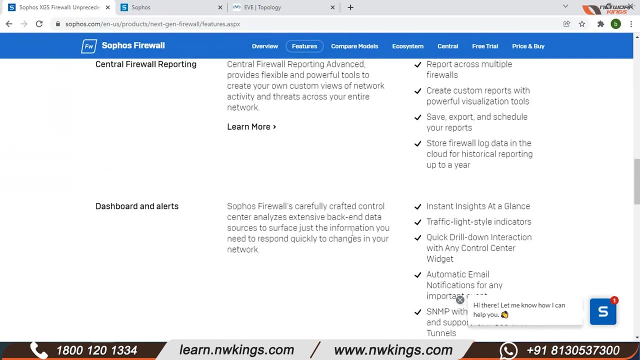 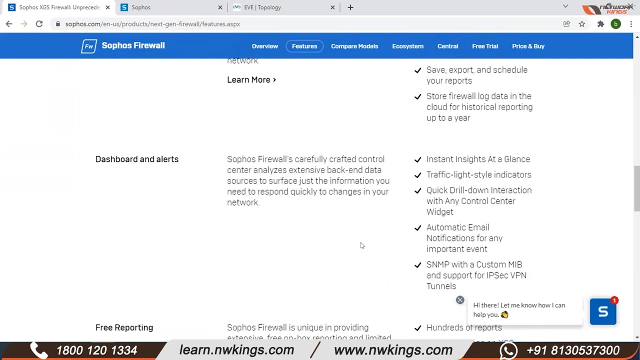 We will definitely see all these features one by one from centralized firmware, how we can upgrade the software from software central, as well as the reporting part. So the dashboard is fine. we will also see what we will do, how we will integrate it from software firewall and how we can serve it in the cloud with all the reports. 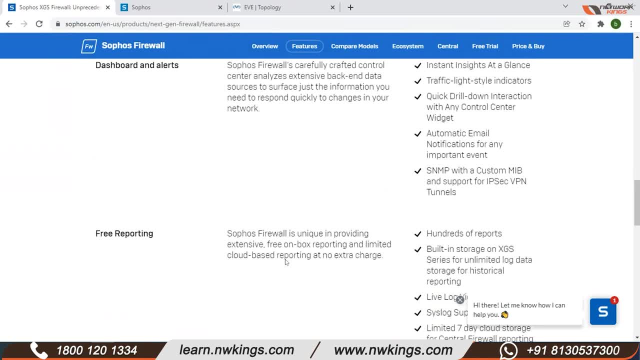 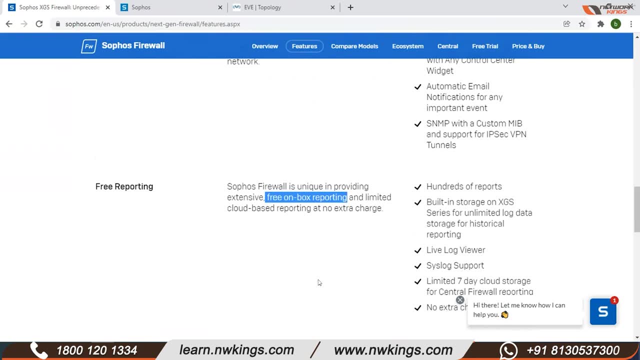 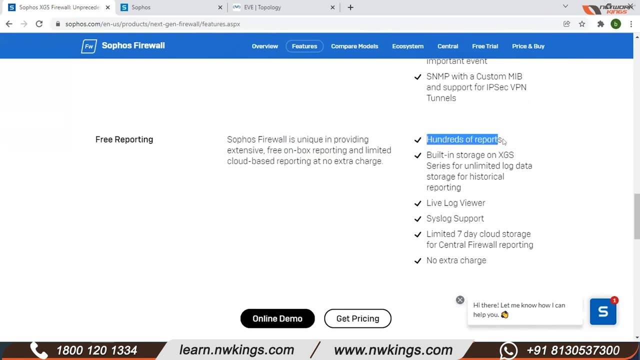 We will see all those features. There is free reporting. if you have purchased it, then it will be free, But if we are managing from central, then definitely you have limitations of 7 days. So we will go into detail about it one by one in the course. 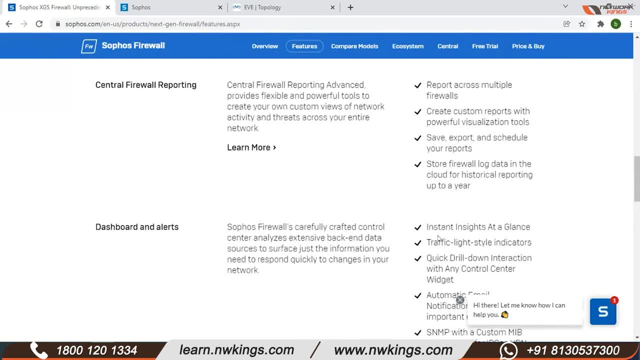 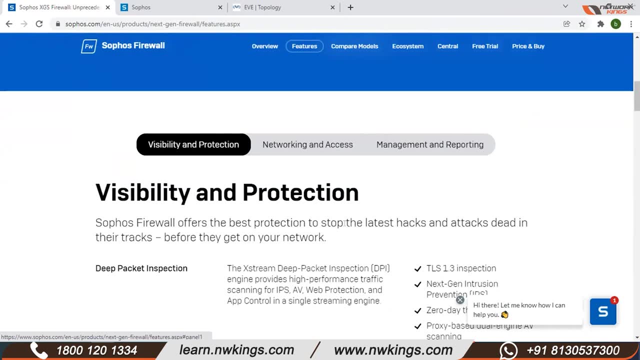 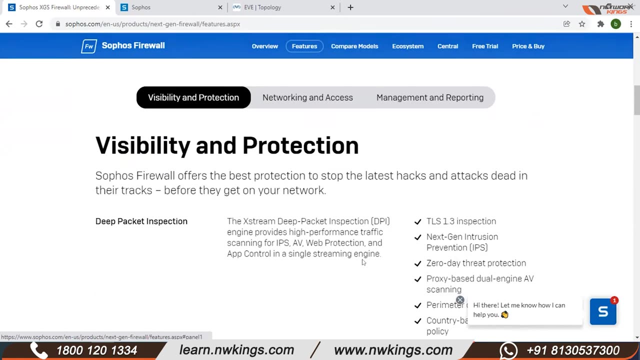 How we can check all this. So these are the features available on Sofos XE Firewall Which help us in small scale businesses, how we can deploy it as soon as possible and secure it, And how we can meet business requirements with firewall. 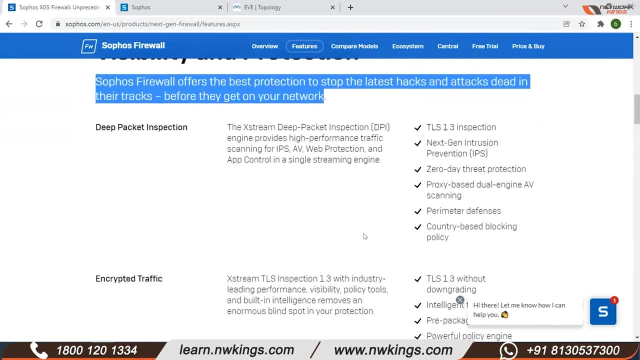 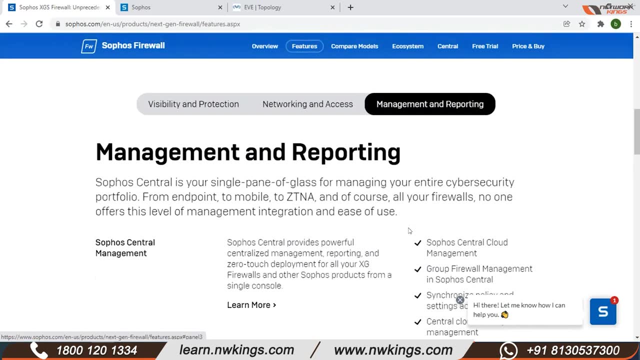 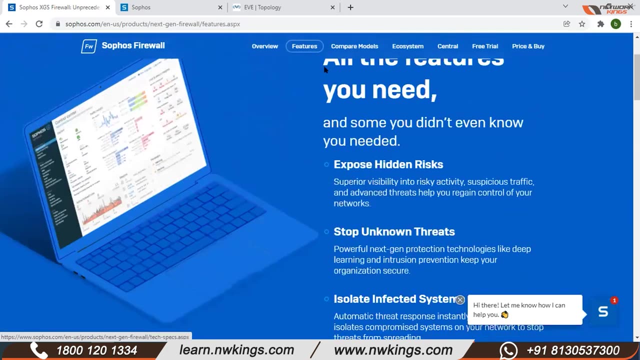 All the features are available which we can use to give the best protection in the world. So we will have a great look through the modules, as well as with the labs. Okay, if we go to the modules, Right, let me go there. 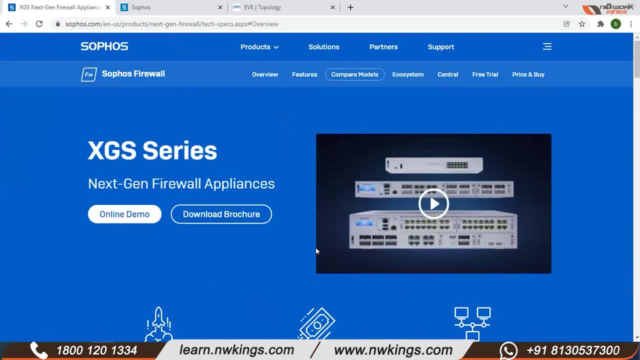 So now there is SG series. As we say generally, this is the new feature, the next generation series. So now it is XGS. So we will also discuss about it, how it is different in XG and XGS. 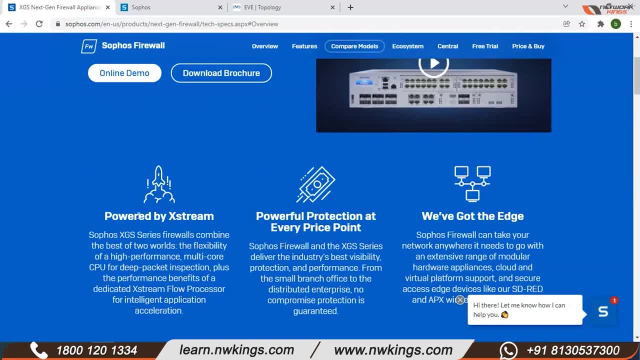 We will see the difference. For example, it is powered by Xtreme. For example, it has flexibility, high performance, It is multi-core, It has deep packet inception. Then we will see the benefits of Xtreme Flow Processor. Similarly, how XG series protects. 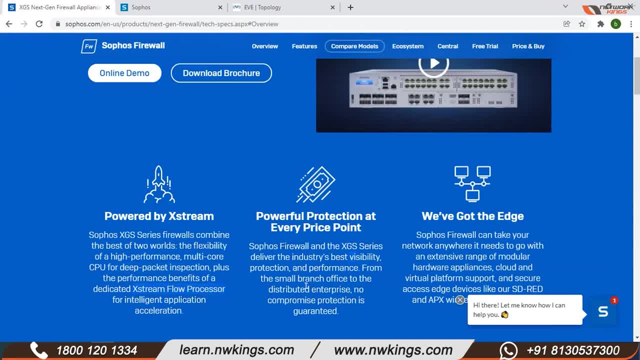 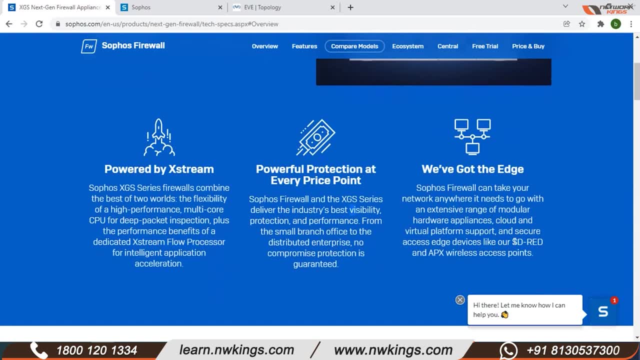 How it has visibility, How it has performance, Small branch to big businesses, how we can meet them. Okay, And a little bit about the different products of Sofos, So we can say that the integrated with XGS we can give you best Synchronized Security. 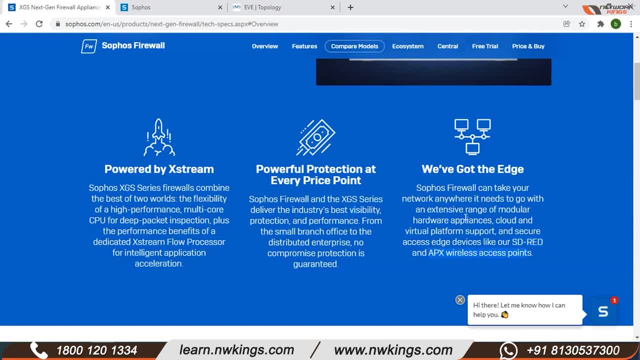 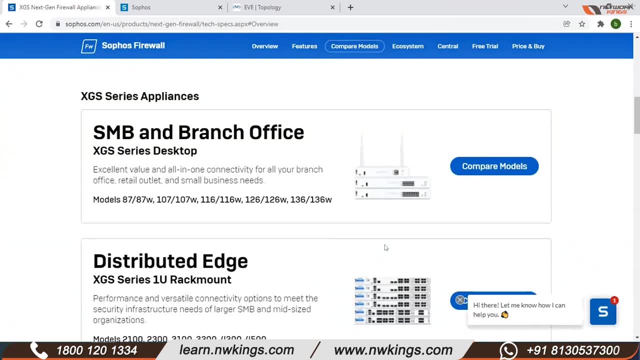 Like if ready or connected with wireless. We will go in detail about that through these modules. So these are the XGS appliances Here. I will give you everything in detail, As well as the hardware components of it. we will definitely cover up in that module as well. 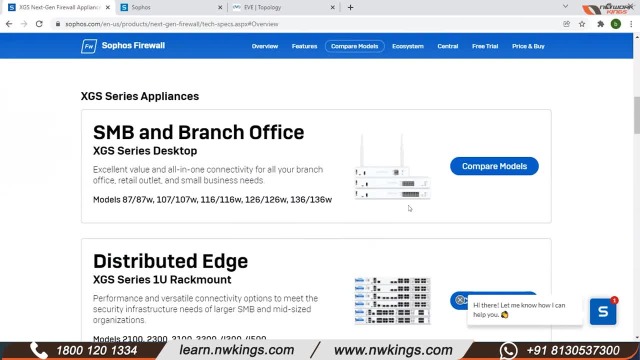 There are some cover-ups in the module, so we will also go through them one by one. So SMB and business offices, like some small offices where you have 5-10 users, 1 user or more than 2 users, but minimum there are 10 users. then you can prefer these modules. 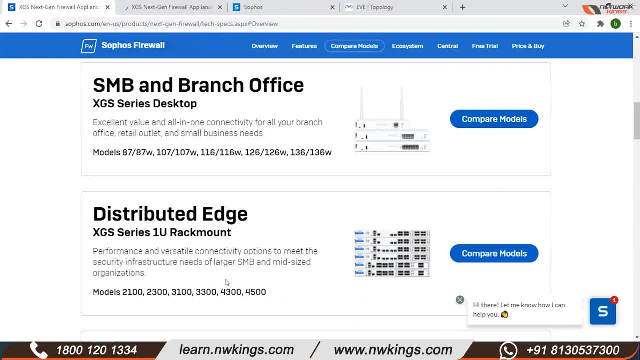 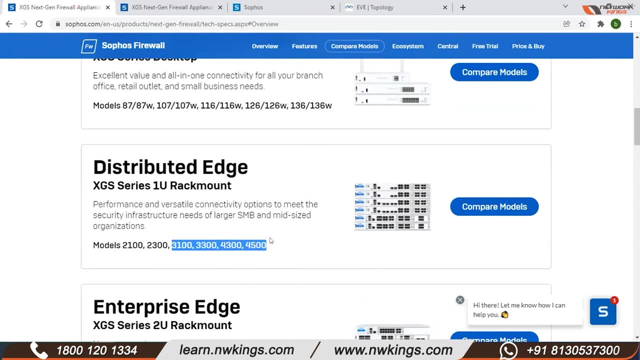 Then if you have more than 100-500 users, we can also take 1-2-0-0-2-3-0-0 modules. So this is a plug-and-play, so it will not take much time to deploy. 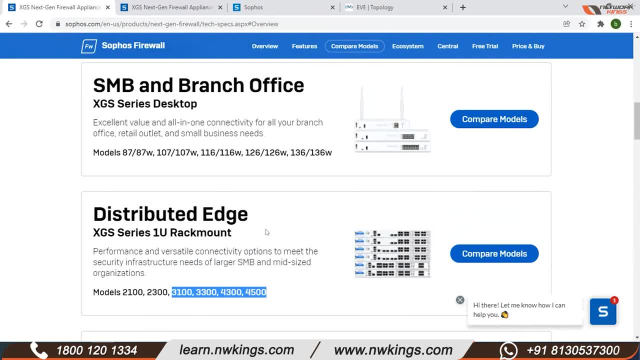 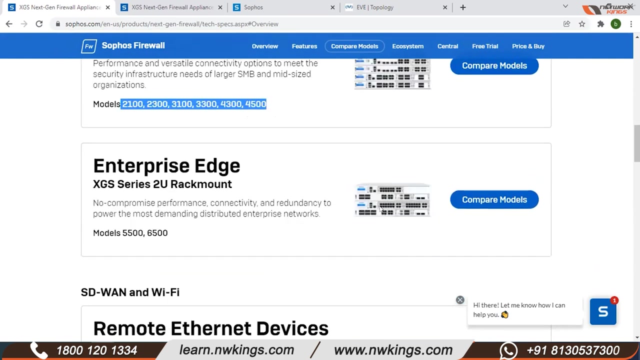 Only once we follow the documentation it will work. After that we can do the configuration one by one according to the business need. So this is the solution. We will also cover the hardware components of all the modules in detail, like medium-sized businesses or large business sizes. 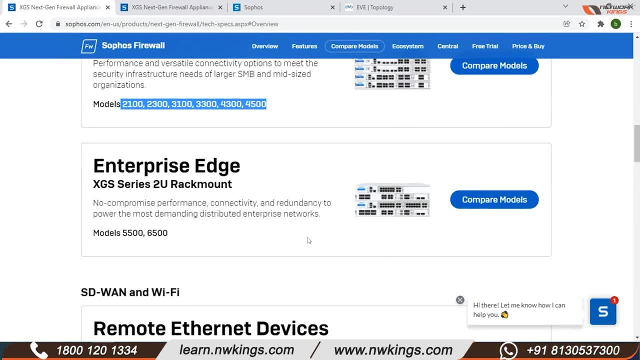 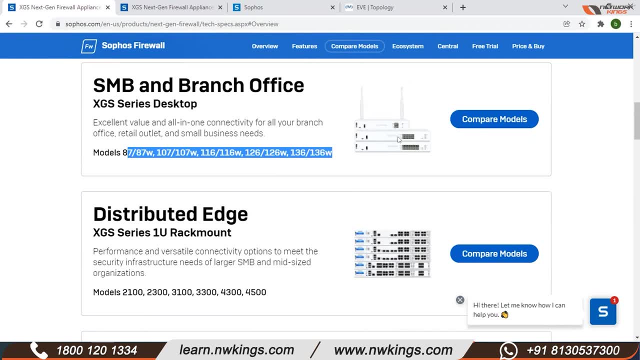 If there is scaling, how can we meet it? We will also cover that in the module. But for the small business also we will look at the hardware component and how we can meet If the scalability increases there. we can definitely do it in this as well. 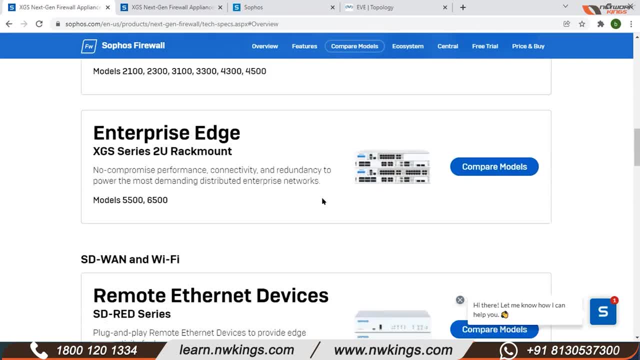 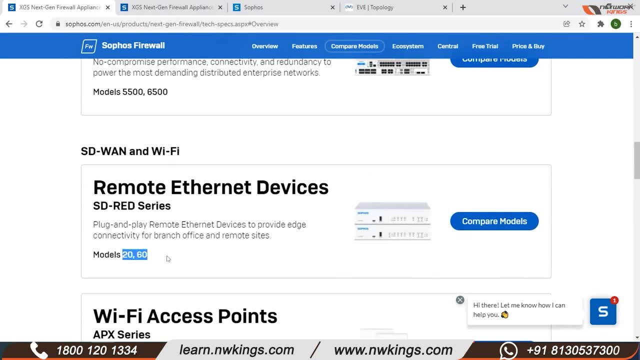 And we will also cover which devices. we can do it in the module, Same way as I said, SD-WAN, the red devices, right? So there are two modules for B, 20 and 60. So if we want to compare it, we can do it. 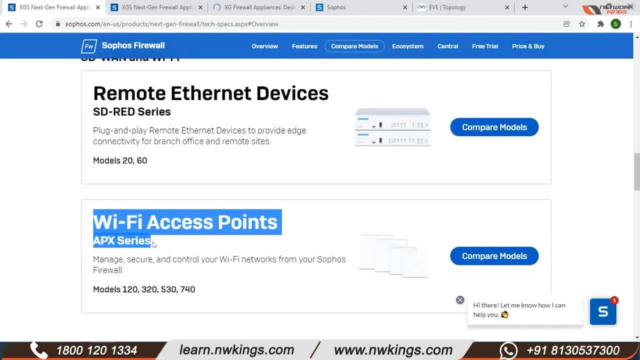 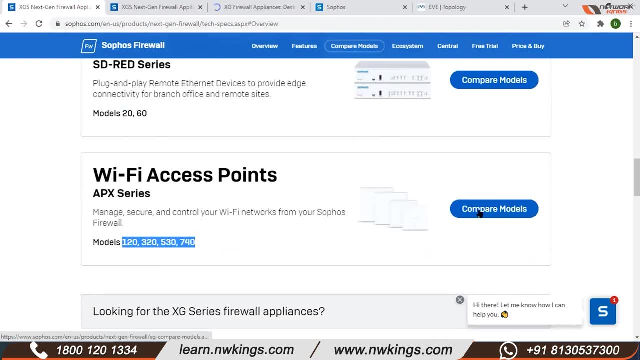 We will get it in detail from here. Same way, we have to deploy the software firewall. Then these are the current modules available that we can deploy. Here we have shift plug-and-play. Let's say, for example, we have to connect it to the switch. 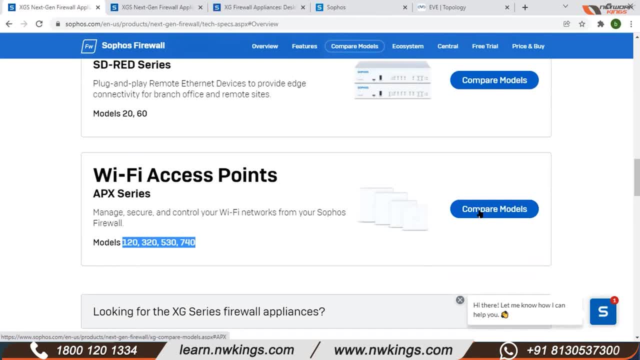 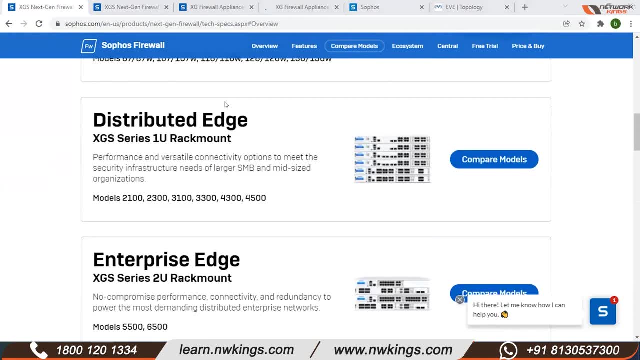 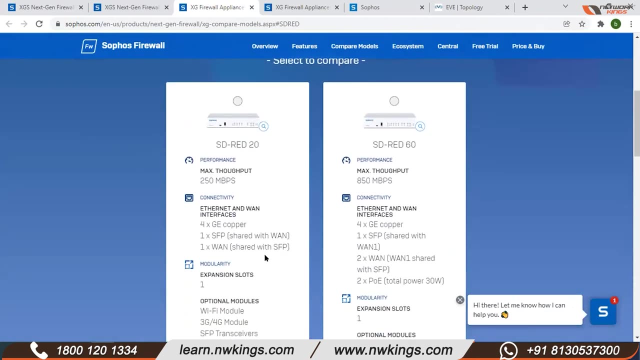 Then rest will be taken care by the firewall. If there is any advanced configuration in it, definitely we can do from XG firewall. So here too you will get all the details of the red device, Generally red device if we have a head office and a branch office. 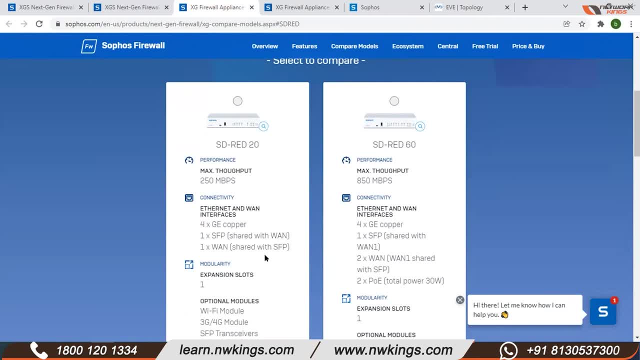 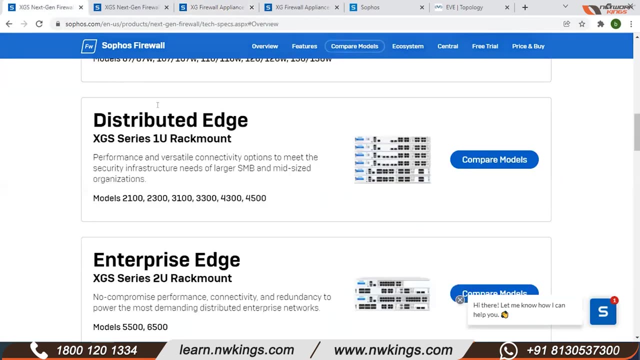 and we have to open a branch office one by one. where there are two users or three users, then we can deploy red there. If the user is going to be constant there and there are very few users, then we can deploy red. So similarly the features in it. as I said here in the features, 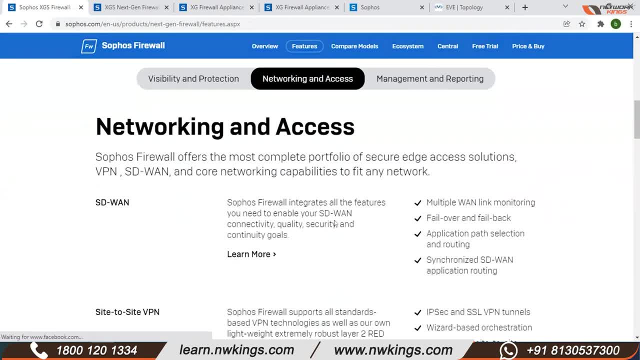 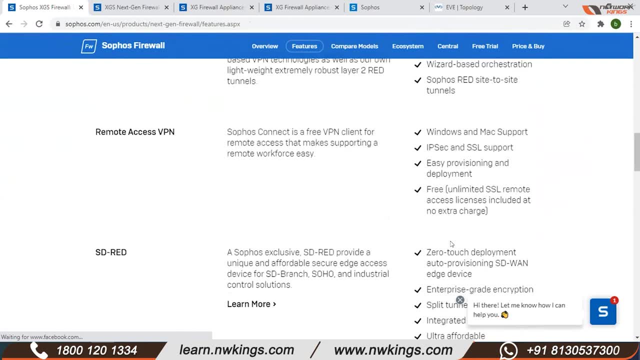 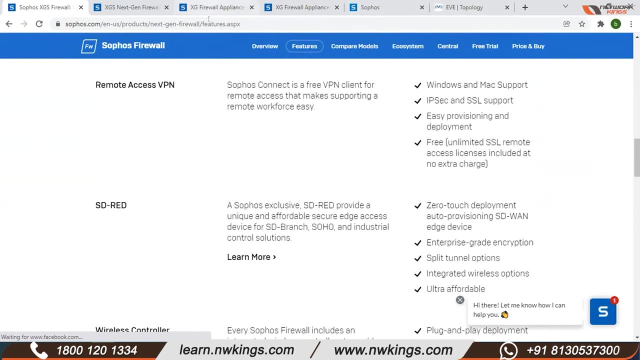 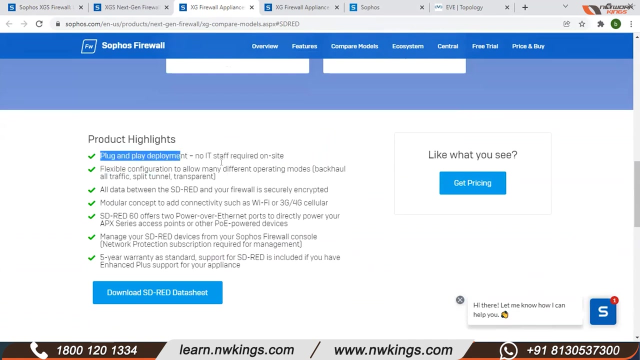 connectivity: SD-WAN. So how can we connect it? We will see all those features later To connect both head office and branch office one by one. So it is as it is, a plug-and-play development. We don't have to do anything there. 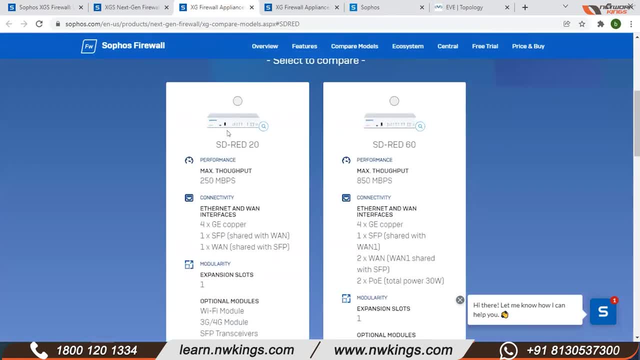 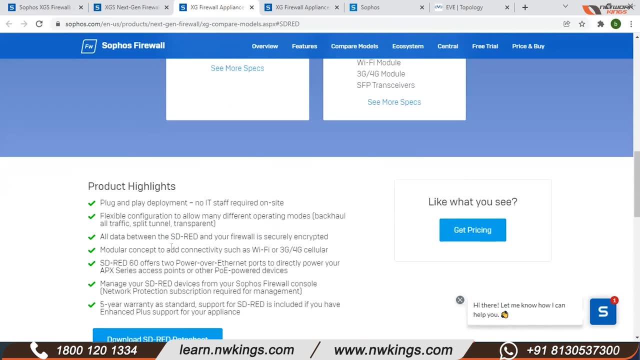 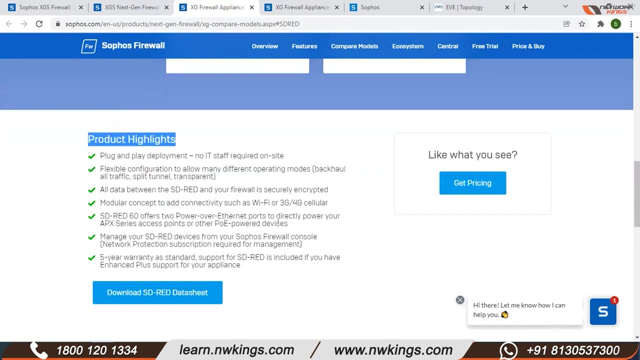 For example, if we are putting a red device there, then we just have to plug-in. We discuss about it in the module in the future, So you will get all the details of it in this website. What are we supporting? The product highlights will be available here. 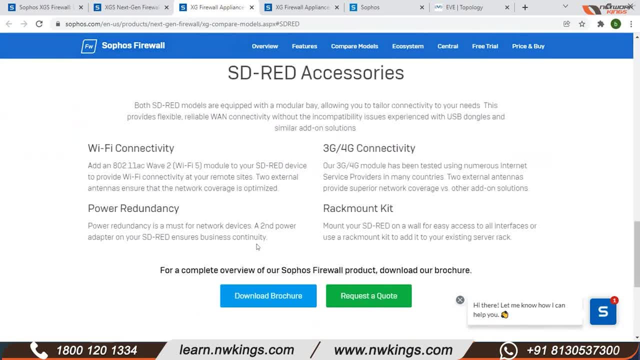 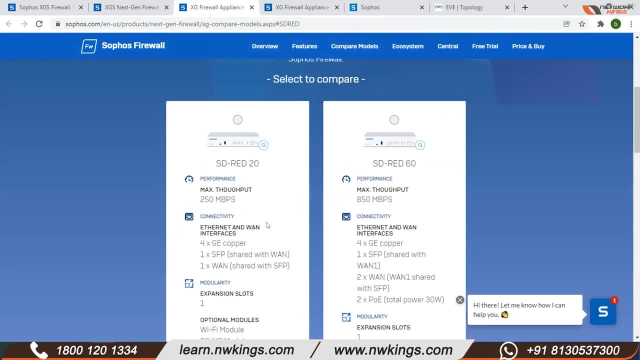 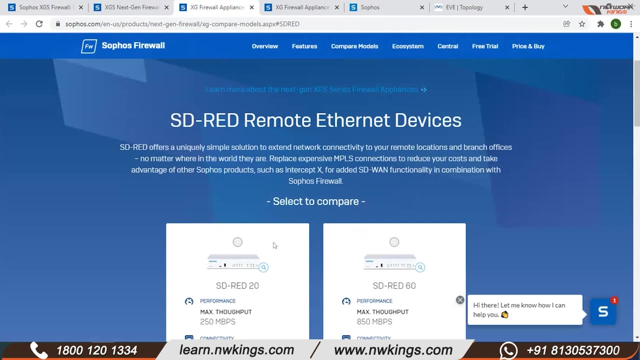 Okay, We will discuss more about that later on, Because we will generally concentrate on the surface firewall the most. Then, as soon as we configure the surface firewall, after that we will definitely if there is any wireless access point or endpoints or we have to do zero security. 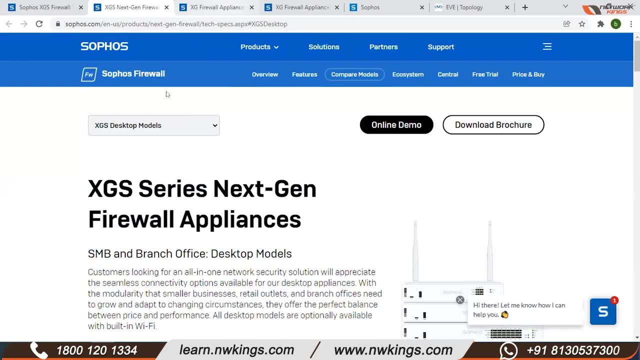 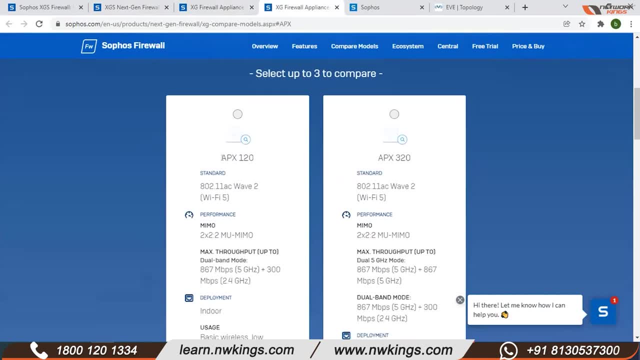 then definitely, we will do that one by one. We will do that one by one. Okay, So these are also the APs of the software here. So you will get all the details of the software AP from here. We will go in-depth about this in the module. 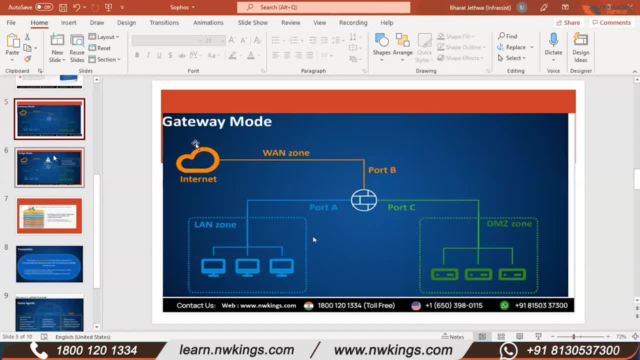 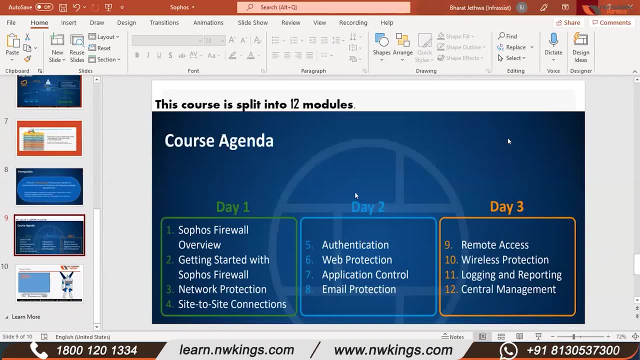 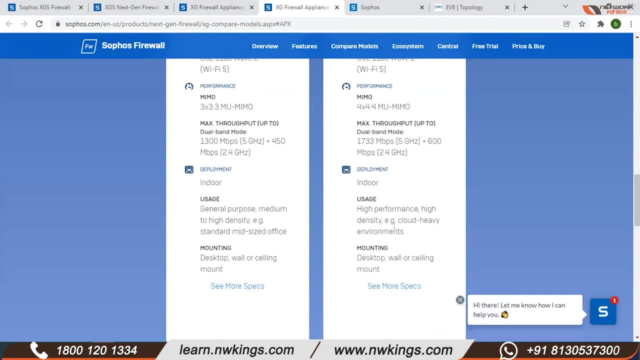 wireless protection. as I told you on the module, We will go to wireless protection. we will take more details in that. Okay, So these are the modules details. You can go through that. Definitely, we will raise all the questions for you right now. 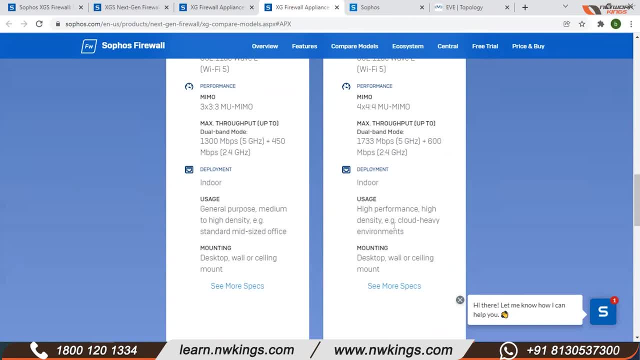 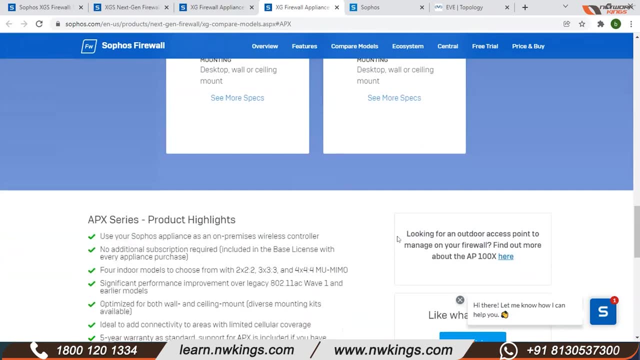 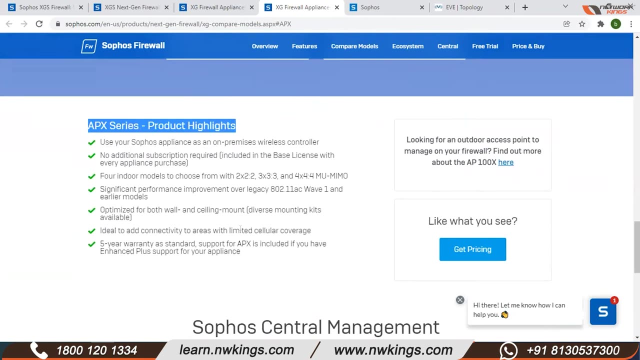 Definitely, at the end of the day, we will cover all the modules one by one. We will resolve all the queries of all the modules one by one. There is no issue. So the product, the APs of the software, the product highlights: 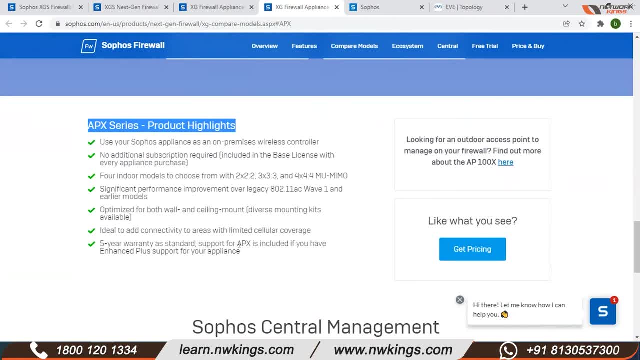 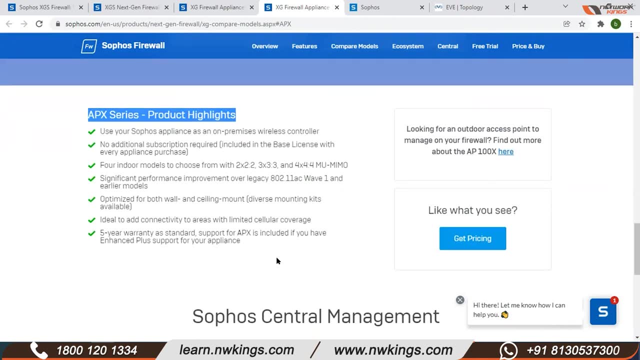 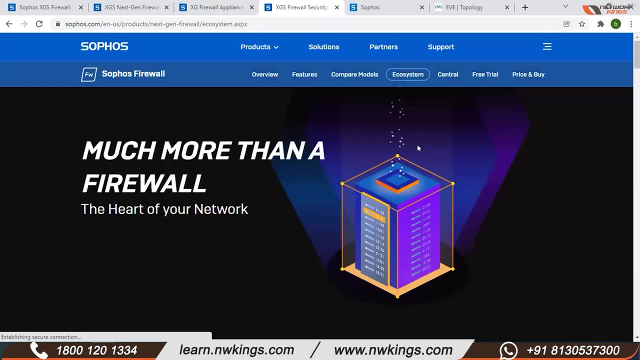 you will get from here, So it is quite easy. They have provided very good information here How we can deploy the software, the software ecosystem, here, Actually. Okay, So the software ecosystem, if we want to go in-depth about it. 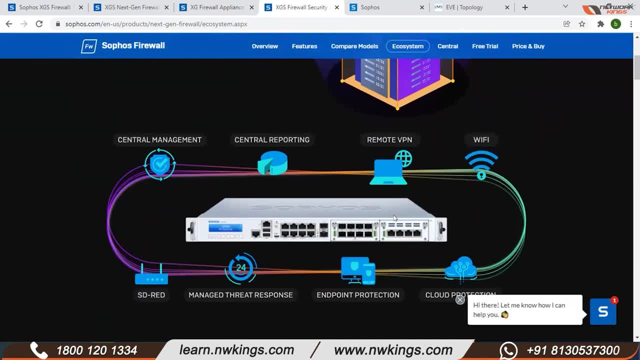 then we will see all the information from here As well, as we will cover all the modules that you see in the diagram. Similarly, it will be covered up. So how red is remote site is Wi-Fi is, end protections are? 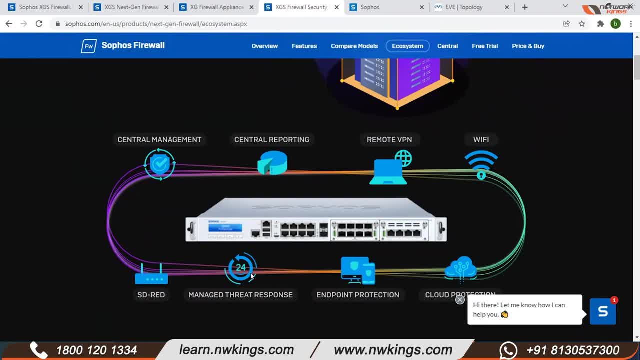 user species are. cloud applications are how to manage everything centrally, how to do thread correspondence, how to do reporting, See, everything is going to be covered up in the module, So we will go into its details as well, Along with 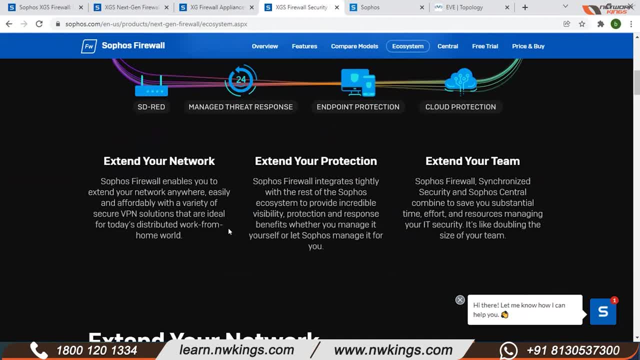 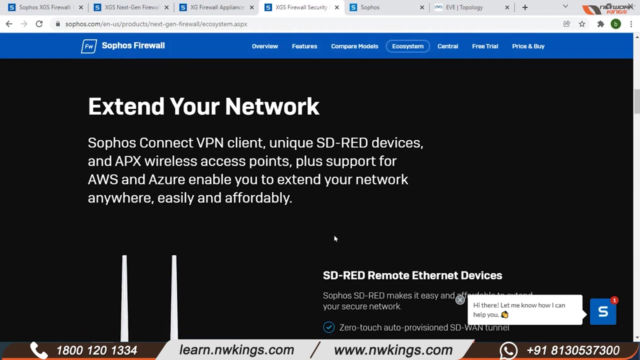 how we can protect ourselves from our software firewall, So how we can reduce the workload of our team With the help of Synchronized Security and Sophos Central, with Sophos XG Firewall. So here how we can. if there is any new project. 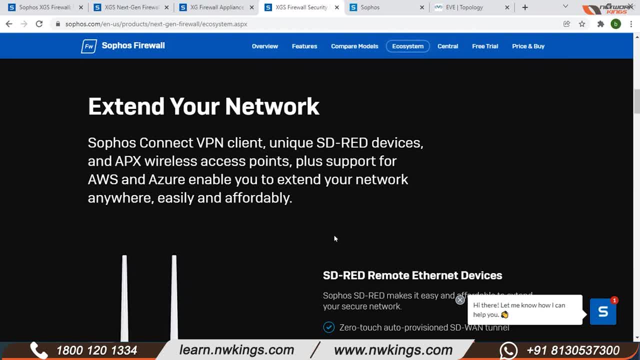 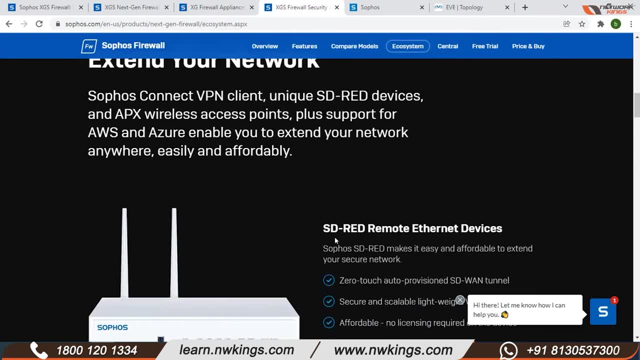 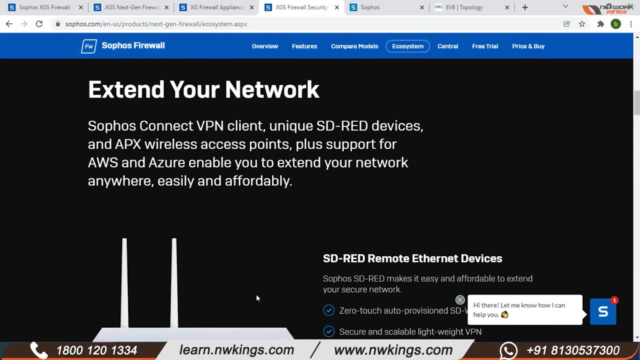 for example, how to deploy it. So here we can get all the details which will come into the ecosystem of Sophos For the best protection, of course, is Okay. So here about red, it is also shown about Sophos API. 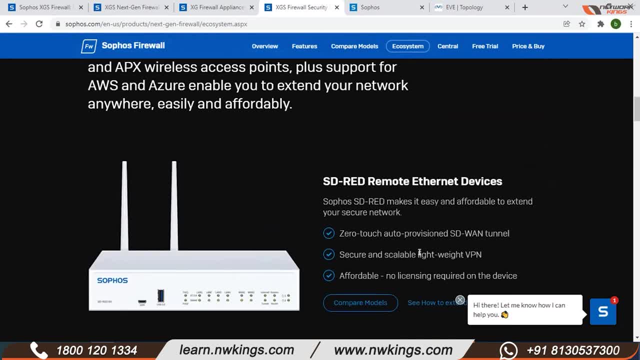 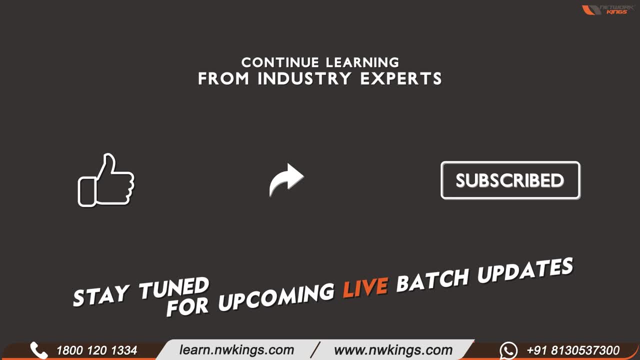 how we can provision it. Hi, you are watching the recording from one of our live sessions. Hit like share and subscribe for more future updates From: with the help of the Sophos Central and Sophos Firewall, how we can connect VPN. 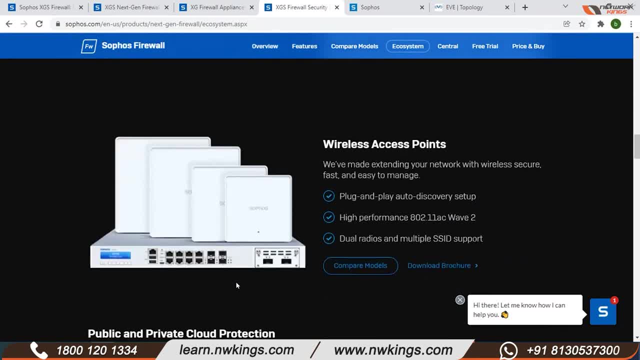 How we can make our network wireless, Just plug and play. So if there is any such scenario where there are Wi-Fi, there are laptops, there are 10-15 users and we have to protect them from Sophos, then definitely we can do that too. 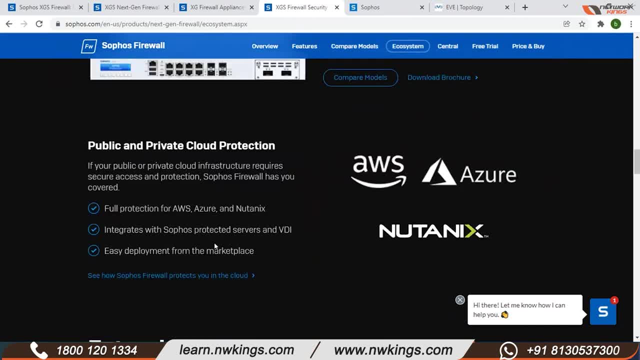 Of course we can also secure it in the cloud. If there is any infrastructure in our cloud, then we can deploy Sophos Firewall there. then we can protect it from Sophos. So we can integrate Sophos Firewall and the VDI. 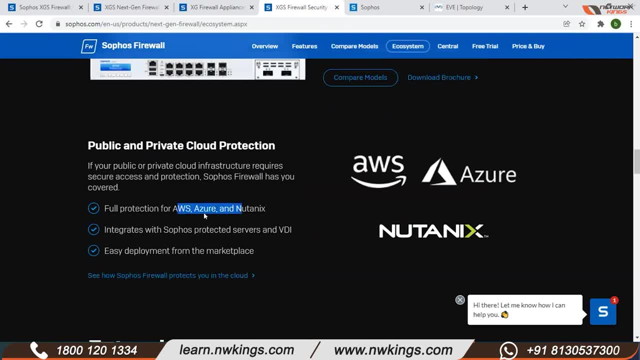 So support whoever is supporting. so Azure AWS, Nutanix supports everything, So all of its, let's say, for example, server, PC server, any application. we can protect it. Yes, We will also go about this. 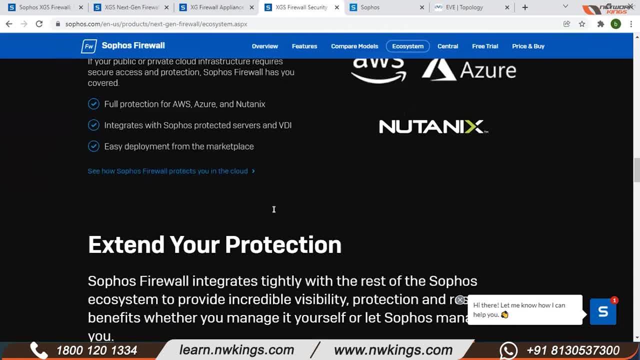 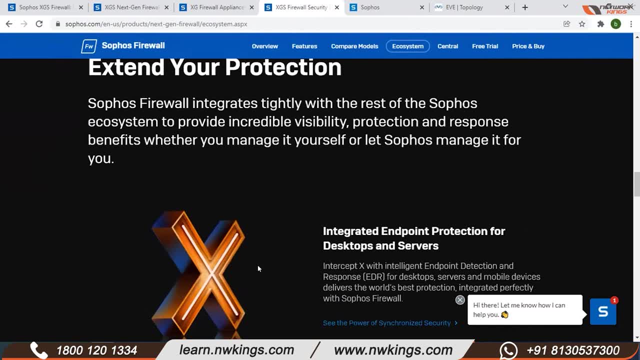 but for now we will concentrate on Sophos Firewall. So we will go in detail about Extend Your Protection, how the intercept that is the end point of Sophos, how it works with the Sophos XG Firewall and its ecosystem. 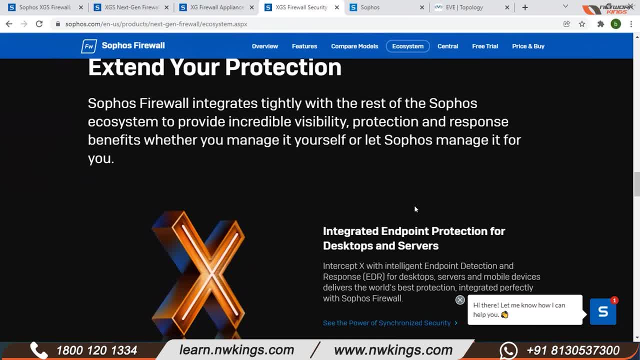 So we will also talk about this. next, Like, most of the modules of Sophos are running out, So after that we definitely. how can we extend Sophos from Intercept X And how can we integrate it And how does Synchronized Security? 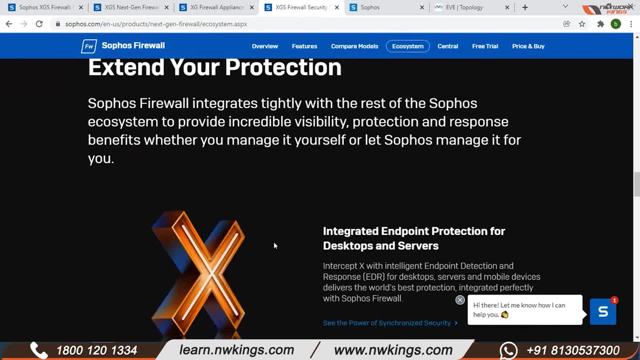 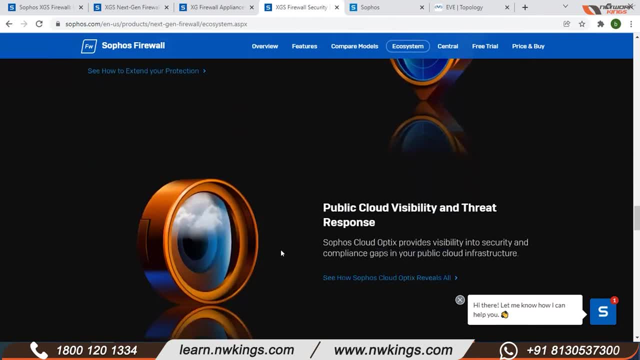 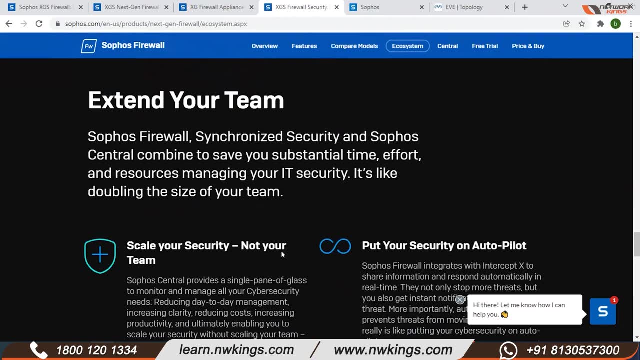 as I told you work. We will check it after covering all the modules In the same way. how can we manage? We will see that too. How can we put public visibility? We will see that too. How can we scale up our team? 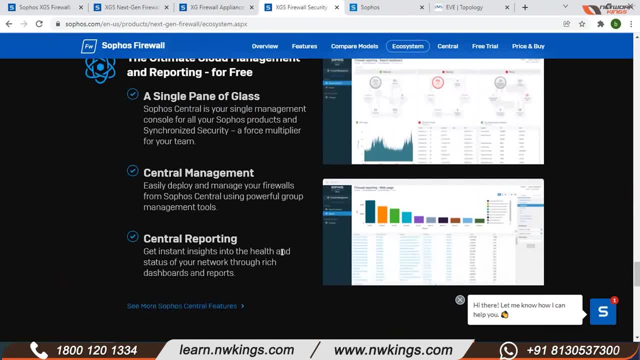 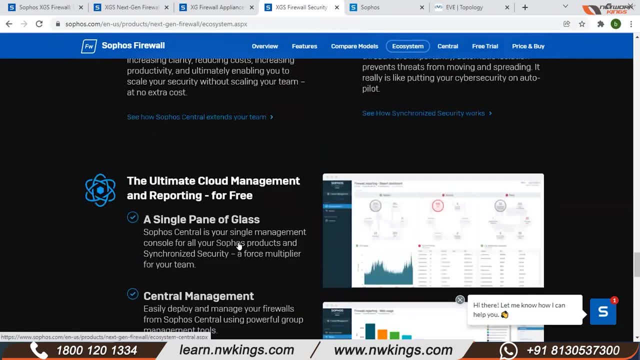 We will see that too. after Sophos XG Firewall. How to report? We will see that too. We will see that too. This part will be covered in the 12th module, This one here. Okay, So. 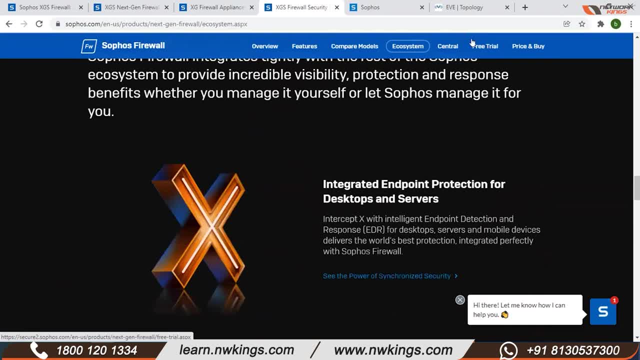 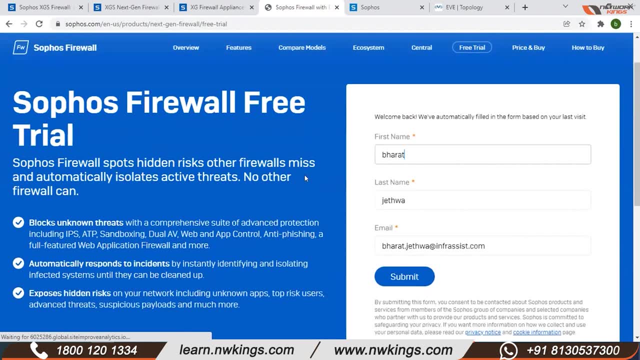 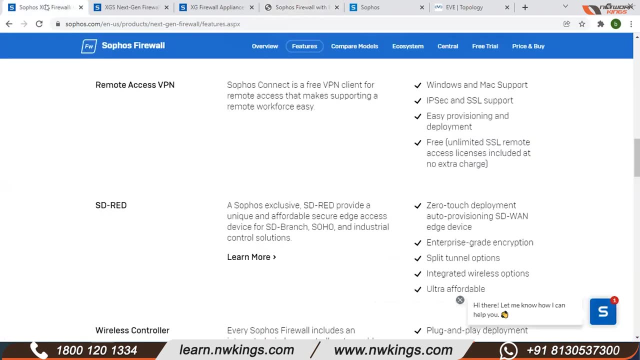 you can also use free trial. We will see about this later. Like, let me just click there. Here you have to fill the details So you will get all this information. We will go about this later. Let's have a look. 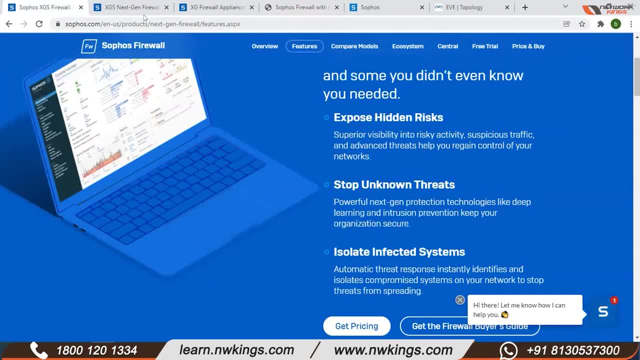 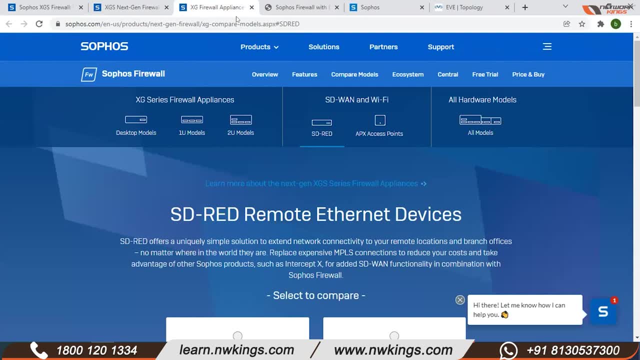 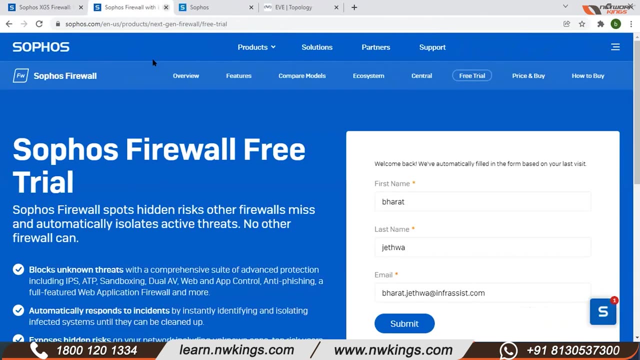 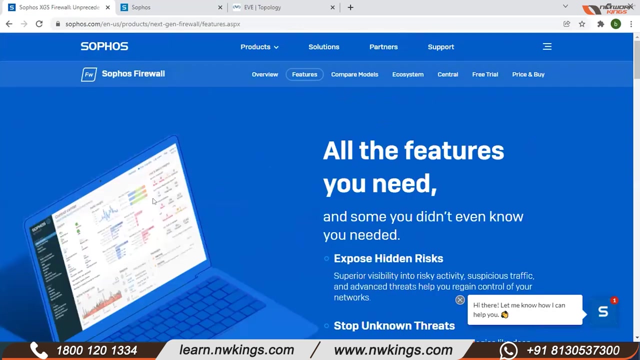 to the Sophos Firewall. So for now I have a Sophos Firewall for you. I will go through it GUI before we move with the modules. For now, what I have done is right now, if you have another screen. 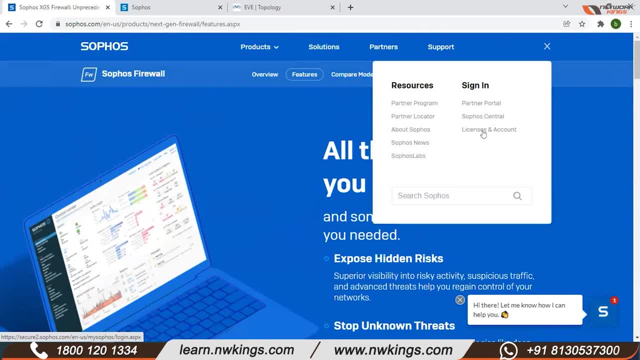 then you can go to Licensing and Account. There is a list of information available which we need to look through. Here I am just showing you. that is, you need to select the watchman and then enter your watchman name. 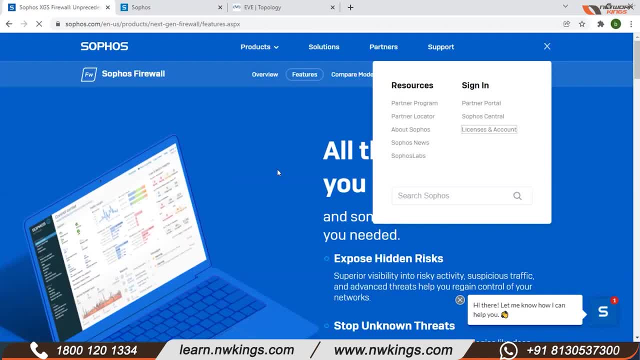 and then here you just need to click on your watchman. You will see that the watchman you choose for you goes for the watchman And here you have to select the watch so you can on the watchman. 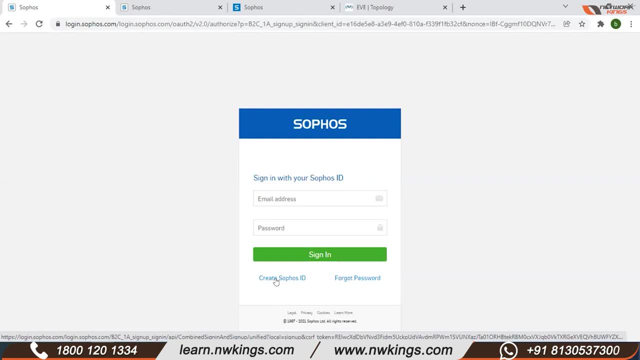 select the watchman. You can see that you have to select the watchman and then click on the watchman icon which is shown here Now you can, and then click on that Then. But if you want to do it now, then make an ID, like I have made one. I will use that for now. 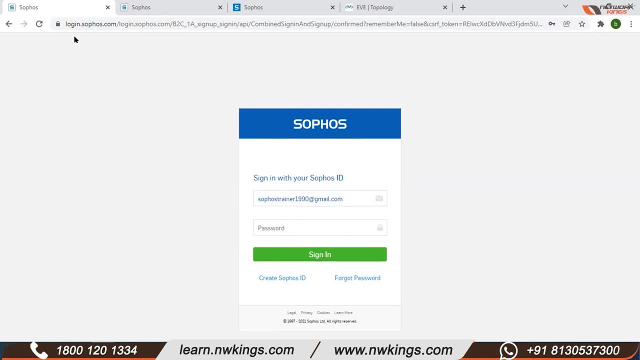 Once you create here, then you have to enter the email address. After entering the email address, you will get a verification code Like this way. let me just show it you up. It will not take much time. Okay, actually I have logged in here. 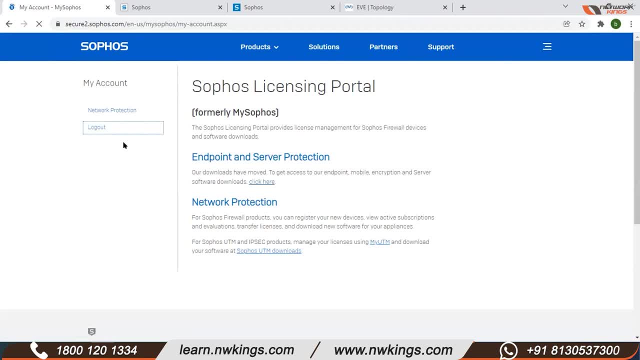 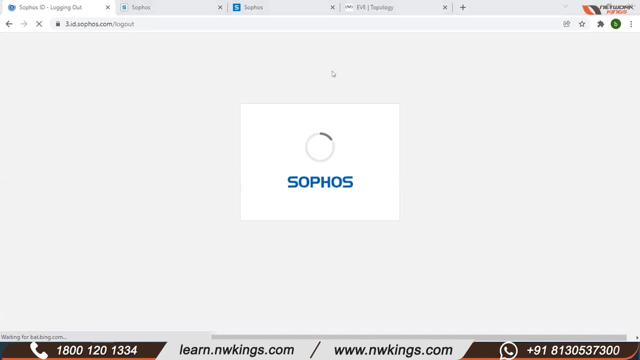 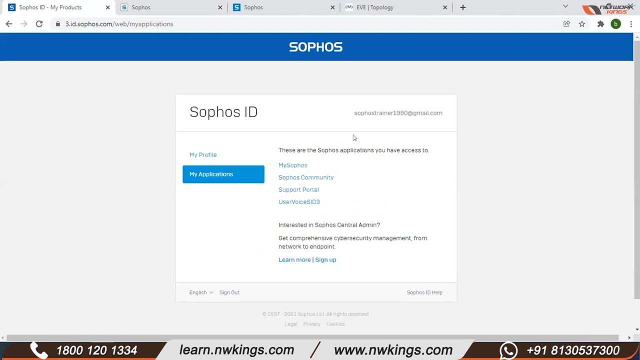 I will log out. Sorry guys, my internet is slow. Let me try again. Okay, so what have I done? for now, I have a VM in which I have installed the OVF file, So where did I download it from? As soon as you log in, 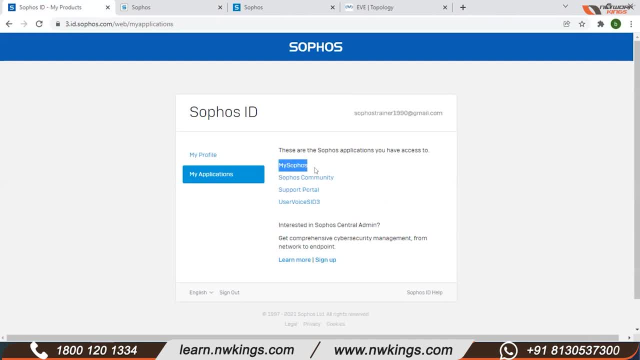 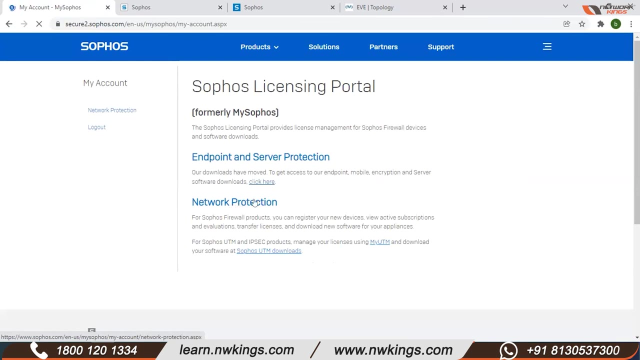 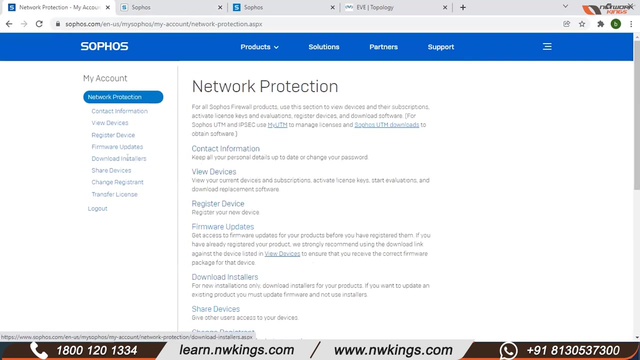 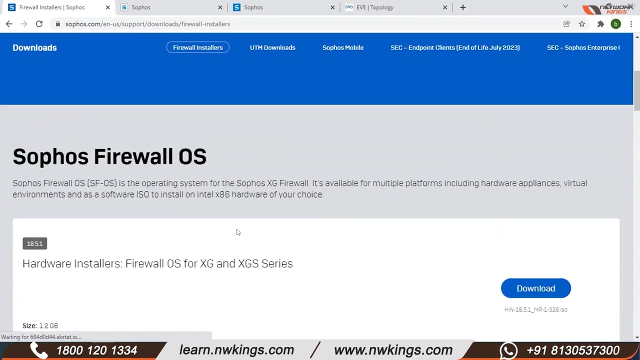 I have created a new account. Then you have to go to mysoforce. Just click there. You will go to network protection And you will click on download installer. You can click it from here. Okay, here you will get the OS of the Soforce firewall. 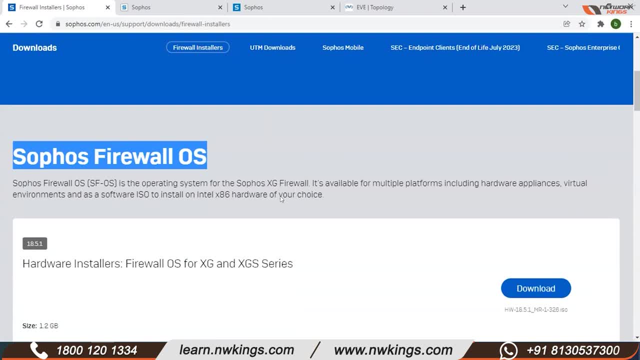 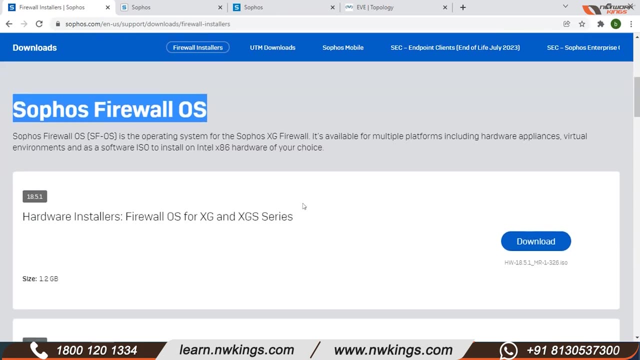 Now you will get this firewall for free for 30 days. That means you can use all its features for the next 30 days. So we will see the same thing in our lab: How we can actually deploy the Soforce firewall And how we can meet all the business needs one by one. 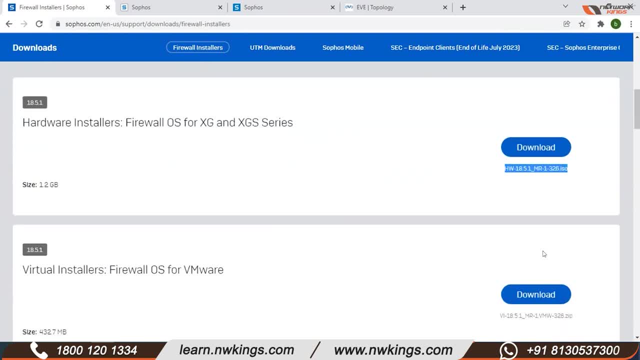 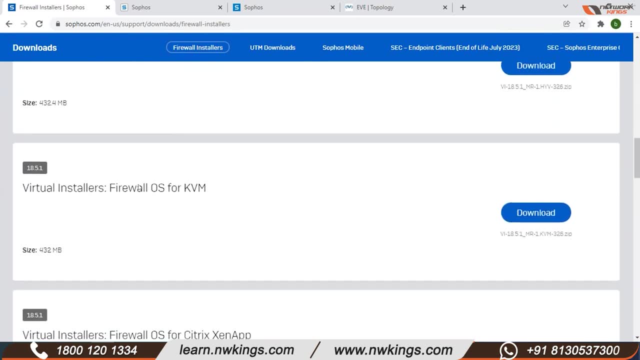 For example, if we want to deploy it on IOS or any hardware, then we will download it from here. For now, I can also deploy it in virtual VMWare, Of course, the Hyper-V. You can go to all the files here. 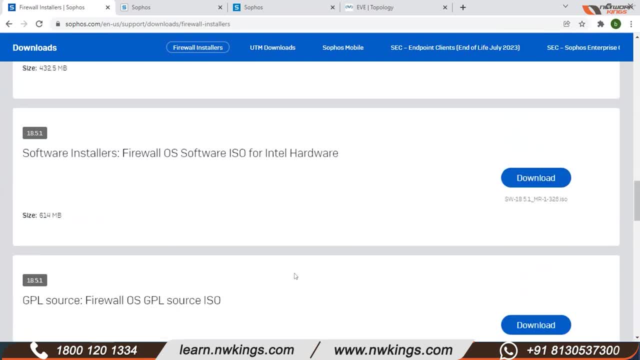 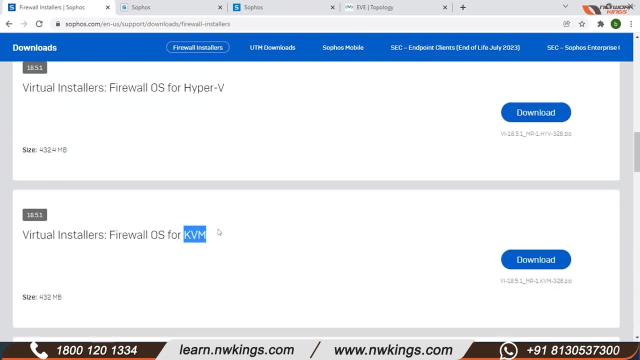 Whatever your environment is, you can download it from there. So if you have Intel hardware or Citrix, or if you have KVM or, let's say, for example, GNS3 or Hyper-V, you can download it from there. 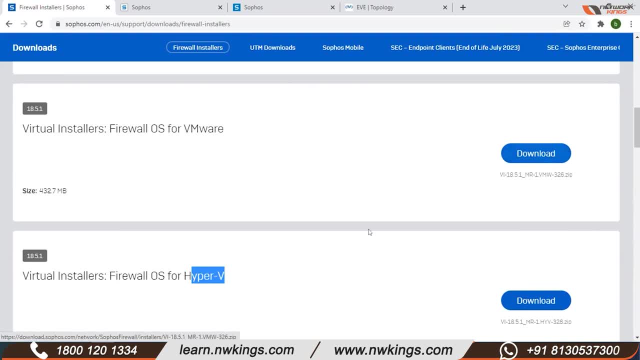 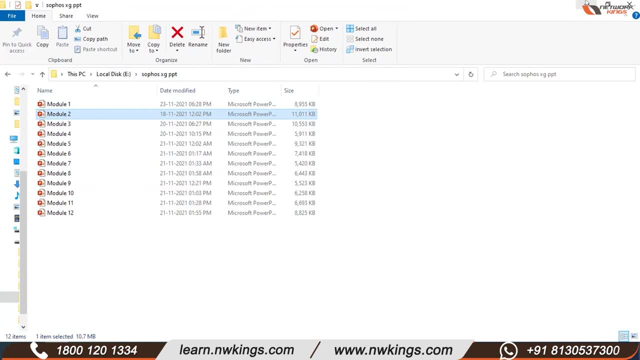 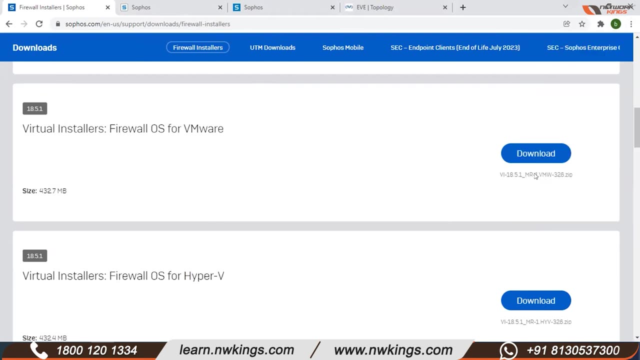 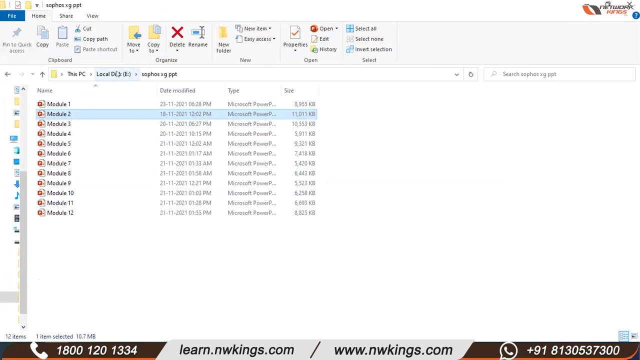 I have used VMWare as a template, So after downloading it in VMWare, you will get it here. Once this file is downloaded, you have to unzip it. After unzipping: just give me a moment. Okay, Okay, Okay. 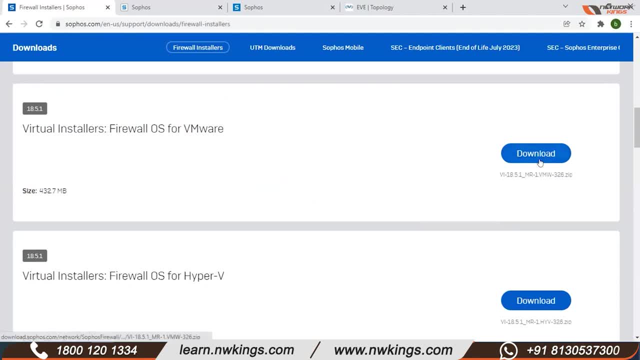 Okay, Okay, Okay, After unzipping. you have to unzip it, Then you will get all the files from there. Then, like VM, you have to install the OVA file. You have to run it. For now, I am telling you. 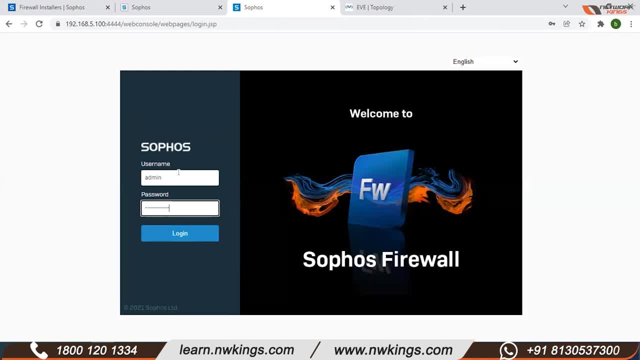 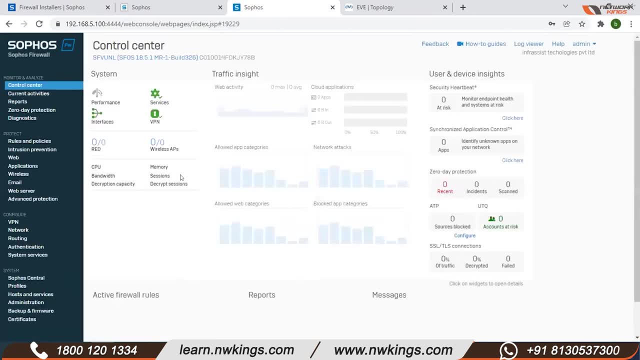 what I have installed on my system, Then next how to install it. If anyone has any issues, I will tell you how to do it on VM. If, unfortunately, someone is not installing the file, then definitely via remote or any other session. 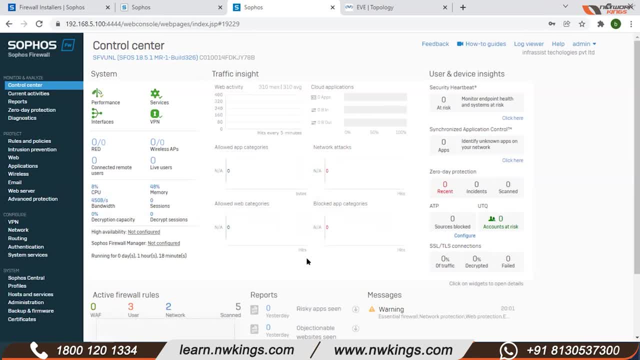 I will tell you how to install it. For now, I have my VM on my PC where I have installed SOPHOS XG firewall. So this is the whole GUI from where we can control everything. Generally, this is also called control central. 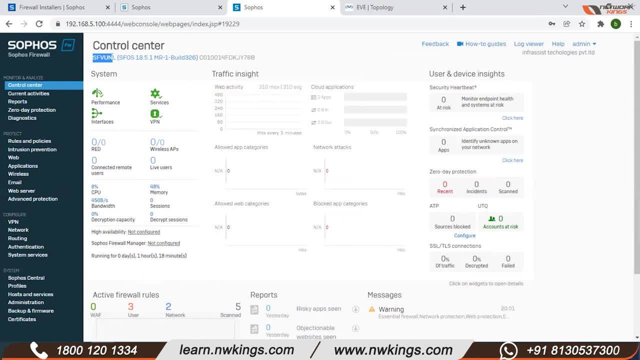 So the model of SOPHOS is shown here. For now I have not shown the model of the VM. It will be software-based, So you will get this information first. Then you will get the firmware current and its appliance key. 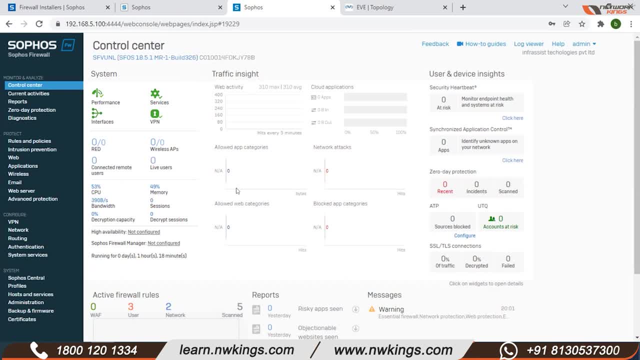 We will definitely go through it one by one, Like it will give you the whole insight about the status of SOPHOS XG firewall. So here you will get the whole system, the status of the system. Here you will get the traffic. insight. 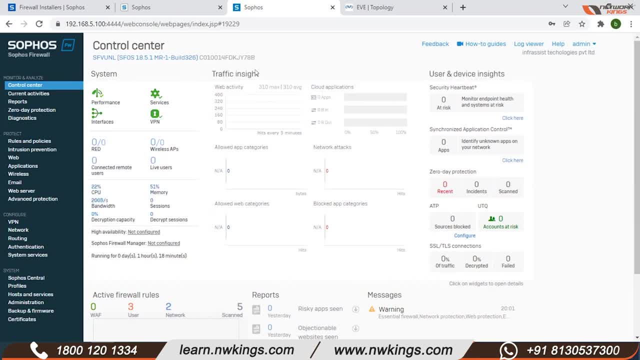 the traffic of your LAN. whatever traffic is going on, whatever interface is going on, you will get it from here. Then, user or identity: if you have any authentication- synchronized security is approachable, properly configured- then definitely we will get all the details from here. 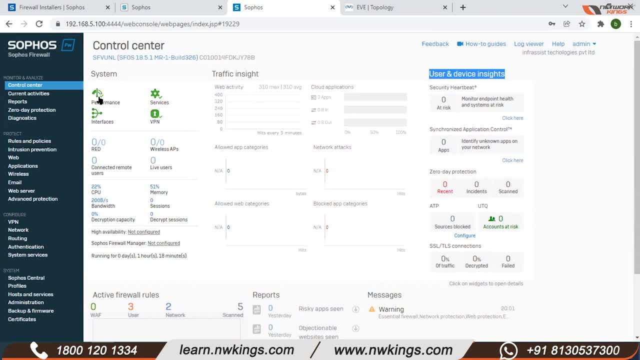 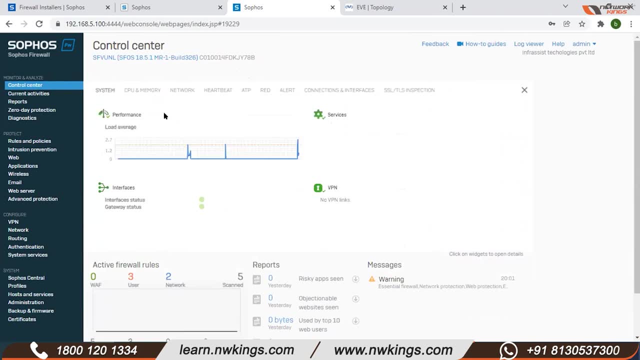 Now we will go through a little bit about this. Let's say, for example, if we just click on performance here for now, you will get the status of the system, that is, the firewall, How to balance the load. 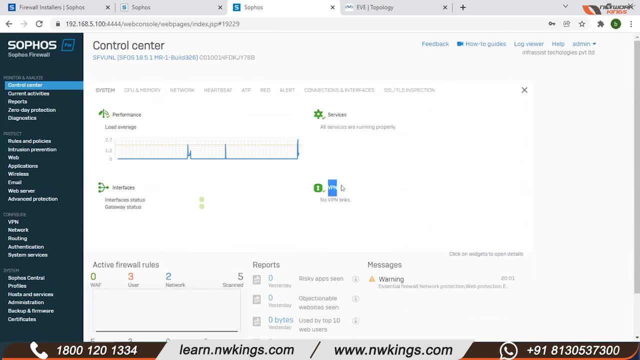 all the services are running. If the VPN is running, then the status of the VPN will be shown. For now, if any VPN is configured, then you will get all the information later when we will configure it. Whatever the gateway is the status of the interface. 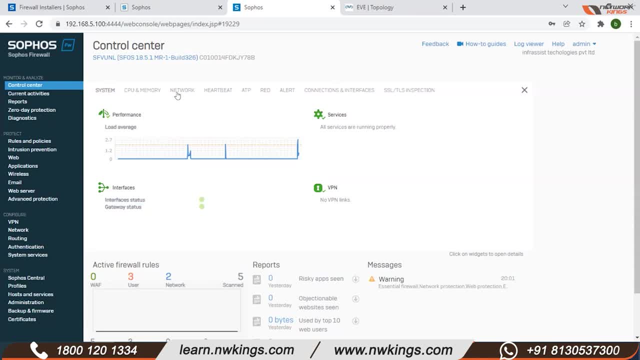 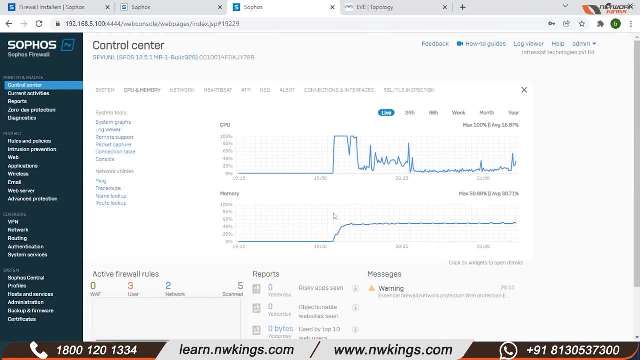 you will get here. You will also get the details of it here. If you need CPU memory details, then we will get it from here. This is just an overview. If we want to go very deep, then definitely we will go and see the reports. 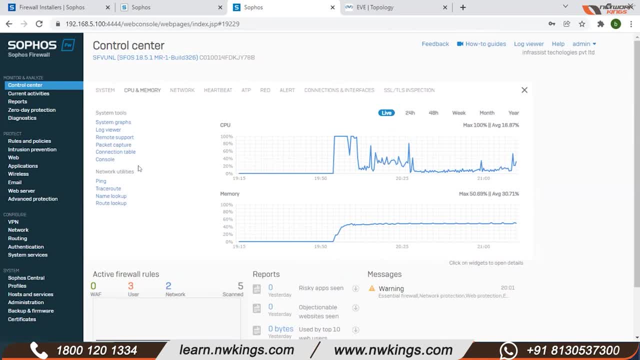 of this session. there. We navigate this one by one today so that whenever we do a lab then you should know at which point I am talking about. So here you will get memory and all this. Plus you have to diagnose these tools. 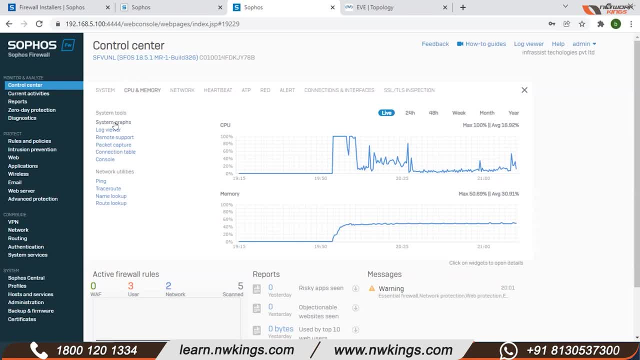 like system graph, how many users are there, how many bandwidth is there on the interface, and all the options will be available here. So how to see it? we can do it from here. There is a log viewer. you can see the logs here. 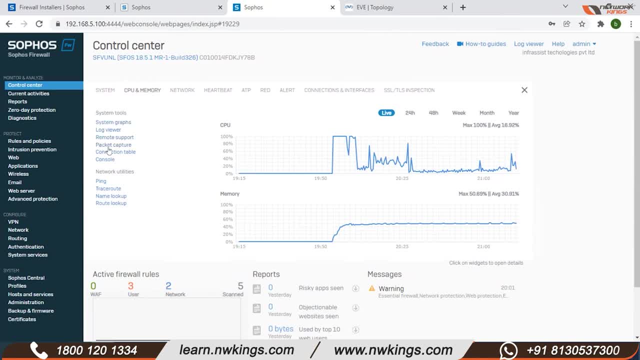 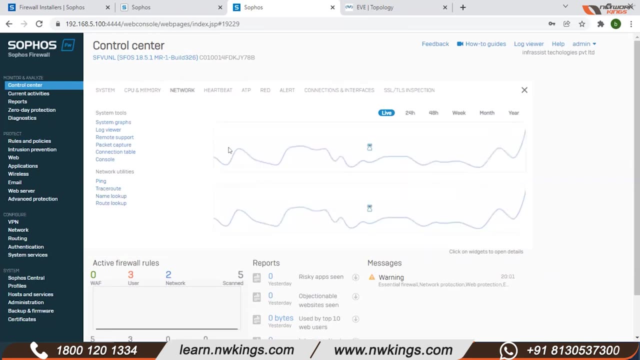 There is remote support. if you want to check the packet then we will see it. Console: we can get the console of the firewall, Then the utility of the network- ping, traceroute, nslookup, route lookup- if we want to do some troubleshooting. 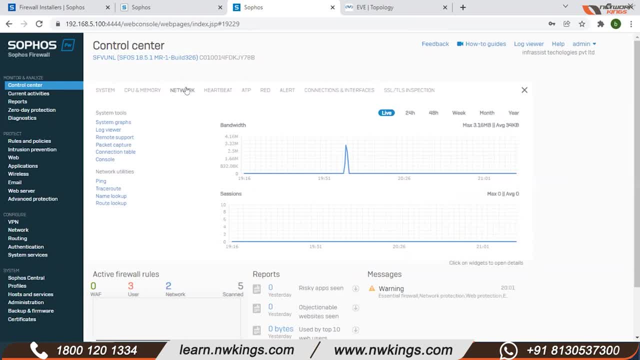 then we can use it from the firewall In the network. you will get networking like interface. Let me just log in there. Ok, you can see it here. Ok, we will have that system graph if we want to filter it out. 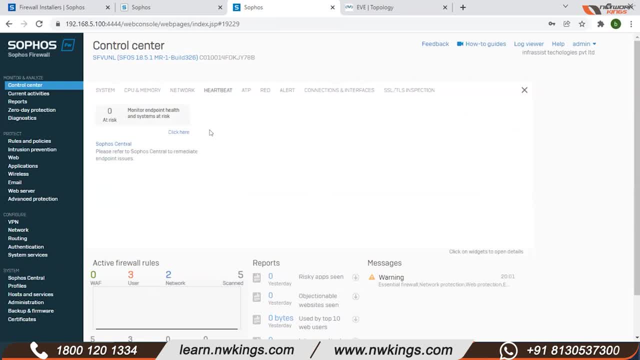 then it will come. I will tell you. Ok, like I told you, we need synchronous security. then this hardware feature comes into work. In this case, actually, we require, we need it on the user and the software central. the software firewall should be integrated. 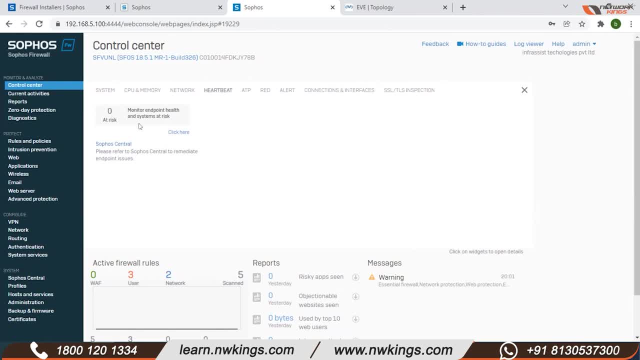 After that we can use this feature. So about this, there is already a cover-up in the module. If possible, I will also show you in the topology. Same way with the advanced red protection. So if some advanced reds are being detected. 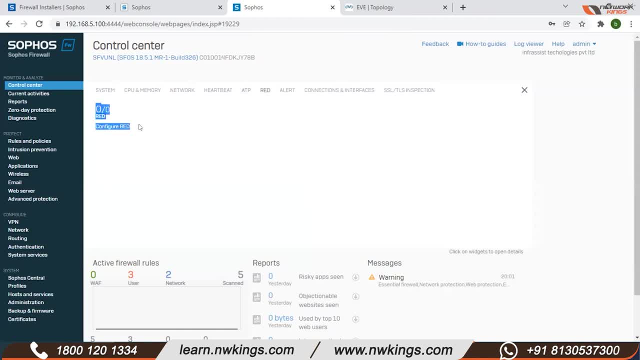 with the help of this configuration, then it will show up here. It will give insight How many reds are there, how many if one is down, if there are two, if one is down, then one will be shown here. 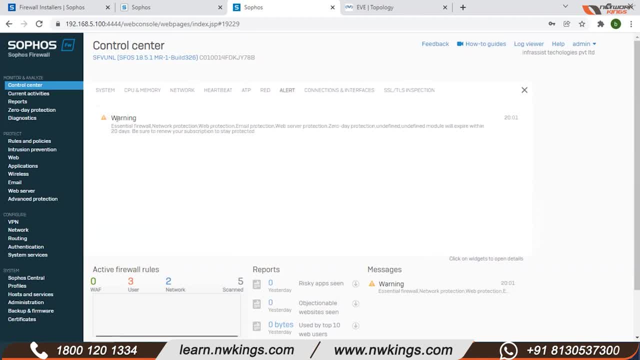 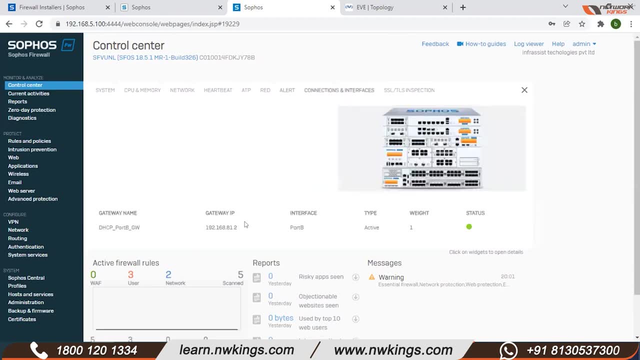 Alerts will be shown as if you have enabled any service which should not be as per the standards, or if the firmware is updated or anything, then that alert will be shown here. Connection and interface. so here all your gateways. 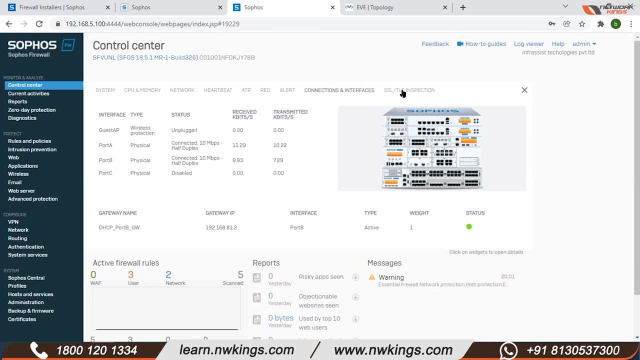 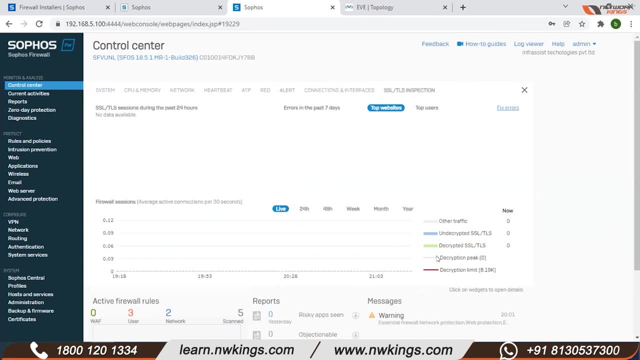 interface will be shown here. Lastly, the TLS and SSL inspection states. we can see from here About this. we will also see where we will use all these tools and where they can be useful. So we will see about this. 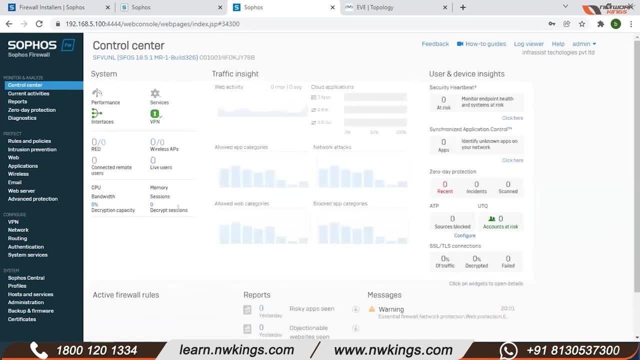 This was the insight system in the control center. So till here, let this get loaded up. Okay, High availability like HA. let's say, for example, you have 50 users and one firewall was deployed. first of all, 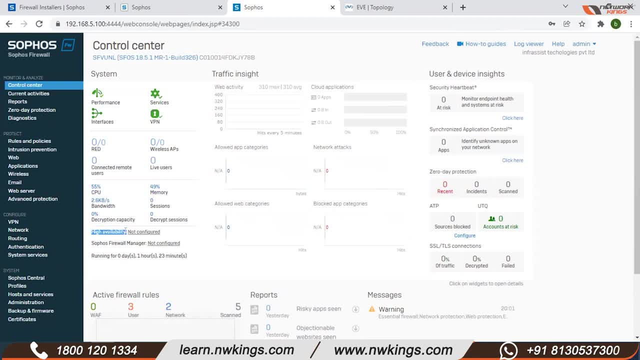 Now the traffic of the users, the traffic of the internet has to be load balanced. So if the users, as the complaint, can come, then in that case we can also configure high availability to meet the requirement, Or else 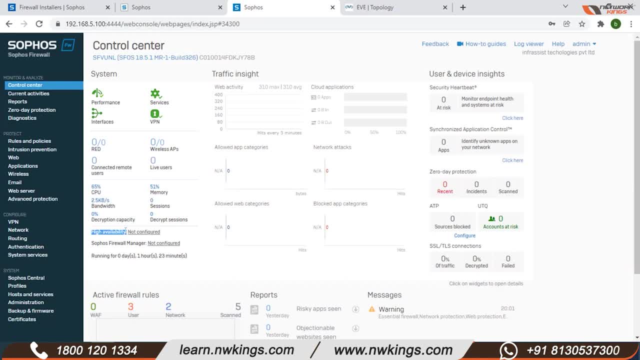 if the load is not coming like this, if there is a firewall down, if there is a failover- active, passive, passive, active- in that scenario, we will use high availability. There is also a cover-up in the module about high availability. 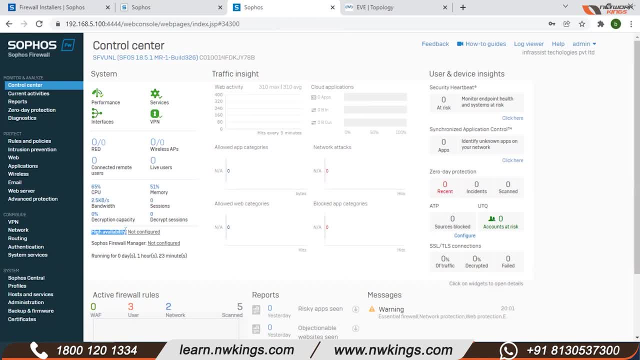 We will also go about this: how we configure it, why we configure it. we will also go about this. As I told you, for synchronous security, we can add the Sophos Manager, Not for the synchronous security. I am extremely sorry. 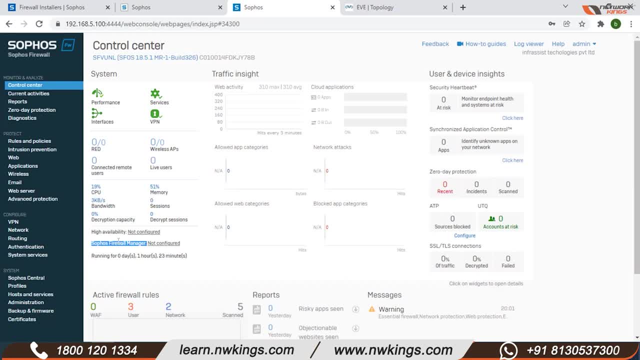 But if we have to manage any other firewall, like if we have to push the configuration, then we can use the Sophos Manager. You can integrate it here. The status of the firewall will tell you how long the firewall is up. Same way. 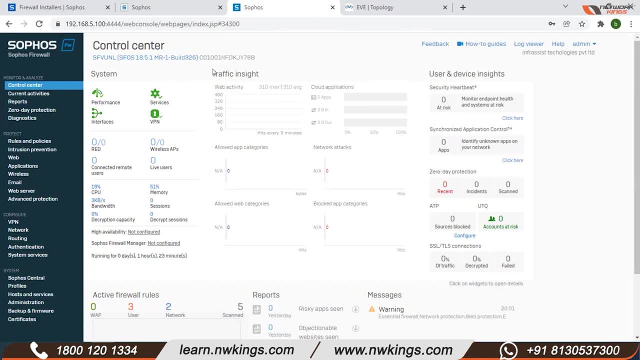 if this is the system. so we will go through in much more detail about these things: How we can install it, for example, how we can configure it and, in the future, if there is any issue, how we can troubleshoot it. 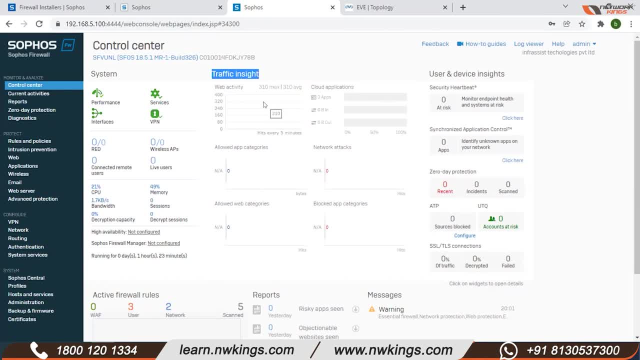 we will see that In Traffic Insight, all the application from the line side, the traffic of your browser, like web activities, will be shown. in short, If you have used a cloud application- Office 365,, for example, all the cloud applications. 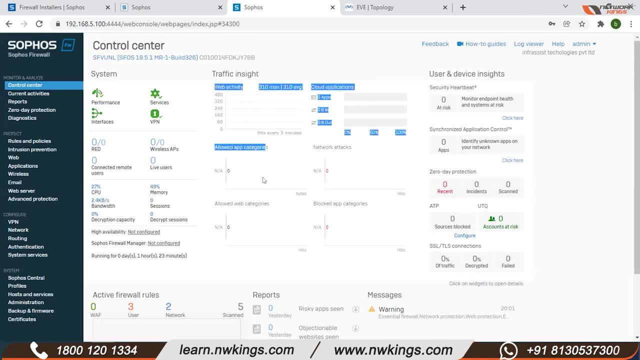 will be shown here in detail. If any application is allowed, then its highest, like streaming media, for example. all the categories will be shown here. If we have installed IPS policies and it has detected something, then its short summary we can see that: 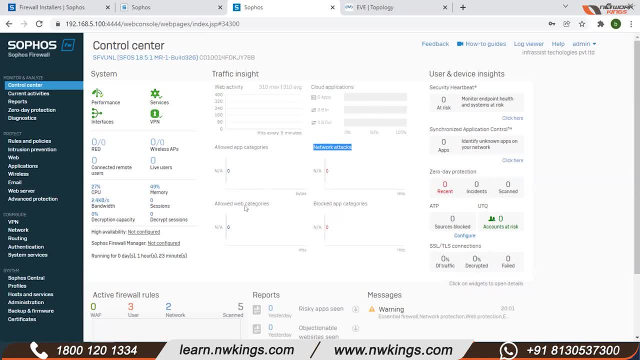 To go in detail, we will definitely see reports and logs in the future. Same way: if there are any allowed categories, we can see the insight from here. This was for the application, of course, and this was for the web. Same way. 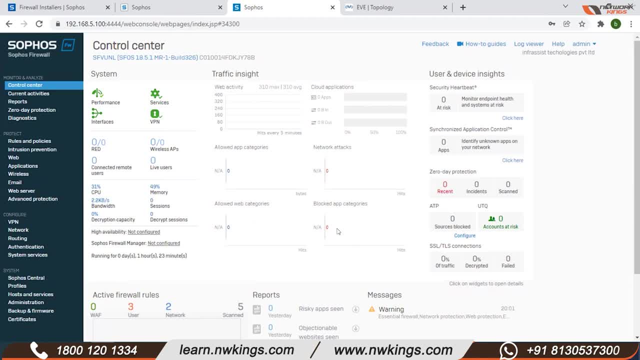 if we have blocked any application, let's say, for example, any chat applications, user device insight in this, as I told you, the security heartbeat feature, synchronized application control and zero protection, ATP Generally in this, the software firewall. 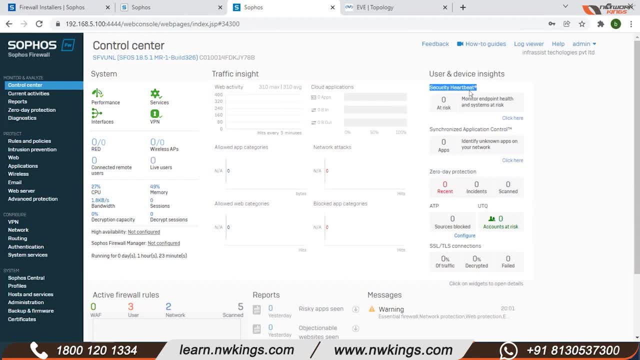 that is, the software ecosystem, should be completed to meet all these requirements. So what will it do? Security heartbeat, for example, in the next module, then software center and endpoints, these three. we can use these features together, the security heartbeat in it. 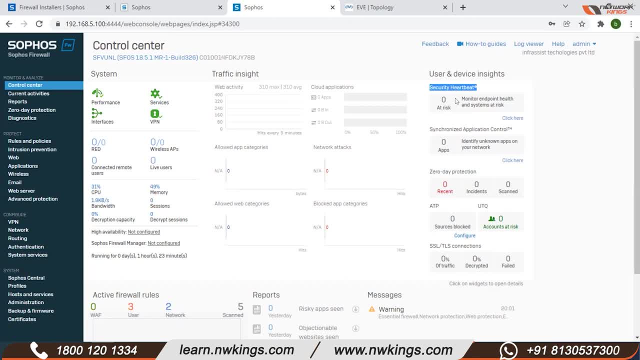 let's say, for example, any system that has been compromised. how does it isolate it? how does it tell it to infect it, its risk factor? you will get it all from here, Same way: application, as I told you. 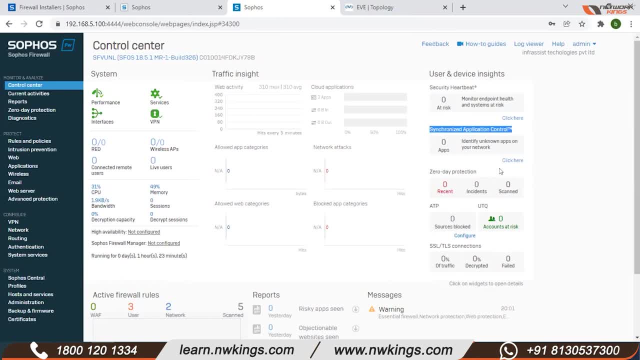 software endpoints, software center and firewall. if any user application is being installed running like this or installing, or there is such an application which is not in the database of the firewall, then it will be synchronized that particular application is running in the user's PC. 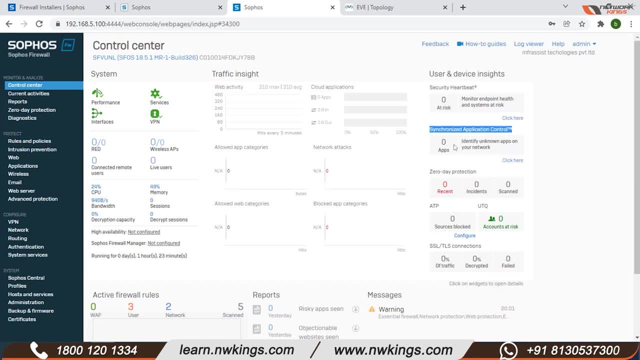 and we can categorize it further. About this. of course, the control center is definitely on the left side. all the types we will see one by one: Zero data protection feature, which I told you. we will see that too generally. 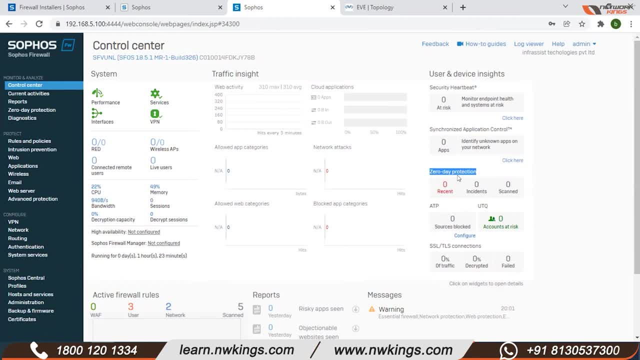 let's say, for example, there is an exe file which is allowed in the organization, then it will generally use the senstrom technology, so you will get the scan result of that file here. About this, we will definitely go how it works. 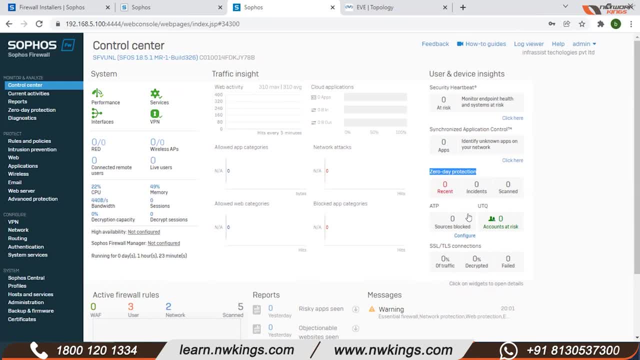 how it comes from the details of the file, how we have to allow or not allow, So generally as it is in the firewall, or we can allow or deny, then we can take that action. Same way with ADP and UTK. 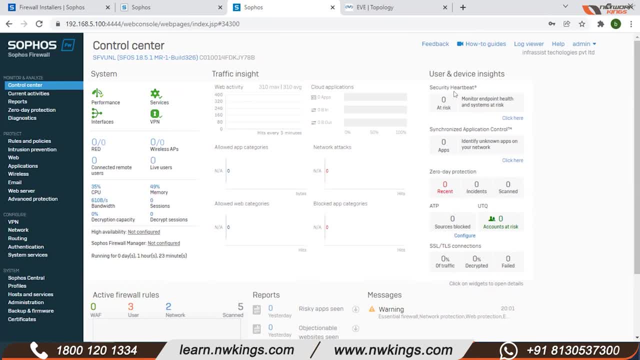 that is user threat quota, as I told you which user is at the highest risk. of course, it should be integrated with exe, So to meet this requirement. Same way, if we are scanning HTTPS through firewall, then we will get all the inside traffic. 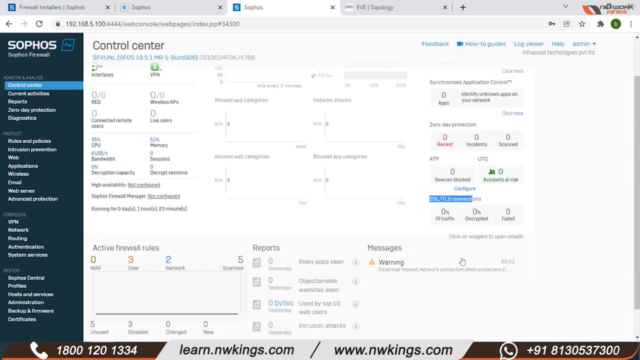 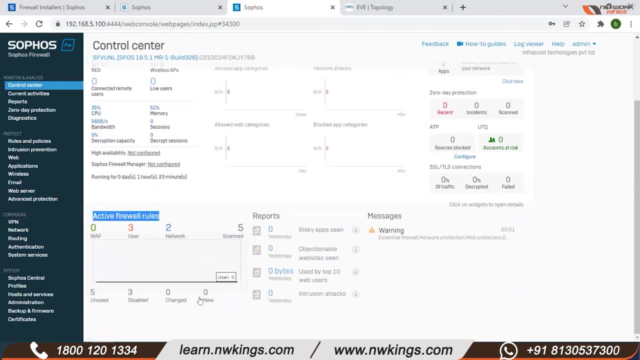 from here and we can deep dive in case of any troubleshoot is required. Okay, here how many WEFs- ie web application protection- you will get. For example, how many web servers you can protect behind the sofos. 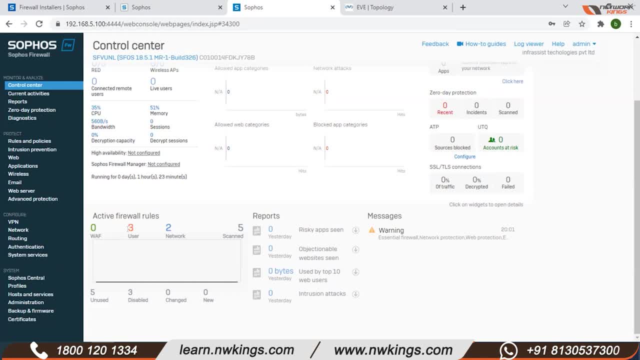 We will tell you the details here. Same way: how many users are there? For example, authentication is enabled And we have users, So we will tell you the details about this. Same way, how many users are there? disabled? 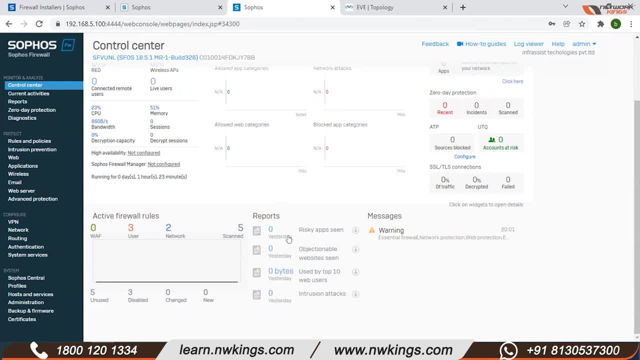 or any changes. Then there is a small report session which will show you yesterday's reports, like risk application scene, objectable website scene which we have put, policies And, finally, how many settings are enabled which are not feasible according to security. 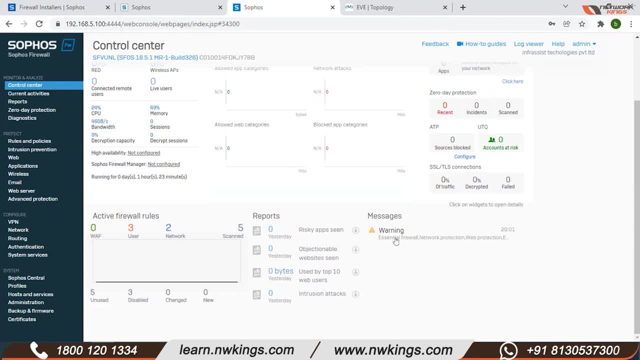 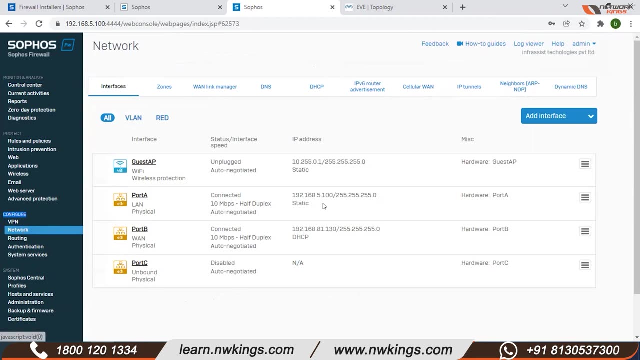 Then we can get those alerts and we can sort it out those things. Okay, So let's start from networking here. Sorry, network. So if we go to configure, then we can configure network here. Generally, port A: 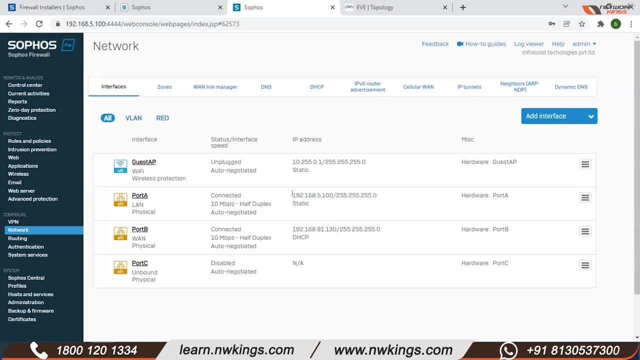 by default, its IP is 172.16.16.16.. Here I have changed it. You can also change it, no issue. But as we are unboxing, for example, if you want to access its GUI, then what you have to do is: 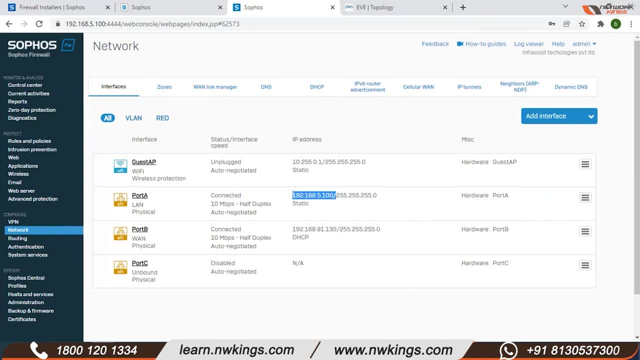 connect its firewall to port A. connect it to any laptop, it will run DSCP already. If you don't get the IP, then manually: 172.16.16.16.16.. for example, with slash 24 subnet mask configured gateway 16.16.16.16. 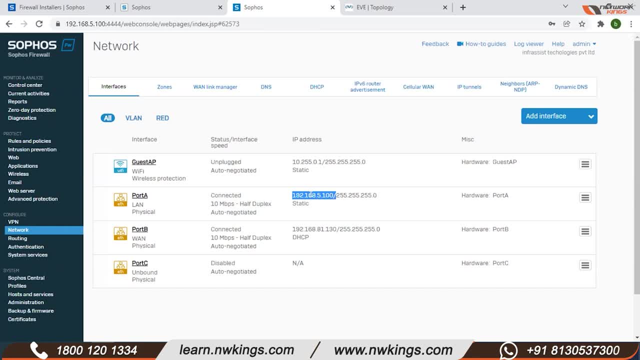 meaning 172, sorry, 172.16.16.16.. By configuring gateway, we can access it. Regarding this, when we configure in our network topology, then we are going to do the same thing. how we will access firewall first. 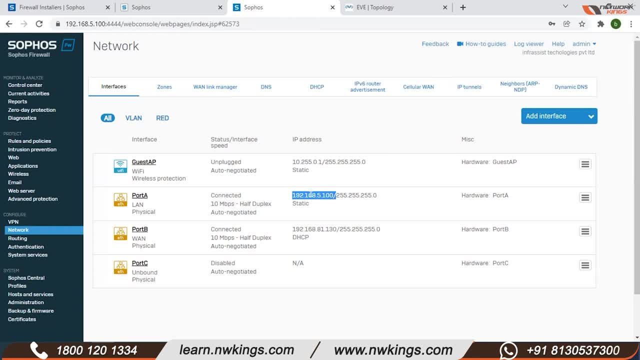 how we will configure interface, how we will configure zones, how we will create users locally or if there is any other AD server, for example, how we will import users, how we will enable authentication, how we will apply web filter, application filter policies. 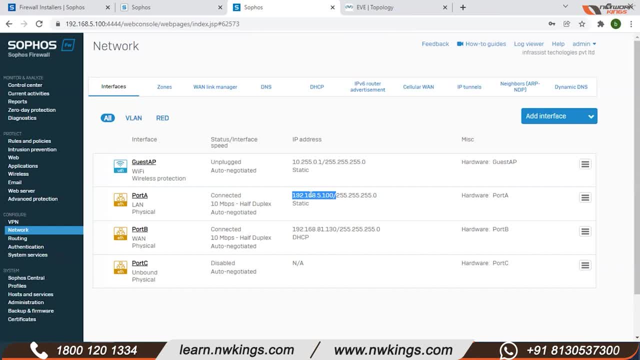 application for the policies? yes, of course, as well as with the IPS policies. if there is any port forwarding or if there is web protection, how we will configure it. that too we will go further and see on the rules. then we will also. 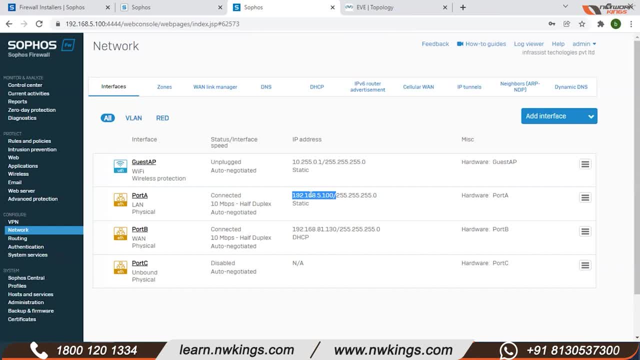 check how to configure email protection. that, too, we will come now on email protection wireless. yes, of course wireless, which is also given here. for example, that is only for Sofos API. no third party will be able to use it. 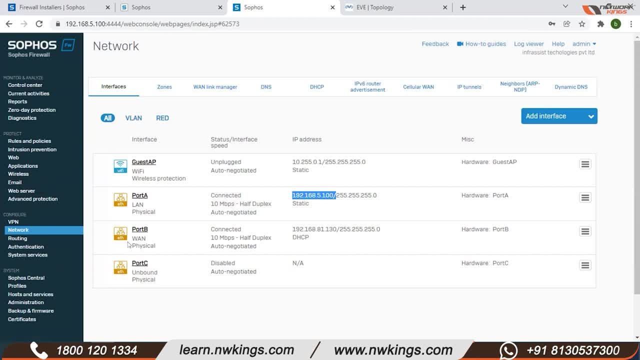 so we will also see those features. so here if we are on the network, then we can configure the interface. here we can configure zones. like if we want to do DMZ zone, then we have to select DMZ, then we can give IP. 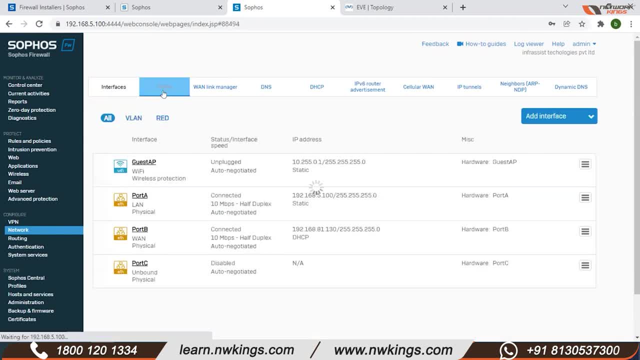 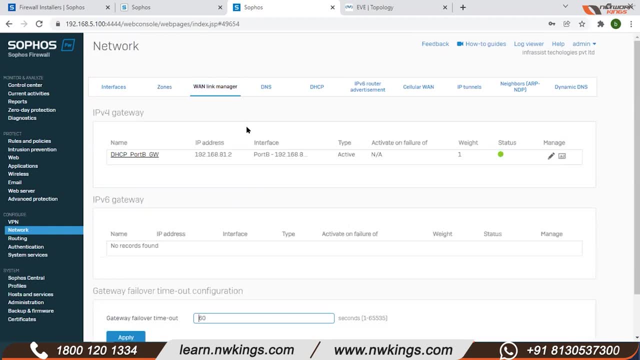 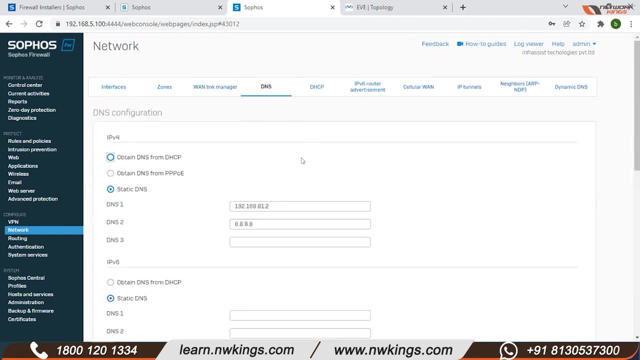 ok, so here we in the modules. everything will be covered up. what are the zones? we will go in detail when manager. if we have multiple ISPs, then how can we manage DNS? of course, how can we configure DNS in Sofos API. 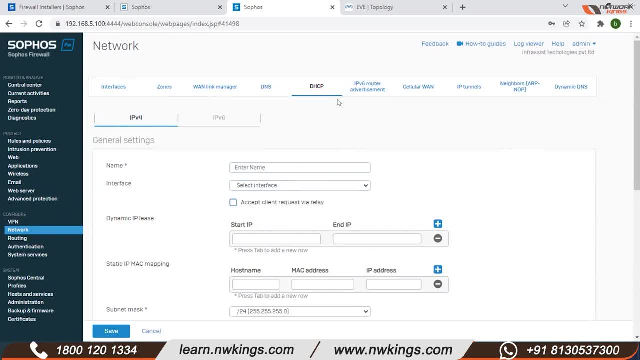 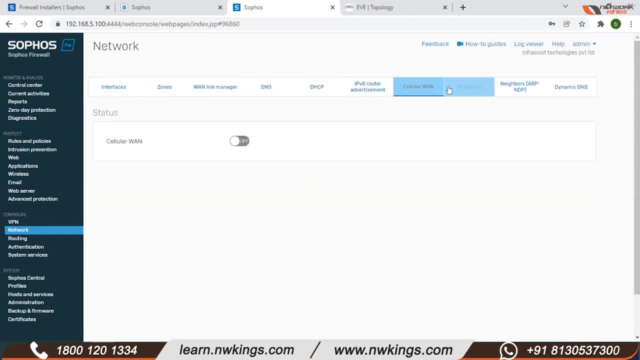 along with DSCP on the interface, then you can select your interface and enable DSCP here. ok, along with IPv6 address management cellular. when we will see how to configure the IP tunnel, we will see that how the neighboring ARP is generated. 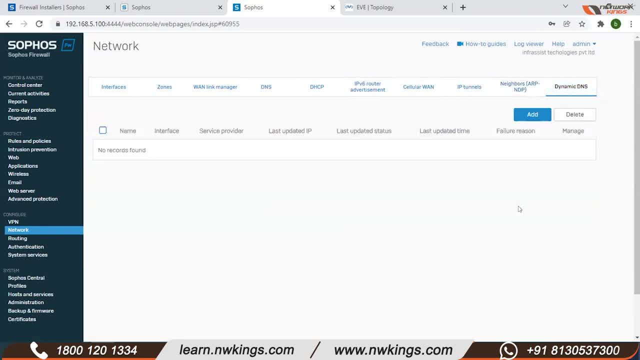 we will cover it in detail in the module with the dynamic DNS. we will also configure this if we want to access the firewall from outside with the hostname. ok, now let's go to the current activities. after the networking, let's move from top to bottom. 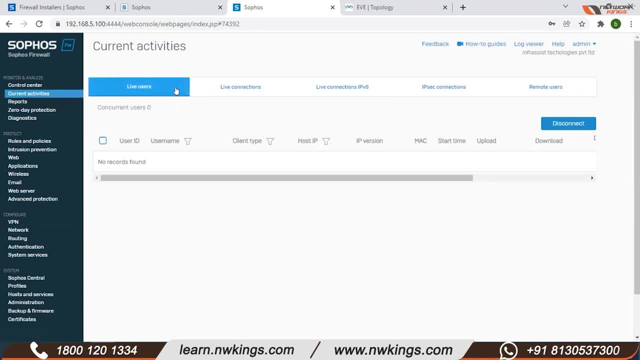 here. so in the current activities you will get these types: live user, live connections, connection with IPv6, IPv6 connections and remote users in live connections, the live users, for example. here all the users will be authenticated. 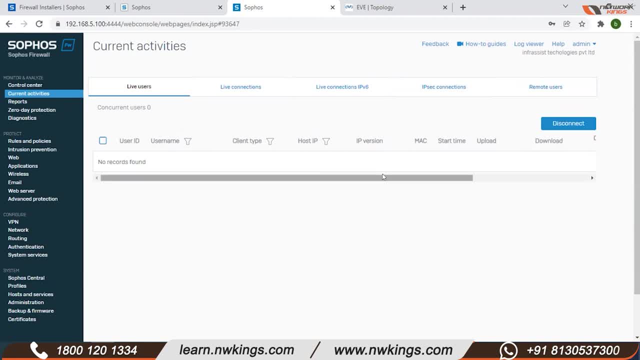 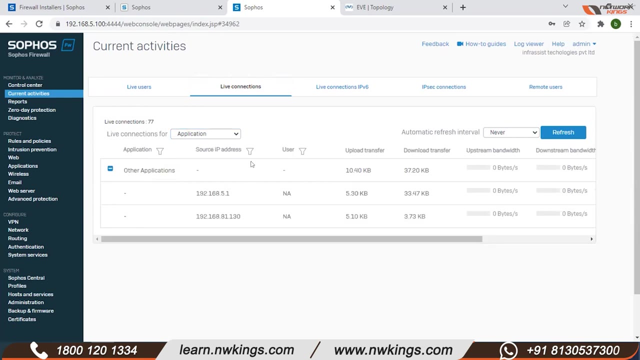 that is, which method you will get all the details here. which authentication method they are logged in: live connections: the application username, source, IP, the connection slide. like the firewall, we can see everything from here. we will also go into detail about this. 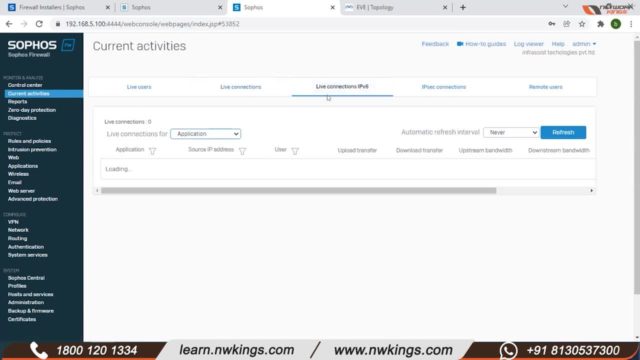 how it maintains live connections along with this IPv4,. same way we will see IPv6, if there is any error in IPv6, then we can see IPv6 connections, like we have connected any head office, branch offices or there is a site. 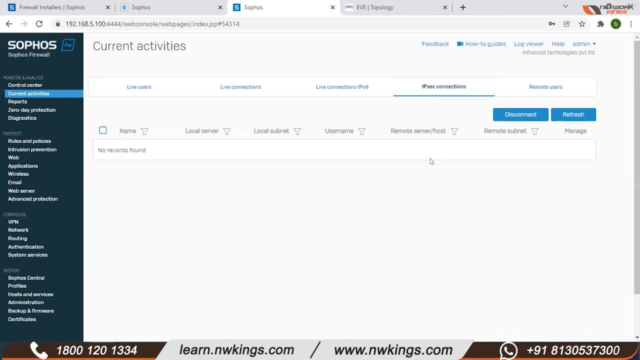 where the third vendor is also connected, then we will get all the details from here. in remote users, you will get all the details like the users are connected to SSL VPN or the users are connected to SSL VPN or IPv6 VPN. 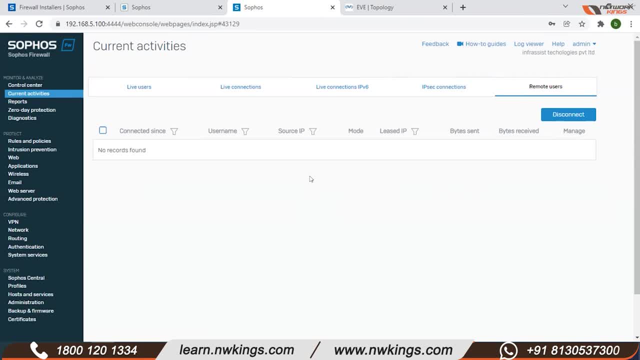 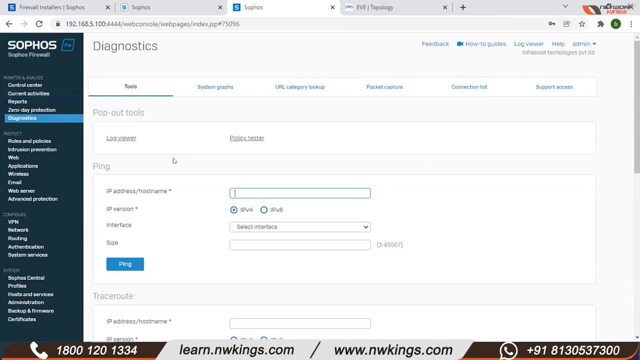 of course connected or the software is connected remotely, then all the details of that you will get in current activities. after control center, before clicking on reports I will go to diagnosis. so in diagnosis if you have some troubleshooting then we will use it. 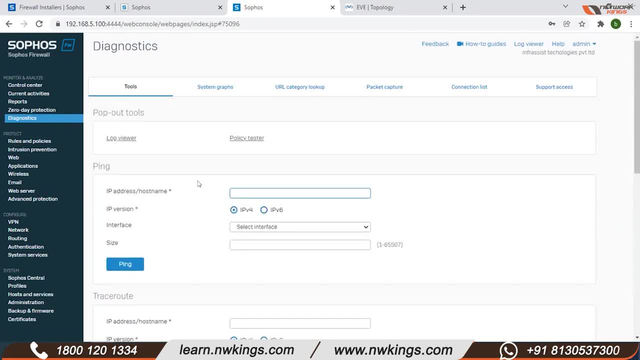 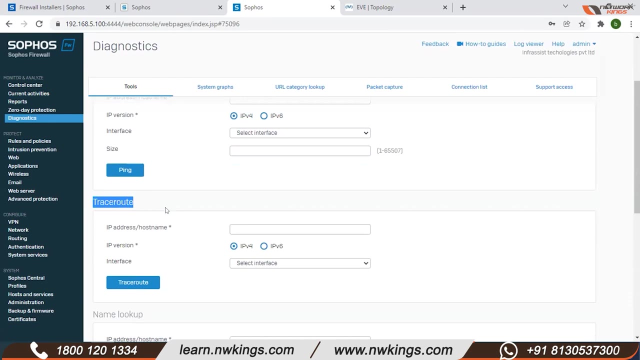 we will use it in the lab because in the future we will see how we can use it like ping to check whether the host is reachable or not. interface from where it is connected. press out. we will do NS lookup. 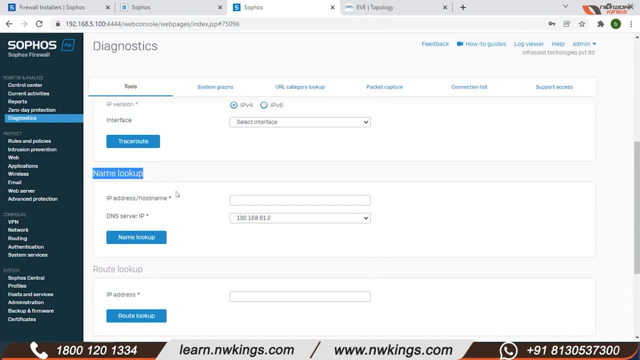 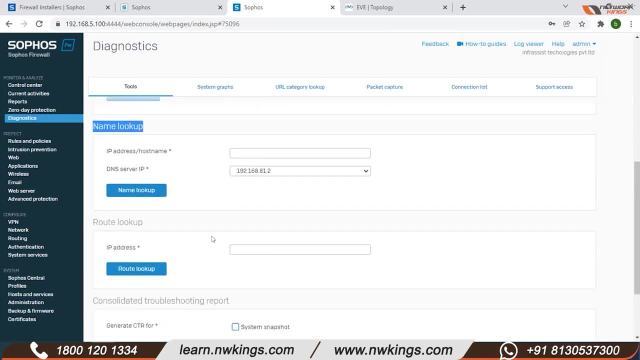 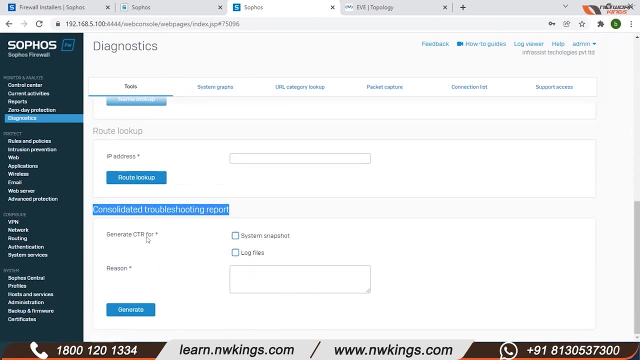 we will lookup and discuss how all these tools in which scenarios we will use and take its output- we will also take route lookup- and, lastly, the consolidated troubleshooting report, CRT, for example. let's say, for example, some policy is created. 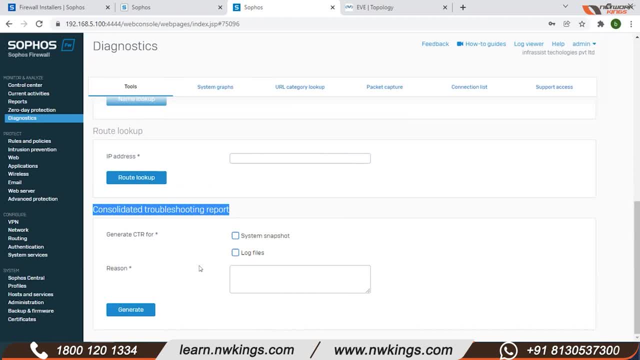 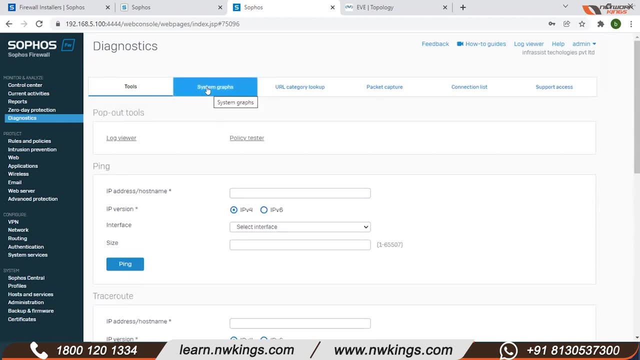 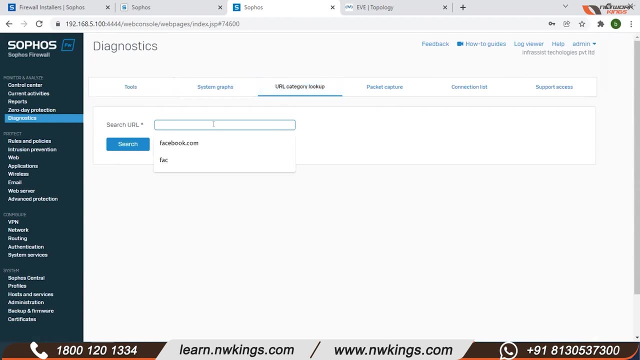 but it is not getting affected. then we will generate these firewall logs, we will support it further. we will see how to do it. before clicking on system graph, I click on URL lookup. so in diagnosis, in URL lookup, let's say: 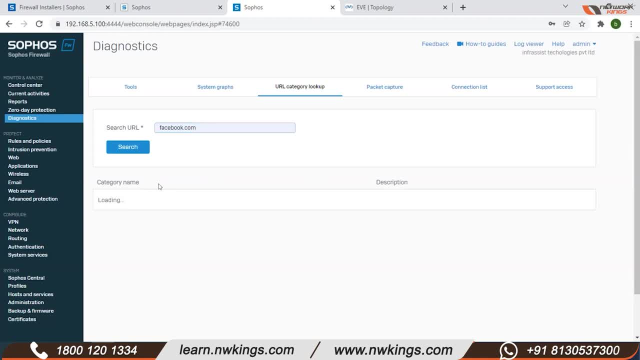 I have written facebookcom, then you will get its category here. so if there is any uncategorized, then you can categorize it. if it is categorized, for example, then you will get its status. let me try sofoscom. 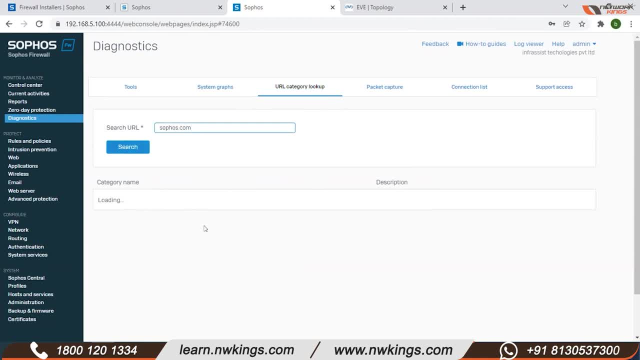 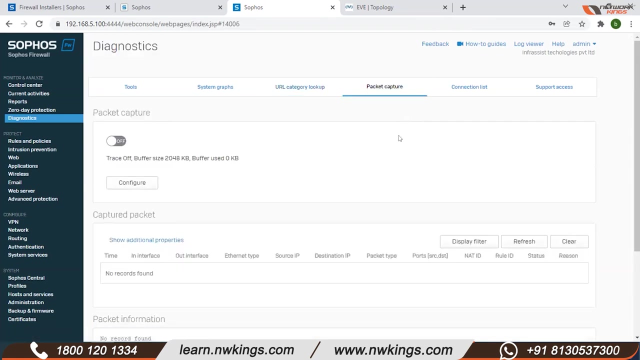 what it says: ok, software, ok. ok, I think the name of sofos. facebook has changed. social network came up. ok, so you can look up like this. we can also do packet capture. let's say, for example: 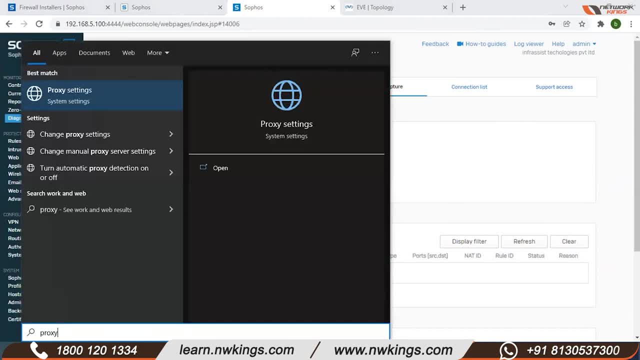 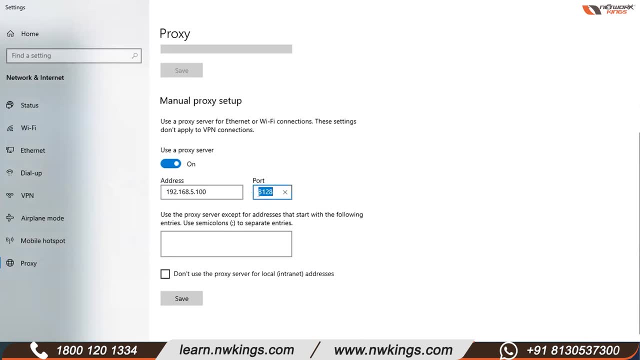 for copy. I use sofos as a proxy. ok, I have kept sofos IP. this is its default port. I will tell you about this where its sofos settings are. so let's say, for example, I have used sofos. 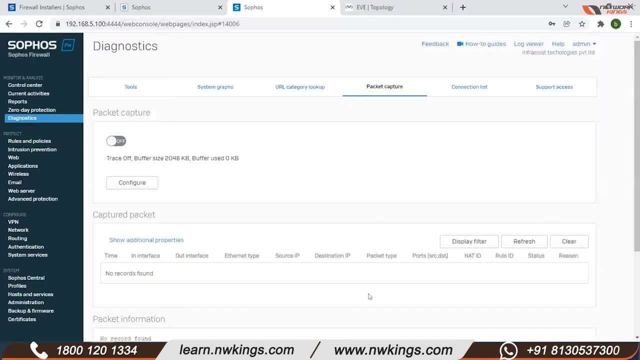 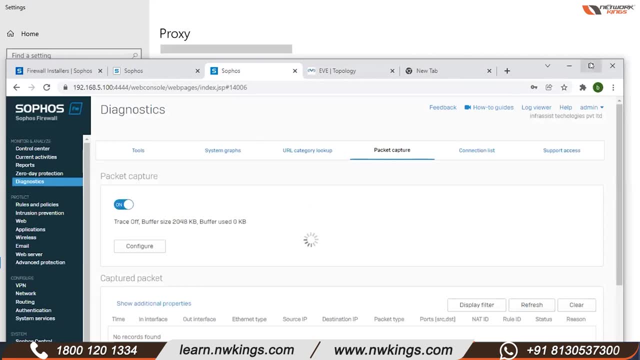 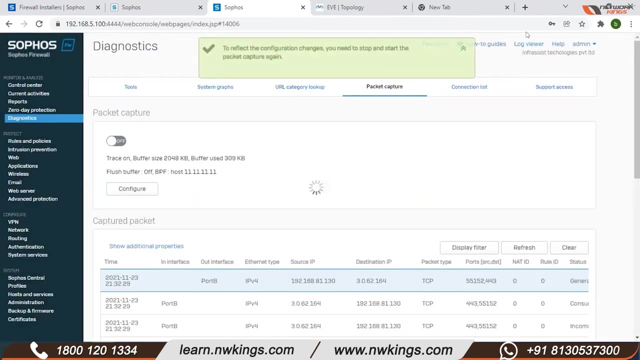 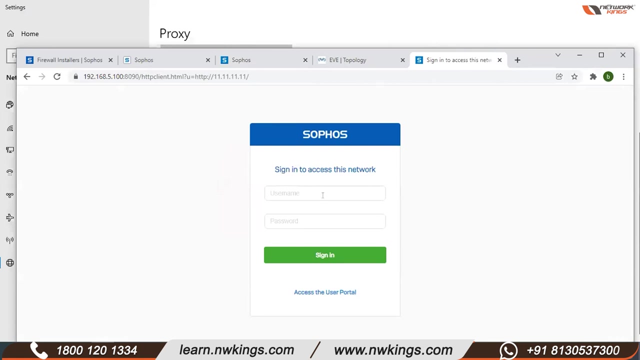 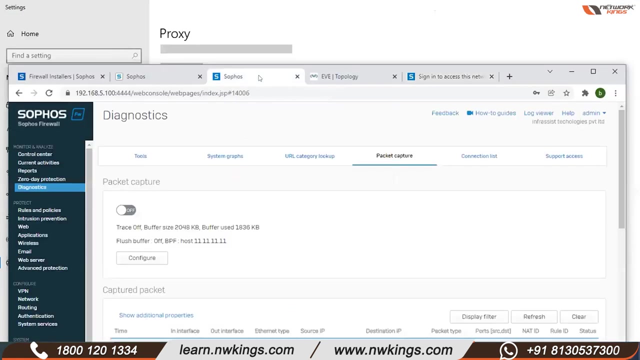 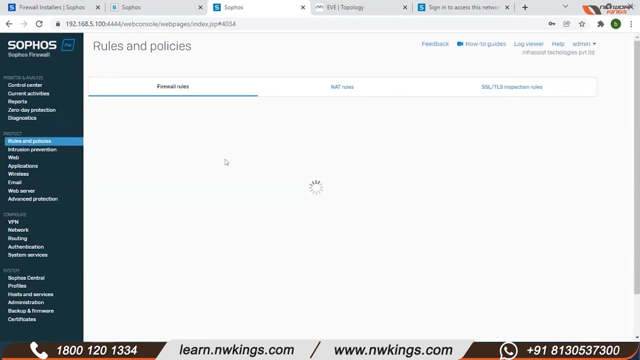 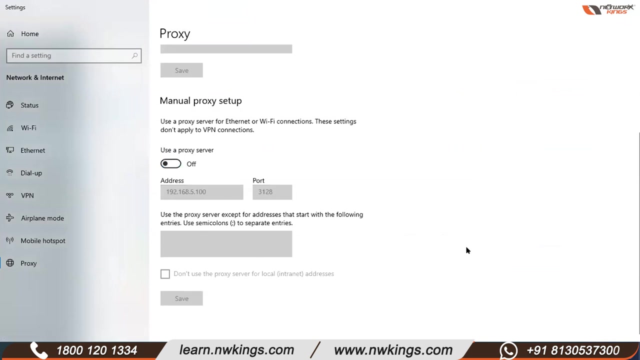 ok. so if I see, let's say, for example: here, let's do this, ok, so here I am. I have come ok, here, I am ok, here, I am ok. so here I am. 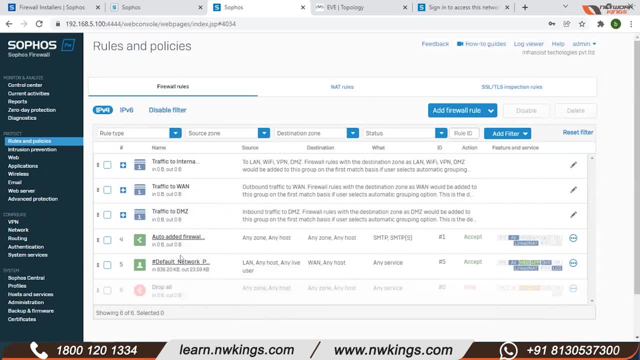 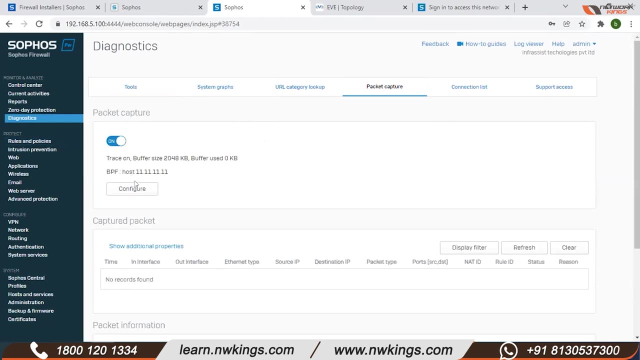 ok, now I am. I have come here for authentication because I have enabled. Let's see, I will tell you about this later. Let's go back to the diagnosis Packet capture. Let's say, for example: I have put an IP here. 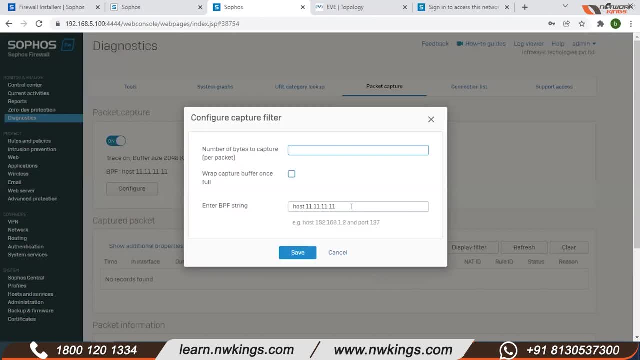 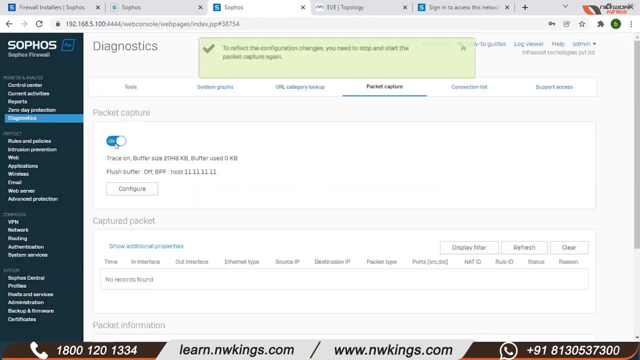 You can also check this one if you have a host power. So this command is host and this IP. You can access this in your browser, So it will tell you which rules it is going by for now. So we will also see about this in the lab. 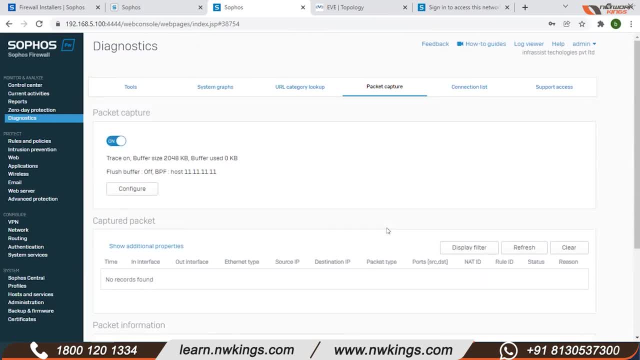 If we have a lot of rules, if we want to see which rules traffic is going by, then we can rectify it from here In the connection list. all the connections are there. As I told you, there is a stateful firewall. 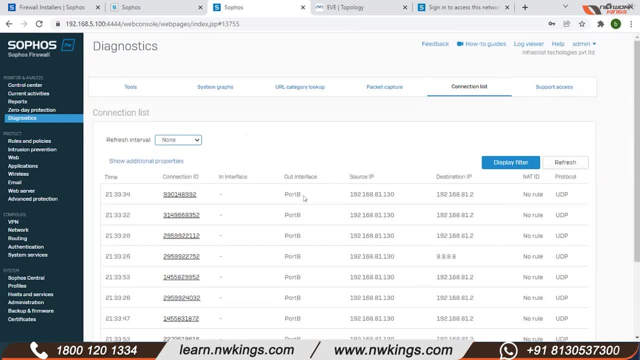 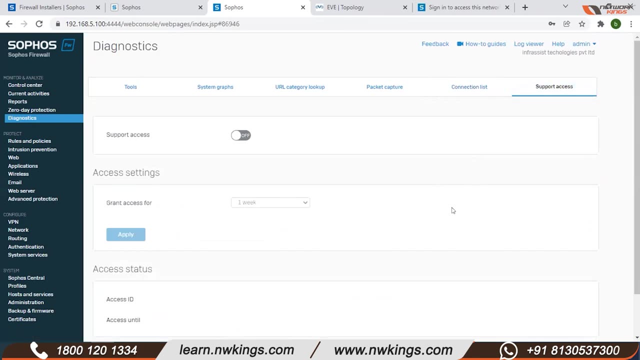 So you will get all the connections from here. We will also go into detail about this. How can we bring it into use To troubleshoot the issue? OK, OK. So this is the access support of Sophos. We are skipping this for now. 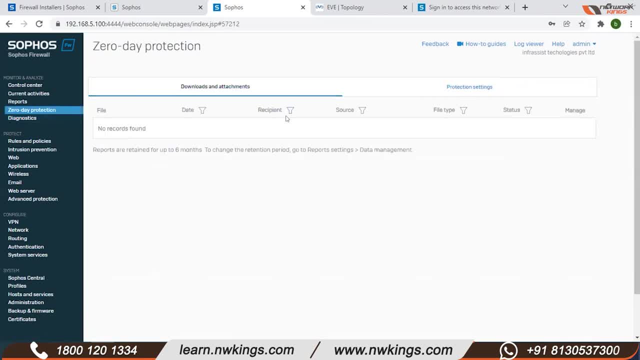 As I told you about zero-day protection, As an EXE file is coming, So you will get the full detail of the file from here, You can manage it accordingly. So we will also enable this and see Zero-day protection. OK. 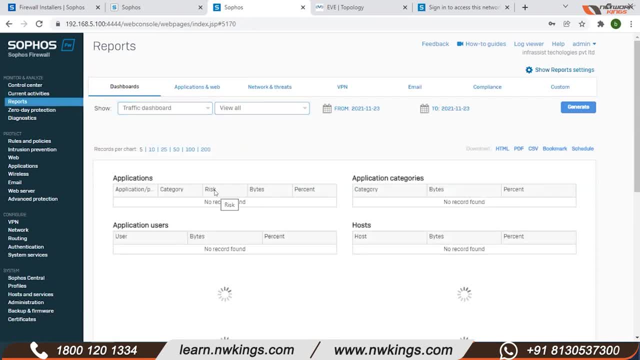 Reports. OK, We will also discuss all this one by one in the reports, So you will get the full insight of the traffic here. So how to filter it out To get the accurate report as per the requirement, Like any requirement, will come. 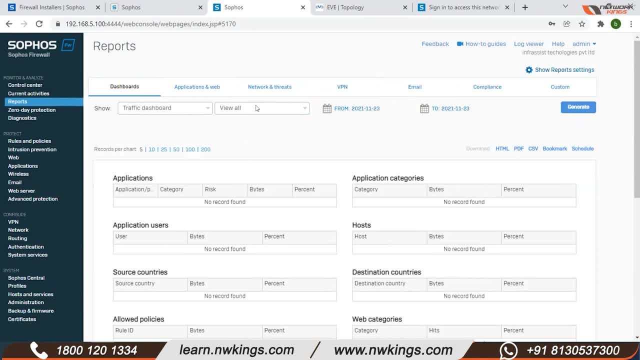 How to generate it Reports. So we will generate accordingly. We will also discuss about this. After the configuration is done, We will generate application and web traffic in it. We will also generate malicious traffic, And then we will have a look here. 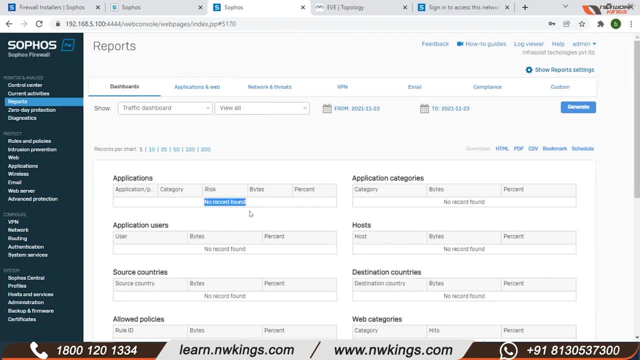 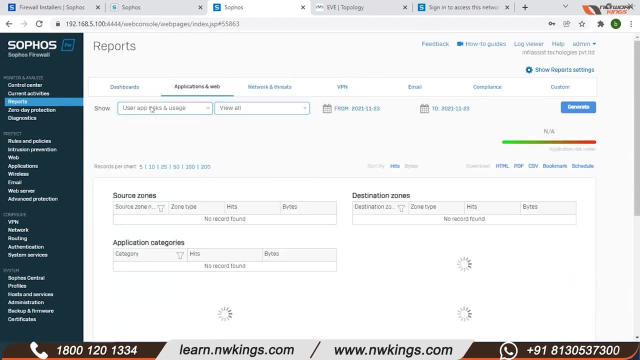 How it works, How it generates the reports And block this, in How it protects its network. Everything will be shown here: Application and web, All the users of LAN, All the reports of applications and web browsers We can take from here. 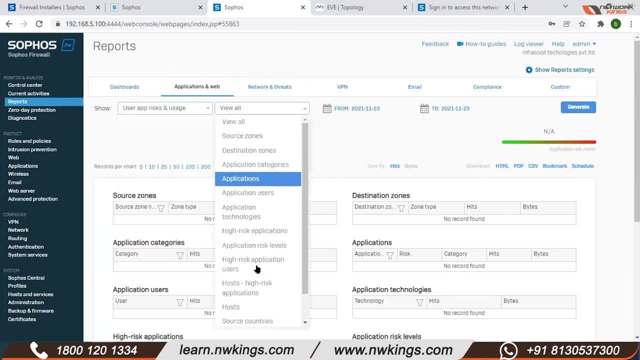 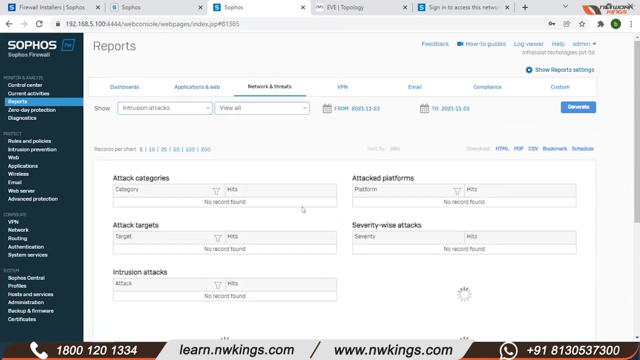 Like, For example, Which top applications have been used, Which high-risk applications have been used. OK And all, We will have one. We will see all one by one After configuration, If the intrusion tuition system, I mean IPS, policies are applied. 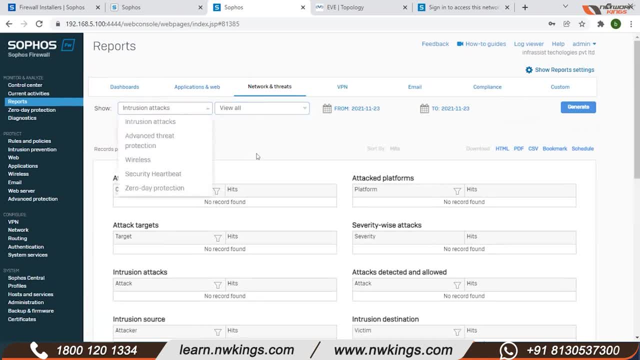 Definitely we will get all the details of all types of attacks here. So we will filter it out accordingly Here And we will generate. So we can also download In these formats: PDF, HTML, CVS. We can also bookmark. We will also go in detail about the bookmark schedule. 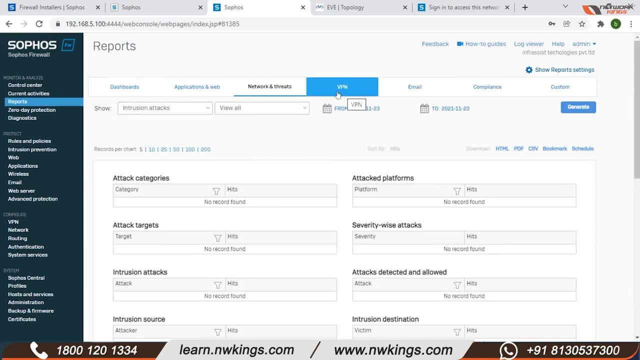 In the future, How we can schedule reports And daily reports on mail. For example, You can bring VPN Like which: How many users are connected to SSL? How many VPN sessions are made? Client list: How many are there? 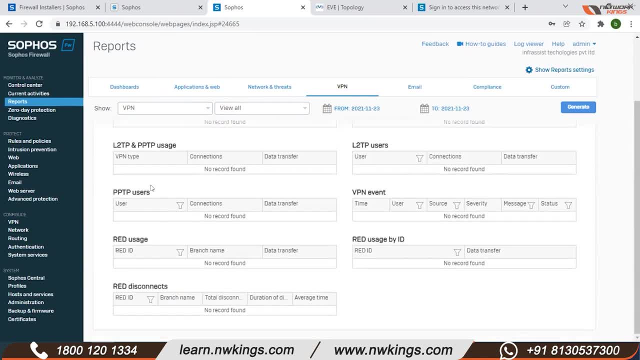 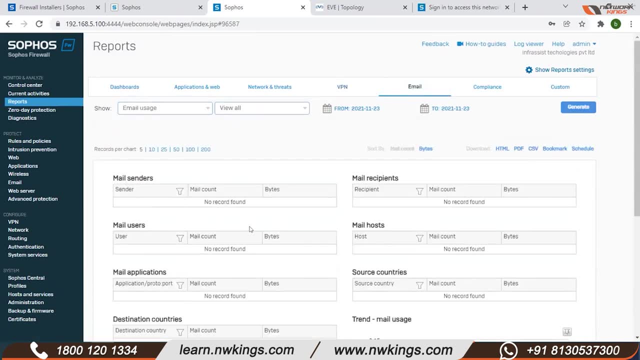 You will get all of that from here. Detail Like PPT: OK. Same way with email. That is, How many Mail sender recipients, How many Spamming? We will get all of that from here. Plus, We can also filter it out. 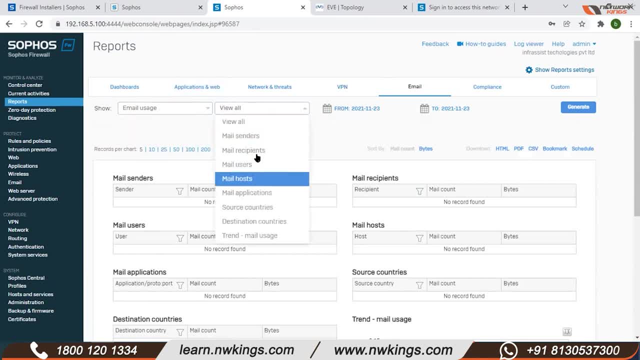 Sender recipients And we can troubleshoot it. We can generate complaints And custom reports. We will also see about it one by one Reports Generally When we test our users on two PCs. In that Different, Different A little bit. 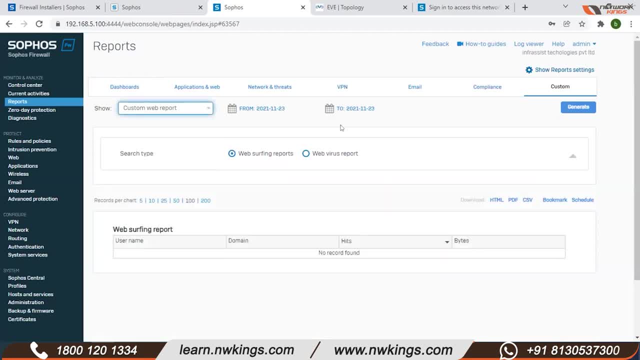 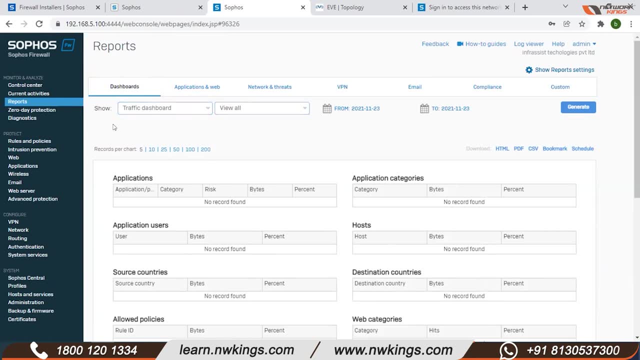 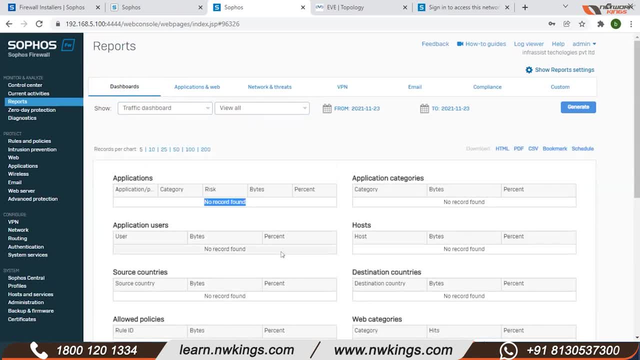 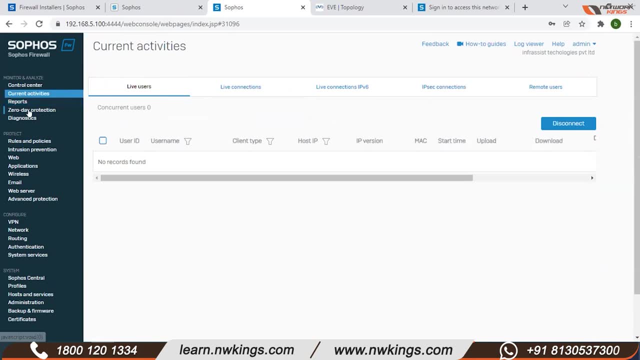 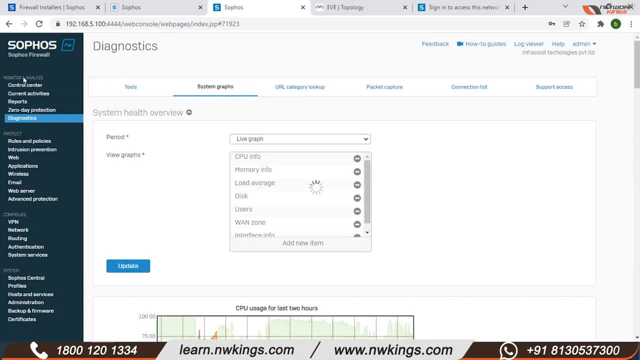 So now, Nowadays- Now I feel cold here, That is because of that- In the Very different OK, 1, That is here. 1 That is here. There, That is here. OK At, you can filter out as you want. now the default is like a live graph. you will get the information of the CPU. 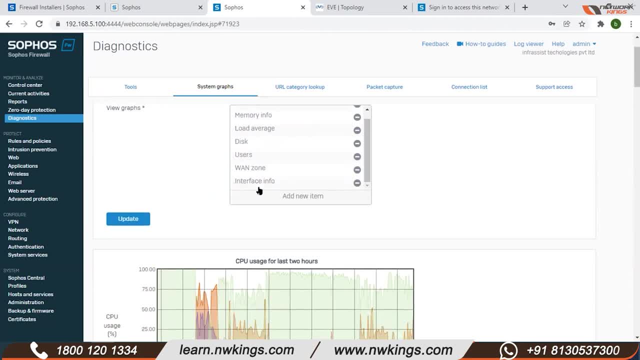 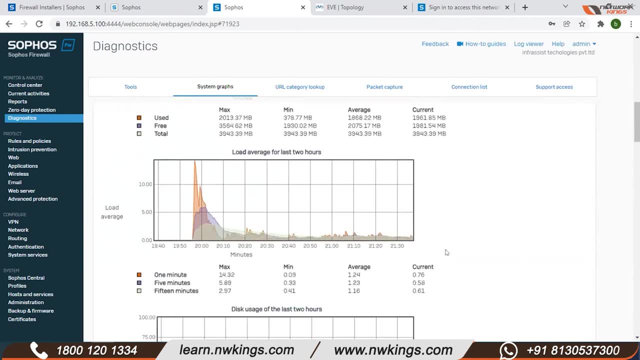 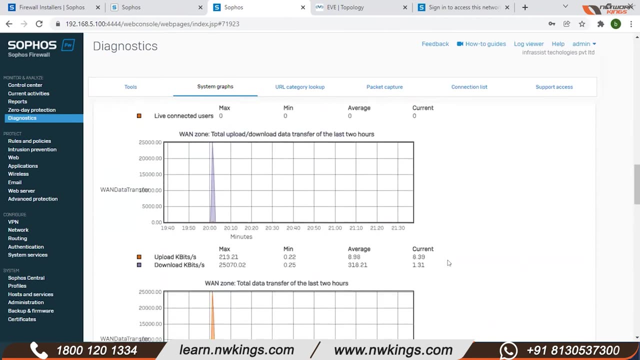 memory disk. how many users are there, when and how much information is there in the interface? you will see it here in the graph form like this: we will go into detail about this too. where can we use this thing? okay, to do everything. 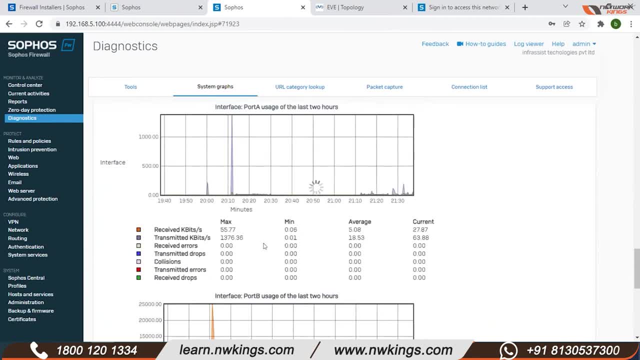 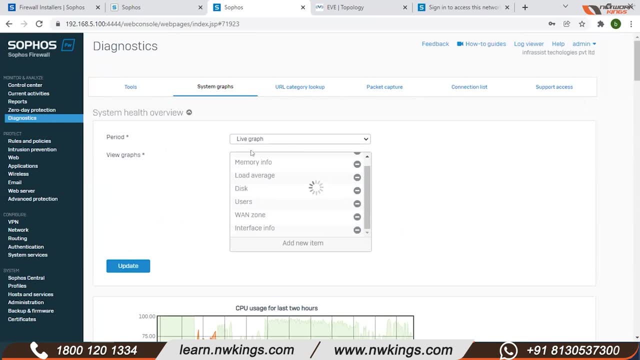 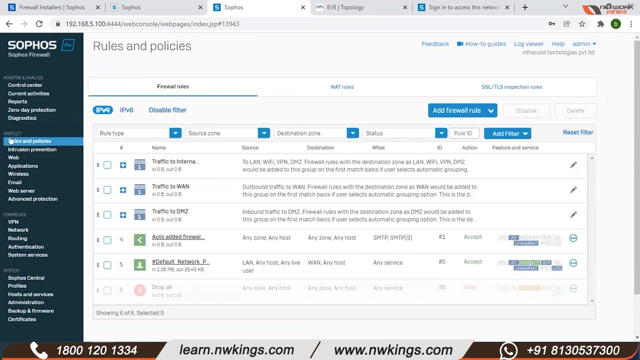 to do everything. okay, interface same way. here we can generate the reports: hourly base, 48 hours weekly, monthly, yearly. okay, then we come to the rules after a while. let's say, for example, we go to protect. there is intuition and provision in protect. 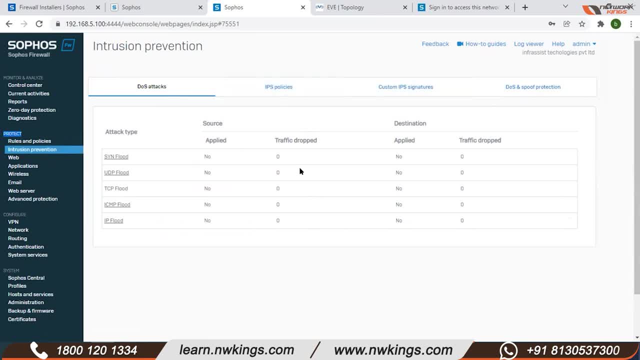 we can apply those settings according to ourselves. this will give you the overview of the door setting we have applied. if there is any attack, then if the sync attack is more than the door setting we have applied, okay, then the traffic drop will give you insight here. 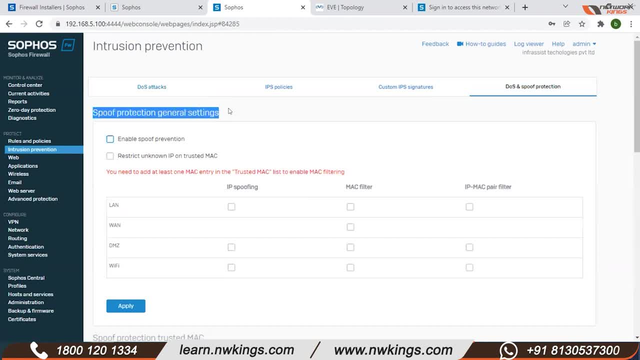 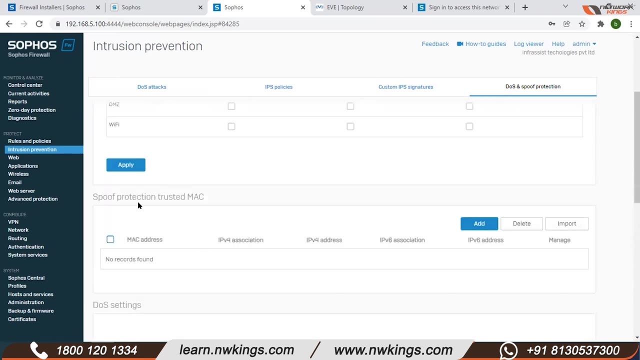 you can configure it from here so we can also do spook prevention. if we want to give the trusted mac internet, then we can enable it and we can use the spook protection feature of firewall in this too. make sure that all macs are added, otherwise the internet will not work for that user. 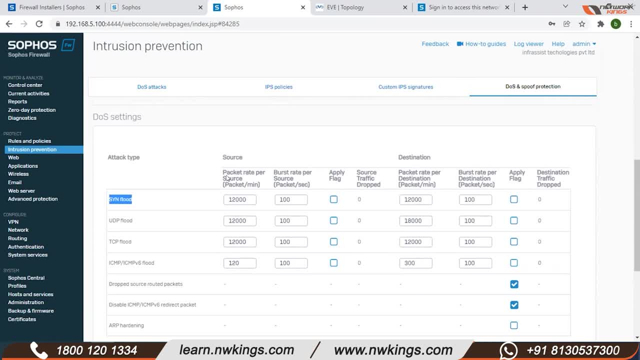 okay, we can do those settings here. like there is a sync flood, so how much source is it generating? on the packet there are default settings of the firewall. how much traffic is generated in our system from outside to outside. accordingly, the packet per minute that is generated, which is legitimate. okay, then we can set it accordingly. 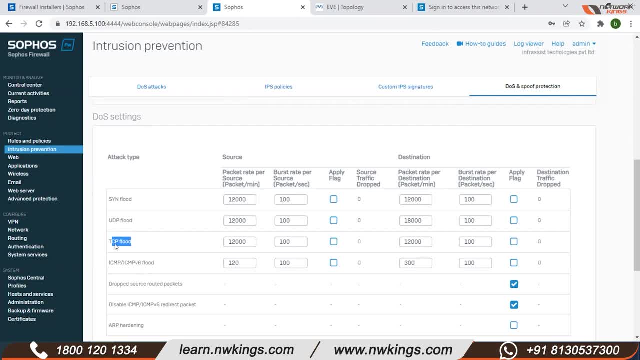 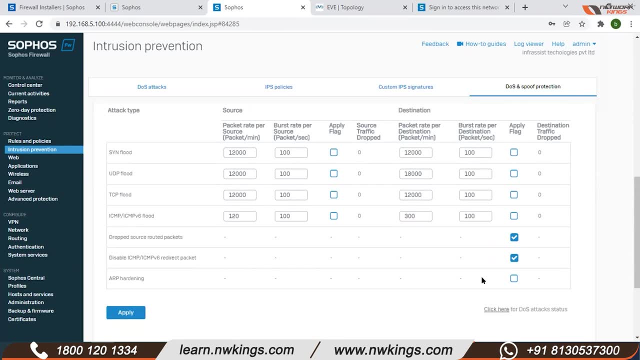 same way with the udp flood, tcp, flood, tcp traffic. how many packets are generated? we can do it accordingly. we can apply the flag here. if it is more than that, then that traffic will drop. like there is a request, there is a sync. 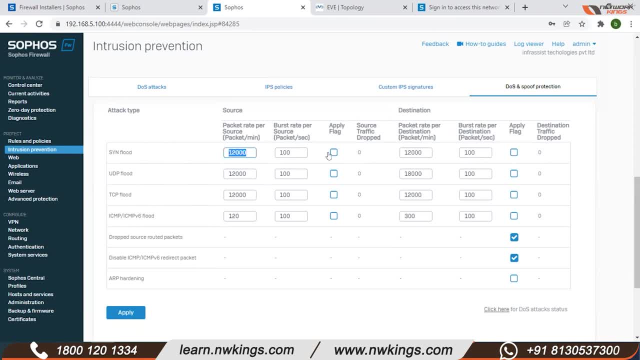 so if we have set it more than that, if we have set it more than that, then it will definitely drop and show us here. we will also get the details of this. we will try about this. if anything can happen in the live environment, then we will definitely see. 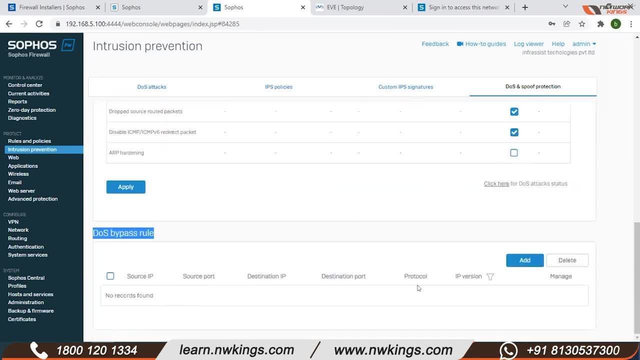 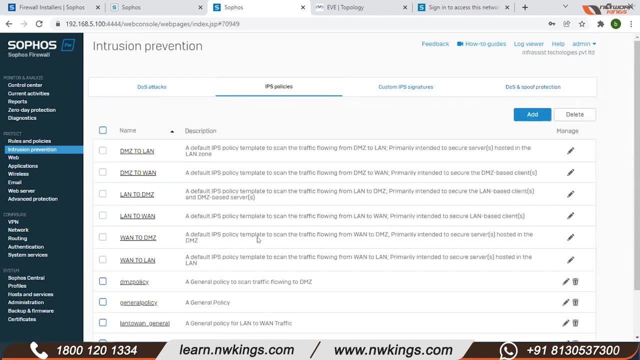 if we have to bypass something, then we will also see that if we have to bypass some port. apart from this, ips policies on surface firewall. here the default ips policies are here, so we can apply the default. like there is land to van, dmz, dmz to van. okay, we can apply these policies. 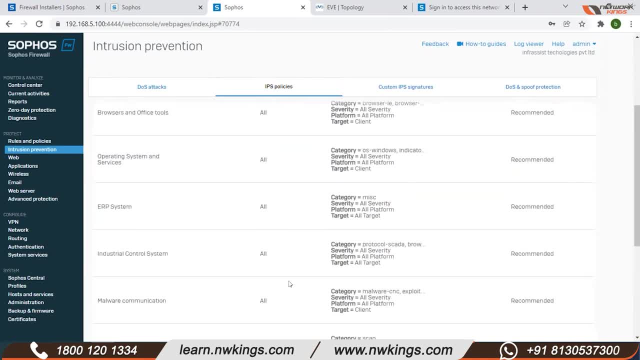 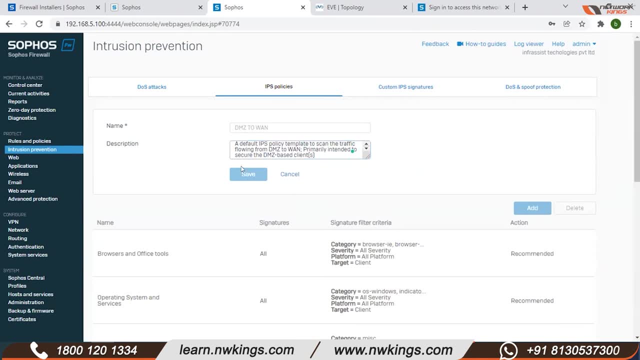 so if you have the insight of the policy, you will get it in detail here in the modules. we will already do it one by one and see how it works. but these are the recommended so we can also apply these policies. we can create our own policies. 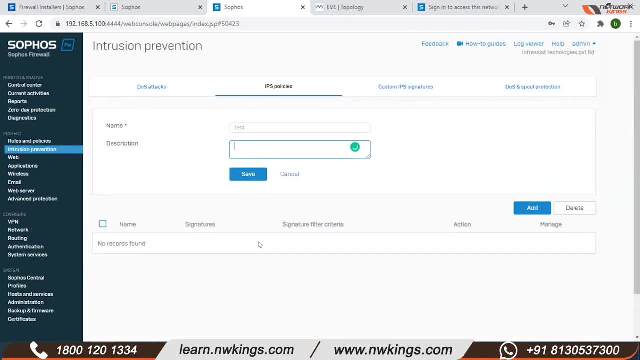 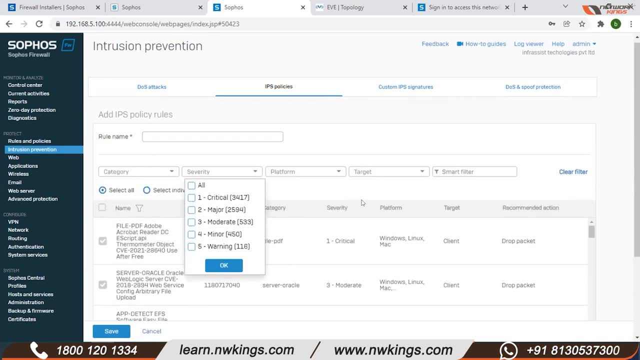 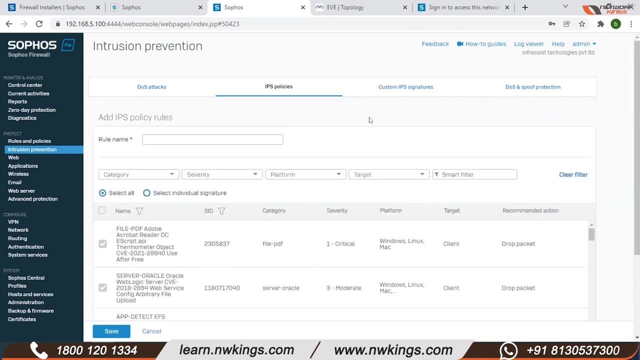 like I have tested here, so I can add: what are the categories, what is the serenity? according to this filter, we can take action by making our own policy, whatever action we have to take. so we will also go into detail about ips policy, how we can use default, how we can use custom. 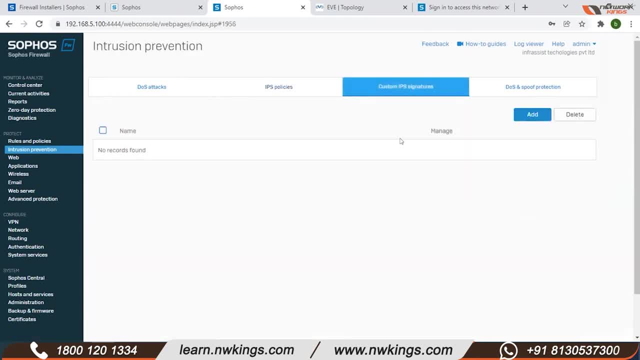 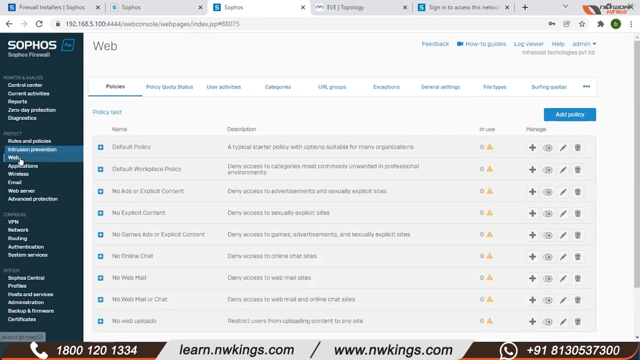 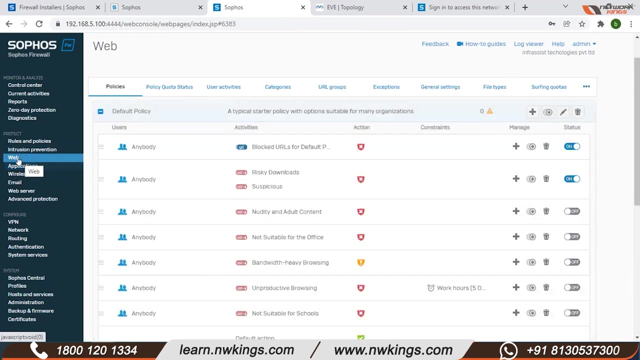 how we can generate its report. if anyone has third party ips signatures, then we can also add it in the firewall, of course. so we will do that as well. how we can import those here. web policies and application policies, ie application filter policies. there are web filter policies here which we can create here. 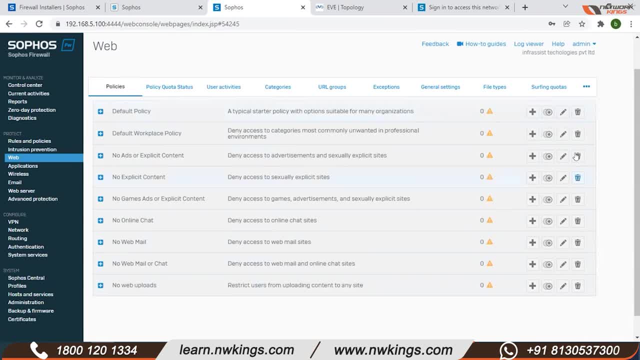 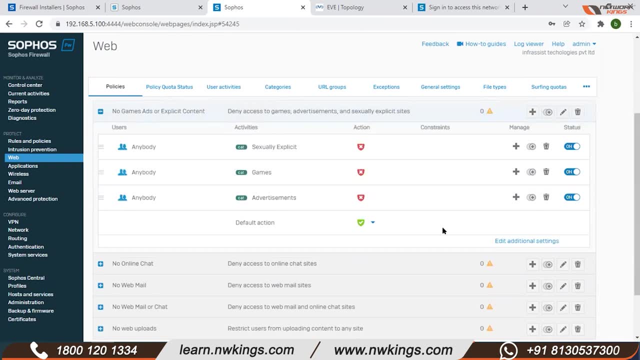 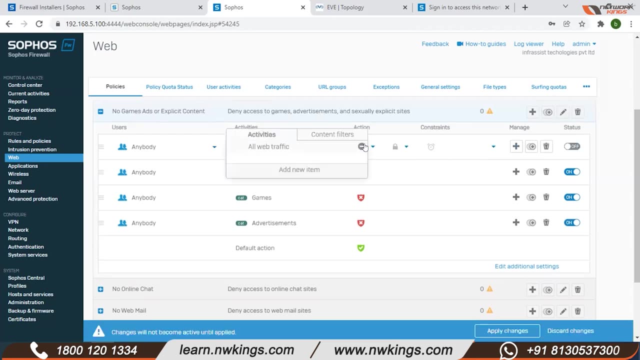 by default. this much will come to you by default as you can apply directly on the file, then all these categories will be blocked. if you want to block something else, then you can go to rule above and block accordingly. here all the categories are available. we will also see that. so this is the default policy of the database. 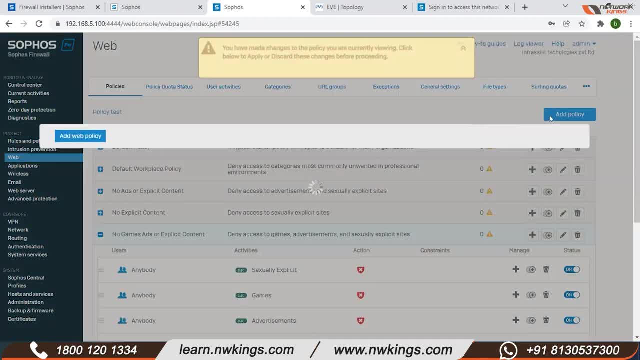 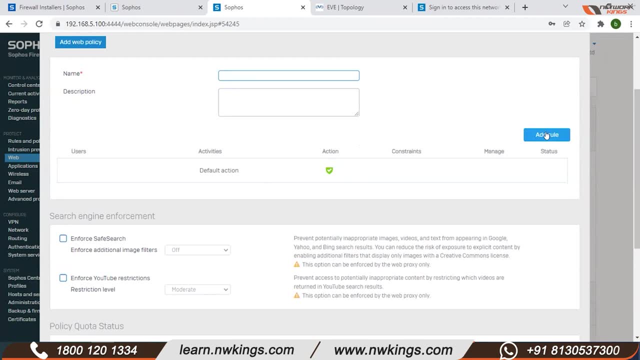 you can also create your own custom policies for policies. this is a template. name it then on the add rule. whatever categories you have to deny can do it. if you want to allow, you can also allow. it exist in file. 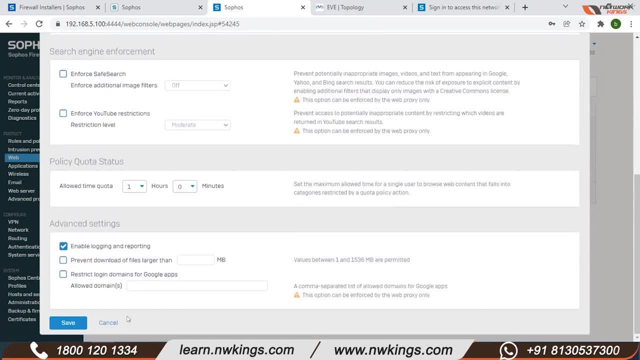 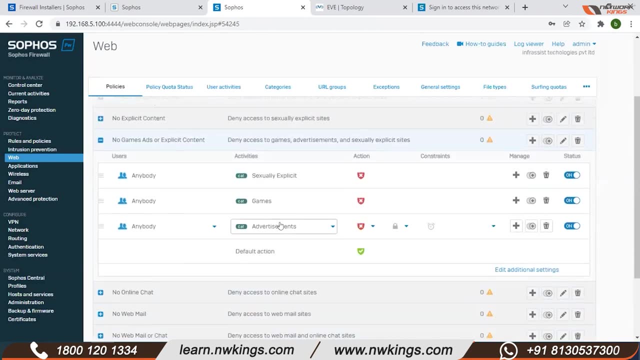 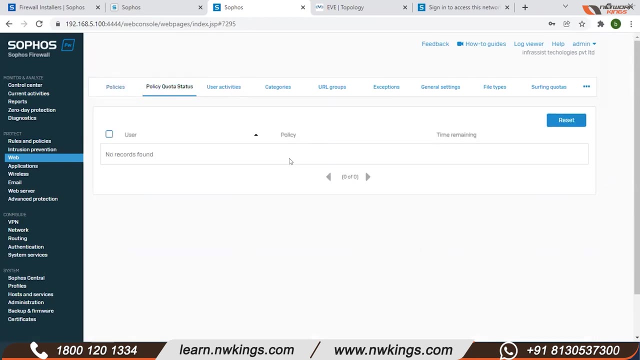 regarding this, we will also see different, different scenarios, especially in the development of applications, web filter, application filter which business meet requirement we can meet generally to block on unvoted activities. so same way we can add, as I said, if there is any quota on policy. 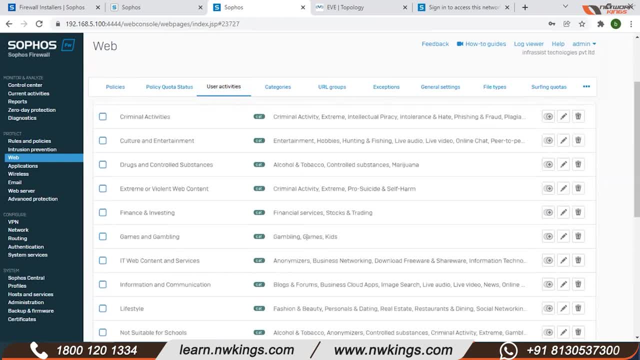 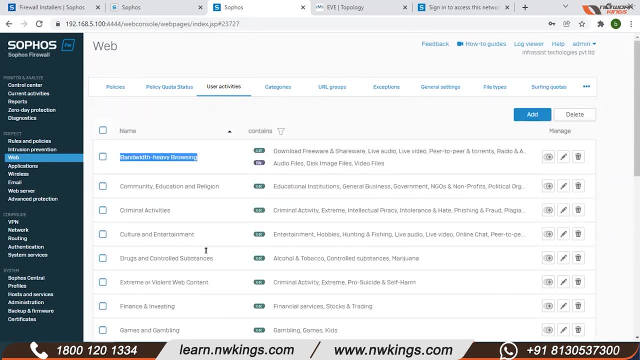 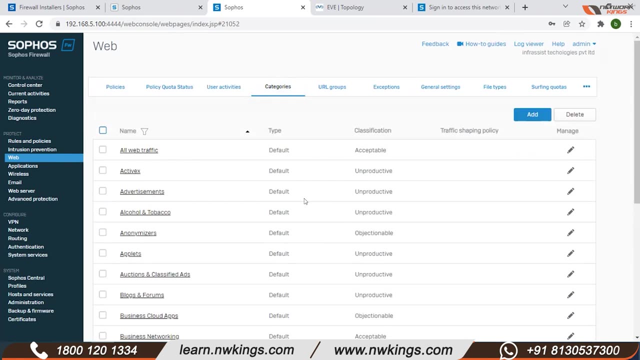 we can see its status here. user activities: we can see here categories already here. default policies. I will provide you same way: all the by default categories you will get here like advertisement. if there is any advertisement, then it will be followed if we blocked it in web filter policy. 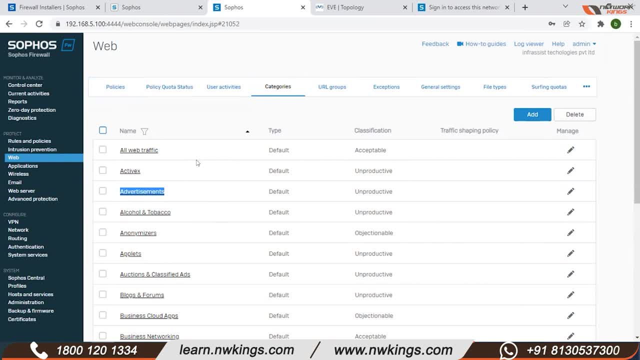 then all the websites advertisement will be blocked. but yes, of course for that we need proper configuration, like, if there is some traffic intercept, then we can enable that, even though, after applying the policies, so that is the best configuration. we will go in detail about that because there should be no loose point. 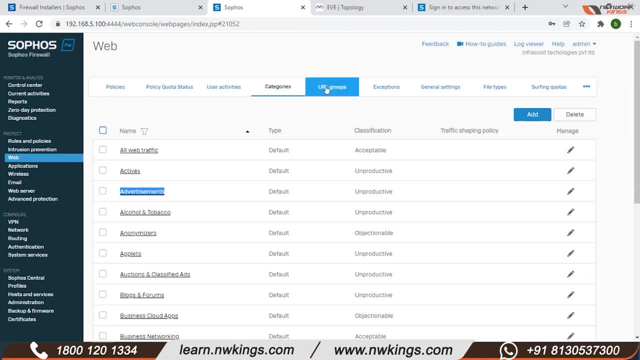 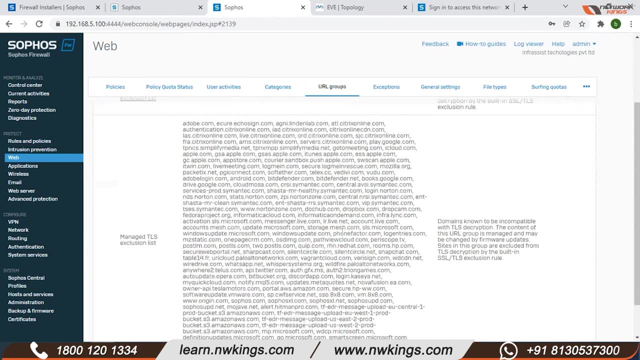 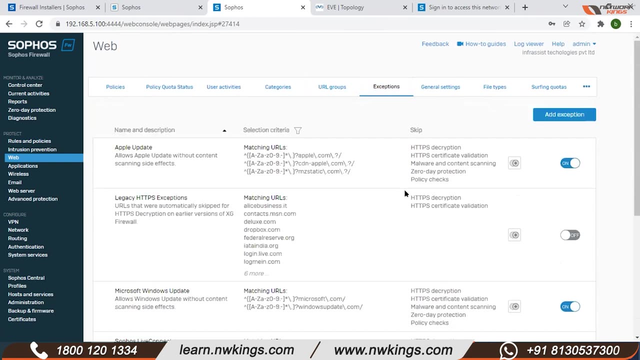 in configuration. if configuration is proper, then we will be safe and secure. if we want to make some url group, then we can make it here. we will see about this. where this can be used. where this can be used, we will see that if we want to bypass something in scanning. 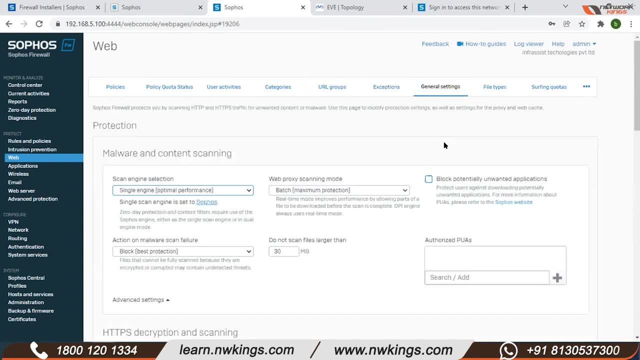 then we can do it from here. there are general settings. web filter means any browser based traffic. we have to monitor it, so we can do it from here. so generally it will scan the whole traffic. you can do it from dual engine or single engine, dual engine and single engine. 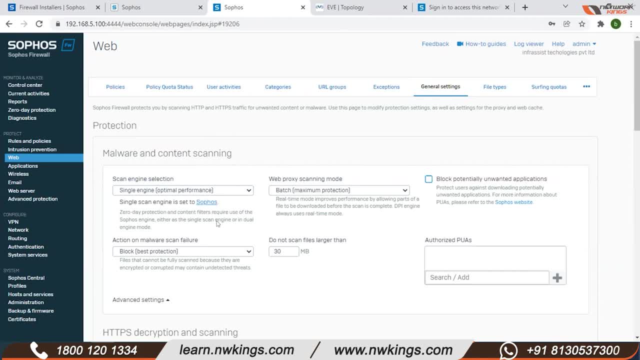 you can use your own antivirus system as well as avira, which is integrated. it has its own settings. I will tell you same way. you can change the scanning mode here you can take action if malware is detected. ok, if file size is high, then we can put restrictions. 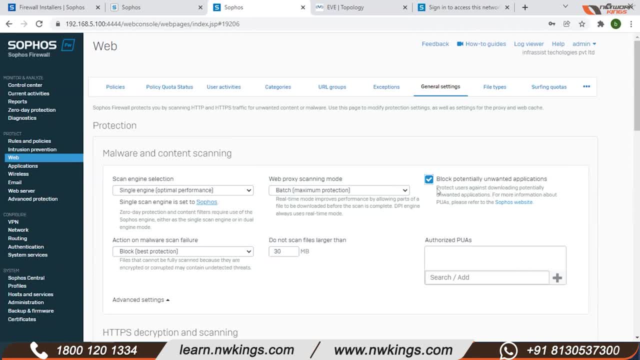 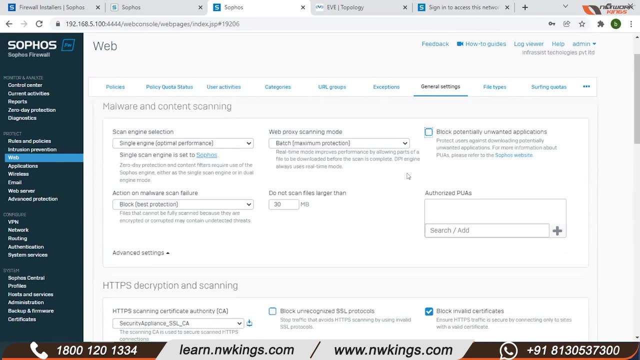 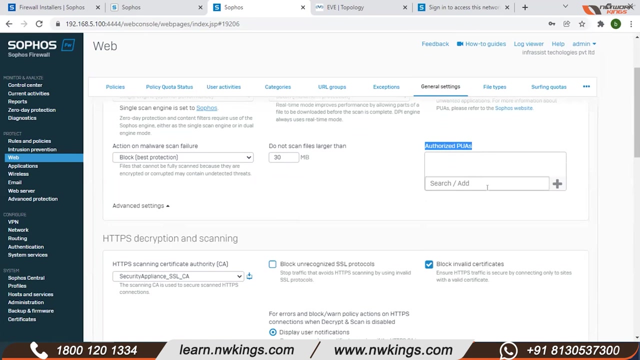 PDU is there. for example, if any website user access- for example mining, for example cryptocurrency- PDU is there, spyware- everything will be detected and blocked. we will enable all the settings and check. by default, it is disabled. if anyone is authorized. PDU is there, we will add it. 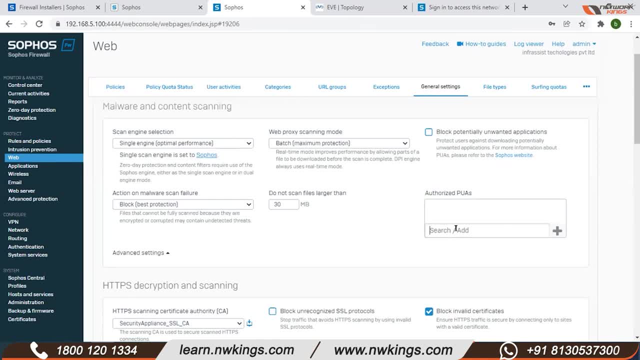 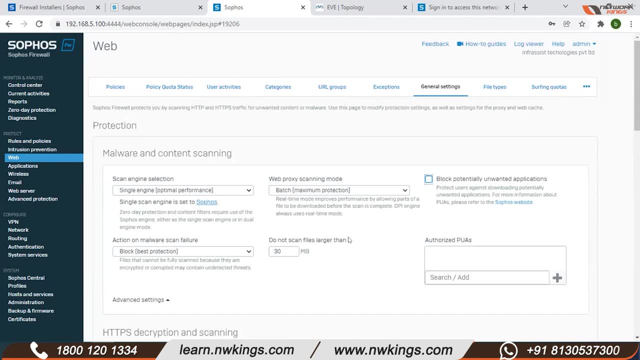 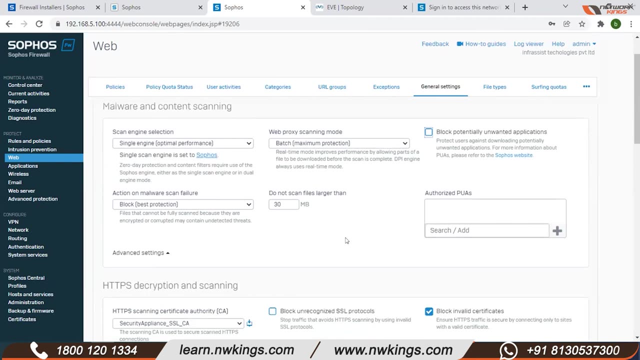 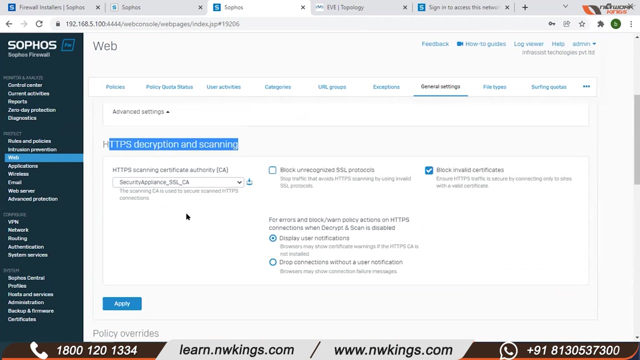 potential unwanted application. we can bypass it if it is enabled. ok, we will see about this. no worries, any configuration. if it is miss out, we will work on it. we will discuss about HTTPS scanning certificate, because this is also very important generally to intercept the HTTPS traffic we have to decrypt. 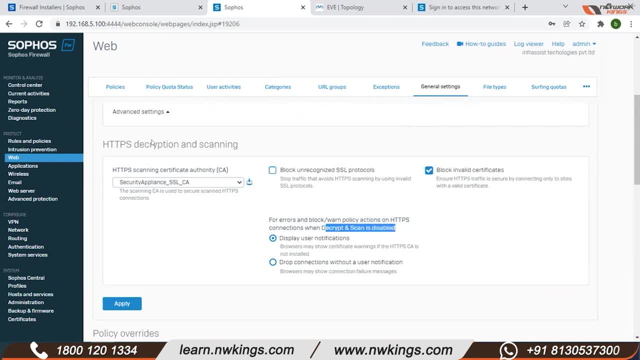 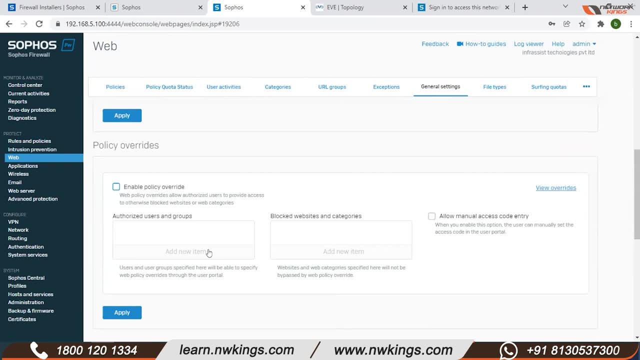 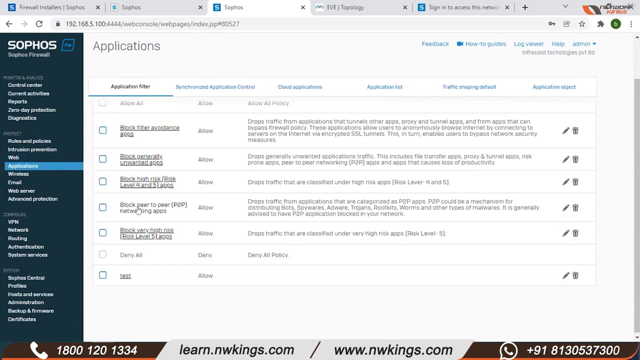 the whole scan how we will do with the software certificate. we will see any policy we have to override generally, if authentication is enabled and we have to bypass, then we will use this feature. about this after authentication we will see. same goes about the application. so these are the default application filter policies. 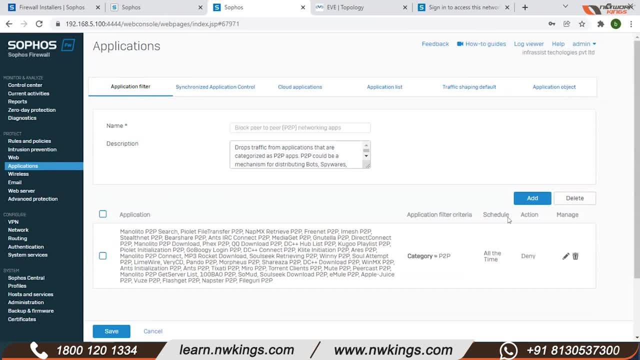 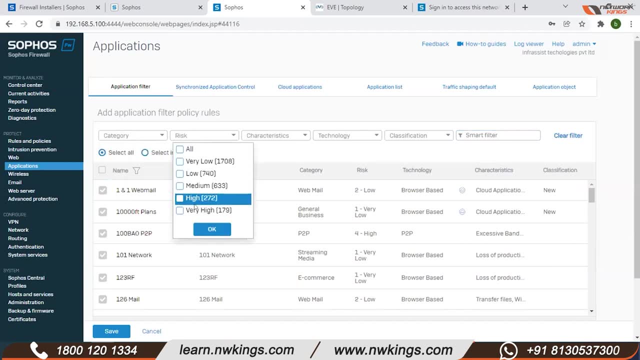 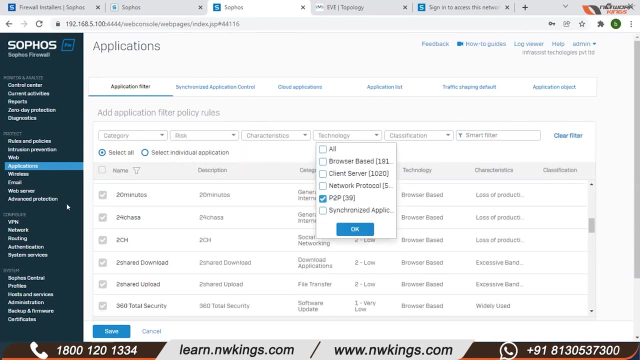 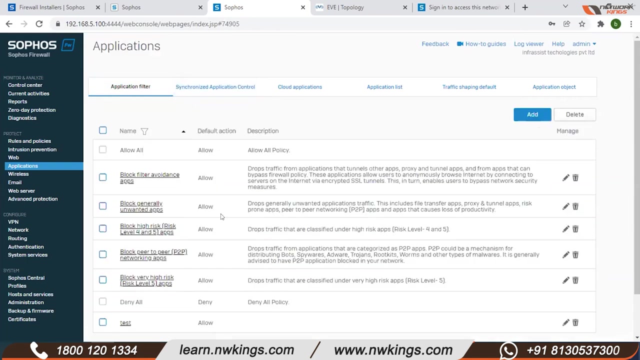 as it is already predefined, so you can directly apply it and this application will be blocked. if you want to block something else, you can block it category wise or risk wise, category wise, same categories or technology. we can select it and take action: allow or deny. so this is application filter policy. 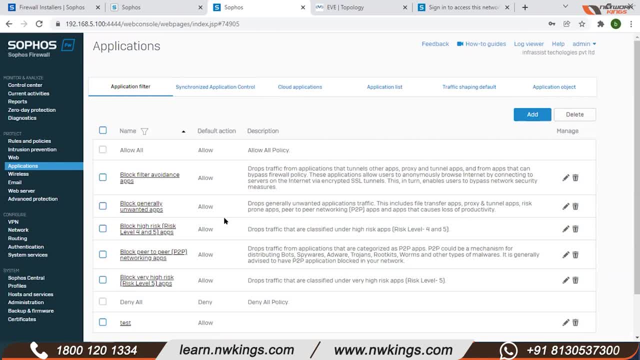 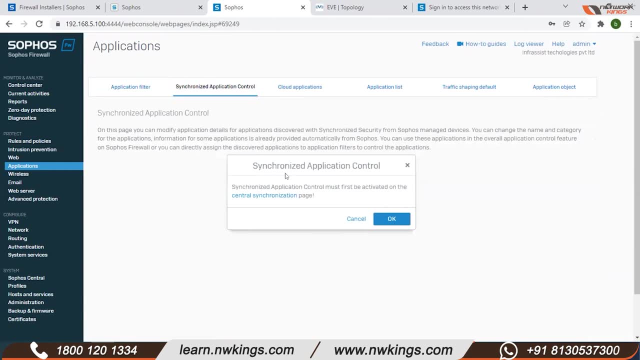 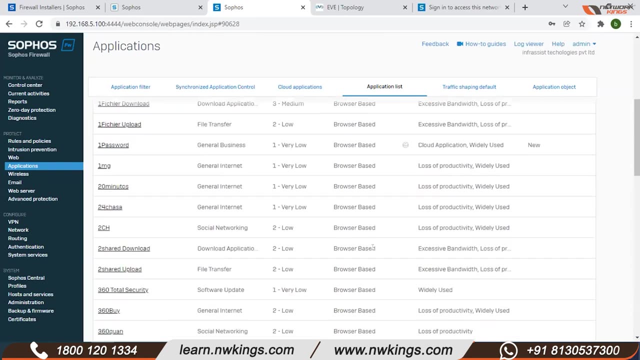 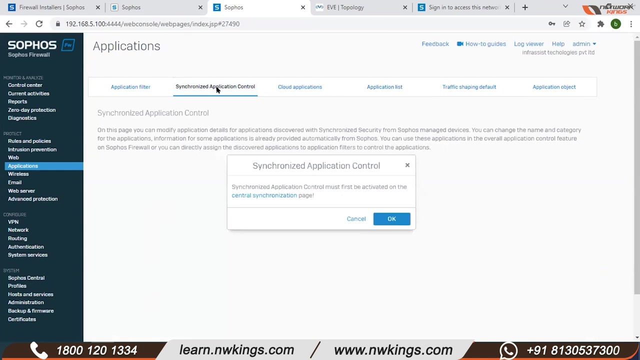 we will create some scenarios: how to allow or block. same way goes with the synchronized security, as I told you, some users have downloaded some application which is not categorized. here is the application list. by default it is not categorized, so we will call it synchronized application, as I told you. 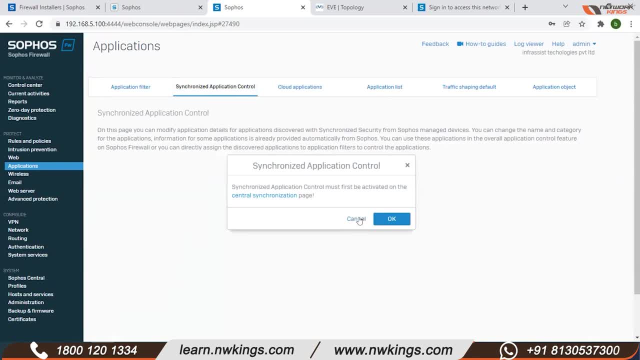 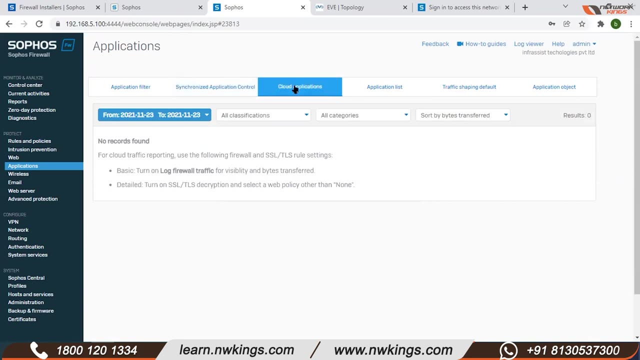 it should be central as it detects. we will see there are a lot of applications. we will put endpoints and see how it works. same way with the cloud application, as the synchronized application works, same way the cloud works. let's say, for example, if I use services, it will definitely tell you. 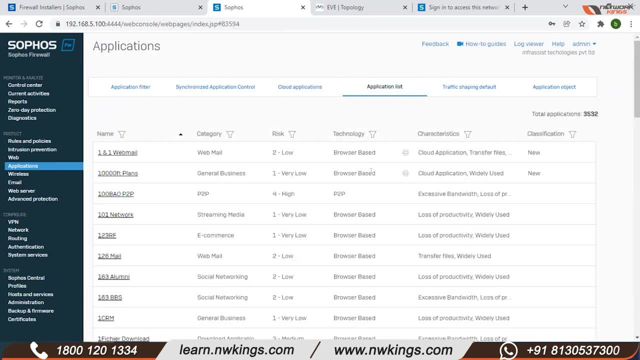 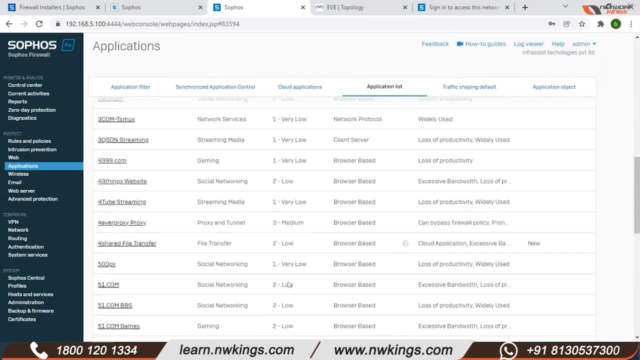 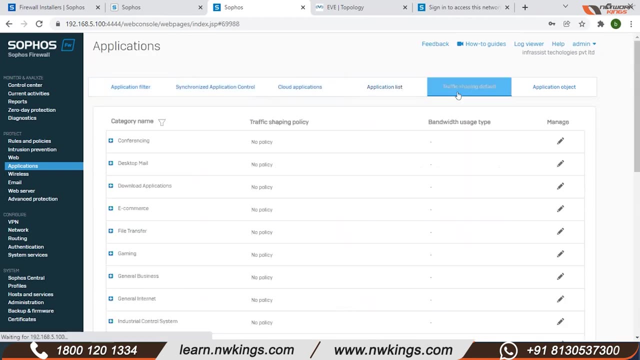 all the details, application list, all the applications in sofos, you will get its database. we will discuss about this in module, how we can use all these things. traffic shaping. traffic shaping is generally bandwidth QoS policy, QoS policy or bandwidth traffic shaping categories. let's say, for example: 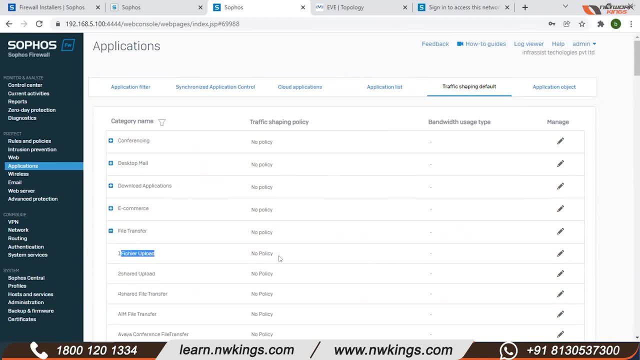 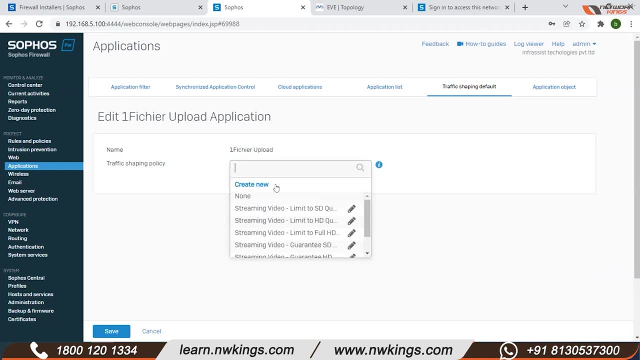 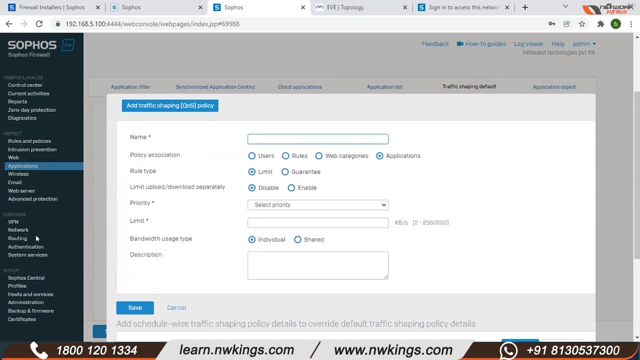 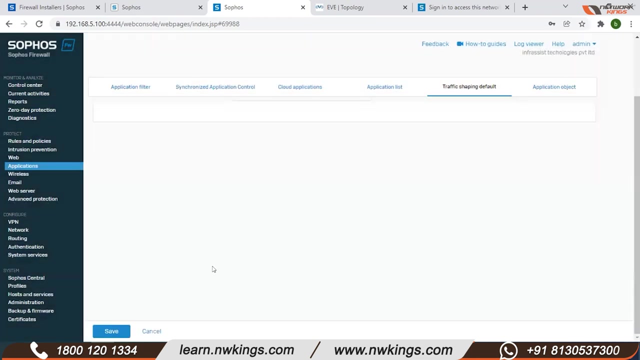 file transfer. in this application we can use bandwidth like 256 kbps, for example. here you will get default policies. you can create policies according to you. we have covered about this in modules: how to make policies. bandwidth policy: we will see like this department: only 5 mbps. 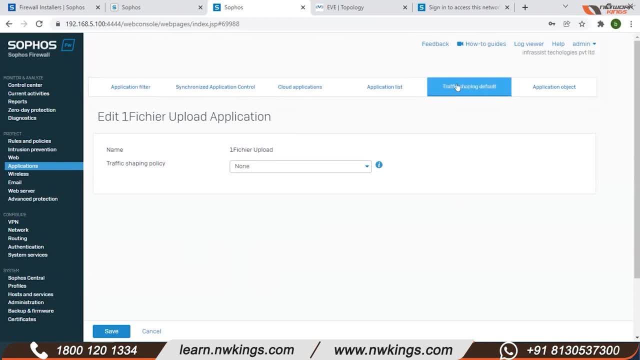 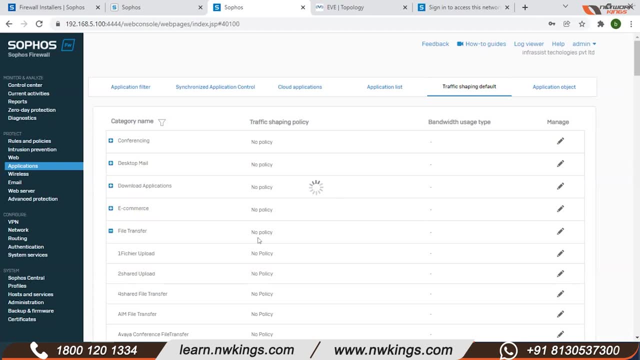 this department, 2 mbps, for example, how we can create QoS policy in application QoS policy, we will differentiate definitely. whenever we have lab access, we will have live session definitely. I have gone through many questions. we will discuss about web and application, as we are talking about. 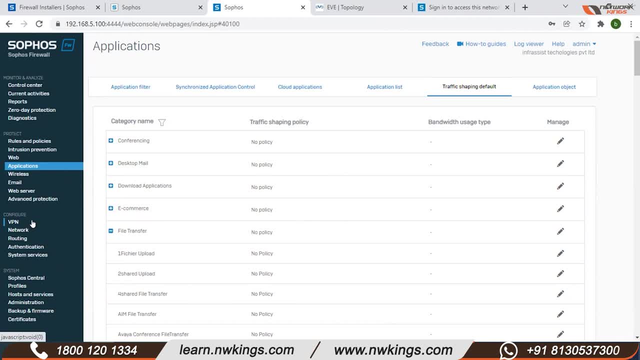 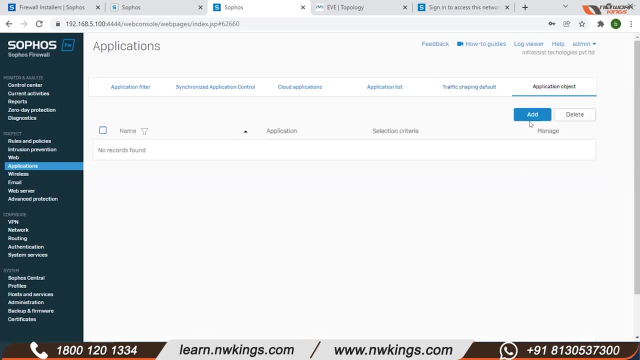 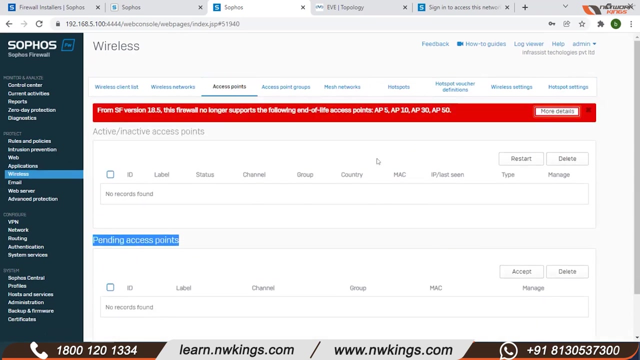 about web and application. SD-WAN can also come, so definitely we will cover all questions one by one and also application objects. similarly, how we can object it wireless protection in firewall generally. I told you about AP. you can see in third tab in pending list. you will accept it. 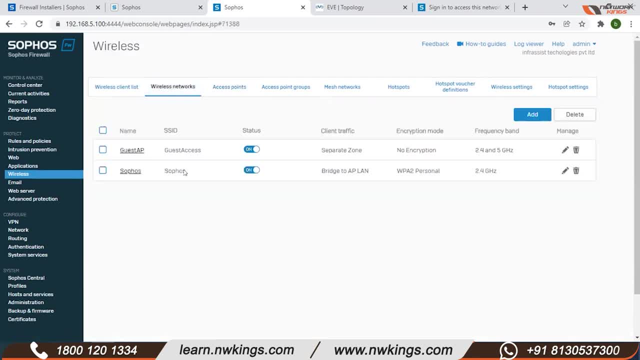 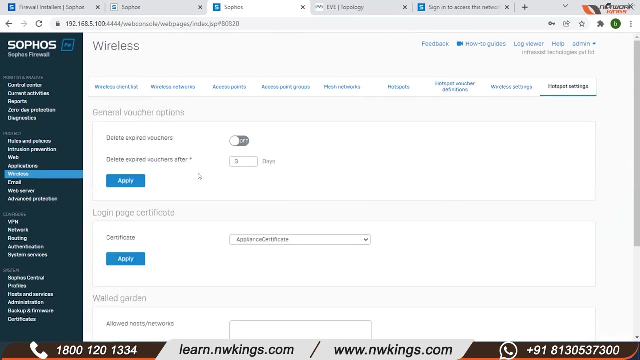 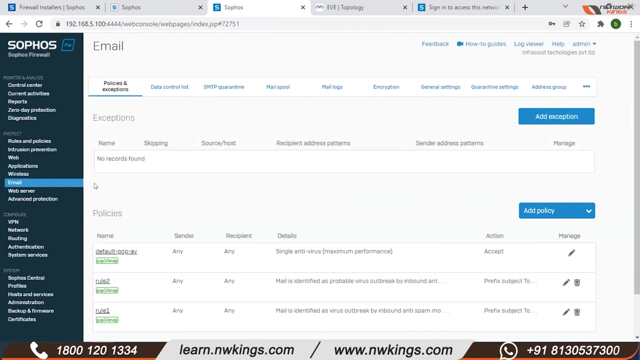 and configure it generally. we can manage and configure it from here. we will see what is mesh network, what is hotspot, what is vouchers. we will see what is wireless settings, what is hotspot settings, how to connect with software. if you have any email, we have email protection. how can we protect email? 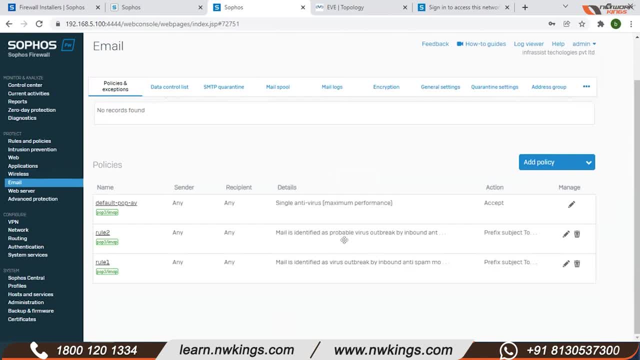 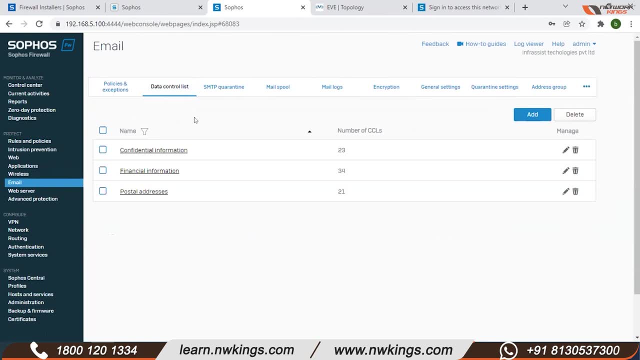 from policies. by default there is policy, so if any suspicious email or probable spam or virus will be blocked. so already it has other 4 features. we will see the difference In the MTA mode, like if someone is sending a mail or receiving it. 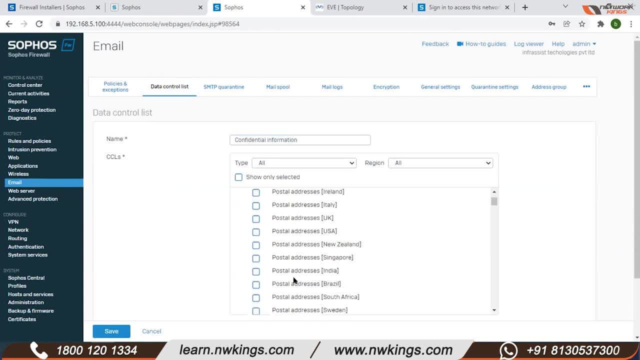 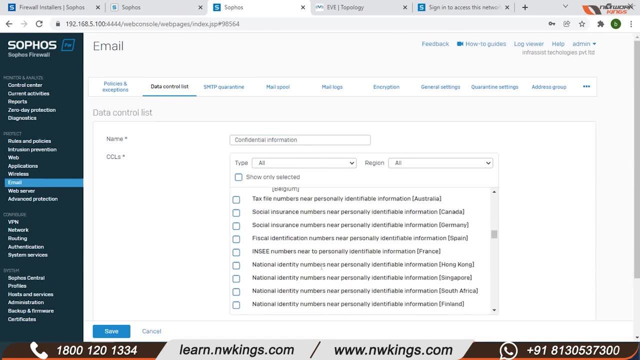 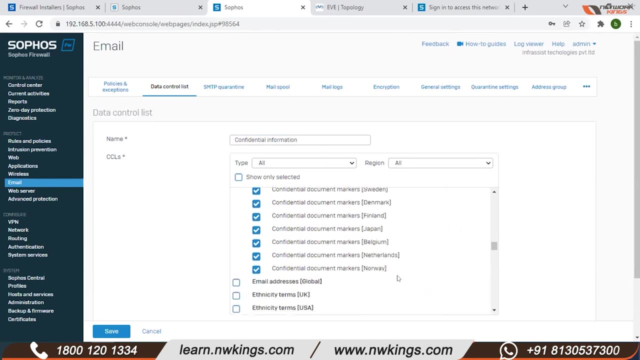 there is confidential information like postal address or something like this account number, etc. Everything is listed. So we will get that mail. We will also get its copy so that we can diagnose and rectify. There is no confidential detail about the organization, So we will also see the data control list in detail. 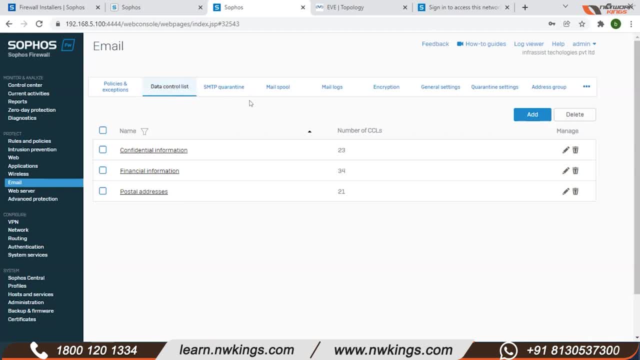 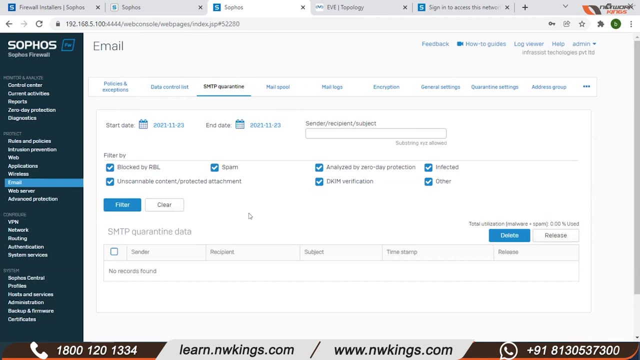 There will also be a lot of questions. For now we will go through the GUI. Later we will definitely cover a session along with the modules. So if there is some quarantine, we can see here. If there is any mail, it will be quarantined from here. 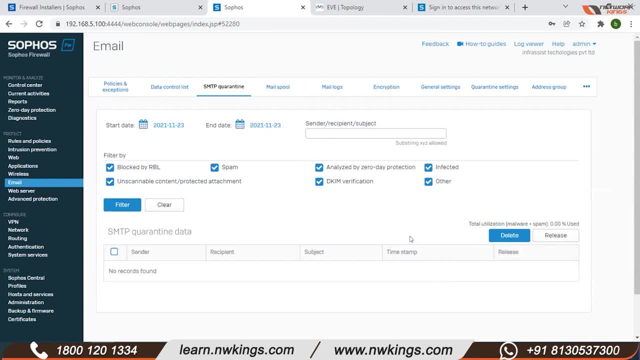 If we want to release, we will do it from the user portal. How will we release the mail? If there is a quarantine and it is legitimate, we can release it. We will also see that. We will also get logs. We can also generate from here. 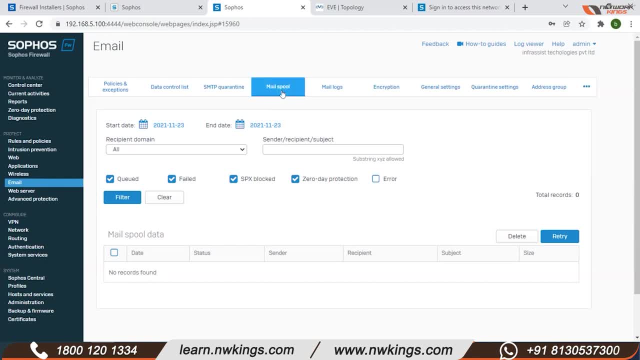 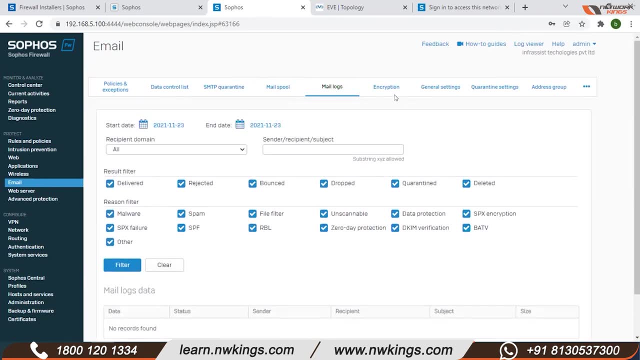 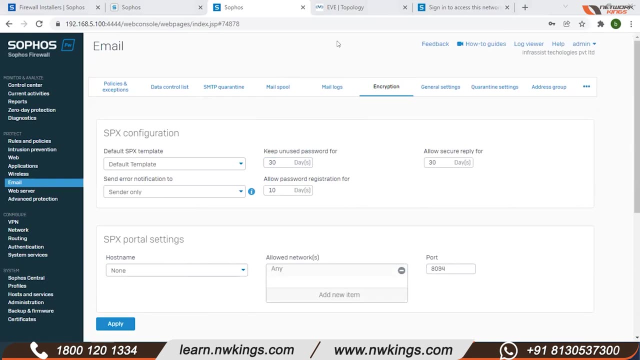 So you will also get the mail from the monthly report in spoof And mail logs too? Yes, according to this. Thank you, Bharat. I think it's very good. So, guys, if anyone has any doubts about this course, what we will cover up, you can ask upfront now. 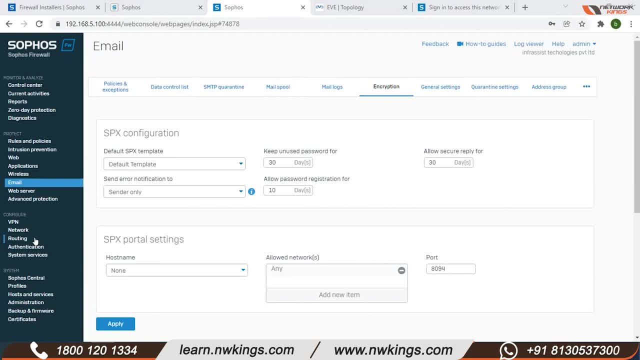 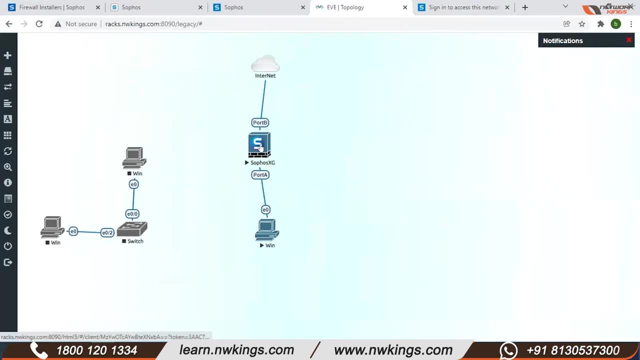 Now we take doubts. If anyone has any doubt or query guys, tell us Sure, Okay, so what we will do. Generally, our network topology: we will work on it. How is the traffic going in and out? We will also see packet capture from sofas. 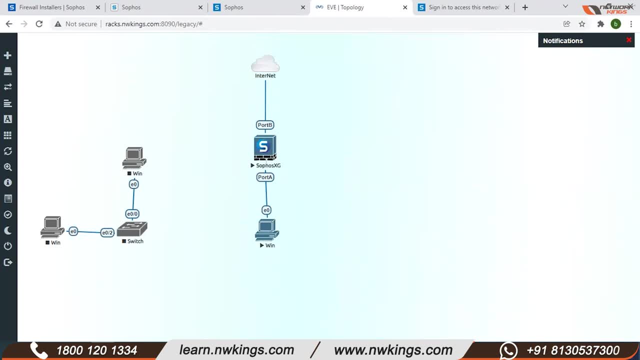 Like there is a three-way handshake, right, For example. how is the three-way handshake going? How is the traffic going in and out? Generally, in any file you have to see the traffic in and out. How is it going from here, Like if you are going to Google, how is the traffic going in and out? 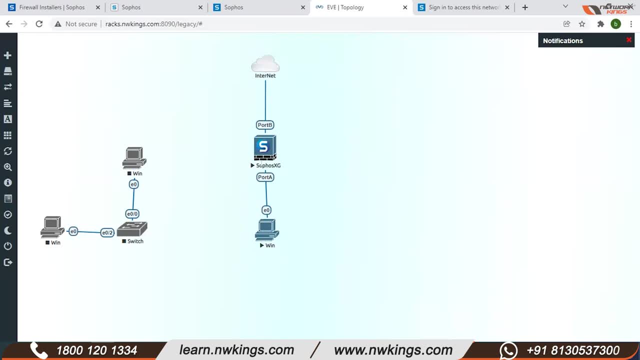 How is it going to Google? How is the return coming back? We will see that whole packet capture. Yes, of course, And as I told you, we will cover up all the configurations in the module. For example, if we make a branch office, we will connect the branch office. 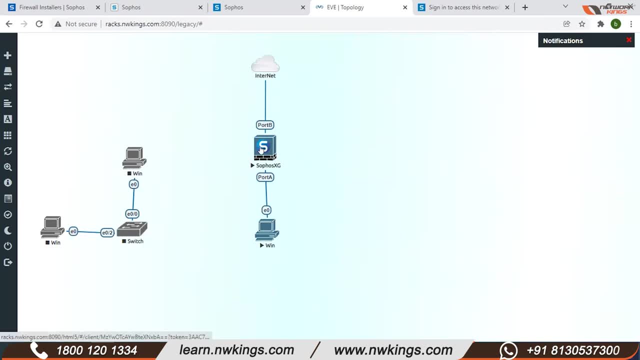 For example, on the branch office. if there is an AD server head office here, we will authenticate the branch office from the AD server. Of course there will be all the departments here, so we will login all the users. How? How can we configure different departments? 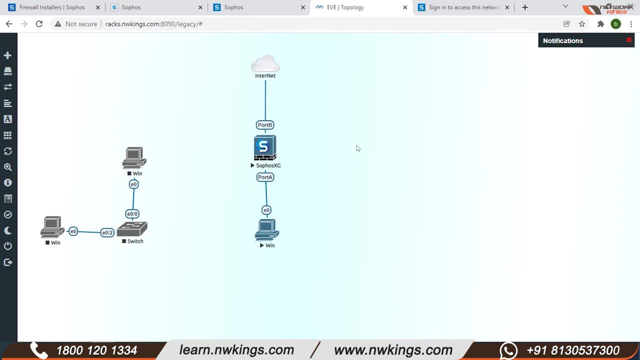 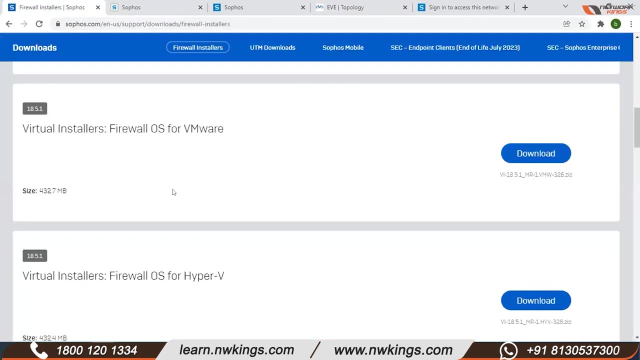 We will generate reports. We will see connectivity. We will see MPLAs. Of course, there are other features. like many people have it on SD-WAN. So how can we easily configure and manage SD-WAN from sofas? We will see that too. 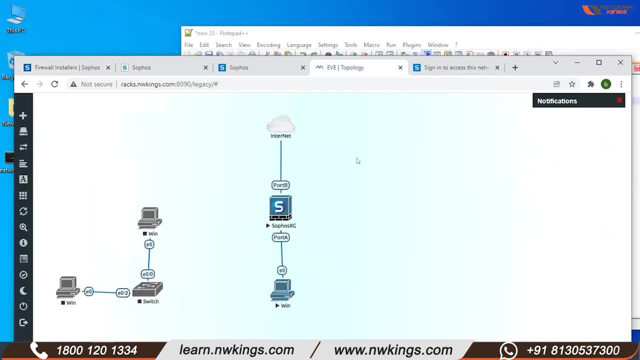 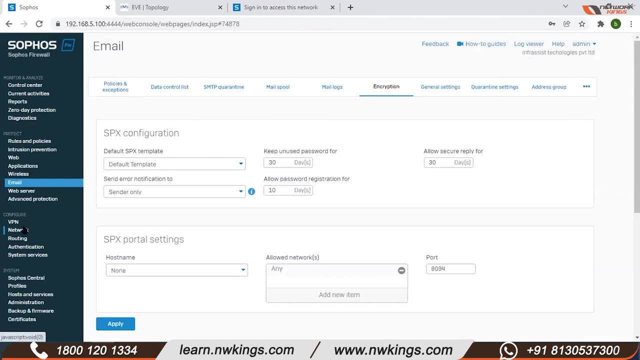 So this would be our topology. We will add it For now. I have added it to show you, Guys. any other questions or doubts? No, I think we have covered everything, So without further ado, let's move on to the next step. 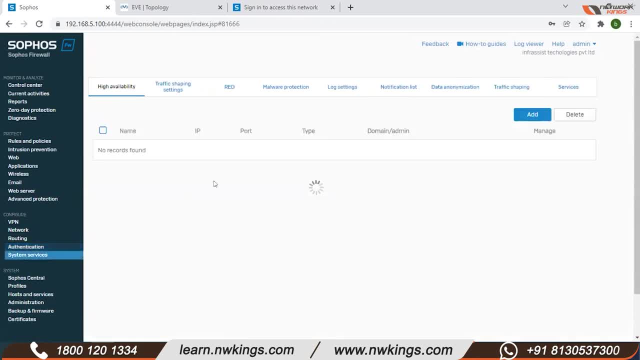 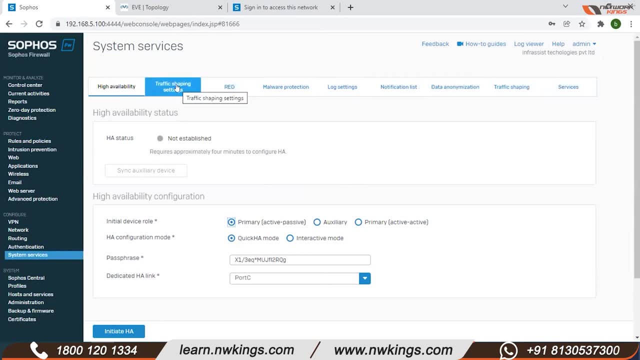 We will check the authentication. We will check all the system services in the modules. All the tabs here will be covered. We will configure and apply it to the users And we will see how it works. All these things are the same. We can enable logs on the file. 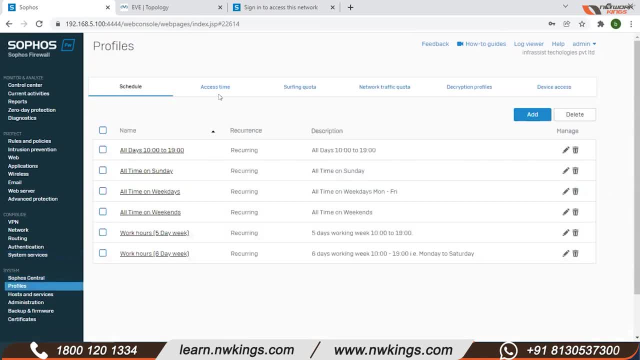 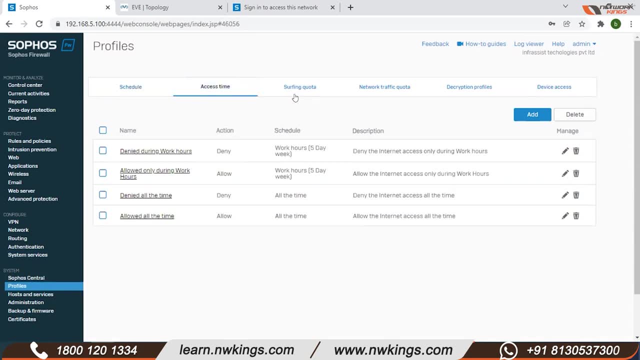 Red. So, for example, we will create profiles from the central. We will make profiles, that is, we will make schedules like Monday to Friday. users can access access time. some surfing quota has to be applied on a particular user. access time has to be applied. 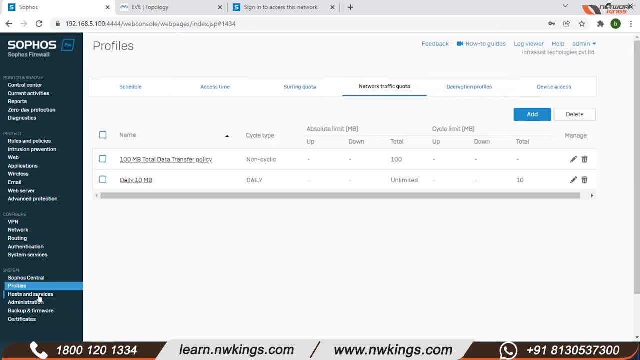 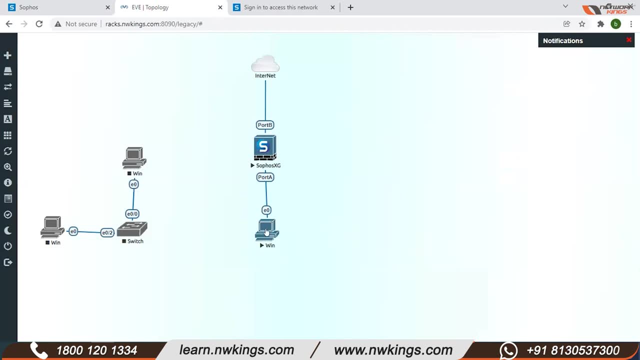 We will apply all these profiles one by one on the users and see in our network scenario. We will keep 2-3 PCs and after logging in the users we will see the in-out of all the traffic, how we can meet our business needs here. 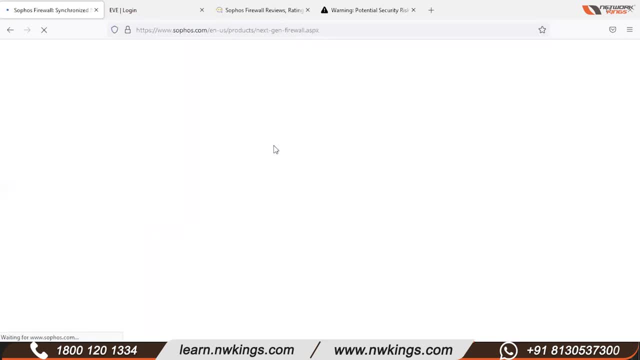 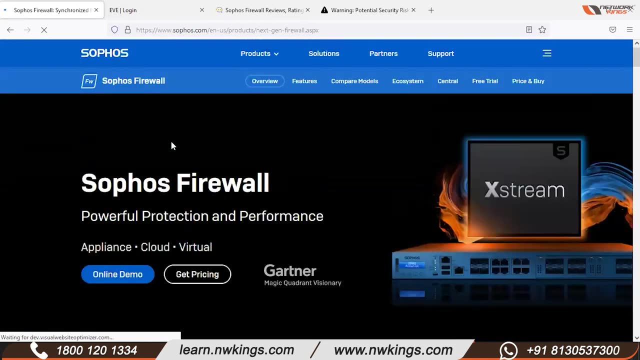 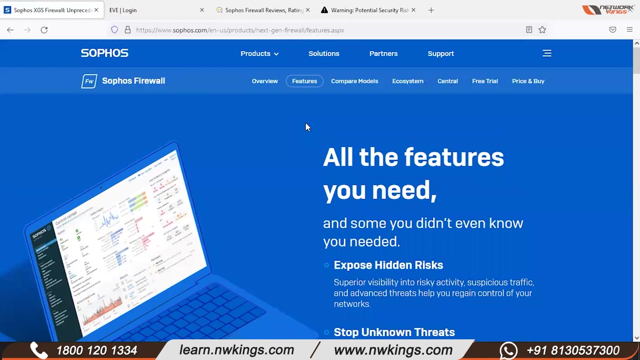 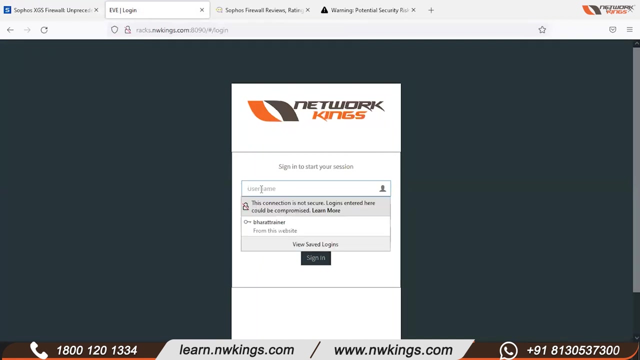 So, as we took an overview of firewall yesterday, so we will go through the Sofos website once in which we can configure all the features of Sofos XGK to meet the business need. so we will see those features once. Then we can have a look at our network scenario, which we will work. 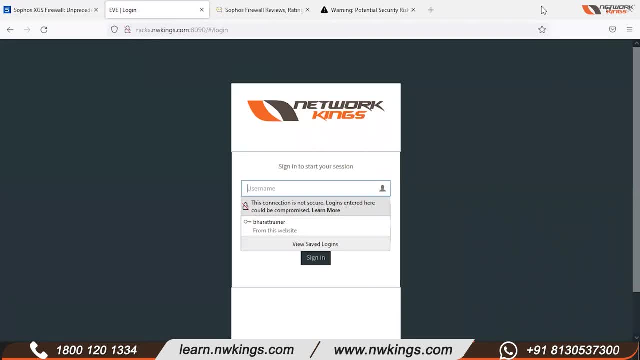 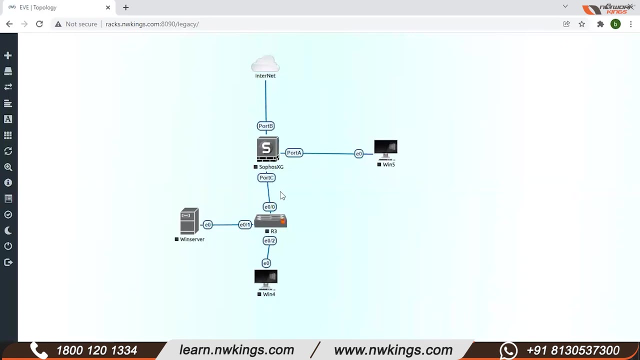 We have already created a network scenario. we will work on it, Okay here. Okay, Excuse me, let me show you that. Okay, So a typical network scenario will be where we will use Sofos firewall as a Git. 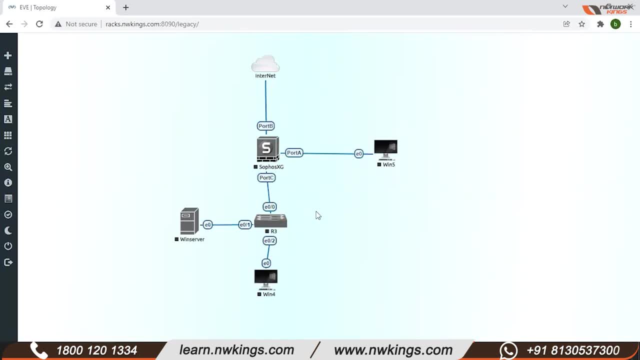 So here I have already created my network properties. We will go through it here after an overview of it, As soon as we discuss the agenda. of our course, we will take Sofos firewall access and we will see how to discuss it in the network topology. 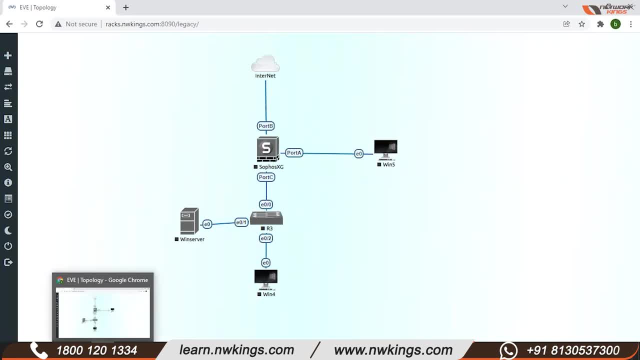 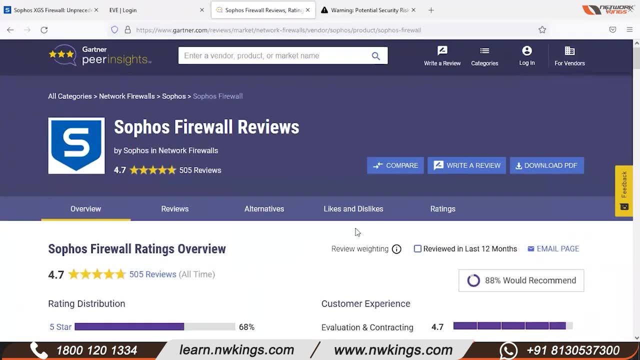 So after the website we will review a topology, All right. Then we will see, as per the Gartner where we will explore the Sofos reviews a little bit, That whatever business need we have or if there is an existing network. 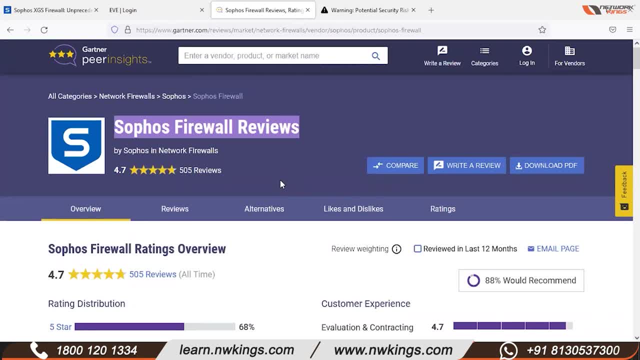 how can we deploy Sofos there? Which options are available? Okay, If we are replacing something with reviews, like an old router, and we want to enhance the security, Sofos is the best firewall we can deploy. So, as per the review and competition with other vendors. 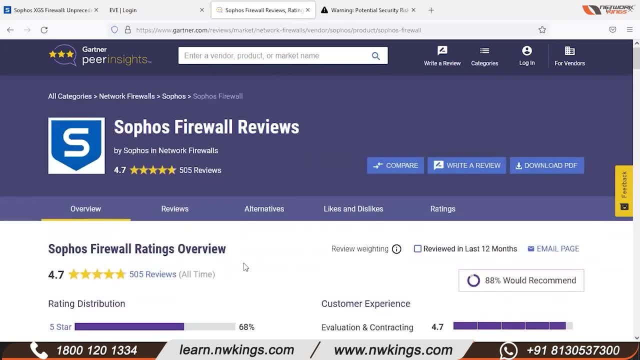 we will see how Sofos firewall enhances the security of the business. So we will also go through it once. So after that, once the agenda of our course, which we will start from tomorrow 8 to 9.. So we will see how Sofos's firewall actually works in the backend. 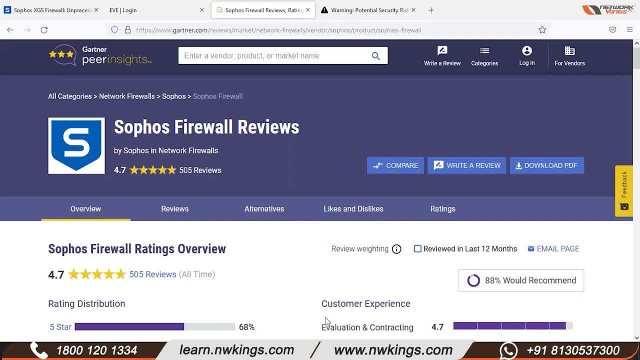 As well as with the installations and configurations, reviewing and troubleshooting. We will create different network scenarios in LAN And other connectivities like IPsec and MPLS, if we have any existing network connections Or if we have to replace an already existing network. 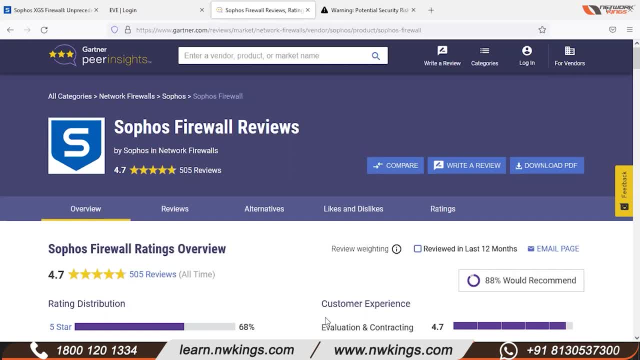 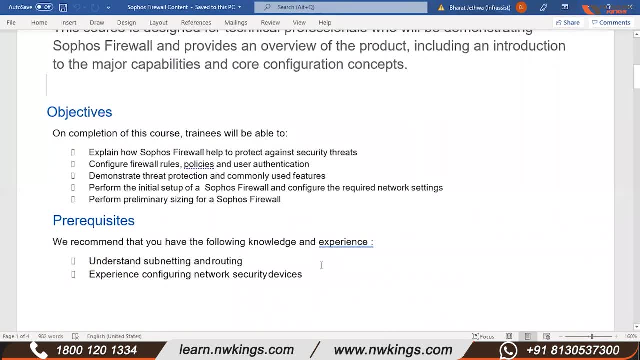 So we will see how we can do it with connectivity with Sofos. So let me just quickly go through the objectives, which are our objectives. So what will we cover in this course? We will explain how Sofos's firewall helps us to protect against security threats. 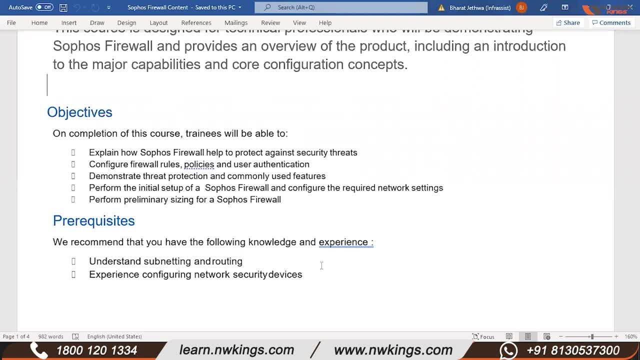 So how Sofos's firewall will currently protect day-to-day security threats. After the configuration, we will see that In the second point we will configure firewall rules, policies and user authentication. That is how we will configure firewall rules in Sofos's firewall. 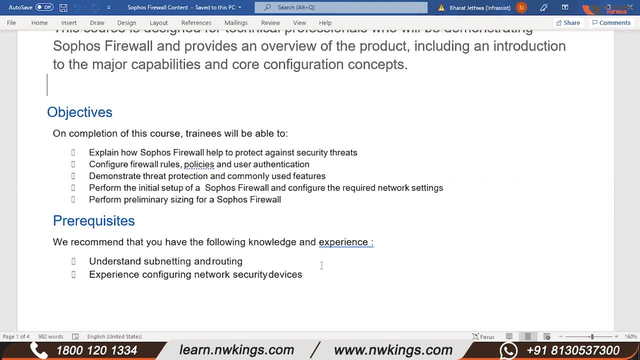 How we will make policies, Which policies are there- We will discuss that- And, of course, user authentication. That is how we will authenticate the user and apply policies on it, and how Sofos protects the firewall from end users for surfing any unwanted websites. 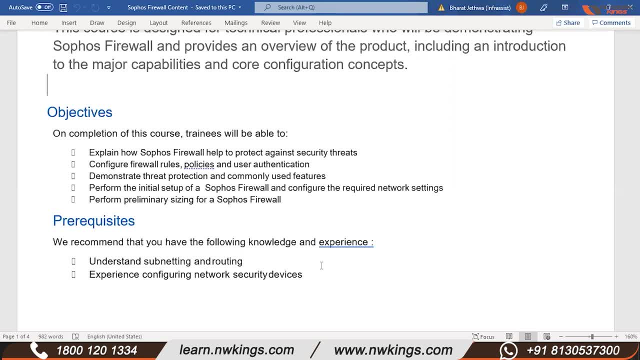 during the business hours, for example. So how can we meet the user who is accessing and authenticating? We will see that. Then we will demonstrate threat protection and commonly used features, All the threat protection features in the firewall which are common scenarios. 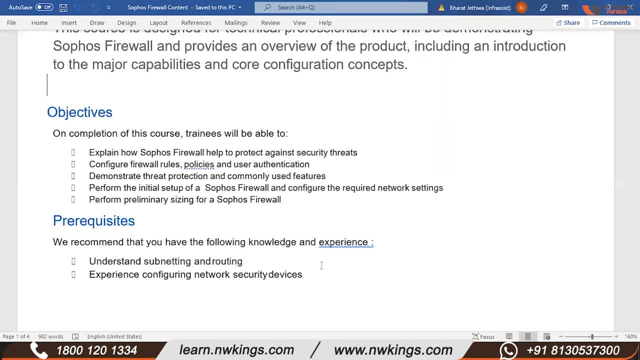 and given articles, we will configure them and create a scenario to see all the features, Perform the initial setup of the XGIF firewall and configure the required network setting. That is, we will install a Sofos firewall in all platforms, one by one. 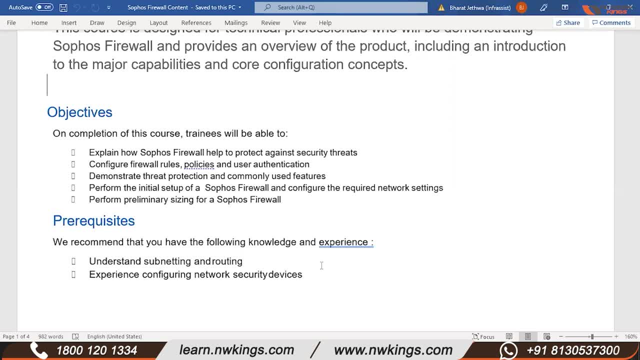 How to set up its initials. Generally, if there is a physical box that arrives, the initial steps, its initial settings, its initial setup in VMware, in any cloud platform- AWS, Azure, wherever the platform we are going to discuss in the future. 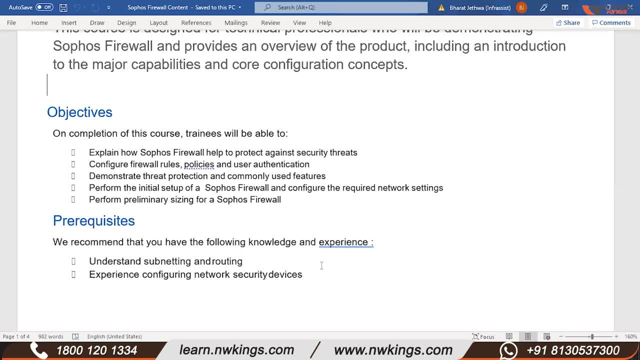 where we will deploy its initial setup and its configuration will be explored. Perform primary sizing for the server. If we have created our network with Sofos firewall, then we have to expand it right. So how can we scale it and size it? 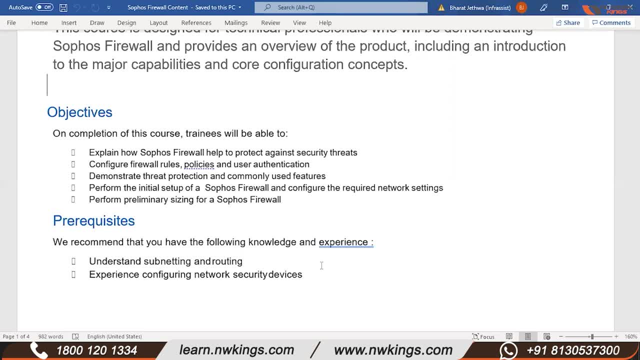 We will see that too. In Requisites only basic understanding of submitting routing, and if we have configured any network devices so far, it will definitely be easy to configure Sofos firewall. If you have configured, then how to configure the rest of the firewall? 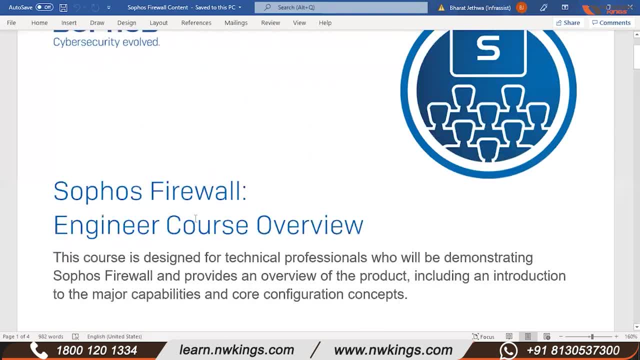 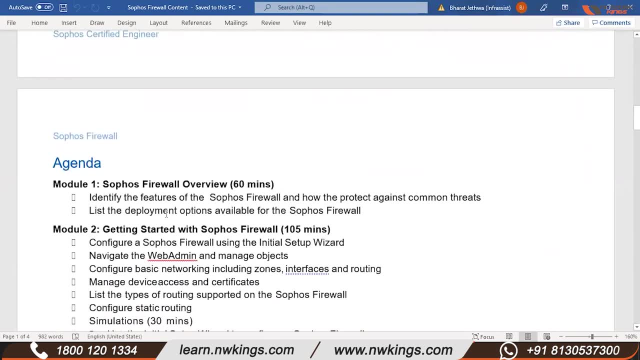 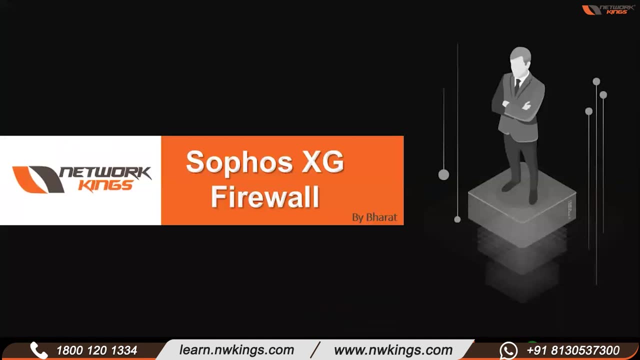 you will also get an idea. So for now, our objective will be this: I will share the objective and requisite in this document and the agendas in detail. So the agenda I will tell you in PPT first. After that we will give a brief summary. 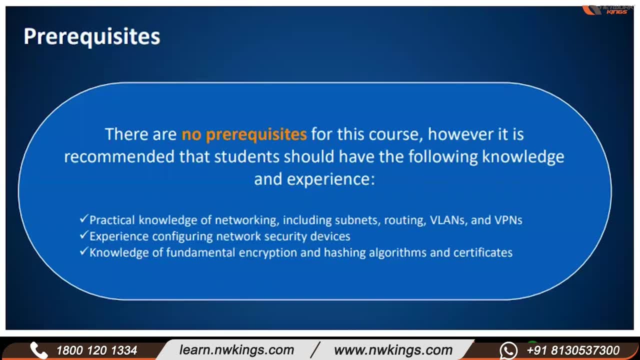 of this document. Okay, So, as I said in the prerequisite, the network scenarios we will create with Sofos firewall, how to deploy Sofos products in an existing business, how to configure or start with installation For that, how can we meet? 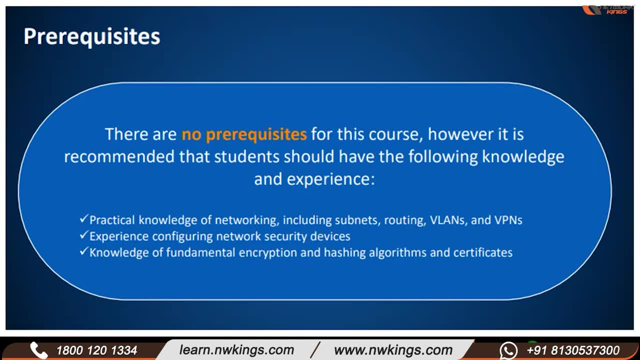 the requirements of the firewall Here. the prerequisite to configure basic practical knowledge of networking- where subnetting, of course, routing, VLAN, VPN. then experience with configuring network security device. If you have configured all these features then you can enable. 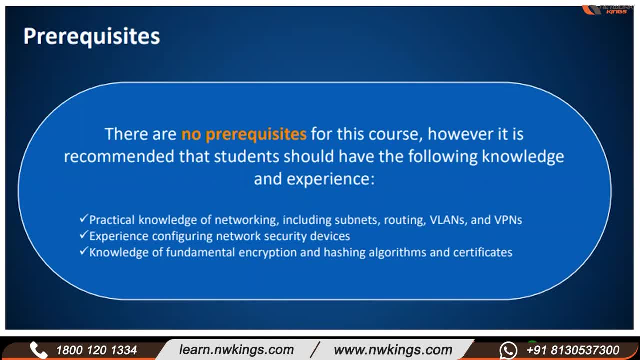 all these features to meet the business needs and its security. related things And fundamental knowledge about encryption, hedging algorithm and certificate will be plus one. Along with this module. we will discuss some basic things like subnetting, routing, how to configure RF, 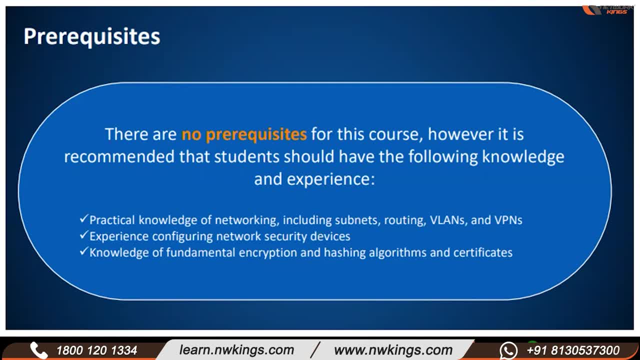 BGP static route, BGP RIP, VLAN. We will definitely discuss those scenarios in the discussion. No issues? So how will we do the same with firewall? We will discuss all these things. For example, I have told you: 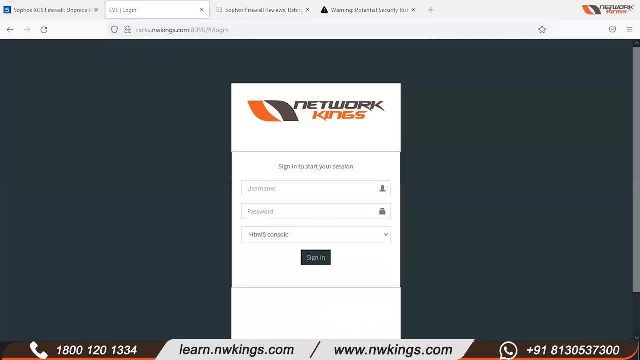 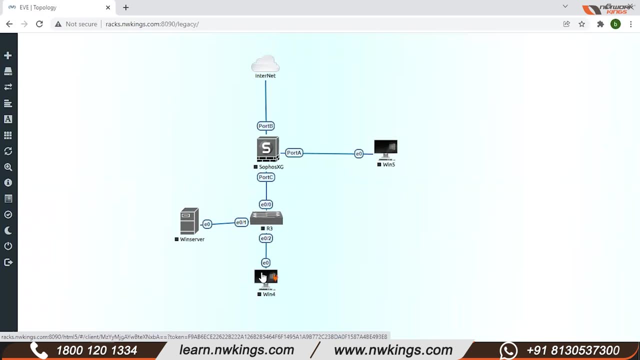 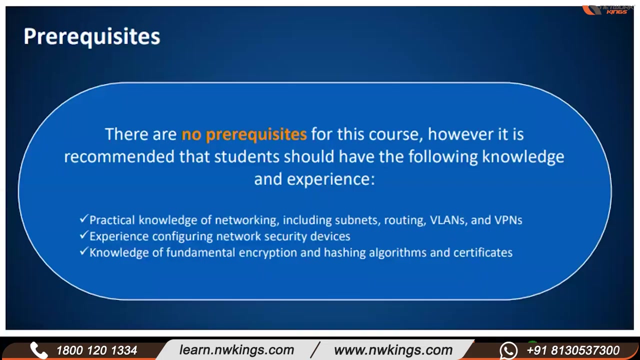 the scenario for a LAN network, For example, if we want to connect any branch office, we will go into details, but for now we will discuss how to protect LAN, DMZ or any other zone. So let me just go back to. 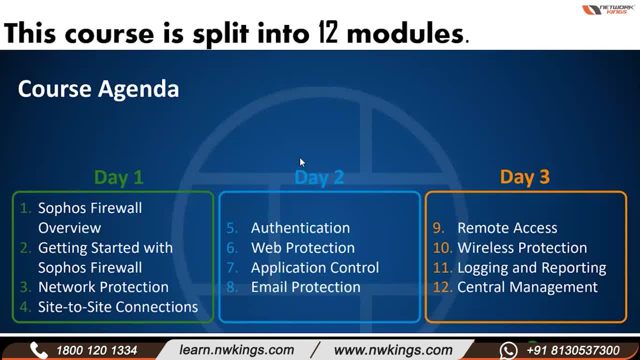 these two slides, So our course is divided into 12 modules. We will go through each module in brief. For example, the overview of firewall: all the features and existing business can be protected from malicious activities. How can we protect hackers? 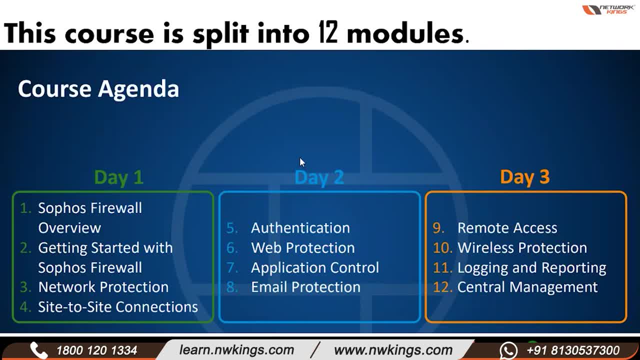 pinterest vulnerabilities. So how will we meet with the first firewall? We will go into overview. After that we will clear out the basics in the first firewall overview. After that the second module is getting started with the first firewall. After that: 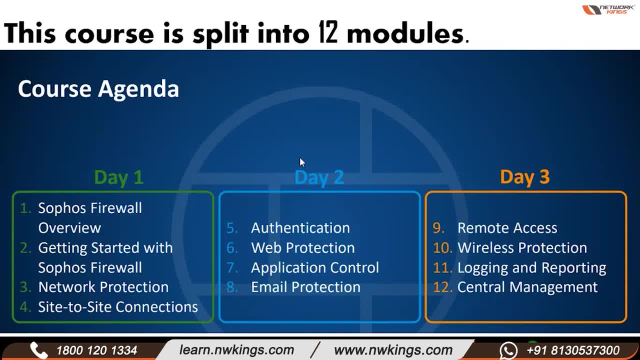 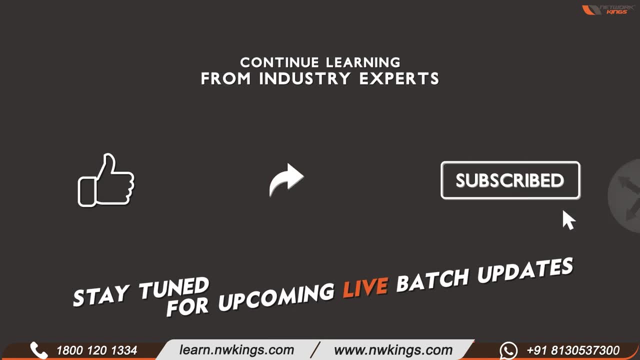 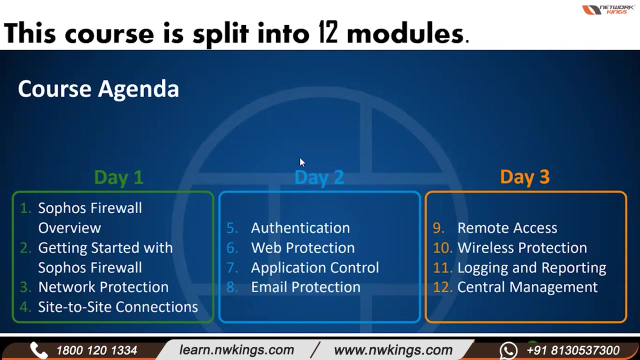 the third module is getting started with the first firewall. After that, the third module is getting started with the first firewall. Then let me just dig it out, the module first. We will verify the module first. The fourth module is site-to-site. 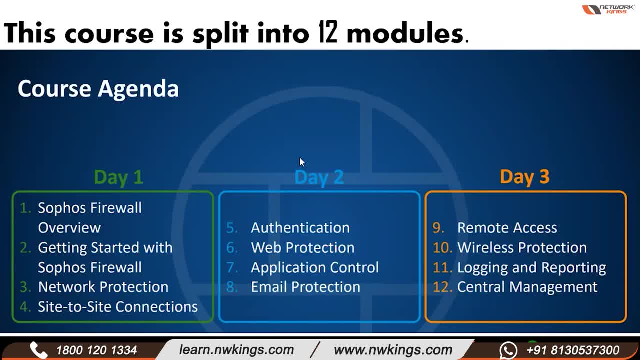 like IPsec, for example. Then we will go to the fifth module, which is about authentication. After that, in the sixth module, we will cover web protection. In the seventh module, we will cover the wireless protection In the eleventh module. 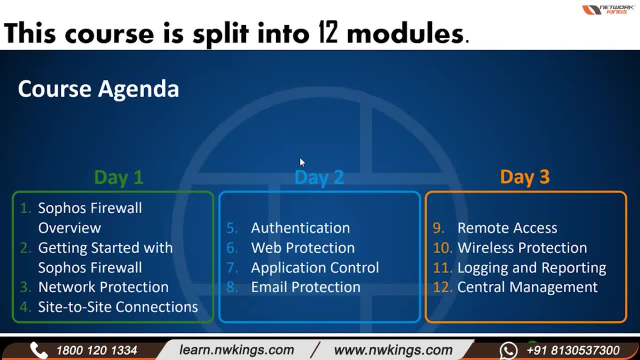 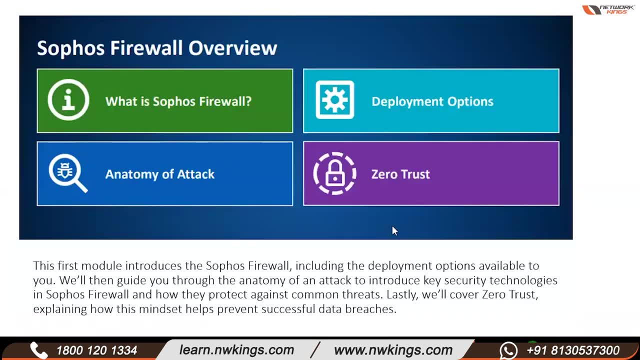 we will cover the login and reporting sessions. In the twelfth module we will cover the central management. As I told you, we will meet all the objectives, like the first firewall overview, deployment options, proxy and so on. We will see. 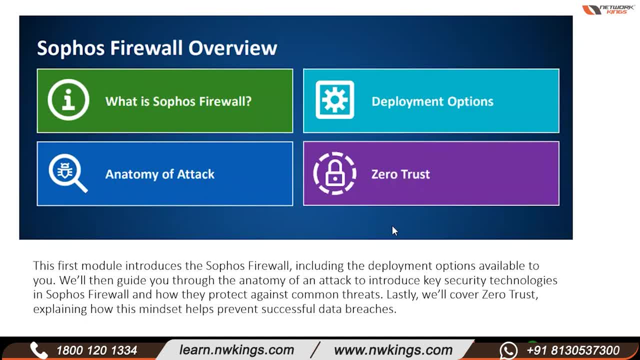 the deployment options in the first firewall. Then we will see the attack on an organization like ransomware or malware. We will see how to protect hackers from the attack. We will see where the attack will play a role in stopping, detecting and taking action. 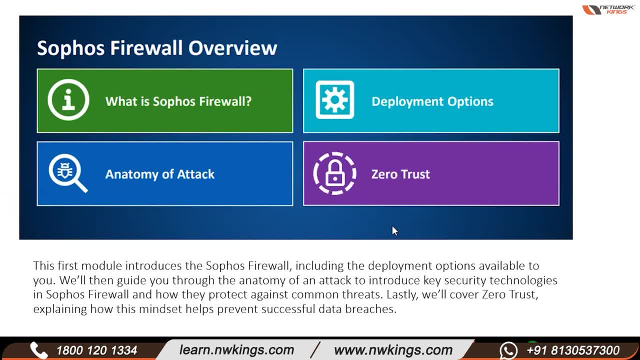 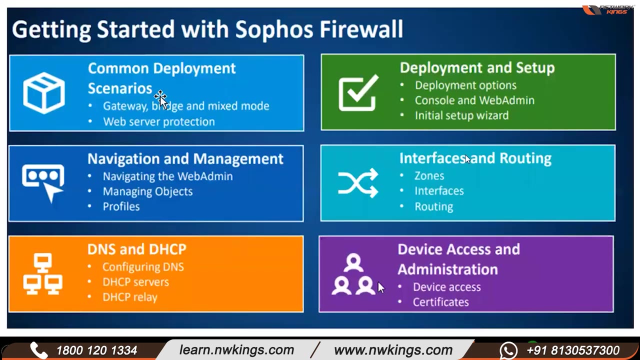 We will see that too. There will be zero trust in the overview. Zero trust is generally allowed in the organization, But we will go into detail. This will be the agenda of the first module. The agenda of the second module. I hope everyone sees the slides. 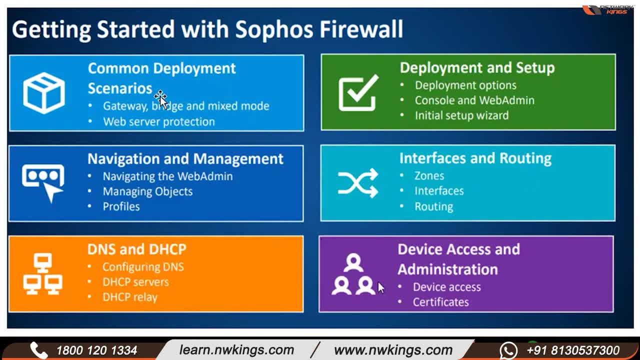 Getting started with the firewall, we will see the common deployment scenarios like gateway, bridge, mixed mode, web protection. We will see how it works in different scenarios like bridge and gateway. We will see how it works in your existing network or the new network. 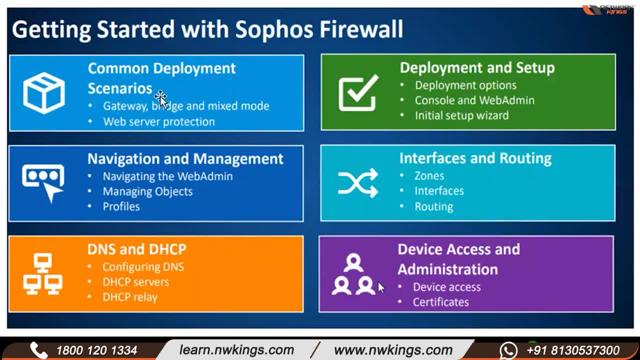 for example. Then we will see the deployment and the security of the console. We will also see the web admin and the initial setup of the firewall. In the same module. we will see how we can navigate the web admin. the object: 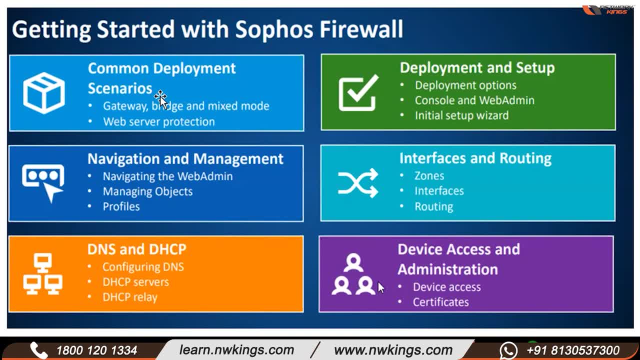 the profile, the interface and the routing zones. We will see the routing in the firewall. Then we will see the DNS configuration and the firewall access. We will see how we can securely distribute the administration rights of the firewall access In the third module. 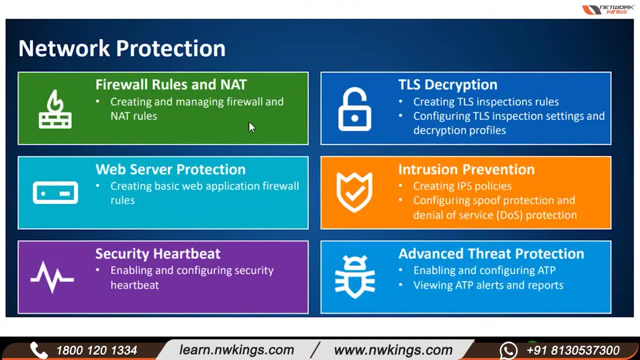 we will see how to configure firewall rules and how to forward the port. Then we will see the TLS description. For malware protection, we will use Sofos Firewall for malware protection and threat detection technologies. For TLS description: we will use HTTPS scanning. 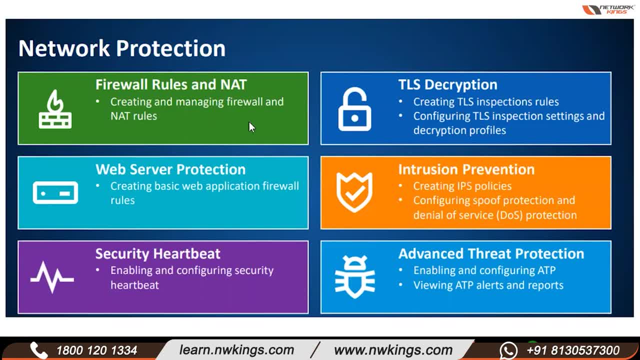 and certificate, along with the practicals. Then we will discuss web protection. If our web protection means that the server is working on ATP or 443, how can we protect it without port forwarding? We will see how to create HPA policies. 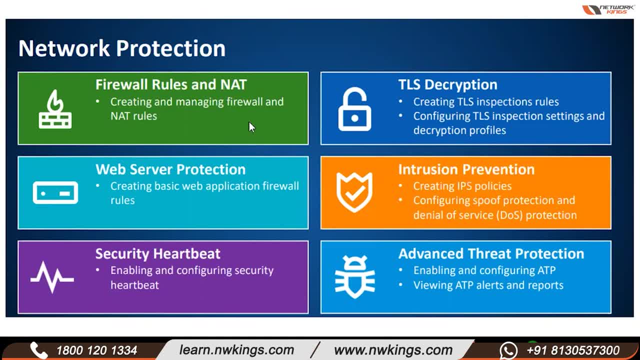 how to use existing defaults, how to enable spoof prevention and risk protection, what are the requirements? how to configure exactly? we will see that. We will also talk about how to configure the security of the web. We will also talk about new technology features. 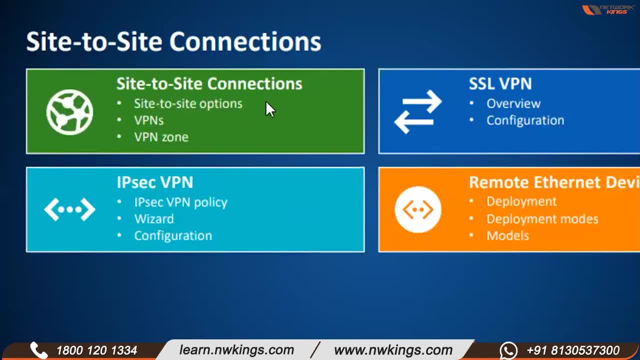 How to enable advanced threat protection, how to clear alerts, how to generate reports. we will see that in the third module. In the fourth module, we will see site-to-site connections, like site-to-site options, available. We will also talk about how to configure. 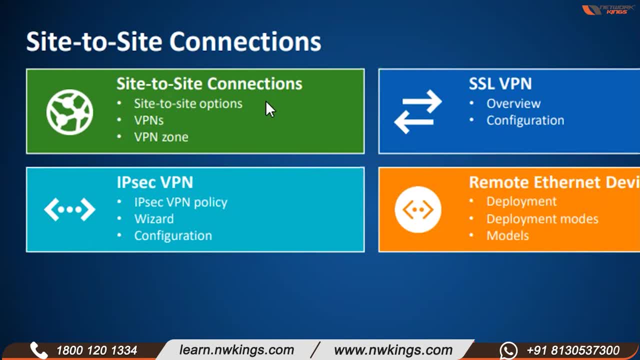 IPsec, L2TP, PPTP VPN. Then we will configure SSL VPN, which is, of course, for the remote users. How to configure IPsec, IPsec, IPsec. how to configure IPsec, IPsec, IPsec. 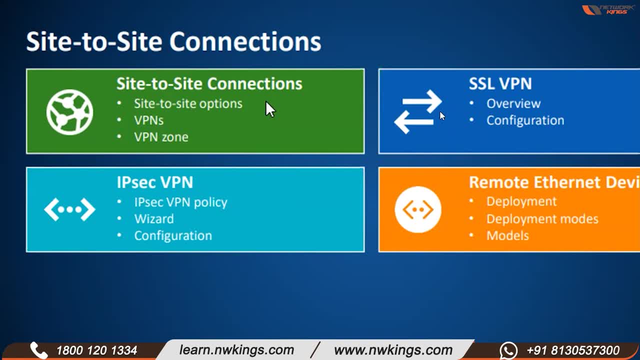 IPsec, IPsec. what we can do is to configure IPsec, IPsec, which is the product of Sofos, as I told you in the last webinar how to flow its traffic. We will see that in detail with models available. 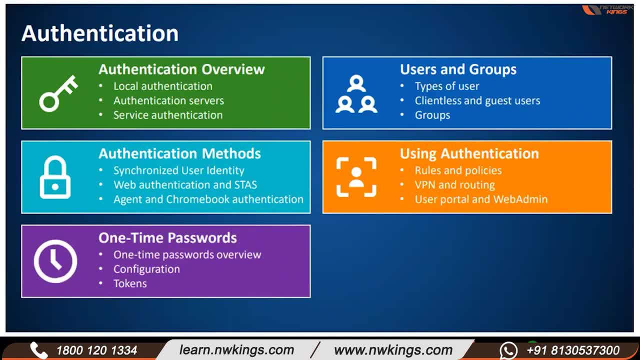 Our fifth module is authentication. We will see that that is how we will enable the authentication on firewall. We will see its overview. How can we authenticate? by creating a user locally, For example, username, password and internet access, So we can do it locally. 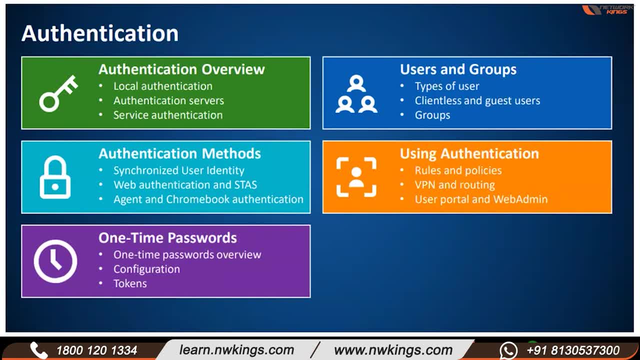 Or third party, like ADE server or any other service authentication, How to integrate it with Sofos firewall. We will see that User and group. if we are creating locally, for example, how to make a group of that user, We will create client-less users and guest users. 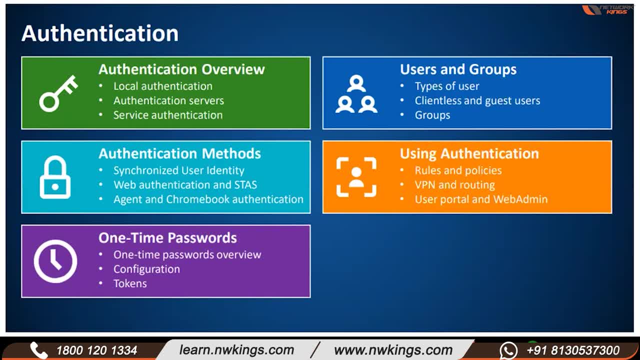 Client-less users. for example, if there are printers, for example, how will we count them in the user? It has a separate configuration with guest users And group In the user group. if we use ADE user, for example, in authentication overview, which is the second point, for example, 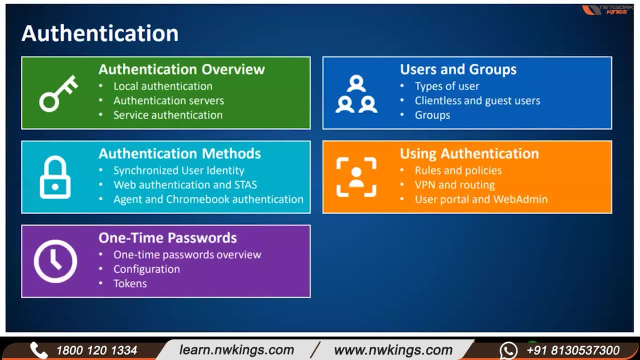 So how to import the user group from that? We will see that too. Then what are the authentication methods? We will see that too. Synchronized user identity like ASTAS. If someone like ASTAS, then generally like the windows environment where currently, if you have all the windows pieces, 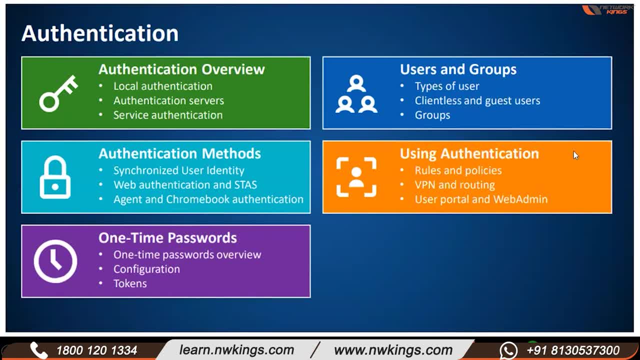 So if users have any particular, that is, multiple, authentication methods, we have to eliminate that. So how do we enable automatic authentication, Like windows login, or if there is a Chromebook, for example, Or if there is an agent, then how do we do that? 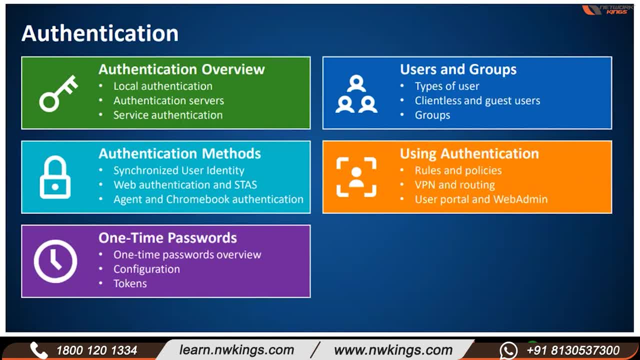 We will see that By installing the clients and PCP we will do it. How to make the authentication automatic? First we will do it manually, then we will do it automatically Because it meets the requirements. Then, using authentication like, we will create firewall rules, policies for authentication. 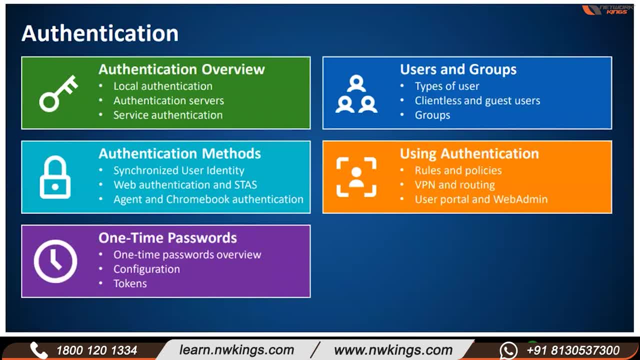 We will fine-tune it. We will do VPN settings- How to give authentication in VPN And VPN and routing, of course. Then there is a user portal. there is a web admin- How to get it authenticated in that. We will see that too. 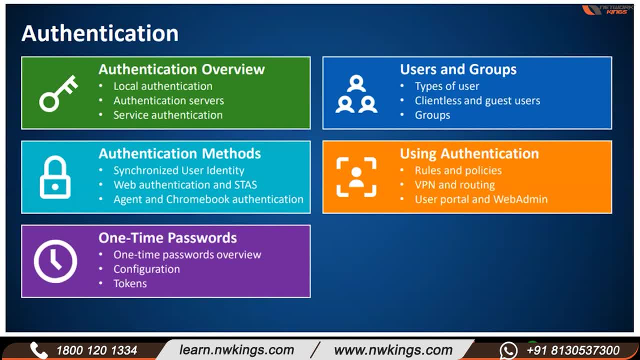 One-time password. This is also one of the features. Generally, if you have any guest user, how can you generate a one-time password? Can you generate tokens? Can you generate transactions in the file? We will see the configuration. We will configure it. 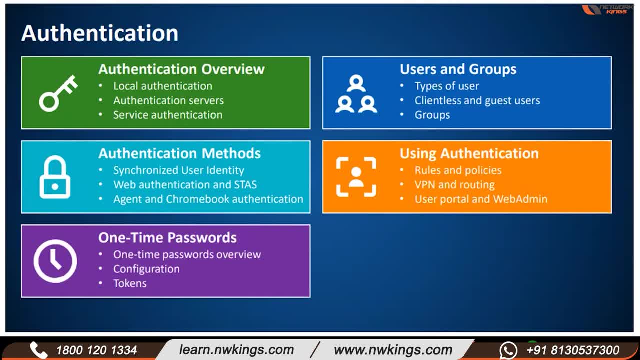 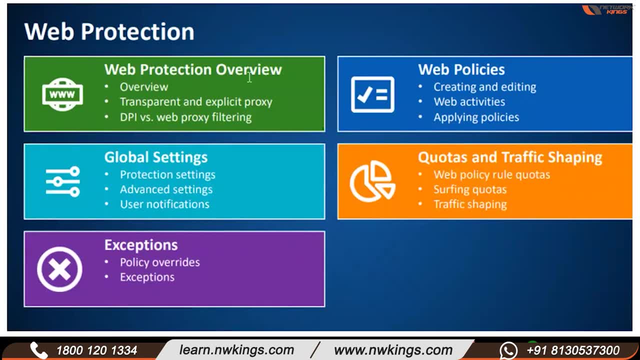 We will generate tokens And we will give temporary access to the guest user according to the policy. Then on the sixth module, we will cover up the web protection Generally. almost all users access the internet from browsers. How can we protect it? 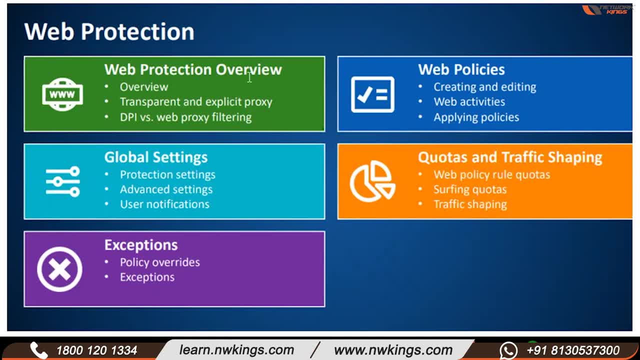 There is web protection. We will see that. In that, we will see the transparent and the proxy- Exploited proxy. Then DPI, Deep packet inspection. As I told you, we will install the HTTP scanning and install the certificate. We will see that. 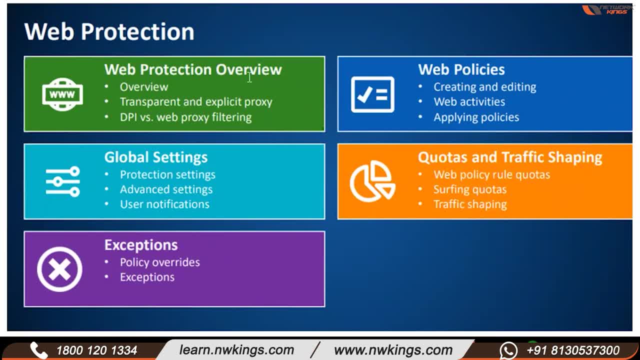 And we will know the difference. What is the difference between DPI and the web proxy filtering? How does it work? We will see that with packet capture. Same way with the web policies. We will create policies So like we will make some policies in it. 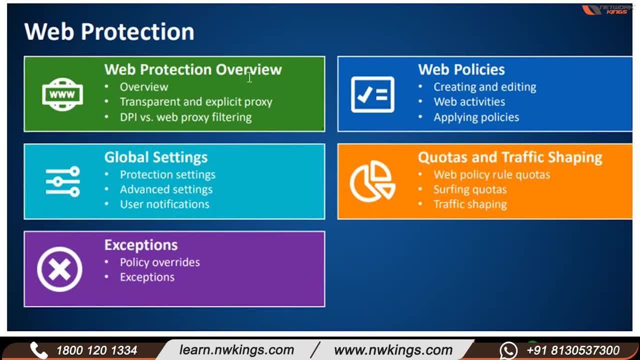 Apart from defaults also comes. So we will go through the defaults once And after that we can create or edit any custom categories. We can apply policies. We will see about this. We will review global settings In that which are the protection settings. 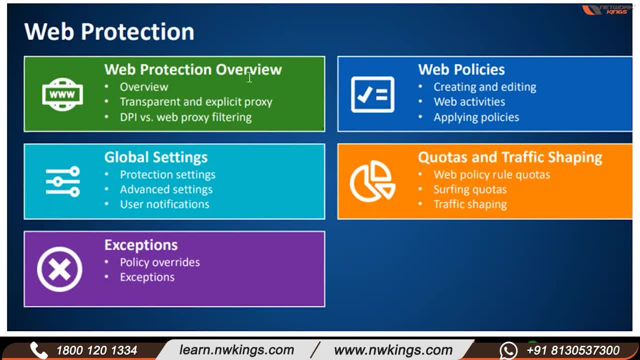 When to enable, When is its requirement And where. We will see that Same way with the advanced settings and user notifications, Which comes after the web protection Quotas and traffic shaping. Quotas means data. The user needs policies. Again, these are policies. 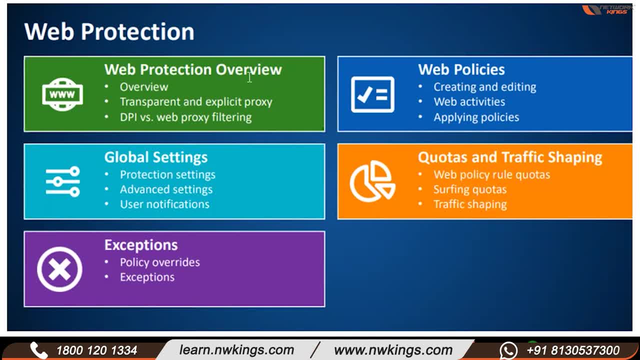 So in policies we will create surfing quota and bandwidth And we will apply it on the user and check whether they are working or not. Okay, If there is any exception or we have to override any policies, we will see how we can do that. 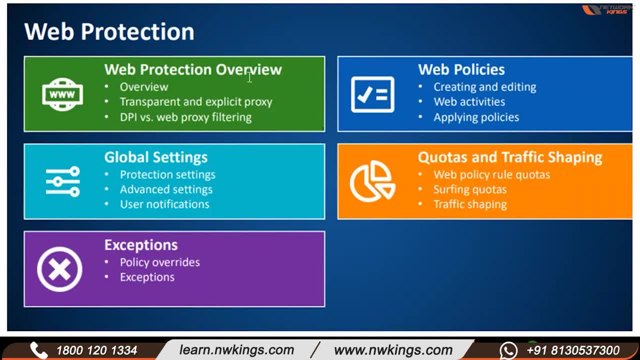 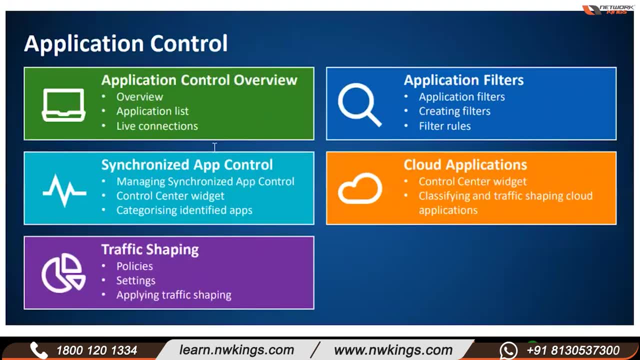 If policies are applied and we have to bypass any particular user. So during the business hour we will see how to temporarily investigate and put an exception in it. We will see that Same way In the web protection. we also checked that we have the access to a full management of traffic. 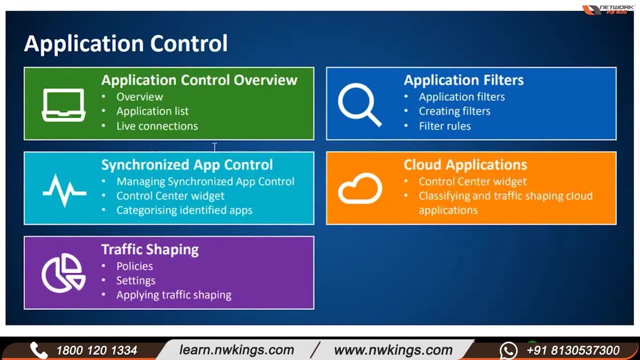 So what we will do here is: We will take an overview, Then we will see the policies that are provided in the application control. Okay, So in application control we will see the application filters And we will look through the application filter policies. 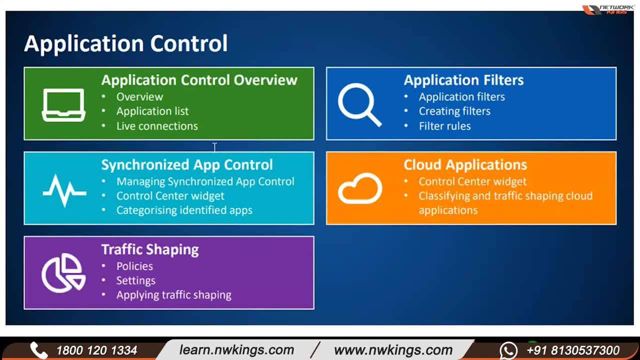 and we will create the new ones in the lab along with the modules. How will we manage the new feature of Synchronized Security in the Sophos Firewall? We will see that. How can we control and categorize the control center? We will see that. 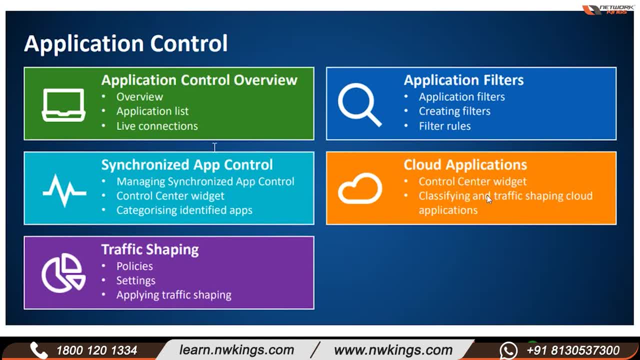 Similarly with the cloud application. how can we manage the cloud application from the Sophos Firewall? We will see that, Again, we can apply traffic shaping policies in the application as well. We will see how to create policies and what are the settings. 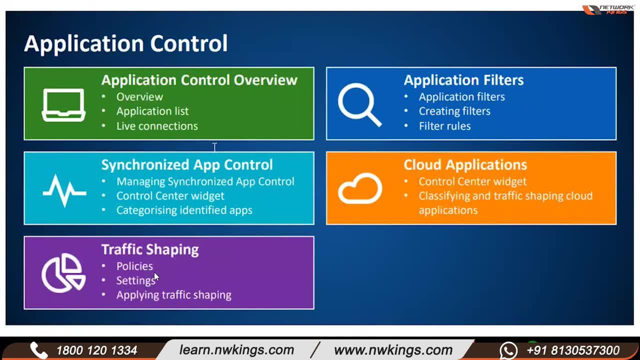 We will see where we can apply it. Like, if we want to give a bandwidth policy, if there are streaming media applications, we have to restrict it. We will see how we can restrict that policy in the application control. Okay, Next would be email products. 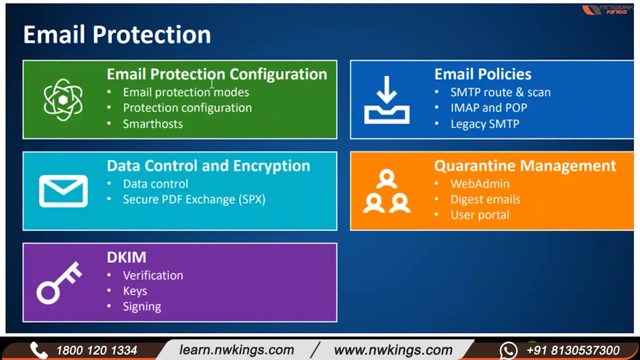 We will see the protection. Sophos XG also offers email protection, For example, if there is a spam mail, if we have a mail server on port 25, or if there is an SMTP that is working on SMTP-S working on POP. 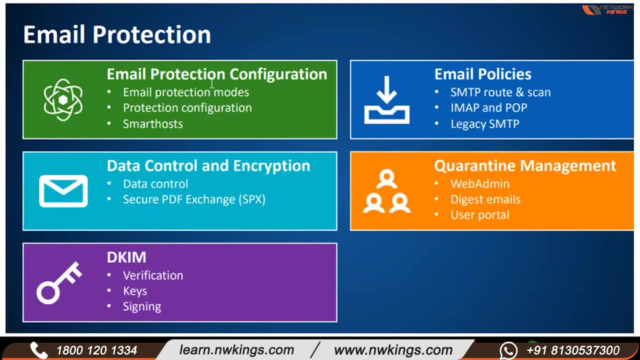 working on IMF right. So how can we protect it from Sophos XG? We will see its configuration once In the user's PC. for example, we will configure Outlook and see how we can intercept mail traffic from Sophos XG. 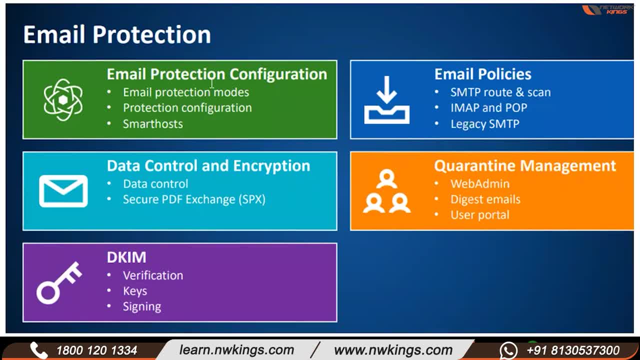 So we will see in email protection. what are the email protection modes Like MTA mode. Sophos XG also works with MTA mode And Legacy mode also works. We will discuss about it along with our module. No issue, As soon as we discuss MTA mode. 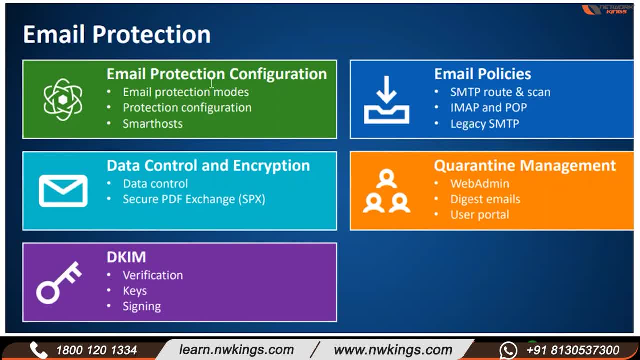 everyone will be able to sync. And let's see, if we haven't done SMTP, then how can we use SMTP protocol? We will discuss this in between IMF, POP and the rest of the protocol as well. So in that we will see protection configurations. 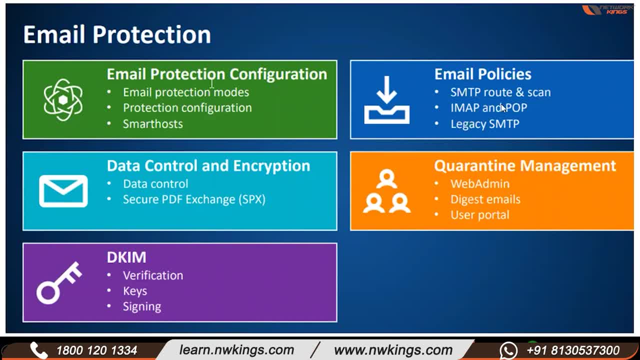 We will see what features are there in the smart host Policies that we can route and scan, which is our traffic, as I told you, IMF, POP and SMTP. we will see how we can intercept it. Then, if there is an email, 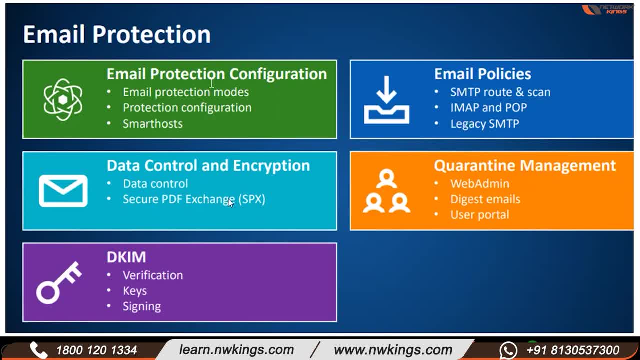 in that there is a data control and encryption feature, In that, for example, there is a secure PDF exchange feature, How to enable it And how can we use it, For example, in our first module? all your doubts will be cleared. 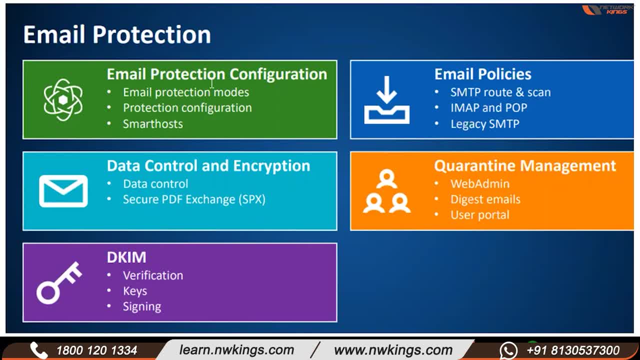 You will find my agenda a little bit fast, But definitely we will clear it one by one, All the features. most probably we will use all of them and see how we can do it. So, for example, there is data protection encryption. 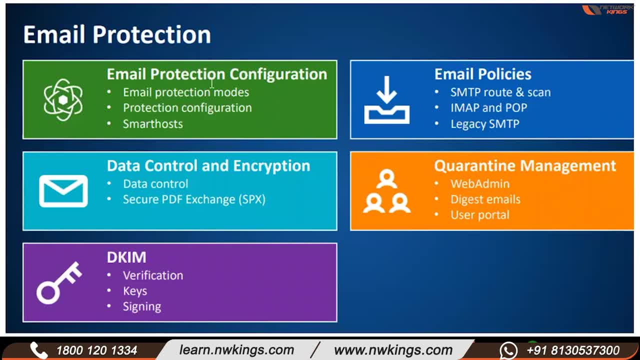 If there is a suspicious PDF in the email, how can we scan it? Or we are sending a PDF, how can we encrypt it? We will see how this feature works by encrypting it In the same way, if there is an email quarantine. 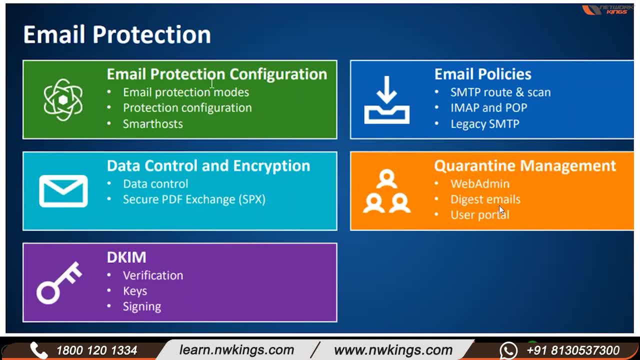 how will we manage it? We will see it through web admin Or we can do it through three ways. We will see the admin portal, the user portal and the digestive email, which are the logs in Sophos. We will go there and see. 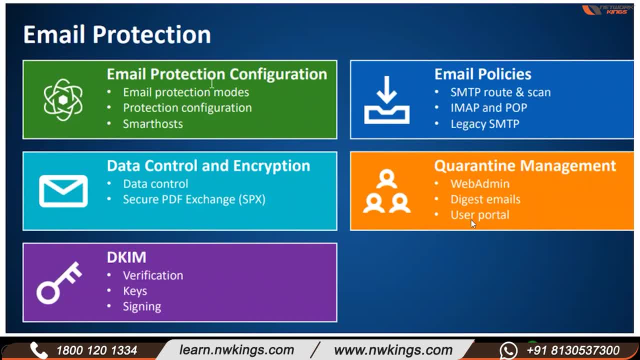 For example, the email has been quarantined. It is legitimate, So we can tell the user that you can release it from there, For example. Or we can do it through the admin. In the same way, we will see the DKI verification. 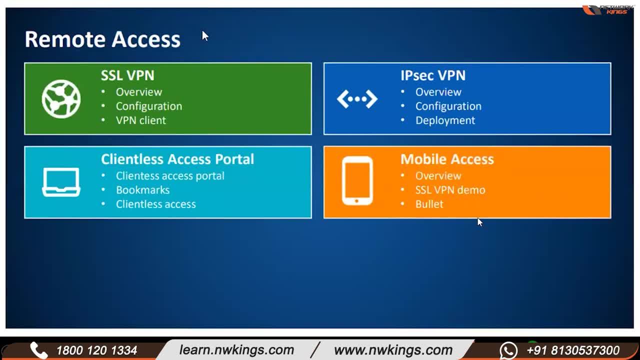 signing and encryption method. We will see it here. In the ninth module we will see remote access. We will see how to configure SSL VPN, how to configure IP, client-less access and mobile access, For example. we will configure SSL VPN. 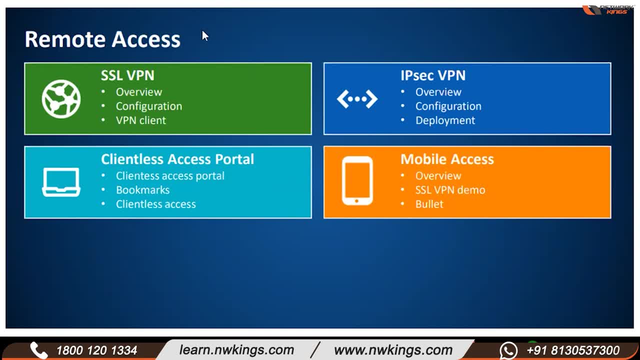 Then we will configure and set up how to access our remote server from outside. For example, we will do configuration on firewall On the client side. we have to download SSL VPN From the user portal. we have to install it, enter username and password. 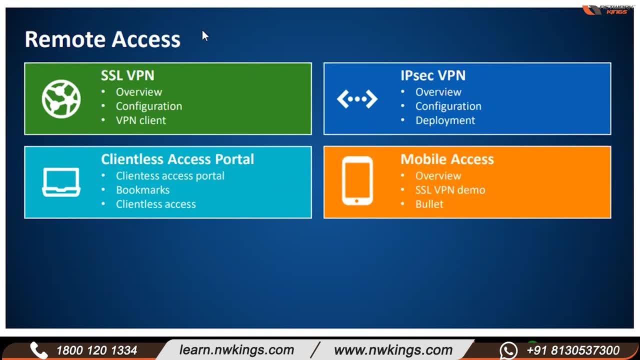 and you will be connected. Then how can we guide that user that you can access your server In the same way? we will see IPSec. We will take an overview of it. What are the options available in IPSec? What are the configuration scenarios? 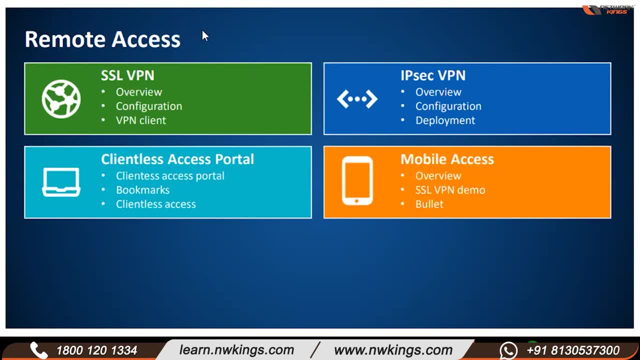 We will see that with deployment In the client-less access model. we will see how we can put a bookmark If there is a client-less user, for example, bring your own device- how can we configure it? How can we configure SSL VPN on mobile? 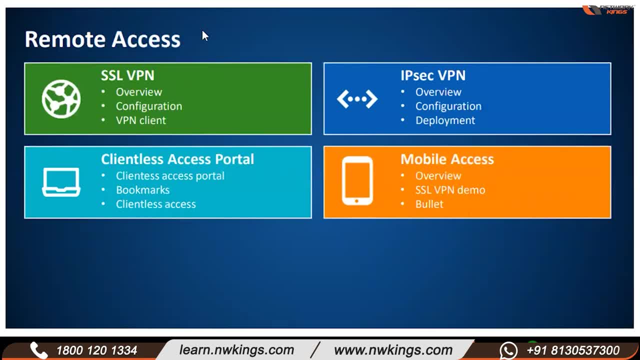 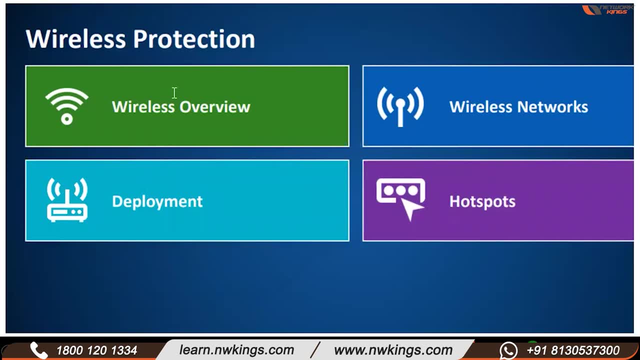 We will see that. If there is a third party device, how can we configure SSL VPN on it? We will see that too. In the 10th module we will cover up wireless protection. When wireless protection comes here, then suppose XG firewall. 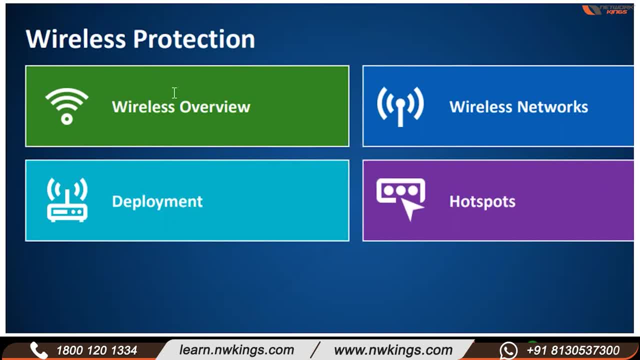 wireless protection, that is, it protects it from any unknown threat. So here, if you want to do wireless protection, then you should have the AP of Sophos. There should be an ecosystem of Sophos, So there is also wireless protection in it. 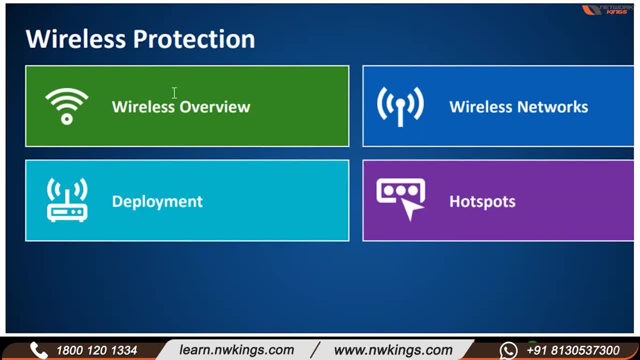 About it? how are its models? What features are available? How can we configure it in firewall? How can we protect it? Like a user is coming from outside and is connected to Wi-Fi, So how can we keep our network configured? 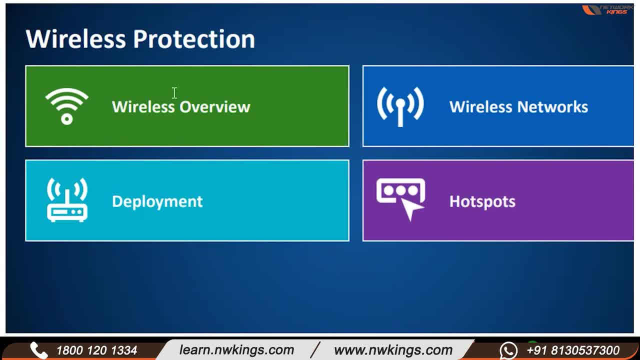 secure, As well as if the user is infected, how can we isolate it? So we will see that with wireless protection. So we will take its wireless overview first, Then we will check the wireless network which options are available. 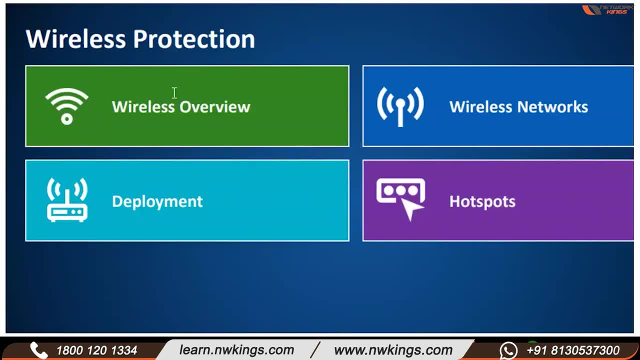 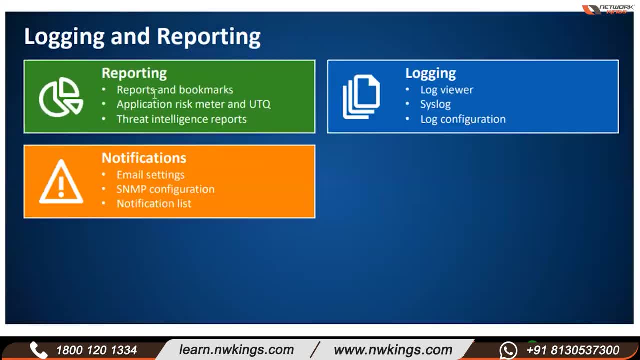 How can we deploy it? We will see the deployment mode. How can we deploy APs? Okay, And we will create a hotspot, Okay. After that, in the 11th module, we will cover up login and reporting. So 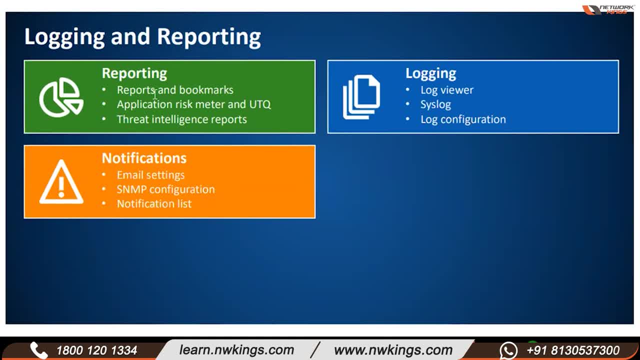 in reporting. we will see how to see reports through firewall And if we are seeing any report, then how to bookmark it. Okay, Application this meter. we will discuss that with the UTQ. that is User Threat Quota. 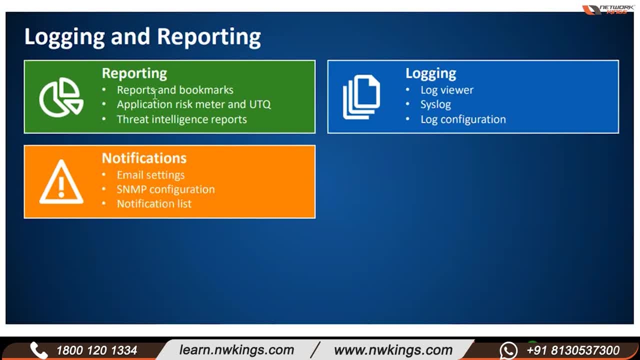 Which users are there, Which are the top users, For example, if anyone is accessing the website most vulnerable. okay, we will see about that. Threat intelligence reports about that. that too, we will discuss in the previous module first. 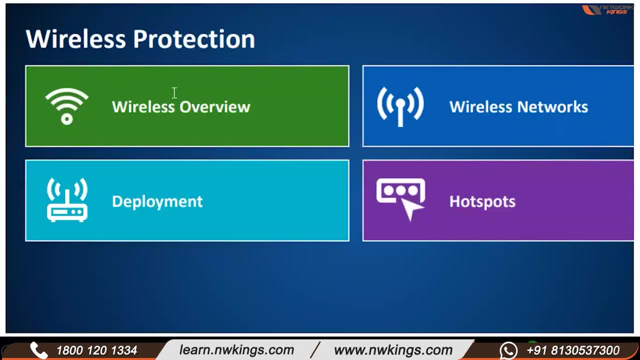 Okay, I was discussing about wireless. How can we enable wireless protection With Sophos AP? So we will see its overview. How to do configuration, We will see that, Okay. How can we set up the network With deployment and hotspot? 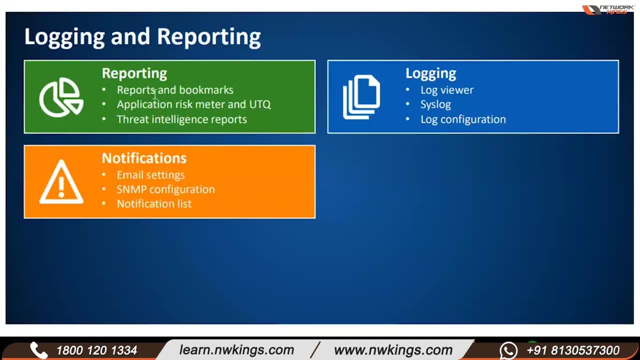 So with the 11th module- login and reporting- we will see. So how will we do with Sophos Firewall? So login and reporting is the also one of the great feature. So to dig down the what's: 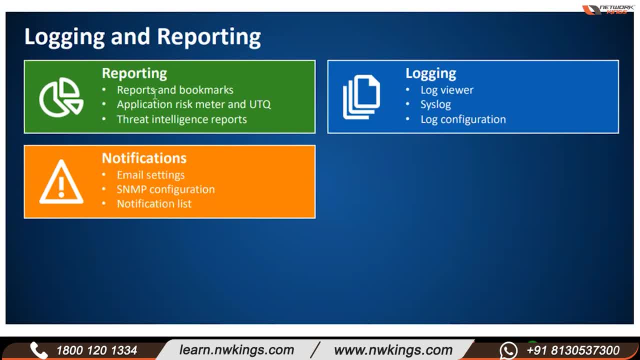 what activity is going on in your network? What kind of activity is going on? Okay, If there are any threat incidents, how to report it? Okay, If there are any users who are accessing an unproductive website, okay, as per the policies. 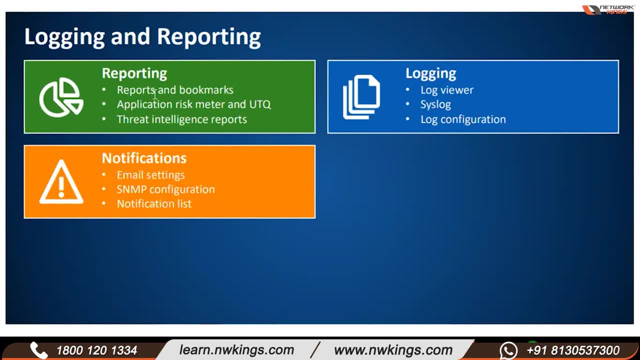 then how do we bookmark it? Okay, So we will see about that. So we will see about that. So how can we bookmark it? We can generate regular reports through mail notifications Over email. We will see all the configurations. 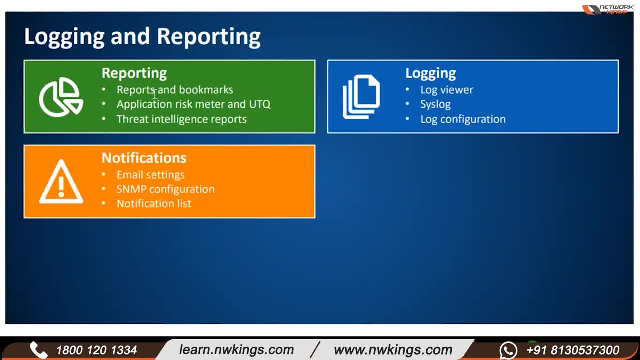 So in that, yes, of course there is logging. So we will see LogWear Firewall. We will see LogWear In that. generally, all the logs will be found In the system application web filter. 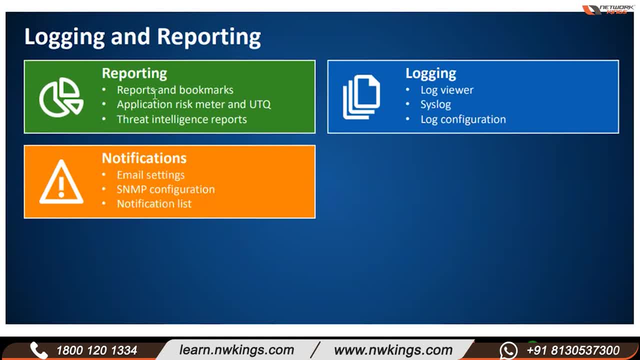 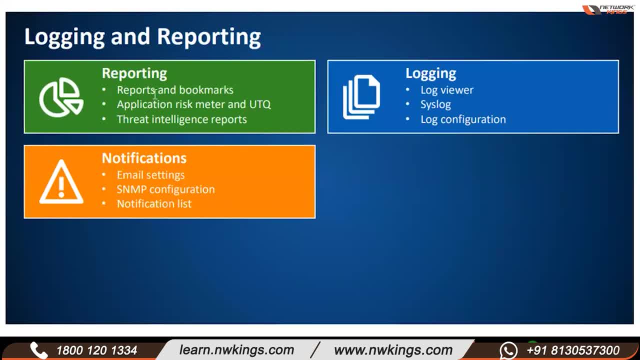 like Sofos's iView In that we can separately save the logs. So we can do that with LogWear As well as. yes, now there is another feature: We can also save it in the cloud. So 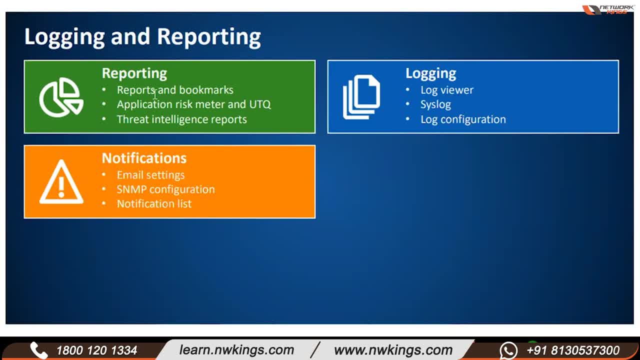 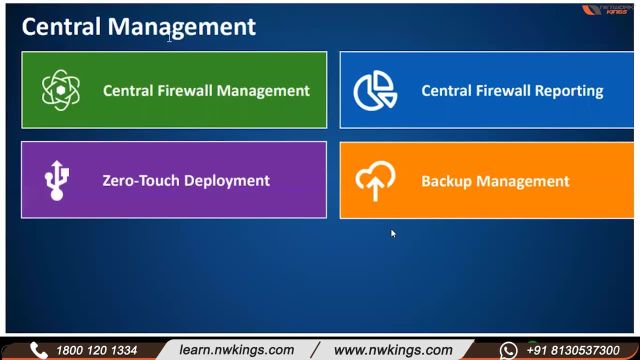 we will also provide all these features in our level and environment when we do 11th module of configuration. So we will see all these features one by one, So log configuration as well. Lastly, the 12th module will be from central management. 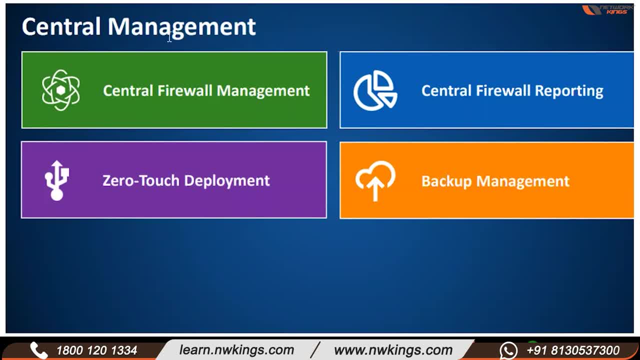 What we will do. Sofos's console, Sofos central, will cover. we will connect it with the software firewall. How can we manage the software firewall from the software center? We will see that If we want to save the reports on the cloud, then that is also a feature. 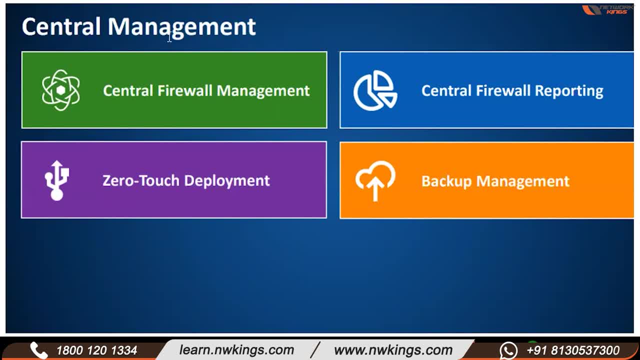 Yes, of course We will discuss its storage price and everything. How can we save the reports? There will be a zero-touch deployment. It is cloud-based, so we do not need any extra hardware. We will see the backup management and how we can manage the software firewall. 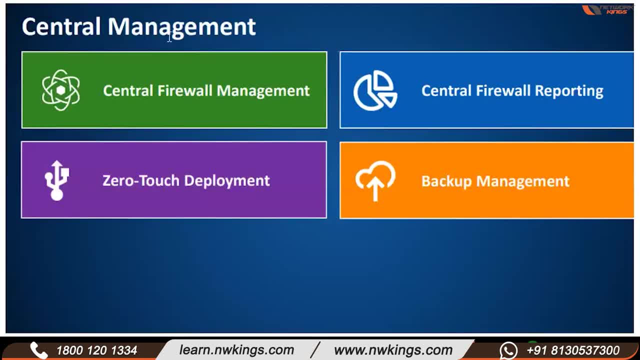 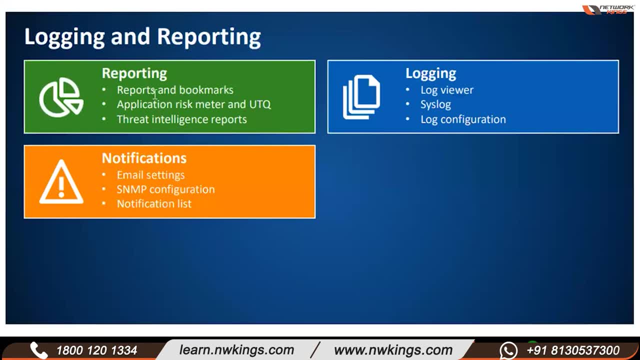 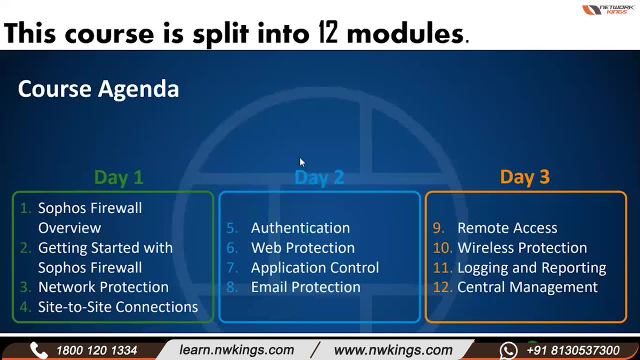 These are our agendas. These are in detail. We will cover all the modules one by one. As I told you, these are our 12 agendas. We will discuss them again. We will see the overview of the software firewall Getting started with the software firewall. 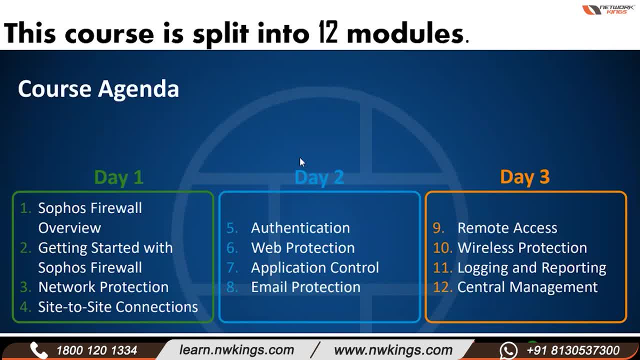 We will see the network protection: site-to-site connections, authentication, web and email control, email protection, remote access, wireless protection, login and reporting and central management. We will dive into all these by tomorrow, from 8 to 9.. 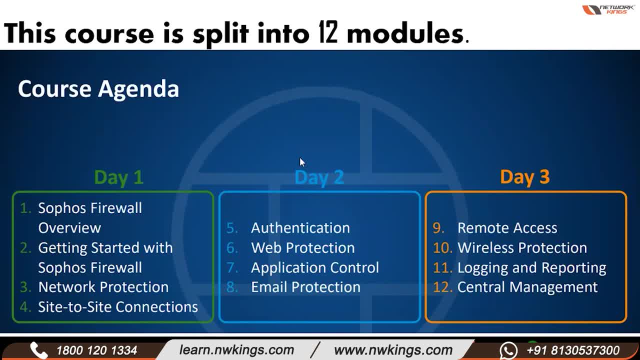 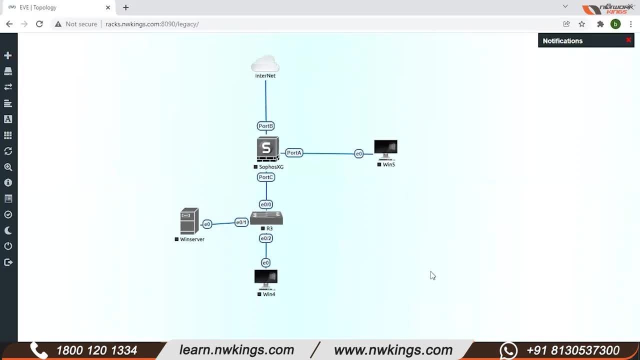 Okay, So let me just switch to the software firewall. So before I go with the software firewall, this will be our lab environment for now. As we move forward in the modules, we will definitely create our scenario, For example, how to do site-to-site IPsec, how to configure remote SSL, how to configure LAN DMC, how to configure SD-WAN. 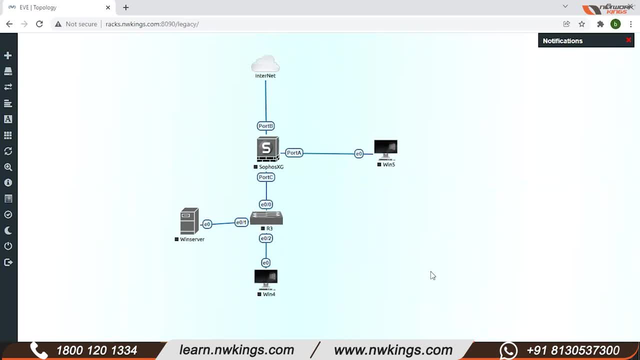 Okay, IPsec and MPLS: failover connectivity. how to check them? We will cover them one by one as we go through the modules. Okay, So let me just again go back to the Sophos website, which we have already discussed. 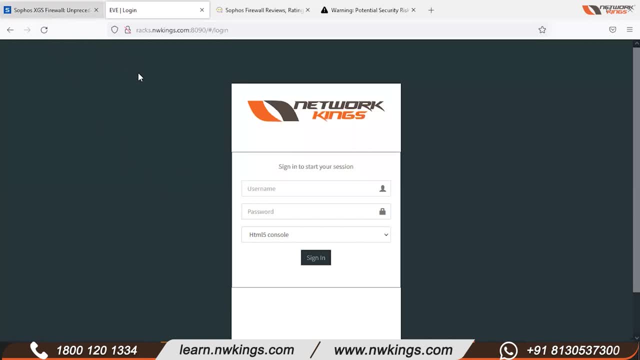 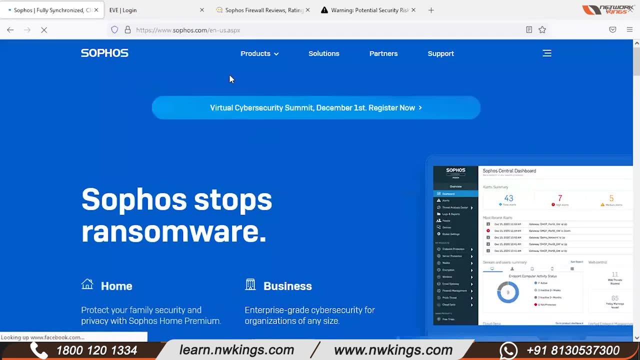 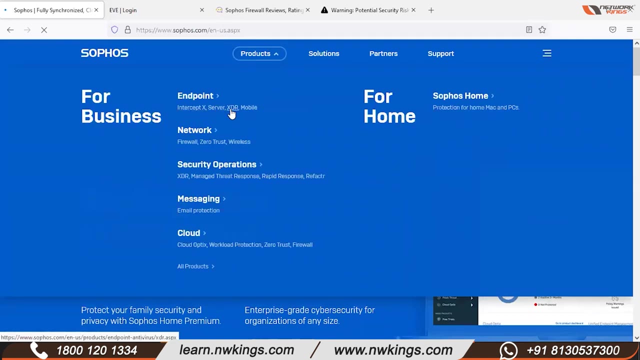 But let me just give you the overview. So there is Sophos. They have a lot of products along with their solutions. So there is interceptX, which is their endpoint, Okay. There is server protection. There is XDR, mobile protection, which we can use in the endpoints. 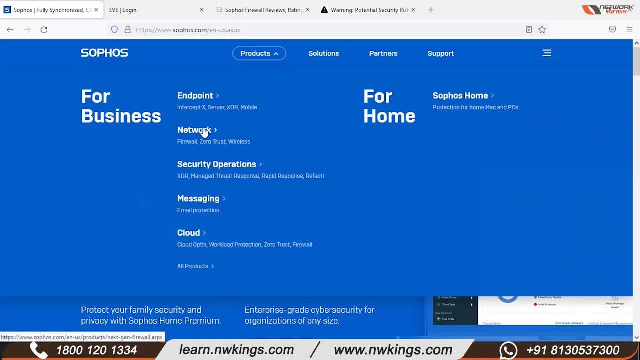 When our course will be over, we will definitely take one more overview Because it helps you if you want to do any new deployment on any firewall, And we have to set up the entire Sophos ecosystem. So how can we use all these features to make the most use of it? 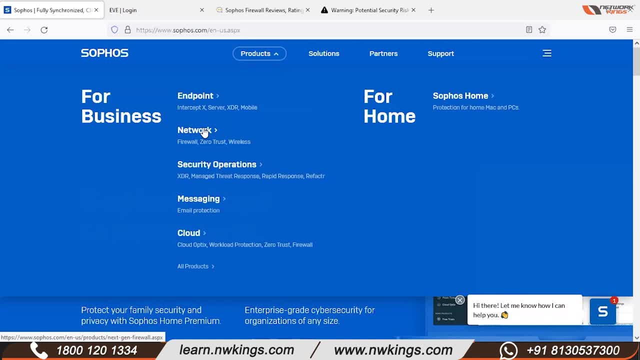 Like whatever their motto is Synchronized security, as I knew in the next webinar. So how can we use all the products? How can we enhance the synchronized security for zero threat protection feature? There are many more features. We will definitely discuss them, along with the modules. 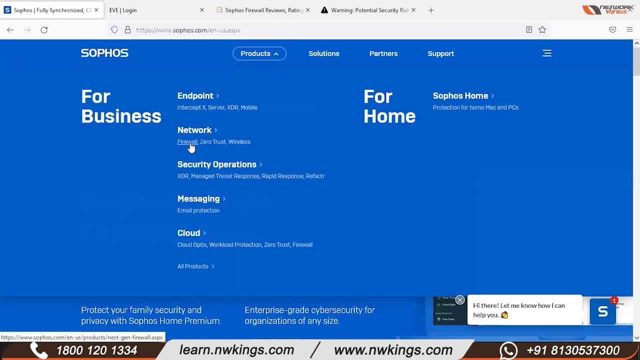 So generally, for now our main agenda is firewall, So we will go to the firewall link. But it also gives APs and zero threats Okay. Their network security operations are also there. For example, there is XDR, which detects, responds and automatically deletes any thread. 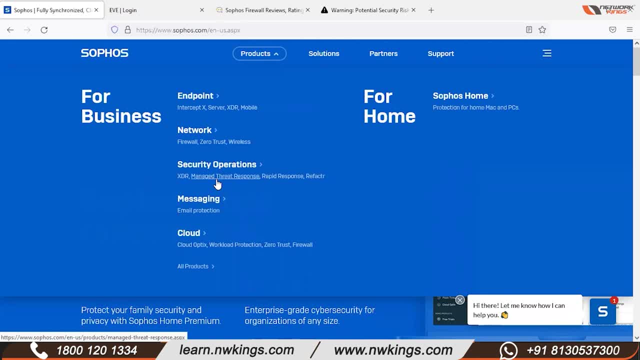 It manages it. There is also a feature of managing response and rapid response. We will go through all of them one by one. There is email protection. Yes, of course There is cloud optics. About this, it is out of scope now. 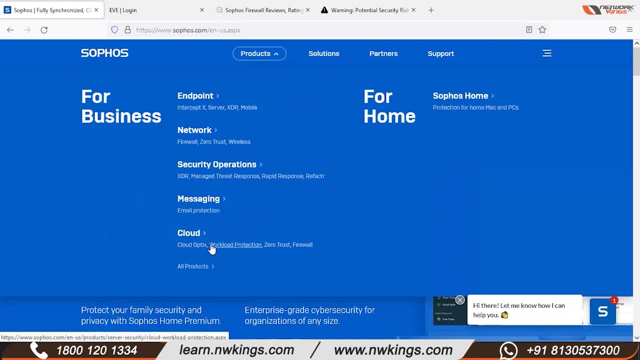 But we will talk about it later. Okay, Bye, So we have all three of them. I am now going to show you the products which the software has with the solutions, But definitely for now we will completely focus on whatever network we have. 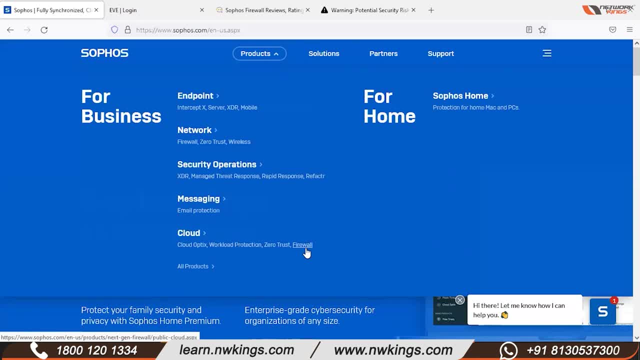 For example, there is a small business, how we can deploy the firewall. So completely now our focus will be on the software firewall configuration. So let me just go through the software's overview, the XDR firewall overview from the website. the only happy, quite to say, it's commitment is kept here. where will be I'm? 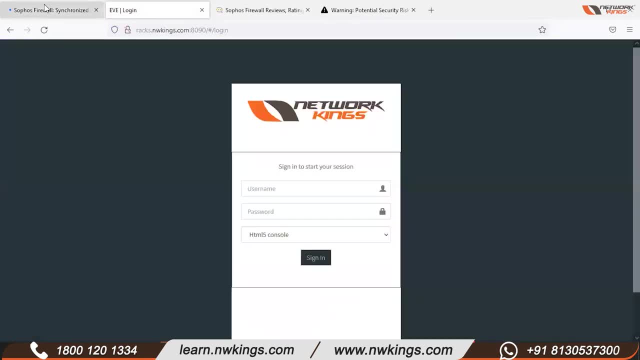 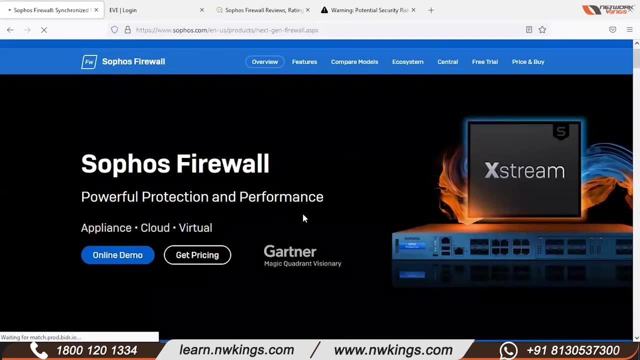 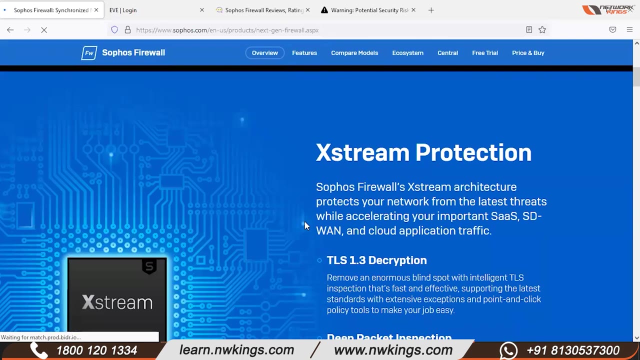 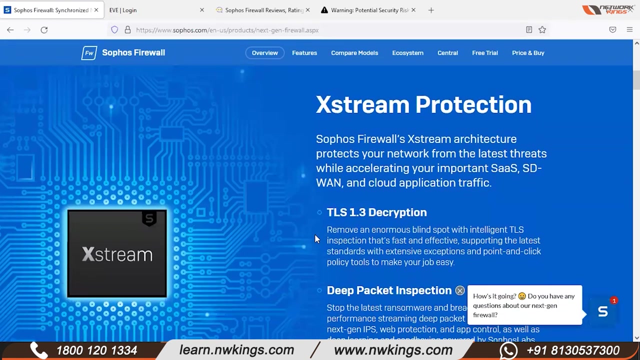 thinking: okay, so just come in up over there- suppose it's a video near your- for for sexy, sorry features of Codiga, for protection from the latest thread joby up will be thread hole ticket was so first of all, definitely, of course, a product trigger to hummus focus, a configure. 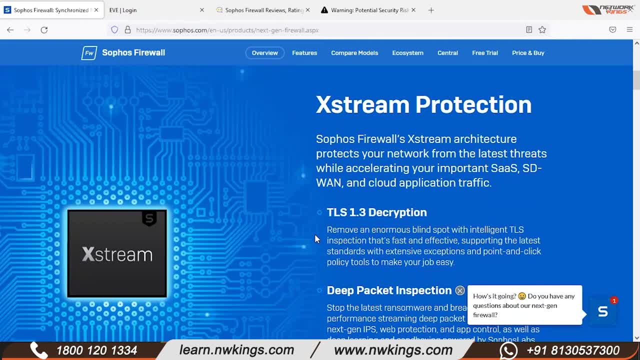 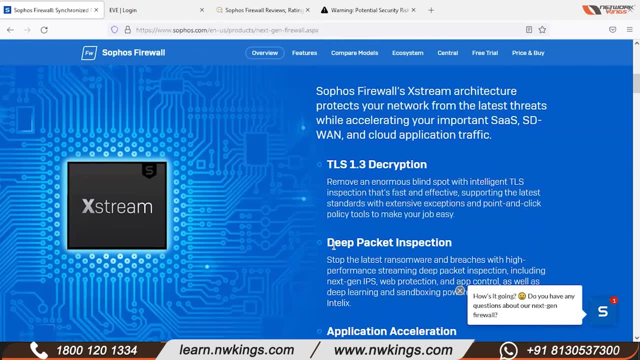 perspective is keep proper configuration. case a hum beat honey chai, a ticket hum, musketeer, major ng. along with the modules we will go up. so sorry, features available in here pay hum, along with the Chubham models caught up. cutting is of course Tom. a kicker came up. is your pack a joby doubts you have. 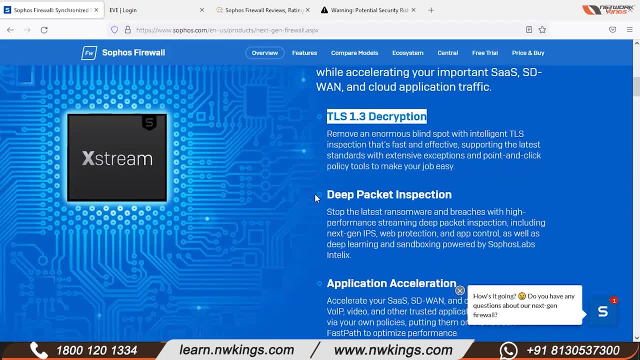 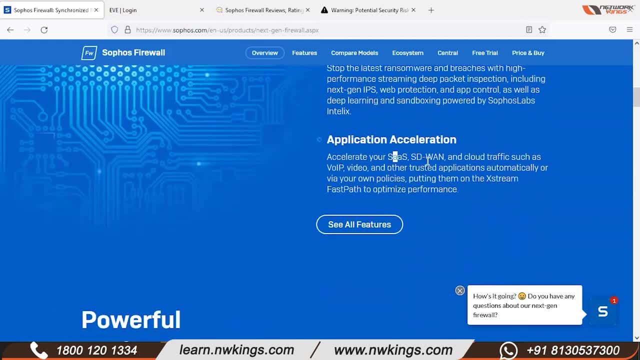 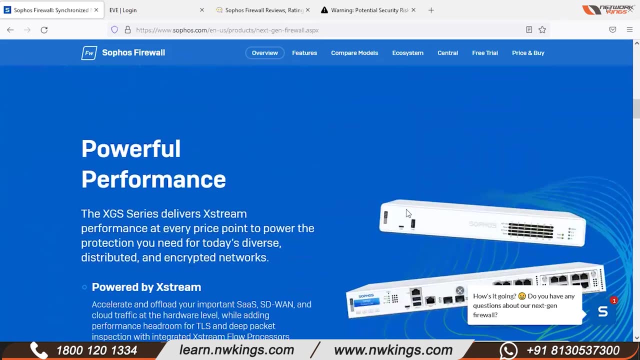 a good late at a, for example, to- definitely- I'm so loud- cutting a jacket to kiss a deep packet in. set in inspection already get X lay application. x-ray kiss a curse of 30k cloud base. a, for example, to go: hum, baking is key configuration. hum, kiss a cutting. or is ca working? they can guess. so it's casual. 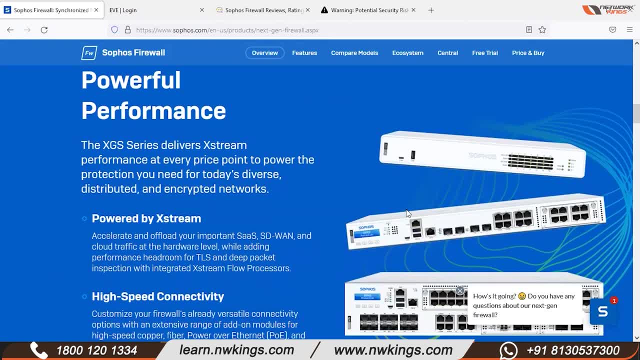 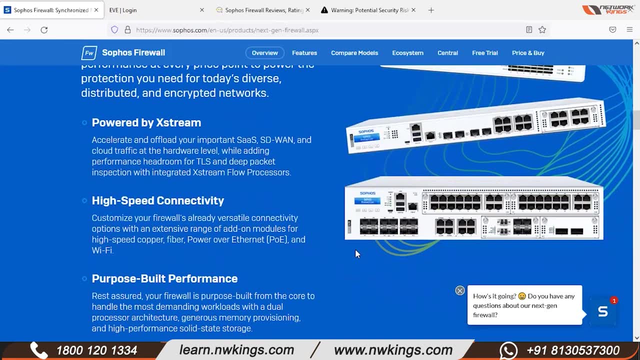 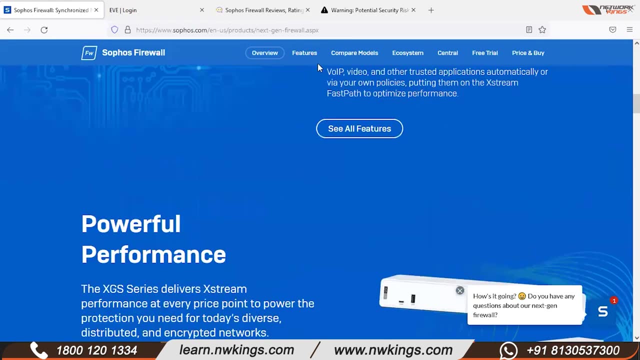 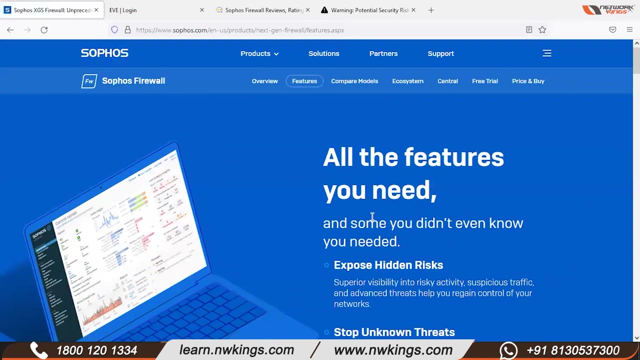 power for performance. a ticket powered by extreme architecture will be hum a bar detail. major in case I work at that ticket is a high-speed connectivity. a ticket purpose: to build in performance. a ticket, guess I'm deploy curse at the home. they can all right. so going to the features, just say you have a features available here. 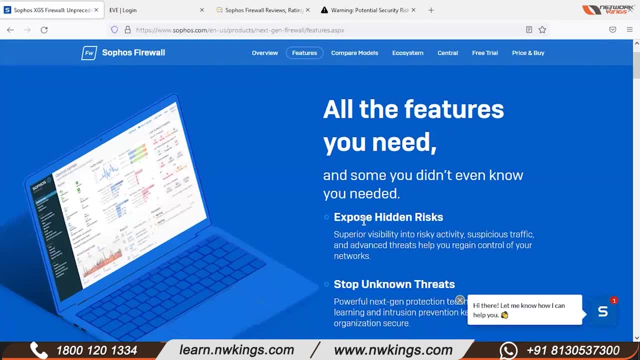 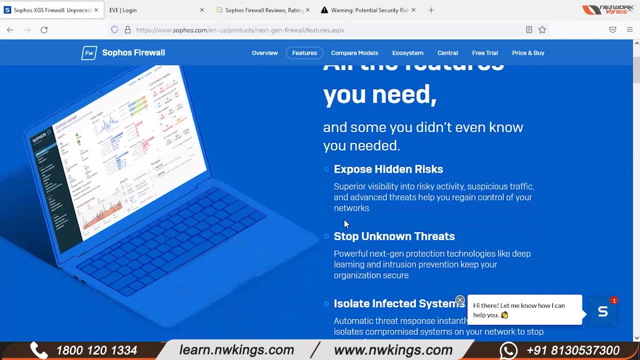 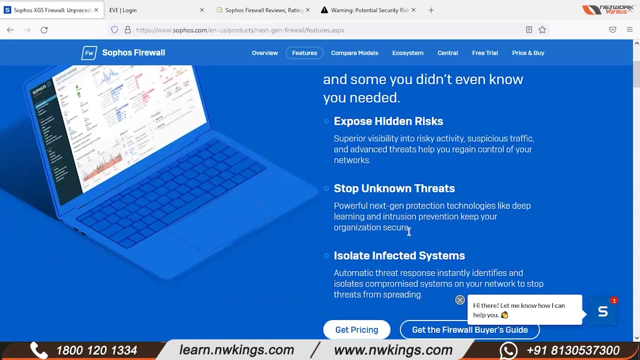 to be other existing network be I'm replaced carousel force for other coherence be those officers could definitely use for eliminate cardiga apnea protection policies. scan goodness. a other coin on thread. sorry us, Kobe, stop career will. let us some of the malware job it up. the technique, those of 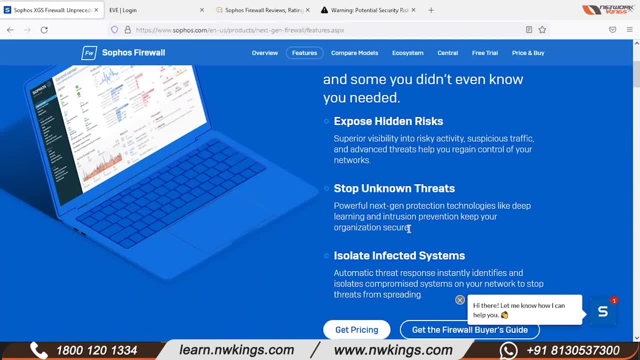 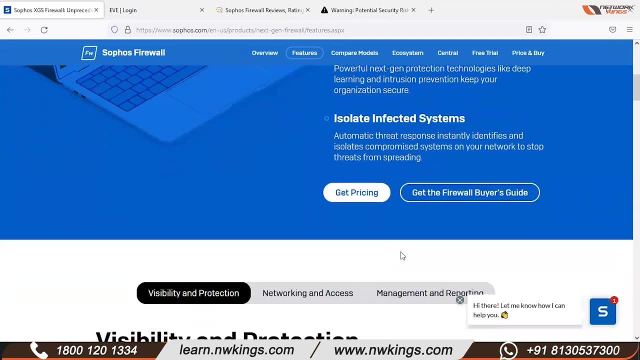 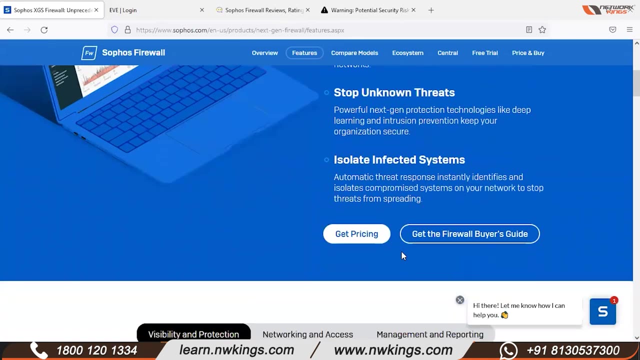 us. you can see that we have a lot of features available here. so, going to the features, just say you have a features available here. so to be other existing mesh. I have no areas another what I wanted to discuss with you. they will go to look at your. 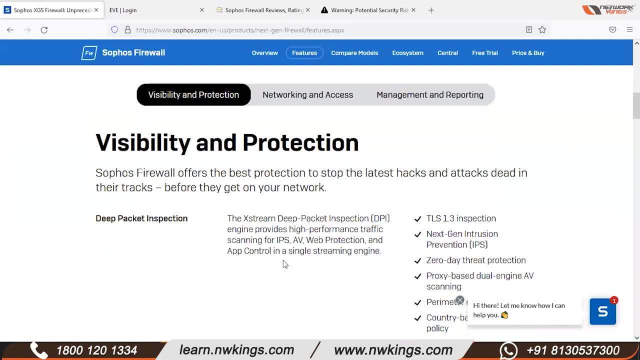 properties. oh yeah, you got all right. so what I mean is just a little separate. dashi, okay, you have planned to lock the palms, so connectivity is a realityENV' room. she, okay, DPS, she failed. that's, we will stay. keep watching the provides, inмер us packs, etc. 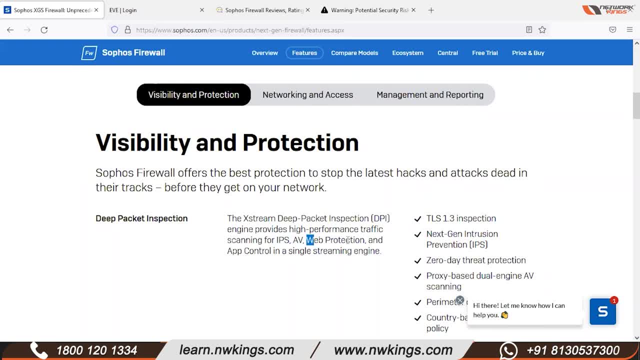 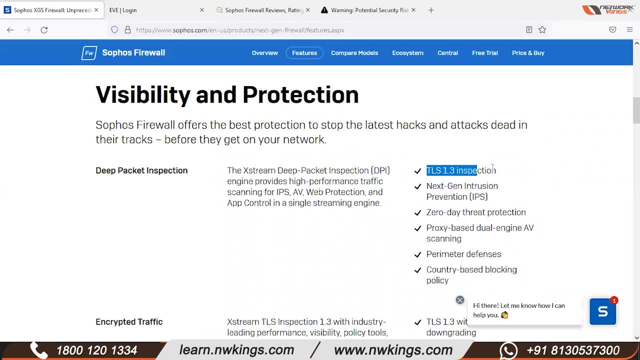 have in their behaviors, so people's theme of concerns will have different rate. that is just a EIPS and Antivirus Scanning and Web Protection, Email Protection and Application Control. How it will work with single engine And which protocol it will inspect, we have mentioned in detail here. 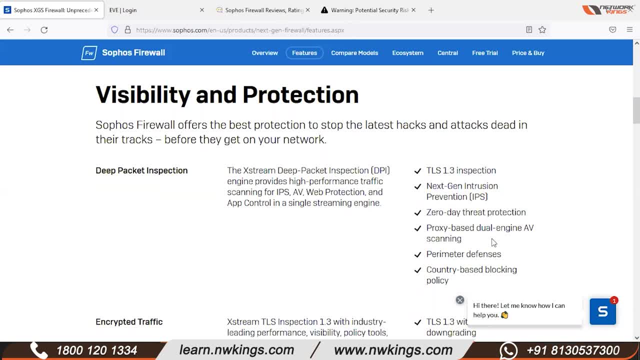 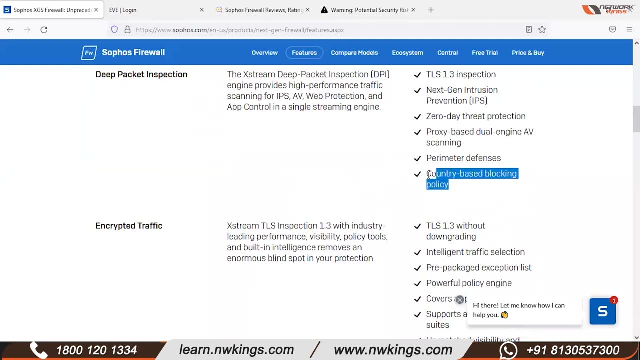 And it has a zero day thread protection Means you will never get thread attack. it will be zero day. You will never get thread attack. so everything can be blocked by this Proxy based dual engine AV scanning parameter defense country based. if you want to block something, then all these features are available. 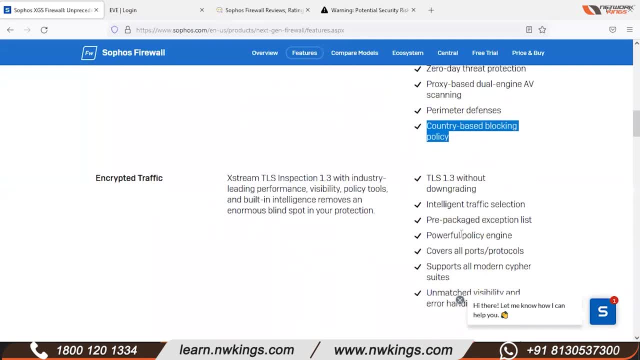 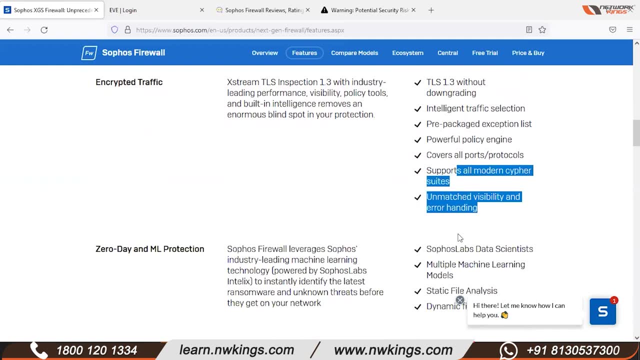 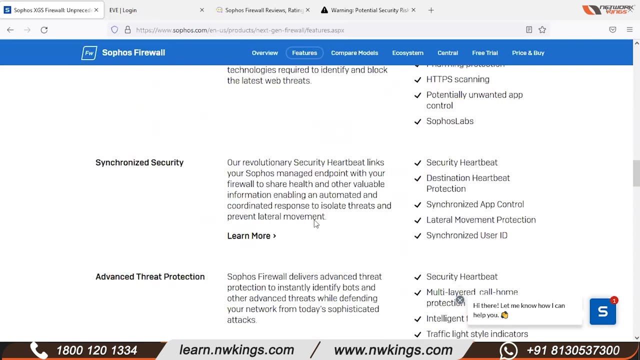 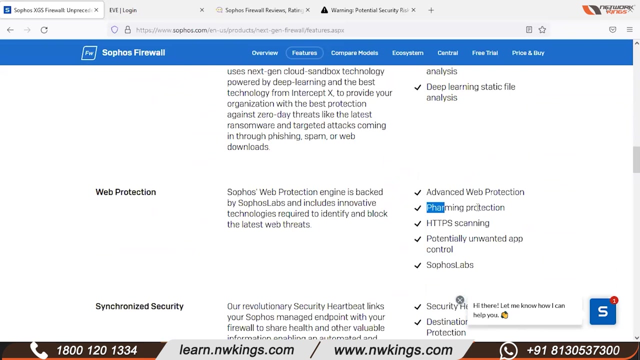 Deep packet inception. Same way, if there is any traffic encryption, then we will go in detail about it. Sandboxing technology, zero day web protection, synchronized security. as I told you, all the features are here Along with our module. We will see one by one, why it is actually mentioned here. 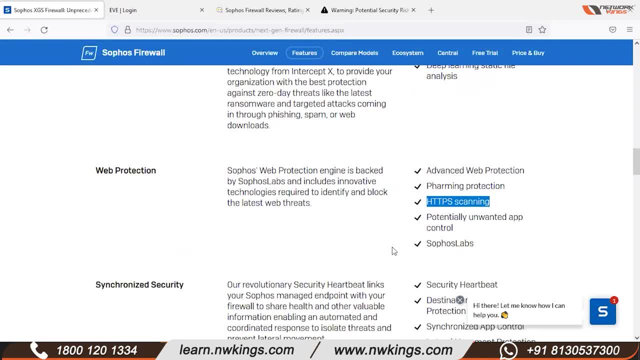 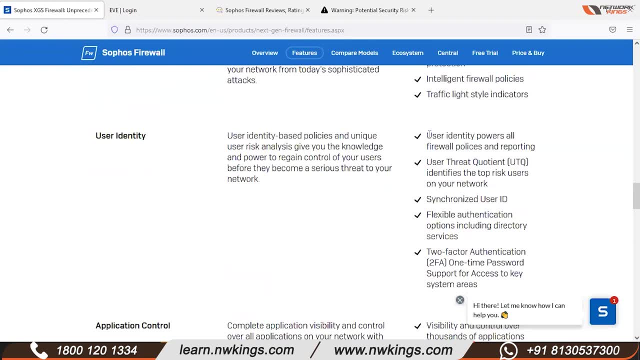 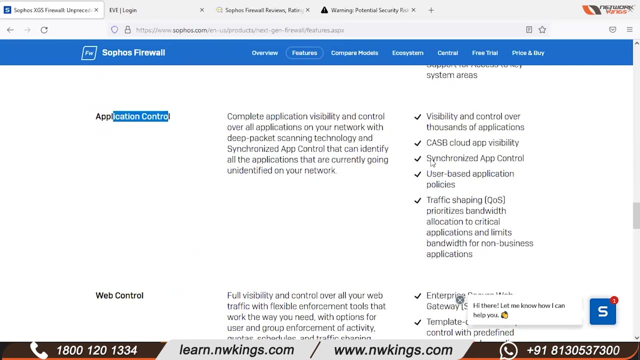 And we will see where it is visible in our Sofos lab environment. in the configuration We will see that it will be easy. User Identity for authentication: as I told you, there is an authentication module. Everything will be covered in it: The features of the application control, the visibility of the application control. 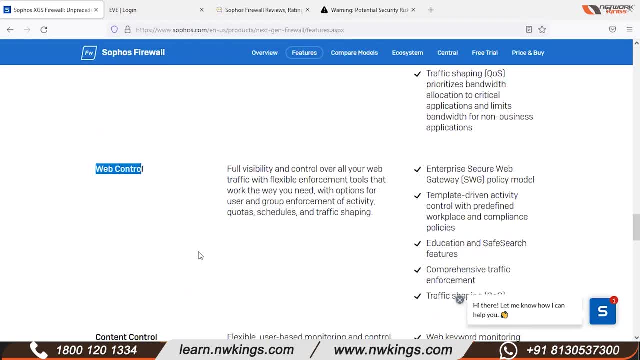 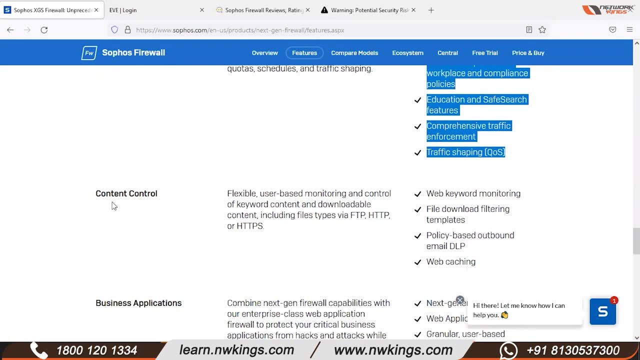 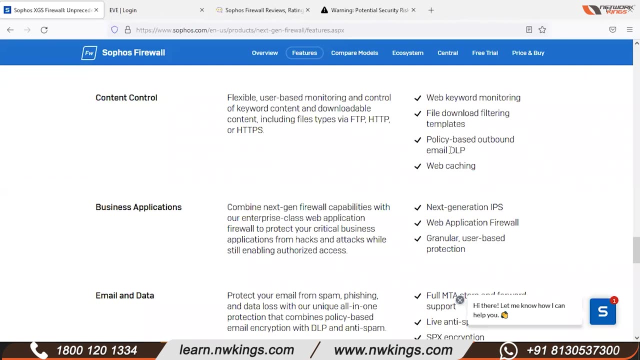 We will see all the features here. Same way with the web protection. As I told you, we will see the web control features. We will verify all these features through modules. Content control: there are business applications, for example. Content control, like if there is an FTP file is being downloaded. I will tell you about it. 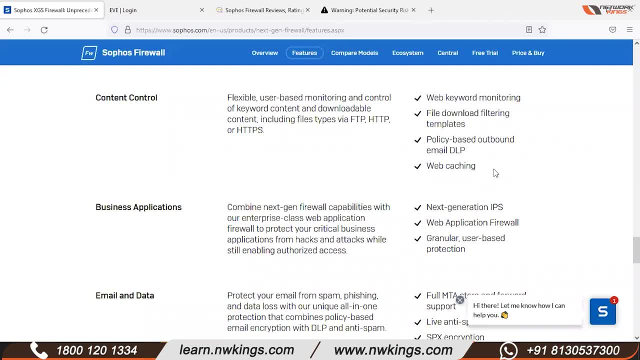 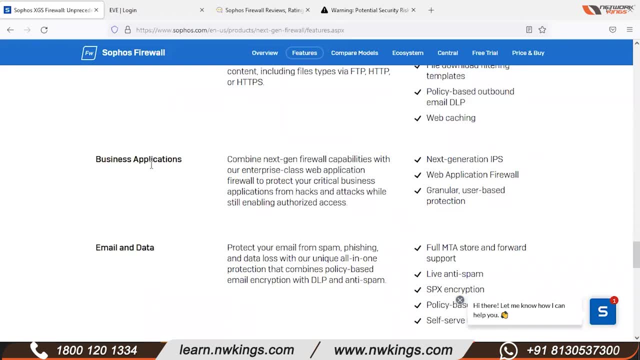 If you have a particular file, it is being detected through sandboxing. So how can we use those features? we will see that through sandboxing Zero day protection Business applications- we will see if we have hosted any business application outside. So we will configure these features in Sofos file. 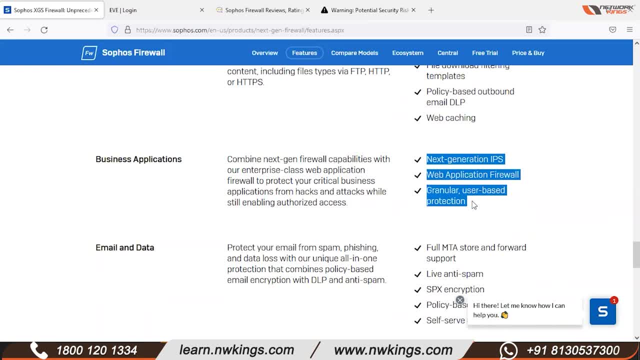 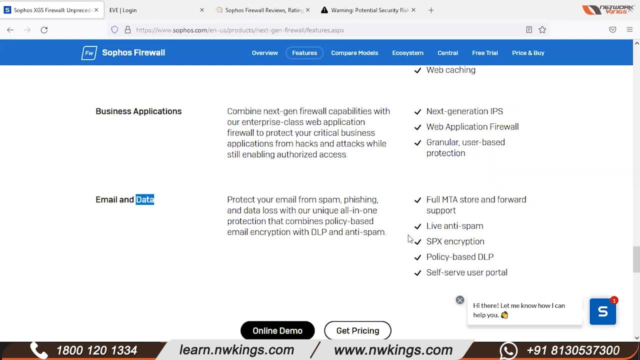 Business application. as I told you, if there is a web server Which is working on port 480 or port 443, How can we secure it? And we will see how this feature comes into pictures. Same way with the email and its data. We will see, as I told you, in email protection. 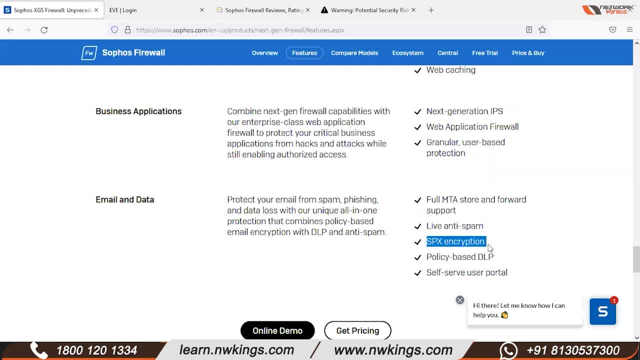 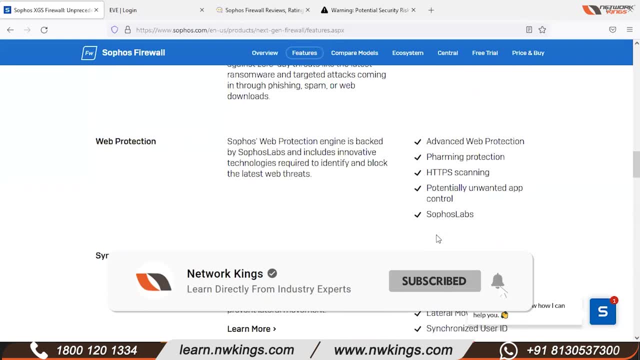 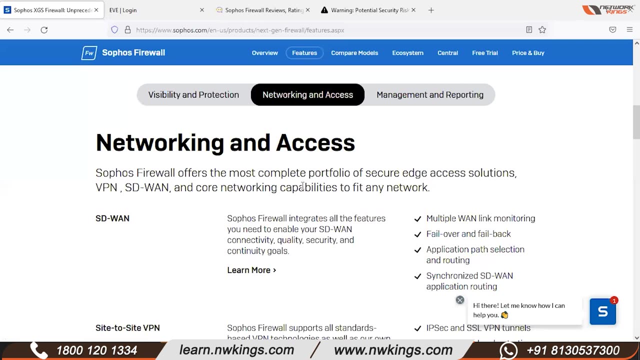 Features of MTM mode: how to spam entries, How is this SPF encryption? How do we use policies? We will see all these features in the configuration modules, One by one, And we will keep this website in reference. Same way, this is visibility protection. In the same way, there is networking. 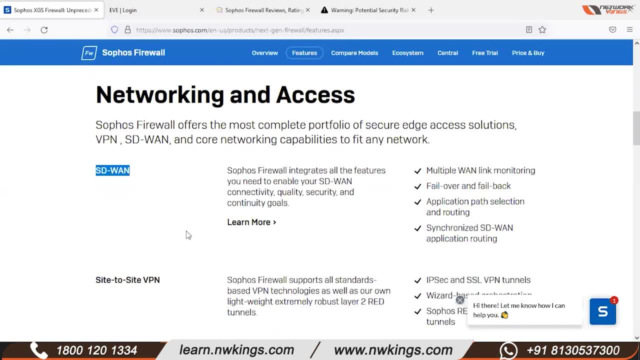 Which is our connectivity. For example, we will see the SD-WAN. If the SD-WAN feature is there, We will see it here on the firewall. How can we configure it to meet the requirement? And we will discuss its scenarios: How, in which scenario, we will use SD-WAN. 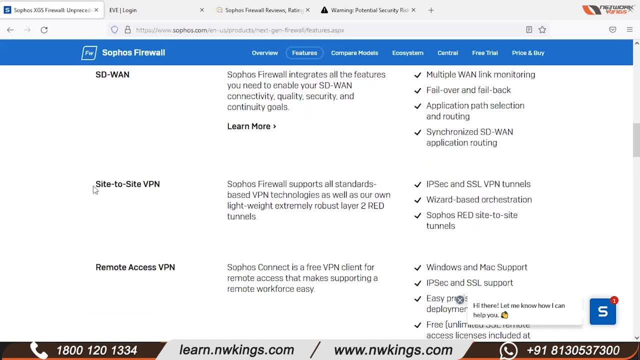 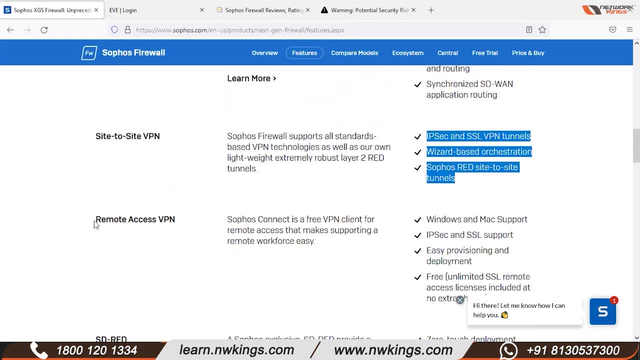 How can we configure SD-WAN? All right, Similarly, site to site, If there is a head office or branch office, We will see all the features In sofos firewall, How all these features work with configuration, Remote access, VPN, As I told you, IPsec and SSL VPN. 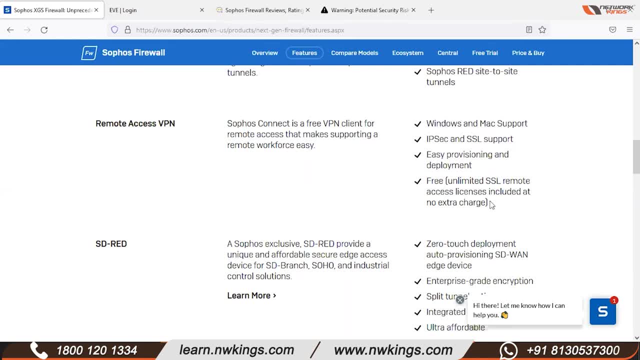 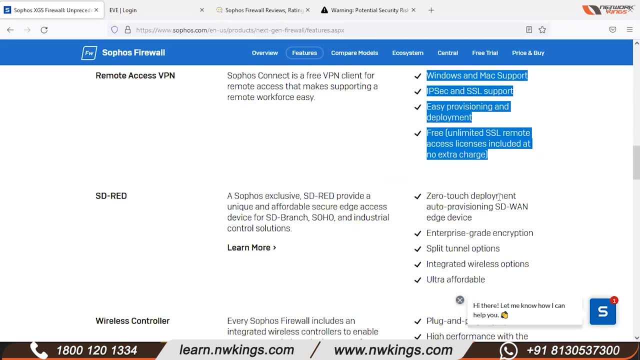 If you want to give some server access from outside, How to configure it in Windows. That is all the features Which are also KB articles How to configure. We will refer that too And we will configure it in our environment. Red: How to configure red, Like 2xg for example. 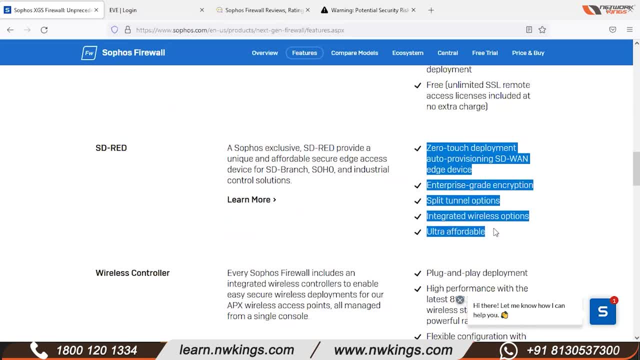 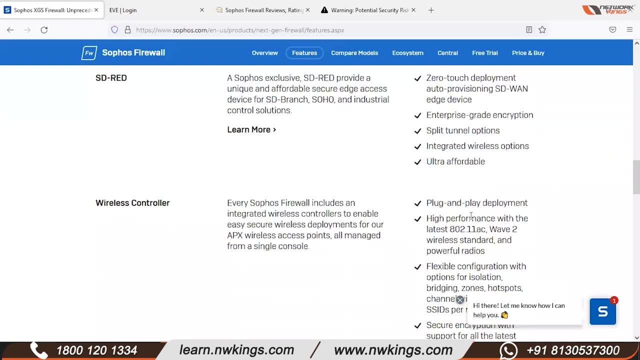 2xg, Both sides. You have installed sofos products, That is, sofos's firewall is installed. So how do we connect both branches? We will see all these features. Same way with wireless controller. We will see all the features one by one. We will see ctna. 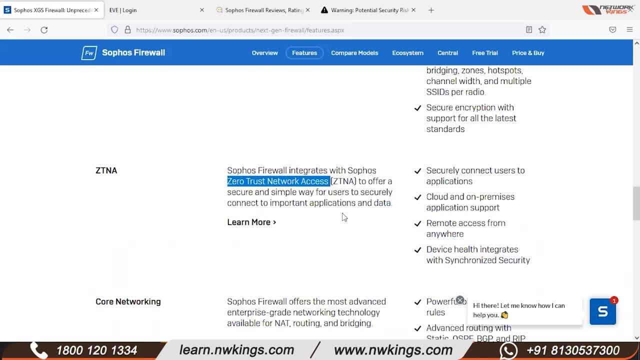 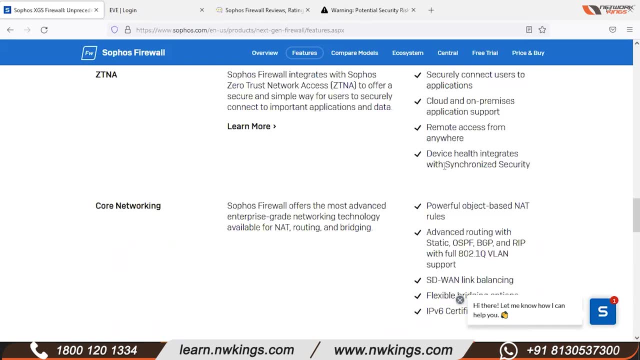 Zero trust network, That is, we will not keep any device unsecured. In short, How we will meet this feature? We will see all these features For synchronous security, Security generally And health of the device. We will also see core networking If we want to do any connectivity. 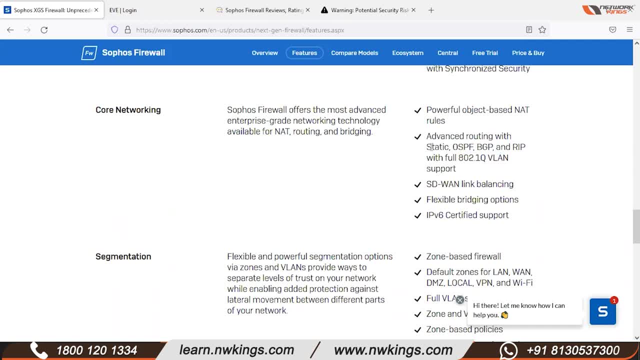 Like OSPF, BGP, RIP. If we want to do any routing, We will see that Static, Dynamic routing, Both will be done. SD-WAN will also be done, Of course, And if there is an IPv6, That will also be done. Segmentation, That is, whatever network. 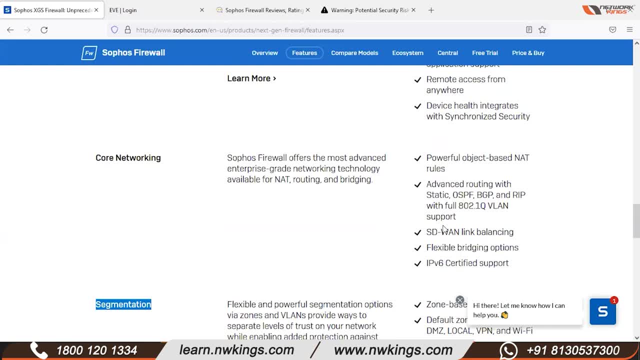 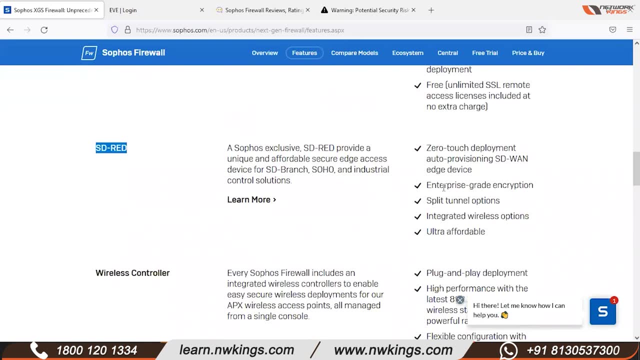 Bharat. Will the concept of SD-WAN be covered in this? Yes, SD-WAN will be covered, Okay, Okay, The features of SD-WAN, Like how we configure in firewall And the current business requirement On SD-WAN. We can prioritize it. How to prioritize it first, 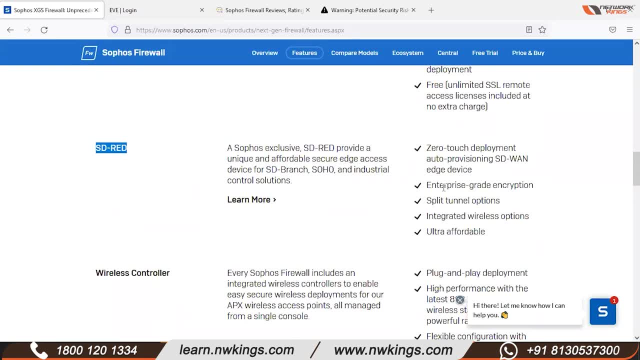 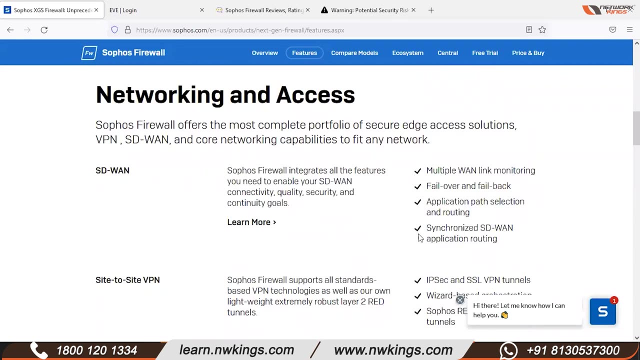 We will discuss those small configurations Along with the articles of the software Through it. And if someone has an existing network, How will we deploy this in it? SD-WAN, Sorry, SD-WAN, So we will also see that, Of course, Okay. Okay, Then Here Segmentation: If here. 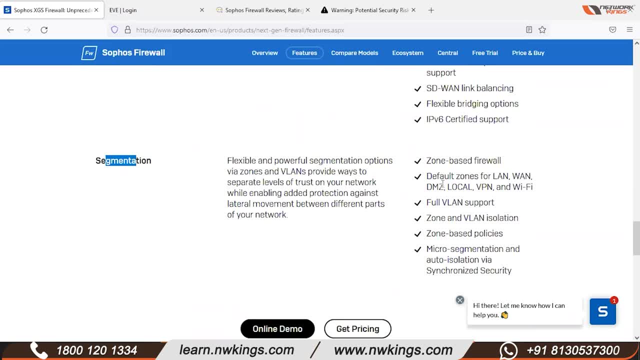 If someone is our network, Okay, If it is large, Okay, If we have configured the same line And that Behind them, Like 50 users And the servers are also in the same line. So how can we segment it So that lateral movement Now, For example? That is the feature. 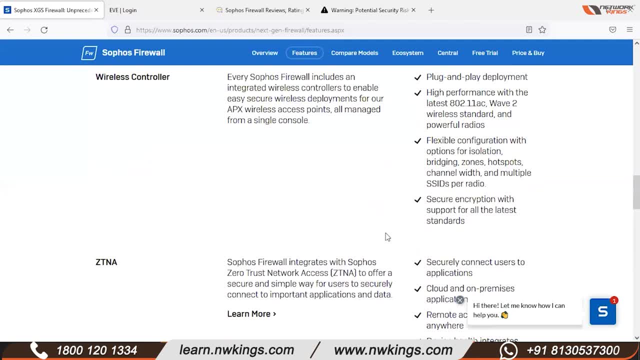 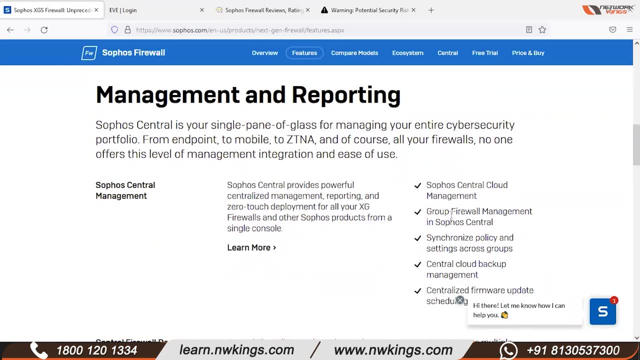 That is also covered. We will see that. So how we will segment, We will also see these features One by one In the same way. In the last module There was reporting, There was management. So the features, They will be covered in all the modules. So how can we manage the software from the center? 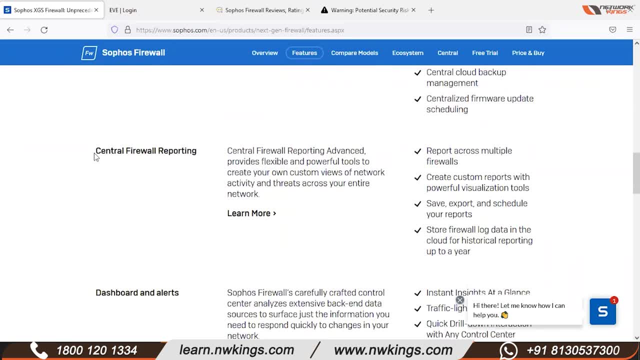 And all the features We will use One by one. There are some features In which, Of course, License will be required. We will discuss it. Articles Which are configuration, basic articles: We will discuss it If possible. Definitely We will work on it, We will work on it And we will talk about it. 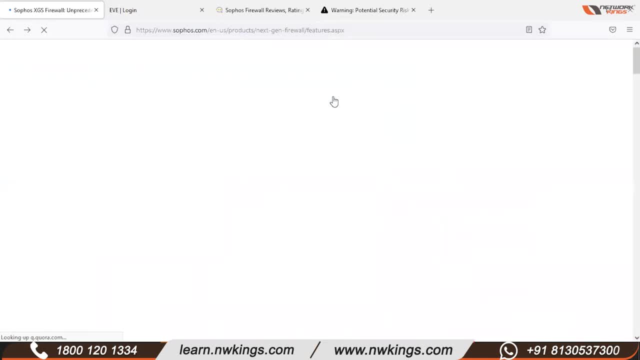 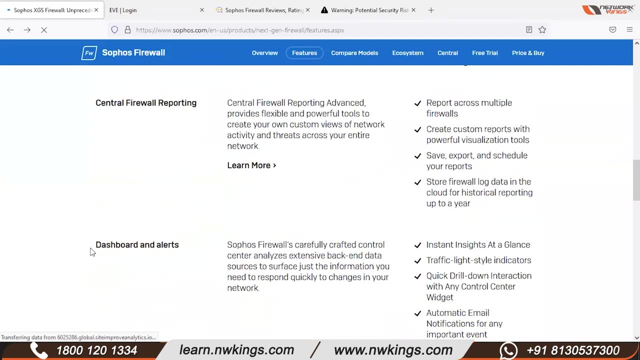 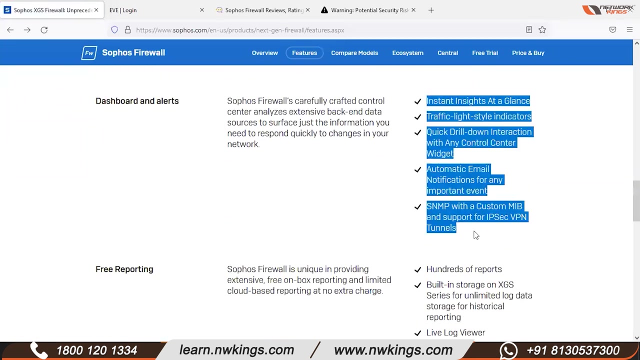 In the next video, Sorry, Okay. So dashboards: Okay. So, whatever We are integrating reporting and firewall, Okay, The alert that comes on the dashboard We will take an insight once, Only Verify Like Something We have to drill down. Okay, We have to do suspicious investigation, Generate forensic reports. 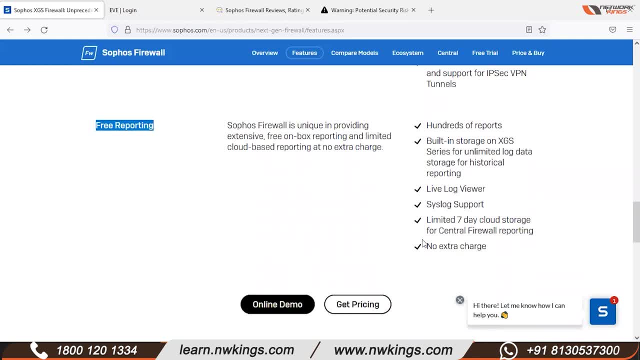 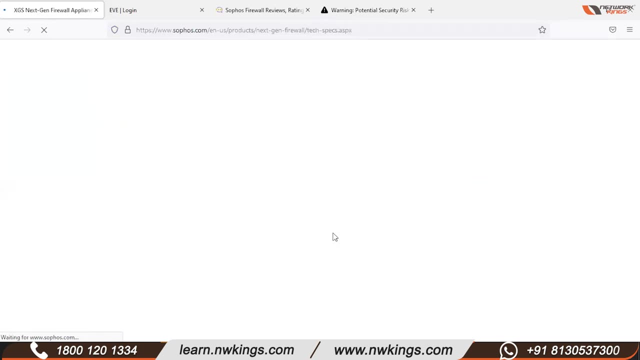 Then we will see. We will also see about free reporting. for example, Sofos provides 7 days of free storage. If you want to give more than that, then what is its core storage? we will see all the features in it. You can also see the models. we just see one overview about it. 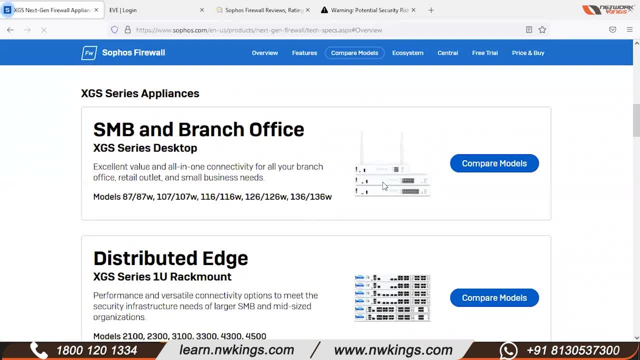 So you will get all the details here. whatever the model is, If there is a small business, you have to protect it. where you have 2 to 5 users, 5 to 10 users, You can install SMB or branch office, ie SGS desktop series there to protect those systems or servers. 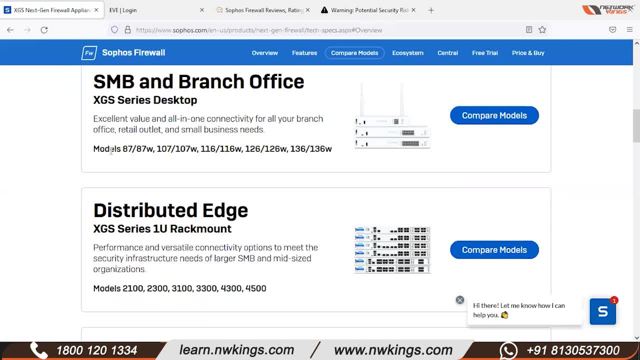 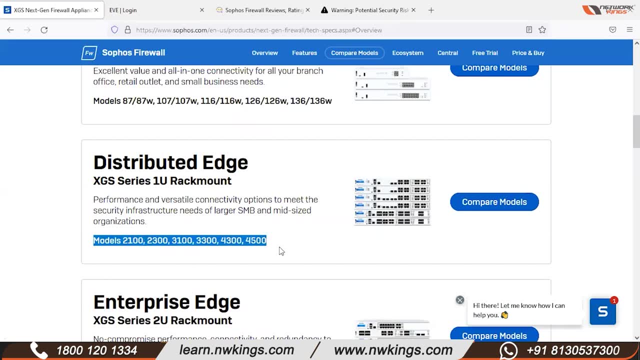 So you can verify these models. Definitely, all these modules will be covered up. we will go about its hardware. We will discuss all the models. like it is a medium scale business, like it has 100 to 500 users, So its models will be covered up. 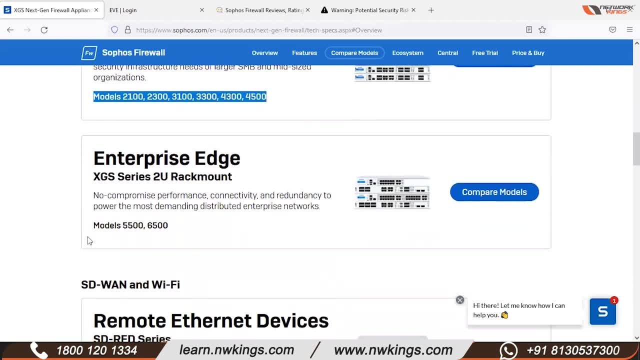 We will discuss the modules and its hardware parts In the same way. large organizations, where there can be more than 1000 users. So we will also discuss those modules, how we can scale it and hardware configuration. All this is covered up in the modules, so we will cover it up. 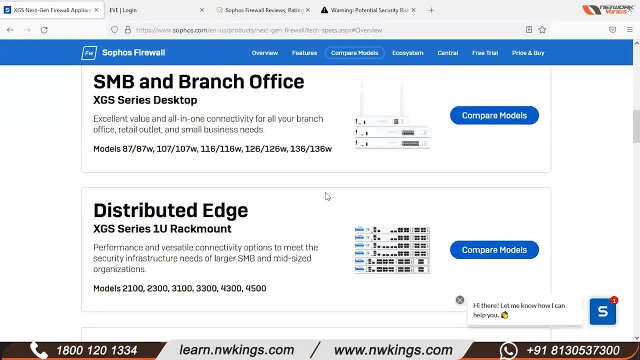 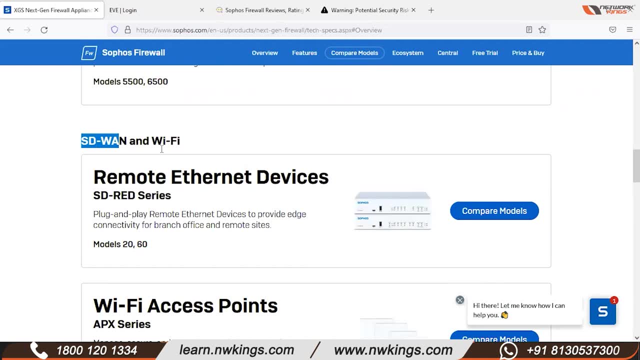 Along with that. whatever information is there on the website, we will verify it one by one. The feature for SD-WAN is also fine in Sofos Files. How can we meet the reds, Red devices, Or Sofos to Sofos? 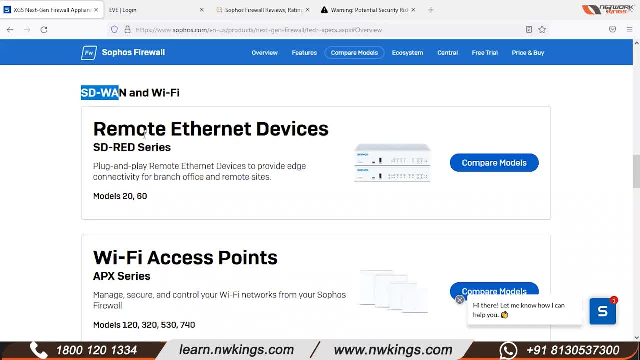 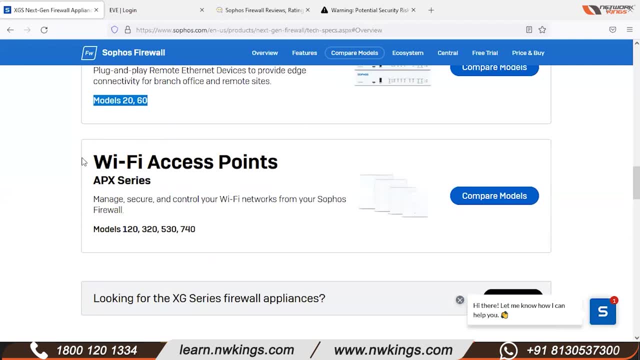 So how can we use SD-WAN? So we will also look at its device scenarios. So we will discuss their modules once Covered up in the modules, Along with, as I told you, the protection module of the wireless module, In that the APs of Sofos, these models, APX series, will only support 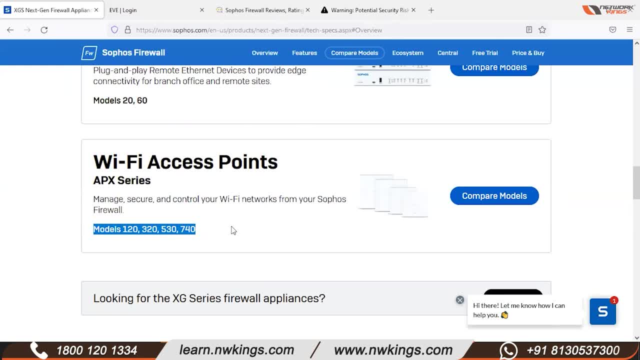 Like there are third party APs, like Netgear or anything. They will not be protected Because they are third-party vendors. we can't do anything to them. But yes, of course we can secure it with Sofos firewall rules. 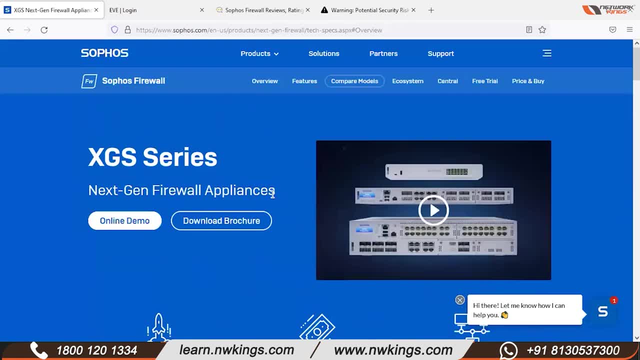 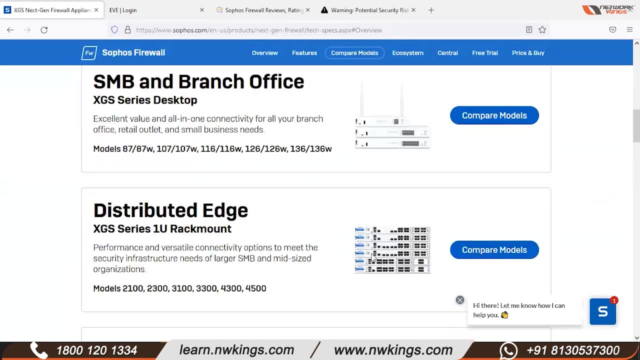 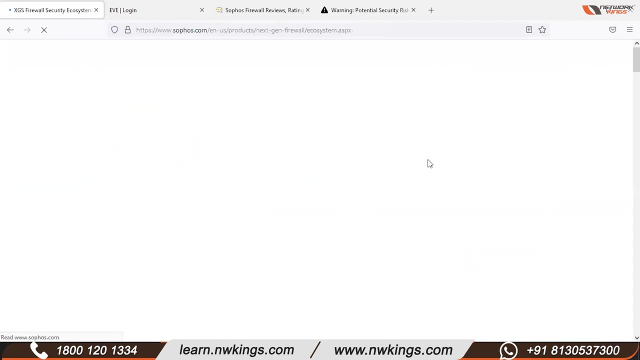 We will discuss about that, Because it may happen that this is not the entire Sofos ecosystem. So how can we make changes in existing- We will see that- And how can we protect it with Sofos firewall? We will discuss that. So there is a little detail about the ecosystem. 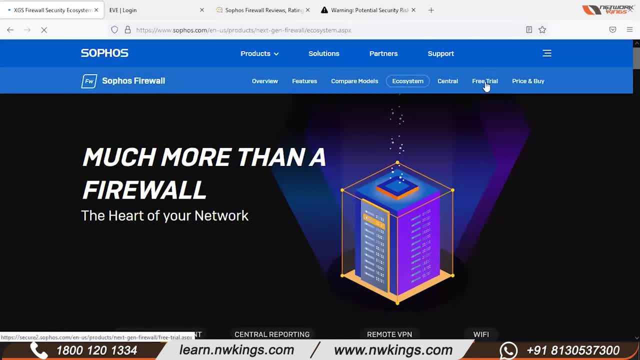 And there are also free trials. So we will show you how we can use free trials in Sofos XG firewall on our laptop, How you can use it for free for 30 days Until you get access to the lab, Until we set the setting. 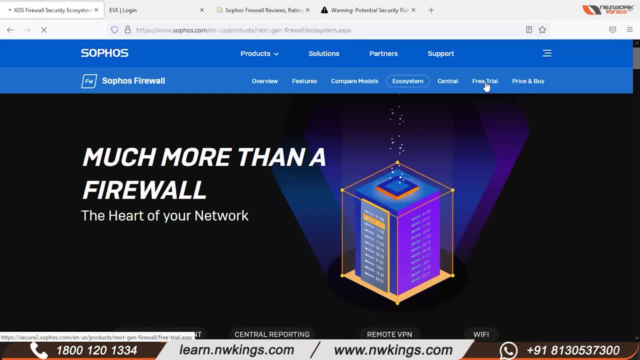 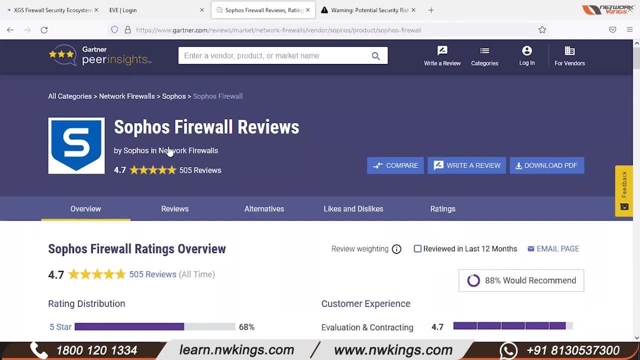 Until then, we will use free trials on our laptop And we will see how the traffic flows. Okay, So, as I told you, there are Gartner reports, So there is a 4.7 review If you want an alternative firewall. 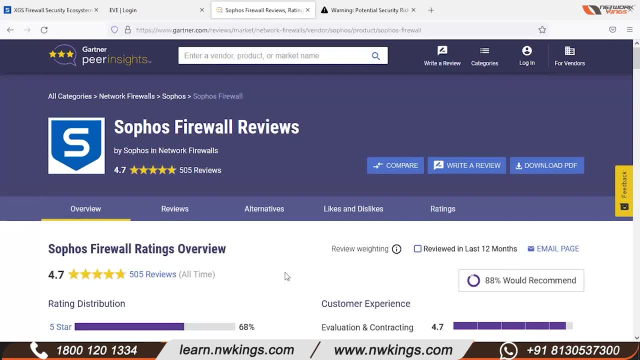 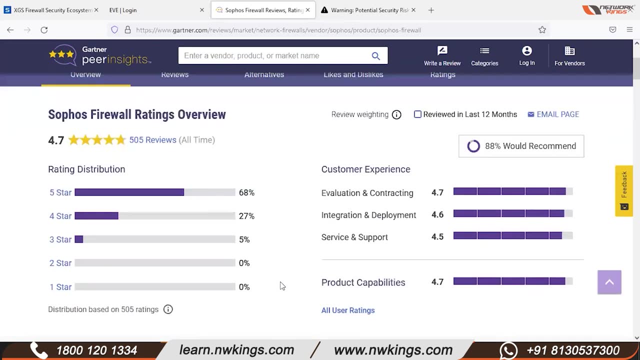 Or you want to replace it, Or there is a new deployment, So you can definitely configure Sofos firewall easily after this course. There will be no issue. Yes, of course. by enabling all the features, you can fully secure your business. 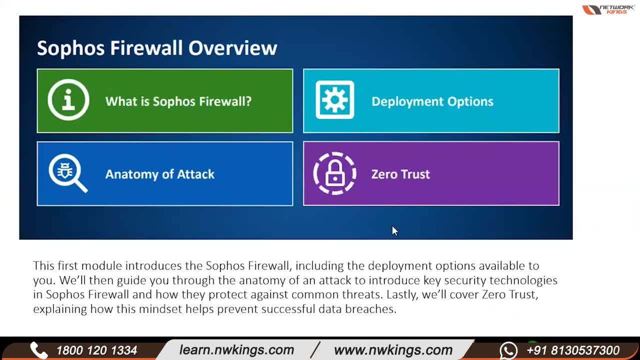 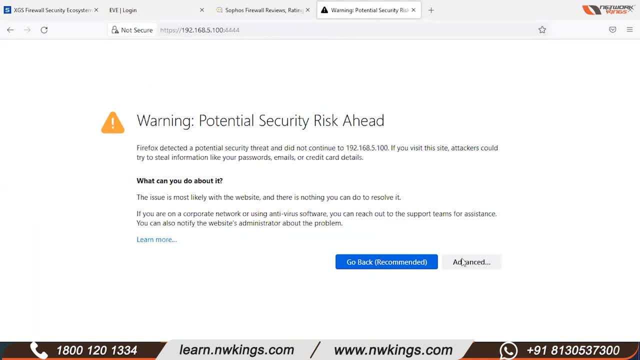 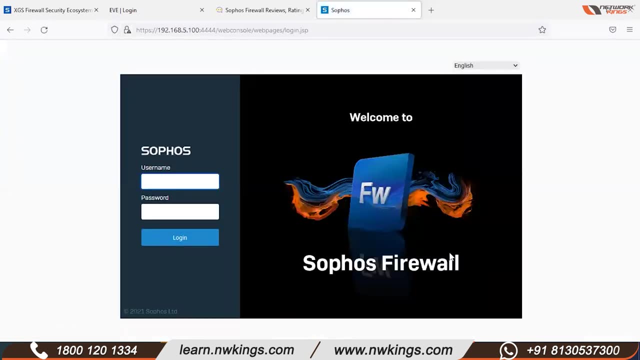 So let's access Sofos firewall once Okay, Just a moment. Okay, Now I have installed Sofos firewall. It is free in my VM, So let me just access to the GUI. I will also take a console with me, Because we will see both. 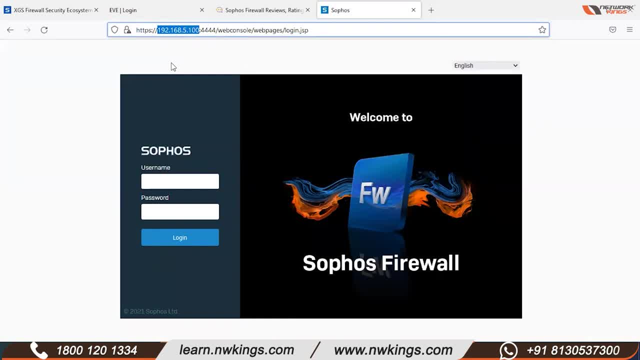 Most of the configuration will be done by your GUI. You will not need much of the console. As I told you, we will see how to install Sofos, How to configure And how to troubleshoot. So the two parts- installation and configure- will be done by the GUI. 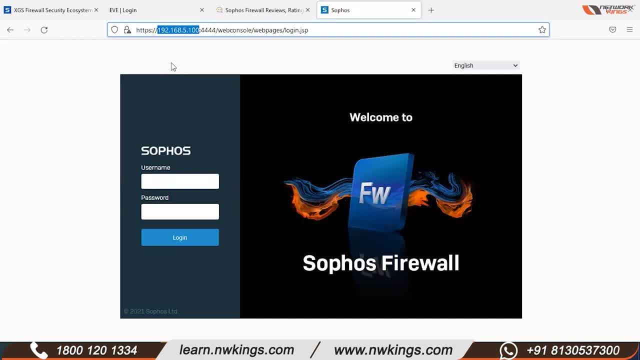 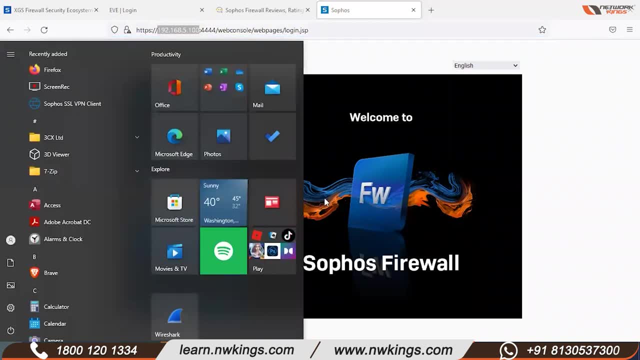 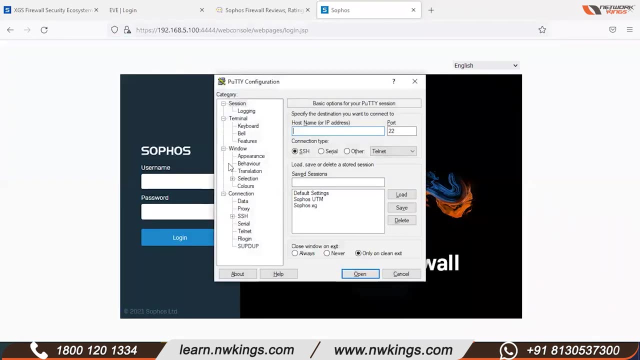 In the third troubleshoot we will mostly use CLIB along with the GUI, Because both methods will be the best. If you want to go to Sofos XG firewall domain, I will also open a putty with me, So let me just put the IP. 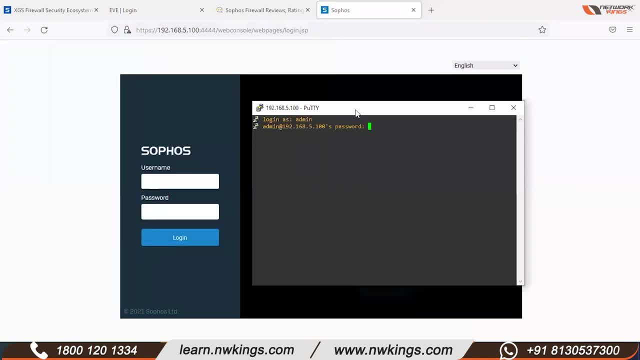 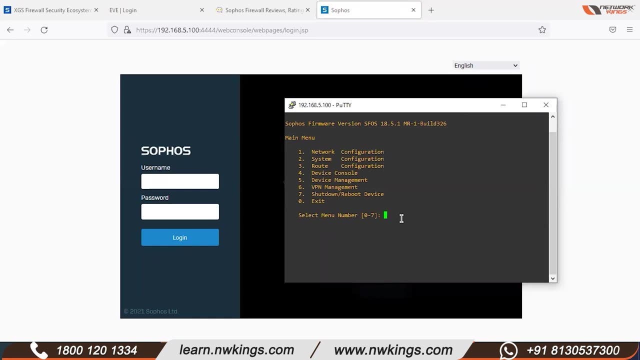 Let me just login here. Okay, So this is our GUI of Sofos. Sorry, it is CLI And we are GUI at the back. So here we will get the options. What can we do? One is network configuration. Second is system configuration. 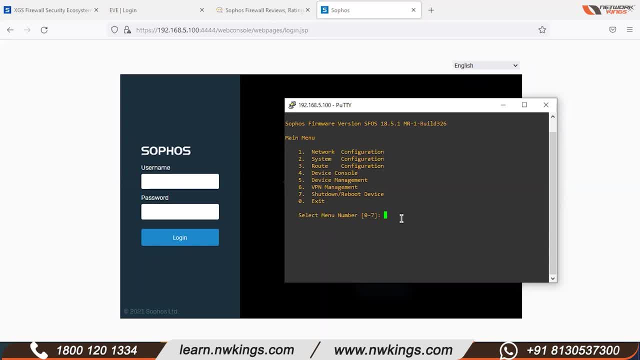 Route configuration, Device console, Device management, VPN management. We will explore all of these, Where we will use it And where we can use CLI as an option, We will cover it along with the module. Let's say, for example, I am selecting 1.. 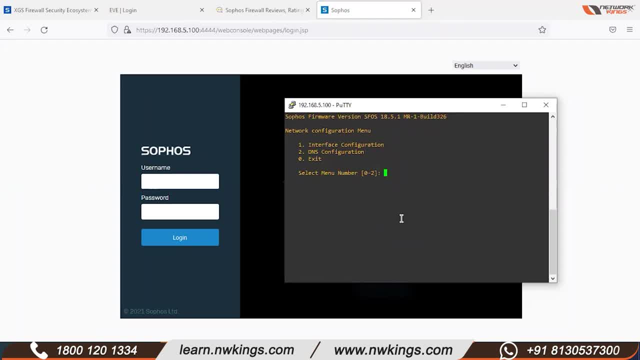 So the interface will also have an option like Interface configuration, DNS configuration or exit. So you will get all the details of the interface here. Okay, If you want to go to device console, there is a fourth option So I can take TCP dump here. 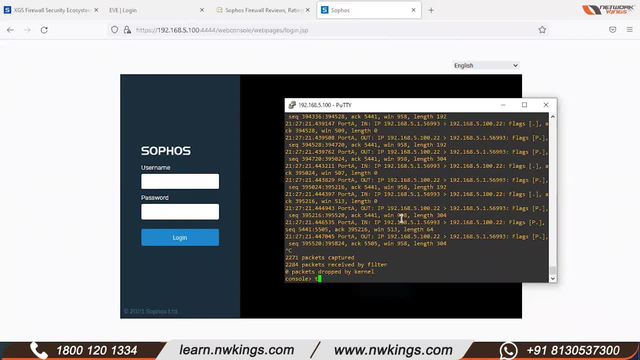 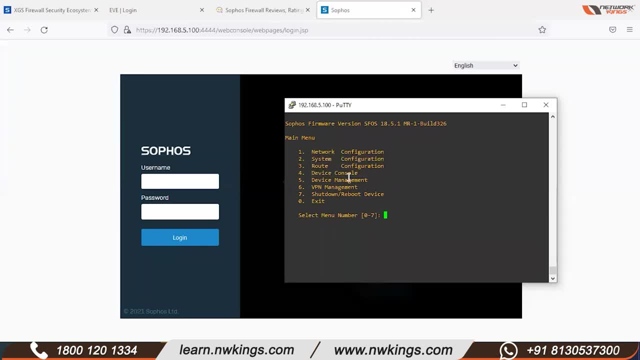 Okay, Okay, There are many features. We will cover the module later. We will cover it in module One by one. We have to see the route configuration. We have to see the system configuration. Okay, We can see everything from the console here. 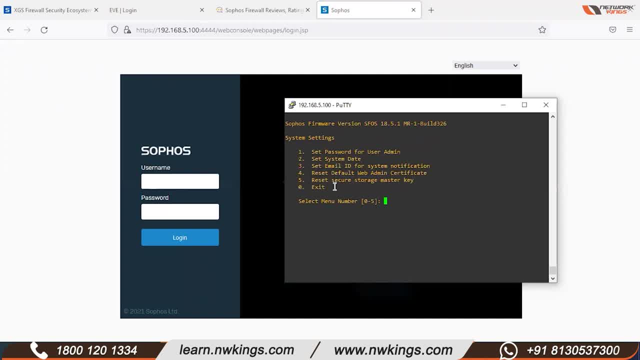 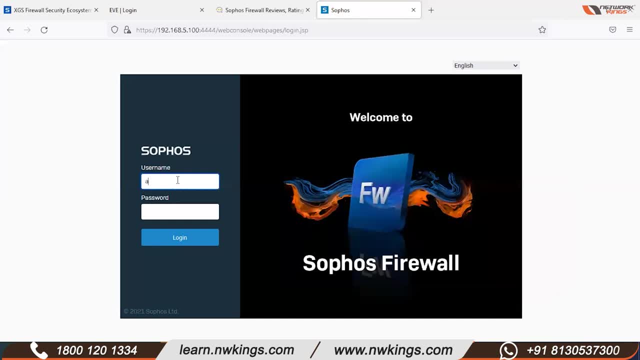 Okay, We will explore all the options, For example, to reset the password. If you forgot the password, then you have to reset the password. How will we do it? It will be covered in all modules With CLI. Coming back to the GUI. 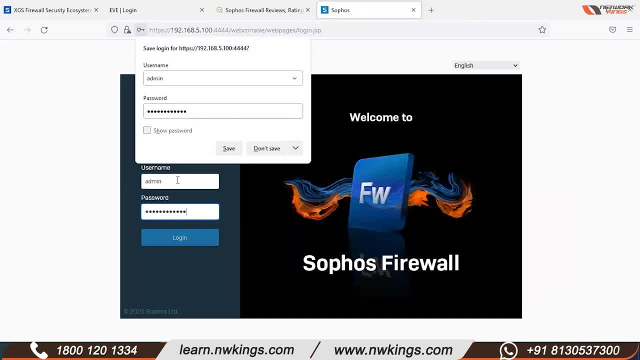 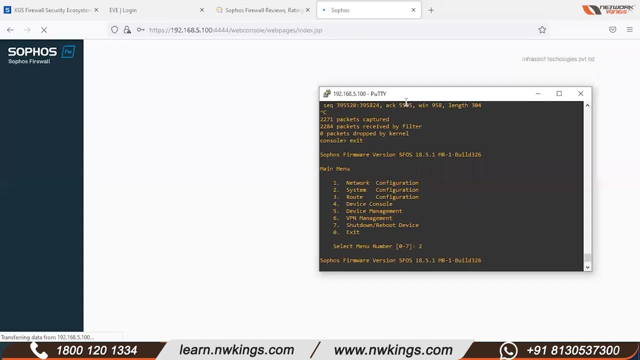 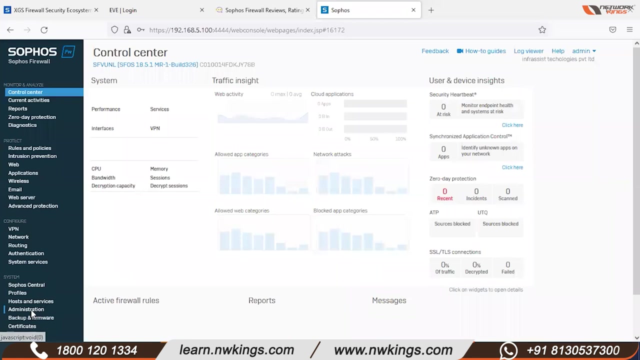 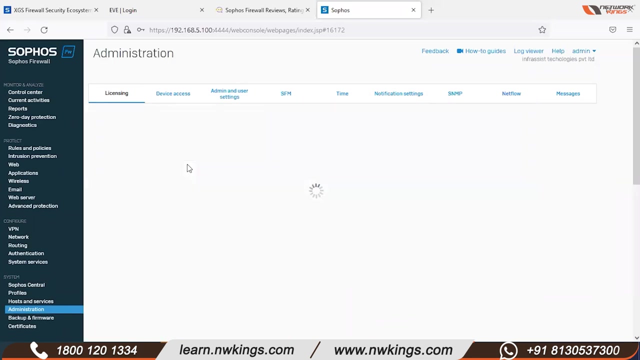 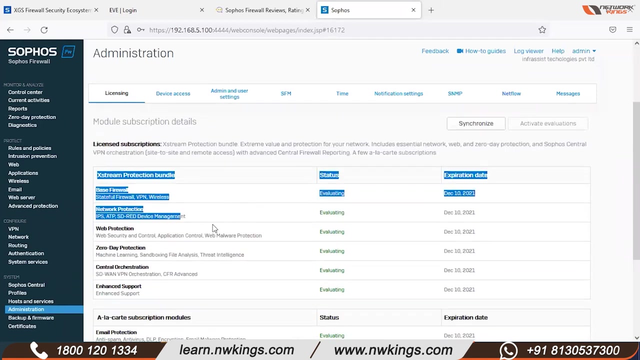 Let me log in here and show you the GUI. Okay, So our GUI is already set up, So we can see all the chips and all the backups. Now let's go to the computer. Okay, So the network is running. Let's see where it is. 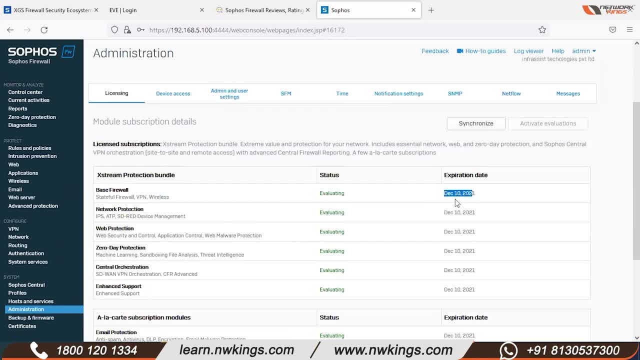 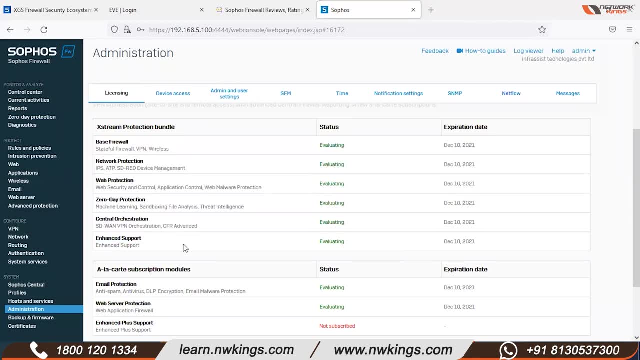 Okay, My last one will expire on 10th Dec. ie I enabled it on 10th November, so I will get all these features in 30 days. I don't get this one. I need an advanced license for this- but we will get this much in 30 days. 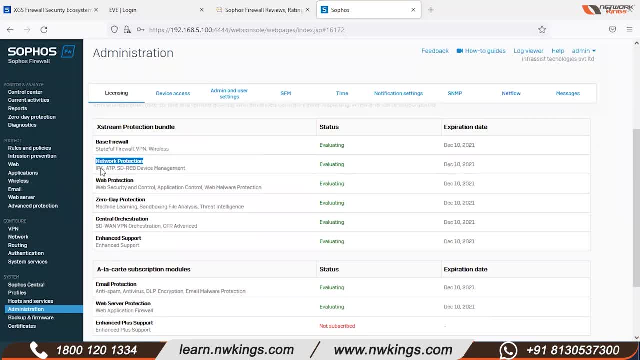 It will have a base license. Network Protection, ie the engine of IPS, is on that license. So you have to install IPS security. so we need all the licenses same way with all these things. So all these licenses are covered in all the modules. but definitely we will go into detail. 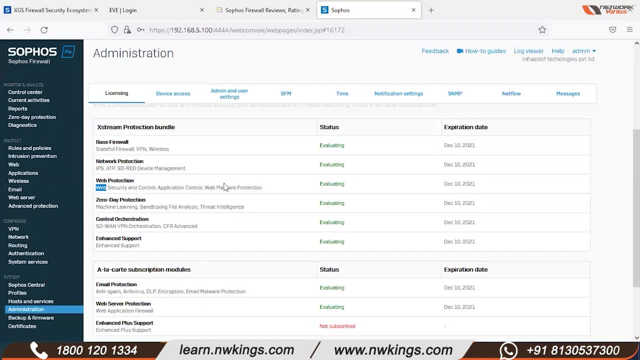 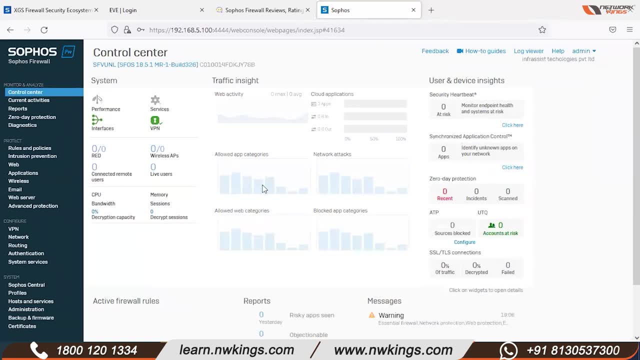 For now we can see this. So as soon as we will login, we will see the GUI of Sophos here. So here you have all the insights that you have configured from the Sophos firewall, Or you have configured it. If any traffic is going on, there are users, you will get all the insights. 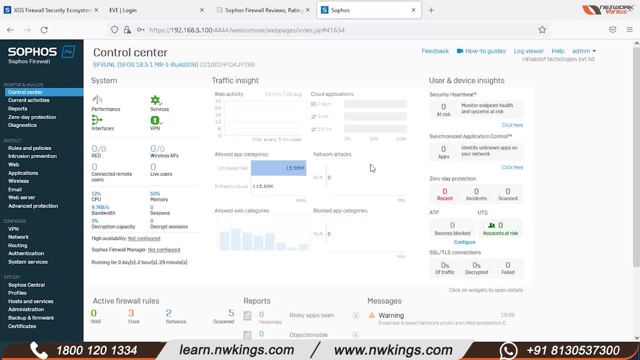 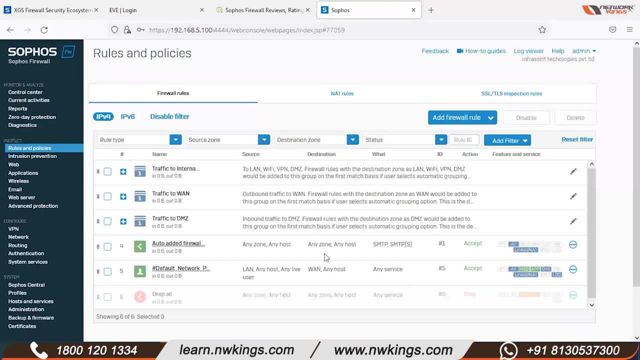 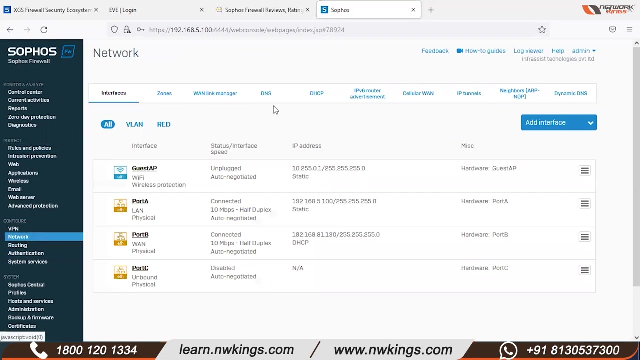 About this, along with the modules. we will go into detail: how to configure, how to configure the firewall rules- So these default rules come as you deploy on the firewall. So how to set traffic policies, how to enable authentication, how to configure the network, DNS, DHCP. 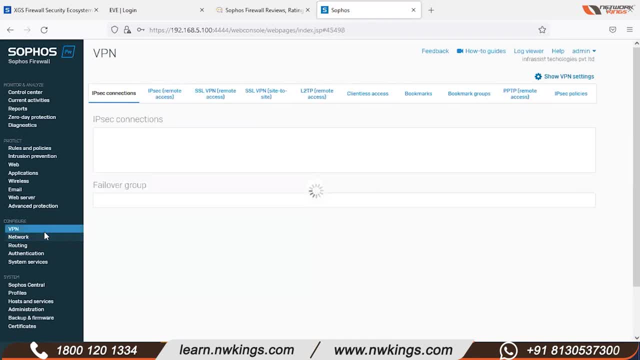 All these features. So we will see them one by one in the modules. How to configure VPN, we can also see it from here. We will configure it in this GUI. So those are also scenarios. There is routing, like how to configure routing. from the questions of many people. 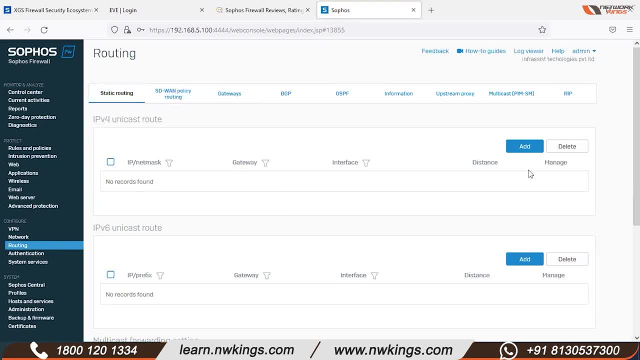 So from here we can do it from GUI. If there is any static, then how to do static configuration. we will also see that in a topology. We will see BGP, OSPR, RIP and the other tabs that are visible here. we will see them one by one. 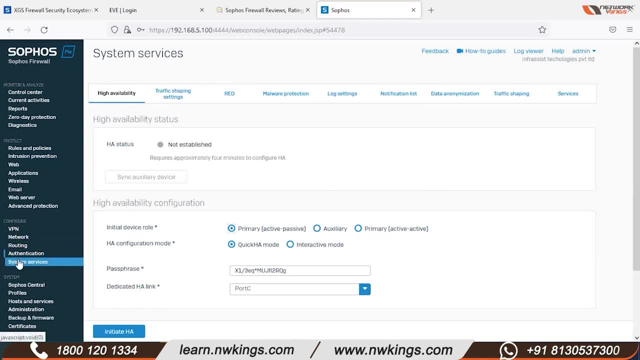 Here you have the system service. we have gone through this in the configuration. there is also system services. That is what is the software. if it is configured in HA, then we can do it from here. We will also go into detail about this in the modules. 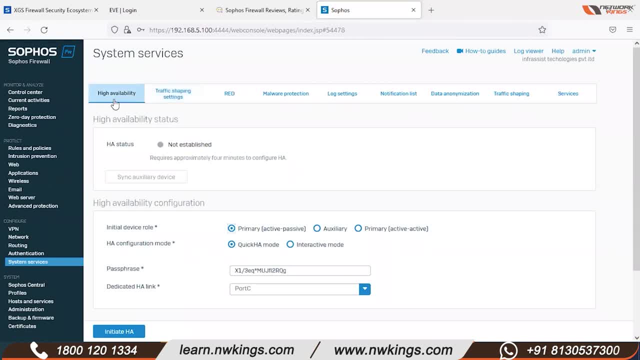 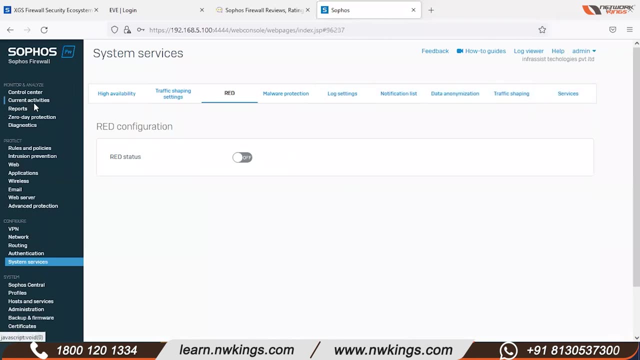 How does HA work? Where is its use in negotiation? How to deploy? Is there traffic shaping? Is it red? Is it a red device? How to enable, How to configure? All that configuration is, from here, All right. Coming to the current activities, for example, if we click here, then we will see the users here. 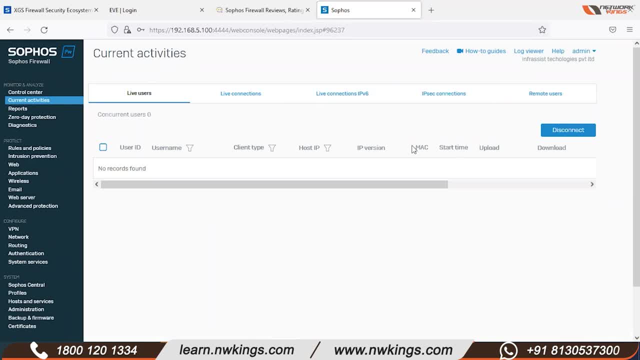 If there is an authentication module and we have followed it properly, then we will be able to see all the live users here with live connections. If there is an IPv6, then we will be able to see it. IPv6 connections- remote users- are connected. we will also be able to see that. 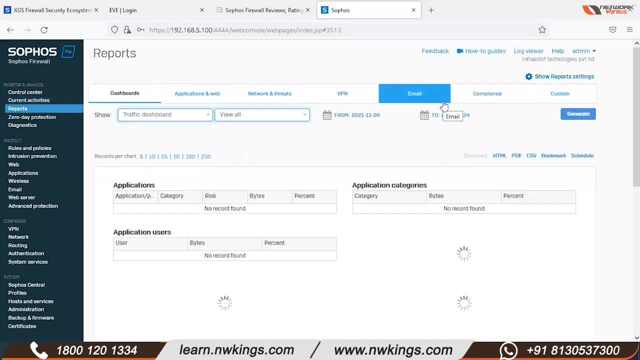 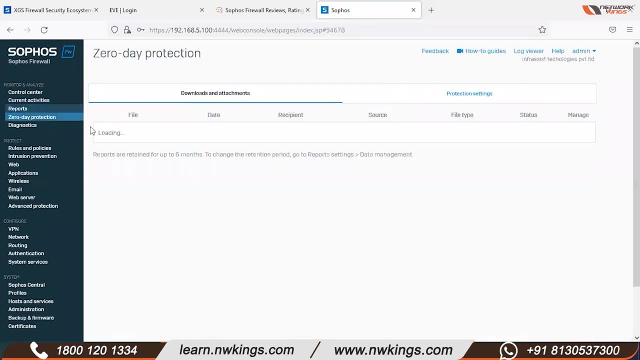 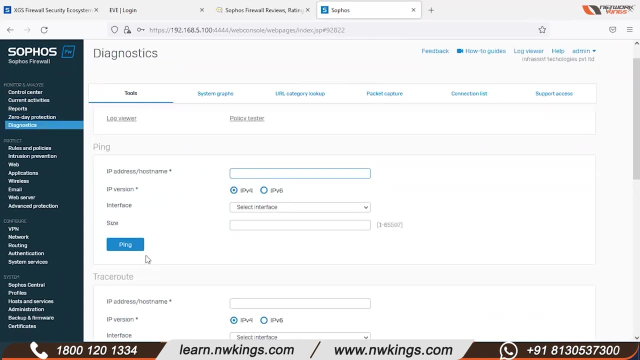 In the report session we will see all the reports in the module as well. Like our length, module is full reporting, so it will be covered in it. There is zero data protection. As I know, Sandstorm technology uses it. Diagnosis: that is the basic, networking, our tools, ping, test route. 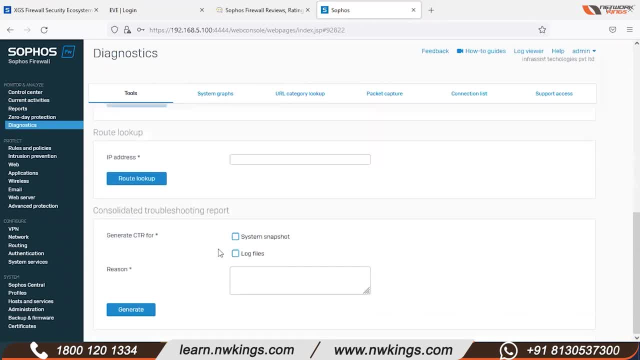 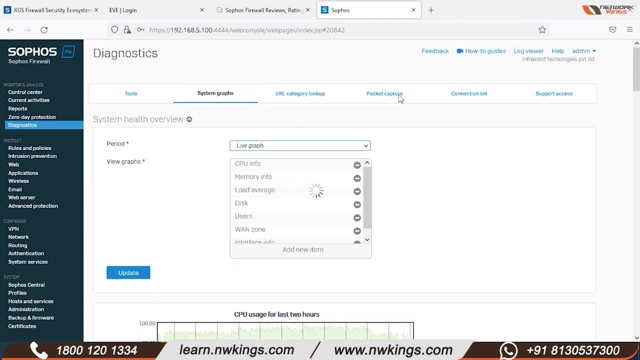 To troubleshoot the network. we will definitely use this. You can see all the system graphs from here. You can look up the UI Packet capture. I will tell you how the packet flows from your user's system firewall to the internet. 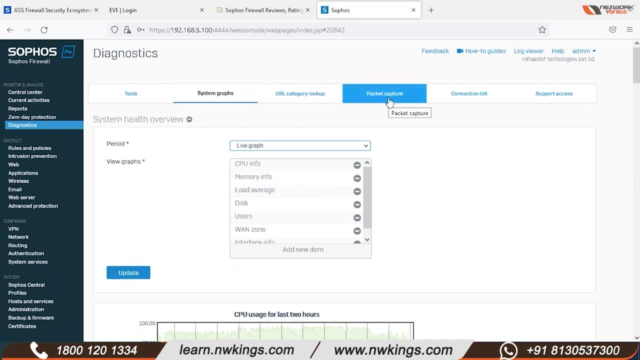 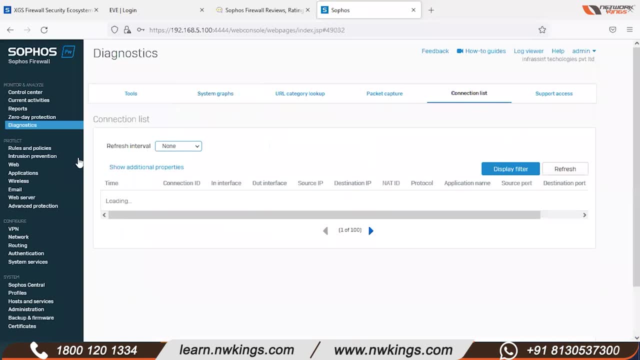 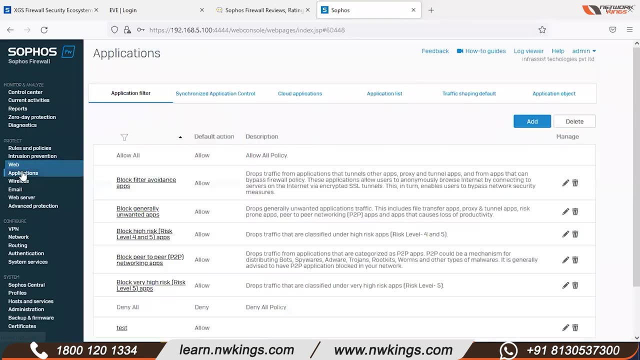 We will see that And there are also all the packet captures that we will see. We will see LAN 7 in the starting. We will see the connection list on the firewall, IPS policies like web protection, email protection, application protection, as I told you. 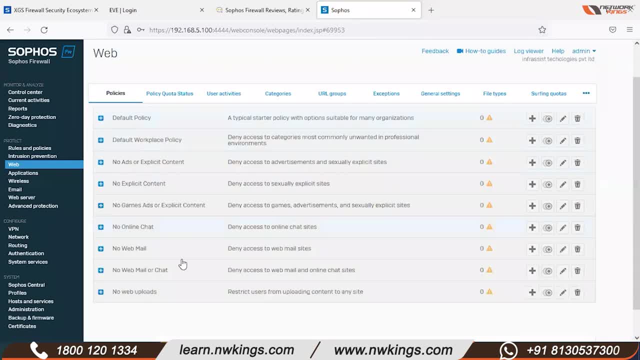 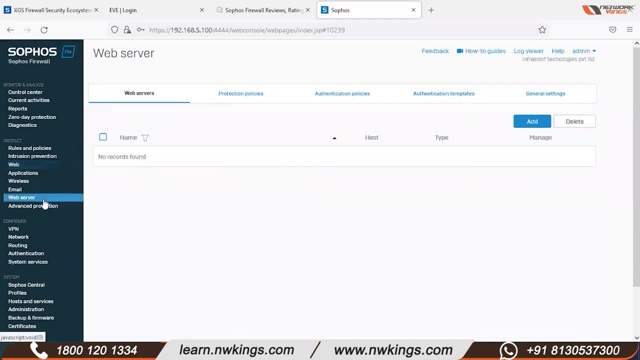 So how to create these policies here, The default policies that are available. we will go through them. We will create a new one. We will apply it on the users. We will see how it works. We will go into detail about the web. 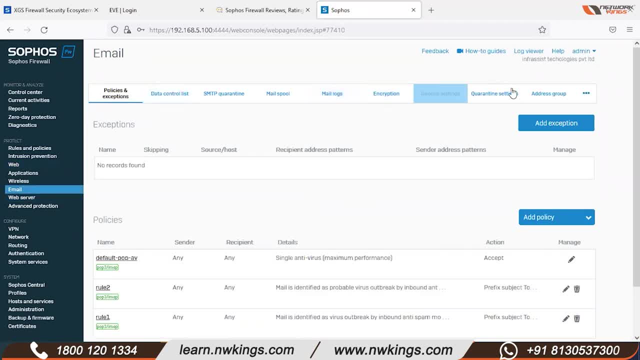 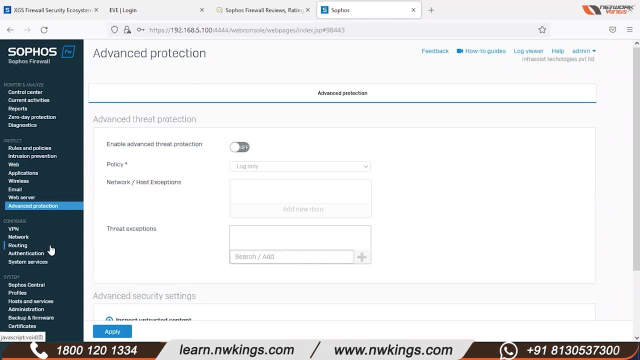 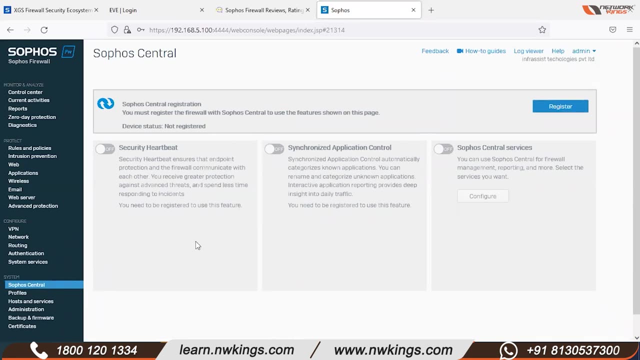 Email protection, as I told you in the module. So here we can configure the entire email protection. We will see the scenarios where we can enable it, In which scenarios. So for central, like I told you in the module, how we have to integrate it for synchronized security. 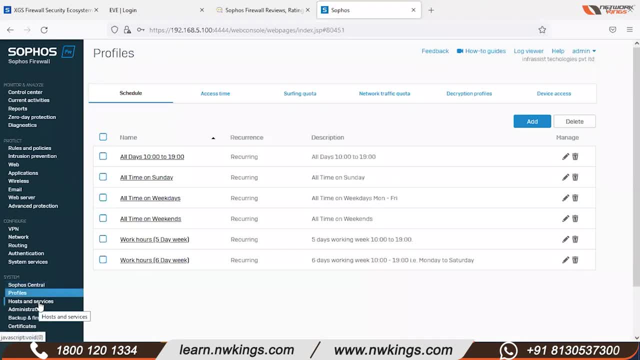 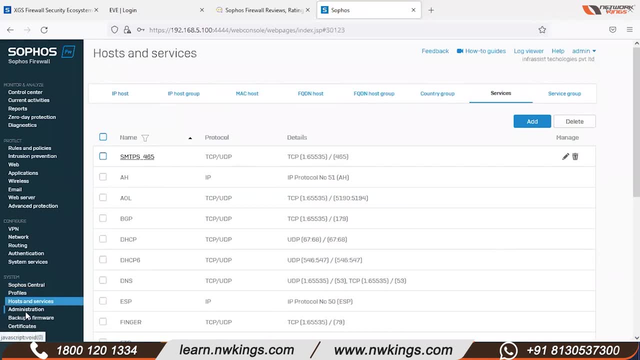 We will see that. How the profiles are created on the firewall, The policies and profiles are created. We will create those services here. There is a cover-up in the modules, No worries. So here in the administration you have license device access. admin. 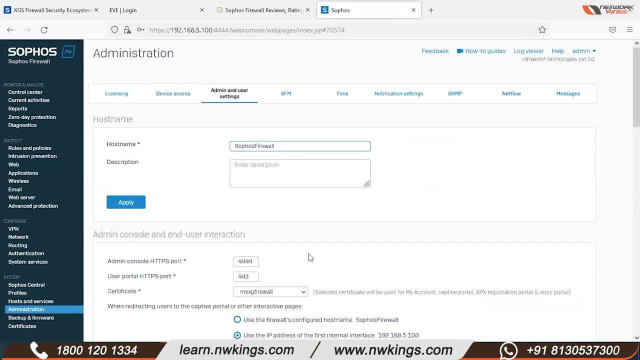 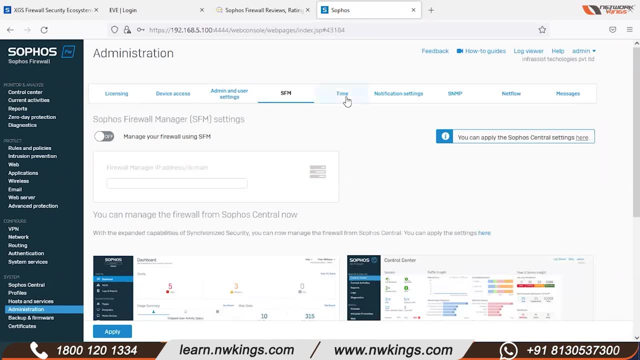 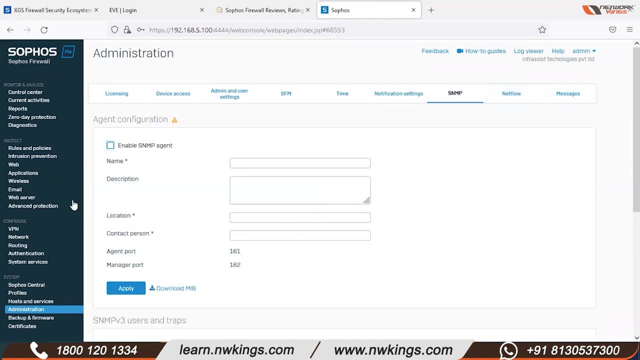 So, like we call it, web admin console, So we will discuss it completely, We will navigate it completely: Where and what we will configure. What is its purpose? Alright, Time settings notifications. if there is To configure notifications, So we will see that too. 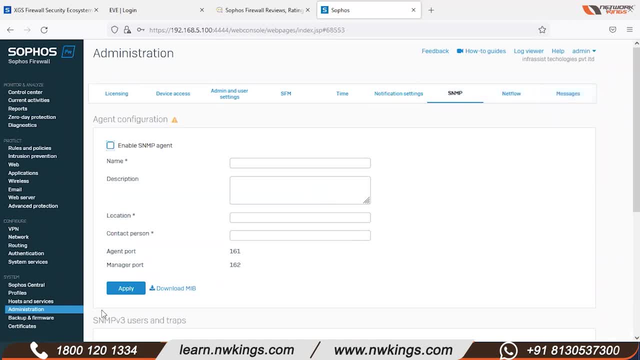 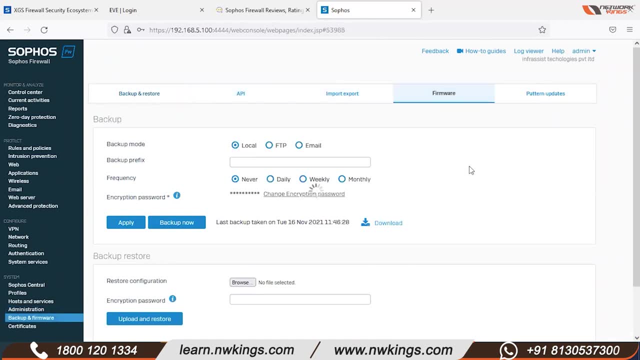 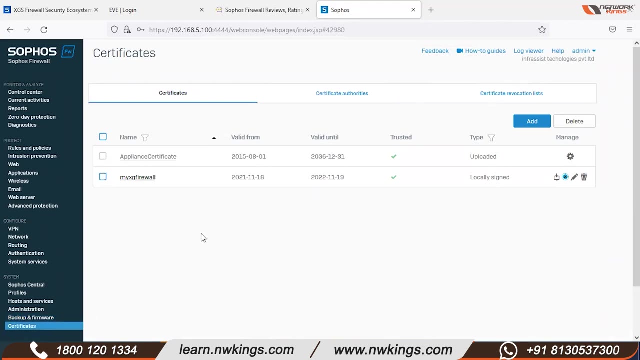 SNMP, NetFlow and custom message. we will configure, Then we will take backup, We will restore the backup. How to restore? We have to take backup. We will discuss about firmware, About pattern update too, And certificates. So if we want to intercept the software, 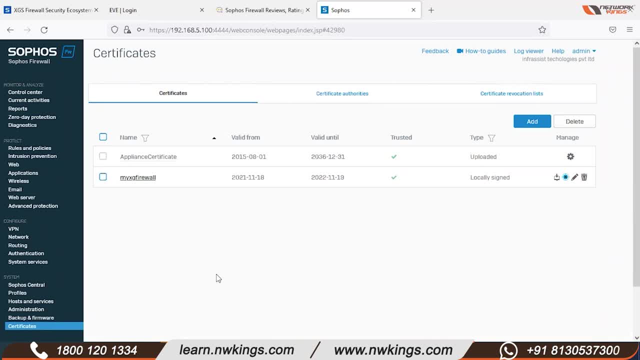 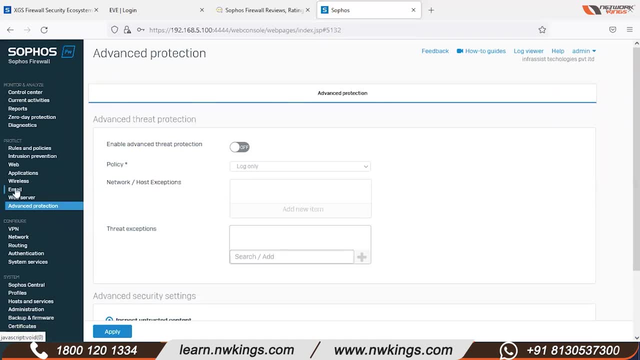 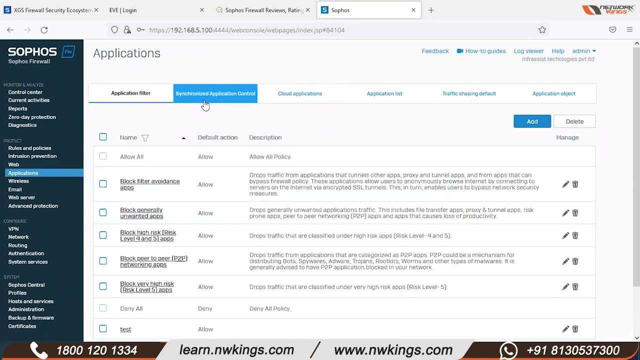 So we will see how the certificate authority is used. Okay, Here we will enable advanced protection Later on. And one last thing: Like there is an application, So like I told you in the modules That synchronized application, control, Cloud application. 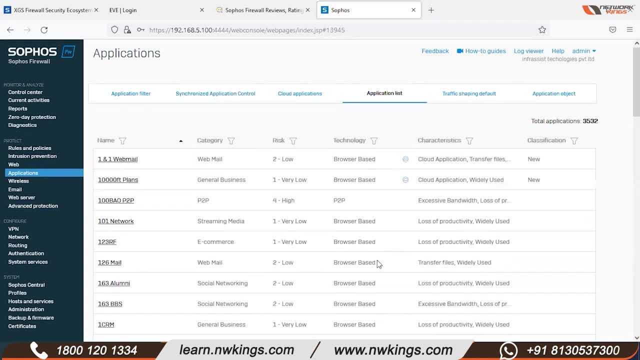 Application list. We will see that, Like I told you in the modules, It is the same, So we will go through it. How to configure it? Okay, How can we utilize each and every feature? We will see that. Intrusion. 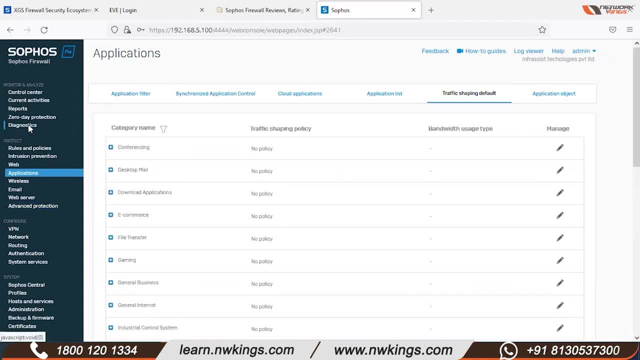 Prevention. Like there are dose settings. Like I told you, Dose can be applied for protection, Spoof prevention can also be applied. If you want to stop spoof prevention too, Then it can also be applied. Followed, We will see. 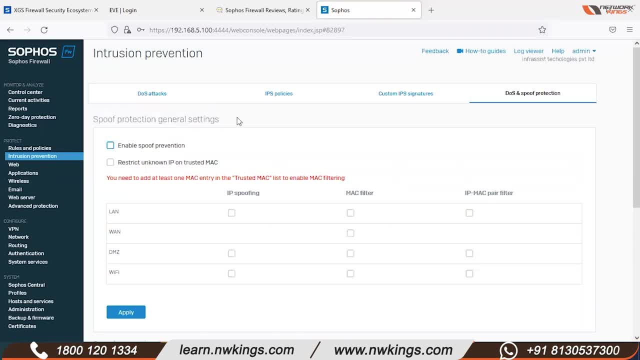 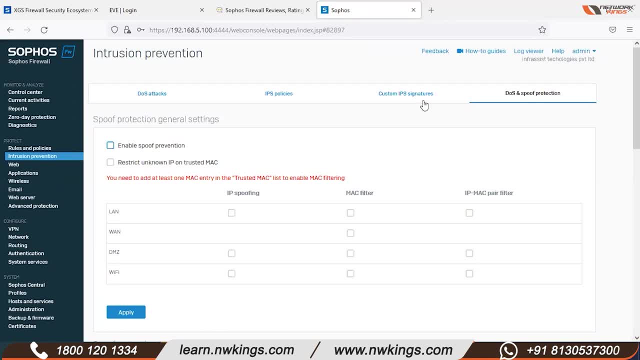 How we can meet in that, How we can meet in that, How challenges come in deploying firewall And how we can resolve it. How we can up and running and secure most. How we can up and running and secure most If there is some new deployment. 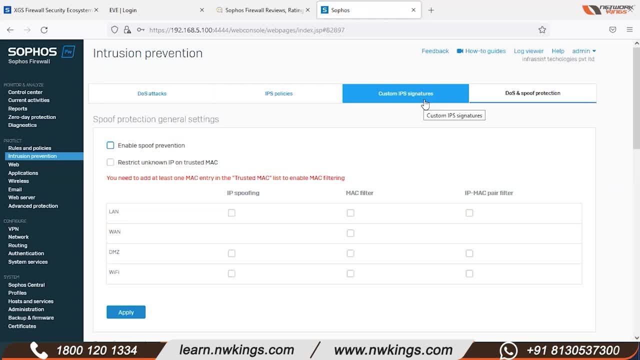 Then how to do it, On which mode? In gateway, In proxy? We will discuss a little bit in SSCI. We will discuss a little bit in SSCI. We will discuss a little bit in SSCI. Most of where sім. 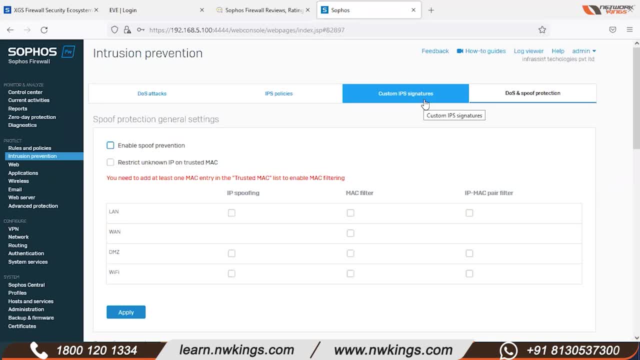 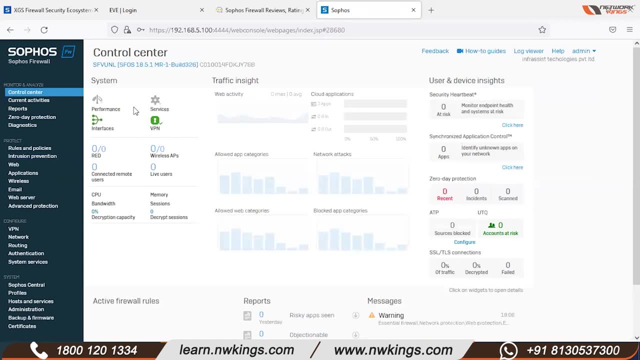 If there is a different file in comparison, Then we will discuss its Most of where SOM6G we can deploy If any other vendors Compilation. If there is another firewall, Then we can deploy it. Then we can deploy that. If we have another firewall in comparison with other vendors, then we will see how we will use Sofos as an alternate. 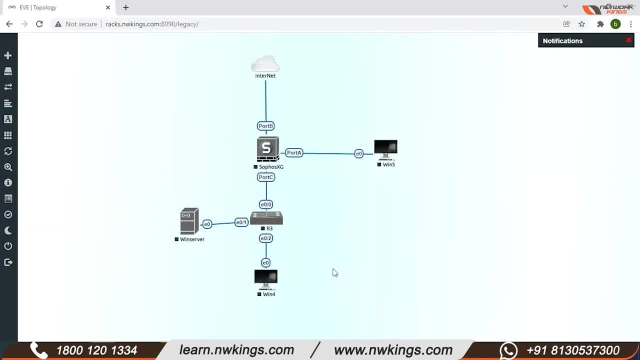 Alright. so what we will do in the next session is that we will initiate installation in VM, That is, we will configure the entire firewall from the PC. that is, we will do the initial setup and bring it live. So there will be a server that will authenticate all the users. 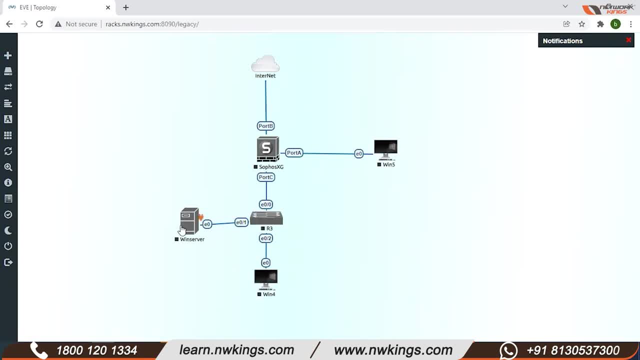 There are different departments. there is a land zone, there is a DMZ zone, for example, and there is a custom zone. All the servers are kept on the DMZ zone. There are different users in different departments, in which different policies have to be applied. 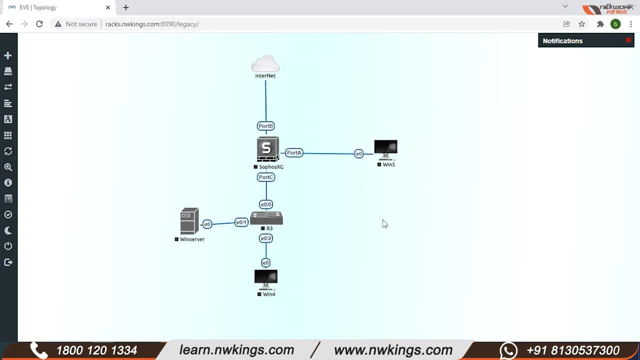 Different policies have to be applied in HR. different policies have to be applied in sales. different policies have to be applied in web filter and application filter. QS policies have to be applied. surfing quotas have to be applied on the users or on the user group. 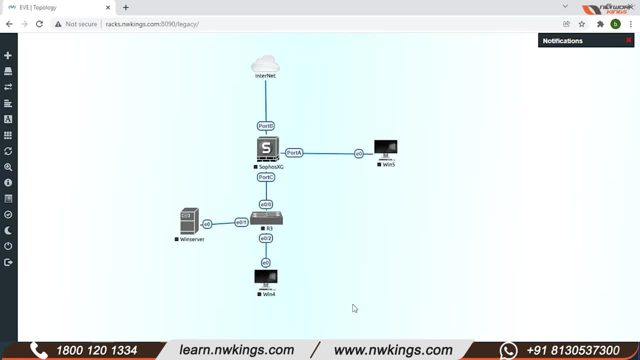 There is a group here. there is a group here. There should be a bandwidth policy applied on it that this group should get 5-6 Mbps. There are many such scenarios. One by one. along with the modules, we will configure it and meet it to see where Sofos Firewall can be useful. 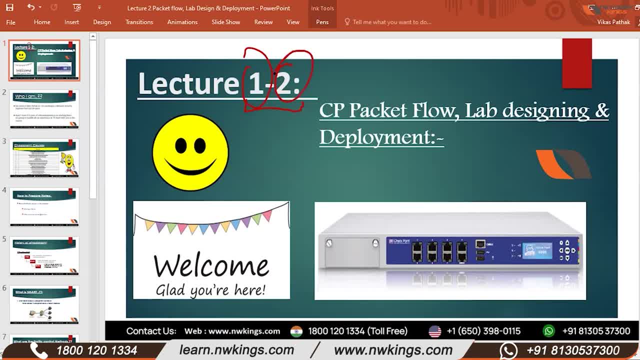 We will cover the first lecture plus, we will also discuss some things in the second lecture. And, as I told you in the last lecture, this is the image. this is the image of the checkpoint hardware. If you go to the industry, if you get a checkpoint device to deploy, then you will get a box like this: 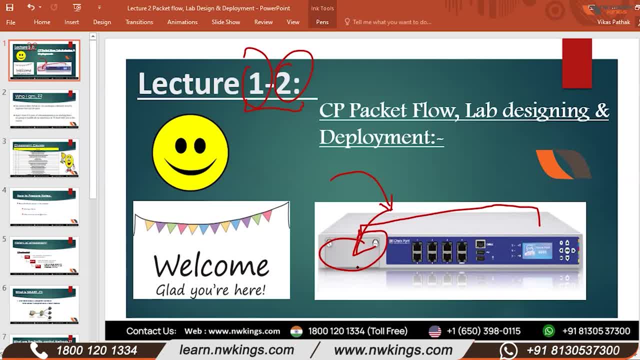 This is open. here you can put a NIC card, whether LAN GIG or anything right, And this is your normal LAN port. this is the console. this is the USB. this is the LEDs. this is the navigation. Okay. 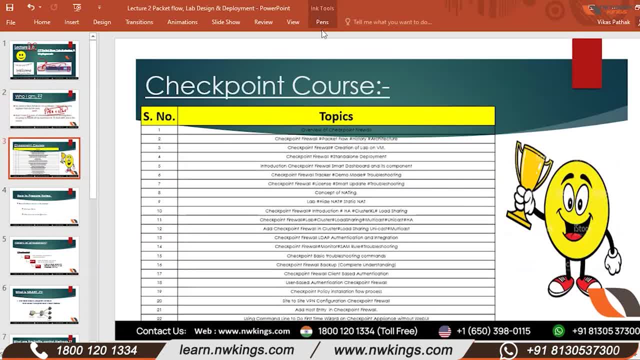 This was the introduction of the course which we will discuss in this course Okay, So if I talk about today, then our main focus will be on this section Okay, In which we will study packet flow, history, architecture, and we will read it in detail. 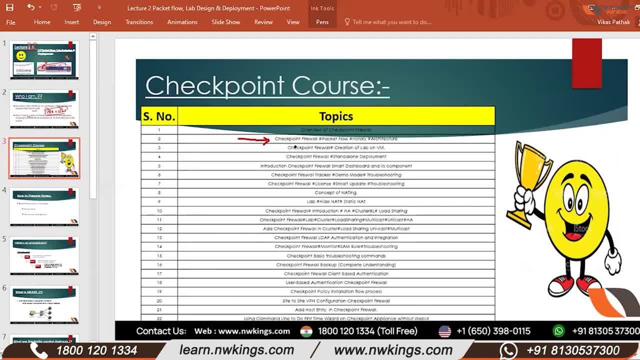 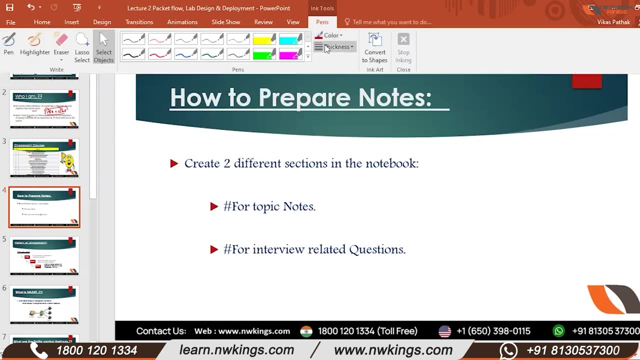 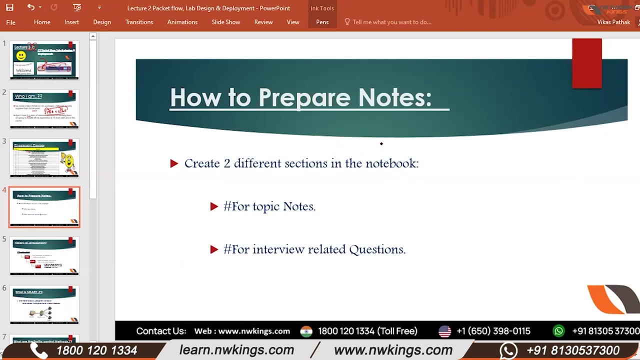 So that after today's session, if anyone asks you any question on packet flow or history or architecture, then you can close your eyes and answer. I will try my best to convey this message to you all. Okay, Okay, One of the major points I will say is that many people have a doubt whether notes should be made or not. 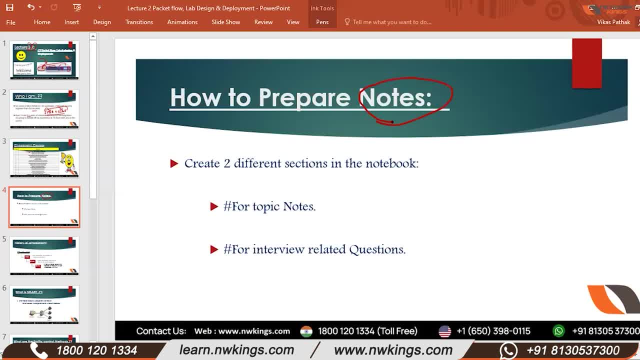 Okay, And how to make it So. first thing, that you have to make your own notes. Okay, You have to bring a copy. You have to divide that copy into two parts. Okay, I am telling you that if you follow this approach, believe me, you will never have to take the. 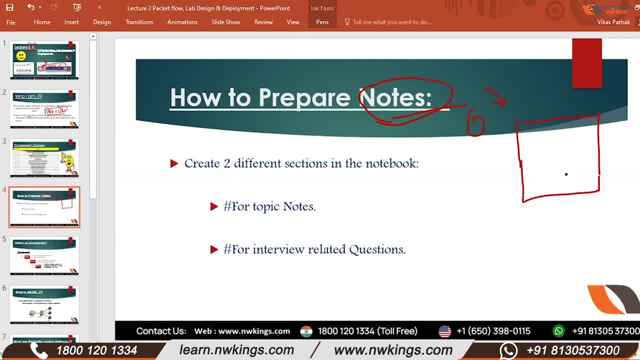 check point classes again until you are in the network security And this approach is followed by me and my friends. And, believe me, we will never have this notebook on my desk, but I will never open it and see it. Okay, Until and unless I have to make sure that I have not said anything wrong. 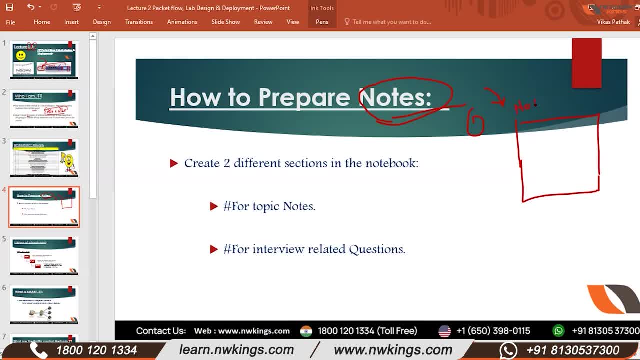 Okay, So what you have to do is you have to take a notebook. Okay, Now assume that you have taken this notebook of 100 pages. Divide it into two. The major part, that is, the 70 pages, will be notes of your topic. 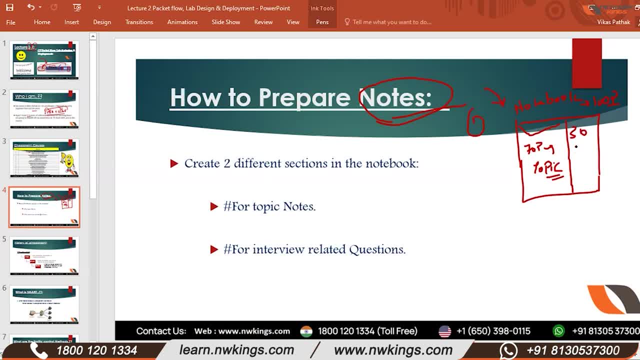 And the 30 pages will be of your interview questions. Whose Interview questions? Interview questions we will discuss immediately after each topic so that you get the idea that whatever we are reading, how to say it in the interview plus how to implement it in. 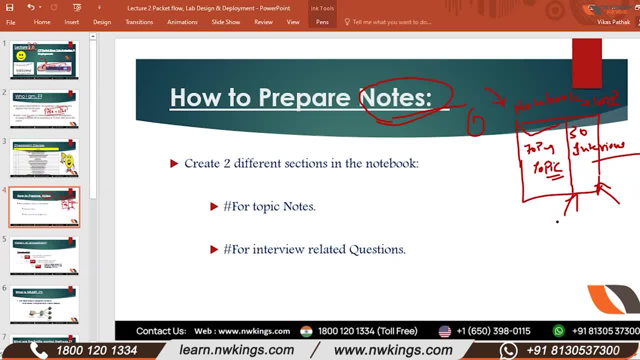 real life at the real industry level. These two approaches will follow us. Okay, So you have to make two sections. The first section will be for your topic notes. The second section will be for our interview related questions. Is this thing clear? 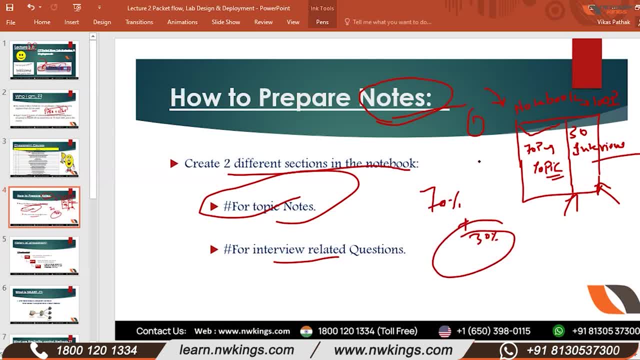 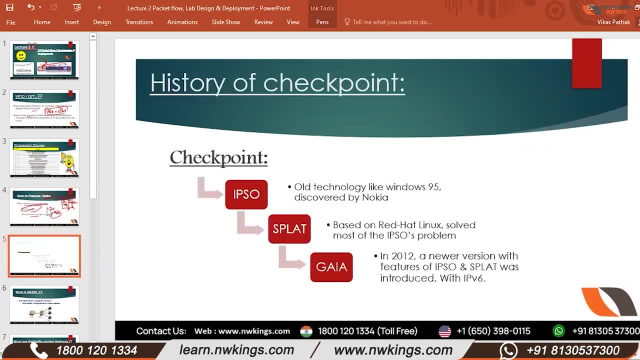 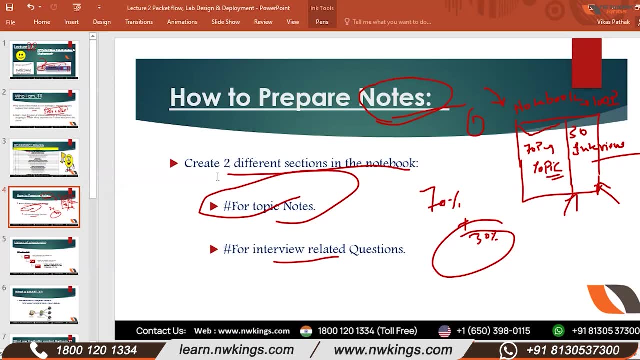 Yes, it is clear: Keep participating, Otherwise I mean, I mean, come on, these things are clear to you, so I hope that you will not get caught up in the class. If you have not taken a pen and paper this time, then maybe you have taken it from next. 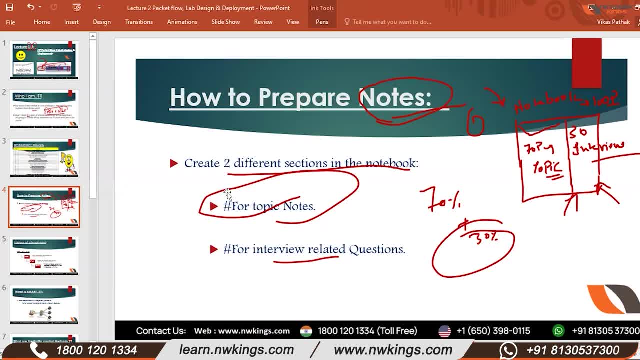 time and this thing is following the rigorously, because the course you are getting paid from you, the time you are spending, you will get the value from here. Okay, If you are not following this thing, maybe 10 days, 15 days, 20 days or a month, you 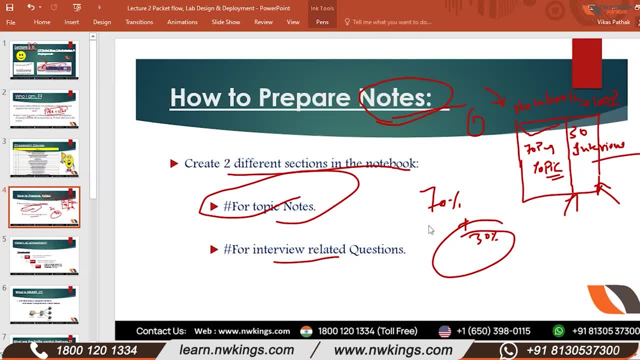 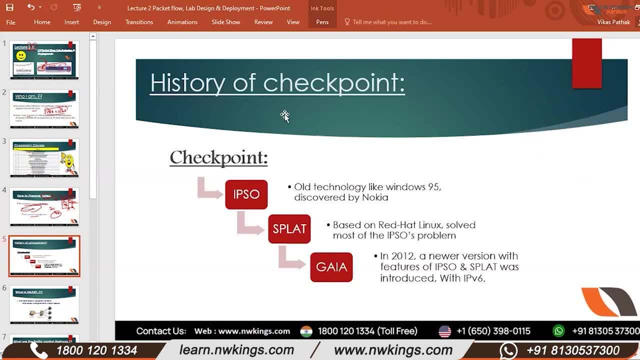 will remember things. well then, slowly, slowly, slowly, they will fade away. Then one day you will have to give a class again. So again, these will be your resources, Okay. Last time we talked about the history of checkpoints, Okay. 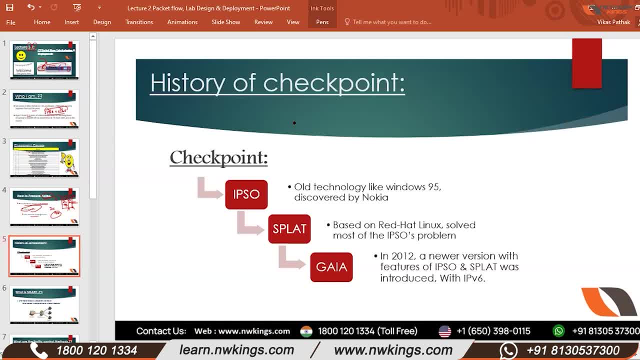 Checkpoint came in the market, How it came, What things it brought, What kind of modification came. This is calculated in history, Although this question, this slide, has no relevance in your industry, But in the interview these things are asked many times. 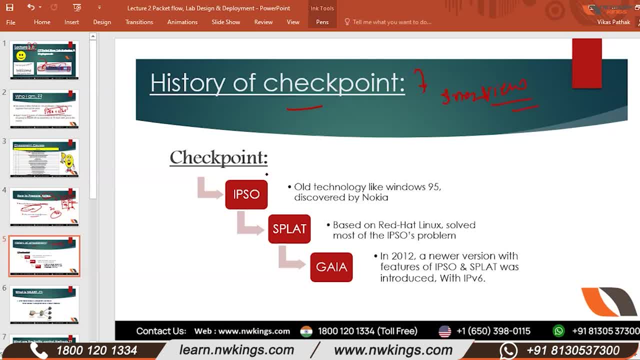 Okay. So the first version of the checkpoint was called Ipso. It came in the Ipso market. Very basic, Very basic interface. Who of you have worked on Windows 95?? Has anyone seen it? Has anyone worked on it? Maybe when you go to the cyber cafe you may have found it. 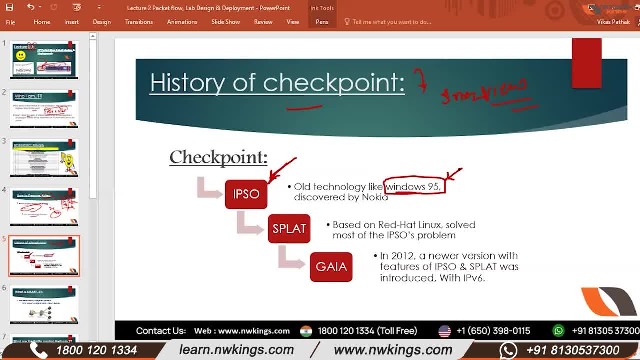 Yes, So I remember when I used to go to the cyber cafe. at that time I had neither a computer nor a laptop, So to check some emails that is, we were around in the eleventh class or maybe in the tenth class. 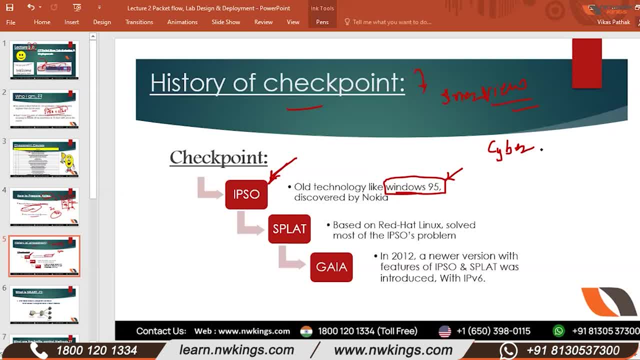 So we had not made an email and we were interested to go and check if there was any new email or not. By the way, there was no elephant, but we were interested. So what used to happen is that we used to get that computer. 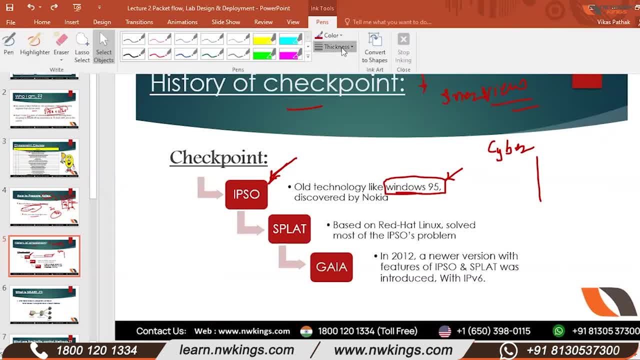 We used to get the computer there. That was very basic. If I compare it with today's computers, it is ok. Simple is this monitor Below the taskbar, and here is the start And what used to be the cursor. it was a very big cursor. 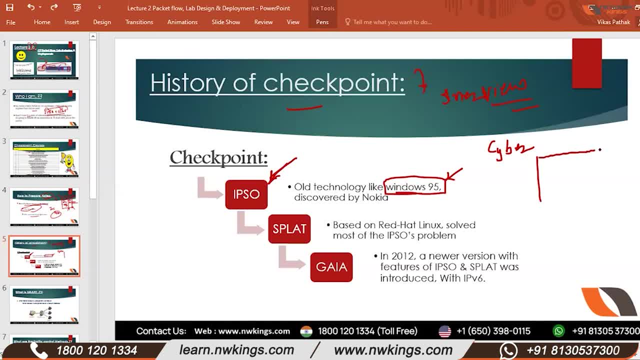 Something of this type, And navigation is very easy. Everything is simple, Everything means that it is very good, But what was the problem? Everything was very simple, It was very simple. What was the problem? Windows 95 had a lot of vulnerability in it. 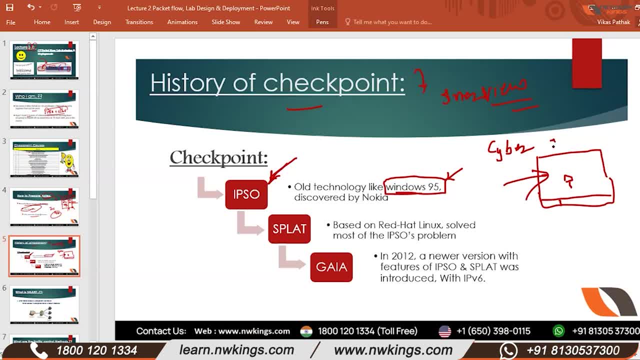 Suppose, if you open a Telnet port on it 21,, then 90-95% of the chances are that if you are using it in any enterprise, then this port will be attacked. It has a lot of vulnerability, although it was very simple, but it was vulnerable. 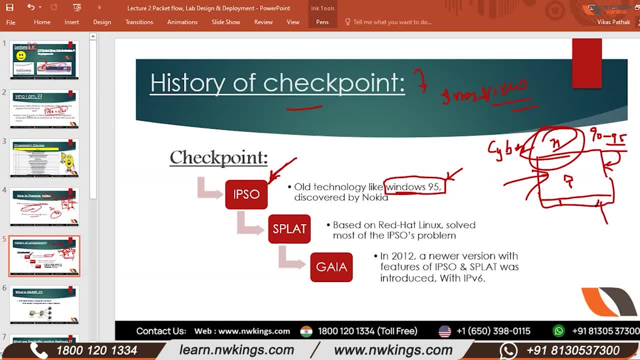 Plus, when high-intensity work was performed on it, on Windows, then somewhere its CPU utilization or other resources were high utilized. So because of this, Microsoft had to obsolete it Gradually. they came to the new version, then XP, then Windows 7, and then 8 and then 10.. 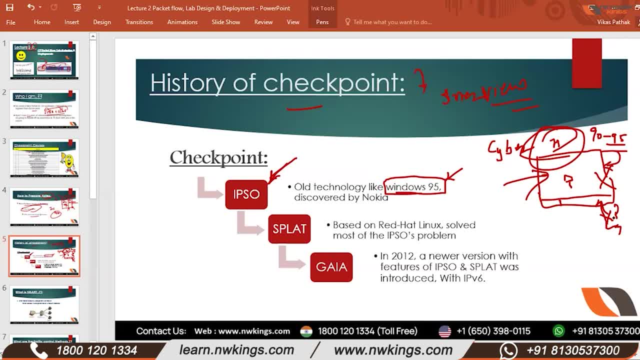 Now they have reached 11.. So, if I talk about it, 95%. There was a major rollout on XP because there was a version in between. They also brought Vista, Windows Vista. That Vista was an enhanced version of 95. And after 95, they brought XP. 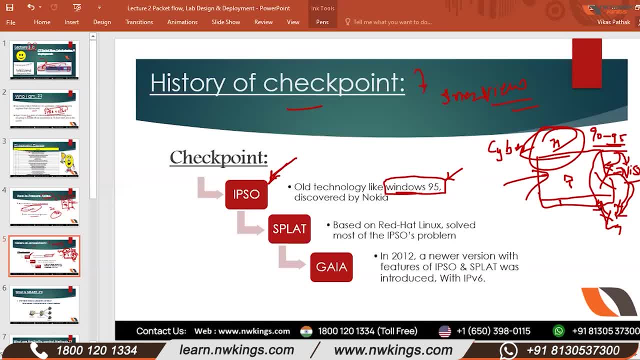 Now, if I talk about 95 and XP, there was a difference between ground and sky. Similarly, if I talk about IPSO and SPLAT, they made a difference between ground and sky How? First of all, they brought Red Hat in between. 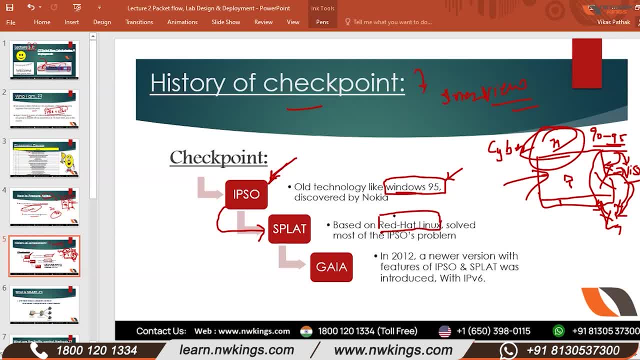 The kernel they were making. they made it on Red Hat. Now there is Linux. First of all it is open source And if I compare, then Linux is much more secure than any other language. But if you tweak a little bit of security in it then it becomes more extensively secure. 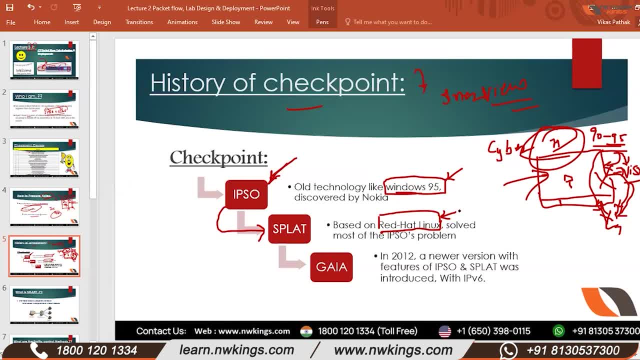 Linux provides a lot of features. Okay, So all the problems of IPSO that Nokia introduced in the market to IPSO, all its problems, were mitigated in SPLAT, In which In SPLAT That is called SPLAT And the biggest advantage was that they developed SPLAT on Red Hat. 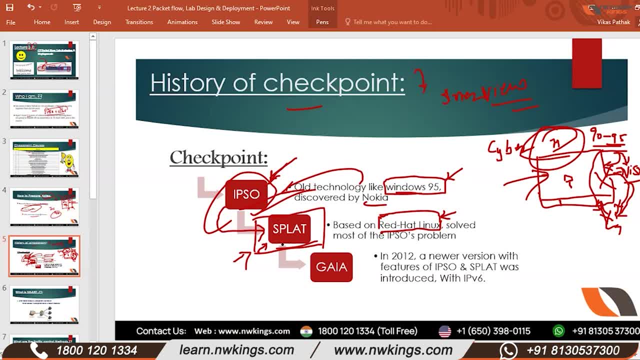 So because of this, security features and the performance of SPLAT was much, much better, Much, much better than IPSO. Okay Now, SPLAT was a new version, like XP, But still there were some problems in SPLAT. The GUI interface was not very interactive. 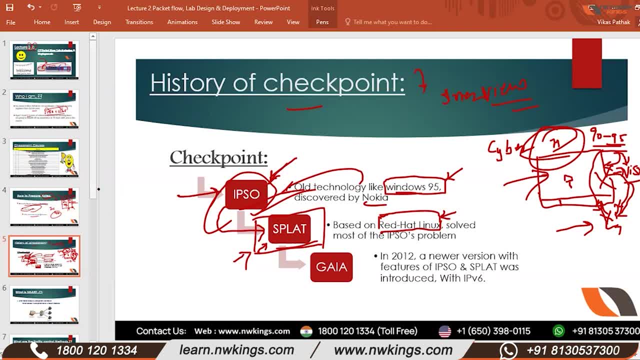 And at that time- if I talk about 2010 or 2011-2012, there was a trend in the market. at that time It was the next generation firewall, That we have to bring the next generation firewall in the market. 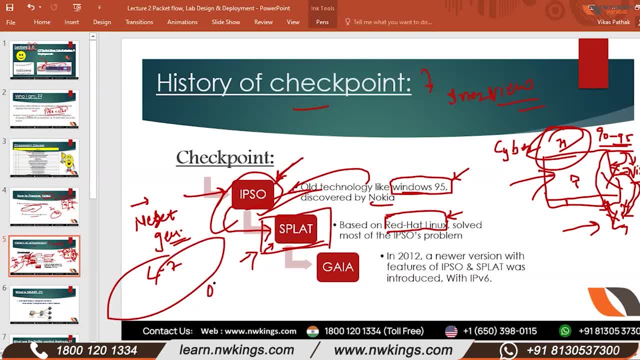 Now, what is the next generation firewall? The one that works on layer 7.. We needed firewalls that work on OSI layer 7.. So to work on that level, we had a very good graphical and stable graphical requirement, which SPLAT did not have. 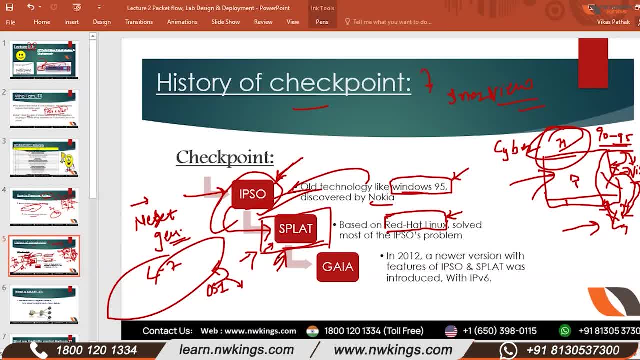 So if I talk about the SPLAT of the checkpoint, then it was not able to perform the work of layer 7 accordingly in the market. Okay, So what did the checkpoint finally do in 2012?? It brought a new version of the checkpoint. 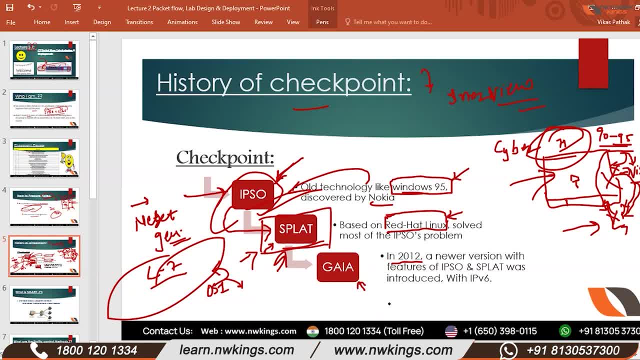 That is called Gaia Okay And in which they analyzed both of these versions And checked what are the vulnerabilities, what are the issues that are in IPSO and SPLAT. All those issues were mitigated In Gaia Okay. 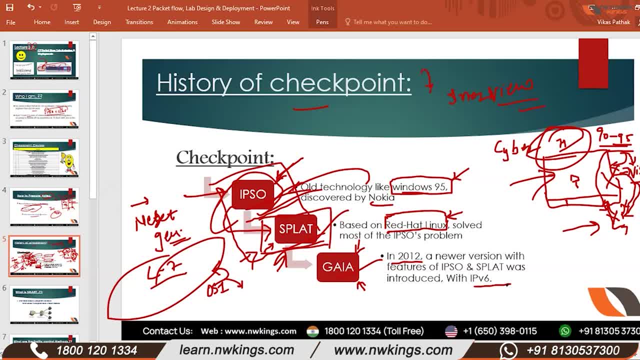 And after doing all this, IPv6 launch was introduced in Gaia for the first time in 2012.. Because at that time there was a trend that IPv6 will soon cover the market, But that thing is still going on. It has not been able to happen yet. 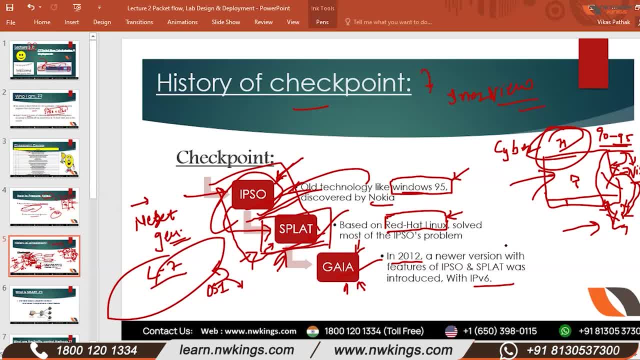 You will not get to see a major rollout until and unless you are not working on ISP. So these were the three stages of the checkpoint's evolution And currently, if we talk about it, then the work we are doing is on Gaia, On which 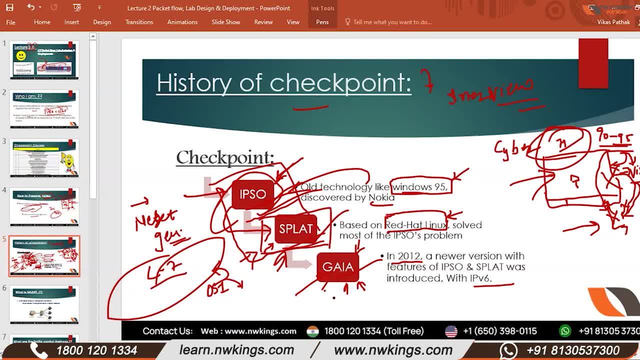 This is called Gaia Checkpoint, Gaia. Okay, Just like Cisco's IOS, the Gaia software is the checkpoint. Now, what had started was from version R75.. Okay, After that R76. Then R77. And R77.30 was a major version of checkpoint. 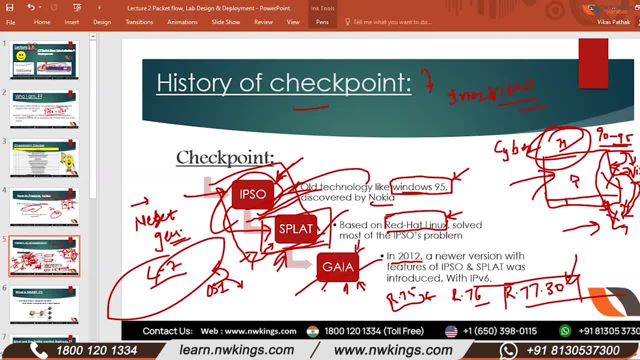 Which made the checkpoint very famous all over the world. Okay, Let me talk about stability first. So R77.30 was the most stable version so far. Now there is a different scene in R80. But if I talk about R77,, 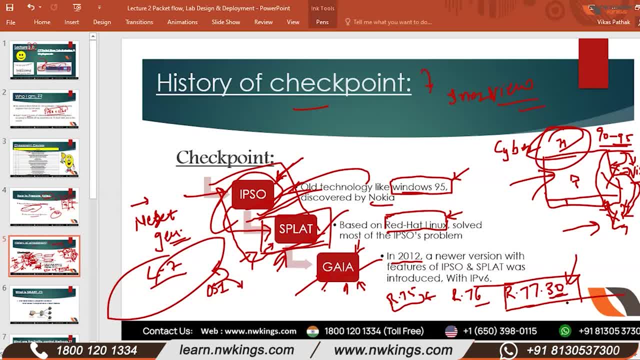 then the most stable version was R77.30.. And simplicity understanding of R77.30 was next level. Okay, This is why the checkpoint in the market, because the logical thinking while working on the checkpoint on the interface of R77.30,. 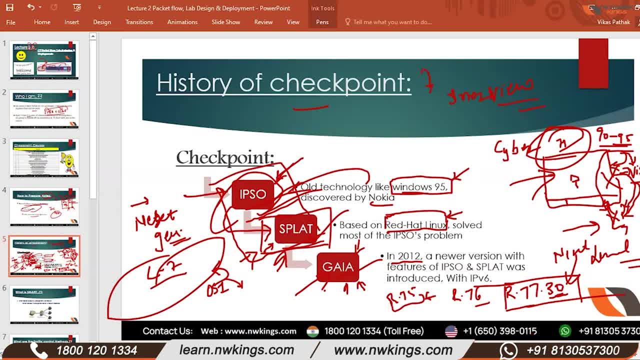 it was somewhere at a very high level when someone was working on it, So his logical thinking was at the very next level. He could think he could relate. I will show you. you will also be able to relate in the annual time. 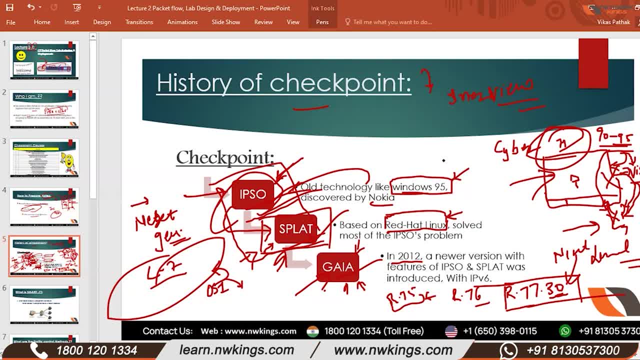 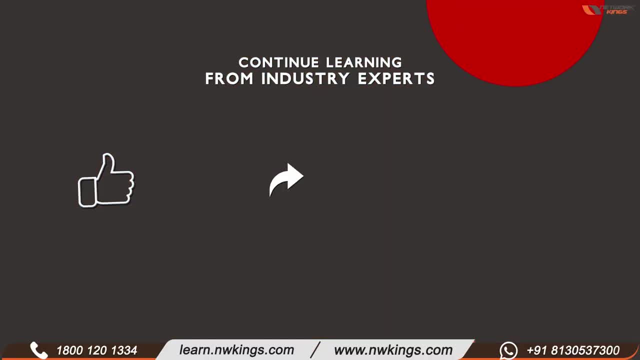 Okay, So the architecture we discussed, so now the relevance of it. if you go to give an exam, then there is no relevance in it, nor do you have any relevance in real life, but in the interview- Hi, you are watching the recording from one of our live sessions. 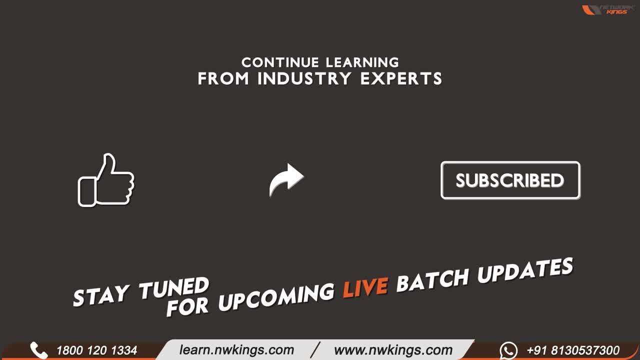 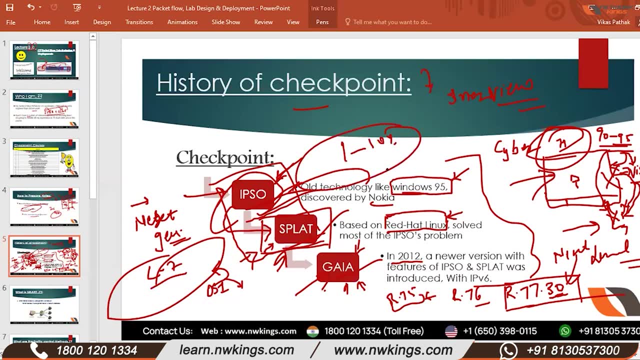 Hit like, share and subscribe for more future updates. Sometimes I mean, if I talk about 1%, there is a chance of 1 to 10% that the interviewer asks: how do you know about the evaluation of the checkpoint? Then you should know that, first of all, 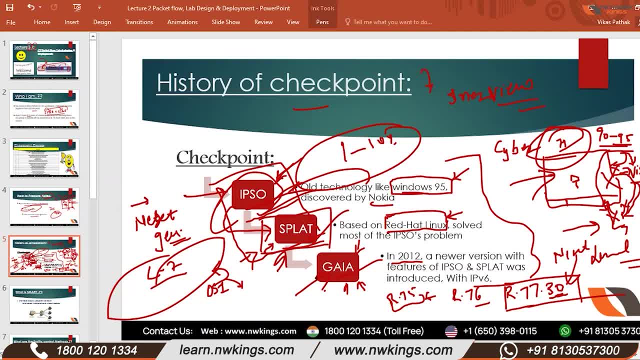 Ipsu came, then Splat came, then Gaia came. What happens many times? let's ask a comparison. What is the difference between Splat and Gaia? We will discuss that further. Okay, but before that discussion you should know about Splat. 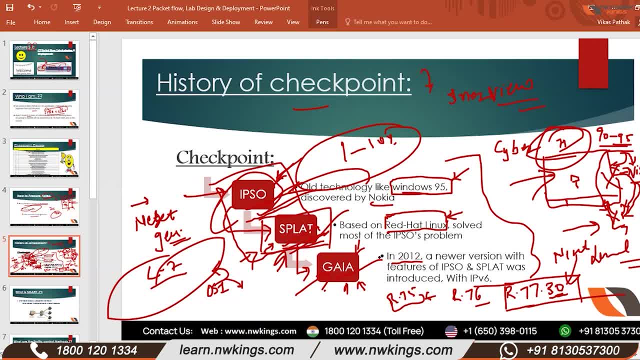 and you should know about Ipsu, who came after Splat and what things were there. Okay, Let's go. Yes, tell me, Sir, when did Ipsu launch? Ipsu? look, according to me, I don't remember any date. 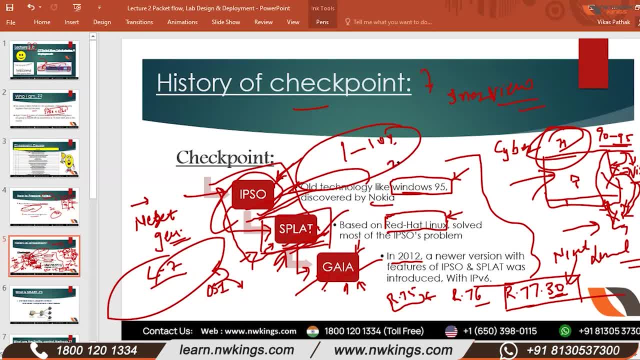 but I believe. I believe that around 2007 or 2008, it was launched. You can easily google it, but I have never done it. No one will ask you about Ipsu majorly, But yes, Splat was launched around 2010,. 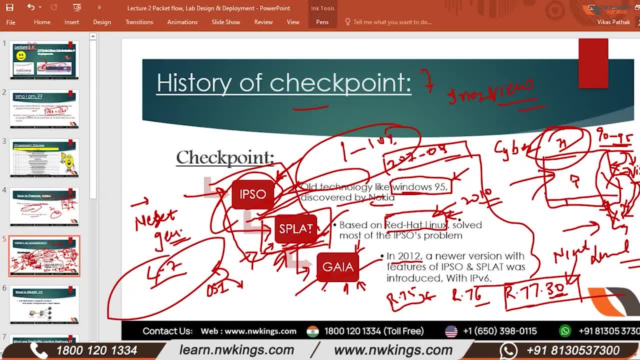 around 10 or 9.. Okay, sir, thank you. Okay, right, Hello, Hello, Hello, Yes, please. What is R4?? What does R mean, For example, .75,, R.76,, R.730.. 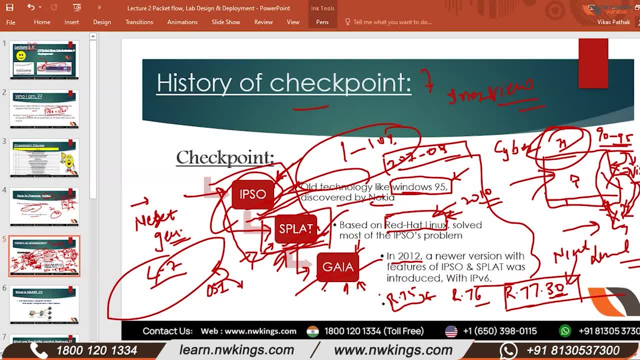 The version of this checkpoint is represented by R- Okay Okay. Before R, it gives its version number. R77.30 is running. R77, R75 is running Okay. It denotes the version by R Okay Okay. 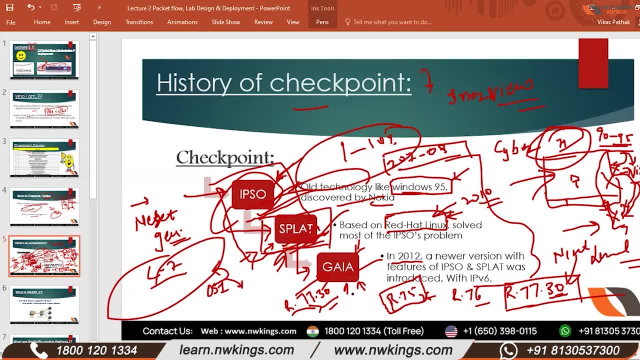 Okay, Okay, Thank you. No one will ask you about R, what is R and what is not, But you must remember that how this history has evolved. Okay, Vikas, which latest version is running? What is running now is R80.. 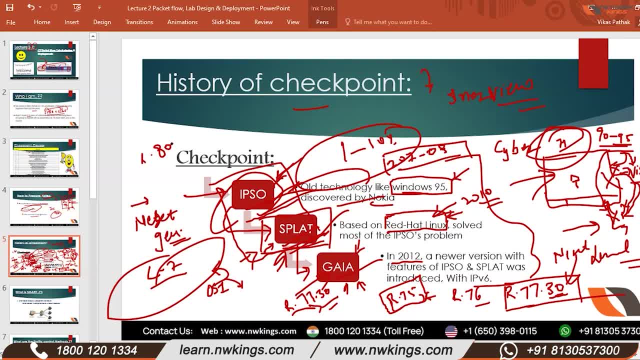 Okay, Where will we do lab? Yes, we will do lab on R80.1.. We will do lab on R80.1.. I am noticing many major changes in industry, which is R80.40 has been rolled out, because R80.40 is also very stable version. 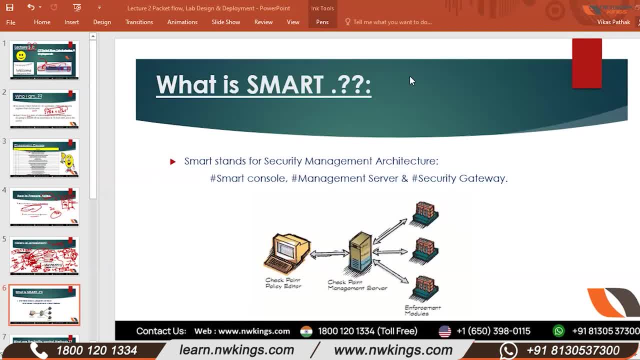 Okay, So we will talk about how the architecture of checkpoint is Okay. In last class I gave brief introduction, But today we will not read in detail. okay, So that you people will never require to read this topic again. The first thing is that there is an acronym for the architecture of the checkpoint. it is called smart. 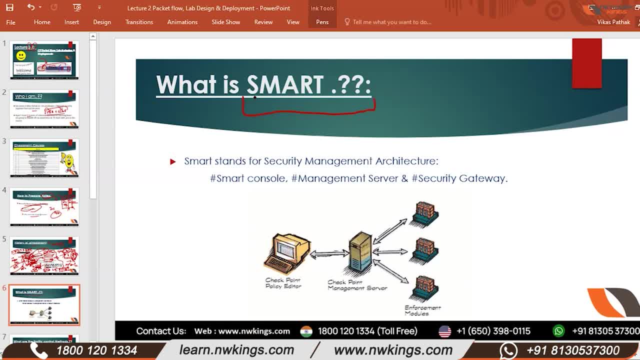 What do you call it Smart? Now, why do you call it smart? Because it is smart. Believe me, Like you guys are smart, similarly its architecture is also smart, and in smart, S stands for security, M for management, A for architecture. 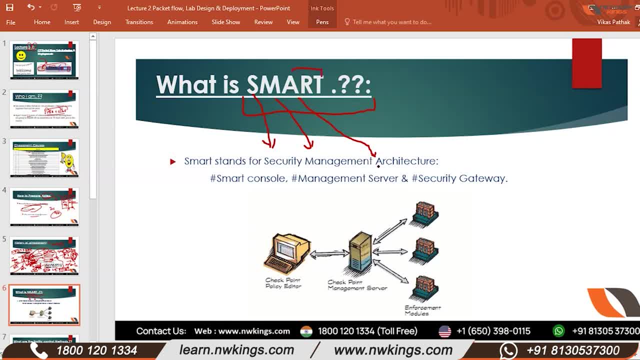 And these three alphabets are taken from the architecture. Okay, So whose smart acronym is it? The architecture of the checkpoint? If someone asks me what is the architecture of the checkpoint, I will say it is called smart, And the full form of smart is security management architecture. 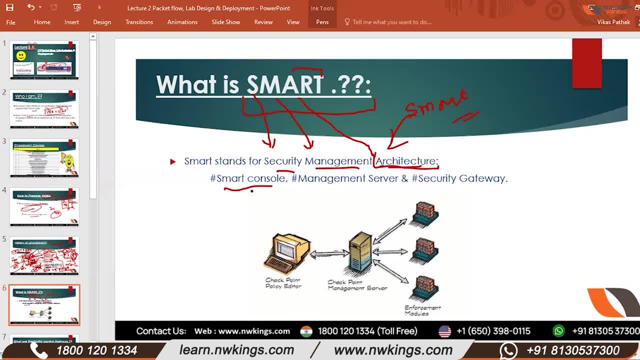 Or you can also call it smart console management, server security gateway. It is called three-tier architecture. Okay, Three-tier architecture. This three-tier architecture is called smart architecture or security management architecture. And why is it three-tier? Because the deployment of the checkpoint takes place in three phases. 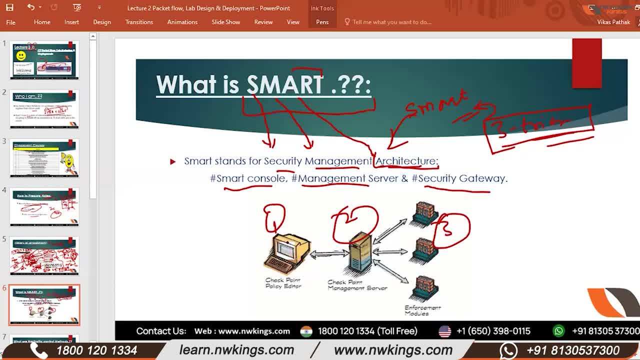 What are those three phases? The first phase is checkpoint policy editor, Second one is checkpoint management server And third one is cluster of gateway. So these are the three phases. that is called three-tier architecture And in these three tiers our first device is called smart console. 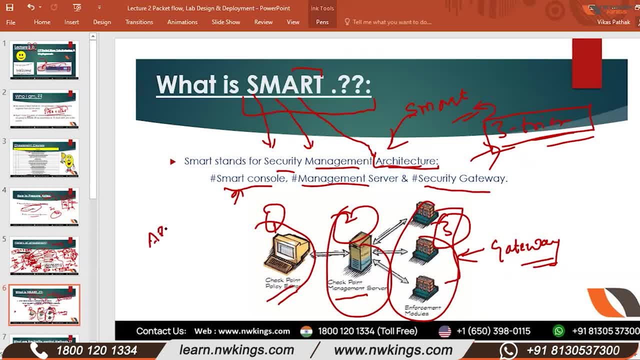 Now, what is smart console? It is an application. What it is? It is an application which you will install on your computer, Okay, And through that computer, through that application, you access the management server. Okay, From the IP of the management server. 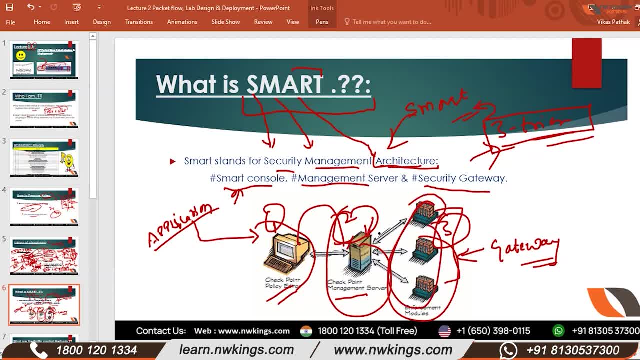 And your gateways are integrated inside that management server. So, whatever the policy modification, whatever the NAT modification, whatever the rule modification, routing interfaces, whatever you want to modify, you will be able to do it on the management server. After doing that, after verifying each and everything, you will be pushing those changes to your gateways. 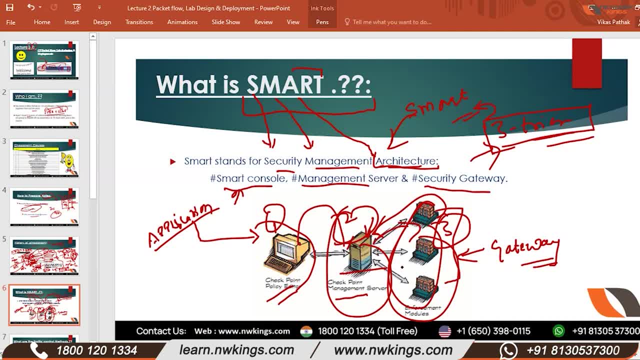 Okay. So this way of working is that you have taken access from a computer- Whose access did you take? Of a management server, And on that management server you have made all the changes. You had to make a policy, you had to make a NAT, you had to do routing, you had to do VPN configuration. 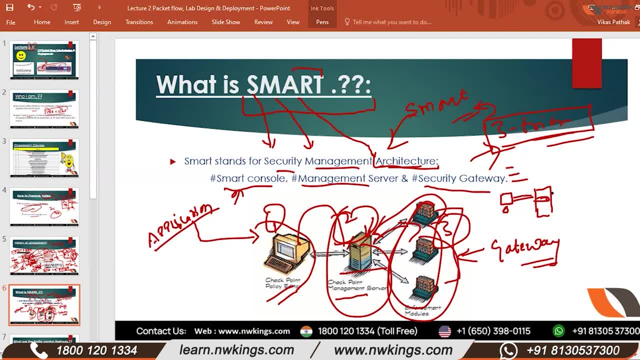 Everything you did on this management server And then, after doing that, after verifying each and everything, you push those changes to your gateway And these were in the gateway cluster. So the configuration you sent to the primary, this is primary, This is secondary. 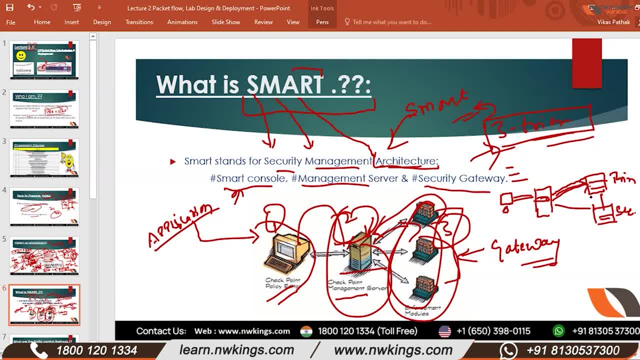 So whatever you pushed on the primary, it was synced to the secondary, So, logically, you didn't spend much time on the firewall. What did you spend time on On your management server And what was the benefit of that? The benefit was that you didn't load much on your firewall. 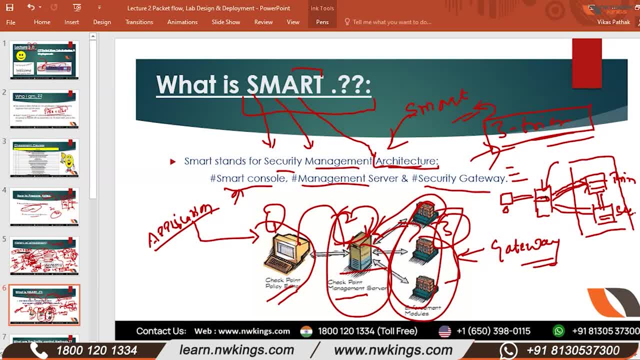 Okay, Whatever you performed, whether it was intensive or it was intensive in nature in terms of CPU utilization or RAM utilization, So whatever happens, it will happen on the management server. There is no impact on your gateway from that. You guys understand what I'm telling you, right? 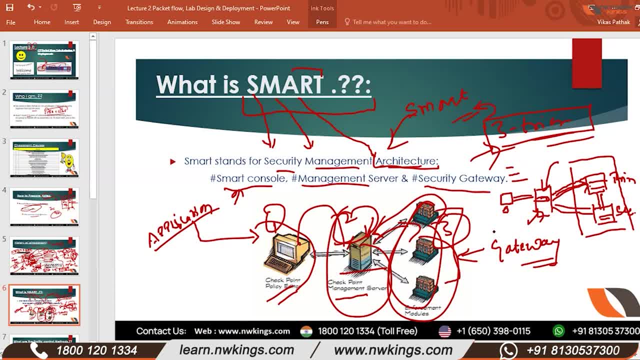 Yes, Vikas, It's clear. Yes, absolutely. But there is a small doubt here Because when we work on the checkpoint in the live environment, it works on MDS and CSN. Can you explain a little bit about the concept of MDS and CSN? 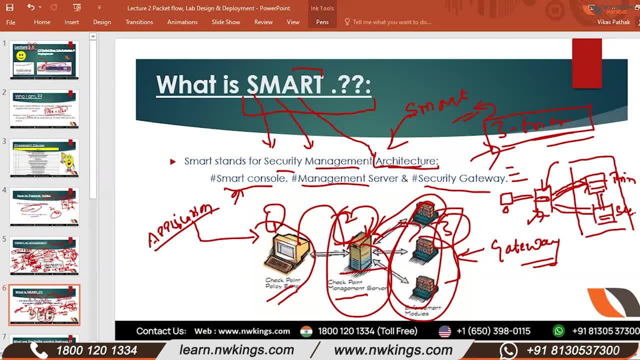 Okay, Let's talk about MDS. What is MDS Multidomain Server-Tier? Now, there is a feature of MDS as a checkpoint. I will tell you later on, But there is a feature of a checkpoint. What is that feature? 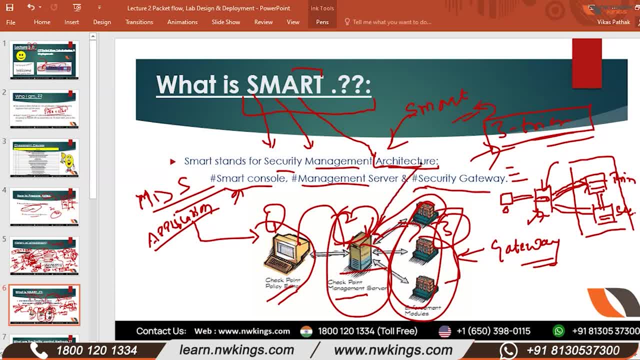 Let's assume that you have three firewalls. Here you add one more firewall. Now you are managing four firewalls from a single management server. Okay, Now what you have done is you have placed these two firewalls in one policy base. 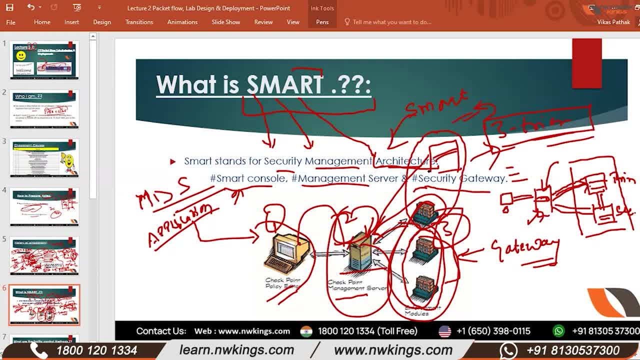 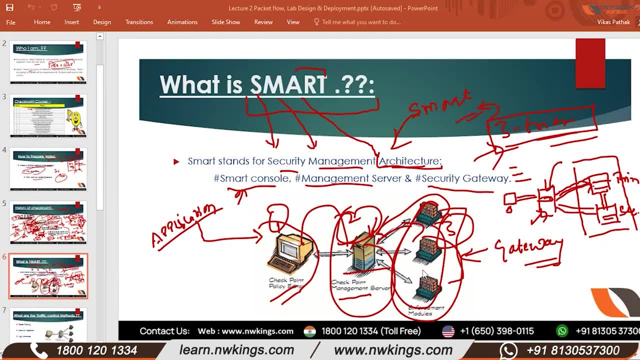 and these two firewalls are placed in another policy base. Now what I have done is I will clean this up a little bit. Okay, So can you see this? So what happens in MDS, Basically, when you make the fourth firewall? 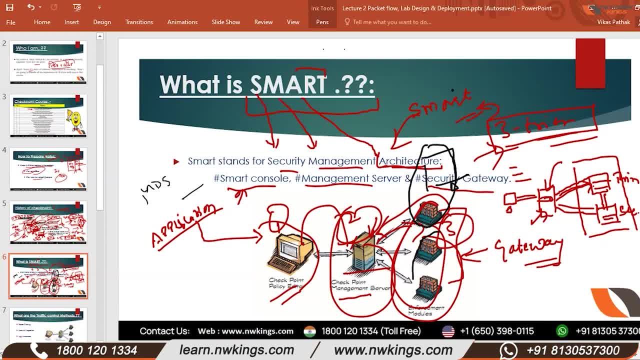 these two firewalls are in one cluster. These two firewalls are in one cluster. Okay, So what you can do is you can make a different policy base for this from a single management server and you can make a different policy base for this. 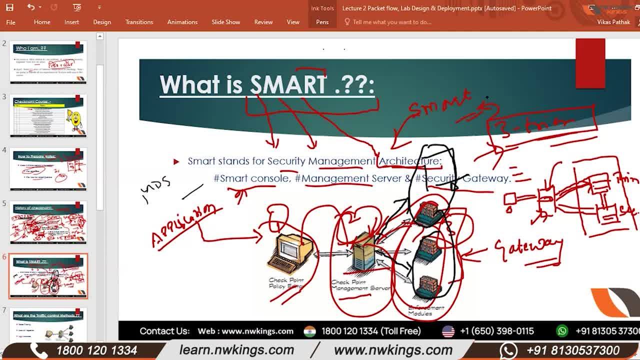 Okay, Now let's assume that while doing this, you have 400 firewalls. So what you can do is you can't manage 400 firewalls from a single management server. In that scenario, what happens is a multi-domain server. 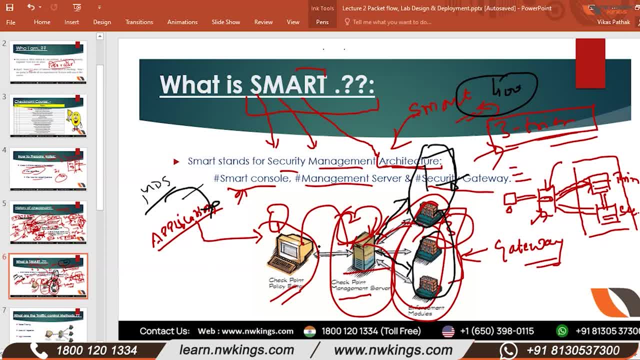 your fourth, assume here a fourth server comes, which is called MDS. Okay, Now on that MDS, your single management server. at least as much as you have 400 firewalls, approximately 100 or more management servers will be integrated on MDS. 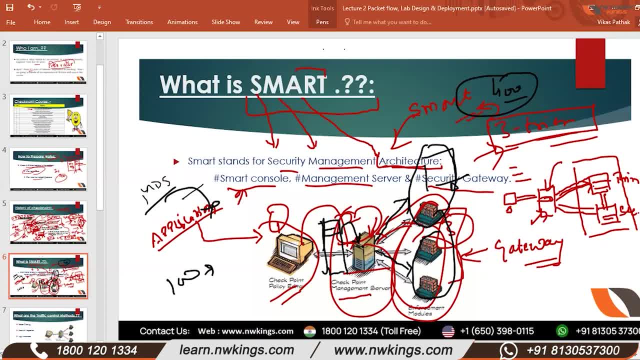 And through MDS you will land on its management server And then you will manage its policy section or firewalls. Do you understand what I am saying? So if I talk about you have a network of 10,, 12 or 15 firewalls. 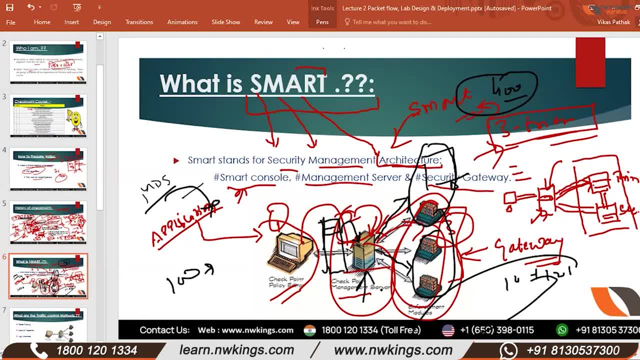 then you can easily access and manage them from a single management server. But when we talk about enterprise level, MDS comes there And then VSX comes. MDS has another technology: MDS and VSX. Both of these come on large enterprises. 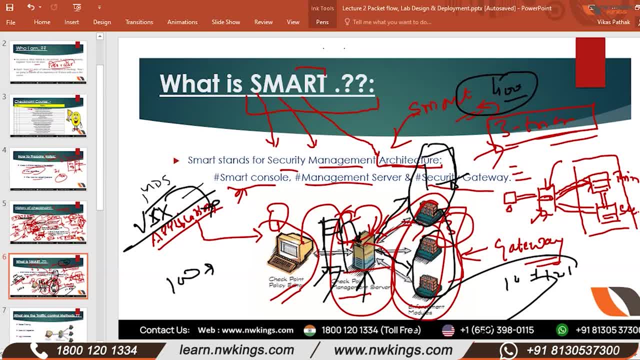 And nothing happens. It's just a way of management: how you manage the distributed environment. Is it clear? Yes, it's clear. now Any doubt? So, no, no. So CSM is like management server. Yes, MDS is the multi-domain server. 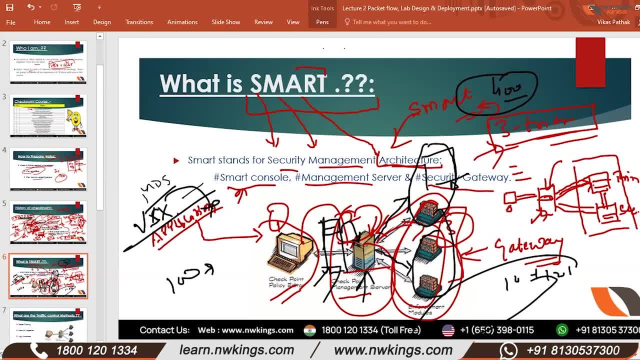 that is implied before the CSM. Yes, Okay, Yeah, fair enough. I have one doubt: If our server is coming in the middle, then is this server in the form of our applications or is it our hardware? now Are we talking about this server? 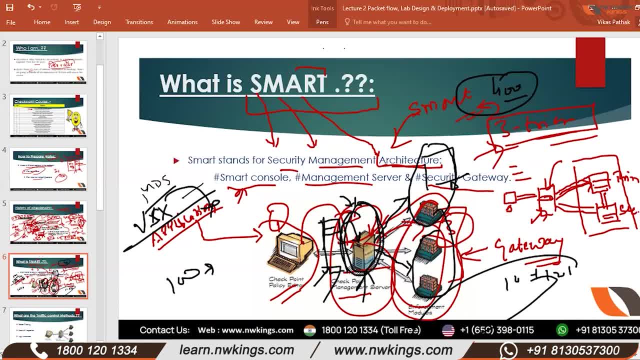 Yes, What is this? This is the Gaia of the checkpoint. Okay, Okay, The checkpoint is Gaia, But when we deploy the checkpoint, we have two options: That you want to deploy this Gaia version of the checkpoint as a gateway. 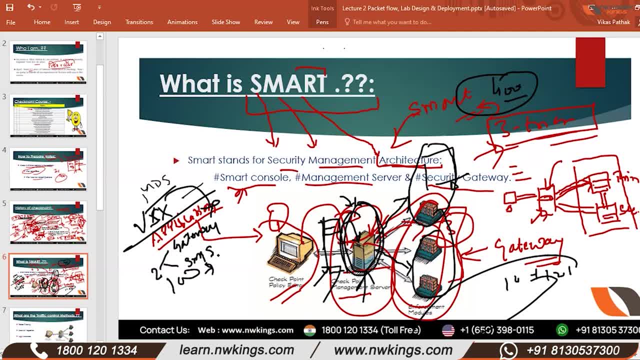 or as a management server. you want to deploy SMS. So when we install that Gaia on the management server, we choose the SMS option. Otherwise we make it a gateway. Okay, sir, You got it. Yes, sir. 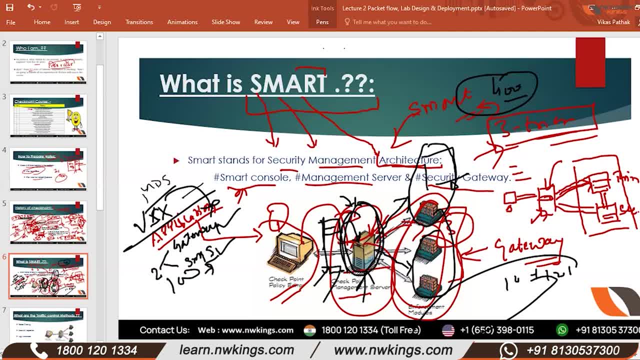 Yes, So as soon as you select SMS and install it, all its features are installed in SMS and all the functionality is done by the management server. SMS stands for SMS Security management server. Okay sir, Okay sir, Thank you. 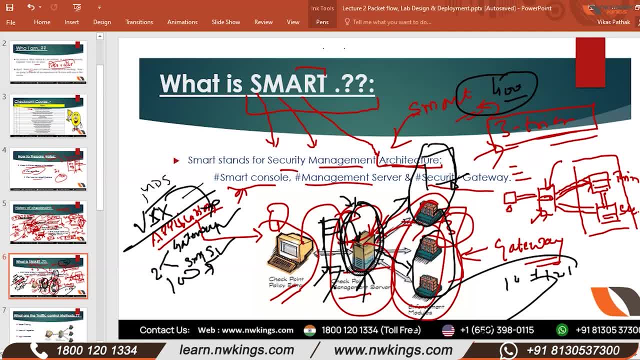 Sometimes the person in front of you is talking in SMS and you get confused. What was SMS? SMS is nothing, only just an acronym for security management server. Okay, The server that comes on the second level. we are talking about that. So, if you have any doubt, any question. 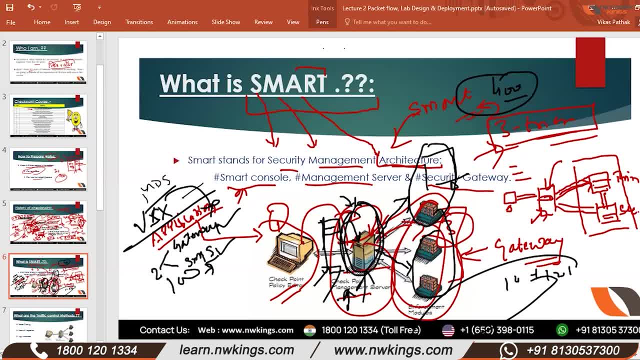 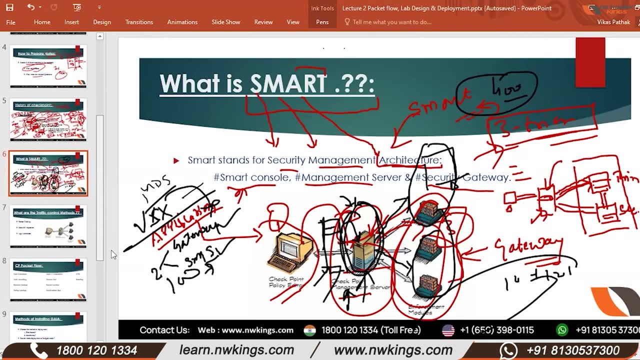 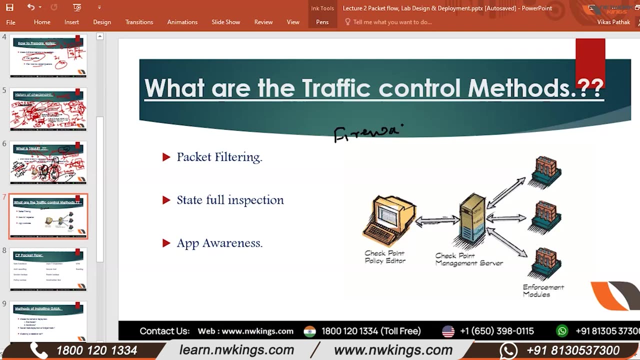 anything which is arising in your mind. let me know Any question. No, sir. Okay, perfect, So let's move ahead. Okay, when we talk about firewall. so what does firewall basically do? Okay, before that, let me ask you something. 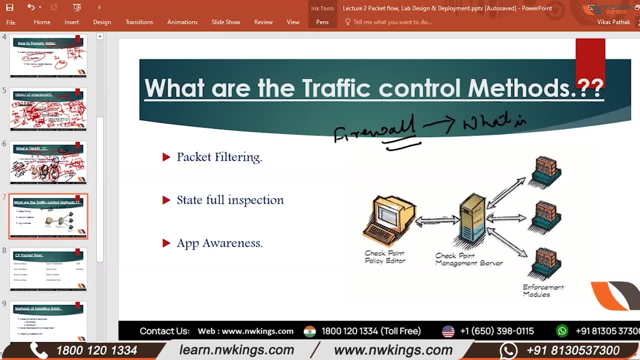 Answer me. What is firewall? Tell me. A firewall is a device which makes sure that all the users who are inside my network can access the internet as well as, at the same time, no malicious traffic from outside can enter my network. Okay, This is good. 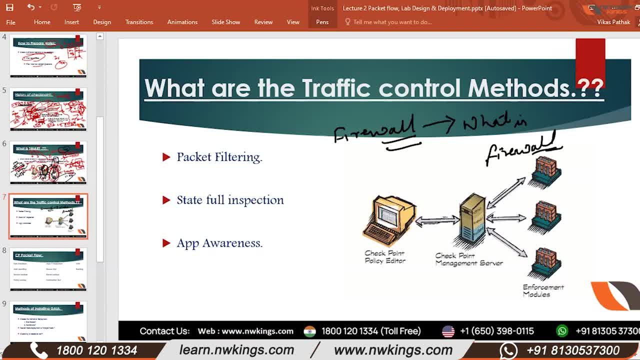 And anyone else. Firewall is something and it achieves this thing where all the inside users can access the internet and no outside traffic can come inside, with the help of stateful packet filtering as well as through connection-oriented approach, where it will form a connection table or a session table. 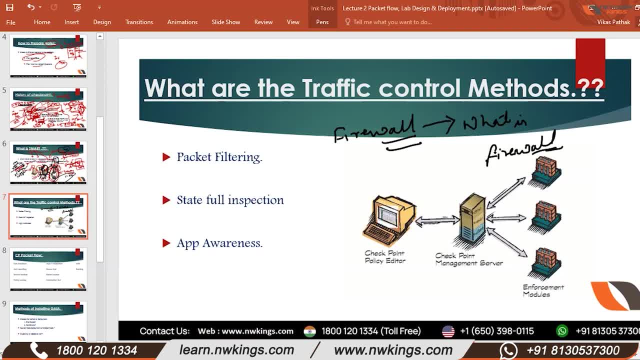 It will check that, or else in the stateful packet filtering it will check whether we have access list with respect to that traffic and only then it allows that specific traffic to communicate over the firewall. I'm not sure about the checkpoint, but I have studied Palo Alto and FortiGate. 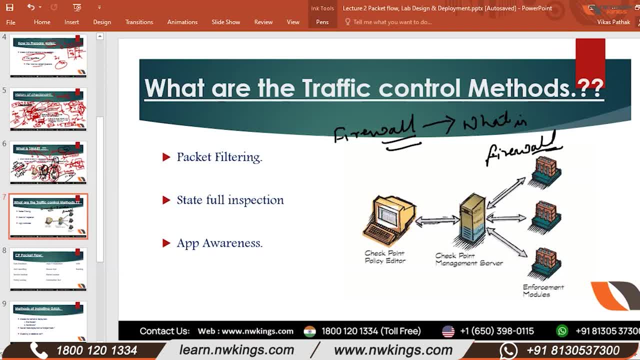 and both of them are following zero trust approach. So, in order to communicate from one point to other point, you need to have- you must have- an access list or we can say, a security policy. Yes, So that's correct, But the question was: 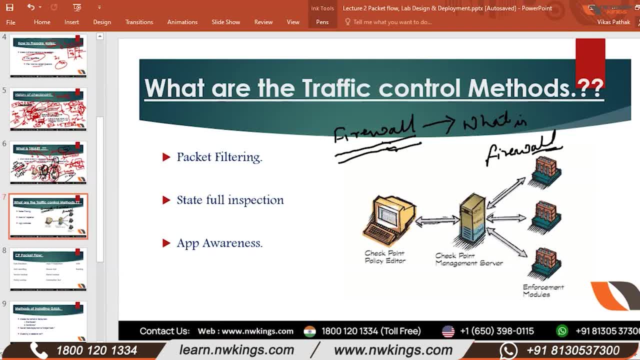 what is a firewall? You told, like you said, like you told me what benefit it provides. right, That you can go from the inside to the outside and no one can come inside from the outside. That feature set is required, right. 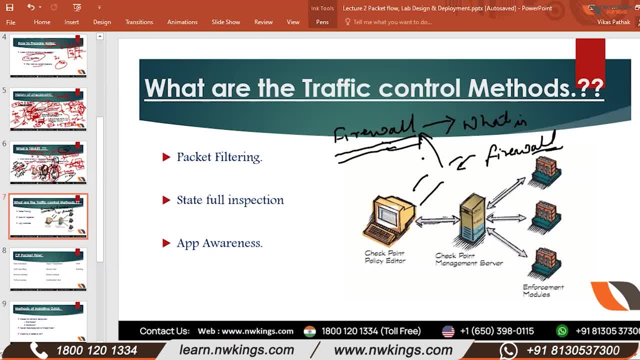 So we can say firewall is something which protects our environment. Yes, That's what the proper definition, but it's also a half definition. You should say L3 device, layer 3 device which provides an extensive security to our network and controlled by network administrators. 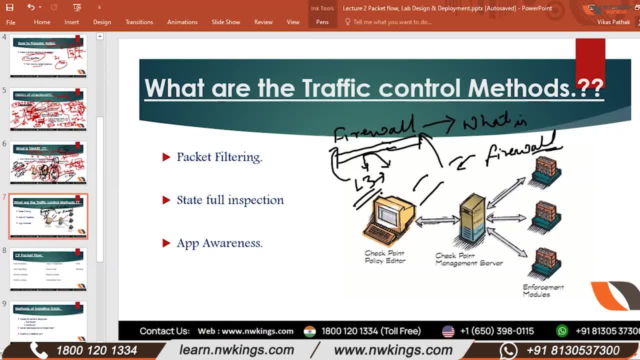 network security administrators. It's called firewall. We can modify, we can create and we can deploy the policy section on the basis of the business requirement. on the firewall right. So let's assume that this is my firewall right And this firewall. 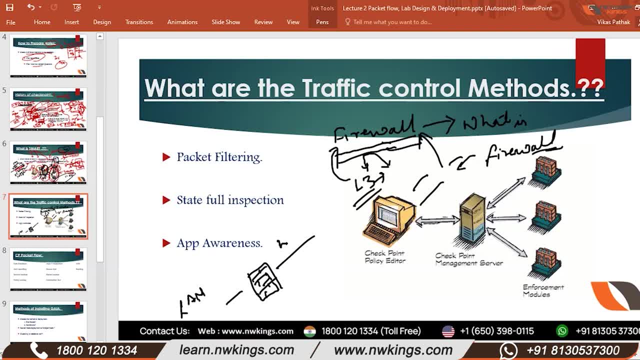 this is my LAN, this is my WAN. right Now, the user comes from here and he has to go here. So, by default, if I talk about any firewall, there is a denial. So what you have to do? 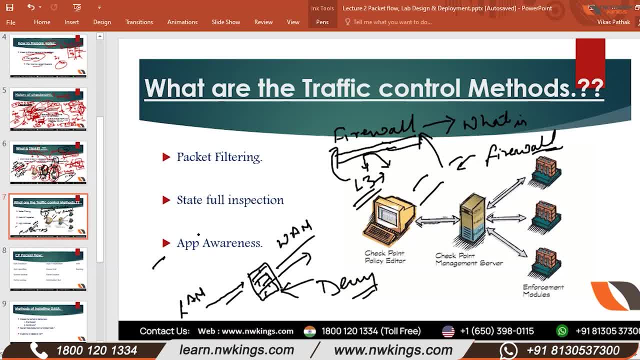 you have to create a policy that, from source this to destination this, the traffic should be allowed And vice versa. That when a person is coming from outside and has to enter the LAN, there should be a policy for that too. Otherwise it will not work. 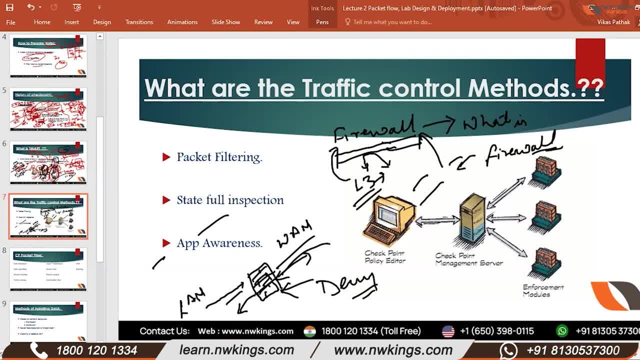 The connection will be dropped at the firewall level. Is it clear? Hope, the understanding of your firewall, the knowledge, I have improved it a little bit. Yes, Vikas. Okay, Now another question which you will hear a lot in the interview. 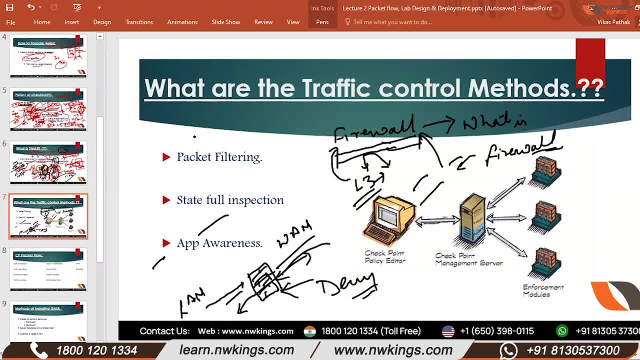 if there is an L1 level or the first round of interview. many times we ask questions: Difference between router and firewall. What is the difference? Firewall also are L3 device. Router is also a L3 device. We are configuring ACL on router. 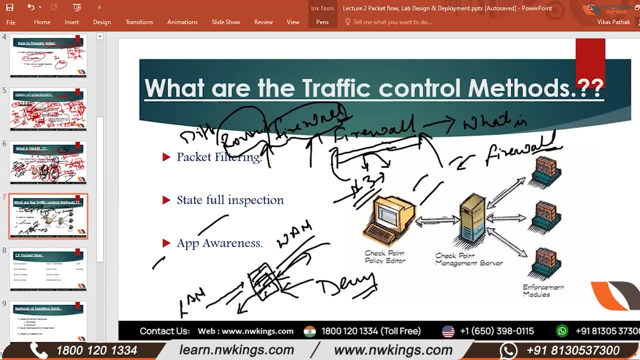 We are configuring ACL on firewall. What is the difference? With router, we can achieve these two things simultaneously. That means I want that if my inside users can access the internet at the same time and outside traffic can't come in, then this thing can't be implemented at the same time. 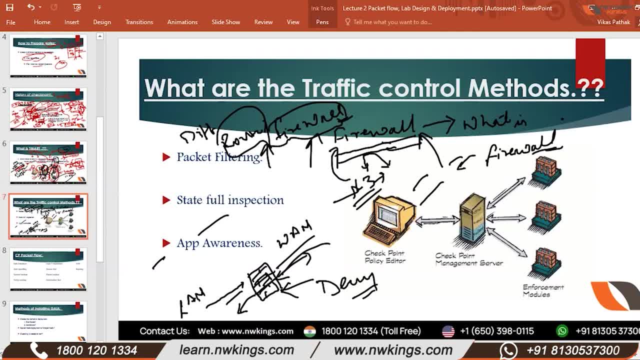 Either my users will go outside from inside or outside traffic will come in, Because if I will imply a NAT on my router and simultaneously if I will place a security policy to deny all the traffic, so ultimately because router doesn't follow, 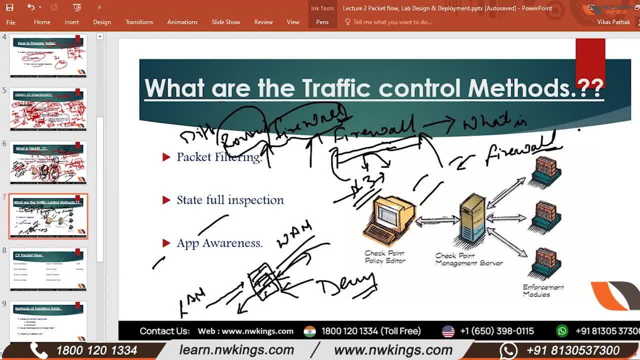 approach of a step-by-step process in order to process a packet, like firewall does, so ultimately, my traffic will be dropped at the router, Traffic will go outside from inside, but its reply will never come. Okay, What if I said that? 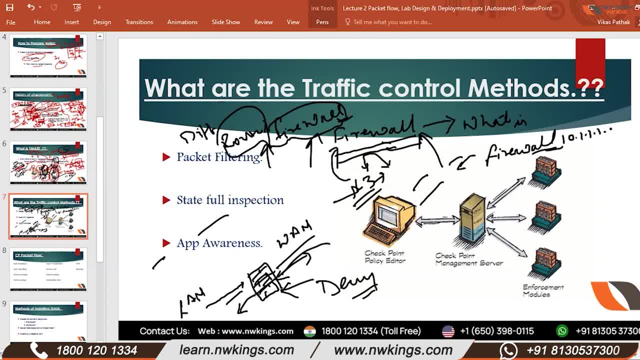 my source is 10.1.1.1, and destination is 20.1.1.1, and connection should be allowed. Okay, And I made one ACL on router and another ACL I made from 20.1.1.1 to 10.1.1.1,. 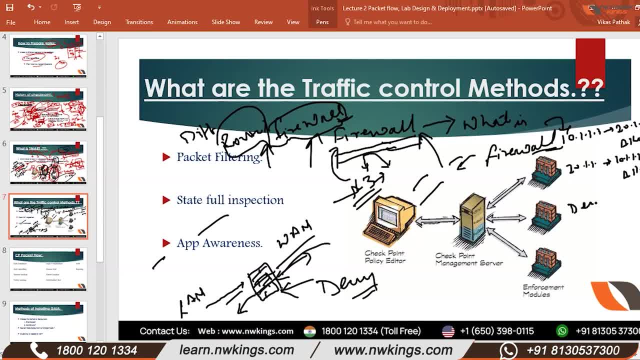 traffic should be allowed, and after that I made an ACL of deny-deny. So won't it happen in this case also? It will happen in this case, but the problem will be that in the case of deny, the traffic will go outside from inside. 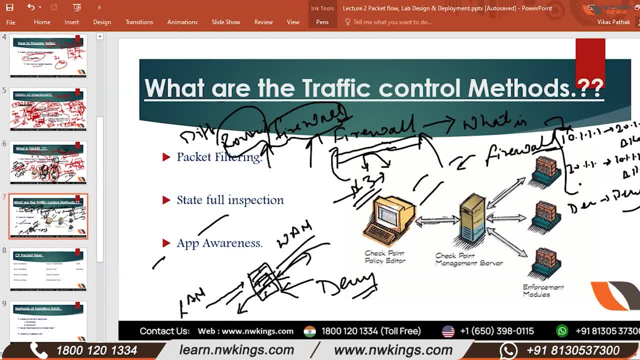 but in firewall, if a traffic is allowed from one side, like TCP and UDP traffic, like the inspected traffic, its reply will come by default. But in this case, the traffic which will be apart from these two, its reply will not be able to come. 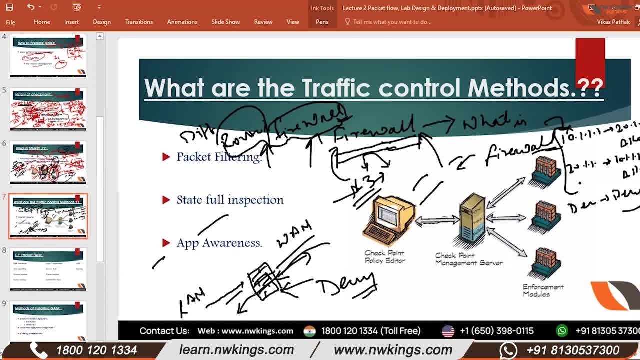 because its policy will not allow it. Yes, So you mean to say that these two communications will be allowed, but nothing else will be allowed, Right? Yes, Sir, I want to say that router adds two networks like 10.1 and 20.2.. 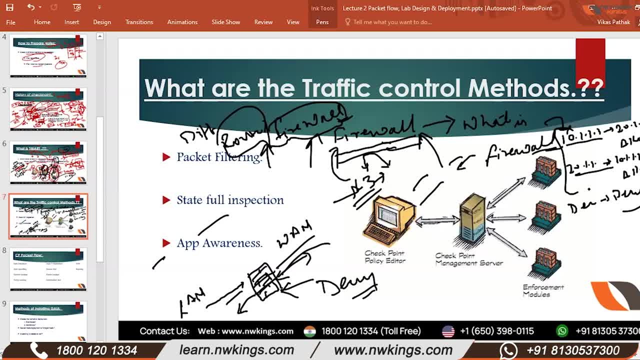 It is dedicated for routing, And if we install ACL in this, if we implement more, then our routing will be slow, Exactly, Exactly. That's one difference actually. Yes, Very good, Very good. So you both guys are correct. 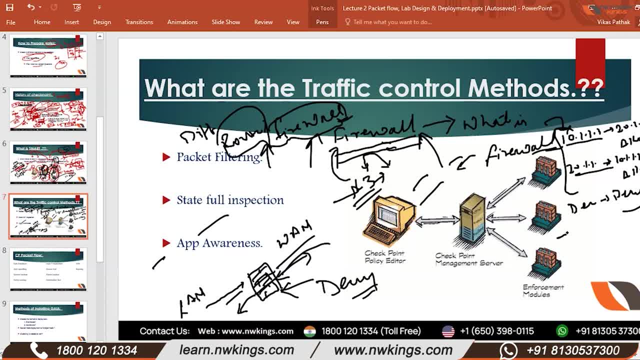 but at some extent the first difference. we saw that the main purpose of routers is routing. What is it Routing? If we make it work for firewall, then in a small organization it will work, But when it comes to a large enterprise, 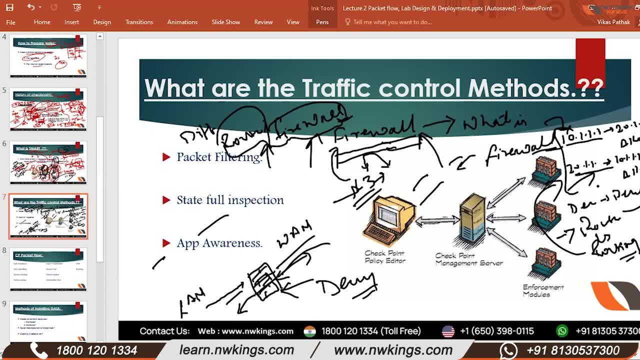 it will burst every third day. Every third day, its RMA will have to be done Because the processing speed will go up so much, the utilization will go up so much, that it will become a deaf and dumb device. Do you understand? 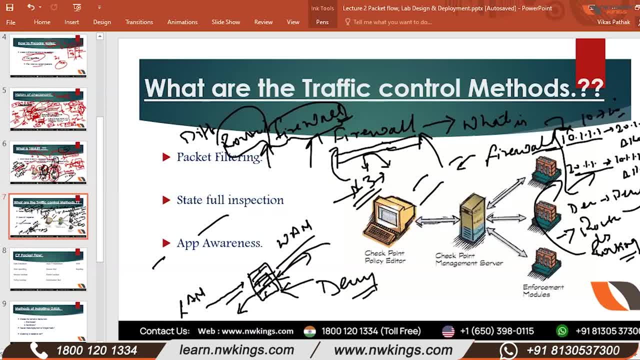 If there are 10,, 20,, maximum 50 ACLs, then configure it on router. But what if we have 5000 ACLs on a single firewall? Now this poor router, tell me, can you verify the RMA or the ACL? 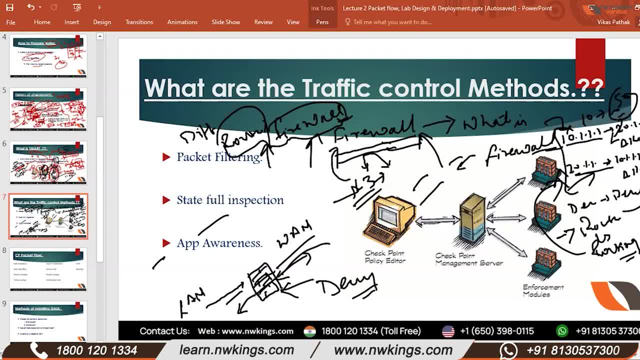 So the first difference between router and firewall is that routers are meant to do routing, whereas firewall is meant to do filtering. So in large enterprises we have to use both at the different level and for the different purpose. And second, and the most important, 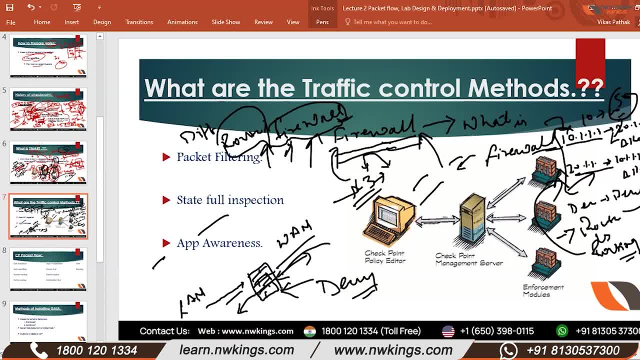 difference is that firewall can be a L7 firewall, but router cannot be a L7 router. How will you do application filtering on this router? Are you getting my point? Yes, sir, Major difference. This is major difference, Isn't it? 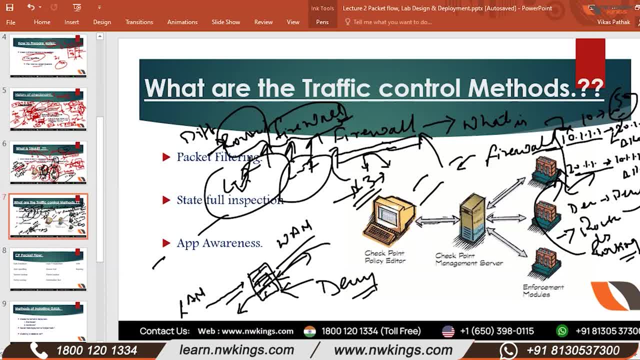 Yes, sir, If I talk about firewall, you will easily do application filtering on it. You said that Facebook is allowed by me. Okay, It is a marketing department. I allowed Facebook, But Facebook games are not allowed for anyone. Facebook games are not allowed. 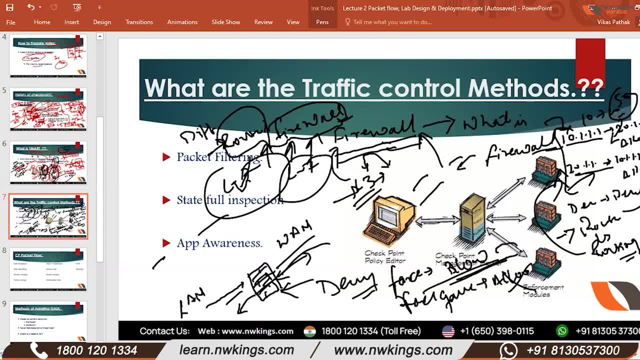 Now, how is this firewall running? Do you know that this traffic is of Facebook games and this traffic is of Facebook? It is of normal Facebook. On the basis of the application, The web traffic will be 443 or 480.. It will choose. 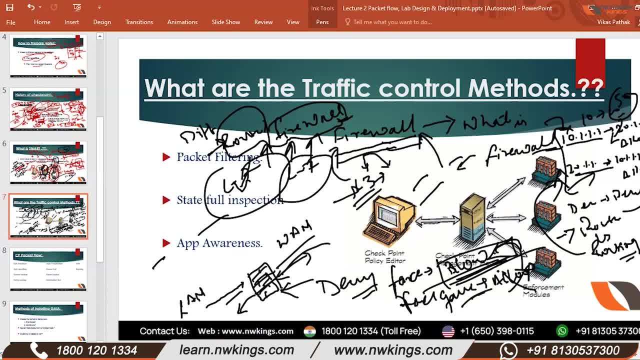 But if I talk about Facebook games, then 443 and 80 will also be working on one or the other. port The game that it will catch the firewall and block it. So this is being inspected inside the packet That is called L7 application. 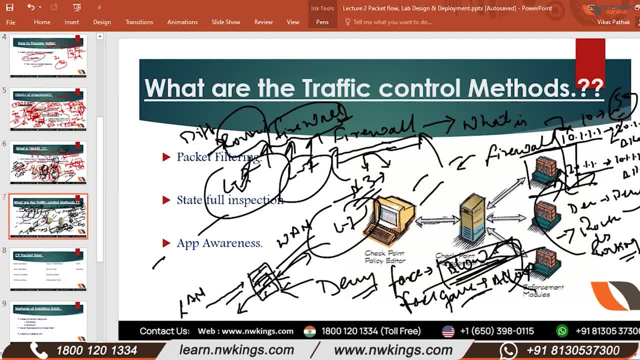 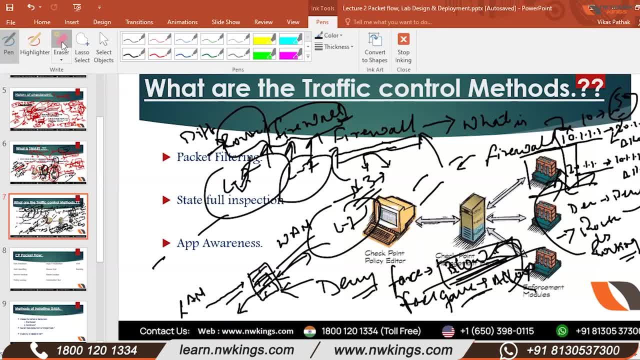 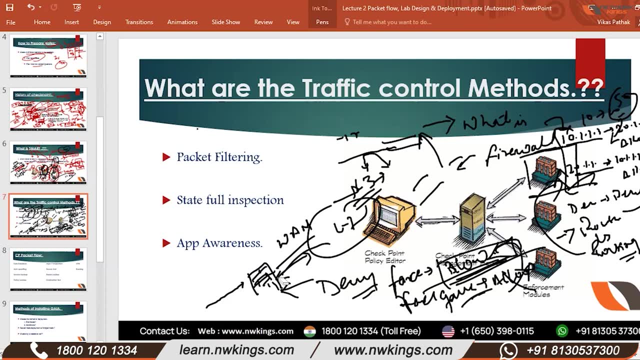 L7 inspection, Layer 7 inspection is being done here. Okay, Okay, Okay, Right, I hope that these small questions are sometimes like interviews. There are three rounds in the interview. There are four rounds In the first round. what happens is that the person 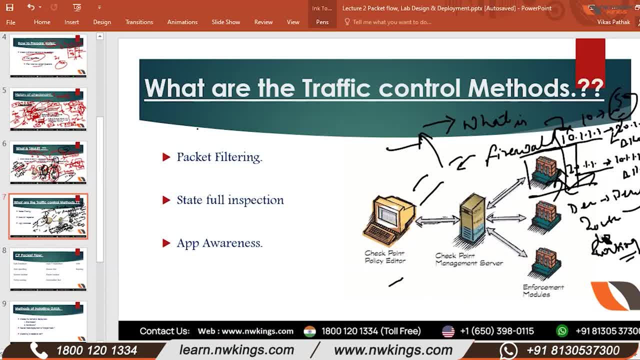 asks you general questions. He doesn't ask you anything major. Major will be asked in the second round or most probably in the third round. In the third round there is also a managerial round, Okay, So in that things related to this will be asked. 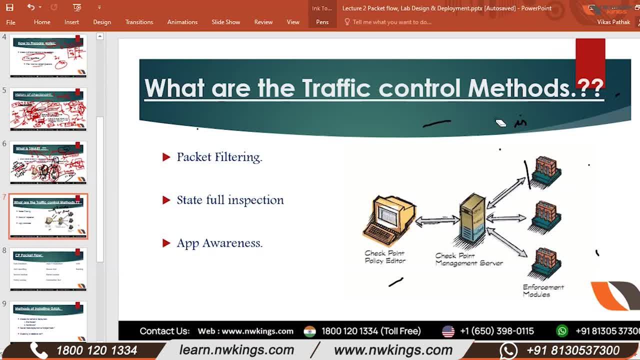 But the second round is most probably very extensively. There are also questions higher than this, But in the first level some questions like this are asked: That you tell me what is the difference in this. You tell me how will the benefit of this ACL you are making 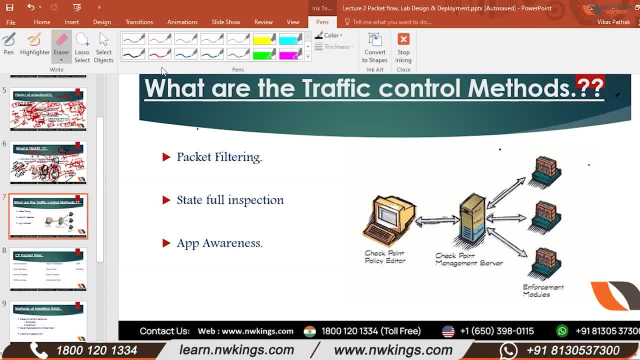 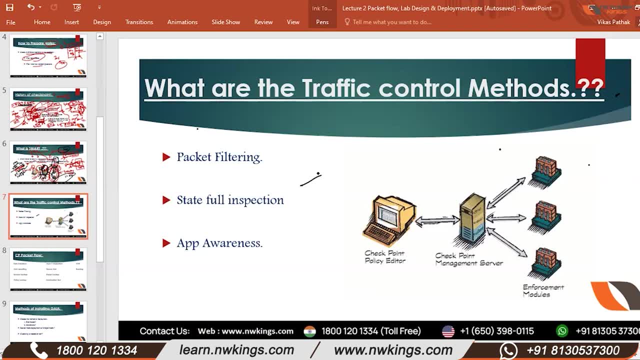 be received. Do you understand? So these two things I have told you, the points I have told you. please note them down, Okay, And always keep in mind what is the difference? Okay, And you should clear a small definition of firewall. 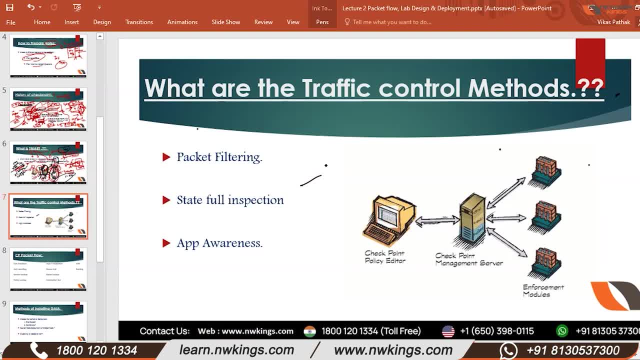 in your mind And, being an administrator, suppose you are working on L3 level security tomorrow and if any student or trainee of L1 comes, there might be a chance that he also asks you a question. So at least you should clear these things. 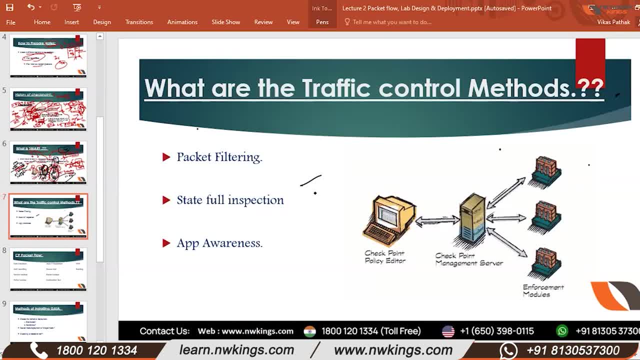 at the understanding level. Correct or not Correct, sir? Correct, Okay, If you are agreeing, then we will move forward. Okay, Any question in mind right now? Any doubt? question any question. Don't feel like I am a teacher. 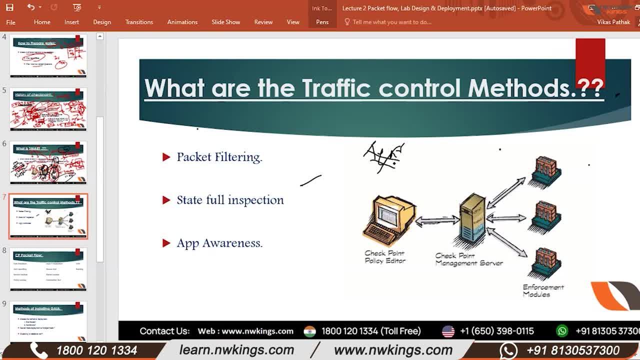 Okay, I don't want to teach like a teacher at all. Consider me as your friend who is guiding you. Okay, So if any question comes to your mind, don't hesitate at all that it can't be a very silly question. There is nothing like that. 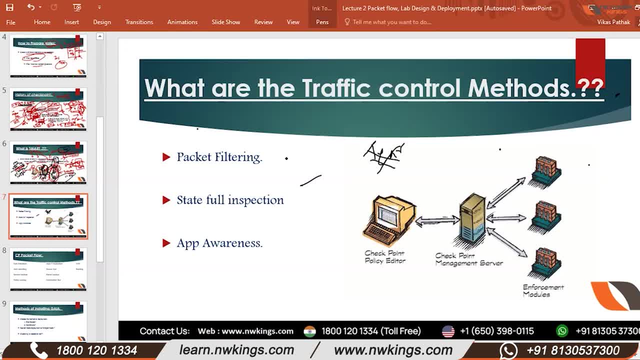 Directly. you can ask If it is silly, I will definitely answer in that way. Okay, Let's talk. now. A general term comes that the traffic flow. till now we haven't read anything specific about the checkpoint. Okay, Till now. 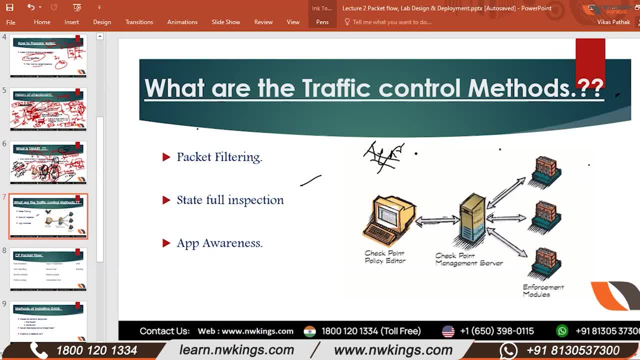 approximately 45 minutes have passed And we have some general meaning. if I just leave the three-tier architecture, then we haven't read anything specific about the checkpoint. We are reading general terms. Okay, We will relate the architecture of the checkpoint now. 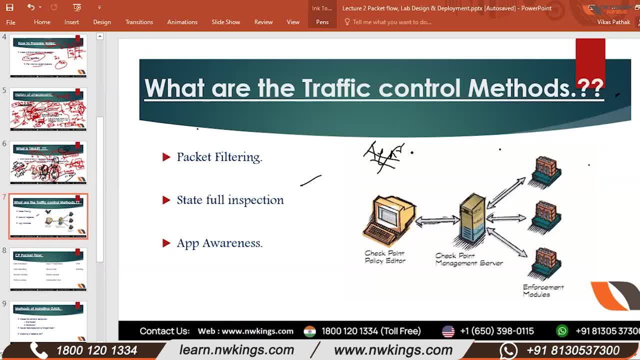 We are reading the course and we will read the general thing and then relate it. Okay, So if I talk about the general term, what are the traffic control methods that we have? Can someone tell me Anyone? Okay, There is silence, so I understand. 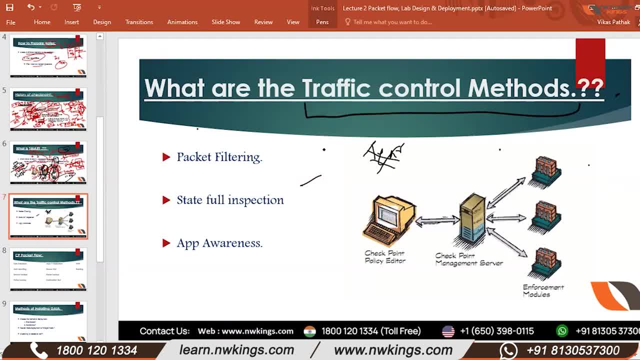 the meaning of no. Our general term is traffic control methods. Okay, If there is silence, then I understand the meaning of the traffic control. We have generally talking about firewall. we have three types of traffic control methods. Okay, Packet filtering. 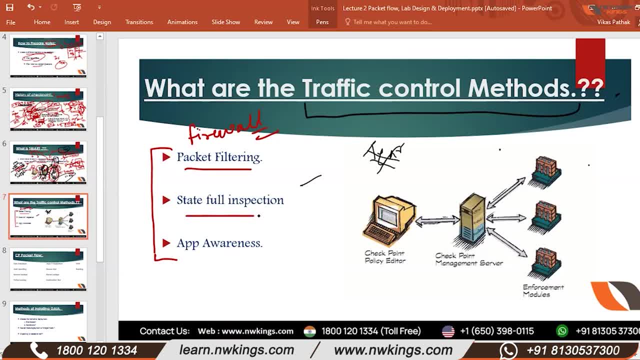 stateful inspection app awareness. Okay, There are three types of filtration methods. First of all, what is packet filtering? What is packet filtering? Packet comes to you with a firewall. This is your firewall. Let me clean it a little. 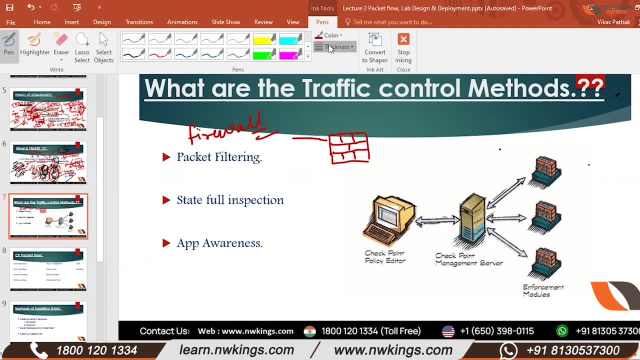 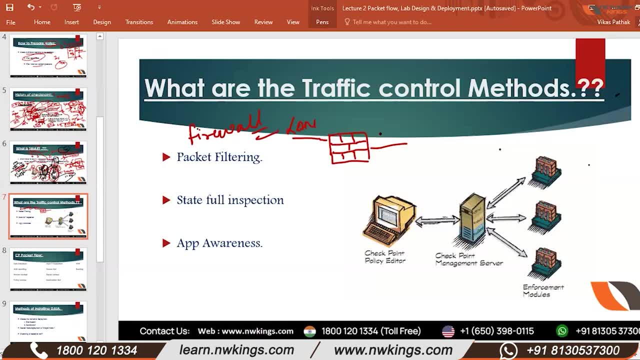 This is my firewall. Okay, This is my LAN. This is WAN. Okay, Now what are we doing in packet filtering? Traffic came to us. We saw the source and destination in traffic And we saw our port number. My source is: 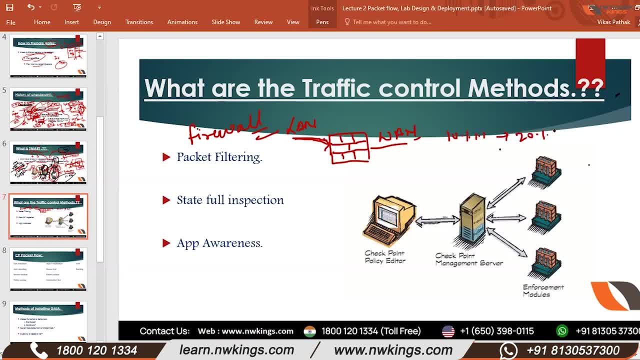 10.1.1.1.. My destination is 20.1.1.1.. And the port is 443.. We saw this source and destination. We said allow. That is called packet filtering. If we look at the port number. 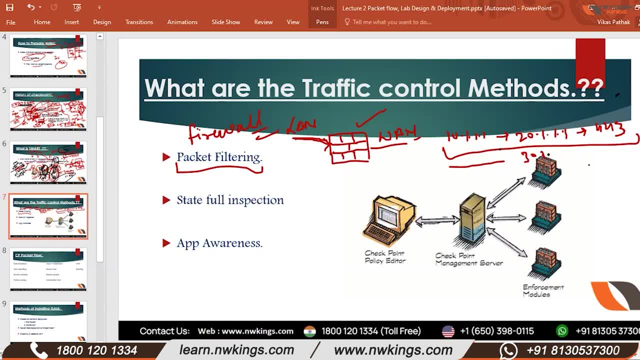 it is 10.1.1.1.. And it is trying to go on 30.1.1.1. on port number, maybe you know 80. Or if you have 10 subnet source and 20 subnet destination, But apart, 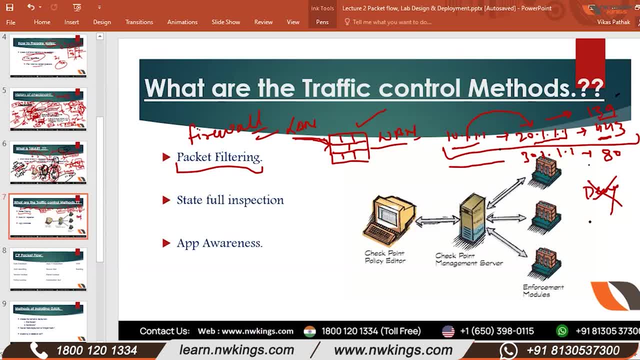 from this we have a simple packet filtering: The port that is allowed, the communication that is allowed, the communication that is denied is denied. This is a common, typical firewall term. If it matches with the information, then it is allowed. otherwise, 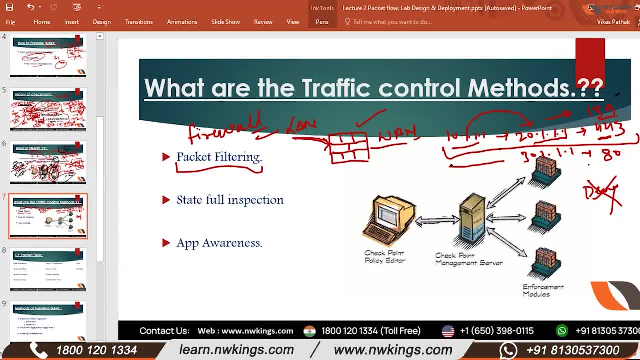 it is denied. Is it clear? What happened to packet filtering? What happens in the packet? How is it filtered? What happens to the information? There are only four things: Source address, destination address. source port, destination port. There are. 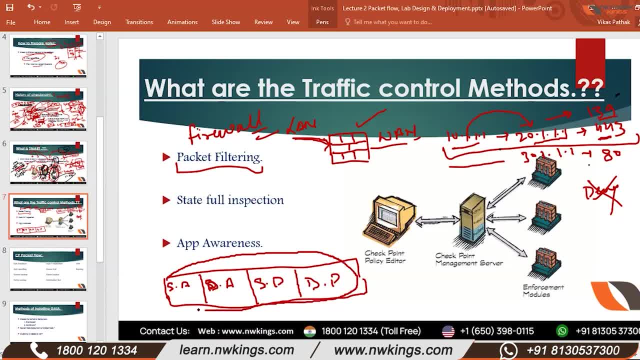 only four information on which the firewall works, On which does allow or deny work: Packet filtering. After that comes the section of an application and through the destination port number you filter the port. So if any firewall is doing packet filtering then it works. 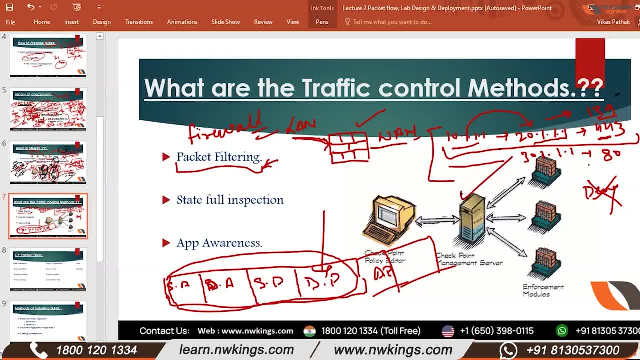 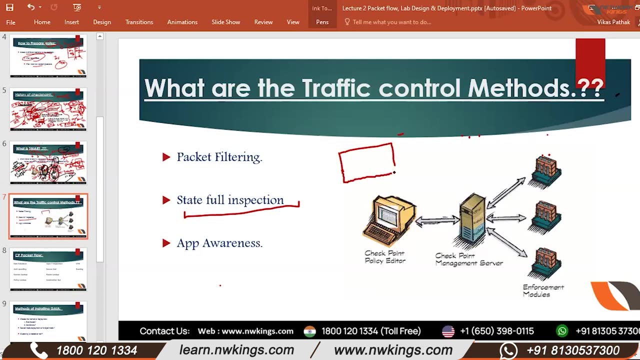 When you talk about checkpoints, it is working. If I talk about ASA, it is also working. If I talk about any other firewall watch guards, all of this works. But what about stateful inspection? Now you can see that this is. 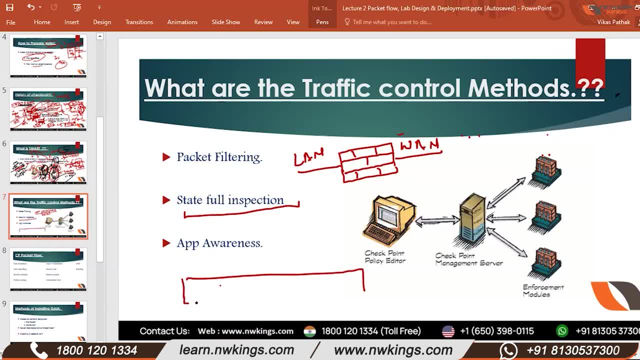 a packet form: Source address, destination address. source port number, destination port number. This packet came to my house. What is source address? destination, source port number, destination port number. what is the policy match? check the policy all. 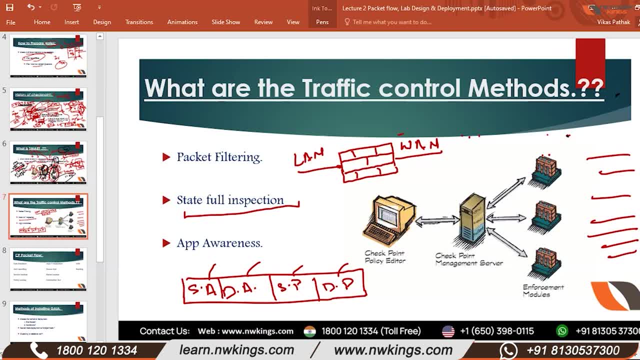 these policies are made. And yes, remember what happens in firewall: the lookup is the same as the default lookup in the default lookup. So if you want to do the same as the default lookup, then you have to change the lookup to the default. 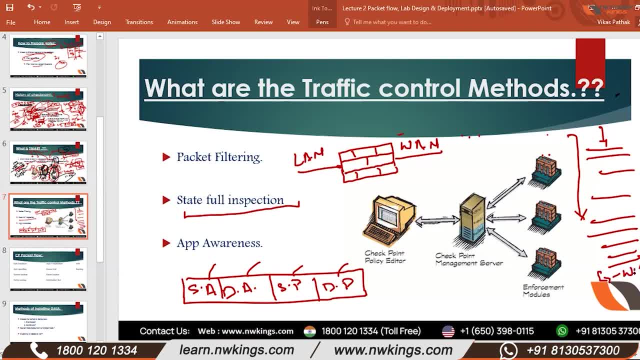 lookup. If you want to change the lookup to the default lookup, then you have to change the default lookup to the default lookup. If you want to change the default lookup, then you have to change the default lookup to default lookup. So if you 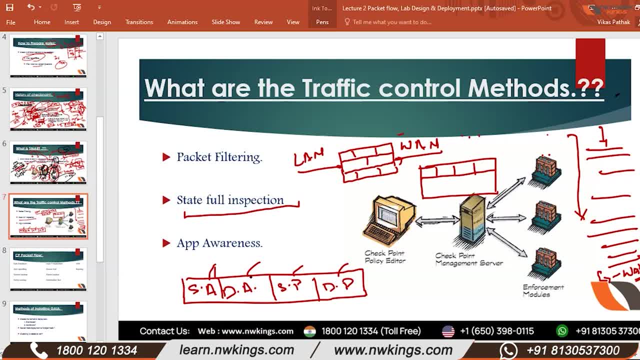 want to change the default lookup, then you have to change the default lookup to the default lookup. So if you want to change the default lookup to default lookup, then you have to change the default lookup to default lookup. If you want to change the 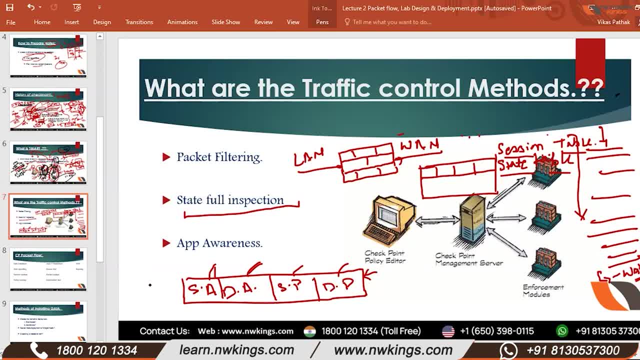 default lookup, then you have to change the default lookup to default lookup. So if you want to change the default lookup, then you have to change the default lookup to default lookup. So if you want to change the default lookup to default lookup, then 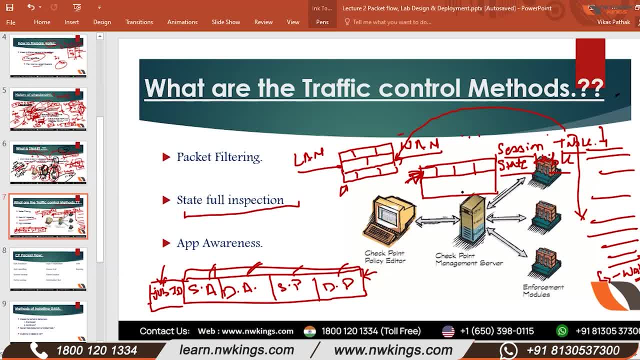 you have to change it to default lookup and then you can change it to default lookup. Then you can change the default lookup to default lookup. So if you want to change the default lookup, then you You will not be able to see how it is working. 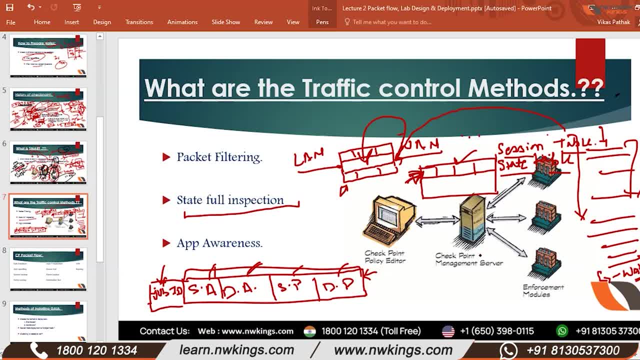 You will not be able to see the mechanism, But yes, I will definitely show you how the communication is allowed. Now, what happened? what benefits did we get from the session table? Let's see the benefits. This is my PC. There is a firewall in the middle. 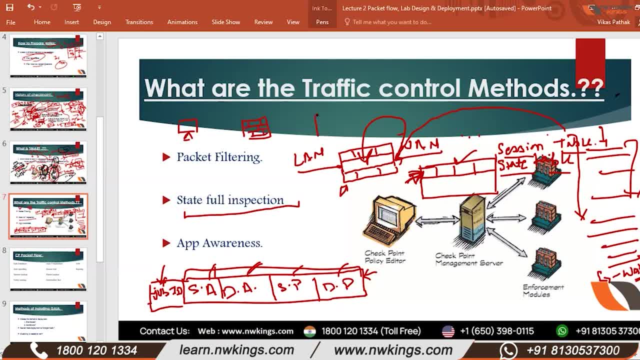 This is my server. Now consider this PC as the application owner. Now the application owner said that: Vikas, This is my server. I will always initiate the connection on it. I will always send the traffic. It will never happen that the connection will be initiated from the server. 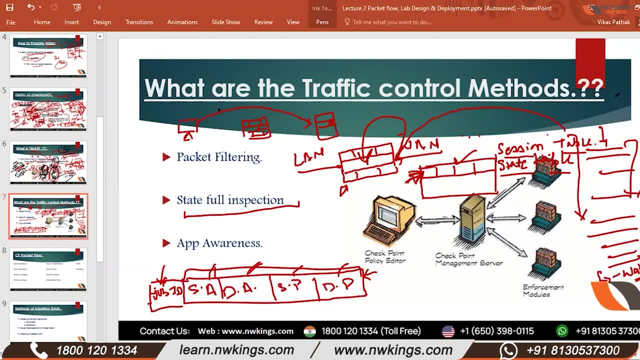 It will never happen So. So if this is the scenario, So if I have a typical firewall, So what will I have to do? in a typical firewall Source Set destination, I will have to open one rule. Am I saying right or wrong? I feel like I am missing something here. 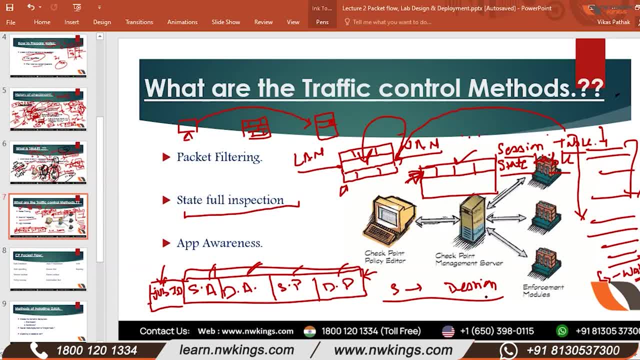 No, no, it's clear. You guys stay unmute and keep talking to me. So you made a rule that source should be between destination. So if this is a normal firewall, So what will I do? I will have to create a source from the destination. Why? 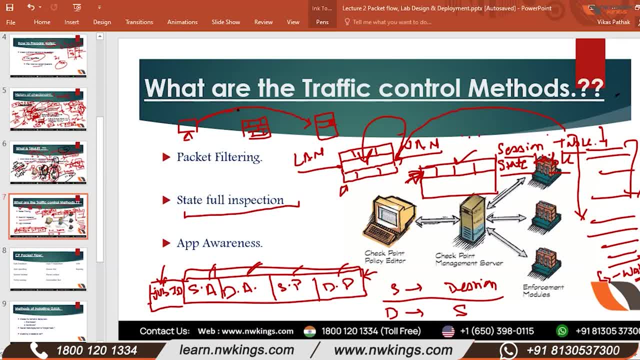 Because the request that has been initiated from here Has gone to the server, Its response should also be accepted. Understood. Now, if you have made a rule That the initiated traffic has been allowed, But no rule has been made for the response, Then it will be denied Right. 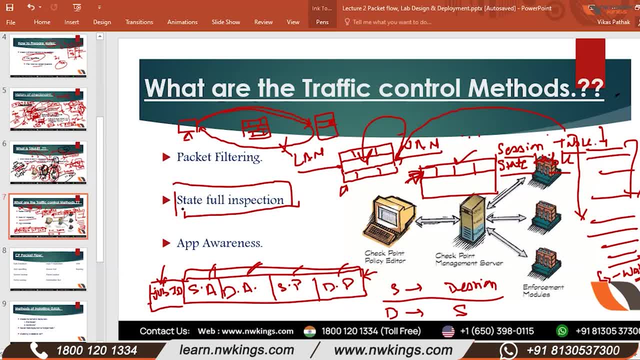 But if your firewall is doing stateful inspection, Then you have made only one rule. No rule has been made from destination to source. You have made one rule: Source destination. it will be allowed. Traffic was initiated from here. It reached your server And when the server will give response to the client. 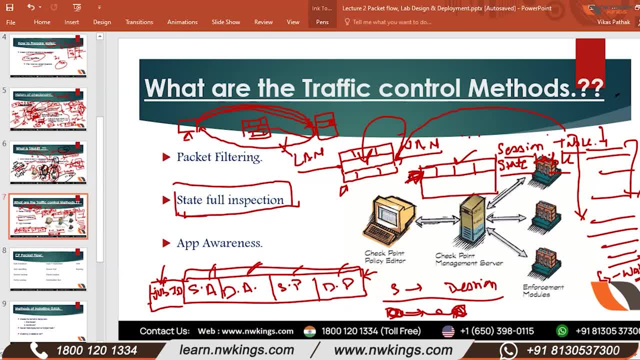 At that time this state table or On the basis of the session table, That communication will be allowed. So where you had the requirement to create two policies There, only through one policy You have allowed the communication. Clear Now what happens: That there is a timer without the session table. 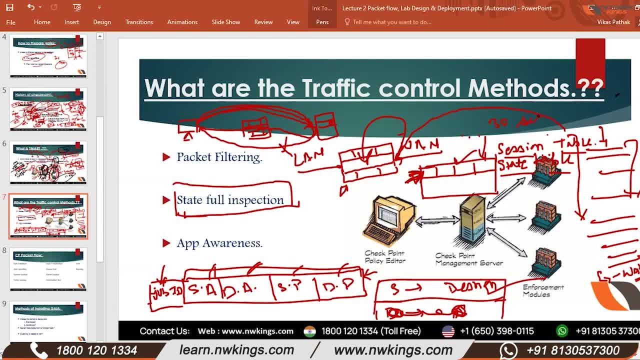 By default 30 seconds And 60 seconds Assume. If in 60 seconds- This one- You have maintained the session, Its response does not come, Then this entry will be flushed. What will be done? It will be flushed, And the good thing is That you can modify this timer yourself. 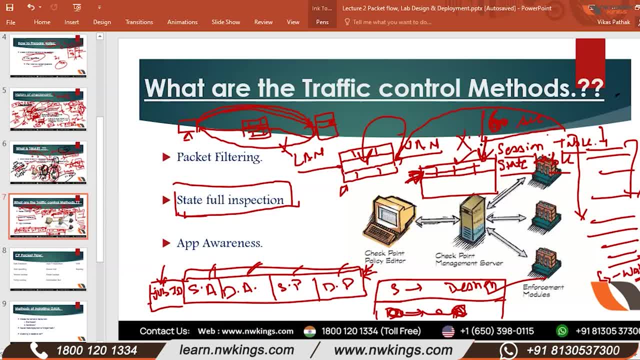 So many times you will get a situation That I sent traffic. It was allowed from my firewall. Whether it reached the destination or not, I don't know. But I don't know if the traffic is coming back To my client Now. the client came to you That check the development. 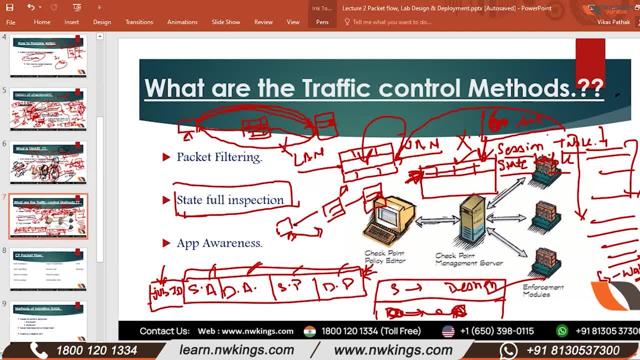 Is there any issue on the firewall? You checked This source destination is allowed. When you check the source from the destination, Then the traffic is not coming. You got it Now the traffic is not coming. So what is the communication from it? Then it broke down. Now what is the reason for this? 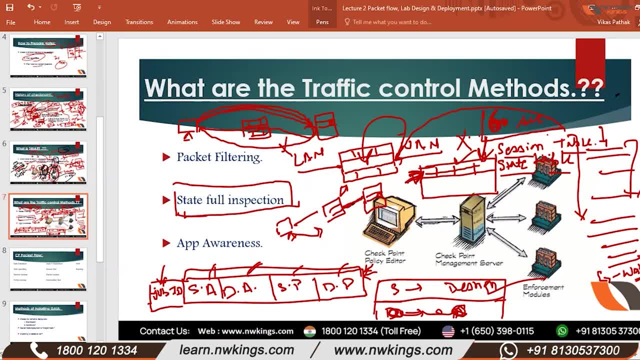 From the firewall to the server, The media, This media- Most probably, In 95% cases, This media will be the culprit That there is some slowness in the media. High utilization Bandwidth is choked Or there is disruption, Because of which Either the packet is not delivering here 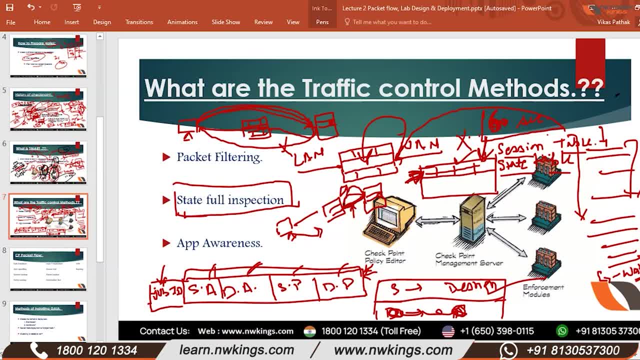 Or if it is delivering here, The traffic coming back from here, It is not able to reach me timely. In that case, You have to capture the packet here. You have to check That. this is your interface, Outside interface. Is there any drop coming on it Or not? And you have to match this too. 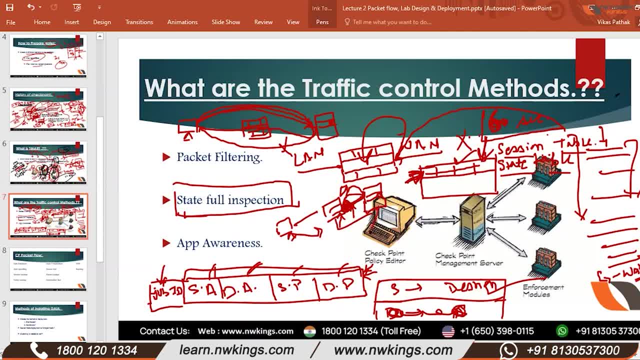 That at what time your packet Was allowed from this firewall? How long after that Is the traffic coming back? If it is more than the specific timer, Then definitely that packet will drop. Or it is more than the specific timer, Then you have to make a new rule for it. 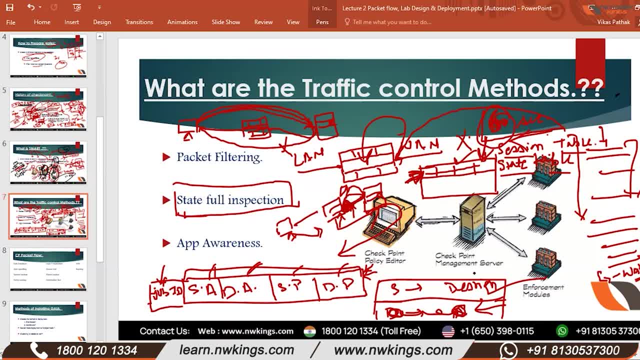 That from destination Source connection Communication will be allowed. So this small story Of the stateful Did you understand or not? And in this, Tell me quickly What are the doubts. I will clear it now, Because if you have any doubt in this, Then you will have a problem. 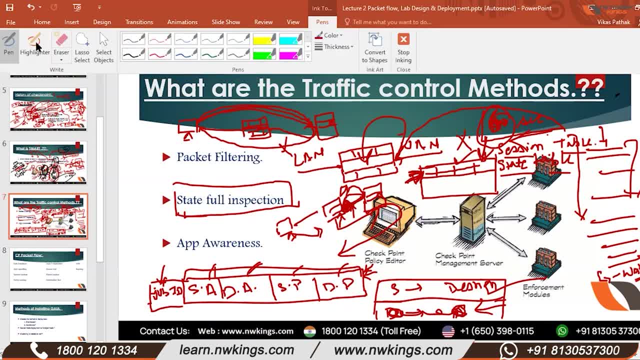 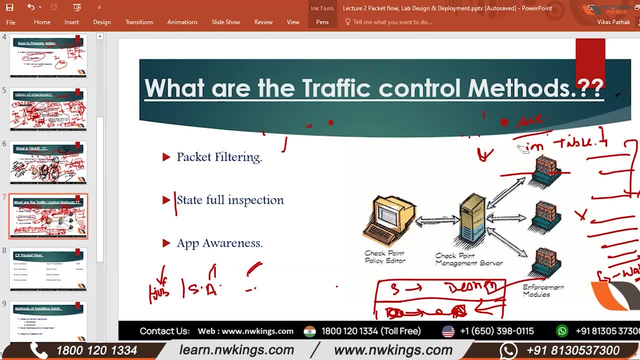 I am telling you first Because it is clear. Should I say something else? Yes, So I hope That this session table, Or the state table, You have understood. We move forward Now. the third point, The third control, Traffic control method. That is called app awareness. What is that App awareness? 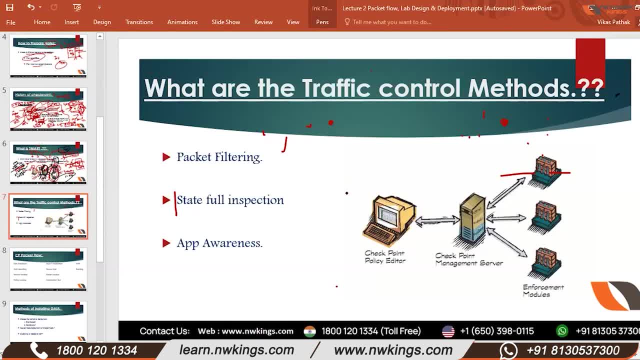 Now, how does this app awareness work? What I gave you Example: Facebook And Facebook Games, This Differentiation That is called app awareness. Now, Assume One: This is a URL. What is the URL? What is the normal URL? Assume that it is the URL of NTP. OK, Now your application manager. 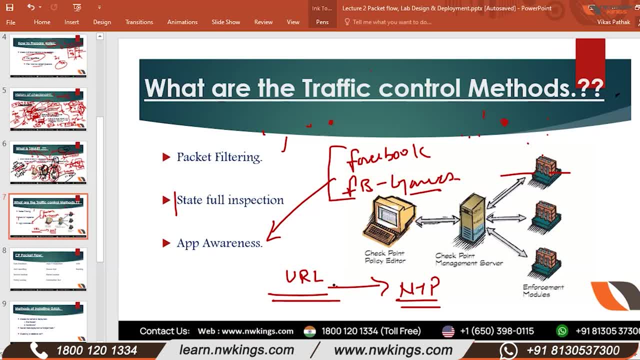 They did not have much knowledge. They came to our- What do you call it? Internet. They searched NTP. They got a URL. OK, They generated you a request That, Because You have this URL Through my application Or for my users, You allow, You said: Open a rule on Fireball. 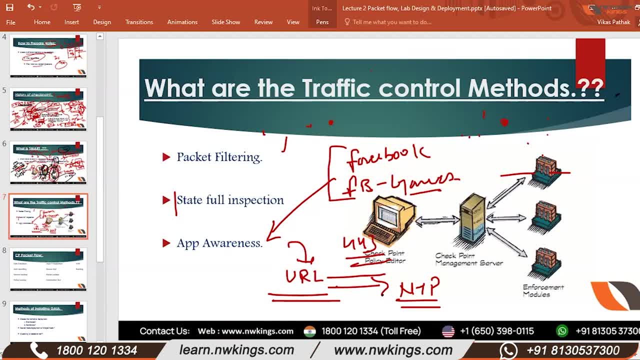 Now 443 Allowed. Now, what happened That 443, Which was allowed After certain period of time? This NTP, The application, was hosted On that URL. It has become a gambling site Now. OK, Now what happened That? unknowingly For your users, This gambling site Is this gambling site. 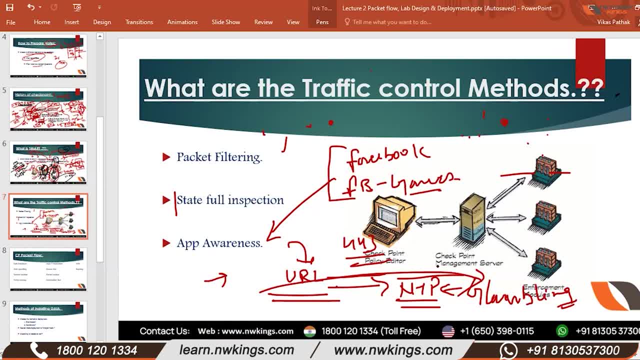 Accessible? Or Is the adultery site Accessible? Or Assume that YouTube is not allowed In your organization, OK, But Anyhow The YouTube is allowed. So How is this happening? Because Those firewalls Are not doing Application Awareness Mechanism- OK, Which Can't catch people One. I give a real scenario. 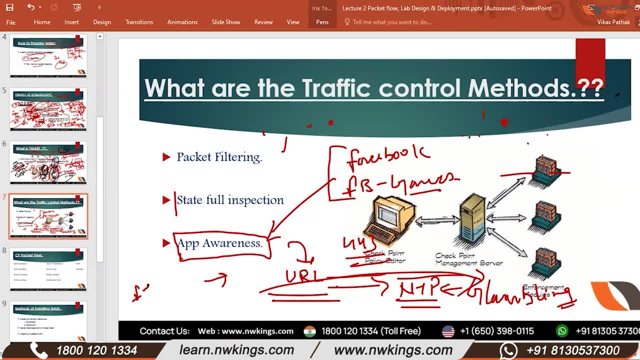 FTP is there. No one will tell me What is the port number of FTP. FTP has two port numbers: 20 and 21. One is for control pin, Another is for data update. OK, I guess It is 20 and 21. 22 is for SSH, 21. 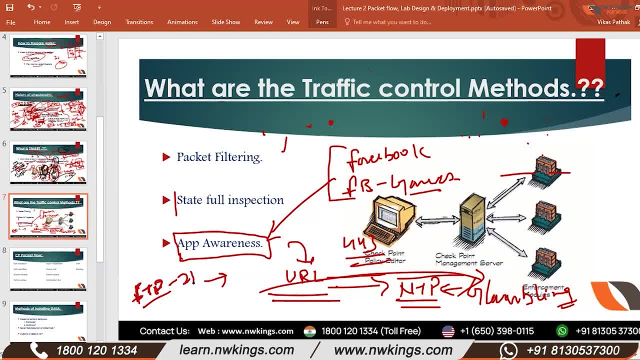 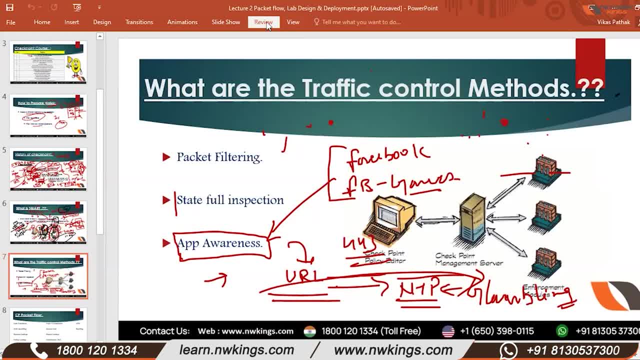 Okay, so you said that the data you have, if it is in 20 or 21,, it will be in plain If I want to do it in encryption. but if it is happening in plain, it is a risk, isn't it? 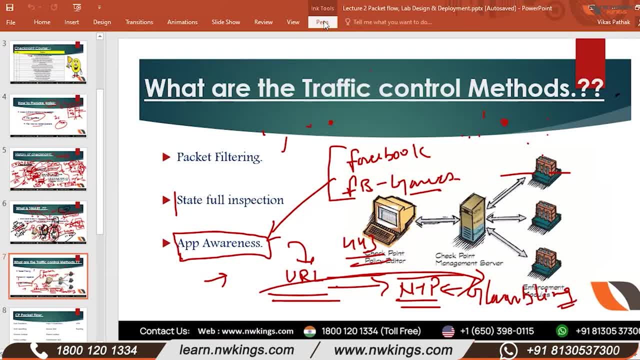 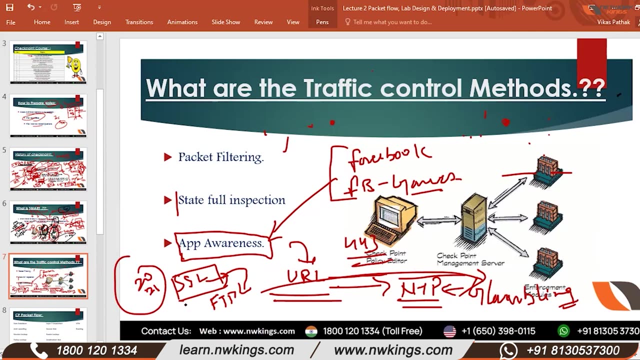 We will use SSL over FTP or we will use any other mechanism. SSL over FTP? Now, if you used SSL over FTP, then you definitely can't use 20 and 21.. No, Then what port you will use? Port 22.. 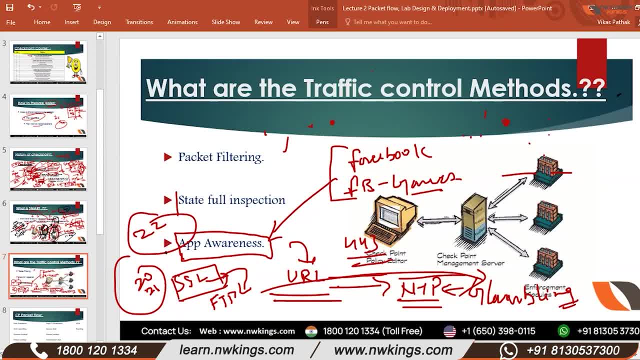 Okay, It will support this. Now see, what is interesting is that if you made a rule and instead of allowing port 20,, 21,, 22 in the service section, if you put FTP, then this encryption. the story of FTP is that I have to forward the traffic in encrypted form. 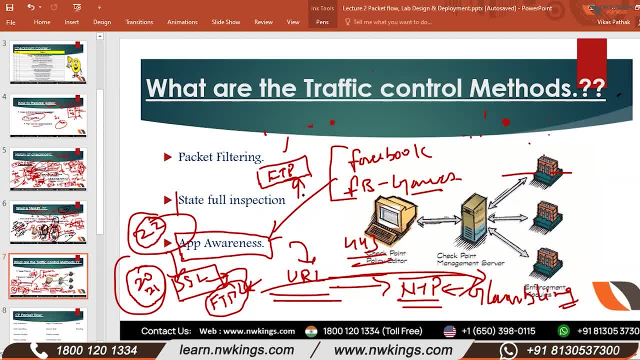 It will never be completed. It will always drop. Why? Because what you have done, FTP is allowed. FTP is allowed And the default port of FTP is 20 and 21. 21. Now you have used application awareness. your 22 will never be allowed. 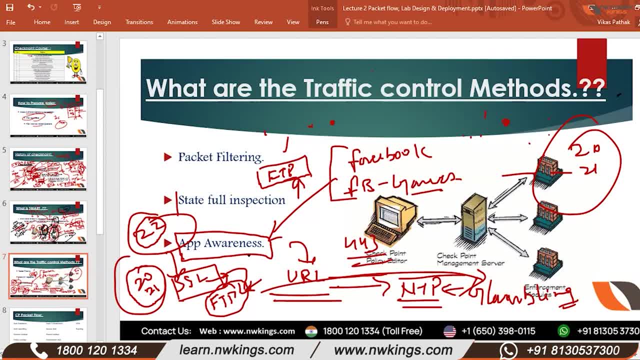 Why? Because firewall is saying that, according to the instruction you have given me, FTP is allowed, And my database says that the default port number of FTP is 20 and 21.. So I am not going to allow anything else, But the traffic coming from your source is 22.. 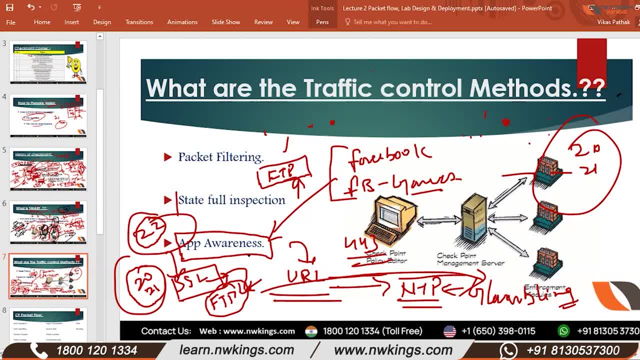 In that case you will have to allow any in the service section instead of default. The application is your FTP, But anyone can come to the service section for FTP, Or you can define in particular that port 22 can come. Are you getting my point? 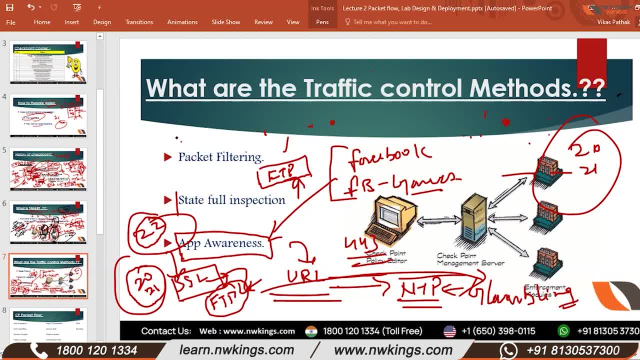 Yes. So what happens? This feature is with everyone, This feature is with someone and this feature is also with someone, But if I talk about major firewalls, follow It follows these three approaches: rigorously, Rigorously, Checkpoint. 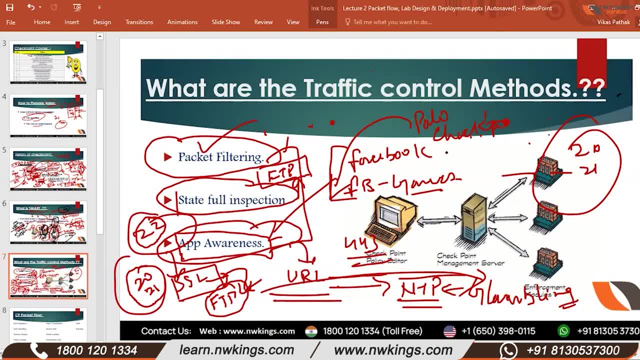 Forty gate. These three firewalls- I told you about these three major firewalls- follow these three approaches, These three features. Vikas, this concept you have explained a little bit again. I actually have a background in routing, So it's fine. 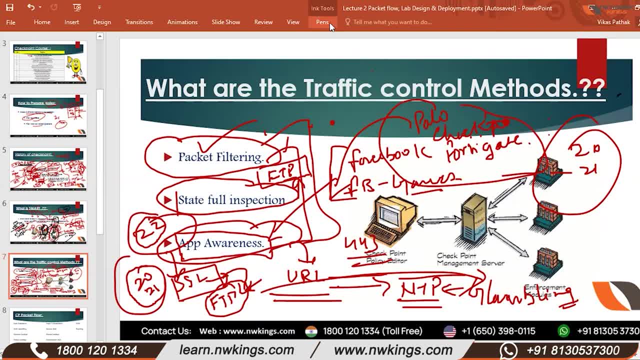 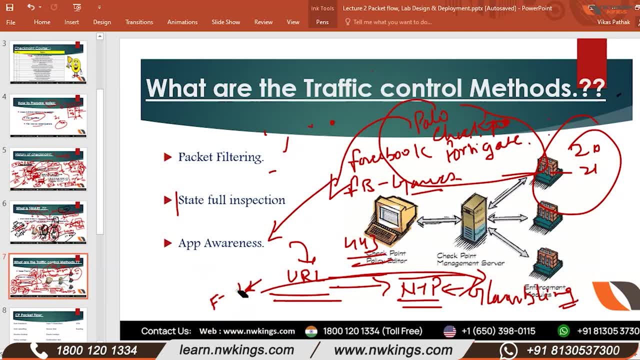 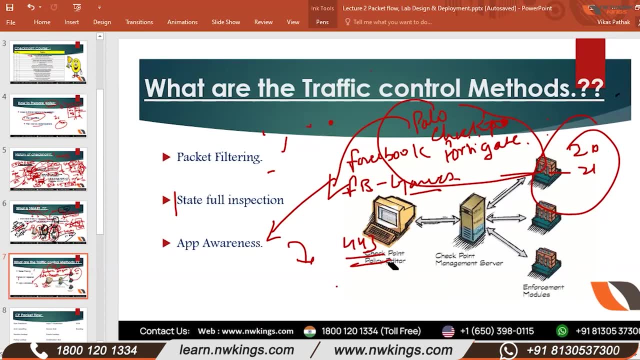 The port for FTP will be 20 and 21.. Other than that, Hmm, FTP, So 22.. I mean, where do we have to allow it to pass through the traffic? I'll explain. Wait a minute. Okay, Do you know? FTP. 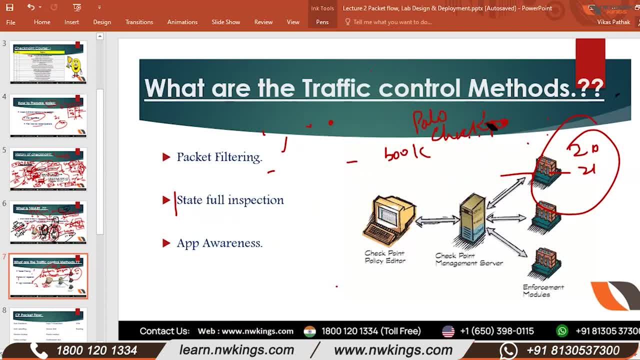 Why do we use FTP? Absolutely Yes, Its port number is known. Okay, Port number 21. 22. Okay, What do we do? Let's make a scenario, Small one, In which we- If I am reading fast, 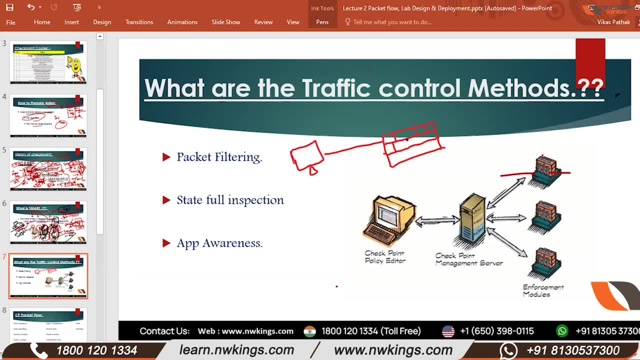 Guys tell me I'll slow it down a little bit. I don't feel like I'm reading fast, But still No, Vikas, It's absolutely fine. This is my client. Okay, This is my server. Now what happens? 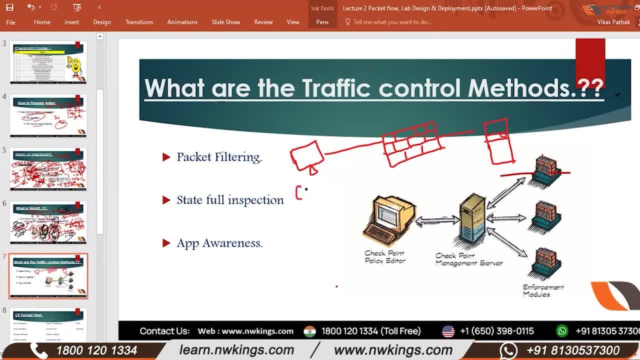 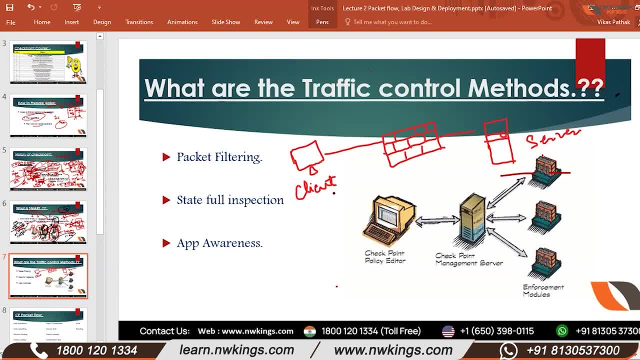 Yes, Yes, Yes, As there is a jede Right. So what happens is that, until the server is not in LAN, we recommend that you use port 20 or 21.. As soon as it goes out of LAN, we recommend that you do one thing: you cannot use port 20 or 21,. you can use port 22.. 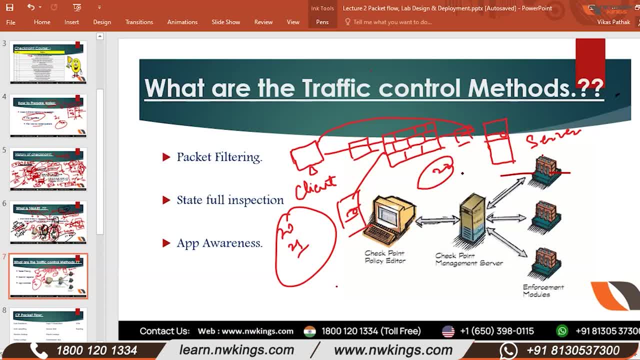 Or any other port you want to use for the encryption. Now, for whom is 22 for? For SSL. What does SSL provide? Encryption Right. So as soon as you have your FTP application, SSL and FTP combined, we call it SFTP. 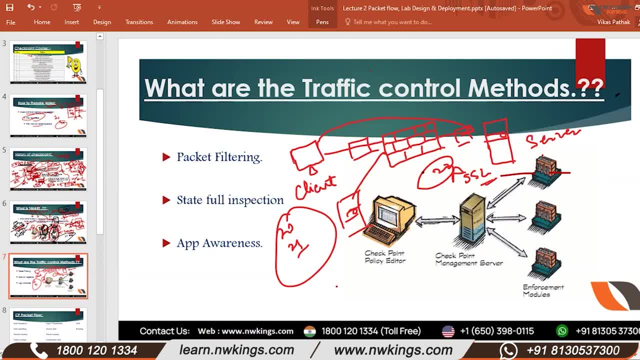 Yes, yes, yes, yes, yes. As soon as you enable SSL on your application, the traffic that it will send by default will be sent to your port number 22.. Okay, But the rule that you have made in Firewall Source address: 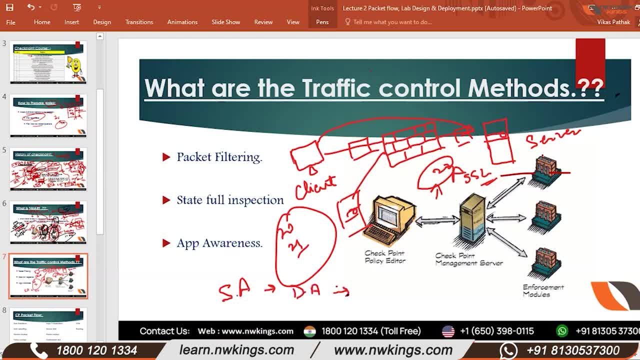 Destination address Application FTP Service. Default Action: Allow Source destination traffic came For FTP application. FTP is allowed. Packet opened. Port 22 user will be checked. Port 22 is being used But the service is default. 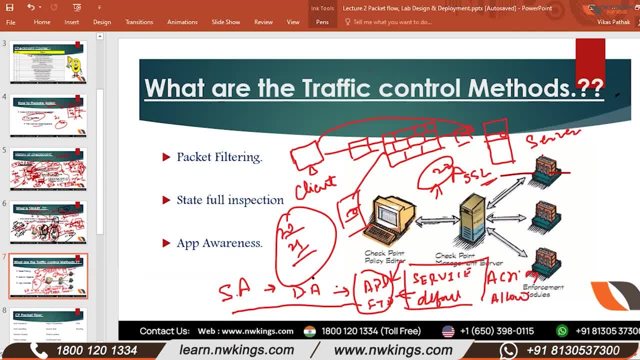 And what is the default service of FTP? 20 and 21.. But the traffic that is coming is coming on 22.. So what happened? Block Deny- Why did it happen? Because this is the application-awareness feature, Sir, can I use 23 instead of 22?? 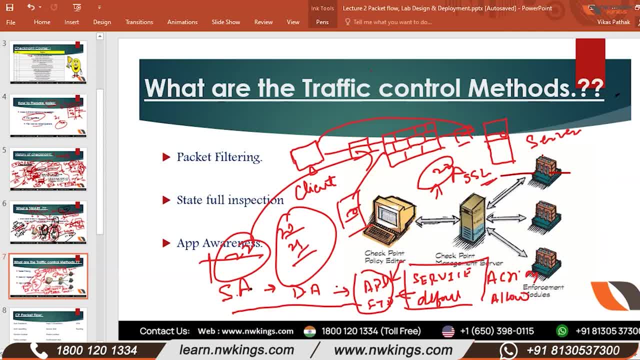 Or is it different? It is different. I think this is different. No, the port 23 is a telnet. It works itself. in plaintext. You give SSL the encryption which it provides to you, So you can use it Or make your own port. 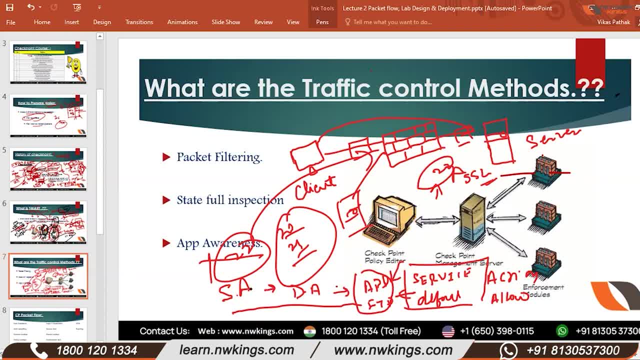 I made FTP on the 5900 port. Now what you have to do is that it provides encryption. there We have created a key, We have put the mechanism of public and private key in the coding there and we are encrypting it, and decryption is required. 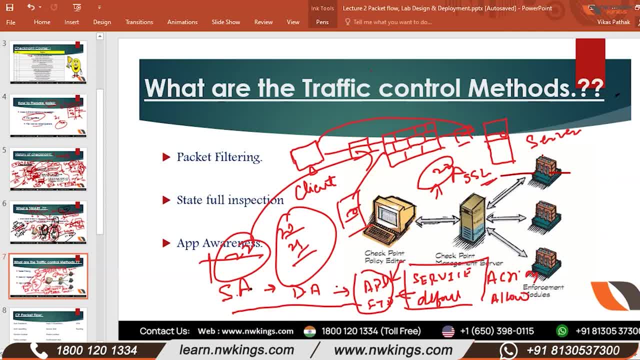 right. so because this is the feature of firewall application awareness. this is the firewall application. now what happens I have seen in many organizations: in rule 443 is allowed and 443 is being attacked. why? because in 443 there is traffic of other application coming. do you understand? 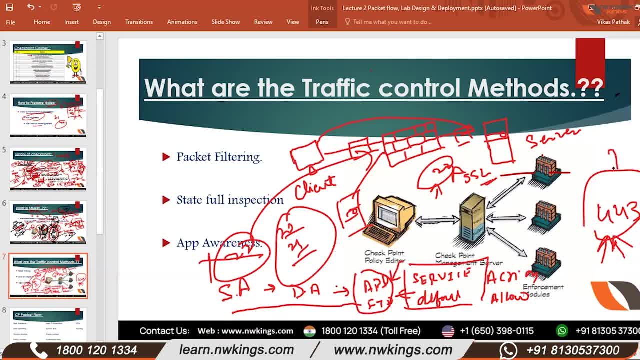 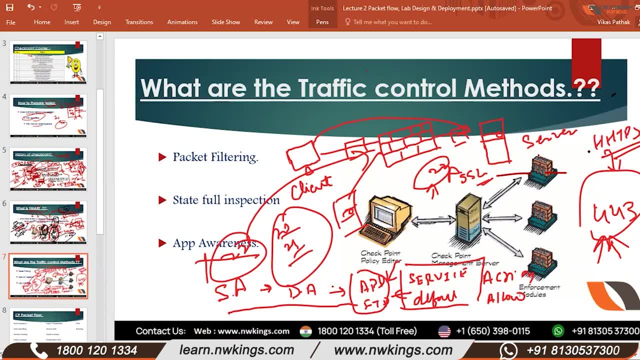 so that's why it is said that you don't allow 443, you allow HTTPS. if you have allowed HTTPS, then what is firewall doing? it will check what is the application- HTTPS. after that. it will not check the packet that what is the port inside? 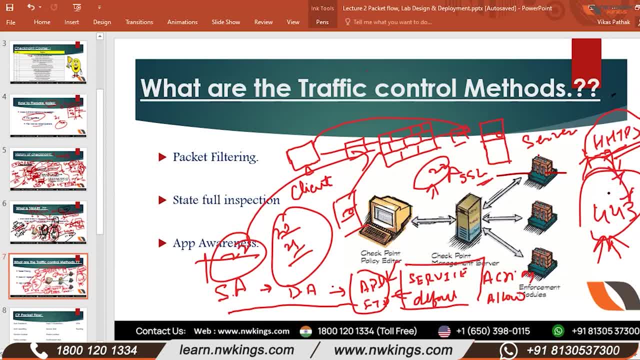 it knows HTTPS for 443, so it will check 443. if there is any other port other than 443, it will deny immediately deny. if you have allowed 443, then consider the traffic and encrypt it. from any other port, it will be denied immediately. 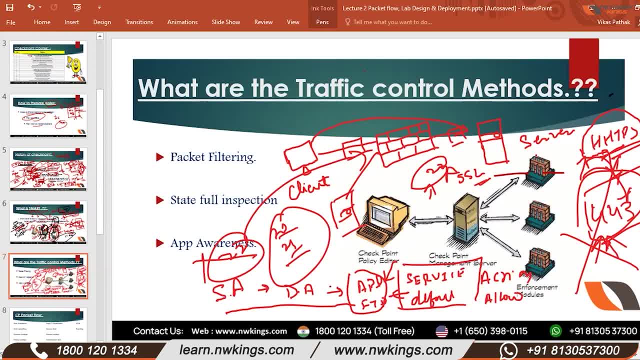 if we have allowed port, either way, from my perspective, 443 you have mentioned, or HTTPS. so in the case of 443, how will it be attacked? what happens? I will tell you. so, on the router, normally we give source to destination port, etc. 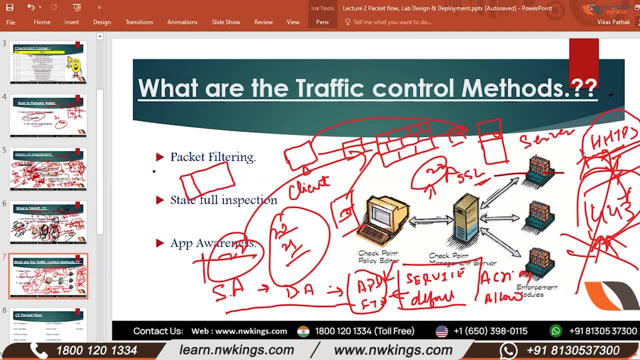 or mention the application. this is your application header. here your 443 is mentioned, but data inside. is it 443 data or is it exe file which is installed on your computer as soon as it reaches you? how will you identify that, bro? you have installed 443. 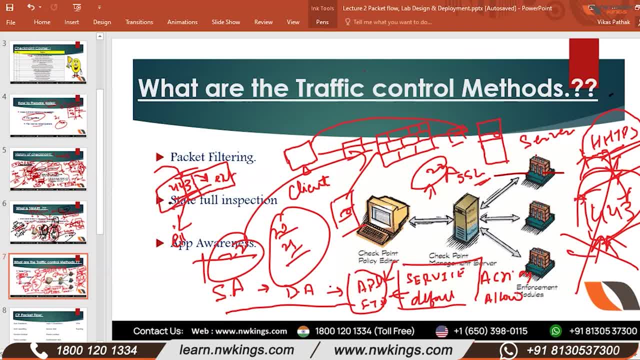 right, you have seen the application header 443, you have allowed it, but this application is exe file. can you attach exe file on the HTTP? it is not feasible. yes, so how will it be identified? yes, sometimes we have clicked on the link. what is the link? 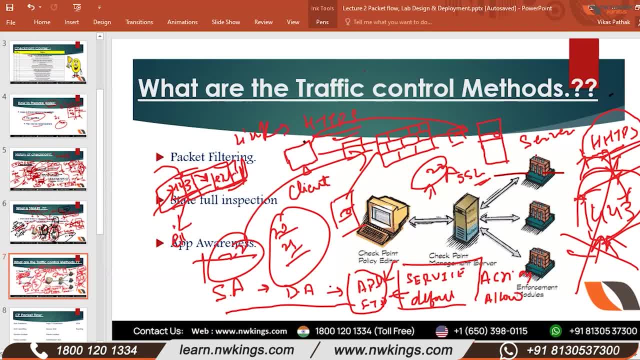 of HTTP and as soon as we clicked on the link, the application is downloaded, it is installed and it has gone. and where it has gone, we don't know. look, phishing attack is done now where it is roaming in your network. nobody knows in that situation what we do. 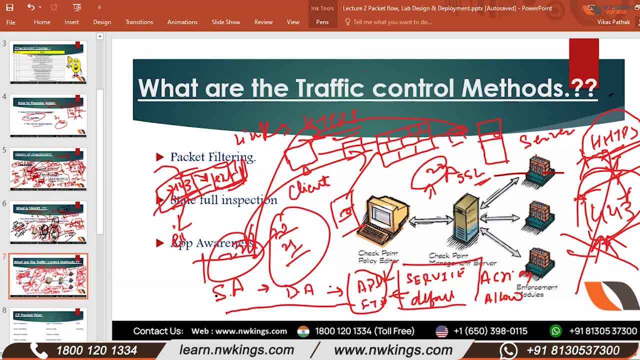 we give a manual call to antivirus that expand the entire network. so that's why, that's why we say: train the user. no matter how many firewalls you install, no matter how many sims you install, no matter how many sim tools you install, no matter how many cyber security teams you set up. 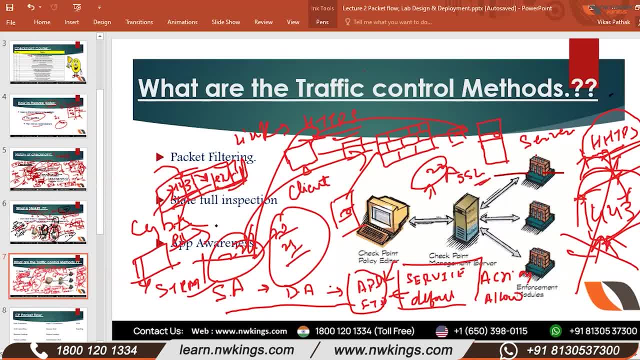 until or unless your user is not aware, you cannot stop any phishing, any DDoS. no, you cannot do that. so one question sometimes means in network security it is not asked, but sometimes there is a scenario where there is a discussion or somewhere: the best, the best protection. 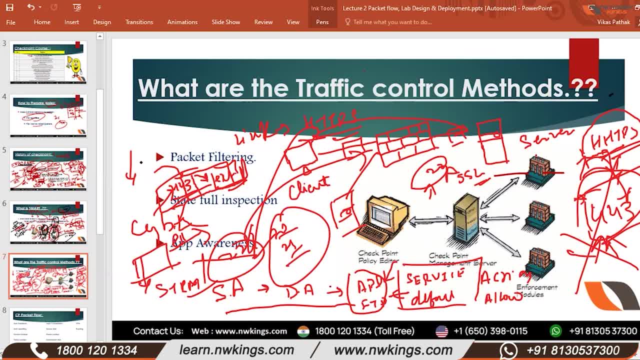 is considered, what is considered in network security, and one of the options is train your users. if you have spent crores of rupees on infrastructure but your user is not aware, believe me, it will not make any, any difference, because links are coming and if your user has to click on the link, 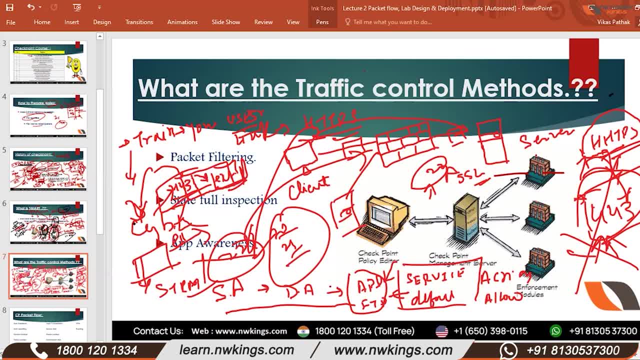 then things are done. but yes, this thing is that if you have made a good infrastructure, policies are made well, you have properly controlled change management. it is not that any L1 in your team, any person is coming, he is opening any rule and going. if you control this thing, 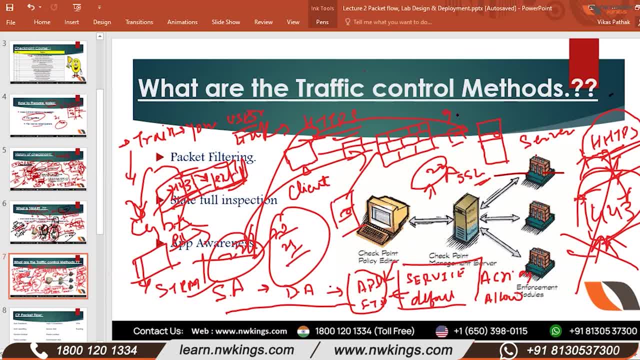 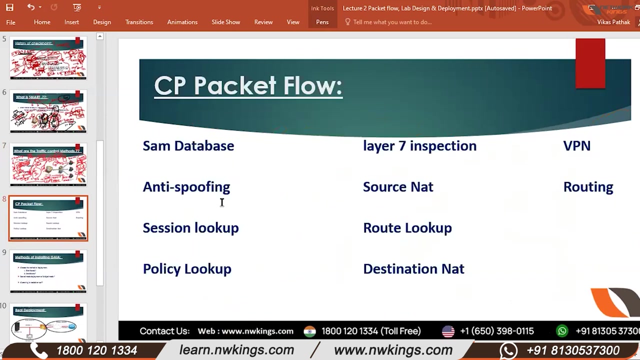 then believe me- 99% success rate- that you can stop all these vulnerabilities at your firewall level, or you can catch them with sim, or vice versa. is it clear? yes, sir, thank you, any other out? no, the way we will go, then I love more things ok. 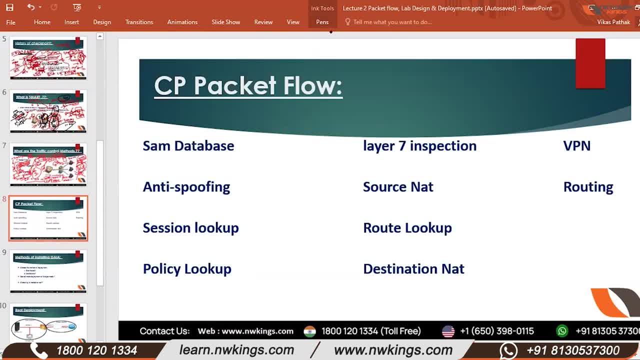 hope you guys are making some short notes, right, right, ok, ok, ok, ok, ok, ok, ok, most, most, most, most, most, most all of these, most 1000 square, the most we will make. that much important topic is this. ok, this is the main topic for today. if you have a break. 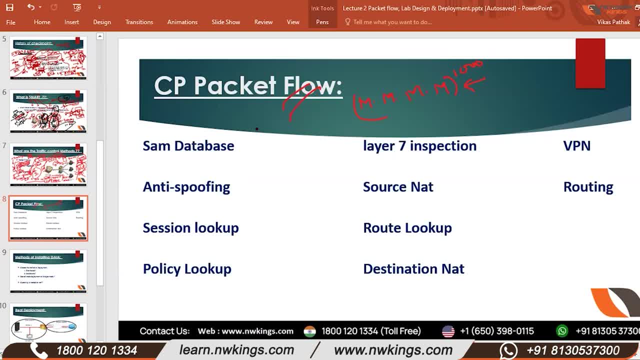 do it. if you have a break, then take a break. take a break 5 min. but this topic don't take very lightly. check point packet flow because it is the topic to read once. there is no rocket science, but if you do not read carefully it will go above the head. 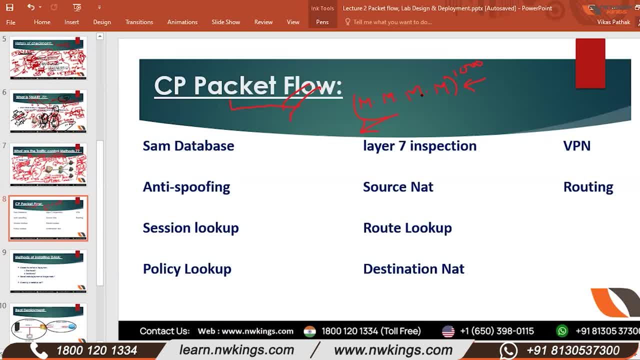 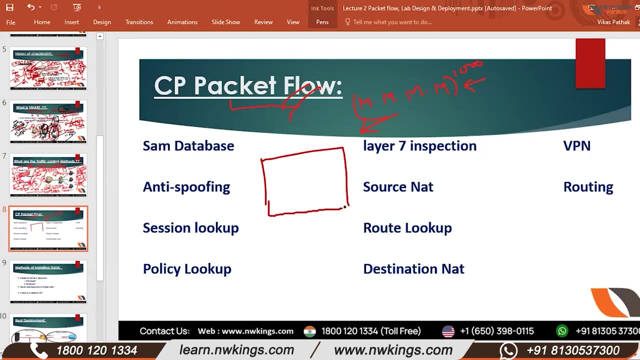 then take a 2 min break. 1.17 are happening. we will start at 1.19. ok, ok, it is ok. Stateful inspection is a Firewall that maintains a table. In that table Firewall maintains Source Destination. Source Port, Destination Port. 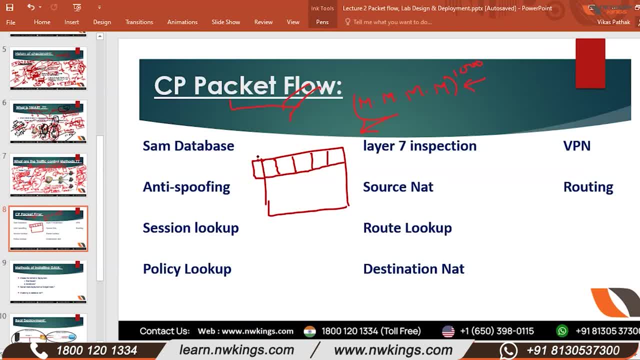 and the Job ID. It maintains all these information For what it maintains. It maintains all the traffic that comes out of the Firewall initially. Why? So that when the traffic reaches the destination and when it comes back under a specific time, it will not check a policy for the return traffic. 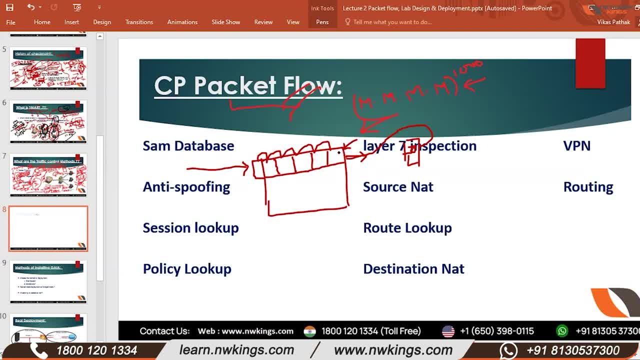 It will check the session table or maybe state table, And that traffic will be allowed on the basis of that table. If the entry is in the state table for that source and destination, it will be allowed by default. Otherwise it will be denied. 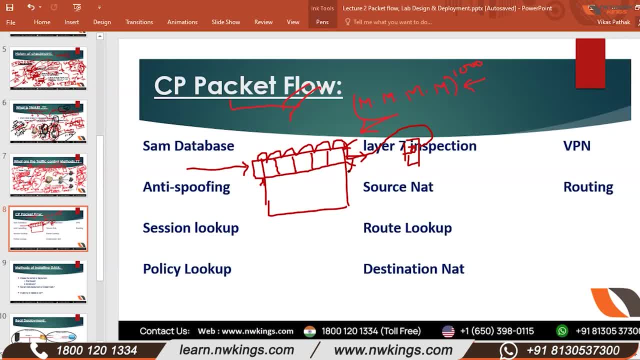 Okay, What do you mean, sir? You mean that it should be returned at a particular time, right? Yes, If we do not maintain the timing, then the buffer of the state table of the firewall will be very large. Okay, How much traffic do we get from here that we can't get back? 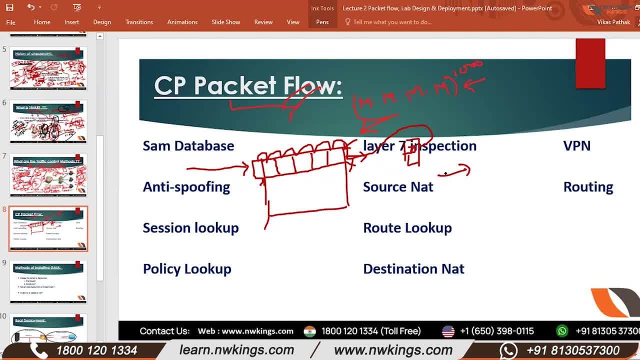 But if we make all of them, then there will be a lot of problem. Okay, got it By default. the timings are 36 seconds. It is between 30 and 60. And these timings are different. I will tell you later. 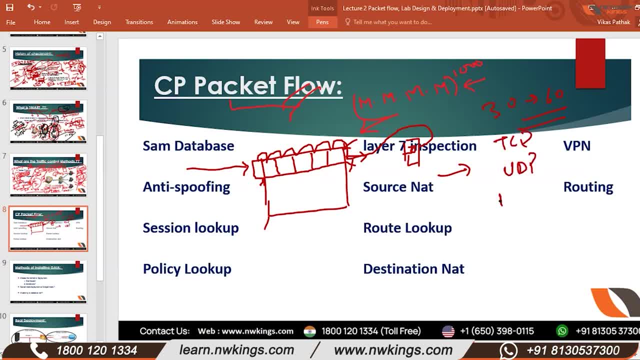 There is a different timing for TCP. there is a different timing for UDP. there is a different timing for NAT. I will tell you later. This is a very important topic. Troubleshooting is very useful for me, So I don't want to make it a part of discussion. 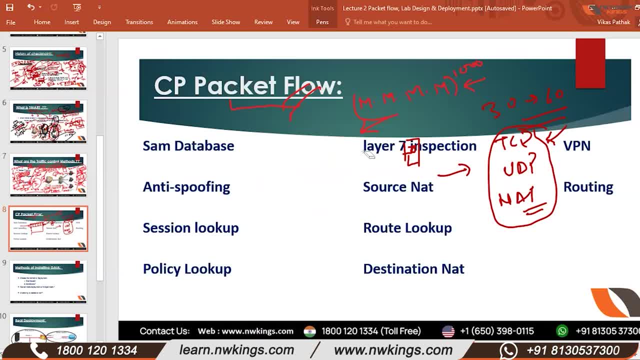 I will tell you later, Don't worry, Just tell me. if you have any doubt in the topic that I am discussing, then immediately you can ask me: Sir, can we clear the session table manually? Manually is not recommended, It is not recommended, but you can do it. 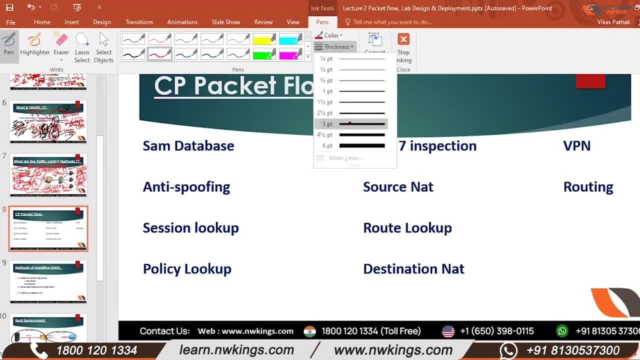 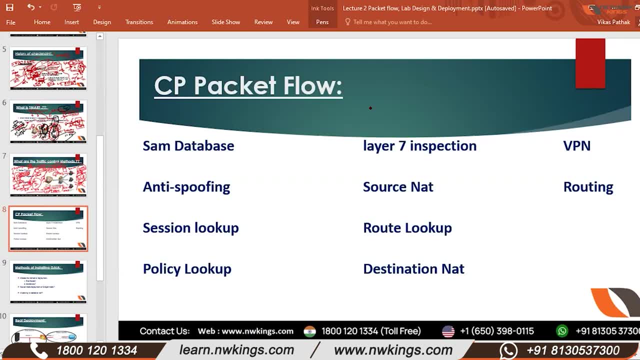 You are saying it by mistake that someone has done it in production. If you have done it manually, then all the connectivity will be lost. It doesn't even happen like this. Is there an option to do it manually or not? There is no such option on GUI. 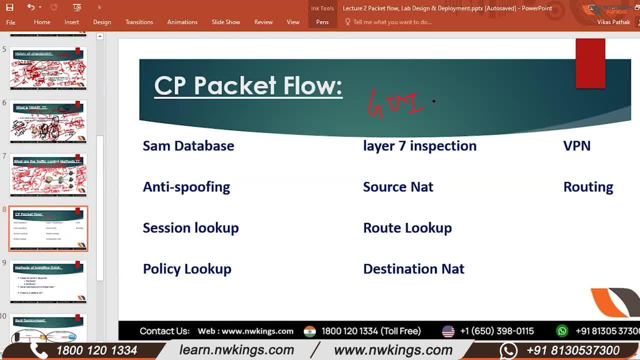 There is no such option on GUI. You can do it through CLI. Can we check whether this session is made in the session or not? Yes, you can check the job ID. Okay, The session is made. you will see it in the log, right. 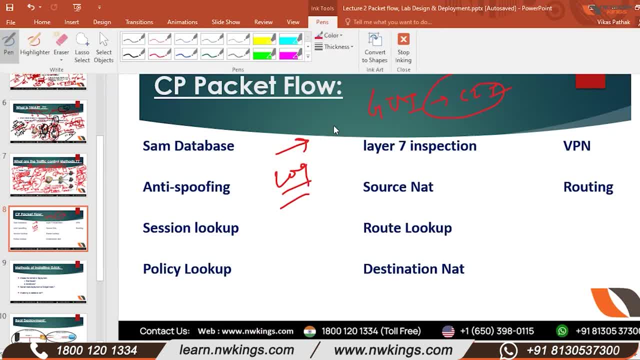 Do you understand? Yes, it is clear. It took a lot of time. It is automatic. The log table will not be clear. The session table will be clear. The log table will not be clear. Okay, Do you understand? Yes, 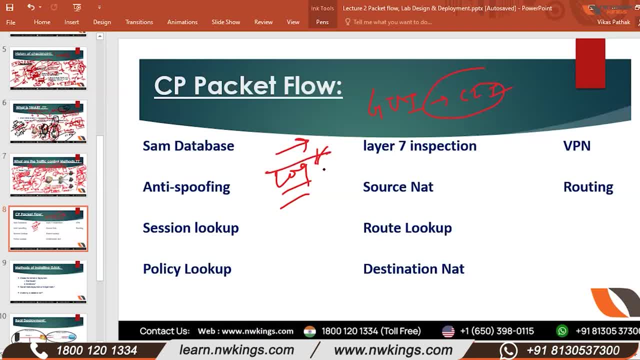 You can see it in the log. Suppose the session table is lost by someone. However, if the session table is lost, then the traffic that is coming back will be denied And the person who works according to TCP will immediately send a request to retransmit. 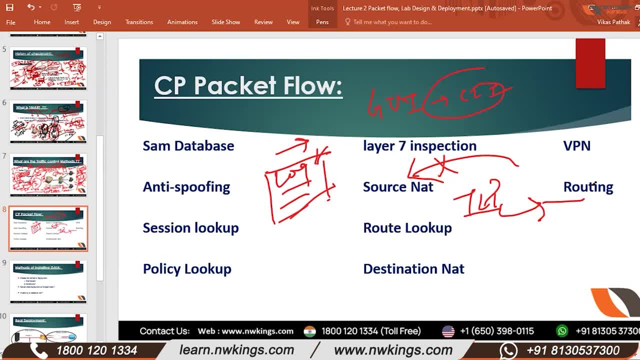 And as soon as the request is sent to retransmit, the session table will be maintained And in the session table, reboot and other devices are clear in that condition. In that case, the whole thing is clear, Sir. a new session will be made again. 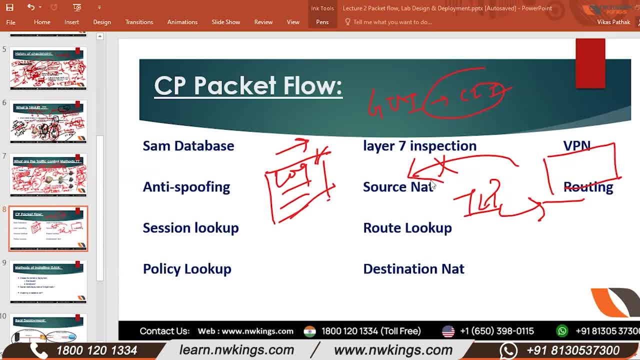 One minute. Say it again. What are you saying? If the device is rebooted, then the whole thing is clear. in that case, right? Yes, in that case it is obvious that you have rebooted the device. Sam, this is our first class. 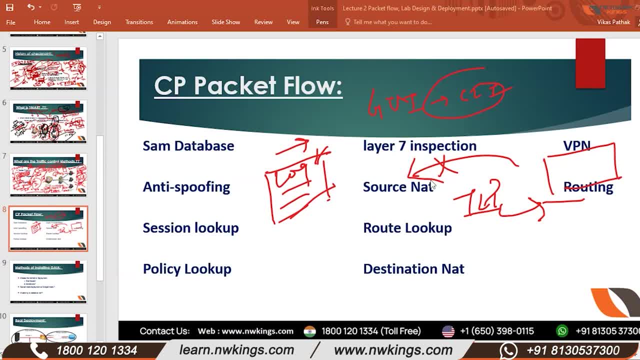 Okay, We did not discuss much in the first class. We discussed the basics, And I have covered that basic in this class too. If you have any doubts, then you can tell me. I will clear it for you. I will try to clear it for you. 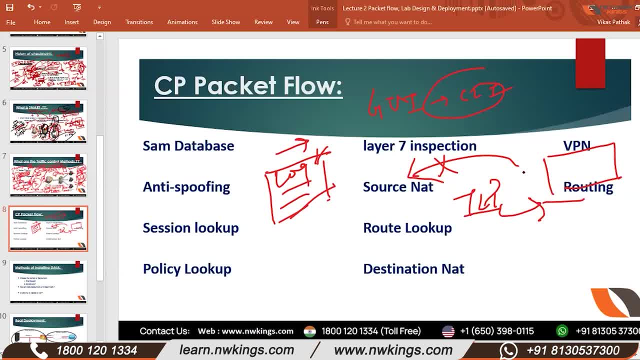 Okay, Thank you. And if you have, If your firewall is rebooted, see this: This is your firewall in the cluster. You are also going here. That session is being replicated here, Do you understand? If this firewall is rebooted, then the connection will be here. 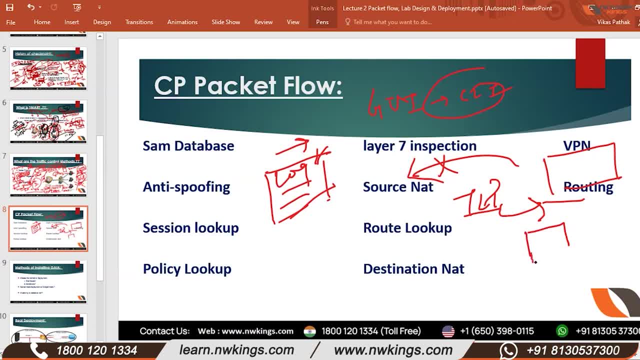 Hi, you are watching the recording from one of our live session. Hit like share and subscribe to our YouTube channel. We will talk to you in the next class. Thank you, You are also going here. You are also going here. We will talk to you in the next class. 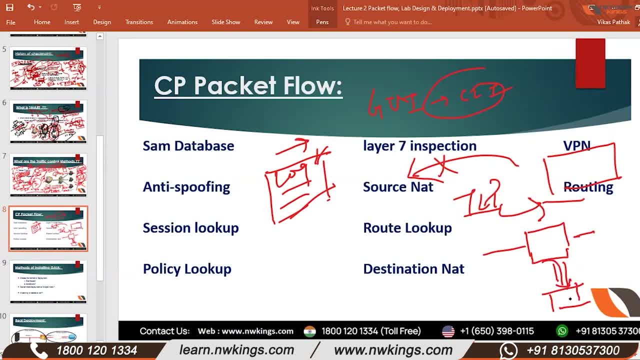 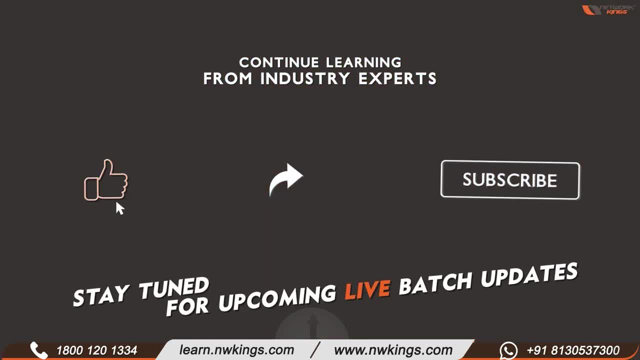 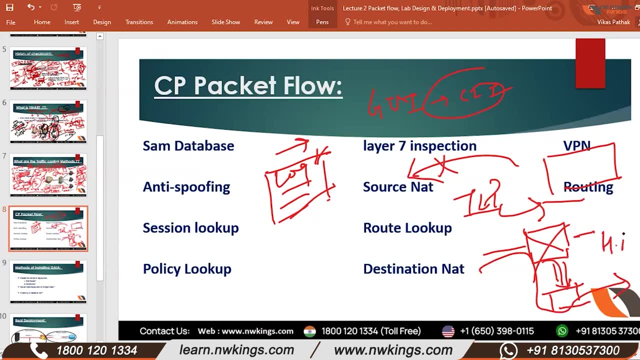 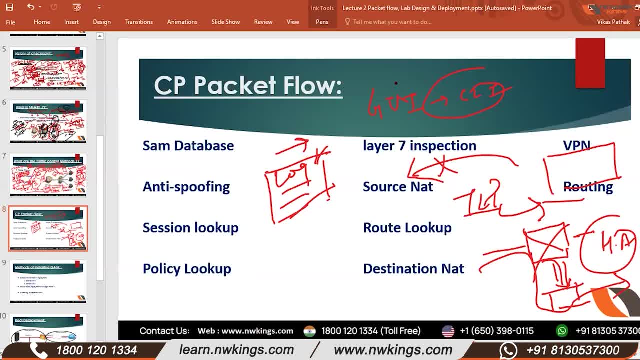 Yes, that's right. Right, Does it make sense, or not? Got it? Thank you? So shall we start guys? Give us a confirmation once And everyone should be ready. This is a crucial topic for us. Yes, sir. 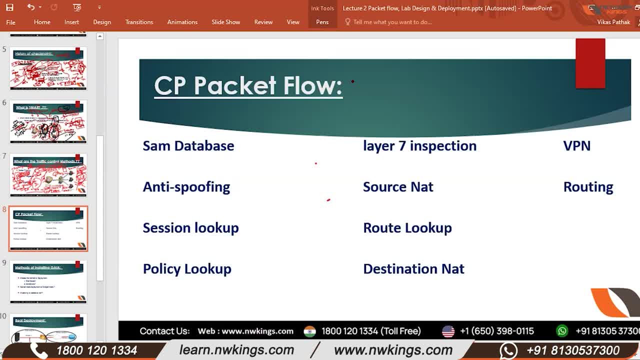 Sir, tell me one more thing. Can we put a capture of this packet? Can we put a capture of this packet on Wireshark? Yes, absolutely, You can put a capture. You can import it on Wireshark, You can analyze it. 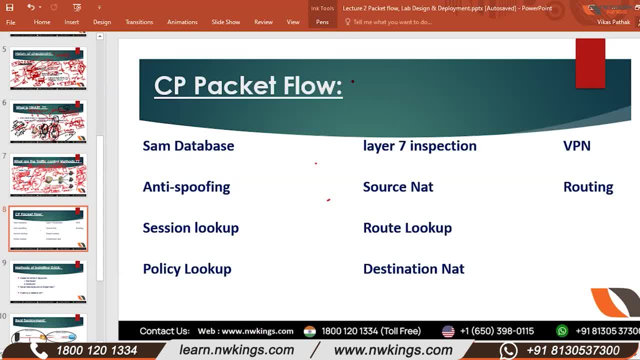 These are basic things. If you can't do this, then what's the use of debugging? Let's go Checkpoint packet flow. It's a very important topic. I will tell you very slowly, Very slowly. I will tell you in easy language. 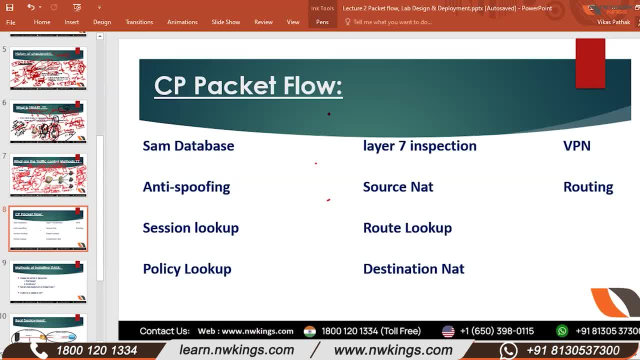 You have to listen, and listen actively. You have to become an active listener. This is firewall, This is LAN, This is WAN. Okay, Traffic came from here, User initiated from LAN side, Or traffic came from outside and hit outside interface. 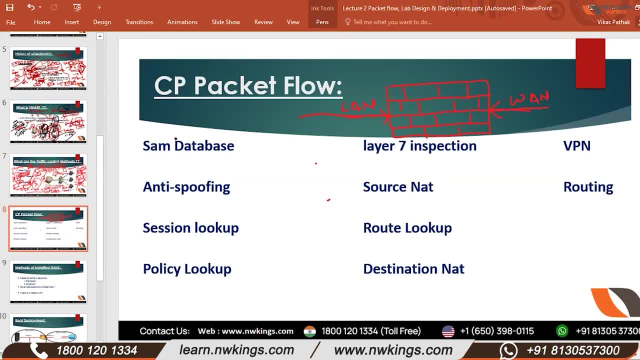 Okay, First of all, what is checked? That is called SAM database. Now, what is SAM database? On the interface level of firewall? Okay, On this interface level, a database is created in which, if you have created a rule of allow, 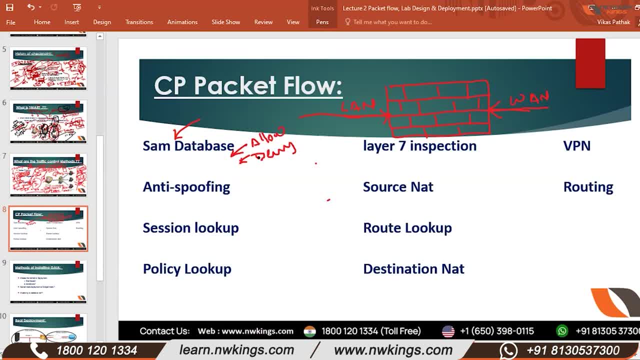 or deny, then that packet will be forwarded from here If it is allowed. Otherwise it will be dropped here. Got it? Yes, sir, Let me repeat: SAM database is a database where, if you have allowed or denied traffic of any source and destination, 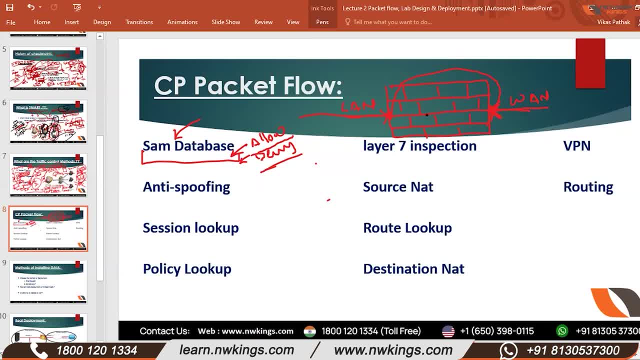 that traffic will not be processed by firewall. Sorry, The database you have created is on interface level. If it is allowed, it will be forwarded immediately to the LAN, Or if it is hit on LAN then WAN, Or if it is denied. 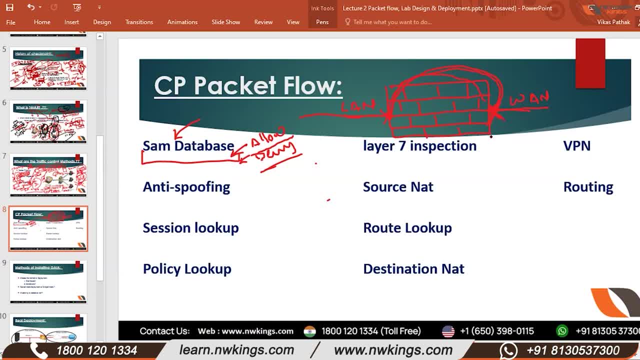 it will be dropped immediately. In 99% cases we make deny in SAM database. In my career I have never seen anyone who has allowed in SAM database. But still there are 1% people who sometimes make it for testing. 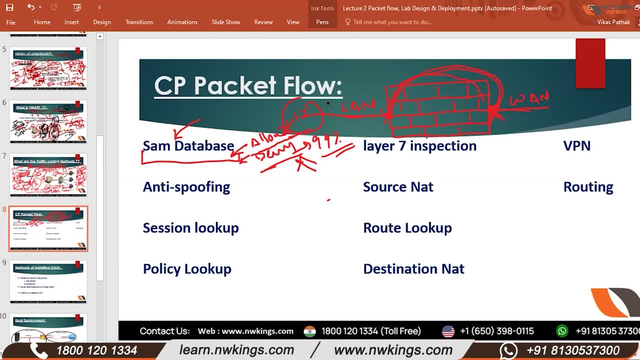 They bypass the firewall. So we make it there, But it is very risky, Very, very, very, If you are allowing any communication through SAM database. it is very risky, Believe me. Okay, Now you must be thinking why we are doing this. 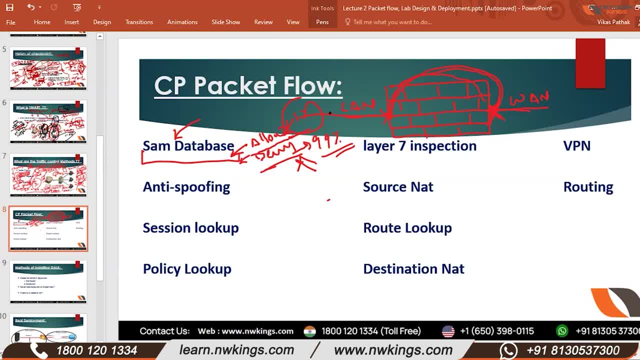 Our firewall is also denying. Why are we doing this in SAM database, Right? No one asked me. If I were in your place, I would have asked this question Because even if traffic goes in firewall, we are denying it. We are denying it. 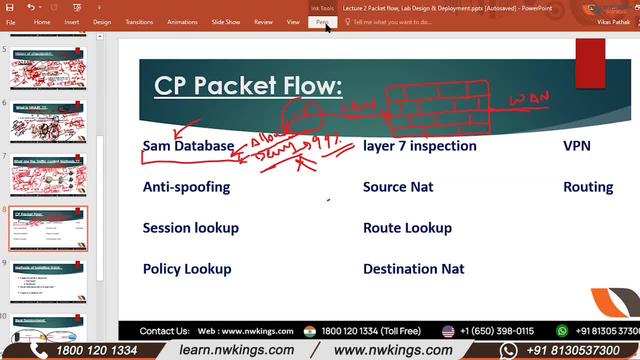 Then why are we doing this, that we have created a proper database in which we are doing this? Why? Because, if it goes in firewall, two things will happen: First, he entered our network And second thing is if he is into the firewall. 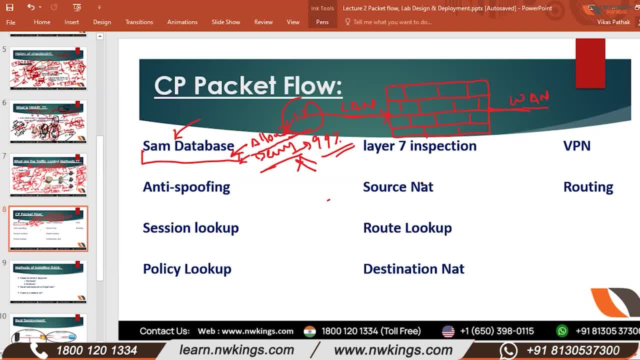 he will utilize the resources of our network. So rather than saving our utilization, we are going to deny him. then, and there itself. Yes, First point, you said he entered the network. Second thing is Firewall utilization. Firewall utilization Utilization. 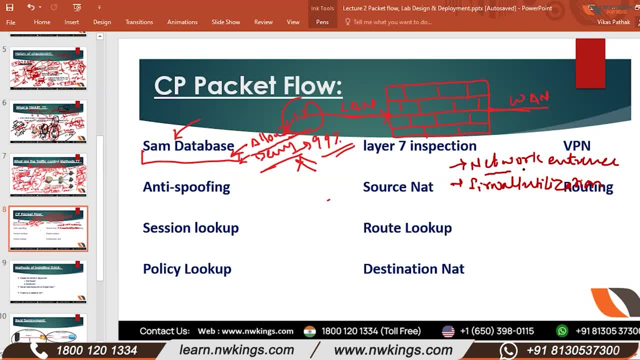 Correct. Yes, The thing about network entrance is wrong. Until it comes out of the interface, there is no network. And if I talk, you mean to say that if my land traffic enters the firewall then it goes to the internet. No, 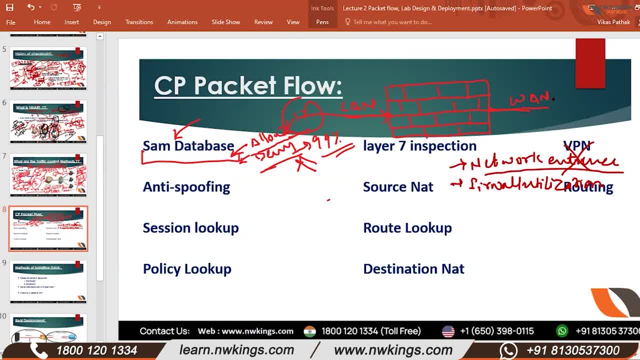 It's wrong. Until it comes out of this interface, it does not go out of the network. Until it comes out of the internet, it will not be called on the internet The traffic that is coming until it does not cross the land interface. 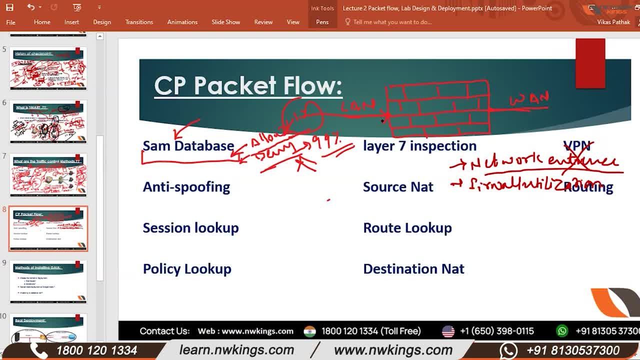 it is not in the network, Correct, Okay, And it will not pass until the firewall is allowed. But firewall utilization? this point is 100% correct And that is the reason we have created SAM database. And what is the logic? 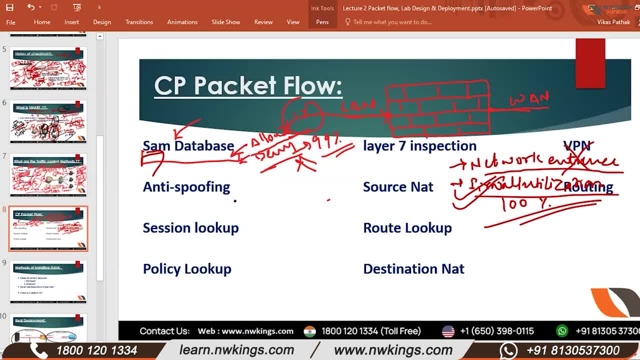 If you talk about logic in the real scenario means okay, I am a person. I have put a request to access a server on the firewall. It should have been blocked on the interface, but it was not blocked on the interface. 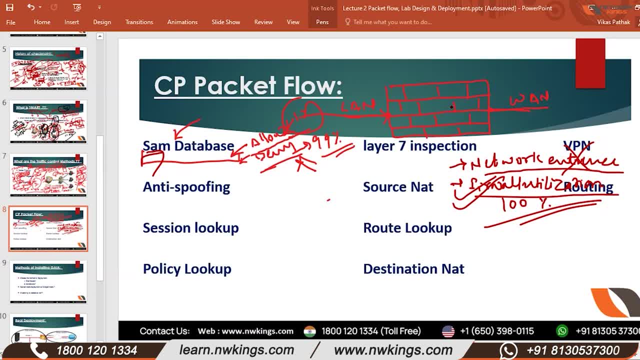 It went inside inside the firewall And the firewall dropped it. So has the TCP utilization increased? No, Nothing happens with one packet. What if there are 1000 packets, 1000 and 1000 packets? In that case, 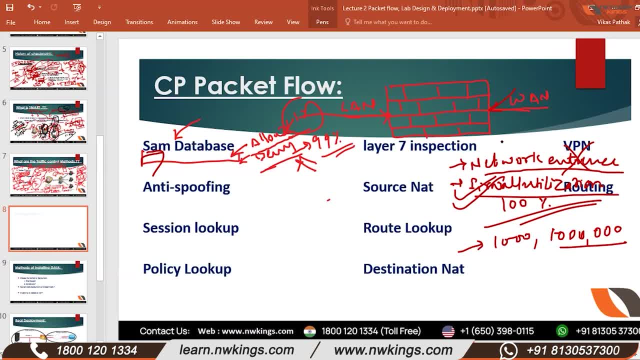 firewall becomes deaf and dumb. Firewall stops working. How to process so many packets And whenever? whenever, okay, leave the firewall. Suppose there is a server. Okay, On the server, you will get these issues in real time. You will work in network security. 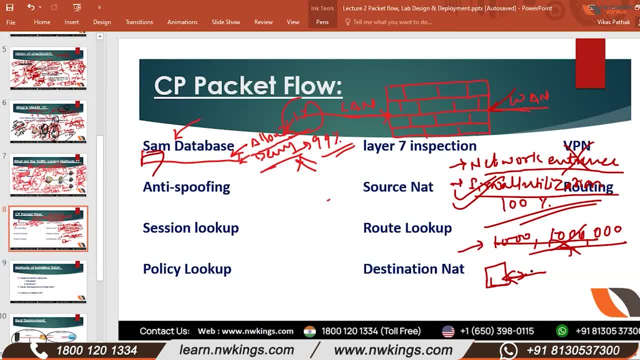 You will have a server guy. He will say: I don't know, there is some unwanted activity on my server. So there are several hits. Where are the hits coming from? From the ESIP. Okay, How many hits are coming? 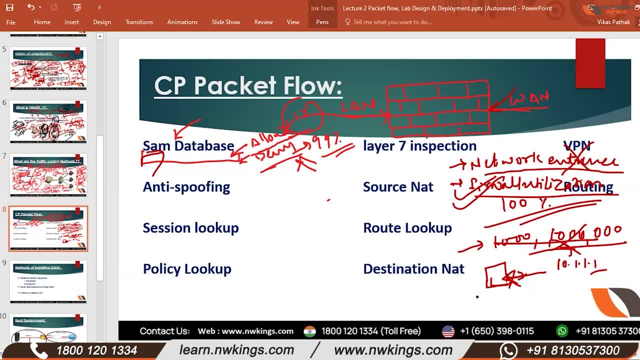 Yes, how many hits are coming? Per second? 1000 are coming. Server utilization is 99%. now Do not ask RAM. I am not doing login on RAM, So I don't need RAM on the server. It will be bad. 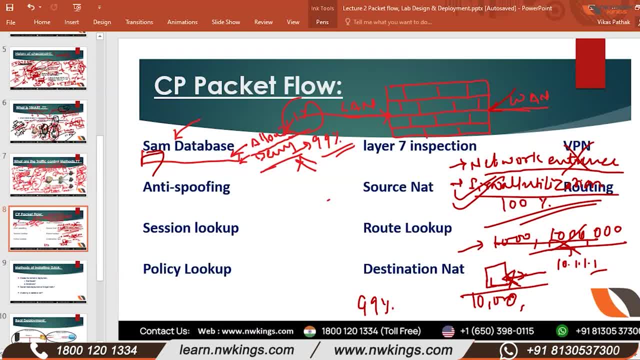 In a few minutes. So what will you do? One option is you go to the change management process. They will say there is a problem with the organization. So go to them and tell them that we are opening a change. what we will do in change is source, is destination. 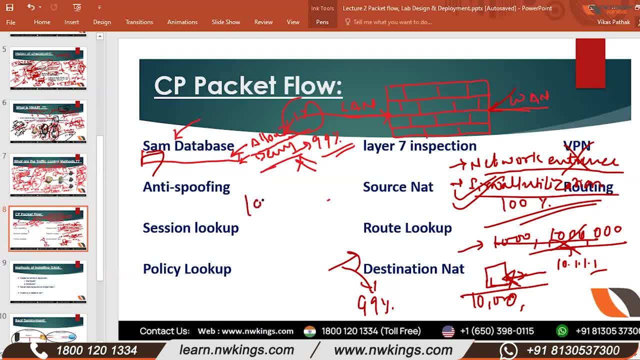 we will make policy now. where will we make policy? 1000 policy is already there, below all. we will make 1001 policy now. when traffic will come on firewall, then first it will check 1000 traffic, after 1000 rule it will drop to 1001. 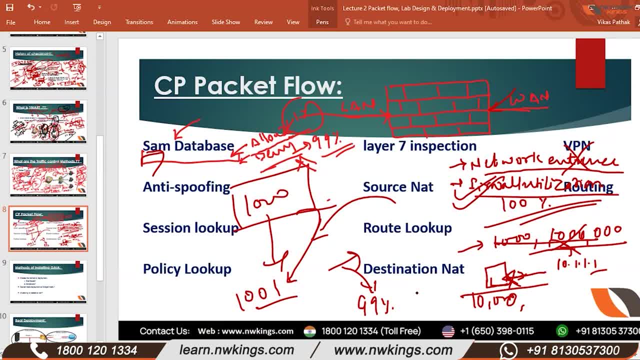 so you solved their problem, increased your problem that every second the 1000 hits that were coming on your server will come on firewall and, in allowing little cpu utilization is less utilized in comparison to deny or drop. I am telling you this experience. so in this situation, 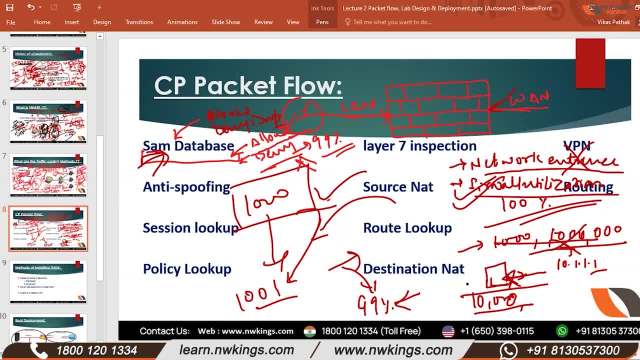 what is the best way? go to the same database. source is this, destination is number 168, 1.1.1.1. and action: anyone allow or, sorry, deny. what will happen is as soon as traffic comes here. source is this destination here: deny immediately. deny on when. 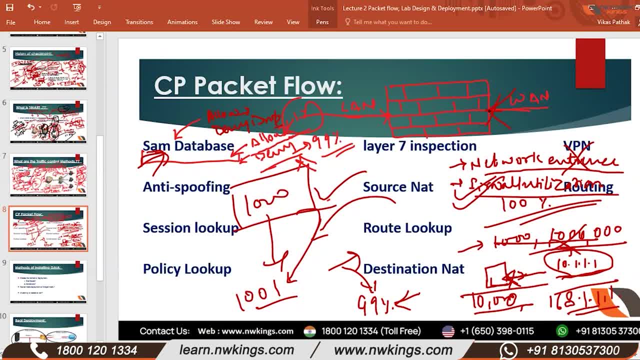 when it will come to the firewall. neither the memory utilization of firewall increased nor anything increased and the server is saved. so this immediate remediation whenever you have to do panic situation, in that case you do this thing and later. this is immediate solution which you can do through emergency change. 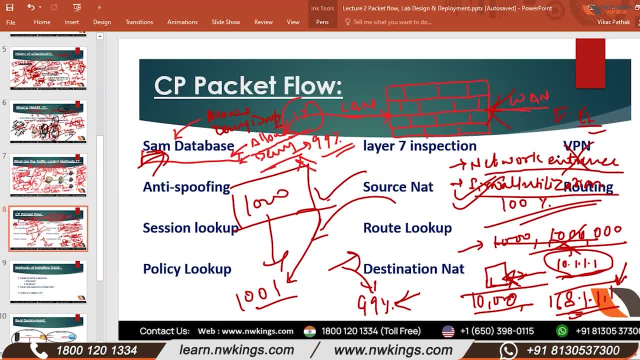 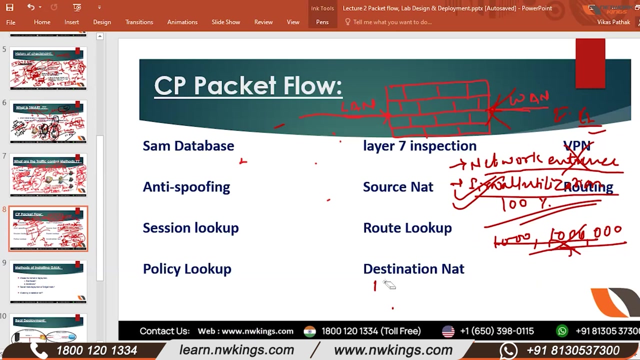 that, brother. you raised the emergency change, you allowed this thing in the same database. after that you have to perform one more change, normal, by removing it from the same database, to bring it in your policy section. got it or not? any doubt? hello, yes, please, sir, sir, sir. 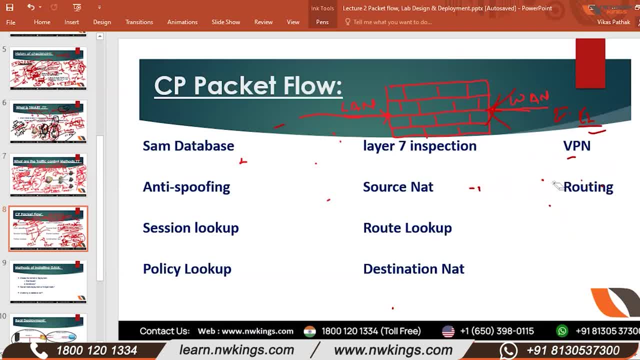 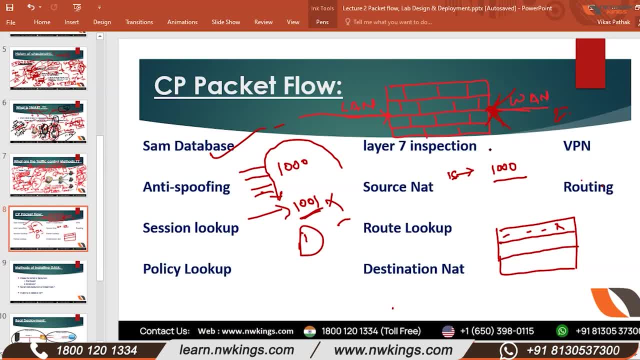 sir, sir, sir, sir. I asked sir, what is SAM database, sir? from where does this topic come from? SAM database: does this CP belong to the packet flow of our checkpoint? we are SAM database. this is the first step of your check point packet flow. if the traffic hits your firewall, then the 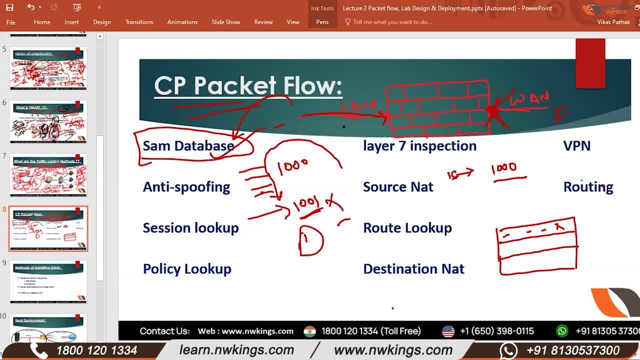 first thing that will be checked is the same database that the source and destination is coming in, whether its entry is in our SAM database. if it is in the same database, then immediately drop it. you got it. so the first stage of the checkpoint is called SAM database. 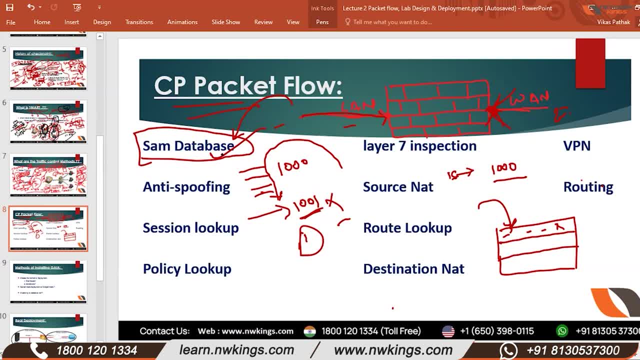 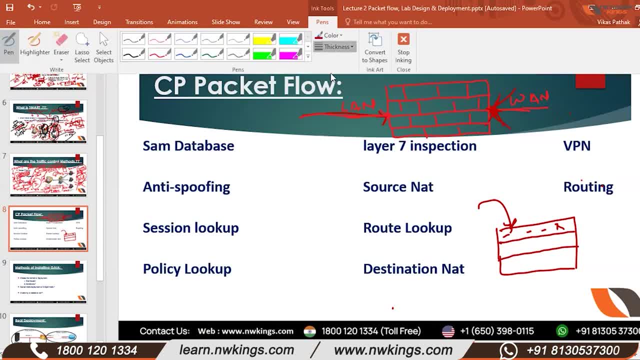 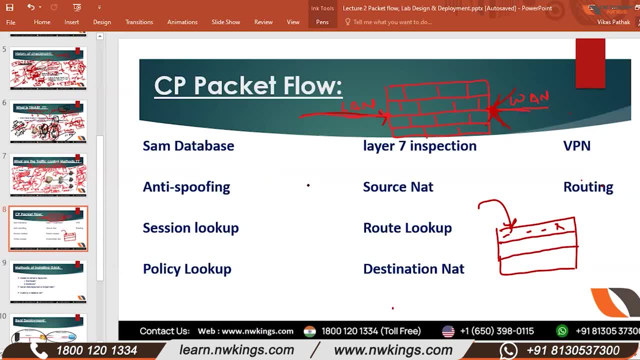 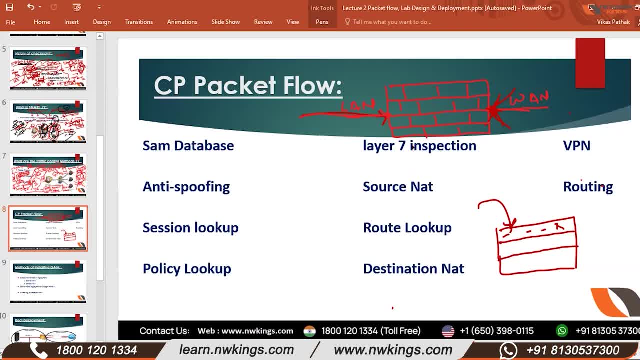 the firewall. yes, see the internal rule, the policy section. there are multiple options. you have to send it to VPN. you have to allow the service. you have to deny it. you have to do logging. you can never match this thing if you have allowed it in the same database. 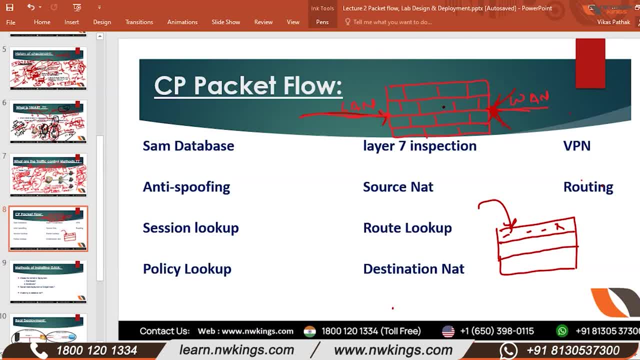 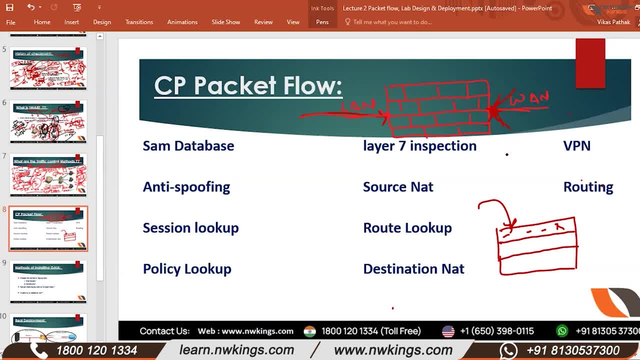 there will be a set of rules which the packet has to pass through. then you will do that policy session, then you will not do the beta, then you will do the policy lookup. it will be the fourth step where you do it, and after that we will do it in a little while. now we 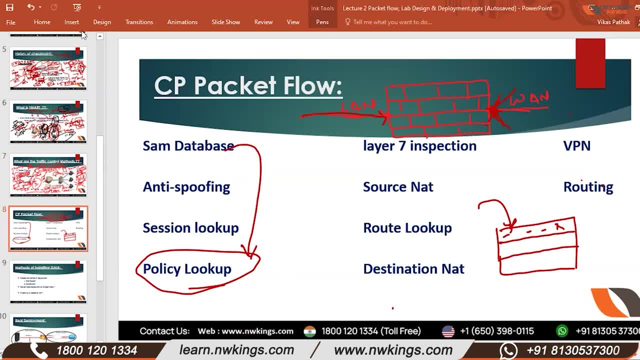 are talking about the same beta base and I have to make sure that this is the same that you did to you, the same that I have done. but everyone has to make sure that that you have done it, then the same thing will happen. I'll do it. I will do it. I say we will not. 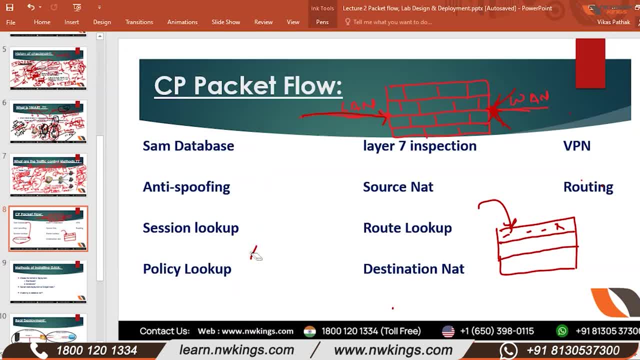 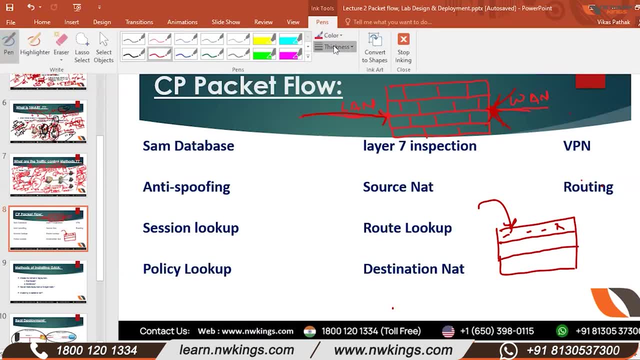 which you were telling that it is a first-level interview. the person has to drop there or go ahead and drop. Yes, yes, exactly. similarly, Brother, leave that too. Leave the first-level interview. Don't call the person for the interview. 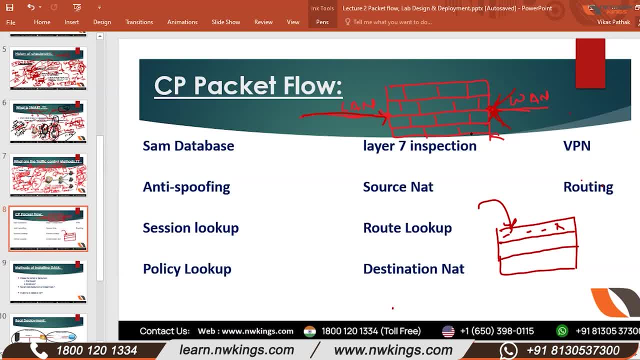 Okay, Drop him. there. You have a resume. You saw that your criteria is that you need an engineering graduate with us, but the person who has come to you has become a graduate and neither does he know the language, which is your requirement. You will have to drop him immediately. 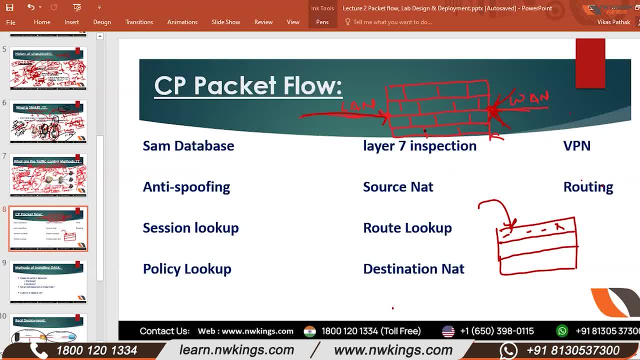 Right. So should I make sure that this SAM database concept is clear to all of you? I want everyone's yes, Yes, yes, yes. When it happens, it will be a little clearer. Okay, I will show you the SAM database in practice. 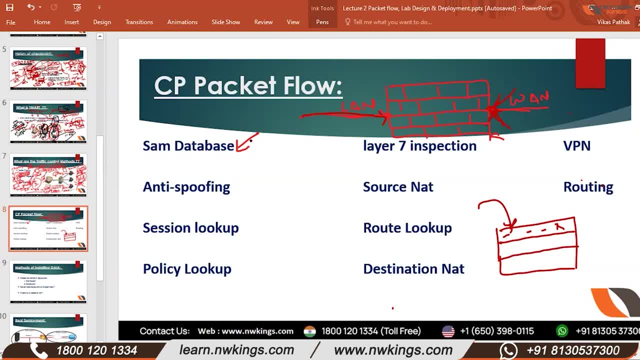 But now what I am telling you theoretically, whether you are able to understand it or not, whether you are able to understand it or not, whether this thing is valid, Yes sir, yes sir, You are able to relate that thing with validity. 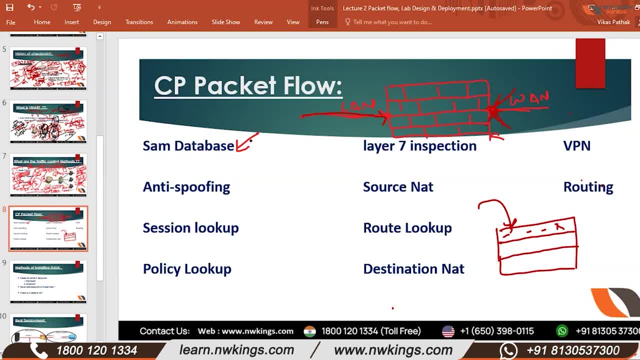 Yes, okay, this concept of SAM database is the first step and why this is being developed: to save time, effort and the utilization of the firewall. You are able to understand this right? Yes, That's all it matters for now. 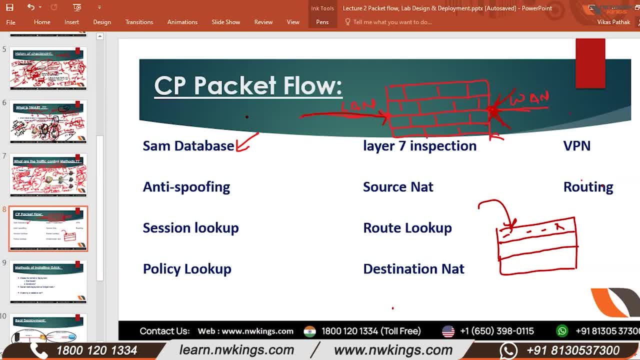 You leave the tension of the rest of the things. Believe me, you will leave the checkpoint certified. Yes sir, Come on, then we will do the SAM database. Traffic came. There is no entry in the SAM database. Second thing: anti-spoofing. 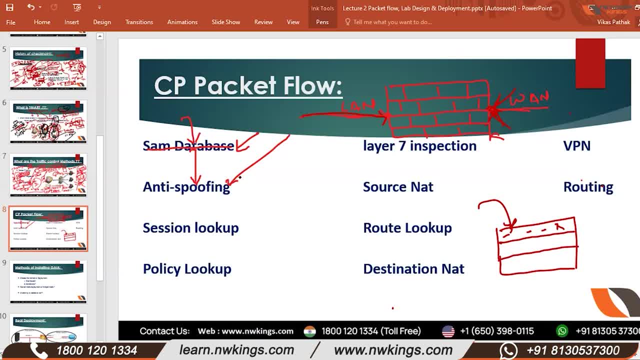 Most, most and next level to most topic which the interviewer will ask you in the concept of L1, even L2 level, What is anti-spoofing? Where do you enable it? Do you understand what I am saying? 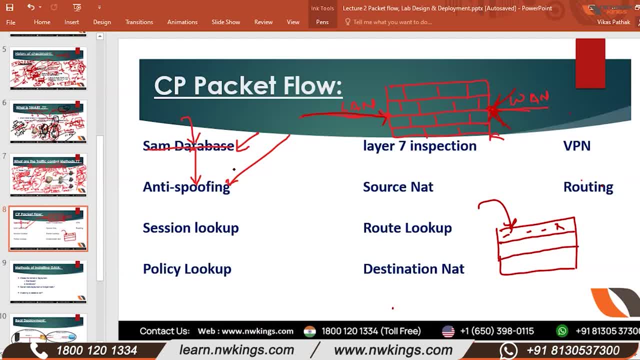 So if we talk about anti-spoofing, then the anti-spoofing feature just checks that the traffic that is coming to me and the source of that traffic, whether it is a legitimate source or not, the source from which the traffic should come. 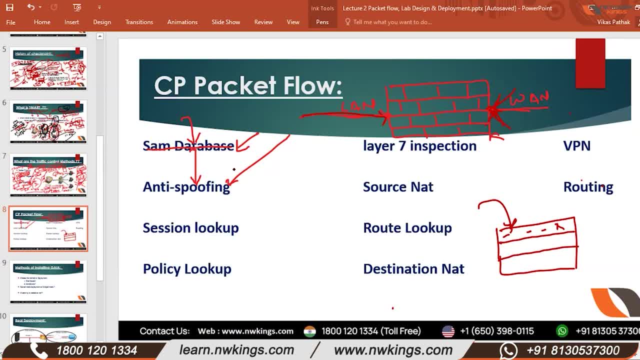 whether it is coming from the same source or not. Are you getting my point? Example: Assume that the traffic that has hit you has happened. You tell me where to hit the traffic: on the LAN interface or on the WAN? Tell me. 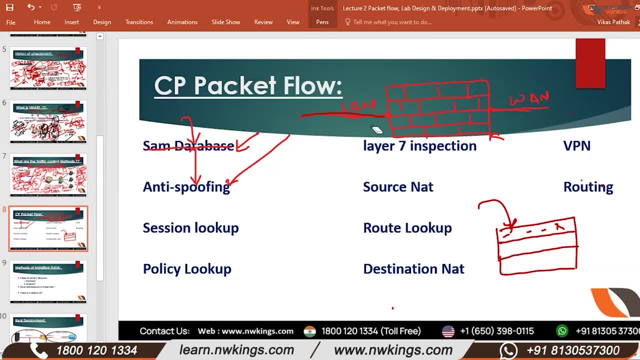 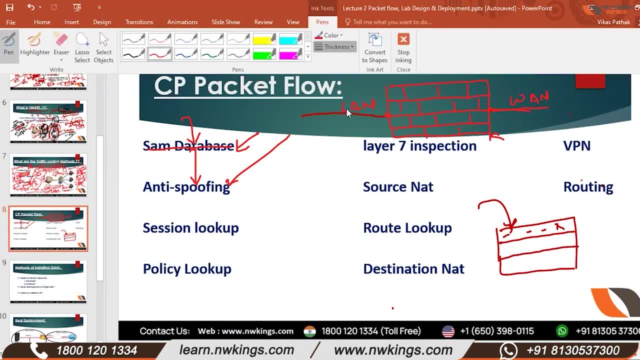 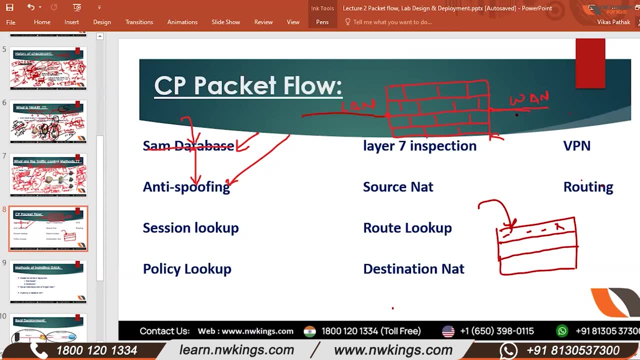 On the WAN, On the WAN, On the WAN. Okay, We do it on the WAN. Here the traffic has been hit. Now what do you think the source IP of the traffic coming from the internet should always be? Tell me It should be from the public IP. 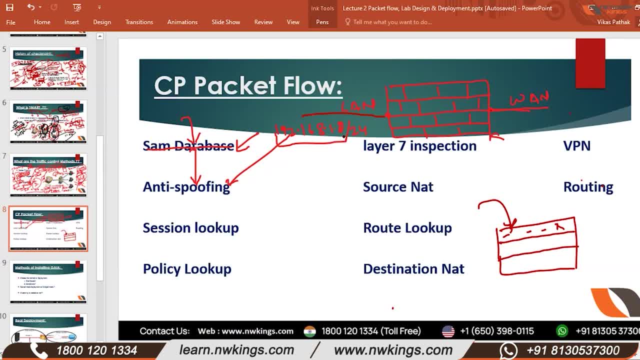 Can it be from 192.168.1.0? No, No. Or can it be from the private range of the 10 series? No, And if there is such a situation that the traffic is hitting this interface and in the packet of the traffic of that interface, 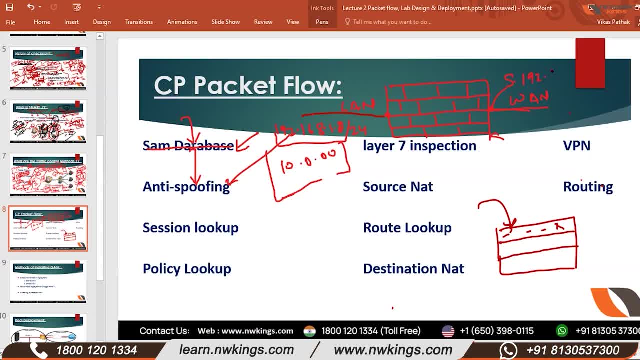 it is mentioned that my source IP is 192.168.1.0.. So what should happen in this case? Go, That's what anti-spoofing does. It makes sure that whatever traffic is being passed through the interface, it's having a legitimate source. 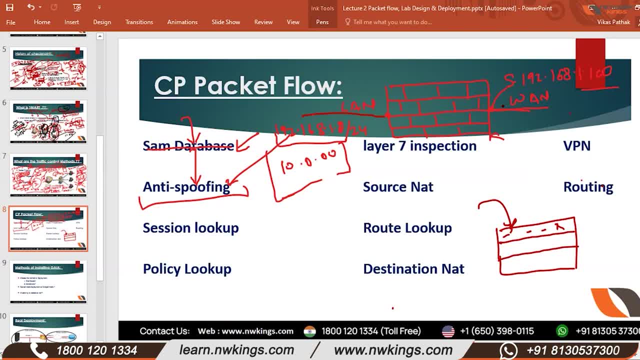 It validates the legitimacy of the source in the packet. Make sense Right And where you have to enable it, most of the cases on the WAN interface, and some of the cases in the LAN as well, From a public IP. suppose there is a public IP in the source. 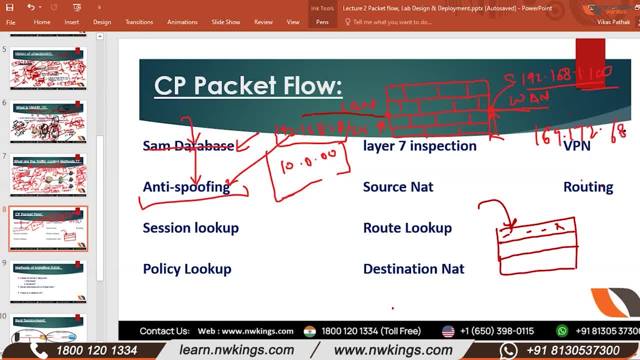 169.172.68.99.. If there is a traffic coming from this IP, this IP in the source and it is hitting the LAN interface, then what does that mean? This traffic should not be allowed And there is someone in between the network who is doing something. 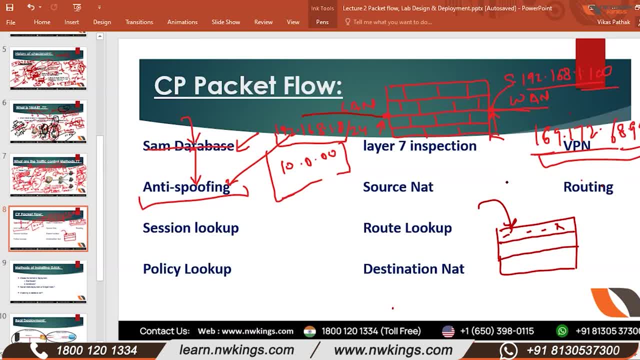 There is a man in the middle. We need to scan the network Right, Right Right. So this is a very debatable topic, A very debatable line, which I have just said. In some cases, do it in the LAN. 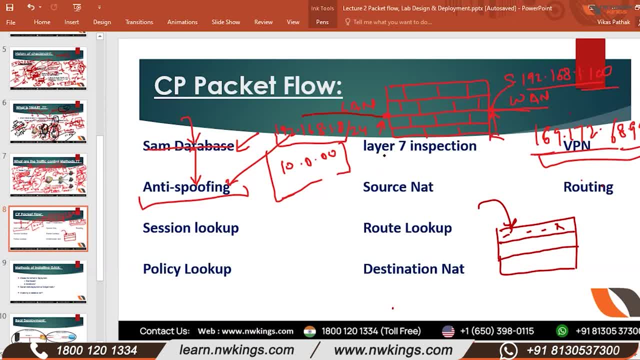 But why should I do it in the LAN Right Now? what happens many times is that when there are more experienced people than me, they cross-question me many times And I answer them in the same way that when I have to do monitoring. 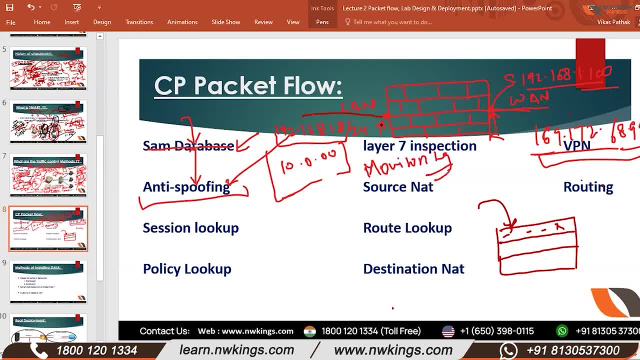 what do I have to do? Monitoring? When I have to do monitoring, then I will do it in the LAN interface, And when I have to take an action, then I will do it in the WAN interface. Now we say okay. 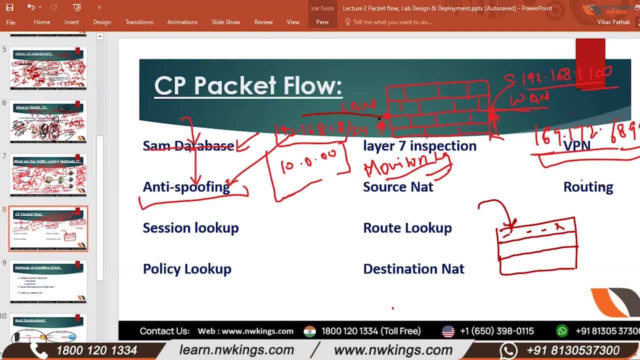 monitoring should be done. If I have to do monitoring on my firewall, then why have we spent money in the other tools? If I have to give all the burden to my firewall, then I will do it in the LAN interface. Yes, you can do that on the LAN interface as well. 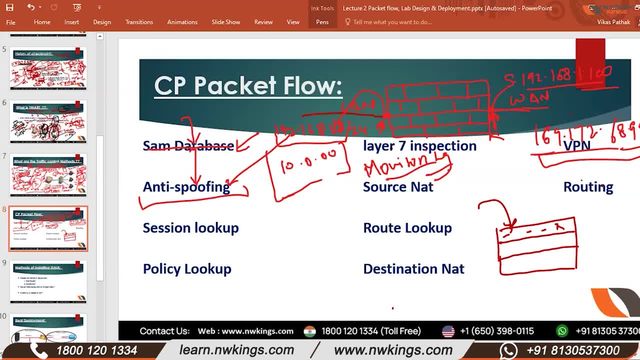 But you should not do that. Why are you increasing the load of the firewall? The scenario is that suppose you don't have a SIM, you don't have scanning tools, then in that case you can go for it, But it will only guide you. 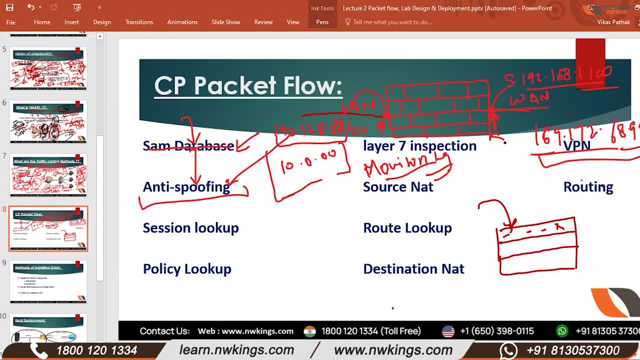 It will only inform you that the traffic is coming on the LAN interface with the WAN IP. It means there is something wrong with the network. There is someone in the network who is initiating the traffic with the public IP. But action drop will also happen by default. 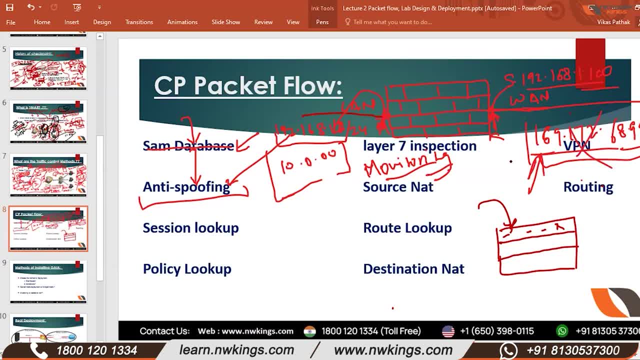 Yes, it will also be dropped. This traffic will be dropped by default. Yes, in the anti-spoofing section, But when you apply this anti-spoofing concept on the WAN interface, it will make more sense in the real scenario. 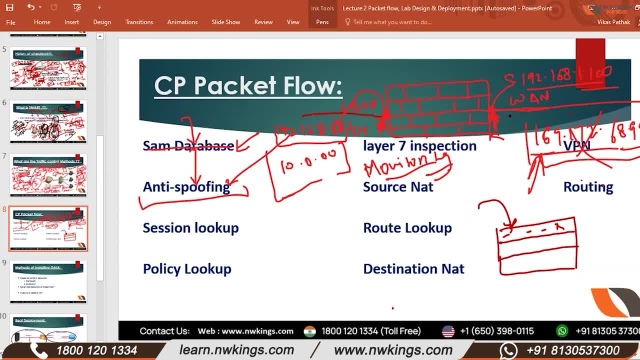 Clear Yes In this. if you are hitting on the LAN interface, then there should be a LAN network. If there is a public IP on the LAN interface, then it is anti-spoofing. If there is a private IP on the WAN. 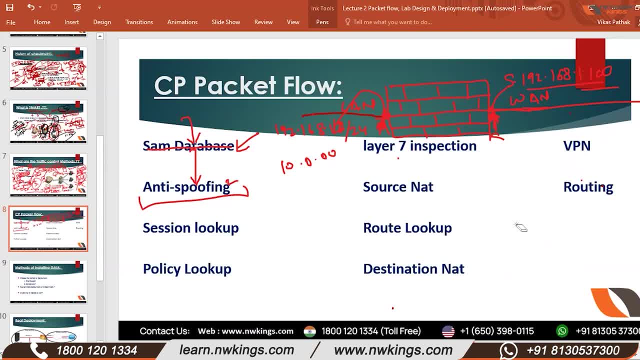 then it is anti-spoofing. It is not anti-spoofing. It is not anti-spoofing. When it is blocked, then it will be blocked in anti-spoofing. Okay, okay, right, right. 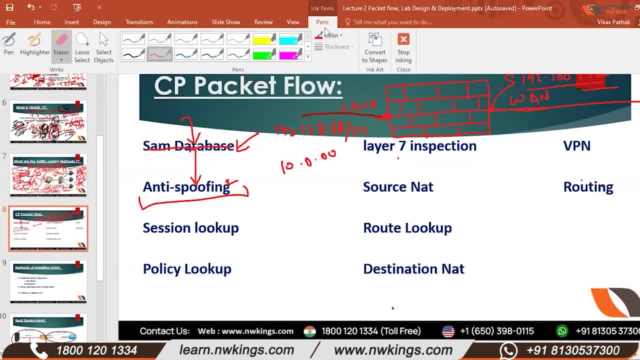 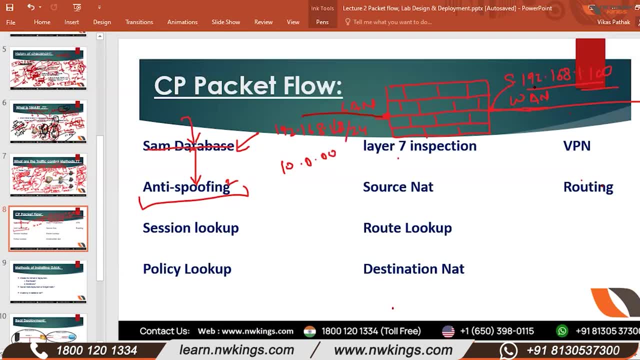 Do you understand When this situation will occur? that situation, one minute. suppose the traffic hits here from the range of 190 to 160 private IP, then when it will be blocked on the interface, it will be blocked in anti-spoofing. 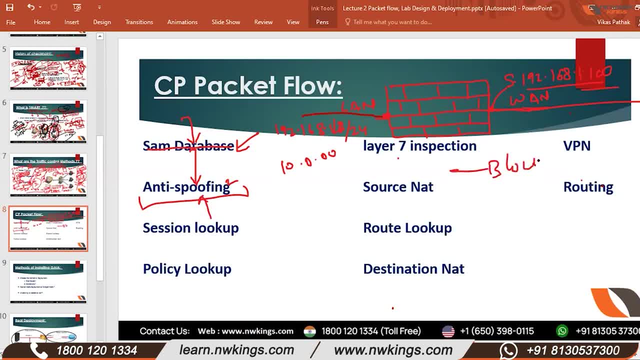 and it will also show you a firewall lock that blocked in anti-spoofing. Okay, right, So you can go and say that the traffic that is coming is not a legitimate source. You tell me the source. What is your source? 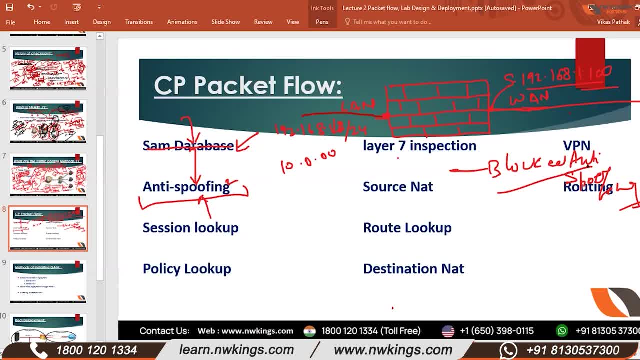 It will tell you 190 to 160.. Tell me how are you traveling on the network? Right, right, Getting my point. So the first thing was that SAM database. we will decide whether the traffic which is coming to the firewall 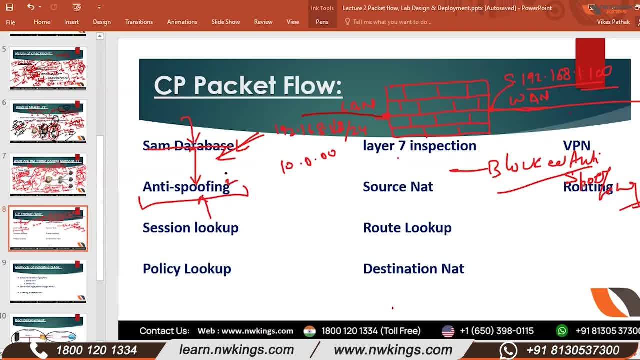 that traffic is required. The traffic is required or not, Whether is there any entry in the SAM database or not. If no entry is there, it will be passed to anti-spoofing, and anti-spoofing make sure that, whether this source is legitimate source or not. 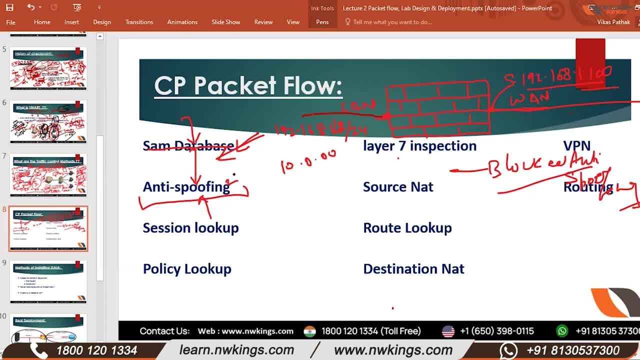 Is the story clear? Hello, sir, Yes, Yes, please go on, Sir. I wanted to ask about the SAM database. This feature is available in firewall, only in checkpoint. Only in checkpoint, Okay, okay, Because we get this kind of request. 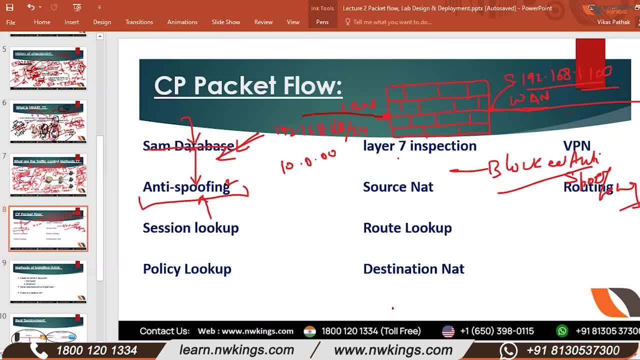 in call on, Because numerous connections were coming and buffer overflow protection was there. The firewall was down. After that the switch was restarted. Then the locks were stopped. sir, We did not block any traffic on the interface, But I don't know. 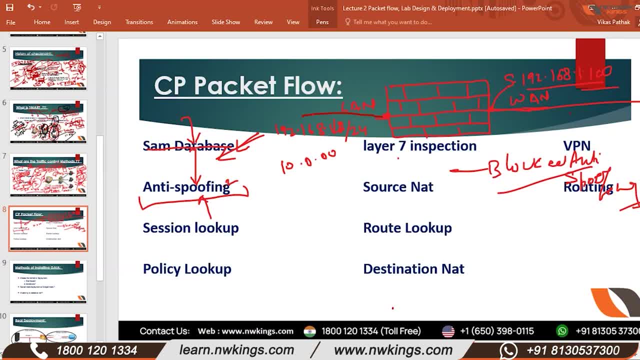 they said that the switch was restarted and buffer overflow protection was there. It was resolved. The locks were stopped. Many locks were coming Unnecessary. It was resolved. So this feature is only available in checkpoint SAM database. yeah, Okay. 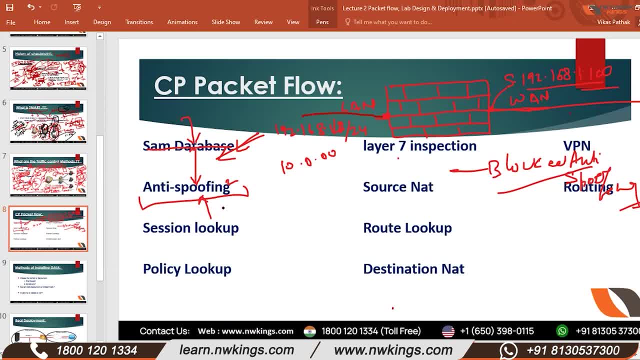 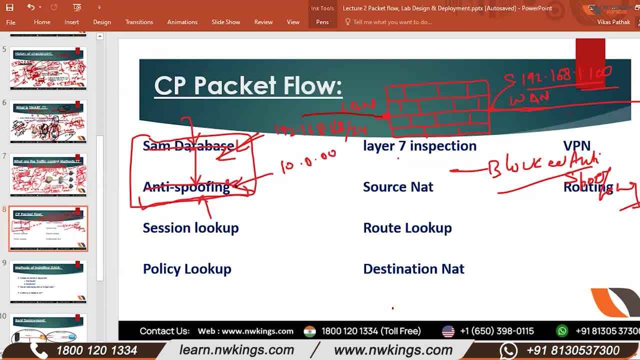 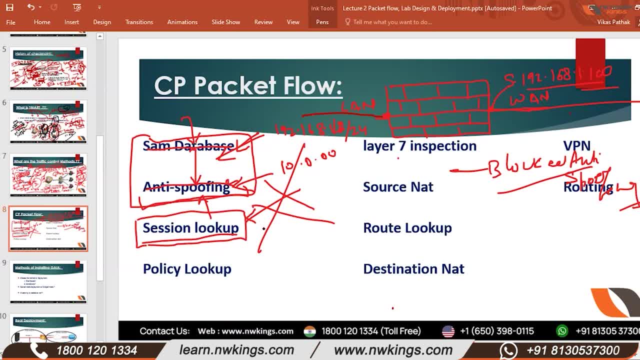 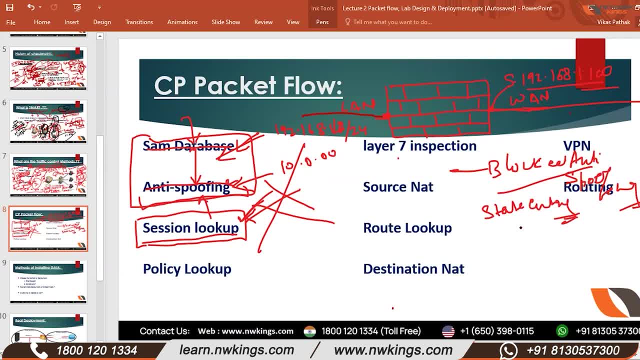 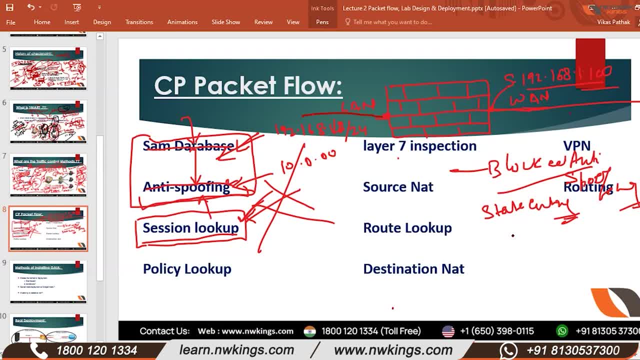 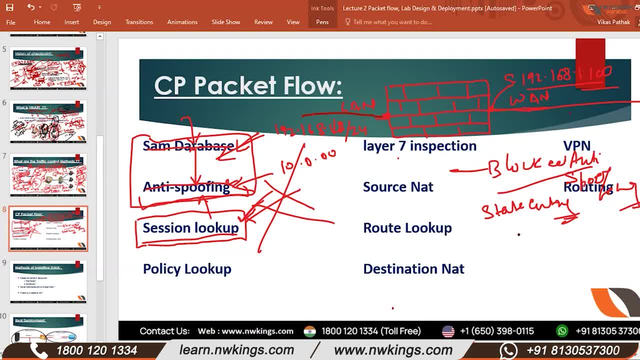 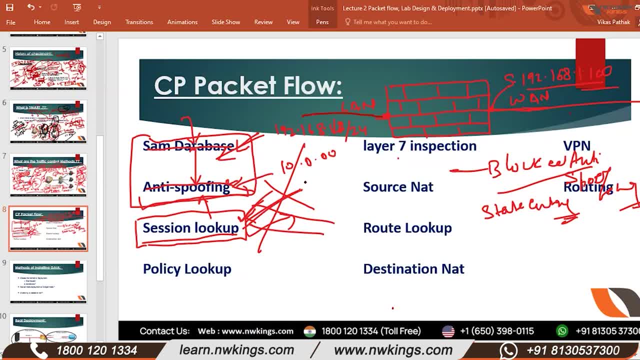 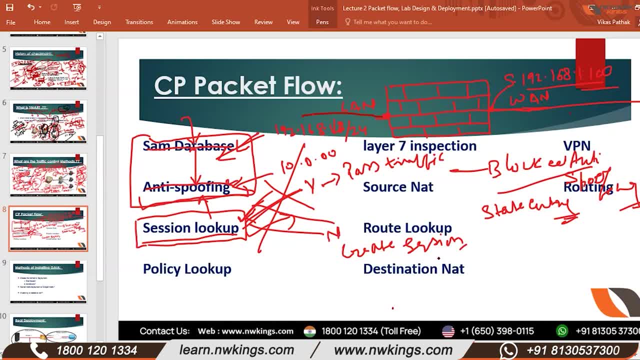 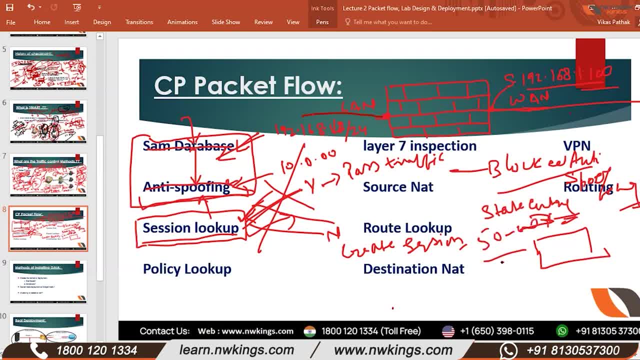 Okay, Okay, traffic connection bypass, so the connection table will be maintained. then that firewall will be slow. Sir, it is not like after some number of session the old session will be deleted. No, that is a timer within a timer, if traffic did not come. 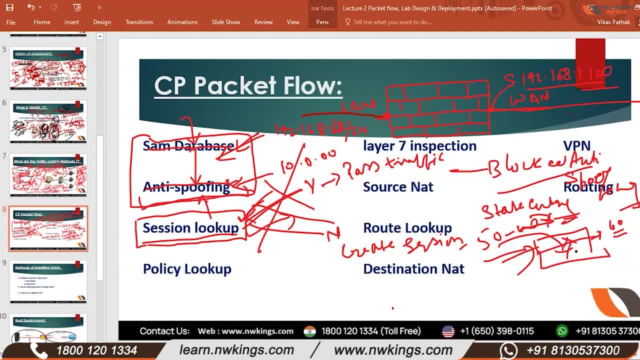 then that entry will be deleted. such an overflow entry will not be deleted. ok, sir, this possibility is: let's say you have 10 logs and suppose you have to enter one more. then check the first one. how much is it? it will be 60 seconds. flush it. 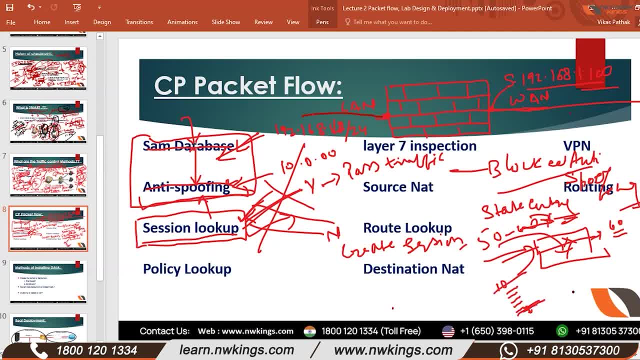 then it will come up and the lower one will be flush. this is how the timer works. then, if someone has to come, then the lower block will be removed and it will be flushed. but timer plays a crucial role, isn't it, ok, sir? thank you, any other question? 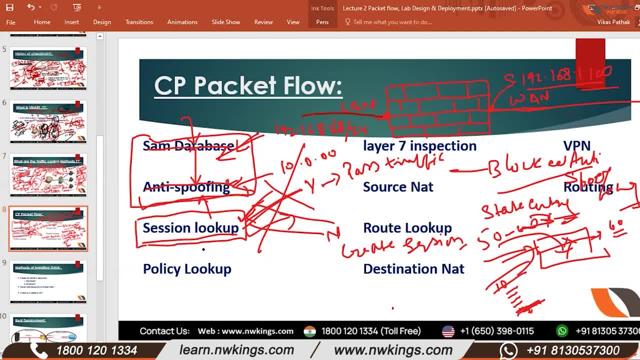 shall we move forward? yes, sir, yes sir, after the session lookup, the policy lookup will be happening. what did you say that you did? session lookup, it is a session. say yes, pass the traffic. when will the session be made? when the policy remains? ok, if it is a session. 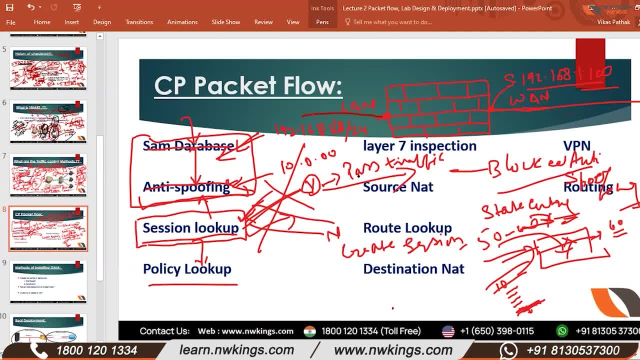 that means the policy is also existing. pass the traffic on the basis of session. if it is not create a session, how will the session be created? on the basis of policy. that policy is allowing or not allow and deny, ok or no. policy means drop, so the session lookup. 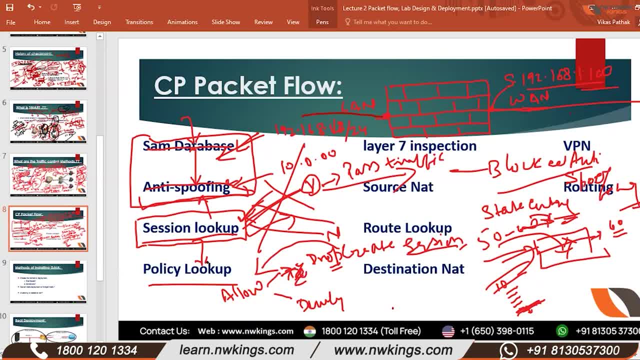 if it isn't, that means the session is not created. it could be 2 reasons: either there is policy and traffic is not initiated, or or the policy is not the traffic initiated and it is dropped. so, ok, cool, now tell me any doubt. our policy on lookup is best. 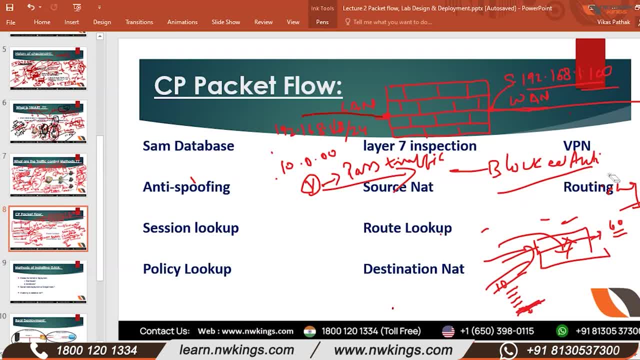 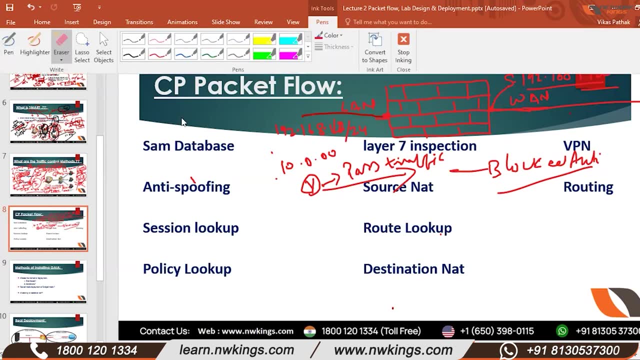 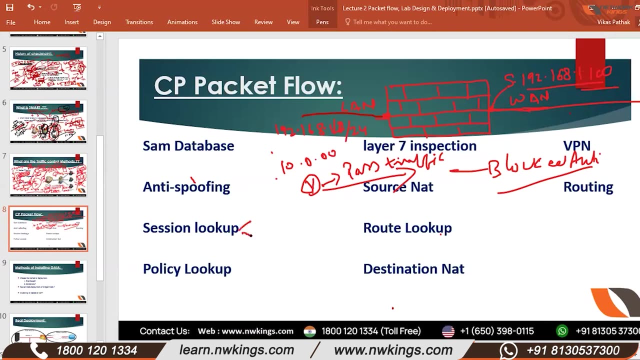 if our policy is good, then session will work right. no, no, after session lookup, result policy will be lookup. ok, both statements are little different, very basic. if you understand, then it will be better. the output of session lookup: yes and no. yes means session is made. when session will be made. 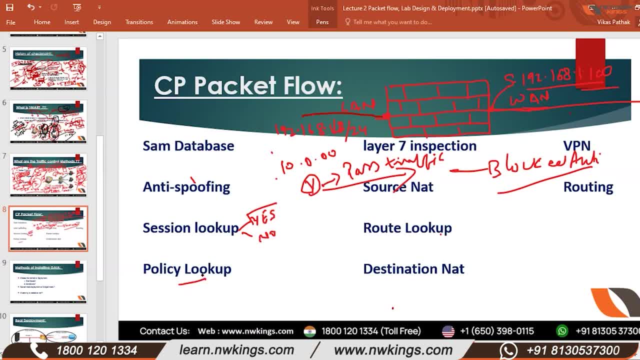 when policy will be made. if there is no policy, then traffic will be dropped and session will not be made, right sir? and if there is no policy, then create session. how will you create session? through policy? so check if there is policy or not. again, yes and no. 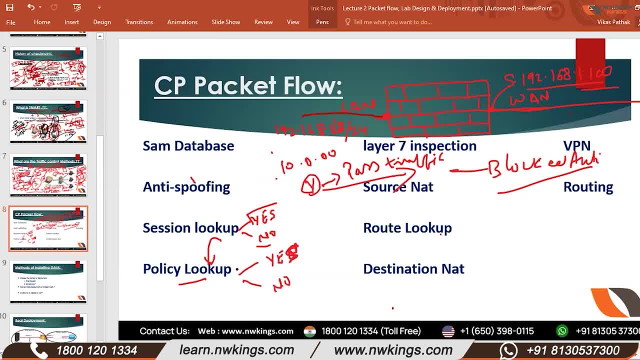 policy is there or not? yes, and no policy is there or not? yes, is there, then check what is the action. is it allow or deny? if it is allow, then create a session and send it to further. if it is deny, then drop it, and if there is no policy, 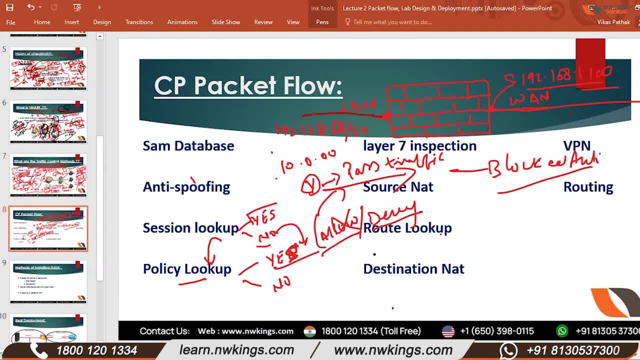 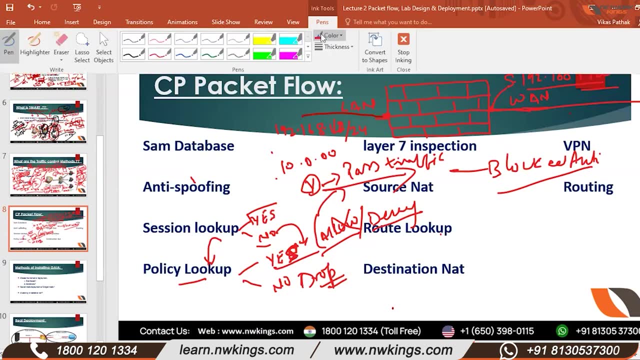 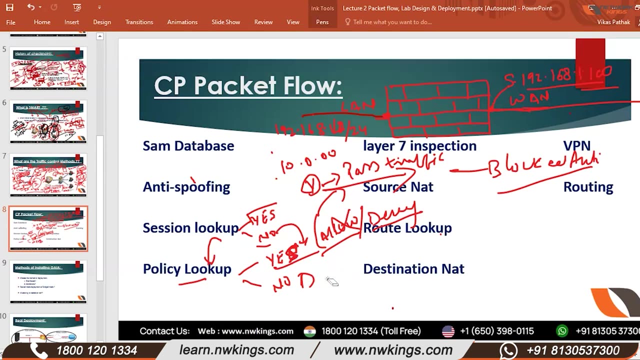 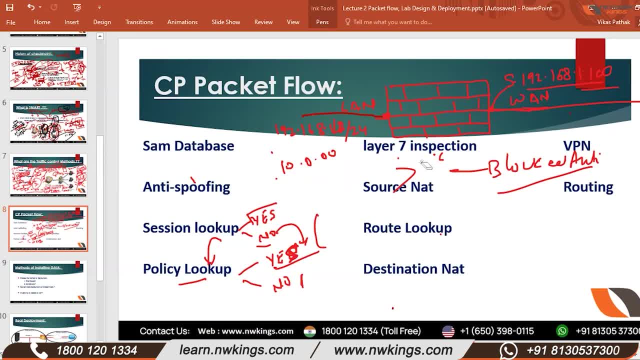 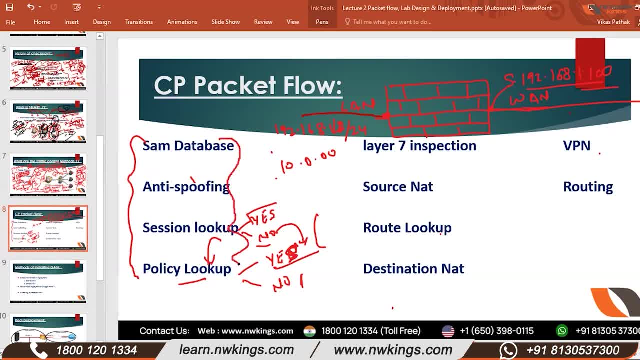 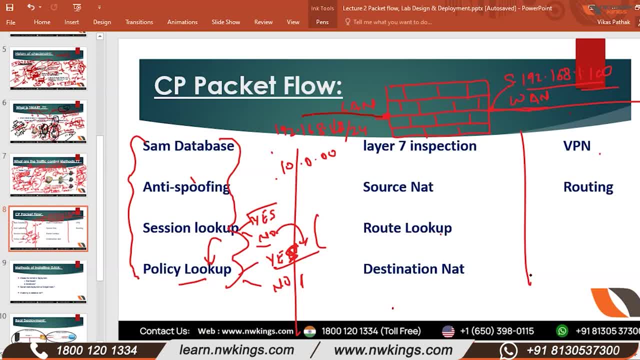 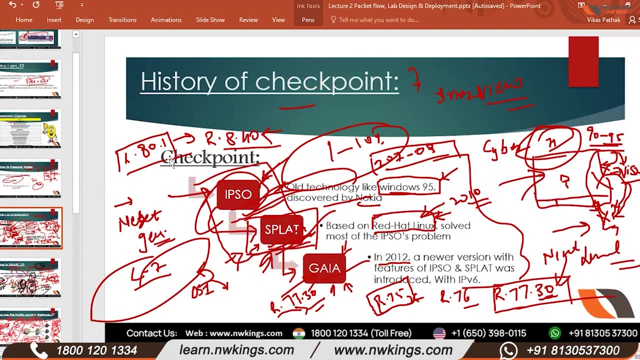 Shall we complete this section, Affirm Done, Okay, perfect. Then we are moving ahead And I was just asking like: do you have any any issues while we have discussed? you know history of checkpoints Or do you have any issues? 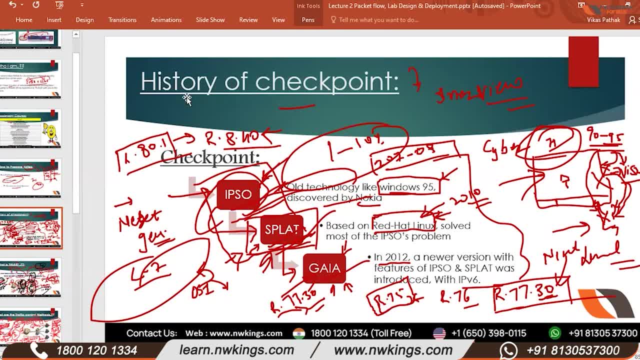 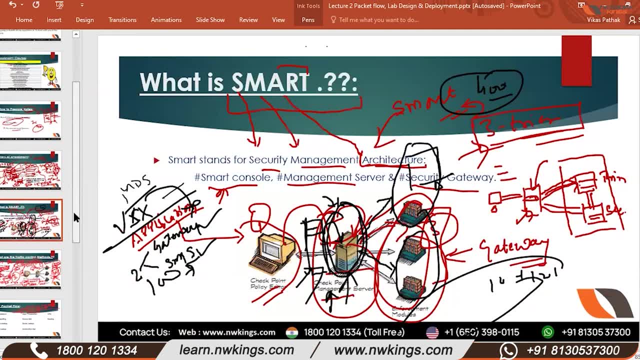 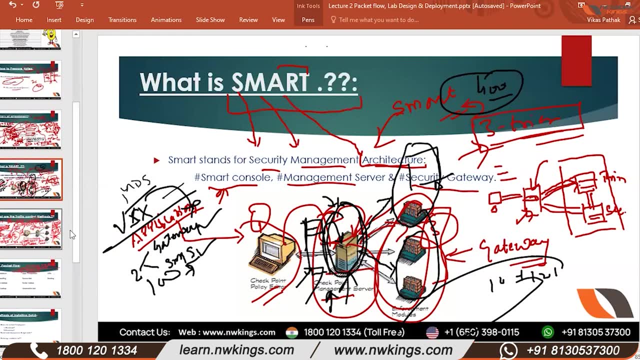 Any issues while we have discussed. you know history of checkpoints Or do you have any doubt in this section? No, no, History in history. I don't have any doubt. Okay, Smart architecture we have discussed. I think this should also be clear. 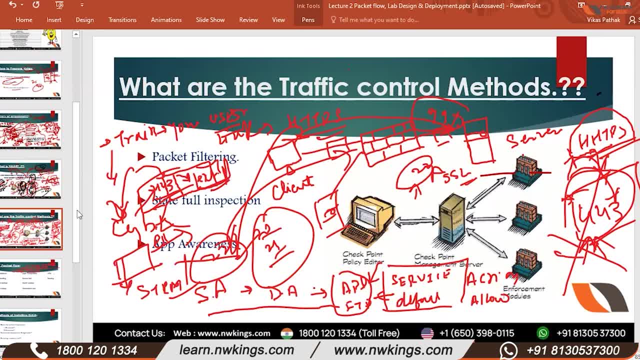 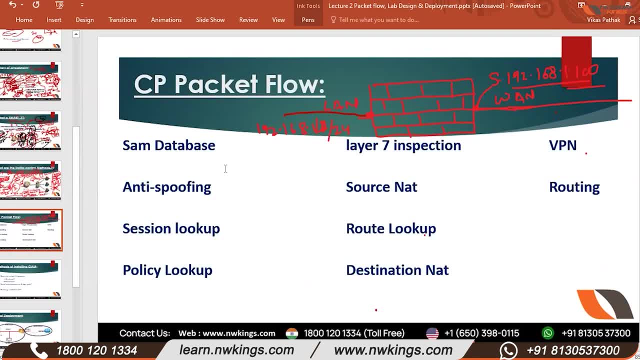 Traffic control methods. I think this should also be clear to you. We have spent a lot of time on this. If there is anyone, you have to tell me. After that, we have done the packet checkpoints. We had a discussion a little while ago, right? 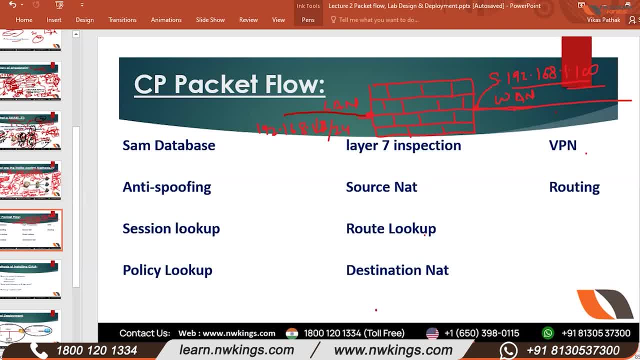 So today we will quickly revise the left section a little bit And so that you remember it right. So the first step was that the traffic hits the firewall. So the first step will be the SAM database. And what is the SAM database? 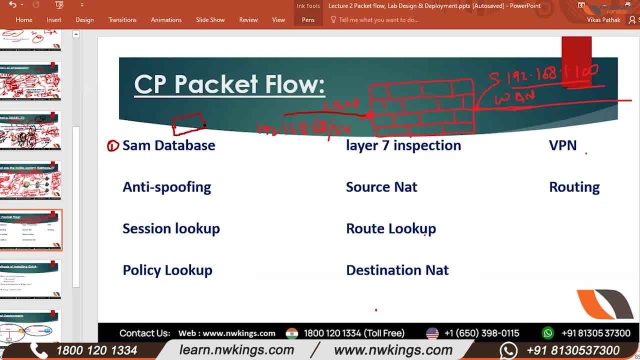 It is a database that works at the interface level of the firewall And it is a database that works at the interface level of the firewall. So what happens in that is that we can make a rule of allow or deny And if the traffic that is hitting the interface level matches with the SAM database. 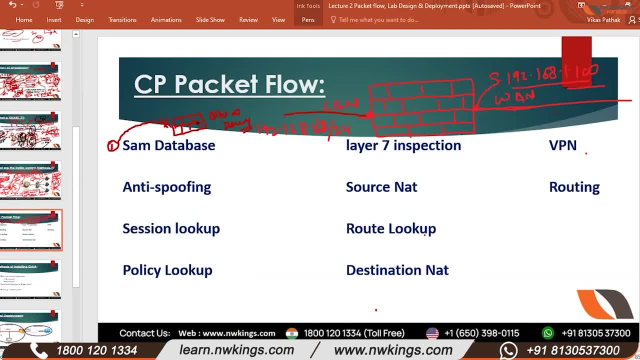 then that action will be performed at the interface level. That traffic will not go to your firewall. It will be processed. Is it clear? The second thing that happens to us is anti-spoofing. What is anti-spoofing? 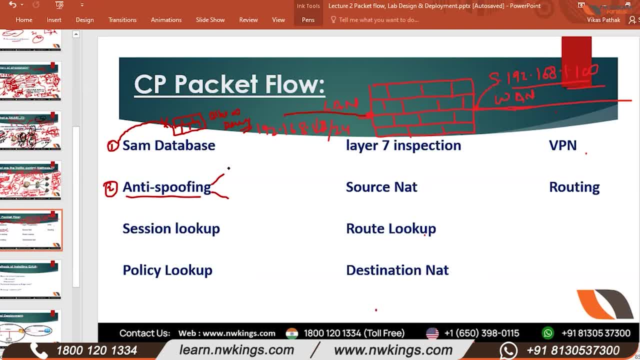 It is responsible to make sure that the source address which you are getting on the firewall is legitimate or not. It should not be that there is traffic coming from a public IP on LAN interface or there is a hit from a LAN IP on the WAN interface. 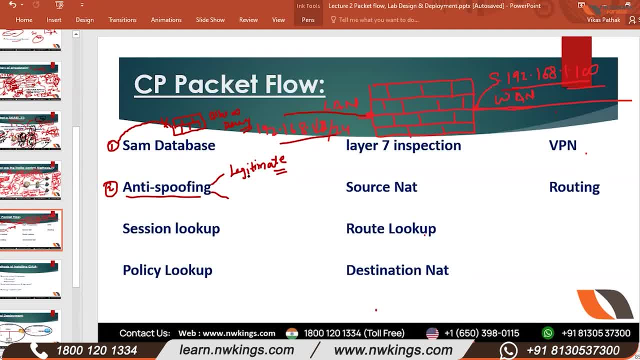 There should not be any such scenario. Anti-spoofing works a lot to check legitimacy And we can enable anti-spoofing on the interfaces. I will show you while we will do the lab. So when we will do the configuration on the interface, there is an option of anti-spoofing. 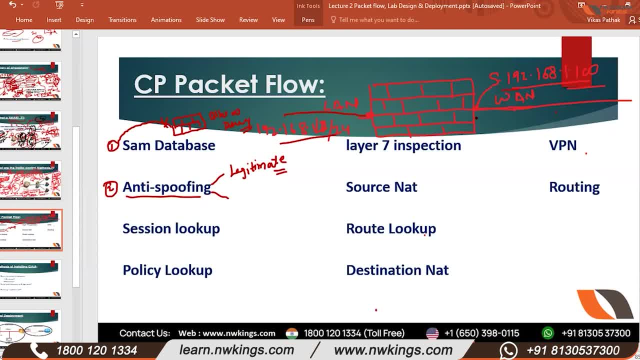 We can enable anti-spoofing on LAN and WAN, But I recommend you to do anti-spoofing on WAN always, And if you need monitoring on your organization, then you can do anti-spoofing on LAN After that. the third step is the session lookup. 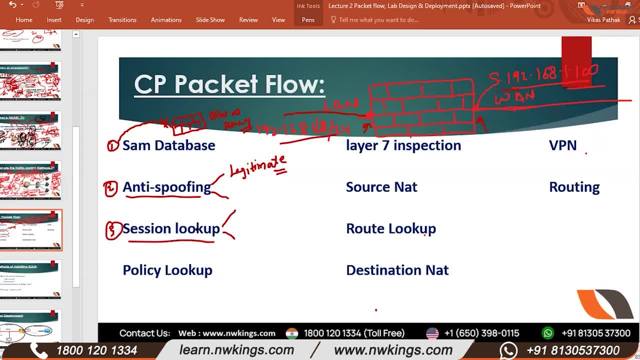 The traffic that has been hit on the interface of the firewall, whether there is an existing session for it or not, Either yes or no. If there is, then that traffic should be passed through that session. If not, then create a session. 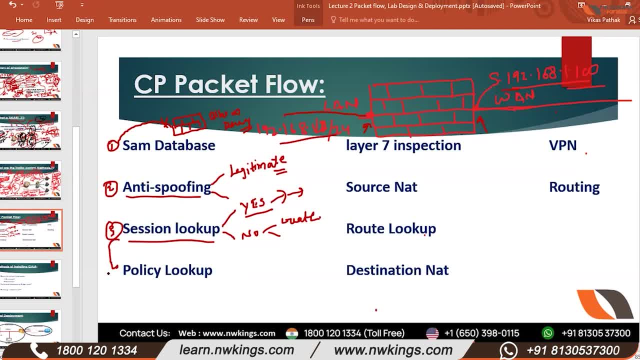 And to create a session. the first policy should be matched. Now check if there is a policy or not. If there is no policy, then drop it in the cleanup rule. If there is a policy, then match the policy and pass the traffic and create a session. 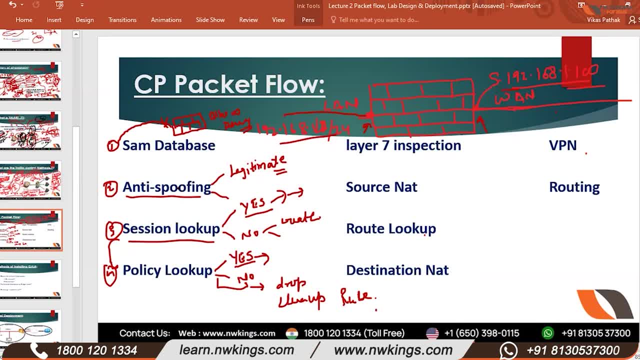 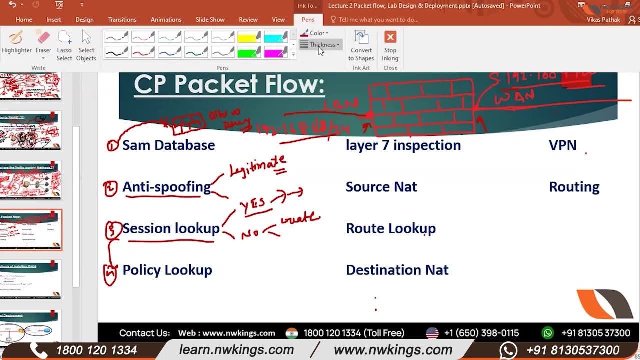 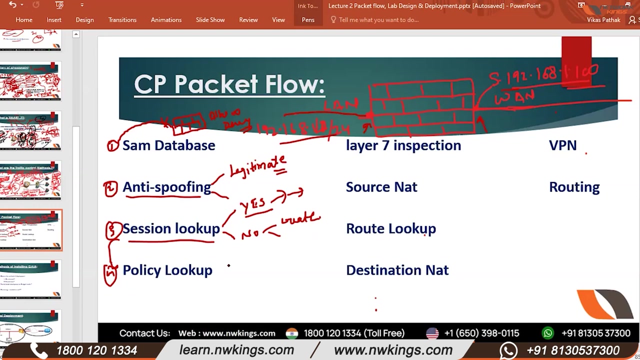 So this is our left side section. It is completely finished. Now, what happens That the ad p o r o n z n e a r 2, 6, 7, 0 E A T layer three, layer four, layer three firewall is a layer three device and uh, but it have the. 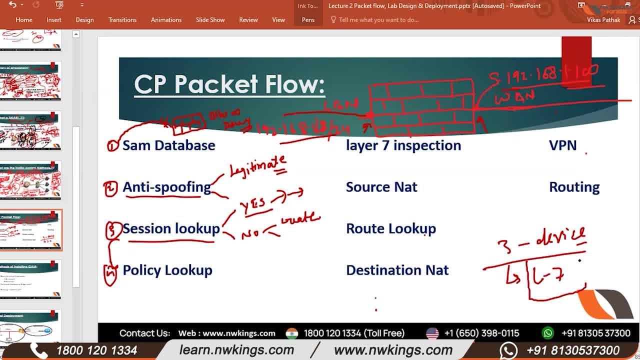 capability to work on layer seven as l7 devices enabled because they are doing ssl inspection. okay, because they are doing ssl offloading. now, where does ssl work on layer seven? yes, that's why we call it layer seven for l7 layer next generation firewalls. okay, now l3, which is, and l4. 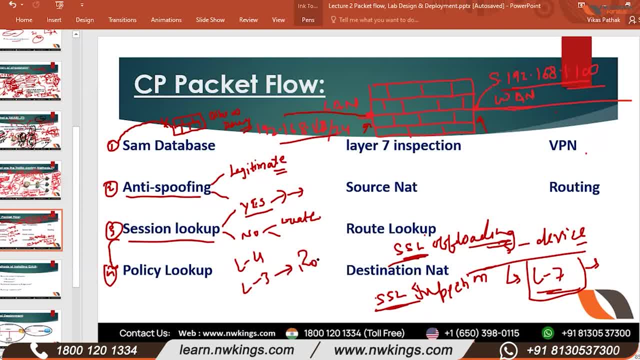 path is defined on l3. okay, through which protocol? this? this traffic should follow this path, whether tcp or udp make sense. so routing capability already have firewall, yes, and up yes, so that is why it is called application layer firewall. so so basically we can say that the 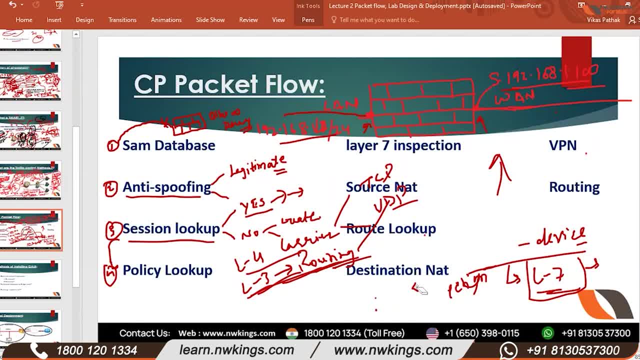 firewall works only layer three, layer four and layer seven. it has capability to work on layer three, layer four and layer seven. you are taking it in a wrong direction. you cannot say that it only works. you can say that it works as well on layer seven. okay, firewall is a l3 device, but it 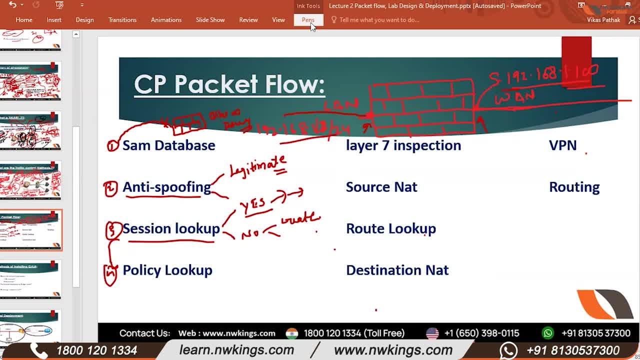 the next generation firewalls are working. make sense that policy look up after yes and no one. in policy and destination. we have policy and in policy we have configured the windows allow, ok, and after that check will be there. rss and thats all. check destination: ip is there. 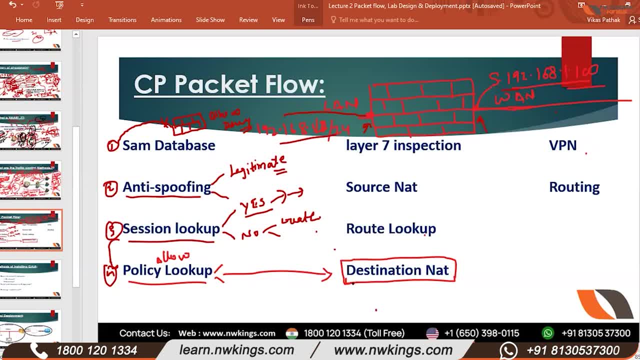 net configured. ok. now, if you understand this line, then a question arise. when you keep public ip in destination or private, so because in the packet flow destination net comes after the policy lookup. so that is why we will keep public ip in the policy. clear. this question is: 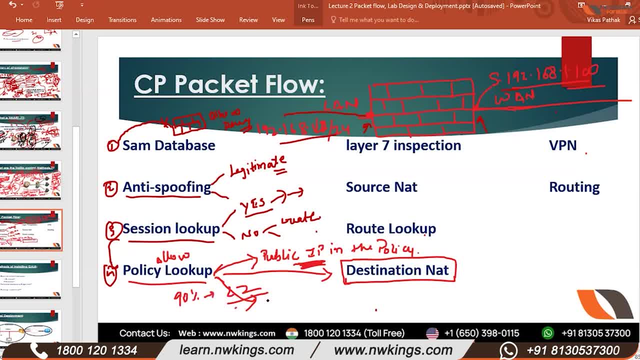 90% till L2 in L2 level interview in 90%. the question is the policy you have made from private ip or public ip. so in check point scenario destination comes after policy lookup. so that is the rule for public ip. debatable question but 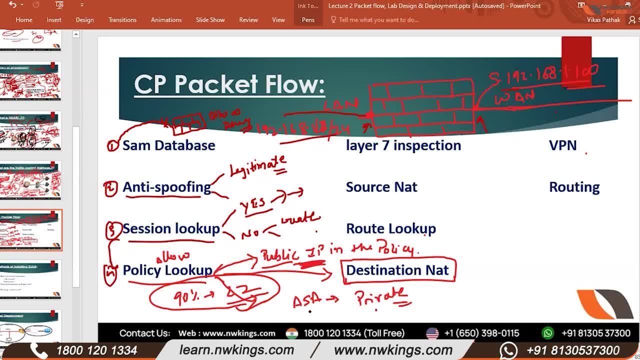 i think cisco has a limited information. but i think cisco is not debatable. but you have to make sure the policy lookup comes before destination net. that is, if you make policy on it, will you make it through public ip or private ip? sir, we make private ip on all. 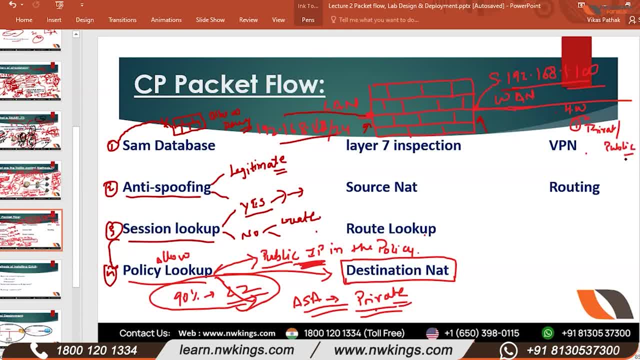 whether it is palo alto or forti gate or asco, i don't know about srx, but in forti gate and palo alto destination net comes first. so here is a little difference. ok, so when policy lookup comes first, that means you have to create the 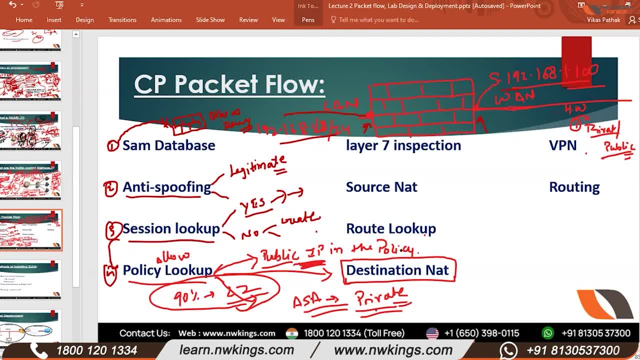 policy on the public ip. is it clear? alright, now destination net is done. after destination net we will check route lookup. what is route lookup based on this destination? do we have any route to route this packet lookup is there? lookup is done on post netted ip or pre netted ip. 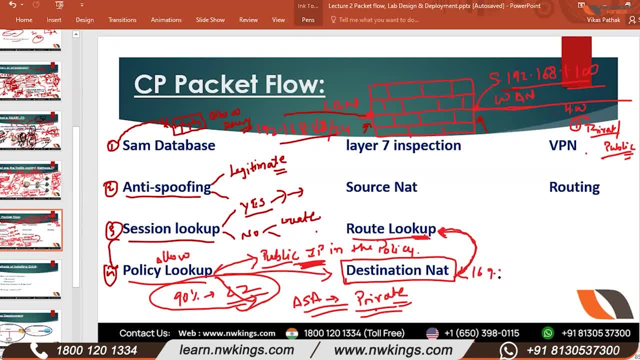 post netted ip. ok, you have public ip 169 from 16.20.1 to 10.1.1. so for this netting you have to check where to send this packet. suppose this is your firewall. this is land, this is van, this is dmg. 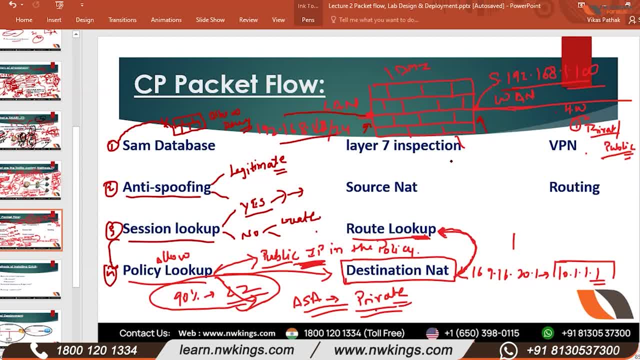 this is dmg. this is global dmg. this is global dmg. this is internal dmg. this is internal dmg. now, as soon as it hit here, after everything is done, it is checking how to send this packet towards global, towards internal or towards land. this is route lookup. so 4: this is 5. 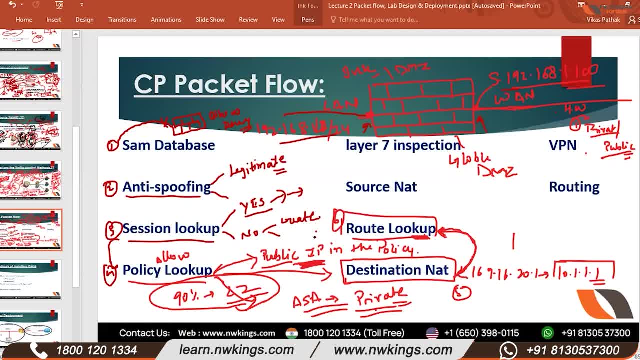 this is 6. ok, ok, after that this is lookup after lookup. there is no routing, only lookup after lookup. 7th step will be source net. the traffic that has come in, that traffic for source ip do i have to net if source net is also configured? 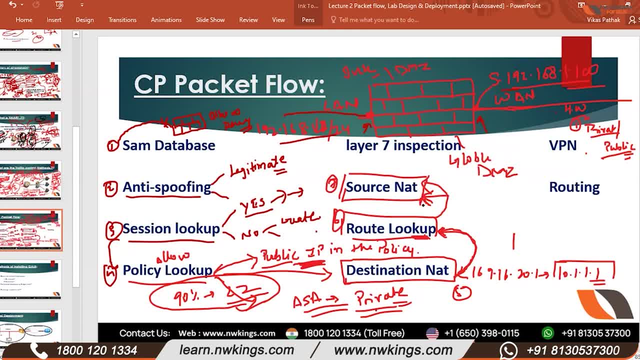 then source net will be configured. sorry, conversion will be done here, ok, ok, after that 8th step comes. source net is done here. after that it will go to l7 inspection. do we have any l7 profile, l7 profile or or rule configured, rule configured. 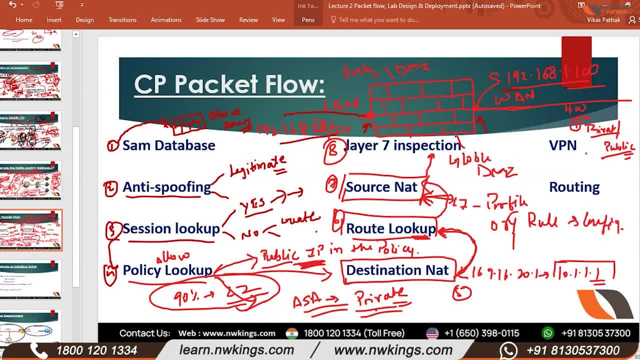 if any l7 profile or rule you have done on firewall, then it will hit here, if not, then it will move forward. now what happened that as soon as after this l7 inspection, next step comes, 9th, that is, vpn firewall will determine that this destination net. 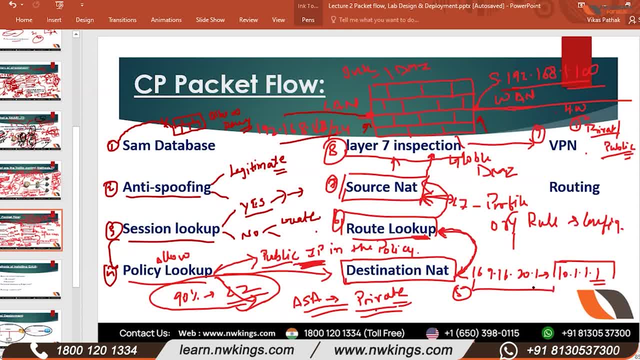 or not. whatever ip i have in my destination right now, is it possible that i have to send that traffic to vpn and again the decision will make here yes or no. if it is yes, then it will be sent for routing, that it will be routed to vpn. 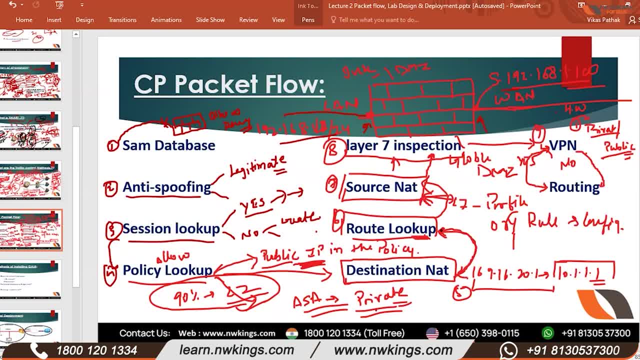 if it is no, then it will be normal routing. whatever routing capacity will be sent to it. the packet will be routed at this step. the confusion is that the packet is sent here. we have not sent the packet here, we have just looked up. ok, we have actually routed the packet. 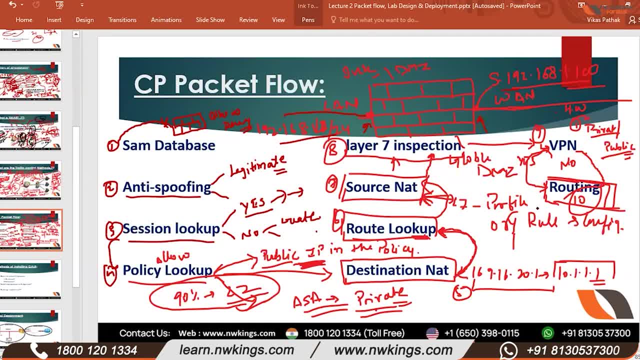 at this 10th step, at this 10th step, at this 10th step. after this, the packet will be routed to our vn interface or lan interface or whatever interface we have to route it. the packet will be routed to our vn interface or lan interface. 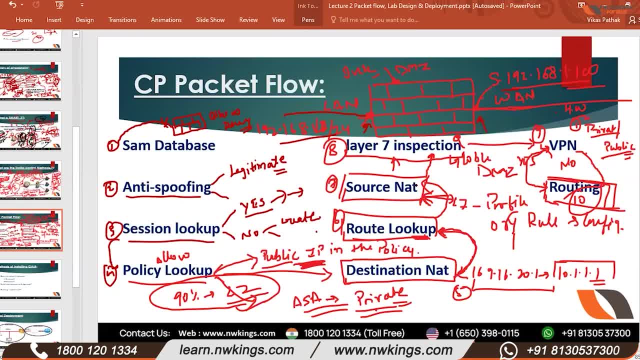 or whatever interface we have to route it. now. this packet flow is completed and i hope you must remember these tips if you are going to interview l1 or l2, no one will ask you in l3. sir, i have a small doubt. where is the ssl decryption? 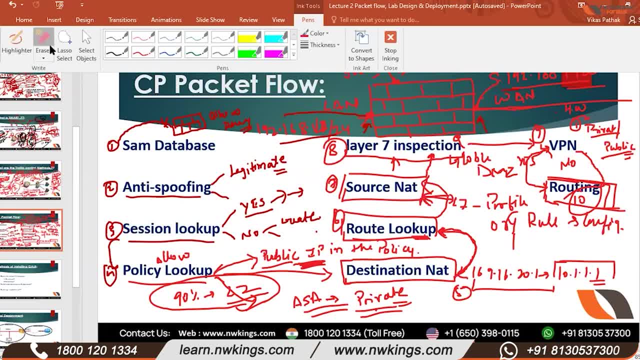 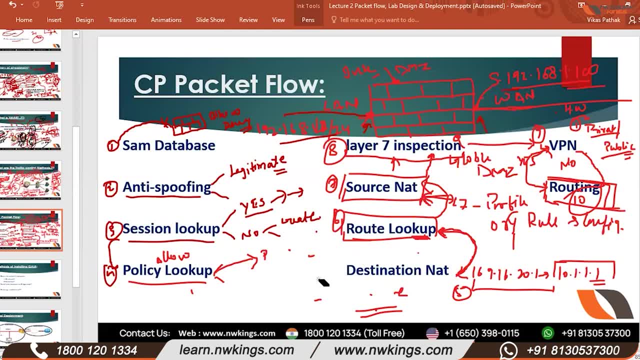 that? wait. before that, tell me one thing: what are you doing in ssl decryption? hmm, let's suppose i am doing inbound inspection. ok, so in actual ssl decryption, what do you do from this term? what do you do with ssl decryption? what do you perform in it, what activity it has? 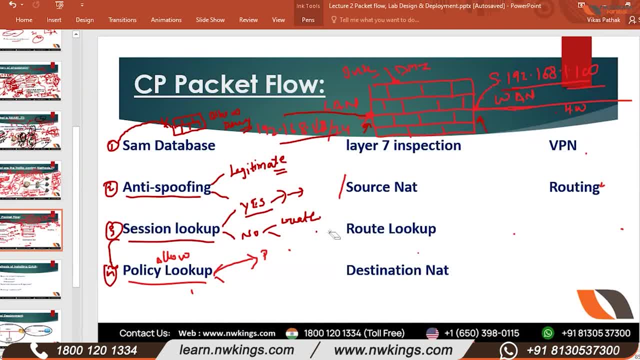 logically, Sir, there are two things, as far as I have read it, for decryption, there are two things in it. one is forward proxy and the other is inbound inspection, That is, the traffic coming in from outside. I am decrypting it, I am reading it and then I am sending it inside. 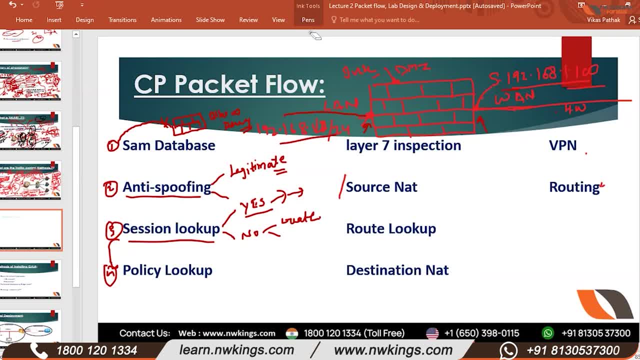 So in that case what I am able to do is layer 7 inspection Forward proxy is that when the traffic is going out from inside, then my firewall will behave like a man in the middle And it will be like a server for my client and it is like client for the server. So it will make two SSL handshakes. 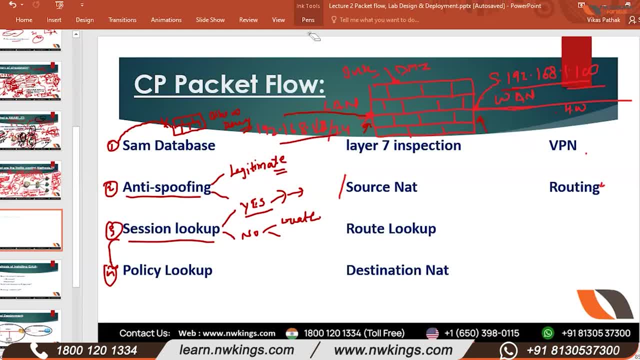 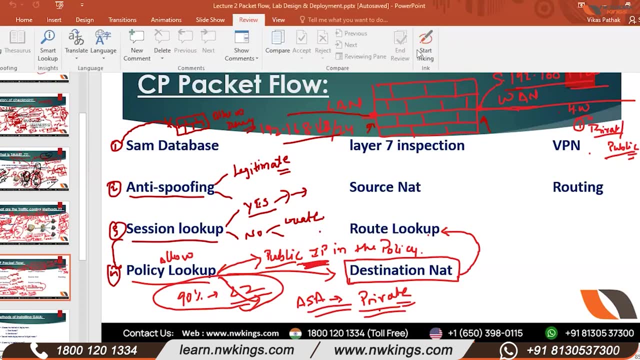 For the user who originated the service, it will behave like a server. He will feel that, though, I am communicating with the real server, but actually the server itself will be a firewall. Okay, okay, you have done a little mix and match, but no problem, I will clear it for you. 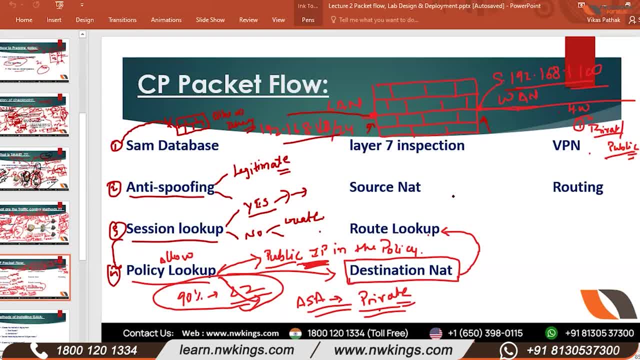 Look, this is my PCM. Okay, we will do a very brief discussion, not a long one, because SSL is a very long topic, But I am telling you briefly. A traffic was generated from this browser here for the destination. This is my firewall in the middle of the destination. 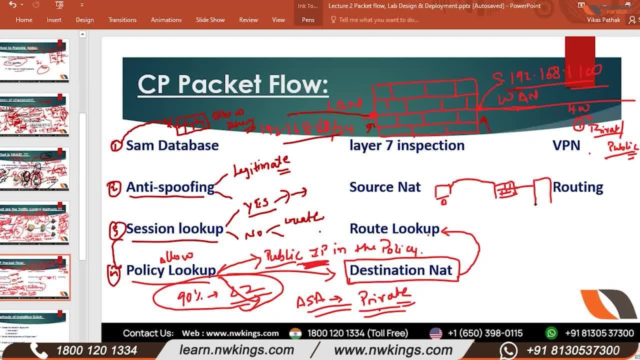 And this is my server. Okay now, why did we do SSL offloading? So that we can offload the work of this server a little bit Now, either the option is that we checked the source and destination of the traffic sent by the client. 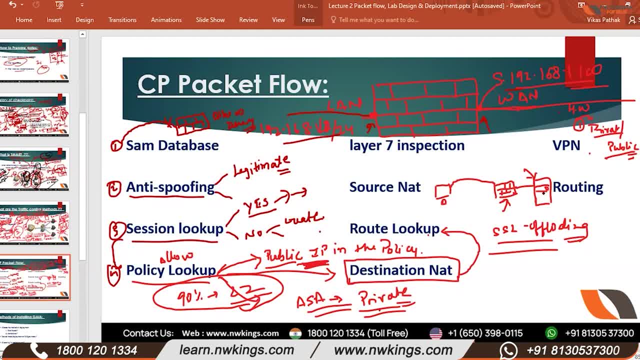 Or we checked the information and routed it to the server. Now it will go to the server, The server will decrypt it, Then it will check the information and send it to us. Now what happened is that this SSL offloading comes here After the source net. 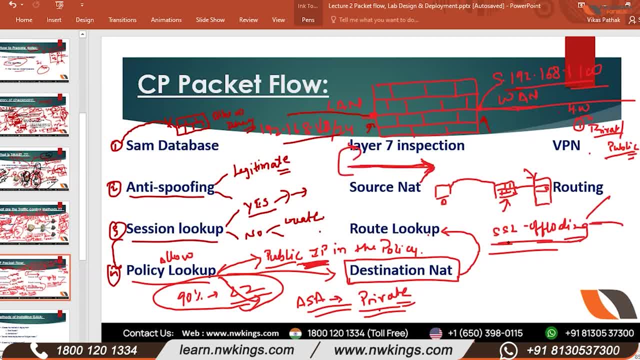 Why? Because if we do SSL offloading, then what are we checking in it? If we talk about SSL inspection, Okay, What are we doing in the inspection? We are decrypting and checking that. what is the SSL traffic coming? Is it legitimate or not? 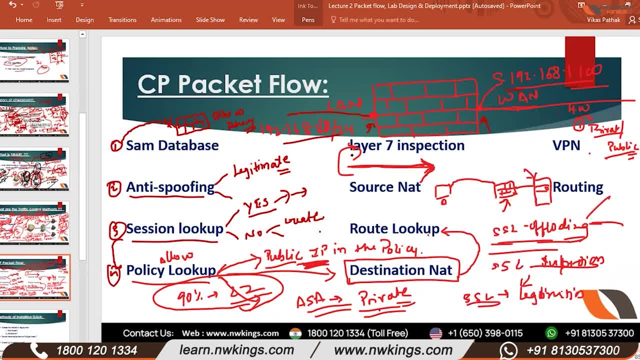 Right, And where is SSL? Does it work in Elsevier? Yes, So this whole area will work here. Okay, Make sense. Make sense, Understand the logic. I am saying that work is done here. Don't get confused, Understand the logic. 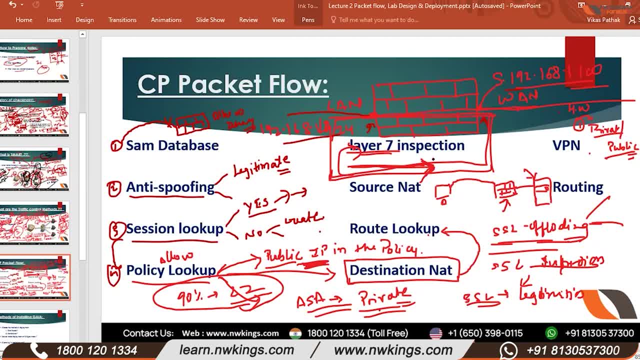 Why is work being done here? Okay, sir, Right, Don't keep this at all. Yes, Vikas has told that here it will be between L7.. Right Source is between L7 and VPN. No, don't do this. 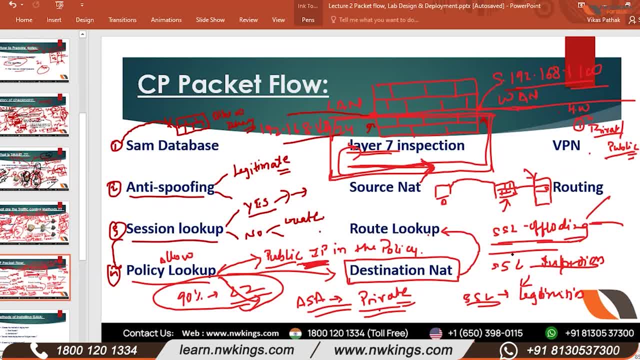 We have to understand why this will happen. If someone asks us a question, then we have to give this definition, Because what are we doing in SSL offloading? We are offloading it. If inspection is going on, then we have to check whether the data is legitimate or not. 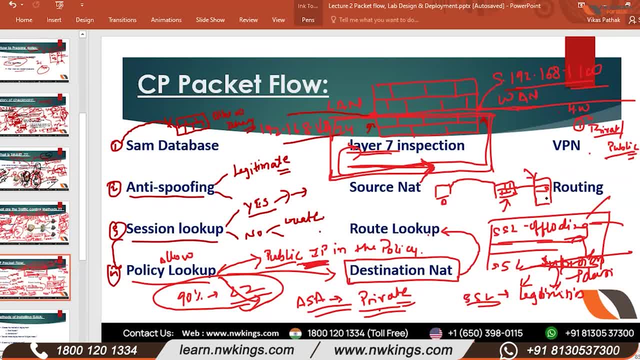 And if we have to do offloading, then we have to offload it and decrypt it. So where does SSL work In L7.. Where is L7 inspection happening? It is happening here, Right, Okay, Okay, Let's go. 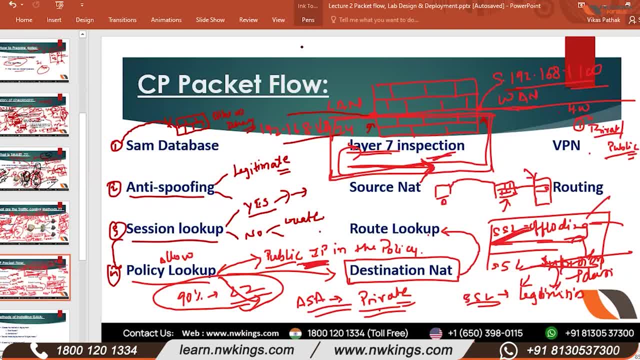 Any other doubt? Negative, sir, I am waiting. As long. as I am rubbing all this, you guys revise it once and tell me if there is any doubt. So on this, Any question, whatever is coming in the mind, right? 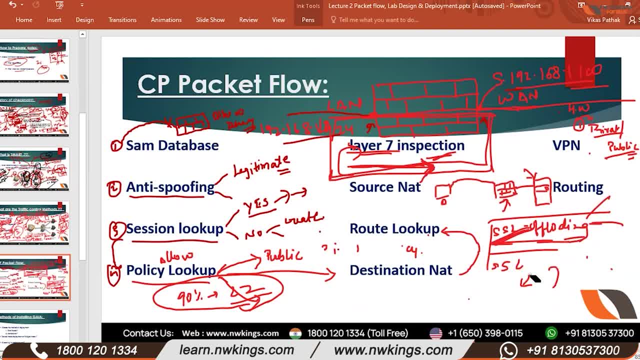 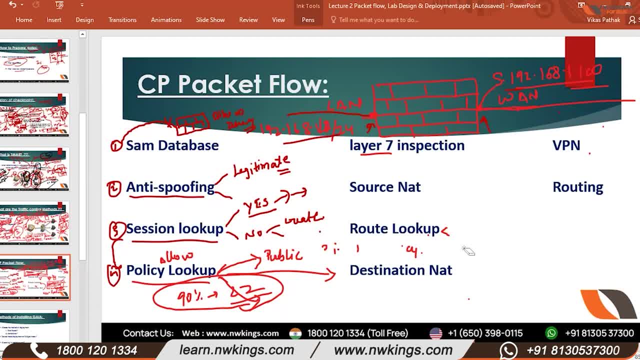 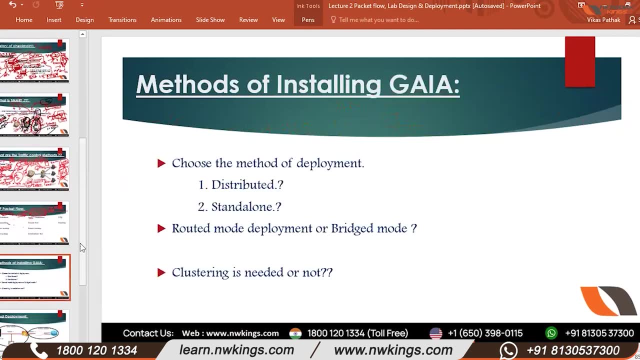 Tell me, And if yourside is not coming to mind, then I am going to ask questions little while now, Because you will have it now. Ok, now let's get to the interesting part. Our target is that when we complete the next step, we can come up with our product, right? 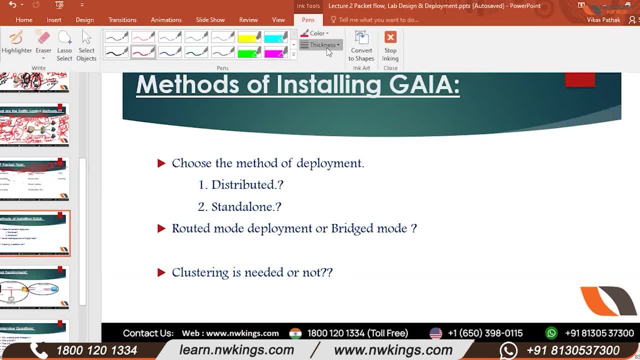 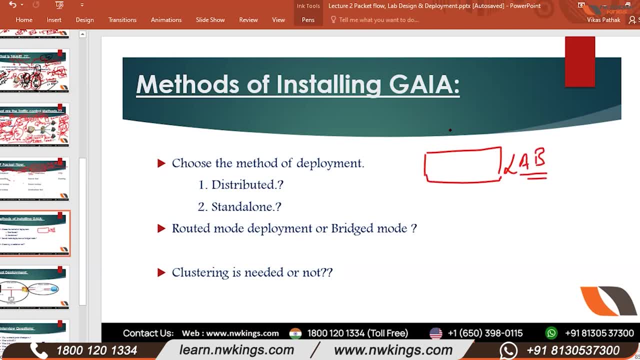 Yes, you are coming for it next Saturday apni class karein, toh usme ham lab perform karein. Kya perform karein Lab Abhi ki jo yeh first 4 ghante class hai. isme hamne theory complete kar deni hai. Aap log notes bana rahe ho na. 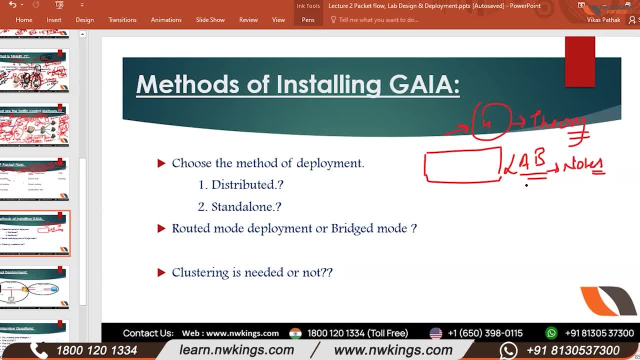 Yeh nahi bana rahe hai. Yes, sir, Tama target. yeh hai ki theory, jo part hai, wo 4 ghante mein complete karke ham lab pe move karein. Next Saturday se ham thodi theory aur most like 70% ham lab pe kaam karein. 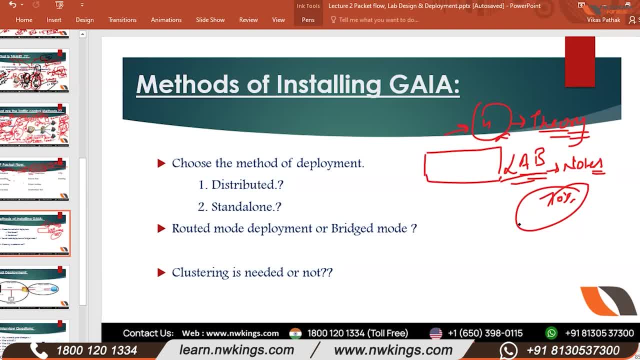 Ab lab ka matlab yeh hai, ki hame kuch lab ke baarein me bhi information gather karne parayi. Toh sabse pehli jo cheez aati hai, wo aati hai, ki jo checkpoint ka software hai gaia Yad hai. aapko gaia ke baarein bataya tha maine. 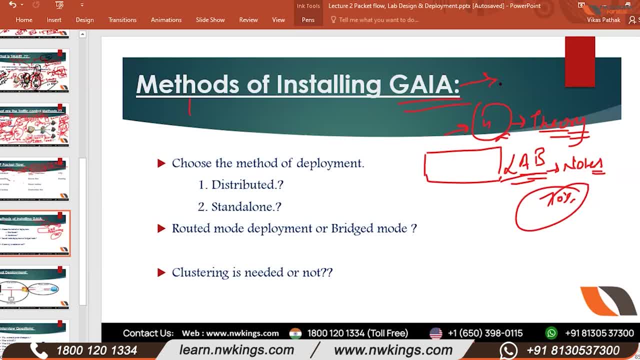 Yes, sir, Agar yad hai bata, toh kab launch kiya tha checkpoint ne gaia 2012? sir, Yes, correct, 2012 mein gaia ko checkpoint ne launch kiya tha, Aur tabse aap tak gaia hi chal raha hai. Uske updated versions aa rahe hai market me. 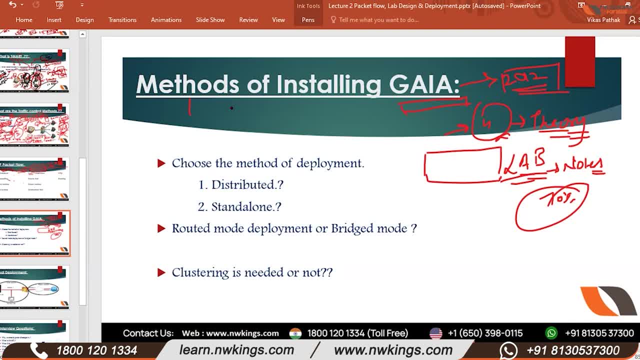 Ab gaia ko install karne ke jo methods hai, wo ham discussion karenge, ki wo method kon kon se hai Tika, Tika Saba se pehli, jab gaia ko installation ke liye aap like maal lo, aap ek IT administrator ho. 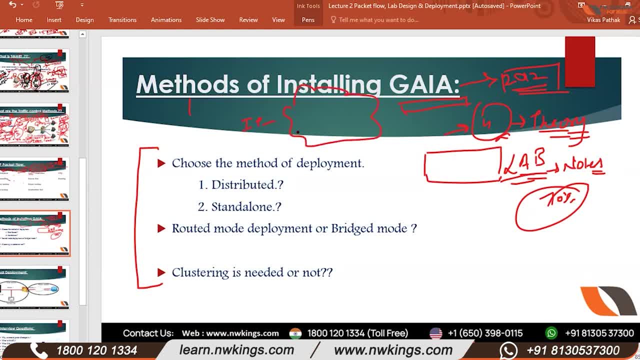 Tika ek organization hai. usme aapke paas aa gaya ji, ki aapko checkpoint deploy karna hai. Toh kuch questions aapko, na either the management, either with your IT manager, ya phir aapko khud decide karna padhega. 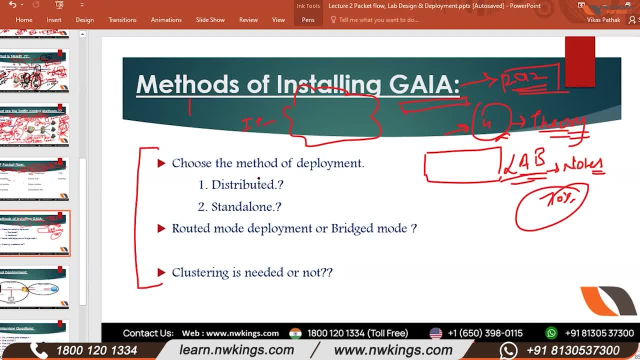 Usko document bhi karna. padhega kiya ki sabse pehli deployment ka method kya choose kar rahe ho: Is it Distributed or Standalone? If you were involved in our first class on YouTube, then I had explained it, but I will explain it again to you. 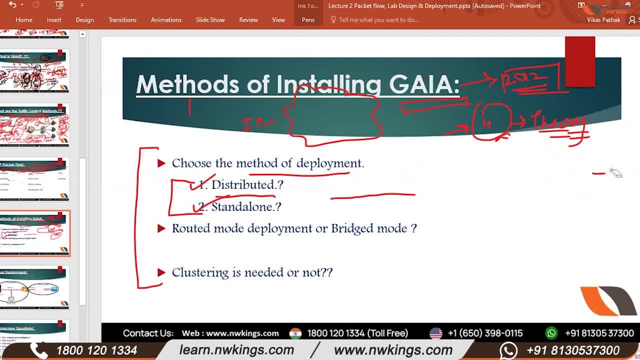 What is the difference between Distributed and Standalone? What is the checkpoint that you should do, deployment and why? Let's talk about Distributed. What is Distributed Environment? This is your client. This is the management server. These are your two gateways. 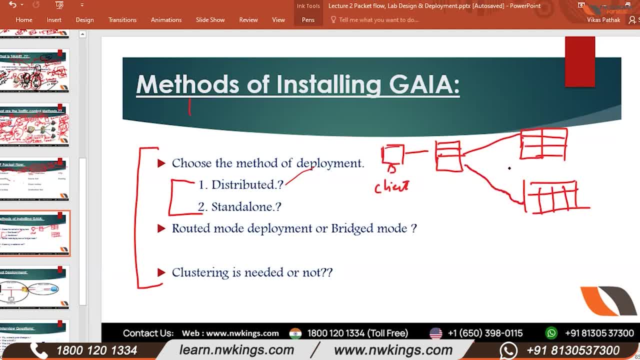 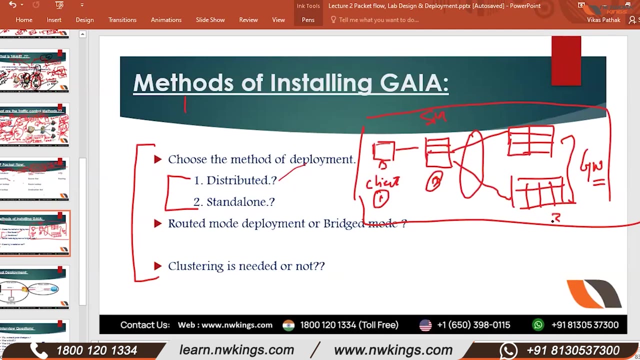 These are your virtual links, This is your SMS, This is your gateway. So this three-tier architecture is called Distributed Environment. If I talk about the physical environment, then here SMS is also your gateway, It is good. If I talk about a good environment, then this is also good. 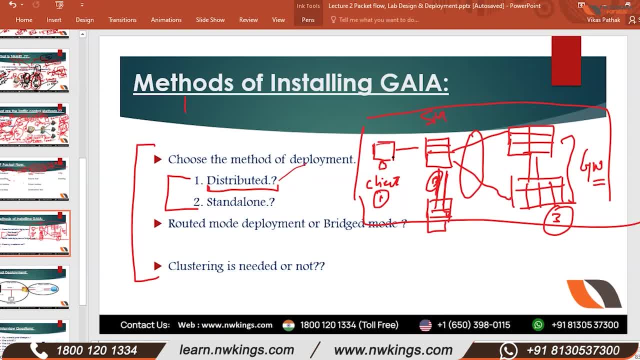 So what happened is that whenever you opened a smart console on the client, you took SMS through the smart dashboard and then after that you sent the modification to the cluster. So this deployment is called Distributed Deployment. Okay, Sir, Sir, where will you keep the firewall in this? 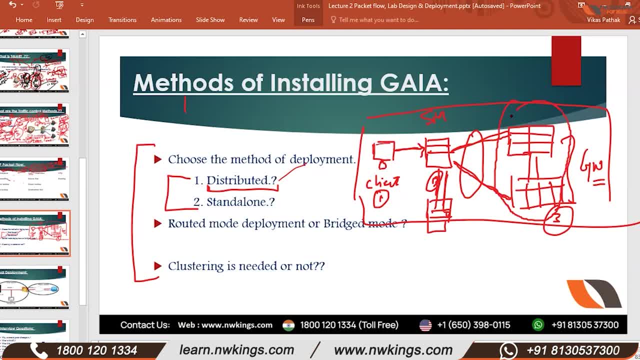 Here it is Gateway. Okay, the firewall will stay here. This is the only one on the gateway. Enabled. on the gateway means understood As I say this request from the server to the client and from the server, No, no, no. 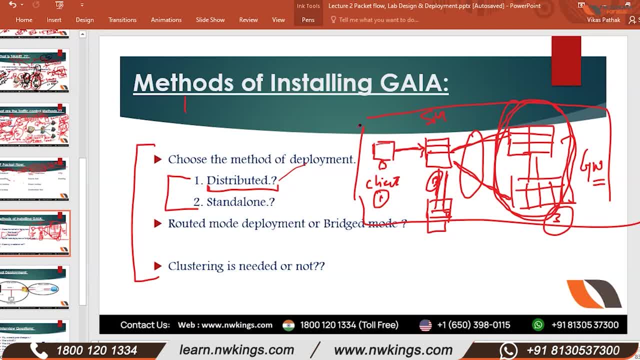 You did not understand this client. This is a smart dashboard client of checkpoint. This is an admin PC. This is not a normal client. This is the administrator's PC. on the administrator's PC, the smart dashboard checkpoint is configured through it. you 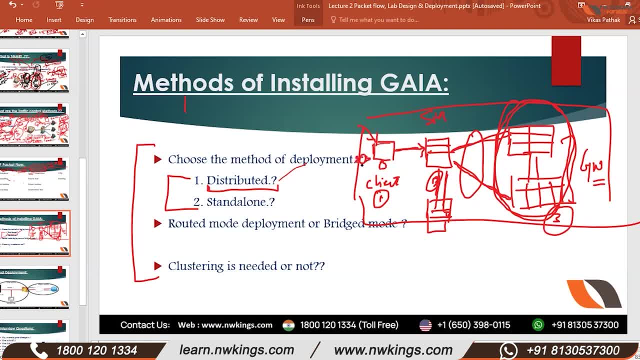 the administrator is sitting here. this is you. ok, now you sit here and take your SMS on the remote. after taking the SMS on the remote, you do configuration and push it on the firewall. ok, the firewall is connected to the gateway. the firewall is connected to the gateway. 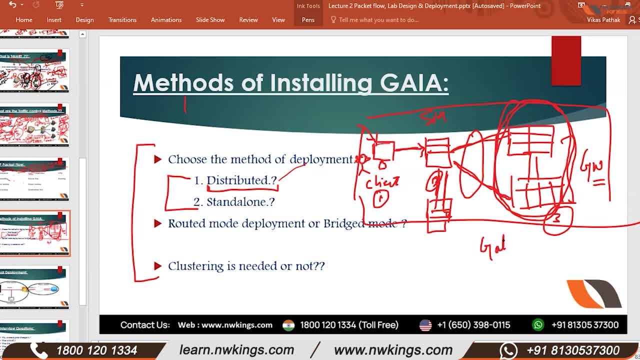 ok, what do you mean by gateway? gateway means no. no, I am telling that we are sending request from checkpoint SMS SMS dashboard to server and server. there are two gateway connected, which is through virtual link. ok, so my question is: the firewall? where? 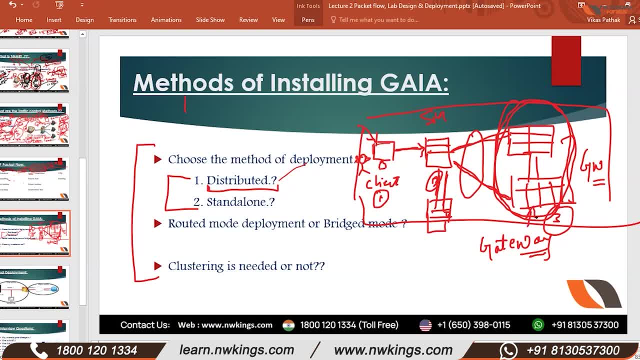 is: where is the firewall located? these gateways are firewall. no, ok, so here there are two firewalls because two gateway? no, yes, because they are in HA. ok, so two firewalls are connected with HA. yes, understood, understood, understood, yes, and similarly. 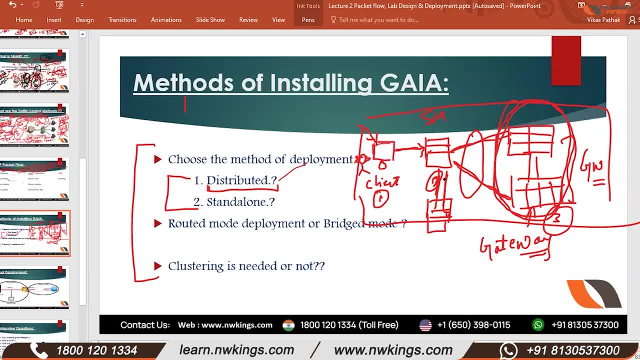 here. if the SMS is also a good environment, then the SMS will be in the server. that too will be in our cluster in the HA server. yes, management server. see, were you in yesterday's class? No, no, because I am in the cluster. 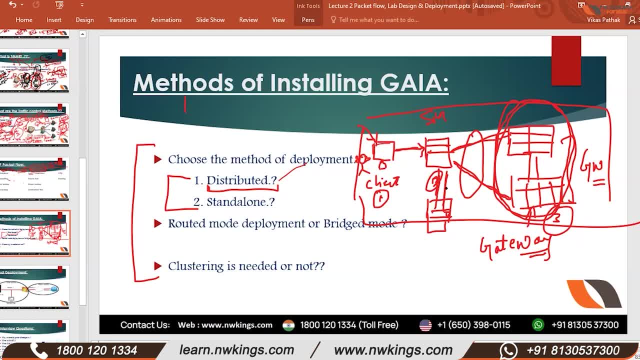 I am doing job, so they will not give me allowing the class permission, so that's why I am confused. ok, oh, ok, it's Neelish, right? Yes, yes, Neelish, I will take a very small quick five minutes and revise it for you. ok, so that. 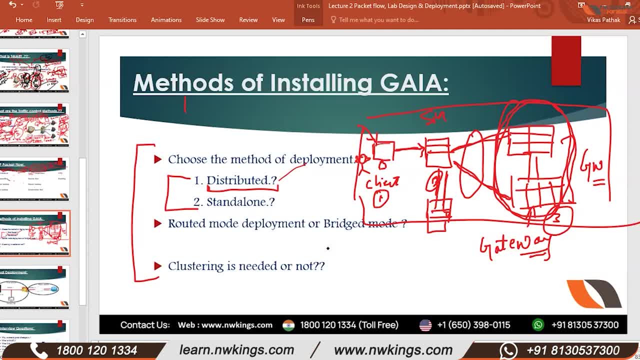 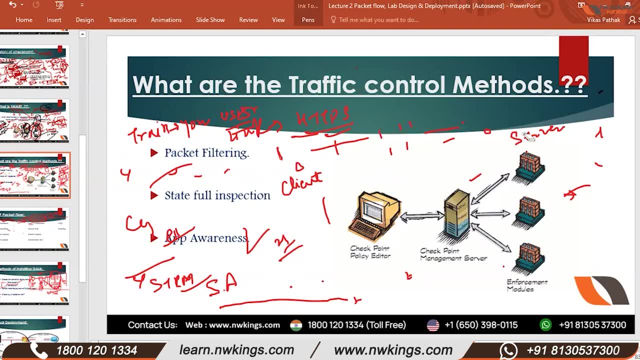 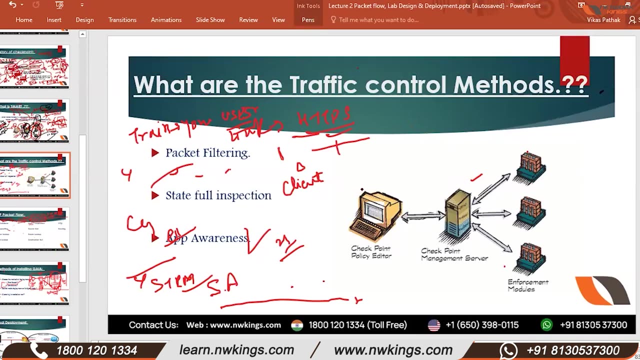 you can mug up with the class. ok two, I will show you this architecture Neelish: Yes, yes, yes, This is the architecture of the checkpoint. ok, this is your checkpoint policy editor. ok, on which you will sit. you will sit and do the policy modification. ok, the policy. 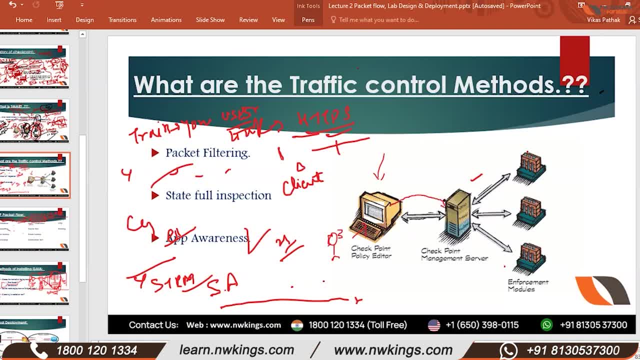 modification you must be doing. you must have picked it from the management server, checkpoint management server. checkpoint management server. yes, and after the modification, when you, when you push the policy from the management server, it will be reflected to your gateways. 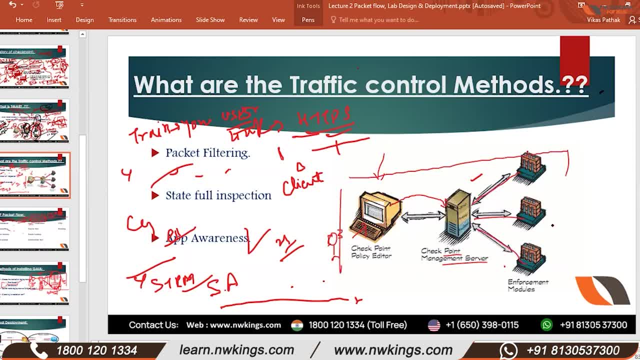 ok, so this is the three-tier architecture, the three-tier architecture which claims the checkpoint. first level is this second level is this third level? is this so first, second and third? this is called three-tier, So it is also known as the distributed architecture. 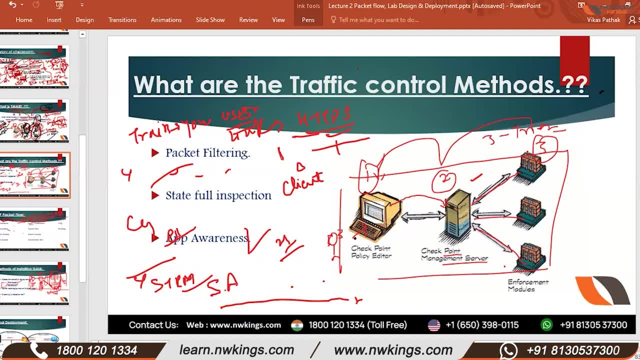 Yes, this three-tier architecture, known as distributed deployment, where you have no dependency of the client, either management server or the gateway, on any of the devices. Ok, understood, Understood. Yes, Hope now you will be able to connect the dots. 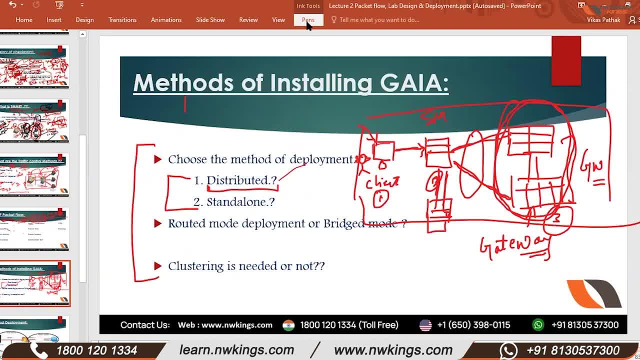 Yes, yes, Right, Yes. So this is also known as the distributed architecture, where we have a separate client, a management server, two gateways and or whatever they are. so this is our one typical environment, a very small environment. this is called distributed. 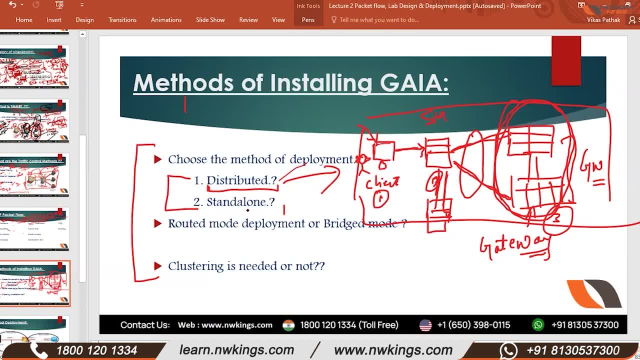 Right Now. what happens in the stand alone? What happens in the stand alone when the network we have is small? in that case, what we do is that our one. this is the client. what happens in the stand alone when the network is small? 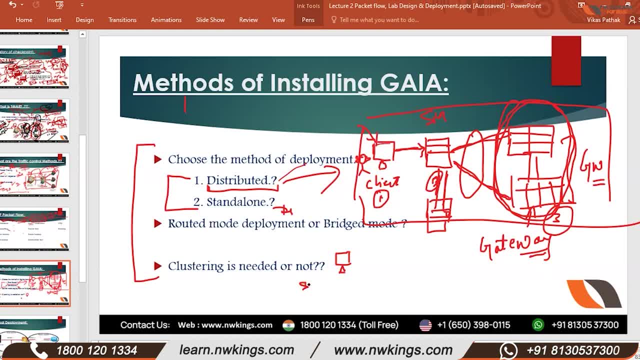 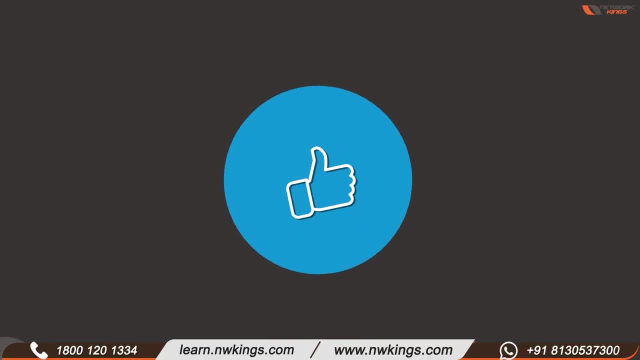 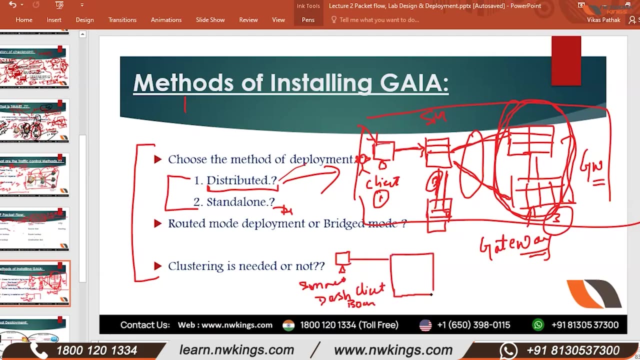 to get client. take a smart dashboard client here. this management server: hi, you are watching the recording from one of our live session. hit like share and subscribe for more future updates. sms server: it is divided into two parts virtually. first part is sms management server. security management server. 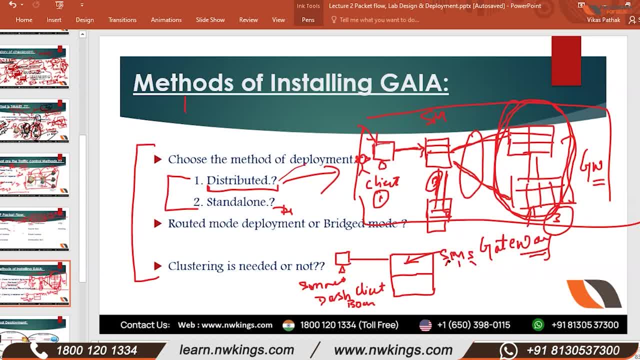 sms is sms's acronym. the second part, that will become the gateway gateway, is also aligned on the management server. yes, that is the standalone. yes, so what happened is see: logically, this is also 3 tiered, right, yes, logically: first level, second and the third level, this is also 3 tiered. 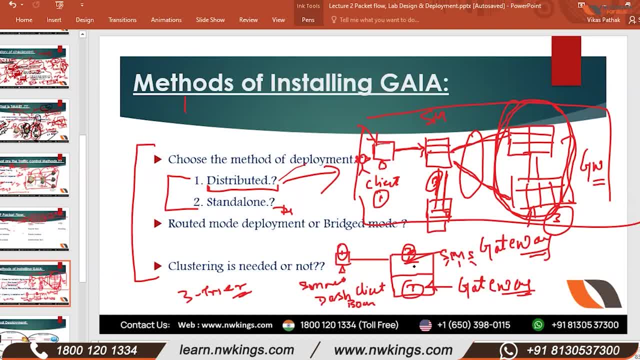 but physically it is not a distributed environment. so this is not a distributed environment. so this is not a distributed environment. if this management server crashes, then your gateway will be sit, so this is called standalone deployment. now you should have two gateways and you have to enable good. for that you need licenses. 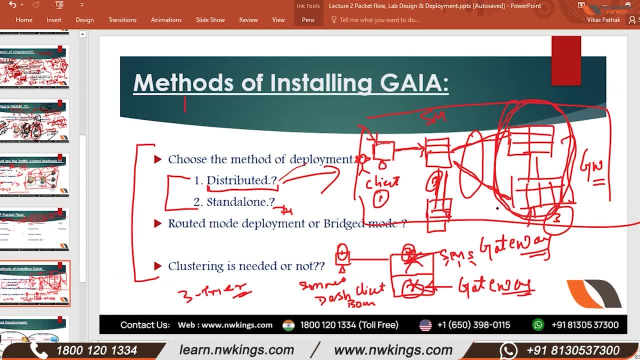 right, so the cost increases on it. so if you have a very small environment and a very small company in which you are deploying, let's say you took a project of some company and the company is small and that is not a- and the company is small, they can't spend much expenditure on their IT project. 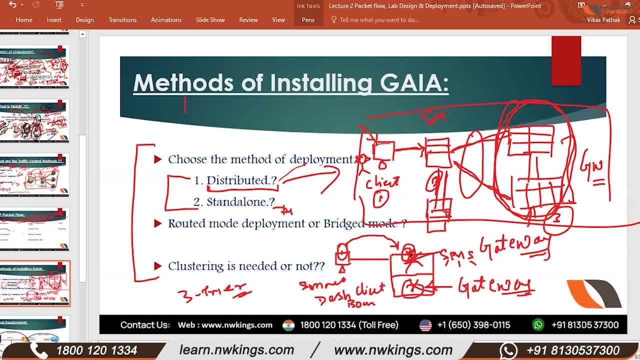 So there this type of deployment after the risk assessment can be done. We can do this standalone deployment. all your features will work at the checkpoint. but the risk is that the day your high utilization or anything happens and it sits, then your gateway will sit and your network will interrupt. 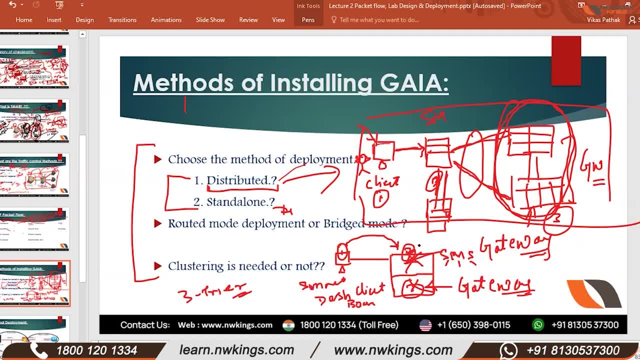 So most of the time client will agree on this risk and you have to deploy this. I have done around 70% of the deployment- standalone and 30% of the deployment is distributed, Because distributed takes time, standalone takes less time and is easy to set up. 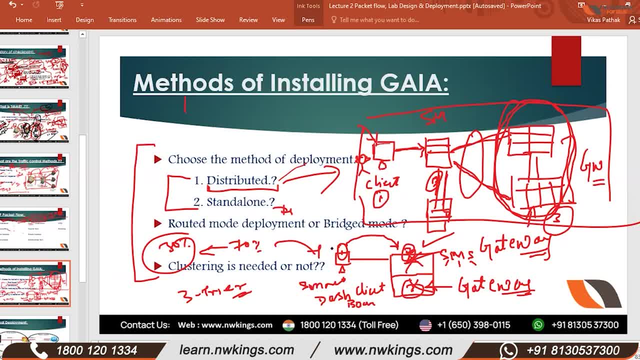 So until and unless it's not a very big organization, very standard oriented organization, they will not go. for the distributed environment They can go, but what I have seen is that 70% of the deployment is done in standalone. Now the second thing is that you have to make this decision, that 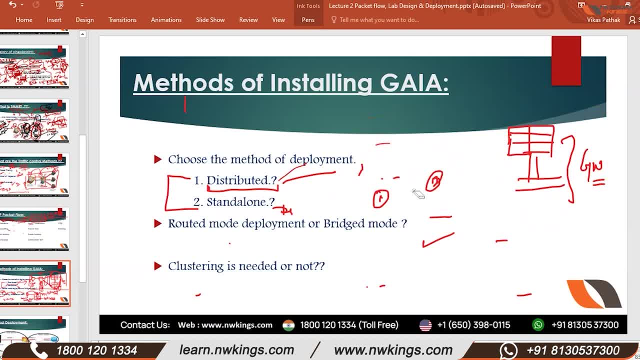 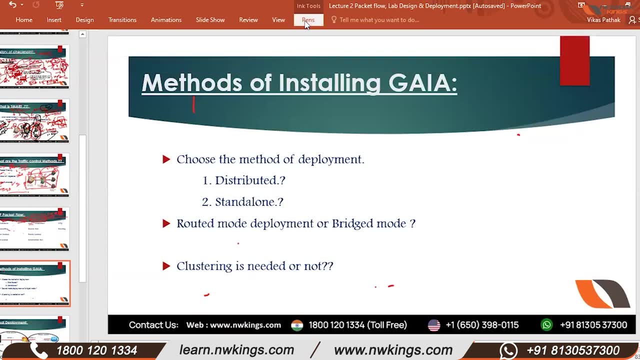 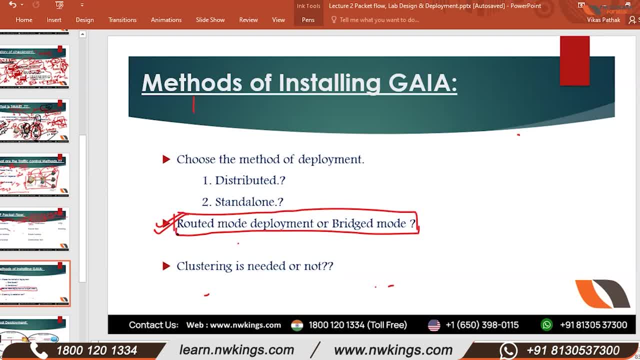 you remember this term: a routed mode deployment, a bridge mode deployment. I will explain it later because it is a little tricky part. You will have to understand a little more things. for that I mark this here as a star. Write it in your notebook that I have to explain the bridge mode and the routed mode. 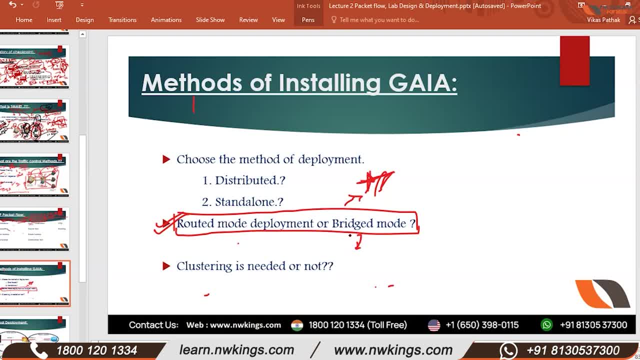 I will define you in next class or in the next class, Okay, But you also have to make this decision. you have to make it initially that in which mode you will do the deployment, Alright. After that comes, third, Which either you have assumed that you are doing stand alone deployment. 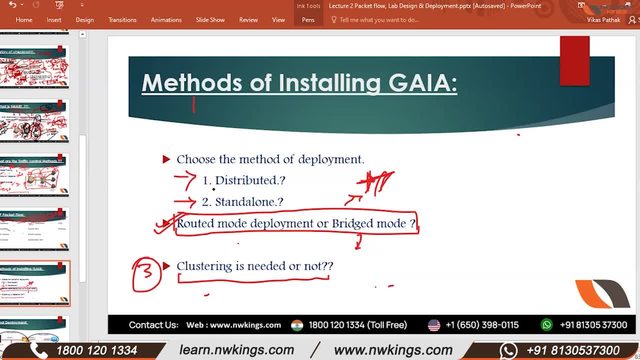 Or you have assumed that you are doing distributed. Now, if you are doing distributed, then you have to take one gateway or two. Many times what happens is that you take a client, take one single SMS and take one single gateway. Say that we will use SMS from client and we are managing one single gateway from SMS for now. 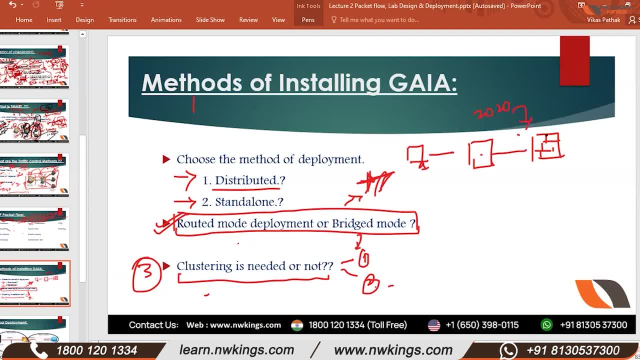 Means, if there is deployment in 2020, then do this deployment In future, in 2021 or 2022. we will take one more gateway and convert it into HMA, Alright, Alright. So this decision also you have to take initially, that you have to create HMA. 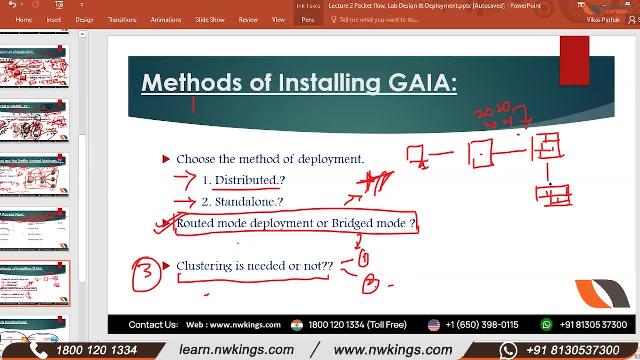 High availability or not to create HMA. Or it is possible that in stand alone person says that this is your client, This is your stand alone box. You do it in this If this person tells you to make this scenario. If this person is a person, then he does not have much knowledge about the risks. 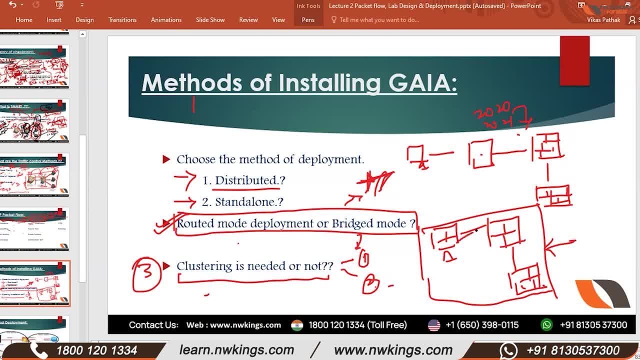 What are the risks, What are the benefits, What are the drawbacks? If this is told to you that do a stand alone deployment, Do it in stand alone box, So in that case you recommend them that, sir, it is better than this. you do this deployment. 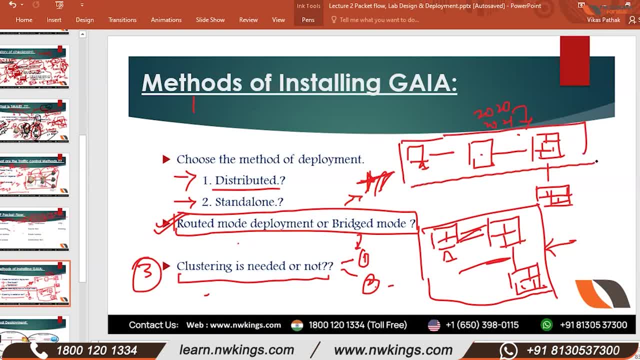 This one. You have two management servers here. Why are you making two firewalls? If you have three resources, then go for this one. This will not make any difference on your single device. Until and unless your traffic is passing very high, You have a lot of users. 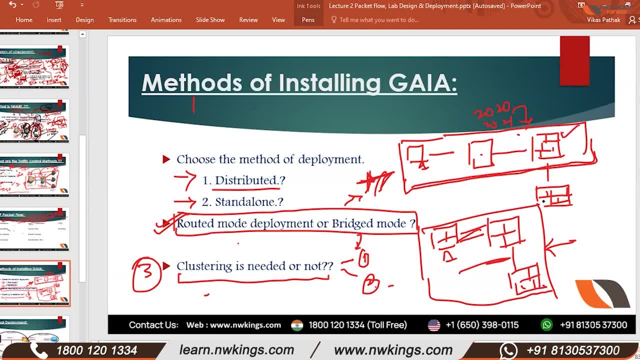 Right And it will also be stable. In doing RMA it will be easy to maintain this environment. All your policy backups are on your management server. If the gateway is sitting, then you do RMA on it, But if it is sitting then you will come on it. 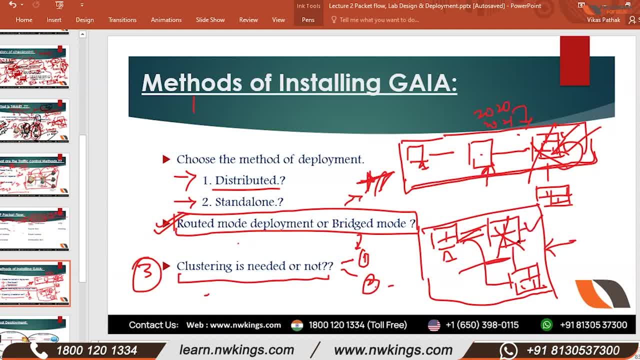 And if it is sitting, then there will be a reason for it, That high utilization or something else. If the same situation is here, then both of them are sitting. But if it is sitting, Your gateway, Your management server is safe. Policies, backups, all logs are safe on it. 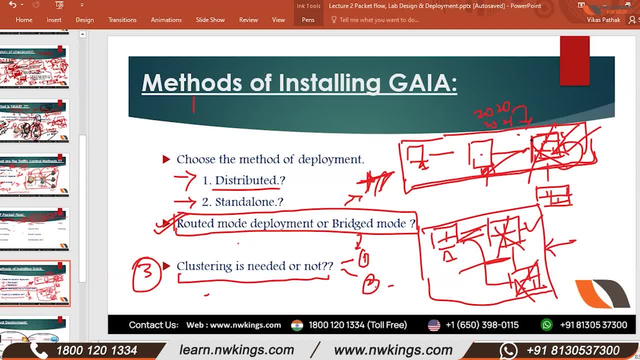 If your firewall comes. What you have to do You just have to plug your firewall. You have to make connectivity from the management server And you have to push the policy. That policy will reflect Your network, will run on the gateway Make sense. 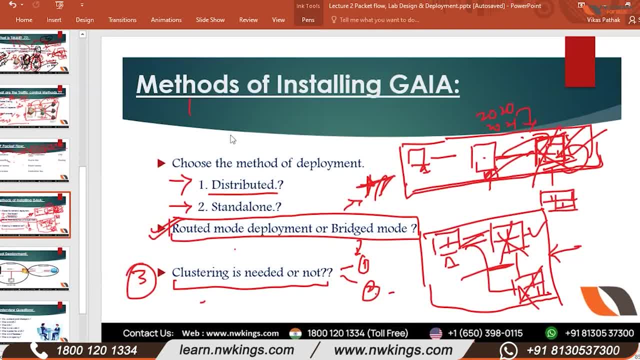 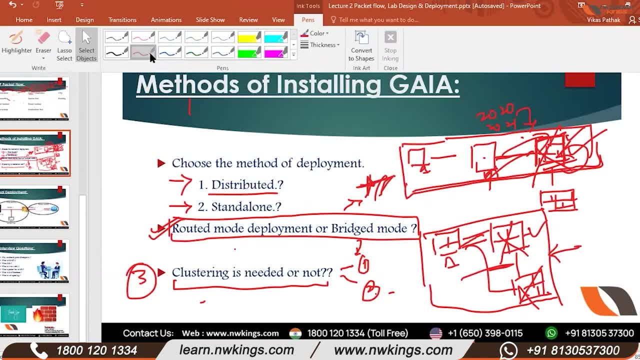 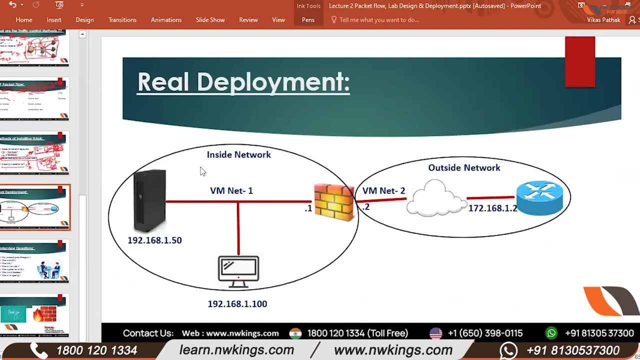 Any question? No, regards Nilesh. No, no, no, sir, No, no, Okay. So If you have understood this thing, Then we are going to make this kind of environment in our lab. Okay, This is our SMS. 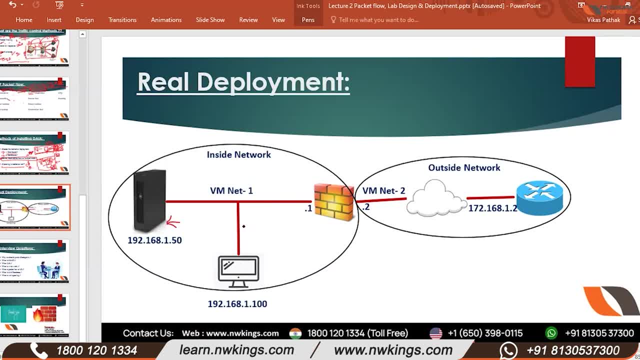 We will change the IP a little bit, We will make a modification, But I will recommend you that this slide Which I am showing you, Take its print screen. And take the print screen and save it in your notepad. Reason, If you are making this lab on your single laptop. 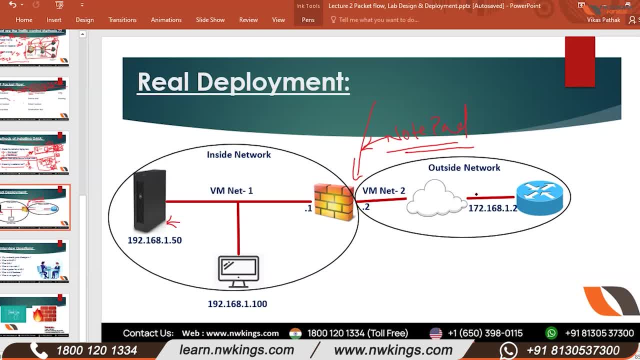 Virtual lab, Then you have to do deployment in this way And this deployment will be easy to set up for you If you do it on your laptop And the lab. I will do, I will demonstrate it to you How to do it. 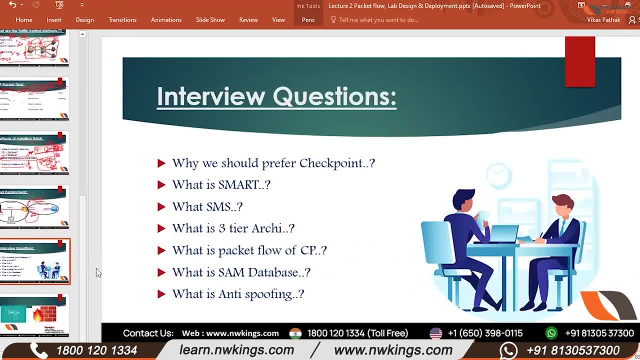 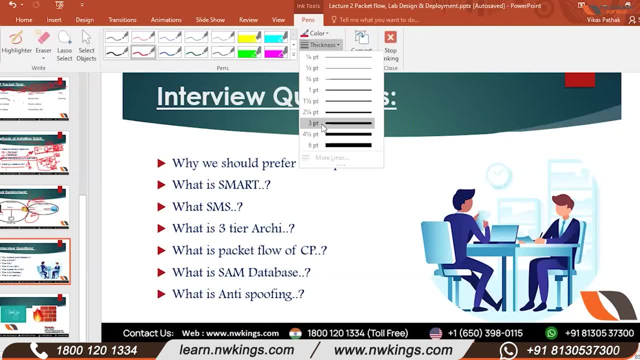 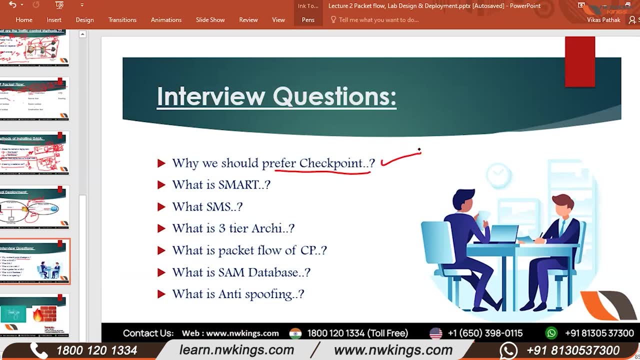 Okay, Let's go Test time. I have to do all these things quickly, within 5 to 10 minutes. Tell me all these things, We move to the next class. Tell me the first question: Who will tell? Because of its next generation firewall capabilities. 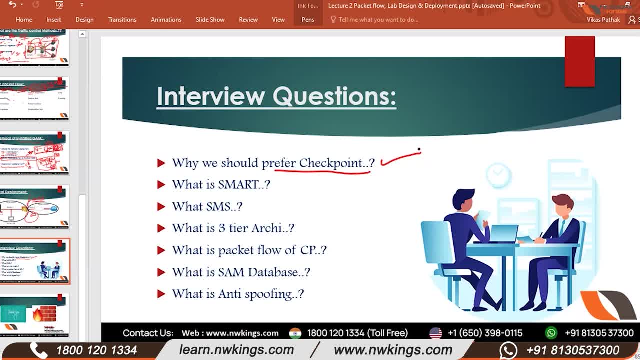 Easy to deploy- Okay, And Secure architecture: Okay. That makes it easy to manage, Okay, Okay. Second smart Smart is secure management: Secure, Secure console, Secure management server And secure gateways. Security management architecture- Yeah. 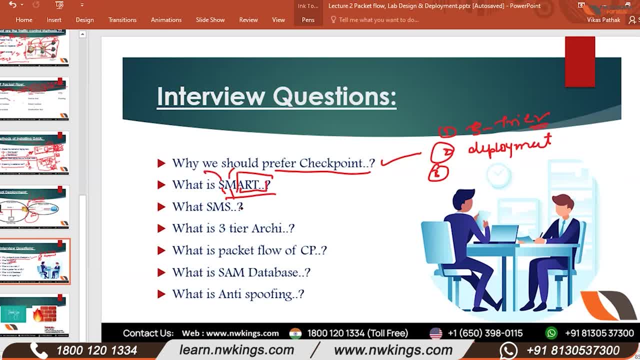 Security management architecture. I was going through the three. SMS is secure management server. Okay, Nilesh, We discussed the definition of smart yesterday. Okay, Smart. Yes, Smart stands for S Means security And stands for management, And ART is taken from your architecture. 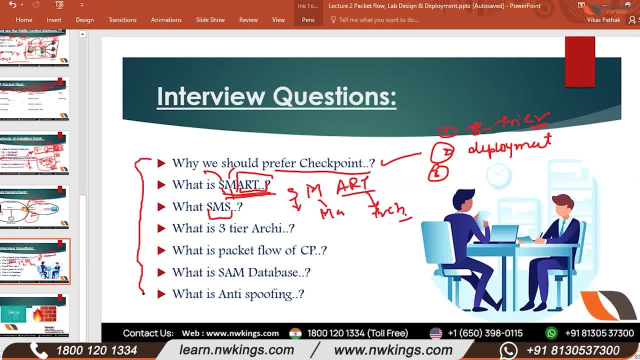 Okay, Yes. Now all these questions I'm asking you because all these questions will be asked in your L1 interview: What is SMS? What is smart? And if you go to pre-sales, There is a pre-sales profile. Yes, 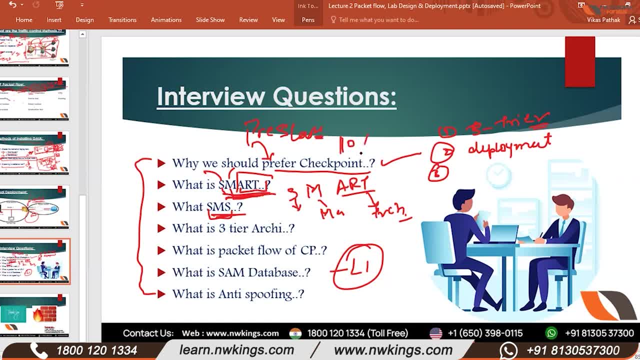 This question will definitely be asked in it. 110%, Sir, For L2 profile. You will get it. The session we have completed so far. These are the questions asked in it And these are questions of L1 level. Okay. 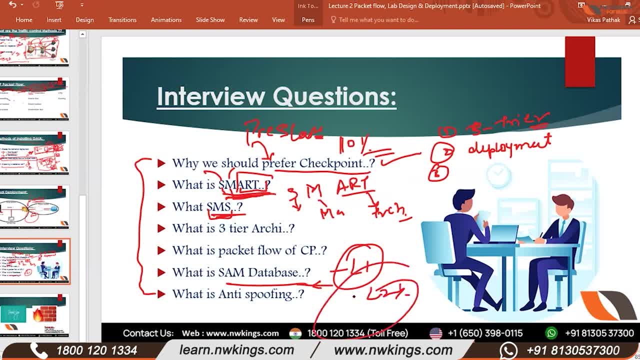 To ask you this SAM database. What is the concept You will ask in L2.. What is the problem? Okay, It's not a big deal, Okay, But I think that all these questions are concepts. These are concepts of L1 level. 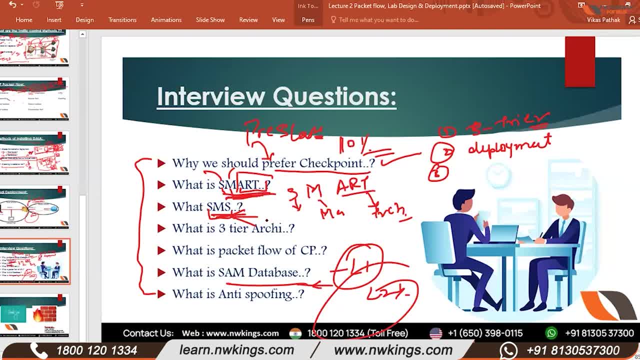 Okay, SMS stands for Secure management server. Perfect. What is 3D architecture? No right, Yes, Yes. What is packet flow? Yes, Yes, Yes. SAM database Anti-spoofing Session- look up. 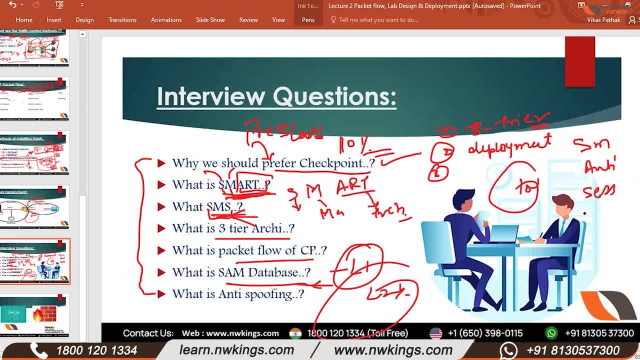 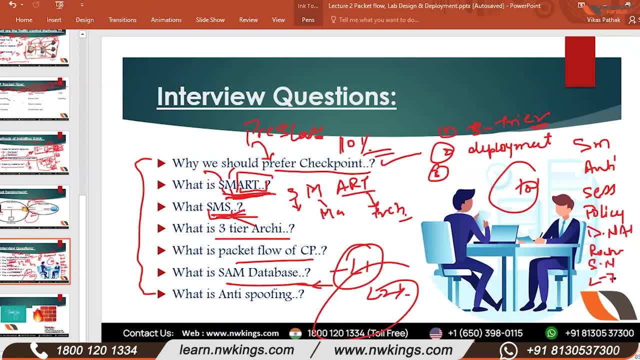 Layer 7 inspection: VPN Route Routing, Routing, Routing, Routing. Perfect Guys, I'm proud of you, Believe me. Do you know the SAM database? Yes, Will you explain it? Yes, Done, Nilesh. both these terms are a bit critical. 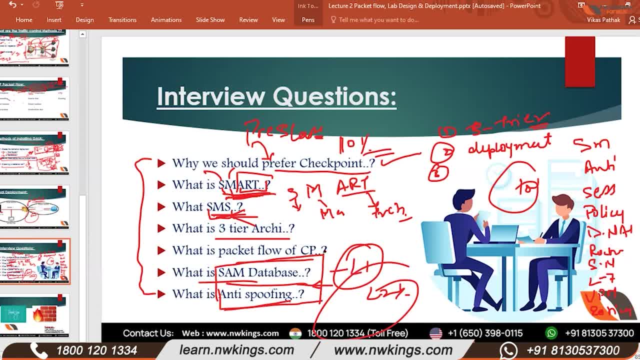 I don't want to tell you in a hurry. Please watch tomorrow's session. We have discussed it very well, Okay, Okay. So, that being said, our first and second lecture has been completed. Okay, Here, Now we will start the third lecture. 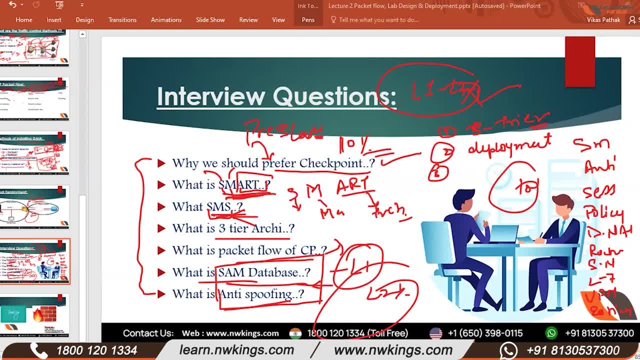 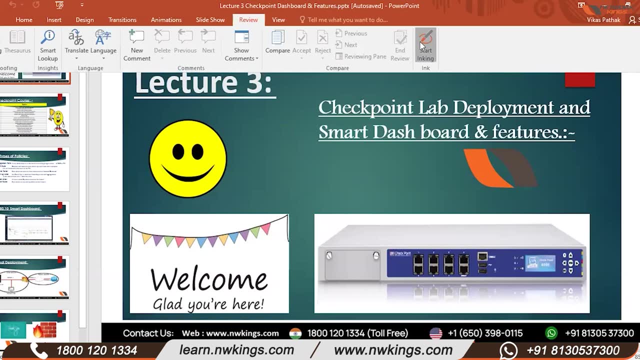 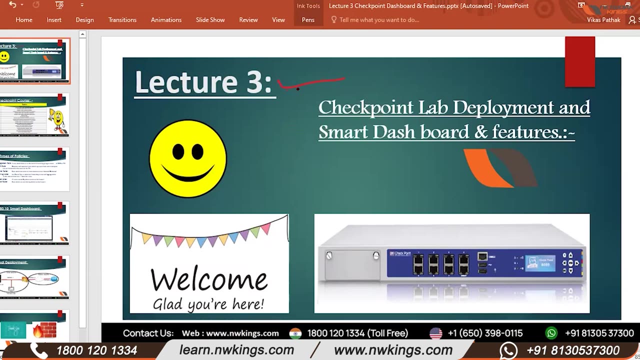 Can you see the screen? Yes, I will share it again. I believe the sharing is: Can you see the new slide? No, We will start the lecture. Okay, Let's start it. So we will start the lecture 3.. 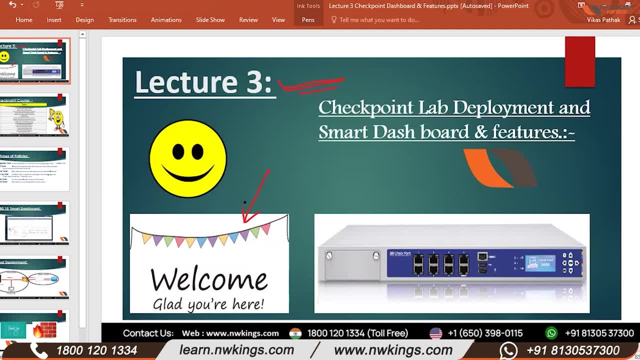 First of all, welcome to all of you who have come here to study the test. The motive of today's session is that we will discuss about lab deployment and, if there is a possibility, we will be able to look at the dashboard features. Okay, if the time is left after two hours. otherwise I will try to get you a lab deployment on EVNG. 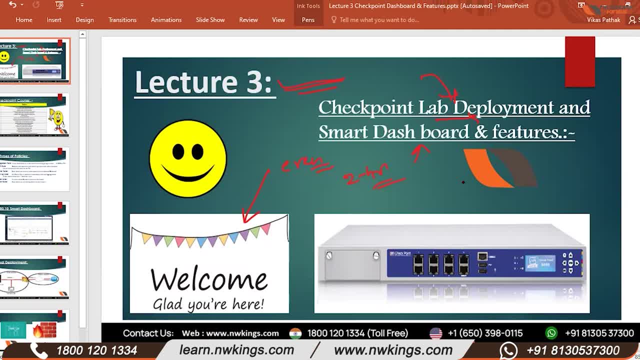 Did you all get access to the lab? Yes, I got access to the lab. Perfect, I will get you a demonstration on EVNG today. So this is the check point box. I told you yesterday that there is a box like this. 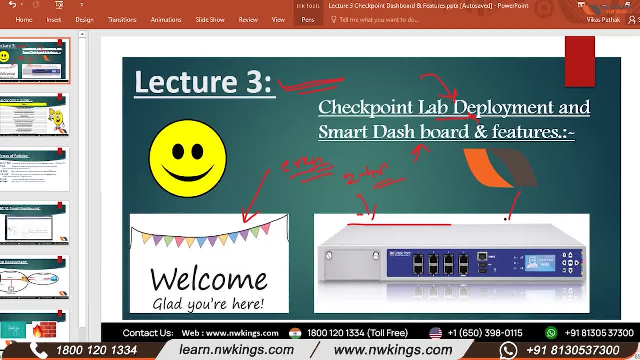 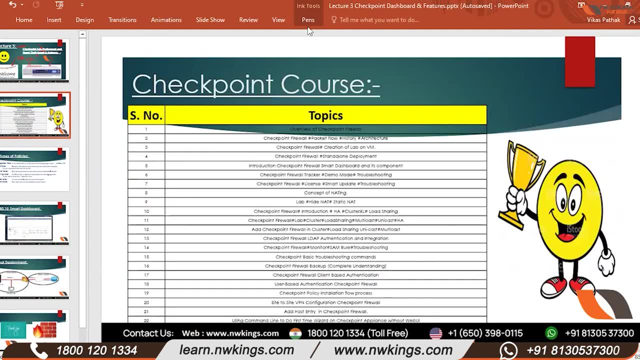 And if you ever get a chance to get a physical box, then you will get a box like this. And if I talk here then we are going on the topic. This one, lecture 3.. We will see lab creation VM. 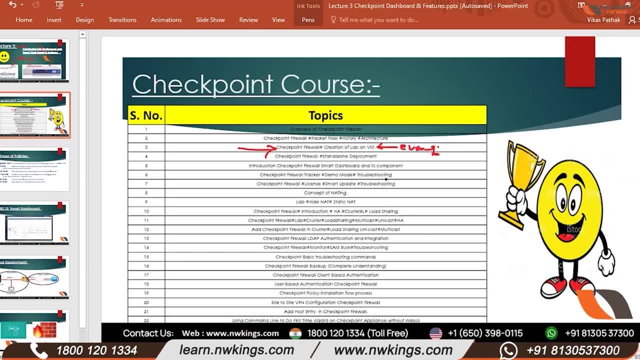 We are not doing it on VM, we are doing it on EVNG. Okay, if you want to do it on VM, then you can do it on your own laptop. For that, the requirement of RAM is that you need a minimum of 4 to 8 GB RAM. 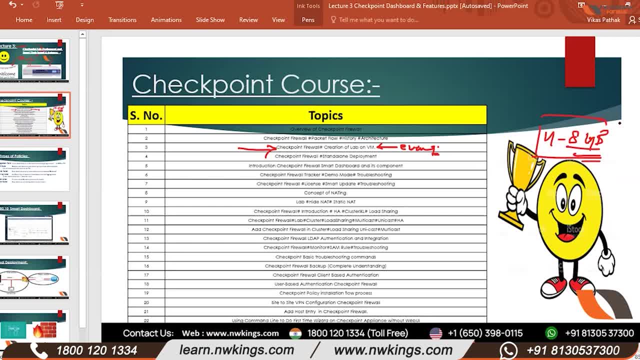 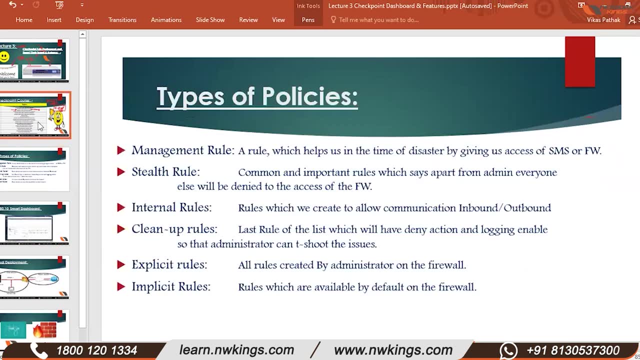 Okay, if you have the hardware, that you have- 4 to 8 GB RAM- then you can easily do it on VM. Otherwise, you can put EVNG in your laptop and do it on EVNG. Okay, So who is this basic good? on whom to do the lab? 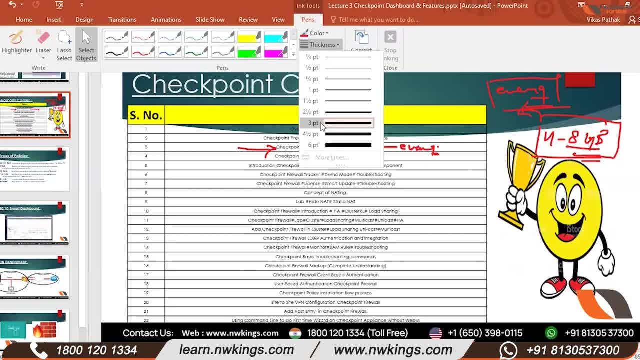 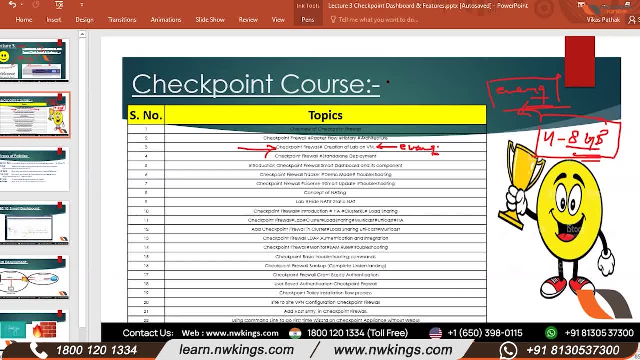 Look the difference between both VM and EVNG. What happens in EVNG? you get a diagram to make a topology. Okay, Suppose this is your PC. from here you go to the switch. There is a firewall in front of the switch. 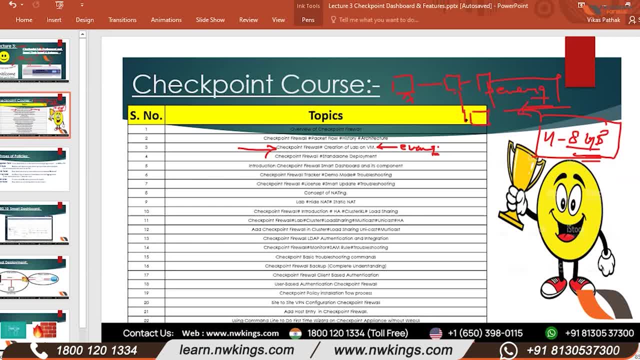 Under that you put another firewall, Then put another switch here, So you get to see all this graphical representation on EVNG. If you make a lab on VM, then you will have to make a copy from your pen and paper. After that you will have to make a logical understanding. 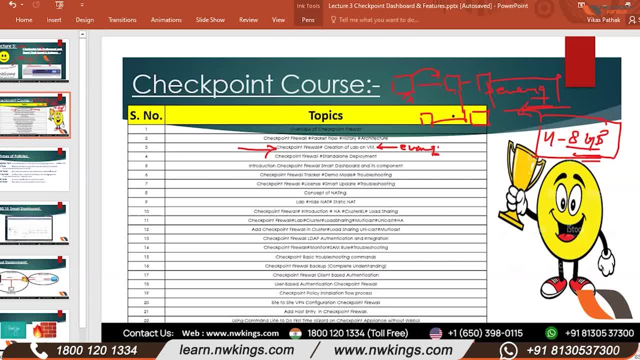 What to give to whom, what IP to give to whom. You have to do all this on pen and paper. There is no graphical representation there. Okay, So that's the basic difference. But I think if you do it on VM, then you face real-time issues. 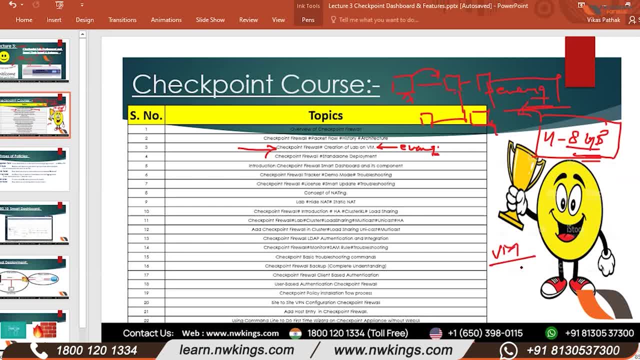 Because mostly the deployment will be either on VM or on physical box, Correct? Yes, So if you get physical box, then there is no problem in doing it. You just have to connect it and do OK, Which we will do in a while. 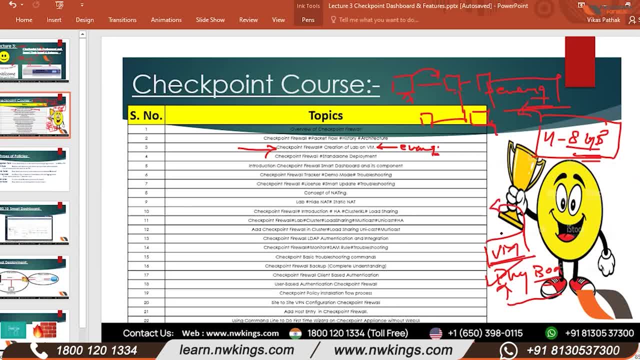 If you do it on VM, then the actual problems you face on VM, in real network, real deployment, you face those things there That the network adapter I have: with whom should I bridge it? How to create its LAN, How to add physical interfaces in it. 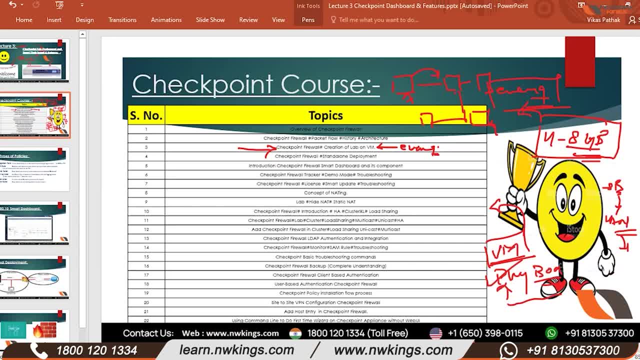 So somewhere when you do troubleshooting on it, then you also get a good understanding of VM. So you were doing the checkpoint lab and along with that you also did a small course of VMWare. Yes, So this is a little benefit of VM. 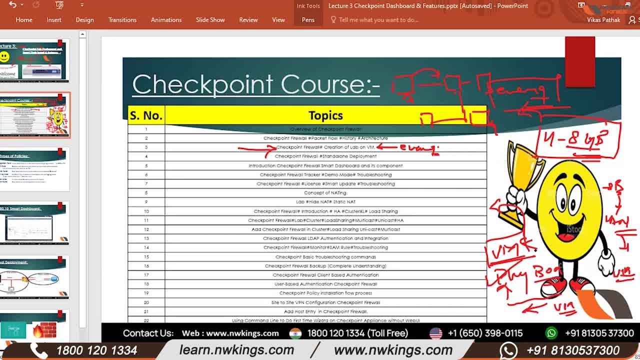 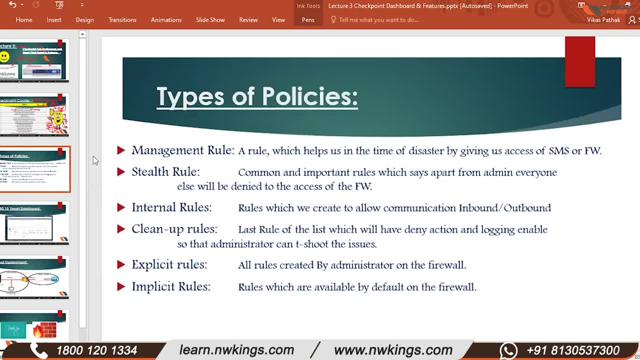 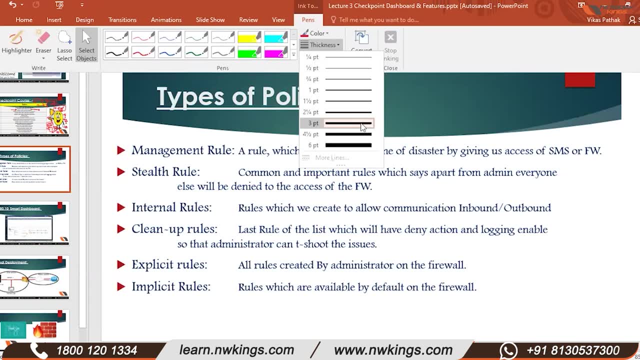 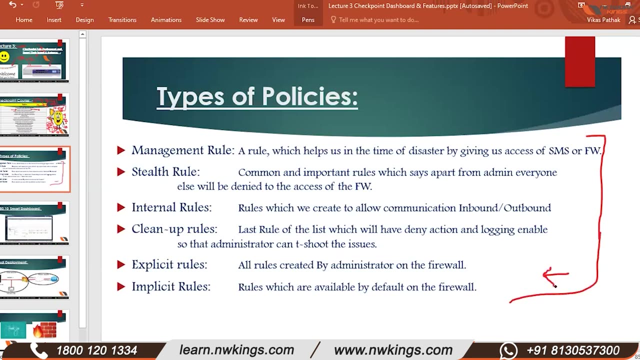 Otherwise, if it has a benefit, then the disadvantage is that you do not get visual representation. Yes, Correct, Yes, Okay, This section. take it as it is print screen and write the manual definition of all these in your notes. You do not have to write the definition of this from here. 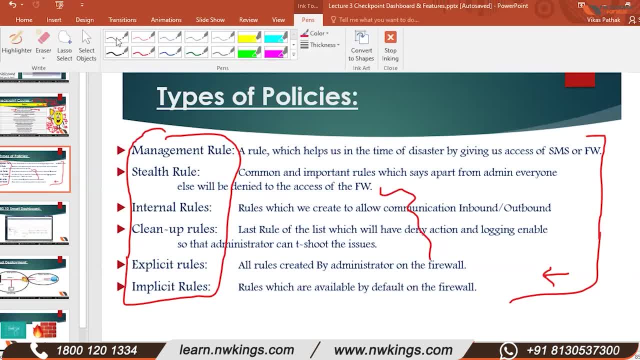 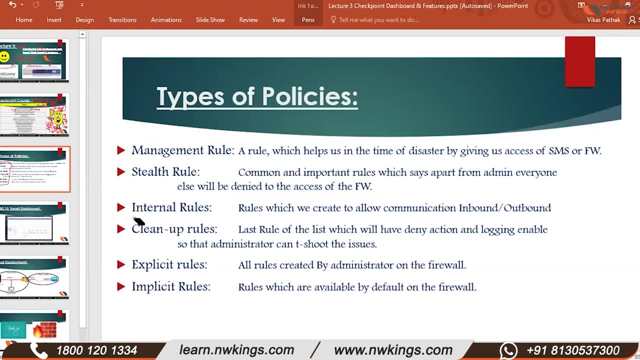 Do not copy and paste it. I will tell you: Okay, Let's go. So when we make the policy of the checkpoint, then to make that policy we use some methods, We say something to those policies. What are those policies? 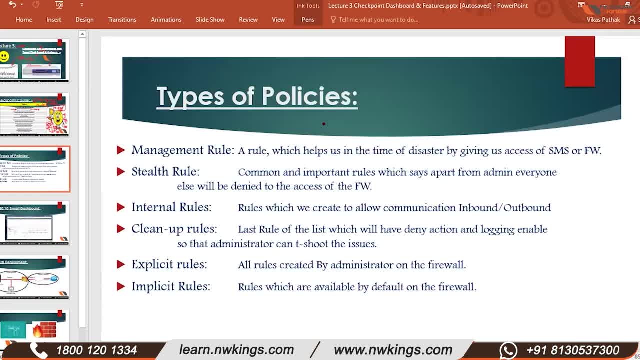 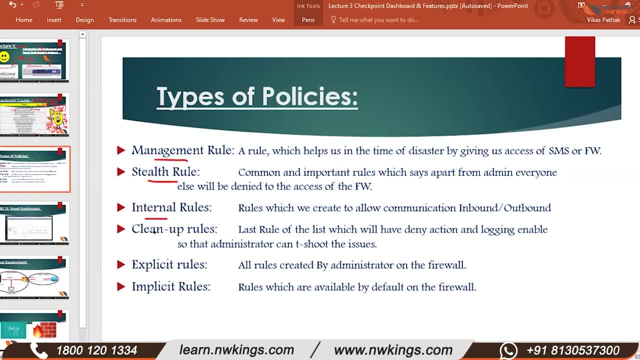 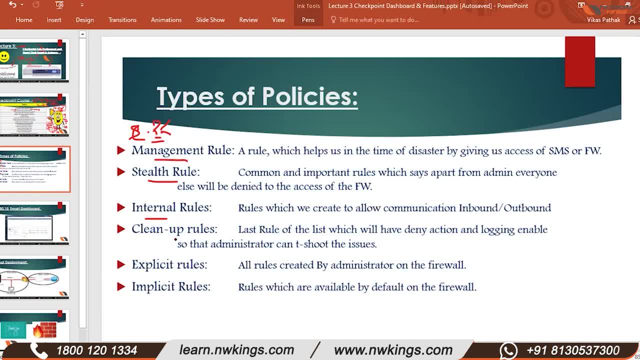 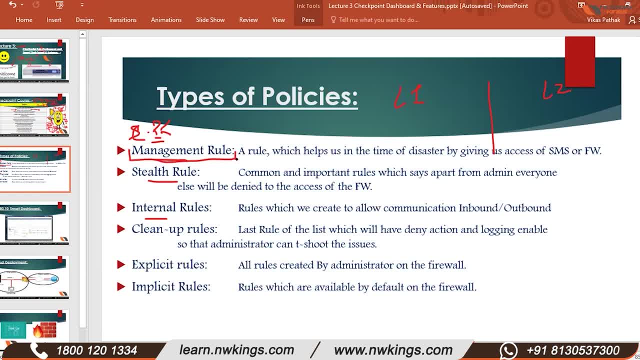 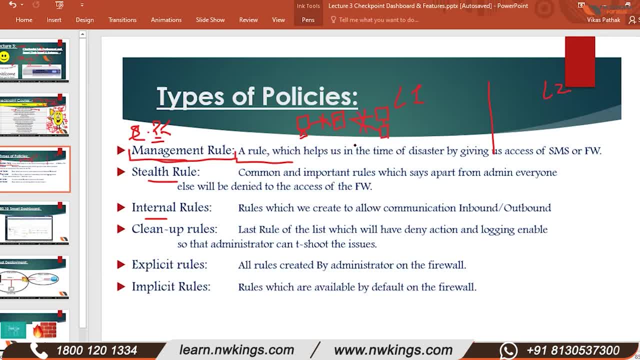 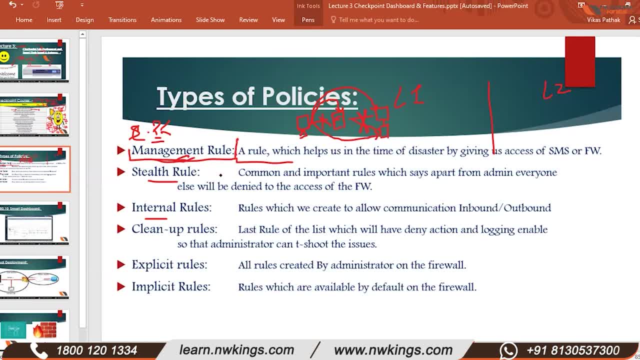 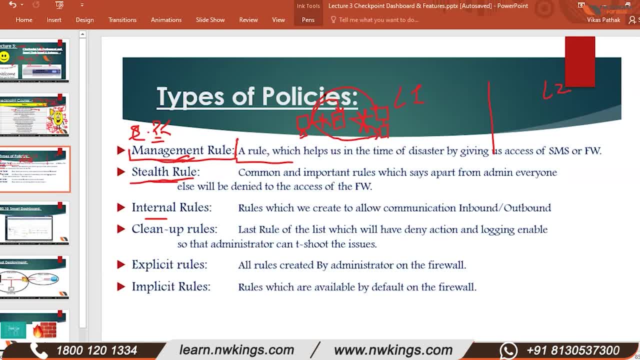 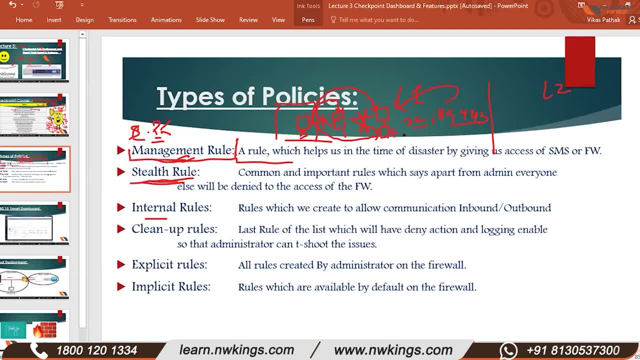 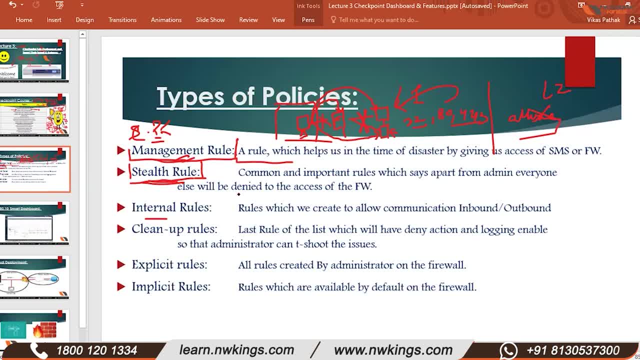 Is it clear? After that comes internal rules. Now, what are internal rules? All the rules which you create on the firewall- Allow, deny, drop, bypass, whatever you create- All of them are called internal rules. Then comes clean up rule. 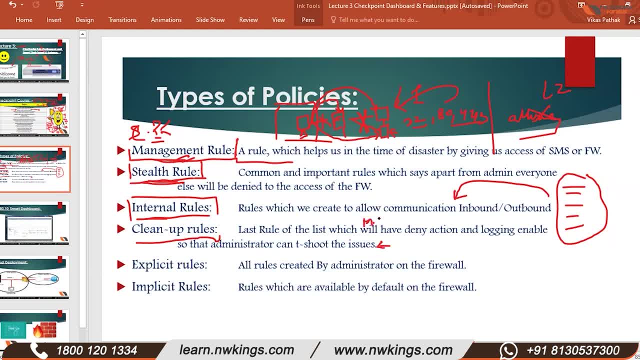 Clean up rule is most important rule. when I say in check point terms. Why? Because most of the troubleshooters You will have troubleshooting, It will happen because of clean up rule. Why? Because what you will do, Assume that you have made 1000 policies. 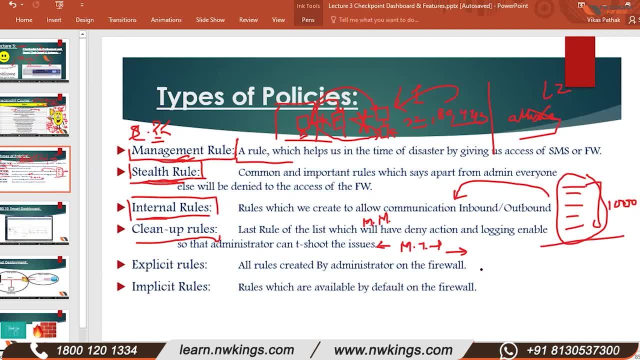 Okay, In the last policy you will configure Which will be source: any, Destination, any And action: deny And drop. So in logging you will do log enable. What will you do? Log enable, So whenever any new traffic comes? 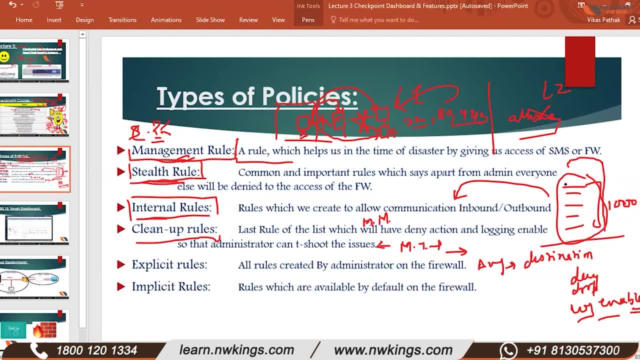 It will go down with all these rules. If it does not match any of these rules, Then it will drop by going to clean up rule And log will be generated. So if your traffic is dropping by going to clean up rule, That means you do not have any rule on the firewall. 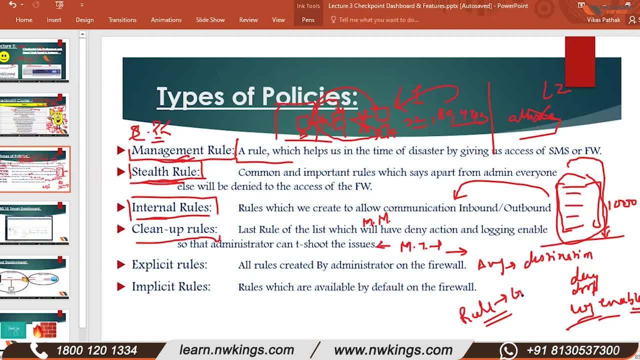 For this source and destination, You need to create one. And if If you already have traffic Sorry Rule is already on your firewall, Still you are getting hit by clean up rule. In that case you need to troubleshoot What is going wrong with your firewall. 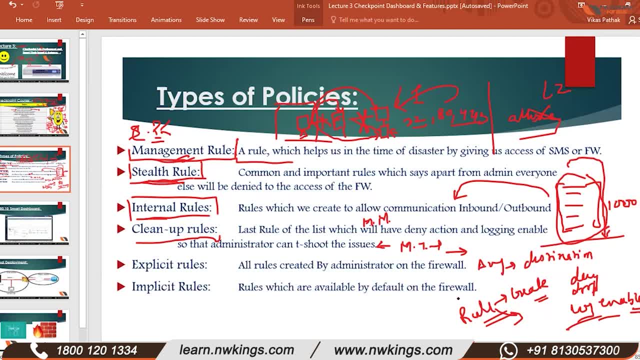 Like now Sanchit was explaining. What was Sanchit? That non-standard port was used. What was that, Sir? not inspected type used, Not inspected. Not inspected type port was used in the rule. That is why that rule was not being used by the traffic. 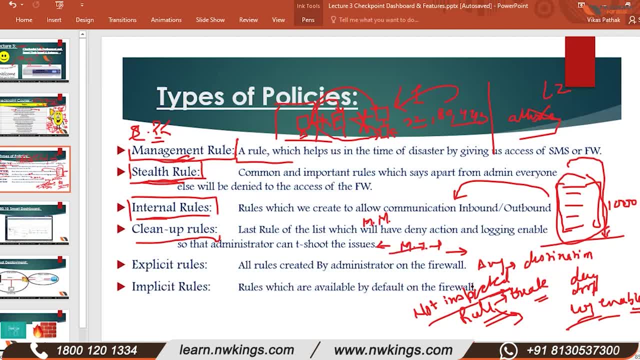 It was getting dropped with the clean up rule. Ok, So to understand this clean up rule- It is very important for you. Its working, as well as its concept. Now, if there is any doubt in these four rule types, Tell us quickly. 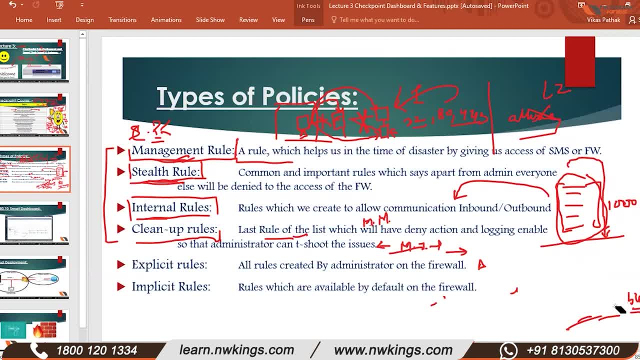 Any doubt, Shamsaad, Sir, first of all, you would like to know that. What is the rule And where is it created? on firewall, Alright, Ok, Yes, sir, See, rule stands for ACL, Stand for access control list. 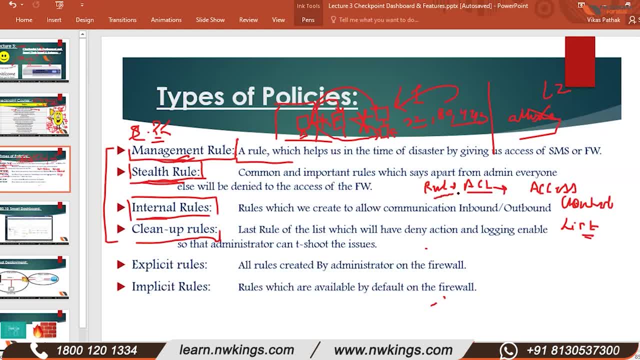 Ok, Now what is this? These are the rules. These are the conditions that we configure on firewall That traffic should be allowed or denied between source and destination. Ok, So these conditions that we make, That is called rule on the firewall. 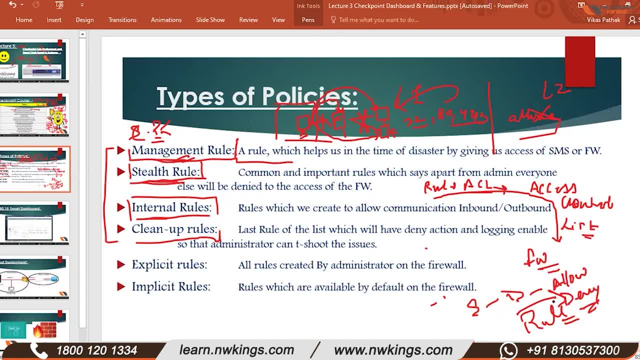 Make sense. Yes, sir, And where is it made? We will see that in a while in the lab. If you don't see it today, we will see it in the next lab. Cool, And don't worry, All these rules. 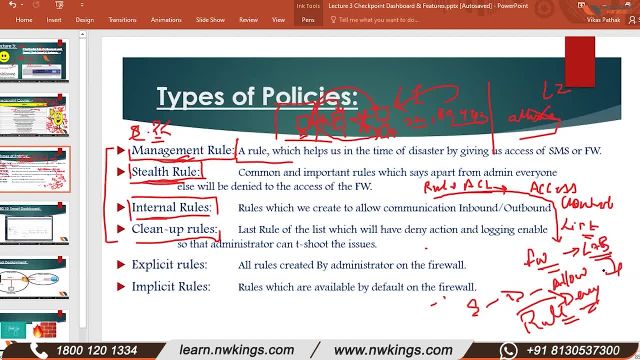 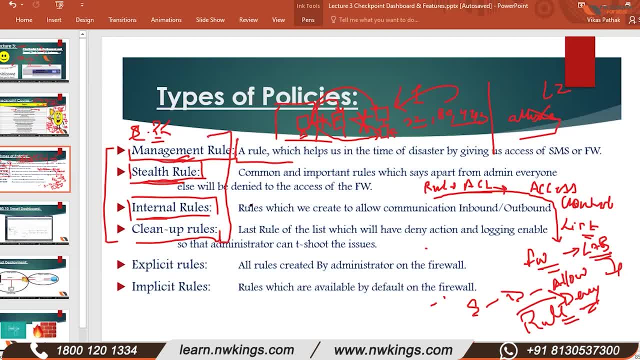 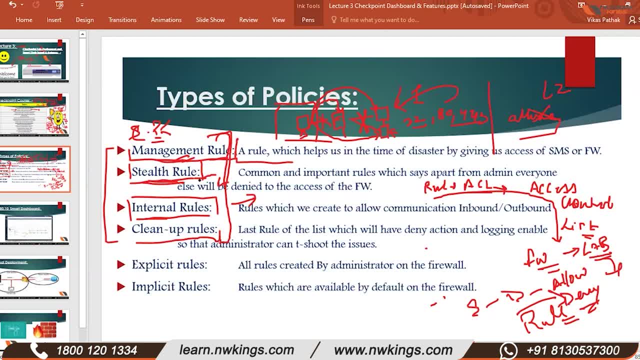 You will not get the order like. the first rule is the amendment rule and the second is the stealth rule. When you look at the policy section, by looking at the source, destination, port number and action, you will get an idea of what kind of rule it is and for what purpose it is made. 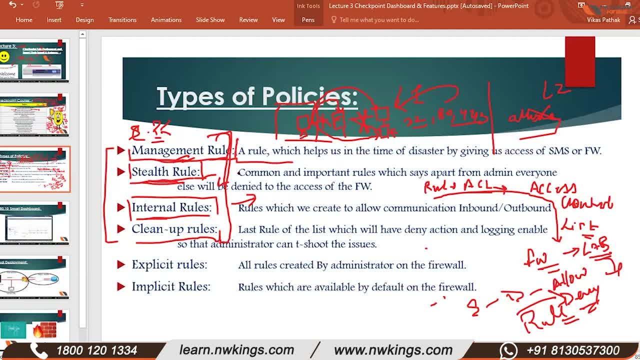 If, in an interview, sir, an interviewer asks me: please break the types of policy, what will we have to answer? These policies- management rule, stealth rule, internal rule, clean up rule- And I'm sure if you are going for L1, it will be asked from you. 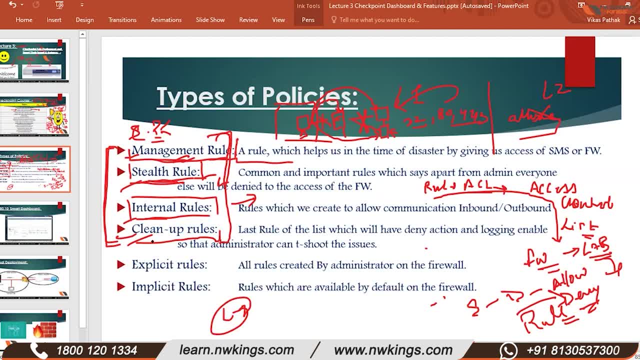 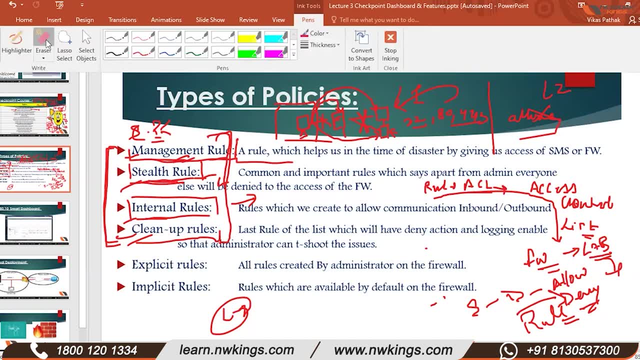 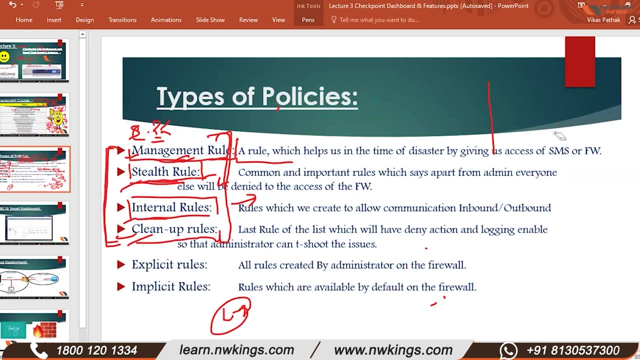 I'm sure, I'm 100% sure. Okay, Any other query Now I will tell you at what level what question can be asked. So at what level you are, accordingly, you can ask- Please pay attention If you are going to L1 or L2, types of policies, management rule, internal rule. these things can be asked from you in the interview of L1 level. 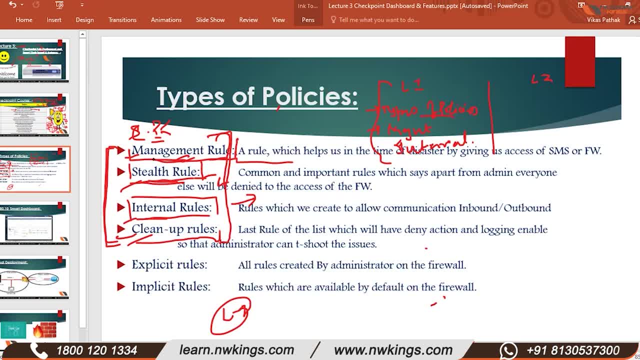 So when you will ask the policies, you will tell me then it may be the same thing from you- that what is the management rule, what is the stealth rule, what is the internal rule or what is the clean up rule. So these things will be asked from you at L1 level. 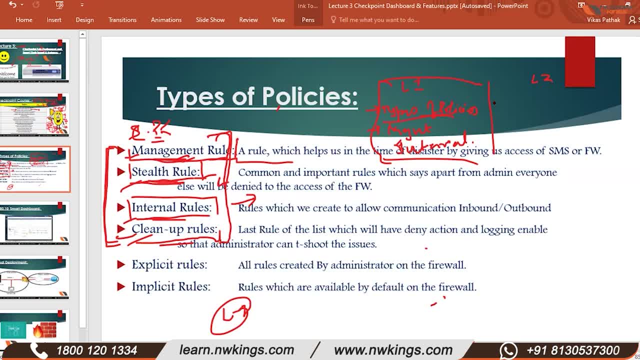 If you are going to L2, then no one will ask you the types of policy. this question will not be asked directly to you. what is the stealth rule And why we create? What is clean up rule And why we create? 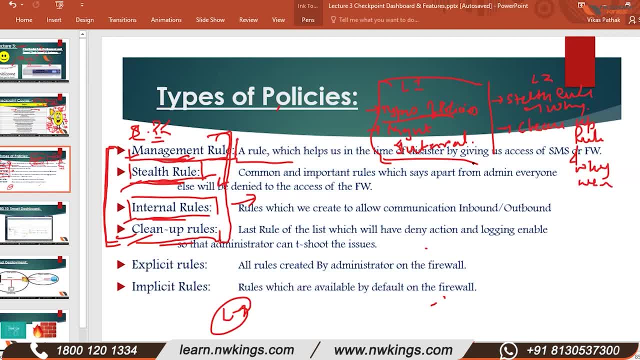 take a and again l2 pay. what is explicit rule? do you the rules that we will discuss right now explicit rule or implicit rule? okay, tell me one thing: you, like you are working now at the checkpoint, so you guys have noted that. I told you about 11 l2, so you guys have to focus on them a little bit. okay, one minute. 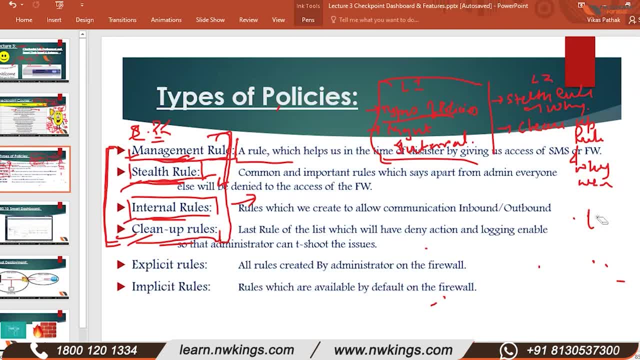 sir, I am done. please go ahead. sorry, I will call you next time. if you want, I can type it like that. sorry, I will call you next time, if you want. I will call you next time. if you want, I can type it like that again. no, no, no, no issues actually, sir, I make notes later. I make notes later. I make notes later. 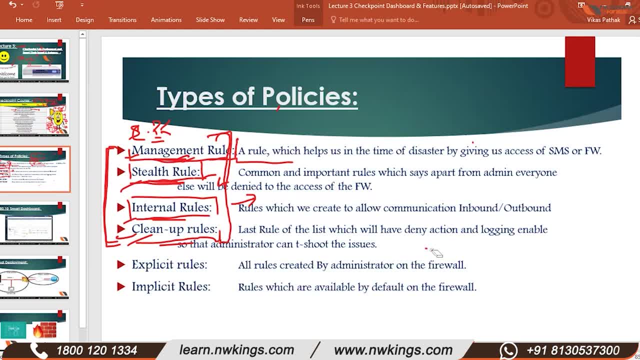 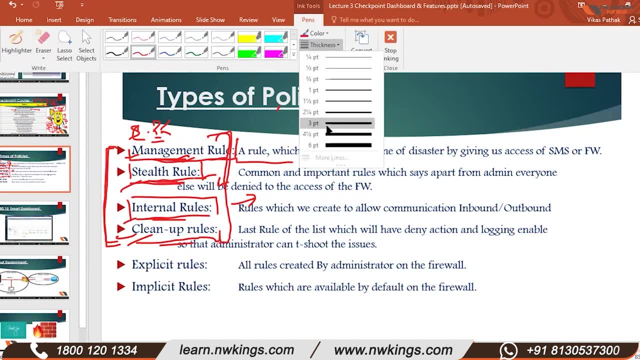 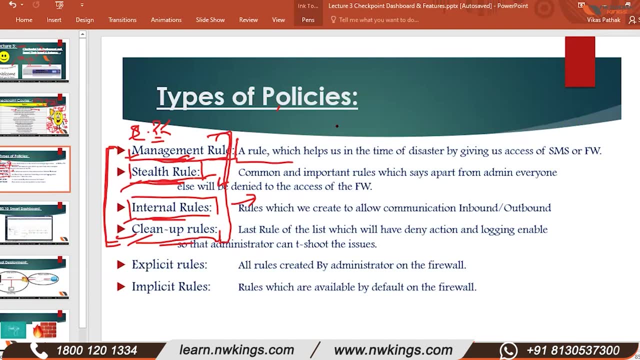 I also take screenshots. yes, that's also a cool thing. you know better approach, excuse me, sir. yes, please, these types of policies. which is this, as it will be a recording session, so I can make notes and write it myself on the computer, right, yes, yes, yes, see this what I have written here. 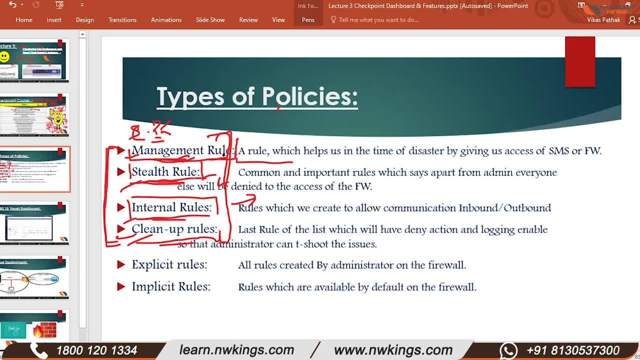 I have written the wording. do not copy paste it. write the management rule and then listen to what I have explained. write that explanation in your own words. Yes, that's what I was saying. Yes, Okay, Let's go. This is a weekly class, so I will go back for five days, so I will write my own words my half an hour, one hour, as soon as I get the time. I can do something by writing it in that world. 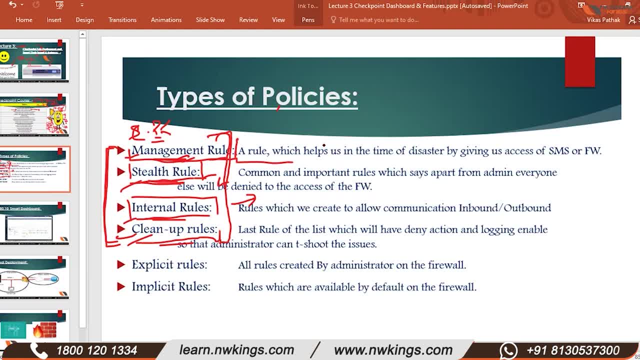 Yes, you can do it Okay. So, Sanjit, I was asking you. if you are working, then I think when you go for the next interview you will go for, I think, L2 or L3 plus right. 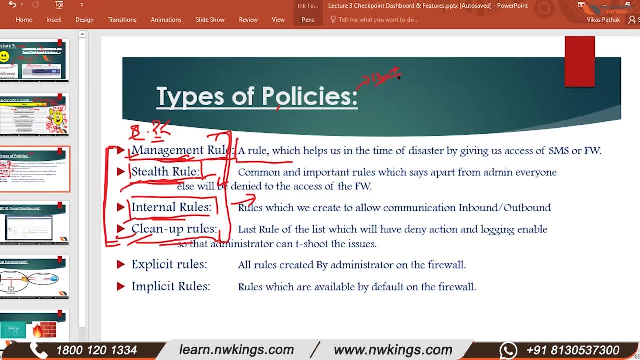 Correct L2 plus right Correct. There you will be asked a question that if we do not make the cleanup rule, then what will happen? Sir, this is still a question. Sir, this is still a question. Okay, So what is your answer to that? 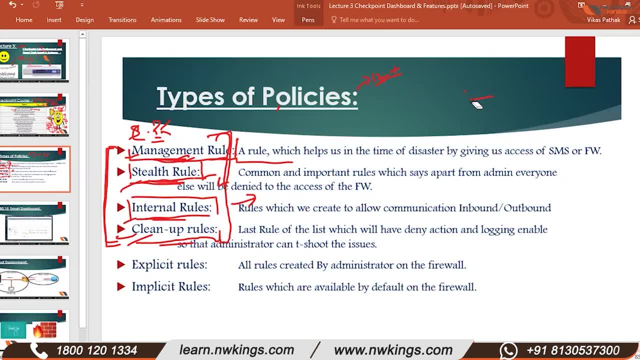 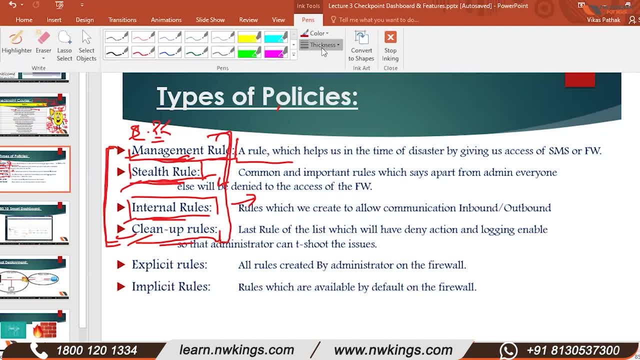 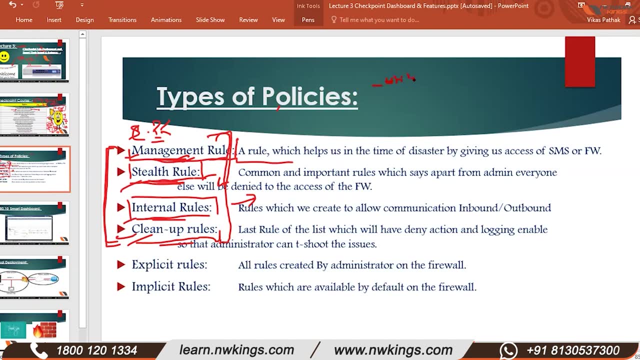 Sir, if we do not make the cleanup rule, then two things will happen. One, there will be an effect on utilization, as far as I have understood it, And second, the thing called zero trust will end. The concept of the next generation firewall is zero trust. 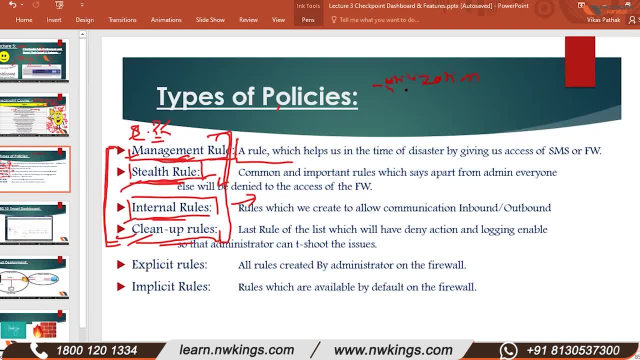 That they don't trust Because they have a cleanup rule, Because they have a cleanup rule at the end that no traffic is allowed from one end to other end, Because in ASA it used to work on security levels That trust to untrust is allowed. 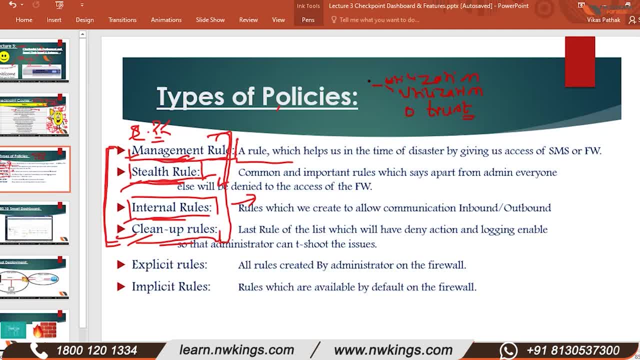 And untrust to trust. by default, traffic is not allowed, So that thing by default. whether it is Palo Alto, whether it is FortiGate or Checkpoint, these three concepts are of zero trust. Whether it is a land or a van, we will not allow any traffic until we have a security policy. 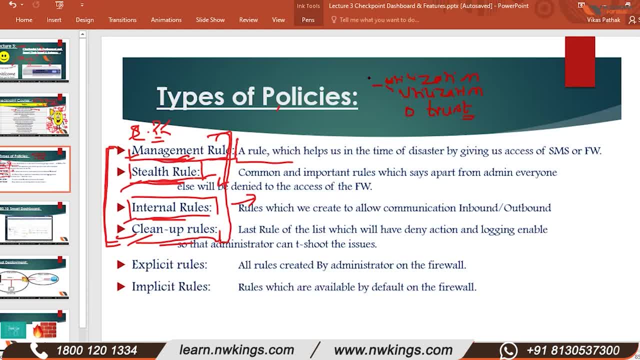 Otherwise it will hit a rule And this rule is a type of an implicit deny. This cleanup rule that we are making, Yes, Okay, I think I am confused in the implicit. I am confused in the implicit or explicit deny. The cleanup rule that we are making is an explicit deny. 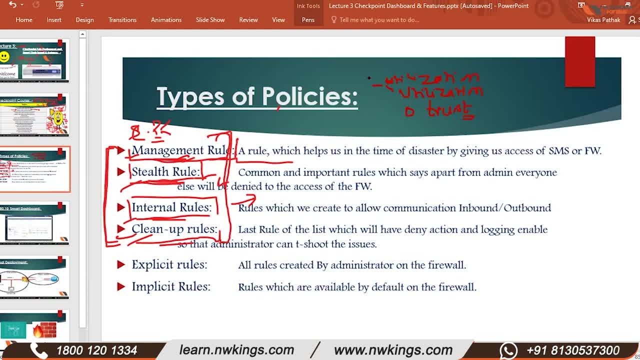 If there is no rule, then that traffic will be implicitly denied. Okay, So you are saying that if we don't make a cleanup rule, then that traffic will be denied? Yes, Right, So if we make an explicit rule, 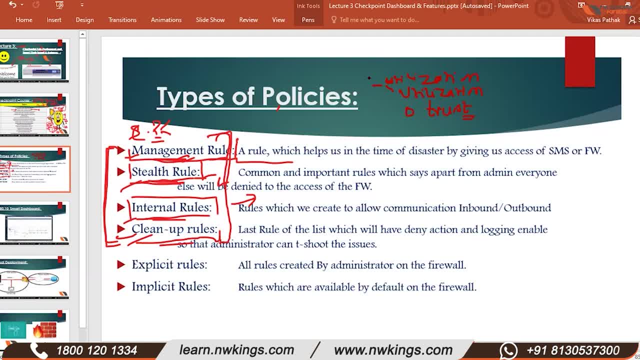 I mean sorry We don't say explicit or implicit now, Otherwise other people will get confused, So let's talk in layman term. According to the cleanup rule that we are making, we are defining that by default, traffic will be dropped. 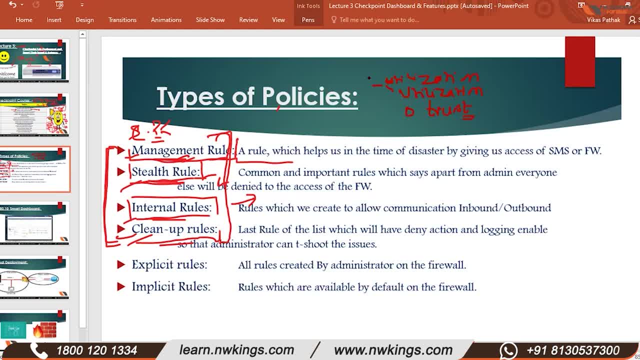 Yes, And if there is no cleanup rule, then by default, traffic is being dropped, Exactly. So why are we making a cleanup rule, Sir? because I don't know so much in depth in this, But yes, I compare this thing with ASA. 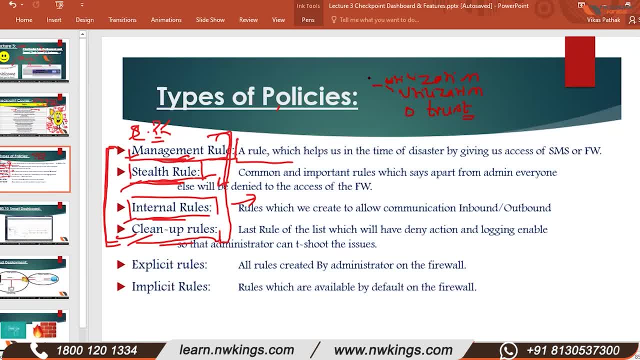 Because in ASA, as I told you, this was the concept that, by default, whatever is more security. what happens in that, In every interface, we give security level Sanjit, Sanjit. I would like to say one thing to you. 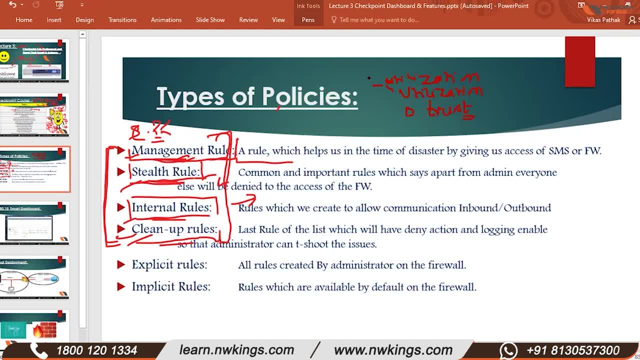 That you don't compare ASA with anyone. Okay, ASA is completely different, Exactly, Isn't it? ASA means I am saying: So, you compare it. Yes, you compare Palo Alto. You do FortiGate, do SonicWall. 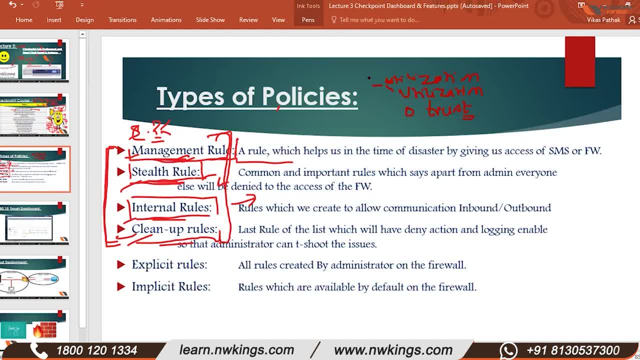 But don't compare with ASA. Concepts are very high and low, Okay. Secondly, you had reached up to 70%, where you should have given the correct answer, But due to no understanding, you were left with a little. I will clear that thing. 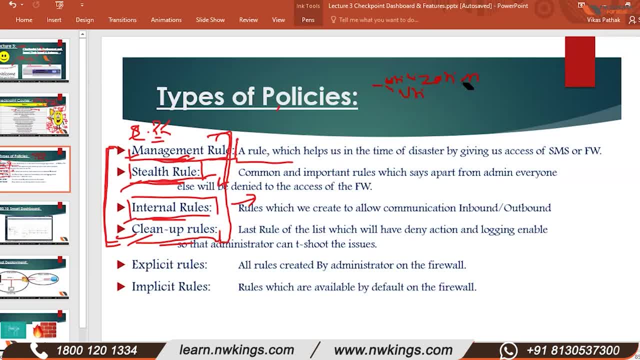 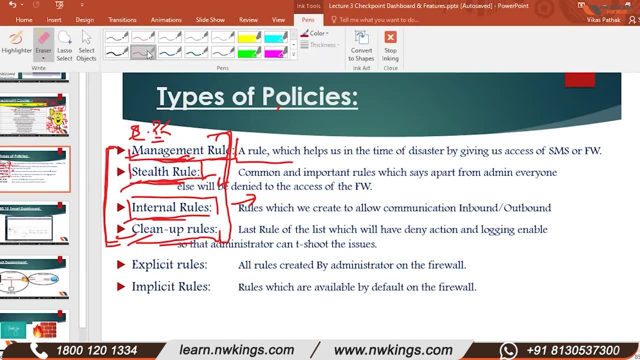 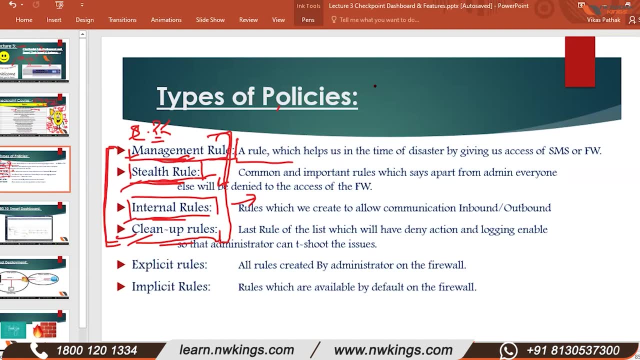 And I will hope that from next time you will give the perfect answer. The trust thing: Don't ever say this in the checkpoint. There is no trust concept in the checkpoint. If you relate it, the trusting will come. that okay, this is my DMZ zone. 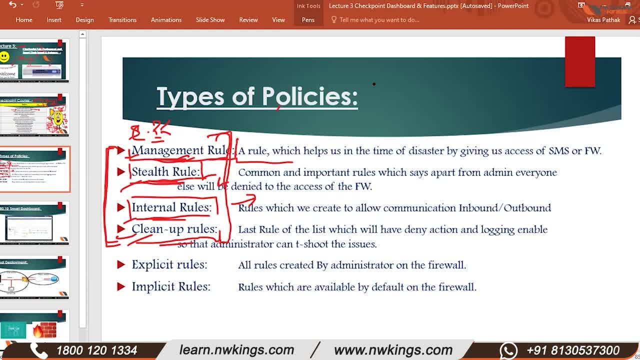 This is mine, But here we talk about no trust, Okay. So the first thing is: why are we making a clean-up rule? If the clean-up rule will not happen, what will happen? Okay, So the answer to the first question is that if we do not make a cleanup rule, then the traffic will drop by default. 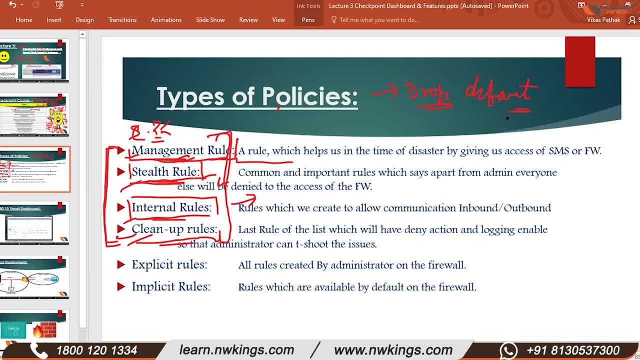 Guys, please note that by default the firewall will drop all the traffic. So if you do not have a cleanup rule, then the traffic will drop by default. So the next question is: what is the difference? If by default the traffic will drop, then why are we making a cleanup? 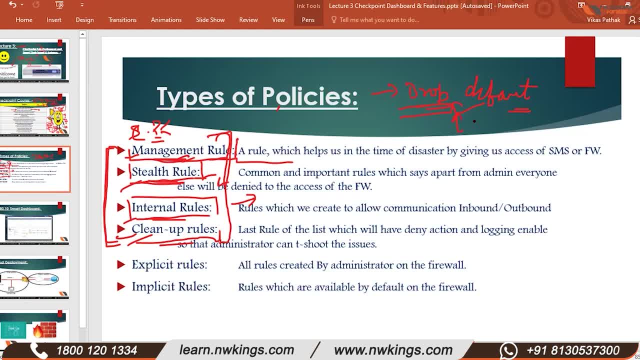 Because the rule of drop does not have logging in it. What does not happen? There is no logging. If the traffic is dropping by default, then it will not generate a log, Correct? And what are you doing in the cleanup rule? You are doing the same thing that source, any destination, any action, drop or deny. 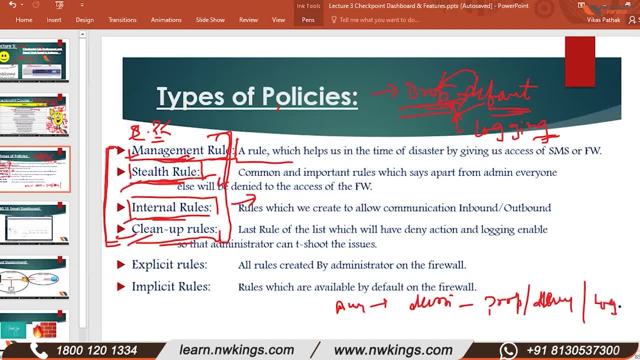 With logging And logging enable. If there is a traffic drop on this rule, then I will get a log, at least So that I can tell my user that this is either a new setup or something has changed in your source and destination, due to which no rule is hitting here. 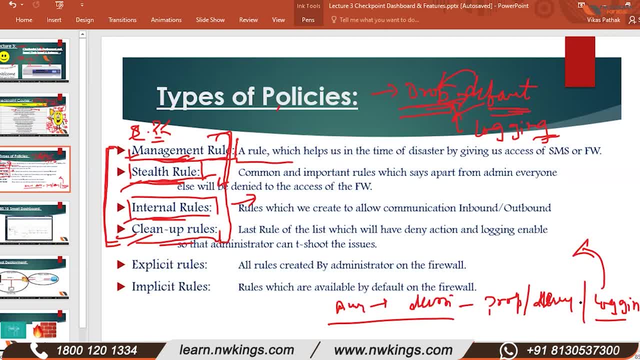 And you will have to make a request for rule creation. Make sense. Yes, sir, Guys, any doubt in this discussion? No, sir, Apart from Sanchit, Sir, I have one thought. Go ahead, Sir. a doubt in checkpoint firewall. 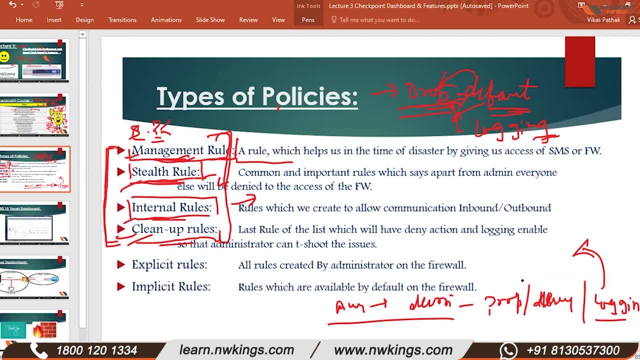 I am working on ASA. I don't know about the checkpoint firewall. In ASA traffic allows from higher security level to lower security level by default. So in checkpoint security level concept is not there in checkpoint. So how traffic is flow from one interface to other interface. 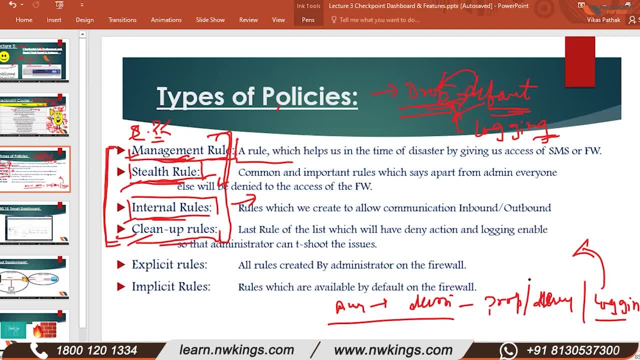 You make it flow, It is by default. it is not allowed By default. There is no concept of high trust, no trust and any trust, No, no. My question is this: But traffic, how can follow in the checkpoint? 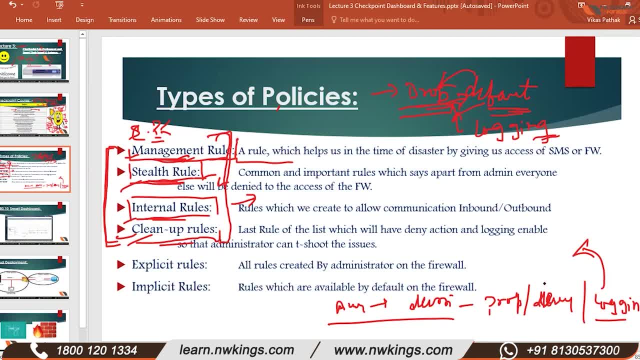 It has to match a security policy: Yes, If you want it to get passed by the checkpoint: Yes, You have to create a rule. Types of policy: Yeah, You have to create an internal rule, Okay. And if there is no rule? 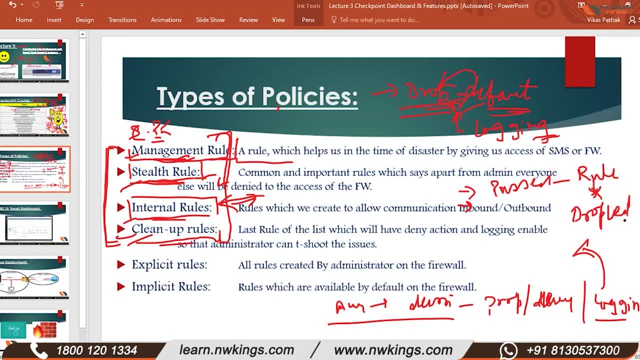 If there is no policy, It will be dropped. Packet will be dropped. Yeah, Okay, So in cleanup rules, cleanup rules. if we are not applying the cleanup rules, then by default packet will be dropped. But we are not able to find any type of logs. 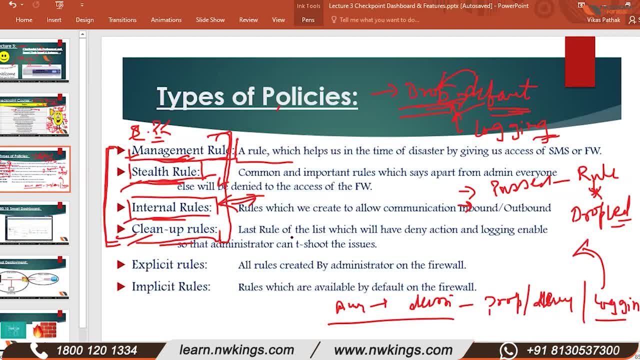 Yes, If we apply the cleanup rules, then packet will be dropped, But we are finding the logs. Hmm, That is the main difference, right? Yes, So can I note on my note paper? Yeah, yeah, You can note. 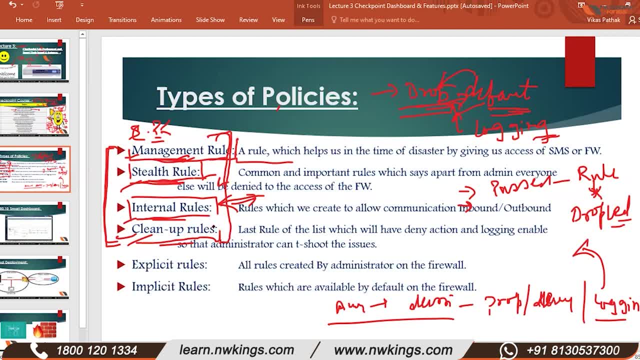 See, first of all, it's not rules. actually, It is not cleanup rules. This is rule. It is only one rule actually. Okay, Cleanup rule. It's my typing mistake, So cleanup rule and, by default, the behavior of the checkpoint is the same. 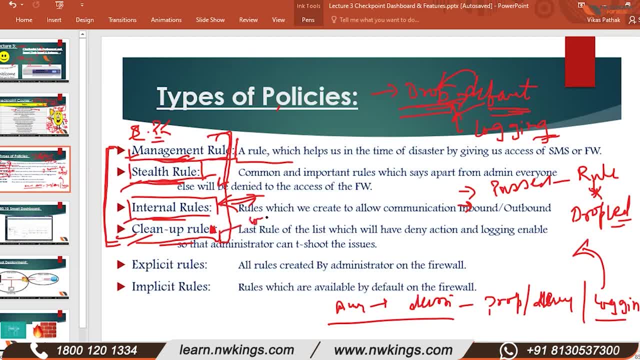 The difference is in cleanup rule we define logging- Okay, And there there is no logging. Okay. Cleanup rule, may we define logging and define logging? And by default, if we not applying cleanup groups, then automatically packet will be dropped and there is no logging. 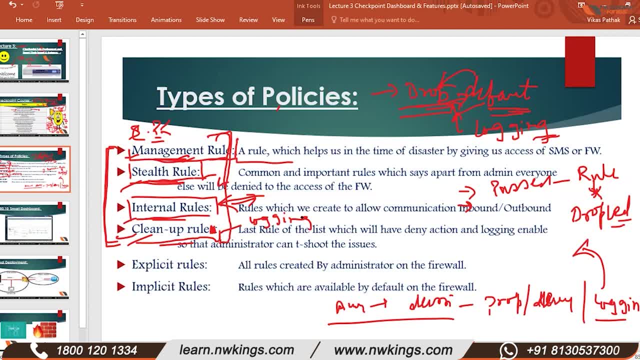 Yes, You will not be able to troubleshoot, Okay. Okay, Now let's talk about explicit rules and implicit rules. Explicit rules are those when you go to L2, then this will definitely be asked, or the difference will be asked. What are the explicit rules that the administrator himself makes on the firewall? 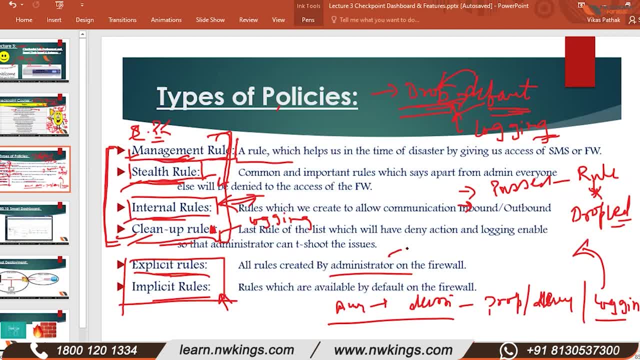 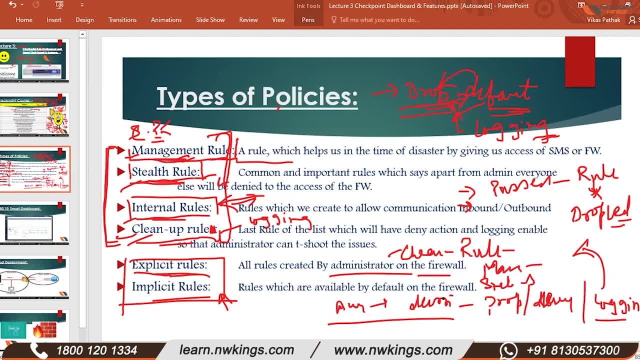 You made the stealth rule. That is explicit rule. You made the internal rules in one year. Those all are explicit rules. Make sense? Yes, And if you did not make the cleanup rule and the traffic is dropping by default, that rule is called implicit rule. 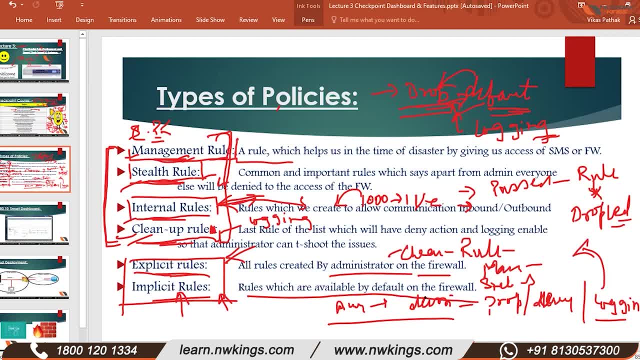 Those are by default in the firewall, Clear, Yes, sir, The notes you are making mention them in a very good way, And these two terms have to be clearly clear in the mind, because there is a lot of confusion. If you ask implicit, you will come after explaining explicitly, you will be disqualified in the interview and then you will say there is no feedback. 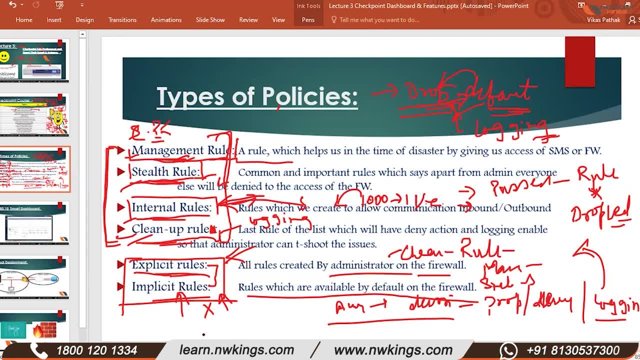 Okay, No, sir, Implicit rules. as far as I know, implicit by default policies are available in each firewall. That is the implicit rule. If we are changing and if we are creating any type of policy on the firewall, that it comes under explicit rules. 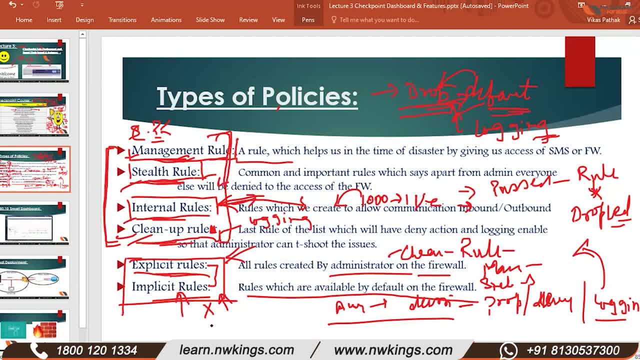 Yes, You are correct, And the cleanup rule will come in the explicit rules category or implicit. Yes, You are making the cleanup, So it will come in the explicit. Yes, Okay, Okay, sir, Any other questions? Okay? 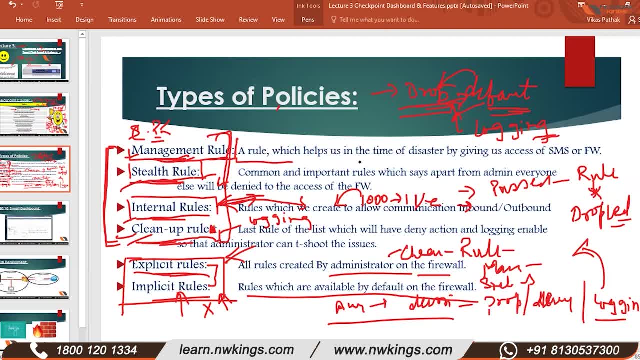 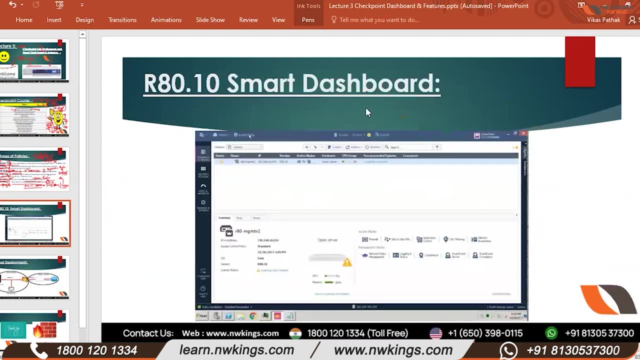 So I hope all these things will be clear to you, And next Saturday, when we will start the class, we will start from here. If you have any doubts, you can ask me. Okay, But please, you must revise. We will come to the next slide. 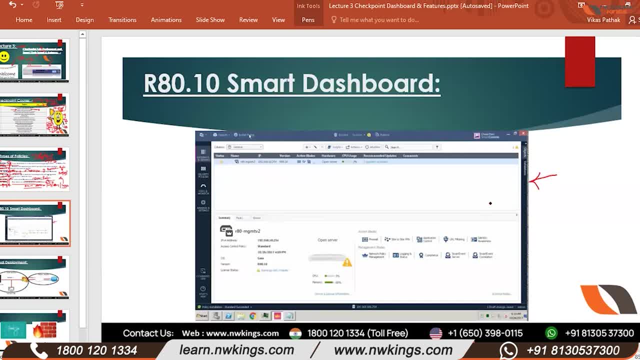 Thank you, sir. We will come to the next slide. Very good, sir, And the next slide I want to show I I'll explain. I'll tell you: See this dashboard and weather check. So when you will access SMS on client, then this window will come to you and this is the logo of Smart Dashboard, something like this logo has come. 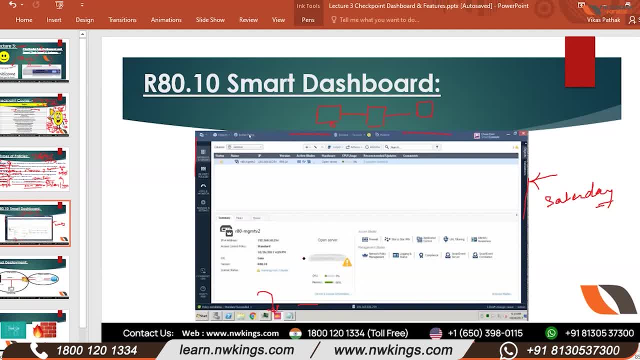 Now someone was asking me that: where do you create firewall rule? When you will access this dashboard, then this is the gateway and services. So here all the gateways, like there is a single gateway or there are two gateways which are in HMA. 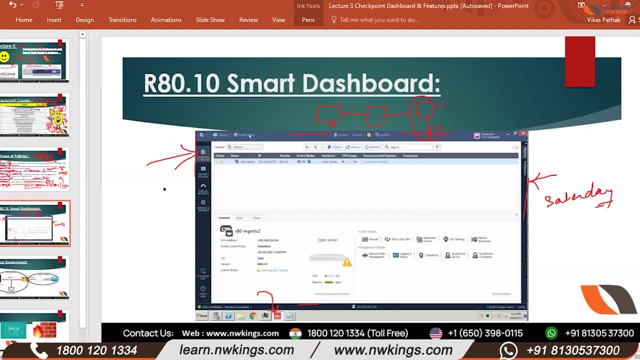 So you will get the information of these two gateways in this section. Second is policy: security policies. here you will go and define policies. Now I am telling you this for general purpose. In a while we will do its department and I will also discuss it. 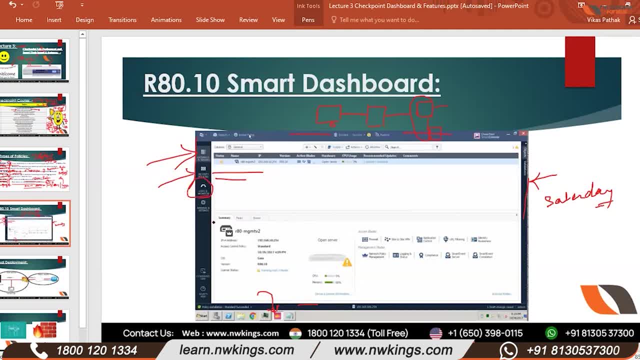 This is your logging feature And this is the settings, This option. from here you publish the changes and from here you install. As soon as you install the access of this management server from here, this policy will reflect on the gateway. Is it clear? 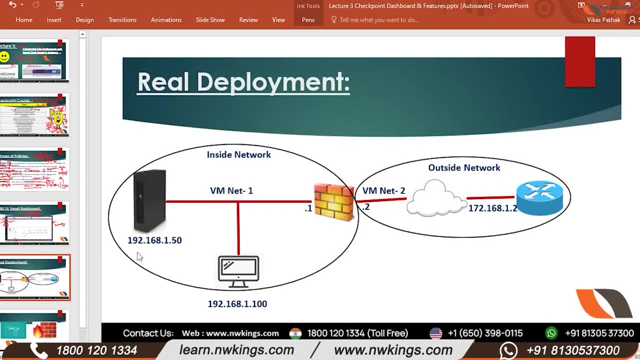 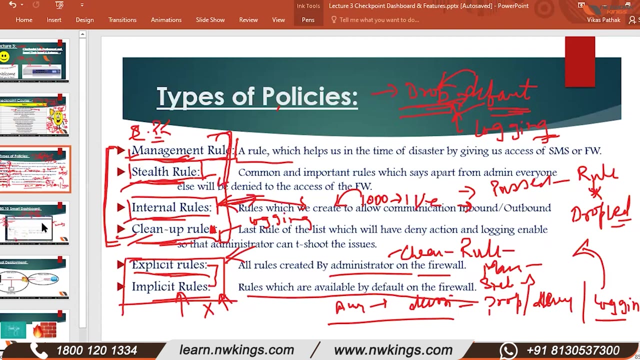 Same same. I think I have lost one slide. Okay, this is the scenario of the same lab. Now there was a section of 11 interview questions here which I think I have missed. I could not save it, So in the interview you can see all these questions once. 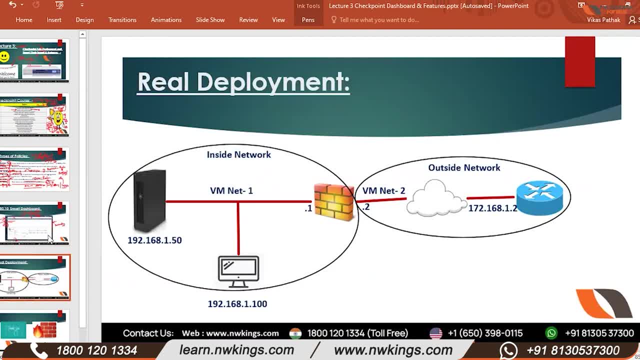 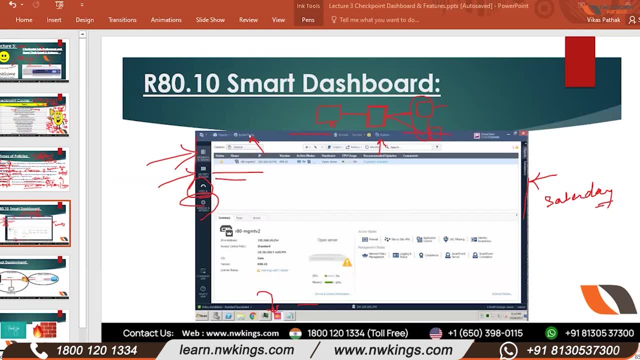 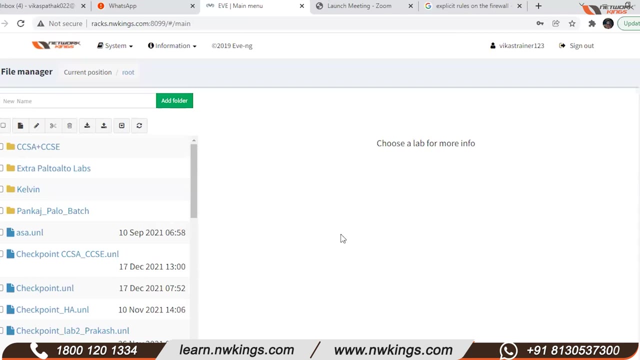 Now let's go towards our lab. Towards whom? Towards the lab. I will access it quickly. Do you see my EVNG screen? Negative, sir. No, sir, Tell me now. Yes, sir, I can see it. Okay, give me one second. 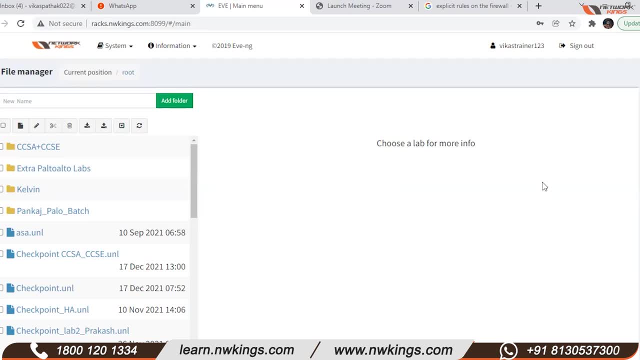 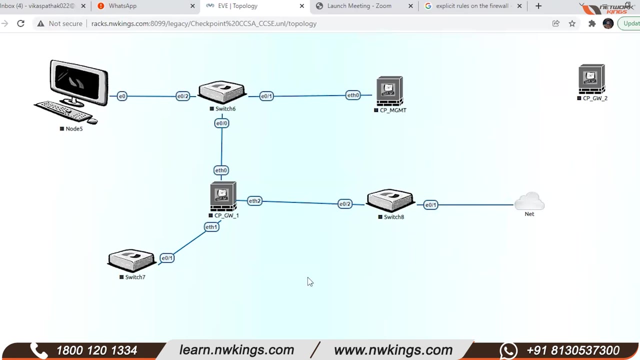 I will pick up my mouse. So you have found a lab like this, right? Yes, sir, Okay, So I have opened a demo. I have made a lab for you, Sir. this is the lab. this is the topology. So how can I configure it in my system? 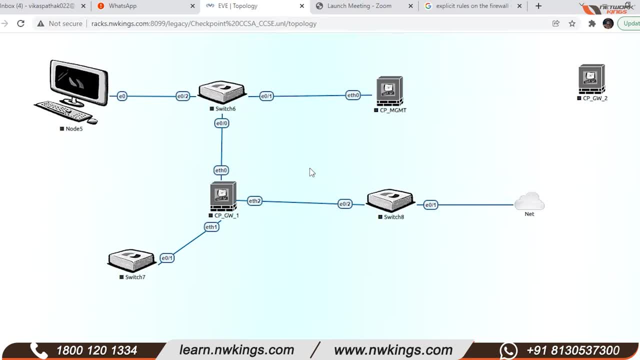 In the system means On the personal laptop. Will you do it on the personal laptop? Yes, we will do it on the personal laptop. So we have to be configured switch. We have to be configured gateway switch 6 management server on my system. 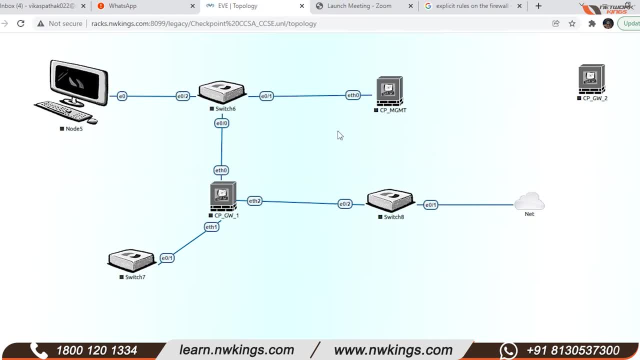 Personal laptop. Look, if you want to do it locally on your physical machine offline, if you want to do offline deployment, then you have to do it with VMware. So actually I have never done a lab in my personal system. Then how can I access it? 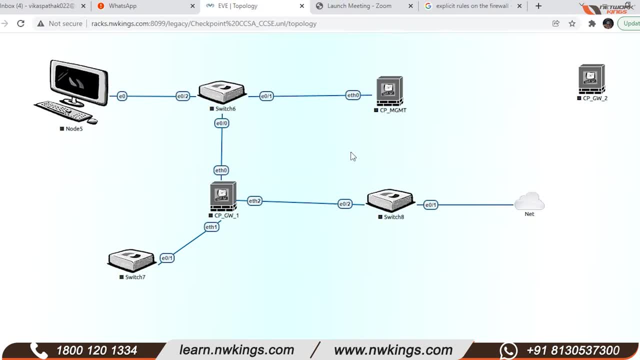 Do it like this: You have internet connectivity right, Yes, So the access you have got from EVNG, the lab you have got from networking, make a lab on it. You configure everything there. I am telling you how to do it. 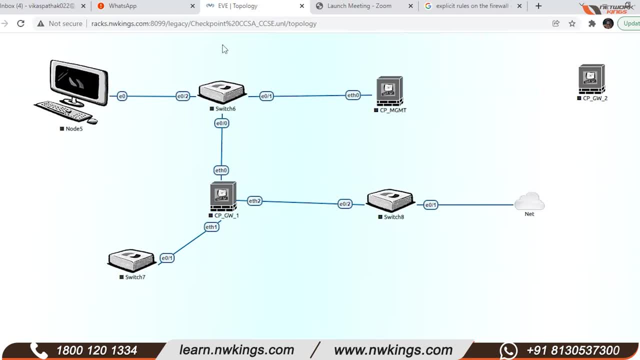 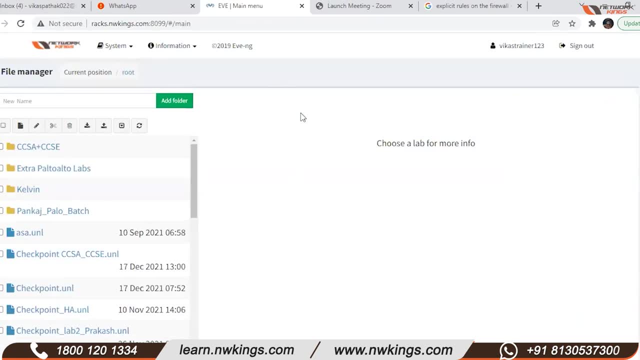 So this is the lab you have. Now. let's do one thing For now: let's close this lab. Okay, When you log in to EVNG, this type of dashboard will come Right. So where will the EVNG login be from? 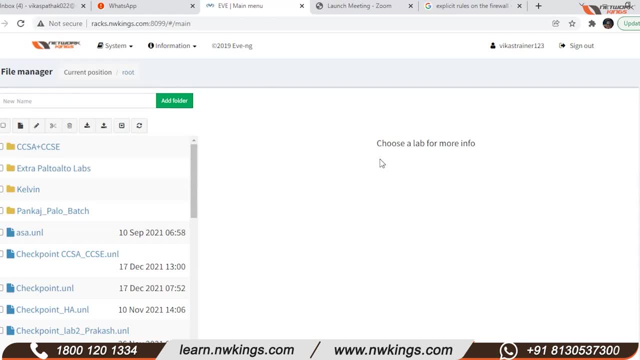 Will I have to do it from Google? Yes, you will get a link. You have got a link from networking, right? Yes, Click on the link, enter the username and password in it and this window will open for you. Of EVNG. 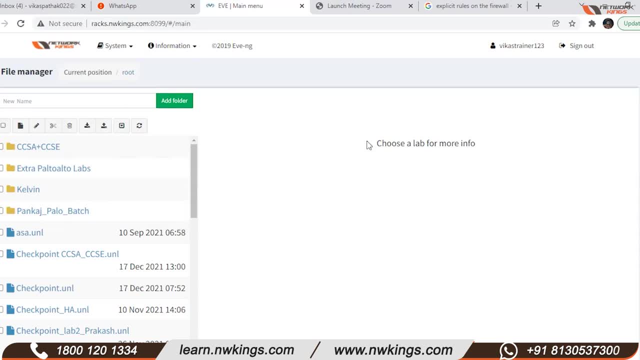 Yes, Is this the window of EVNG or this window? Yes, Racksnetworkingscom, port number 8099.. Okay, Okay, Yes, Okay, I have made this folder CCSA plus CCSE. Now it is not opening due to some reason- restrictions maybe. 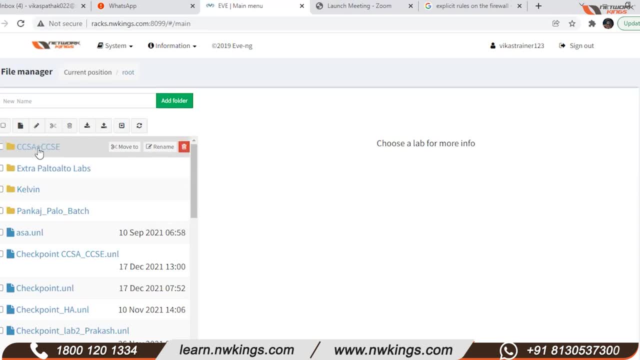 I will talk to Gaurav and get access to it And I will make sure that all our labs, all the labs, are stored in this so that you can take their reference in the future. Okay, Yes, Now what happens is that as soon as you land on this page, you have all these options. 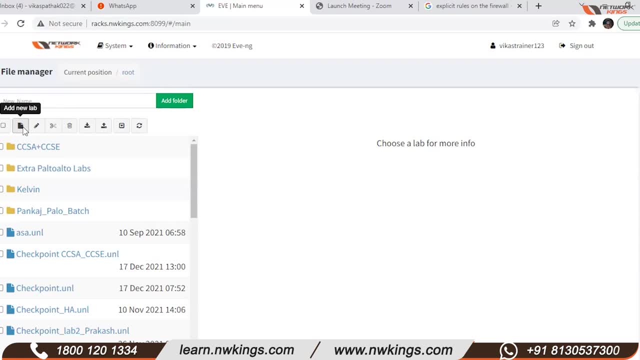 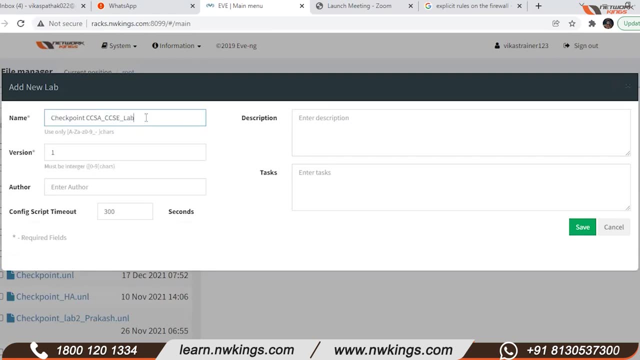 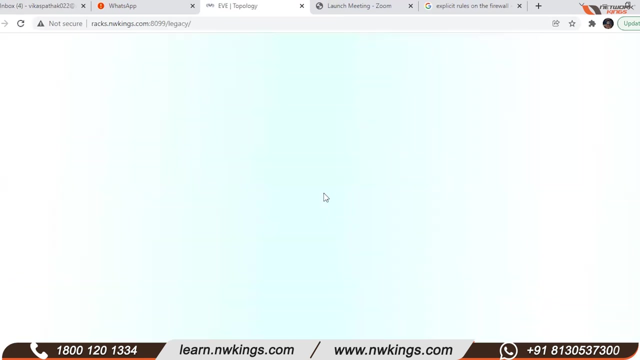 Right. Yes, Go to add new lab on this. Yes, Checkpoint, CCSA, CCSE, underscore lab, underscore one. Okay, Version one: author. Yes, I don't think we have this access Meaning to add this lab. Link has access, but we can't add lab. 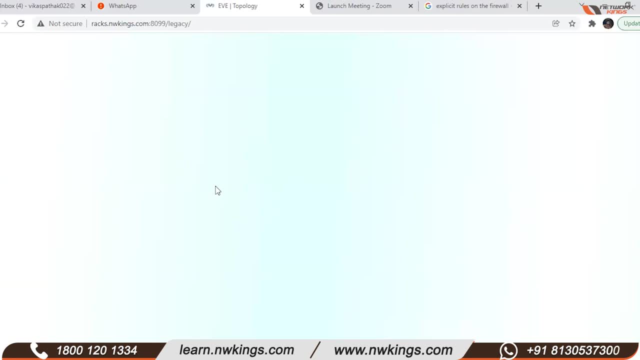 Talk to Gaurav once he will get access. No, He had said in the session yesterday that if you need any topology then let me know. We will provide you that topology within 30 minutes, But they will not give access to it. 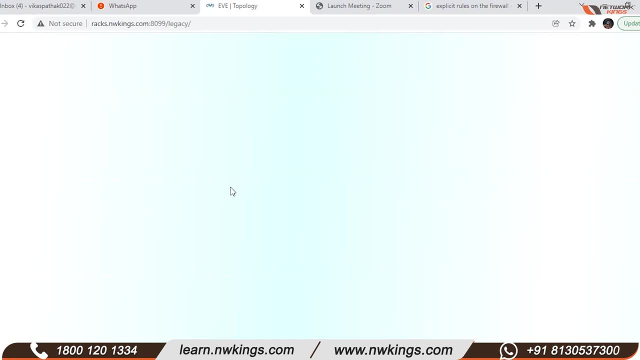 Of new tab of EVNG. Yes, Yes, They will give you a topology which will be required for you. Okay, Yes, Okay, If you get the topology, then what is the problem? You do configuration in it. No, No. 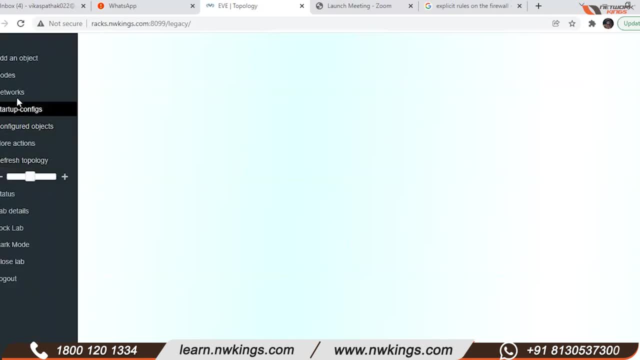 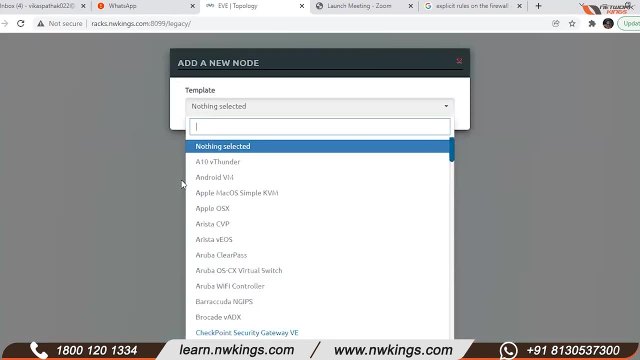 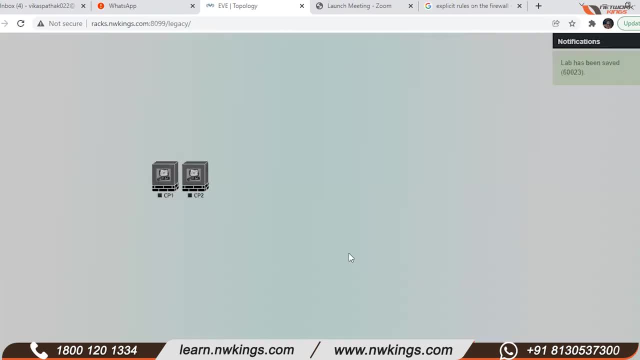 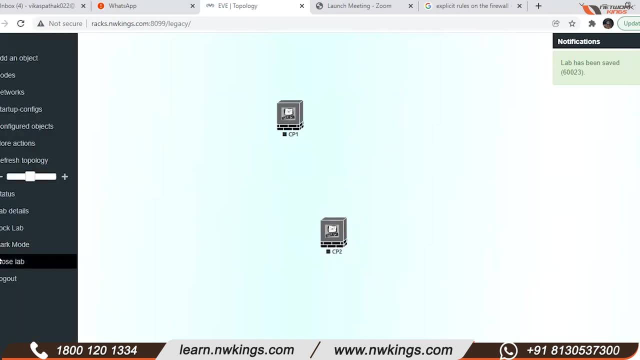 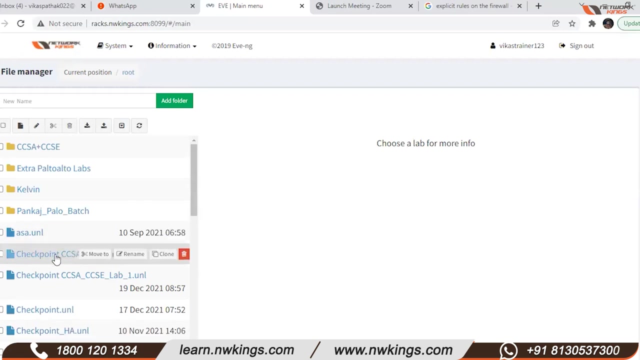 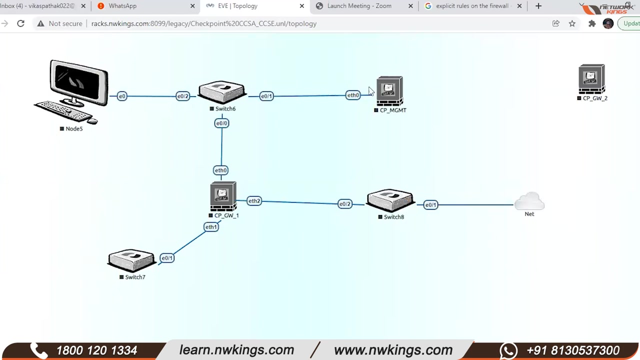 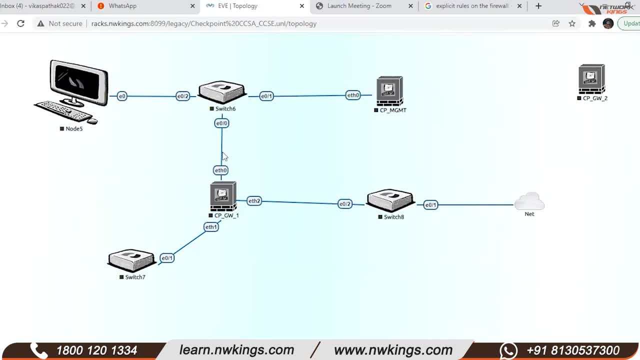 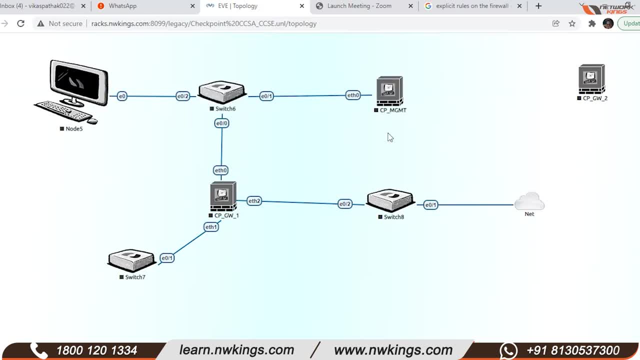 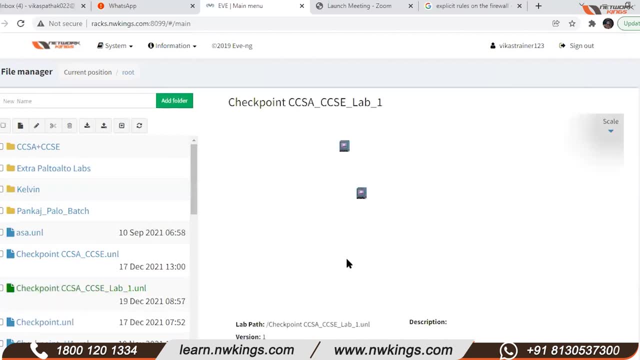 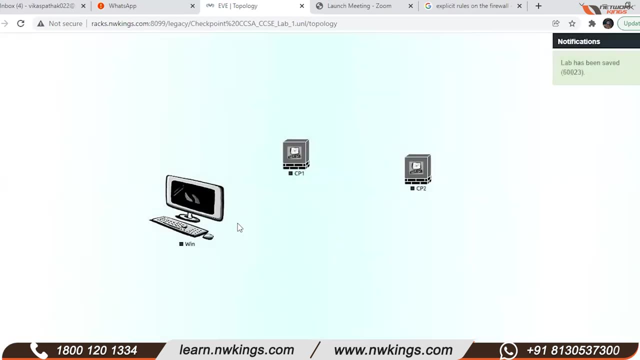 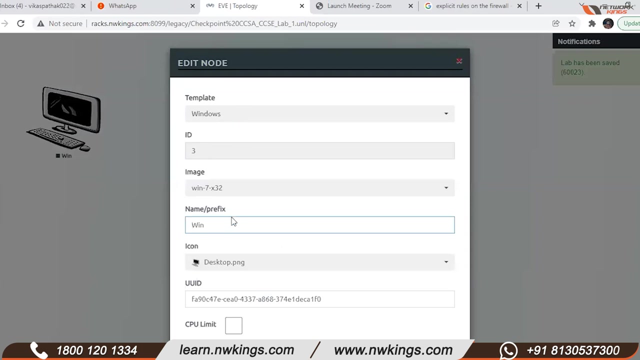 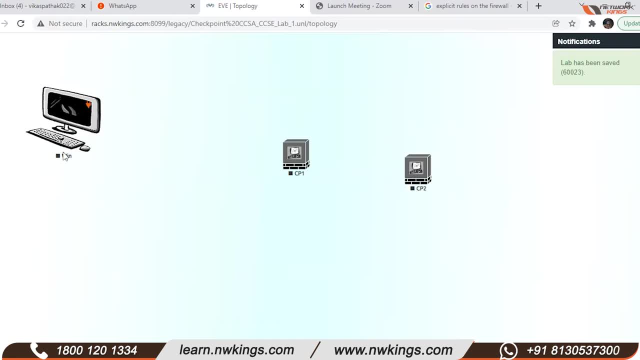 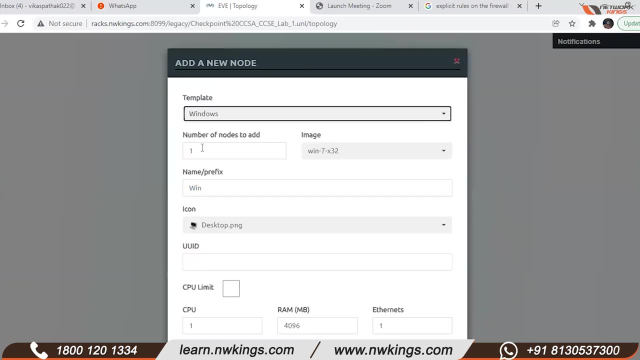 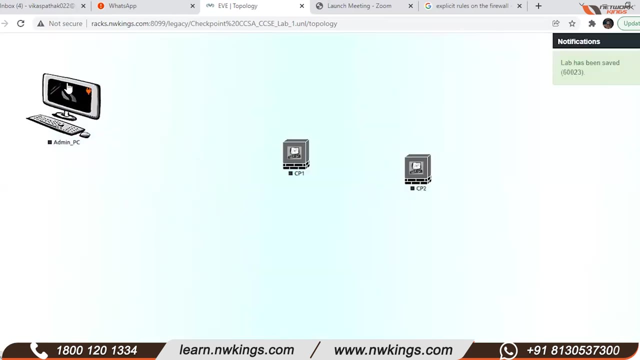 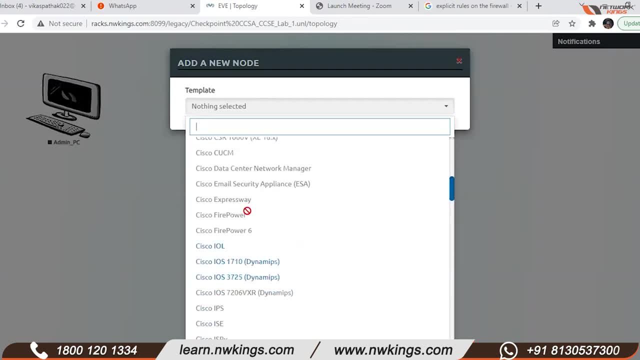 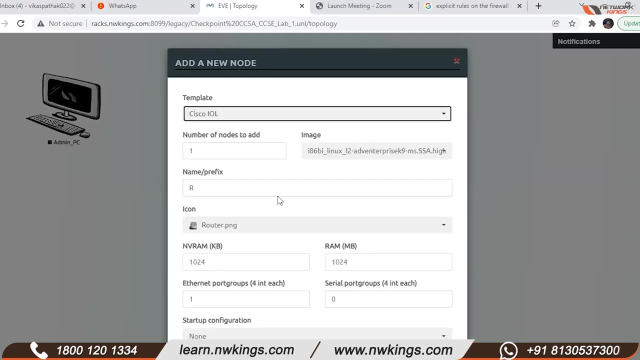 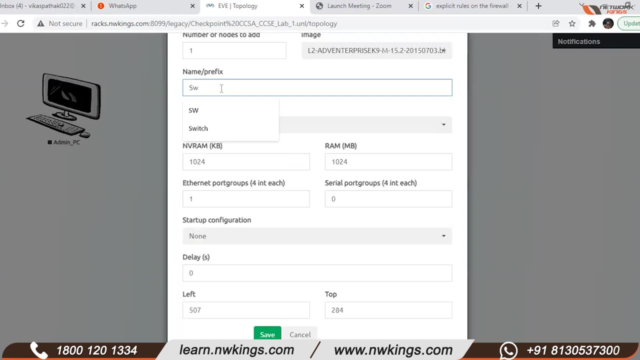 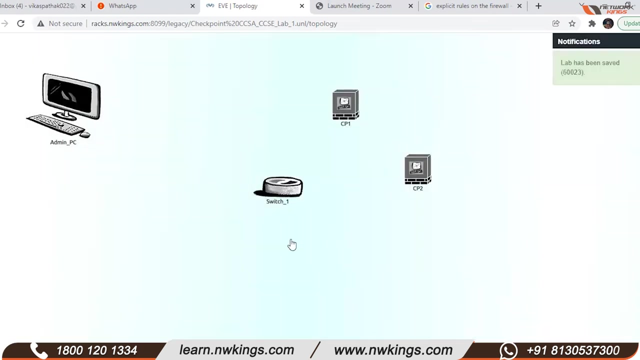 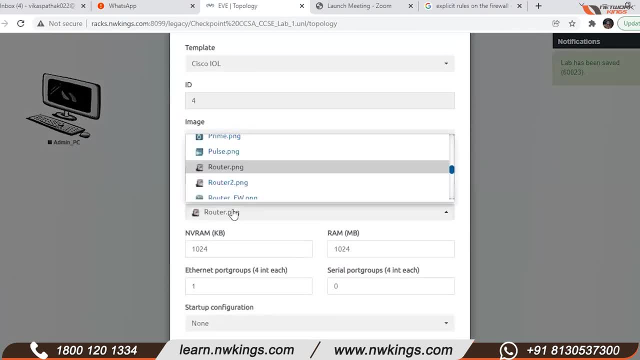 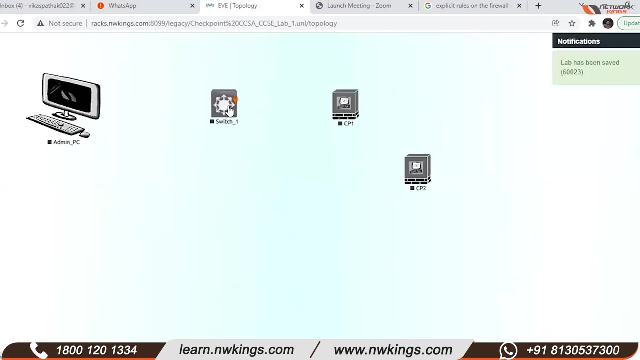 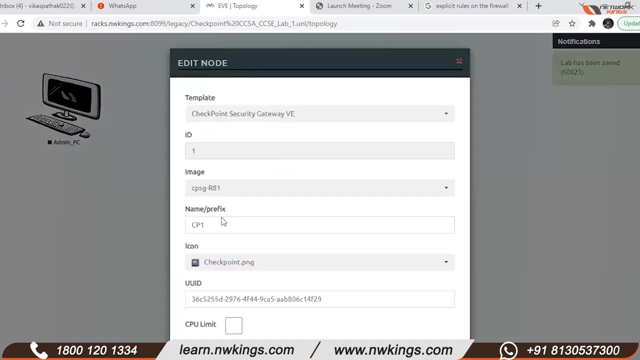 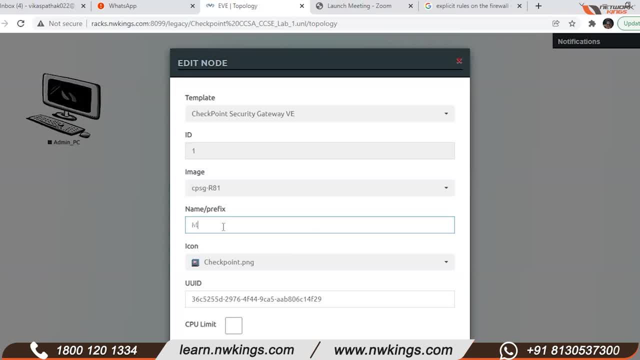 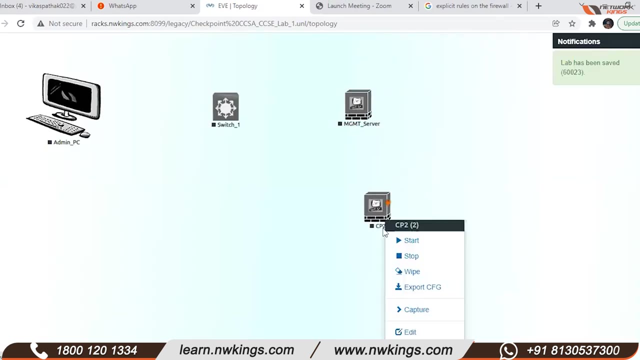 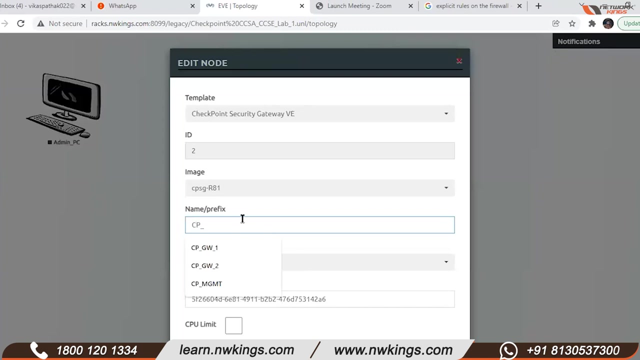 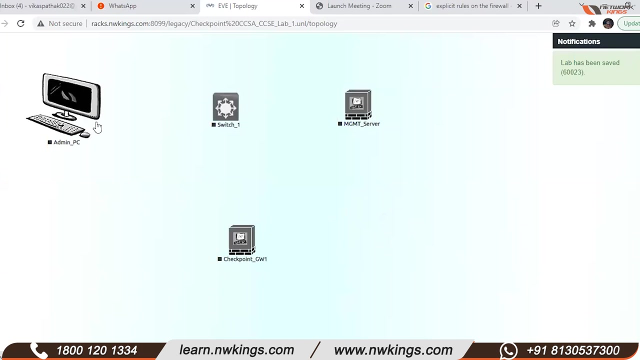 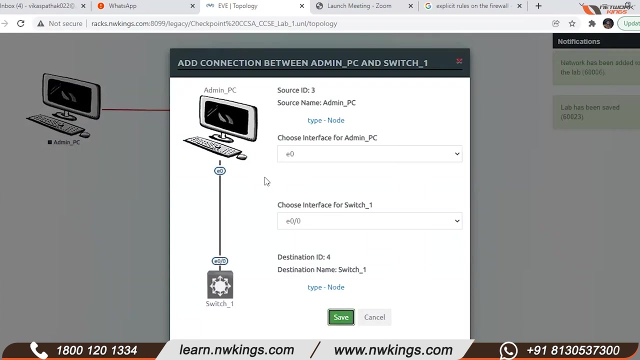 9-minute server: okay, and this is your edit: cp underscore gateway: okay. checkpoint underscore gateway one: okay, yes, I have made this first connection. after that I have made the switch connection. I have done ethernet 0 by 0, okay, I have done ok. after that, I have made this. 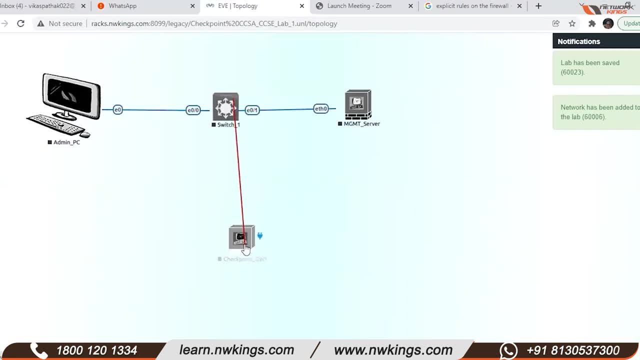 switch connection. This gateway is here. network 0 by 0, okay, Any doubts, Any doubts. Now, what do we do? Turn everyone on. Let's turn everyone on. Let's turn everyone on. Let's turn everyone on. 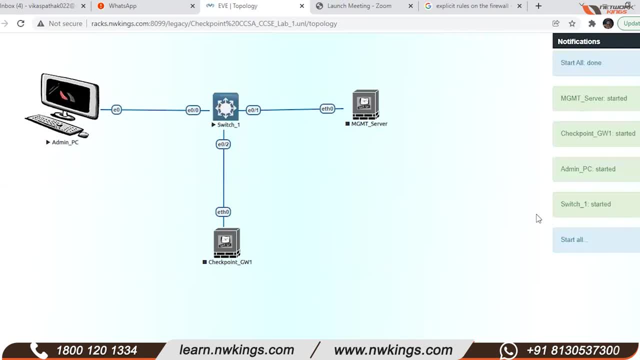 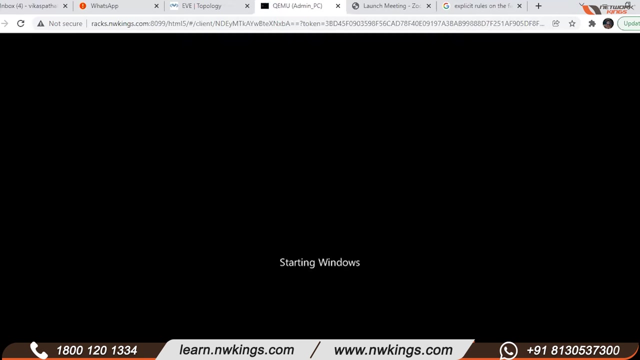 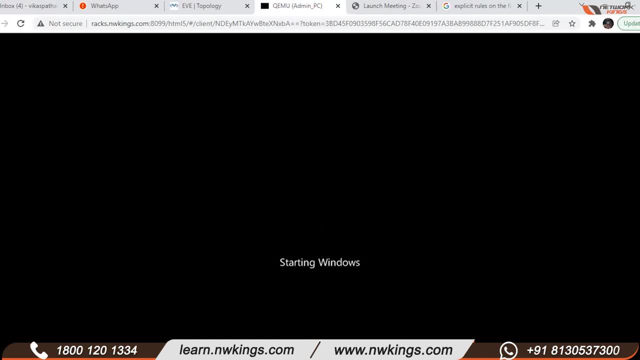 Normally the window starts. Now we can enter it once again here. You don't have to check. OK, MIts, OK, Yes, we have. Ok, Now we can enter. Now your window machine will be launched. Similarly, let's launch the server. 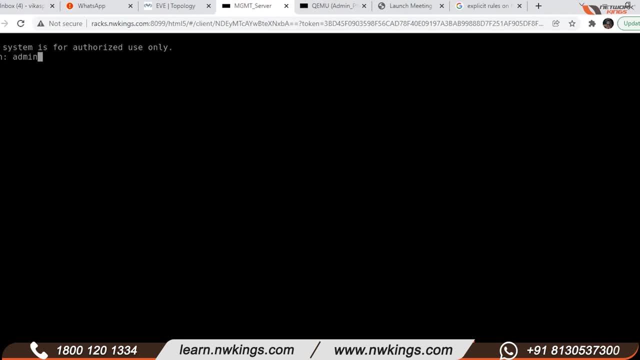 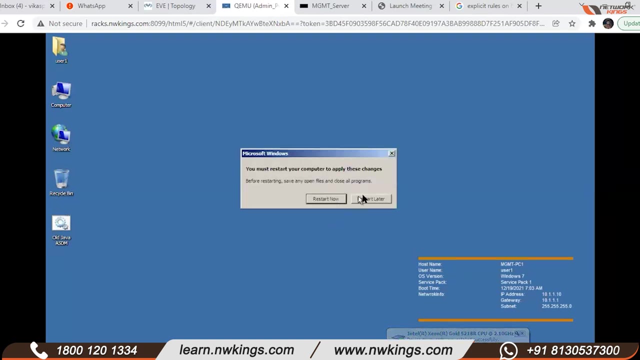 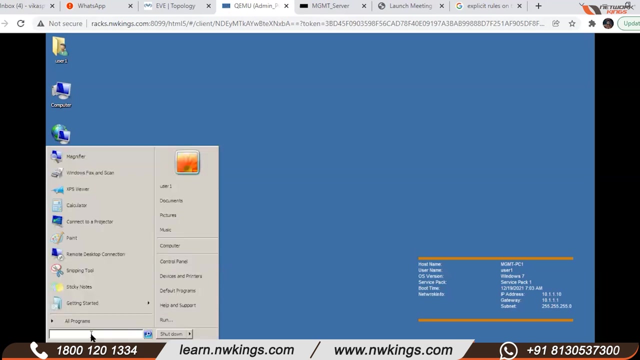 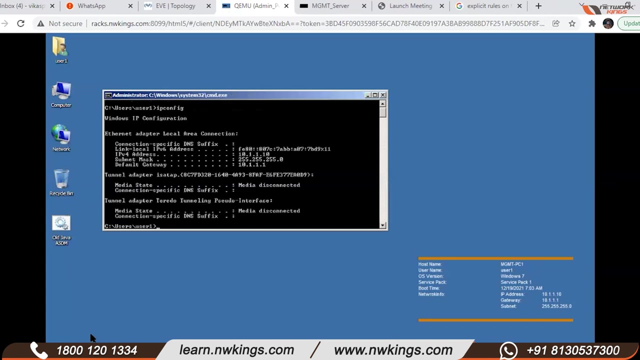 By default. its username is admin123.. We got access to the gateway. This is our management server. First of all, we have to go to CMD. We have to check the IP config. The IP config is 10.1.1.10 and the gateway is 1.1.1.. 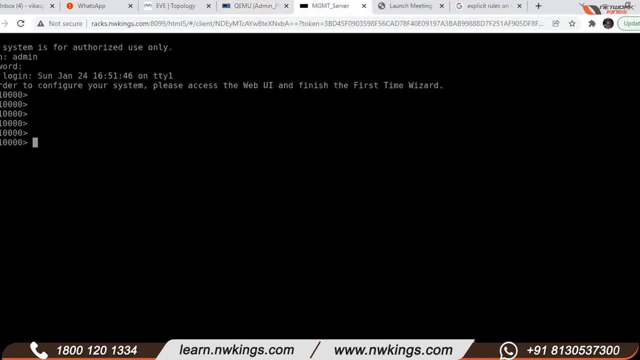 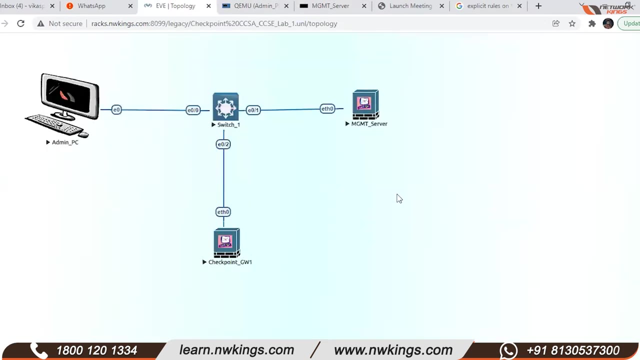 Now we will go to the management server gateway. We will check the show interface eth0.. Why eth0?? Because our firewall is connected to eth0.. Can you see it? Yes, That is why we have checked the configuration of eth0. 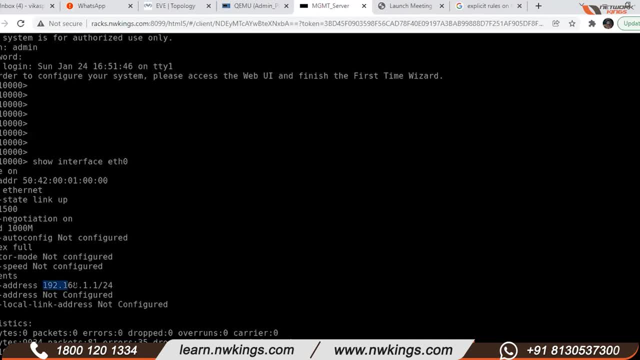 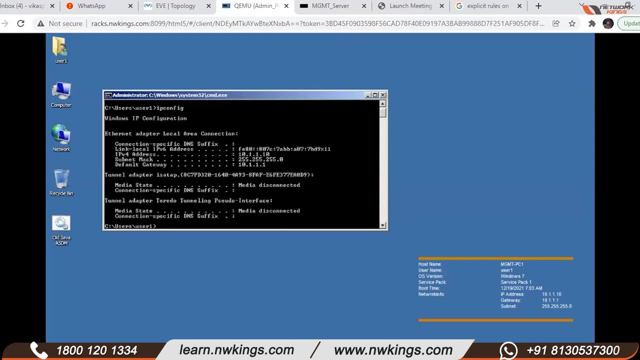 By default, the IP that is assigned to it is 192.168.1.1.24.. But you cannot access it through this IP, Either you bring this admin PC to 192.168.1.1.24.. Do you remember this topology? 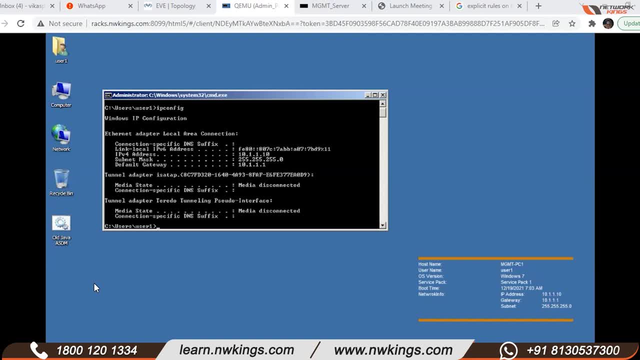 This one. If you bring your PC and the management server to a similar network and bring the interface of its gateway to the same network, then this network will be created and you will be able to access it. Right, So what we do is better than this. 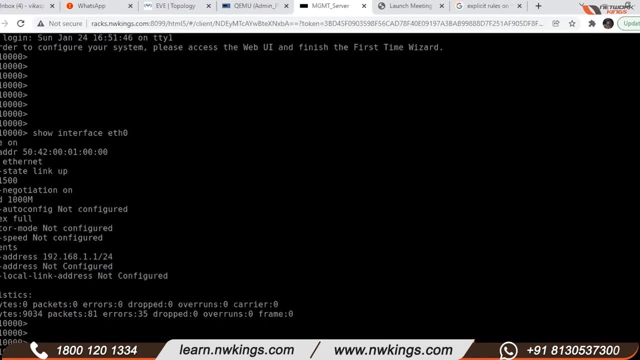 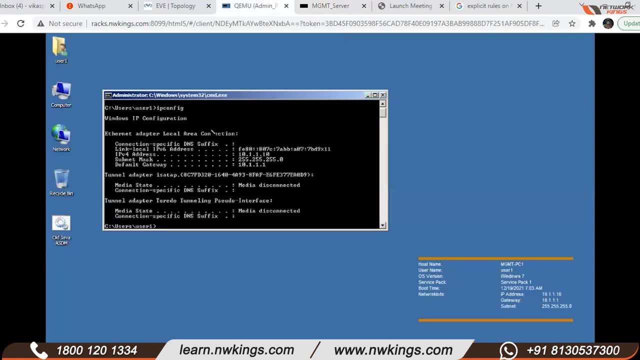 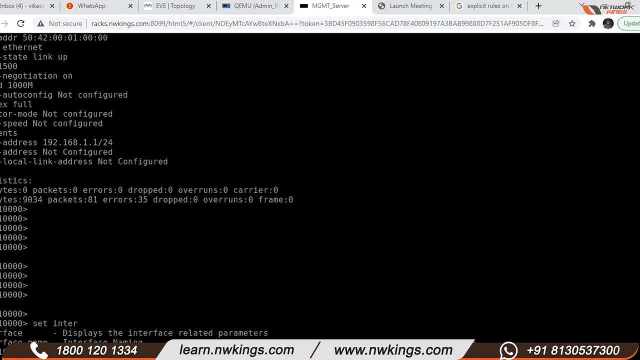 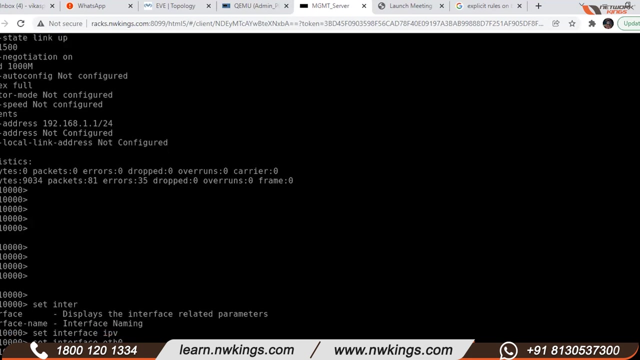 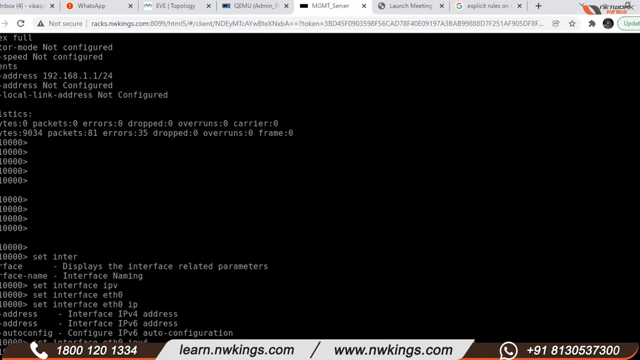 We go to our management server. Okay, What we do is that we change the IP of the series to the IP of the client. Okay, So what we will do is that we go to the management server, Set interface eth0- IPv4- 10.1.1.50.. 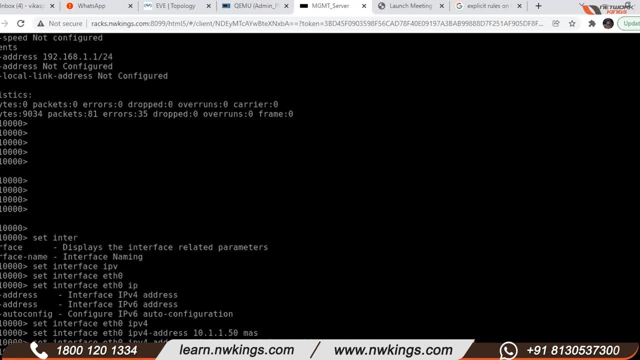 Mask length 24.. Okay, So what we have done is that we have said, through this command, that our eth0, on which our current IP address is 192.168.1.1, change its IP to 10.1.1.50.. 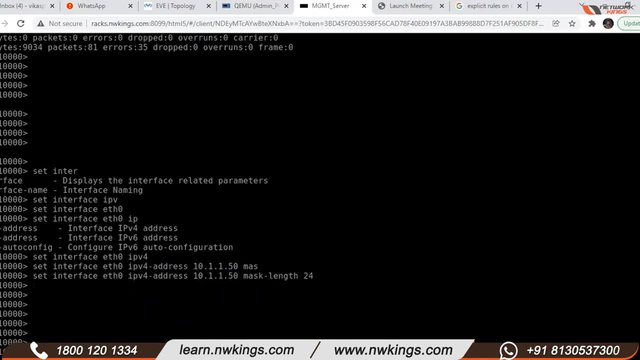 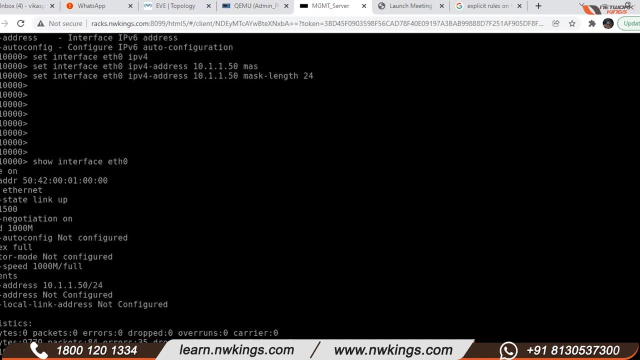 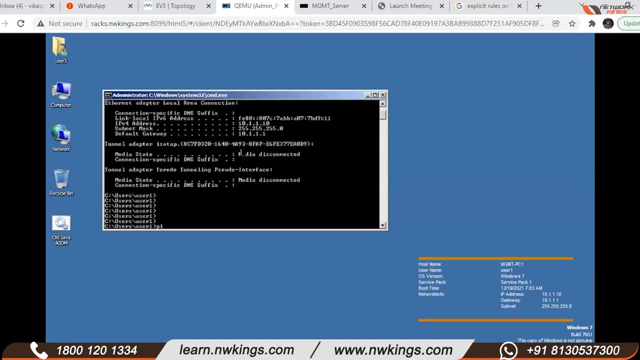 Okay, Now you have done the configuration. You can also check from above. If you do show interface eth0, then you will get this IP. Okay, After getting this, you go to your client. Go to CMD, First of all, ping. 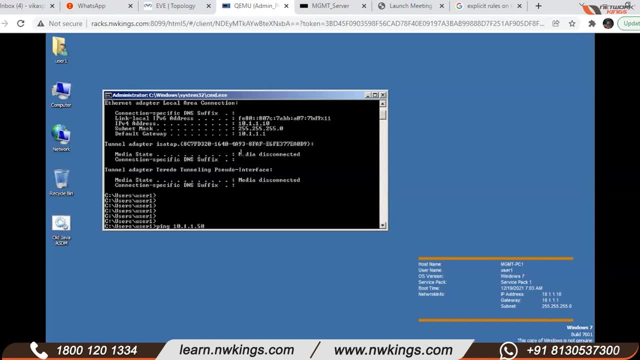 10.1.1.50.. Did you get the ping Now? is the story clear or not clear so far? This is the basic requirement to start the lab. Okay, This is the basic troubleshooting. Now, what many people do is that the IP of the client is in 10 series. 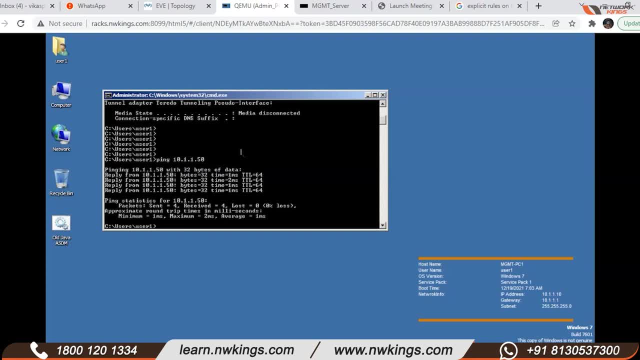 The IP of the gateway is in 192 series and they are starting to access it. The gateway is not being accessed, So until or unless you will not make it a part of your own LAN, you won't be able to access it, Cool. 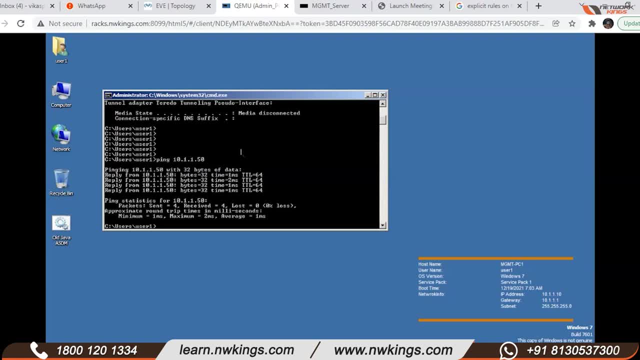 If you have any doubt, tell me. I am taking a pause here for two minutes. Sir, this is one dot. I have one dot. Just show me topology. This is sample topology. The same topology we are not building there. If you want to see the topology we are building, 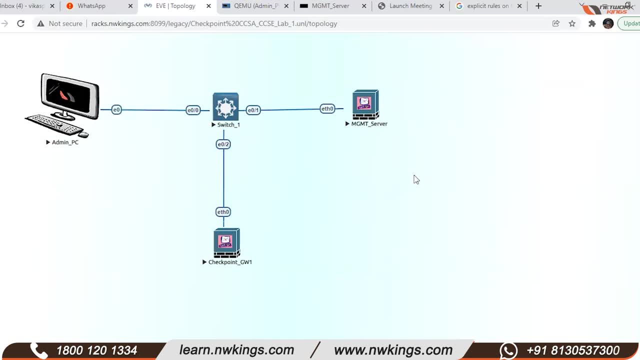 this is the topology we are building. So here the checkpoint firewall gateway is there and switch is connected to the PC and management server is connected. So that is my question. is that that is the three layer architecture? Yeah, this is distributed environment. That is the distributed environment because gateway is different place. 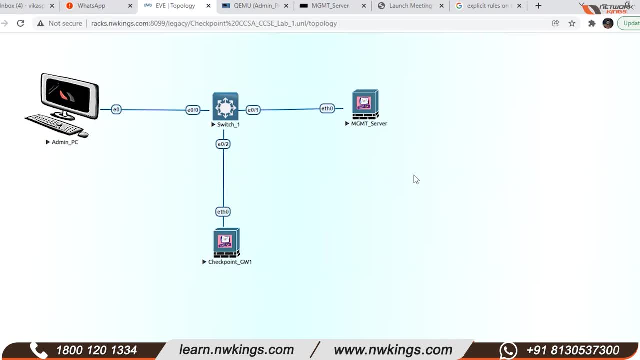 and management server is in different physical place. Yeah, yeah, Okay, Okay. So just that's why I asking you: Yeah, this is the distributed one. We will do deployment once, No problem, We will do standalone as well. We will do it in the next lab. 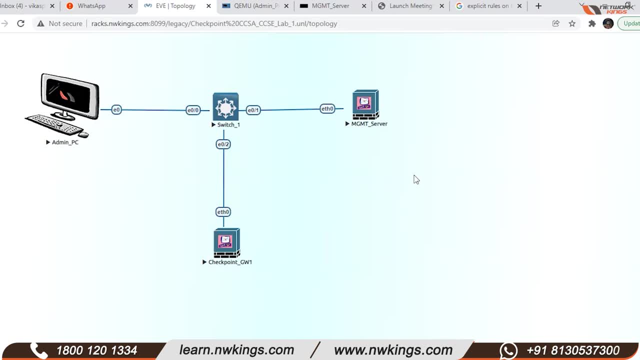 Sir, there are two firewalls here. One is checkpoint gateway one, and the other is management server. See, I will show you now. The management server we are making is a firewall, But we are saying it manually that you are making activities of firewall. 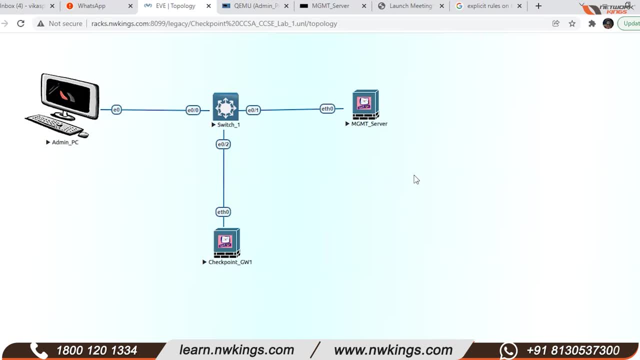 But you are not performing it manually, So you have to perform the activities of management server. So I will show you now, I will demonstrate how we will tell it and what changes we will make after that. I mean to say that we have installed two firewalls in topology. 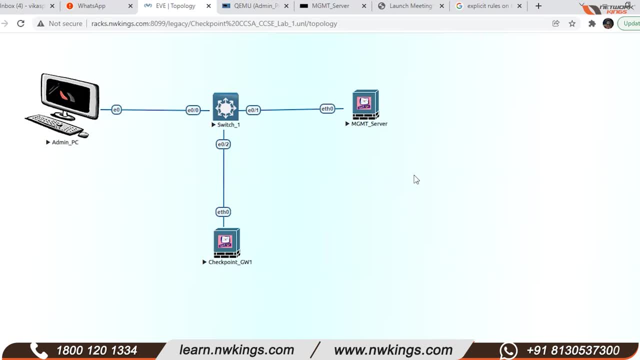 Okay, One is management server and the other is checkpoint. So it is the same in production as well, that when we develop, checkpoints remain double. One is server and the other is checkpoint gateway, And in fact it is not double. Maybe you will get six or seven firewalls. 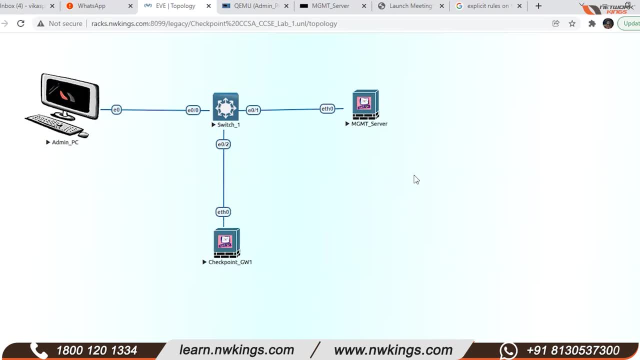 Sir, I want to say that one is checkpoint firewall and the other is management server. Okay, So basically here in observing there are two firewalls, One management server and checkpoint. So we have to create all policy on the management server And pushing that all policy through gateway on the firewall. 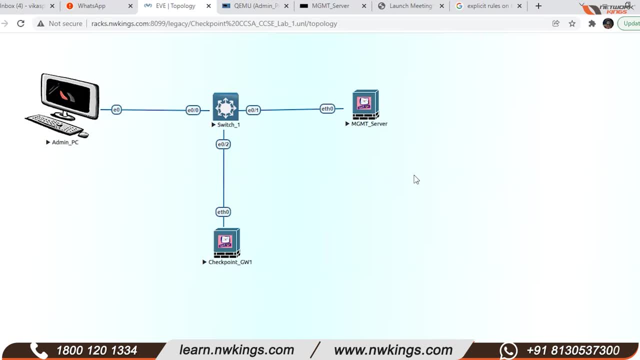 Hmm, And basically why we are using management server to protect our firewall. Yes, To protect the firewall. This is the main quality of its checkpoint: that it checks the management server first and then deploy it on the checkpoint. Okay, So the concept of the server is that we deploy the server so that we can deploy the firewall. 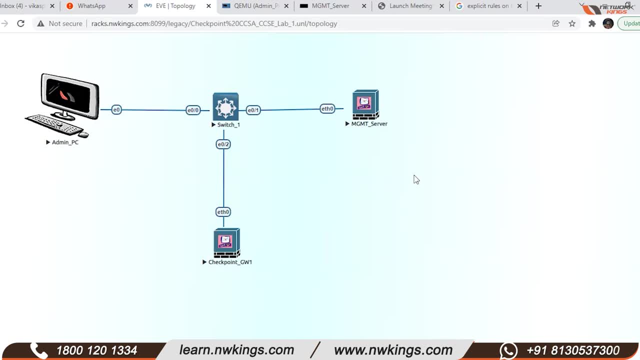 at any cost, Because all policy, everything is done virtually in the server and we push it on the firewall through the gateway. Hmm, Okay, But, sir, one thing can be asked. If we look at it for security purposes, then the three-tier architecture is much more secure. 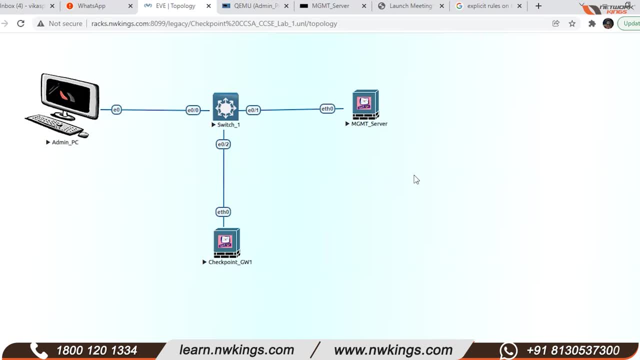 as compared to the standalone architecture. That is why checkpoint recommends to do that three-tier architecture, right? Yes, That is why checkpoint recommends to do that three-tier architecture, right? Yes, Okay, That is why they recommend to do distributed deployment. 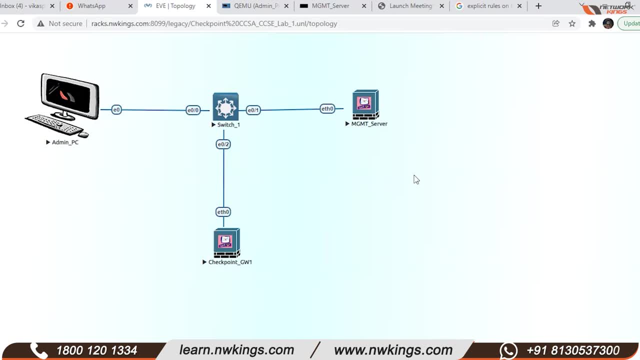 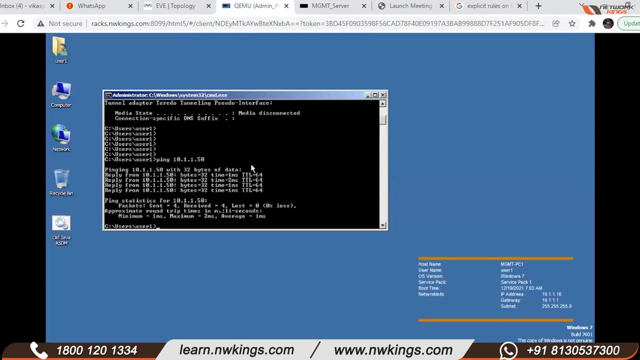 Okay, Okay, Understood, sir, Understood, understood. Any other question? No, sir, go ahead. Okay, give me a minute. All right, So all these things are being discussed, Okay, So till here, everything is clear. and what we have done, this activity, why we changed the IP of the interface and the connectivity we have made here of our client and management server. is it clear to you? 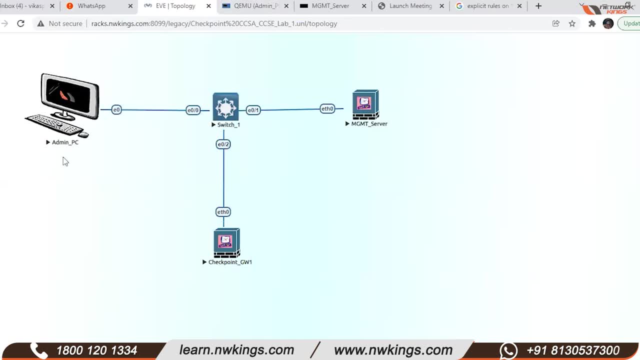 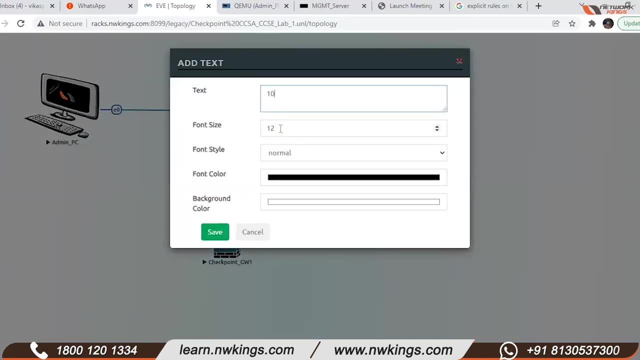 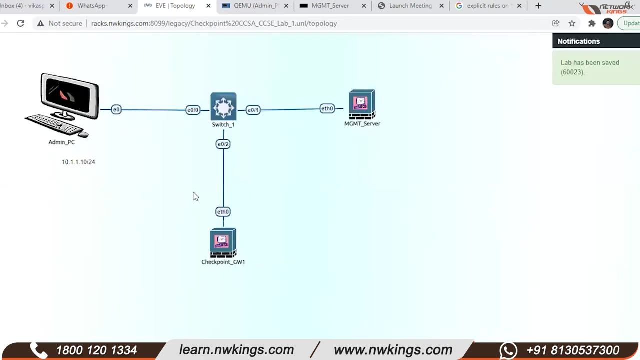 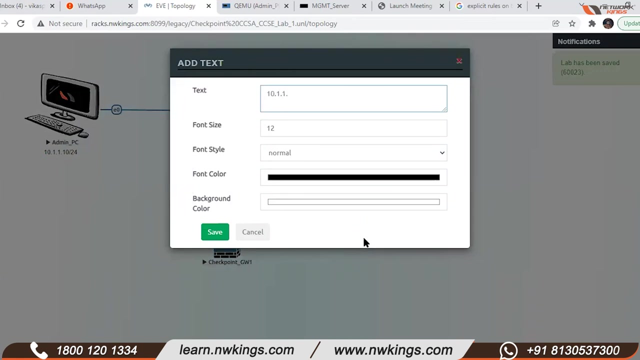 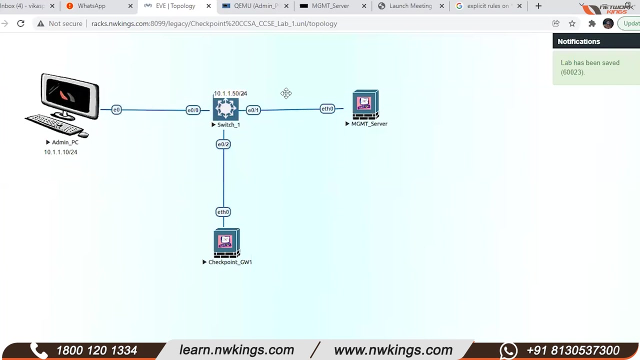 Yes, sir, if you write on topology, then it will be better. sir, Can we write on topology? Yes, sir, 10.1.1.10.24, 10.1.1.50.24. Ok, Yes sir, Yes sir. 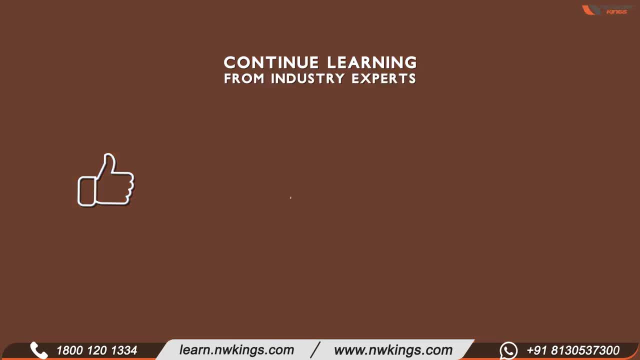 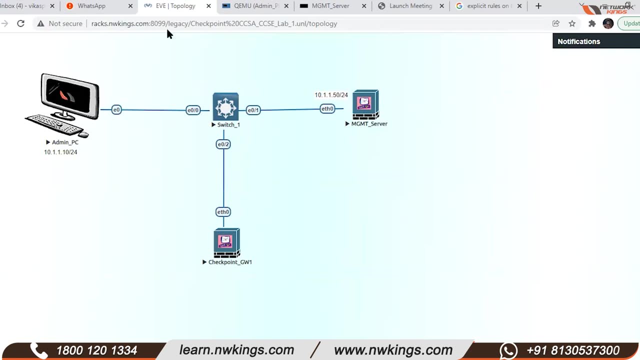 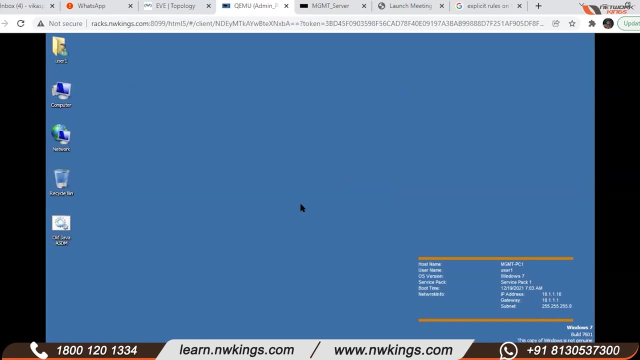 Thank you, Any other doubt? Hi, you are watching the recording from one of our live session. Hit like share and subscribe for more future updates. Ok, Now what do we do? We minimize CMDU from here. We go to internet explorer. 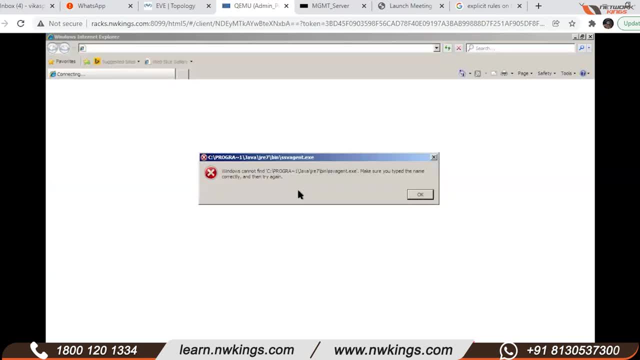 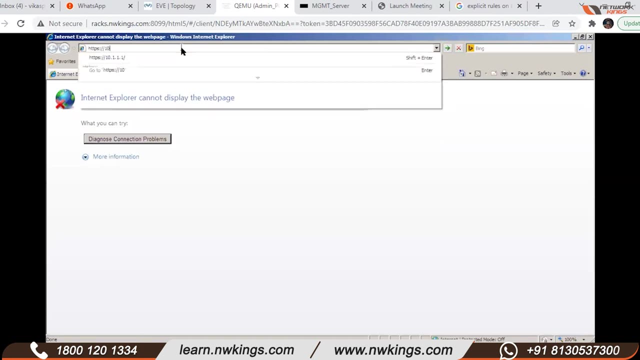 Now see the first time access of checkpoint. the first access you have to do is on browser. Ok, The first time access you have to do is on browser. How to do it? HTTPS 10.1.1.50.. It will be a little slow. 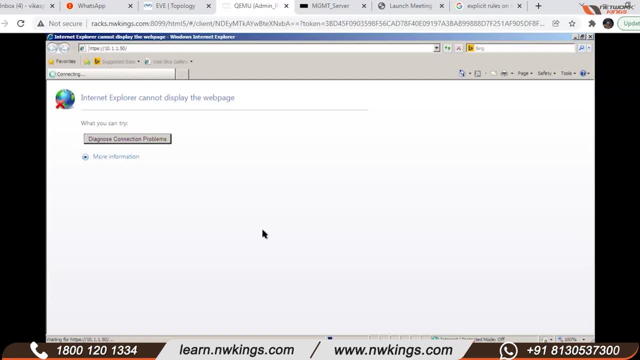 I don't know why this server is coming here. PC should have come here. But let's see, Checkpoint GUI can be accessed. Yes, Yes, Web GUI. This is called web GUI. You will access it on the web page. 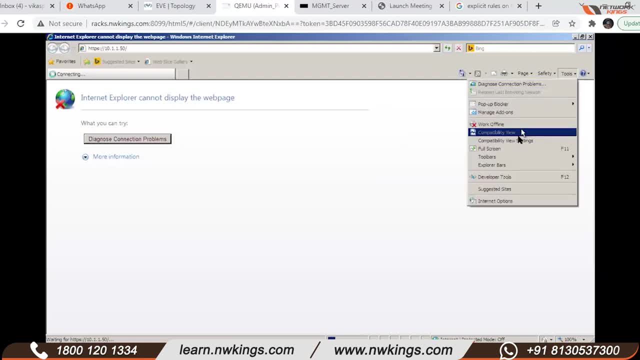 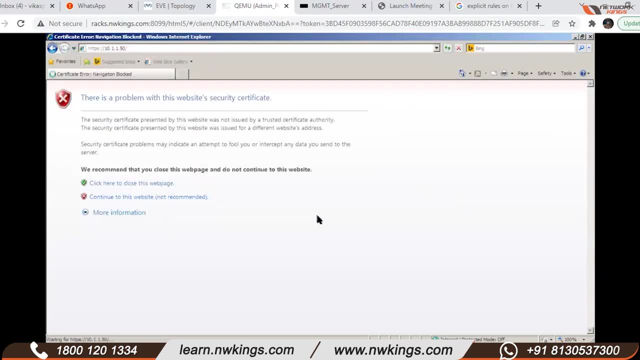 And if your little bit of flow is running here, then it will be compatible. By the way it has come. As soon as you do this, you will have to continue it here, Which is not recommended Because there is an error of SSL here. 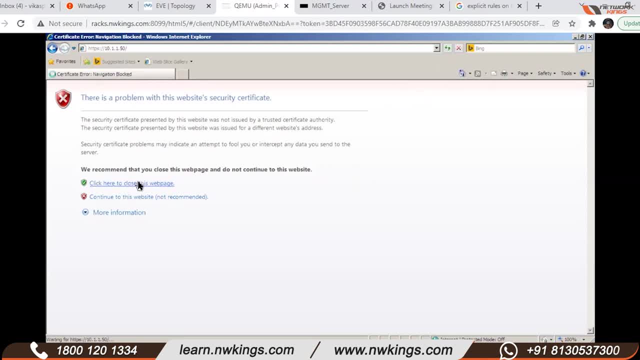 SSL certificate. This browser does not have any SSL certificate for this URL. That is why it is giving this error. Click on continue And now just go to compatibility setting And just add this one in your browser compatibility mode And I hope that it will come here. 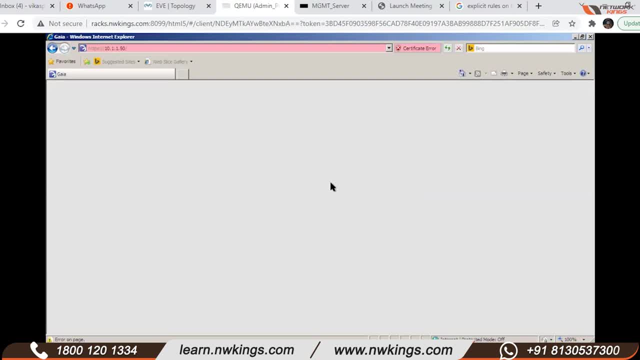 Let's refresh it once. I think the login page is not coming. I will have to talk to Gaurav about why this server is launching here when I am launching the PC. Okay, So I think we will have to stop for today. 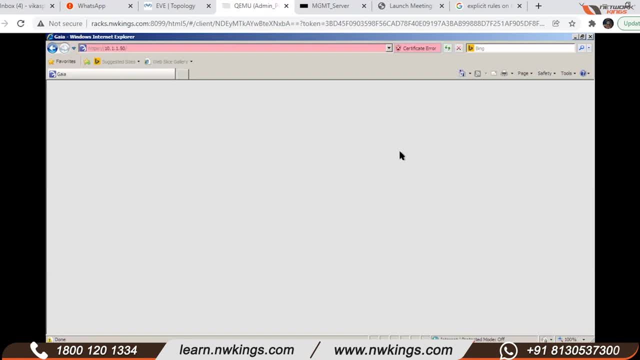 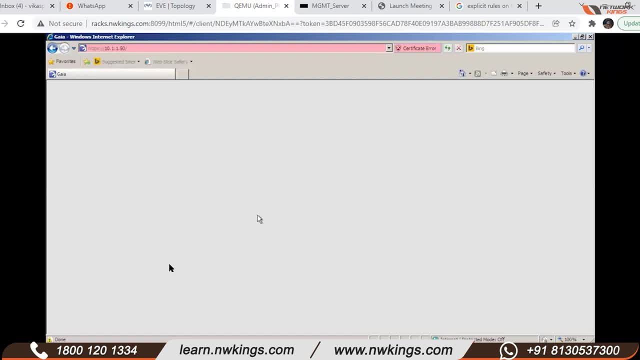 But it is not coming And apart from this compatibility setting, there is no other setting we can do here. Okay, Let's do one more thing. HTTP is 10.101.. Yeah, This one Will it take it like this: 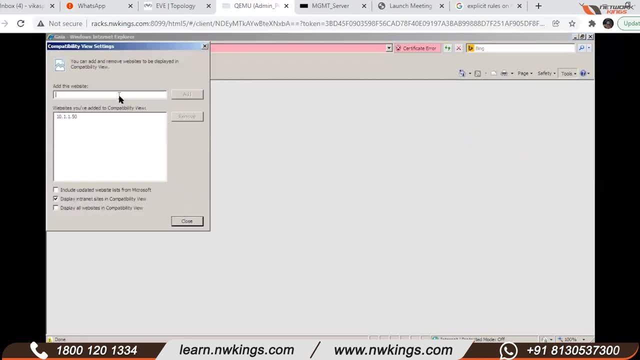 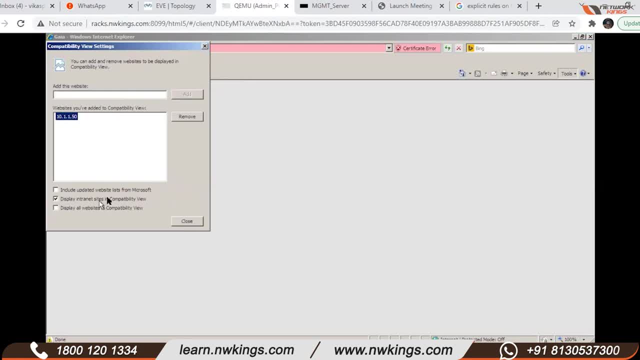 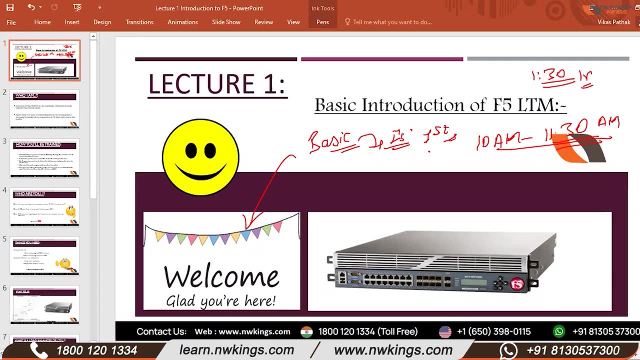 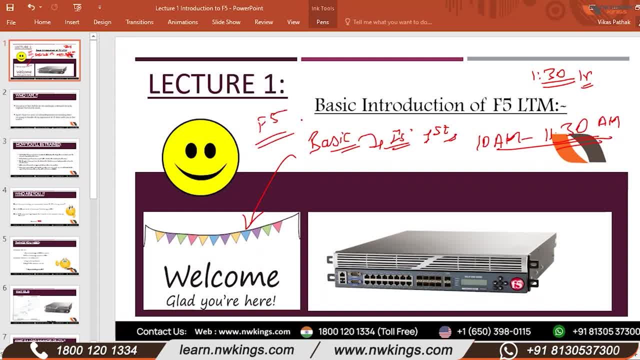 There has been a lot of technology in market. who gives LTM feature set? If I talk about specific LTM, then they are giving it, So why we should move on FI? We will discuss that thing, Okay. So if I talk about physical appearance, some devices like this: 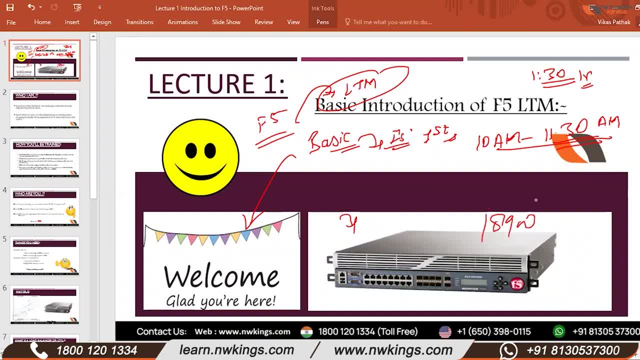 Yeah, This is an F5 box of 8900 series, which is a very beautiful box. I have worked on it a lot and its features, its processing, works in a very fantastic way. All the boxes of F5 are very good, but this one is a high-end box actually. 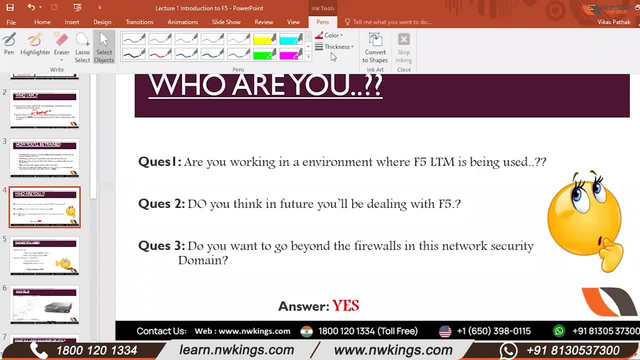 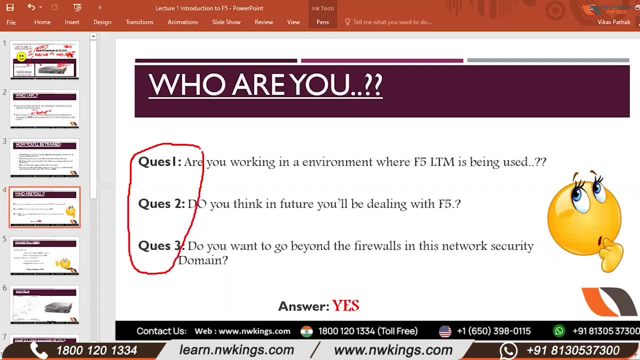 Major three questions. I always recommend to all of the joiners to ask to themselves Why you should join this course, Or maybe you can say why we should attend this F5 course. You can ask these three questions to yourself. First is: are you in such an environment where F5 is being used? 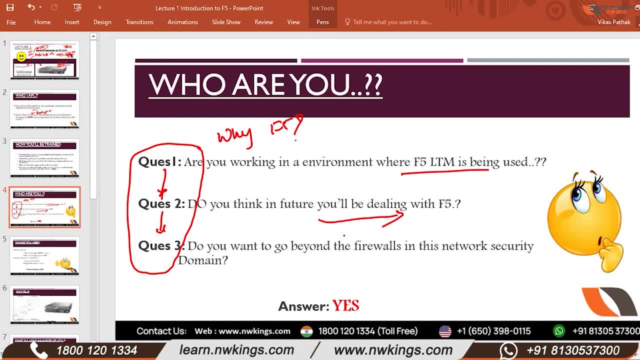 Or is F5 going to be installed in the future? Second is: are you in the network security domain from the last 3-4 years and you want to try something new? You are done with the firewalls- right, You are mastering the firewalls, but you want to learn something new apart from the firewalls. 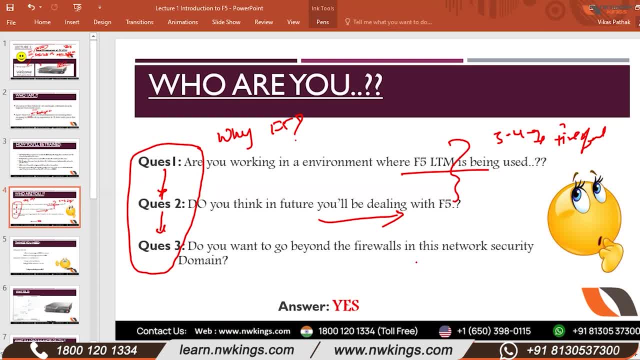 So you want to enhance your knowledge beyond the network security or firewall security domain, So you can learn F5.. So, again in all these questions, if the answer is yes, then you are at the right place. So these three questions are very important before joining any course. 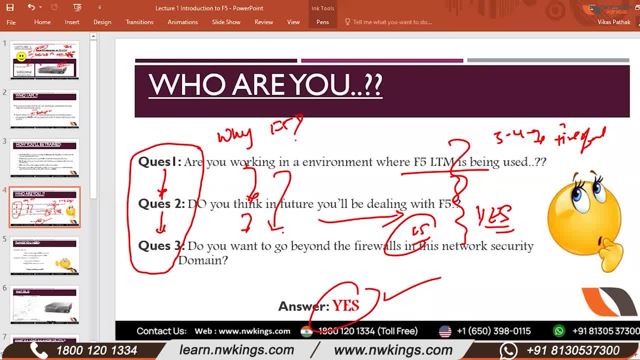 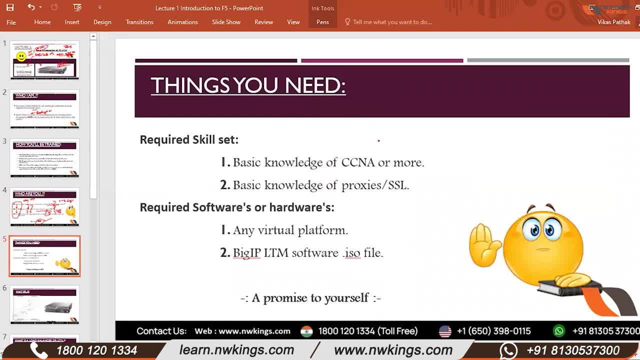 So their answer should definitely be yes. Now let's talk about the prerequisites to join this course. First of all, you should have CCNA and more knowledge than that. Okay, You should know what is. you know SSL. You should know what is TCP. 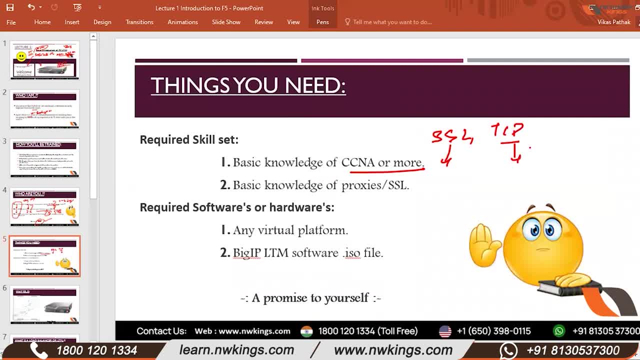 SSL handshake, TCP handshake. You should know right how packets are exchanged between client and server, Because mainly our focus will be on client and server architecture. We have to play the whole game on this. So the communication between client and server is happening through SSL. 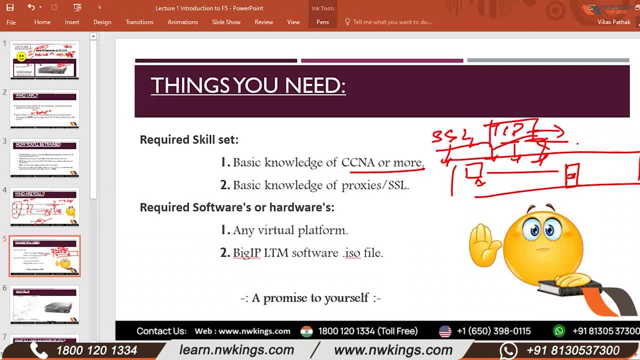 So what is the handshake process? So what is the handshake process Briefly, we will discuss in this course as well. But you should know like deep understanding of what it is I mean if I talk about the algorithm. 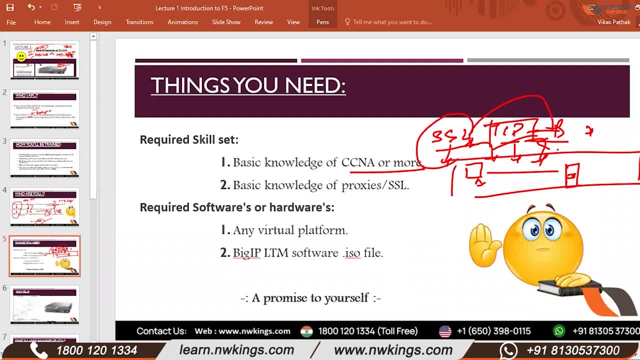 which algorithms are exchanged in the handshake of SSL from the browser side. You should know that, right. Proxy SSL. Yeah, you should know like what is the proxy, Because if I talk about big IP, big IP, big IP, like F5, the product is F5, big IP, its full name. 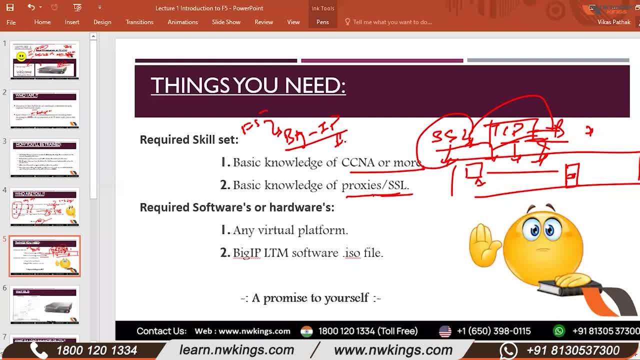 So if I talk about big IP, then big IP is full proxy By default. it is full proxy. Now, how is it? I will discuss it in the next slide. Lab is simple. If you want to set up a lab on your laptop, then you need a virtual environment. 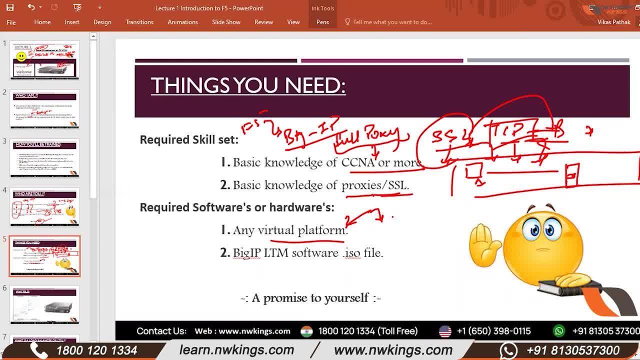 You need VMware, or if you purchase a course of networking or you enroll yourself, you will get a virtual lab on which you can perform all these tasks. You just need an internet connection. All right And after, like, if you want to do your own personal lab, offline lab. 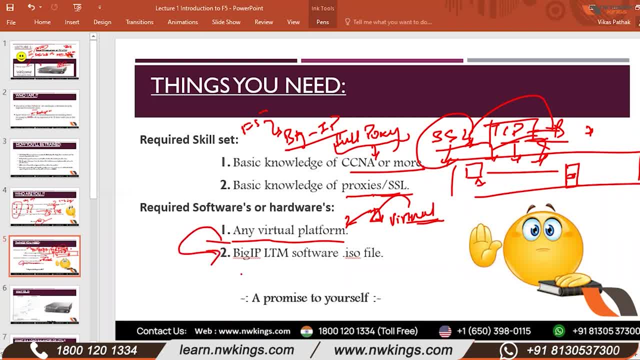 then if you install VMware, then along with that you need big IP software ISO file which you can download from F5 website. Okay, Easy, It's very easy. You just need to mention on the Google that download F5, big IP LTM ISO file. 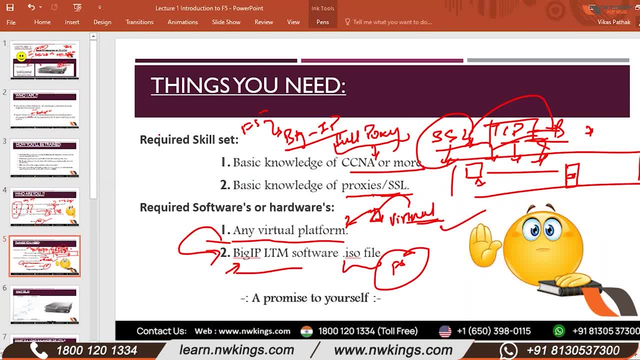 It will be downloaded And these things are fine. You should have these things. Apart from this, I promise what you will do with yourself that. yes, okay, I took classes on a course on a weekend. I will give this topic, this technology F5, 10 to 15 minutes a day. 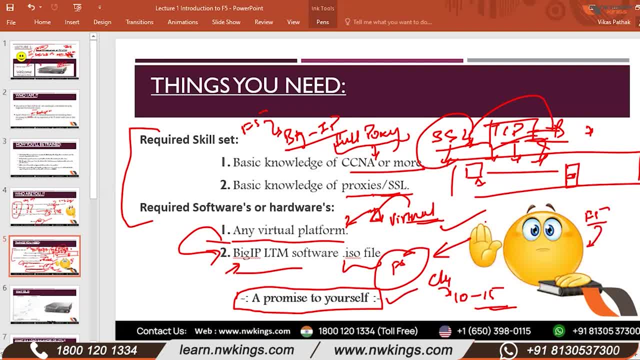 whether I watch a YouTube video, whether I revise my lecture, whether I read notes, whether I read its admin guide, but I will give 10 to 15 minutes daily And if you make this promise to yourself, then, believe me, you will be F5 administrator soon. 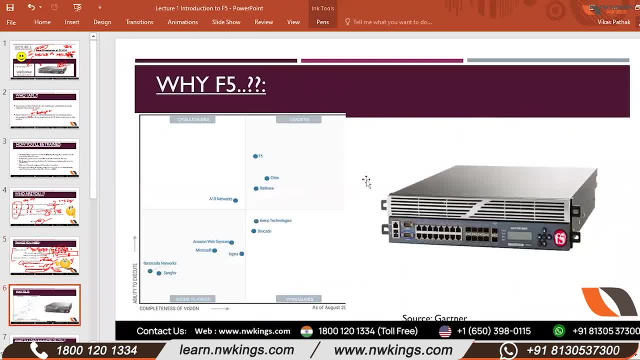 Okay. Now the question is: why F5?? Okay, I'm teaching F5.. Okay, And for me, F5 is a very good technology. But why should you believe me? Right? Why will you believe me? I'm just a person. 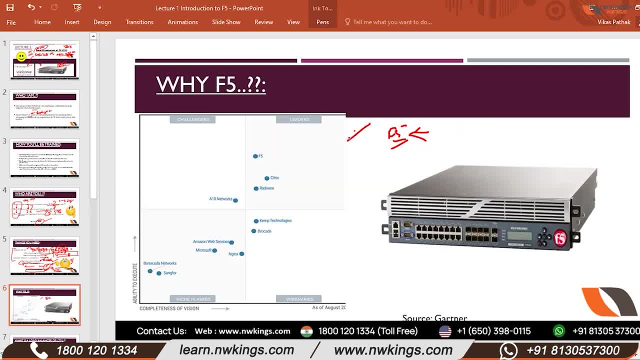 Right, But there is one other thing, But there is one organization which evaluates technologies on the basis of their performance, support, technology and vision, And their organization name is Gartner, And this is the report of Gartner, published in 2019. 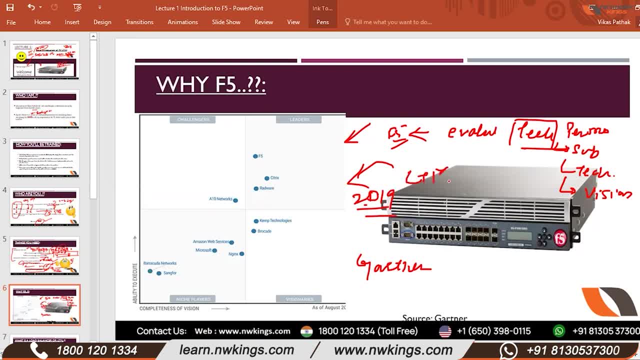 for LTM And see what is the stand of the F5.. There are three market leaders right. There are three market leaders in LTM section where F5 is one of them And I believe it's on. it is the first one. 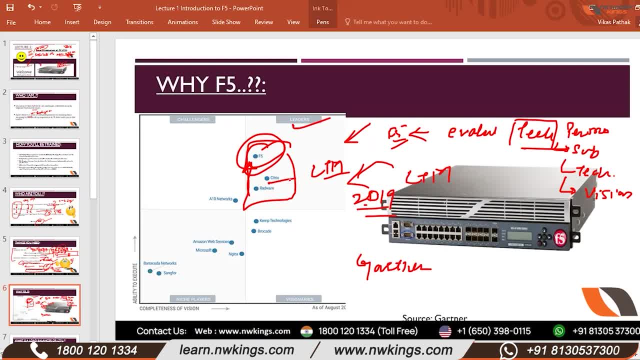 maybe I'm not sure, like whether the Citrix is on number one or the F5 one, but I think I think it should be F5. Right, So so this, this, this report, says that F5 is the market trend right now. 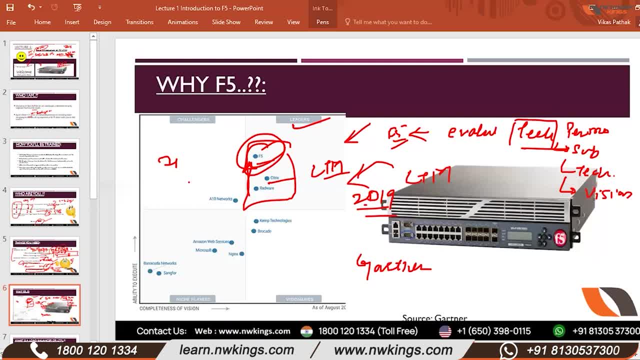 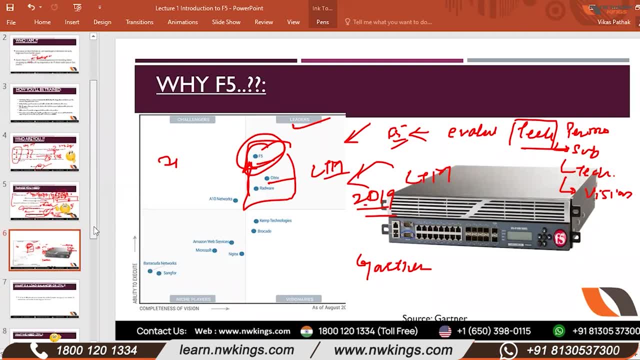 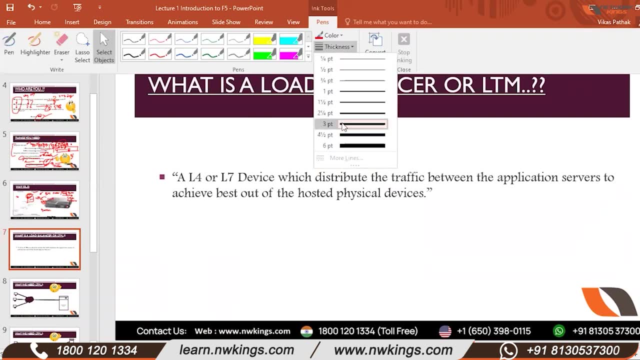 And if you want to learn, you should not be doing delay. Okay, Without any delay, you should. you should learn this technology, All right, Okay, So next, you know question. next: you should have this question in mind. 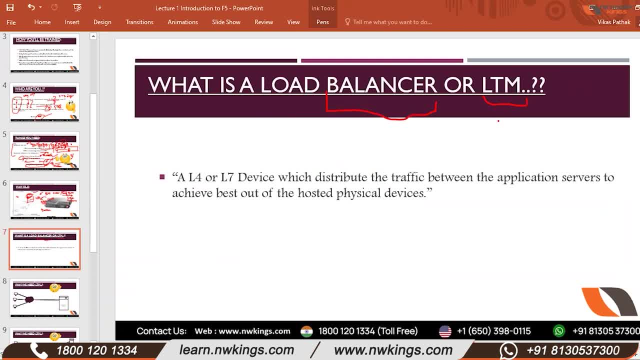 What is a load balancer or LTM? LTM stands for Local Traffic Manager, Okay, And load balancer is a term which indicates a device which does the load balancing. Okay, It's a very basic, very basic thing. It might be. 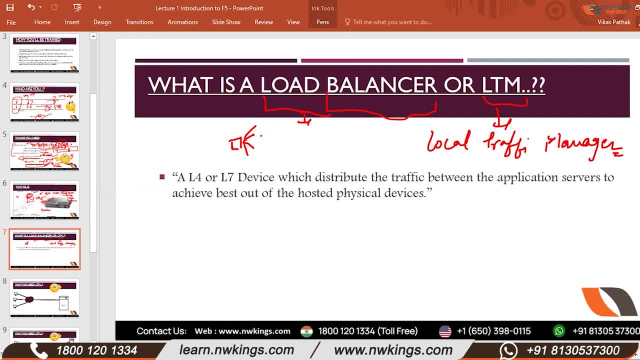 some of you might know this term, but I'm trying to explain it in a very basic way. I'm trying to explain it in a very basic way. If I take a real-time example, if there is a team, there are five members in the team. 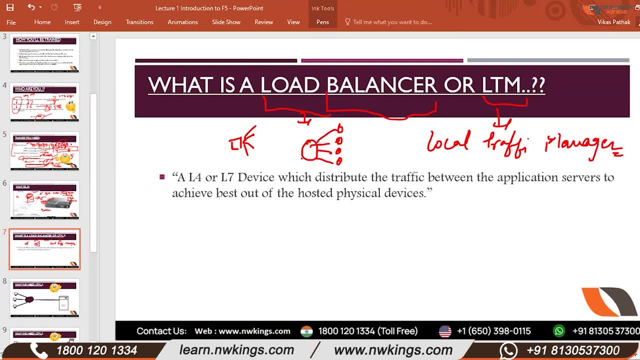 To manage those five members, there is a team leader. That team leader is a load balancer. What he does, basically: whatever work is coming to the team, distribute that work to everyone, Right? What will happen with this? The proper efficiency of all these teammates. 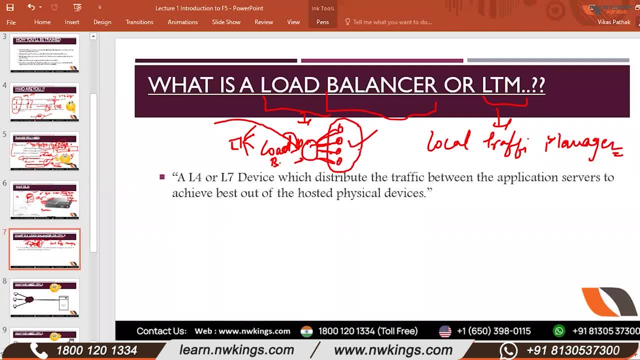 will come out Correct. So F5, a L4 or L7 device which distributes the traffic between the application servers to achieve best out of the hosted physical devices. If I assume that these five- we just said team members- these five servers, 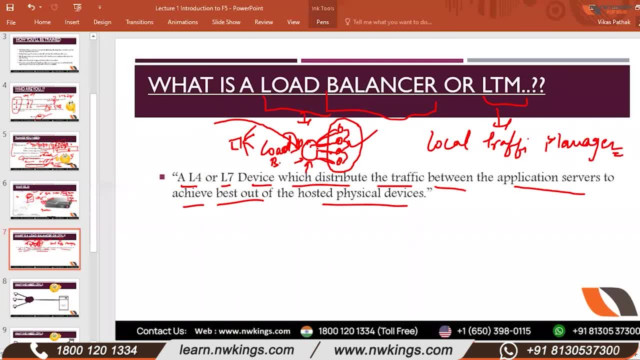 so the load balancer here. what does that load balancer do? It distributes the traffic equally on these five servers so that the resources of these five servers can be properly and equally used And we get the best value of our investment Right. 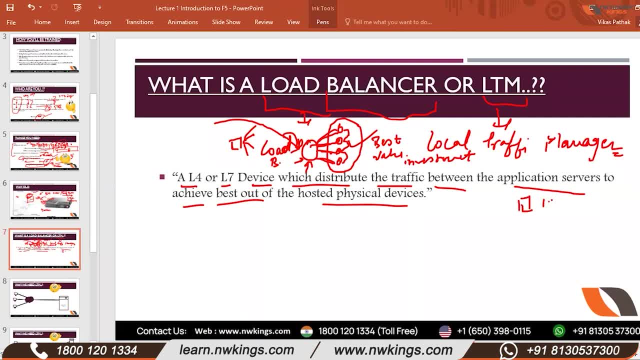 Now let's assume I have spent 10,000 rupees per server Right And I have five servers. The total sum is 50k. Now, if I assume such a scenario that the traffic is only going to these two, 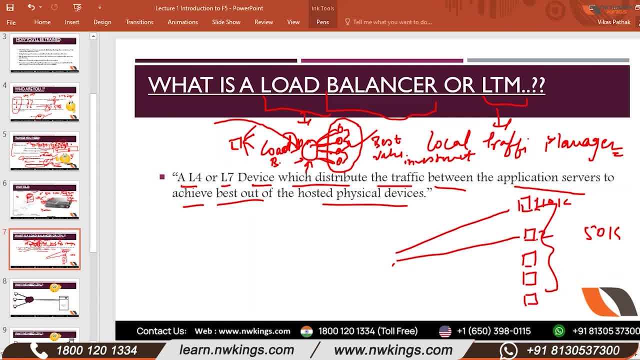 the first and second virtual servers, the real servers. So the value of the first two servers is going to be 20k, which we are using properly. But what about these remaining 30k? This is a waste. They are sitting idle. 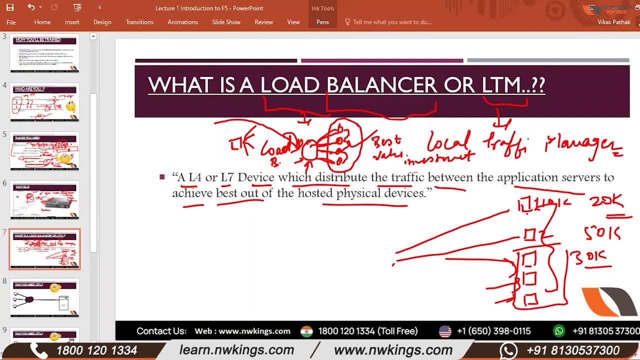 They are doing nothing. Maybe they might be doing, you know, backup for these two servers. Okay, let's take, let's consider these two servers as a backup, But still, after doing the backup, what they are doing? They are doing nothing. 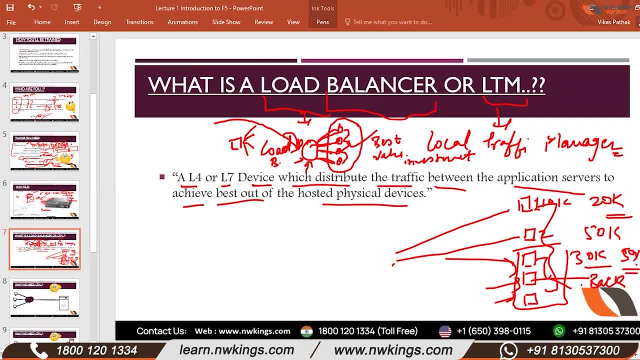 Right, 50% of the cost, I think. still we are. we are like losing. And for the fifth one we are losing 100% Right, So to secure 100% of the investment we can say. 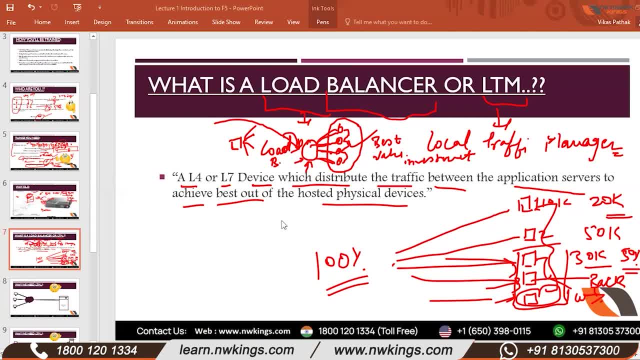 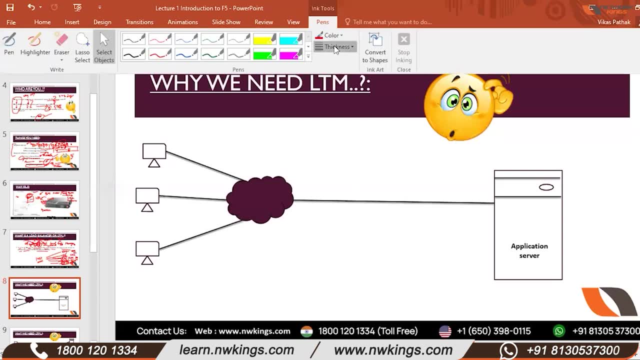 we use load balance Right. Any any doubt till till here? No, sir, Perfect. Okay, So you understood what is LTM, What is load balancer Right, But why we need it. We have read a big definition. 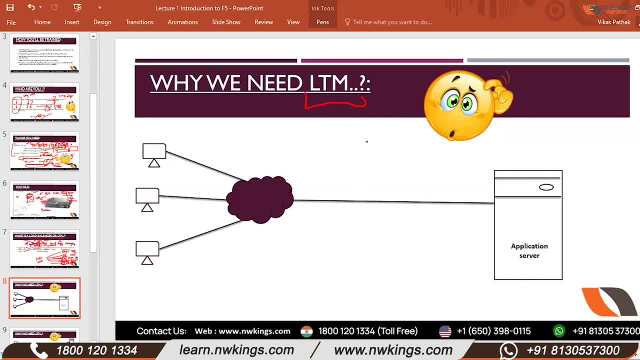 that we need proper utilization, or maybe you know, efficiency- all of the available resources, then we should use load balancer, Right, But if there is no load balancer, then what will be scenario? Let's discuss. let's discuss. 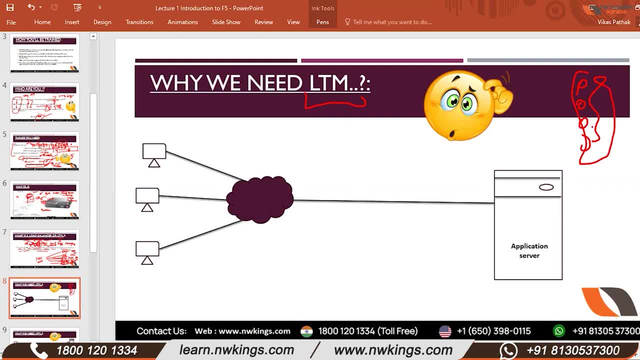 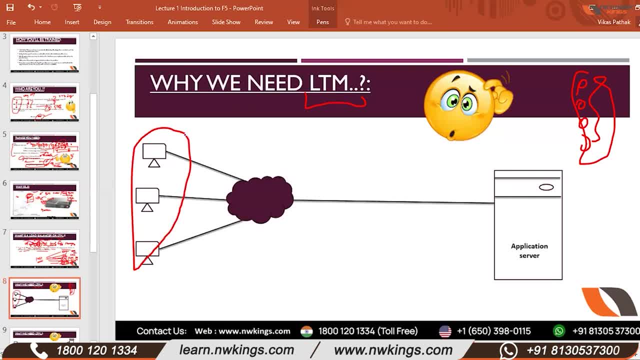 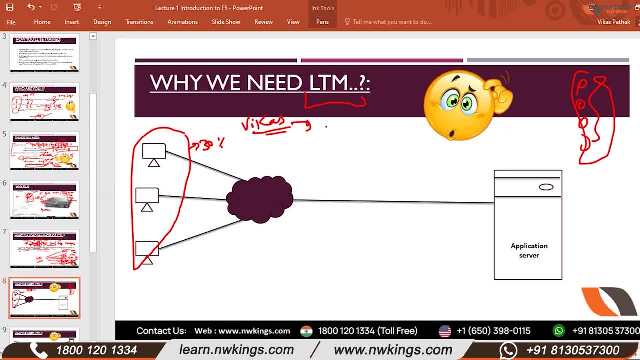 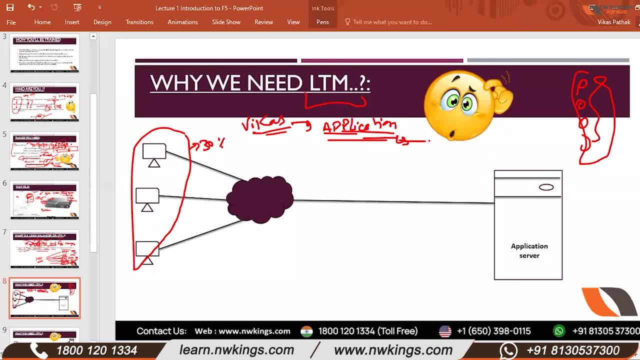 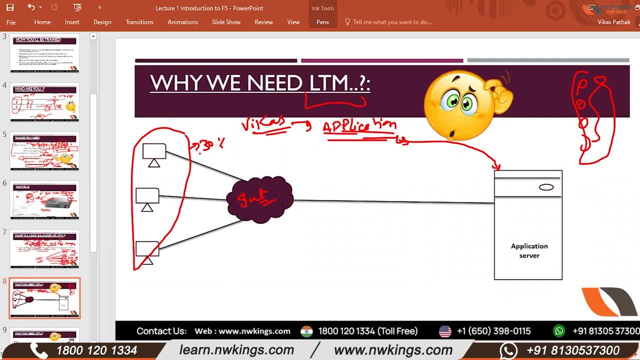 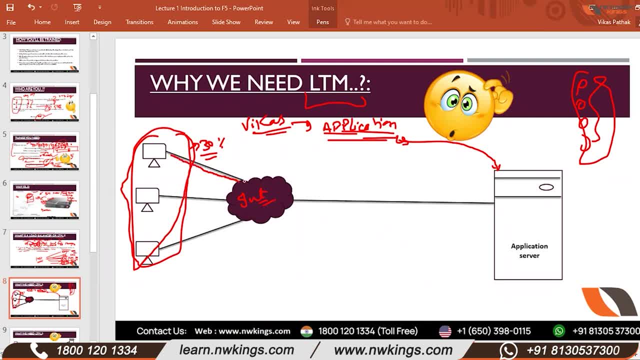 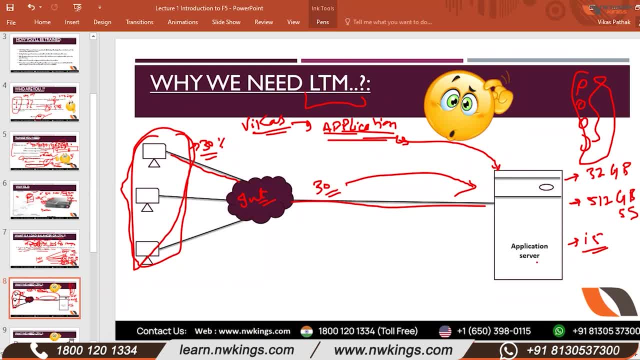 actually, uh, with the server in the, in the term of server terminology, right, so these users say up after a month, so 25, 25 in six months. this user base, which was 30 users earlier, now it's 3000. then what will happen? this application? 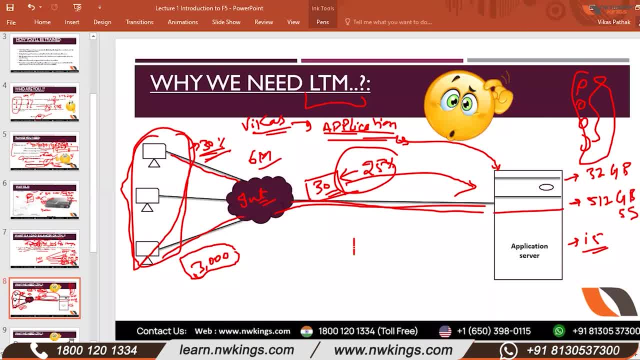 slowly, gradually, number of users will increase. these resources will start to decrease. okay, now, if these resources decrease, then what will happen? response time will increase. the application, which was responding within one ms, uh microsecond, it is taking now five seconds, and five seconds for application server is a big delay. okay. 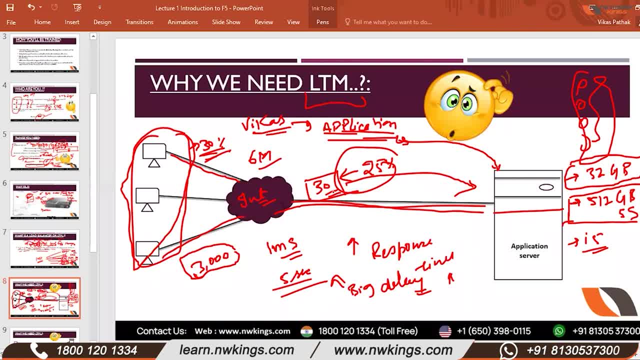 so let's go in this scenario. okay now the obvious thing is that if i have an application server and my user base is increasing, then i will have to increase my application server. okay, i have to invest in my iot infrastructure. i have purchased one another server here and let's say i have. 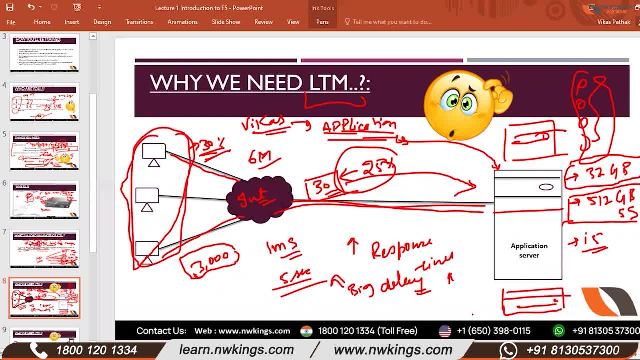 purchased two of them. another one is here. what is the method through which i can communicate to these 3000 clients? i have sufficient, you know, resources and when they access these resources, so equally, connection distribute. let's say, if 3000 are coming, then 1000 go to this server, 1000 go to this server and 1000 go to this server. 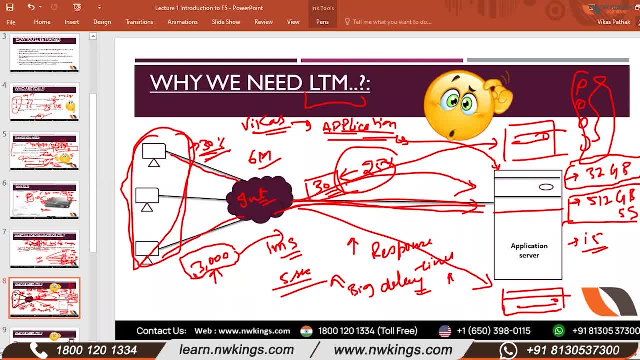 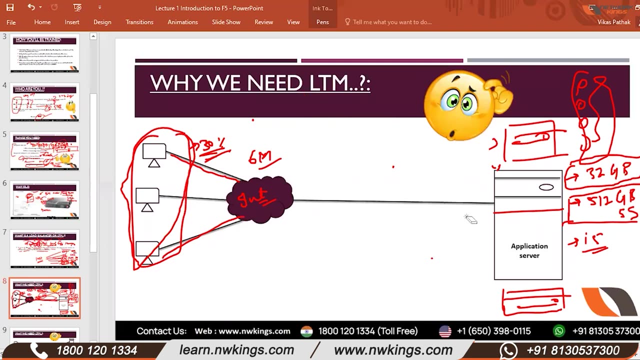 go to the server. what is the guarantee of this? how can i do it? any idea, anyone, anyone. i think for this we have to use a 5ltm. i think definitely that will will use like we will use that. but apart from that ltm, what is the matter? method, do you have anything in mind? 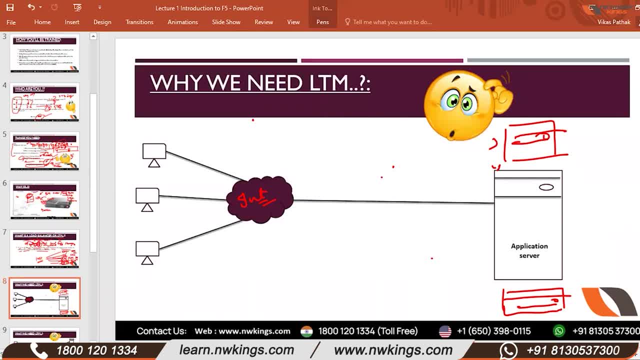 for distributing equality, you have to use this app app, yes, you, what? like this application server? yes, okay, all right, let me explain. because when, when we use 3000 users, so if there will be traffic, so, for example, server cannot increase the speed, so, for example, server cannot increase the speed. 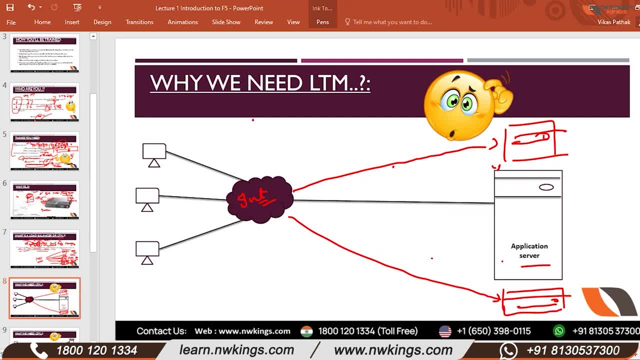 so that time we will use another application. i think. see, we have one application server here, we have second one here, we have third one here. we have three application servers now, right then, how we can distribute this 3000 connection between all three of them, just like, as you said? 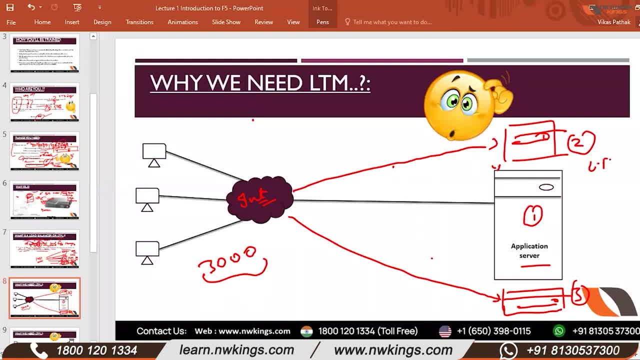 that you won't be able to collect time in same way. user in same way. let me change points. user in same way. user in same way like a expected, so that conversations withGOD is witha DNS and I have given xyzcom Now. till now my users were accessing xyzcom going to. 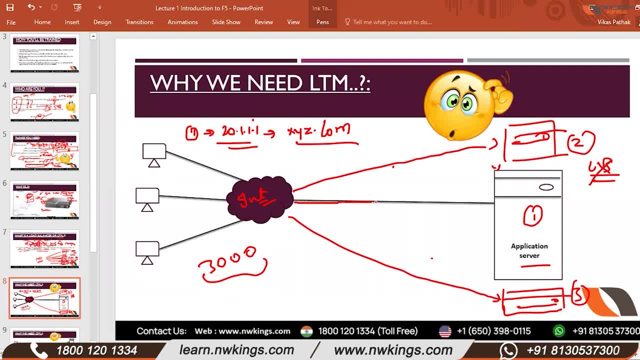 internet and resolving DNS in this IP and that request was landing on this server. Now, if I have increased two application servers, then one method I have is that my two servers will also have some IP, let's say 20.1.1.2.3.. These are my two application servers. I. 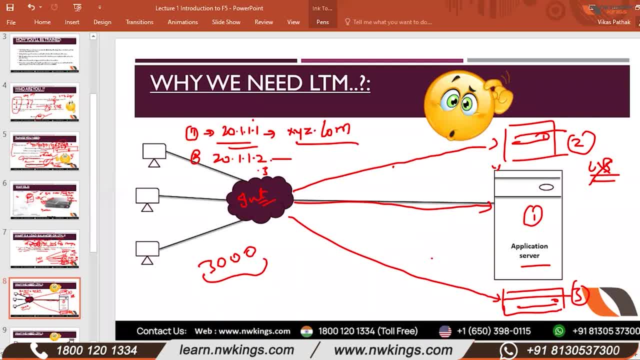 will also map them with some new URL, map them with DNS: xyz1.com, xyz2.com. and I will manually tell these 3000 users to go and use the previous 1000, this one, the rest of the 1000, use xyz1.com and the rest of the 1000. 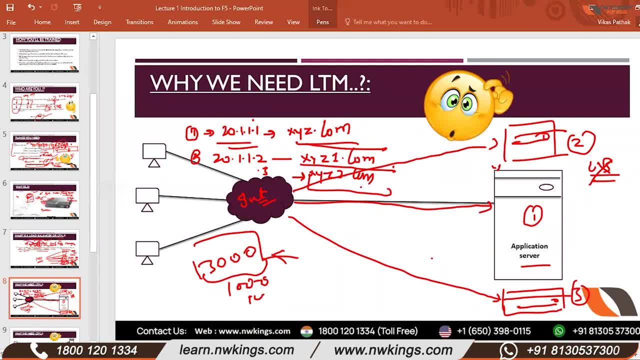 The rest of the people can use this one, So this is the only way. But this is the worst way of managing your application server and the connection In the first way. it will take a long time. I think No. how will you tell the client? What will you say to the client? Let's say you have 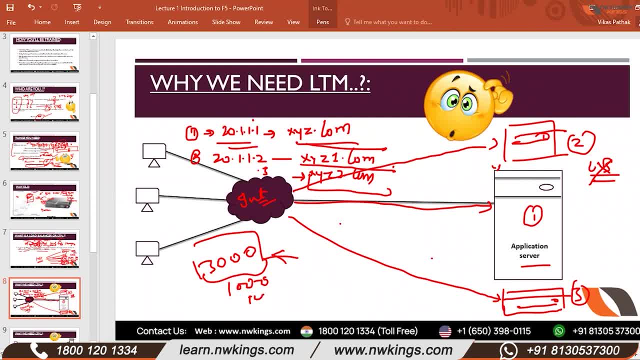 flipkart. tomorrow you will get a mail from flipkart that from today we have an application server. Let's say you are not in 2021, right. Let's say you are in 2003. or let's say you are in 2002, right- I don't know when this 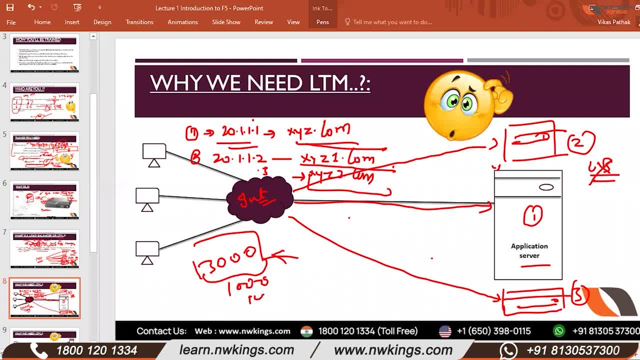 invention happened. but let's say you are in 2002 and flipkart comes to you, that our application server resources were getting less, so let's do one thing. what will we do from today? You will use flipkart 1,, you will use flipkart 2,, you will use flipkart 3.. Now, if someone 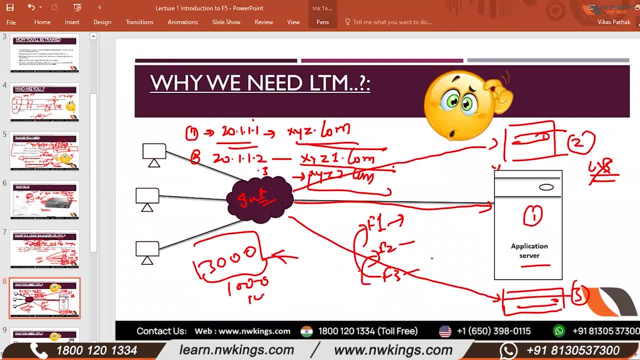 is using flipkart 1, someone is using flipkart 2.. No one remembers using flipkart 1 or he didn't read the mail. he is going to normal flipkart and he is going to flipkart. he is getting slowness. what happened to him? The user base. 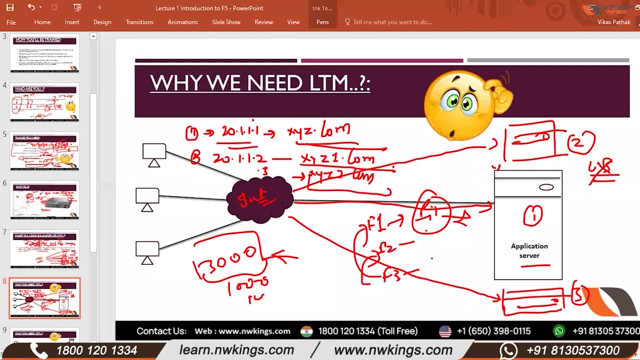 is damaged. Sir. can we do this, sir, that if we use the old method then we can do a net that a lot of local IPs, as you are, inside the web server, so they can translate the pool of IPs against a public IP? 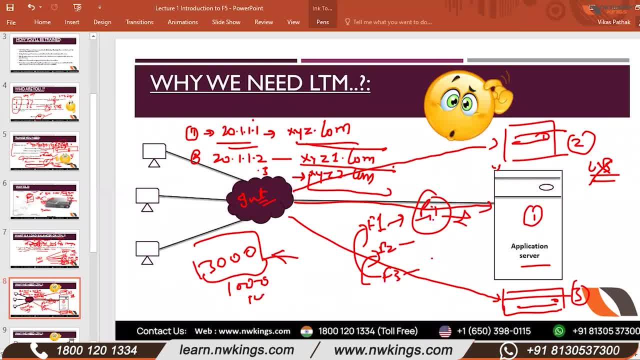 Yes, Translate it. Yes, Translate it and do it. that is the IP will be one. whoever is accessing from outside will see one IP, but inside, what is it under its port? port address translation will be done on the port. so we will do it. do something like this: 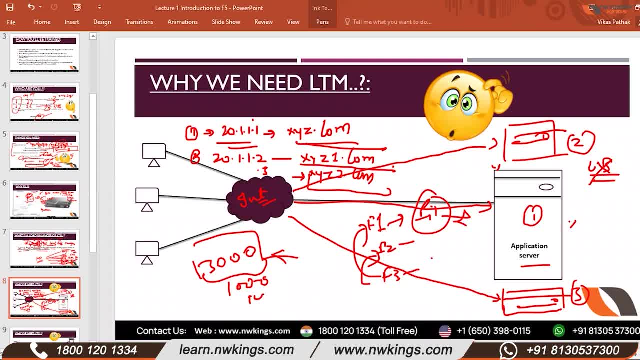 Okay, it's a great approach, it's a very good approach. okay, And here too, here too, Through network, through network, we can send a message to client or whatever. No, no, no, Look In terms of practicality. look, if you want to read load balance, then you will have to. 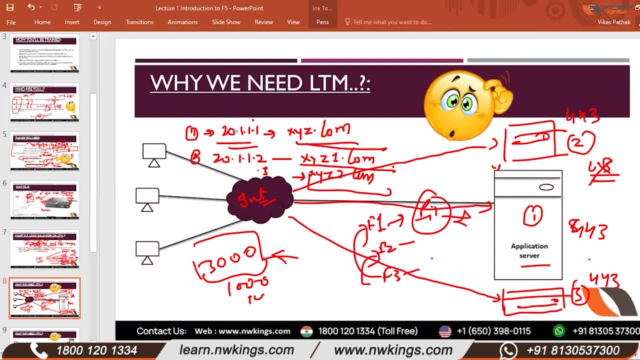 think about practicality. you will have to open all the gates of the mind first of all. First of all, I give the answer of the first suggestion, that, brother, we put a firewall here. we took the traffic on a virtual IP from the firewall and sent it inside by translating. 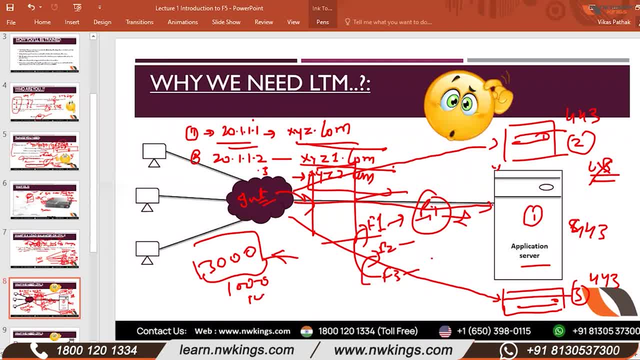 it again, but the question was that how to distribute the traffic of our 443, the traffic of our 443.. Yes, Yes, Yes, You gave us that problem, but we did not have the problem that we are ordering traffic in multiple IPs. our problem was that how to distribute our 21 Stock or 21 Eyes working. 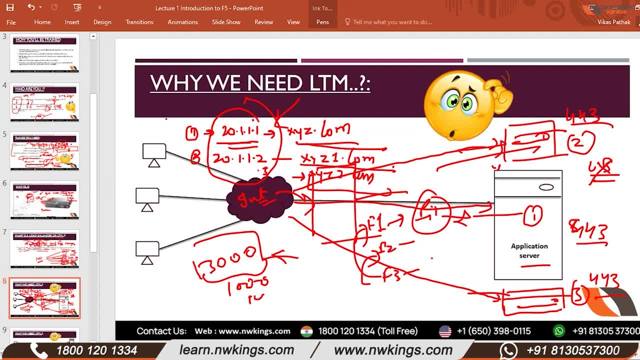 out full quiz, is that Okay? I receive it on that IP, translate it and go ahead, but not send warn someone. No, Sir, they have to take help of distributor. Sir, if we can do equal load balancing and unequal load balancing, can we do dynamic protocols or not? 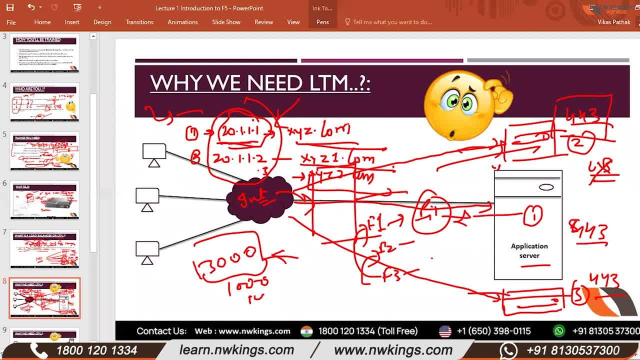 If there is any protocol, like EIGR used to do equal weight paths, can we do it this way or not? See, routing is only for routing that traffic is sent to you from me. Now, if there are six people in your name and six people are capable of doing the same work, then how will they distribute that work to six people? 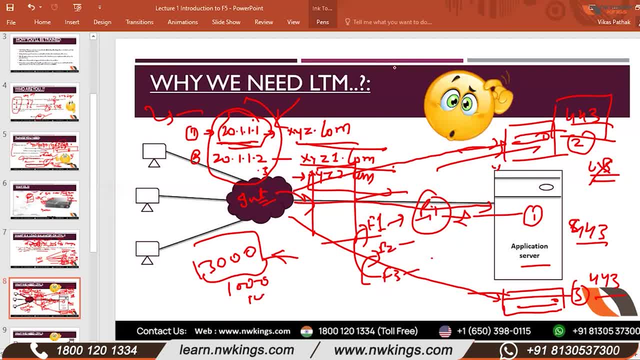 Sir, then the ports will be different. It will have to be done at different ports, Like if there is a virtual IP from outside for us and we will map it against different IPs. Like our load balancer, it will be either static or dynamic load balancing. 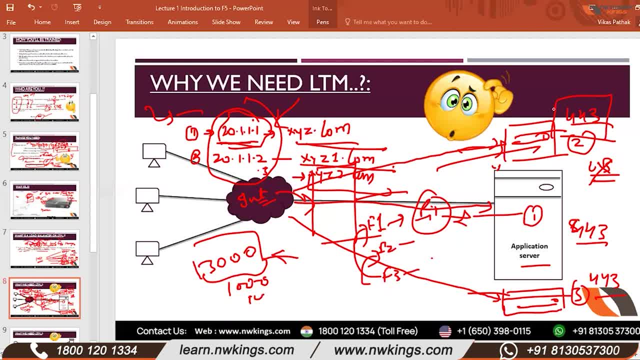 It will divide it that way: If we do static, it will divide it equally, And if we do it dynamically, it will divide it equally according to the load. Okay, okay, I have a simple question: What port did your traffic come on? 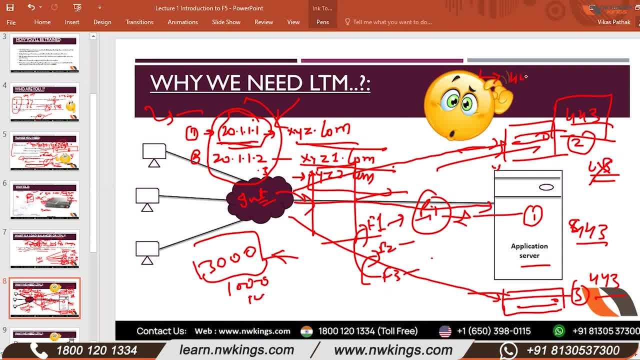 It came on 4.4.3.. Sir, the traffic was received on 4.4.3.. Okay, What do you want? at which port should it be sent further? The local port inside. this is your public right. Your public is coming on 4.4.3.. 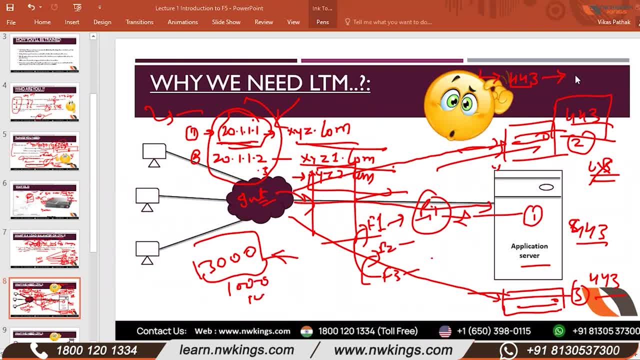 Okay, how will you send it inside? You can customize the port inside. I think you can customize it. The service of 4.4.3 will run on 4.4.3,. right, sir, Right, right, right. okay, It will have to be sent on 4.4.3,. it will have to be sent on this. 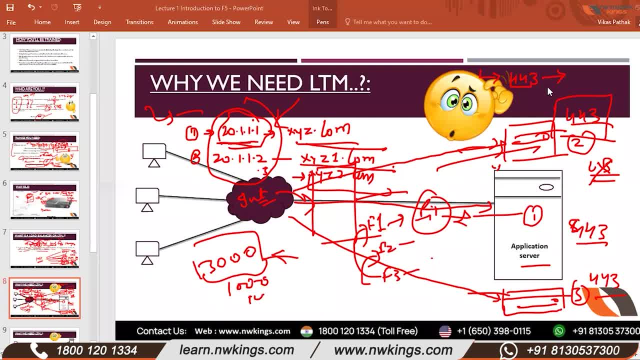 Right. So how will you do the padding? Right, So how will you do the padding? That's right, right. This is why I am saying that: look, This is why I am saying that: look, Sir, the padding role. I think internet will be done, I think. 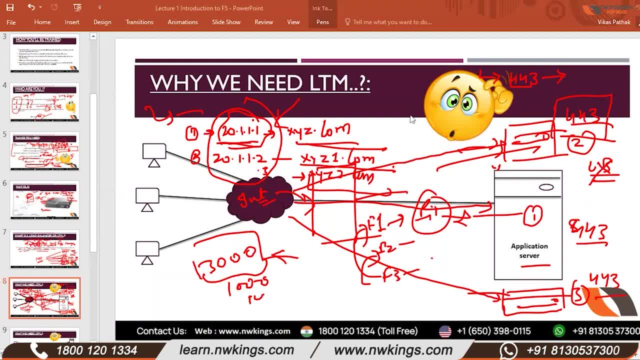 No, no, no. I mean here: No, no, no. you are right, Sir. then how will he do it? He will go on one and then how will he take it on others? Understand, I mean, close your eyes and think that what's happening in the communication. what I want to say first, 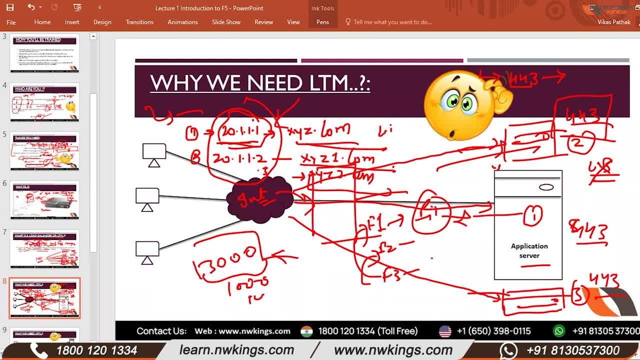 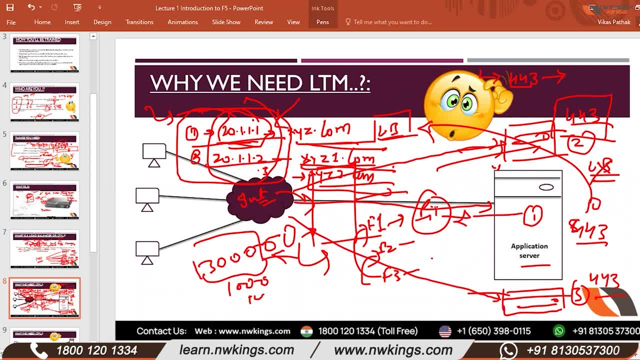 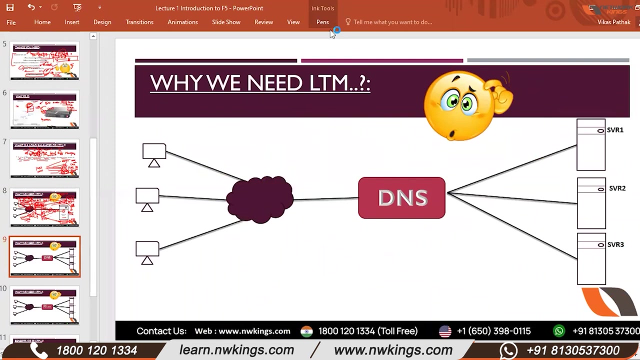 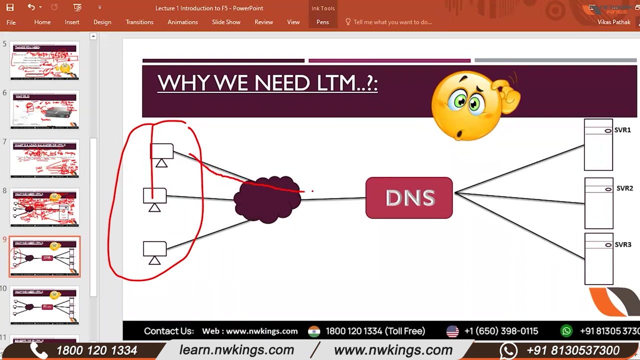 you, let me tell you, let me tell you, let me tell you: torture two- Corinne in Media TV, foreign, foreign, foreign. I thought there will be DNS, but I didn't expect it. How will we involve DNS? When we make an entry for DNS, we will ask the user to take a query for these servers and make an entry for DNS. 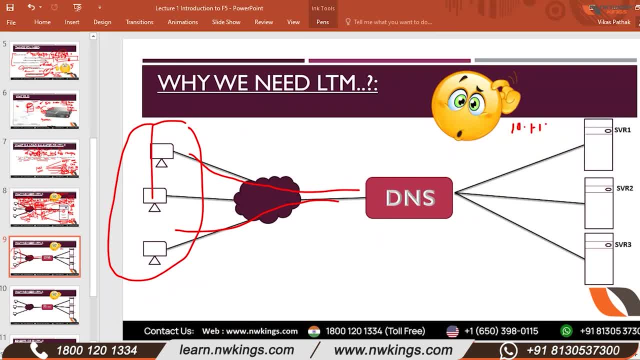 For server 1,. you have given 10.1.1.1.. We can use a pack file as well, right? Yes, We can use a pack file as well. You are making a pack file for an internal user, right? 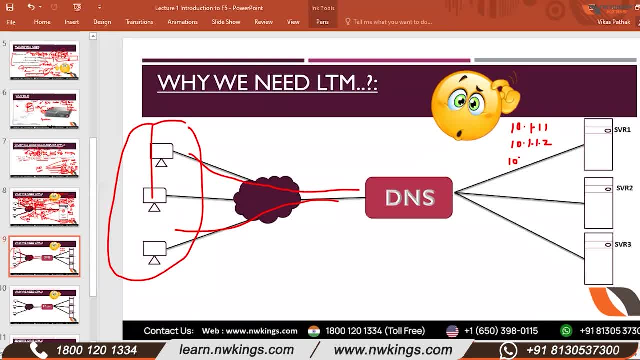 Suppose there is a user sitting in Jammu and Kashmir, Will you make a pack file for him for your application server? No, But we can assign a port to IP address, right? Let me explain. You told DNS that you have three application servers, right? 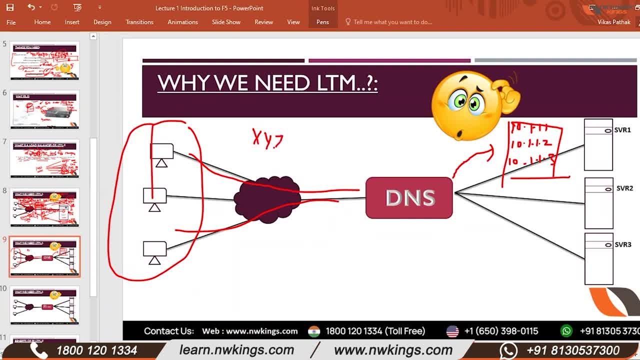 One is the URL: xyzcom. You said that when you get the first request, send it to 1.1.. Send the second request to 1.2.. Send the third request to 1.3.. Problem solved: Distribution is done. 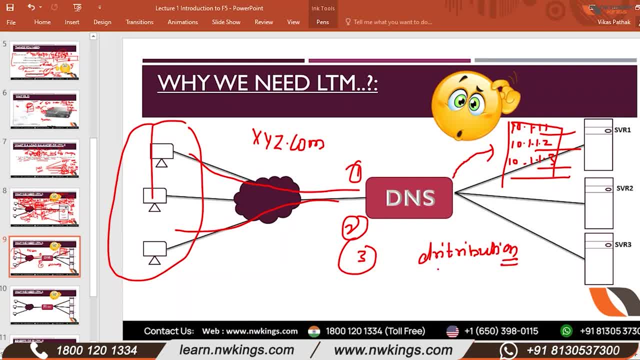 Just like IP forwarding. Yes, You said that. when you get the traffic, send the first traffic to server. 1. Send the second traffic to server. 2. Send the third traffic to server. 3. Send the fourth traffic to server 1.. 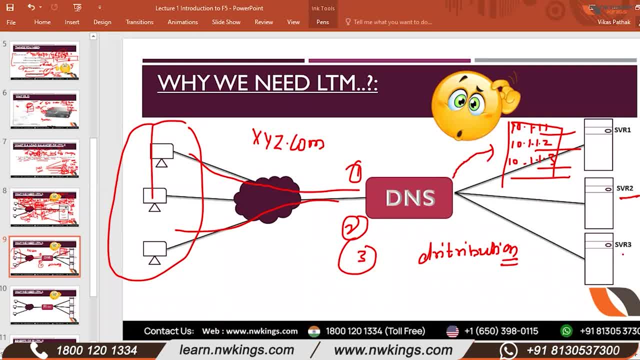 Send the fifth traffic to server 2.. Send the sixth traffic to server 3.. And this is how you have to distribute the traffic. You have to distribute the traffic between these three servers, And this method is called round robin. What is it called? 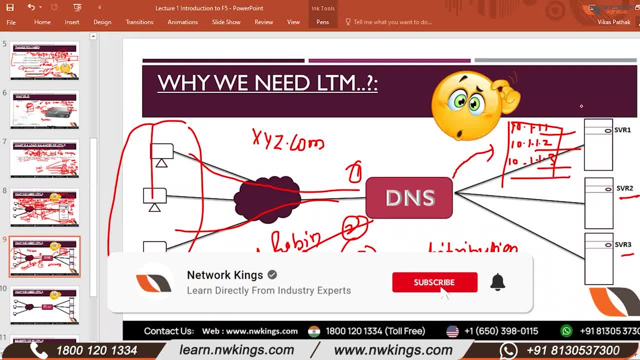 Round robin method that you are distributing the traffic one by one and sequential, And this is the most, most, most used method for load balancing, Not with the DNS, With F5 also, With Citrix also And the any other LTM also. 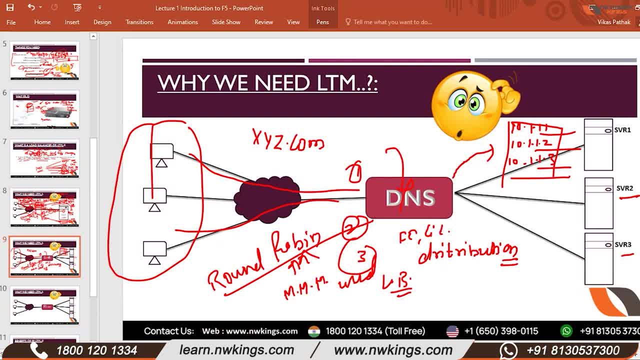 Round robin, Until. and unless you do not have a very big environment, a very big application server, you are managing. If it's small organization, small infrastructure, you are managing. small application server, you are managing it will be 100, like, not 100%, 90%, it will be a round robin. 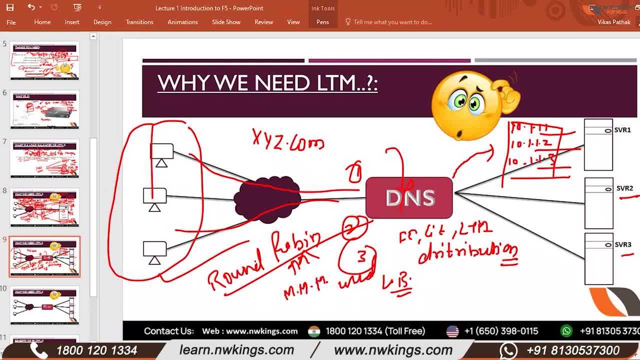 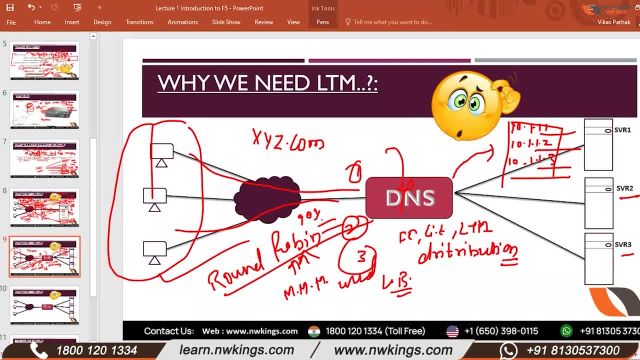 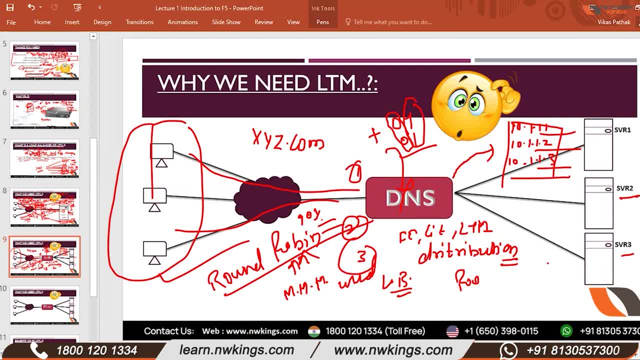 itself cannot maintain a session table like based on the source and destination. I'm coming on these those parts as well. okay, give me some time. I'm going like step by step. okay, sure, so the this thing, this part is clear or not, like the problem which we had here when we had nothing in nothing. 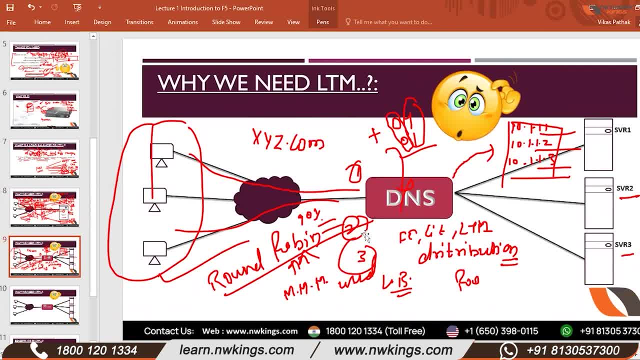 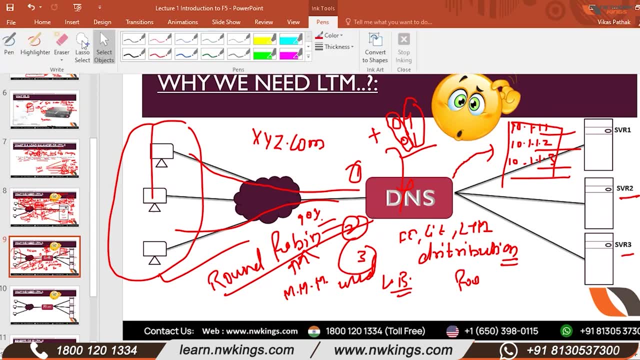 as a solution. that problem is being solved. solved right. yeah, do you think there should be some problem? yes, there are many problems. yes, because we have. we have to be enter manually, each and everything's enter manually whenever we require such kind of 5p, so we have to be. 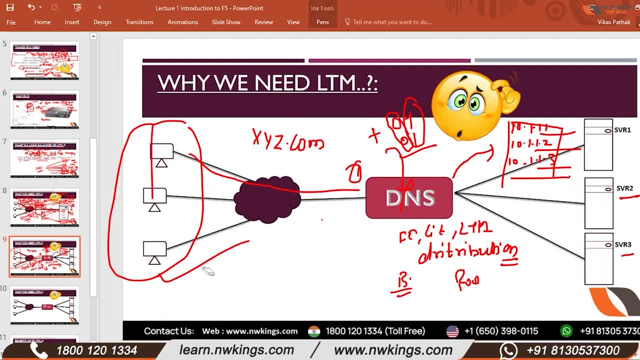 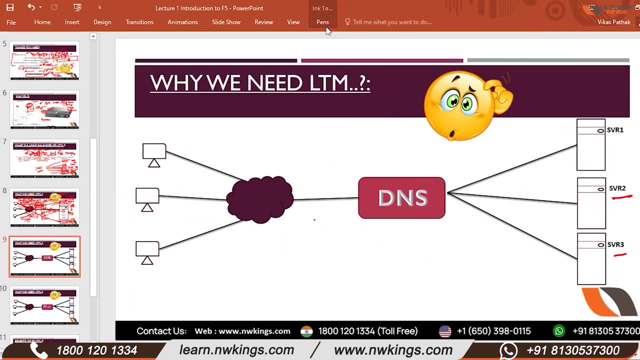 enter manually. the round Robin will not be effective. configuration, same in key power, same servers, then it will be very good method. no, if you do not have the same configuration and same service is being hosted on service. I'm not talking about the services I'm talking about. 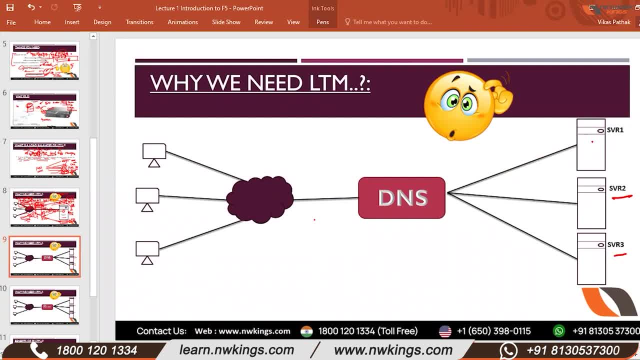 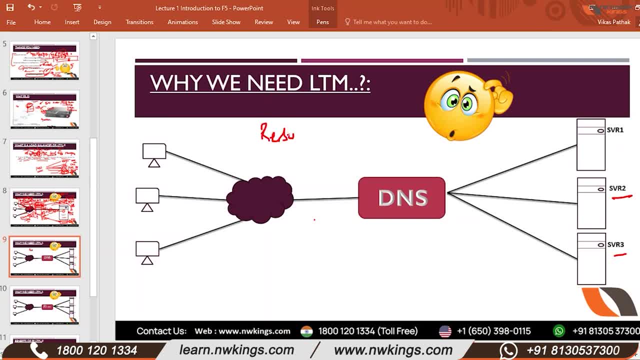 so in that case we should utilize it more. so it means round robin will be one by one: first it goes to 1, then 2, then 3. so then in that case it will not be effective. exactly, no, no, no, that's a problem of that DNS. 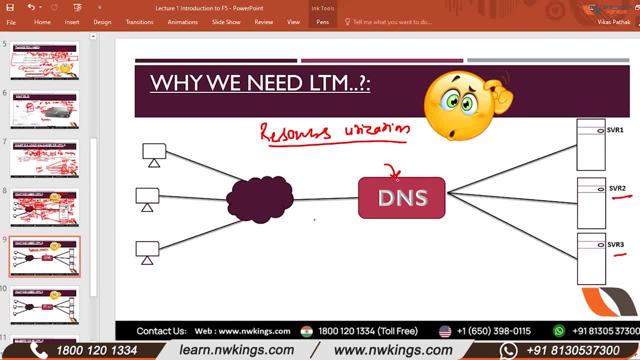 and the round robin we are using in DNS. right, yeah, but we have a see. I am telling you a little bit about next class. if you are doing round robin in load balancer, then you can do what it is called means. there is a mechanism in which you can do resource management. 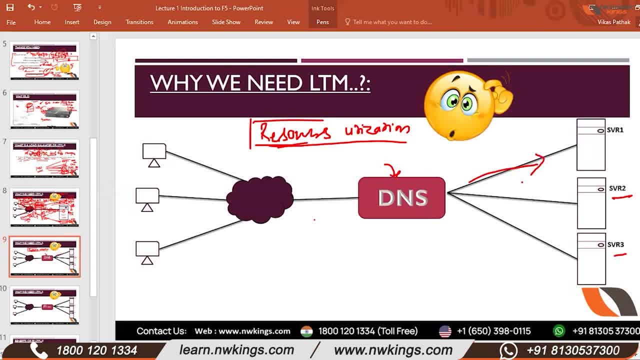 so what round robin will do? it will send two traffic to here- one is here, one is here- and again two traffic here. one is here, one is here, again two traffic here. this is how round robin will perform, right? I think it is called weight ratio method. yeah. 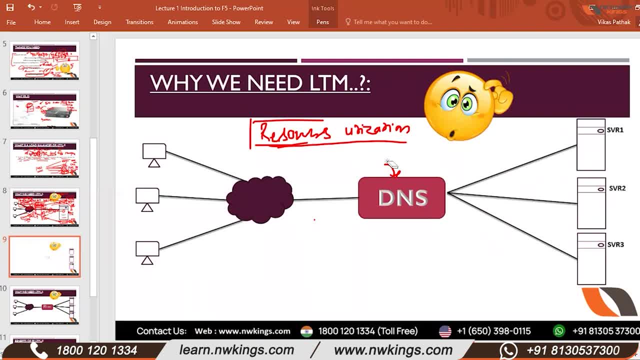 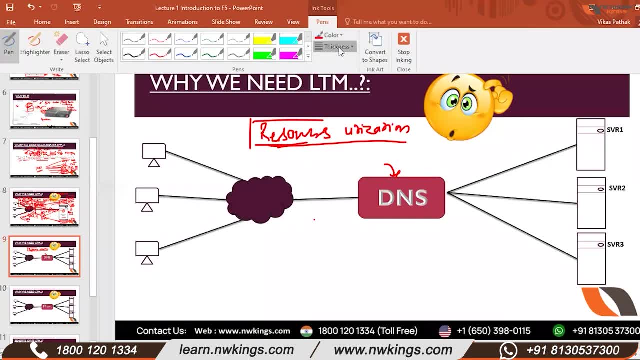 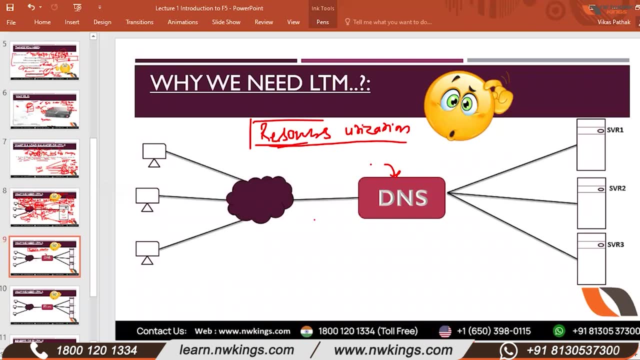 when we involving the DNS for distributing equality. but here, as you said, sir, there is distributing one by one application: one, two, three, so when it will send at the same time, to send to every one server when it can possible. I didn't get your question. at the same time all the servers should have. 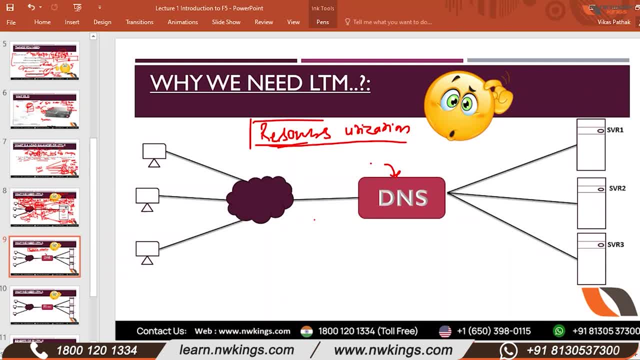 data send. why? why do you want that? because when DNS is sending one by one, it will take time. aha, see, it's not doing like one packet is receiving and one is sending. it's not like that, it's just it's a very fast process. it's not like it's very slow process. no, 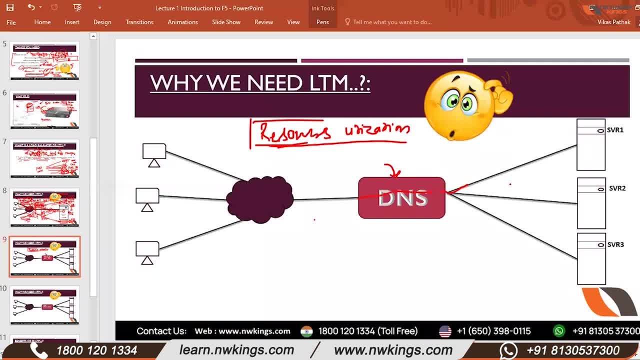 I am explaining this to you- that send one by one. this is to explain otherwise. one by one it's very quick process. yeah, I am sure it will send 50 of seconds. ok, but what is the reason we are involving DNS? ah, to solve our problem which we had in earlier session. 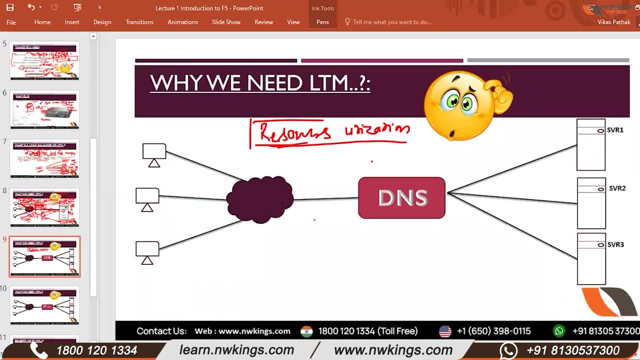 earlier. slide right. distribution. what about the balance of load of balance? wait, wait, wait. I am coming to that point. so just tell me this: in your previous session, the problem of distribution, was it solved or not? yes, sir, I think it should be yes, right, yes, what about weight management? 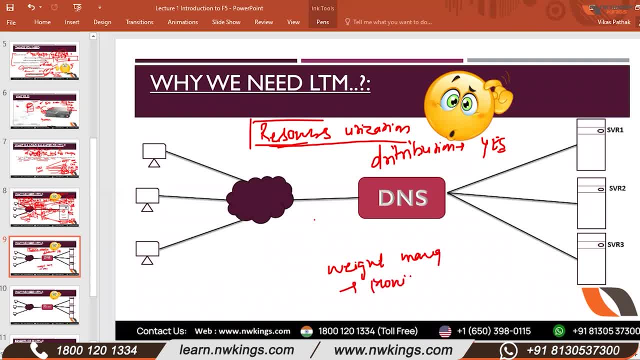 what about monitoring? what happened? what about availability? 443, 443, 443, 4GB, 4GB, 32GB. this should get much more traffic in comparison to these two, right? yeah, it is. so what about that? DNS can't do that. hmm, let's say: 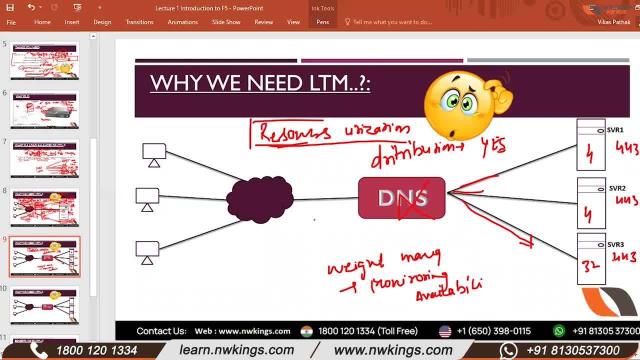 yes, let's say, this is your server 3 443's service is stopped. ok, ok, this service is stopped, then DNS doesn't have any mechanism to monitor it. what it will do? it will send the traffic here, here, here, here, here, here. so the client you have. let's say, suppose this is the first client, its traffic is going to the first server, the second client's is going to the second server. the traffic of the third client should have gone to the third, but in the third 443's service is stopped, but DNS doesn't know. 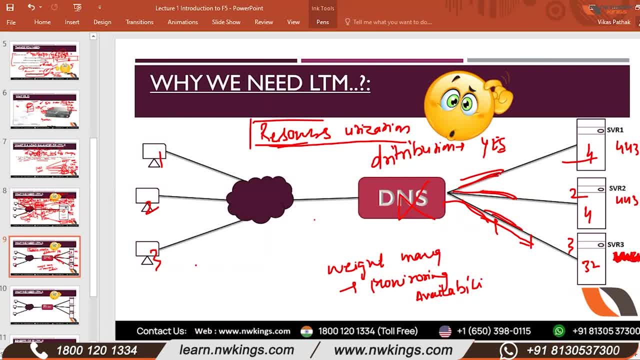 it has sent it to the third and it got page does not respond. so what happened? it is like a hub, yeah. so what happened? as soon as it got page does not responding. what happened? it thought that flipkart is not working. what to do? go to amazon. 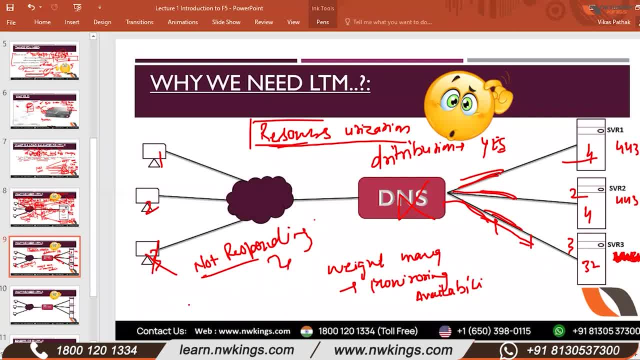 the customer went from here. yes, so monitoring is the problem. the server got stuck. in that case, what it will do? same problem if 443's service is stopped. what will do? DNS? it will send to another application, or no? no, no, it does not have any mechanism. 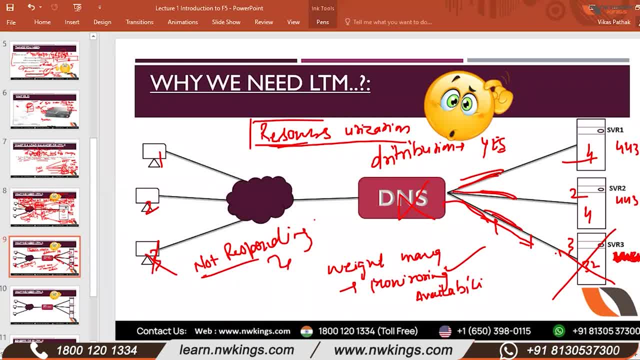 to do that, ok. ok, now server got stuck. destination host: unreachable, sir, but alert will be raised if that will be with you. you are, you are IT administrator. you should have alert. if you don't have alert, then it will continue. that user will never be able to access. 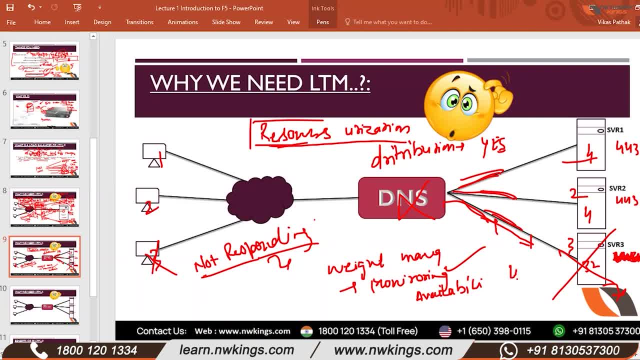 the application. but for, let's assume, alert is raised, it will take 4 minutes to restart that service. for that 4 minutes traffic is coming to it. or you went to DNS and you said don't send it. ok, now alert has come. that alert now. it is not like. 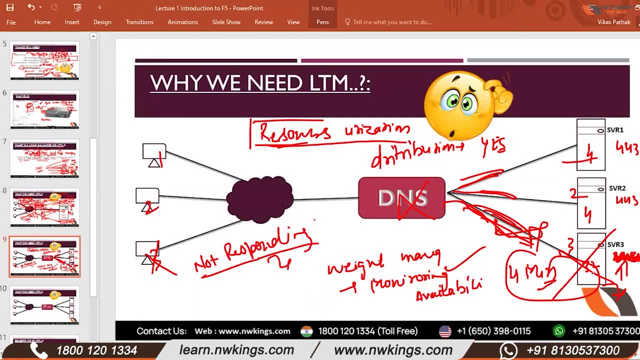 within a second alert is generated and the engineer understood that server 443 is down within a second. he logged in and sent a problem in a second. it doesn't happen in real life. yes, at least I mean it is a very good environment. it will take 2 minutes. 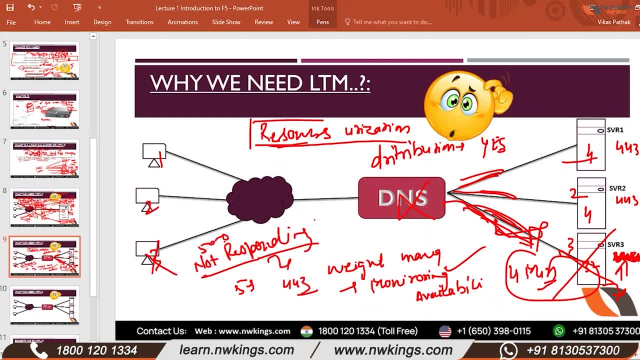 to update this service and for 5 minutes. if, let's say, 5000 users came to your server and they saw destination host, they will say: flipkart is not working, we have to order a bottle. let's go to amazon. so 5000 customers are flipkart. 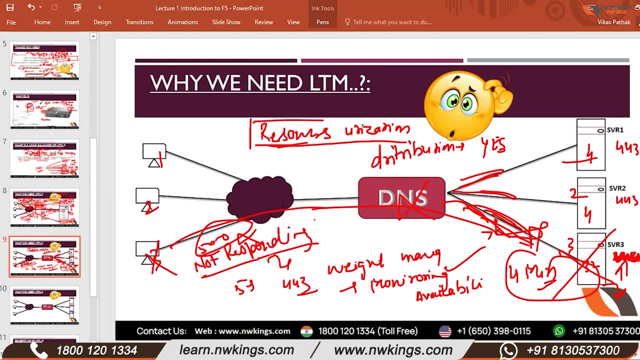 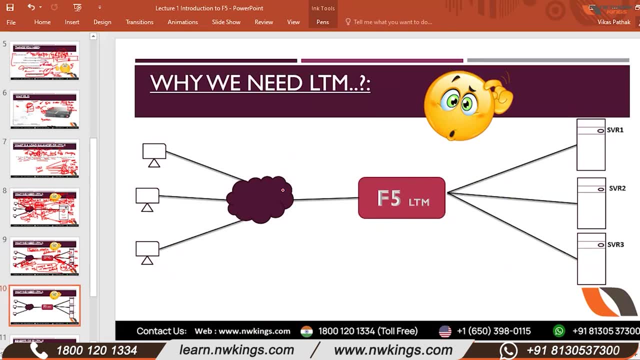 right, yes, so these, these are the problem with the DNS, right? because of this what we did, we brought the answer: yes, yes, yes, ok. now all these problems, all these problems. number 1: distribution, for which it is made, he is doing it, ok. number 2: monitoring. 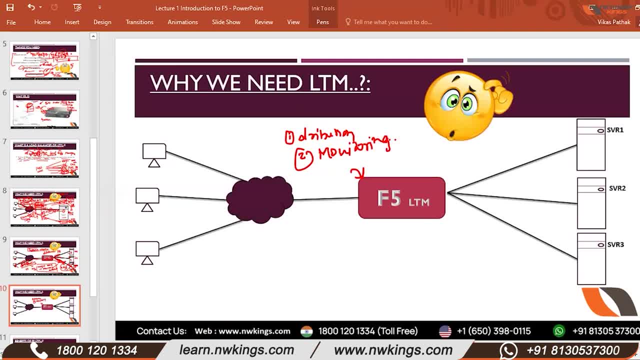 he will also do this how, always at some time interval it will keep ping 443 service and it will make sure that the traffic it is sending to server 3, then 443 service, is running on server. otherwise it will not send the traffic on this server. 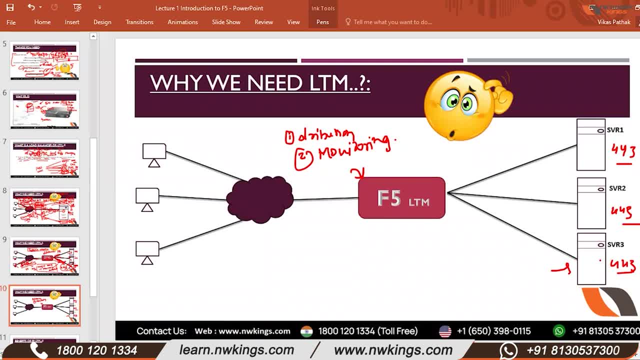 also, if the service is running, then only it will send. otherwise it will not send. otherwise, can we can? it will be indicate to user. no, why? why should? is user should indicate like server is not running. we can monitor. it can indicate to user. the server services is stopped. 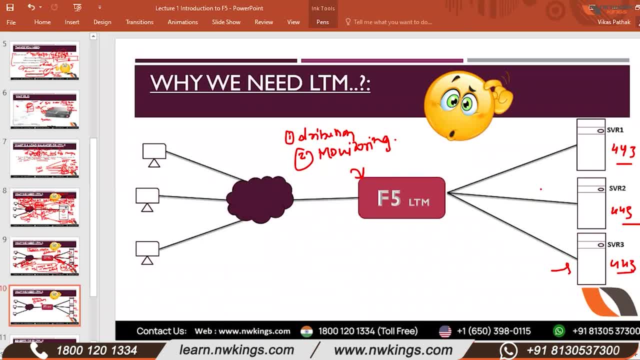 user don't know. that's why we are doing these things. what what you need to monitor if some server is getting a problem with the alert. but is there any monitoring tool we have to check about the alert? see, there are multiple monitoring tool in the market- solar. 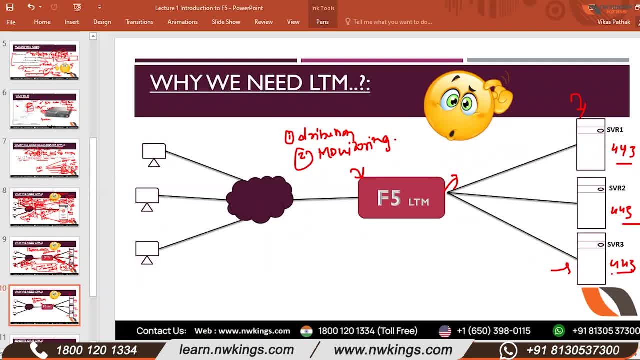 wind op manager spectrum. multiple tools are available to monitor the server, but this port is not responding. take care, so can you tell me the what exactly error we get? error is not responding, the port is not working, so there will be a black status that it's offline. 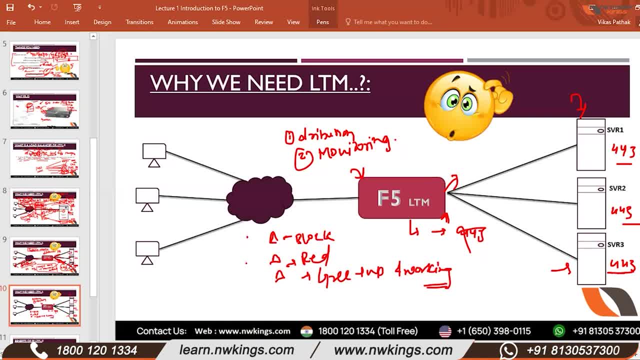 red down and green. it's up and working correct. so these are the states which so on the right about member member member service is not responding. this will be the error. okay, so you have ip dna 1.1, 1.2, 1.3. 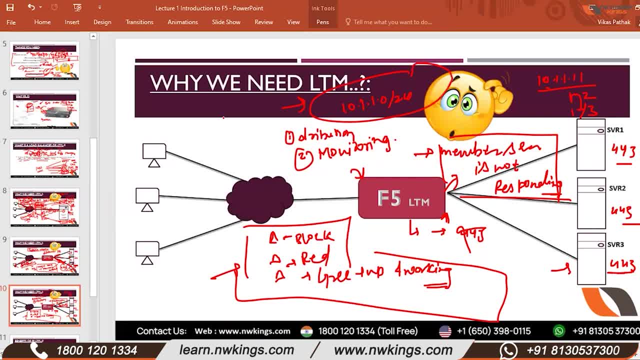 so this is called pool, what it's called pool pool, what is pool pool is the sub, like network of the of the, in which we create the servers. right, and i think someone is speaking without mute, okay, so this, this was the you know um basic, okay, key by. 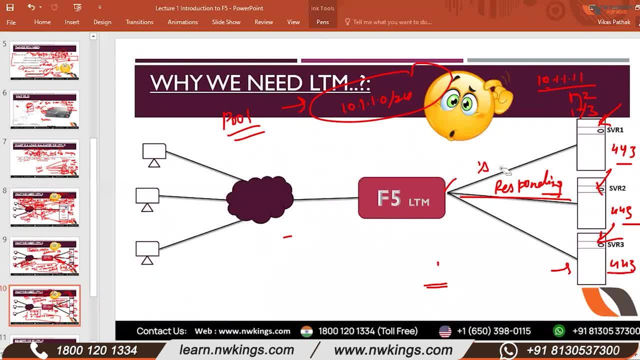 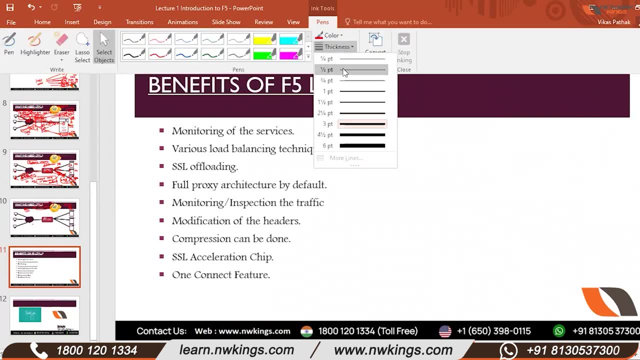 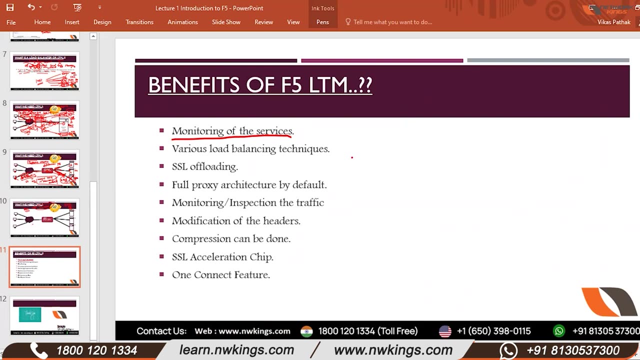 load balancer to um and what benefit we got from load balancing. now i will tell you some benefits: monitoring of the services. you guys understood right. yes, this is setup, okay, okay, monitoring. so i explained to you that when i talk about f5 or lte, various 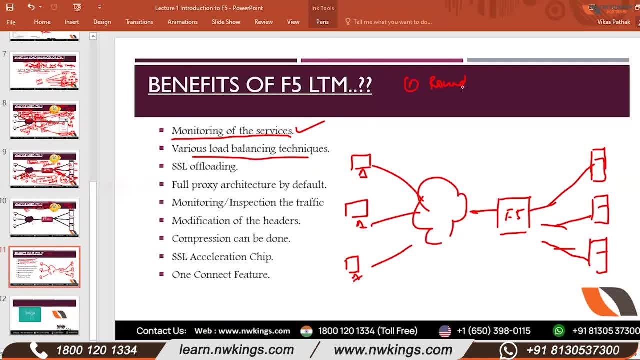 load balancing technique. first load balancing technique: i told you round robin. see, if i talk about a practical scenario, then never application servers are created like this. that i gave one. this is how application servers gets, get deployed. so round robin works very well, but in any case, let's 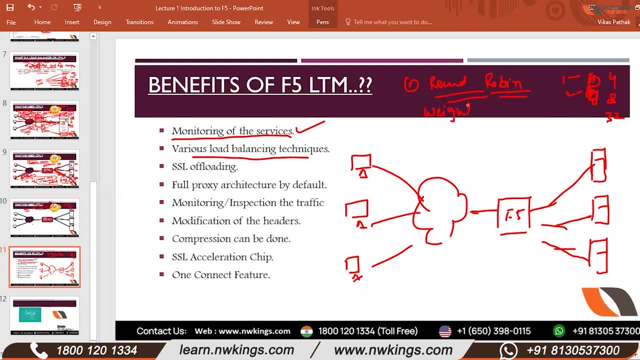 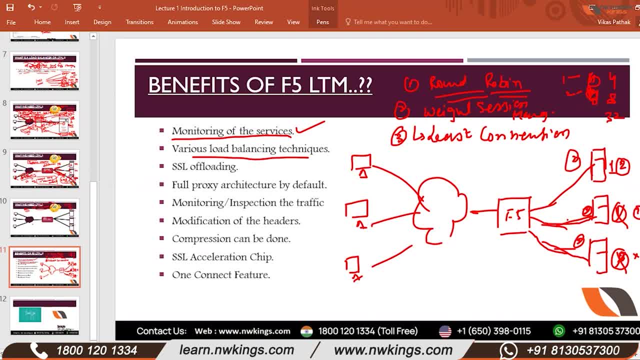 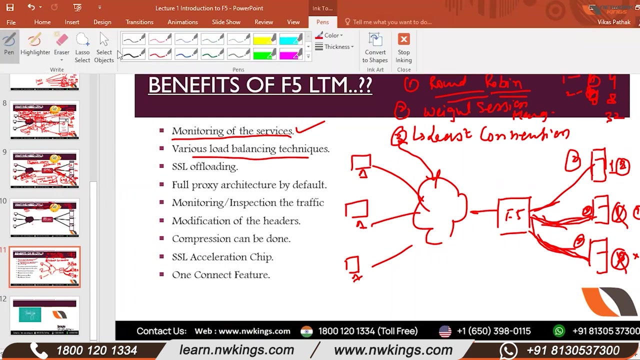 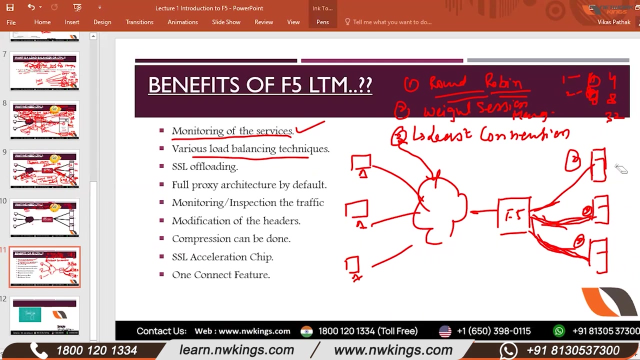 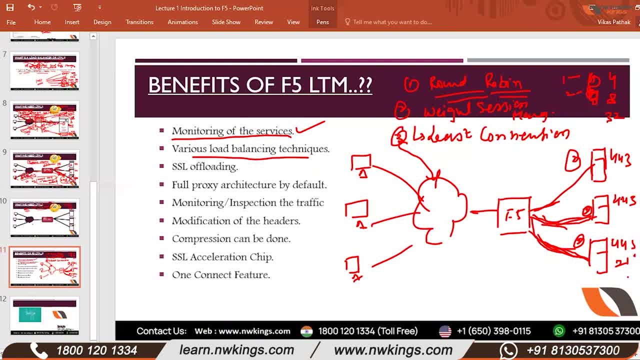 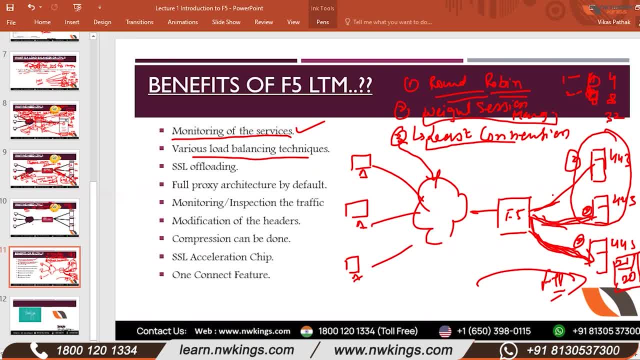 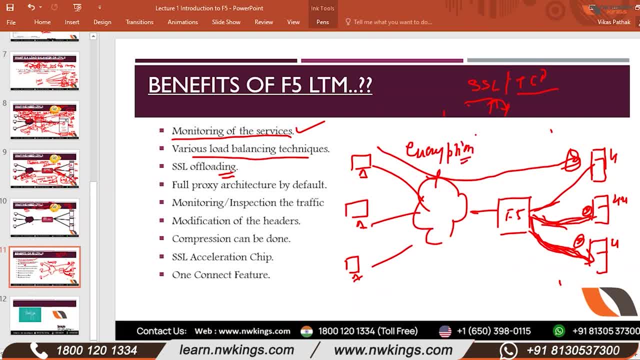 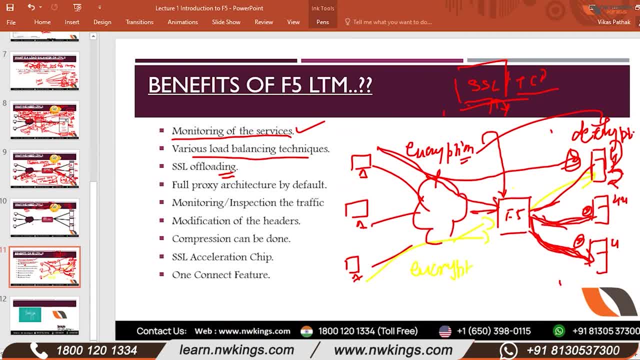 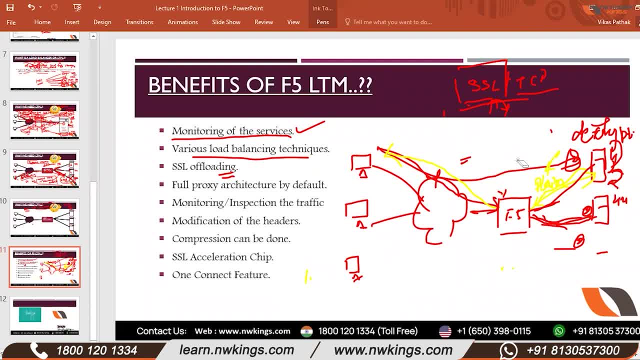 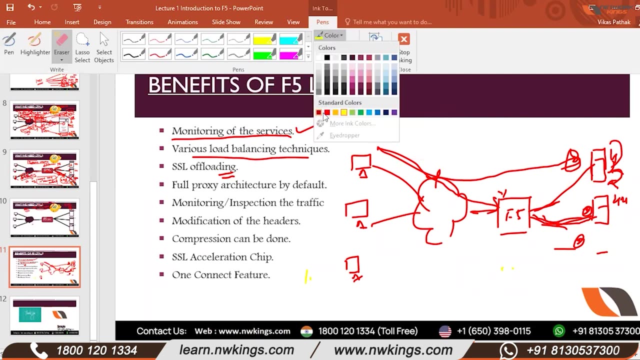 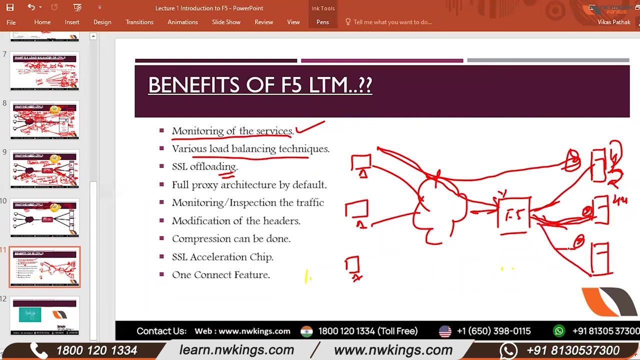 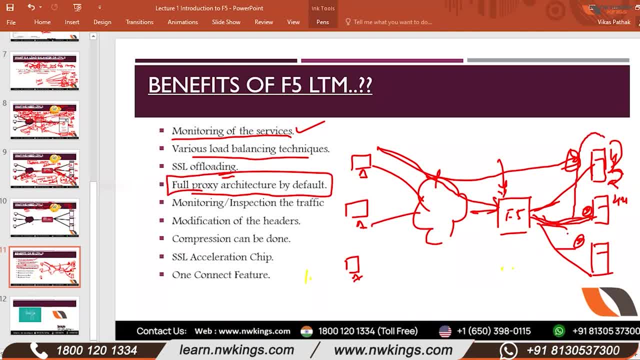 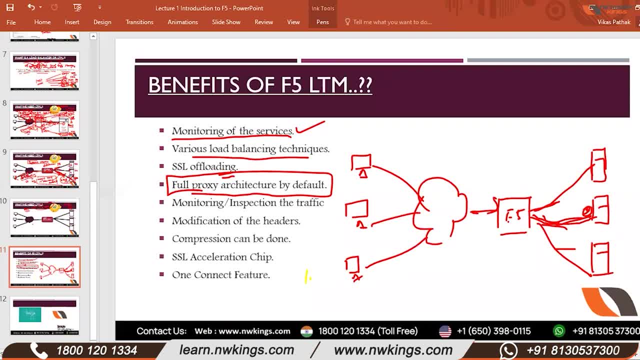 Make sense. I mean F5 will make a table, ACL will make a table, monitoring and inspection will be done here. What is monitoring The traffic of port 20 or 21, how the F5 will know that. I will send it here. F5 knows that. 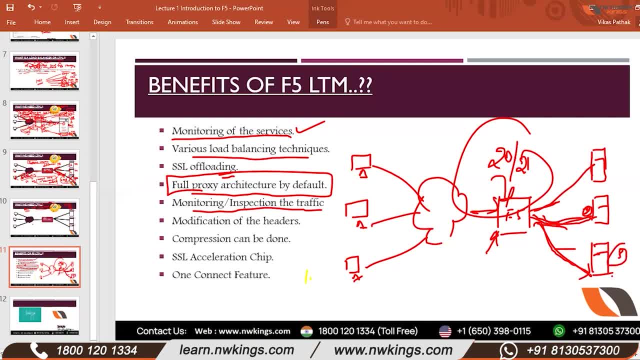 on this server, on this specific third number server service of 20 and 21 is hosted. But the packet that has come in that request of this port, how it will know It will inspect the packet Right, If there is an inspection then it will understand that send it here instead of 20 or 21.. 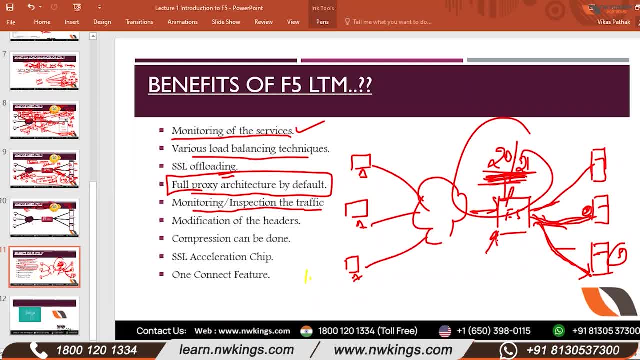 Right By the monitoring, By the SSL offloading, Decrypted the packet, checked inside that. what is the application send it here of 20 or 21.. Inspection And what does monitoring mean? Means that if the traffic I am sending here, make sure that this is the server and service. 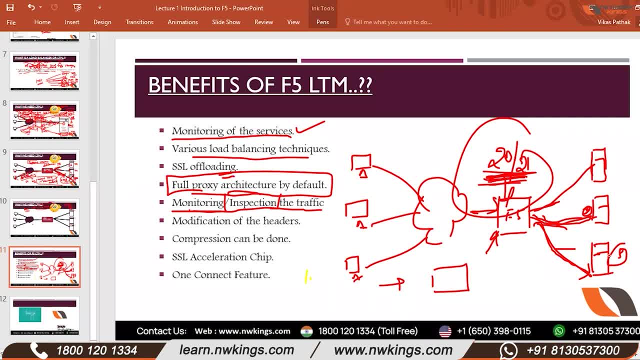 is done. this is the monitoring here, Correct? Yes, Come on, we have monitored, Okay, And we also did the inspection. Apart from that, another feature is modification: Modification of headers. I just told you that there is a traffic from client to virtual IP. 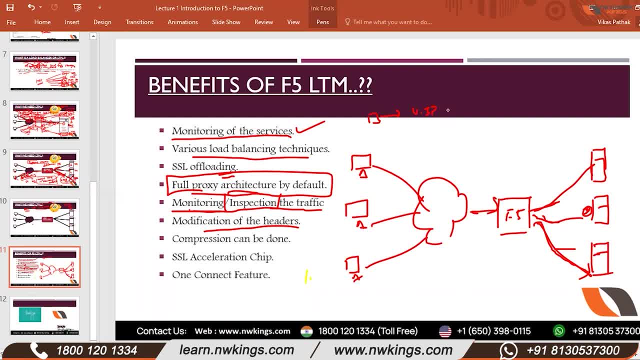 Sir, I have a doubt. In this infra which you explained, there is a single point of failure. You said multiple servers are being managed by one F5. You can connect one more here, Okay. okay, For redundancy, we have two F5s. 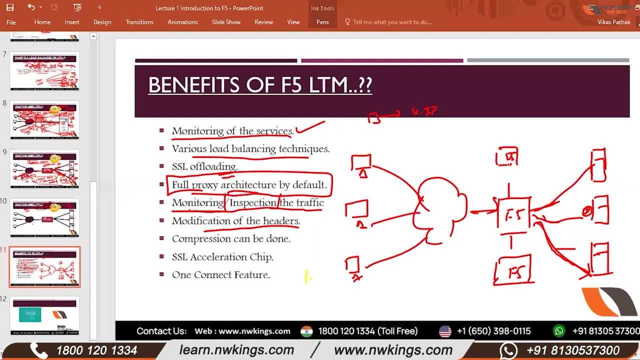 You can create one more here. It's up to you. It's absolutely up to you. We are not talking about high availability feature set here. We are talking about F5.. Why do we need to use it First? we have to understand this well. 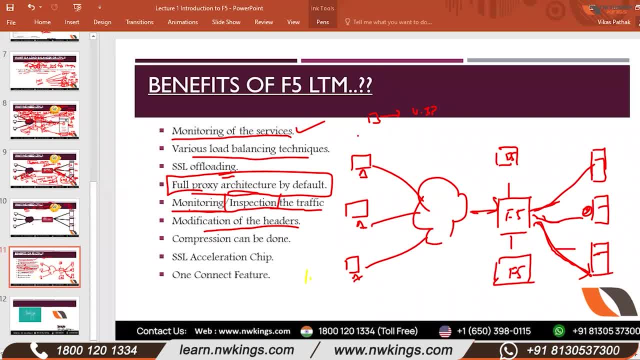 Okay, okay. Modification of headers. We said that there is a traffic from client to virtual IP. Where is virtual IP On F5.. It is on F5.. F5 converted virtual IP to physical IP. Where is physical IP Here? 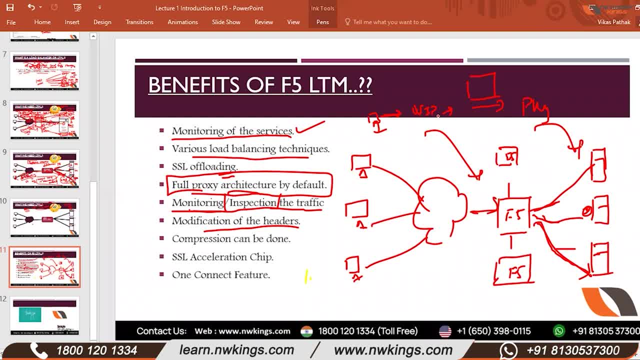 So what did it do with the packet Before routing? did it change the destination IP? It did. Did it modify the IP packet's IP header? It did. So it's similar like an adding right. Yes, Okay, Compression can be done. 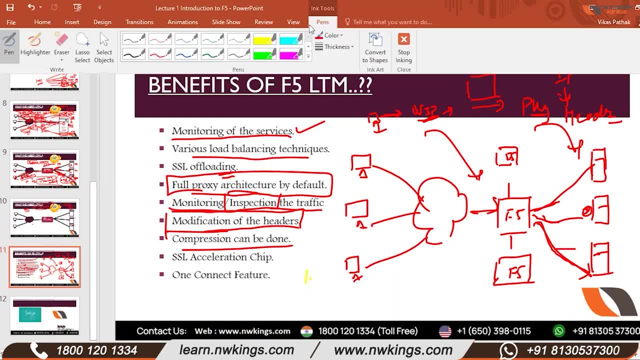 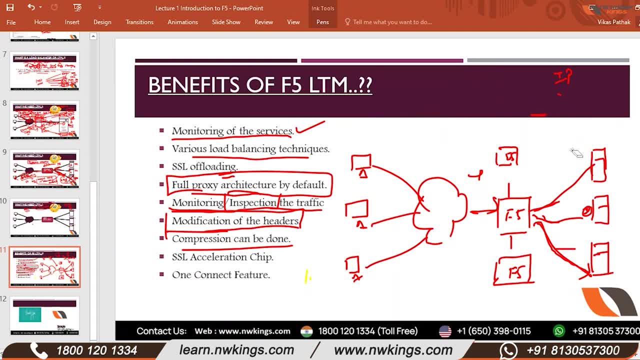 Tell me quickly what is compression. Tell me in a very short time. I do not have much time actually, So tell me quickly in a short time what is compression. You are compressing the size of the date file. You can make it lightweight so that it is easy. 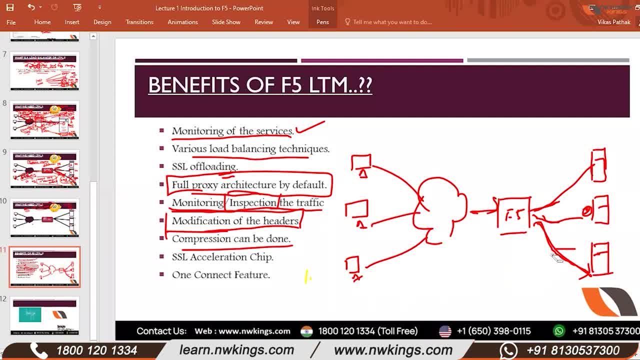 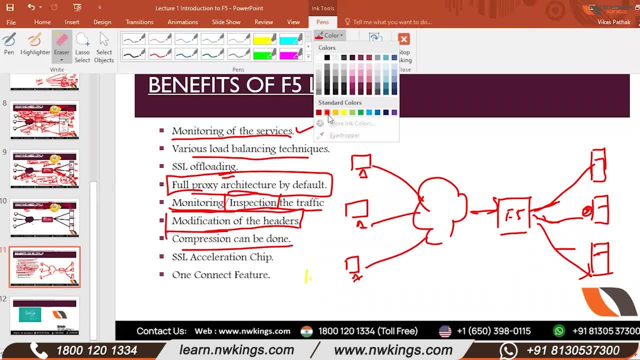 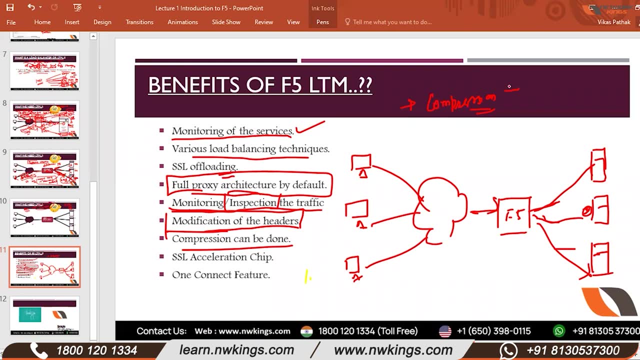 Producers can send it to the receiver And it is not stuck in the network. Hmm, What type of compression is there, Not sure, sir, You have told me the meaning of compression. I used to say the same Compression. It is a general term, that compression. 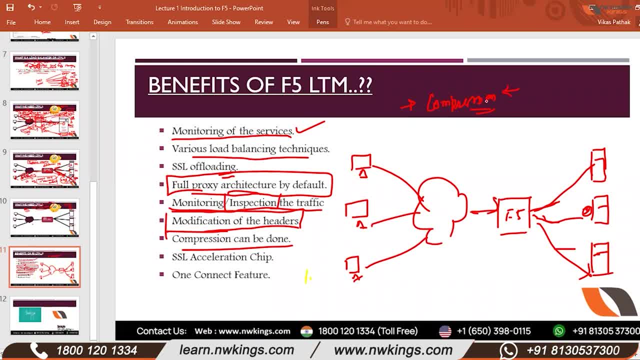 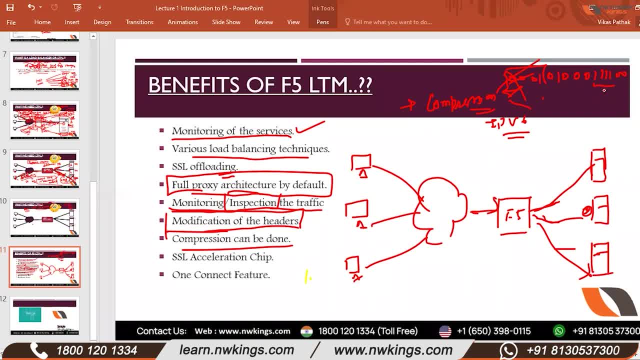 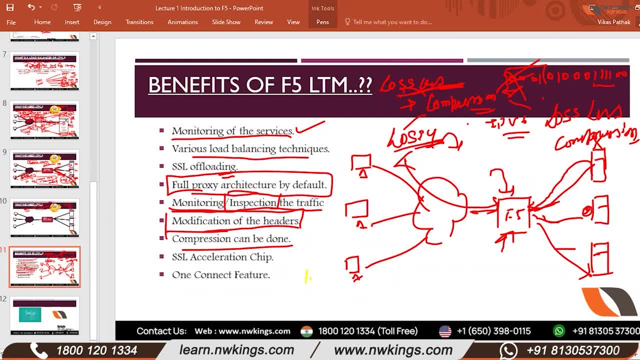 whereas in lossless compression it's not possible, right? okay, so i have one more questions. i'm not about to this infra. we are talking about the server only, right? so whenever we have connect virtually from like a vpn- uh, usually now we can work like work from home, right? so f5 we can use as a client to, you know, connect. 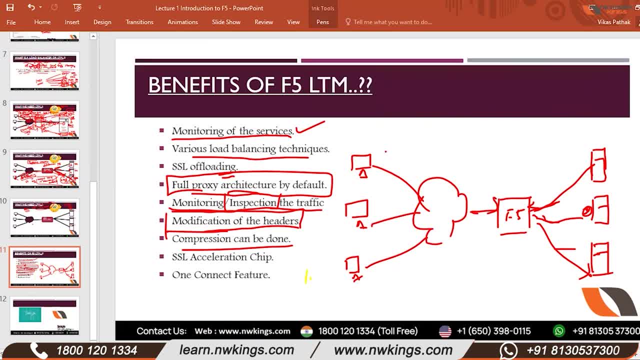 uh, vpn process. vpn process, i mean. my question is that somehow we have right away- we work as a work from home, so we have to use a like a big ip client here- some of vpn tunnels to access our organization servers switches out. so how, if i can be, uh help to do that? no, there will not be. 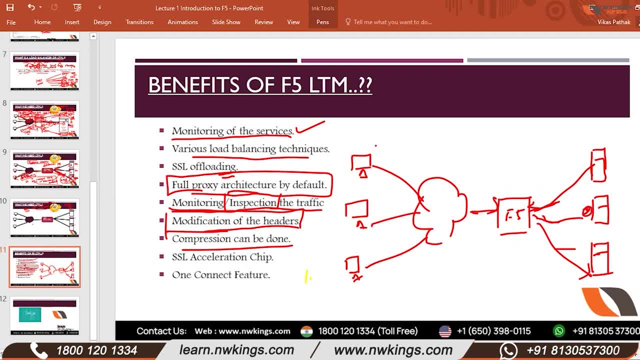 any help in work from home setup from f5: see: try to understand the difference between a firewall and a load balancer. firewall is to protect your network and give you access right. load balancer is to give you maximum availability and better utilization of resources. but we can create the policy right rules on the f5 too. 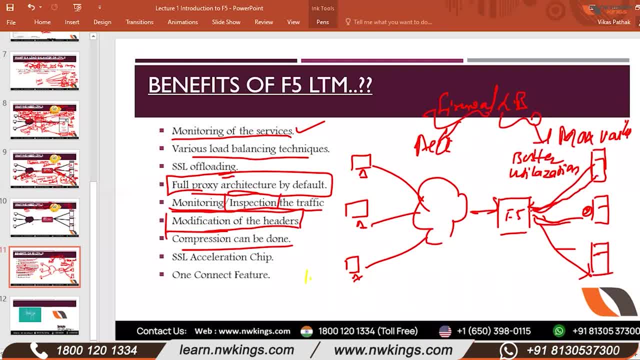 rules to access this thing, you cannot deny. so where we built this f5 device? actually before your server, before your application server. so it means we can access the access. access from anywhere, i think, f5. why you want the access of f5 from anywhere, like, uh, as he said just before the guy was. 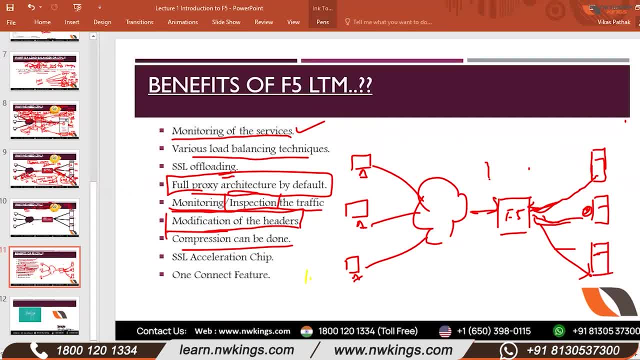 see administeredMI. for administrative purpose. you can access, just like before, the thing. you don't have a dual and network as, so i have no idea of what it. is it from anywhere, but the user don't have any visibility of F5. it's an administrative job. 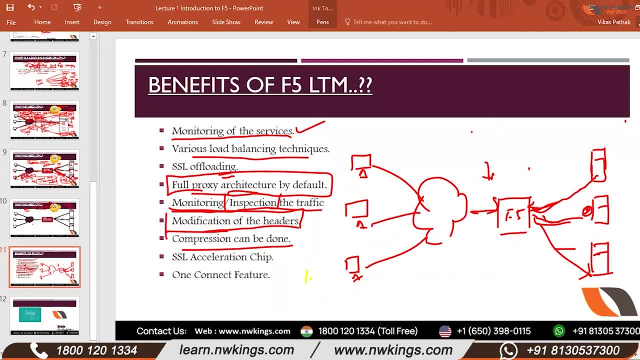 VPN may user. yes, please, yes, sir. actually what he means that in our organization client use a big IP client to connect the VPN to our organization. so he mean that, whether this big IP client software is configured, managed by F5 or not, well, I'm not sure. I need to check. 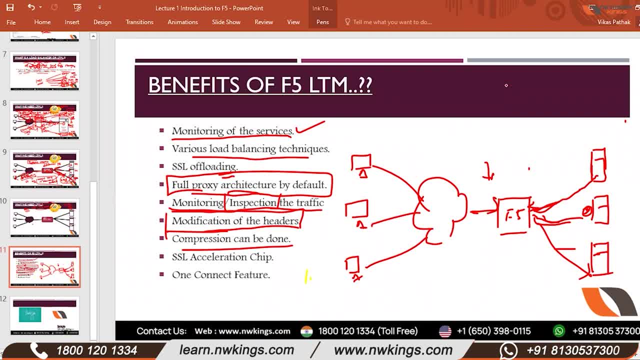 because it's. it's a F5 or what. how infra is in our premises, that big IP client which is installed in the end user system, which is managed by F5? correct, this is in our infra. that's why we want to know whether VPN kind of connectivity give, provided by F5, or not. see till now I don't think. 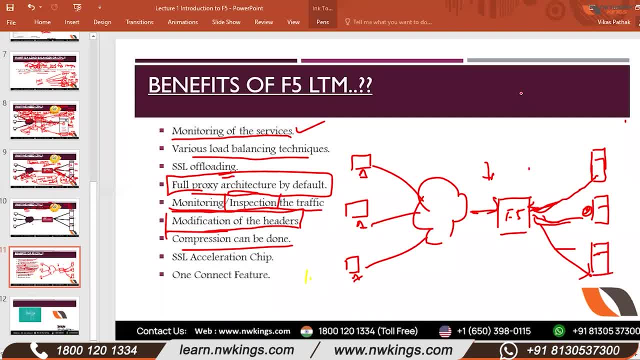 that such sort of connection, like a solution, is being provided. but definitely I'll go today and I'll check if such kind of setup is available, but I don't think so this will be available, I think, when we build a F5 device in our organization as a administrator, wherever whoever can use possible. 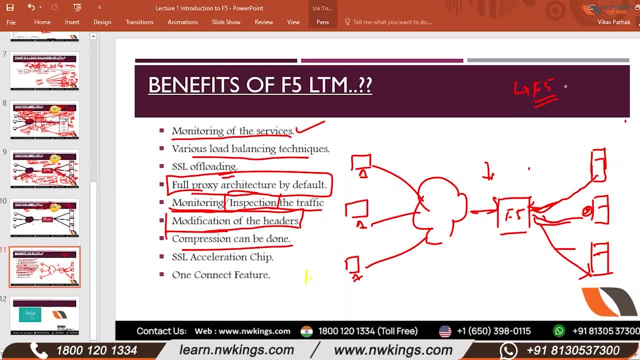 if possible. so it means automatically F5 using the in the network. I think hello hi Atul, this side from networking. so basically, guys, yes, F5 provide SSL security layer, but that is a different module, which is ASM. ah, web, okay, yeah, web, basically application security manager that support SSL VPNs and 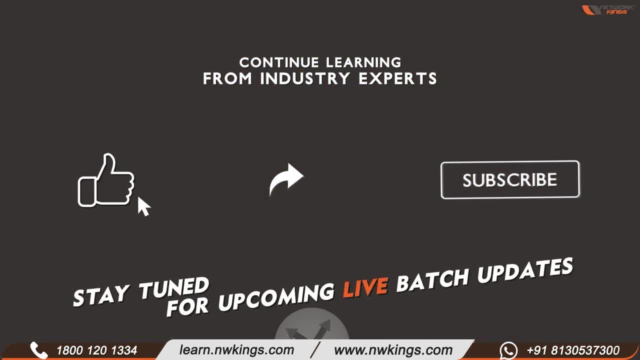 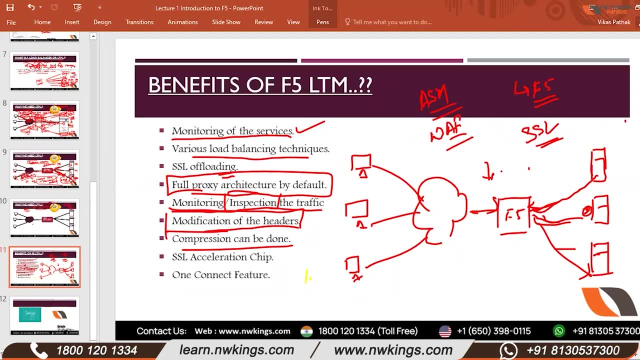 I think, hi, you are watching the recording from one of our live session. hit like share and subscribe for more future updates. these guys are asking about this. yeah, yeah, I thought I thought the question is for live session. yeah, yeah, I thought I thought the question is for live session. 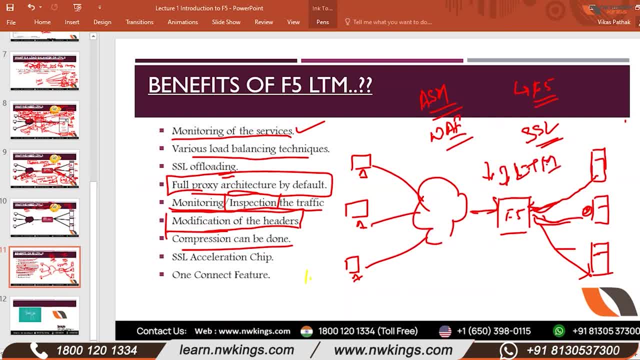 like ltm. through ltm we are connecting. what we are covering here is ltm module which is going to load balance the traffic to the servers. so if you want to learn that apm also, you guys can put your inquiry to networking. we will definitely come up with the apm module also. okay, thanks for the. 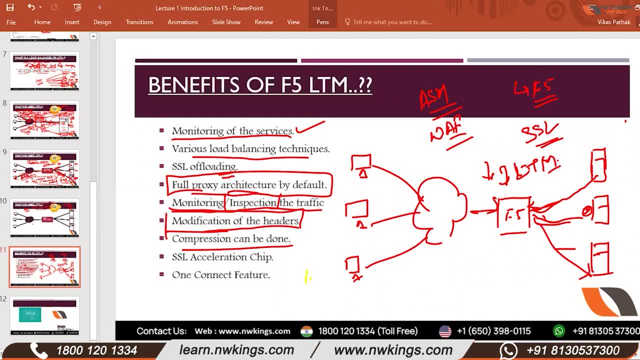 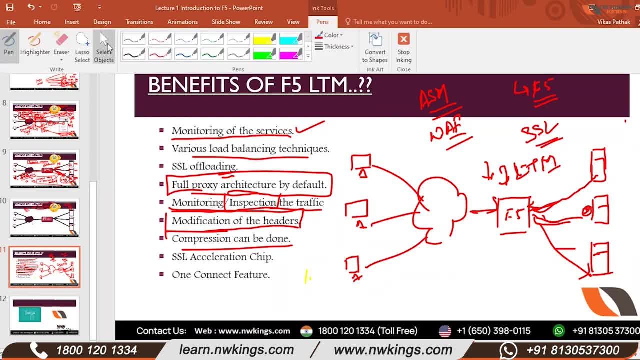 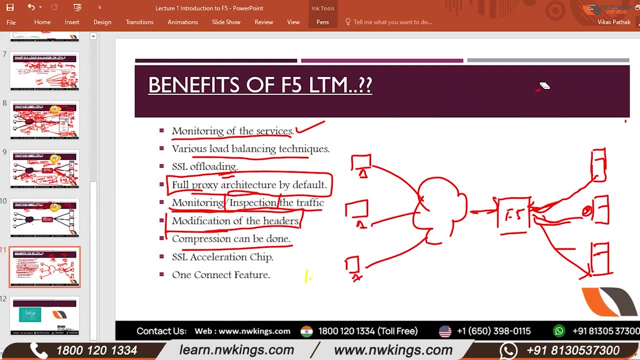 yeah, thank you. okay. so, guys, two more things are there. okay, let me just quickly cover these things too, because we have. we are running out of time, so, um, i think another thing is ssl acceleration chip. you know, um, i will recommend that we will discuss it in the next class. okay, about acceleration chip. 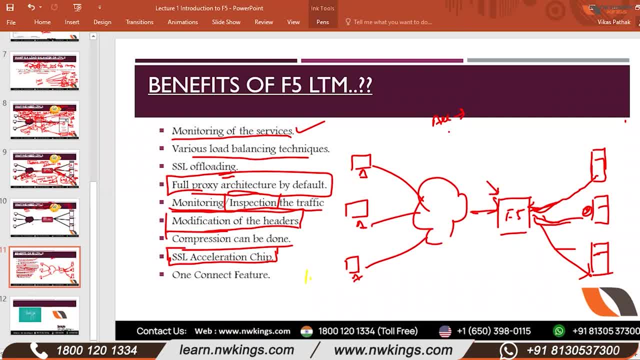 which is inbuilt in f5. actually, i am telling you okay, but we will go into deep understanding about this in the next lecture. before that, we will give one connect. sir, wait for five minutes. one class is going on for five to seven minutes. it is just ending. 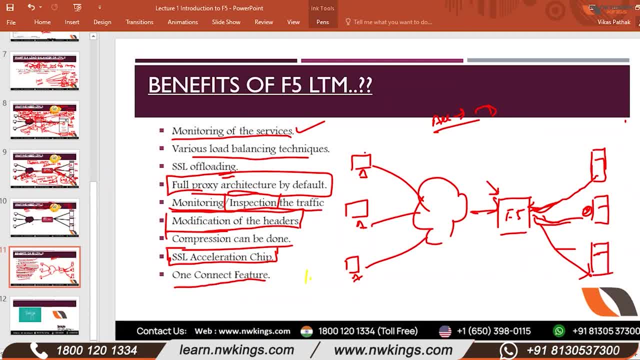 one connect, okay, one, what is one connect, gaurav, i think you are on on unmute, okay, so guys, um, okay, what is one? okay, sorry, guys, you can continue. i'm so sorry because actually i forgot to mute myself. thanks, thank you. so one connect, one, what is this feature? one connect. 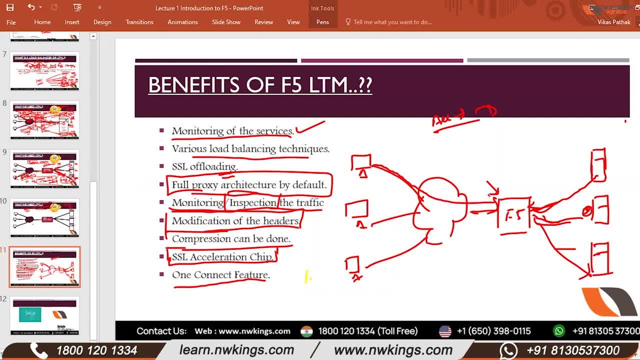 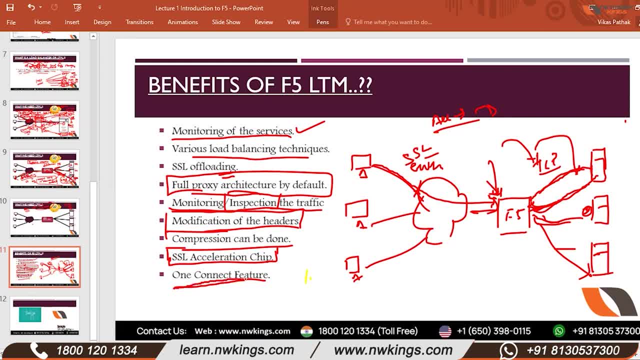 is a feature in f5 which is called one connect. what f5 will do. f5 will terminate the session which is being, which is established, between client and f5, but it will not terminate the session between f5 and the server. okay, so what it will? 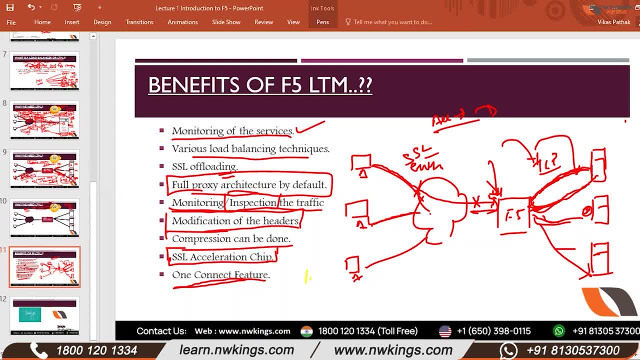 do when another client will access, will request for the resource which is available on server one. it will use this same existing session to provide the information. that is called one connect okay and to like one. one more feature is there in f5 which is called I rule it's. 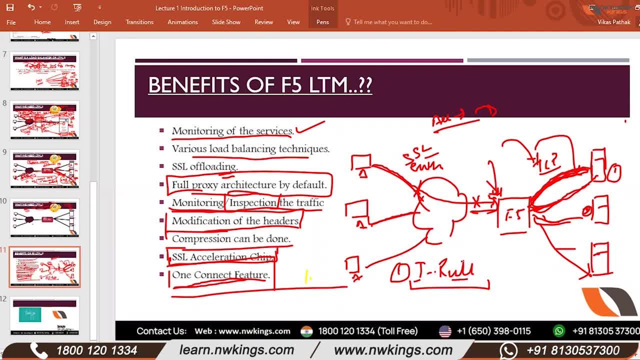 it's a very big feature and very big concept, basically introduced by f5. what it says: okay, router met refused. yeah, yeah, OSPF used here. oh, I didn't. someone is speaking on thanks, thanks. so, Malaysia, I refuse, but the working of OSPF is not sufficient for you. 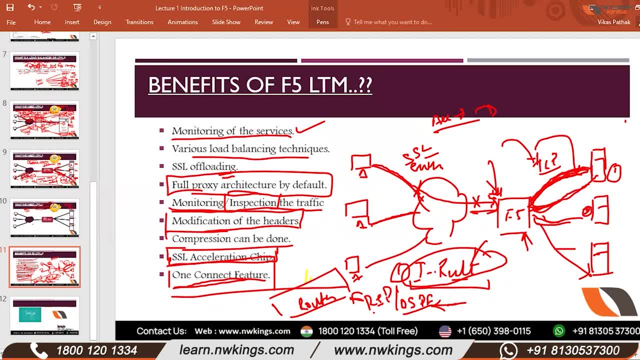 then you cannot tweet this ospf, you cannot tweak rip, but you can tweak f5. you can create i rule, skip through a scripting language and you can. you can run that, that that program on f5 and f5 will behave as per your- uh, you know- command. 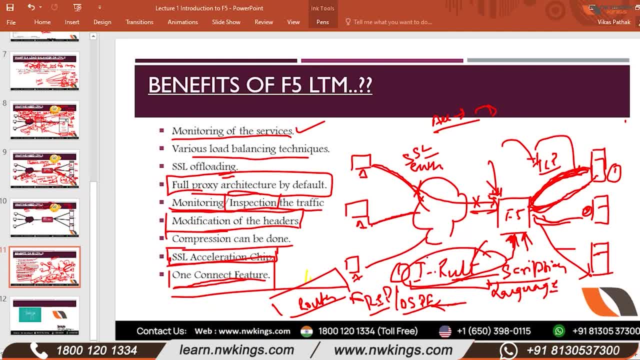 that is i rule and it's it's a fantastic feature provided by i rule and i think personally this is the one of the feature through which f5 is leading the market now, because everybody want to modify, everybody want to tweak the, you know, tweak the devices as per their uh. 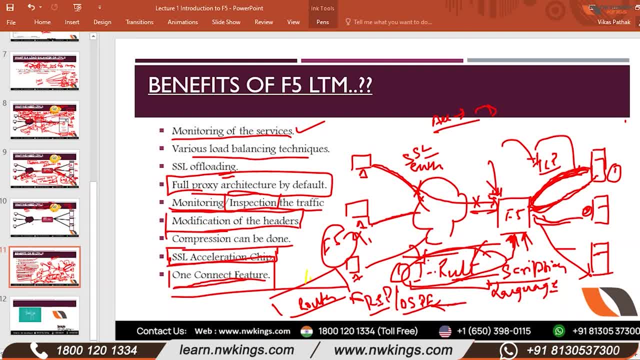 requirement flexibility f5 is providing, i think i think basic of f5 i have discussed here, apart from this ssl acceleration chip, because i think i will take at least 10 minutes to you know, explain this. so that is why i'm leaving it for now. for sure, in next session i'll discuss. 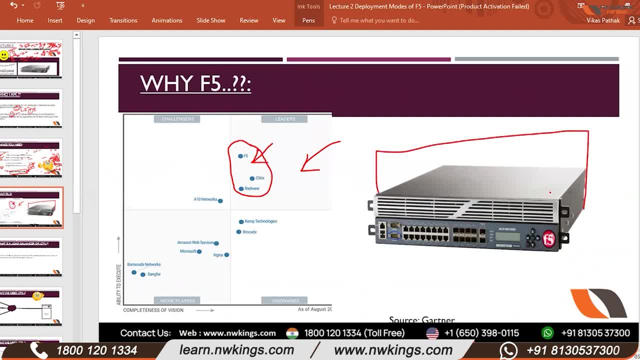 f5. this is the box of f5 8900 series. this is a very good box. i say i have worked a lot on it. if we talk about the ports, then something like this is our whole section which is attached to the nick card. this is the ethernet. 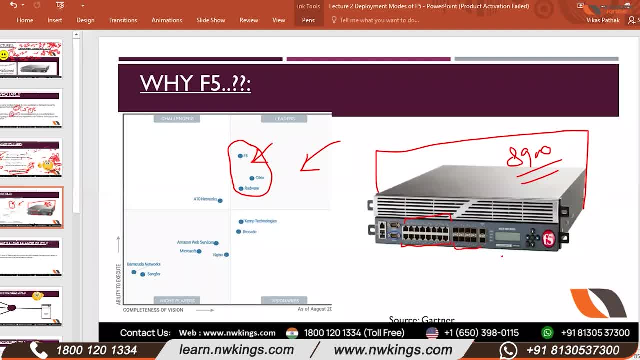 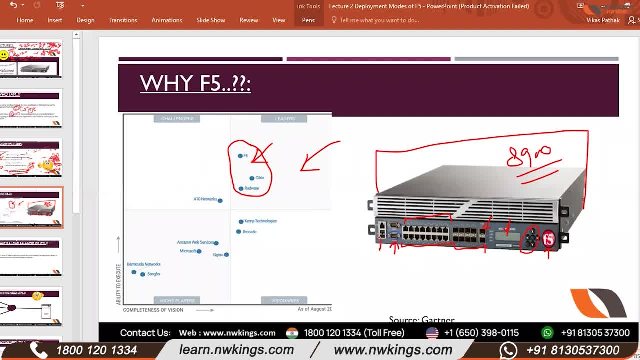 so now we are going to see the pieces in detail. so this is the management of f5 automatic admin: you di 192, 168, 1.245, etc. default IPs: It has password set By default when we buy new If there is something new. 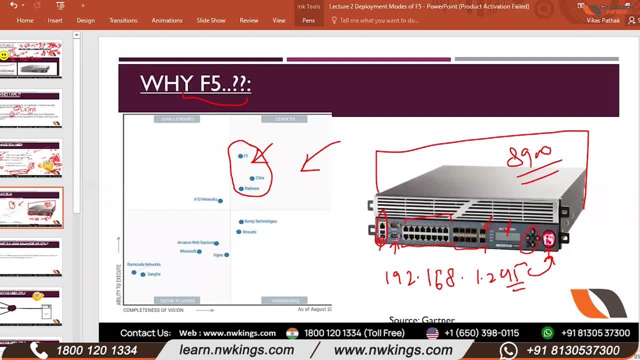 then you can check on google for this model. what is the default password? Ok, What will google do? The admin guide of this particular model, which will be published. in that admin guide, username and password will be published on the front page. Ok, Ok. 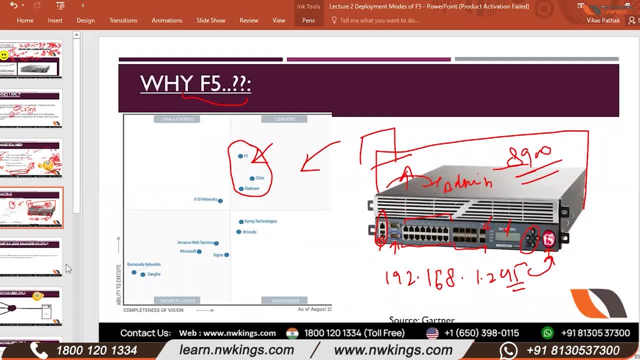 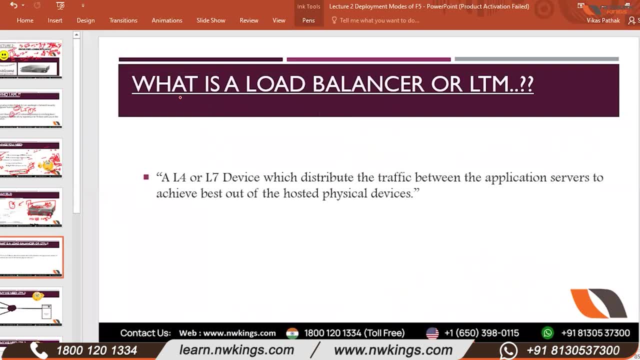 Ok, Ok, Ok, This question comes first. This question comes first. What is a load balancer or LTM? What is a load balancer or LTM? LTM stands for stands for local traffic, local traffic manager. Ok, Load balancer. 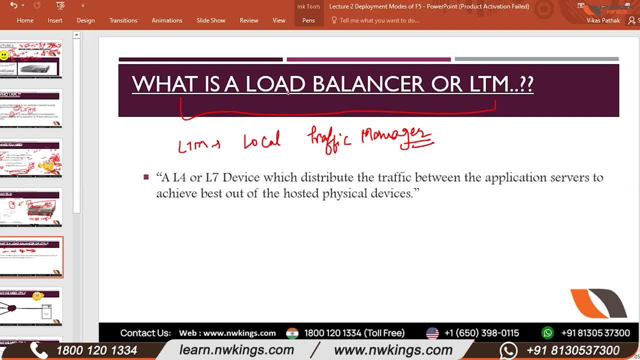 will be used very less in the market. This is a load balancer. Load balancer is everything which is balancing the load, But if I talk about F5 and the module which we are going to read, that will be our traffic, local traffic, local traffic. 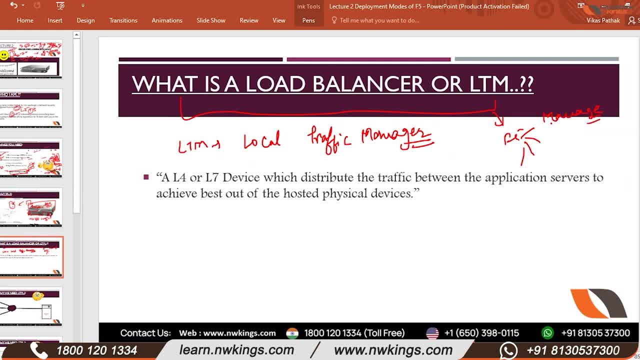 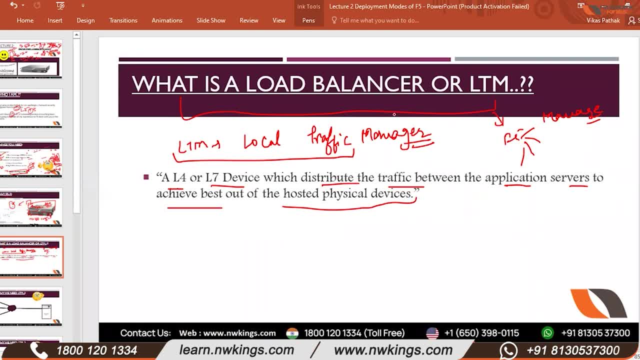 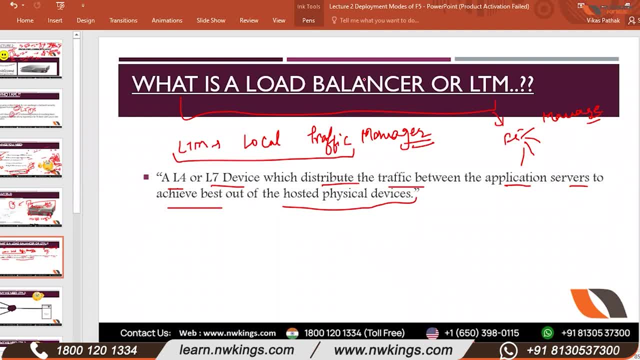 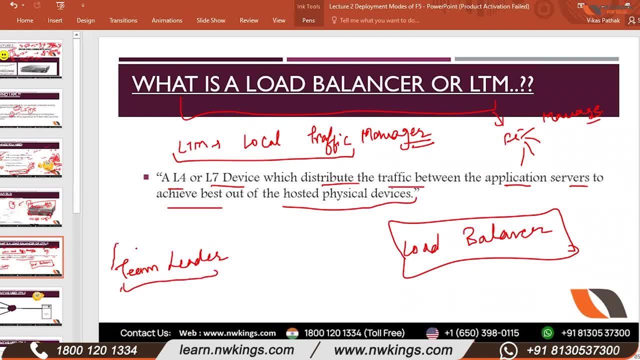 manager What he does. he knows that my person A is good in R&S, my person B is good in monitoring, my person C is good in both R&S and monitoring and my person D is good in communication. Right, Awesome. Now let's suppose. 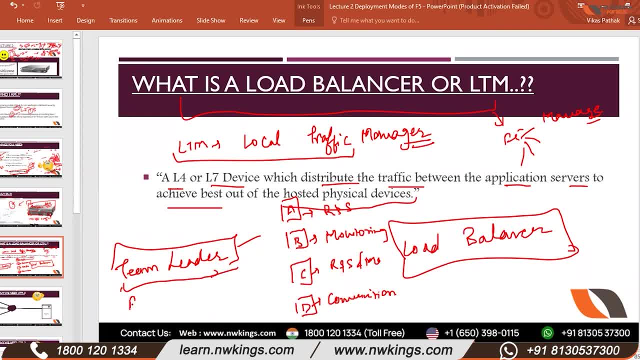 we have an activity where all the top management persons will be there, right, And your team is doing the migration, Okay, Okay. So when team leader comes into the picture, what he will do? He will align person A and person C for in the front for the activity, right? 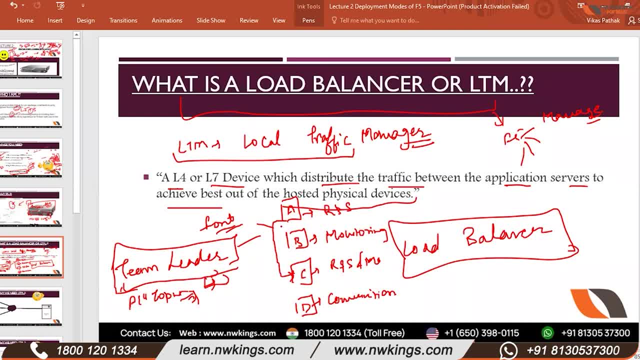 You will be performing that activity, Person B. he will align that you have to monitor the tool and you have to inform immediately if something goes wrong. Correct. And he will assign person B that you have to do a fair communication between all the. 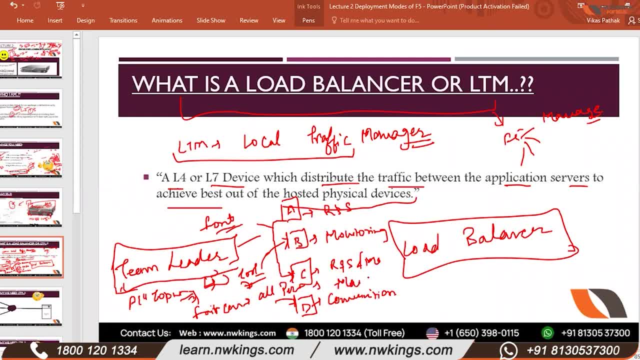 parties like my management as well as clients management, about the work has been done Correct, So sorry. So basically what he did was that the people who had the resources were all specialized right. So basically what he did was that the people who had the resources were all specialized. 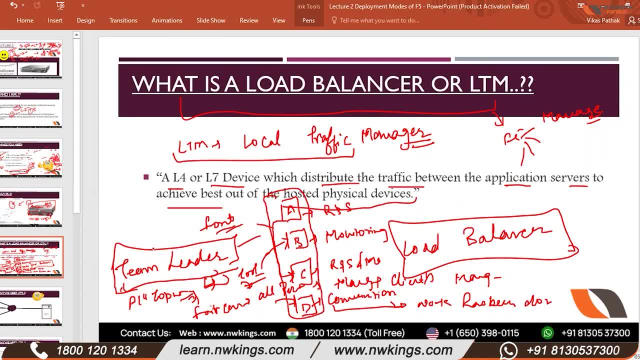 right And he had a load. What was the load? Migration. What did he do? He destroyed the load of migration. Correct, Distribute Kar Diya. Make Sense, Load Balance Haan To Usne Kya Kiya Jo Load Tha Usko Kya Kiya. 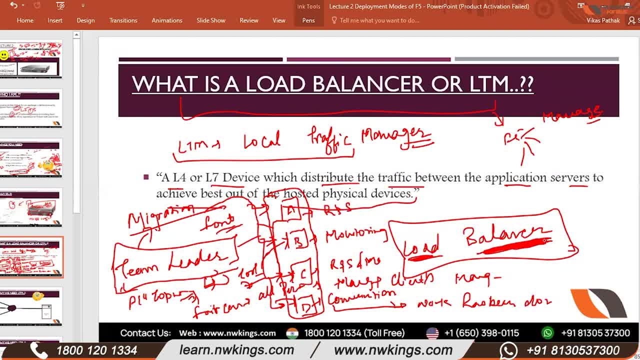 Distribute Kar Diya, Better Balance Kar Diya. Yes, Ya, Fir Ek Approach, Yeh Bhi Ho Sakti Hai Ki Team Leader Hai, Uske Paas Char Bande Hai Unne Ne Bola Bhai Morning Hours Ke Support Tum Dogay. 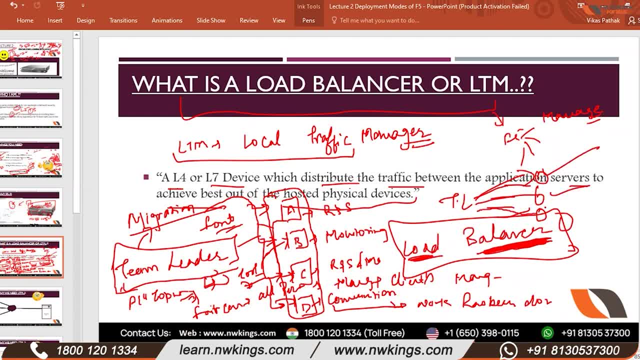 Afternoon Hours Ke Support Tum Dogay, Evening Ka Tum Dogay Aur Night Ka Tum Dogay. This Is Also Load Balancing. Make Sense, Yes, Agar Yeh Cheez Nahin Kare Hum To What Will Be The Scenario Ki Ek Banda Aaya Morning Mein. 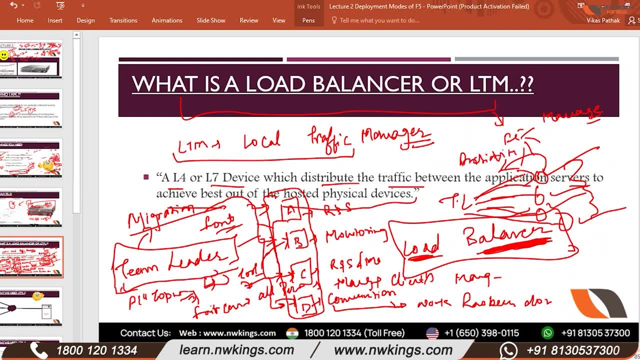 Activity Start Hoi Now Throughout The Activity. Pichara Baitha Hoa Hai Kewki Handwork Concept Hi Nahin Hai Load Balancing Hoi Nahin Paari Kewki Doosre Bande Ko Toh Bola Hi Nahin Kya Kaam Karna. 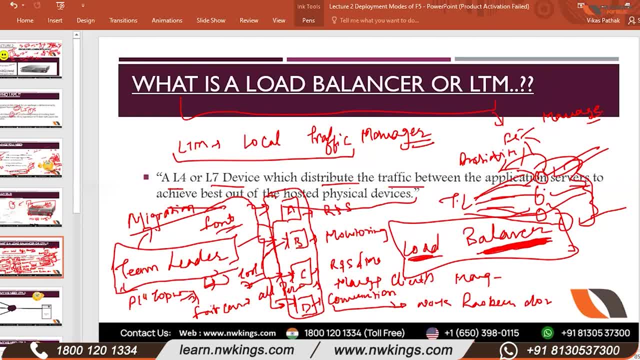 Agar Mutual Consent Se Ko Kar De, Toh Theek Hai, But Physical Devices Ne Mutual Consent Namke Koi Cheez Hoti Hi Nahin Hai. Right Servers Aapas Sa Baat Tho Nahin Kar Sakta Hai, So They Do Need Something. 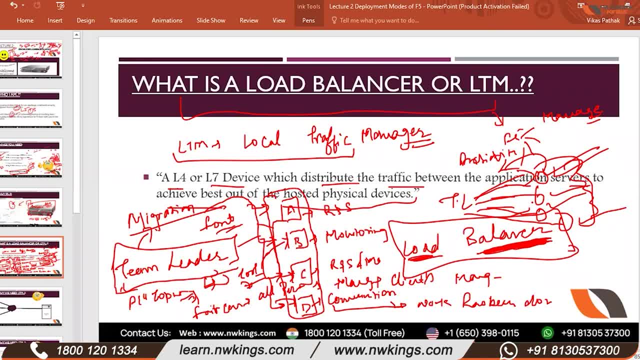 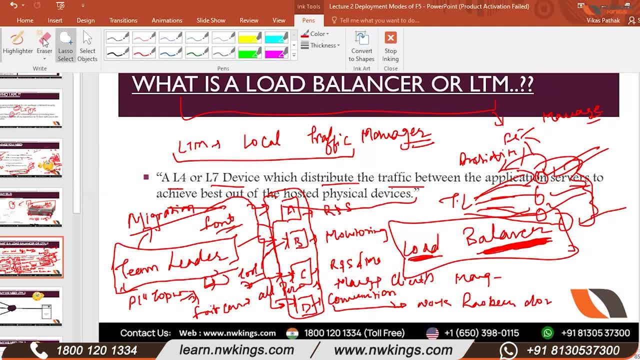 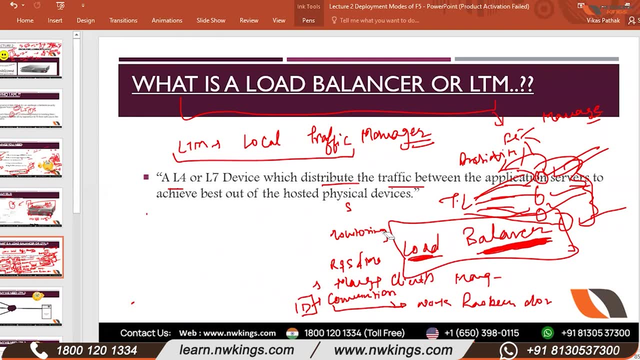 Which Will Do This Mutual Communication Sort Of Thing Between Them Theek Hai. Ab I Hope, Ki Load Balancing, Jo Term Hai, Yeh Aapko Achay Se Clear Hoi Hoi Hoi Right. Ab Hum Baat Karte Hai Ki LTM Theek Hai. 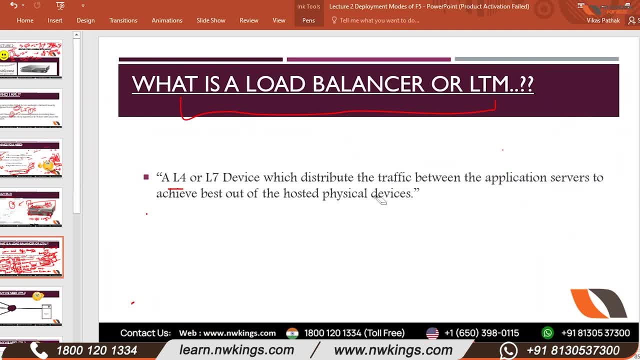 Ab Hum Baat Karte Hai, Aapne LTM Ke Baat Aaya, Yeh Mera F5 Hai Theek Hai. Yeh Pura LAN Hai, Yeh Pura DMZ. Hai DMZ Mein Ek Application Ke 3 Servers Rakhe Hoi Hai. 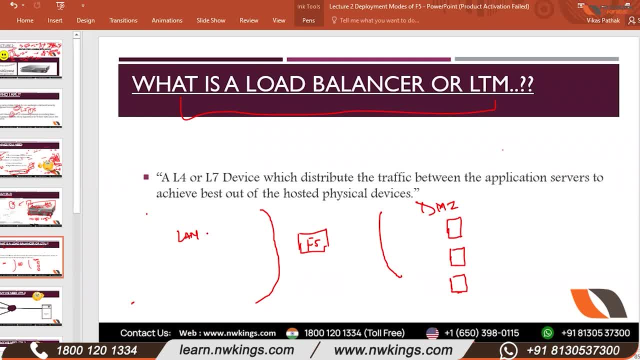 Theek Hai, Ab LAN Se Toh Traffic Continuously Hit. Aare Right May Be A Thousand Users Are There Ab Maan Ki Chalo. Yeh Jo DMZ, Mein Jo Application Server Hai. Na, Yeh Hai Resource Management. Ka Resource Management Kya Hota Hai? 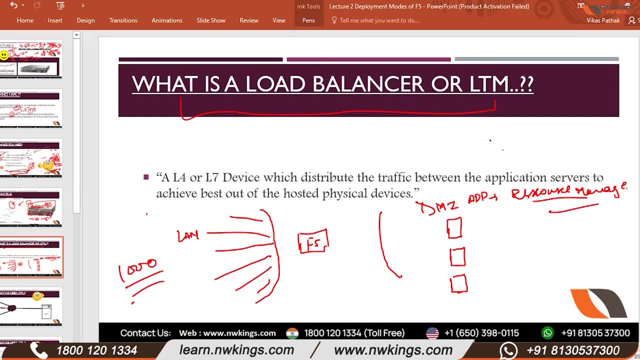 Attendance Jahan Pe Manage Hoti Hai. Kisi Ko Attendance Mark Karni Hai, He Will Login And He Will Mark The Attendance. Kisi Ko Agar Application Leave Application Deni Hai, Woh Kar Sakta Hai. Kisi Ko Maalo Sick Leave Deni Hai. 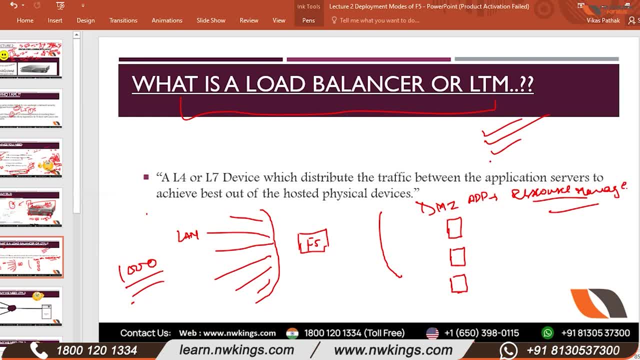 Ya Half Day. Chahiye Woh Kar Sakta Hai Kisi Ko Leave Plan Karni Hai Approval Ke Liye. Chahiye Tho Woh Wahan Pe Apply Kar Sakta Hai To Yeh Saari Cheese Usse Wahan Pe Is Application Servers Se Milti Hai. 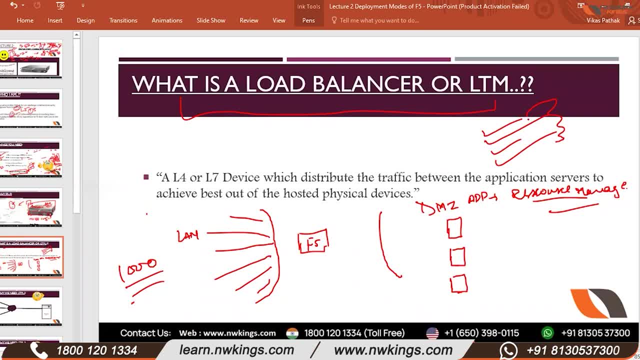 Theek Hai, Sorted Hai. Demilitarized Zone, DMZ, Basically Woh Place Hota Hai, Jahan Pe Aapke Saare Servers Rakhi Hota Hai With The Highest Security Level. Demilitarized Zone Server Room Hota Hai. Usse Ko Matlab Kya Kya. 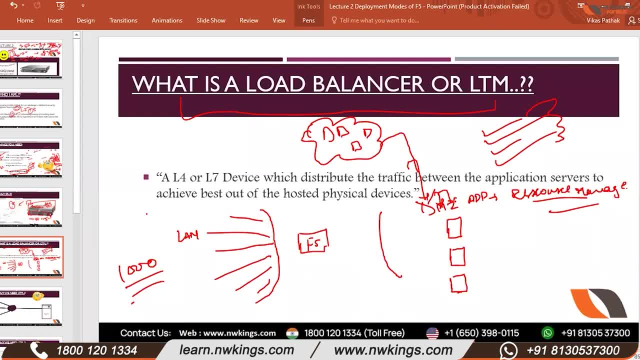 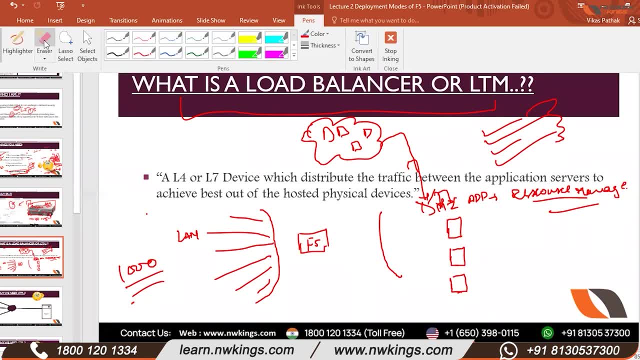 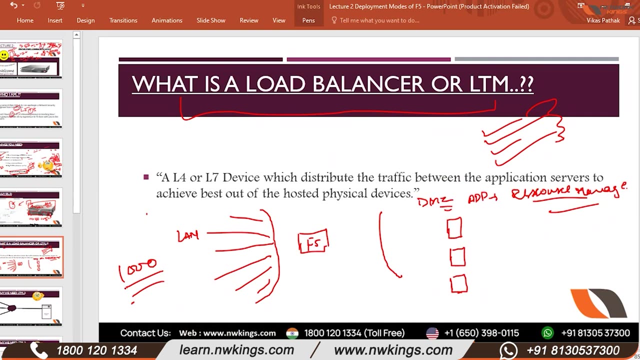 Haan Ok Gun, Copy This Hone. Do You See, Sänder Sender Change Saath Korean Universe Broke выглядity. April J represent June, August, Sunset Under Shi Dis, heavily Population For log in right to mark attendance, correct or not? now the traffic of 1000 users is coming to me on my f5 box. 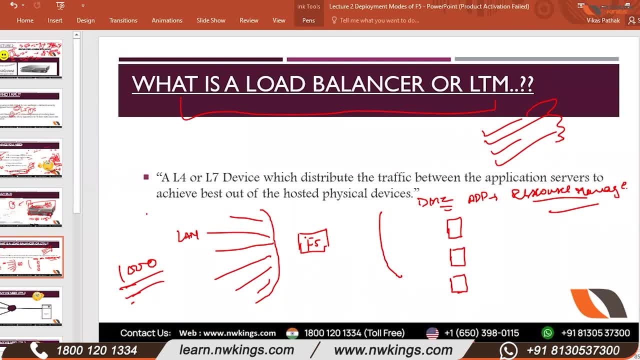 so what is the scenario? that either I remove f5 and send all the requests on the same server one time it will come after some time that the CPU utilization of the server, for example, after one year the company has grown 1000 to 2000 users have come here, but we have only one server in use. 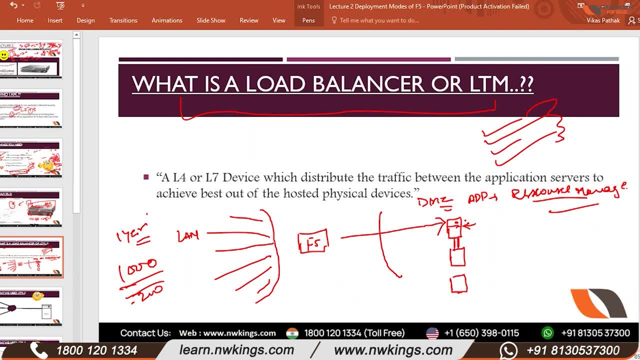 we have considered the primary and secondary between these two. if it goes down, it will go up, but now my load is going to the primary server now. now my traffic of 1000 users is coming here. now what is happening is that it is going to 2000 users. 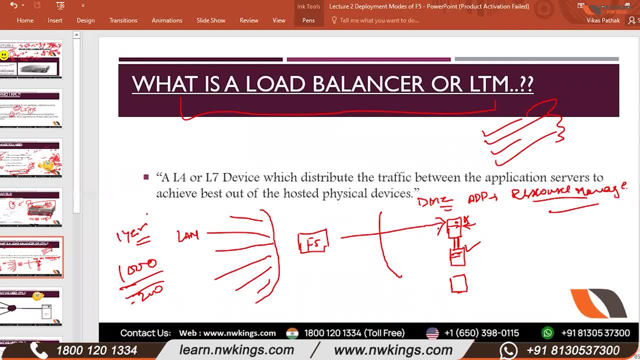 so the obvious thing is that if the user rate has doubled, the traffic count has doubled, then my utilization will also be doubled. let's assume it was 40% before. now it is 80%. right, and any server, any device, if it has to work properly, then the utilization of that device should be below 80%, whether it is a router, whether it is a switch, whether it is a server or PC, anything. 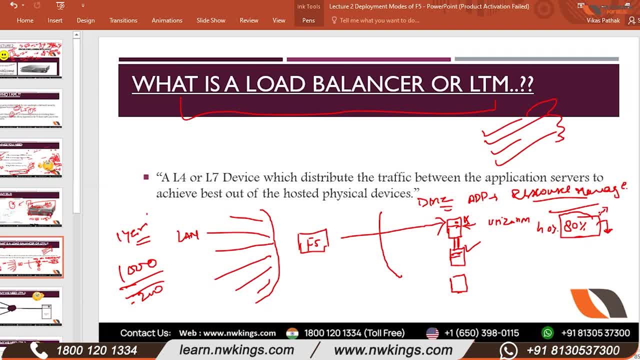 if it goes above 80, then it will start to misbehave. so now my second server is live right. so now my second server is live. right now my second server is live right now my second server is live right. 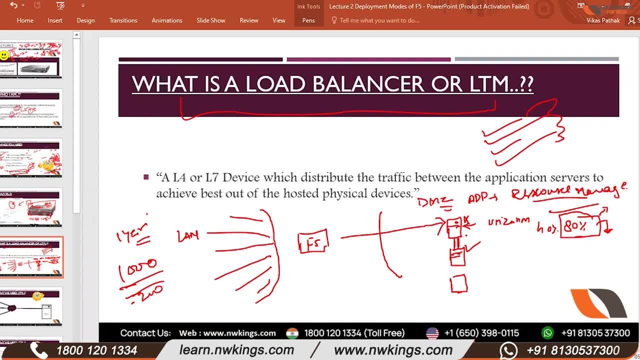 so currently the level is about 50%. whether it likes it or not undecides it is live. if I consider that if I have purchased this in $5000, then it should also purchase this in $5000, because both capacity is the same right. 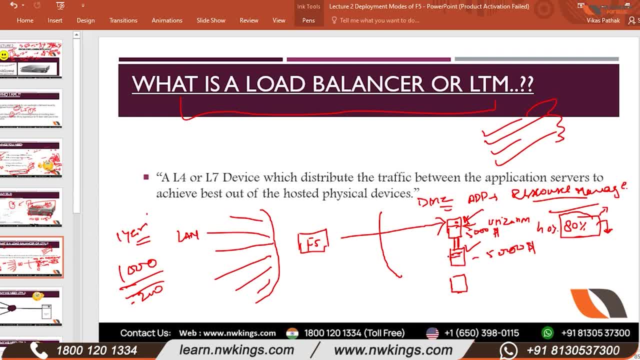 but the entire company is doing this. this poor idle is behind. one way we see this $5000 who is my investment? isispaced idles, Whereas I am creating an array and creating share as well. so that is acraful, obviously. 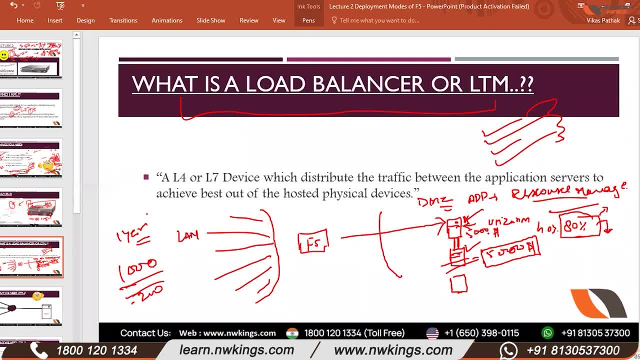 sorry because too late I was theme in the tour. sorry everybody. thank you very much. from watch to watch, a risk that any time this server can fail, and if it fails then I will have to give maintenance charge again to fix it correct. so what LTM did, local traffic manager, what he did, that. 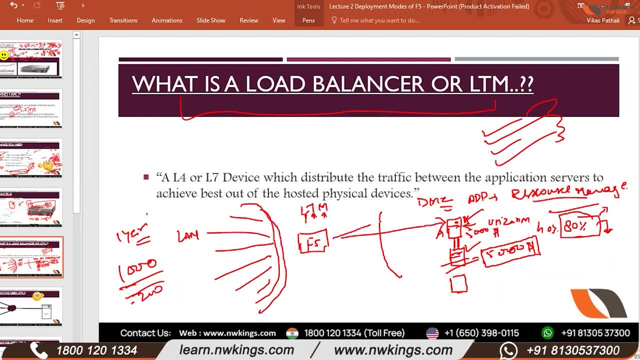 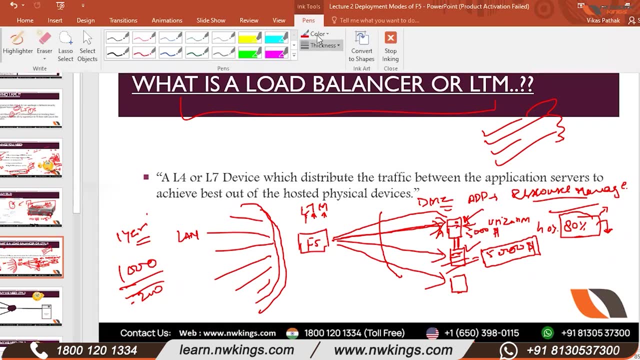 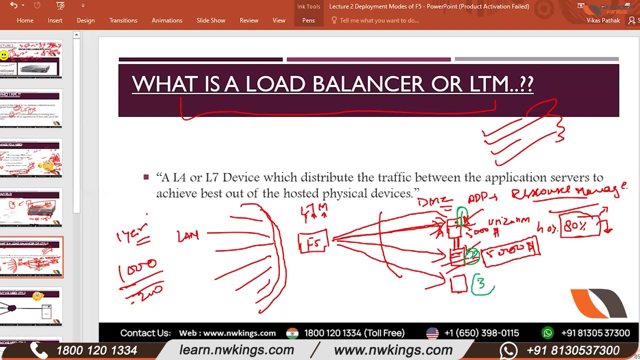 how much it完 does distributed. first request you take second, you take third, then you take fourth, then you take 5th, then 6, and you take 60, then you take 12 интерprint, then you take 300, then you take toda. so this was done, ie. 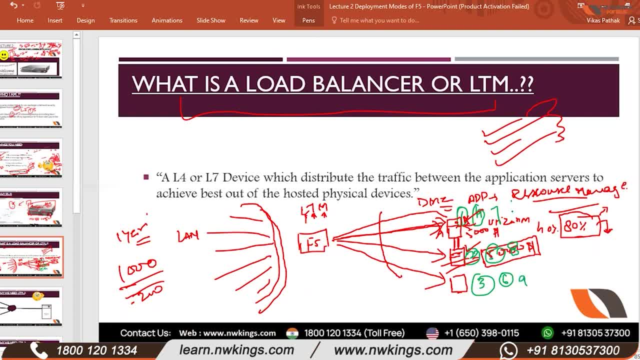 again: 7, 8, 9, 10, 11, 12. this is how this number, this number, goes on. now, what happened? that the traffic 12 connection was being made from my server 1. now those 12 connections are being made from 3 servers and only 4 connections are being established on a single server. 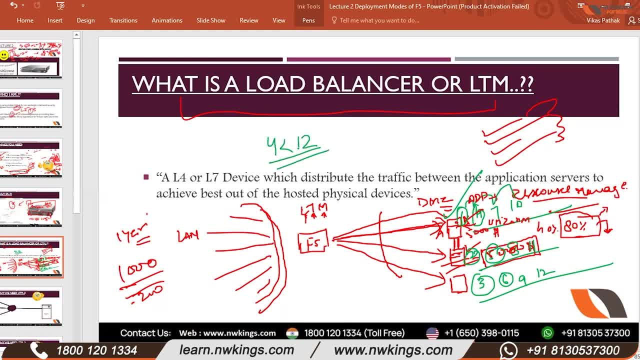 so 4 is lesser than 12. now, in 12 sessions memory will be more utilisation, or in 4, so 4 is lesser than 12. close 2, 6, 7. 1, 2, 3, 4, 5, 5, 6. 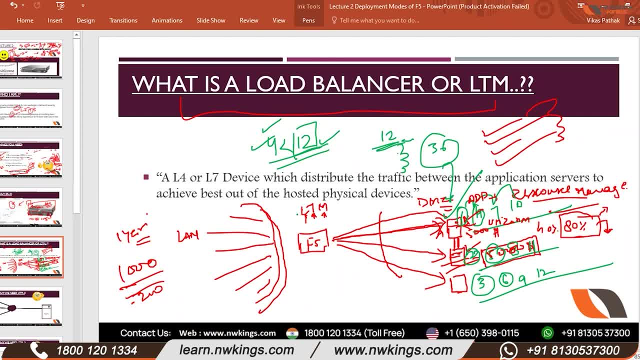 6, 7, 8. Obviously, its utilization will be high. So this is the work of LTM. Now, there are many different methods to do this thing. The traffic management is going on. Send it here, send it here, send it here. 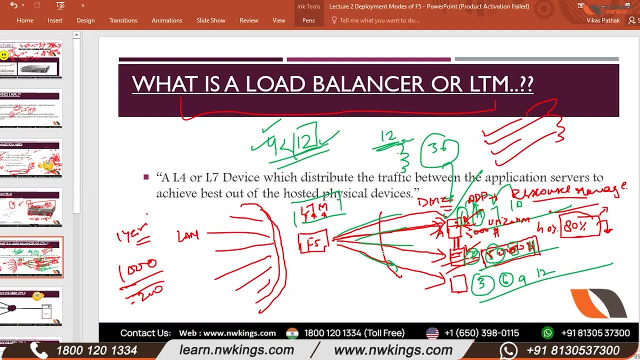 There are different methods to do this thing. We are going to discuss those methods in this whole series. Did you understand or not? Tell us everything quickly And if you have any doubt, tell us We are going to read further. We are going to decide on the scenario. 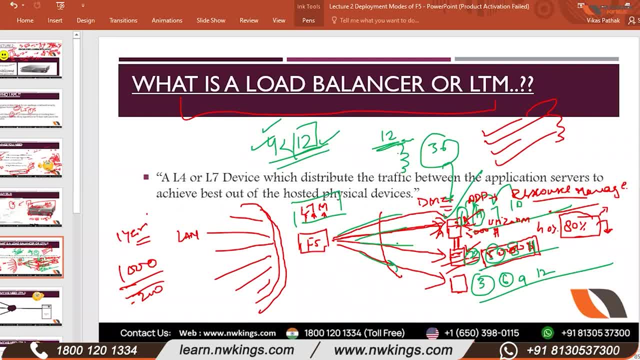 What is going to be the scenario and how to introduce it in the load balancing market. All clear, sir. All clear, All clear, Sir. this load balancer has come now, But Before this, when there was no load balancer, 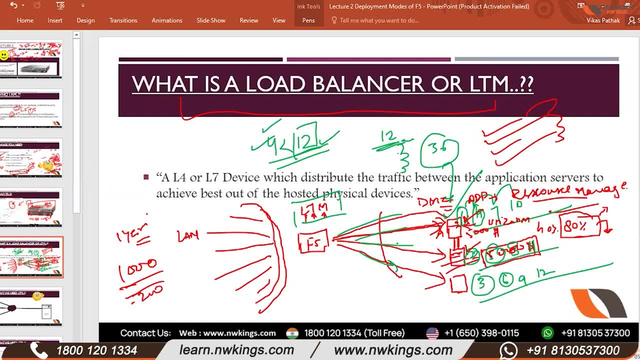 was there any other tool to manage this thing? We are going to discuss this in the next stage. Okay, Okay, sir, Let's move ahead. Is there a load balancer like this? They are firewalls, Firewalls, They are firewalls. 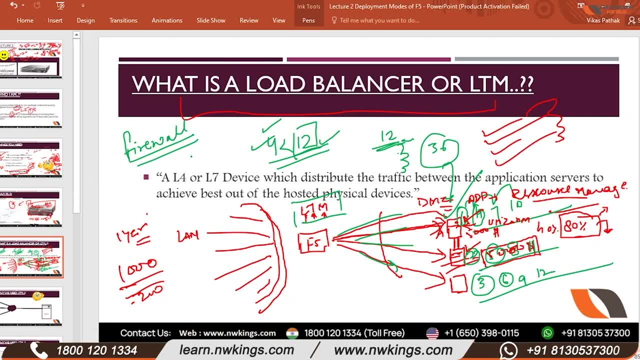 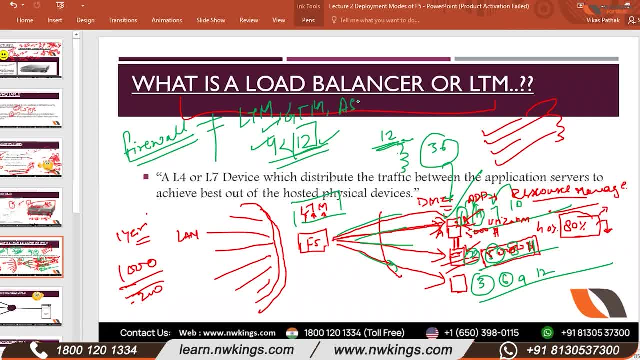 GTM, ASM related to firewall. There is no relation between them, ASM, Just like the company has Soforce firewall and FortiJet. They are not load balancers. No, No, No, firewall is a load balancer, Okay. 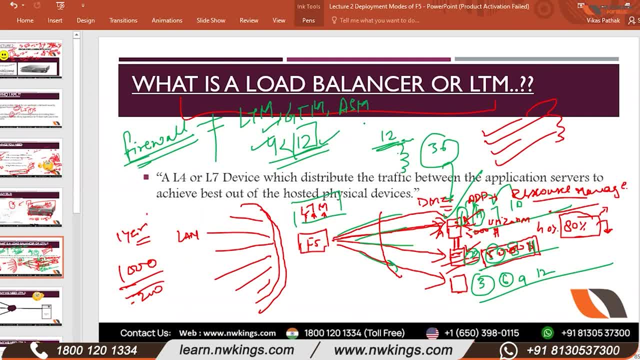 If this is someone's perception that firewall does load balancing, then it is a myth. It is a wrong perception. My confession is correct. Thank you so much. I was thinking that all firewalls, like full-auto checkpoint, DeFi, like this, all of them do load balancing. 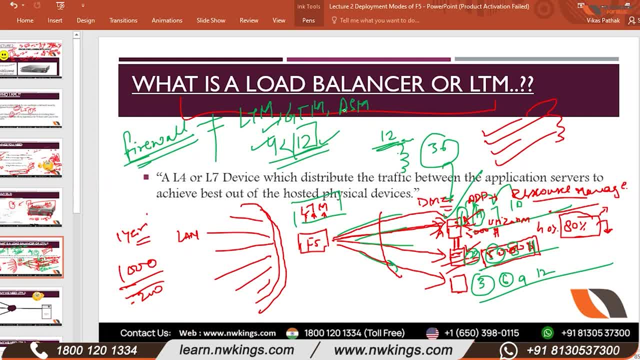 No, no, no, no, no. Thank you so much. ASM- ASM- Okay, Application Security Manager. This is also called a web Web Application Firewall. Right, There could be some relation between the firewall, Okay, Between the firewall and the ASM. 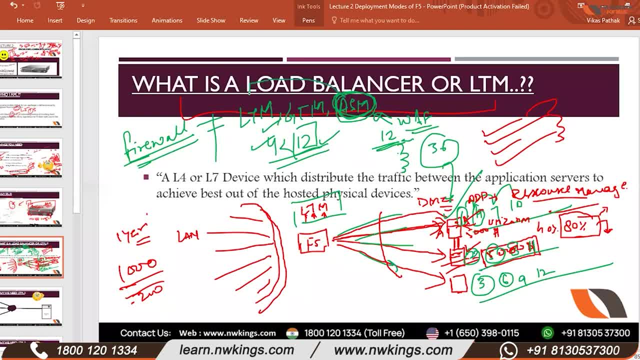 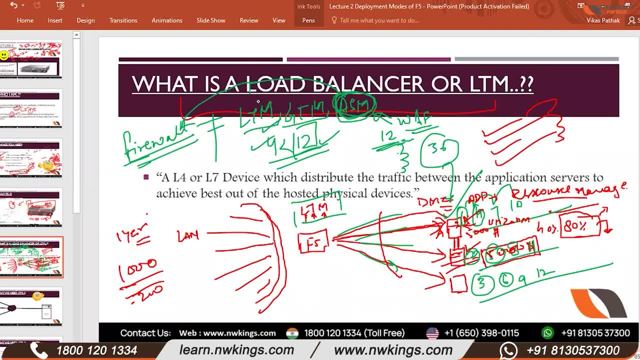 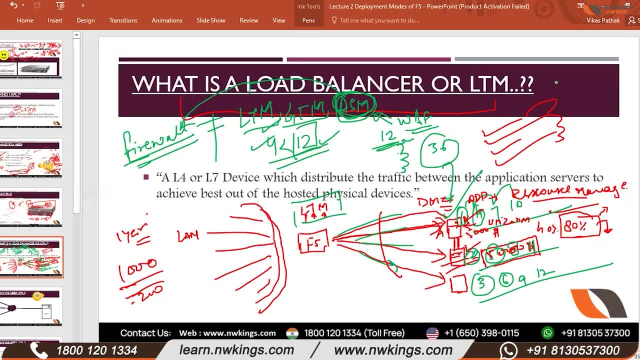 No, Okay, Okay, Why do you是的? Why do you qualidade a firewall? I think OK, OK, why The DKOO aren't against closed to video mare intersection? Yeah, All I just do is Yeah, If someone is used to the. 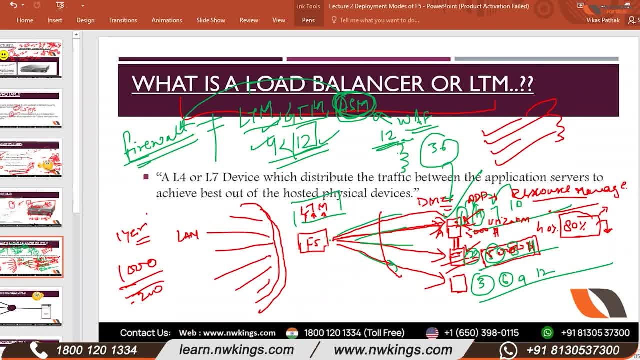 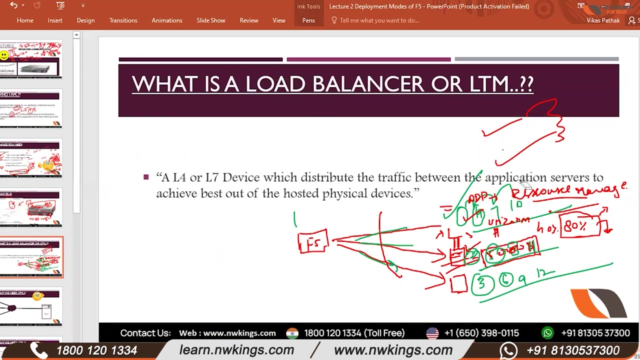 you need to Tell me what operational work do you perform on firewall. Basically, you are doing L1 type of work: reporting and monitoring. Yes, If there is any problem, I will tell you at the next level. If there is any problem, please see it. 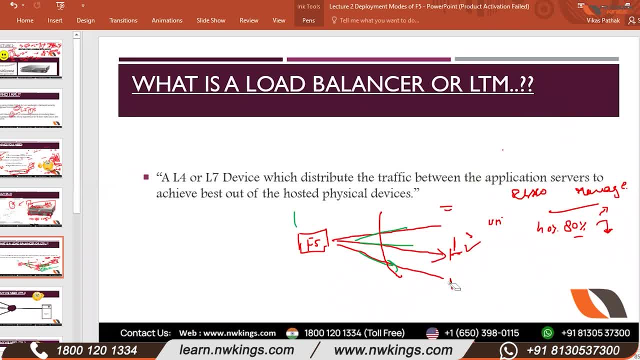 Cool. So I will tell you one thing. What do we do on firewall? We apply restrictions on firewall. Do you understand? The work of firewall is to apply restrictions. What to do? For example, we have to block a site. 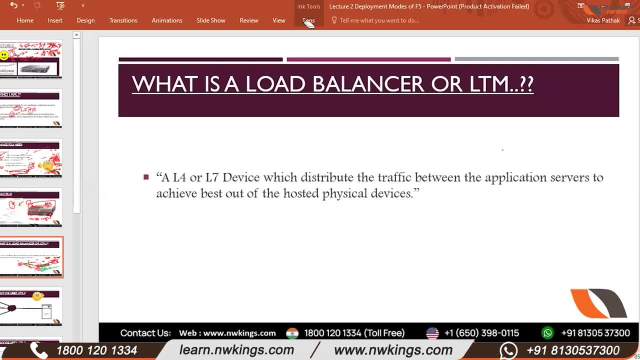 Yes, We decide which person will have what accesses through firewall. Okay, If my DMZ has a server, if that server is not a web server, then who will have access to that particular server? We decide this thing through firewall. For example, if a user is running YouTube, 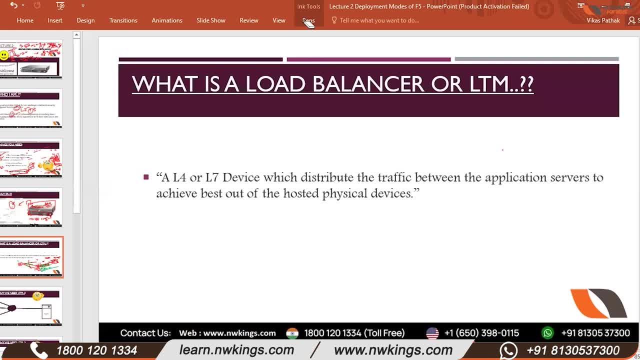 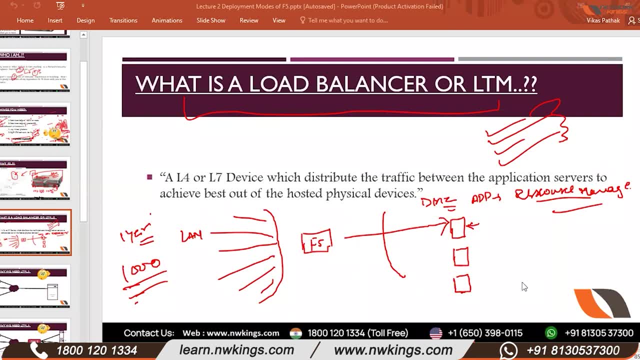 and he is running out of bandwidth, then we can take the proper IP, integrate it on firewall and block the site of YouTube. We can block it there, Yes, But we cannot do that on F5.. On a certain level we can do that. 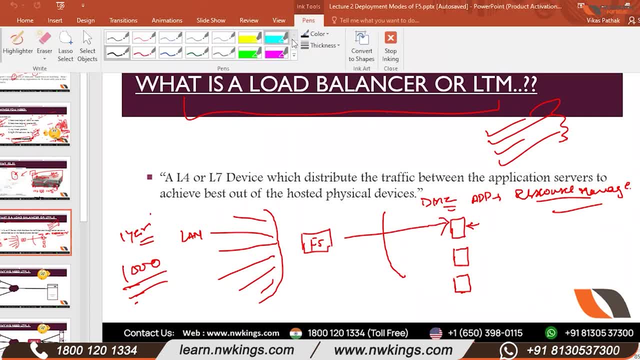 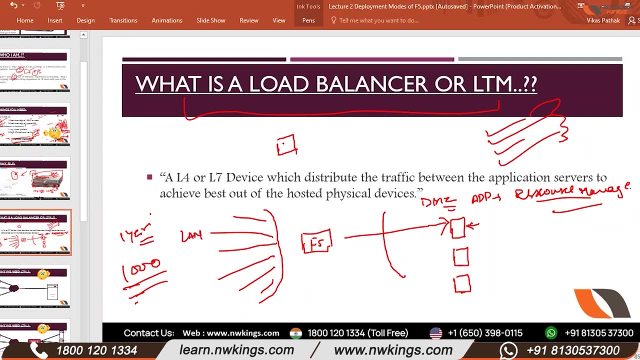 But on a bigger level. we cannot do that. On a bigger level, it is not possible. Okay, Now there is a firewall. What did you do? This is my firewall. Here is LAN. This is WAN, This is F5.. 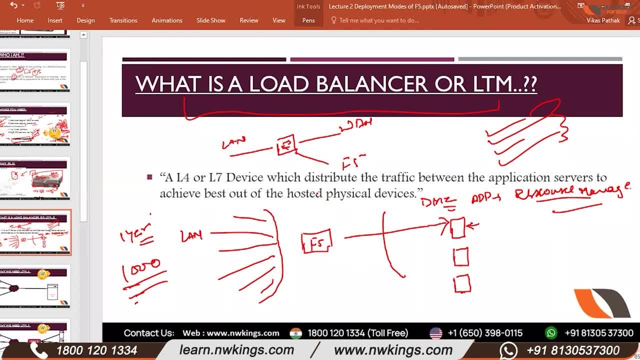 Okay, This connectivity is for your firewall. Now a person is going on WAN through LAN Firewall will check whether the access is there or not. If the access is there, it will pass the traffic. If access is not there on that particular port, 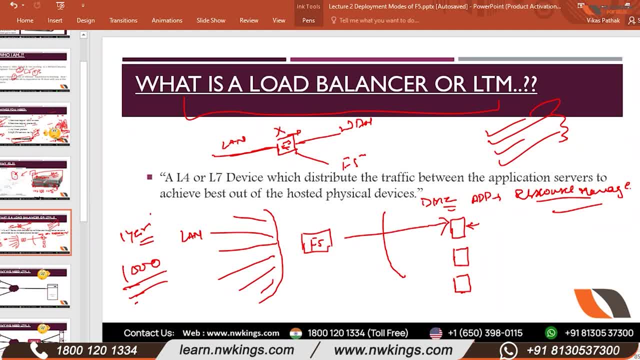 it will deny the traffic. Okay, Traffic is coming from LAN. DMZ is going. It is going on a particular application of DMZ. It will check whether, for this particular server, is that person is having the access. If yes, the policy matches. 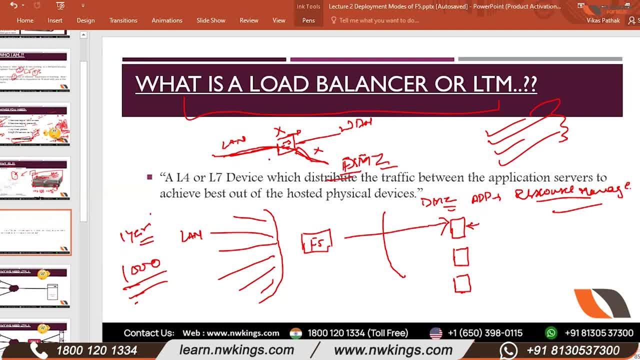 it will pass, Otherwise it will drop, Whereas the main motto of F5 is: the traffic is coming and a bulk traffic is coming from the LAN or maybe from the WAN. if it's a web server And we have multiple servers, We have to distribute the traffic between them. 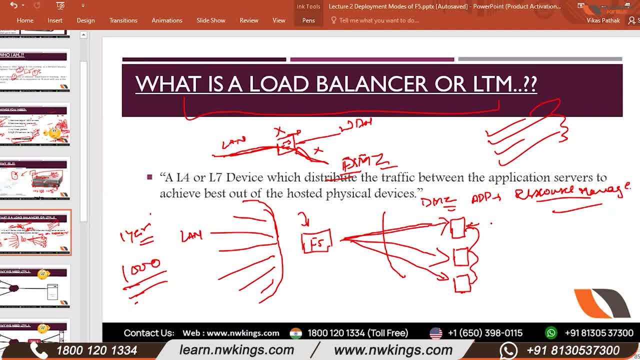 The availability of the service is the main motto of the load balancer. Make sense. Yes, sir, Firewall, or I think you have sorted the LTM right. Yes, sir, Thank you, It was a big confusion. Yes, sir. 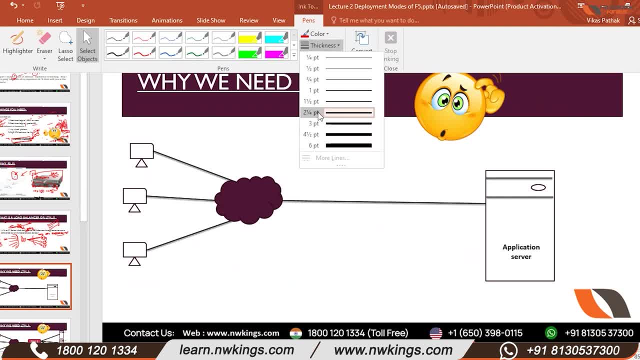 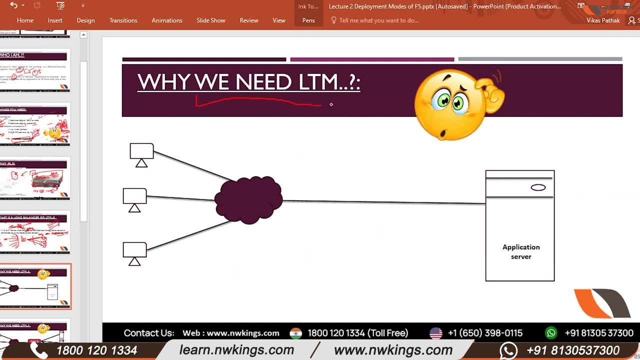 Okay, Now someone asked me a question: Sir, when there was no LTM, what happened? Okay, Now the same question is why we need LTM. Now, we have discussed a little while ago that there is no LTM. 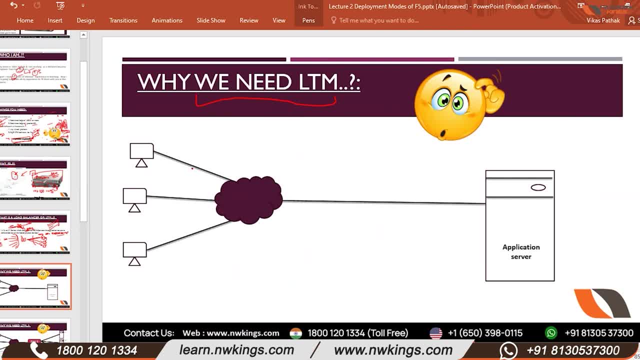 Right, This is my LAN. LAN came on the internet. Sorry, This is my WAN. Okay, This is the internet. This is my cloud. These are all my users. Now, let's assume I made an application. Let's say: 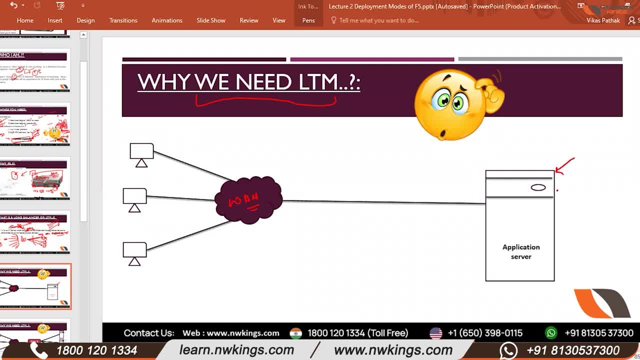 I made an application. Let's say I made an application. Right, What does an application do? It delivers groceries. Okay, What did I say? I went to relatives- To relatives, Right. I went to relatives. I said I have started. 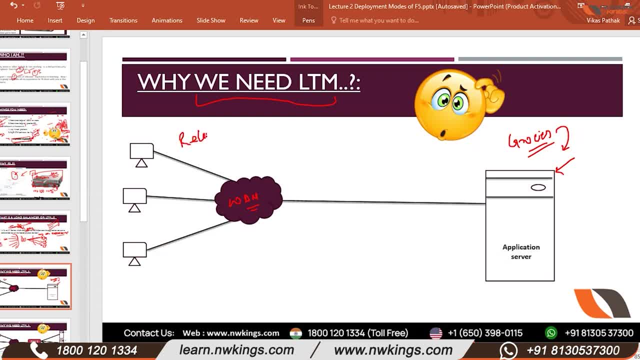 this work. You will get good discounts If you like it, you can order your groceries from me. Okay, I went to relatives. I said that I have started this new work. You will get good discounts If you like order. right, all of them understood me. 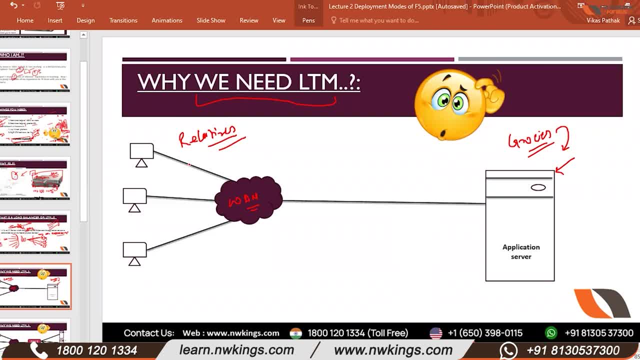 although relatives don't understand, but still let's assume that they understood, right, these three relatives. they downloaded the application, ok, my application, which I have made. it loaded three users. now what I have done: I have tied up 2-4 shopkeepers. I have tied up 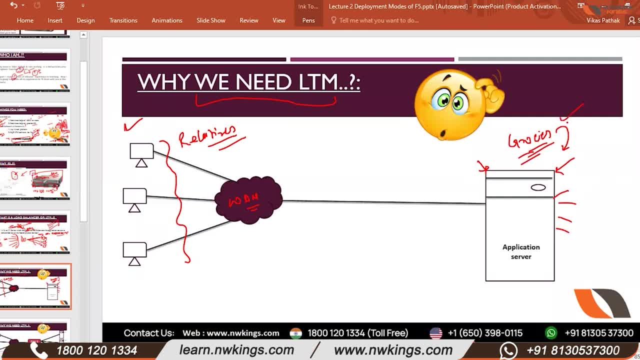 that if someone comes from my application, then your sale will increase. what you have to do? that? the material they will order. they have to keep only 5% margin rest. they will deliver and those shopkeepers are ready to do this. now let's assume there is a pencil box. 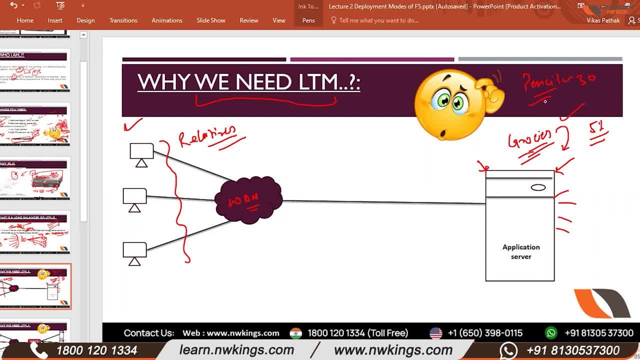 the market price is 30 rupees. from your app, that is 21 rupees. your relatives are happy because children are in every house and they need a pencil box. similarly, what is the packet of maggie? the packet of 10 rupees. your application, delivered in 9 rupees. 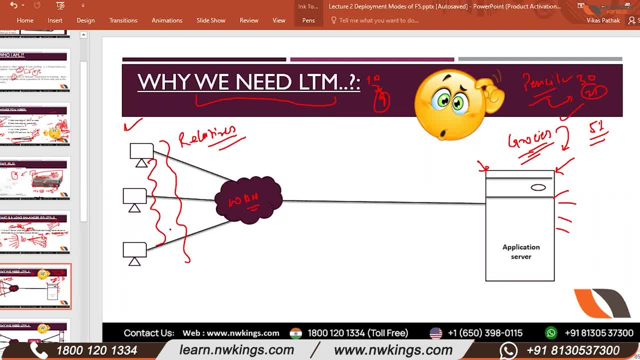 relatives are more happy over the time. these three relatives, they are 100% satisfied with your delivery, with your application, what they did. they all are having a WhatsApp group which is called family members, and they referred your application in that group and mentioned that this is a very good application. 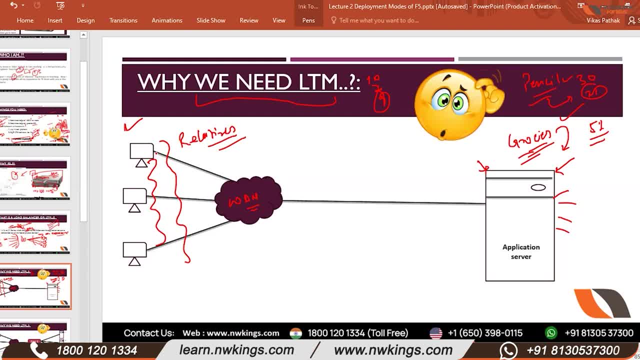 the services are very good. you all can download this application and you can use it and you all will get benefited. everyone listened. now one, two, three, three groups. let's assume there are 50 users, 25 out of 50 installed. now the three: now I have. 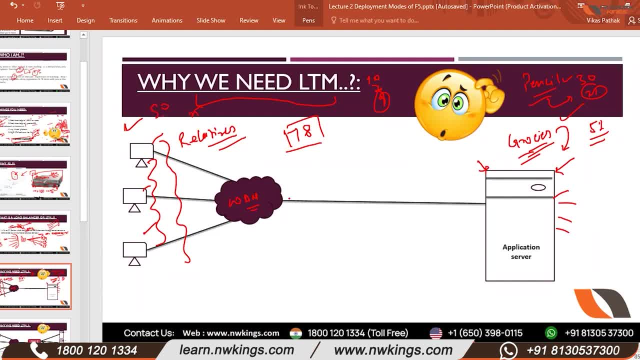 total 78 users. is it sorted? 78 users now the traffic of 3 users is of 78 users. after a month, these numbers 80. 78 users now: 70 780 users. after one year, this number increased to 3000. Vikas is now. 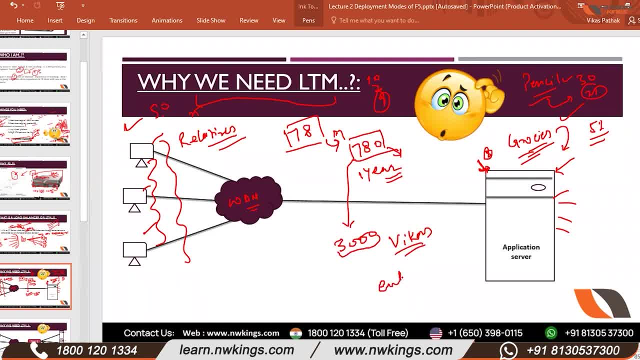 an entrepreneur: ok, 3000. previously there were 3 users. 78 users, 780, also ok, the server endured. but what about this 3000 users now? what option is left? first option is that you increase the specification of the server. suppose RAM was 16 GB. 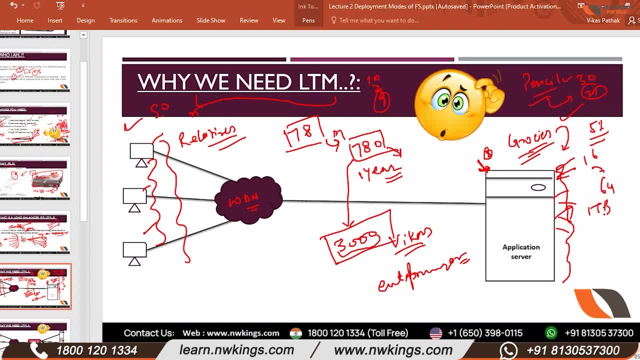 64 GB hard drive was 1 TB. now this may be 16 GB. CPU processor, which was i3, suppose you 4 core processor. suppose you put octa core 2 processor, suppose octa core, octa core. you increase the specification. but to increase the specification, 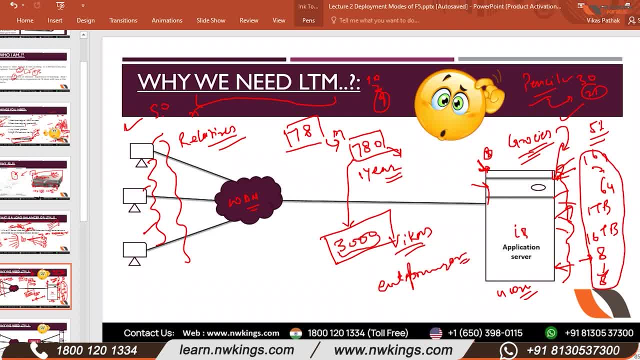 you also need downtime. or either you again deploy a new server and this connection shift here and then- this is one method- or you take downtime. now, at the time of downtime, if from 3000 users, 2 users, the application is open, then the service is available. 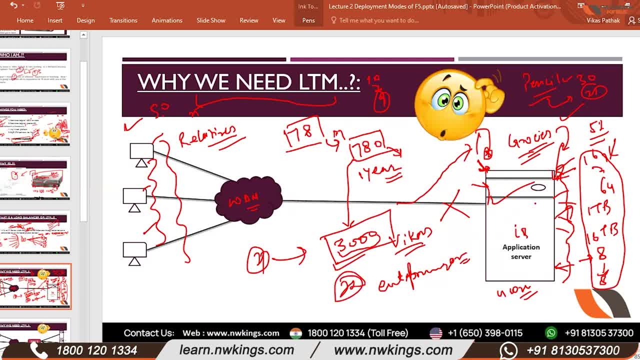 then your 2 customer base is gone, correct or not? you? ok, you tell me you use flipkart or not 100%. as soon as you have to order something on flipkart, you see that option unavailable on flipkart. now what do you do immediately? you open amazon. 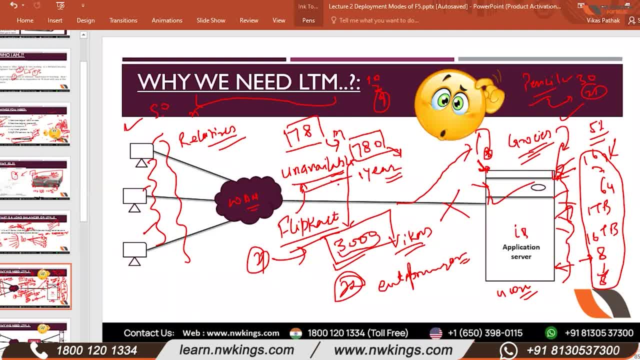 yes, you open amazon. so ultimately, what happened that the flipkart customer? why is the customer of flipkart? because he first opened flipkart. that's why he is a flipkart customer. but the service on flipkart was unavailable. that's why the customer was diverted to another website. so what happened? basically that that customer base got damaged. suppose if 2 customers also got damaged, then it's a loss. now, suppose you did not take downtime, you sent it to a new server. now you have this server. now, to upgrade this server, you shifted your traffic to another server. 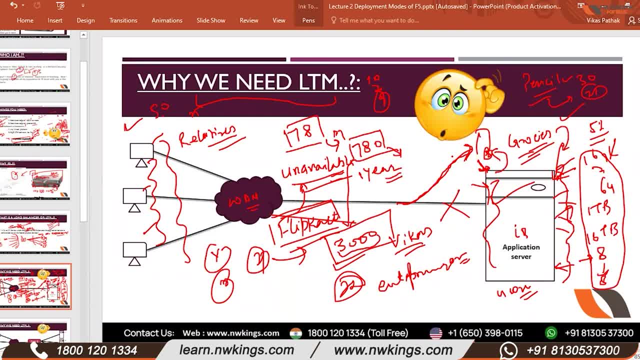 you have invested on this other server also. that's why you got another server. now you upgraded this. after upgrading, what will you do with this server? it will be stuck in your side. do you understand the problem? what is the problem here? what is the root cause here? 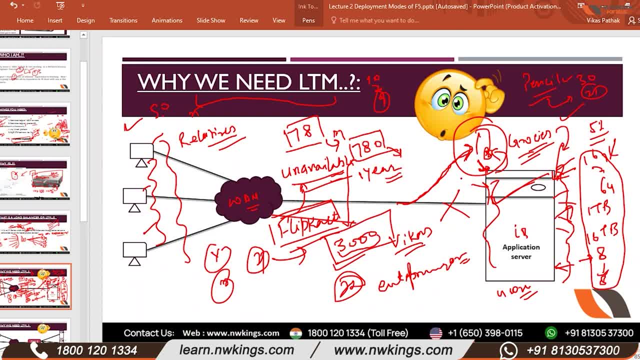 primary is going, secondary is not going. brother, you built a major server. you did a very good job. suppose your vision is good. today there are 3000 users, tomorrow there will be 30,000 users. for that you need a good configuration. so what you did? 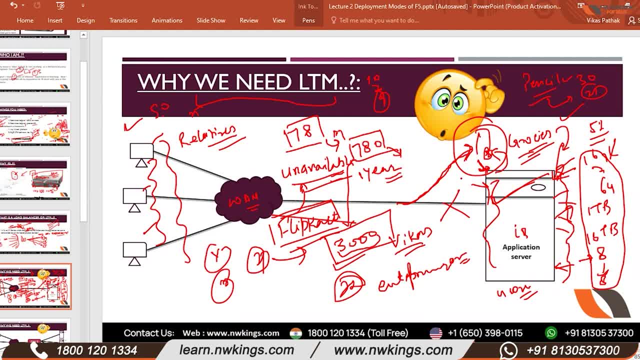 you increased the configuration of your server but the backup server you configured after primary got upgraded. it increased in side. now the configuration of this backup server is not that much that you make it primary and secondary and in any case suppose the user base of 3000. 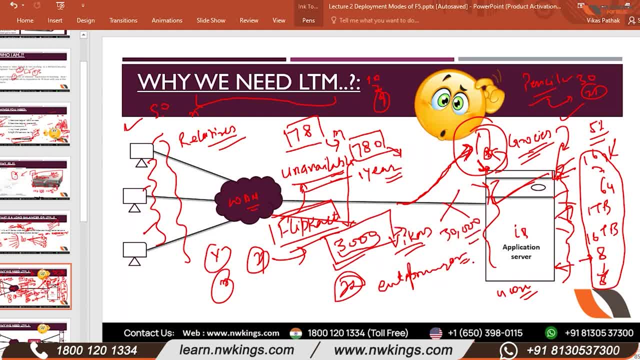 or even if it reaches 30,000, suppose then what will happen? if this server fails, then the secondary backup server will not be able to handle the data of 30,000 users, correct or not? yes, sir, yes sir, service is failure, all the sites that people visit. 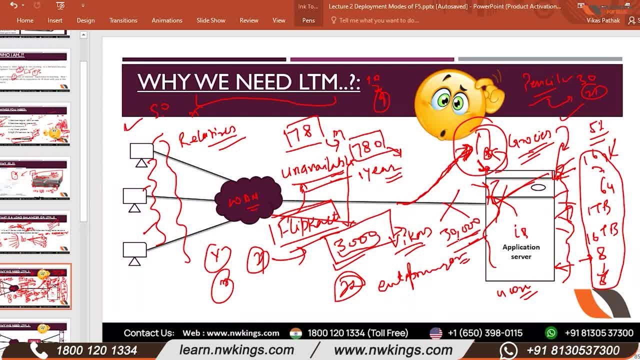 will be divided on multiple servers. suppose if it is from India, then the servers of India 100. approximately. there are more than 100 servers. if I talk about any one, if I talk about flipkart, then, as per me, there will be more than 100 servers. 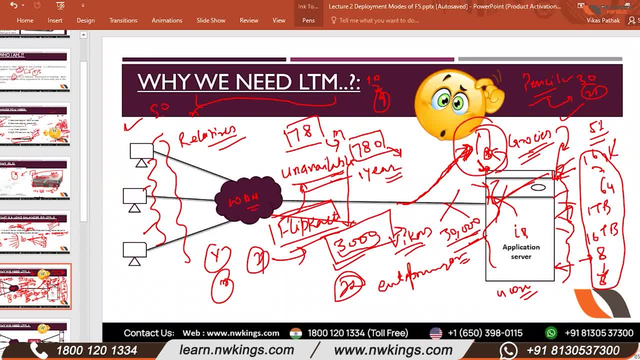 suppose don10 went on India's server, so all the servers will not be able to handle that particular. so how to route the traffic that has gone on India's server on another server? hmm, so we will do it with LTM. yes, there is LTM, but before LTM. 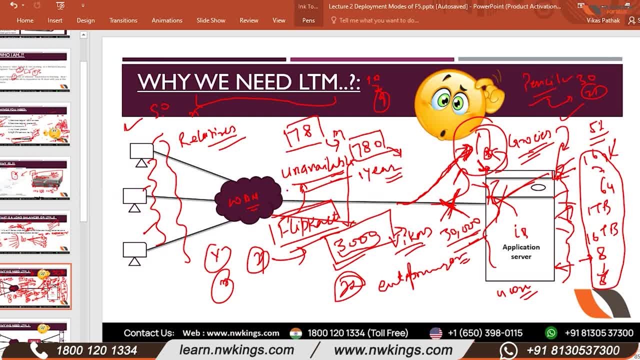 there is one thing- this thing is sorted- which I have explained to you. this is very basic and I have taken too much time, but today I have explained it very easily. so, whether you understand it or not, yes, sir, if you understand the problem, then the solution will be clear. 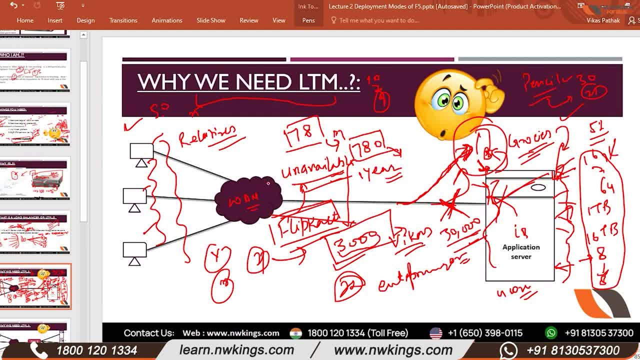 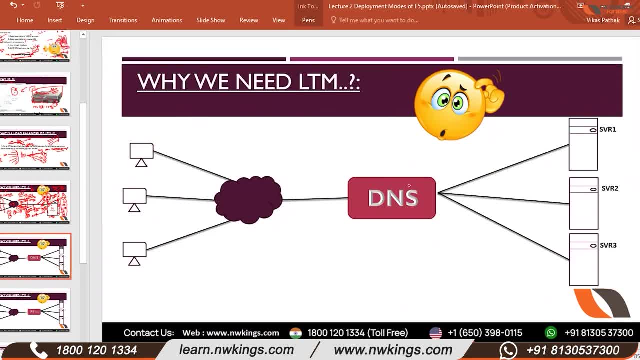 it is very important to understand the problem. here is the first solution. we have what happened? the first solution: we have dns. introduce the dns, that is, dns in between communication. for example, the name of my application is xyz dot com. suppose this is my server, one that I built initially. 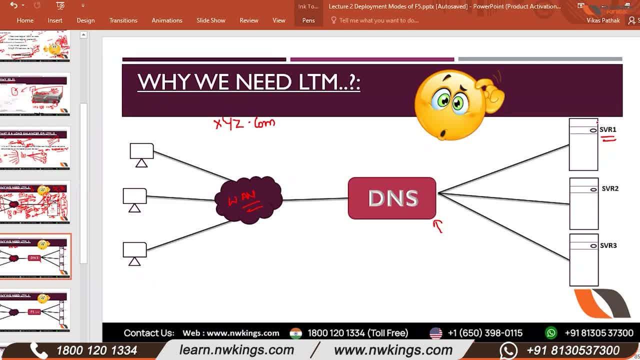 when I had only three users. ok, Now my xyz is hosted here. its ip is 10.1.1.1,. make sense. Now I went to my dns. I told my dns that whenever any connection comes to you and ask you for 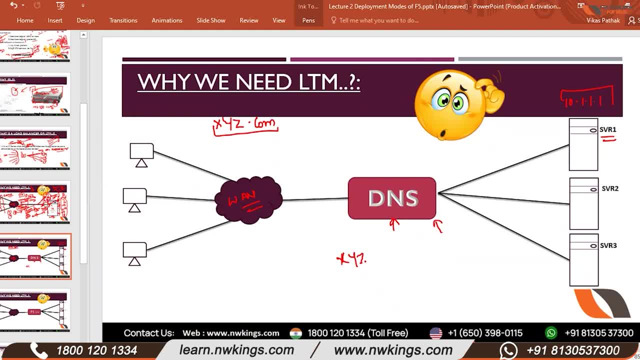 the IP address of xyzcom. you should resolve the first connection in 10.1.1.1.. You should resolve the second connection in 10.1.1.2.. And you should resolve the third connection in 10.1.1.1.. 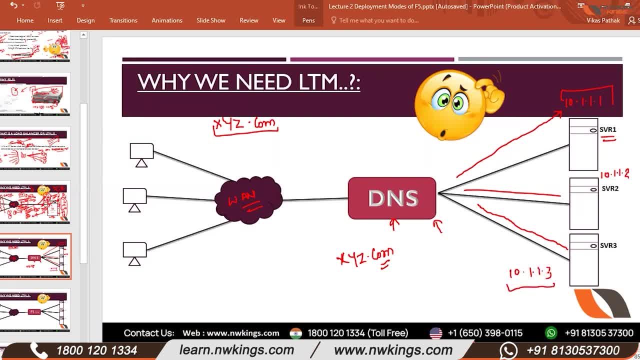 Ok, So what happened ultimately? as soon as the first client came to the DNS, he added xyzcom and its DNS lookup took place. In the first DNS lookup, the IP that was resolved was 10.1.1. And that traffic went from source to destination and landed on this server. 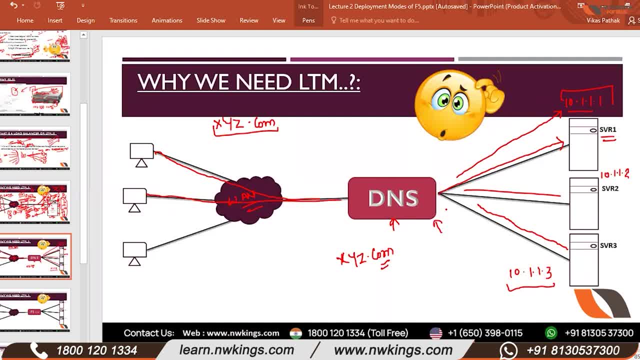 In the second DNS lookup, the DNS request was added and the DNS request was resolved in 10.1.1.2 and the service went from client to server. In the third DNS lookup, the DNS request was added and the IP that was resolved was 10.1.1.3 and the third DNS request went to this server. 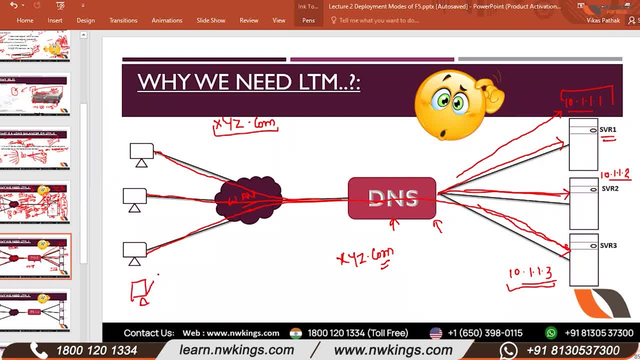 Similarly, if a fourth client comes, the DNS request will go Again- this DNS will resolve this query- to this IP address 1. Again, if a fifth client comes, it will go to the second IP address and if a sixth client comes, it will go to this IP address. 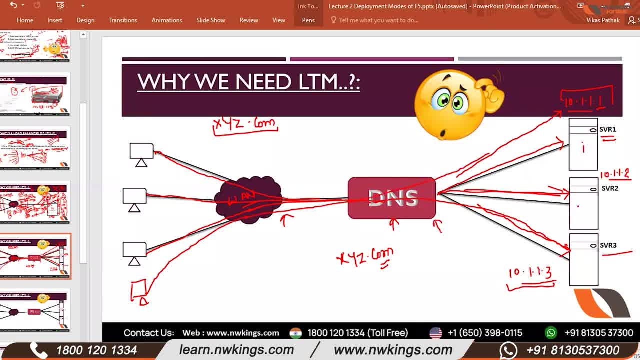 This method, like first request here, second here, third here, then fourth here, fifth here, sixth here, This method is called round robin. What is it called Round robin? And this method will be used from 75% to 90% in deployment for distribution. 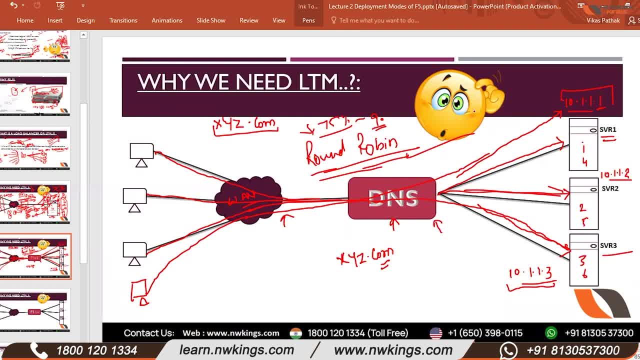 Sir, what is the second best method? We will discuss in coming slides or lectures. We will go one by one. Now we have to understand round robin very well. Round robin is a very sensible concept. It is a very old concept and it is very simple. 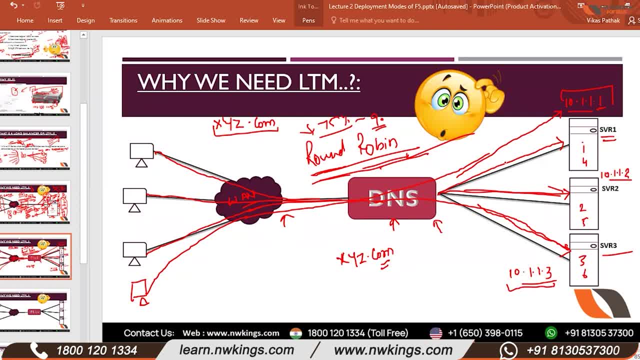 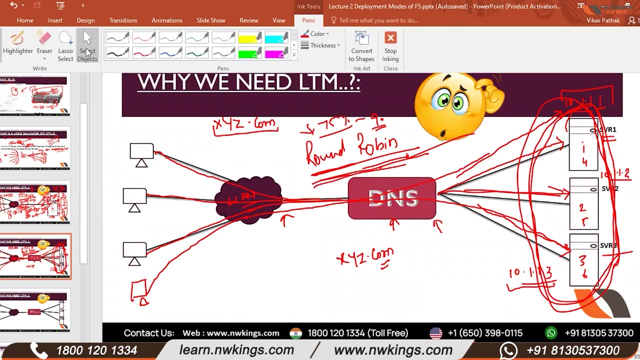 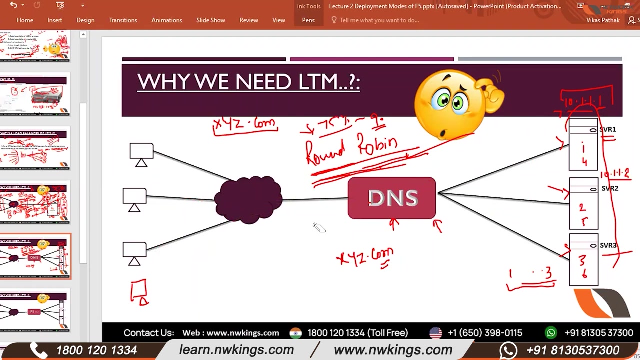 Keep rotating all the connections that are coming among the servers. Okay, This circle will keep rotating like this. Is it sorted? Did you understand this much story or not? Yes, sir, Now I want you to give me a quick answer to the question. 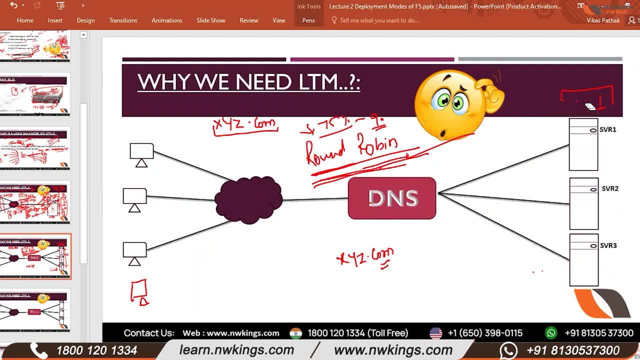 Yes, sir, What problem do you see in this setup? This setup is a problem Like 10.1. It will be more than load. This divide is not visible On which particular load should not go more. This divide is not visible. 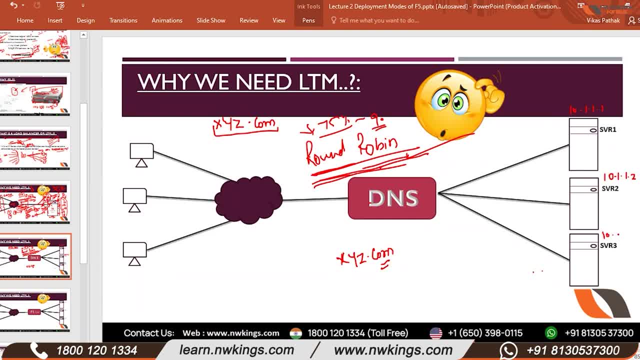 Traffic means on which particular should go. This divide is not visible in this. So why do you have to do that thing? Because there will be more load. We will not be able to use the service. How will there be more load? Let's take a small number. 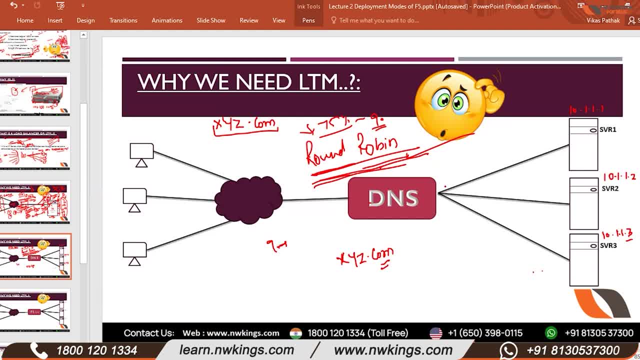 Nine connections are coming. Nine connections are distributed on three connections. So where is the load increasing After that? if a traffic comes Like a server comes down, Then the load will increase by two. If it goes down, Then distribution is still happening. 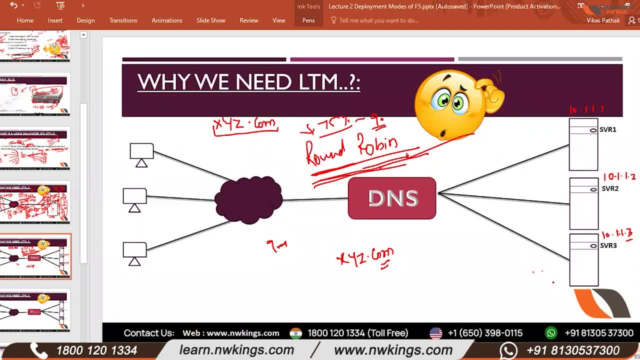 Then your server will be a failure. Yes, sir, What is the problem in this? If the server fails in any distribution method, Then you have to replace that hardware. But what is the problem in this? The problem is that if a server goes down, 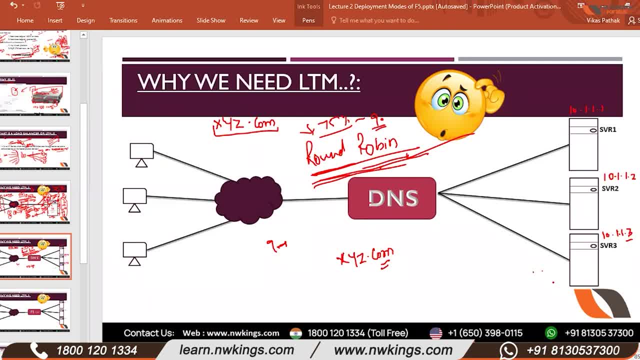 When it will come back to return back up, Then DNS will not send it a query: Why, Why? What will happen in round robin, One by one, First server, Second, Third. So when one goes down, Then there will be two active servers. 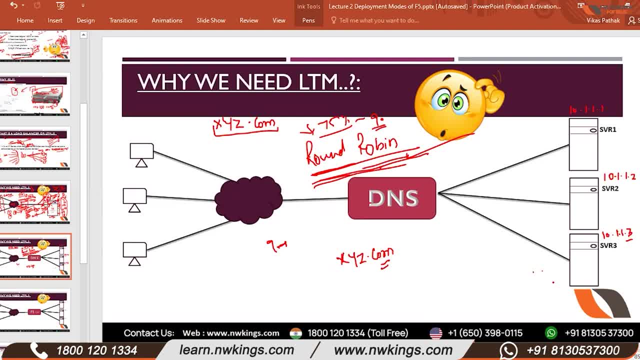 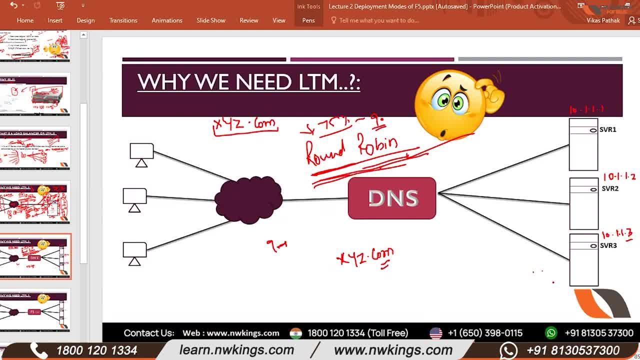 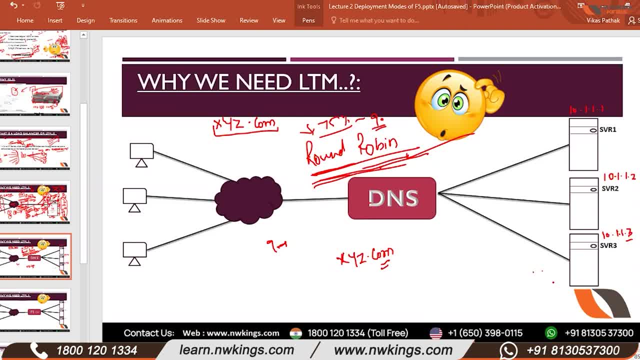 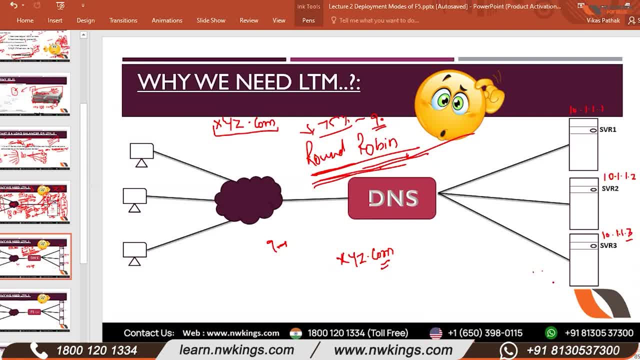 Sir, DNS server bhi bad jaye. tab issue: DNS server to multiple honge nahi yaar. Agar local bad jayega to global, hai Aap DNS me. basically, jab hum entry banatay hain, na ma trot sa insight deyata hu DNS ka. 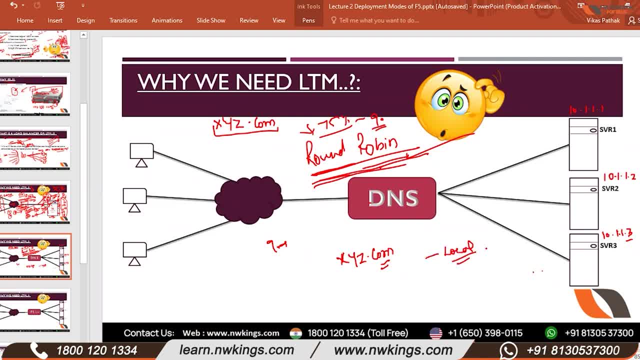 Jab hum DNS pantry banatay hain, to ek local DNS se bantay hain, jo hamare organization pe hota hai, ek banatay hain global DNS se To globally us URL ko IP me resolve kar To local, bad jaya to global hai. 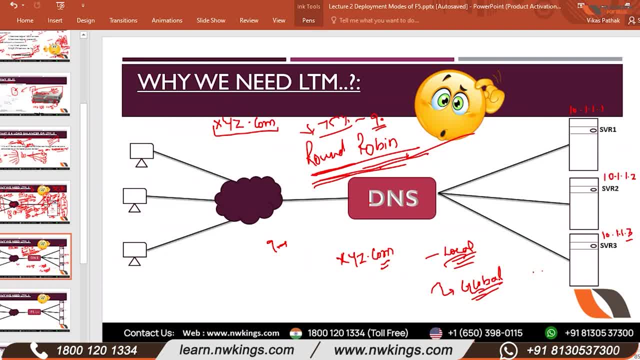 Global ek to hai nahi, yeh 4 to hai nahi, yeh 6 to hai nahi. Multiple servers. aate yaar, Aur koi problem. aapko nazara Mala, apne dimaag ko na bound mat koro khol do usko socho. 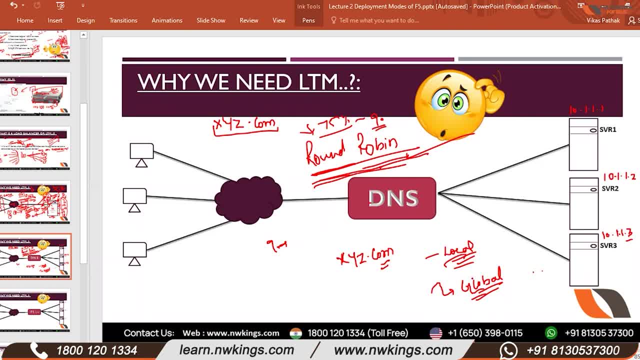 Sir, problem hai hi hai na, agar ek server down hota hai, phir yeh server jo down hua hai, jo user the woh kis server jayenge dobara? 1 pe jayenge hai, 3 pe jayenge hai 2 down hua hai. 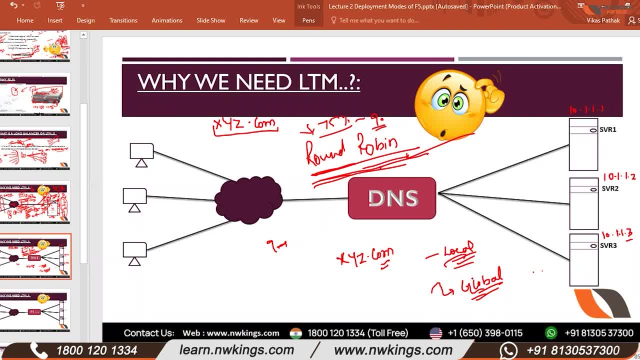 To iski liye bhi load by answer ko use karna parata hoga, Sir. yeh bhi ho sakta hai, na, sir, jese aapne 3 IPs ke liye 3 alag alag DNS bana hai. 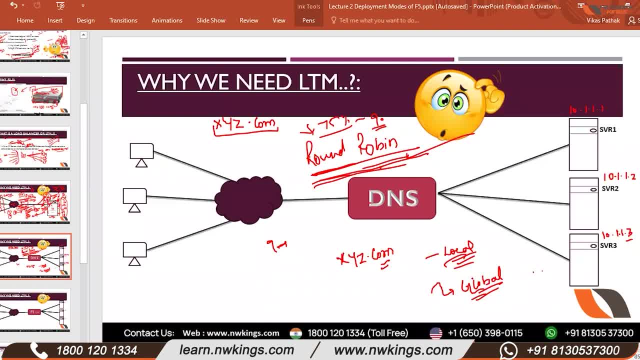 matlab xyzcom 1 aur 2,, 3, to apne IP bind kara unse? No, no, no, abhi humne IP bound nahi kara. Humne DNS ko bola hai ki ek query aayegi. 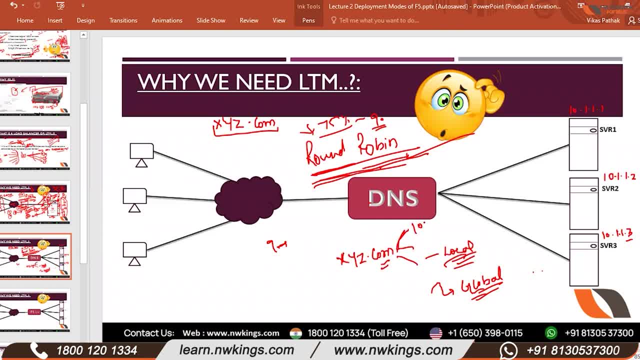 to aapko: agar xyz ki ek query aati hai, usko 10.1.1 me resolve karna hai. duzra aata hai to 1.1.1 me resolve karna hai. Sir, jese 2 pe gaya. 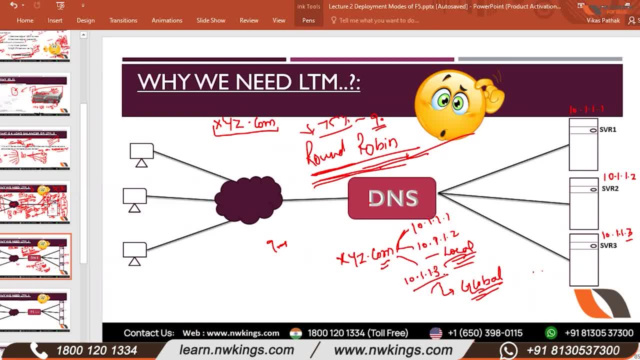 1 pe gaya 1 request. second pe gaya. second pe gaya third. agar down hua hai to third user ko to server unavailable, ya server not responding, like that is a message milega. Hmm, To wahan pe third user jo hoga. 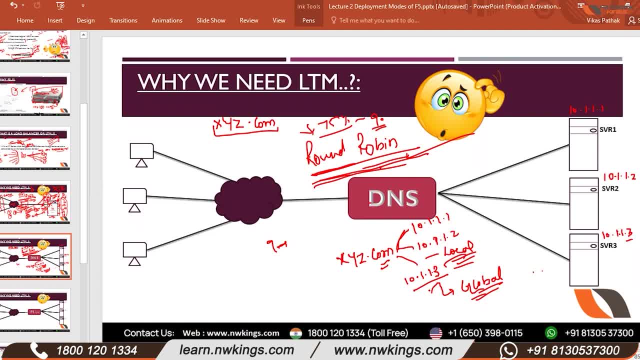 wo application ko avoid kare, like yeh, ko shopping website hai, to wo phir dusse shopping pe jayega. To yahan se hamara ek lost. yeh ho sakta hai, ki third user humar se lost ho raha hai. 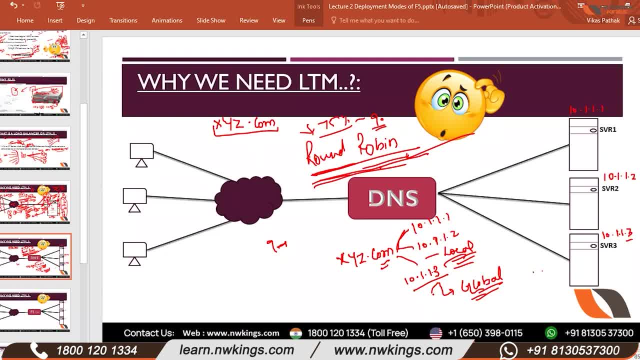 Hmm, Correct, Aapne first lecture attend kiya tha kya? No, sir, actually bata raha hu me aapko yaha pe jese aapne DNS ka bola to ek to yeh possibility aur dusra aapne jo round robin bola hai. 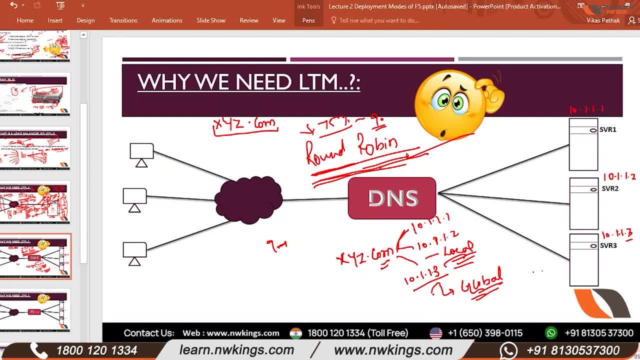 to wo third DNS, jo round robin method ke according to third server down hoga aur wapas up aayega, to wo usko query nahi bijega. toki yaha pe isa koi mechanism me nahi hai. 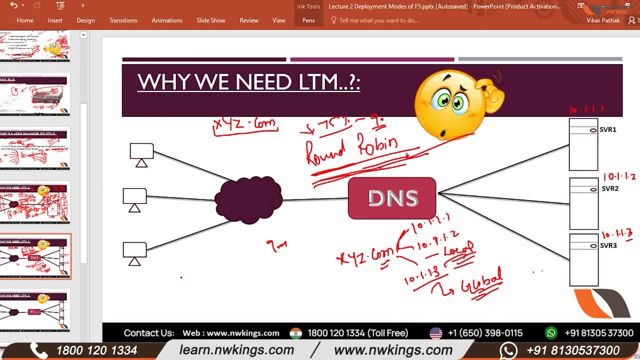 ki jo wapan usko bata hai ki active stand by se active me gaya, active se stand by gaya, to wo usko respond kare. Thik hai Aur kuch, aur koi problem aapko nazar aa raha hu? yaha pe. 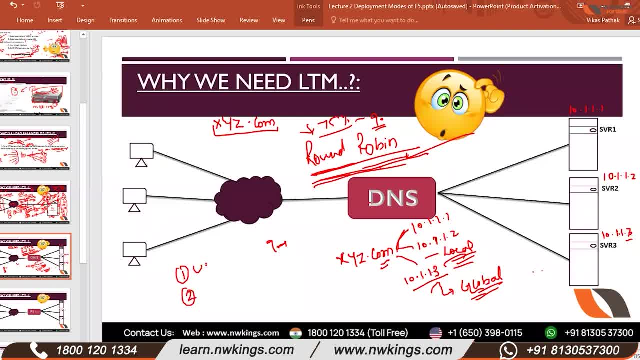 Aapne ek bola ki user loss. Ek. aapne bola: no mechanism of availability Right. yehi chiji boli aapne dono Thik hai. yeh maine note ki abhi discuss karenge. 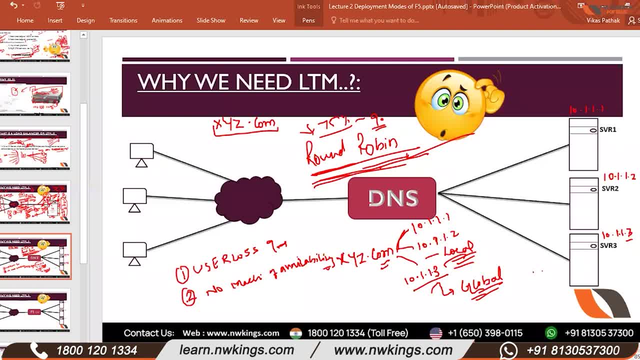 Aur koi solution, kisi ki mind maka kuch aa raha hu, Koi problem aapne nazar aa raha hu. isme I can see 21 participants hai aur 21 meze sirp 2 ya 3 ki awaz me agar. 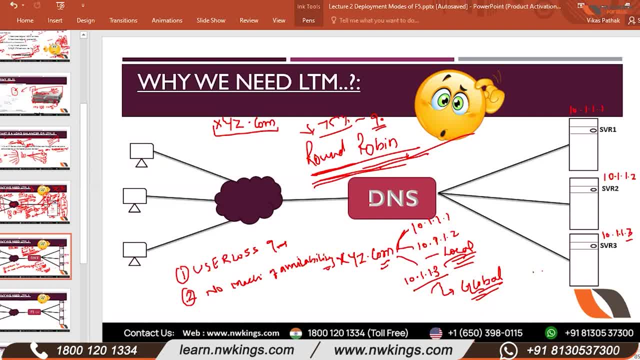 me sun pa raha hu, to mujhe lag raha hai, Baaki ko yaha to interest nahi aa raha hai. ya, fir, if I basically devise traffic, I think chai Jitika nahi question me pucha. 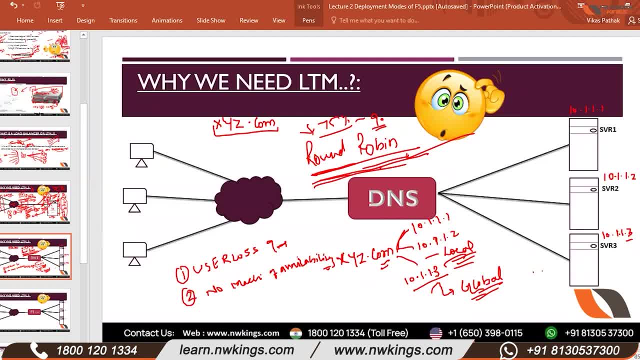 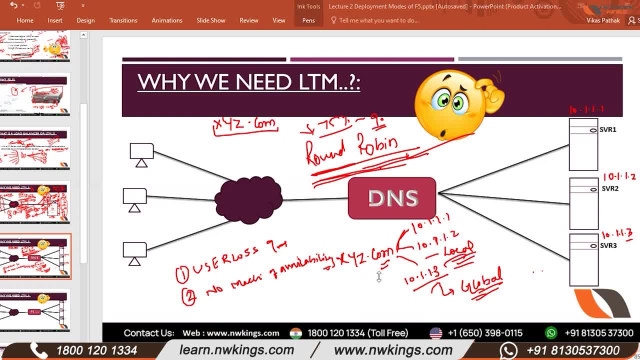 I don't know, I don't know, I don't know everyone moving to cloud, Working to leverage load balance service, Moving to cloud. I am not innovative 工作. tap 빛ص See pehli though. 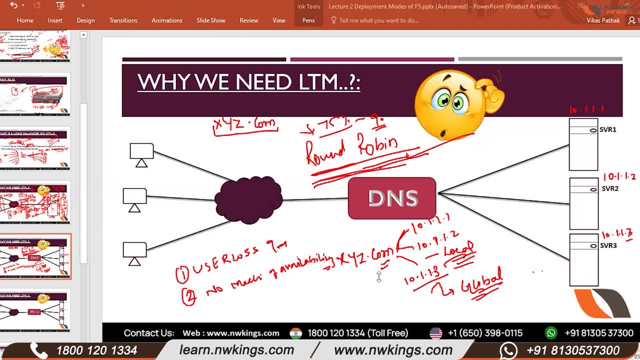 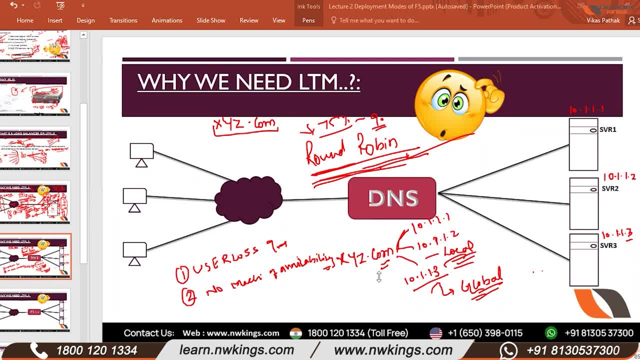 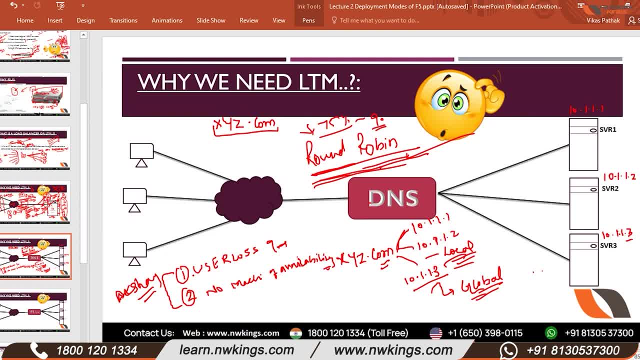 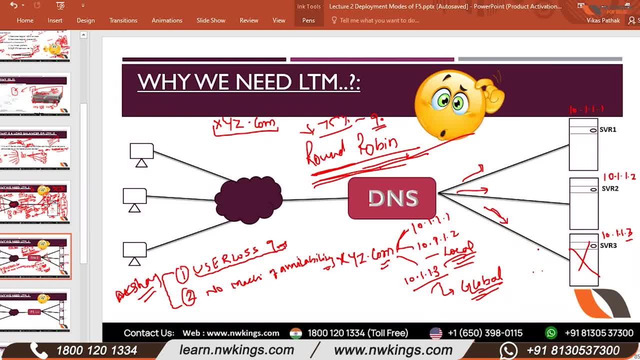 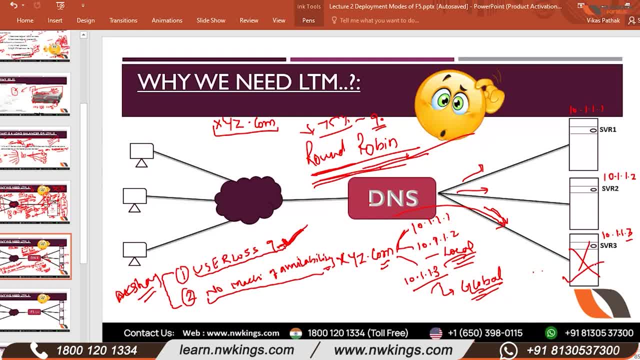 that this server is up now and I have to send that traffic on the third one also. right, Akshay, Right, But there is a problem. You are 50% correct over here And your statement is 100% correct- 100% wrong. 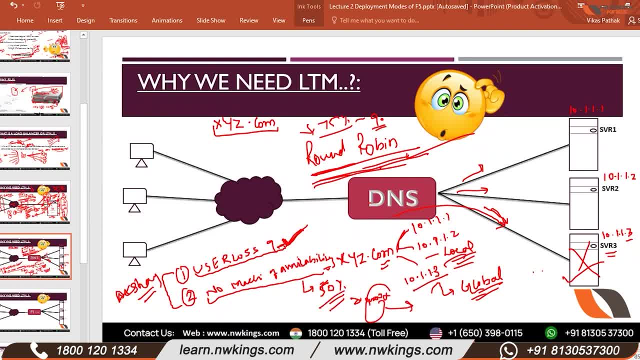 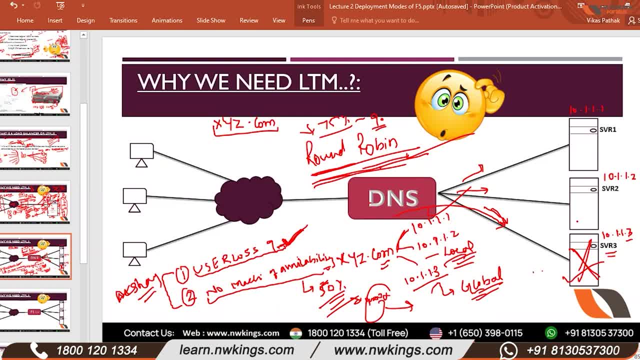 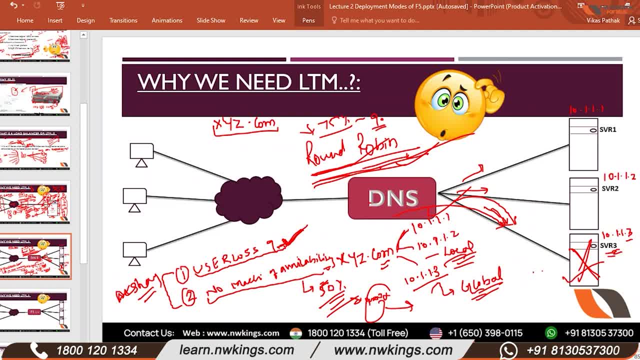 like getting landed on server 3. they are getting a web page error called service is unavailable. hello, hello, uh, check. If it is sorted now, then listen to it carefully. Out of the 100,000 users that were landing on this server 3,. 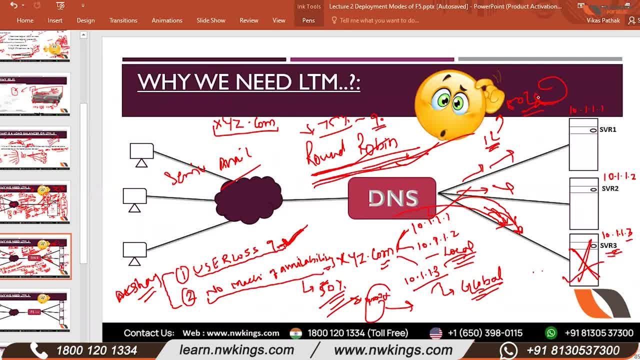 what did 50,000 of them do? They refreshed that page, Refreshed it, so it either landed on this page or this page, And the 50,000 users said: this application is useless, let's go somewhere else- Lost. 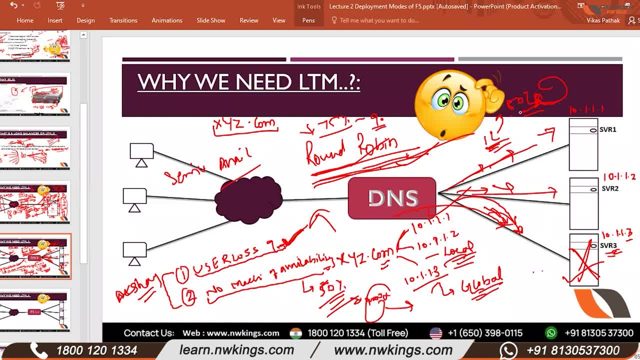 Or it is also a possibility that the 50,000 that they refreshed out of that, 25,000 were distributed here and the rest of the 25,000 landed on it again. So 50,000 went first, then 25,000 went later. 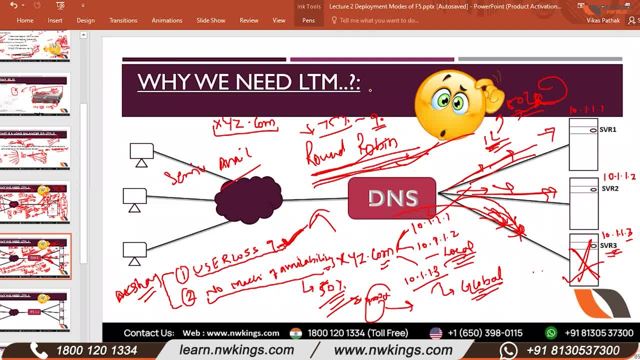 Or let's say 15,000 went, then 15,000 went, So 65,000 users for a time being lost. And if we talk about real business, and if there is such a big outage, such a big loss, 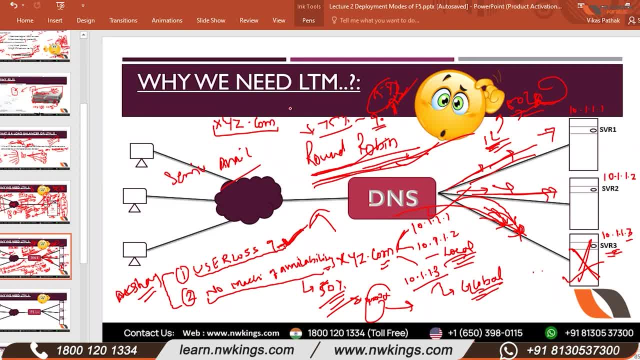 if 65,000 users have been diverted, if, let's say, they order a product of 1 rupee, then it was a revenue of 65,000.. It's a huge, huge, huge loss. Losses become billions. Employees go away in a flash. 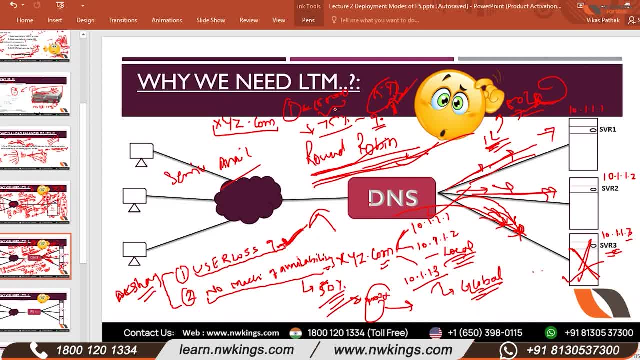 Has it ever happened to you- I mean, maybe in your team or in any other team- something like this has happened- that there was a down time and then in the end, the company fired the poor guy. This happens in real scenarios If you haven't highlighted the risk in the risk register. 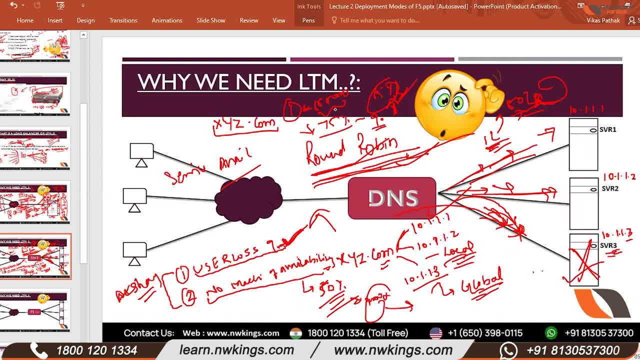 then, the day such a scenario will be made, you will have a risk. So always try to maintain a risk register and always try to inform your higher management, as well as the client, that we are sitting on a risk, So that, if that risk occurs tomorrow, 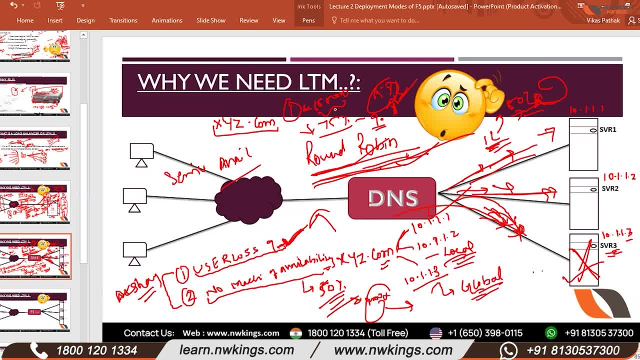 if there is a threat, then you tell me that. I am shouting from day one that there is a risk, there is a risk, but you guys are sitting with your eyes closed, Sir there is a doubt? Tell me, Sir, in case, in this scenario, if the FI was here, 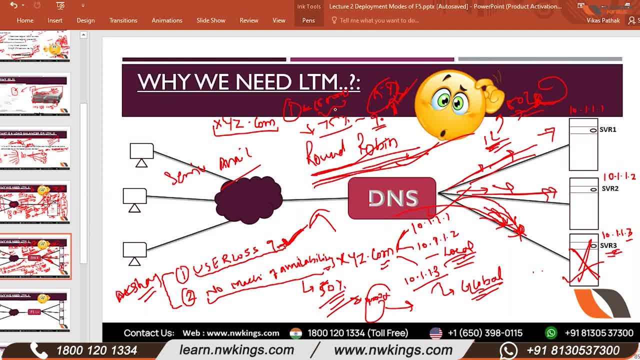 then this server, this application server, before it goes down, it will trigger an alert. right, Let's do it Now. in the next slide, FI is also coming in the place of DNA. Okay, Akshay, did I modify this second line in your mind, or not? 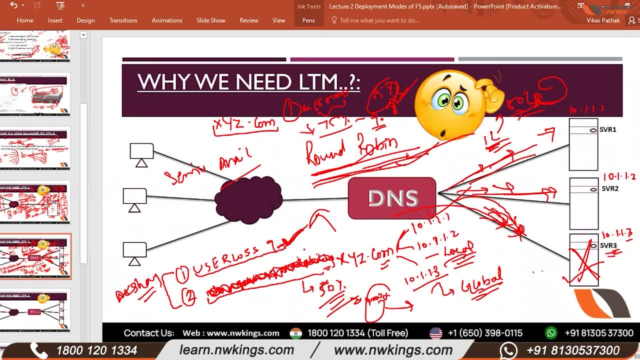 Yes, sir, I got a little clear. Did you get it? Yes, Is there any doubt? Can we move on now? Yes, sir, So with DNA. The problem was that it did not have any such mechanism that if any server goes down- or let's assume that the server is still there- 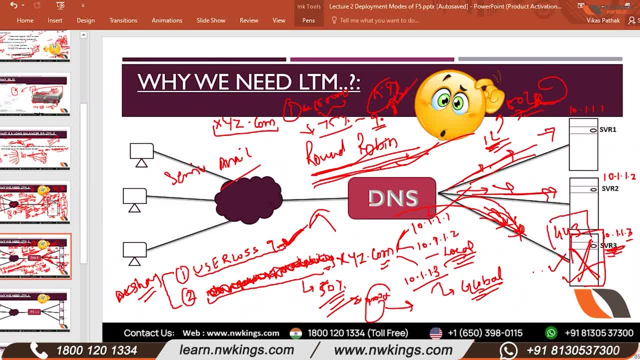 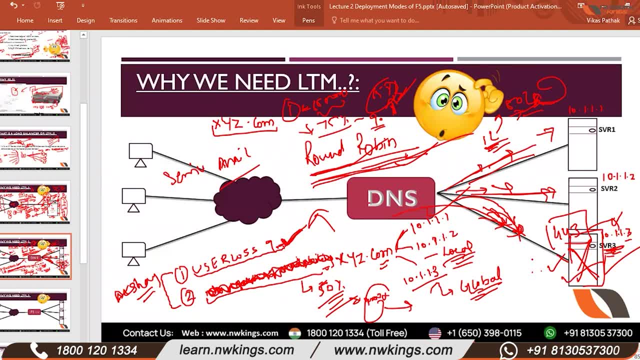 this service. if I am hosting the service of 443, this service is not up on this server, then it can do something about it. DNA has no such mechanism that it can stop its connection distribution that this service is not being hosted on this server. 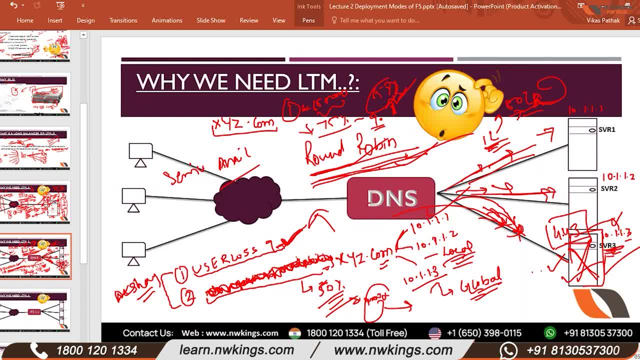 If it is not responding now, I will not send a connection request to it. DNA has nothing like that. Is it sorted Now the problem that we have come here? do you understand that problem? Then only you will be able to understand the solution. 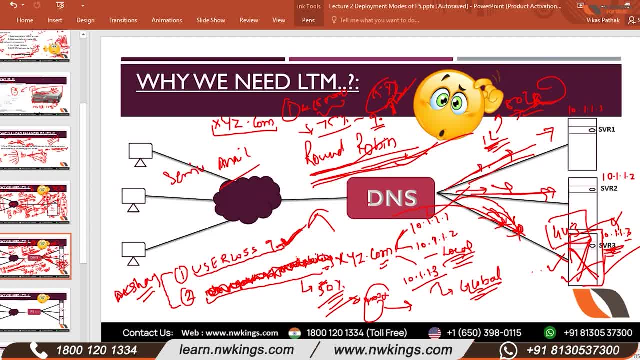 Yes, sir, absolutely. Did you understand everyone? Is it clear? Yes, sir, it should be clear. Yes, sir, it should be clear, Sir, what is the problem? Yes, sir, what is the problem? What is this? 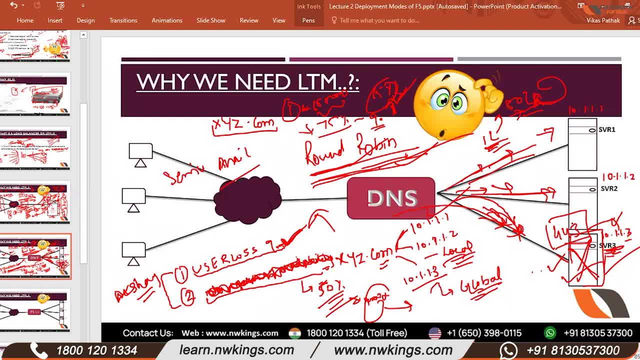 Sir, the problem was this: Yes, sir, this is the problem. Yes, sir, this is the problem. Like if there was a service hosted in the server and the server goes down, then the DNS doesn't know that the server is down. 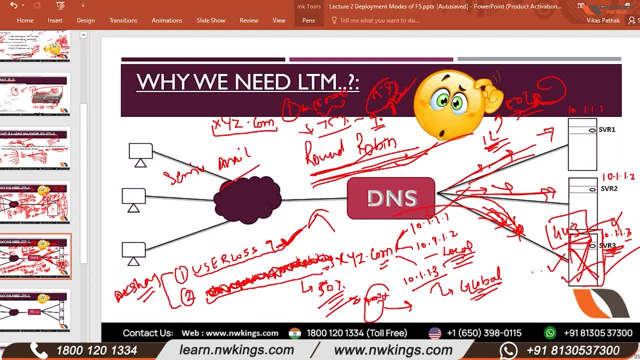 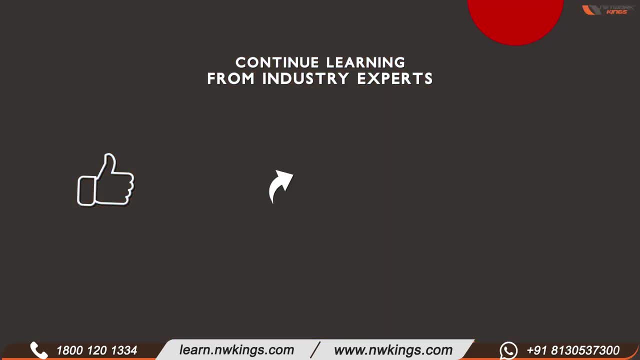 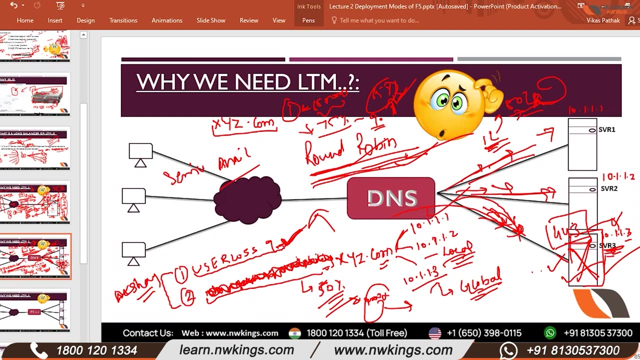 Meaning if there is any loss in the infrastructure, then the DNS doesn't know. Okay, First of all we have to tell the DNS that the server is down. You can't tell, You have no mechanism For that. one option is to bind different URLs for the IPs of these three servers. 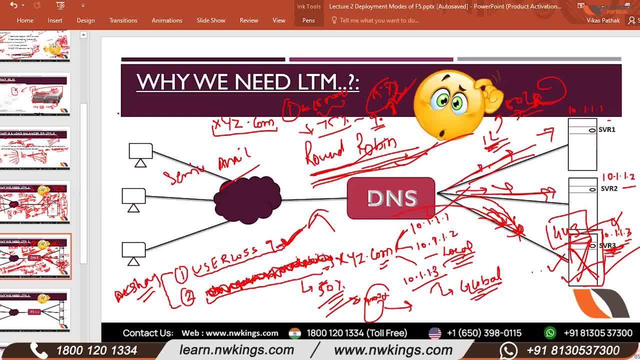 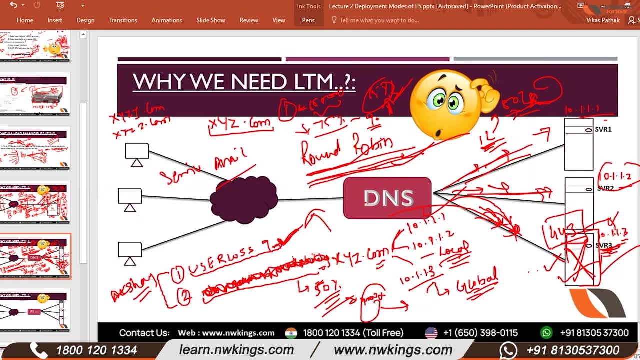 I am telling you the solution. If anyone wants the solution, then xyz1.com will be in 10.1.1.. xyz2.com will be in 10.2.. This is your second server And xyz2.com will be in 10.2.. 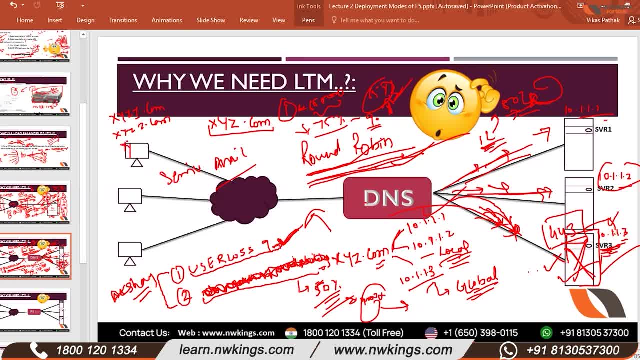 And xyz2.com will be in 10.3.. And you go to your users and you tell them that Sir, you are the first 100,000 users, So you have to use xyz1.com. Second, go to 100,000. 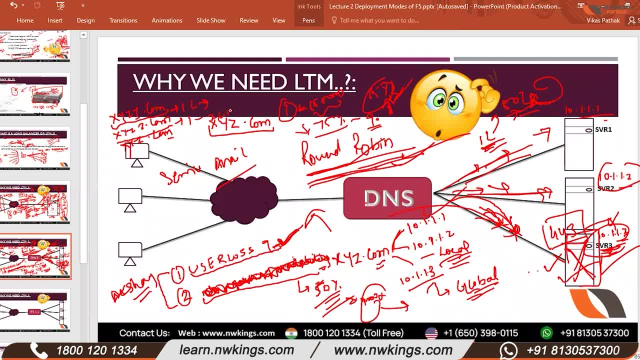 Meaning how many users come between 100,000 and 200,000?. Go to them and tell them that you are xyz2.com, Use xyz2.com, And the rest go to the users of 200,000 to 300,000 and tell them that you use xyz3.com. 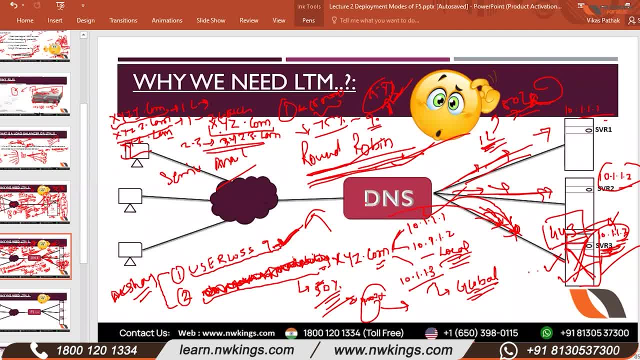 This is a solution, But you tell me, is it feasible? No sir, No sir, It is a solution, It is feasible. It is feasible, It is not. Flipkart cannot go to clients and can say that you have to use flipkart1, or you have to use flipkart2, or you have to use flipkart1000, 1000 servers. 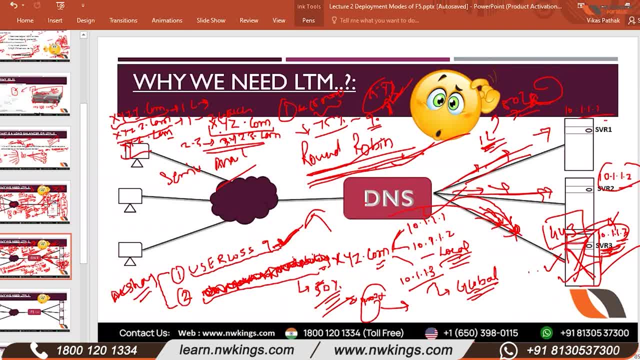 Amazon cannot do this, Flipkart cannot do this And we will create a big problem for ourselves And the client base will break. It will break Cool. So we don't have any mechanism that we can resolve the issue through DNS. 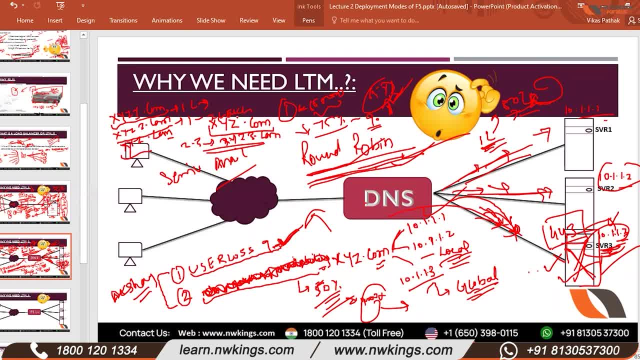 But in today's market this service will not be used. sir, The DNS column, If there is a small infrastructure, then for the time being this can be used. Okay, Let's assume flipkart. we are talking about the client. 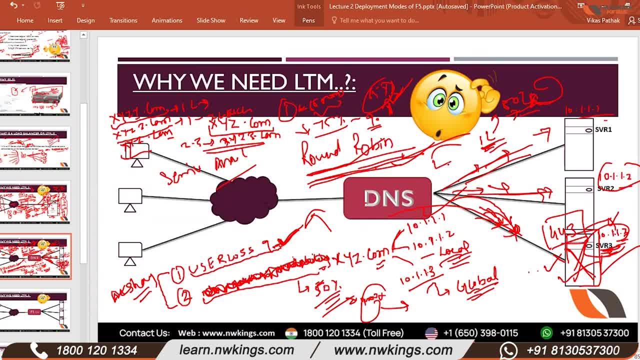 The problem of attendance. The problem of attendance Where we hosted. You assume that it's an internal application. Assume that you have 100usr- 100 employees. You have to mark an attendance of 100 employees. You have created two application server for it. 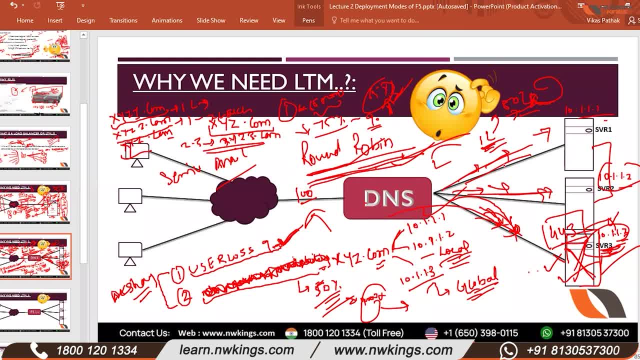 And by DNS center load valence. you are doing it There somewhere. if you are using this problem of DNS and if small problem comes, you can ignore it. Suppose there is an employee. He did not come for 4 days. 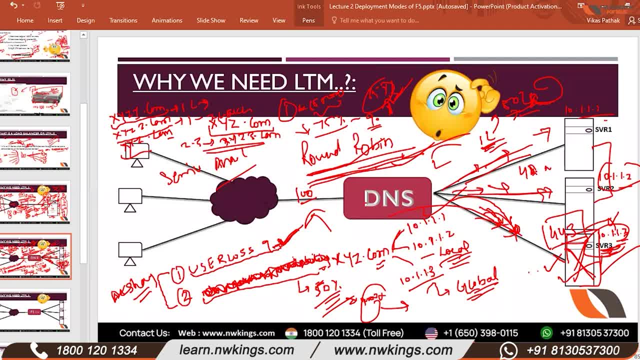 Small. There are 100 employees, or 5-10 out of 100 employees, who did not fill attendance today because the server was unavailable, so we will fill it out tomorrow. right, There is no problem in that right. But if you are there and you need a pencil box for your child or you need it for your niece, 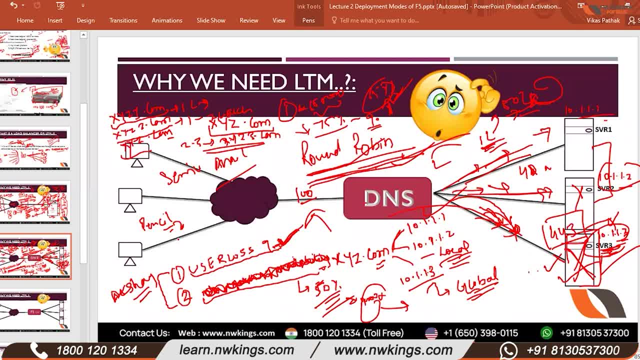 then you need it today, right? So if you order it today, then it will be delivered tomorrow. If you do it tomorrow, it will be delivered the day after tomorrow. your child will go crazy by the road that there is no pencil. should I read it? 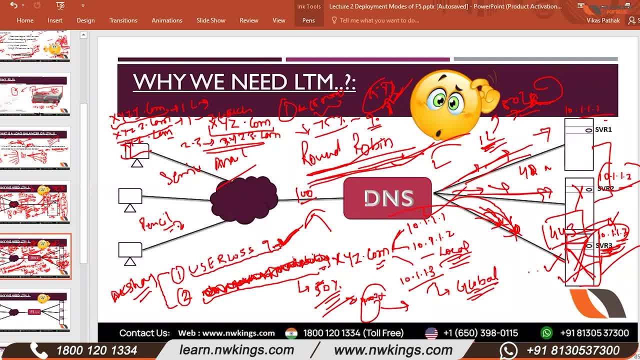 Your wife will say that I don't have flour, so how can I make bread? So there are many small infrastructures where the criticality of the application is not so much there. this can be used for a tool for a time being. see, this is not the ideal solution. 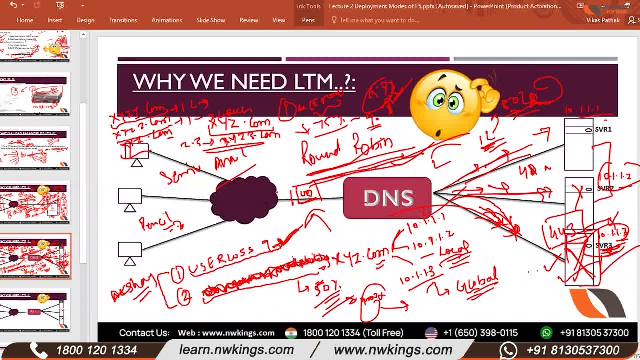 for a time being you can do this, but bigger infrastructure is not recommended for critical applications. this was the initial process when F5 means like load balancers- were not there. then it was done initially that okay, use dna now. what is the problem in that? one person was continuously monitoring that. the server is up. the service is up. the server is up, the service is up. 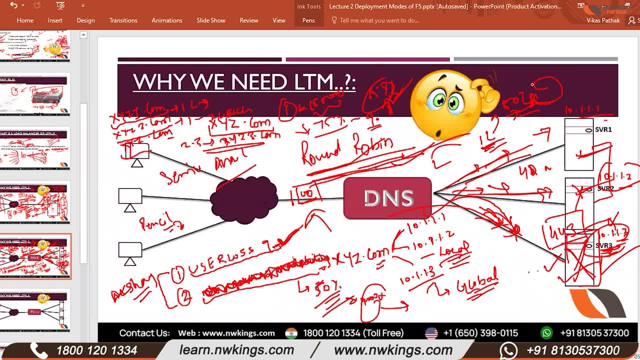 if you remember, if someone around 2010 from the computer, if it is familiar- ever entered in the server room, then one body did screen nothing work with. it was working server's ping small boxes were open and pings to check the availability were running on that big screen. 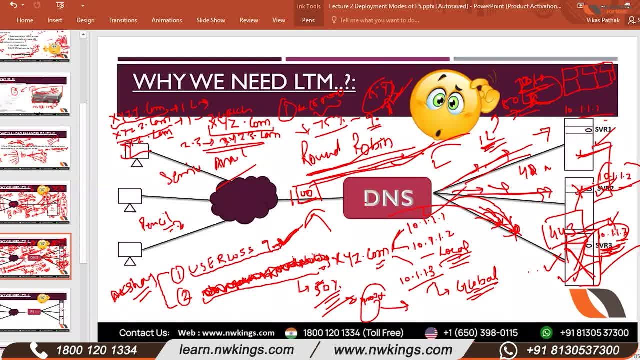 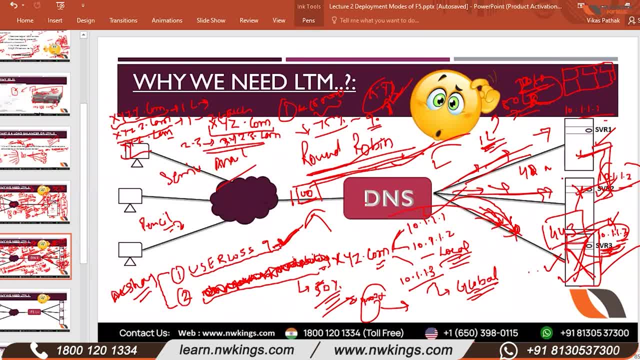 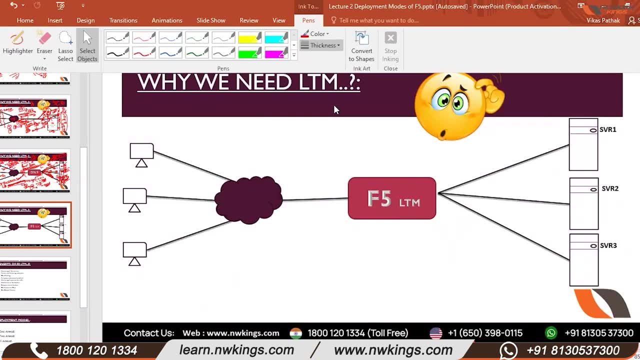 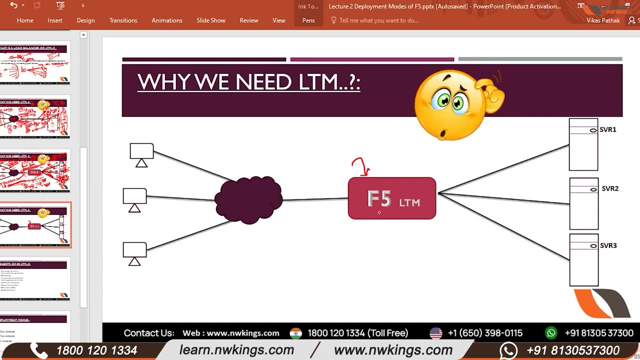 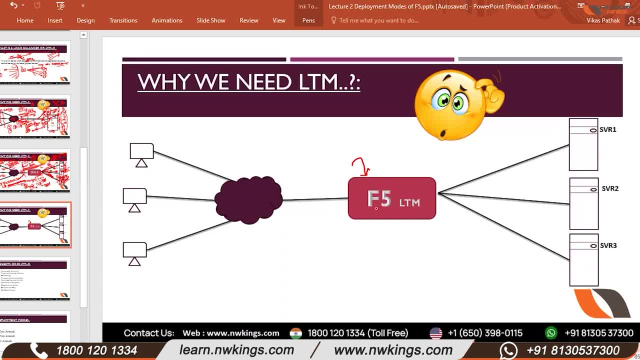 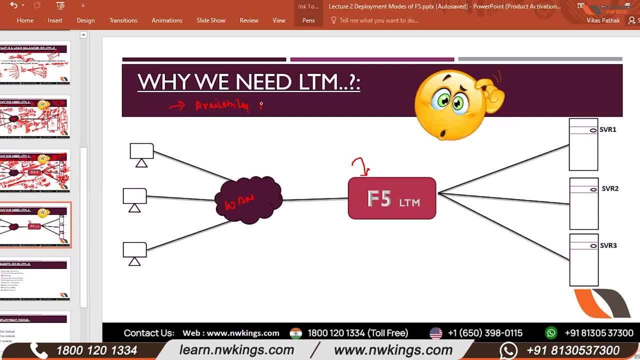 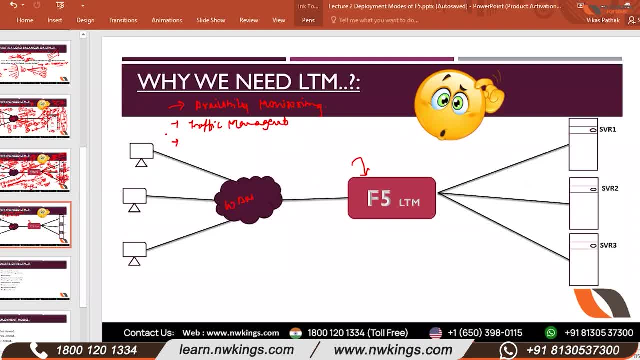 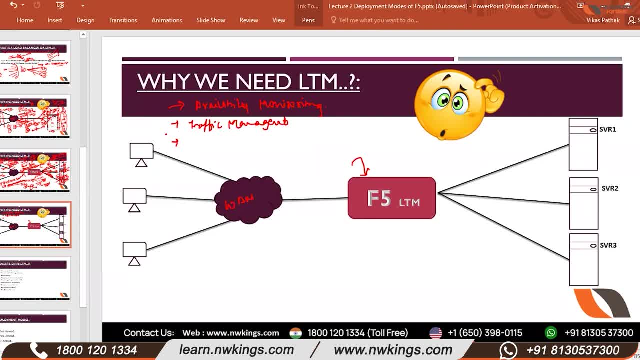 Yes, Yes, Yes, Yes, Right, Right sir. So, Akshay, we have to discuss the problem. We have read about the problem, So we have to discuss it. Okay, let's listen to you. You have said that you do monitoring. 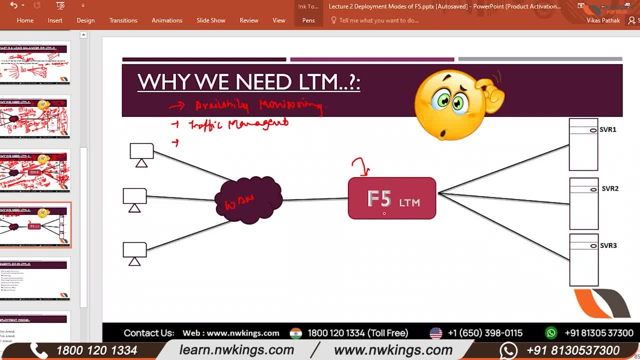 How do you do it, Sir? I don't know that. I know this much As I do some work. I have some idea. Okay, nice, It should be like this: You should take some understanding in any session. So what will happen is that: 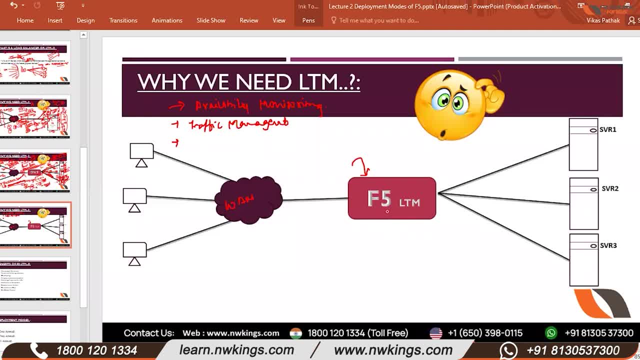 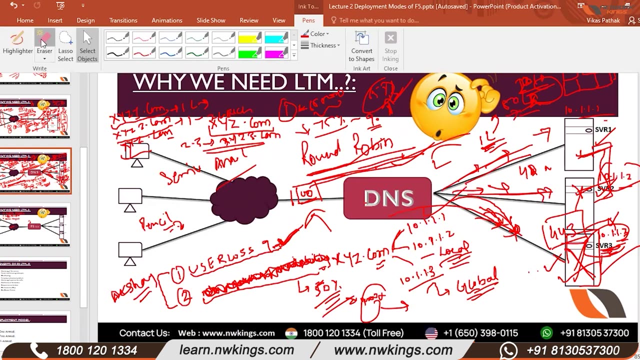 the discussion becomes interesting. Right, Okay, nice. So what did we do? First of all, we had availability monitoring, traffic management. One problem was service monitoring. Okay, I didn't discuss one problem here. Let me quickly discuss it. 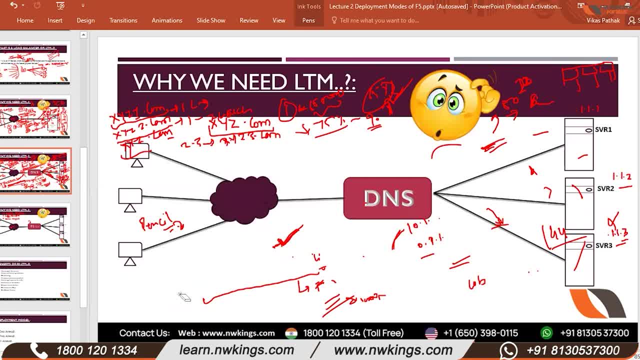 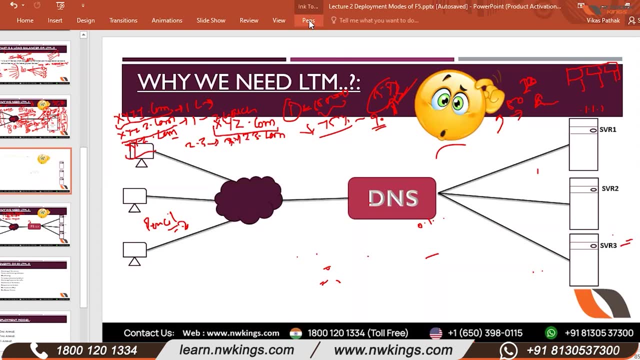 Otherwise you have told me. Now tell me this: Does everyone see Server 1?? Yes, sir, If I assume that Server 1 has 64 GB RAM, Okay, It has octa-core processor. It has 512 GB. 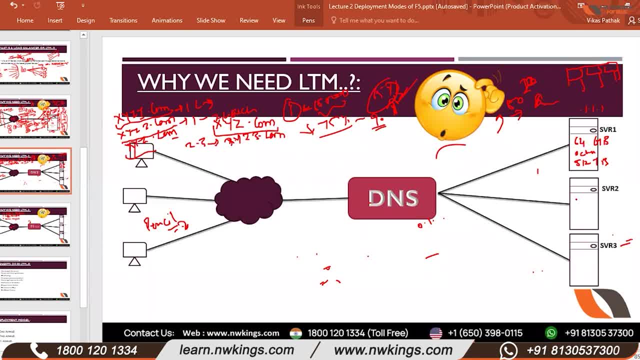 hard drive. Server 2 has 128 GB RAM. It has octa-core processor And Let's say 1024 GB, It has hard drive. Okay, Server 3 has 8 GB RAM. It has 4-core or 2-core processor. 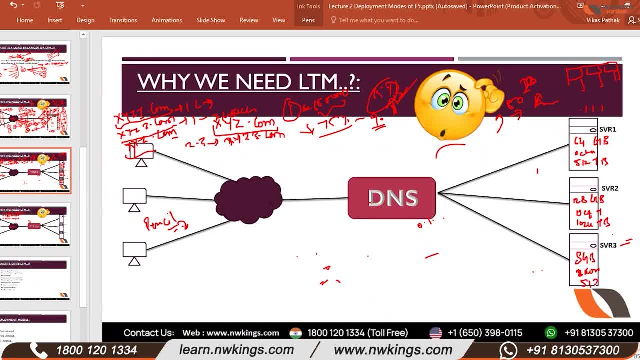 It has 512 GB hard drive. Hard drive Which is the most sufficient high configuration server, Server 2,, sir, This one. Now, let's assume that Server 2 has 8 GB RAM, If this server is the most sufficient. 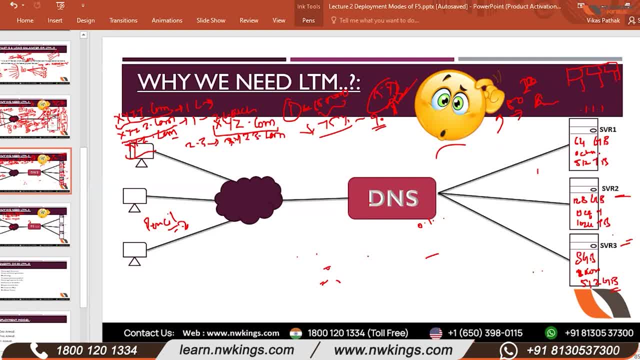 the most high-end configuration Approximately. this server has double configuration And this server has 4 times the configuration of the second one, Right. So in comparison, if my Server 1 is handling 2 connections, then Server 2 should handle at least 4 connections. 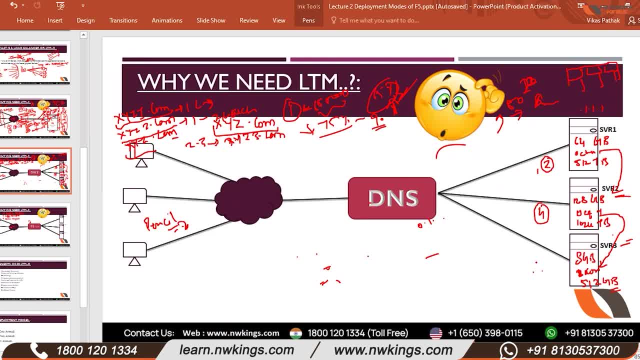 Correct, And if my Server 3 is handling 2 connections, then it should handle at least 8 connections. But if I am using round robin here, then is it feasible Through DNS? Nope, DNS doesn't have any mechanism to do this. 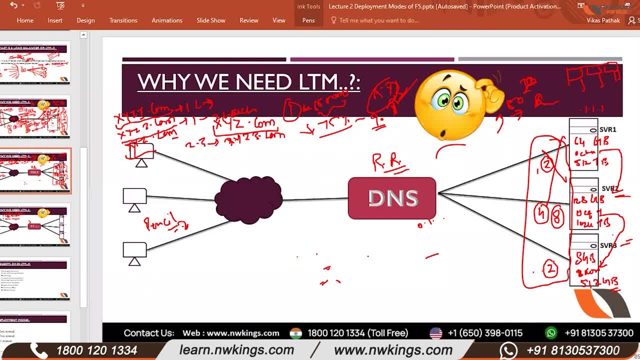 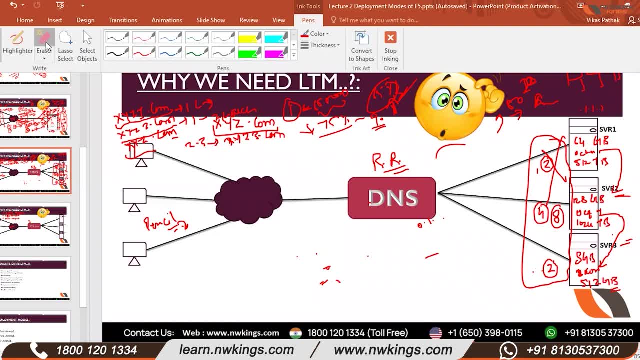 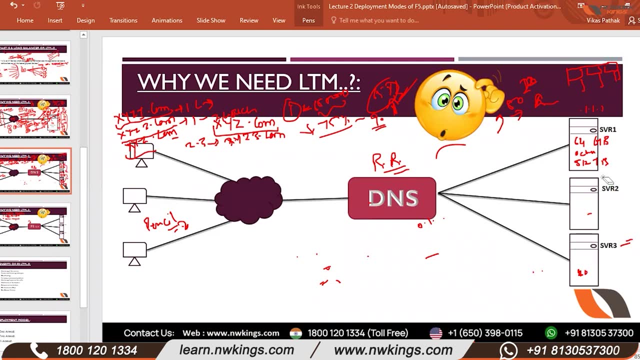 According to the capability. the connection should be provided. Make sense. Yes, sir, There is one more problem which you guys didn't ask. Ask: what, Sir? what? Note this first: What Capability? Resource management, Capability Management. 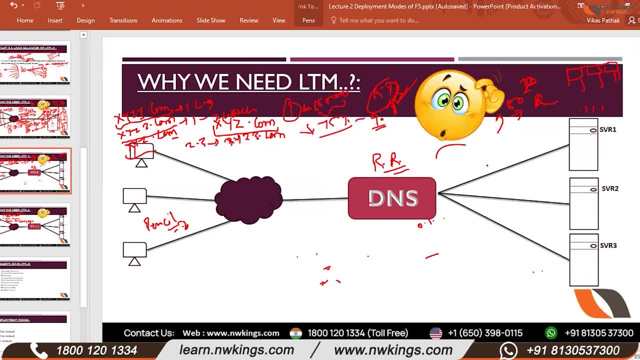 What is that problem which we are going to discuss? last, There is one connection to Server 1. Akshay Akshay opened F5.com on Akshay's PC. Akshay is a very curious person. Okay, His connection. 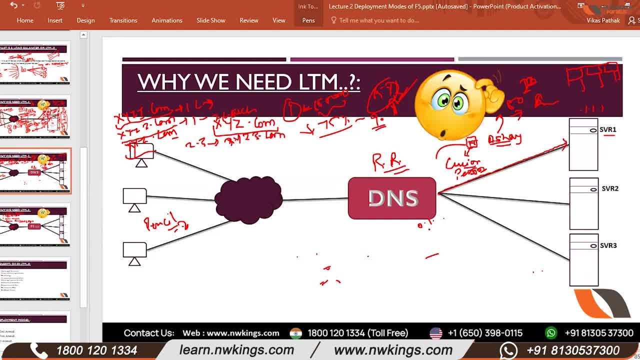 went to Server 1.. Akshay logged in at 9 am in the morning. Akshay thought: today I have to take all the things of F5. Today I have to take all the things of F5. Today I will search. 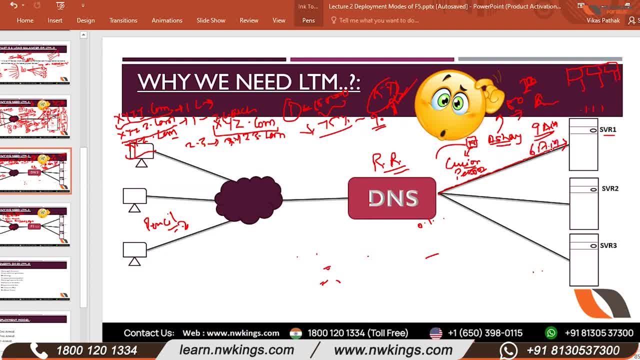 all the things of F5.. It is 6 pm. Akshay is still on the website. Akshay has put a lot of things like admin guide manuals and a lot of things on download. Another person is Vikas Vikas. 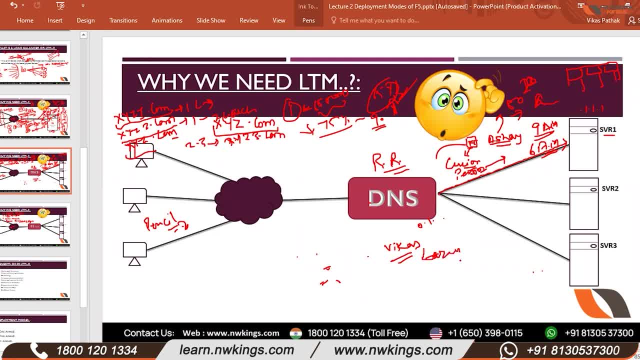 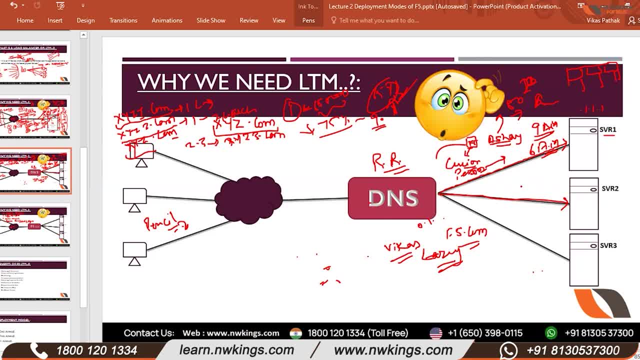 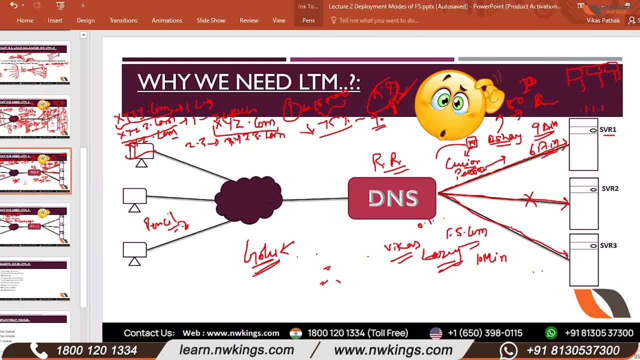 Golu, Golu, Golu, Golu, Golu, Golu Golu. So Akshay is still sitting near server 1 and R&D is being pressed on it. Server 2 is idle and server 3 is idle. Round robin is going on. 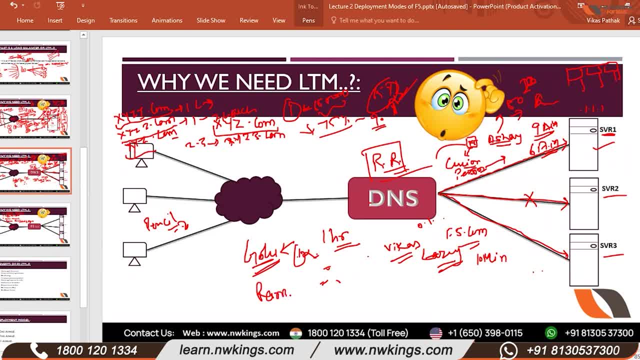 Number 4 is Raman. Now we have read the question of Raman, right. Let's see the name quickly. Rohit, Rohit, Rohit Maan, Rohit is the question. Are you Rohit? No, sir. 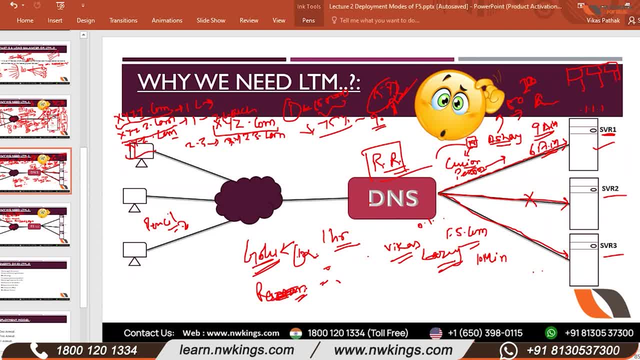 Okay, Let's assume Rohit. Let's assume Rohit. Rohit is also a very interesting person and curious to understand everything. He said that today Vikas had told that there was something like this. Let's go to FI and see what happens. 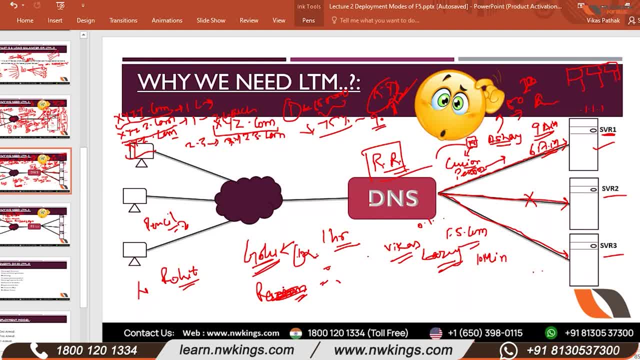 What he did. He went to DNS and DNS saw that there are four connections. Where will the fourth connection go? On server number 1.. Now tell me one thing: A very typical data transfer is already happening on server 1.. And server 2 and 3 are idle. 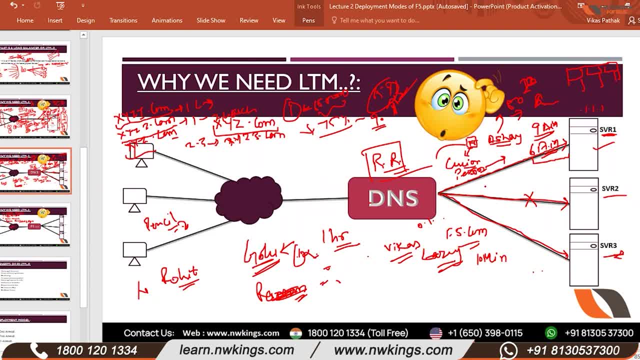 So logically, shouldn't that connection be routed on server 2?? Distribution should have been done this way Or it could have been done on 3.. But what happened? It went to 1.. Let's assume there is a scenario that 60% of the cases of connections and typical users are landing on server 1.. 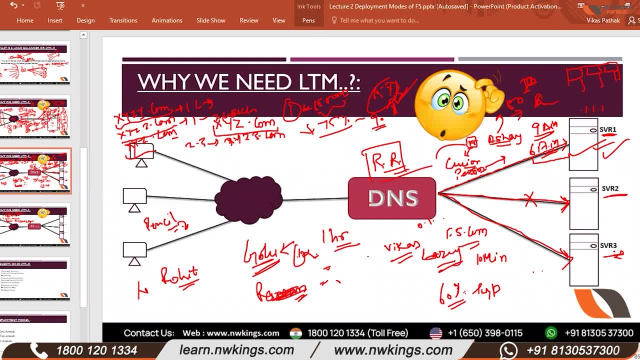 And the remaining 40% or 20% are doing it on server 2 and 3.. So what will happen over the time is that the active number of sessions will be more on server 1 and less on server 2 and 3.. 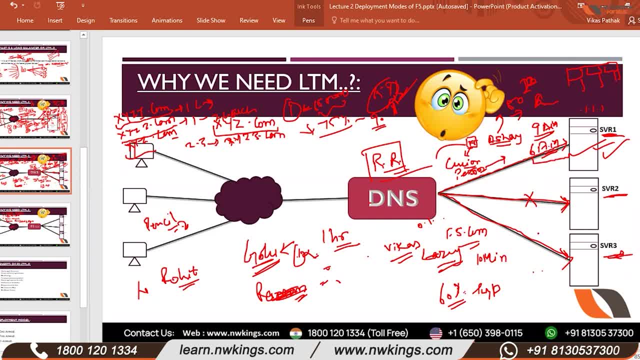 Because their users are coming quickly. They checked and left Right, So ultimately what happened? Server 1 will be highly utilized over the time and it will sit. Akshay will say: oh man, what a cheap website. When the website is so cheap, the product is so cheap. 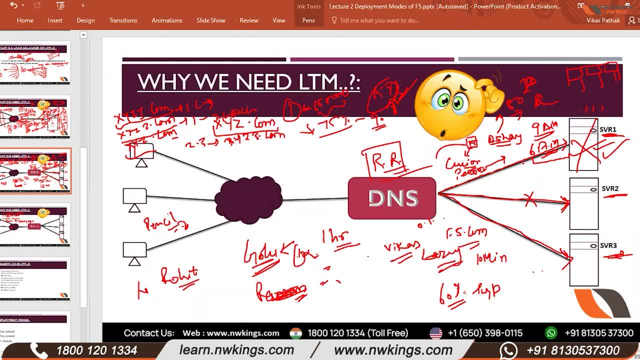 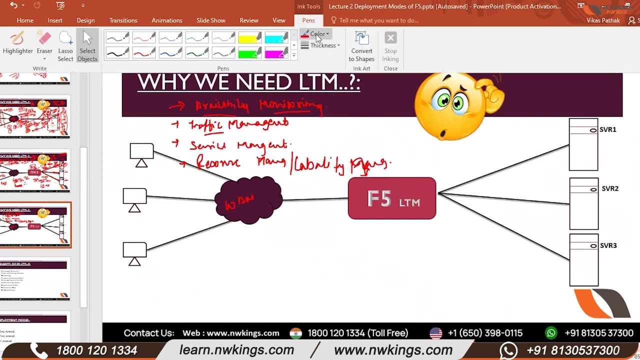 And Akshay is an IT manager in a company, He will say: no, I don't want F5.. Bring Citrix, Bring Netscaler, There is no problem. Yes, We will bring the solution, What it is called. 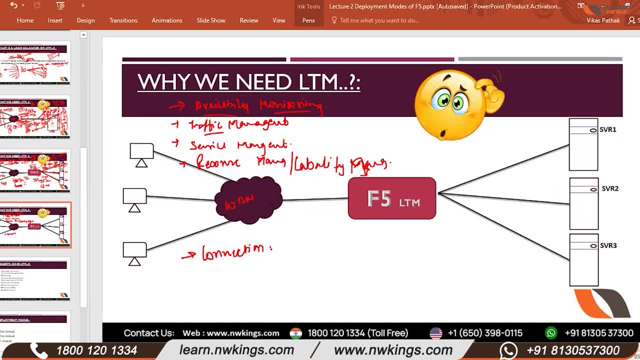 Connection management. This was the main problem of our DNS Or before load balancer. Whatever method we were using, This was their main problem. After that, one solution came: F5. And it sorted out all the problems. What did you do first? 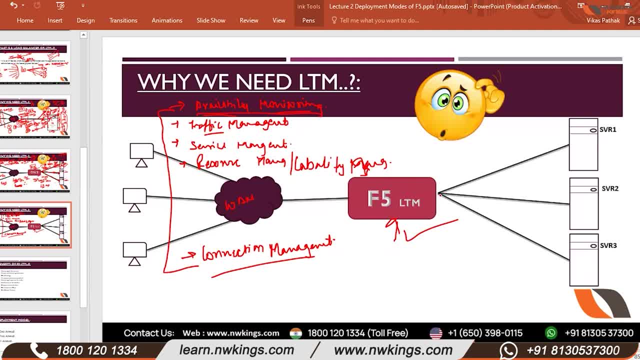 You started polling on the server. What did you do, Akshay? What did you do? Polling, Polling, Why he did- Or, sorry, why it did- To check the availability, Whether the server is available to accept the connection or not. 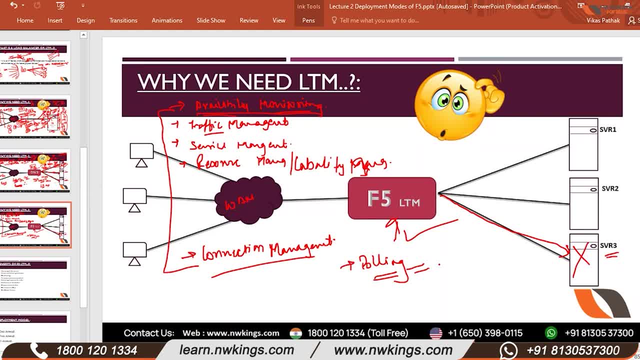 Server three down Poll ka response nahi kiya. Three poll miss huve. It will remove server three from the list And it will start transferring the data between these two. Similarly, service monitoring: Server up hai. Server up ka up hai. 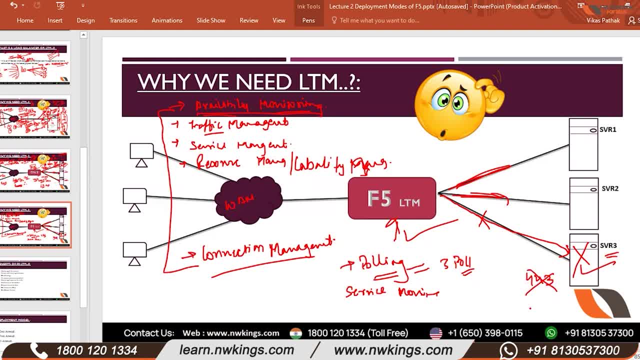 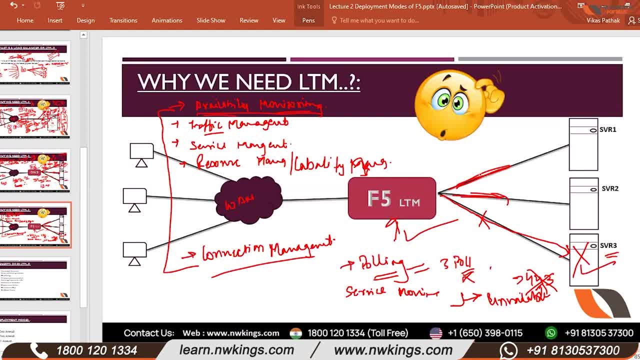 Service unavailable Service unavailable- Directly Distribution: start hokey en doho. har ke bichi main Okay. availability monitoring chale gayi- Sold ho gayi. Availability monitoring chale gayi- Sort ho gayi. Availability monitoring chale gayi. 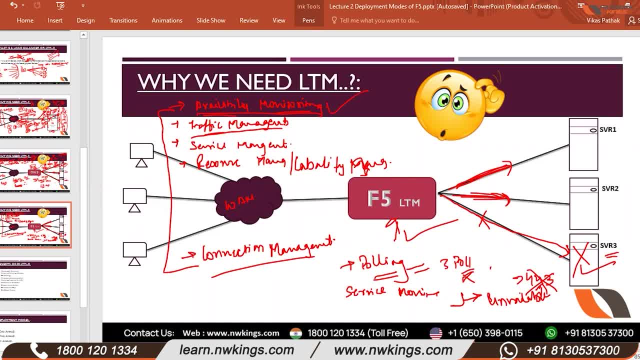 Sort ho gayi, Traffic manage, Traffic manage. What you can do is take Trafic Management or Connection Management. Let me explain it to you separately. This is server 1. I have set 443 on this. 443 on this. 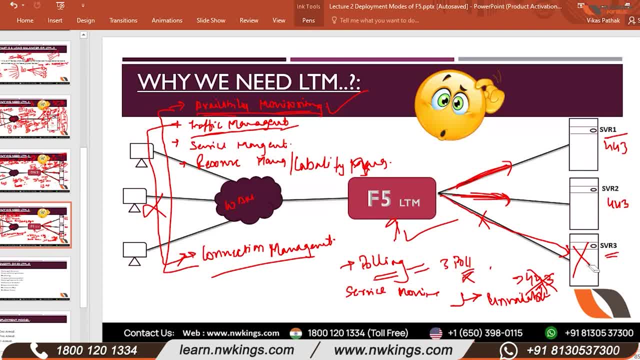 And this is not my server down. Let us call this: This is up. So what did I do on this? I hosted 443.. Plus, I hosted port number 21 on this. So traffic management: If there is traffic of 443, distribute it on all three. 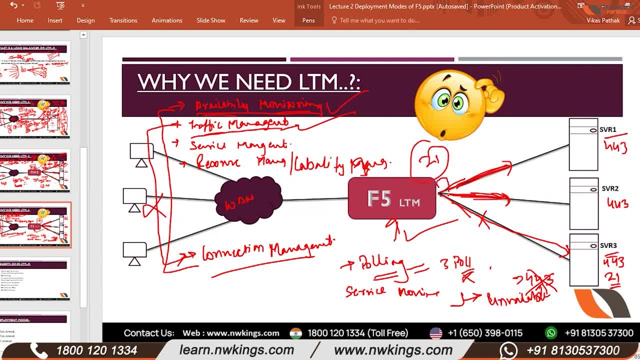 If there is traffic of port 21, where should I send it? Say it fast: On server 3.. Definitely it will not send that port 21 traffic to server 1 or server 2.. No, Never. Traffic management. 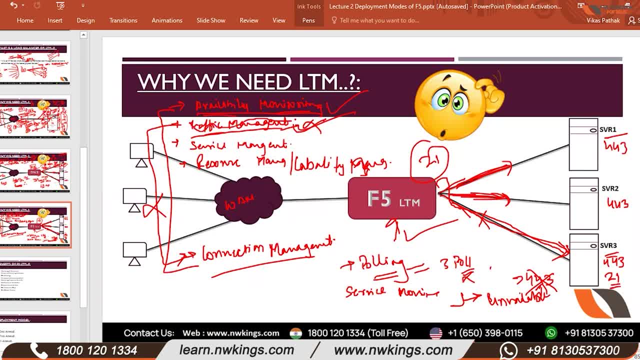 It is sorted, No problem. No problem, Service management. Do the polling of service? Is it sorted That we are monitoring the hardware, We are doing the poll? That is okay. We are also monitoring the service too, If two services are active on our server. 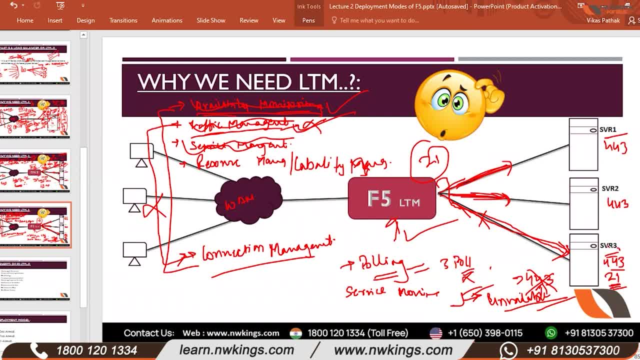 443 and 243.. We will do monitoring of both of them. If the hardware is down And if the service is not responding after 3 polls, Before removing it from the list, It will generate an alert to the administrator That this particular server is not responding. 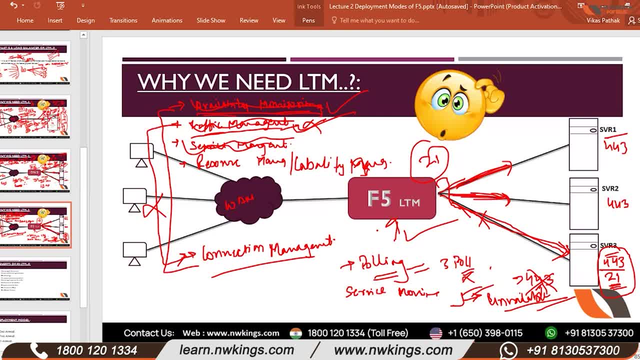 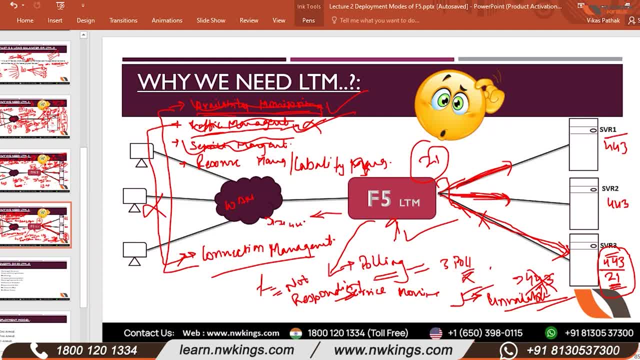 This particular server, On that server, This particular service, 443 or 21.. Is not responding? Go and check, Sir. one doubt. Yes, Sir, when any user comes And request for that service, Then FIA will find out That this service is down. 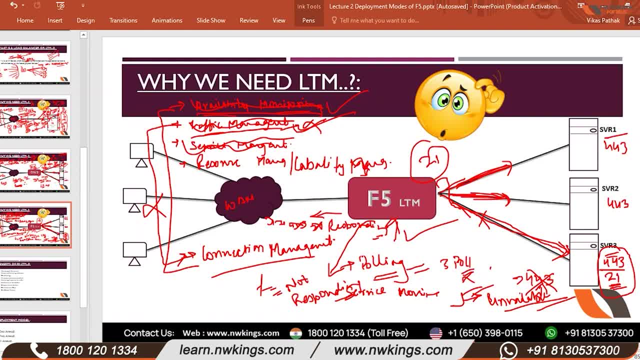 Say, or Continuously in the background, it will keep on doing it. It will keep on sending some kind of messages. Yes, It will not keep on checking when a connection comes. It will continuously be doing it, Whether the service is up or not up or not up or not. 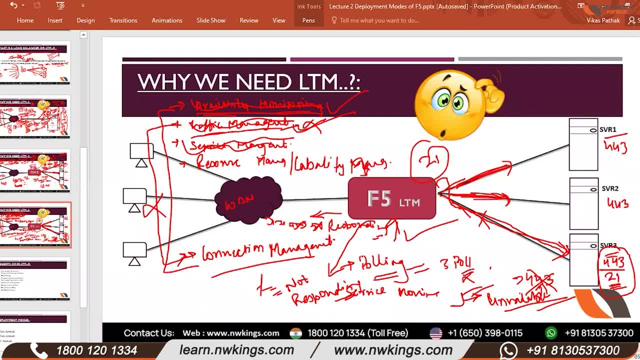 In a particular interval. What will be its time range? sir, Time range, you can modify it. If you want it in 5 minutes, you can do it. If you want it in 30 seconds, you can do it. Okay, okay, got it. 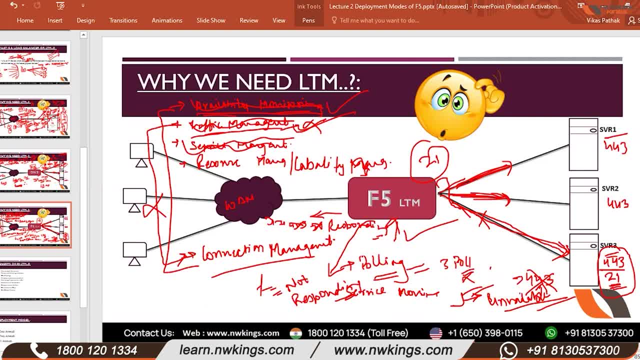 There will be a default time as well, right, sir? I don't remember the default time as such. We will enable it when we are in the lab. we will see it okay. Okay, Actually, in most of the cases it is 30 seconds. 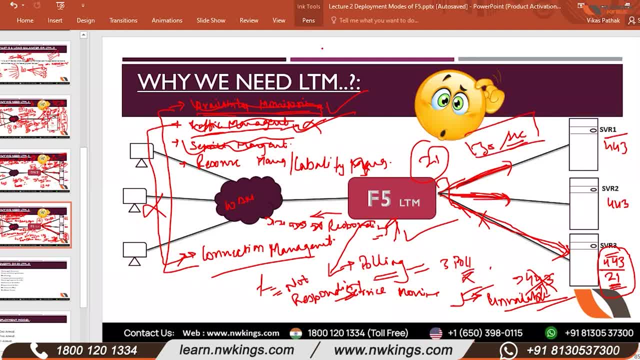 But actually we will see it there, okay. Okay, service monitoring is done, port monitoring is done, hardware management is done, traffic management is done. The highest configuration is of server 2.. It will check and we can distribute the ratio-based traffic. 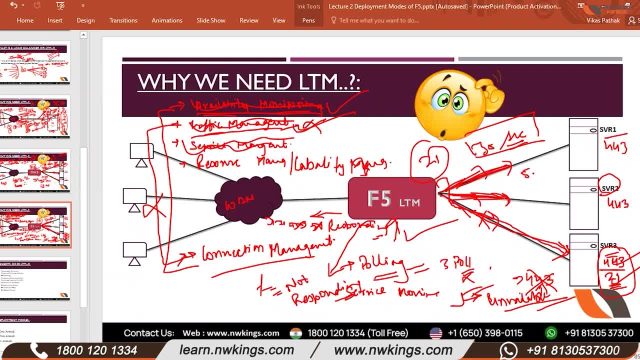 That if I have 5 connections coming, then 1: 1 connection goes to 1 and 3, the remaining 3 connections go to my server 2. This we can do with FIP. Okay, traffic management is done on the basis of hardware. 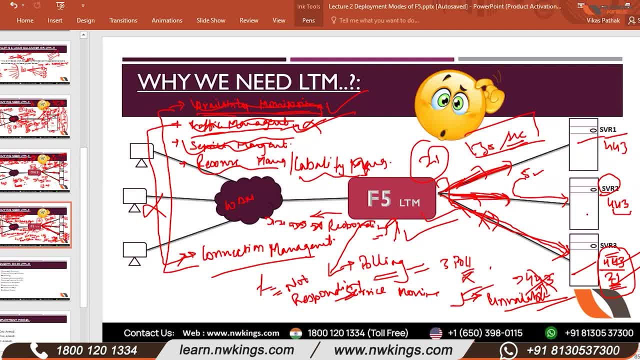 Resource management is not done. Our server, which was highly configurable. what did we do with it? We sent 3 connections to it. The rest of the servers were ours, Or we can also do this. We sent 2 on this, 2 on this and 1 on this. 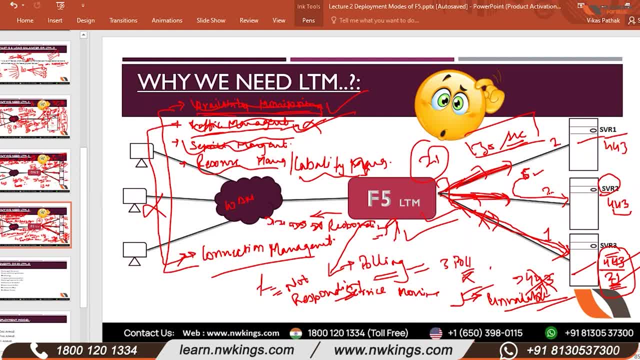 Or if there are 6 connections, we can send 3 on this, 2 on this and 1 on this. We can do that, okay. Last connection management: There are 100 live connections on this. There are 4 live connections on this. 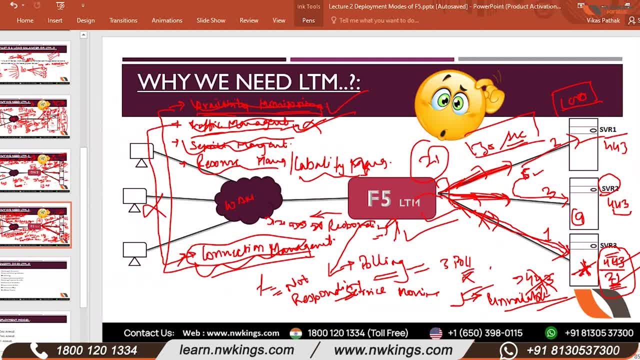 This is idle By default. the next connection will land on the server 2.. The next connection will land on server 3. Until or unless it will be having 4 connections. As soon as there are 4 connections, the traffic will start redistributing between these 2.. 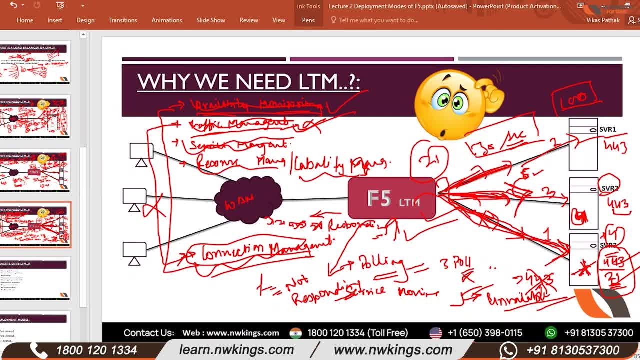 Not redistributing, it should be distribution. Distribution will be happening between these 2 servers, Until or, unless it will be having 4 connections, These two will be having at least 100 connections As soon as all 3 will have 100 connections. 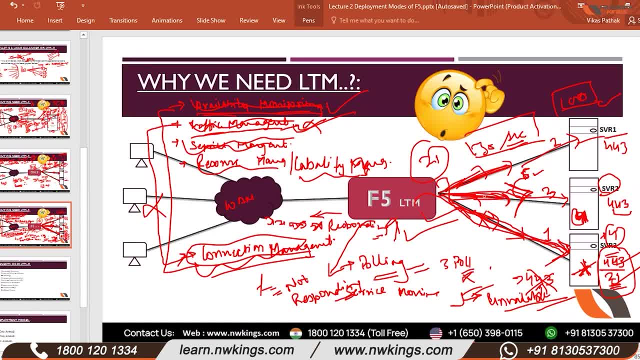 all 3 will have 1 connection unit. That's called connection management. It will maintain a table that which server is having how many active current sessions. Is it sorted, Sir? there was a question. Sir, when a server goes down in F5, what will we do to check that the server is down? 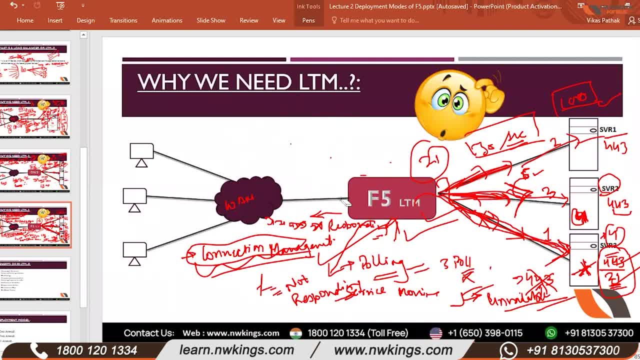 We will involve the server team to check that the server is down. Yes, Then we can monitor the server down with our answers. then the server team will check. If the application is down, the application team will be informed. If the server is down, the server team will be informed. 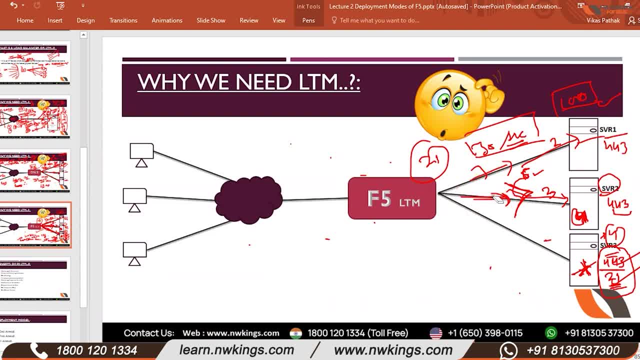 Or we can do one more thing. We have provided one more thing here. Ask what? Yes, Okay, okay, okay, Let me ask one more question. Okay, I was expecting that you will ask me, but you didn't ask. I will ask you. 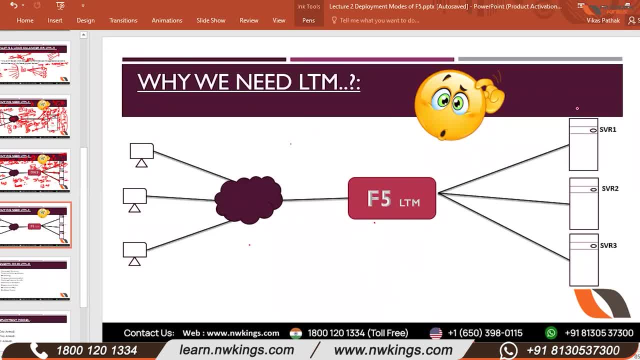 Do you remember that we were using DNS? You don't remember? Yes, sir. So what were we doing? We were resolving the IP through DNS in 1.1.. In 1.2.. In 1.3.. In 1.3.. 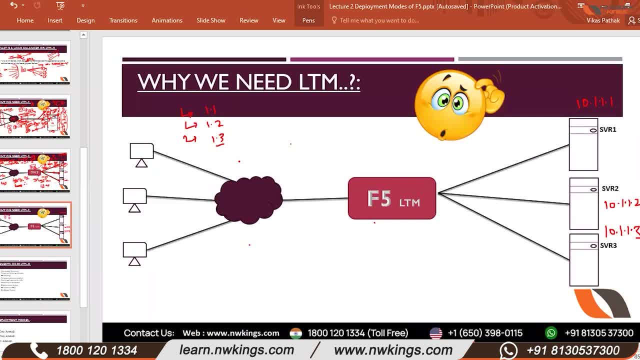 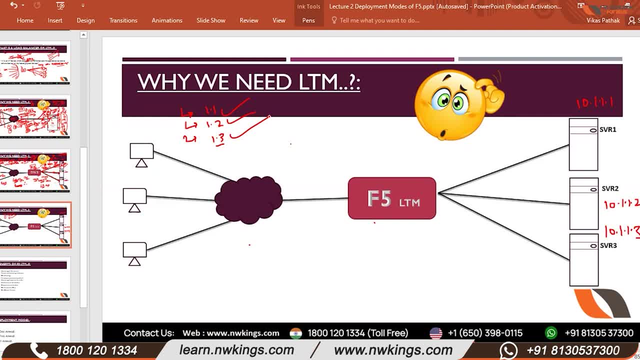 That is dependent on the service, right, sir? All three are using 4.43 right now, So when we install the service, it will go with round robin method. Yes, it will go. So you are XYZ, right? Yes, sir. 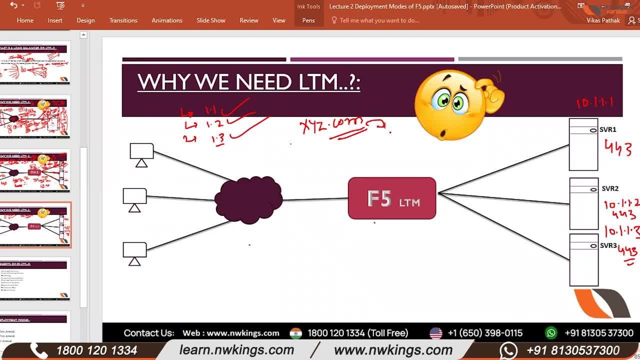 What resolution is it getting on DNS? Earlier, we were getting resolution on these three. right Now, in which one are we getting resolution? Is there anything in mind? No, sir, What is the most important virtual IP? The most important virtual IP is the most important virtual IP. 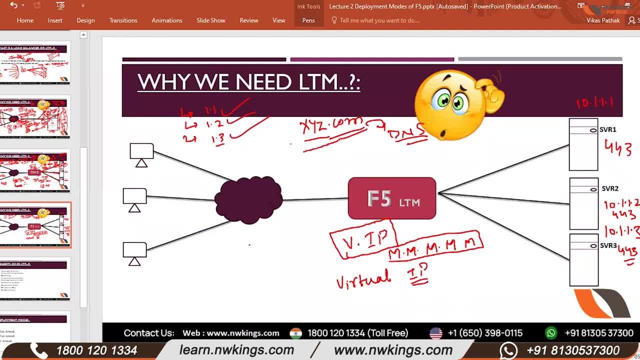 We will create DNS entry on XYZ. We will create DNS entry on XYZ in a public IP. If it is a web server, Let's assume it is a public IP- 91198201.38. All my clients all over the world will access XYZ. Their DNS lookup will be in this IP. 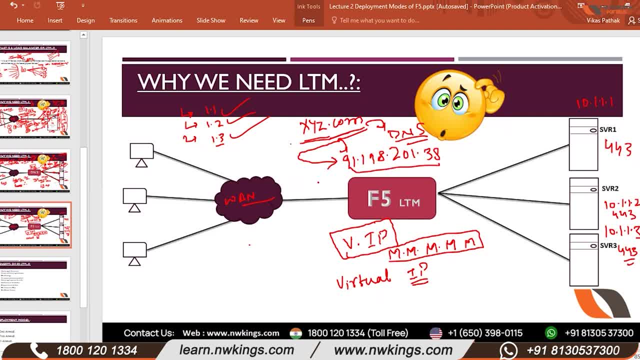 This IP will be routed, It will come to my infrastructure, It will land on F5 And then F5 will resolve it, And then F5 will resolve it Into the physical IP And it will distribute it, And that conversion is called, And that conversion is called Reverse Proxy. 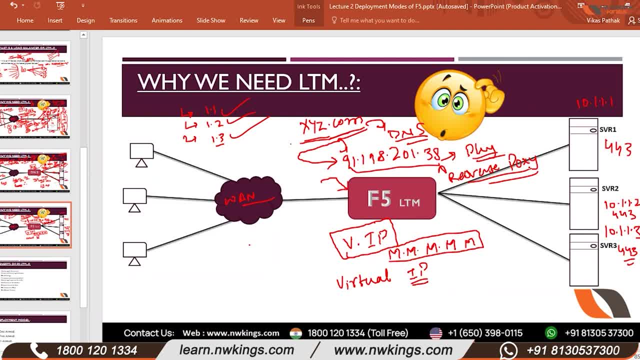 What it will call Reverse Proxy, Sir, it can also do NAT, Sir, it can also do NAT. Yes, Logically you are doing NAT, I think. Ok. Destination NAT: Ok, But concept: It is called reverse proxy, Proxy. What is forward proxy? Um, If in IP, If it is going to domain name? 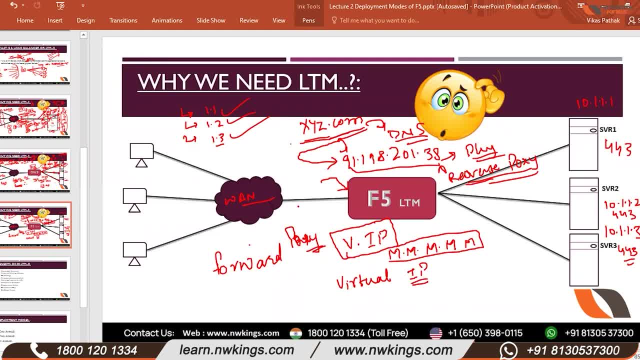 No, it is ARP. No, it is ARP. If you are going to security L1 to L2 interview. forward proxy, reverse proxy, virtual IP- most important questions. forward proxy is what we use in the LAN that the user accesses something, that request goes to the proxy. 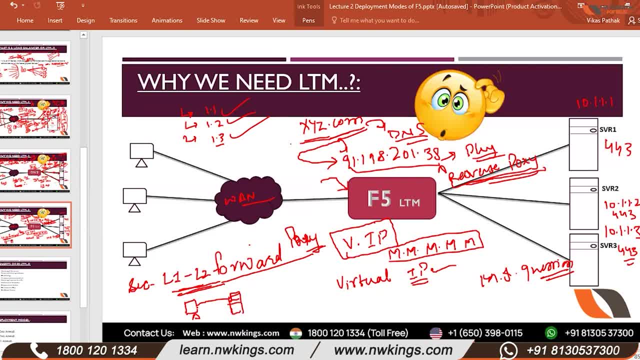 What the proxy server does is, instead of sending user's IP, it will send its own IP to the internet and when the request is received, the request will be sent to the internet. request will come to proxy and proxy will fulfill that request to the client. 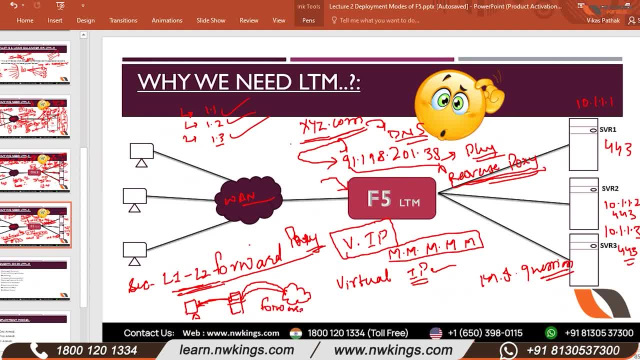 This is called forward proxy Here, when client is making a request to get a connection of xyzcom instead of real servers, F5 virtual IP is accepting that traffic and it is passing to a real server. that is called a reverse proxy. Make sense or not? 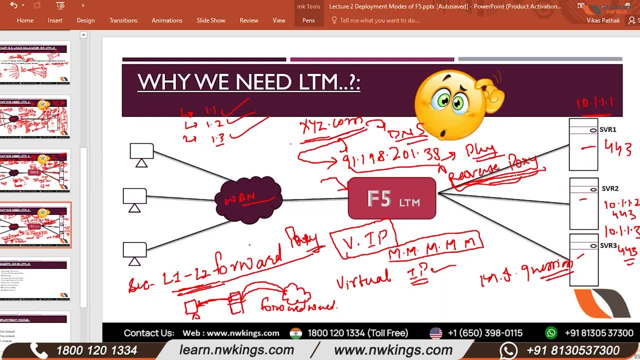 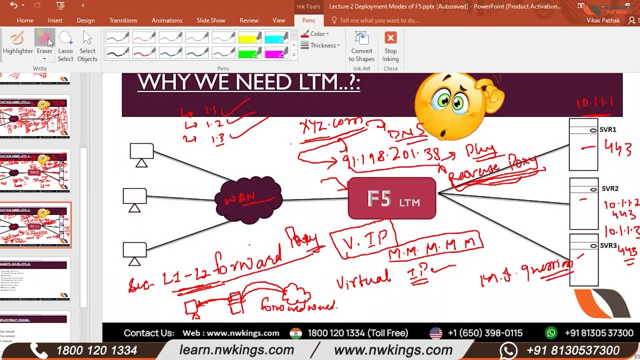 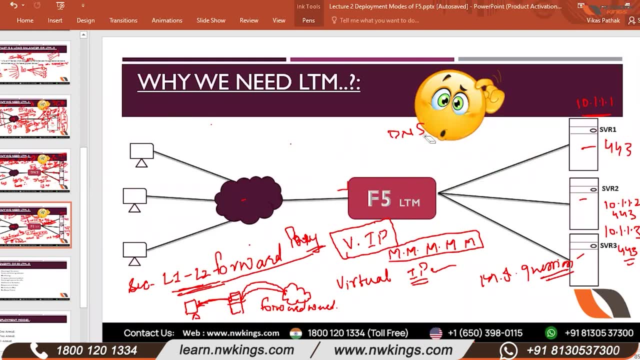 In LAMP language. the user traffic that is generated by F5 virtual server is taking the traffic to its own Right. Yes, It is distributing the traffic to the servers through reverse proxy, Sir. reverse proxy means that the data that is being sent to the physical server by virtual 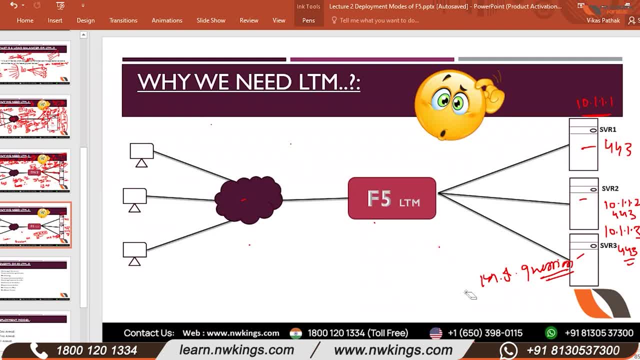 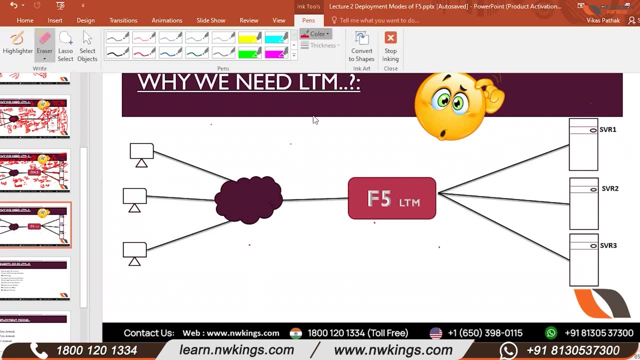 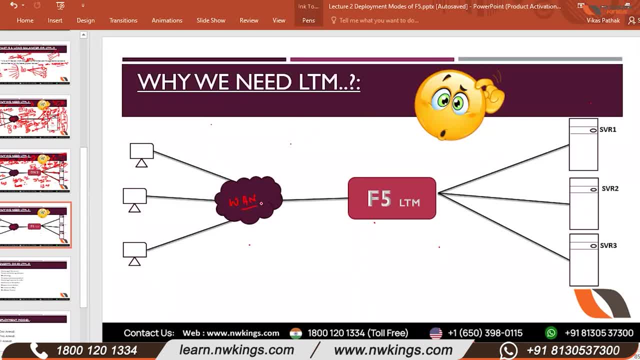 Has the server started. Any doubts, Sir? I have a doubt, sir, Sir, we have to configure server with virtual IP or with public IP. Now let's test. No, No, No, Why did you do that with public IP? 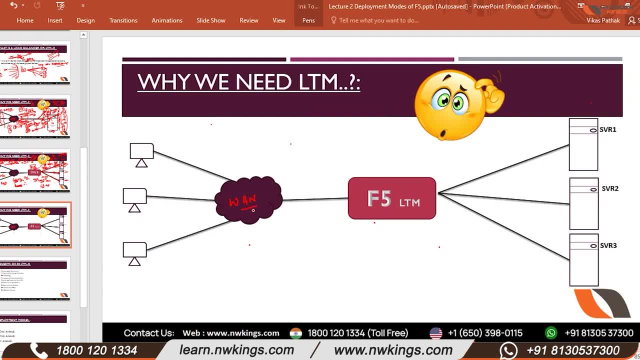 Server doesn't know who are my clients, Client don't know who are my servers. They know my clients, Then know that the servers with return is mined, ie They know that the customer is my client and yours is else one from other parts of the.